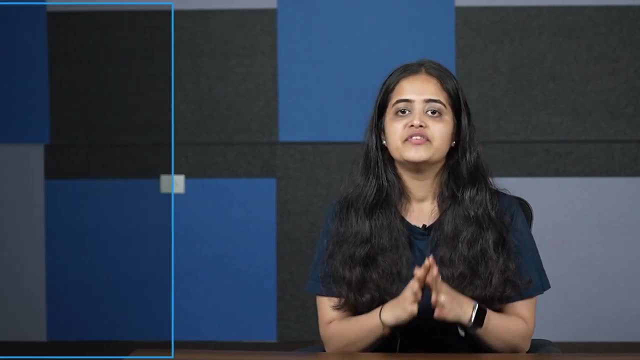 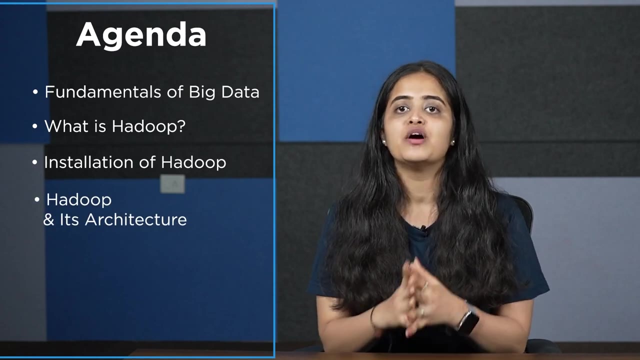 answer all your questions. What are we going to discuss today? We are going to highlight the fundamentals of big data. what is Hadoop? installation of Hadoop, Hadoop and its architecture, followed by which we will cover in-depth understanding of Hadoop Yarn, HDFS MapReduce. 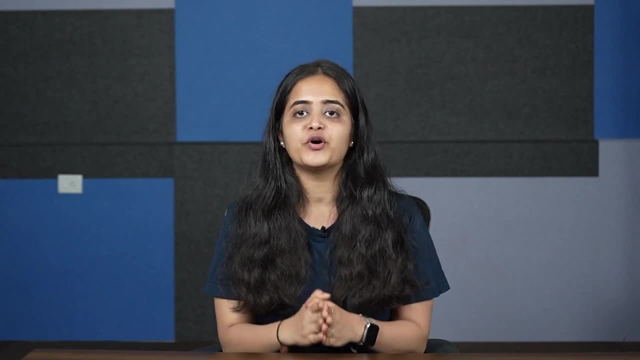 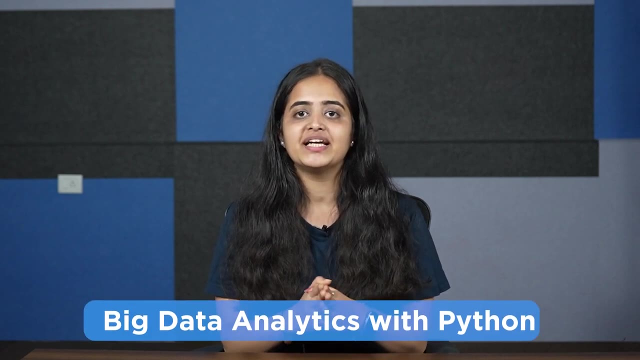 and its example, Post, which we will understand. another important processing layer, Apache Spark. Once we have a decent understanding of the fundamentals, we will dive into big data analytics with Python. And finally, to make things easier, we will cover the fundamentals of big data analytics. And finally, to make things more interesting, we will cover the 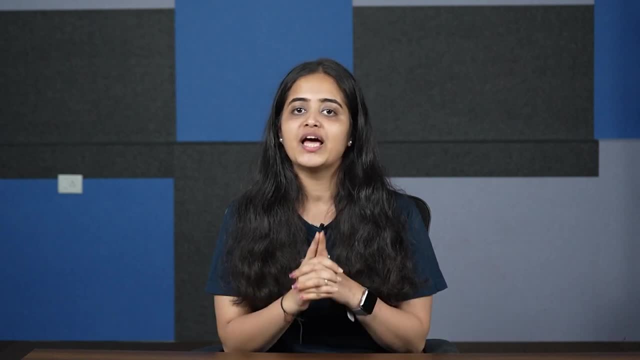 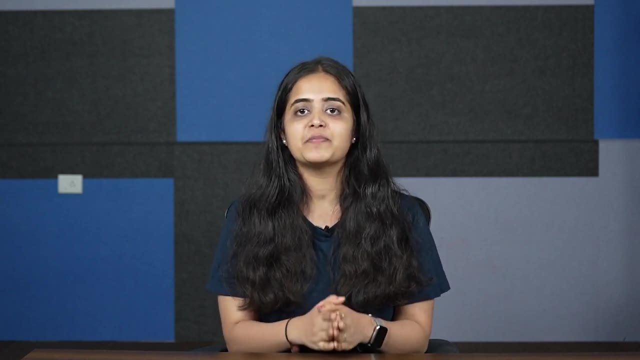 most frequently asked Hadoop interview questions, which should help you stand on the safer side in your upcoming interview. But big data is an ocean of topics. If you are an aspiring big data developer and keen to get your certification training, then we have the best offer for. 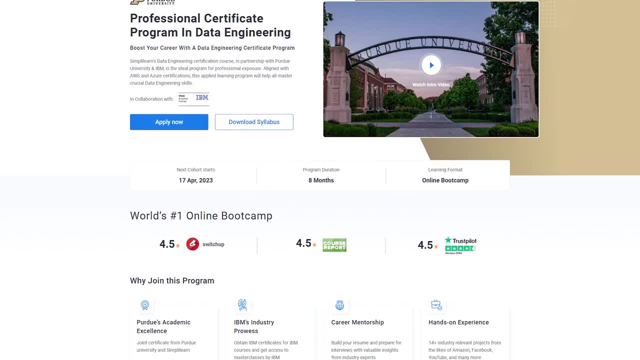 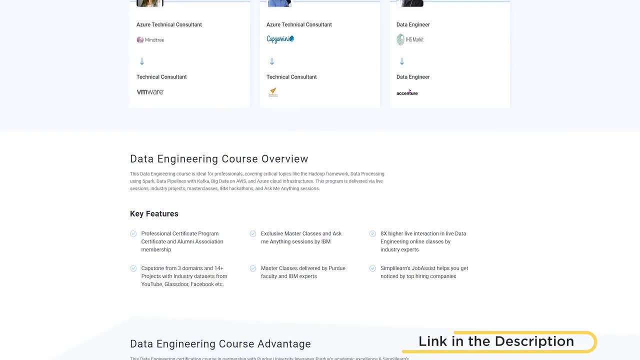 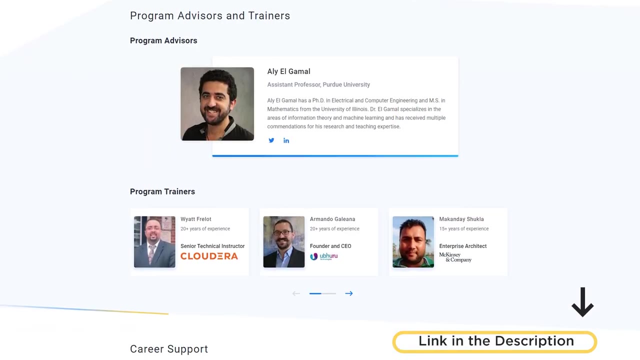 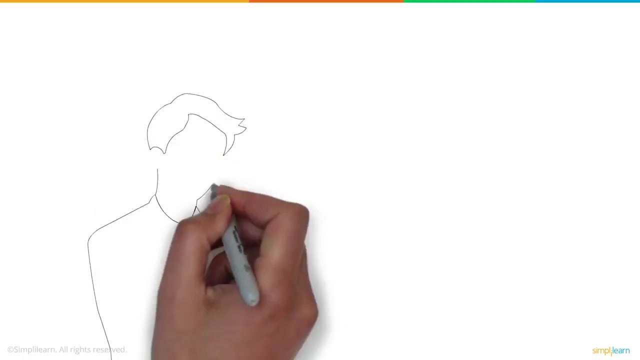 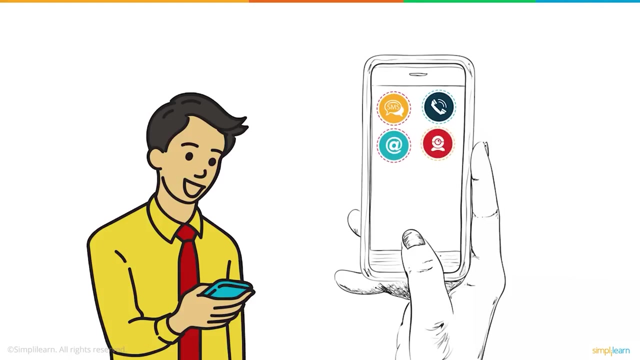 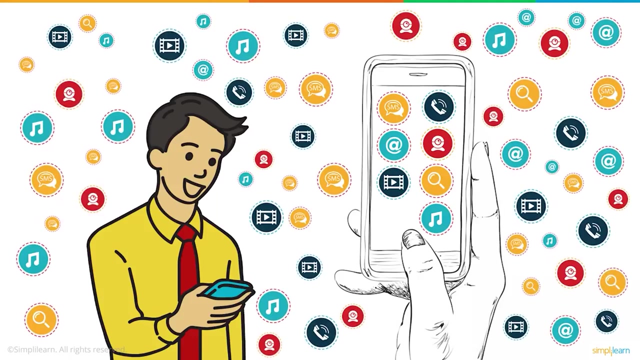 you Now over to our training experts. We all use smartphones, but have you ever wondered how much data it generates in the form of texts, phone calls, emails, photos, videos, searches and music? Approximately 40 exabytes of data gets generated every month by a single smartphone user. Now imagine: 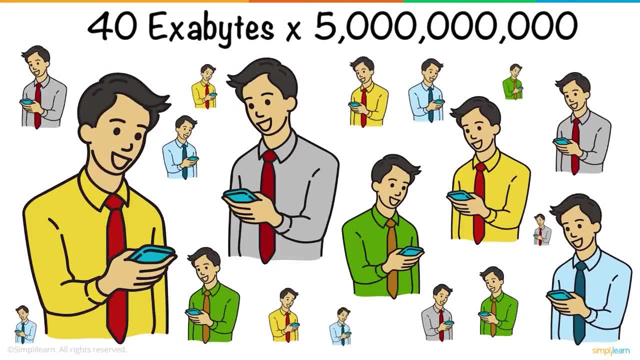 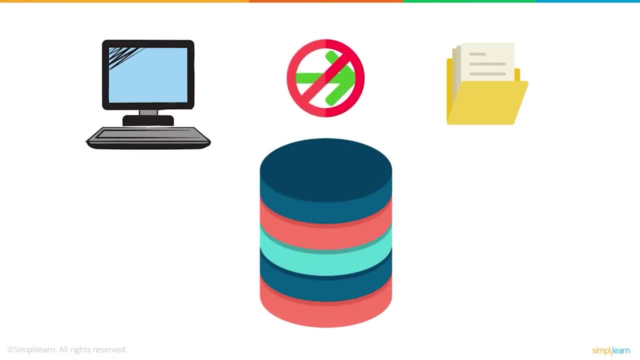 this number multiplied by 5 billion smartphone users, That's a lot for our mind to even process, isn't it? In fact, this amount of data is quite a lot for traditional computing systems to handle, And this massive amount of data is what we term as big data. Let's 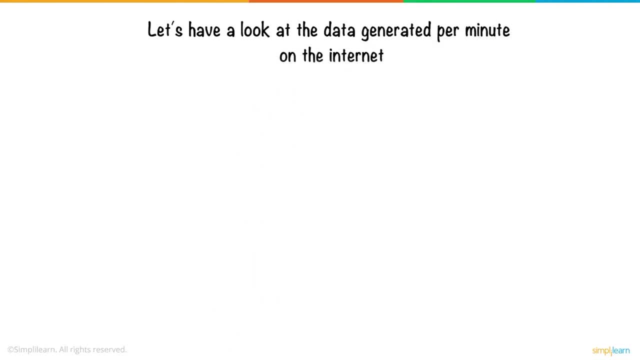 have a look at the data generated per minute on the internet. 2.1 million snaps are shared on Snapchat. 3.8 million search queries are made on Google. 1 million people log on to Facebook. 1.5 million videos are watched on YouTube. 188 million emails are sent. That's a lot. 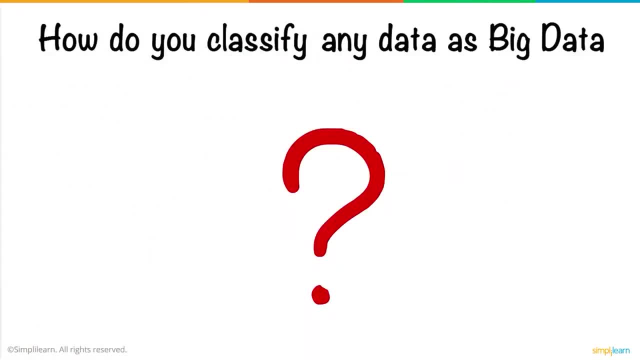 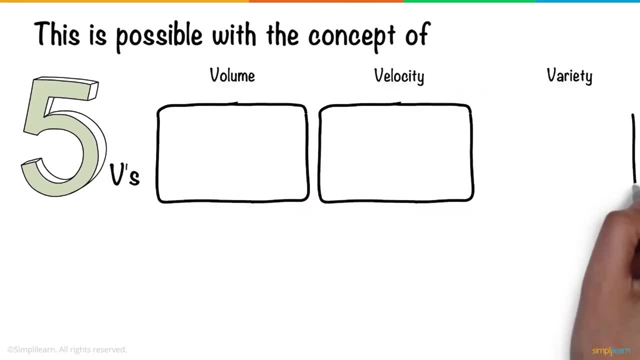 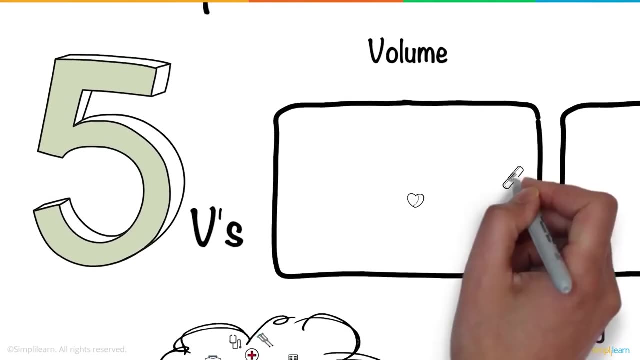 of data. So how do you classify any data as big data? This is possible with the concept of five Vs: Volume, Velocity, Variety, Veracity and Value. Let us understand this with an example from the healthcare industry. Hospitals and clinics across the world generate massive. 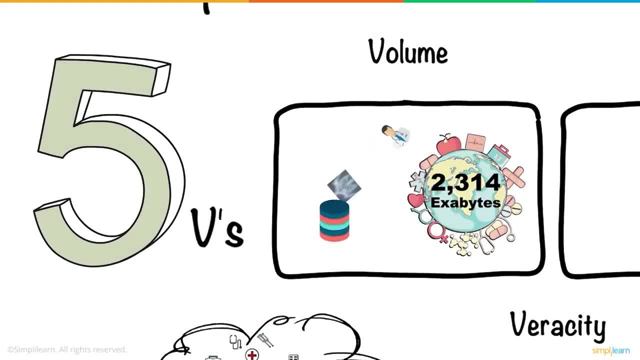 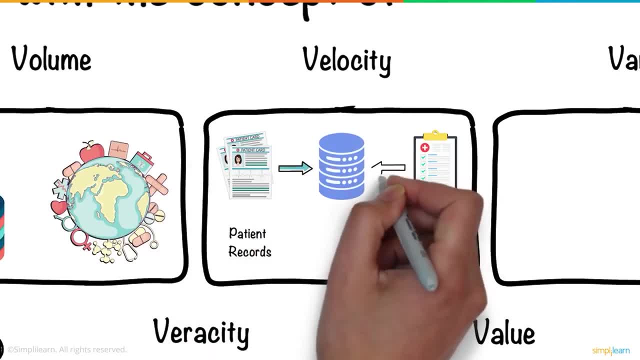 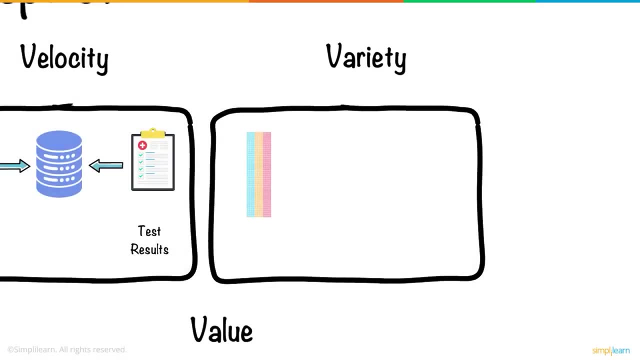 volumes of data: 2,314 exabytes of data are collected annually in the form of patient records and test results. All this data is generated at a very high speed, which attributes to the velocity of big data. Variety refers to the various data types, such as structured, semi-structured and unstructured. 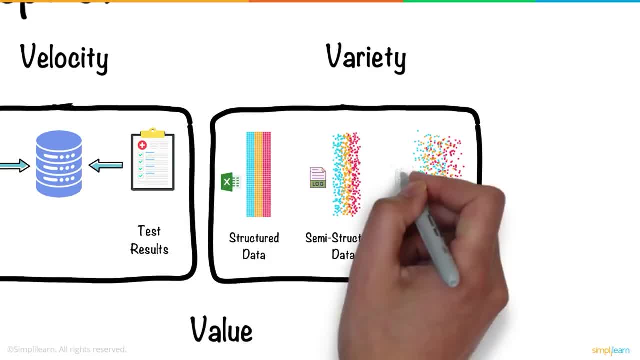 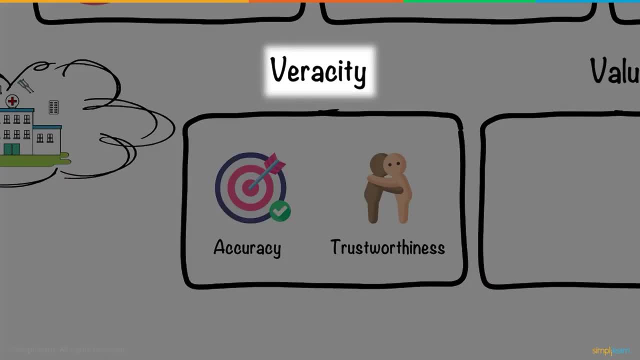 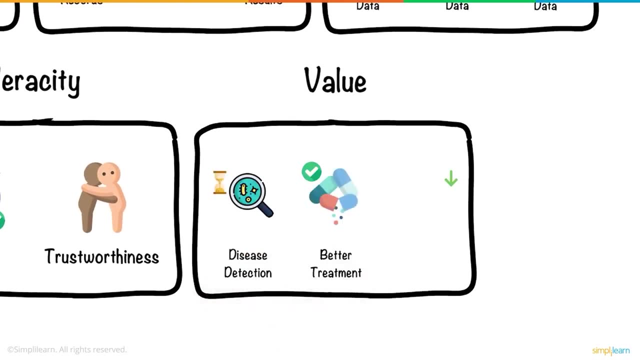 data. Examples include Excel records, log files and X-ray images. Accuracy and trustworthiness of the generated data is termed as veracity. Analyzing all this data will benefit the medical sector by enabling faster disease detection, better treatment and reduced cost. This is known as the value of big data. 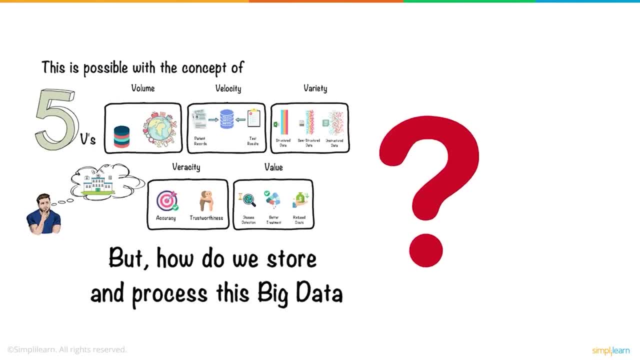 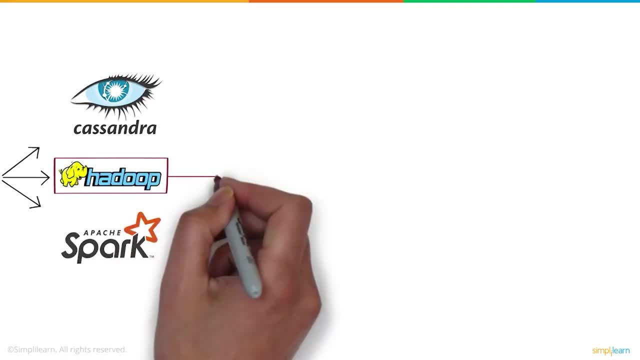 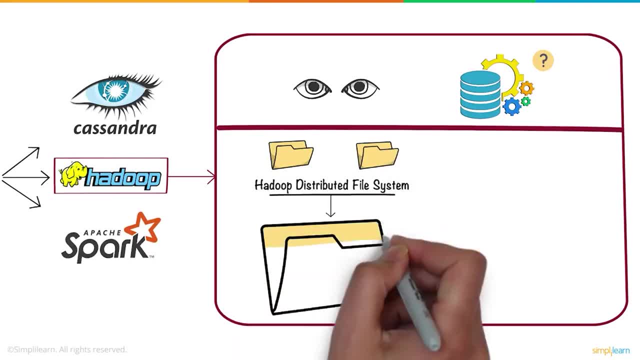 big data. Hadoop has a redistributed file system, known as Hadoop Distributed File System, to store big data. If you have a huge file, your file will be broken down into smaller chunks and stored in various machines. Not only that, when you break the file, you also make copies of it, which goes into 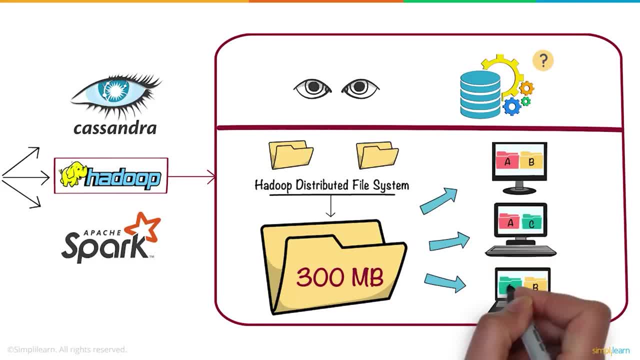 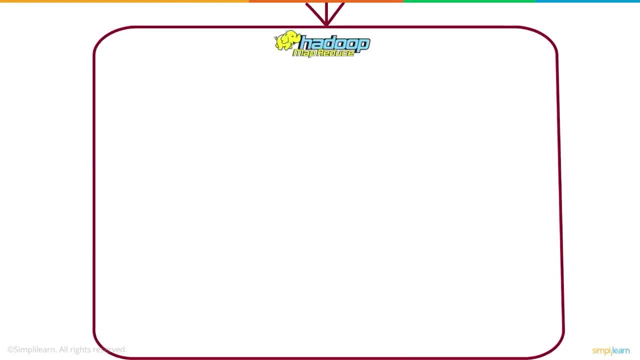 different nodes. This way you store your big data in a distributed way And make sure that even if one machine fails, your data is safe on another. Map Reduce Technique is used to process big data. A lengthy task A is broken into smaller tasks B, C and D. 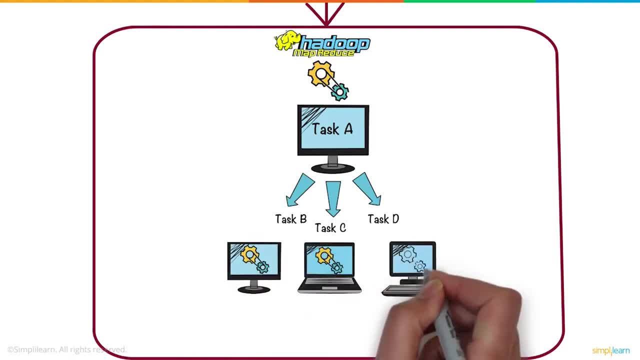 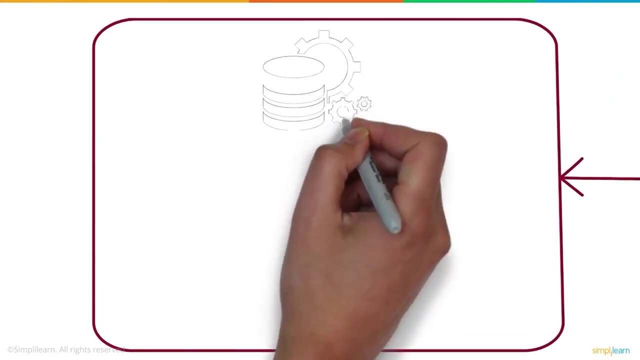 Now, instead of one machine, three machines take up each task and complete it in a parallel fashion and assemble the results at the end. Thanks to this, the processing becomes easy and fast. This is known as parallel processing. Now that we have stored and processed our big data, we can analyze this data for numerous applications. 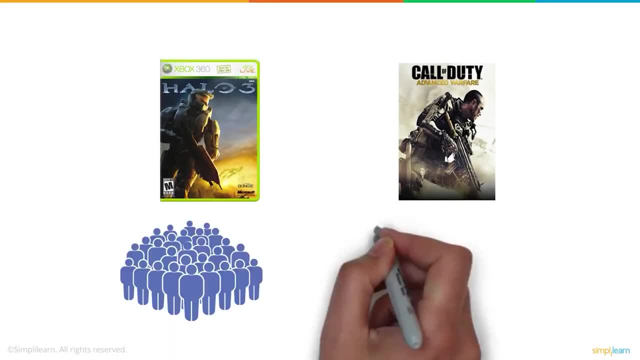 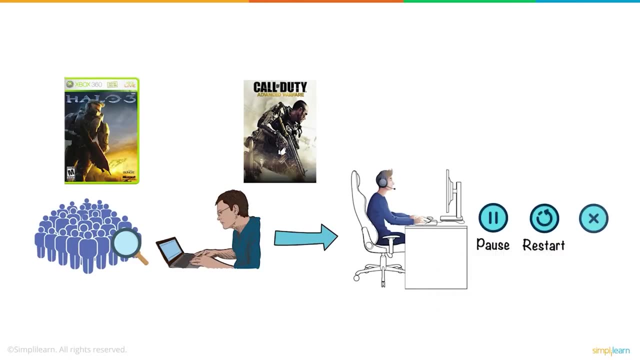 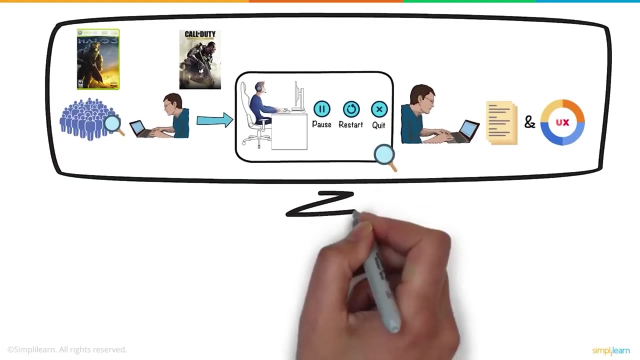 In games like Halo 3 and Call of Duty, designers analyze user data to understand at which stage most of the users pause, restart or quit playing. This insight can help them rework on the storyline of the game and improve the user experience, which, in turn, reduces the customer churn rate. 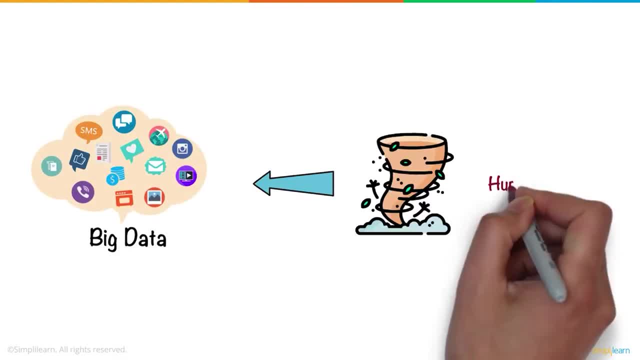 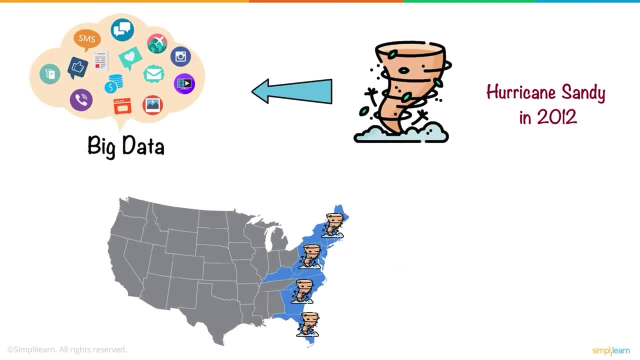 Similarly, big data also helped with disaster management during Hurricane Sandy in 2012.. It was used to gain a better understanding of the storm's effect on the ecosystem. It was used to reduce the risk of an earthquake in the east coast of the US, and necessary measures were taken. 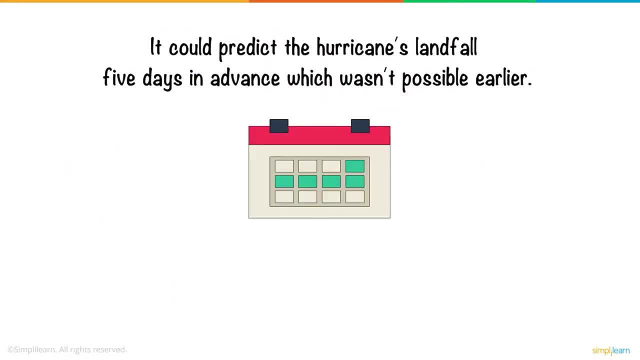 It could predict the hurricane's landfall five days in advance, which wasn't possible earlier. These are some of the clear indications of how valuable big data can be once it is accurately processed and analyzed. Let's rewind to the days before the world turned digital. 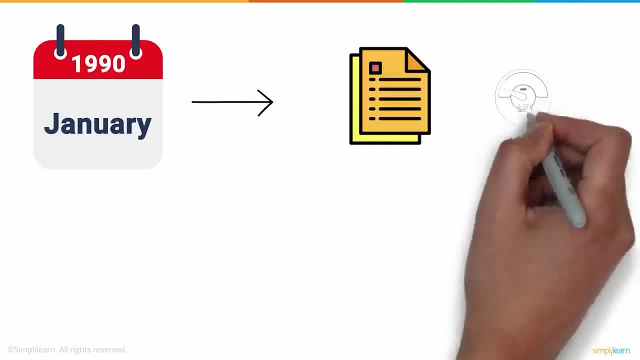 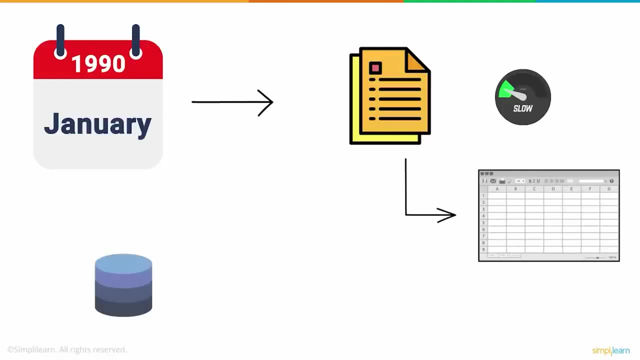 Back then, miniscule amounts of data were generated at a relatively sluggish pace. All the data was mostly documents and in the form of rows and columns. Storing or processing this data wasn't much trouble, as a single storage unit and processor combination would do the job. 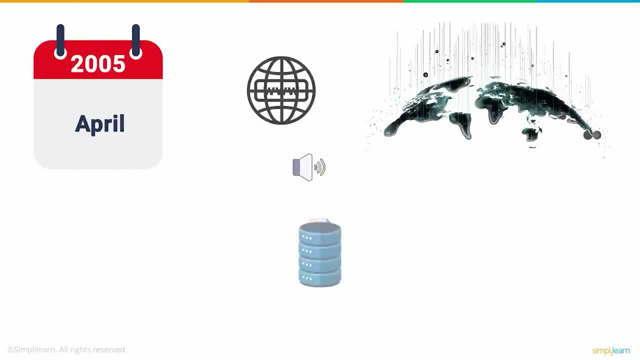 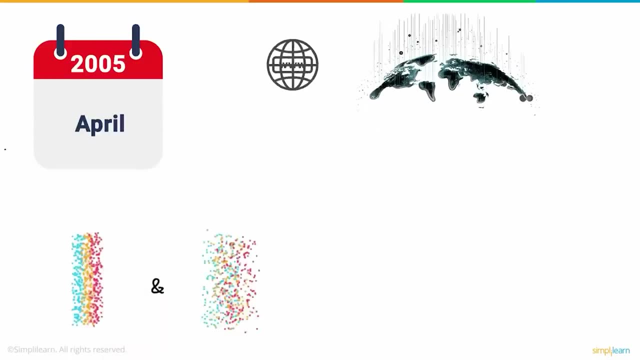 But as years passed by, the internet took the world by storm, giving rise to tons of data generated in a multitude of forms and formats. every microsecond Semi-structured and unstructured data was available now in the form of emails, images, audio and video, to name a few. 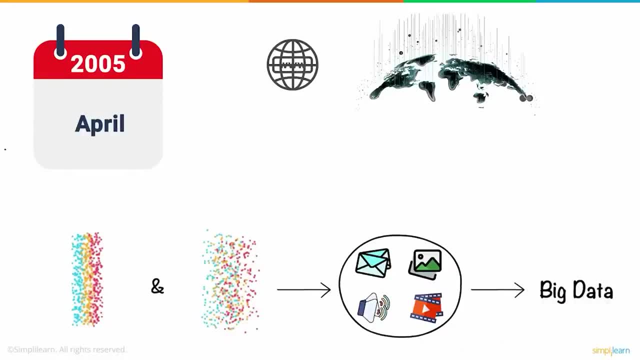 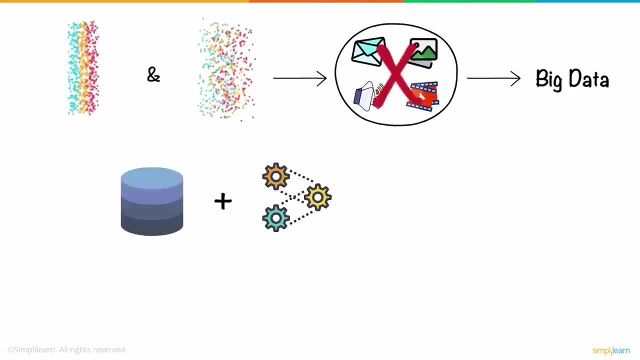 All this data became collectively known as big data. Although fascinating, it became really popular. It became nearly impossible to handle this big data, and a storage unit-processor combination was obviously not enough. So what was the solution? Multiple storage units and processors were undoubtedly the need of the hour. 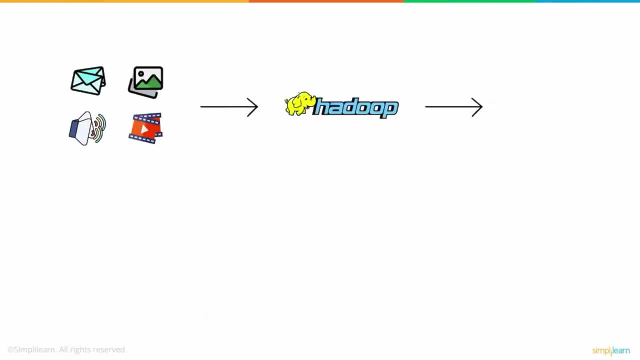 This concept was incorporated in the framework of Hadoop that could store and process vast amounts of any data efficiently using a cluster of commodity hardware. Hadoop consisted of three components that were specifically designed to work on big data. In order to capitalize on data, the first step is storing it. 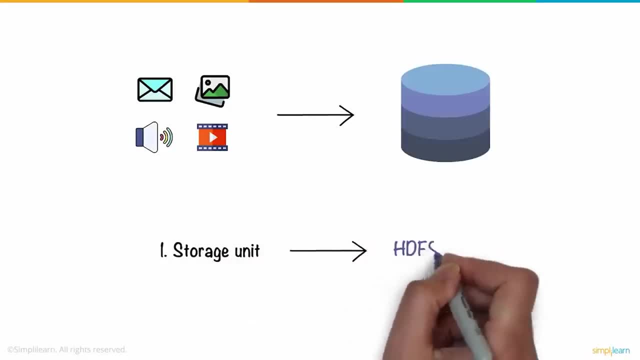 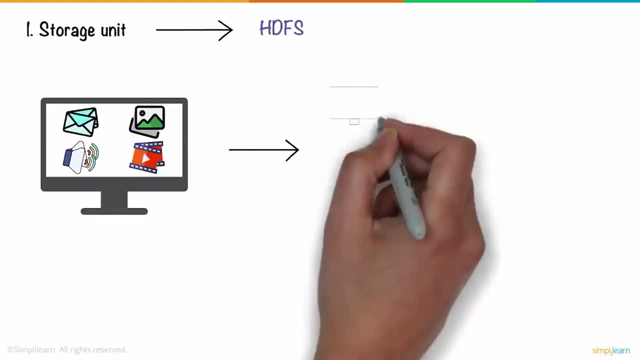 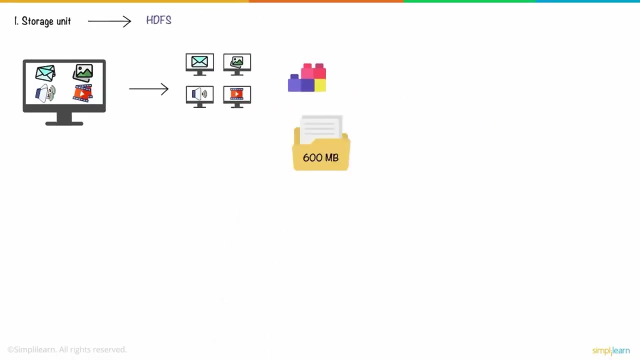 The first component of Hadoop is its storage unit- the Hadoop Distributed File System, or HDFS. Storing massive data on one computer is unfeasible. Hence data is distributed amongst many computers and stored in blocks. So if you have 600 MB of data to be stored, HDFS splits the data into multiple blocks. 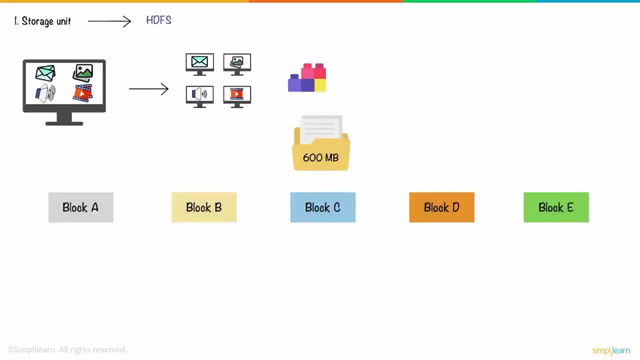 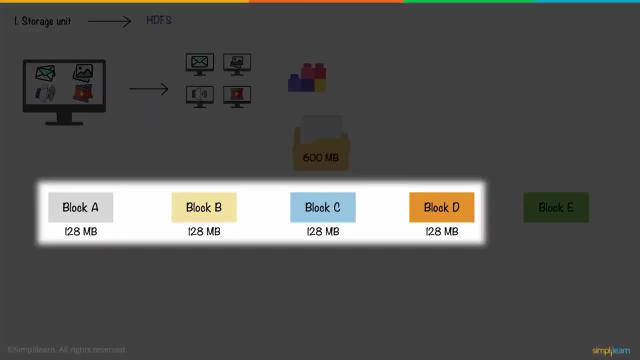 of data that are then stored on several data nodes in the cluster: 128 MB of data. 128MB is the default size of each block, Hence 600MB will be split into four blocks- A, B, C and D- of 128MB each and the remaining 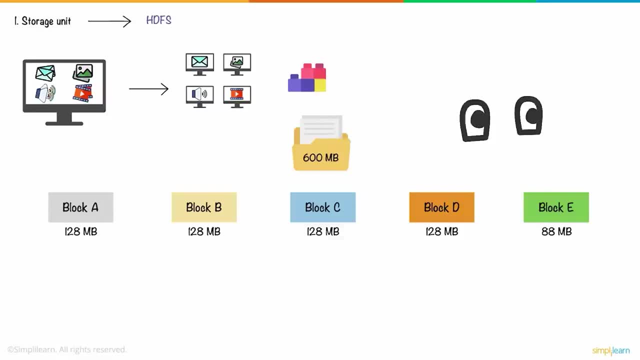 88MB in the last block E. So now you might be wondering: what if one data node crashes? Do we lose that specific piece of data? Well, no, that's the beauty of HDFS. HDFS makes copies of the data and stores it across multiple systems. 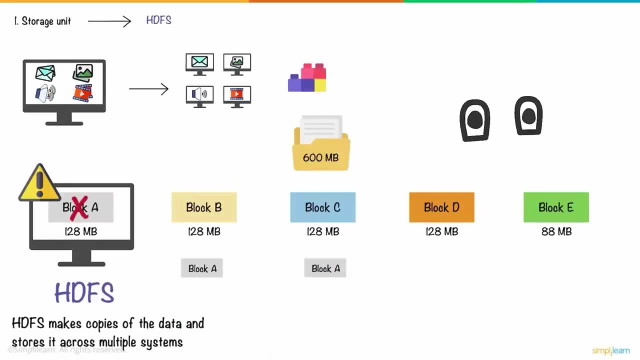 For example, when block A is created, it is replicated with a replication factor of 3 and stored on different data nodes. This is termed the replication method. By doing so, data is not lost at any cost, even if one data node crashes. making HDFS. 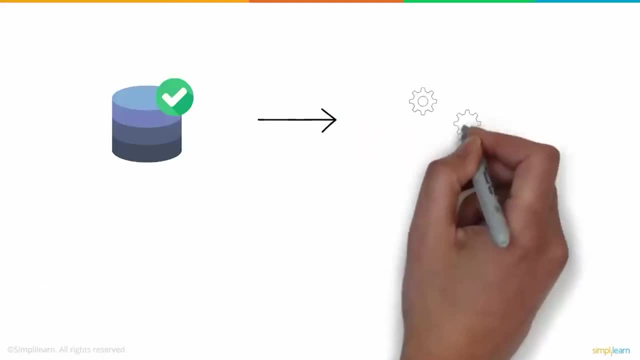 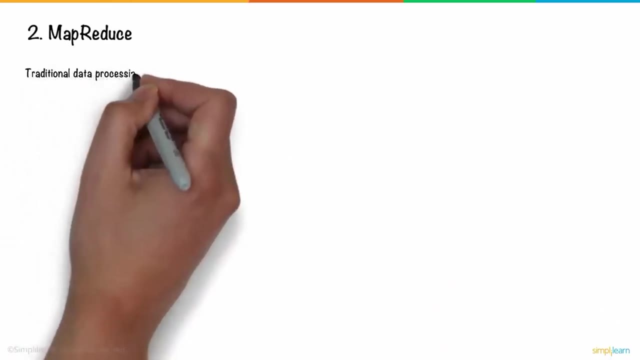 fault-tolerant. After storing the data successfully, it needs to be processed. This is where the second component of Hadoop MapReduce comes into play. In the traditional data processing method, entire data would be processed on a single machine having a single processor. 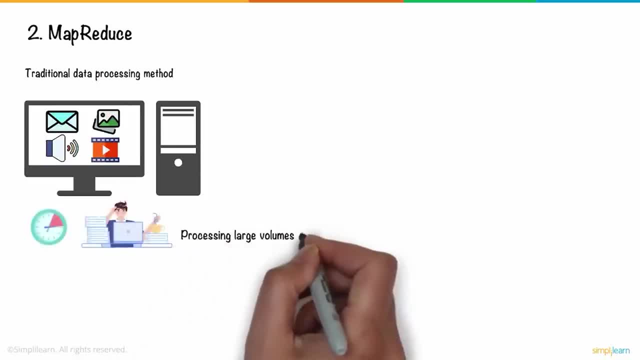 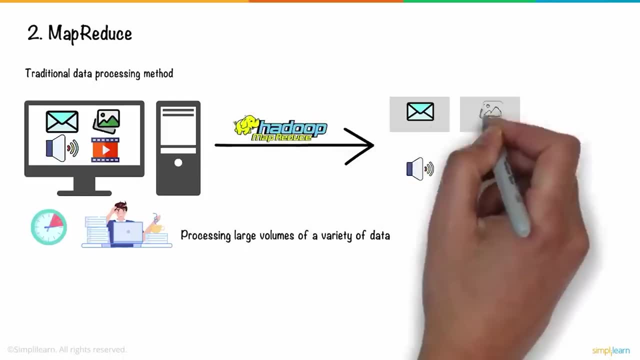 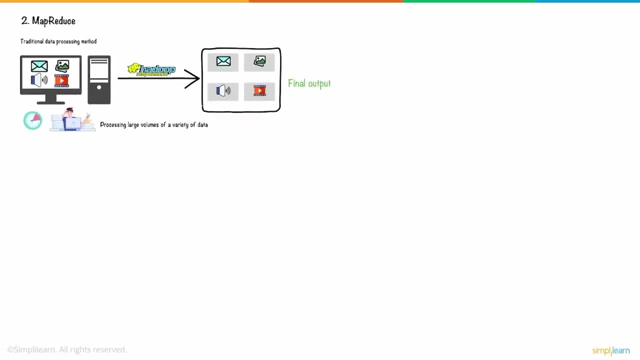 This consumed time and was inefficient, especially when processing large volumes of a variety of data. To overcome, this, MapReduce splits data into parts and processes each of them separately on different data nodes. The individual results are then aggregated to give the final output. 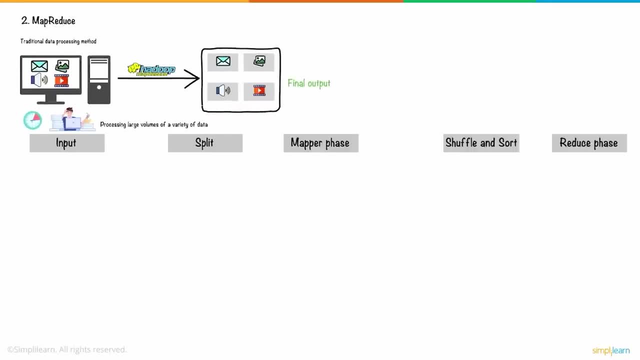 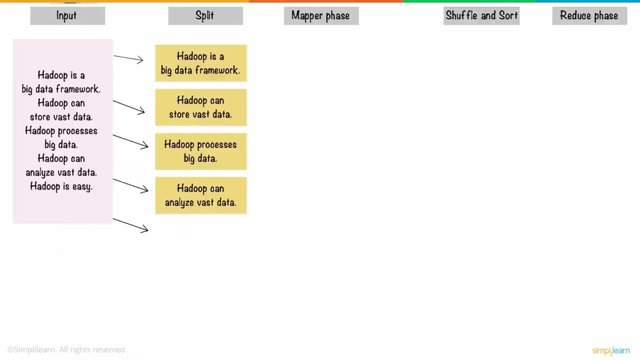 Let's try to count the number of occurrences of words taking this example. First, the input is split into five separate parts, based on full stops. The next step is the mapper phase, where the occurrence of each word is counted and allocated a number. 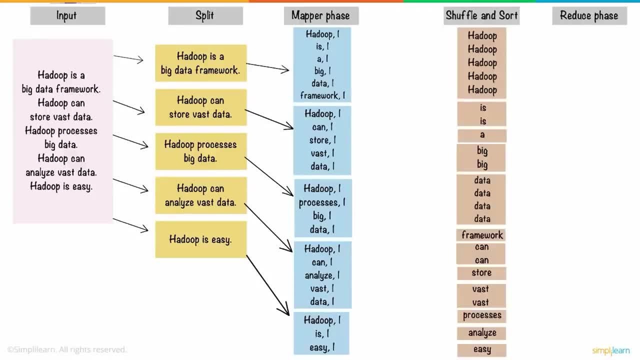 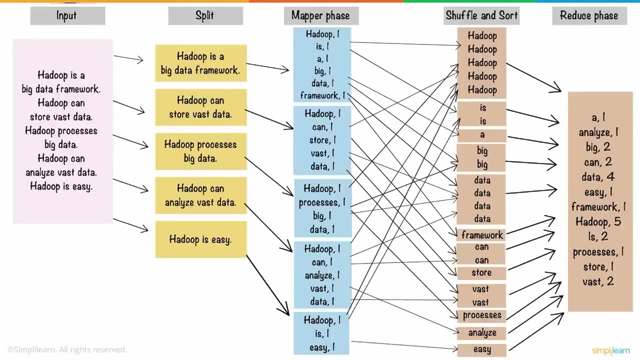 After that, depending on the words, similar words are shuffled, sorted and grouped, Following which, in the reducer phase, all the grouped words are given a count. Finally, the output is displayed by aggregating the results. All this is done by writing a simple program. 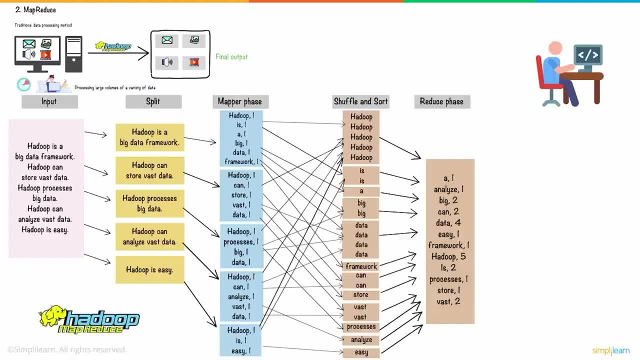 Similarly, MapReduce processes each part of big data individually and then sums the result at the end. This improves load balancing and saves a considerable amount of time. Now that we have our MapReduce job ready, it is time for us to run it on the Hadoop cluster. 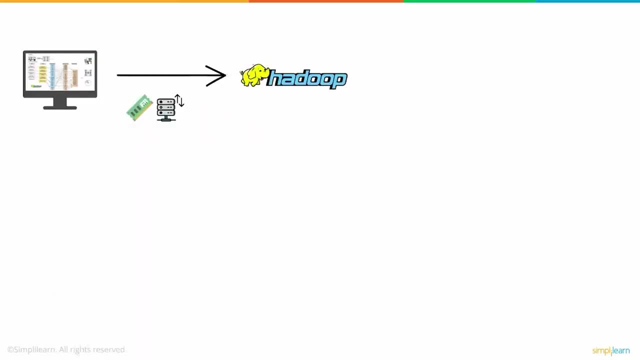 This is done with the help of a set of resources such as RAM, network bandwidth and CPU. Multiple jobs are run on Hadoop simultaneously and each of them needs some resources to complete the task successfully. To efficiently manage these resources, you need to run them on the Hadoop cluster. 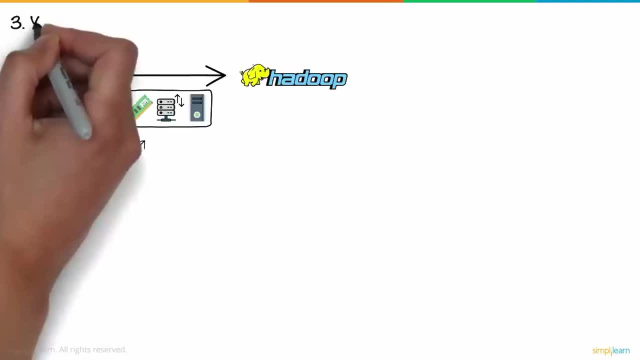 This is done by writing a set of resources such as RAM, network bandwidth and CPU. Multiple jobs are run on Hadoop simultaneously, and each of them needs some resources to complete the task successfully. We have the third component of Hadoop, which is YARN. 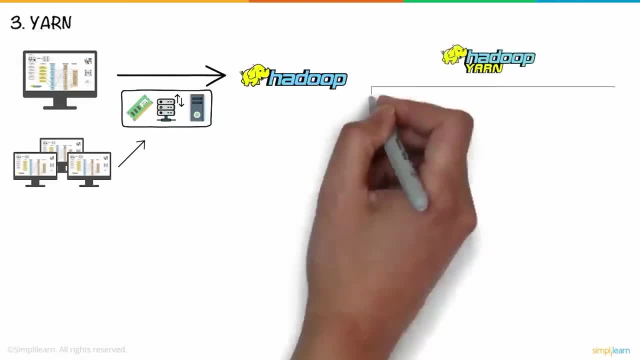 Yet another resource negotiator, or YARN, consists of a resource manager, node manager, application master and containers. The resource manager assigns resources, Node managers handle the nodes and monitor the resource usage in the node. The containers hold a collection of physical resources. 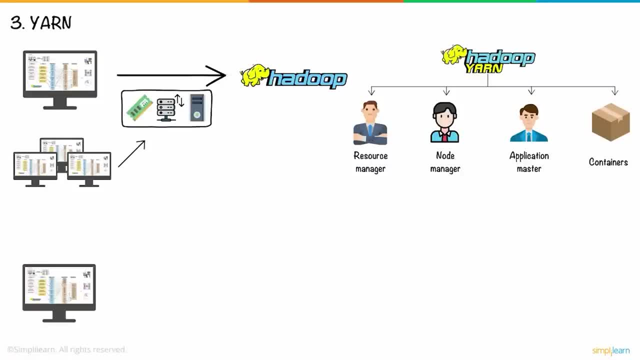 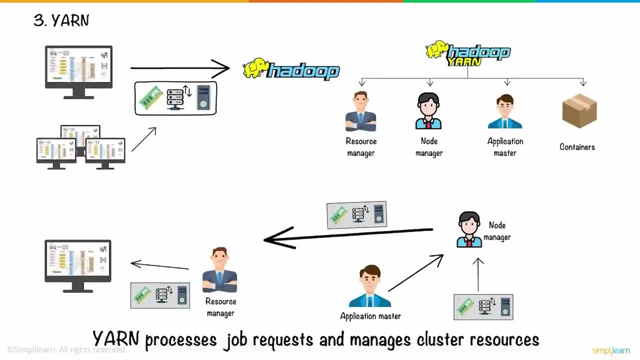 Suppose we want to process the MapReduce job we had created. First, the application master requests the container from the node manager. Once the node manager gets the resources, it sends them to the resource manager. This way YARN processes job requests and manages cluster resources in Hadoop. 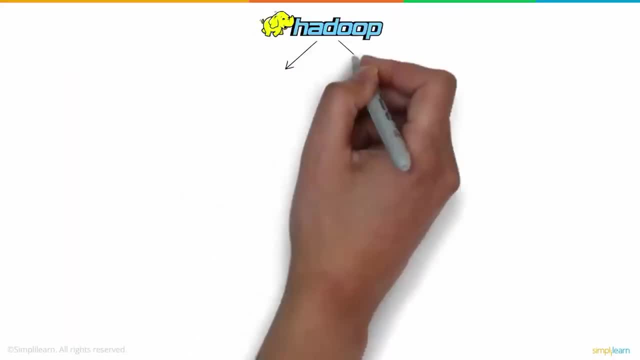 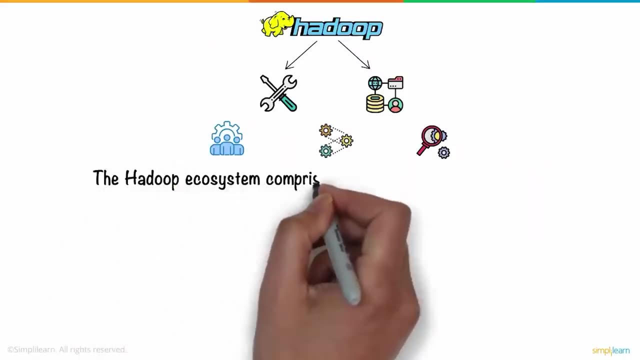 In addition to these components, Hadoop also has various big data tools and frameworks dedicated to managing, processing and analyzing data. The Hadoop ecosystem comprises several other components like Hive, Pig, Apache, Spark Flume and Scoop, to name a few. 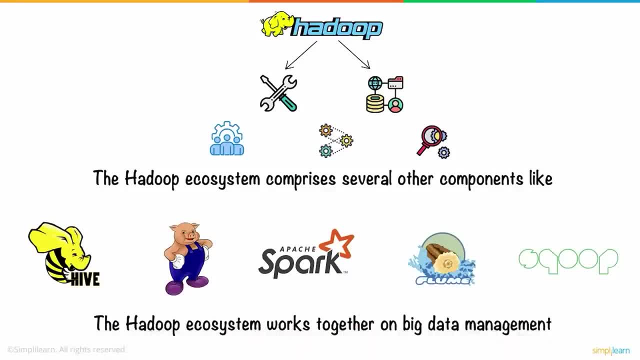 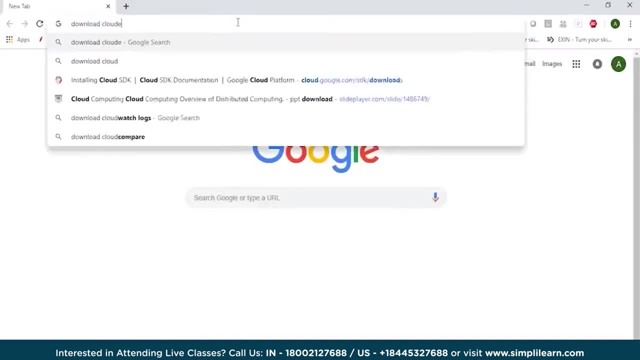 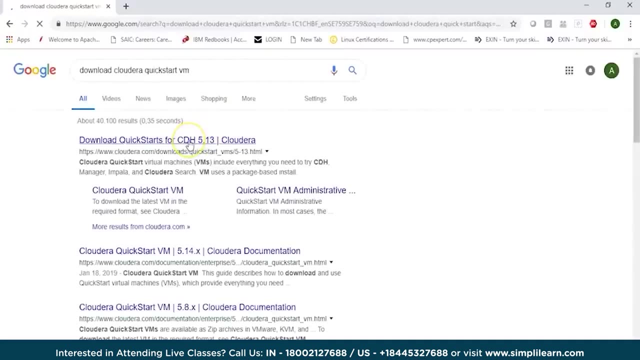 The Hadoop ecosystem works together on big data management. You can download the Cloudera QuickStart VM, So you can just type in download Cloudera QuickStart VM and you can search for package. Now this can be used to set up a QuickStart VM, which would be a single node, Cloudera-based cluster. 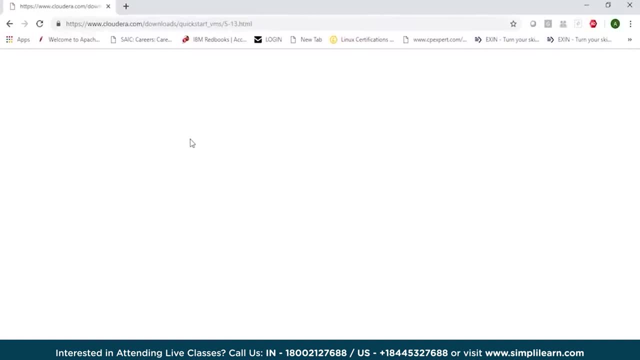 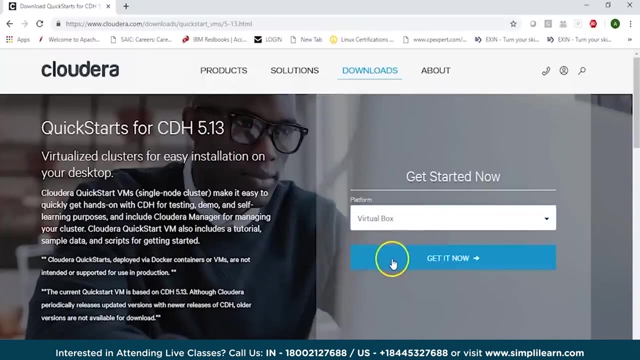 So you can click on this link and then, basically, based on the platform which you would be choosing to install, Such as using a VM box, or which version of Cloudera you would install, So here I can select a platform, So I can choose virtual box, and then you can click on get it now. 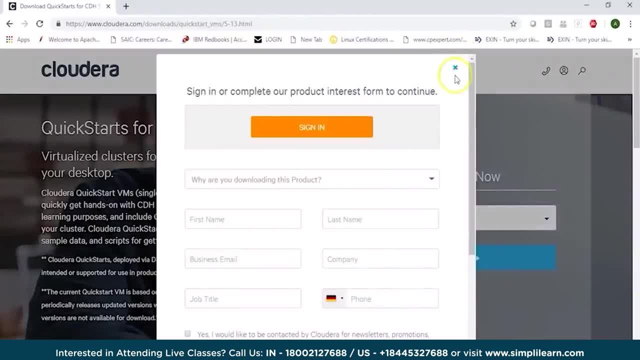 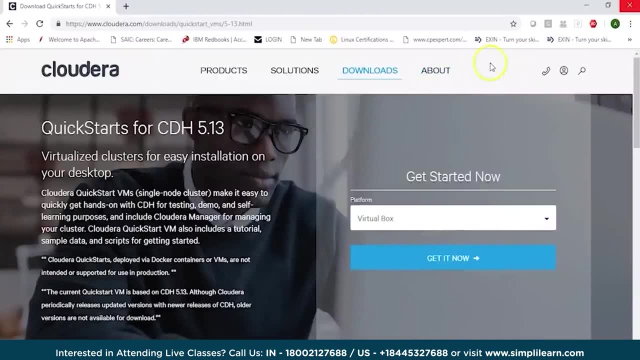 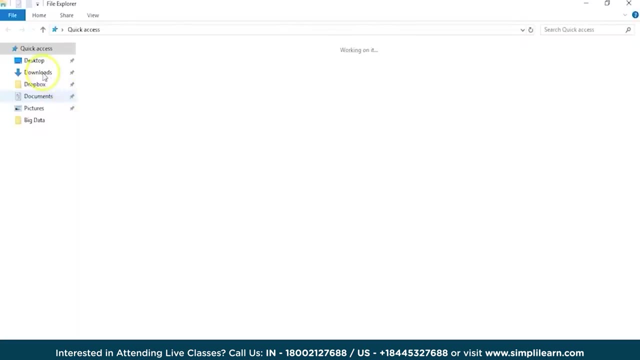 So give your details and, basically, then it should allow you to download the QuickStart VM, which would look something like this, And once you have the zip file which is downloaded, you can unzip it, which can then be used to set up a single node Cloudera cluster. 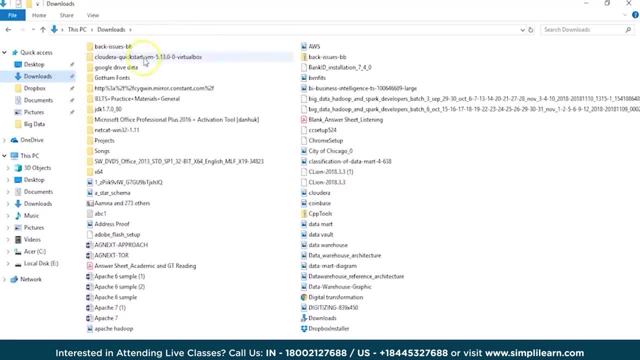 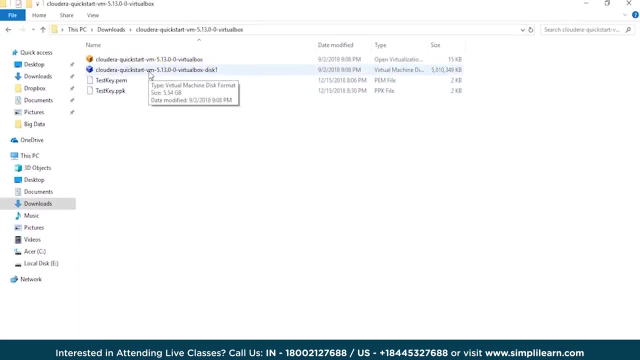 So, once you have downloaded the zip file, that would look something like this: So you would have a QuickStart virtual box and then a virtual box disk. Now this can be used to set up a cluster. Ignore these files which are related to Amazon machines, and you don't need to have that. 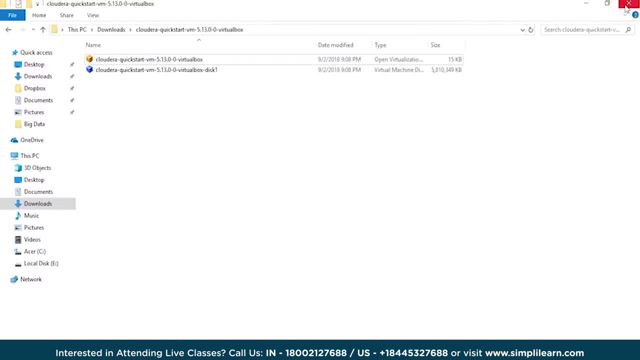 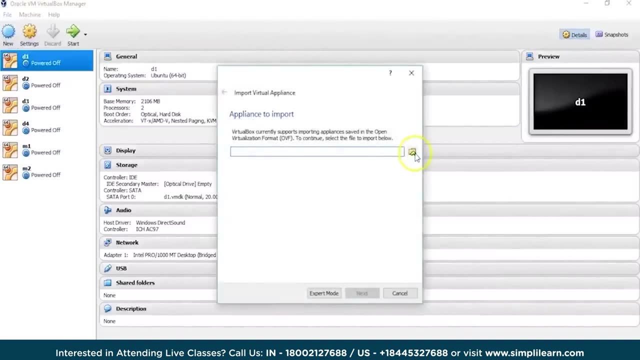 So you would just have this, and this can be used to set up a Cloudera cluster. So for this to be set up, you can click on file import appliance and here you can choose your QuickStart VM by looking into downloads. 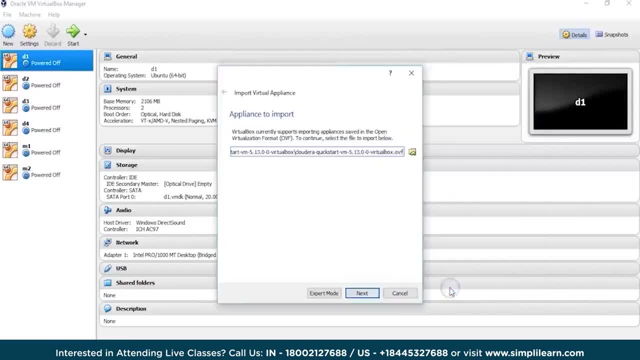 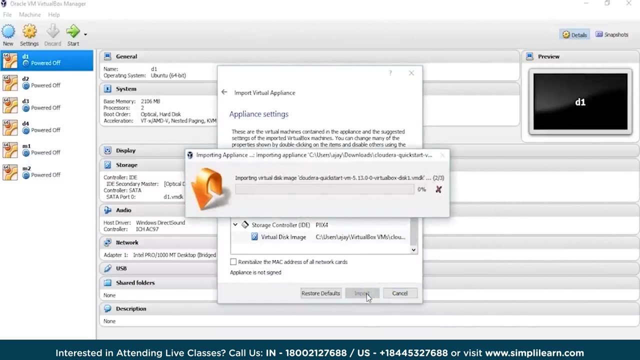 QuickStart VM, select this and click on open. Now you can click on next and that shows you the specifications of CPU RAM, which we can then change later, and click on import. This will start importing virtual disk image dot VMDK file into your VM box. 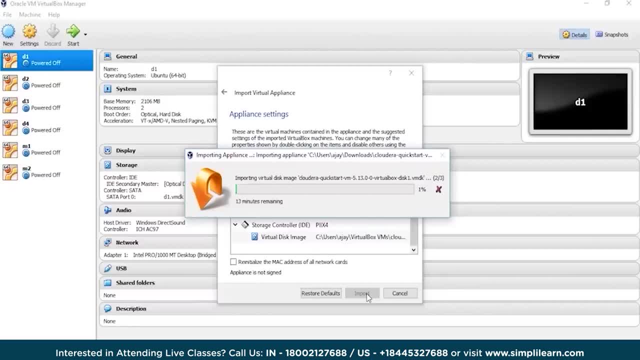 Once this is done, we will have to change the specifications, Our machines, to use two CPU cores minimum and give a little more RAM, because Cloudera QuickStart VM is very CPU intensive and it needs good amount of RAM. So to survive I will give two CPU cores and 5 GB RAM and that should be enough. 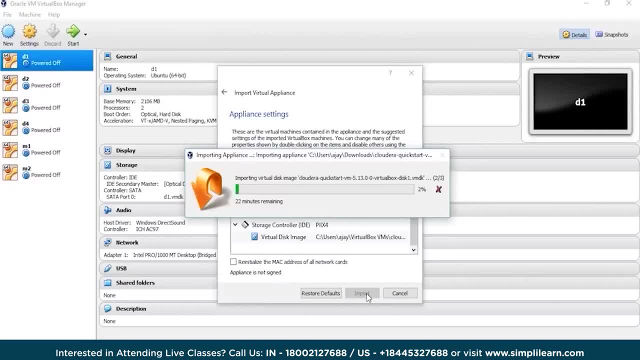 for us to bring up a QuickStart VM which gives us a Cloudera distribution of Hadoop in a single node cluster setup which can be used for working learning about different distributions in Cloudera, Cloudera clusters working with SDFS and other Hadoop ecosystem components. 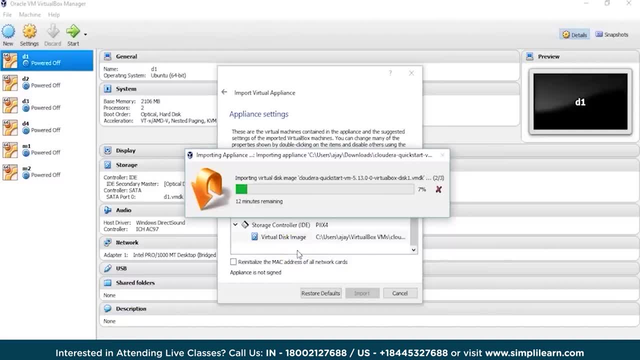 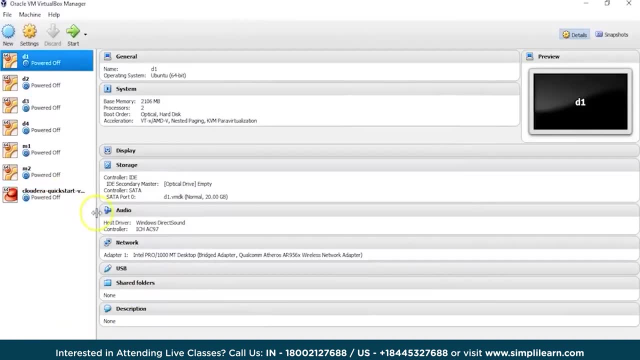 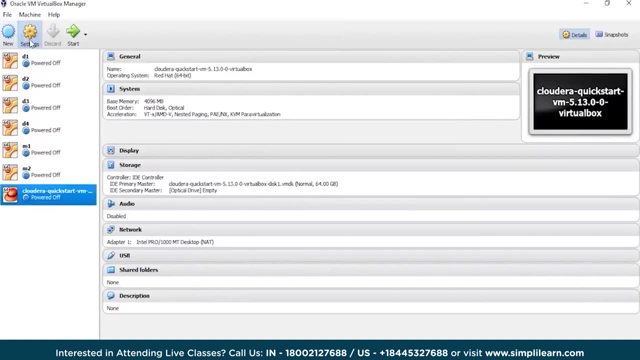 Let's just wait for this importing to finish and then we will go ahead and set up a QuickStart VM for our practice Here. the importing of appliance is done and we see Cloudera QuickStart machine is added to my list of machines. I can click on this and click on settings. 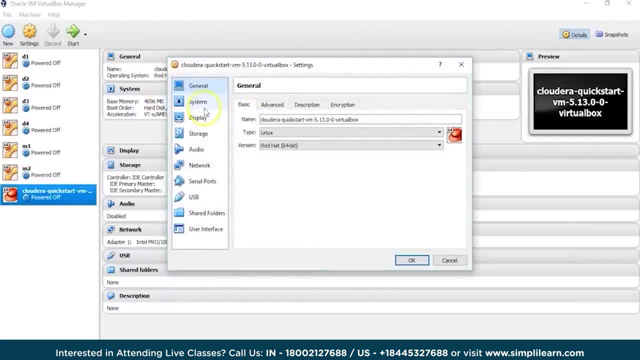 As mentioned, I would like to give it more RAM and more CPU cores. So click on system In here, let's increase the RAM to at least 5 and click on processor and let's give it two CPU cores, which would at least be better than using one CPU core. 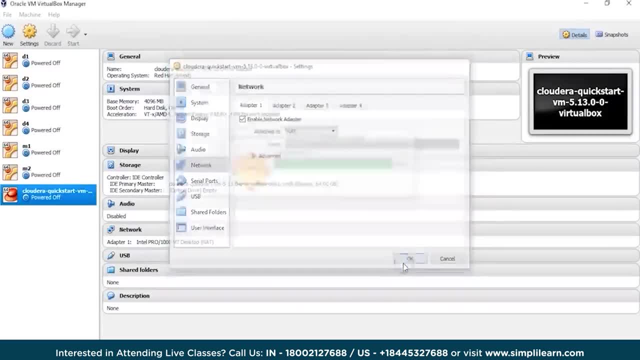 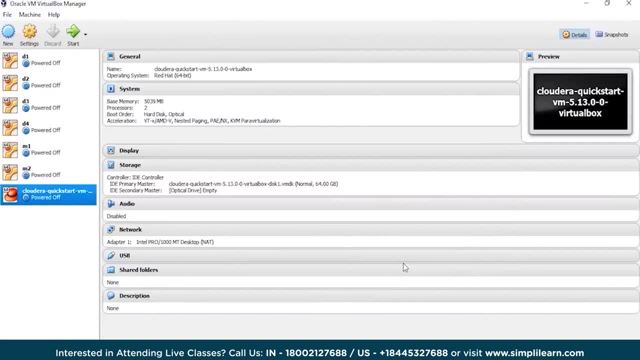 Network. it goes for NAT, and that's fine. Click on OK and we would want to start this machine so that it uses two CPU cores, 5 GB RAM, and it should bring up my Cloudera QuickStart VM. Now let's go ahead and start this machine. 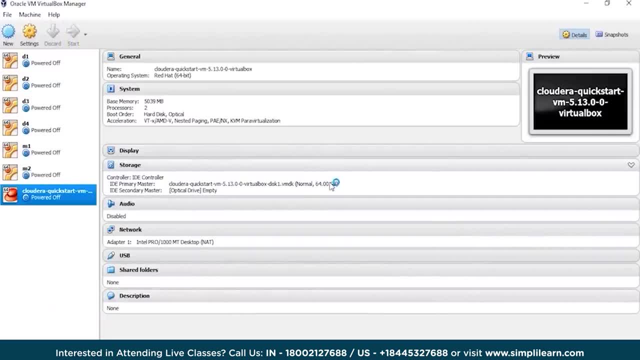 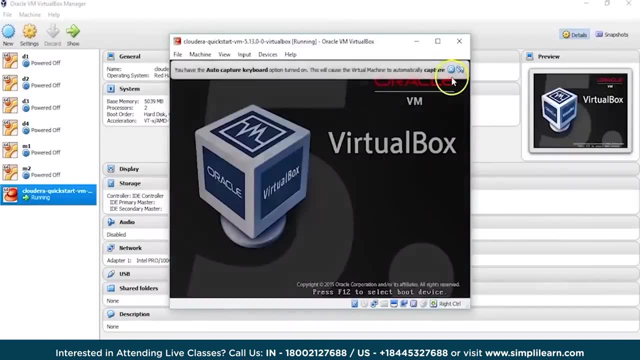 which has our QuickStart VM. It might take initially some time to start up because internally there will be various Cloudera services which will be starting up and those services need to be up for our Cloudera QuickStart VM to be accessible. 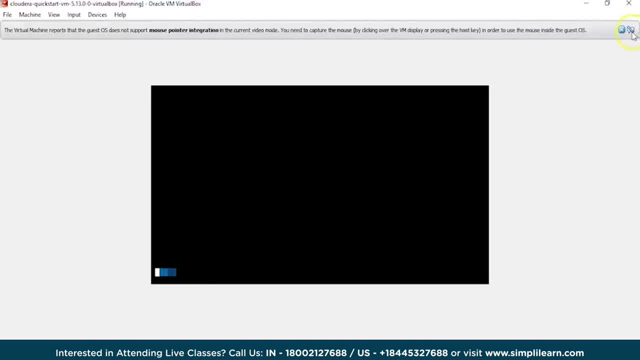 So, unlike your Apache Hadoop cluster, where we start our cluster and we will be starting all our processes, in case of Cloudera, it is your Cloudera SCM server and agents which take care of starting up your services and starting up of your different roles for those services. 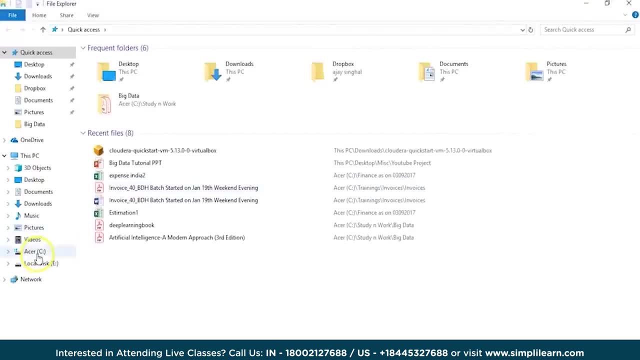 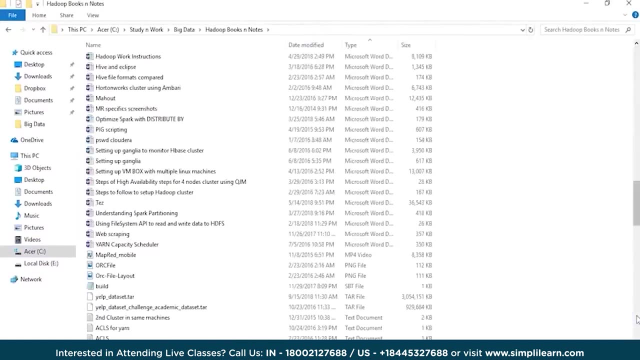 I explained in my previous session that for a Cloudera cluster it would be these services. Let me just show you that. So in case of Apache cluster, we start our services, that is, we start our cluster by running script and then basically, 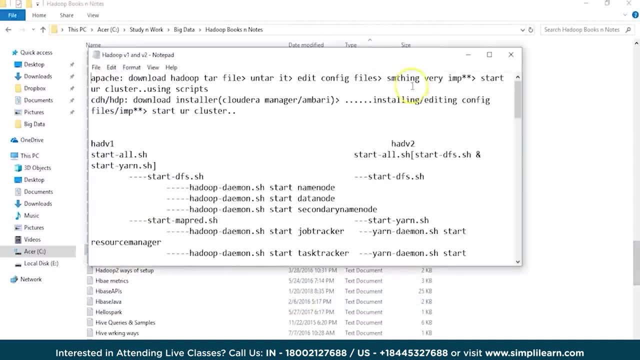 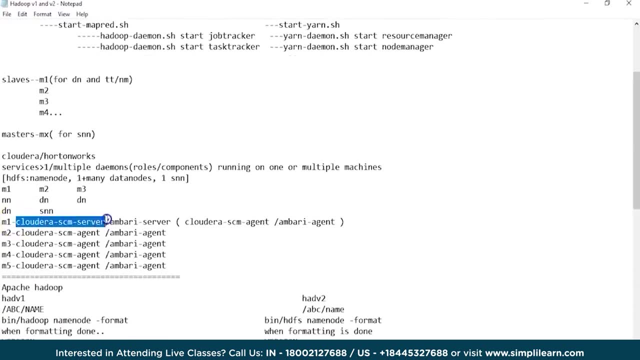 those scripts will individually start the different processes on different nodes. In case of Cloudera, we would always have a Cloudera SCM server which would be running on one machine, and then, including that machine, we would have Cloudera SCM agents which would be running on multiple machines. 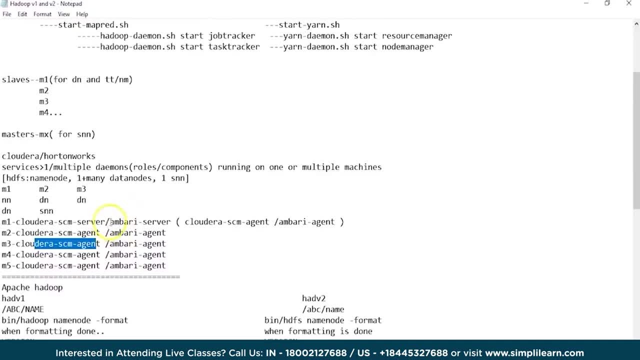 Similarly, if we had a Hortonworks cluster, we would have Ambari server starting up on the first machine and then Ambari agents running on other machines. So your server component knows what are the services which are set up, what are their configurations and agents running on every node. 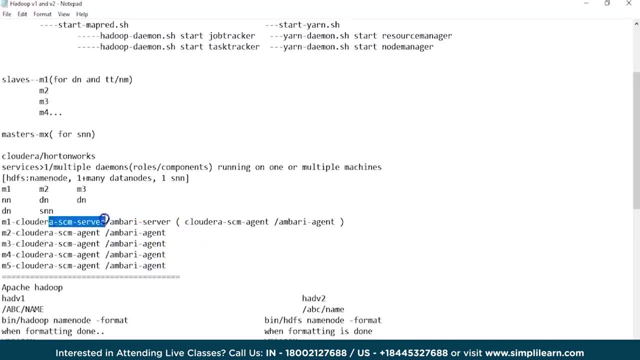 are responsible to send heartbeats to the server, receive instructions and then take care of starting and stopping up of individual roles on different machines. In case of our single node cluster setup in Quickstart VM, we would just have one SCM server and one SCM agent. 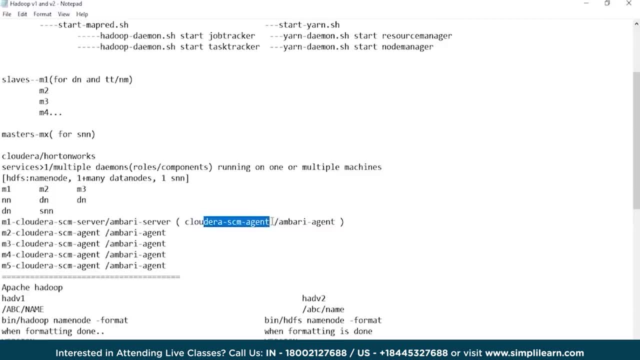 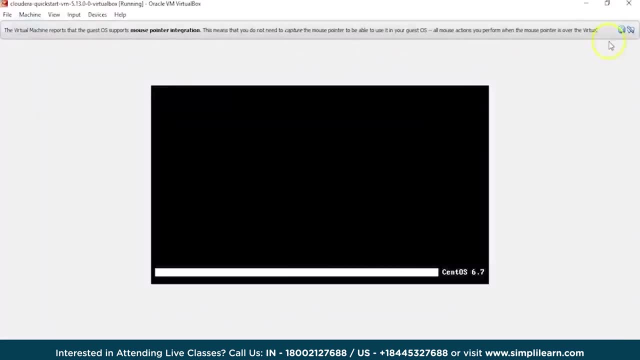 which will start on the machine, which will then take care of all the roles which need to be started for your different services. So we will just wait for our machine to come up and basically have Cloudera SCM server and agent running, and once we have that, 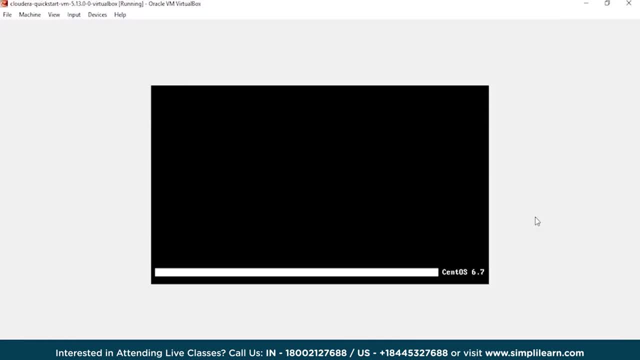 we need to follow few steps so that we can have the Cloudera admin console accessible, which allows you to browse the cluster, look at different services, look at the roles for different services and also work with your cluster, either using command line or using the web interface that is Hue. 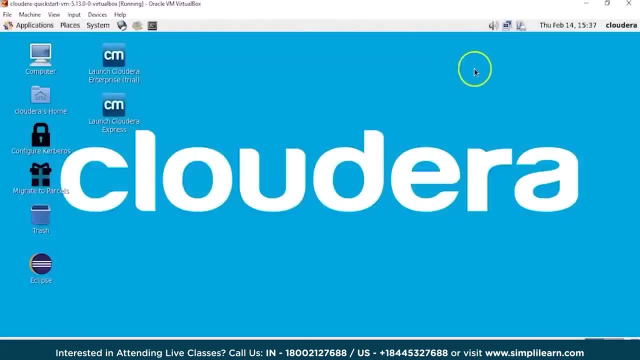 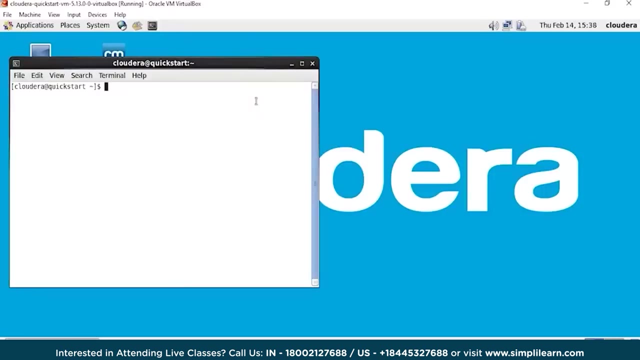 Now that my machine has come up and it already is connected to the internet, which we can see here, we need to do certain things so that we can have our admin console accessible At this point of time. you can click on terminal and check if you have access to the cluster. 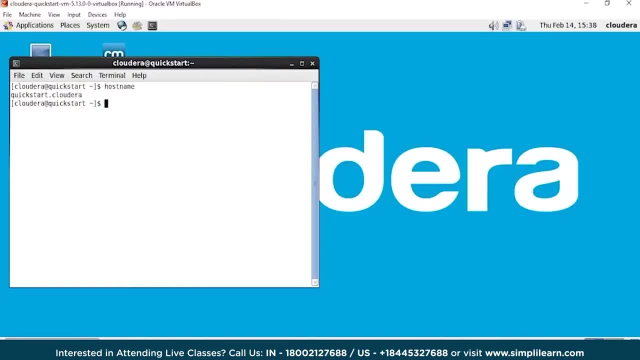 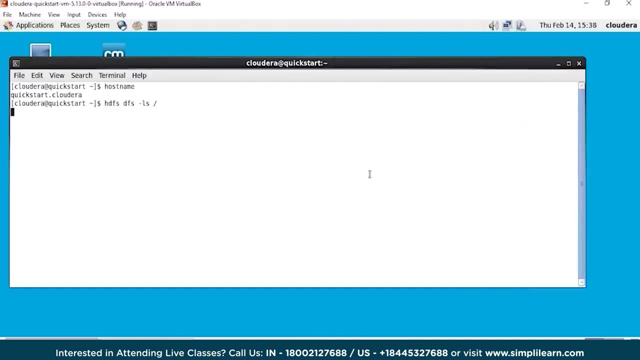 So here type in host name and that shows you your host name, which is quickstartcloudera. We can also type in HDFS command to see if we have access and if my cluster is working. These commands are same as you would give them in Apache Hadoop cluster. 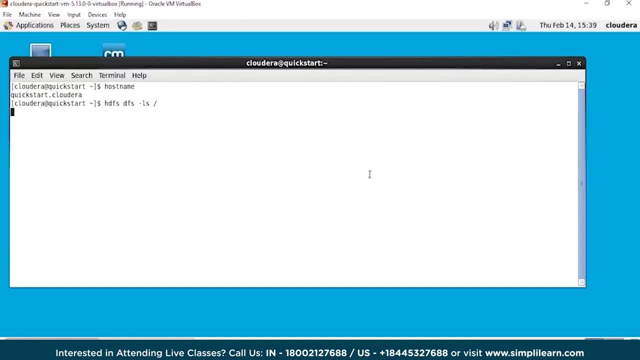 or in any other distribution of Hadoop. Sometimes, when your cluster is up and you have access to the terminal, it might take few seconds or few minutes before there is a connection established between Cloudera SCM server and Cloudera SCM agent running in the background. 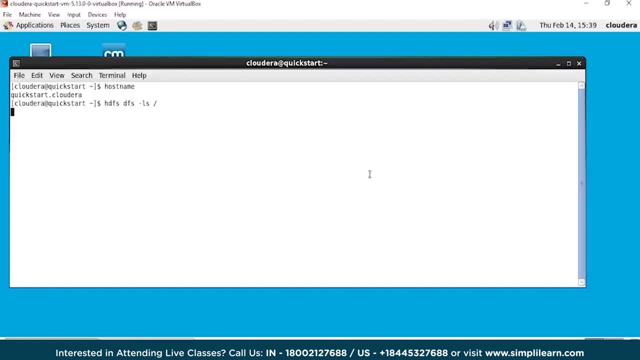 which takes care of your cluster. I have given HDFS DFS list command which basically should show me what by default exists on my HDFS. Let's just give it couple of seconds before it shows us the output. We can also check by giving a service. 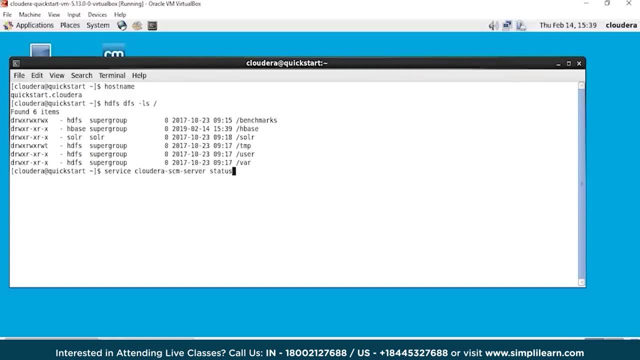 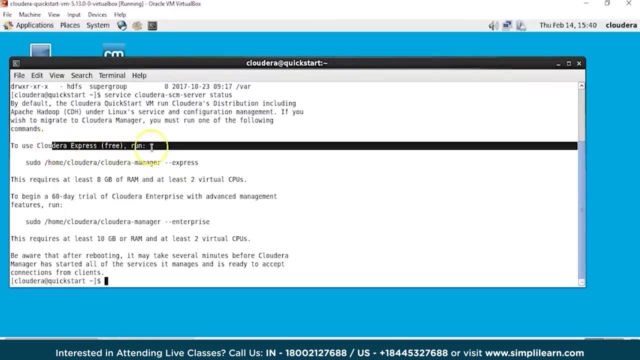 Cloudera SCM server status. and here it tells me that if you would want to use Cloudera Express free, run this command. It needs 8GB of RAM and at least 2 virtual CPU cores, and it also mentions it may take several minutes. 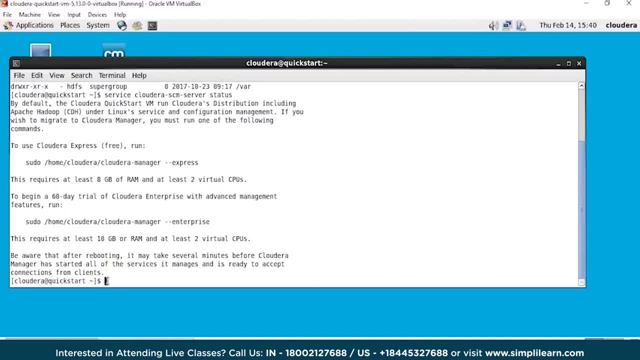 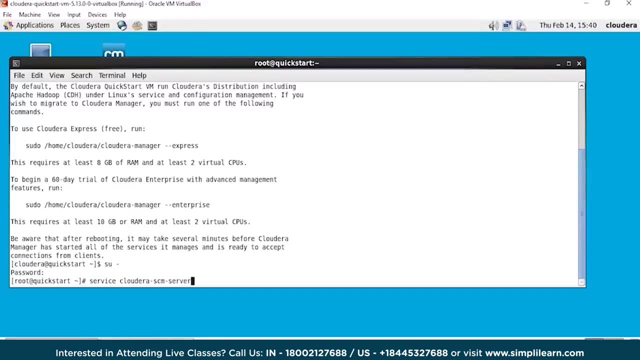 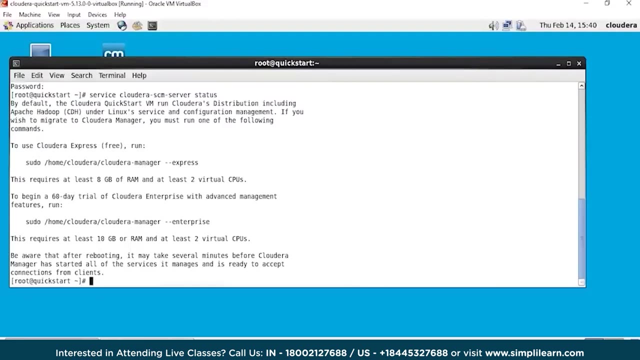 before Cloudera manager has started, I can login as root here and then give the command service Cloudera SCM server status. Remember, the password for root is Cloudera. So it basically says that. if you would want to check the settings, 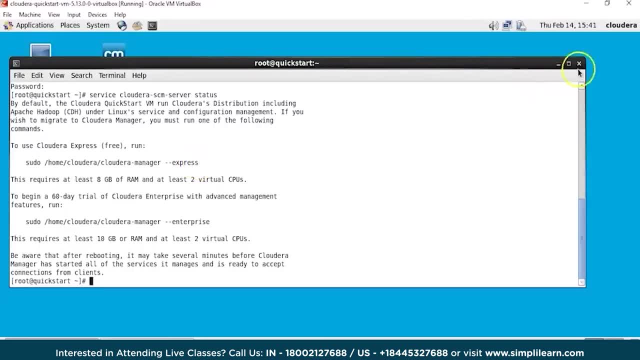 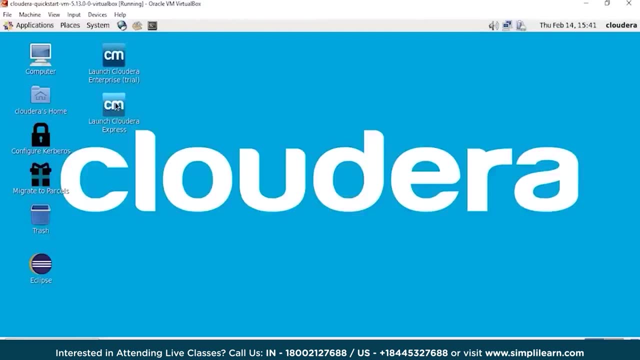 it is good to have Express edition running So we can close this. My HDFS access is working fine. Let's close the terminal and here we have launch Cloudera Express. Click on this and that will give you that you need to give a command. 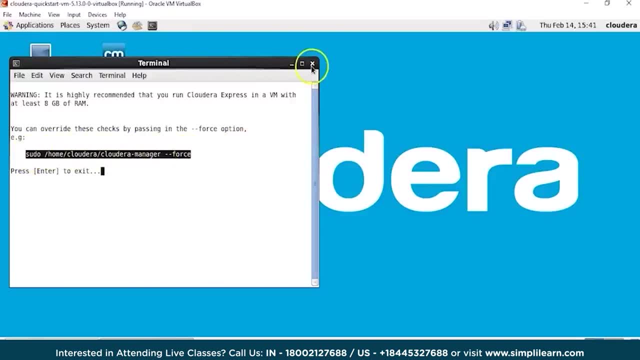 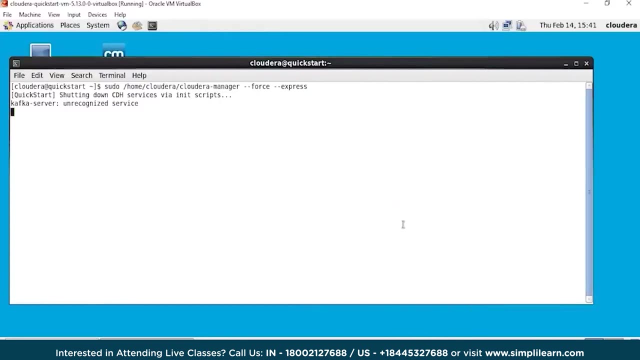 which is force. Let's copy this command, Let's open a different terminal and let's give this command like this, which will then go ahead and shut down your Cloudera based services, and then it will restart it, only after which you will be able to access. 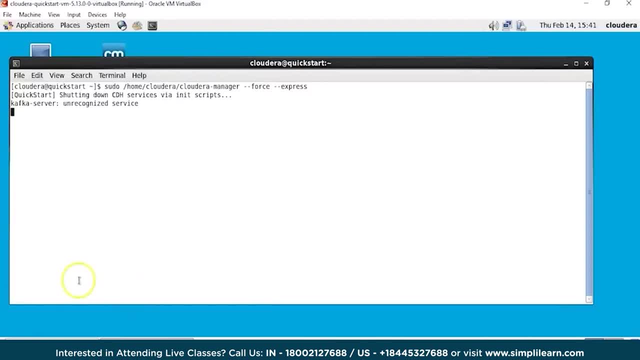 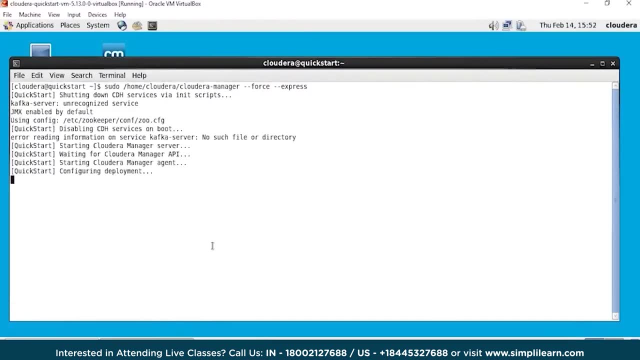 your admin console. So let's just give it couple of minutes before it does this and then we will have access to our admin console Here. if you see, it is starting the Cloudera manager server again. It is waiting for Cloudera. 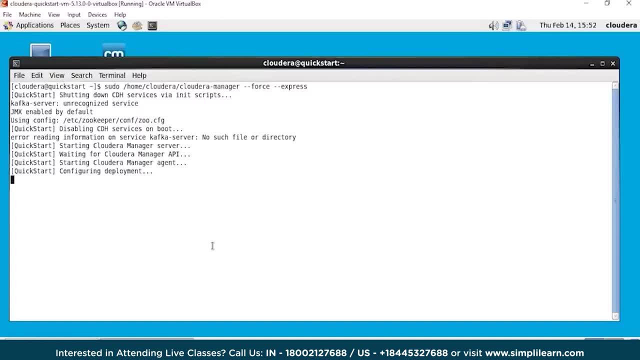 manager API, then starting the Cloudera manager agents and then configuring the deployment as per the new settings which we have given as to use the Express edition of Cloudera. Once all this is done, it will say the cluster has been restarted and the admin console. 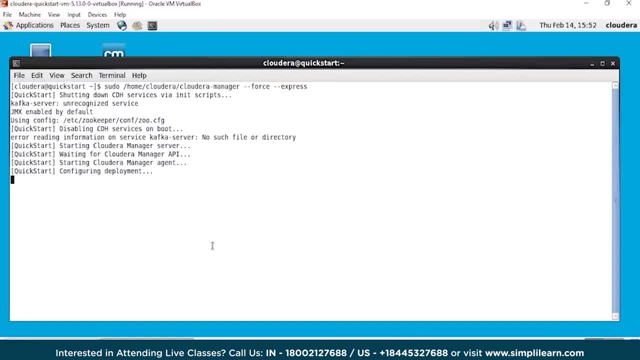 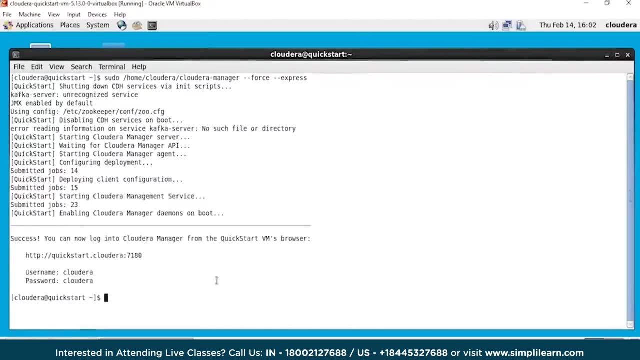 can be accessed by ID and password as Cloudera. We'll give it couple of more minutes And once this is done, we are ready to use our admin console. Now that deployment has been configured, client configurations have also been deployed and it has restarted. 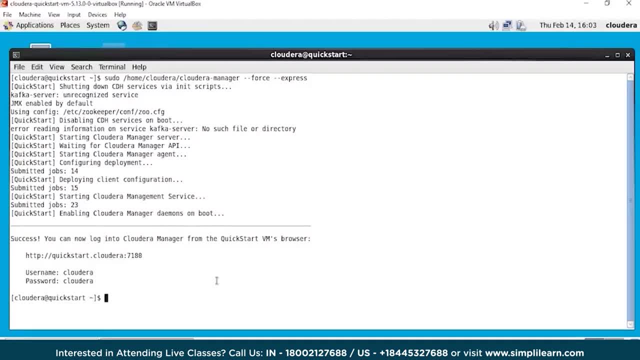 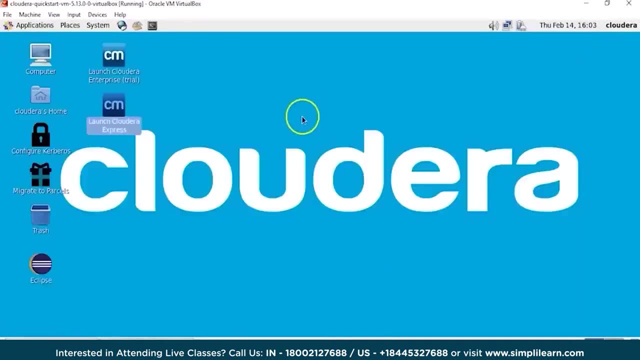 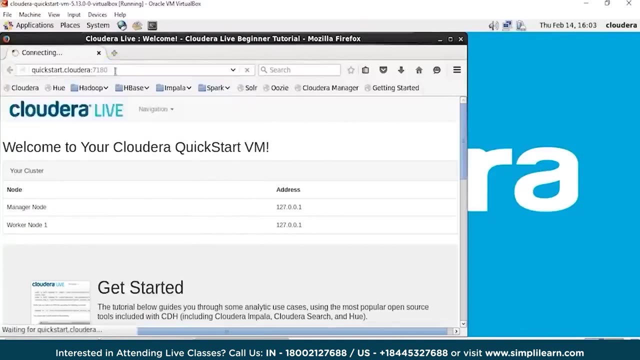 the Cloudera management service. it gives you an access to quick start admin console using username and password as Cloudera. Let's try accessing it So we can open up the browser here and let's change this to 7180.. That's the default. 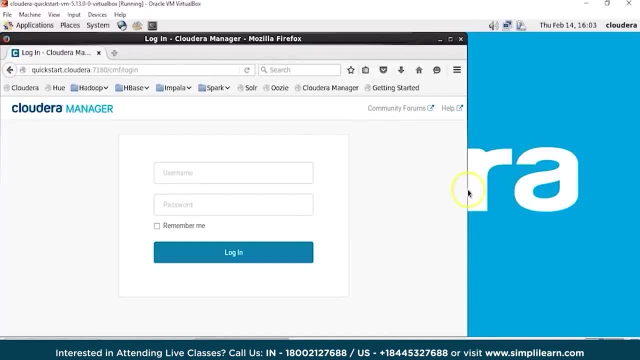 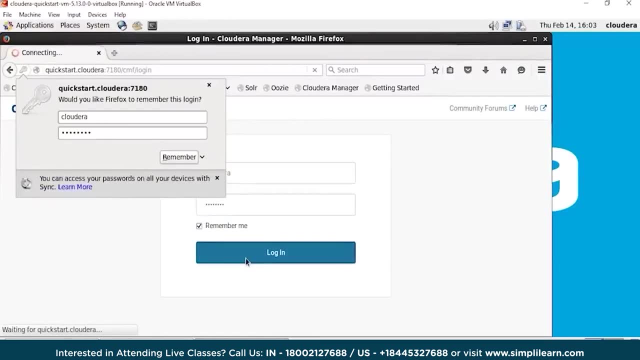 and that shows the admin console which is coming up Now. here we can log in as Cloudera Cloudera and then let's click on login. Now, as I said, Cloudera is very CPU intensive and memory intensive, So it would slow down. 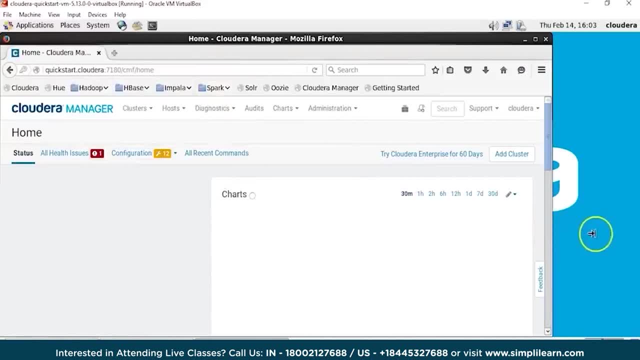 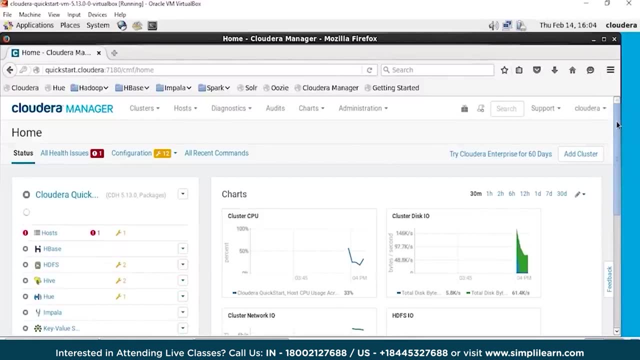 since we have not given enough GB RAM to our Cloudera cluster, and thus it will be advisable to stop or even remove the services which we don't need Now. as of now, if we look at the services, all of them look in a stop status. 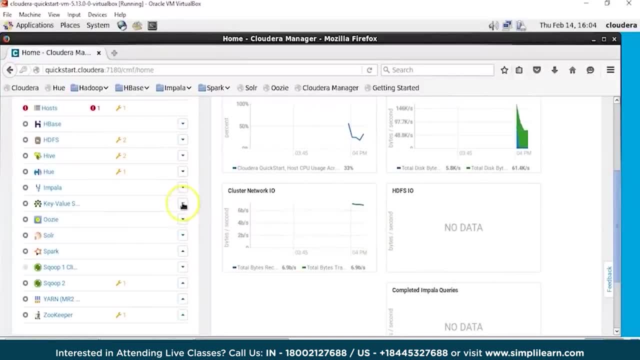 and that's good in one way, because we can then go ahead and remove the services which we will not use in the beginning and later we can anytime add services to the cluster. So, for example, I can click on key value store here and then I can scroll down. 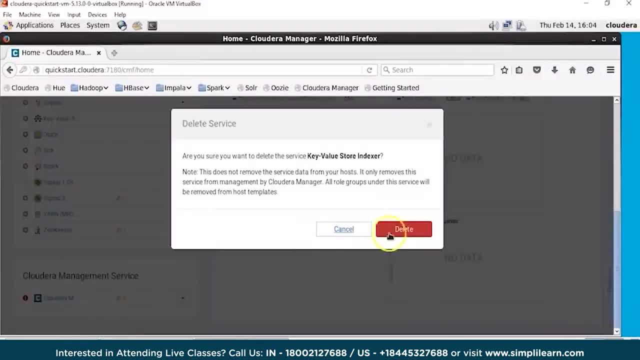 where it says delete, to remove this service from the admin console. Now, anytime you are removing a particular service, it will only remove the service from the management by Cloudera manager. All the role groups under this service will be removed from host templates. 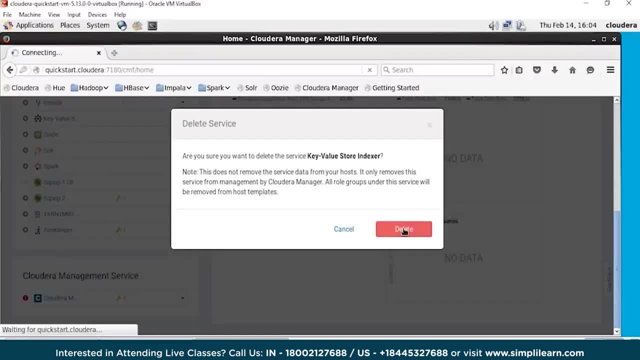 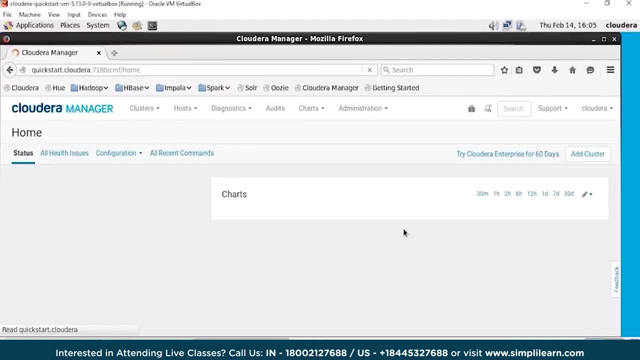 So we can click on delete Now. if this service was depending on some other service, it would have prompted me with a message that remove the relevant services on which this particular service depends. If the service was already running, then it would have given me. 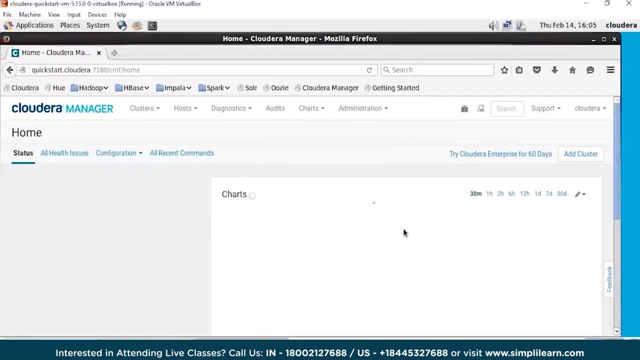 a message that the service has to be stopped before it can be deleted from the Cloudera admin console. Now, this is my admin console, which allows you to click on services. look at the different roles and processes which are running for this service. We anyways have access. 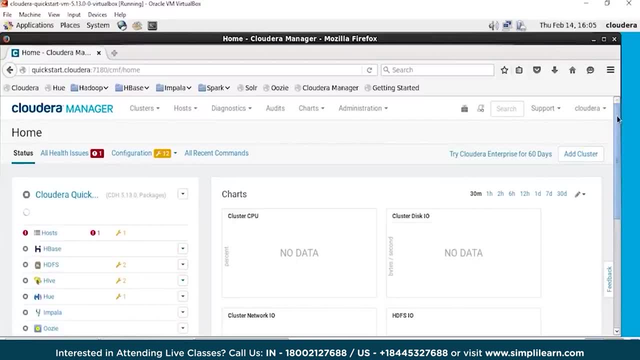 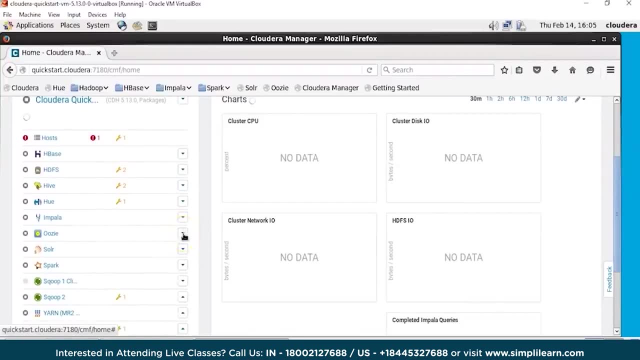 to our Cloudera cluster from the terminal using our regular SDFS or YARN or MapRed commands. Now I removed a service, I will also remove Solar, which we will not be using for the beginning, but then it depends on your choice So we can here. 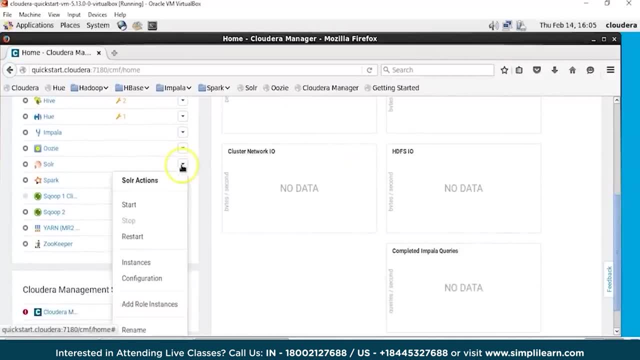 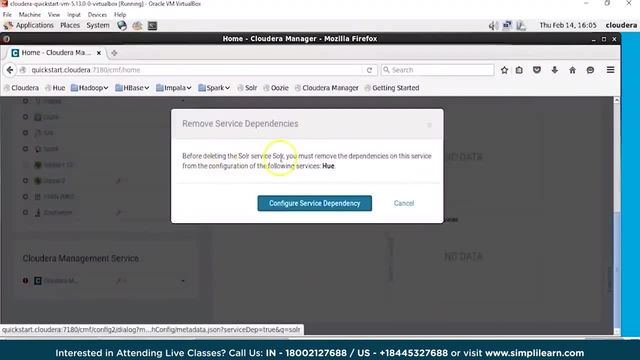 scroll down to delete it. and that says that before deleting the Solar service, you must remove the different roles and processes which are running for this service. So we can click on this. You must remove the dependencies on this service from the configuration of following services: 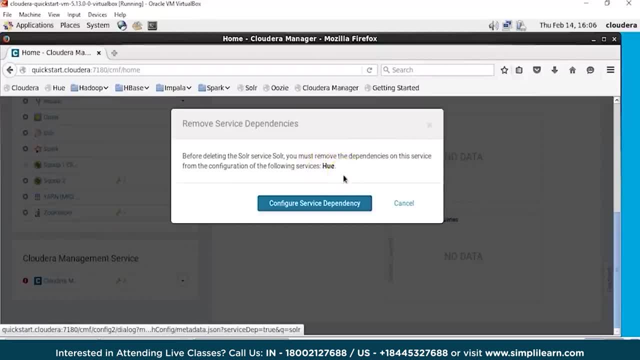 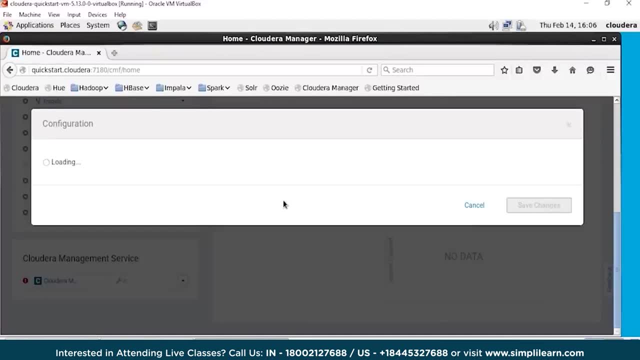 that is Hue. Now, Hue is a web interface which allows you to work with your SDFS, and that is depending on this. So click on configure service dependency and here we can make sure that our Hue service does not depend on a particular service we are removing. 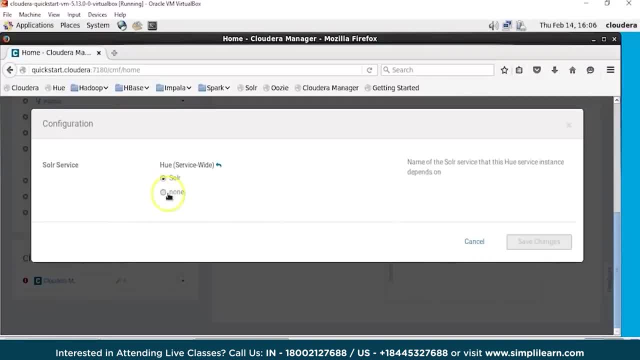 so that then we can have a clean removal of the service. So I will click on none and I will say save changes. Once this is done, then we can go ahead and start by removing the Solar service from our admin console, which will reduce some load. 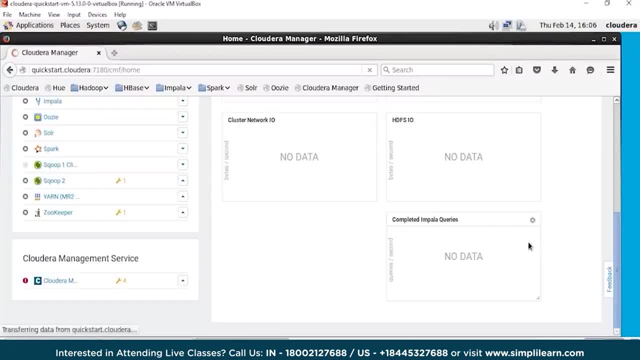 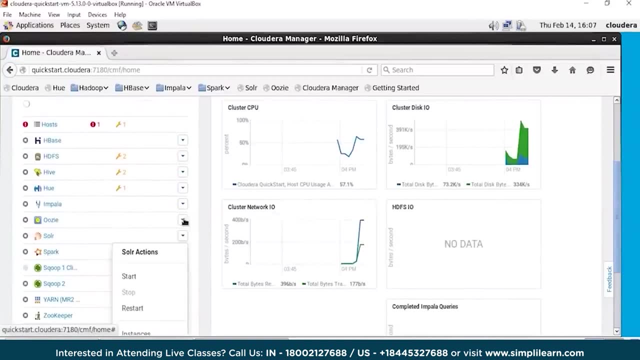 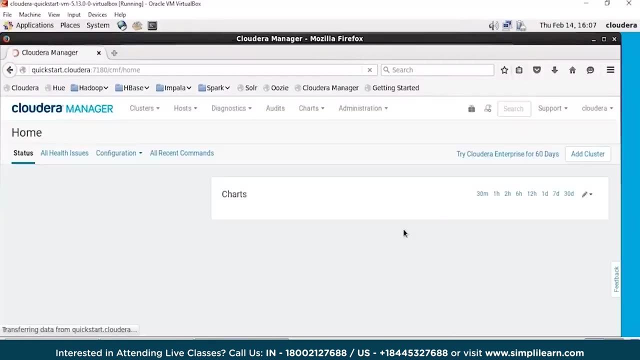 on my management console, which will also allow me to work faster on my cluster. Now here we have removed the dependency of Hue on Solar, so we can click on this and then we can delete it. Remember, I am only doing this so that my cluster becomes little lighter. 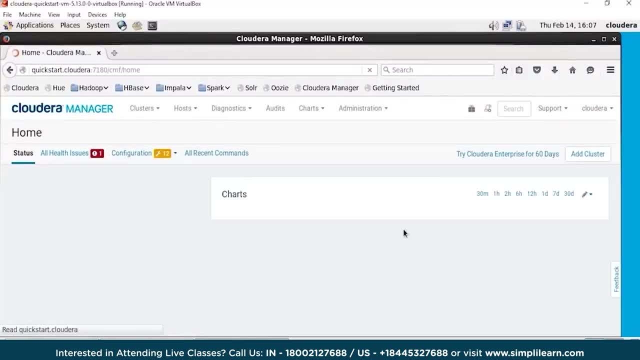 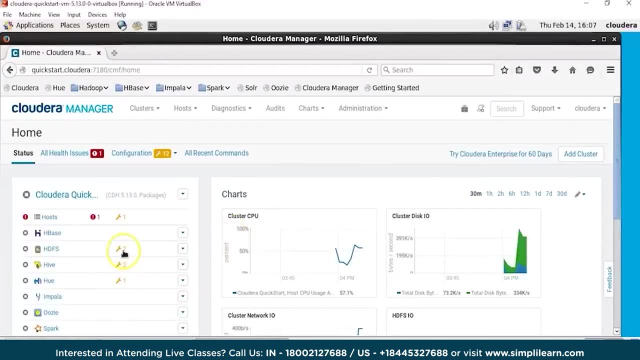 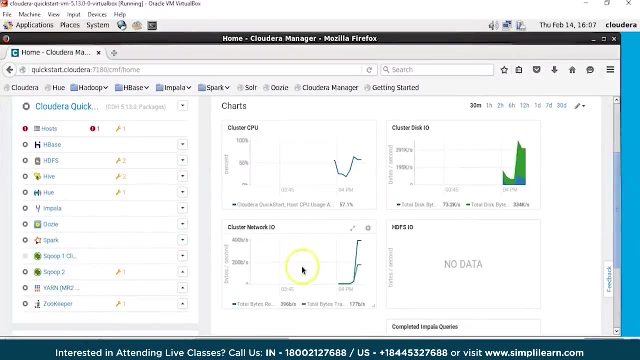 and I can work on my focus services at any point of time. if you want to add more services to your cluster, and any time, do that. you can fix different configuration issues like what we see here, with different warning messages, and here we have these services which are already existing. 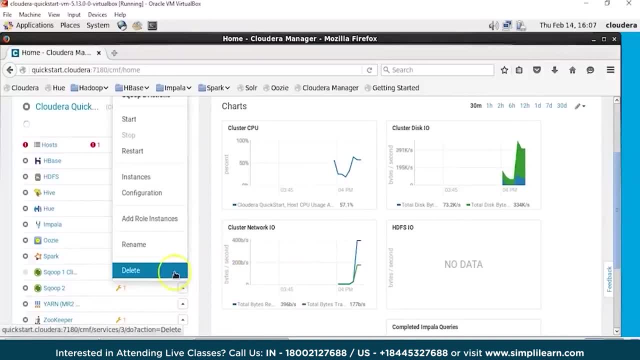 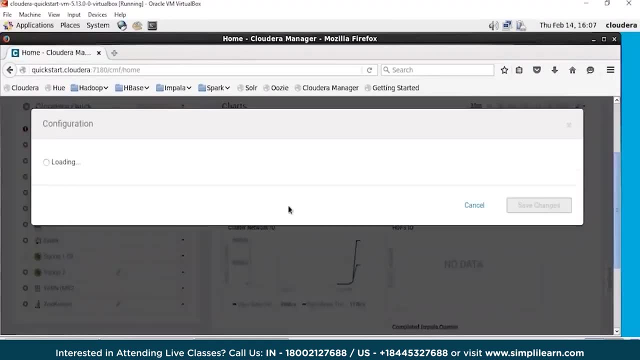 now, if we don't need any of the service, I can click on the drop down and click on delete again. this says that Scoop2 also has relevance to Hue, so Hue as a web interface also depends on Scoop2. as of now, we will make it. 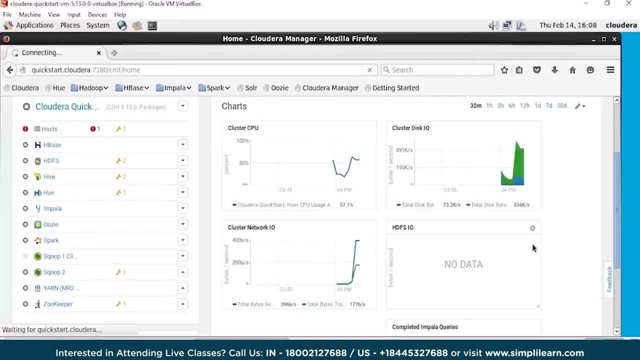 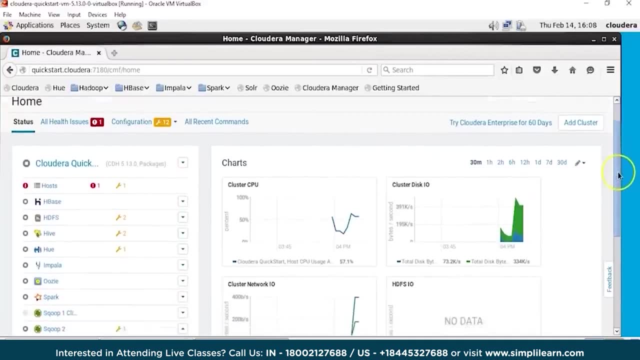 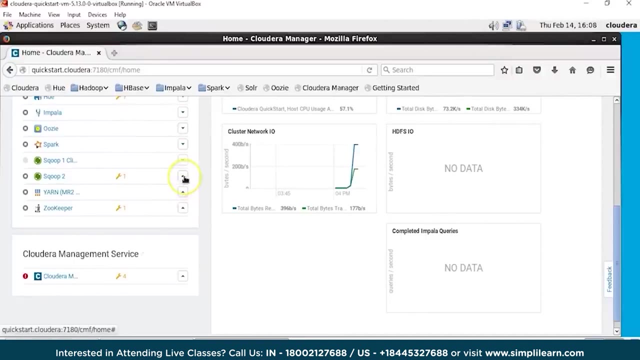 none. you can add the services by clicking the add service option. now this is a cluster to which you have admin access, and this is a quick start VM which gives you a single node cloud error cluster which you can use for learning and practicing. so here we will click. 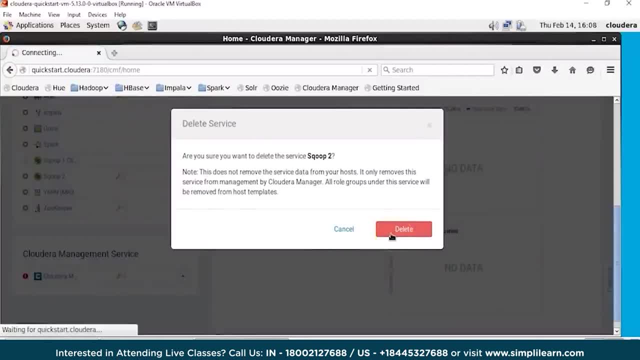 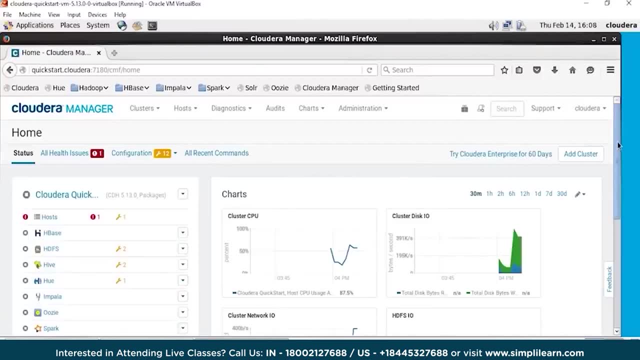 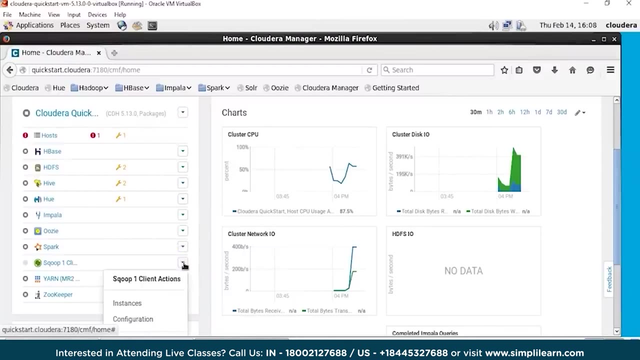 on Scoop2 and then we will say delete, as we have configured the dependency now and we will remove Scoop2 also. once this is done, we have removed three services which we did not need. we can even remove Scoop2 as a client and if we need, 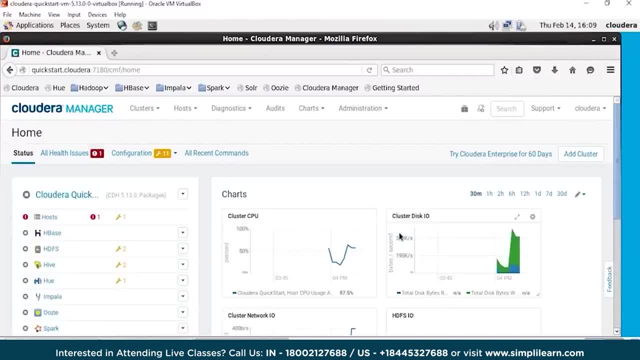 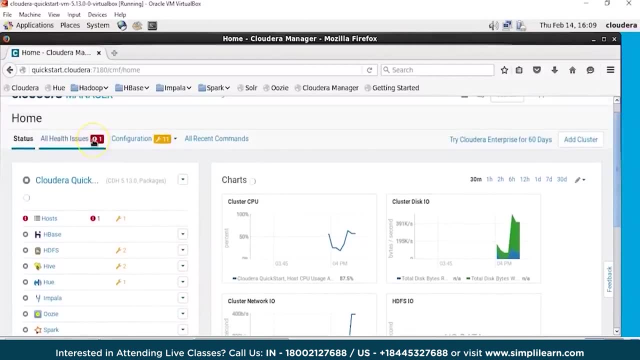 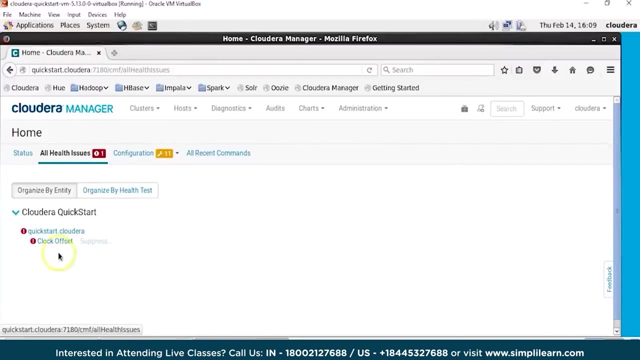 we can add that later now. there are various other alerts which your cloud data admin console shows and we can always fix them by clicking on the health issues or configuration issues. we can click here and see what is the health issue and we can see that there is. 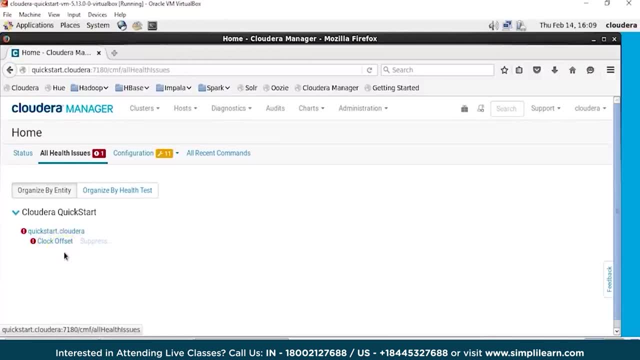 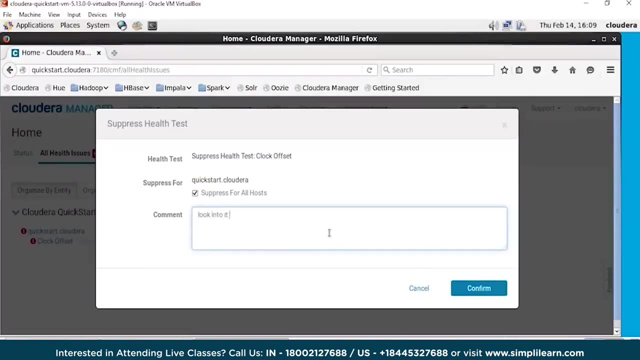 a clock offset which basically relates to an NTP service network time protocol which makes sure that one or multiple machines are in the same time zone and are in sync. so for now we can click on suppress and we can just say suppress for all hosts and we can say: 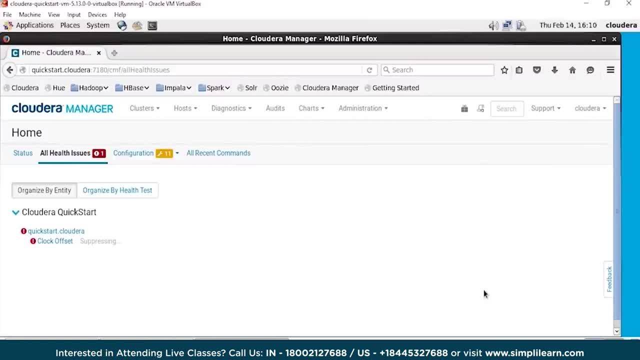 look into it later and confirm that it might not be in sync now. that does not have an impact for our use case as of now, but if we have a Kerberos kind of setup which is for security, then basically this offset and time zone becomes important, so we can ignore. 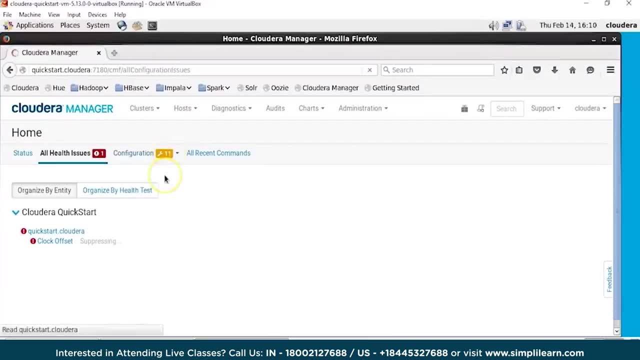 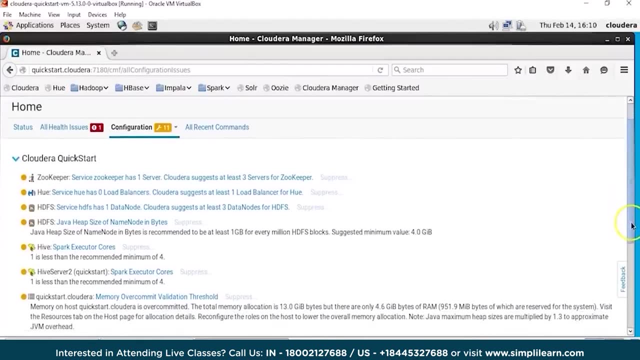 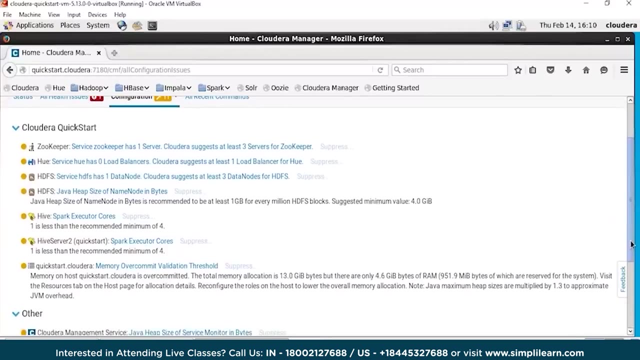 this message and we are still good to use the cluster. we also have other configuration issues and you can click on this which might talk about other issues, like the cluster should be in odd numbers. Q does not have a load balancer. SDFS only has one data node. 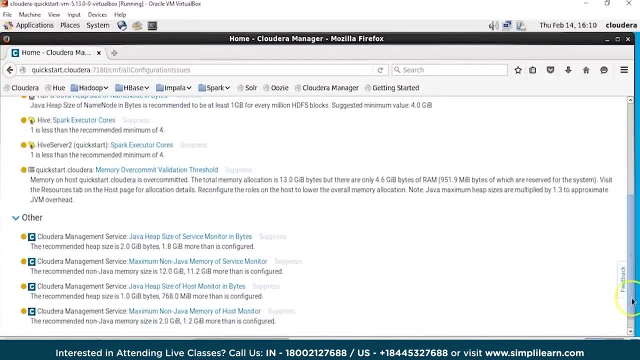 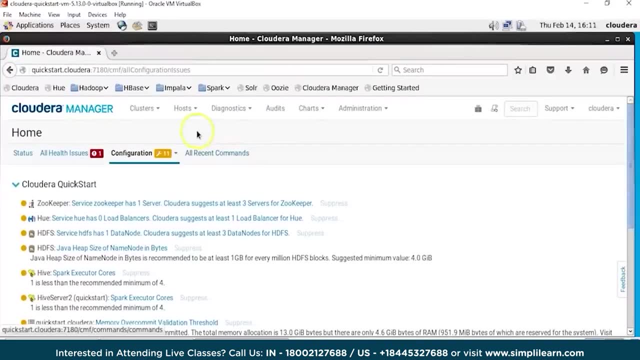 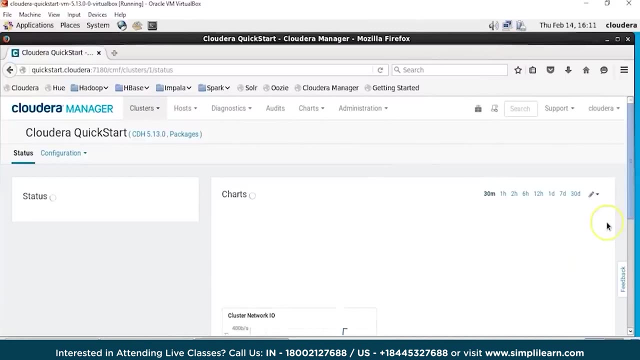 but all of these issues are not to be worried upon because this is a single node cluster setup. so if you want to avoid all of these warnings, you can always click on suppress and you can avoid some services which we don't intend to use now. I have also 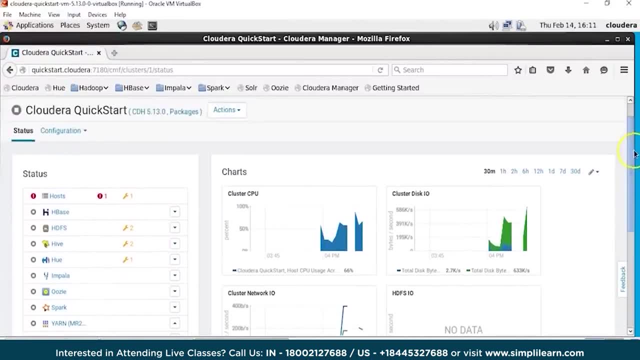 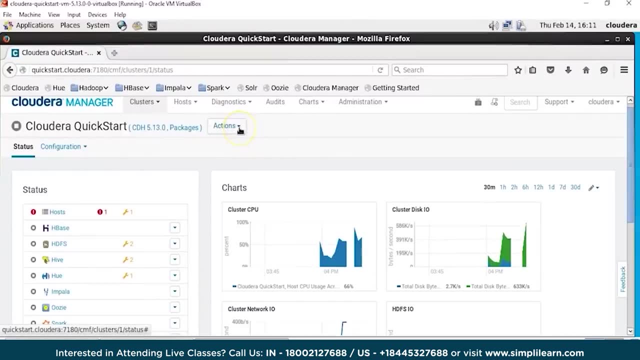 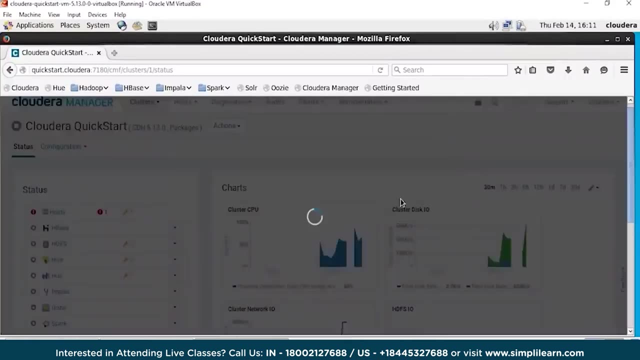 suppressed a offset warning, which is not very critical for my use case and basically I am good to start the cluster at any point of time. as I said, if you would want to add services, this is the actions button which you can use to add service. so we will. 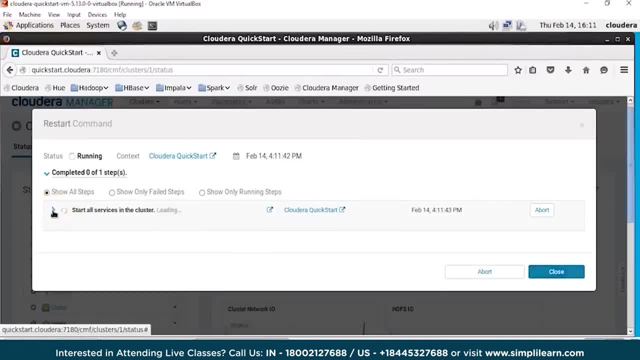 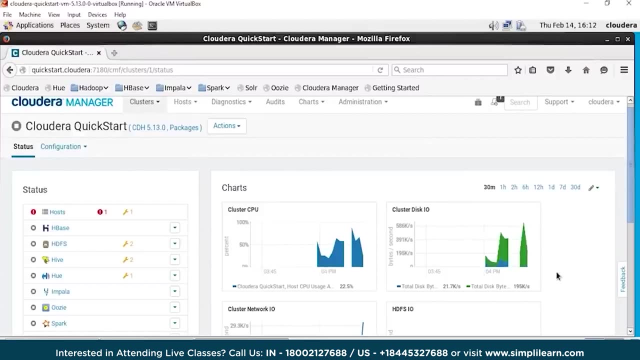 just say you can always click on this arrow mark and see what is happening in the services, what services are coming up and in which order. if you have any issues, you can always click on the link next to it, which will take you to the logs and we can. 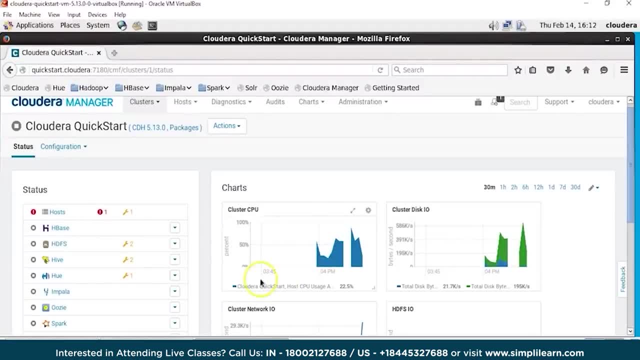 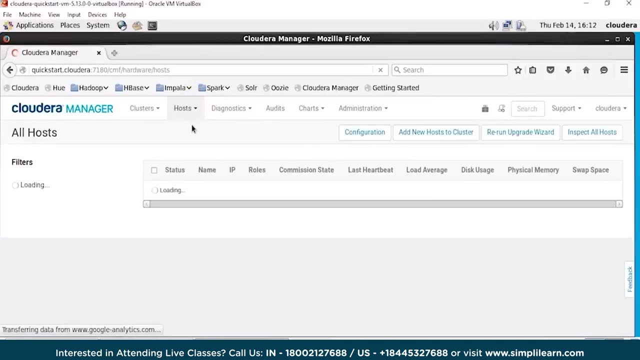 click on close to let it happen in the background. so this will basically let my services restart as soon as you have your commands. now, while my machines are coming up, you can click on hosts and you can have a look at all the hosts we have as of. 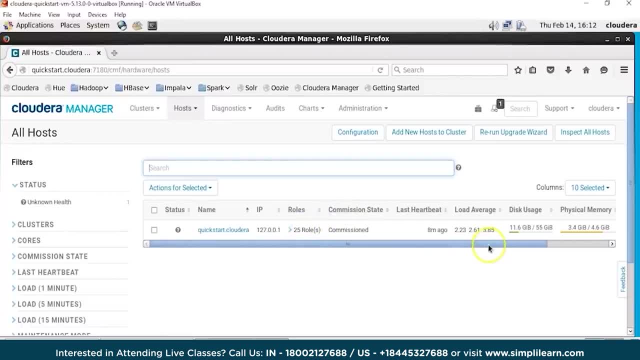 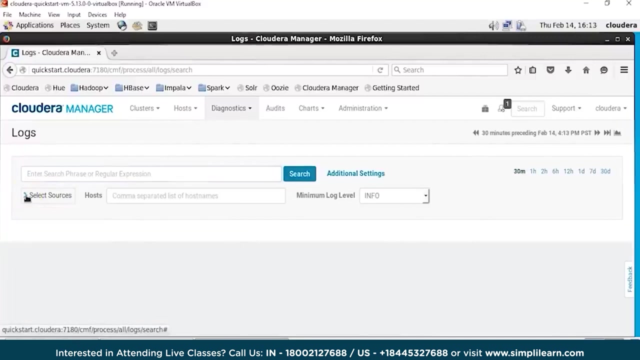 now only one, which will also tell you how many roles or processes are running on this machine. so that is 25 roles. it tells you what is the disk usage. it tells you what you have. so you can also look at the logs, which will give you access to. 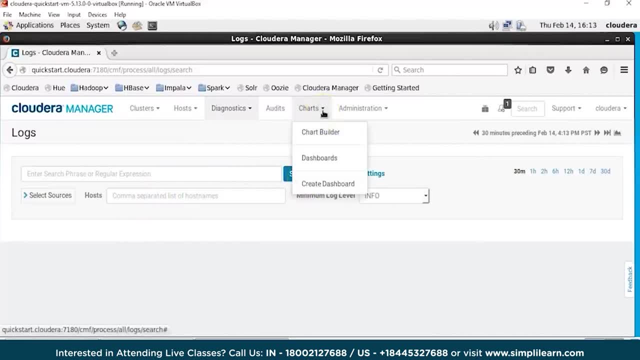 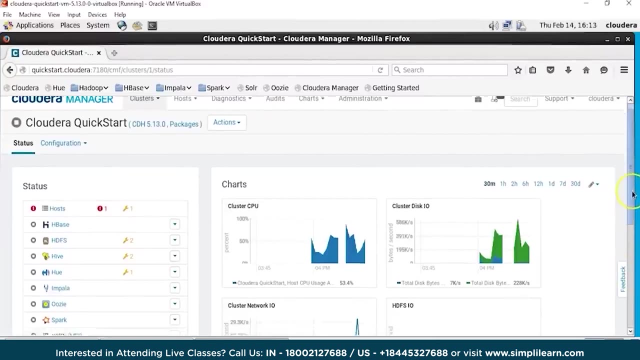 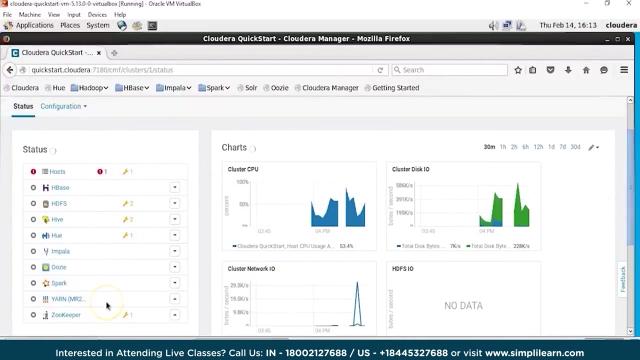 all the logs. you can even select the sources from which you would want to have the logs, or you can give the host name. you can click on search, you can build your own, And once we have our cluster up and running- whether that is showing all services in green or in a different status- we still should be able to access the service. 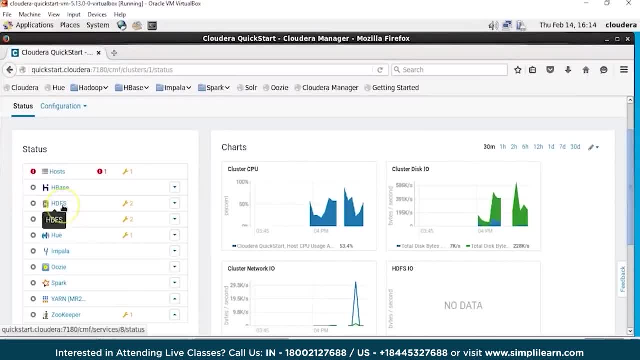 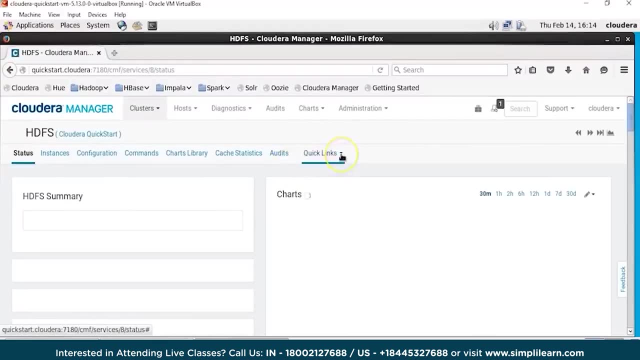 Now, as we saw in Apache Hadoop cluster, even here we can click on HDFS and we can access the web UI once our HDFS service is up by clicking on quick links. So the service is not yet up. Once it is up, we should be able to see the web UI link which will allow you to check things from HDFS web interface. 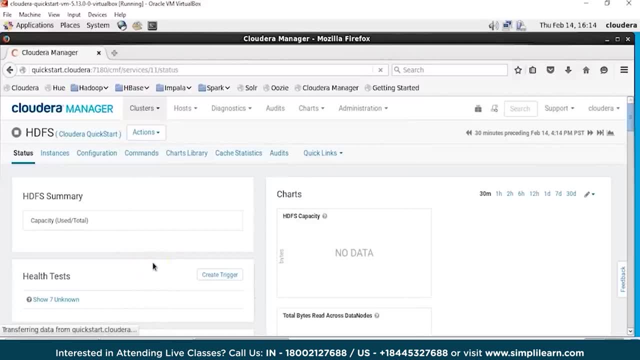 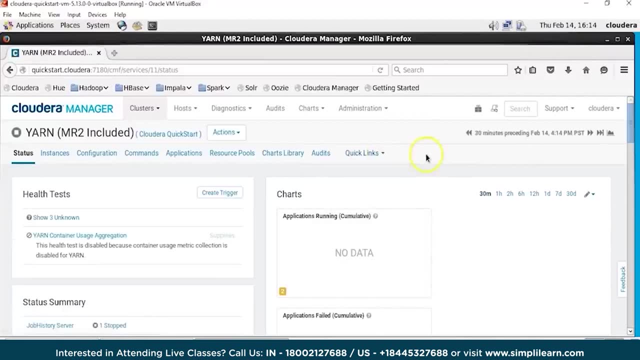 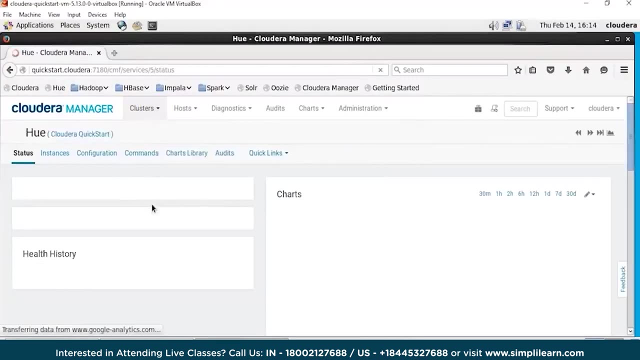 Similarly, YARN as a service also has a web interface. So, as soon as the service comes up under your quick links, we will have access to the YARN UI And, similarly, once the service comes up, we will have access to Hue, which will give you the web interface. 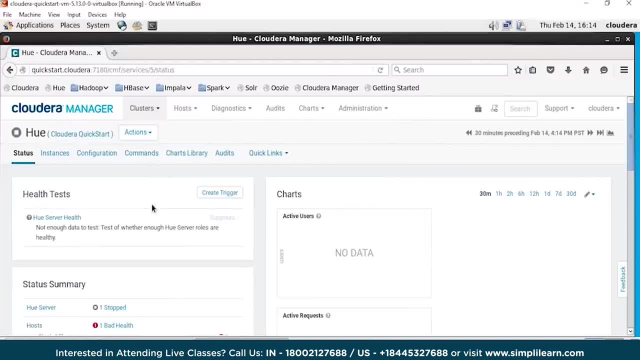 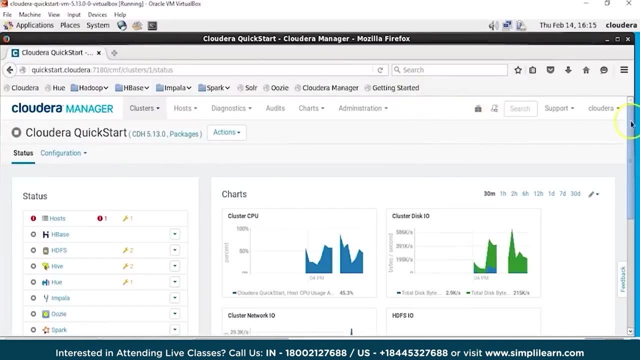 which allows you to watch the service. You can also work with your HDFS, which allows you to work with your different other components within the cluster without even using the command line tools or command line options. So we will have to give it some time while the Cloudera SCM agent on every machine will be able to restart the roles which are responsible for your cluster to come up. 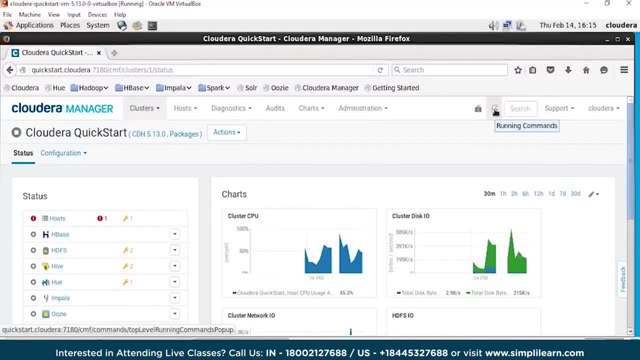 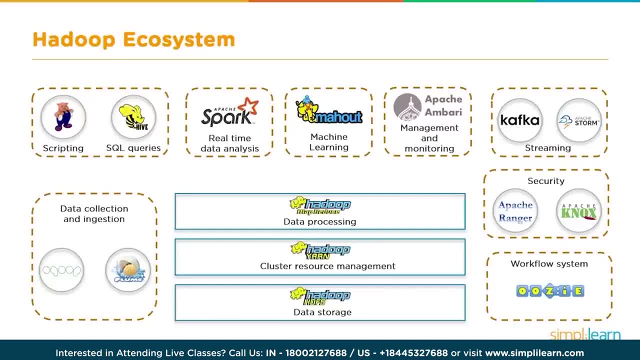 As HDFS we can go to the terminal and we can switch different things added in. There's a lot of overlapping in a lot of these tools, but we're just going to cover these basic tools so you can see what's available in the Hadoop ecosystem. 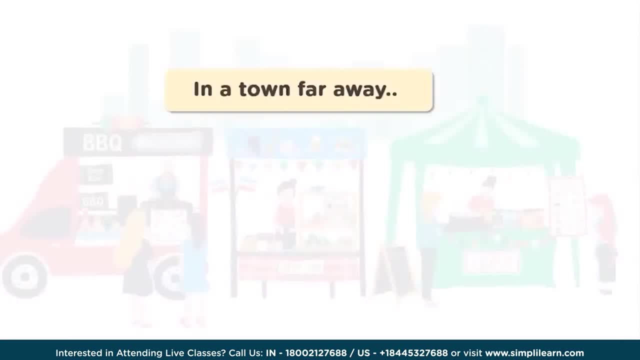 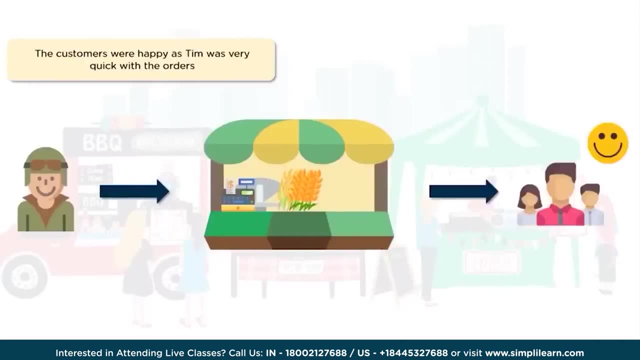 The question is: why Hadoop? Now let's understand that with an analogy. Just imagine, in a town far away, Tim sells food grains in his shop. The customers were happy as Tim was very quick with the orders and Tim sensed a good demand for other products, so he thought of expanding. 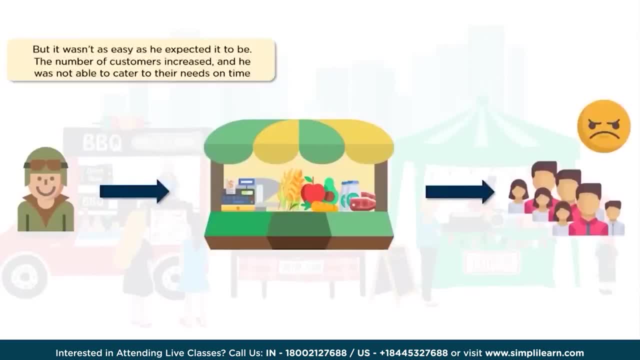 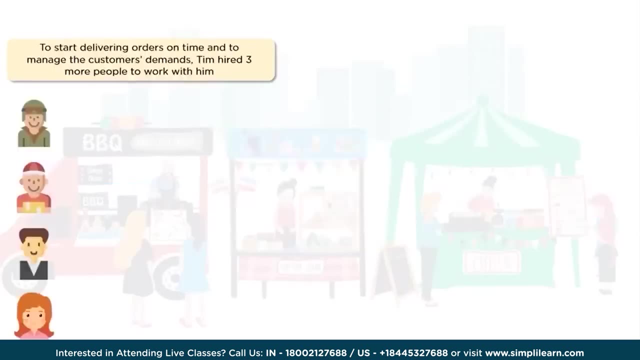 his business, But it wasn't easy as he expected it to be. The number of customers were increasing and he was not able to cater to their needs on time. He had to look into assisting his customers with each of their orders and billing. It was too difficult for him to manage alone. So what does he? 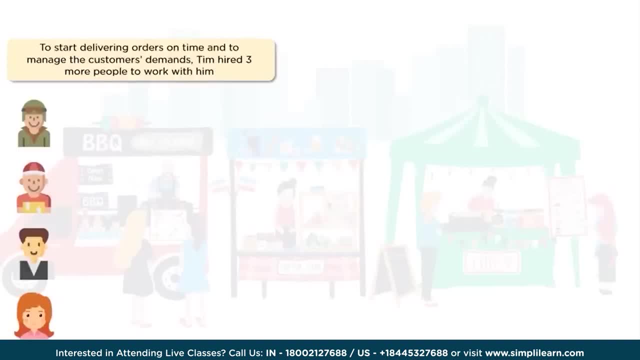 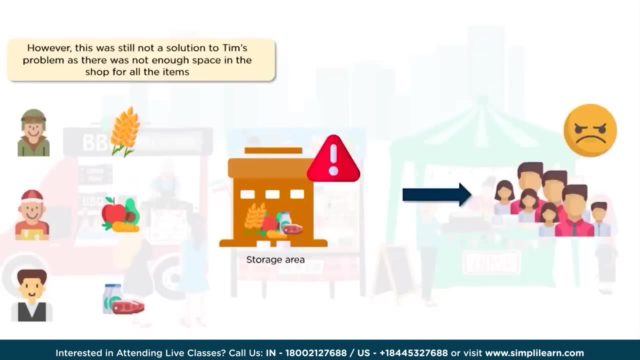 do To start delivering orders on time and to manage the customer's demand. Tim hired three more people to work with him, So it was Tim, it was Matt, Luke and Ann. Now there was still a problem. The problem was with storage area. So solutions which Tim was looking. 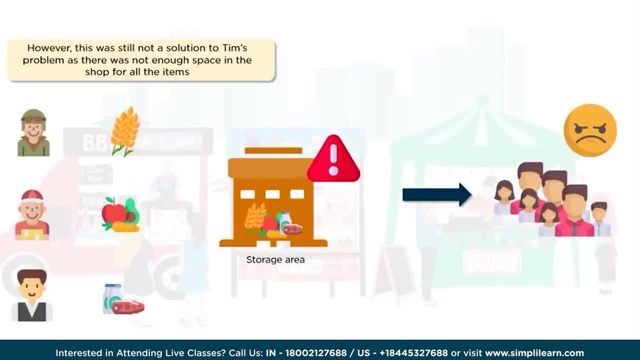 for was that he should have enough space in the shop for all the items so that he can cater to different customers for their different needs. And, as it seems, storage was a bottleneck, since storing and accessing became more and more difficult with increased supply and demand. 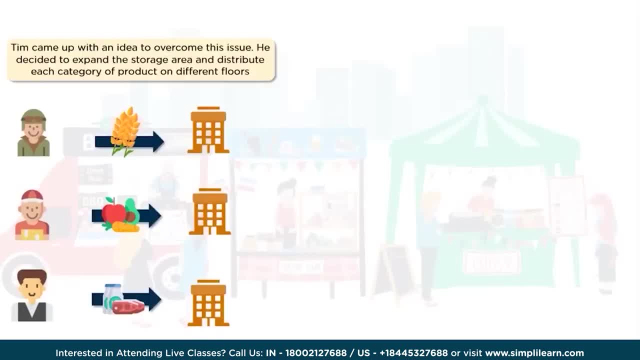 So what does Tim do? So Tim came up with an idea to overcome this issue. Basically, he decided to expand the storage area and distribute each category of product on different floors. Now, that's a smart thinking. Customers were happy and after picking up their 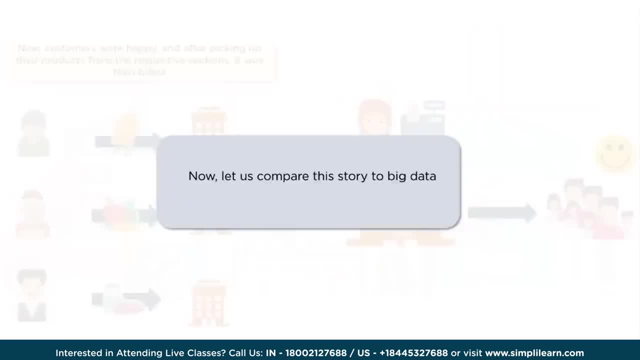 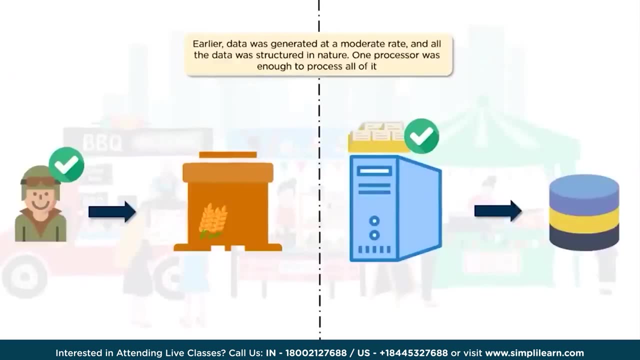 products from the respective sections. the products could be built. Now, if we compare this simple story of Tim to what we call as big data, let's talk in technical terms now. So we know that data has been critical and important for organizations. However, in the past, data was 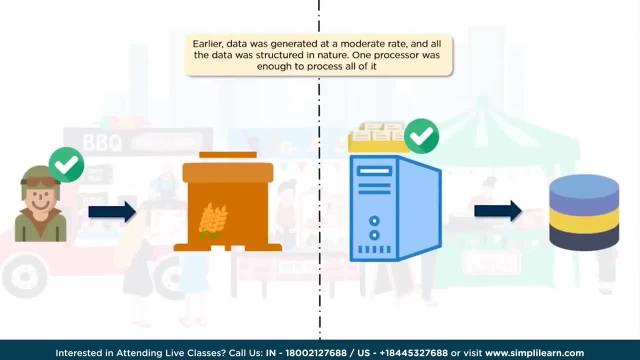 structured in nature. So when I say structured, data can have different types. Data can be structured, it can be semi structured and it can be unstructured. Now, when we talk about structure, semi structure or unstructured, the main difference is presence or absence of schema. 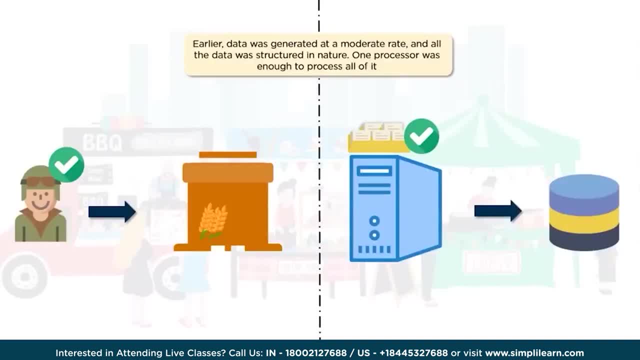 So if you can have schema defined well before the data comes in and then your data fits into that schema, we would call it as structured. If you have intelligently defined your schema, expecting your data to get stored within that schema. however, the data pattern breaks it. 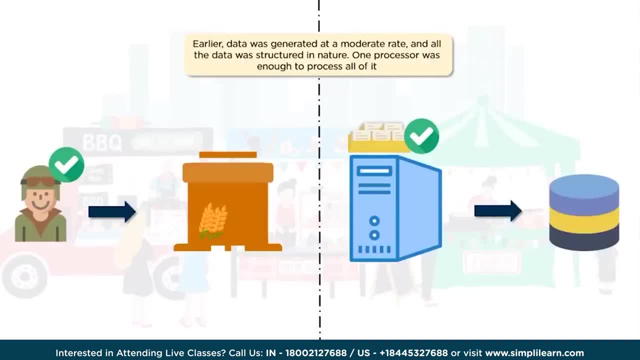 Then we are talking about unstructured data, or absence of schema in the data. You could have semi structured data, which basically means that you could have a mix of structured and unstructured data. Now, in the past, data was mainly structured and pretty much one processor was enough to process all of it. Now, as the data generation 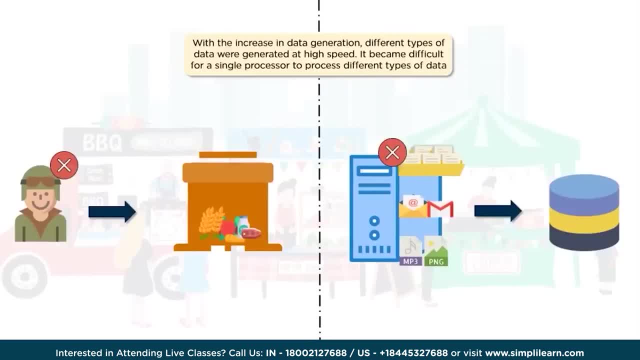 increased. there were different types of data, data which were getting generated, or I would say different type of data sets which were getting generated, and that too with a high speed. so it was evidently becoming difficult for a single processor or a single machine to store, to cure, to process, to mine, to analyze different types of data and data. 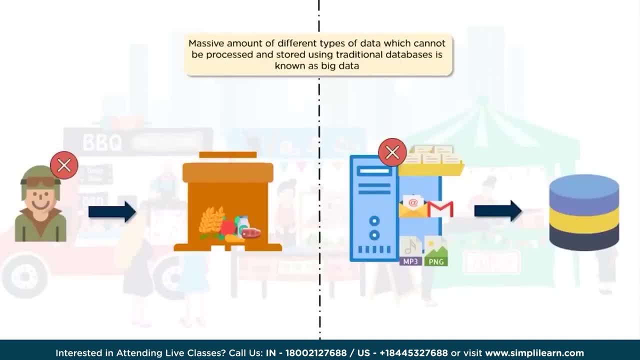 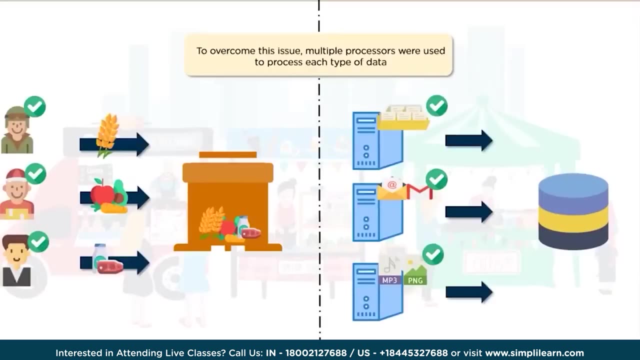 sets. now, with different types of data existing and they getting generated in massive amount, it posed a challenge that this data could not be processed and stored, and the known storage solutions were traditional databases. to overcome this issue, multiple processors were used. so this is where we started seeing a shift in paradigm from single processor to multiple processors. so I 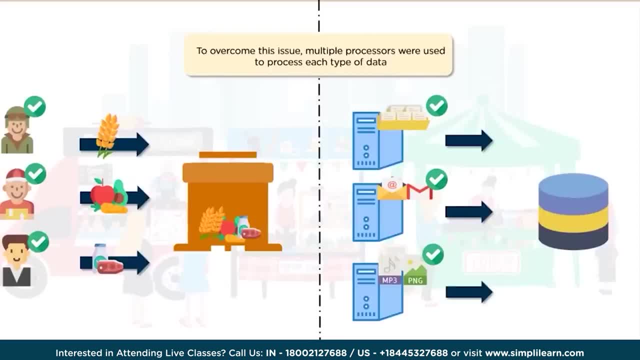 would say from a vertical scalable solution to a horizontal scalable solution. so when you say vertical scalability, we talk about increasing the number of processors that are stored and the number of processors that are stored and the capacity of a machine. when we talk about scalability, we mean a 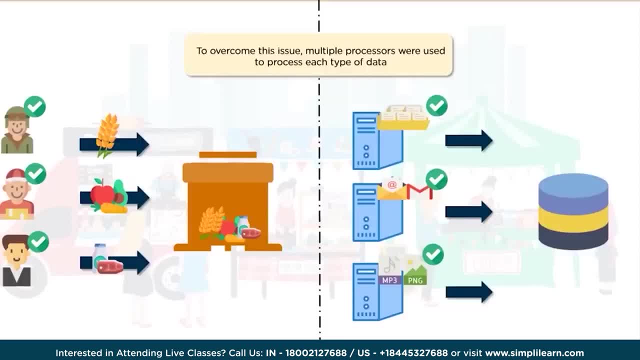 capability to scale, capability to expand and when we talk about a single processor, that is vertical scalability, where you would have one machine or one server with limited amount of RAM, limited amount of storage, and you could think of expanding that by adding more RAM, adding more storage, but that would 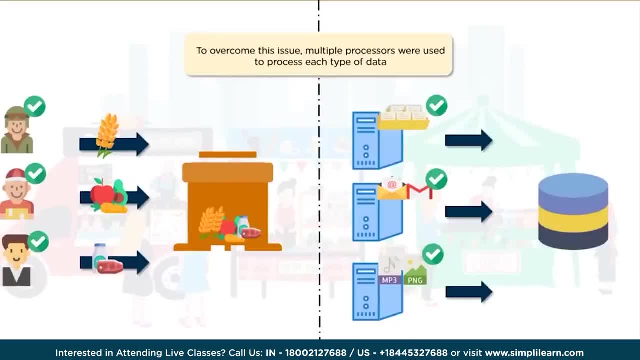 have some limits. you could not go beyond a particular limit. you probably would have to be locked in based on the number of processors that are stored and the based on the vendor, because you cannot change your internal components to suit your requirements and if we talk about horizontal scalability, that is multiple. 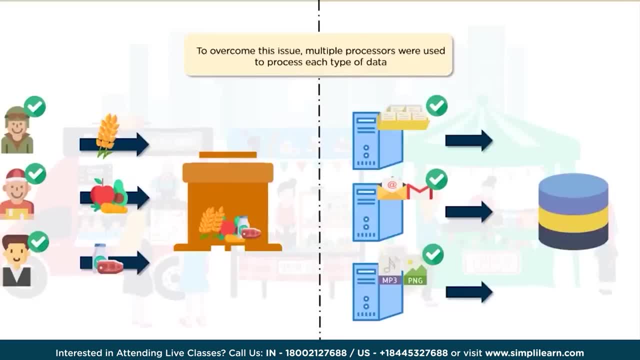 processors. in this case, we are talking about adding more machines so that you could have a horizontal, scalable architecture. now the problem which we were talking about: to overcome that issue, multiple processors were used to process each type of data, and here we see a similarity in Tim's approach to 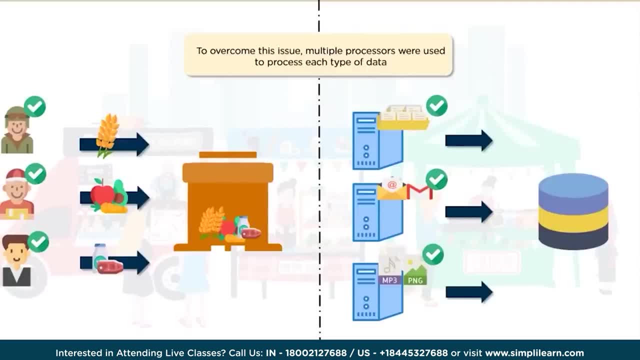 with the technical approach of going for a distributed platform which would handle huge amount of data, data coming in in different formats, data getting generated with a lot of speed and thus helping the organization. now what happens is when you think of having multiple solutions or having multiple systems which can be used to store or process your data. one of the major 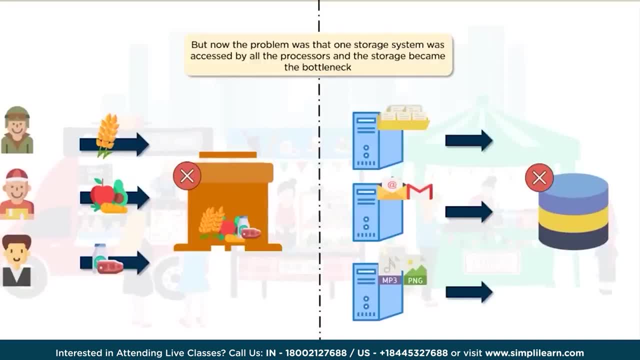 challenge is one storage system being accessed by all the machines becomes a bottleneck, and that is again a problem similar to what Tim was having when he decided to cater to multiple customers looking for different products, but then he was limited with the storage space he had and to keep all the products in one. 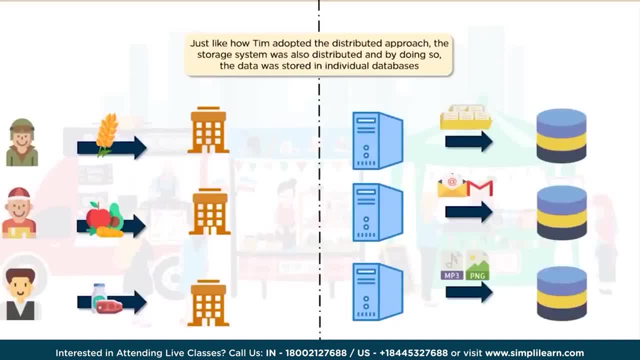 place. so, just like how Tim adopted the distributed approach, the storage system, which was a bottleneck, was also then distributed. so in this way, your data could be stored in individual databases or in individual machines, on their disks. however, it could be accessed from one place. so if we look at this story, we 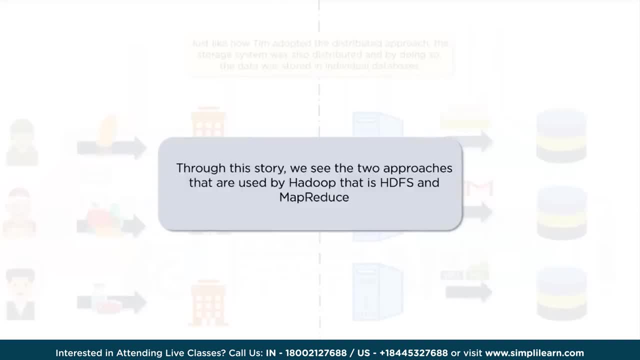 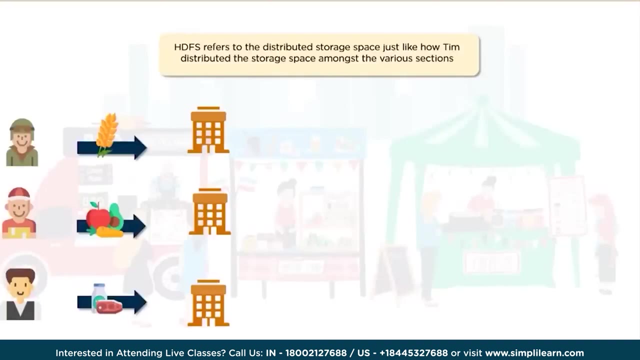 see two approaches, and these two approaches are the ones which are used by Hadoop, which is a framework, and these approaches are your storage layer, that is your SDFS, and your processing paradigm, that is MapReduce. now, what is SDFS? let's understand this. SDFS stands for Hadoop, distributed file system. so 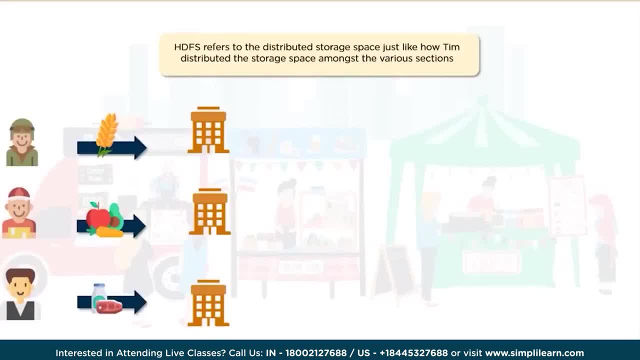 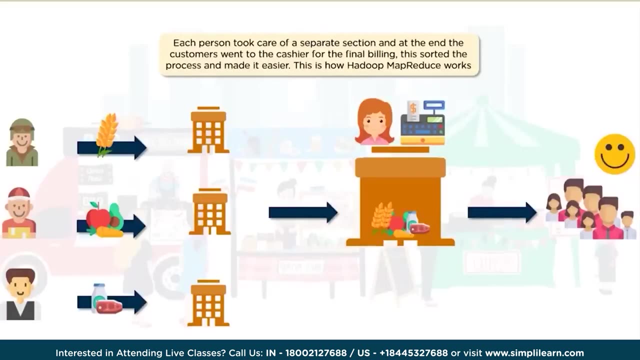 that's a logical storage layer. it's distributed storage space, just like our example of Tim having distributed the storage space amongst various sections. so each person was taking care of a separate section and at the end the customers went to the cashier for the final bidding. they sorted the process and make it easier, or made it easier now. 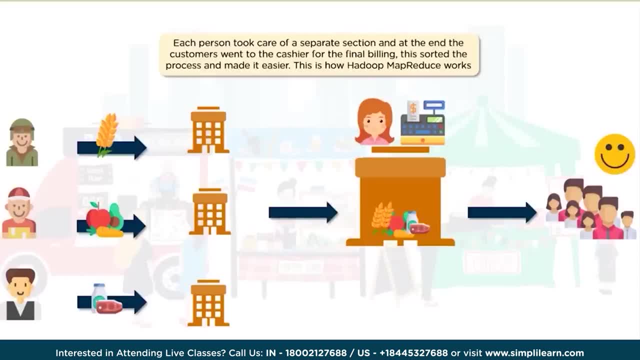 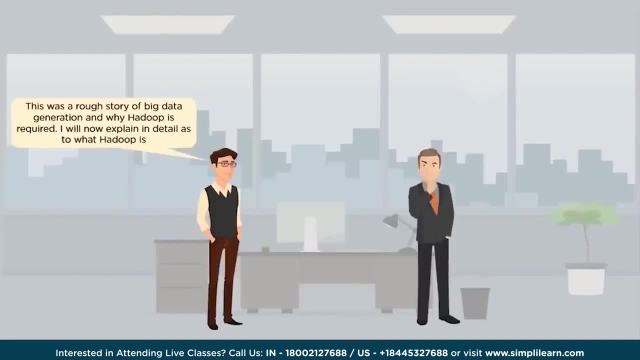 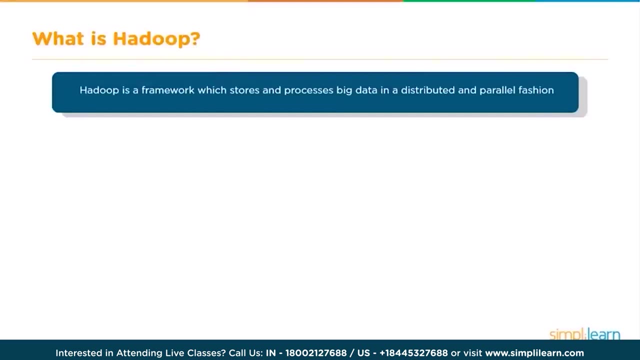 this is how similar or this is how Hadoop MapReduce works. now that was a rough story of big data generation and why Hadoop is required. right, let me explain what Hadoop is. so if we talk about what is Hadoop, it's basically a framework. it's not a programming language. it's not an architecture, it's not just a 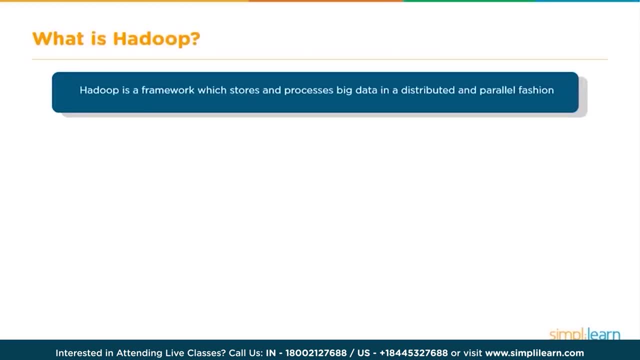 hardware. it's not just a software. it is a framework which allows you to store and process big data in a distributed and parallel fashion. now there are a lot of users which have made big data case study a famous and a popular one. so here are some companies, say Facebook or 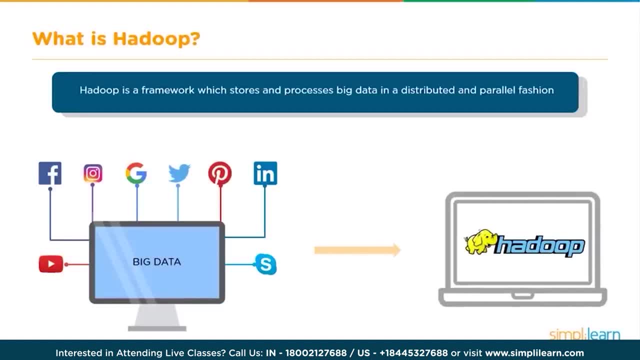 Instagram, Google, Twitter, LinkedIn, Skype, YouTube and many more, and these and many more organizations across the globe are using Hadoop for their storage and processing requirements. however, it would not be just Hadoop. Hadoop also comes with its own ecosystem, which has various set of open source technologies and 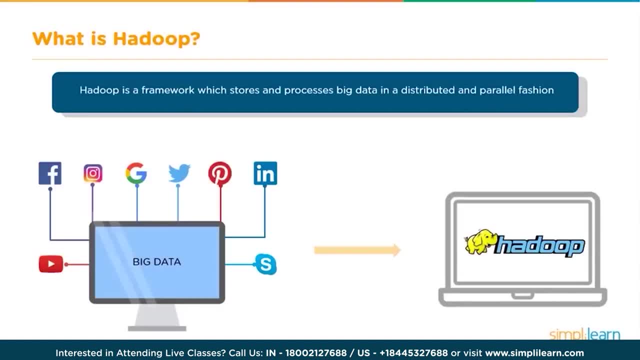 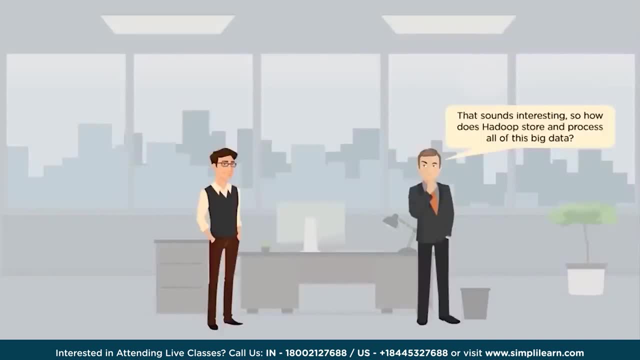 packages, all packaged together to help an organization in various facets of its data life. so the question is: how does Hadoop store and process all of this data, or I would say this big data? or, before we even talk about Hadoop, which has individual components which are 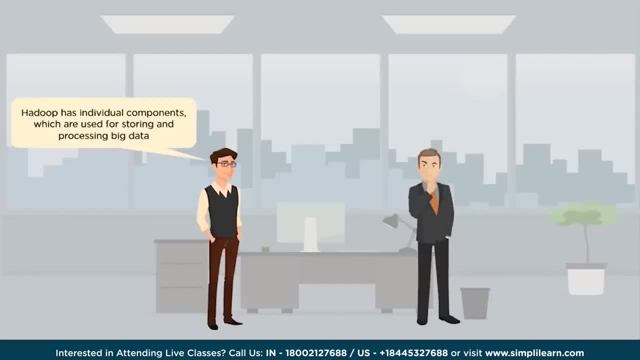 responsible for storing and processing big data. we also need to understand what is big data. so big data is just a term. data has been exponentially growing in past decade and now we don't talk about gigabytes or terabytes. we already are talking about petabytes and exabytes, or even zettabytes. that is, 10 to the power. 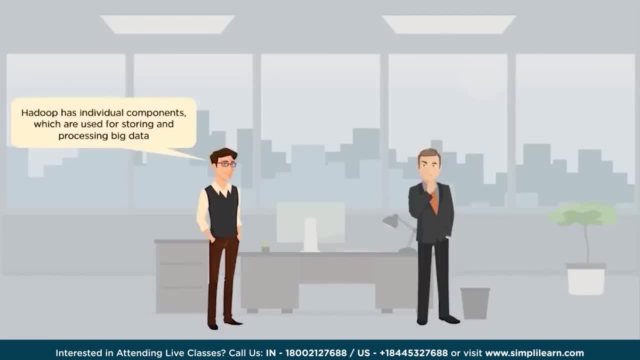 of seven bytes. however, in own factors, any organization is not processing zettabytes of data. but yes, there are organizations which are processing petabytes and exabytes of data. so how does Hadoop help them? and what is this big data? so big data is a term coined to explain the data which is very complex, which is huge. 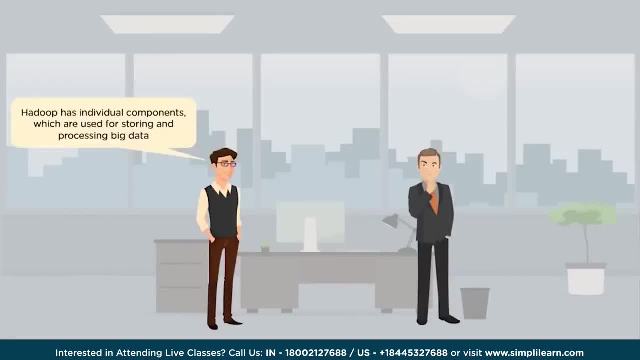 which is getting generated with a lot of speed, which has a lot of variety, and then it becomes a challenge to store, to capture, to analyze, process this data and derive useful information out of it. now we are talking about huge amount of data. we are talking about different V's, that is V. 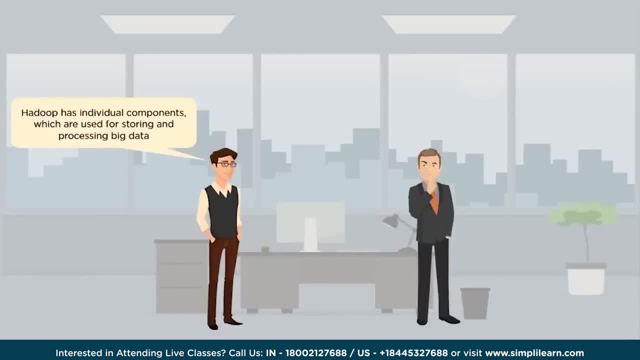 for volume, V for velocity, V for variety, V for veracity and other aspects like viscosity, validity, virality and many more. so when your data comes in with all these characteristics, it can be easily categorized as big data, and organizations in recent past have realized that they cannot ignore any data, considering it as an economical so they 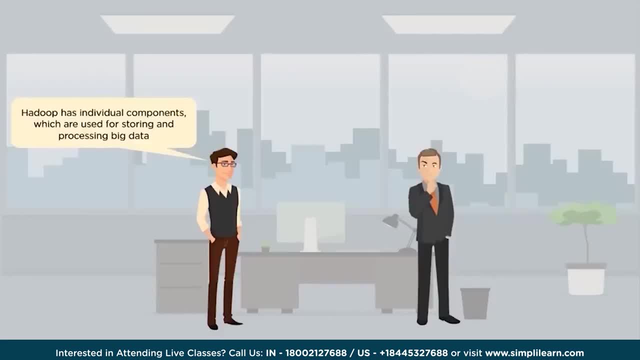 would want to work on all of it, and when I say all of it, that is one of the drawbacks in terms of our DBMS. so in our DBMS, usually you will never have 100% of data online. you would still have your data. it would be consistent, you could do. 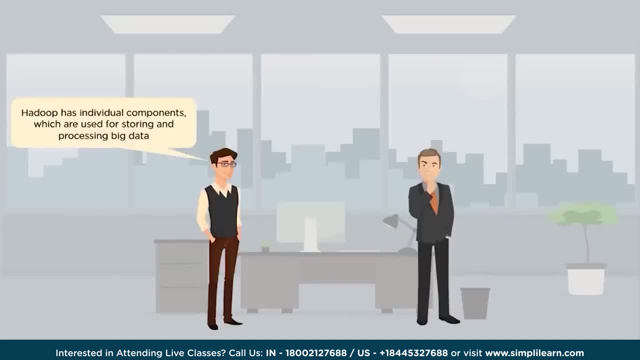 transactions, but you would not have access to all 100% of it, because that would be a costlier option. so in our DBMS you would have 10 or 20 or 30% of data which would be online and rest of the data would be archived, which basically 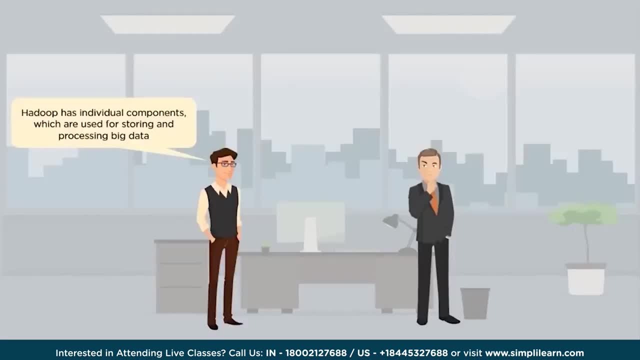 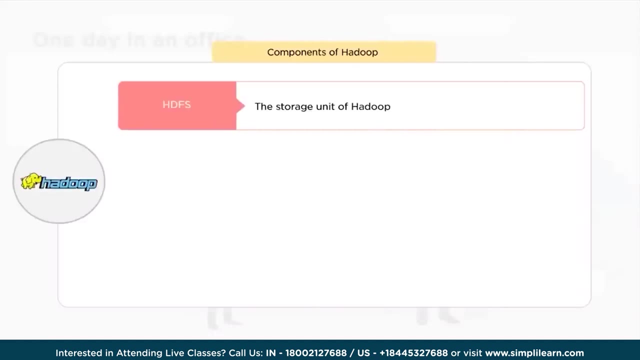 means that if you would want to process that data, you would have to bring it from the storage layer to the processing layer, process it and then store it back. now, how does Hadoop help in this approach or this requirement? so when we talk about components of Hadoop, we have a storage layer that is HDFS. now you can. 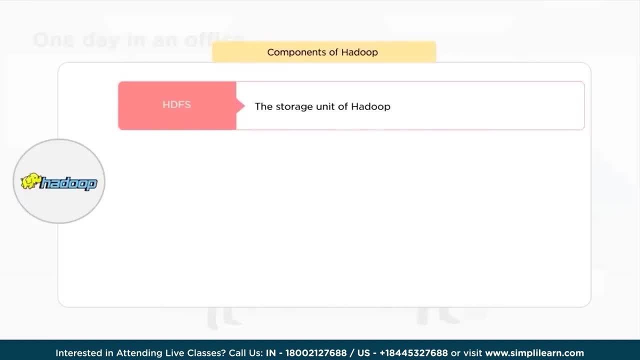 compare this with your own laptop or PC. every laptop or a PC has two layers. it has a storage layer, that is, your disk or your external hard disk, which is attached to your machine, and your machine also has the processing layer, which is your RAM and CPU cores. so HDFS is the storage layer of Hadoop, so it's a. 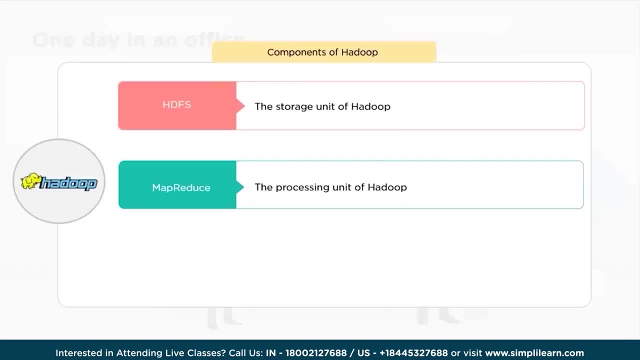 logical storage layer which, technically speaking, does not exist, but then, yes, it exists because it depends on the individual file system of multiple machines. we'll learn about this in a few minutes. the other layer of Hadoop is the storage layer, which is the storage layer which is: 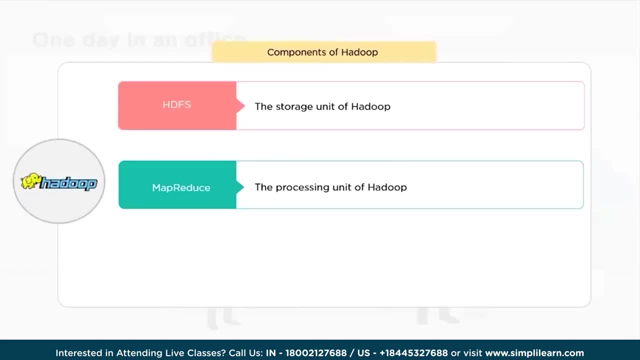 the processing layer. so when you talk about MapReduce, it is a programming model which allows you to process the data in one particular way. now, MapReduce has been oldest and the most mature. so when I say most mature, it has evolved over time. since the time Hadoop came into existence. MapReduce exists. it is. 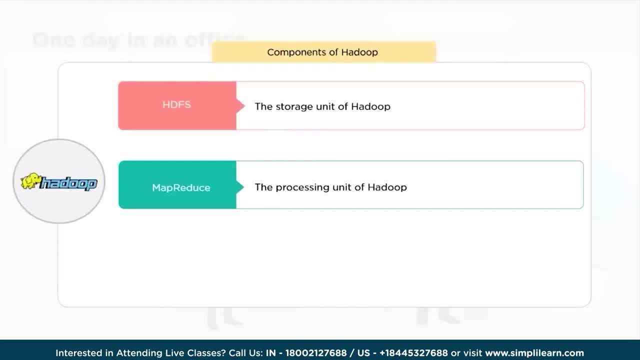 still being used by organizations for doing processing. and when we talk about processing here, we are not talking about processing on one single machine, but we are talking about processing on multiple number of machines where each machine's RAM and CPU cores contribute to the processing. so we have two main components. 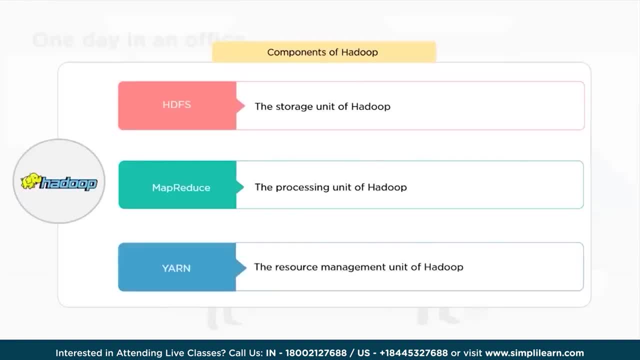 one is your HDFS, one is your MapReduce, and for your MapReduce, or basically any other processing framework, MapReduce is one of them. so for any other kind of processing, say massive parallel processing, say graph processing, say MapReduce processing, say structured query language being processing, for all of these processing, 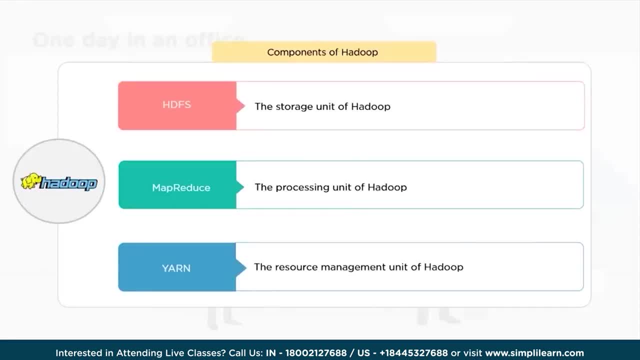 needs. there is a processing layer called YAN. now YAN stands for yet another resource negotiator, so basically, YAN takes care of your resource management. that is when the processing happens across the machines. who would take care of RAM and CPU core, which would be required for processing and that would 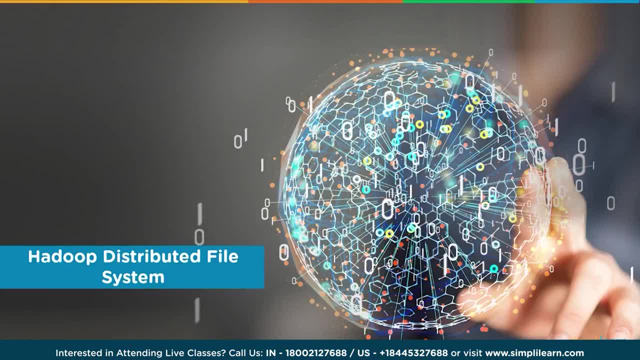 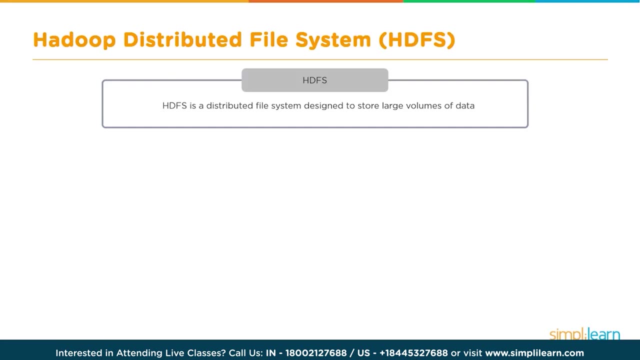 be your YAN for a Hadoop cluster. HDFS is fault tolerant, is reliable and is scalable. so let's understand and learn on the working of HDFS. that is the logical storage layer for a Hadoop cluster. HDFS is a distributed file system which is designed to store large volumes of data on commodity. 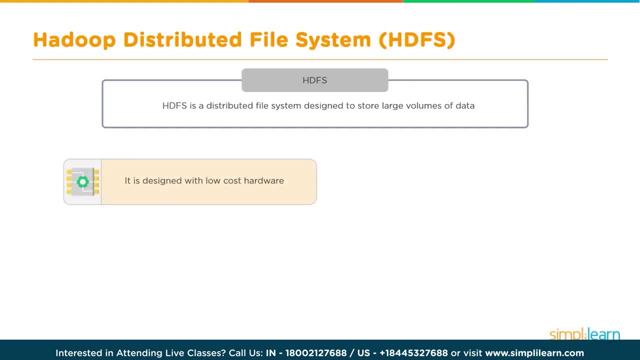 machines. it is designed with a low cost hardware- and that is what I mean when I say commodity machines, so we could have a cluster of tens and hundreds and thousands of nodes which can still scale and accommodate huge volume of data. it provides access to data across multiple Hadoop. 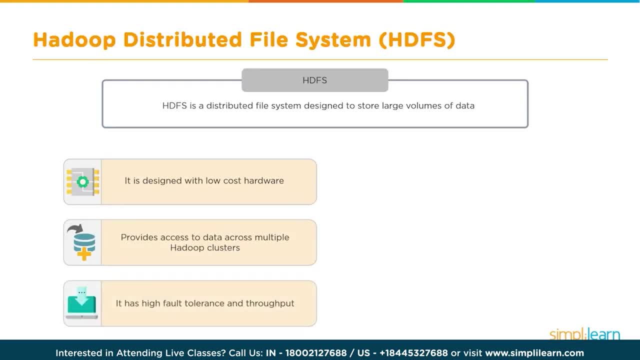 clusters, it has a high fault tolerance and throughput, and HDFS stores data in multiple servers instead of a central server. now, earlier, when we were discussing on how storing data on a single machine can lead to more read or processing times and basically lead to high seek time that can be taken care by 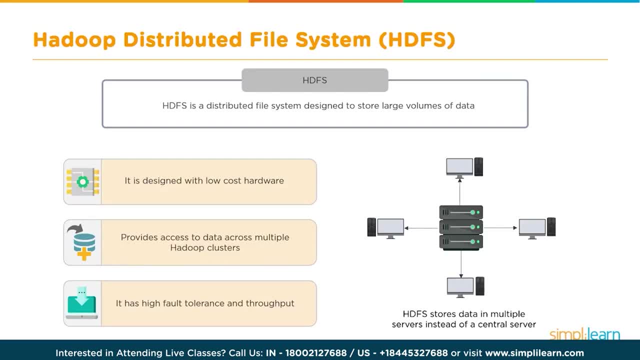 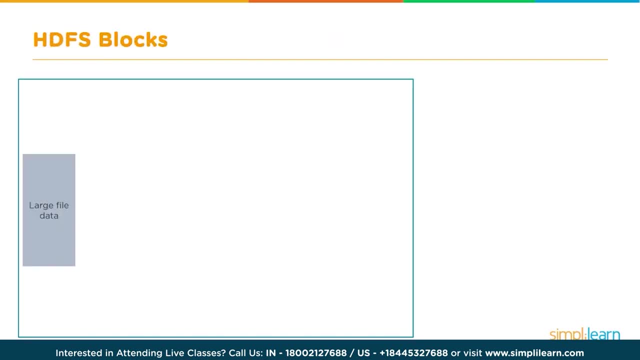 a distributed file system such as HDFS, which would rely on file systems of multiple machines which form a single machine and which can be stored in multiple servers. now let's understand how HDFS works. for example, we have a large file which is to be stored on HDFS. now that file would be broken down into blocks and 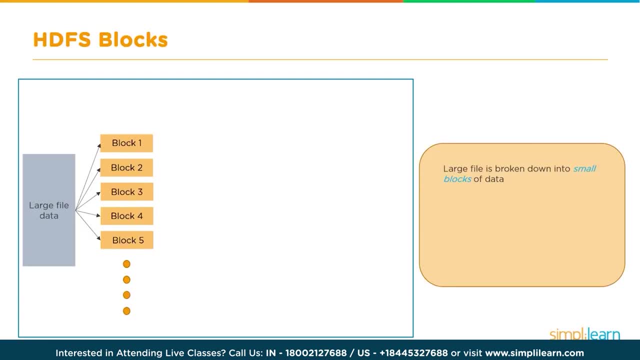 the block size by default is 128 MB. these blocks would then be stored across different slave machines or different nodes which are responsible for storing data, as the FS has a default block size of 128 MB, which can be increased as per requirement. now that could be in megabytes, gigabytes, terabytes or even 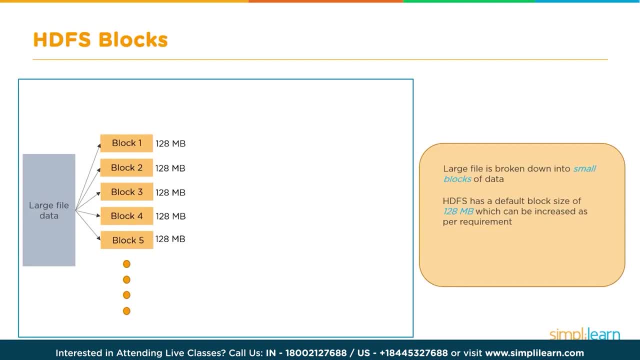 bigger than that. the default block size is 128 MB from Hadoop version 2 onwards, and your previous versions of Hadoop had the block size of 64 MB. here the point to be remembered is: block is a logical entity which basically takes the data and stores it on the underlying machines in their disks. now, this is how it would. 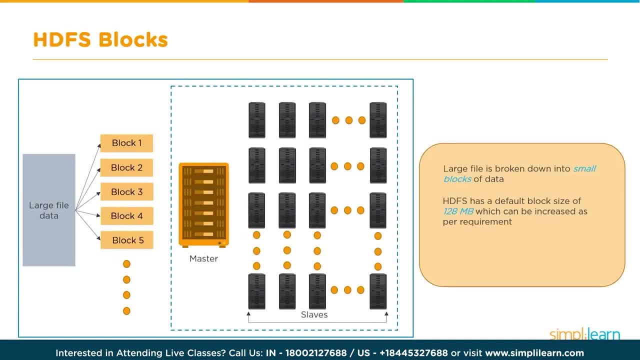 look, in a normal Hadoop cluster we would have one single master, unless it is a high availability cluster where we could have multiple masters, that is, two masters, one being active and one being standby. in a normal Hadoop cluster you would have one master and multiple slave nodes where these data blocks are. 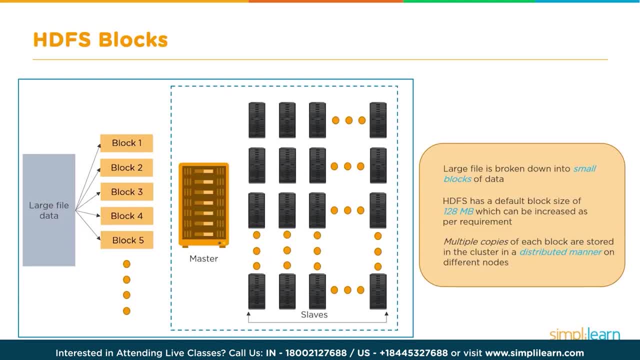 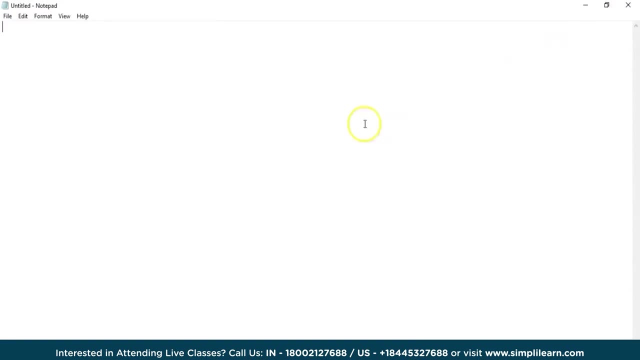 getting stored. now, before we understand the MapReduce algorithm, let's also understand the working of HDFS and how data gets stored overall. how does it work? so let me just open up a notepad file and I would explain about HDFS. now let's imagine that this is. I would like to have, say, five machines. 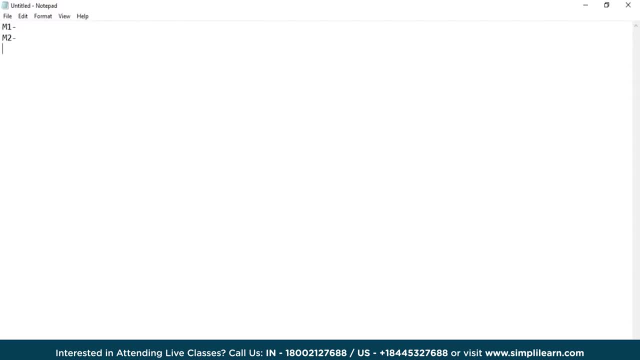 which could be forming my cluster. so I would have machine one, machine two, machine three, machine four and machine five. now if I say my Hadoop cluster is running on these machines which could be of a Apache Hadoop core distribution or having a vendor specific distribution, such as Cloudera or Hortonworks or MapR or IBM Big Insight, etc. so these are 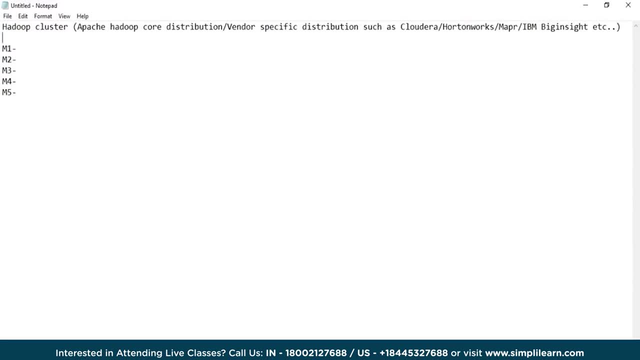 some vendor specific distributions of a Hadoop cluster. now here we can discuss later on how or what processes would be running on these machines now in case of Apache Hadoop cluster. in case of a Apache Hadoop cluster, to have a Hadoop cluster running we would have to download the Hadoop related Hadoop cluster. 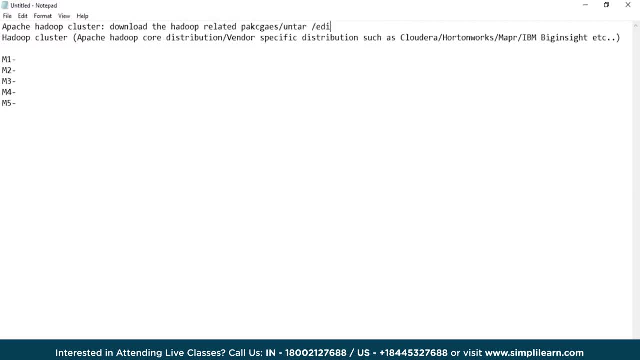 packages we would have to untar, then we would have to edit config files to specify which processes would run on which nodes and then basically we would be formatting HDFS and then onwards we can go ahead and start our cluster. so it looks like in Apache Hadoop cluster we would have to manually do various things. 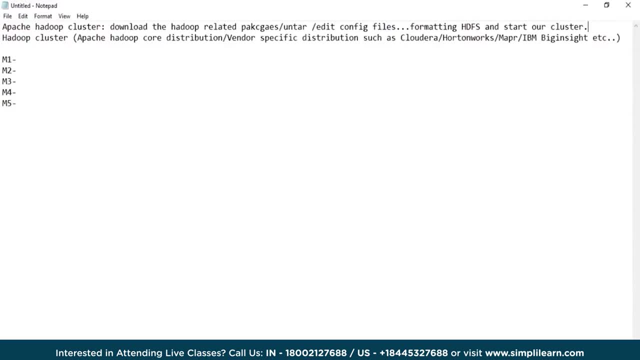 such as downloading the Hadoop related tar file, untarring it, editing the config files, formatting HDFS and then going ahead and starting your cluster. in case of a vendor specific distribution, such as Cloudera or Hortonworks, let me split it here so you would have. 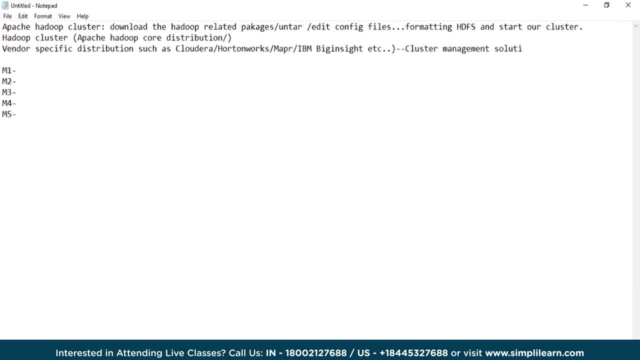 basically a cluster management solution that would help you in doing various things to set up your cluster. in case of a Cloudera distribution of Hadoop, you would have a Cloudera installer file and then you would have a Cloudera manager which will help in deploying a. 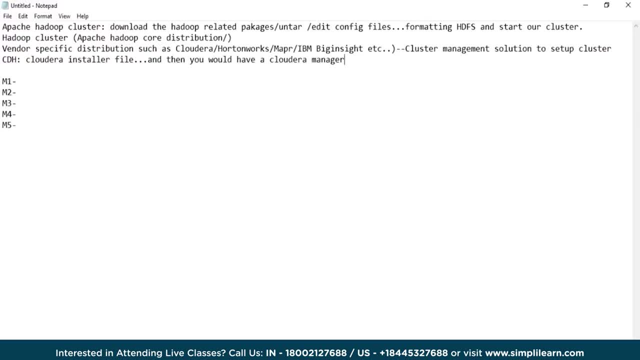 cloud error cluster. so downloading Hadoop related parcels or packages, untiring them, editing config files, formatting as DFS and basically starting your cluster would be taken care automatically by cloud error manager. in case of Hortonworks data platform, it would be Ambari software that would be. 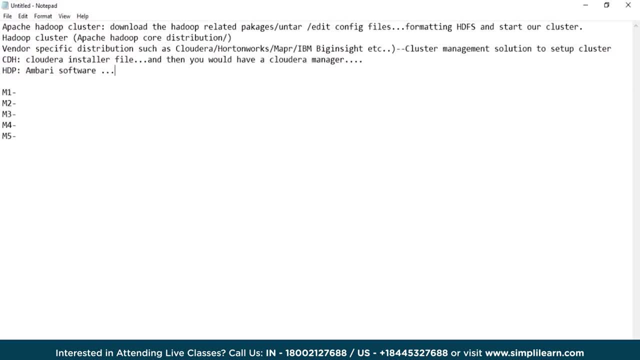 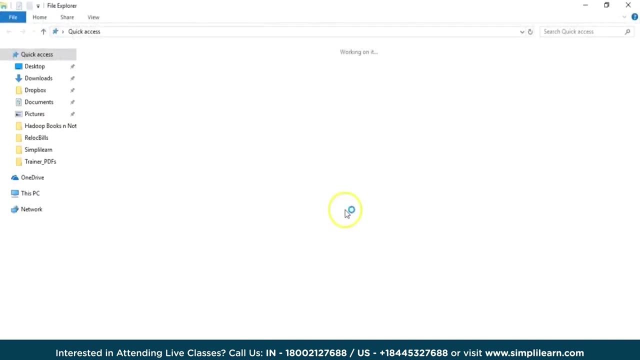 used for deploying your cluster. now, no matter which distribution of Hadoop you would be running, you would still have the same roles or processes which would be running. let me just briefly discuss here about the terminologies. so let me bring up a file here which could explain these details. so let's look at this now. 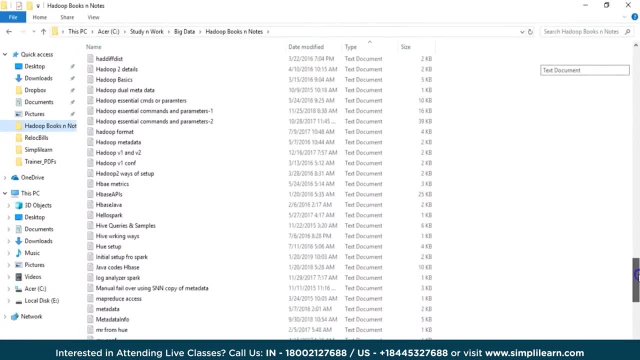 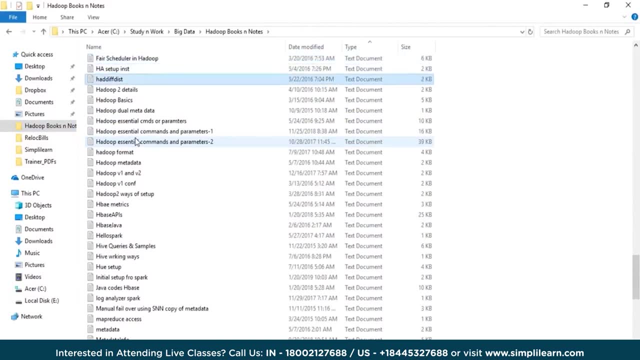 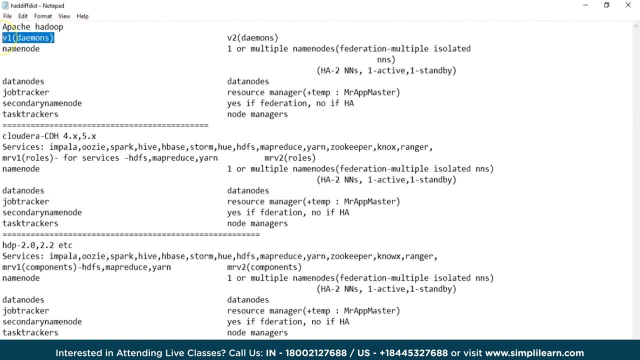 here I have documented how it would look in different distributions of Hadoop. so we have Hadoop version 1 and 2 and let me just look for files. yeah, so this is the one. now, if you would look in version 1, Apache Hadoop. we would call demons, or 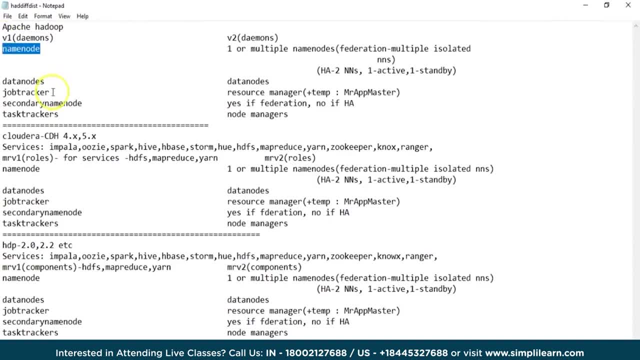 processes. and if you look at the names, we have the name node, we have data nodes, we have job tracker, we have secondary name node and we have cast records. in case of version 2, you would still call them demons. you could have one or multiple name notes if it was a Federation or a. 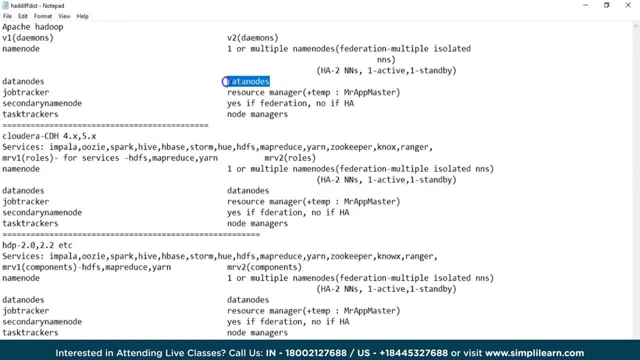 high-availability kind of setup. you would have data nodes instead of job tracker, you would have resource manager and then there is a temporary Devin called mr-app master. if you had a high availability, name node would not be allowed, and if there was a Federation kind of setup, 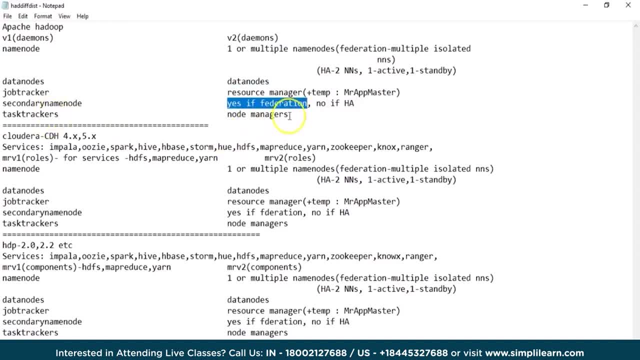 secondary name node would still be existing. instead of task trackers, you would have node managers. now, in case of vendor specific distributions such as cloud era, whether you are talking about older version or newer version, which is five point something, you would have what we call as roles. so in Apache Hadoop, we 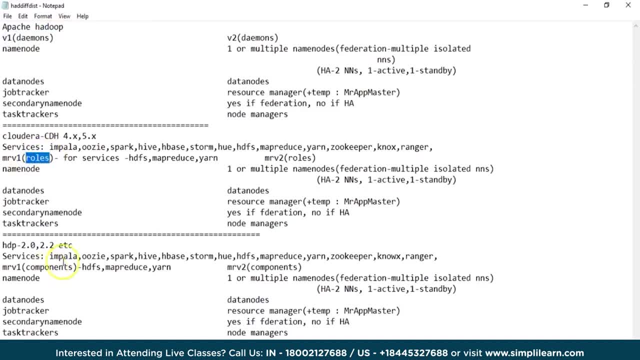 call them demons in cloud enough. we call them roles. in Hortonworks we call them components, but we are talking about the same thing. in case of cloud era, you would have services which would be part of the cluster, such as impala, uzi, spark, hive, edgebase, storm, hue, HDFS, map, reduce, yarn and so on. similarly in Hortonworks. 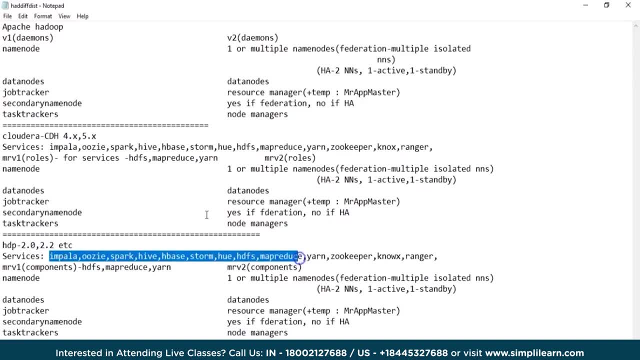 also, you would have these services which would be running. in case of Apache Hadoop, we would not have so called services seen, but then the functionality still exist. and how is that? that is depending on these demons. so, basically, if you look in Apache, Hadoop or cloud era, 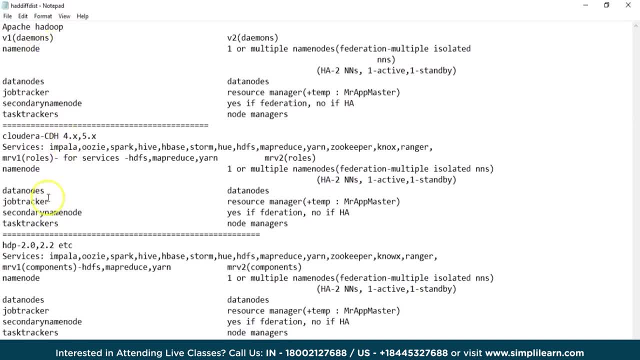 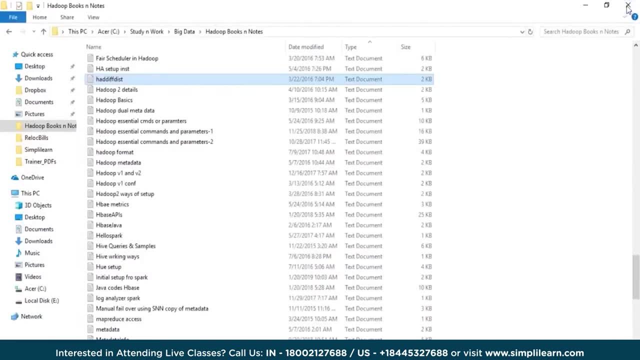 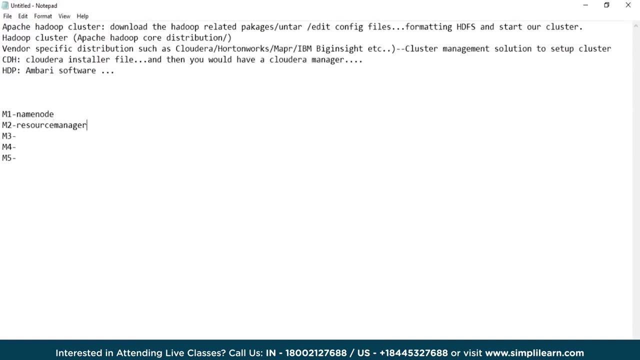 there are Hortonworks everywhere. we have these daemons and we have these would be running on one or multiple nodes, so we could have different kind of setups and just to briefly discuss on that, so we could have a name node running here, a resource manager running here and you could. 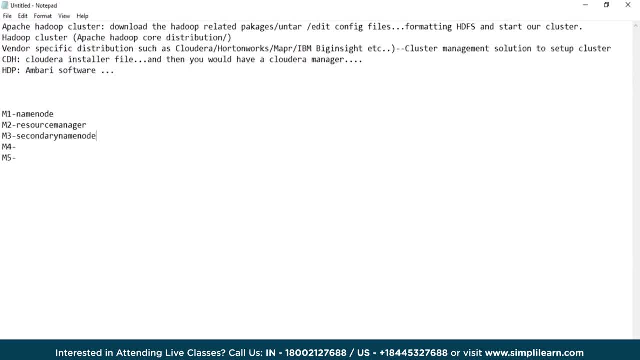 have a secondary name node- now don't go by name, it's not a second name node, we'll discuss about that later- a secondary name node, and then we could have data nodes running in machines. so this is one kind of setup where I'm talking about data node node manager and here we have a data. 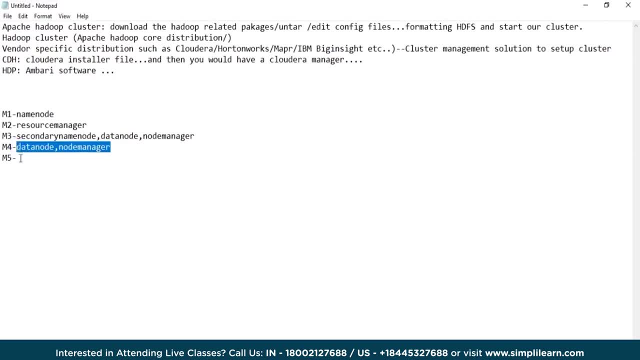 node, node manager and similarly we would have that on one more machine. now this is one kind of setup. this is not the only setup possible. you could have a different setup where, on the same machines, you could decide to have data node and node manager running on every. 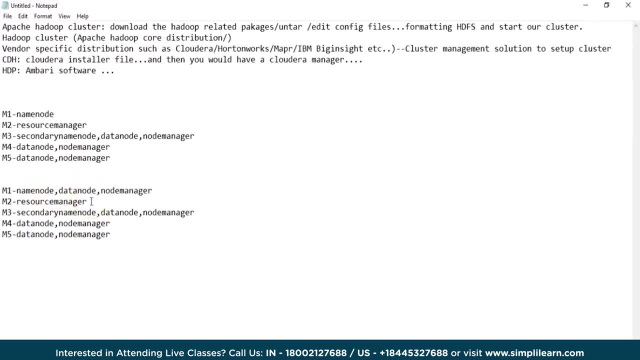 node. however, that would not be preferred because you wouldn't want the slaves and the masters to run on the same machine. however, this setup is also possible. you could have a high availability kind of setup which basically is good for cluster and for an organization where you could have 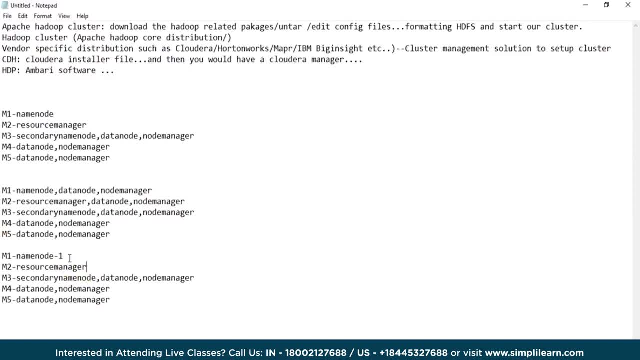 name node one which would be running here and say we can have a name node two running here, we could have a resource manager two running here and then we could have a resource manager one running here and I could still have my data node and node manager running in the same fashion. now, this would not be allowed in a high availability cluster because we 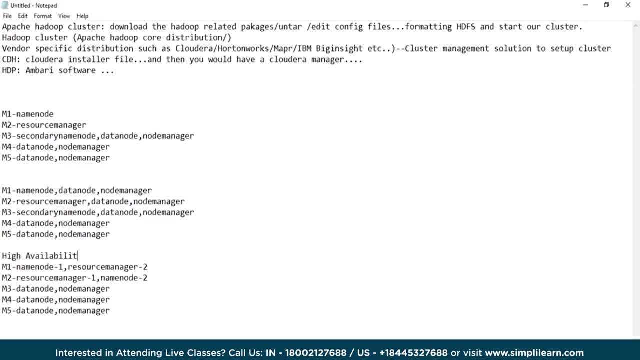 have a standby name node. so this is one more setup which is possible and then you could have a single node setup which could be everything having on the same machine, that is, name node, resource manager, secondary name node, data node and node manager. so these are different setups and if you're going to 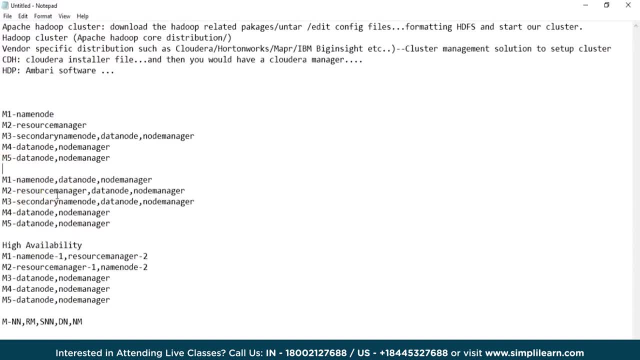 have somebody asks which is a preferable setup, then I would still go for either this one, which has multiple data nodes and node managers, not this one, or your high availability setup. now, a single node or a pseudo distributed cluster is basically good for testing or some development, kind of. 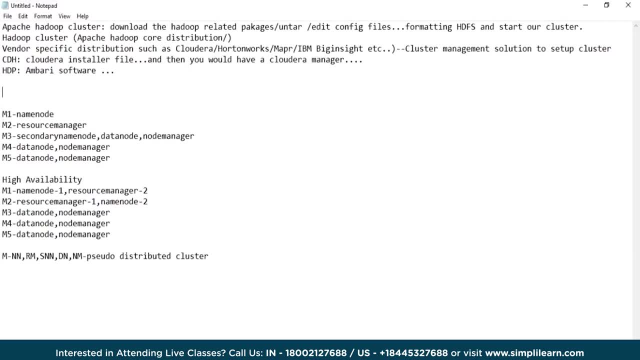 activities and these are your distributed clusters. now, if we closely see, we basically have the roles or components or elements running on these machines to take care of mainly two functionalities or two services: that is your HDFS, which is your storage layer, and yarn, which is your processing layer. so in a Hadoop, 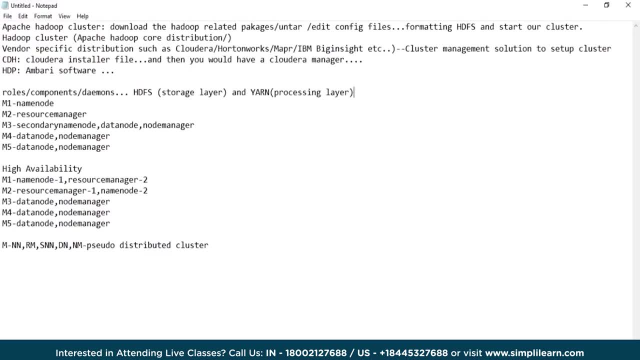 cluster. we have a storage layer and we have a processing layer for storage layer, that is SDFS. you basically have one single master and you have multiple slave processes running. so I could say: for HDFS to work, fine, I should have a name node running, multiple data nodes running and then a. 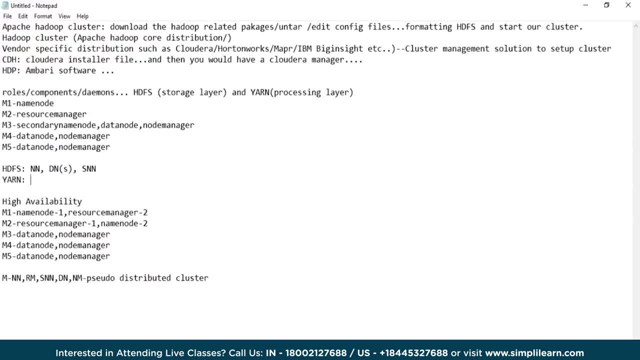 secondary name node running for yarn as a service. that is my processing layer. I would need minimum one resource manager and multiple node managers running on one or multiple machines. so these are the two processing. these are the two layers, one being the storage layer and one being the 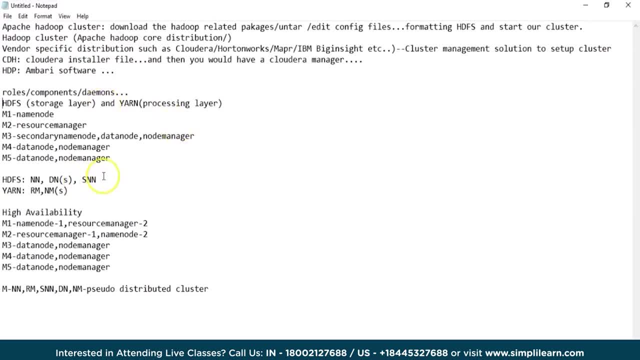 processing layer and for your storage layer. you have these processes running on one or multiple storage layer. you have these processes wherein your name node is the master and your data nodes and secondary name node can be considered as the slaves. you have your resource manager as the master for your processing layer and node managers. 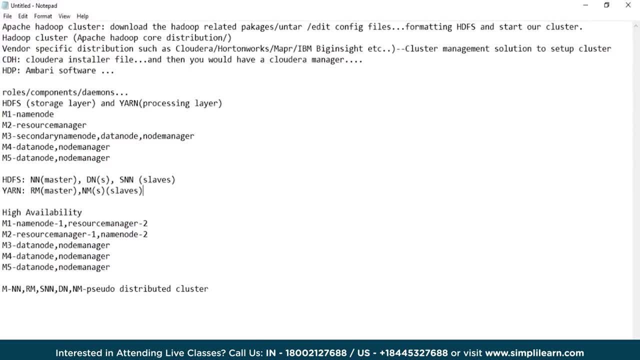 are the slaves. now, this is briefly about the set up which could be in a particular environment. now, say the Hadoop related packages or parcels have been downloaded, whether it is a vendor, specific distribution or Apache Hadoop cluster. say: untiring of that is done. editing of config. 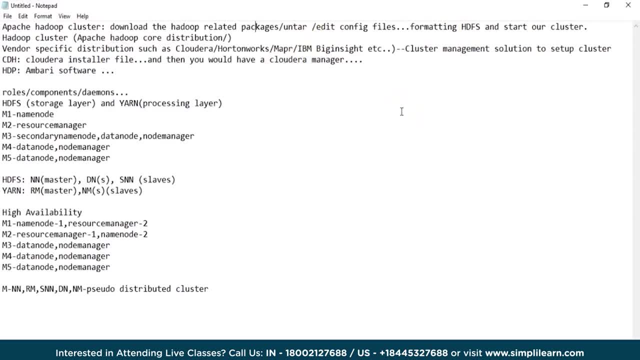 files is done, formatting is done and your cluster is started. In that case, your cluster would be up and running and then we could basically have- and once your cluster is up, we would have the SDFS up and running, ready to allow to store data. Now let's imagine that this 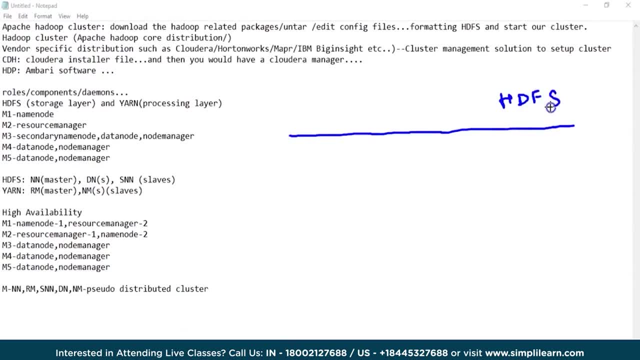 is my SDFS which is up and running, or SDFS as a service is up and running. Let's imagine that these are my nodes, which is M1, M2, M3, M4, and M5.. Now, while the config files were edited, 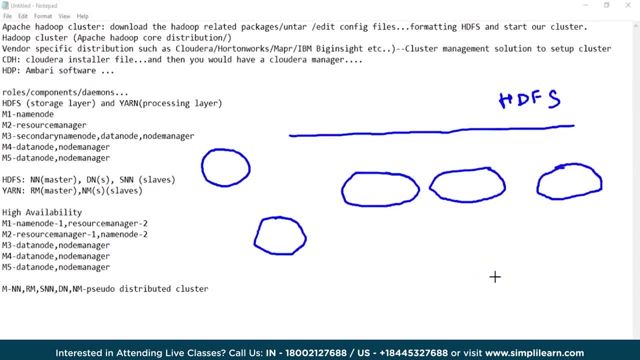 for each of these nodes, it would have been defined which processes will run and we would have also given path where these processes will store the data. So let's say that this is my M1, this is M2, M3, M4, and M5.. M3, M4, and M5 have data nodes running, So we would 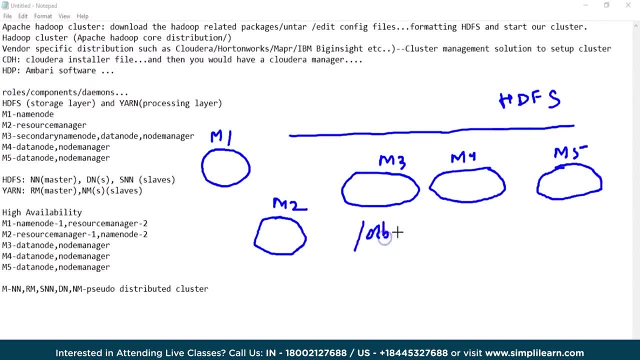 have defined a path. let's call it, say, ABC slash data, ABC slash again data, or D and ABC. So this is the path which has been defined on every node to store Hadoop related data, and on one where we would have name node running, we would have still defined a path. let's call it abc slash. 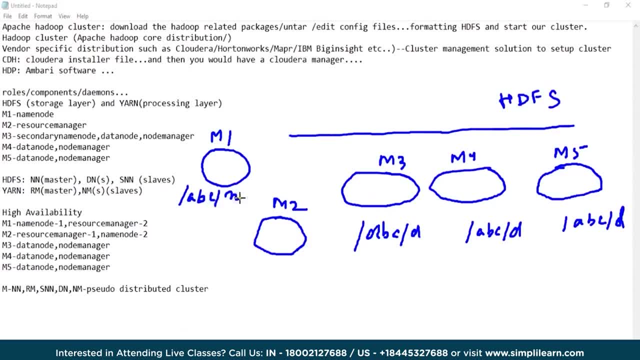 n, where name node could store its data. so once your cluster is up and running and your sdfs is available, we can have our data stored on sdfs. now let's understand how does that work. so any client or an application which would want to write data to the cluster needs to interact with the master. 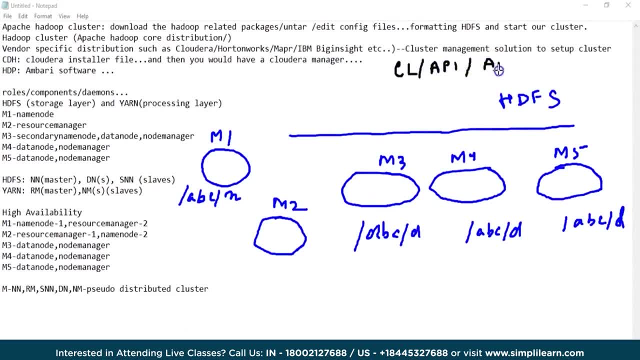 to begin with say, let's say, client machine or an api or an application would be interested in writing the data. now how would name node know about available data nodes? so as soon as the cluster comes up, the first thing which happens is these data nodes would be sending in their 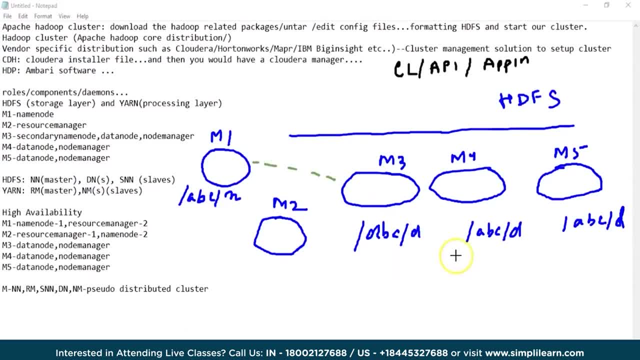 heartbeat to the name node every three seconds. so data nodes send the heartbeat to name node every three seconds to let the name node know, to let the master know that they are available. what does name node do with this? name node is building a metadata in its ram. 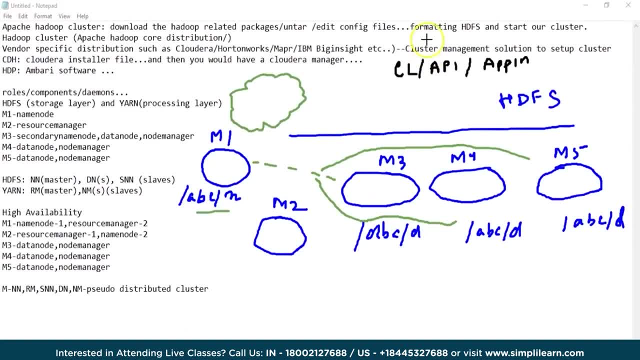 so it already has some metadata in the disk which was created as a result of formatting sdfs, and now we would have metadata in ram which is getting built. so initially name node would have information of which data nodes are available in the cluster. now, if a client or an application 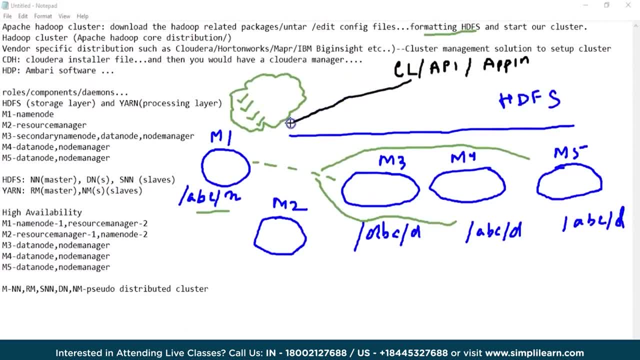 wants to write data to the cluster, it gets in touch with the name node inquiring the slave machines or inquiring about the data nodes where the data can actually be written. Your name node refers to the metadata collected so far and responds back mentioning the data nodes or the slave machines which are 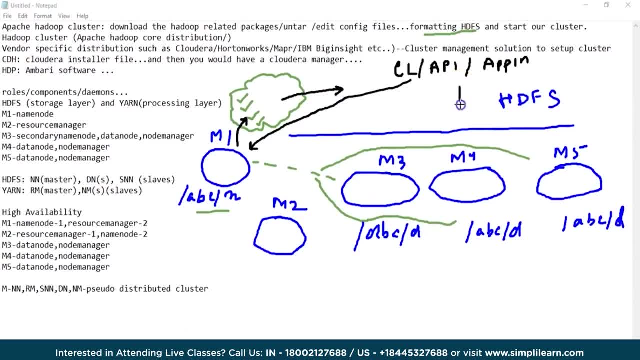 available for data storage. Based on this response, your client takes the file to HDFS, intending to write it to the cluster. Now in Hadoop, we basically have two things. One is the default block size, which we discussed earlier, is 128 MB. So you have 128 MB as the default block size, which is customizable, and that can. 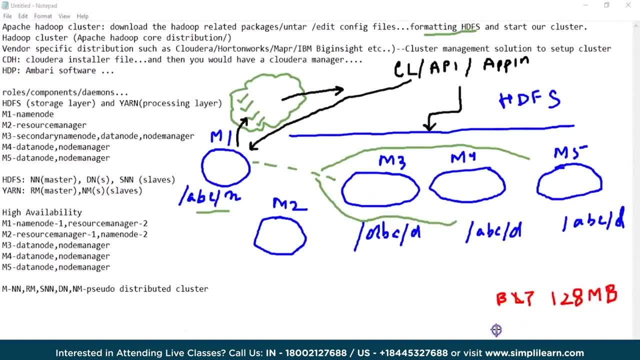 be changed depending on the average data size and you have the default replication, which is 3.. Now imagine the application or API or client would want to write a file which is 256 MB, which is bigger than the block size, and this file has to be broken down into what we call as blocks, which are logical entities. 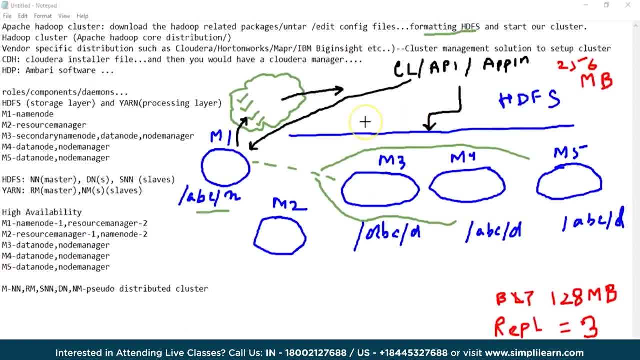 So the file is taken to. the framework Framework will split the file into blocks. So let's imagine that this file is 256 MB. It will be broken down into two blocks- B1 and B2, and these blocks will then be randomly distributed to the slave machines, that is, the data nodes. So we would have block 1,. 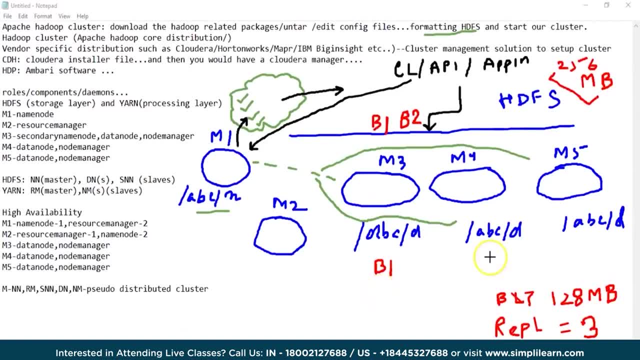 say getting stored here. Now you could also have block 1 getting stored on any of these data nodes, So we would have block 1, and then we could have block 2, which could be written here, and then you would also have their replicas sitting on the machine. So the rule of replication is: 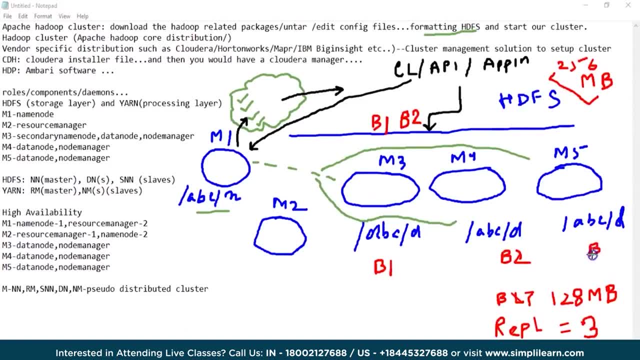 you will never have two identical blocks sitting on the same node. So if I have block 1 here, then I will never have a replica of block 1 again on the same machine. So we will have a replica of block 1 sitting on the same machine. So we will have a replica of block 1 sitting on. 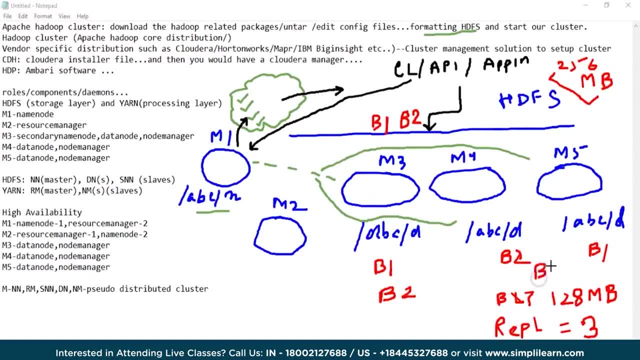 the same machine. So we will have a replica of block 1 sitting on the same machine. So we will have a replica of block 2 here, block 1 here and you have a replica of block 2 here. There is no differentiation. 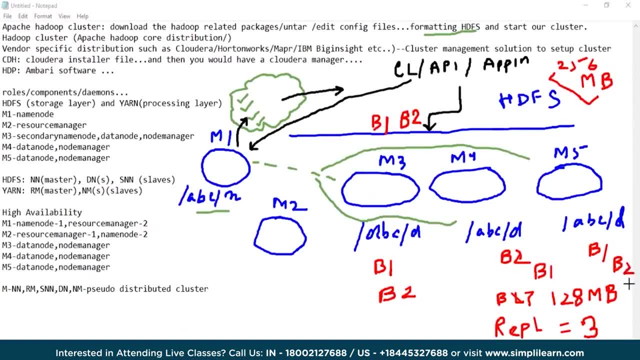 between which one is the original and which one is the replica. For the cluster, all the blocks are same, And what also happens is, after the blocks are written, your data nodes are repeatedly sending their block report to name node every 10 seconds And this information is again updated in the name. 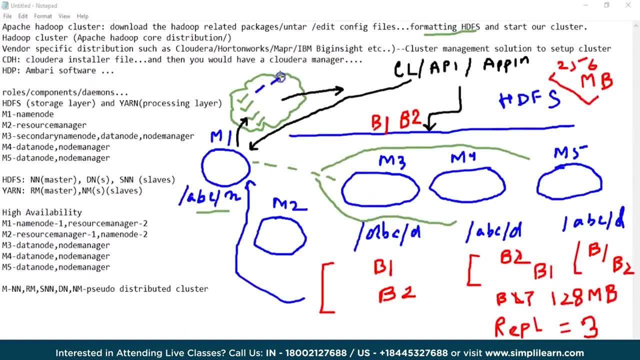 replica of block 2 here and you have a replica of block 2 here. So now we have a replica of block 2 here. So now name node will have information. what are the files? the files are broken down into what? 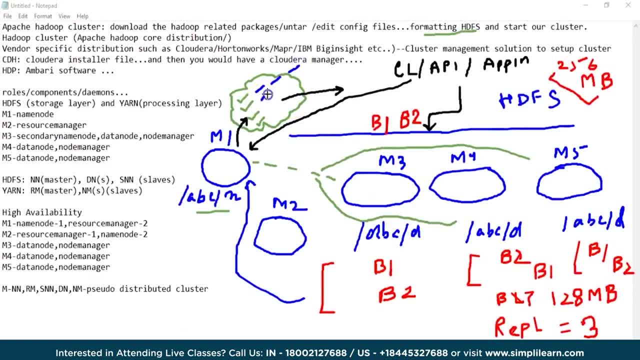 blocks. the blocks are residing on which data nodes, And this metadata is getting built in the name node, as data nodes respond with their heartbeats and also every 10 seconds with their block report. Now we need to remember one point here: That name node is basically a master and 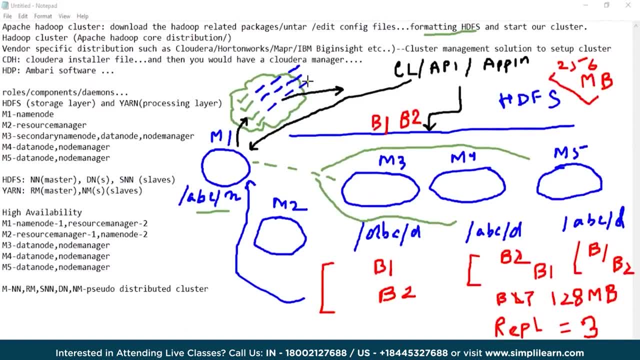 data nodes are the slave. Hadoop, as a framework, has been coded in Java, which basically means that every directory, every file and file related block is considered as an object which is getting stored and for every object which name node is tracking, 150 bytes of. 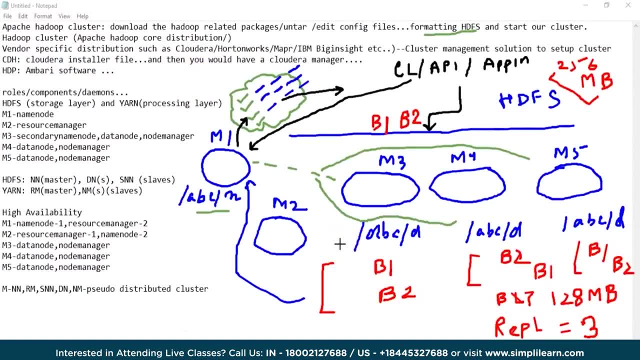 name nodes RAM is utilized, which also tells us that if the block sizes were smaller than 128 MB, then for the same file we would have more number of blocks, which would mean that name nodes RAM would be overutilized and overload name node. so block size has to be chosen with a lot of consideration on the 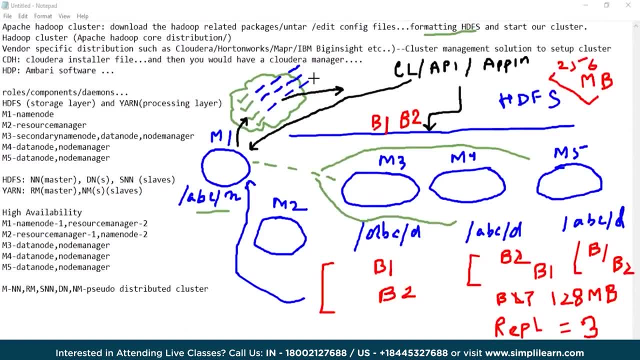 master's RAM and what is the average size of the data. now, this is how the data is distributed: in blocks and distributed across the data nodes. thus, SDFS is very fault tolerant, because if any of the data nodes fail, then you still have other data nodes which have the replica of data, thus making it. 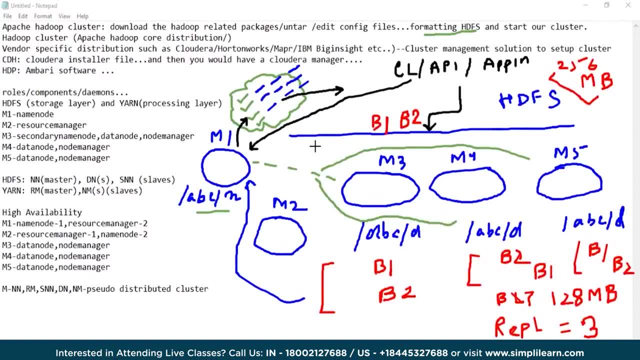 possible to read the data and access the data, even if multiple data nodes go down. now there are other internals. that is how data nodes are placed in racks or what has rack awareness to do in block placement. but we will learn on all that later. so this is how your SDFS works. now there are 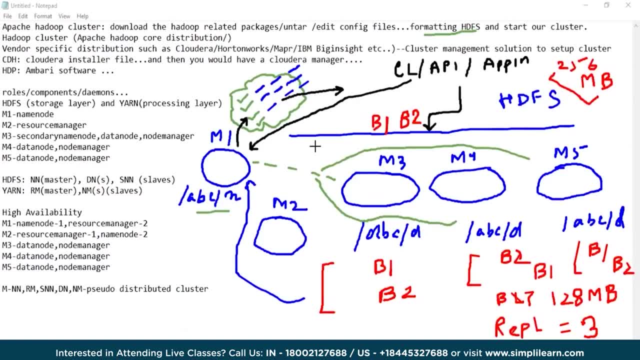 many other things, such as the read and write process, which is taken care by your methods, such as open and create, which internally are playing a role when a read or write operation happens. also, facts like replication is a sequential process, but write activity is parallel. so we can learn more functionality of SDFS in later sessions, but this is in 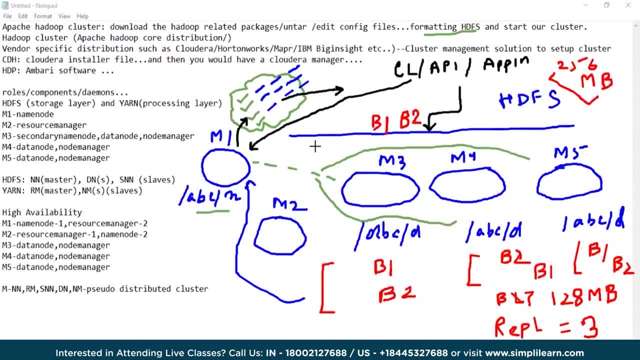 brief on how SDFS works, how your file is split into blocks and the blocks are getting stored on the disks. note that the block contains the data. so even if you have a file which is one kilobyte and if this file is to be stored on, 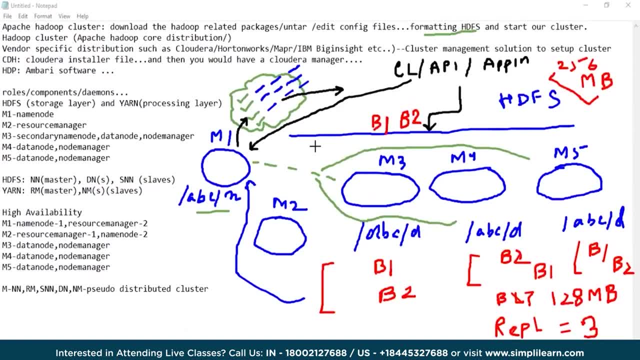 SDFS, it will still you a block of 128 MB, which does not mean that there is a disk space getting wasted. when the block resides on the data nodes disk, it will only occupy 1 kilobyte of space for the data it has, which means that block is a logical 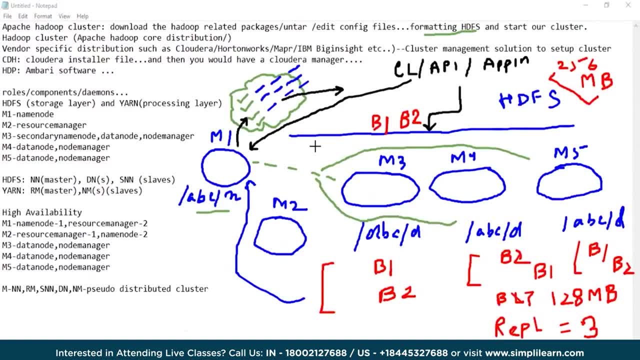 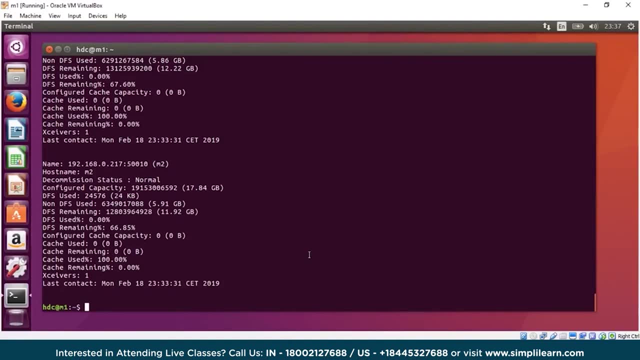 entity to take your data to the disk and get it stored on the disk. this is how your SDFS works and basically takes care of reliable data storage across machines in distributed fashion. now that we have set up a two node cluster, which has two data nodes, two node managers, one master machine, let's try working with SDFS. 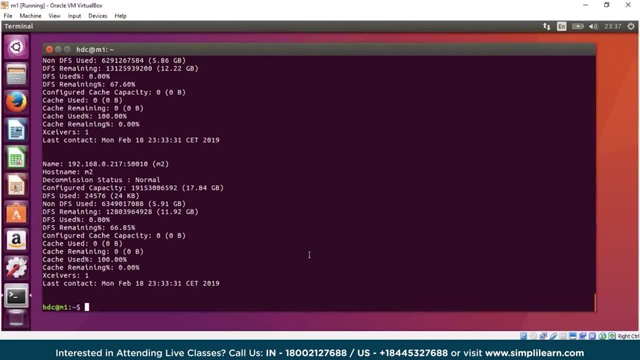 let's look at quick commands which allow you to write data to the cluster, although there are different ways. the first way is using commands, the second is using an IDE and where you could write your code to use Hadoop's file system API, and the third is 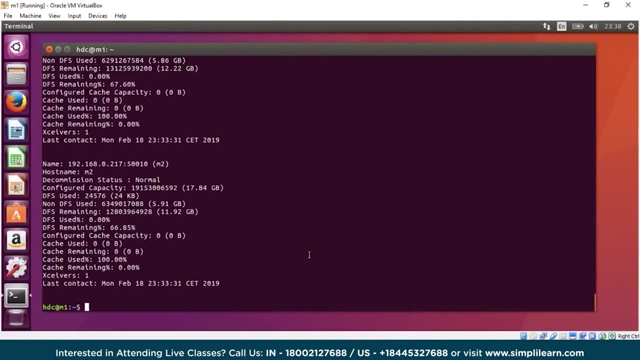 a graphical user interface called hue, which normally does not come with Apache, although it can work with Apache. it comes as a service with Cloudera and other distributions to work with HDFS. we need some sample data now. there are various websites from where you can get some sample data so you can open up your 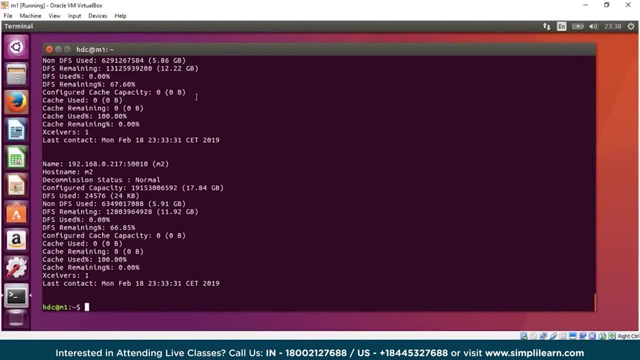 browser and let me show you some sample places or sample data set links from where you can download bigger or smaller files, which then can be used to write data to your cluster, your HDFS, although you could just pick up a local file or you could create your. 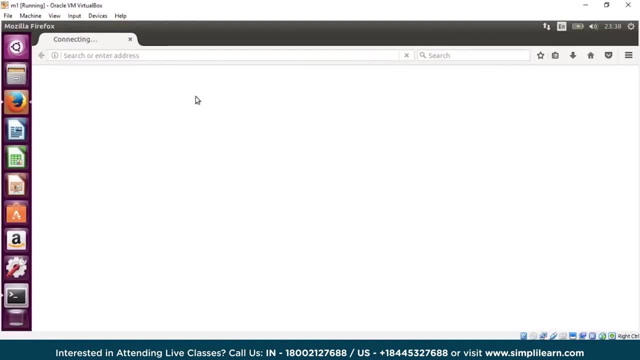 own files and write them to HDFS. there are various data set sites which can be used, so, for example, you can type in machine learning UCI data sets, and this is one link which has more than 200 data sets which can be used for even data. 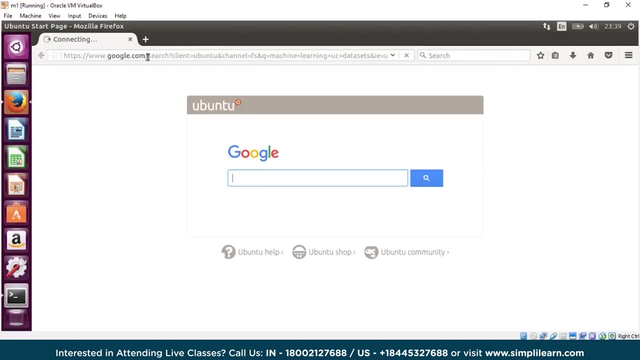 science kind of activities which can be used for testing with your algorithms, and you can download data sets from there, download data from here onto your local machine and then from your local machine we will be writing the data to HDFS, which then, based on the size of the data, 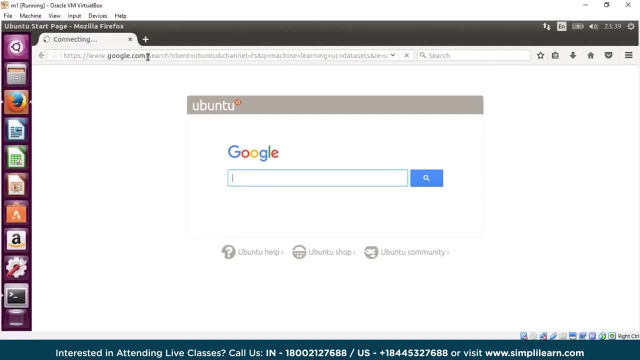 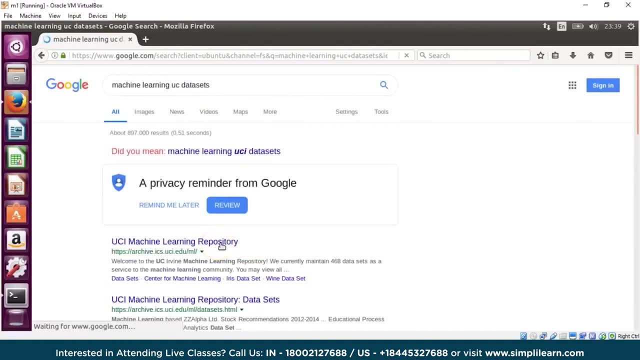 splits the data into blocks, and your blocks would get stored on your underlying machines wherever data nodes run. so I can click on this UCI machine learning repository or even just on data sets. to be very specific, all we need is some sample data sets. you can get Kegel data sets, for example, for performance. 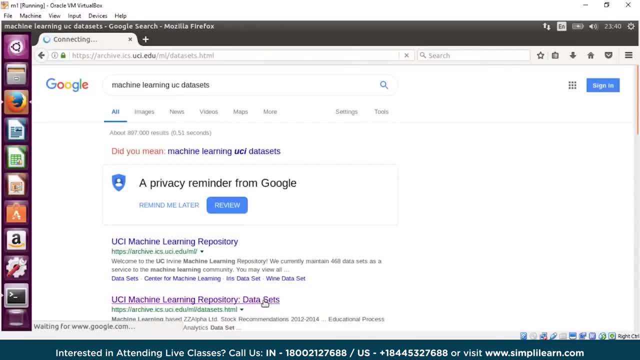 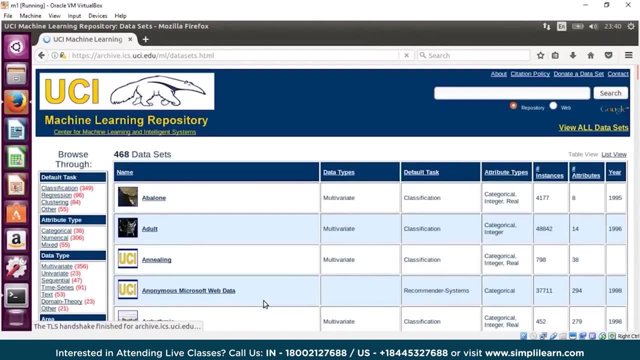 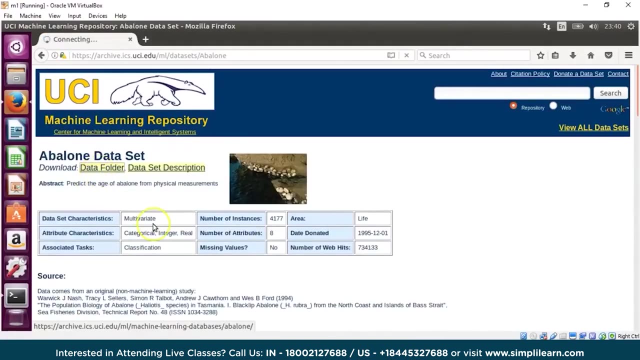 sets. you can get data sets from Yelp website which are bigger data sets zipped and you can be using them to write data to see how your files split into multiple blocks. now, here we have a lot of data. we can click on any one link to begin with, and here I have, the data folder shows me the some file and I can. 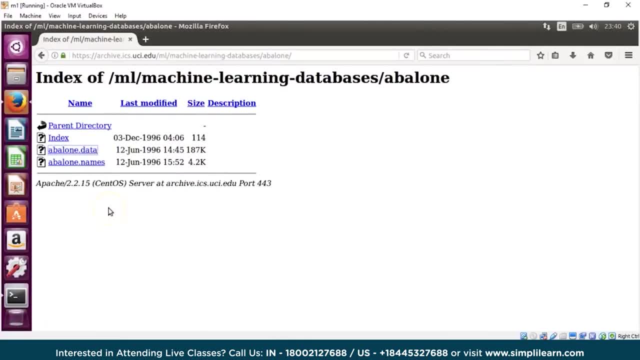 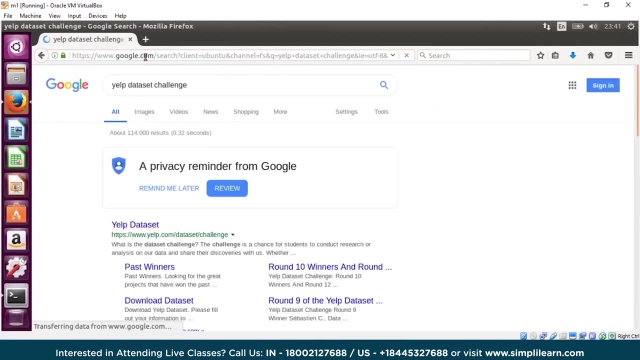 just right click on this save link as and save the file. this is a simple text file and we can save it and you can get various data sets from here. you can even go to Yelp data set challenge and that has bigger files which are zipped and 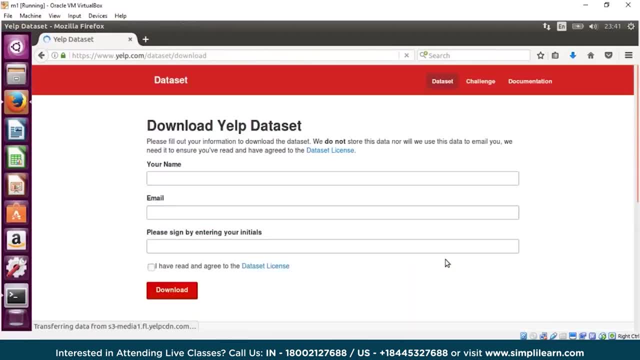 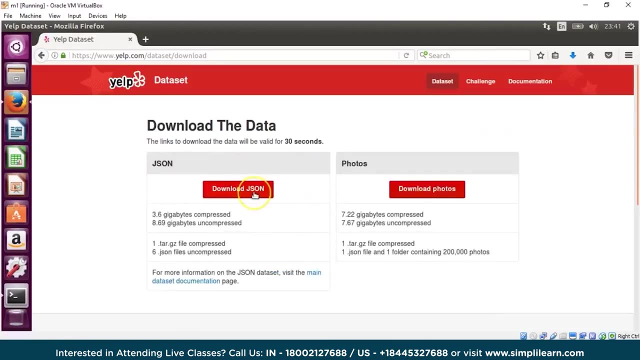 they can be downloaded. so you can click on download data set. although I will not start the downloading here, you can just give in your name here, just some email ID, some initials, and you can click on download. so this is one more website where you can download the JSON data. 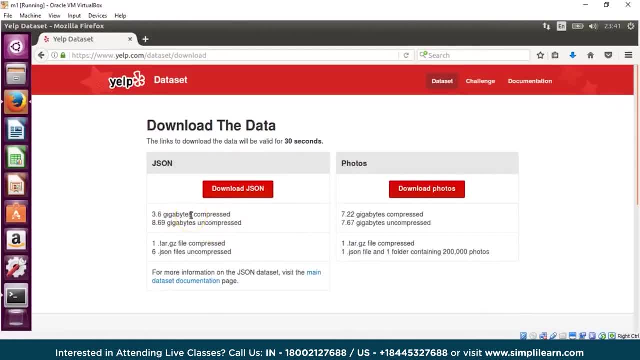 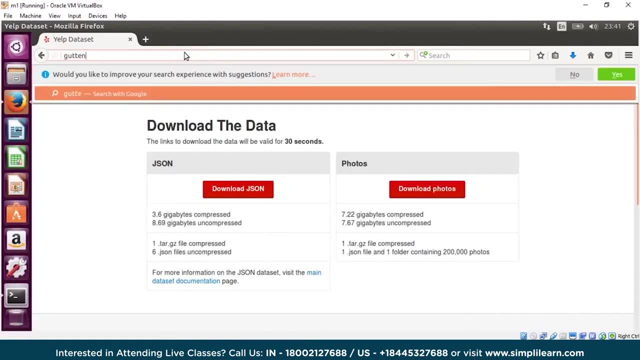 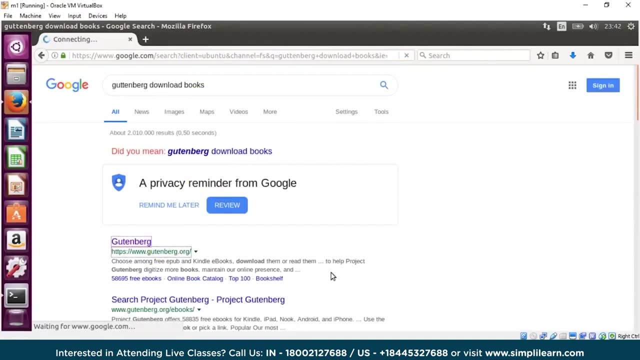 sets which are 3.6 gigabytes in compressed format, and then you have photos which are in 7.2 gigabytes. you can also say Gutenberg download books, and that is again a website from where you can download free data sets which are not very huge. so try to get some variety of data sets in different. 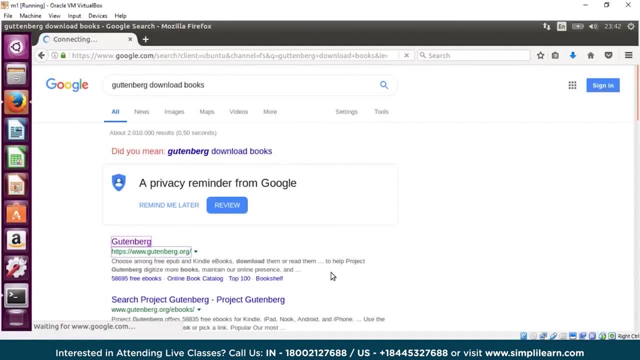 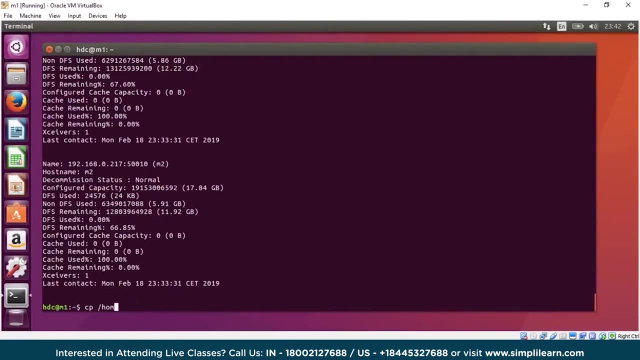 formats, which then you can write to HDFS. you can even use your HDFS log files, which already exist on your machine, and you don't need to download anything from internet now. let's close this for now. so I already have some file. let's copy this from home. HTC downloads that. 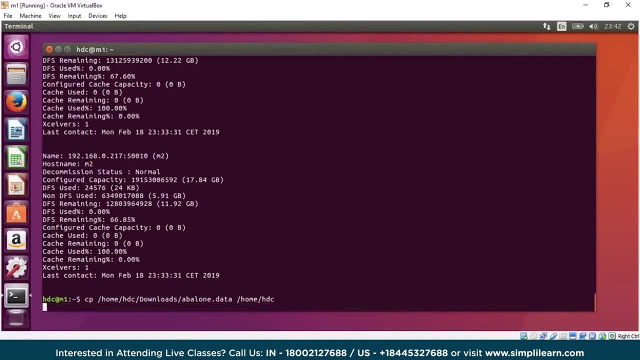 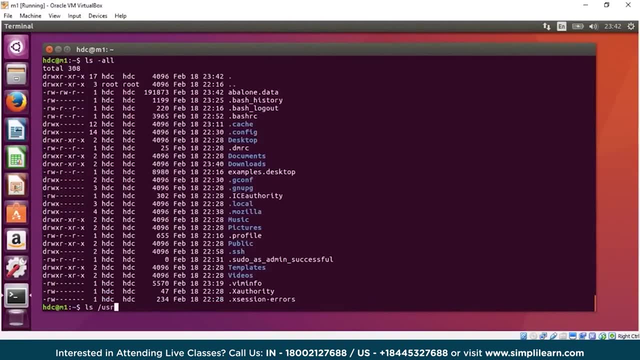 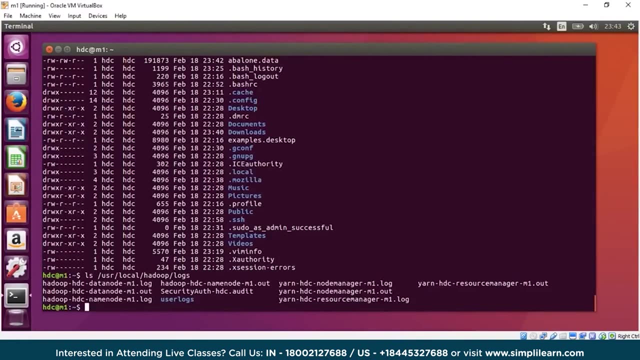 was my file. let's copy it to home. HTC, and here's my file. I can check the permissions so that's owned by HTC. I can even look into user local Hadoop logs and there are some already log files so you can even copy some of these files using. copy user local Hadoop logs and. 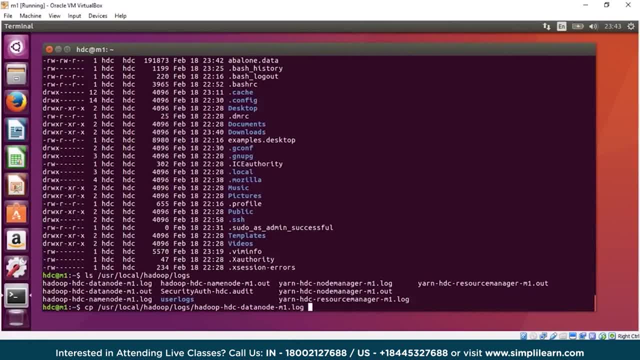 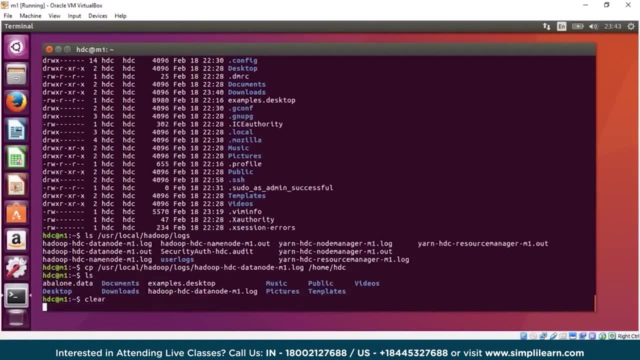 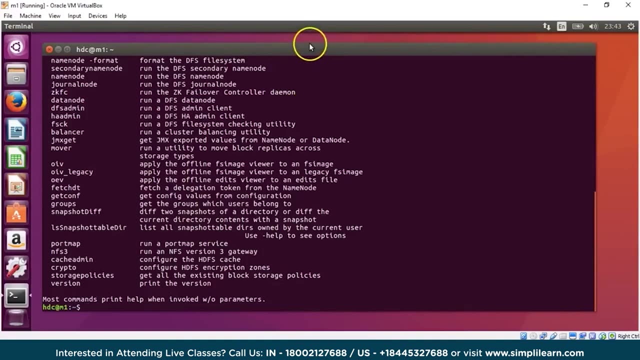 let's take Hadoop data node related log and let's copy to home STC for our testing. and now we have some other files now to work with HDFS. as I said, you can always type in HDFS and that shows you various option. now we already used the 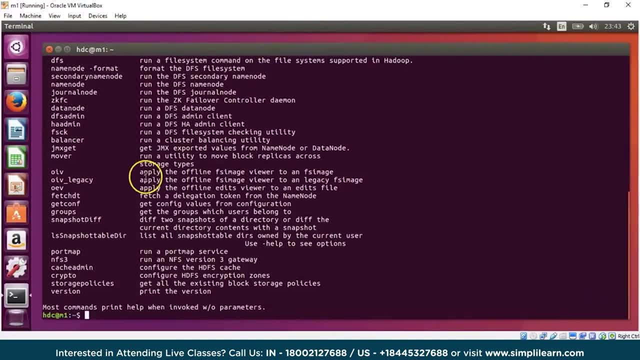 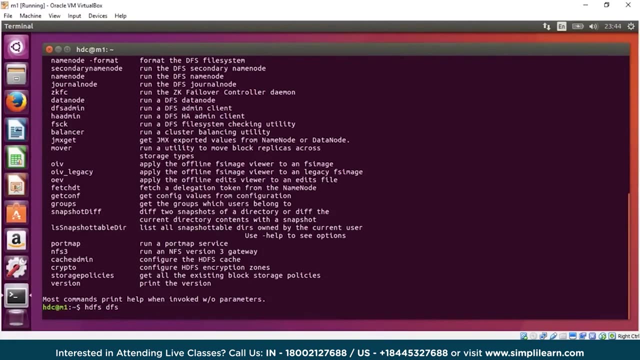 first option, which is name, node hyphen format. we also used HD DFS admin to look at how many nodes we have and to work with your HDFS file system. the option is DFS, so you would say HDFS, DFS and then you can always hit on enter. it shows you various options to work with your. 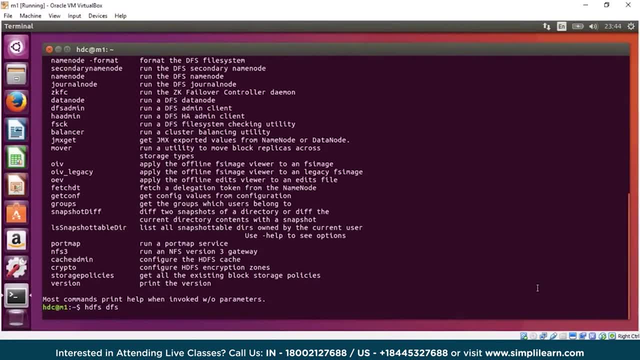 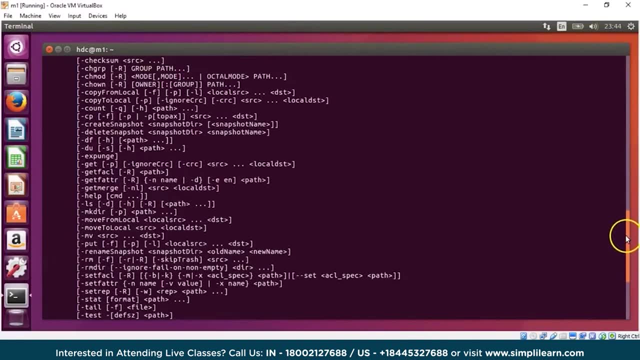 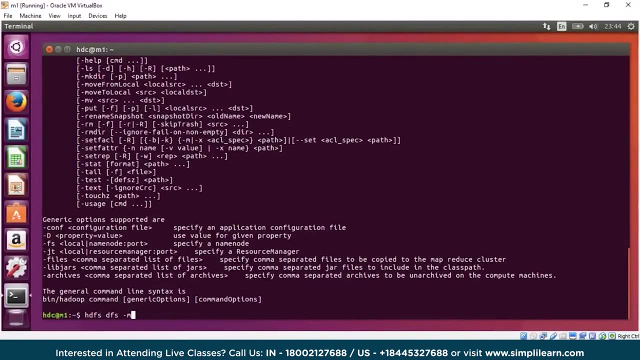 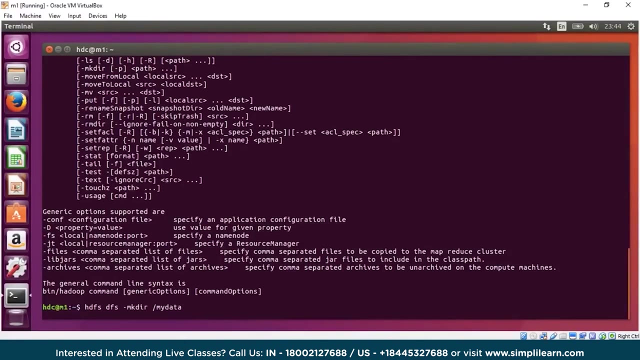 distributed file system, like creating a directory, copying some files, getting data from your SDFS to your local machine, changing the permissions, changing the replication and many other options. so here let's click on HDFS, DFS, let's create a directory and let's call it my data. so this is a directory I am creating on HDFS. remember this directory. 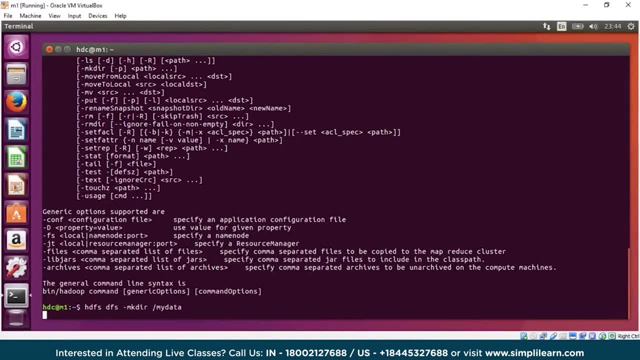 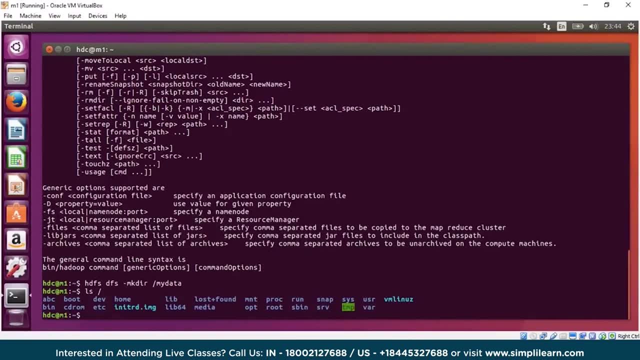 will not be seen on your local machine. it is a HDFS directory. now, if I look in my route, I don't see my data because that says DFS directory which is technically getting created on HDFS. and once you start writing data from HDFS, the relevant blocks will start getting stored under ABC slash data. so 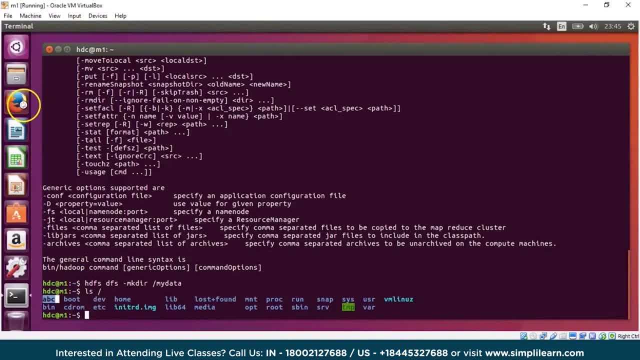 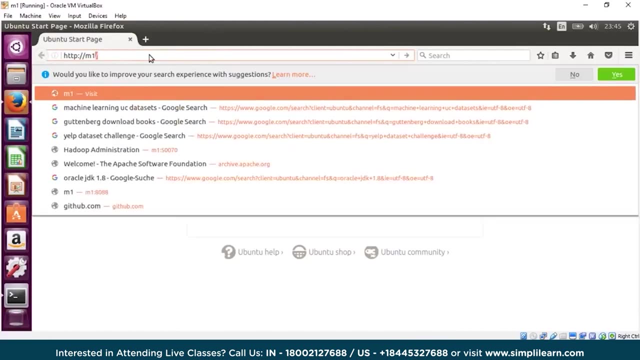 as of now, we can always keep a browser open to see, as we work with HDFS, how does the data propagate or come to your distributed file system using the web interface. so here let's say HTTP slash, slash and one, five, zero, zero, seven, zero, and that's my browser interface. 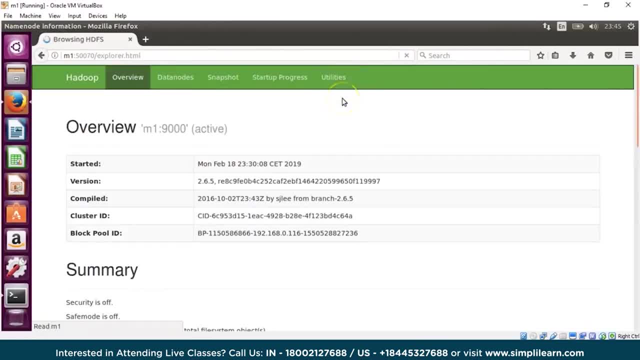 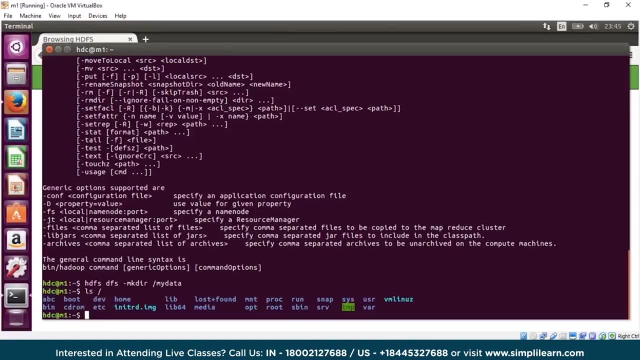 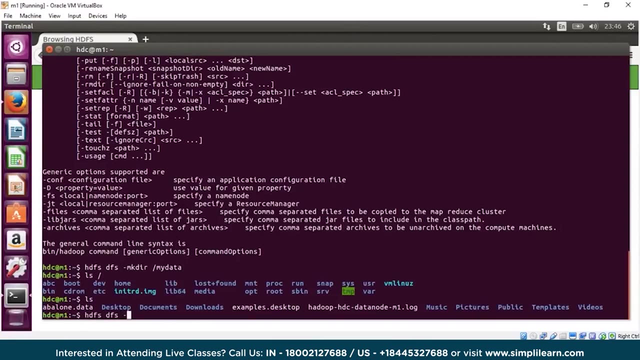 let's click on utilities and let's click on browse, the file system, which will show the directory which we have created, although that does not have any data. as of now, let's go in here, and now we know that we have some files here. so I will say HDFS, DFS, and this has two options: either I can say put or I can. 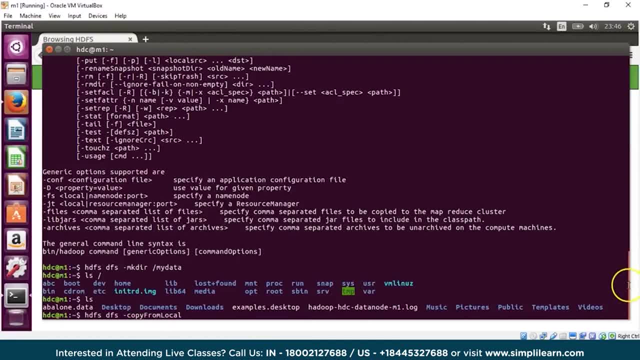 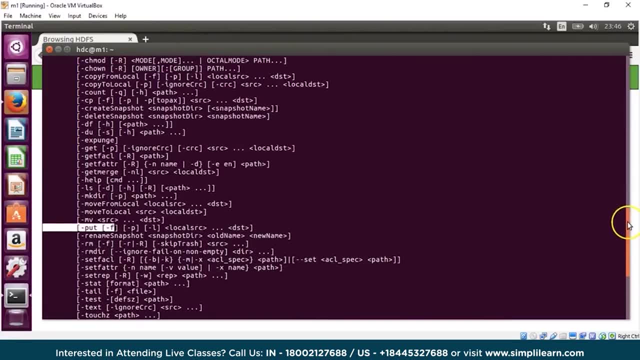 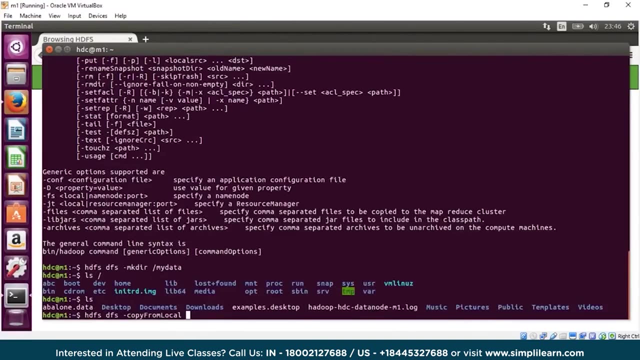 say copy from local. both of these do the same thing and both of these you can find here. so we have put and we should have copy from local. that is, you are copying the data from your local machine to your HDFS. so now I will say copy from local. I will say: take the ABA directory or file. 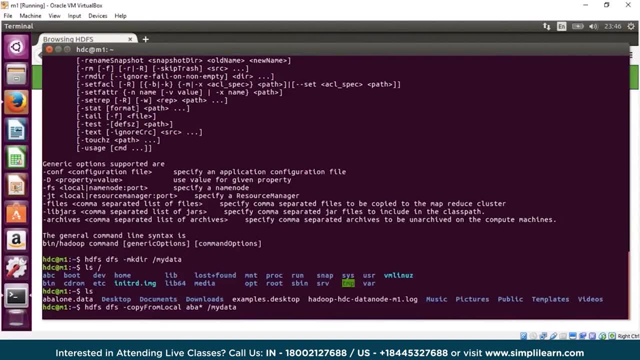 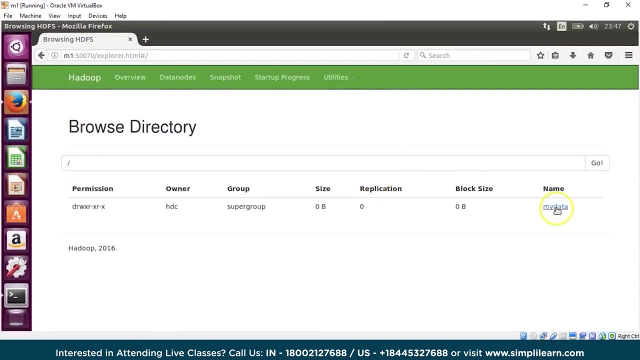 and put it in my data. so now I am technically copying a file from my local file system to my HDFS, which is then using again my local file systems path. so this is done. let's quickly check by clicking on my data if my file is written now. if you see, this file is 187 kilobytes. however, this will still use a. 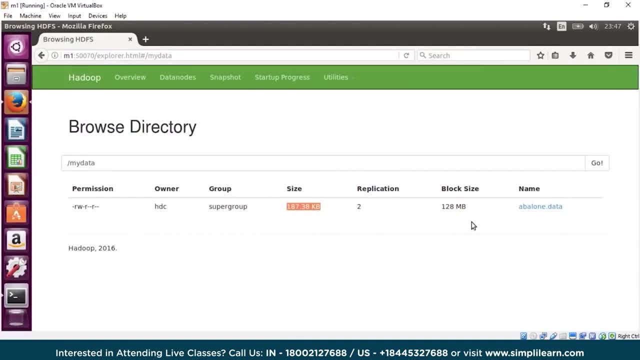 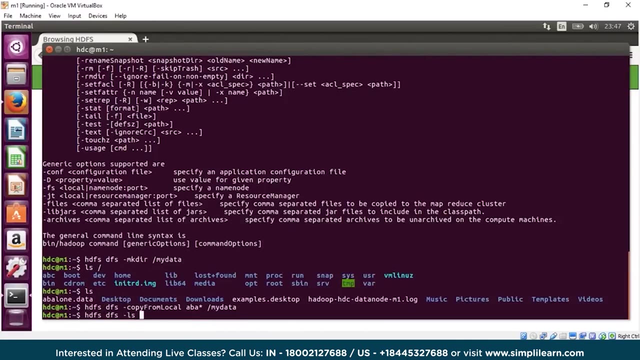 block of 128 and in my previous sessions I already explained why a block of 128. but when it goes to the disk it will only occupy the space for the data the block has. we can quickly go in here and we can do a HDFS, DFS. listing of my 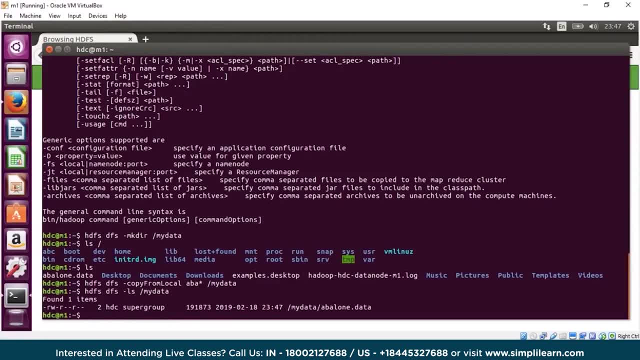 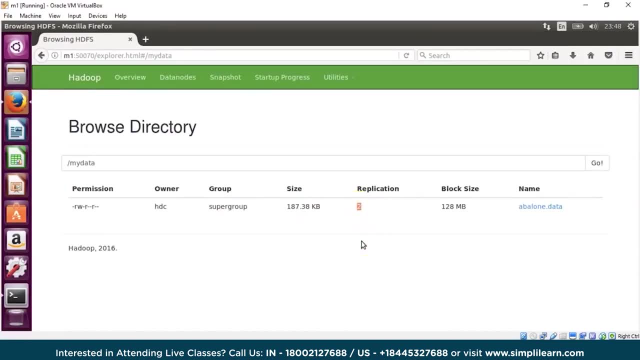 directory which should have my file now, and we can quickly check if my file is replicated either using the web interface, which says replication is 2. that means the file related blocks should be getting stored on the underlying data notes. We can always click on overview if we would want to browse and scroll down, which says: 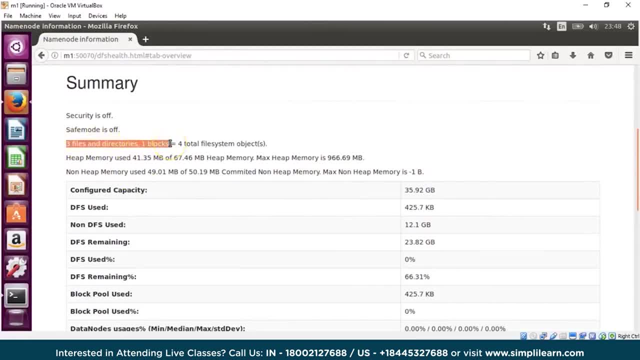 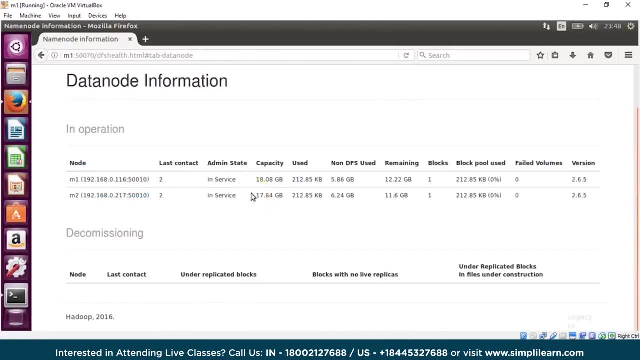 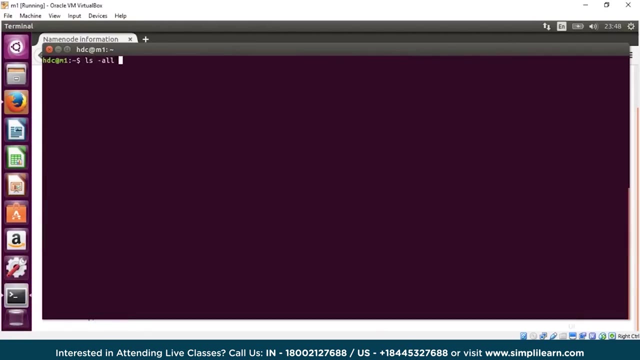 there are three files and a directory. The file has one block, so totally you have four file system objects. We can scroll down to show or see. we have two live notes and if you see each node has one block. We can always look from our data path by looking into ABC slash, data slash, current that has 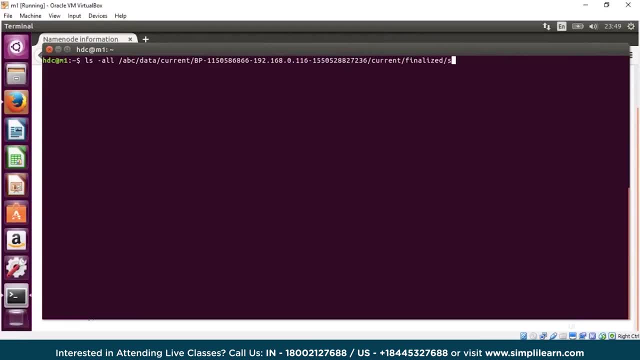 block pool directory that has current, that has finalized, that has subdirectory, subdirectory and the block. Look at the size of the block: it is 191, which relates to the kilobyte size which we are talking about. Similarly, we can check on M2 machine which also has a data note running, to make sure. 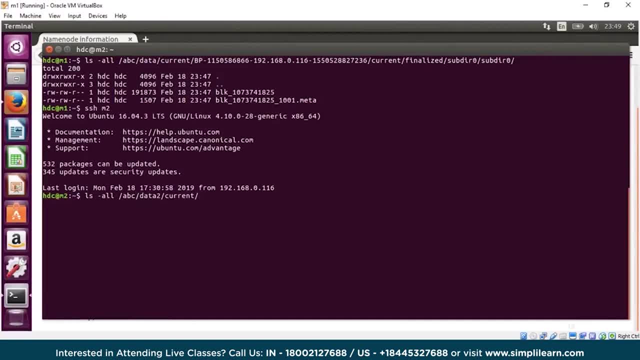 our file related block is replicated. So look in block pool, current finalized subdirectory subdirectory and that shows me the same block which is replicated with its meta file and with the same size. This ensures that my data is getting replicated as per whatever factor we have set and my 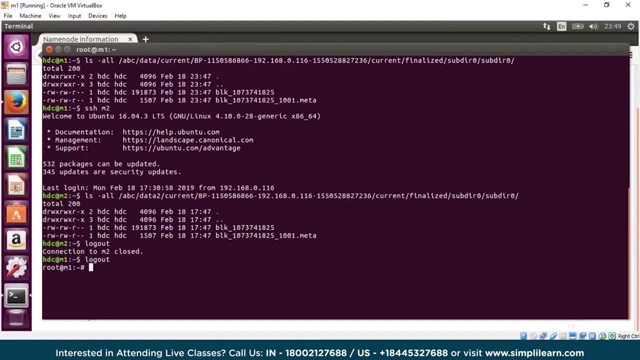 file is written to HDFS. And now I can also see my data. I can also see my data. I can also see my data. I can also do a complete listing. I can just say a recursive listing to show me all the directories and all the files which 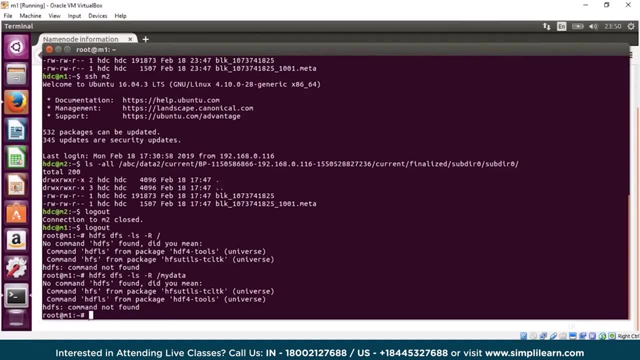 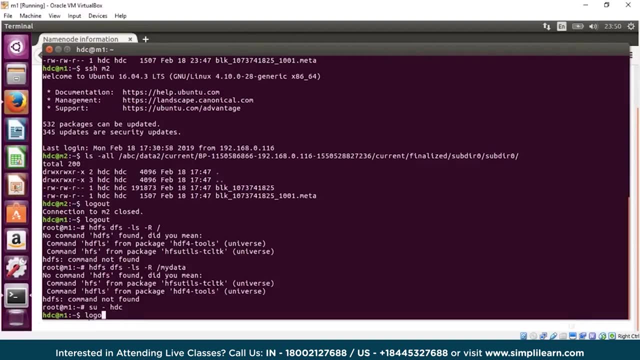 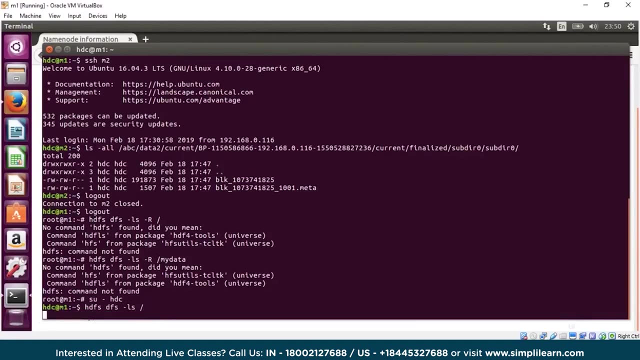 I have in my HDFS. I think we are forgetting something. we are logged in as root, which is not right. So we need to be logged in as HTC and then we can try our commands. that is HDFS, DFS, hyphen, LS, slash, which should show me my directory. but then, if you would want to do a recursive, 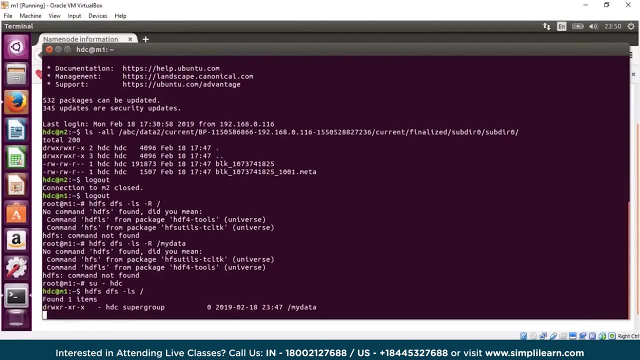 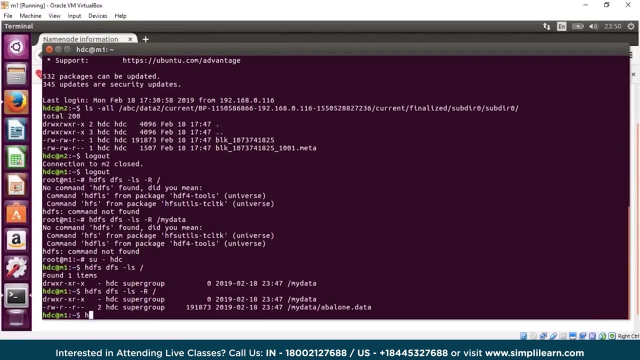 listing of showing all the directories and files. you can just add hyphen R. So we have written a file to HDFS in my data directory. Similarly, I can write using a put command. Last time we used a copy from local, I will use a put command. 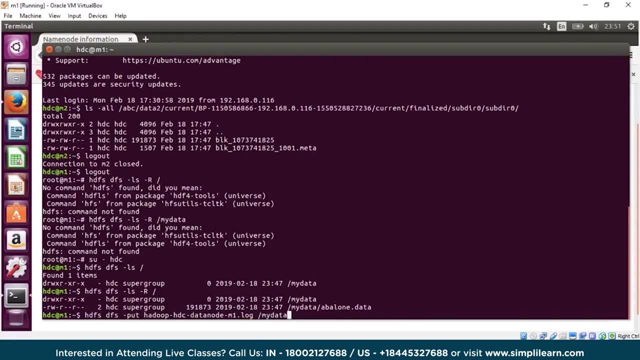 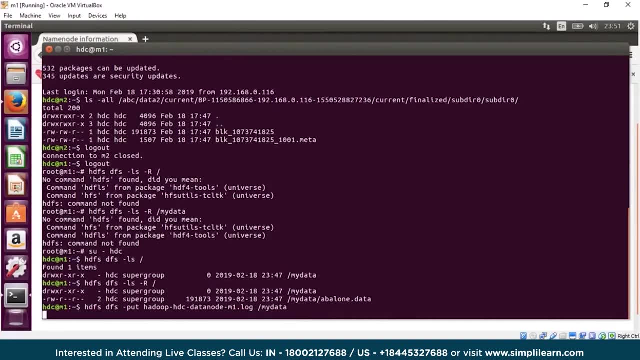 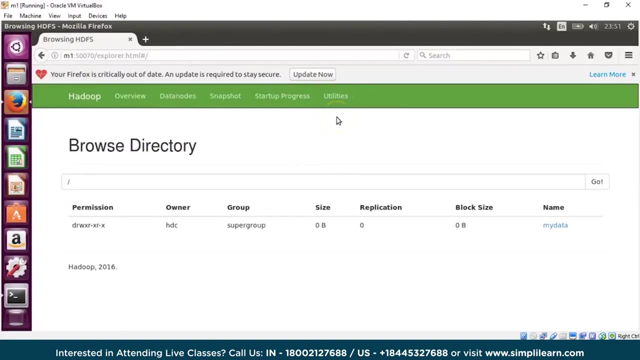 I will say: let's take this log file and let us write it to the my data directory instead of copy from local. I'm using a put command which also allows me to write the file to my HDFS. Once this is done, let's go to the web UI and let's go to browse the file system. 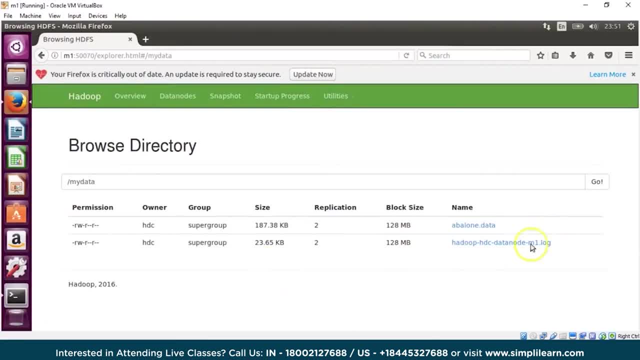 Let's look in our directory and that shows me that I have a log file which is even smaller than the first file which we wrote. It is in kilobytes. however, it is replicated, It is using still the block size and we can always go back and look at the terminal to. 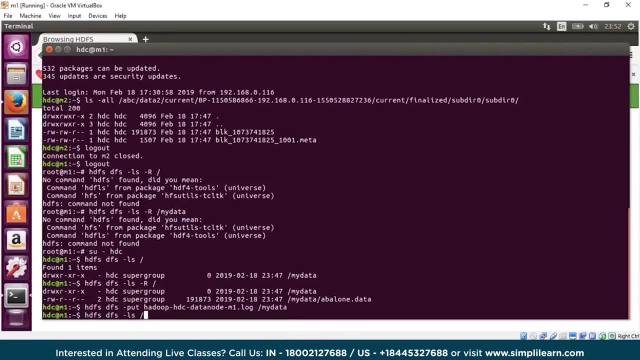 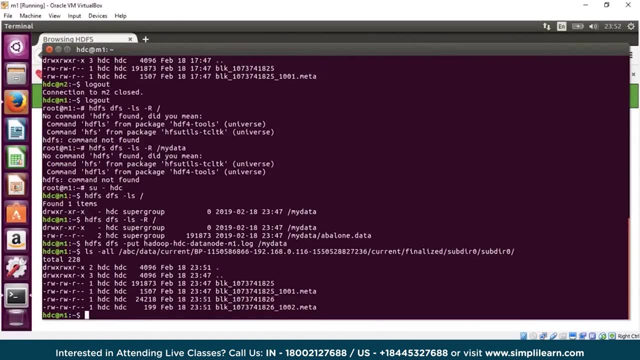 see if, for my new file, I have a new block which should be in my data path, and if you see this, This is my block, which will also have an application on machine 2.. So this is how you write one file, or you could write multiple files. 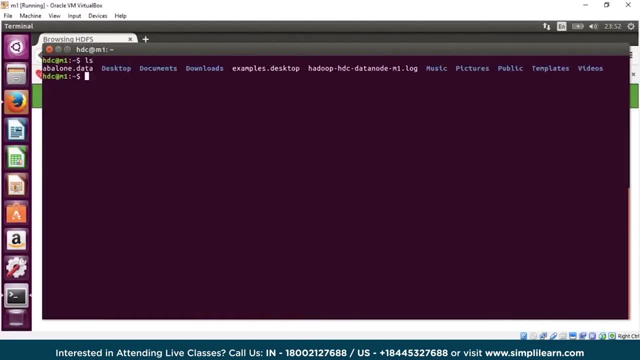 You could write multiple files. Let's create some files here. So I have these log files, Let's say Hadoop log and let's give it a name like this. So now, if you see, I just created multiple files and I can also say HDFS, DFS, make directory. 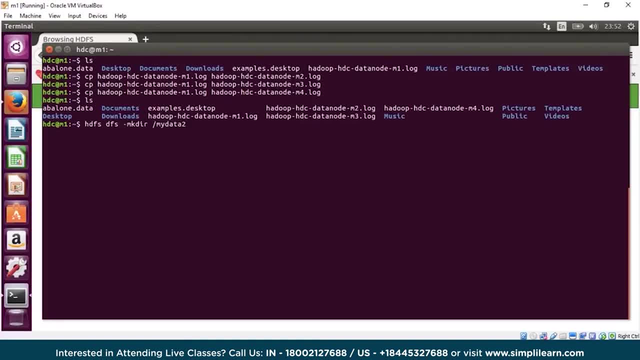 Let's say my data 2.. So I'm creating a new directory on my HDFS and then I can even copy multiple files or a complete directory. So all I need to do here is give a matching pattern or a directory. So I'll say HDFS, DFS, put, and then I can say: take all the directories of files and put. 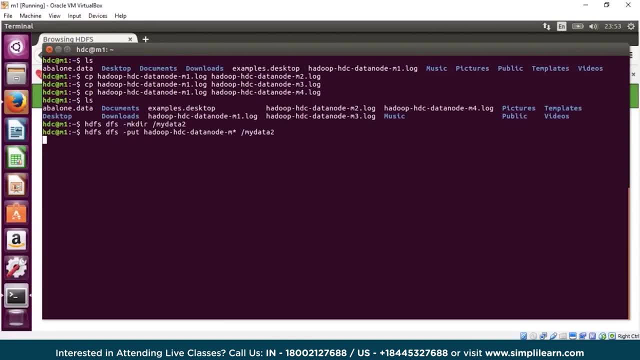 it to my data 2.. Remember this: one file, or multiple files, are following the replication. It has been set at a cluster level. Now, if we do a recursive listing, where I would want to see all the directories and the files which are within my HDFS, 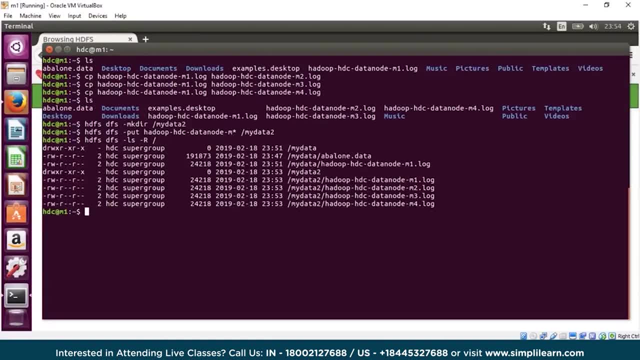 I see that I have a my data directory and I also have a my data 2 directory which has multiple files, and all of the files within the directory are following the replication set at a cluster level, So all of them are having their blocks replicated twice. 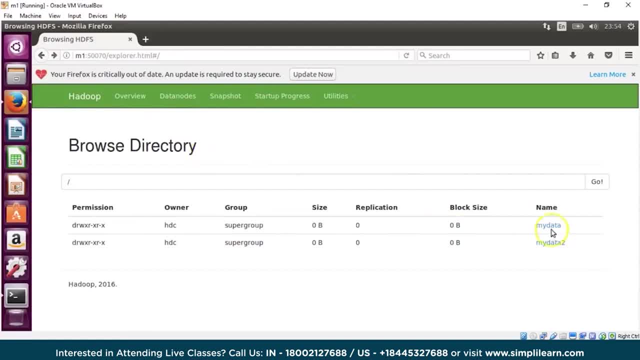 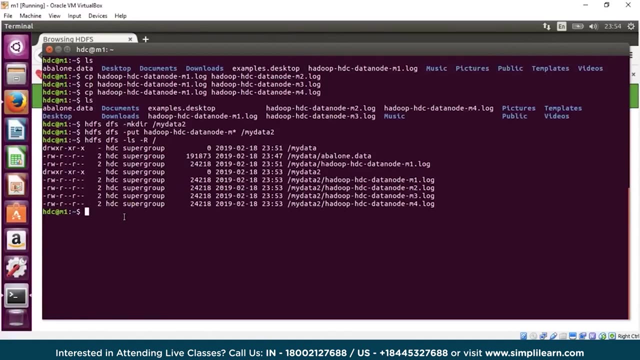 We can always go back here. We can just do it, Go back, and that shows me what I have in my data. 2. Everything is replicated twice. What I have in my data is also replicated twice. Now HDFS also has a functionality where you can write data with a different replication. 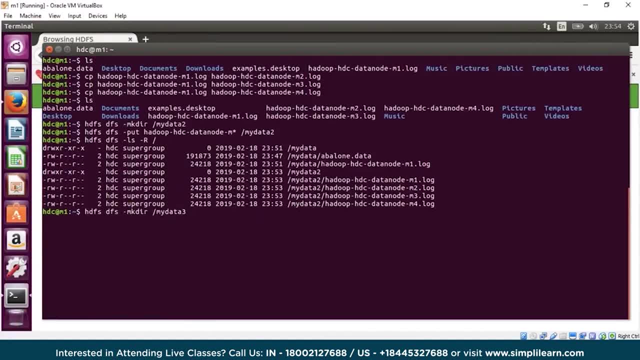 So let's create one more directory and now let's write data with a different replication. So the way I write my files, I follow the same thing. However, now I will say hyphen DFS Replication and I will specify it as one. 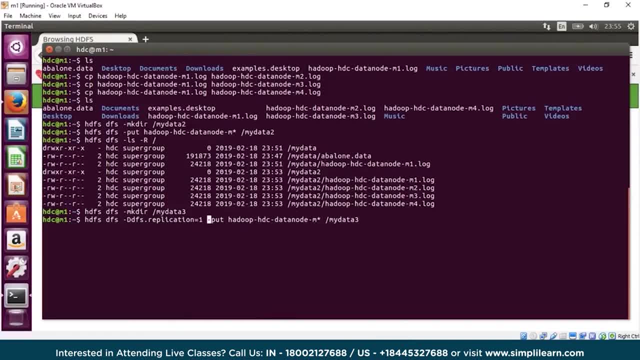 So I'm passing in as argument and I am specifying that I would want to write data with the replication of just one. So my blocks will not be considered under replicated and I'm choosing to write these files in this directory with the replication of one. 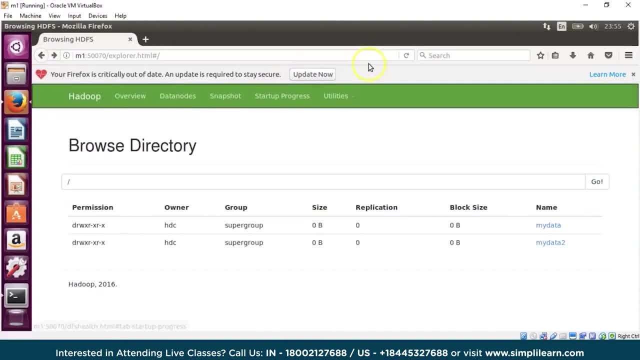 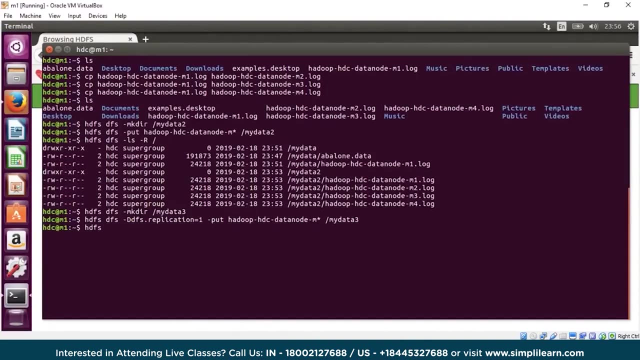 We can check from our browser interface by just doing a quick refresh, and here, if I click on my data 3, it shows it follows a replication of one. There is also a command to check your replication status using HDFS. So we can say HDFS, fsck, slash files, slash, blocks, and if I would want to see only blocks, 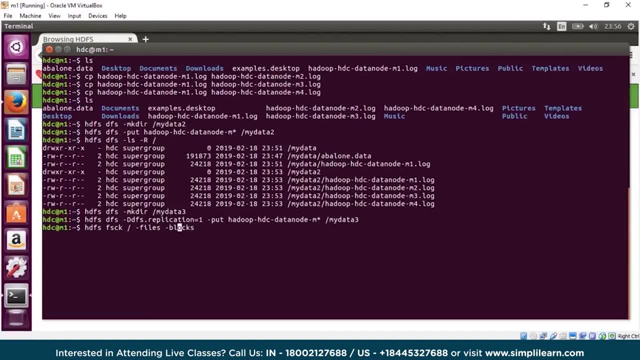 or only files. I could choose one of them. Now, here I have given a complete HDFS file system. I can replace that with slash- my data, So I can say my data 3.. This is what I would want. I want to see, and this will show me within this directory how many files I have, how. 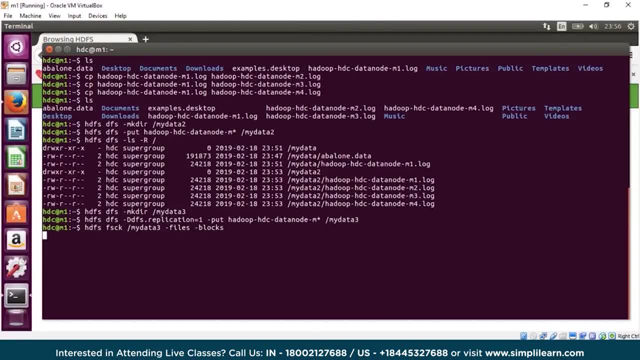 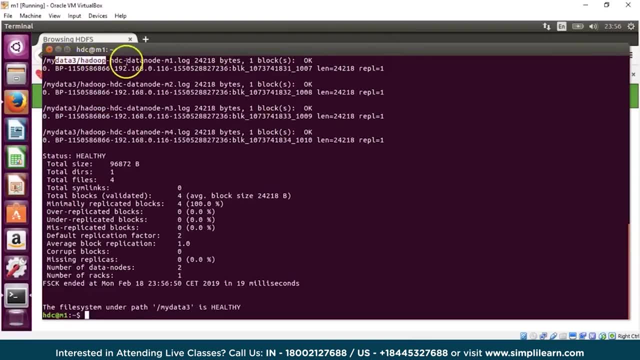 many blocks does each file use and is it replicated correctly? So my fsck command gives me an information that in my data 3, I have one file which is 24 kilobytes- uses one block because it's very smaller than 128 and it is replicated. 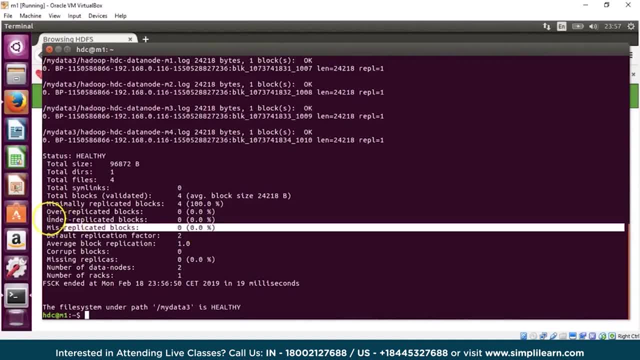 only once. So there is no situation of over under misreplicated blocks. We have our files correctly Replicated as they were specified. while writing, Same thing can be seen for other files, say my data 2, and that will tell me that all the 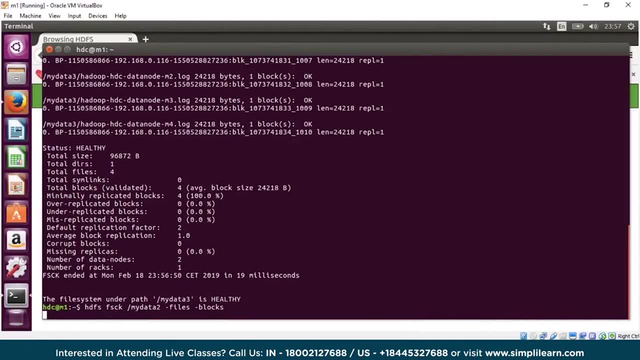 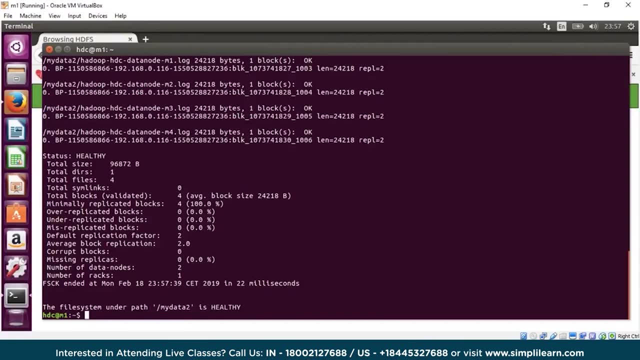 files within my data 2 were replicated as per the default replication, which was at a cluster level, And if you see, here everything is replicated twice. We don't have any over under misreplicated blocks and my file system status is healthy. 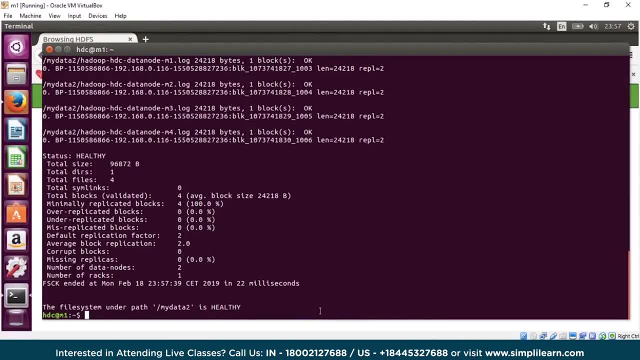 So this is the HDFS command to make sure that your files are replicated correctly. So that's it. So we have seen how your files are written with default replication. We have seen how your files follow a dynamic replication, what you specify on the command. 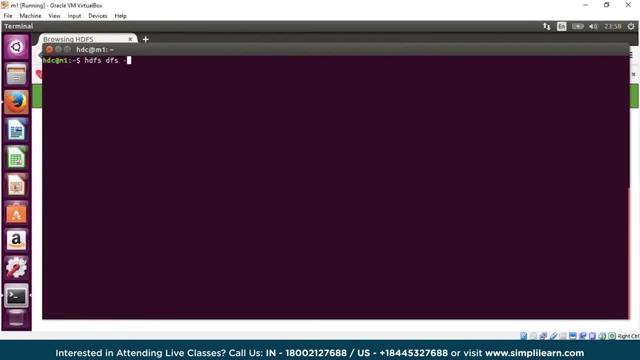 line. Now we can also see a command which allows us to change replication after the data has been written. So I can say set rep and I can say path. that is my data 3, where I initially had all my file related blocks replicated only once. 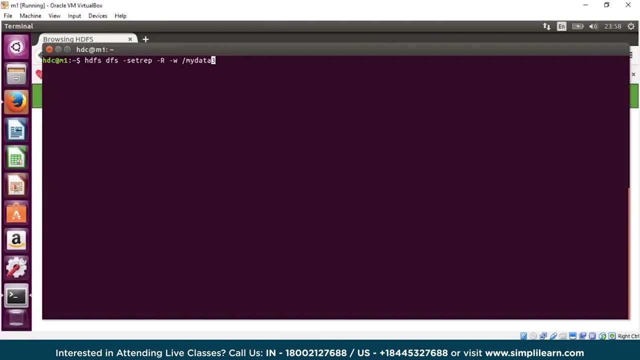 And now I'll say my data 2.. And I can specify that this should follow a replication of 2, which basically means that it will look into the directory, it will check all the files which had only one block, and now it will create a replica of those blocks across other data nodes. 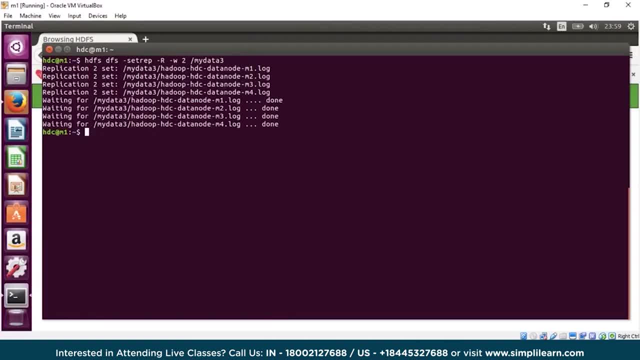 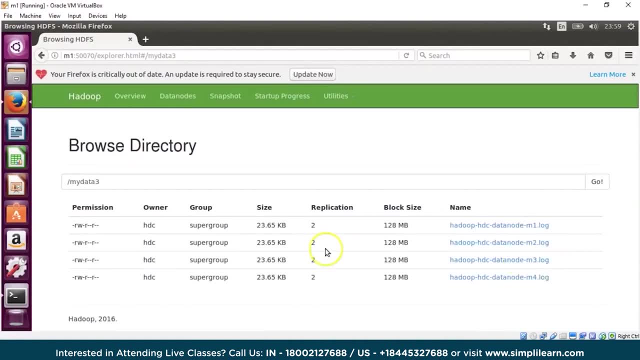 We can always go back and look into the data node logs to see the replication happening. We can also look from the browser interface, which initially was showing a replication of one, Now it shows a replication of two. So this is the command to change the replication after the data has been written. 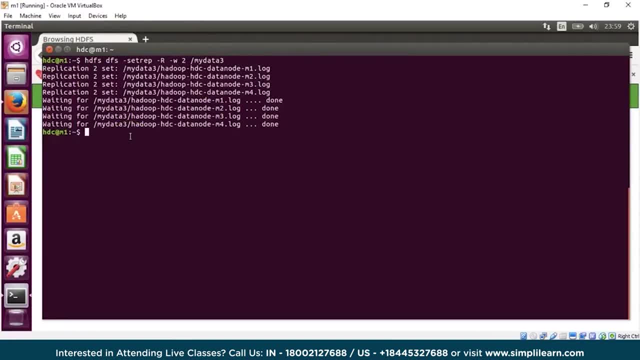 So our writes can have default replication. We can write files with a different replication. We can change the replication after the data is written. Not only that, we can even get the data from our HDFS to my local machine, And for that I'll give HDFS get command or copy to local. 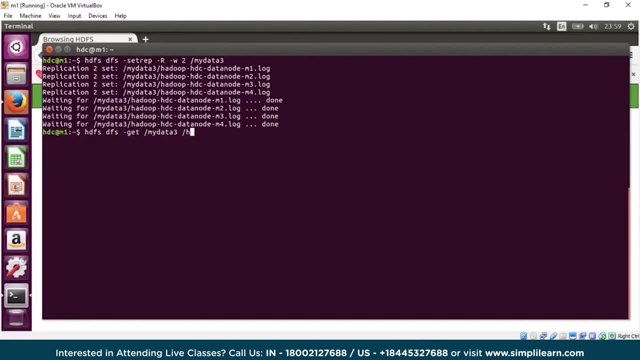 So I can say: my data 3.. And then I can bring it to my local machine. And then I can bring it to my local machine, And then I can bring it to my local machine in home HDC using a get command. So this is to get data from your HDFS to your local machine using a HDFS command. 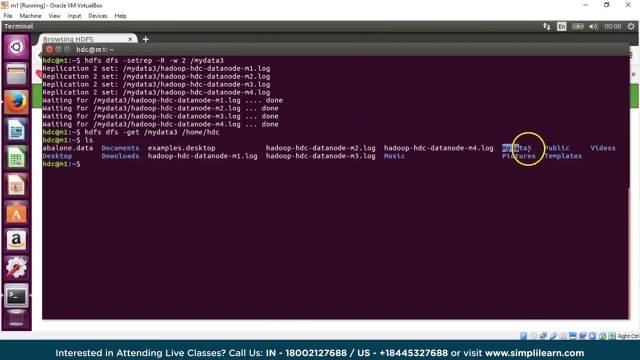 Now, if you see, I should have a my data 3 directory which is in my local path And we can look in my data 3.. It has all the files which we had on HDFS. So we were not only putting data from our local machine to HDFS, we also successfully- 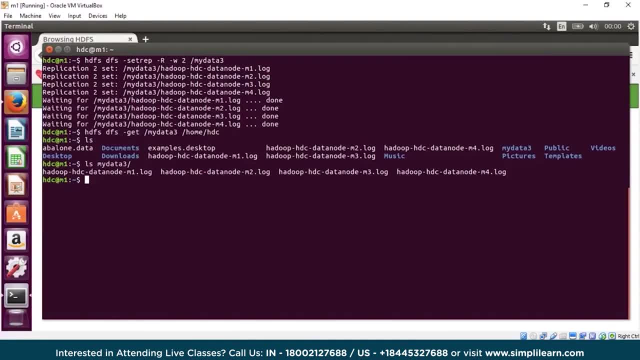 brought data from our HDFS to my local machine. So this is to get data from our local machine. We have written data with different replication. We have checked the status of nodes, We have checked the status of blocks And if we would want to delete some data, HDFS also has options for that. 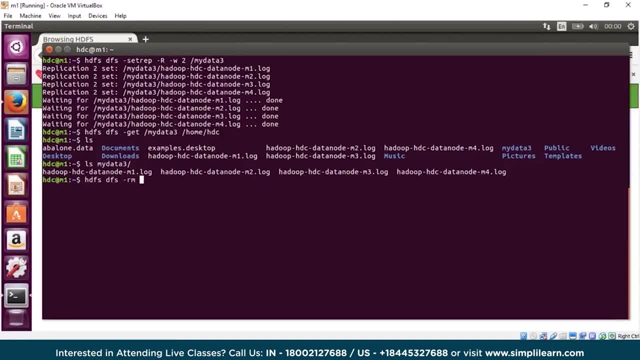 So I can say HDFS, DFS, remove, And I could also do a recursive remove to remove everything, including the directory, from my data 3.. So this will delete data from my HDFS. However, if that is not possible, I can also remove the data from my data 3.. 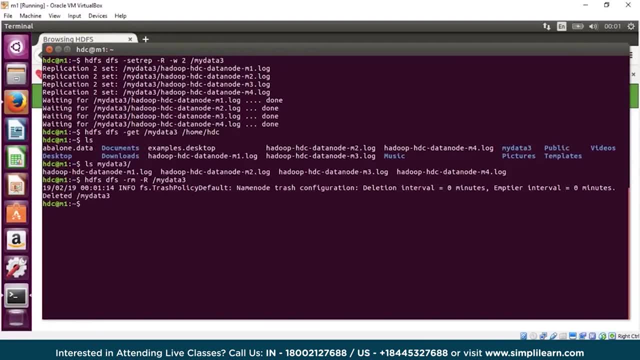 So this will delete data from my HDFS. The second step is to set up a thrash. So what we have done is we have set up a thrash Now. thrash is basically means recycle bin, which depends on a property in the core-site. 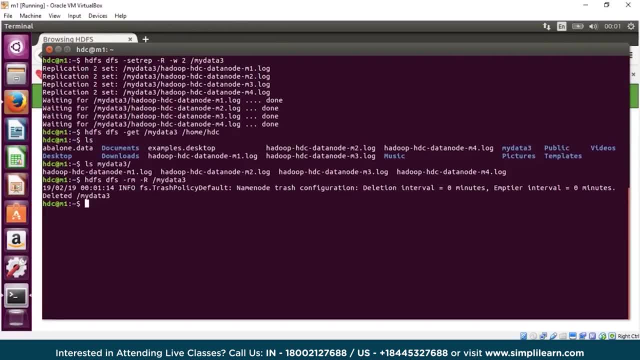 file. We have not enabled it. If thrash is enabled, then your data will be deleted from HDFS. However, it will not be permanently deleted. It will sit in thrash for a time interval that admin has specified in the configuration file. 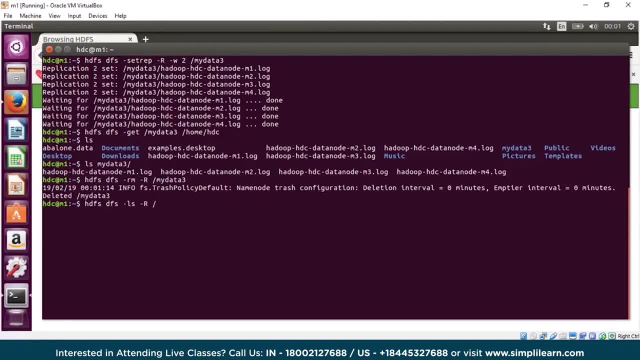 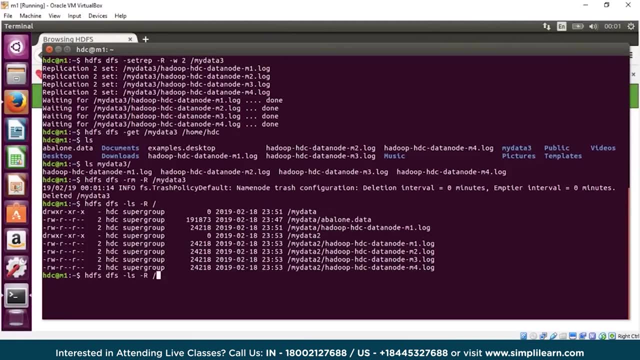 So right now I deleted thrash and this seems to be gone from HDFS because we have not set up any thrash. It will not go to the storage. However, if it's not set up, then it will be removed. is set up, then either you can decide to have your data deleted and still be in. 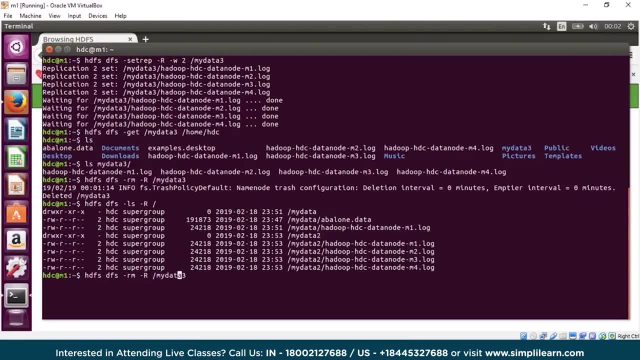 thrash so that it could be restored or you could delete it permanently using a skip thrash option. however, remember, this skip thrash option makes more sense if the thrash is enabled in your cluster and you do not want your deleted data to be sitting in thrash even for whatever time interval has been set, because even 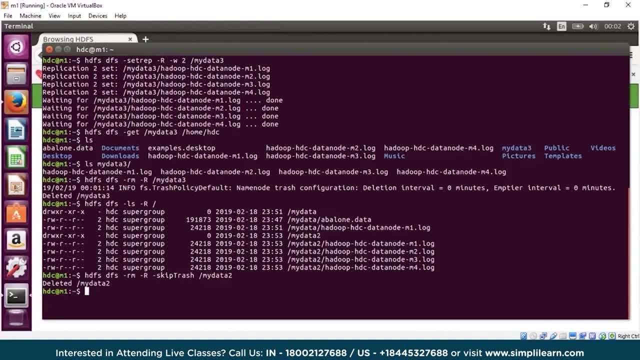 if the data sits in thrash and your thrash is a directory structure on HDFS, all the data will still be replicated. so we have seen how you can write data to the cluster, how you can get data from cluster to your local machine, how you can write it with different replications, how you can delete it from your cluster. 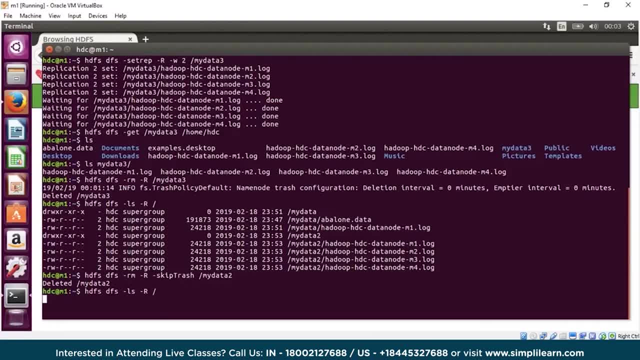 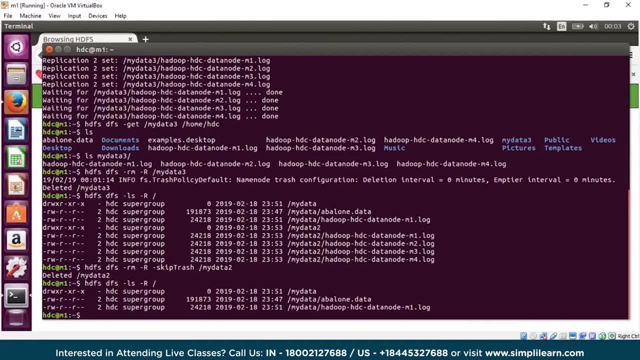 and do a recursive listing of your directories and files. now there are various other commands which can be used, for example, something like copy or move, or delete or delete something like that. so if you want to delete or delete something or change permissions and many more. thanks, ajay, now we have richard and ajay. 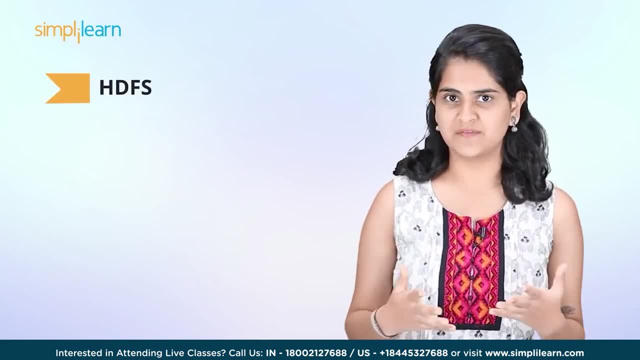 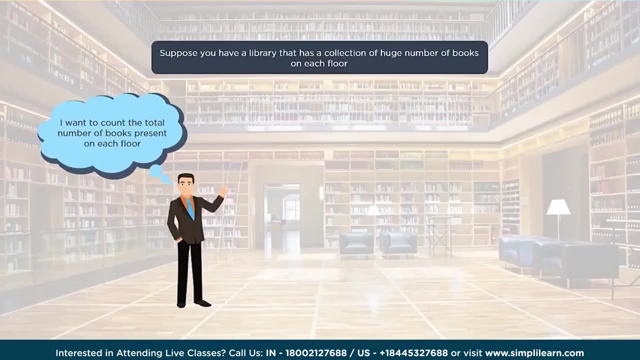 taking us through the hadoop ecosystem. we will look into HDFS, map reduce, yarn, scoop, hide pig and hbase. suppose you have a library that has a collection of huge number of books on each floor and you want to count the total number of books present on each floor. what would be your approach? you could say: i will do. 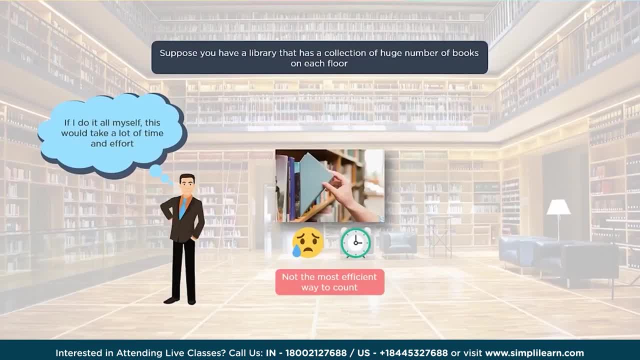 it myself, but then don't you think that will take a lot of time and that's the obviously not an efficient way of counting the number of books in this huge collection on every floor by yourself? now there could be a different approach or an alternative to that. you could think of asking three of your. 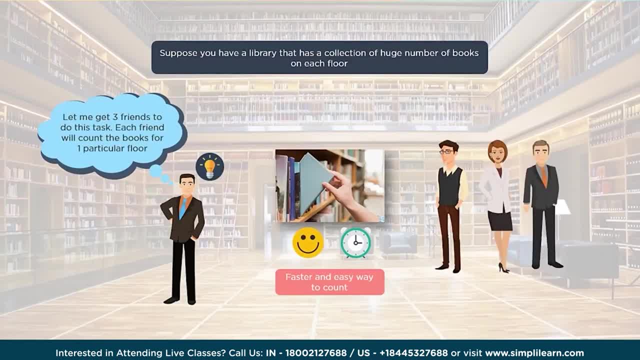 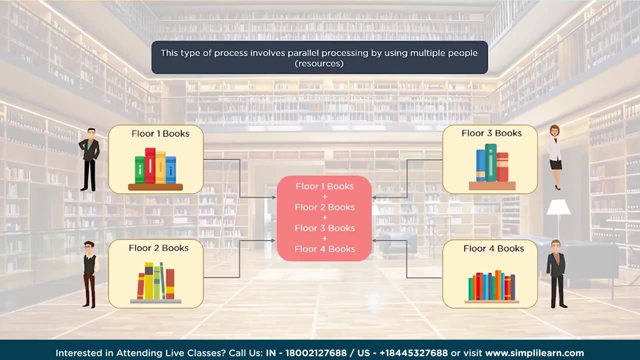 friends or three of your colleagues, and you could then say: if each friend could count the books on every floor, then obviously that would make your work faster and easier. to count the books on every floor. now this is what we mean by parallel processing. so when you say parallel processing in technical terms, you're talking about 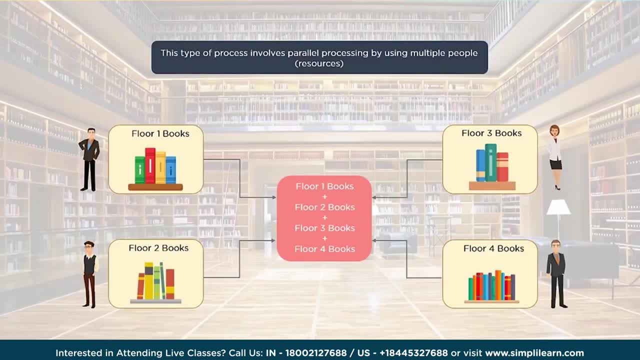 using multiple machines and each machine would be contributing its RAM and CPU cores for processing and your data would be processed on multiple machines at the same time. now this type of process involves parallel processing, in our case or in our library example, where you would have person 1 who would be taking 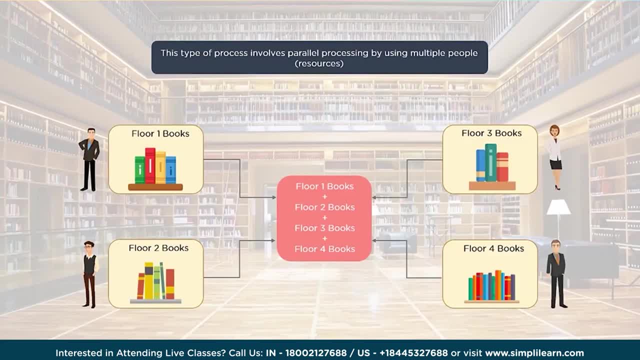 care of books on floor 1 and counting them person 2 on floor 2, then you have someone on floor 3 and someone on floor 4, so every individual would be commenting the books on every floor in battle, so that reduces the time-consuming for this activity. and then there should be some 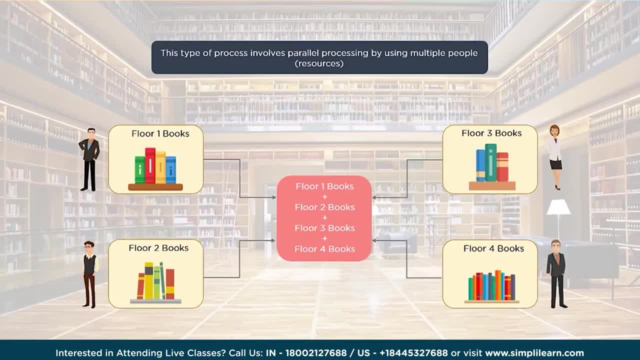 mechanism, all these phones from every floor can be aggregated. so what does it with him doing here? each person is mapping the data of a particular floor. all you can see. each person is doing a kind of activity or basic ico, ico, a task on every floor, and the task is counting the books on every floor. Now then you could have. 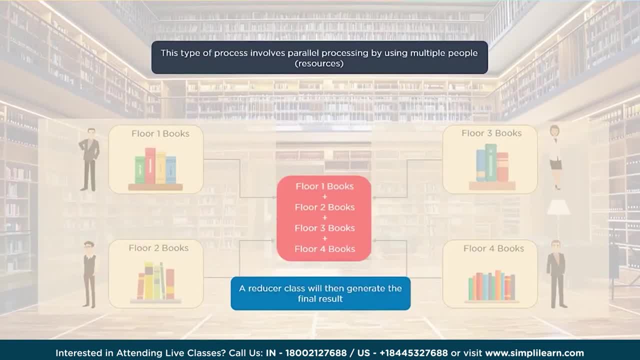 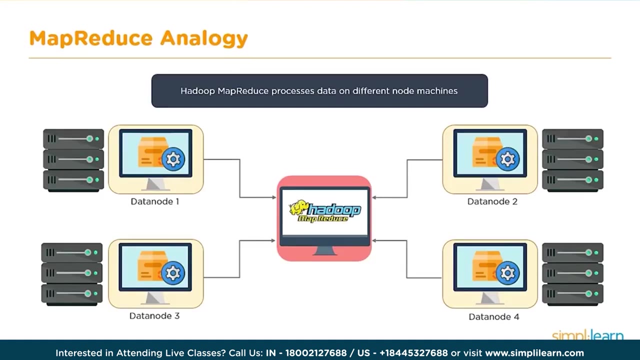 some aggregation mechanism that could basically reduce or summarize this total count and in terms of MapReduce, we would say that's the work of reducer. So when you talk about Hadoop MapReduce, it processes data on different node machines. Now this is the whole concept of Hadoop framework. 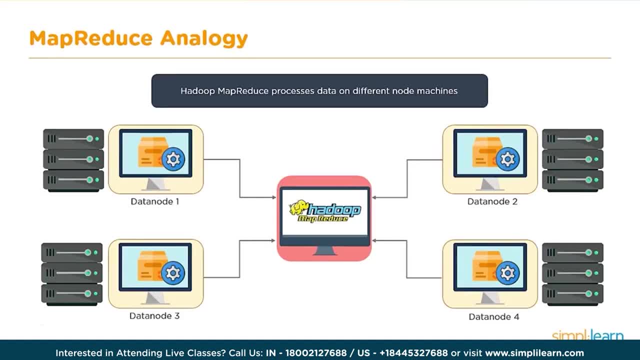 right that you not only have your data stored across machines, but you would also want to process the data locally. So instead of transferring the data from one machine to other machine, or bringing all the data together into some central processing unit and then processing it, you would 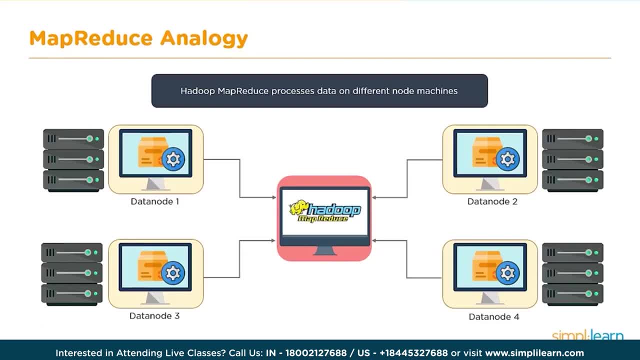 rather have the data processed on the machines, wherever that is stored. So we know, in case of Hadoop cluster, we would have our data stored on multiple data nodes, on their multiple disks, and that is the data which needs to be processed. but the requirement is that we want to process this. 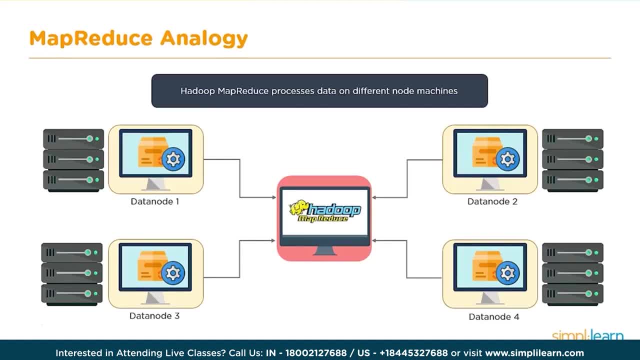 data as fast as possible, and that could be achieved by using parallel processing. Now, in case of MapReduce, we basically have the first phase, which is your mapping phase. So, in case of MapReduce programming model, you basically have two phases: one is mapping and one is reducing. Now who takes care of things? 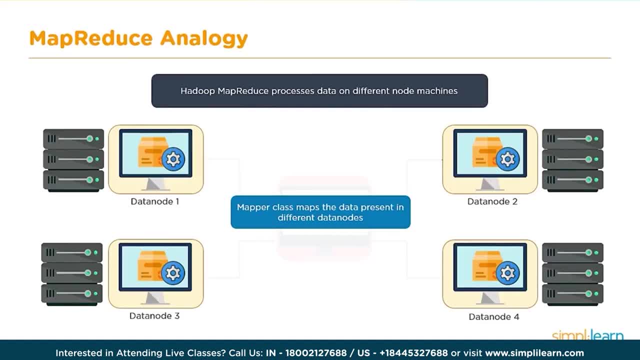 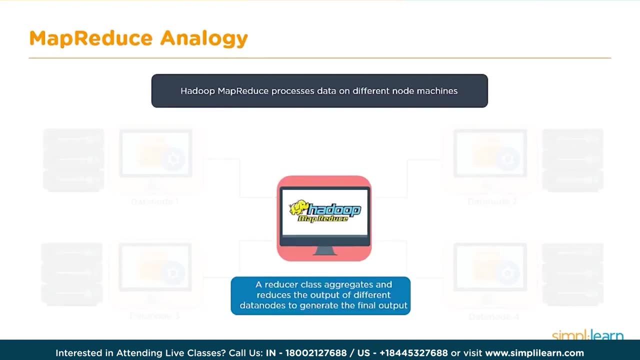 in mapping phase. It is a mapper class and this mapper class has the function which is provided by the developer, which takes care of these individual map tasks which will work on multiple nodes in parallel. Your reducer class belongs to the reducing phase, So a reducing phase basically uses a reducer class which provides a function. 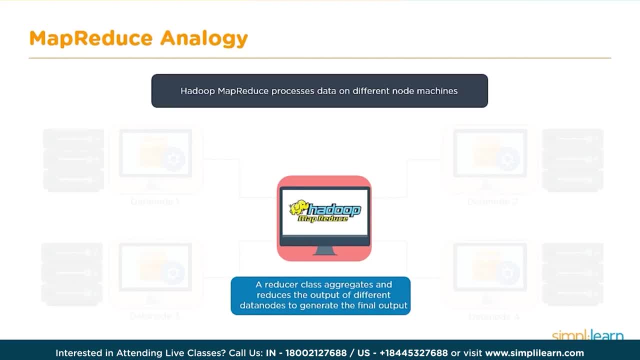 that will aggregate and reduce the output of different data nodes to generate the final output. Now that's how your MapReduce works, using mapping and then, obviously, reducing. Now you could have some other kind of jobs which are map only jobs, wherein there is no reducing required. but we 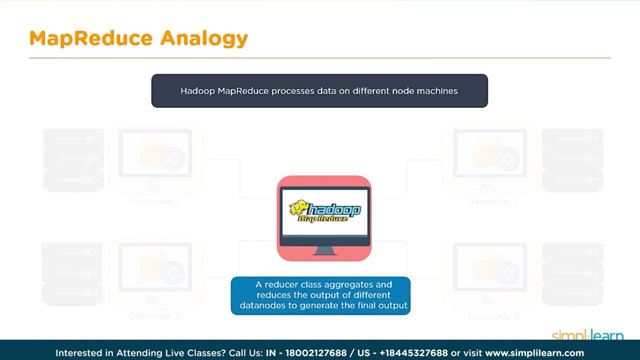 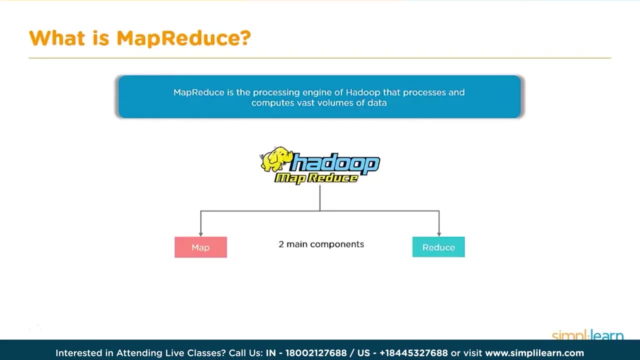 are not talking about those. We are talking about our requirement where we would want to process the data using mapping and reducing, especially when data is huge, when data is stored across multiple machines and you would want to process the data in parallel. So when you talk about MapReduce you 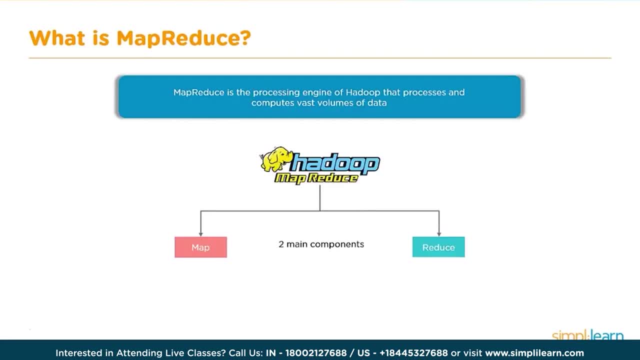 could say it's a programming model. you could say, internally, it's a processing engine of Hadoop that allows you to process the data in parallel. So when you talk about MapReduce, you could say it's a processing engine of Hadoop that allows you to process and compute huge volumes of data. and when 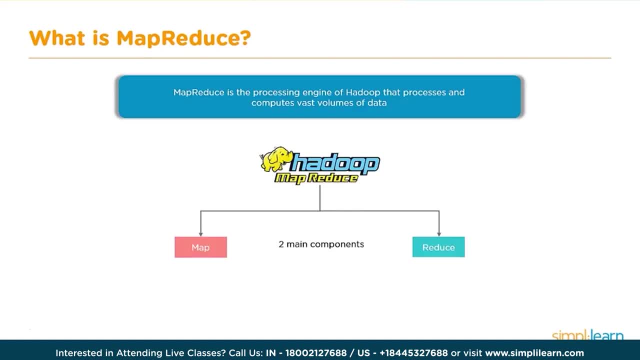 we say huge volumes of data, we can talk about terabytes, we can talk about petabytes, exabytes and that amount of data which needs to be processed on a huge cluster. We could also use MapReduce programming model and run a MapReduce algorithm in a local mode, But what does that mean? 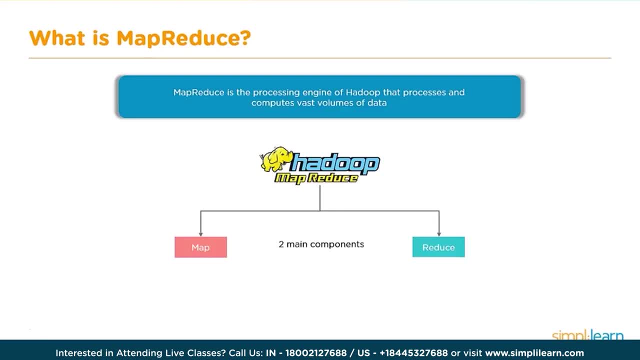 If you would go for a local mode, it basically means it would do all the mapping and reducing on the same node using the processing capacity that the data is stored across multiple machines. You could also use Hadoop MapReduce, that is, RAM and CPU cores on the same machine, which is not really. 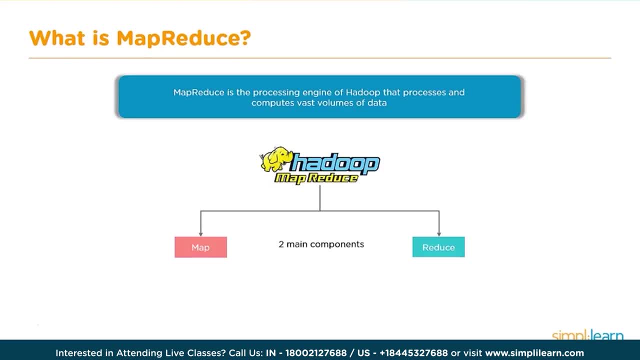 efficient. In fact, we would want to have our MapReduce work on multiple nodes, which would obviously have mapping phase followed by a reducing phase and intermittently there would be data generated. There would be different other phases which help this whole processing. So when you talk, 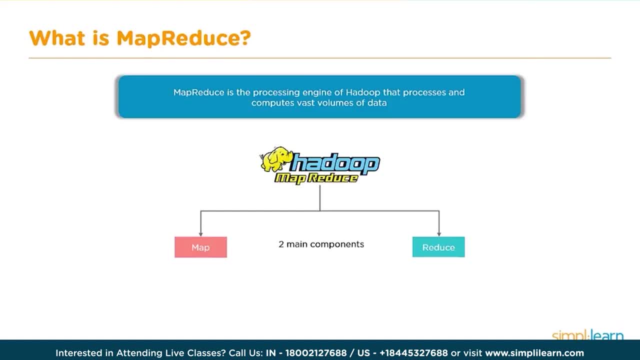 about Hadoop, MapReduce. you are mainly talking about two main components or two main phases, that is, mapping and reducing mapping, Taking care of Map Tasks, taking care of reduced tasks, so you would have your data which would be stored on multiple machines. now, when we talk about data, data could be in. 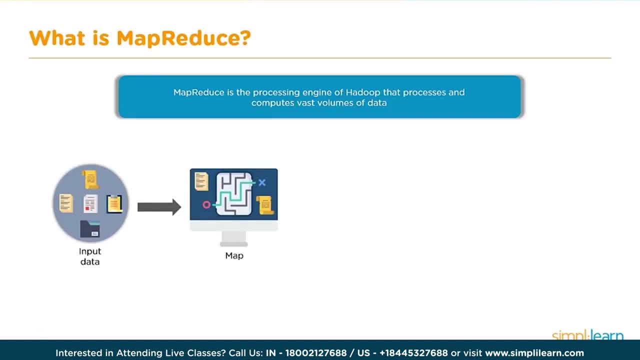 different formats. we could, or the developer could, specify what is the format which needs to be used to understand the data which is coming in. that data then goes through the mapping internally. there would be some shuffling, sorting and then reducing, which gives you your final output. so the way we 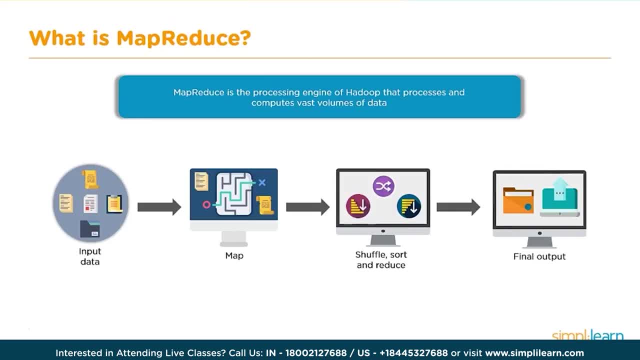 access data from sdfs or the way our data is getting stored on sdfs. we have our input data, which would have one or multiple files and one or multiple directories, and your final output is also stored on sdfs to be accessed, to be looked into and to see if the processing was done correctly. so this is how it. 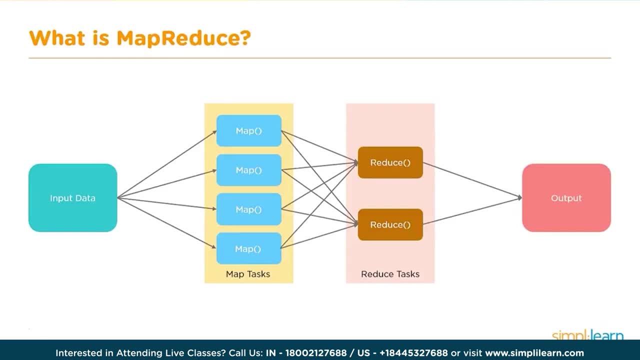 looks. so you have the input data, which would then be worked upon by multiple map tasks. now, how many map tasks? that basically depends on the file. that depends on the input format. so normally we know that in a hadoo cluster you would have a file which is broken down into blocks. 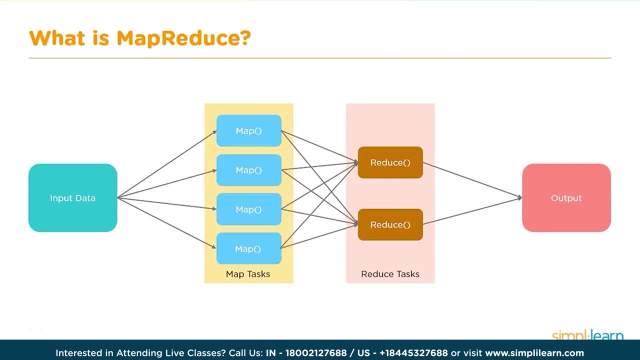 depending on its size. so the default block size is 128 mb, which can then still be customized based on your average size of data which is getting stored on the cluster. so if i have really huge files which are getting stored on the cluster, i would certainly set a higher block size. 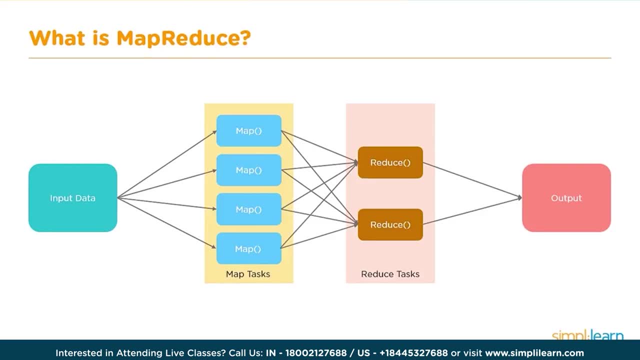 so that my every file does not have huge number of blocks creating a load on name note size. so if i have a huge file which is getting stored on the name notes ram, because that's tracking the number of elements in your cluster or number of objects in your cluster, 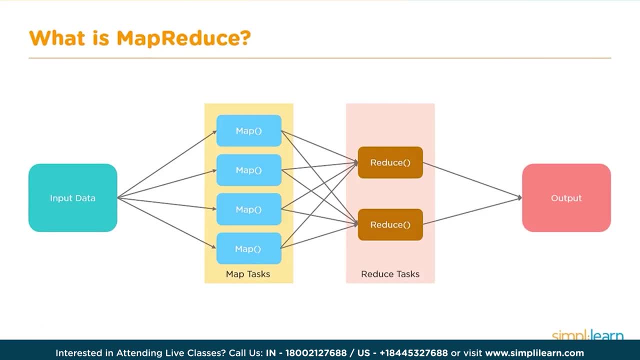 so, depending on your file size, your file would be split into multiple chunks and for every chunk we would have a map task running. now what is this map task doing? that is specified within the mapper class. so within the mapper class you have the mapper function, which basically says: 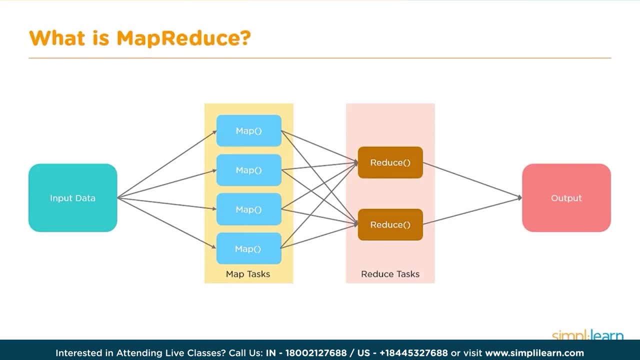 what each of these map tasks has to do on each of the chunks which has to be processed. this data, intermittently, is written to sdfs, where it is sorted and shuffled, and then you have internal phases, such as partitioner, which decides how many reduced tasks would be used or what data. 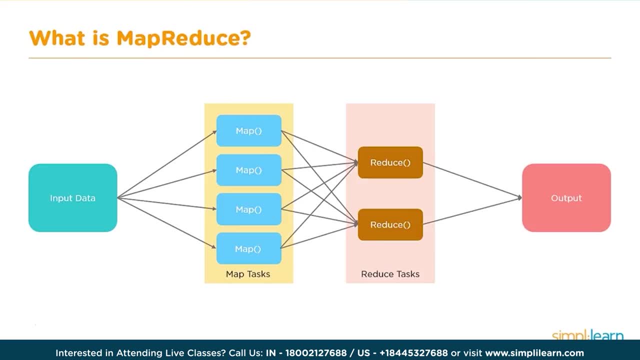 goes to which reducer. you could also have a combiner phase, which is like a mini reducer doing the same reduce operation before it reaches reduce. then you have your reducing phase, which is taken care by a reducer class and that can be used to monitor the user function provided by developer, which 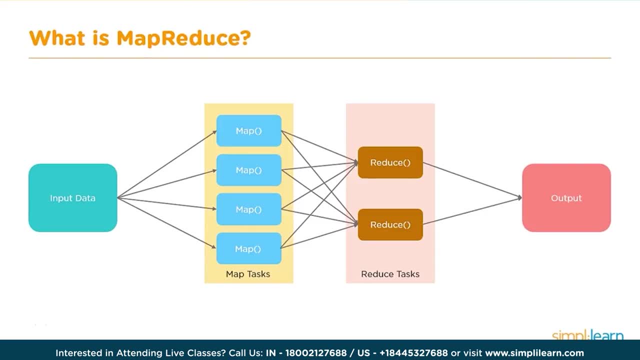 would have reduced task running on the data which comes as an output from map tasks. finally, your output is then generated, which is stored on sdfs. now, in case of hadoop, it accepts data in different formats. your data could be in compressed format. your data could be in parquet. your data could be in avro. 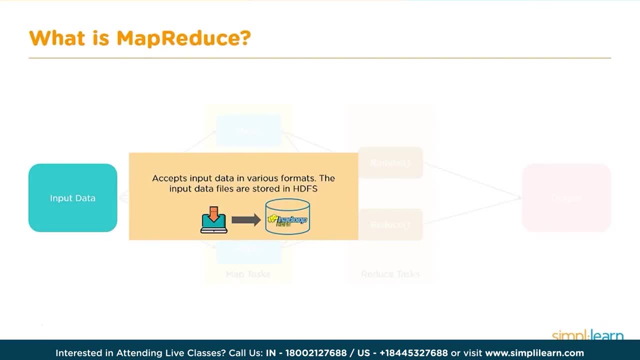 text, csv, tsv, binary format and all of these formats are supported. however, Remember, if you are talking about data being compressed, then you have to also look into what kind of splitability the compression mechanism supports. Otherwise, when MapReduce processing happens, it would take the complete file as one chunk. 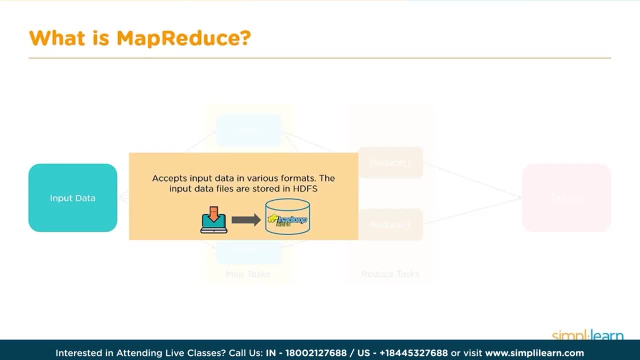 to be processed. So SDFS accepts input data in different formats. This data is stored in SDFS and that is basically our input, which is then passing through the mapping phase. Now what is mapping phase doing? As I said, it reads record by record. 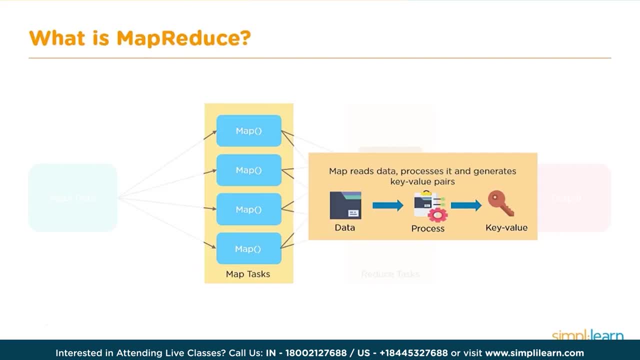 Depending on the input format, it reads the data. So we have multiple map tasks running on multiple chunks. Once this data is being read, this is broken down into individual elements, And when I say individual element, I could say this is my list of key value pairs. 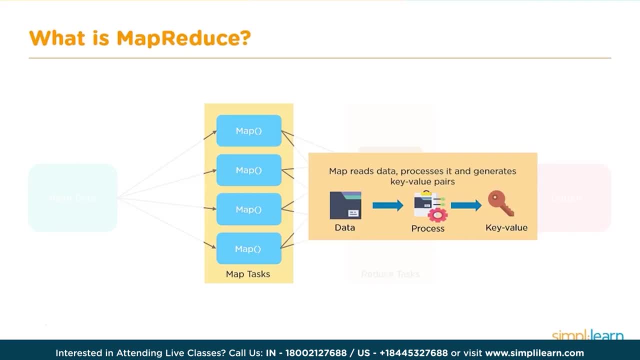 So your records, based on some kind of delimiter, or without delimiter, are broken down into individual elements, And thus your map creates key value pairs. Now, these key value pairs are not my final output. These key value pairs are basically a list of elements which will then be subjected to. 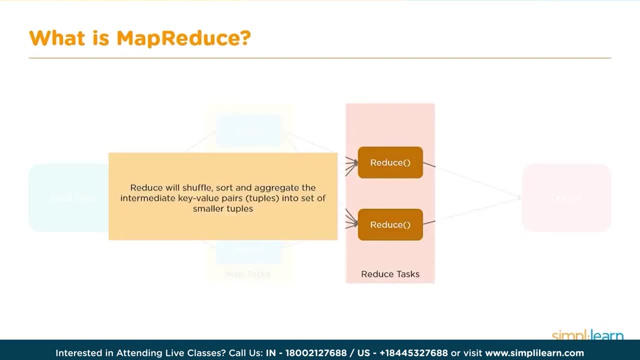 further processing. So you would have internally shuffling and sorting of data so that all the relevant key value pairs are brought together, which basically benefits the processing, And then you have your reducing, which aggregates the key value pairs into set of smaller tuples. 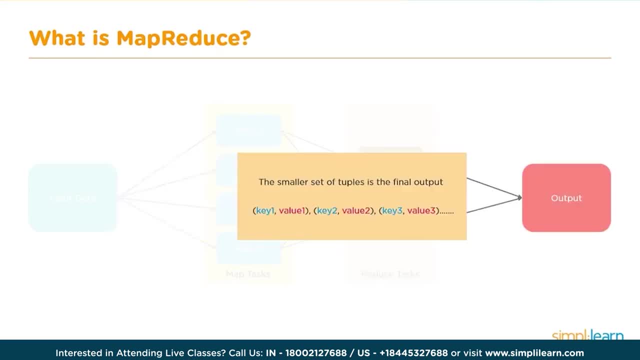 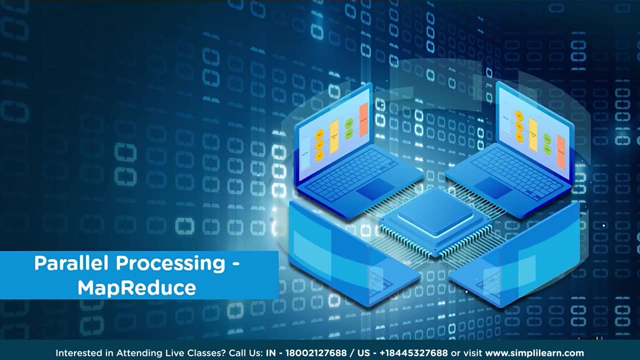 or tuples, as you would say. Finally, your output is getting Stored in the designated directory as a list of aggregated key value pairs, which gives you your output. So, when we talk about MapReduce, one of the key factors here is the parallel processing. 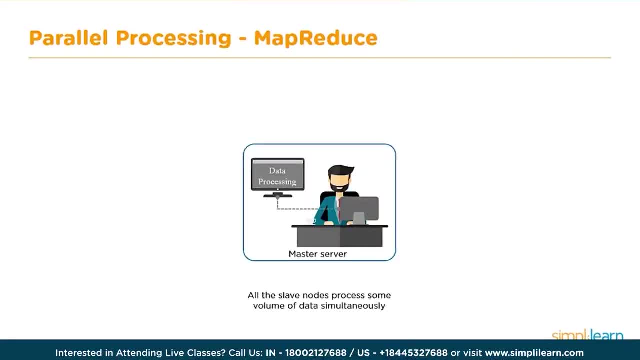 which it can offer. So we know that our data is getting stored across multiple data nodes and you would have huge volume of data which is split and randomly distributed across data nodes, And this is the data which needs to be processed And the best way. 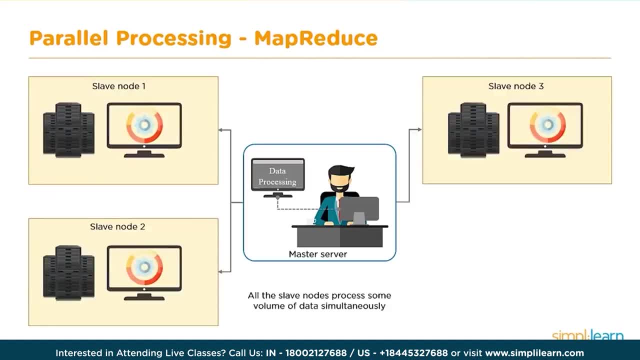 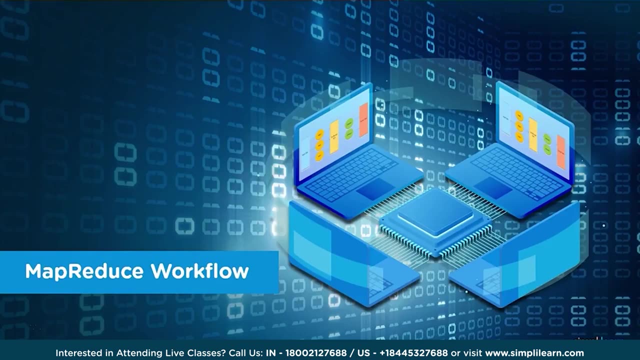 Would be parallel processing, So you could have your data getting stored on multiple data nodes or multiple slave nodes, and each slave node would have again one or multiple disks to process this data. Basically we have to go for parallel processing approach. We have to use the MapReduce. 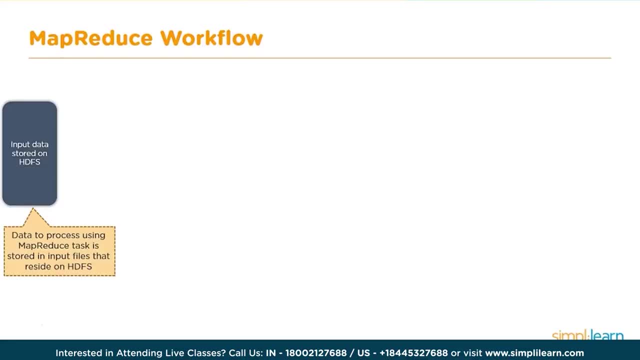 Now let's look at the MapReduce workflow to understand how it works. So, basically, you have your input data stored on HDFS. Now this is the data which needs to be processed. It is stored in input file And the processing which you want can be done on one single file or it can be done on a. 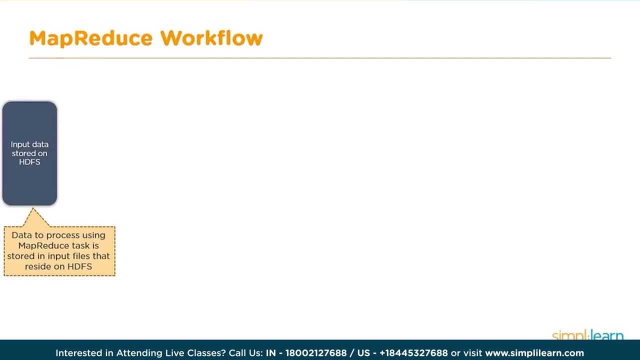 directory which has multiple files. You could also later have multiple outputs merged, which we achieve by using something called as chaining of mappers. So here you have your data getting stored on HDFS Now. input format is basically something to define the input specification and how the 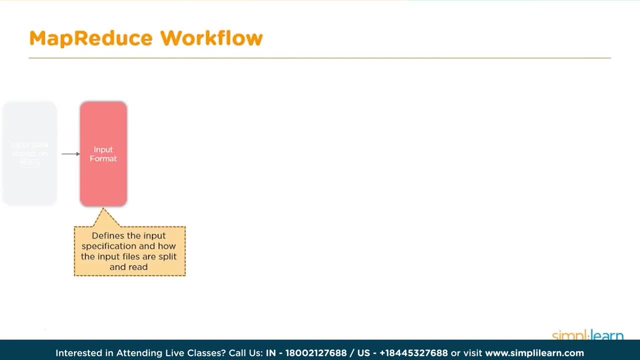 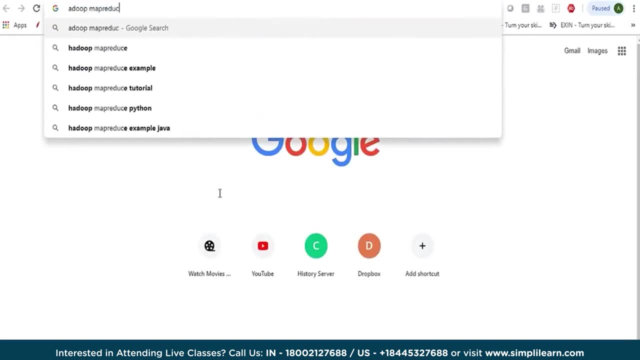 input files will be split, So there are various input formats. Now we can search for that, So we can go to Google and we can basically search for Hadoop, MapReduce, Yahoo tutorial. This is one of the good links And if I look into this link I can search for different input formats and output formats. 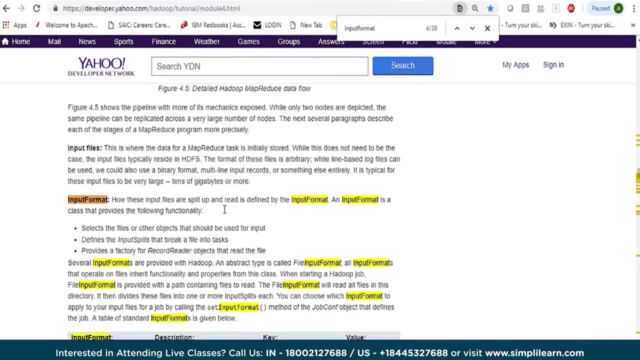 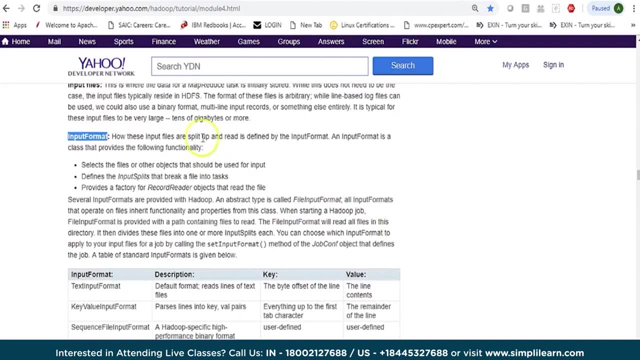 So let's search for input format. So when we talk about input format, you basically have something to define how input files are split. So input files are split up and read based on what input format is. So this is a class that provides following functionality: 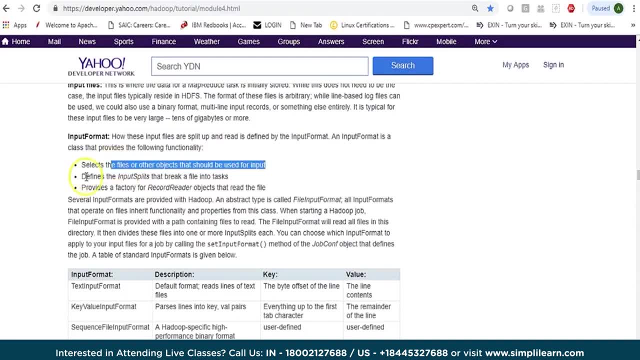 It selects the files or other objects that should be used for input. It defines the input split that break a file into tasks, provides a factory for record reader objects that read the file. So there are different formats if you look in the table here. 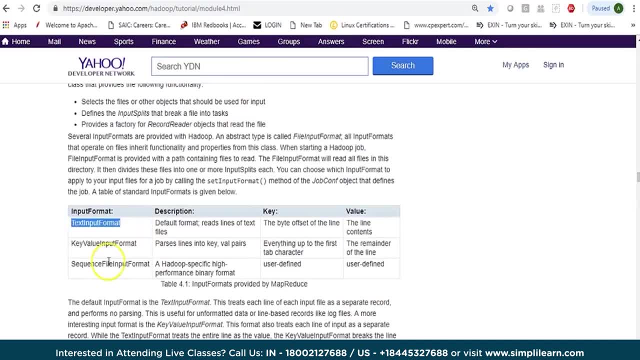 And you can see that the text input format is the default format which reads lines of a text file and each line is considered as a record. Here the key is the byte offset of the line and the value is the line content. It says you can have key value input format which parses lines into key value pairs, everything. 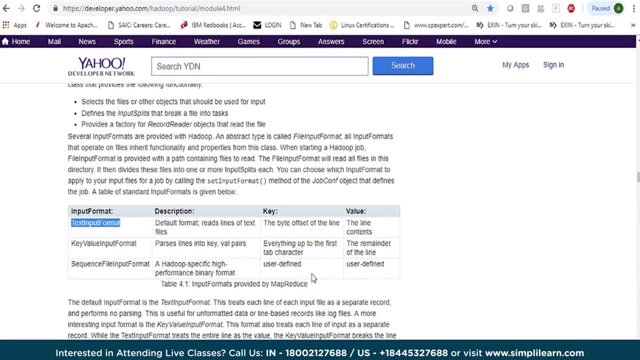 up to the first tab, character is the key and the remainder is the line. You could also have sequence file input format, which basically works on binary format. So you have input format and in the same way you can also search for output format. 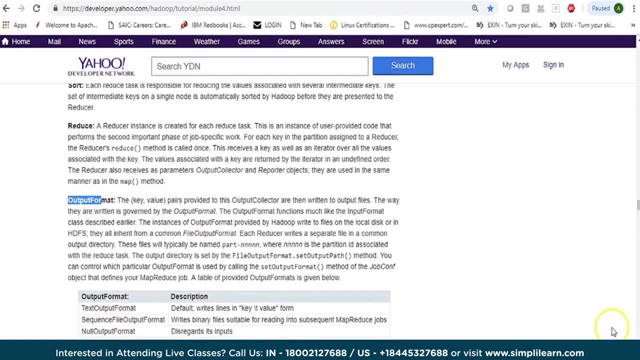 which takes care of how the data is handled after the processing is done. So the key value pairs provided to this output collector Are then written to output files. The way they are written is governed by output format. So it functions pretty much like input format as described in earlier right. 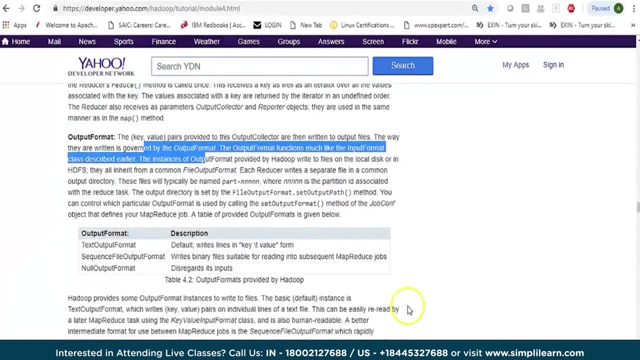 So we could set what is the output format to be followed. And again you have text output sequence, file output format, null output format and so on. So these are different classes which take care of how your data is handled when it is being read. 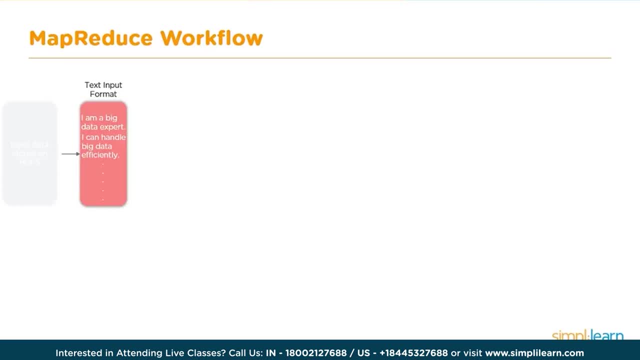 for processing, or how is the data being written when the processing is done. So, based on the input format, the file is broken down into splits and this logically represents the data to be processed by individual map tasks, or you could say individual mapper functions. 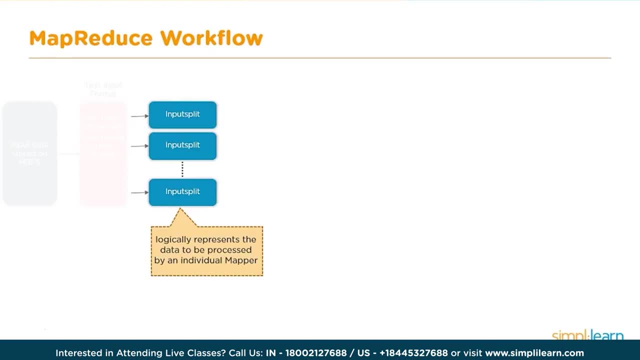 So you could have one or multiple splits which need to be processed, depending on the file size, depending on what properties have been set. Now, once this is done, you have your input splits which are subjected to mapping phase. Internally, you have a record reader. 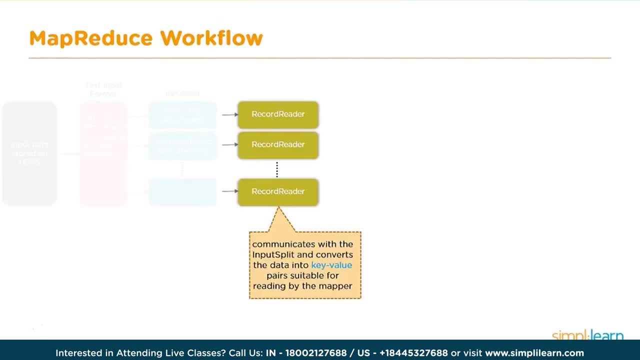 Which communicates with the input split and converts the data into key-value pairs suitable to be read by mapper. And what is mapper doing? It is basically working on these key-value pairs, the map task, giving you an intermittent output which would then be forwarded for further processing. 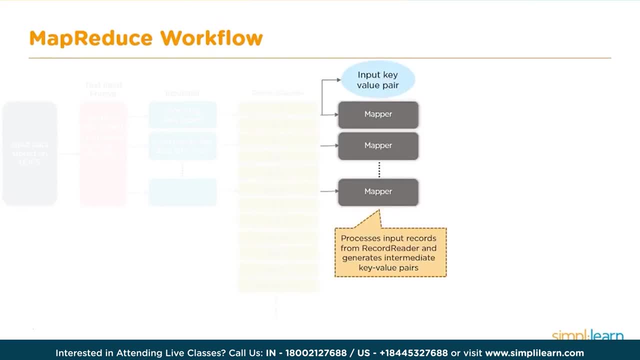 Now, once that is done and we have these key-value pairs, which is being worked upon by map, your map tasks, as a part of your mapper function, are generating your key-value pairs, which are your intermediate outputs to be processed further. Now you could have, as I said, a combiner phase or, internally, a mini-reducer phase. 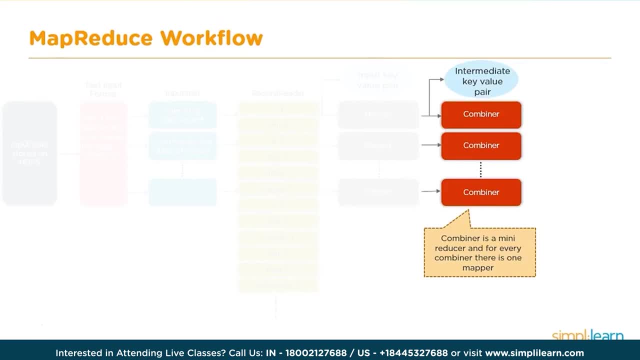 Now combiner does not have its own class. so combiner basically uses the same class as the reducer class provided by the developer and its main work is to do the reducing, or its main work is to do some kind of mini-aggregation on the key-value pairs which were generated. 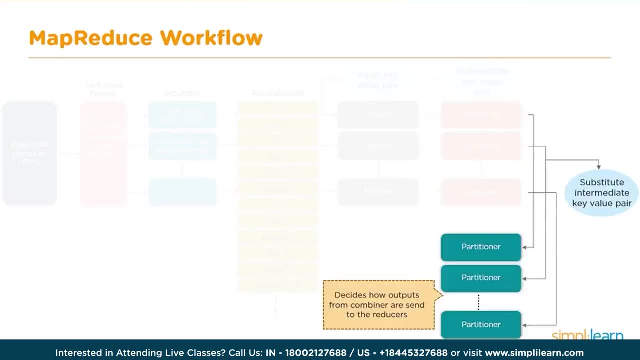 by map. once the data is coming in from the combiner, then we have internally a partitioner phase which decides how outputs from combiners are sent to the reducers. or you could also say that even if i did not have a combiner, partitioner would decide based on the keys and values, based on the type of 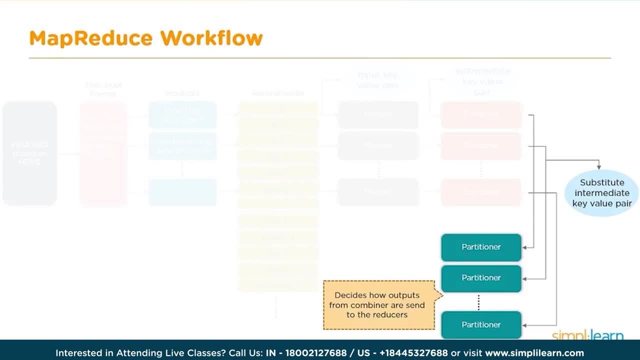 keys, how many reducers would be required or how many reduced tasks would be required to work on your output, which was generated by map task. now, once partitioner has decided that, then your data would be then sorted and shuffled, which is then fed into the reducer. so when you 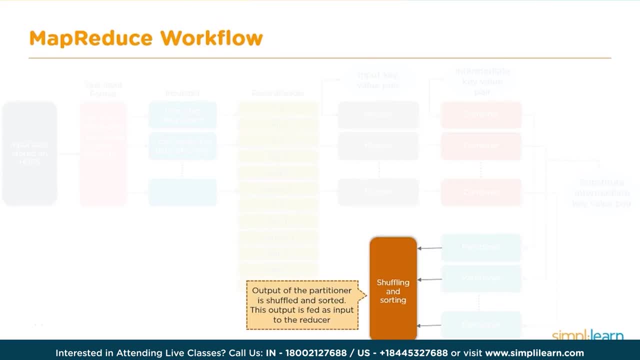 talk about your reducer, it would basically have one or multiple reduced tasks. now that depends on what or what partitioner decided or determined for your data to be processed. it can also depend on the configuration properties which have been set to decide how many reduced tasks should be used now internally. all this data is obviously going. 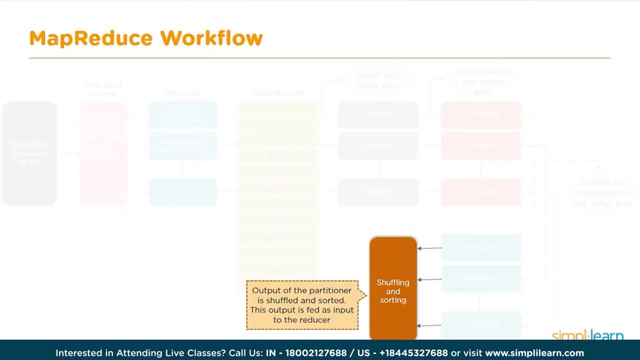 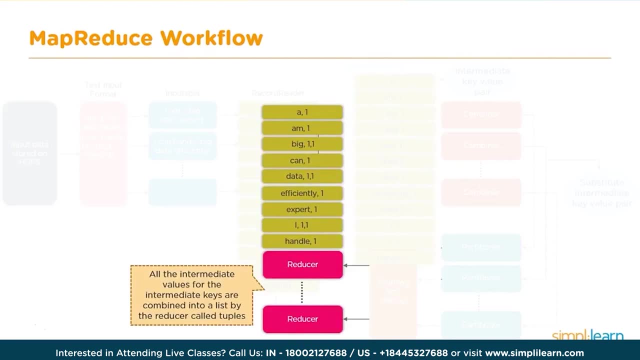 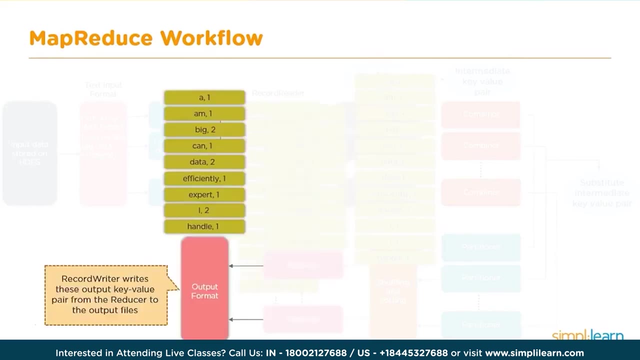 through sorting and shuffling so that your reducing or aggregation becomes an easier task. once we have this done, we basically have the reducer, which is the code for the reducer is provided by the developer, and all the intermediate data has then to be aggregated to give you a final 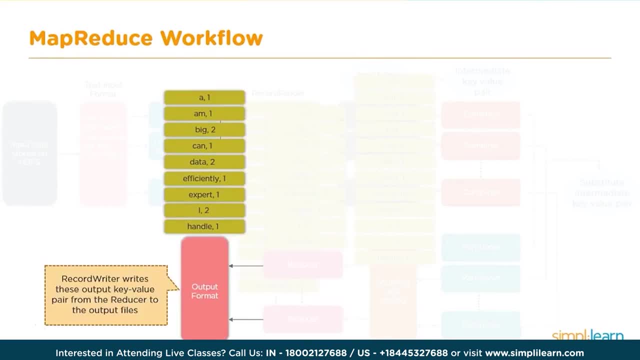 output which would then be stored on sdfs. and who does this? you have an internal record writer which writes the output key value pairs from reducer to the output files. now, this is how your map reduce works, wherein the final output data can be not only stored but then read or accessed from sdfs or. 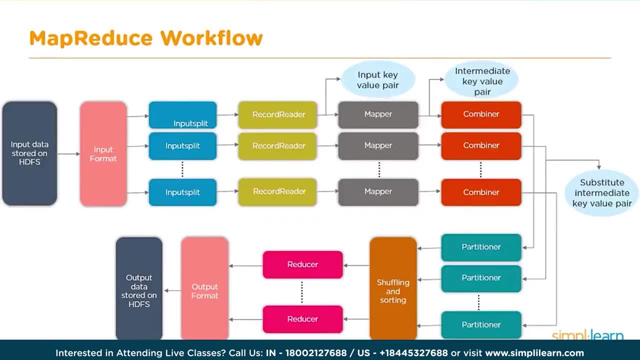 even used as an input for further map reduce kind of processing. so this is how it overall looks. so you basically have your data stored on sdfs based on input format. you have the splits, then you have record reader, which gives your data to the mapping phase, which is then. 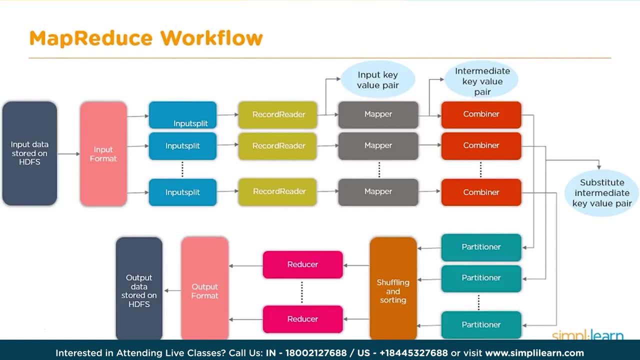 taken care by your mapper function, and mapper function basically means one or multiple map tasks working on your chunks of data. you could have a combiner phase, which is optional, which is not mandatory. then you have a partitioner phase, which decides on how many reduced tasks or how. 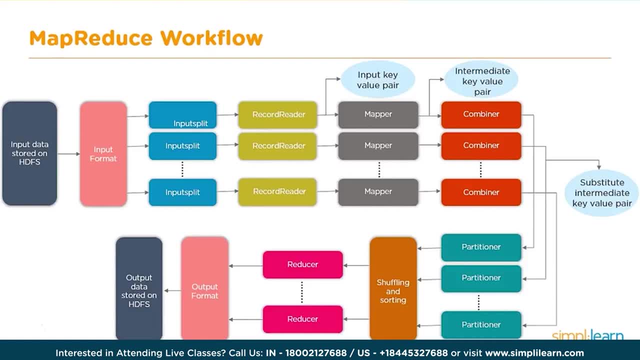 many reducers would be used to work on your data. internally, there is sorting and shuffling of data happening and then, basically, based on your output format, your record reader will write the output to sdfs directory. now, internally, you could also remember that data is being processed locally, so 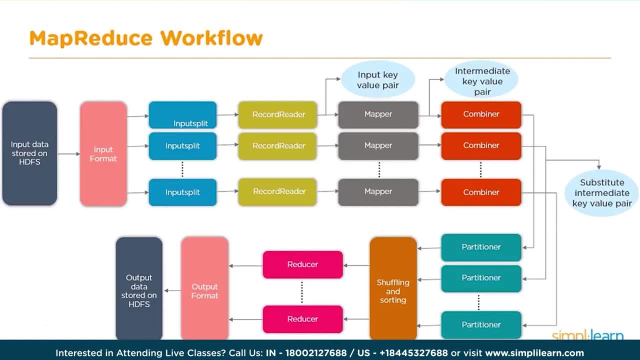 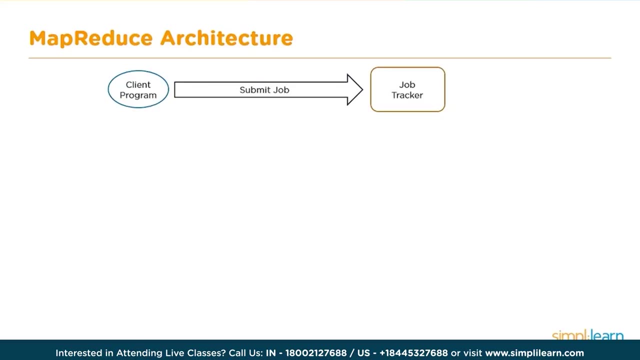 you could have the output of each task which is being worked upon stored locally. however, we do not access the data directly from data nodes. we access it from sdfs, so our output is stored on sdfs. so that is your map. reduce workflow when you talk about map. reduce architecture. now, this is how it. 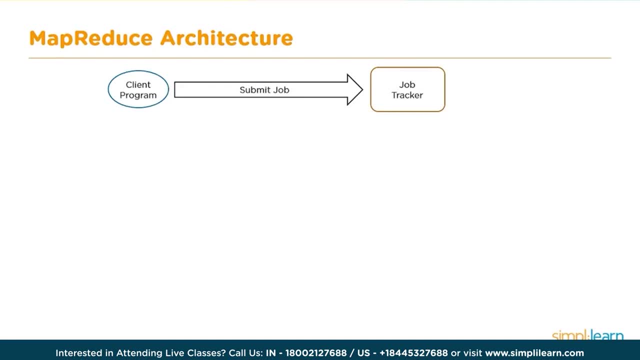 would look so you would have basically a edge node or a client program or an api which intends to process some data, so it submits the job to the job tracker, or you can say resource manager in case of hadoop yarn framework. right now, before this step, we can 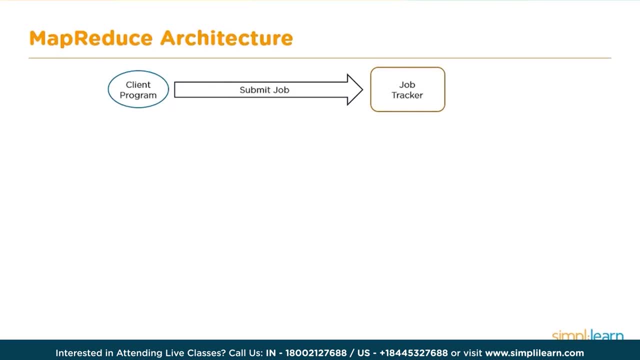 also say that an interaction with name node would have already happened, which would have given information of data nodes which have the relevant data stored, then your master processor. so in hadoop version one we had job tracker and then the slaves were called task trackers. in hadoop version two, instead of job tracker you have resource manager and instead of 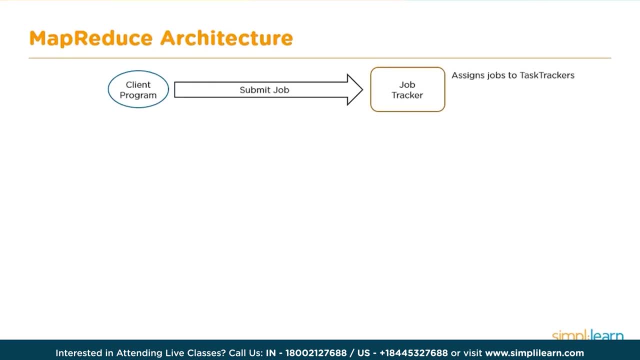 task trackers. you have node managers. so basically your resource manager has to assign the job to the task trackers or node managers. so your node managers, as we discussed in yarn, are basically taking care of processing, which happens on every node. so internally there is all of this work. 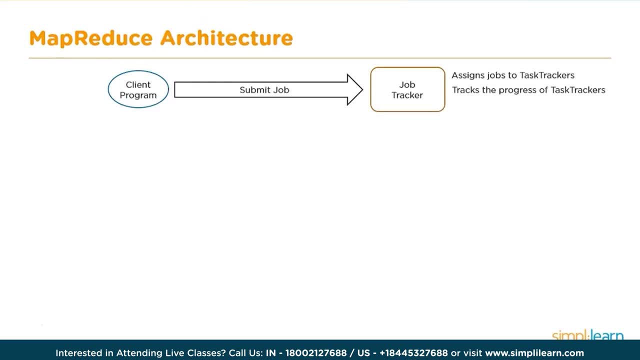 happening by resource manager, node managers and application master, and you can refer to the yarn based tutorial to understand more about that. so here your processing master is basically breaking down the application into tasks. what it does internally is once your application is submitted, your application to be run on yarn processing framework is handled by resource. 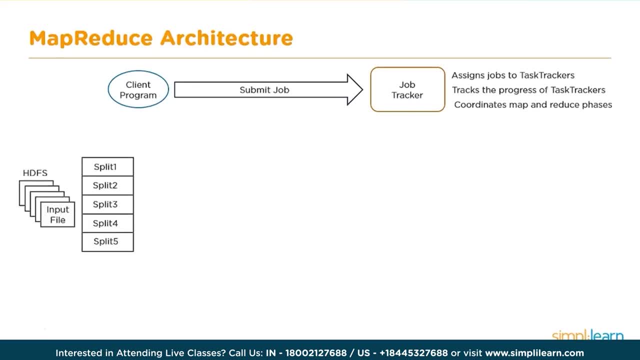 manager, now forget about the yarn part as of now. I mean, who does the negotiating of resources? who allocates them? how does the processing happen on the nodes right? so that's got to do with how yarn handles the processing request. so you have your data, which is stored in. 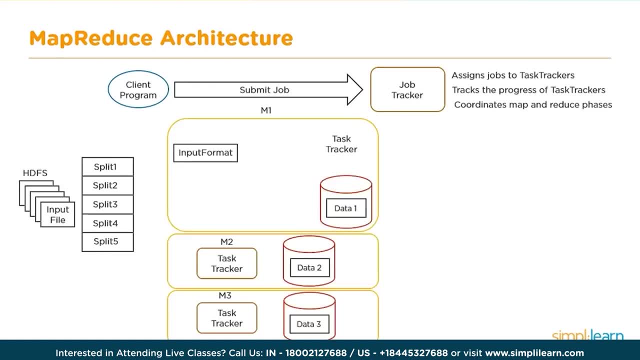 sdfs broken down into one or multiple splits, depending on the input format which has been specified by the developer. your input splits are to be worked upon by your one or multiple map tasks, which will be running within the container, on the nodes. basically, you have the resources which are. 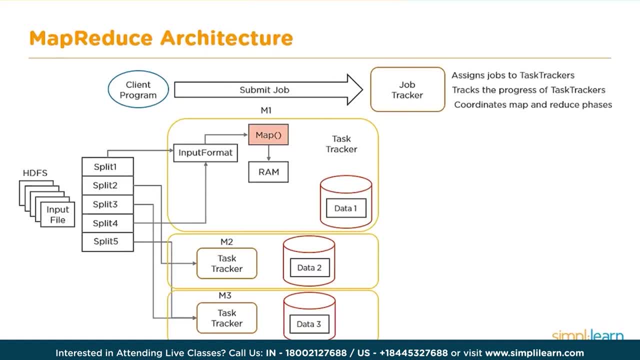 being utilized. so for each map task you would have some amount of RAM which will be utilized, and then further the same data which has to go through reducing phase. that is, your reduced task will also be utilizing some RAM and CPU cores. now, internally you have these functions which take care of deciding on number of reducers, doing a mini reduce and basically. 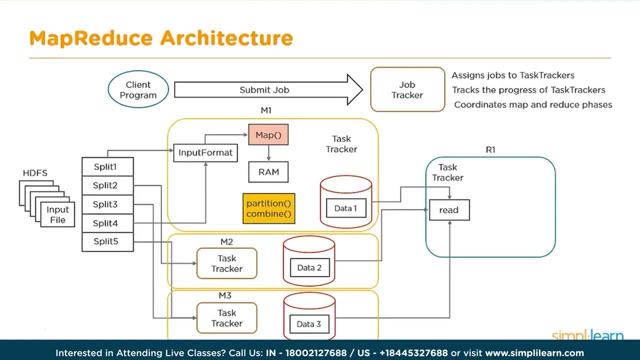 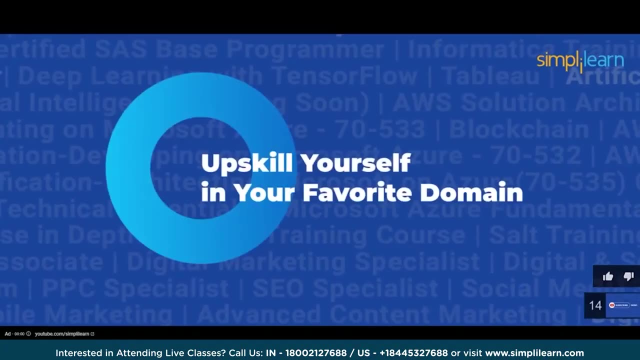 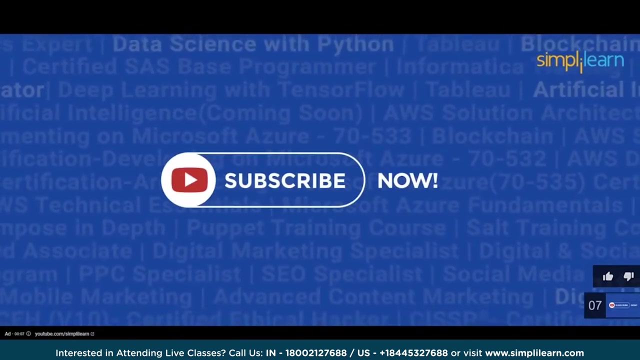 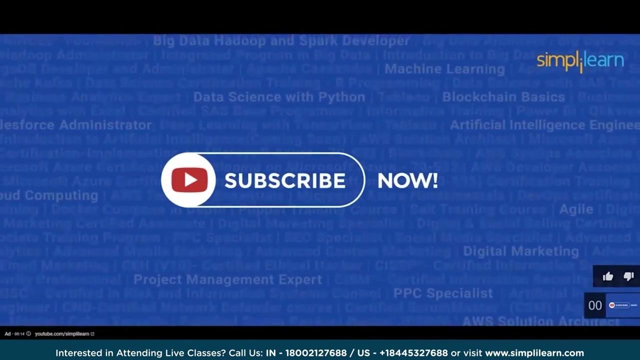 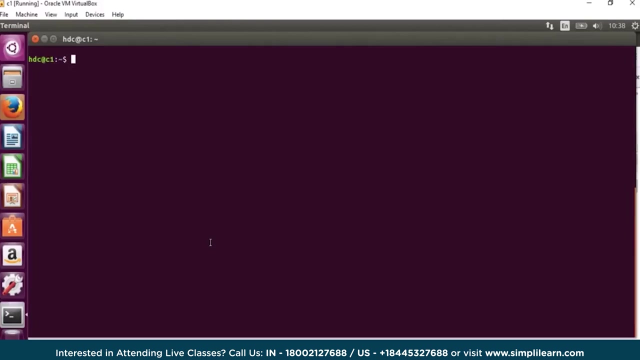 reading and processing the data from multiple data nodes. now this is how your map reduce programming model makes parallel processing work or processes your data, which is stored across multiple machines. finally, you have your output, which is getting stored on sdfs. so let's have a quick demo on map reduce and see how it works on a Hadoop cluster. now we 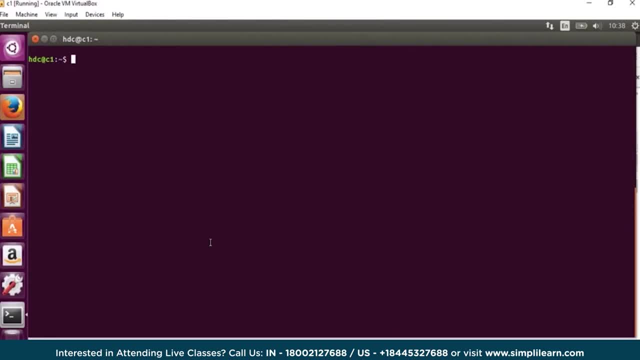 have discussed briefly about map reduce, which contains mainly two phases, that is, your mapping phase and your reducing phase, and mapping phase is taken care by your mapper function and your reducing phase is taken care by your reducer function. now, in between, we also have sorting and shuffling, and then you have other phases, which is partitioner and 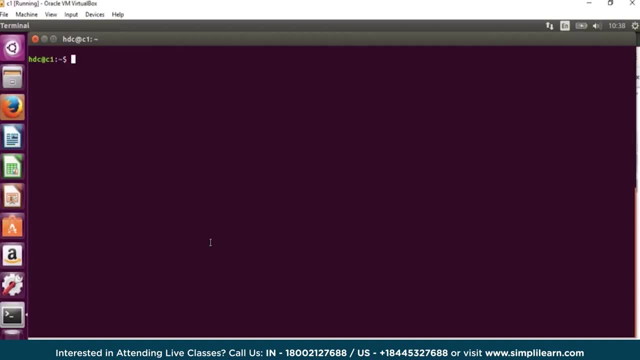 combiner, and we will discuss about all those in detail in later sessions. but let's have a quick demo on how we can run a map reduce which is already existing as a package jar file within your Apache Hadoop cluster or even in your cloud data cluster. now we can. 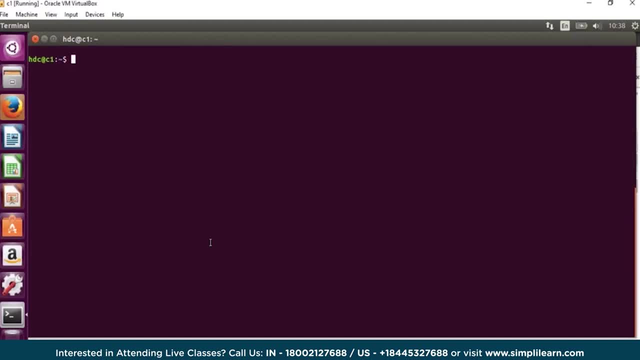 build our own map reduce programs. we can package them as jar, transfer them to the cluster and then run it on a Hadoop cluster on yarn, or we could be using already provided default program. so let's see where they are now. these are my two machines which I have brought up and basically this would have my 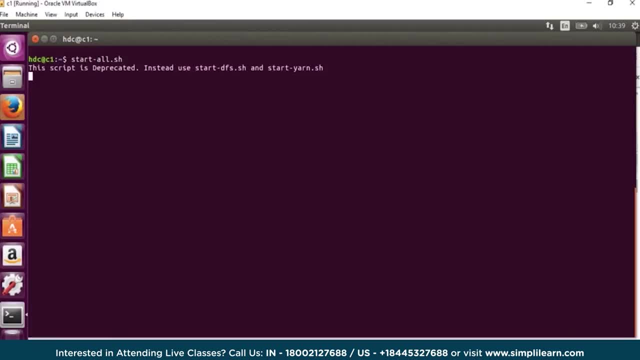 open all dot sh. now I know that this script is deprecated and it says instead use start DFS and start yarn, but then it will still take care of starting off my cluster on these two nodes where I would have one single name node, two data nodes, one secondary name node, one resource manager and 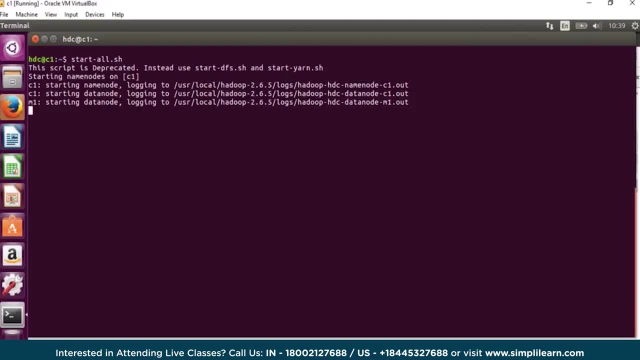 two node managers. now, if you have any doubt in how this cluster came up, you can always look at the previous sessions where we had a walkthrough in setting up a cluster on Apache, and then you could also have your cluster running using less than 3 GB of your total machine. 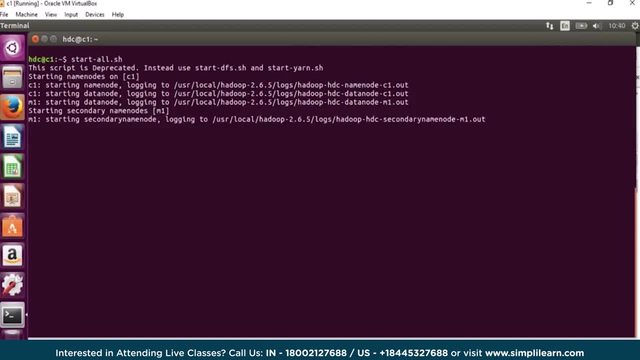 RAM and you could have a Apache cluster running on your machine. now, once this cluster comes up, we will also have a look at the web UI which is available for name node and resource manager. now, based on the settings, what we have given, our UIs will show us details of our cluster, but remember: 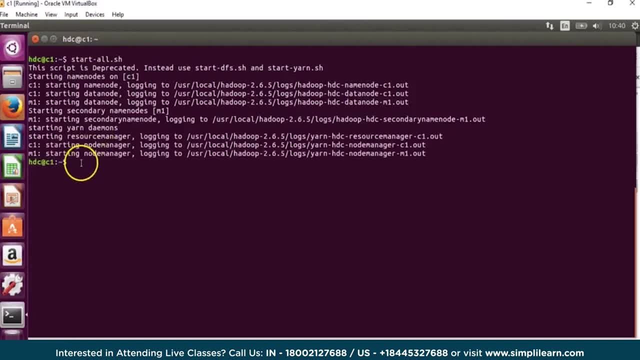 the UI is only to browse. now here my cluster has come up. I can just do a GPS to look at Java related processes and that will show me what are the processes which are running on C1, which is your data node, resource manager, node manager and name node, and on my M1 machine, which is my second machine, which. 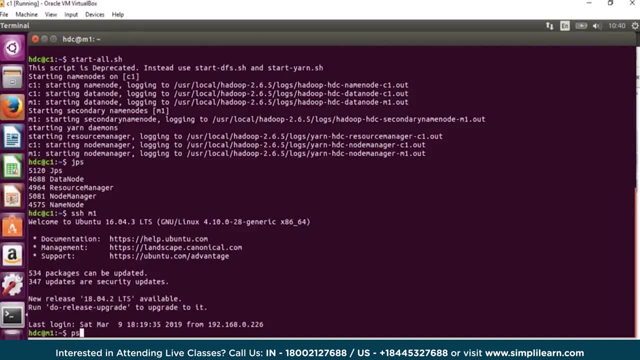 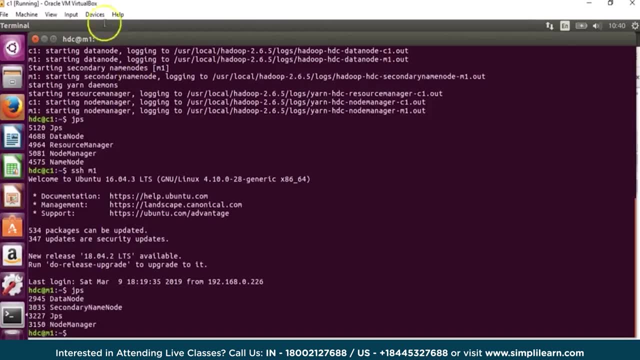 I've configured. here I can always do a JPS and that shows me the processes running, which also means that my cluster is up with two data nodes, with two node managers, and here I can have a look at my web UI. so I can just do a refresh. 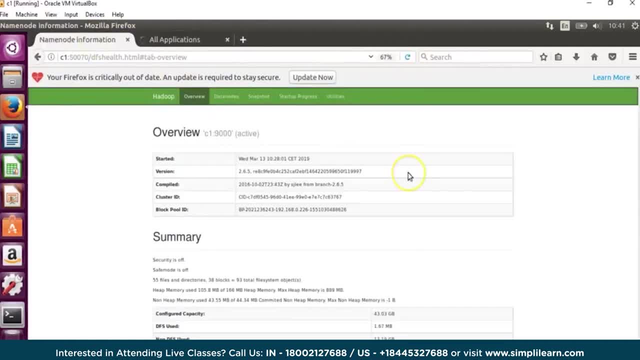 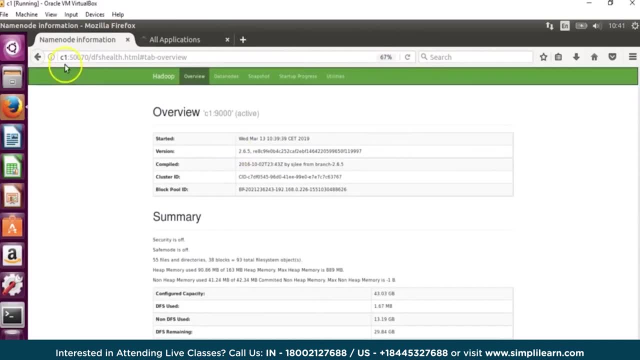 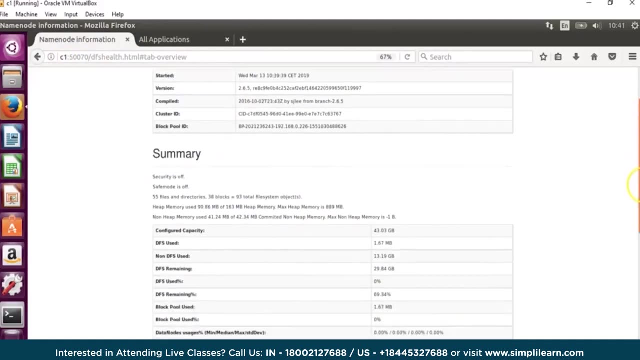 and the same thing with this one. just do a refresh. so I had already opened The Web Pages. so you can always access the web UI using your name, notes, host name and 570 port. it tells me what is my cluster ID, what is my block pool ID. it gives you information of what is the space usage, how. 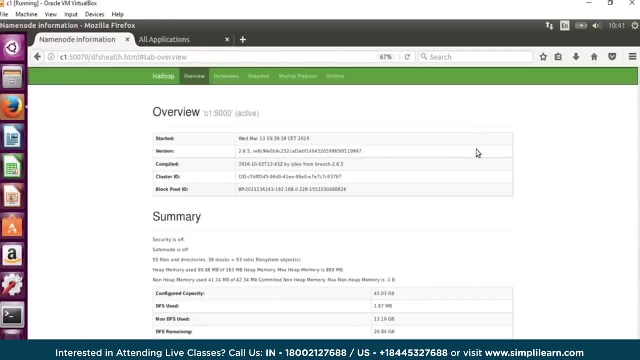 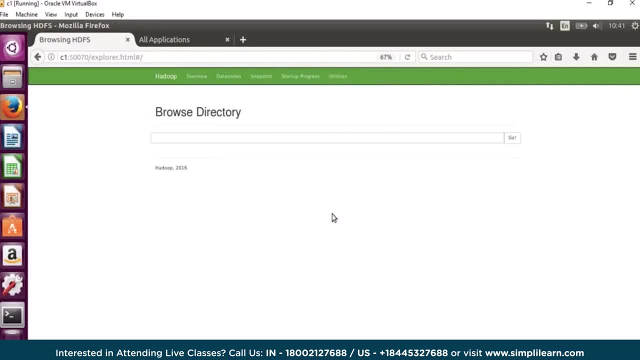 many live notes you have and you can even browse your file system, so I have put in a lot of data here. I can click on browse the file system and this basically shows me multiple directories, and these directories have one or multiple files which we will use for our MapReduce example. Now 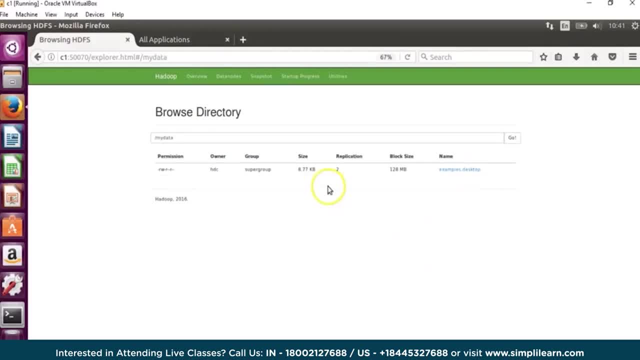 if you see, here these are my directories which have some sample files, Although these files are very small, like 8.7 kilobytes. If you look into this directory, if you look into this, I have just pulled in some of my Hadoop logs and I have put it on my SDFS. These are a little bigger files. 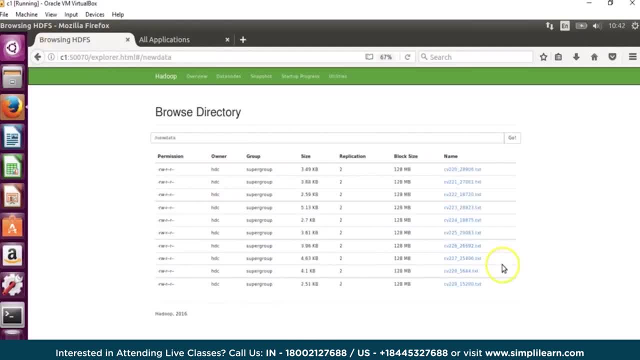 and then we also have some other data which we can see here, and this is data which I've downloaded from web. Now we can either run a MapReduce on a single file or in a directory which contains multiple files. Let's look at that before looking at demo on MapReduce. Also remember MapReduce. 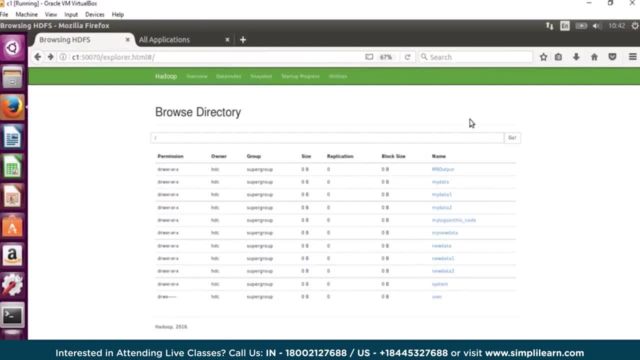 will create a output directory and we need to have that directory created. plus, we need to have the permissions to run the MapReduce job. So by default, since I'm running it using admin ID, I should not have any problem. but then if you intend to run MapReduce with a different user, 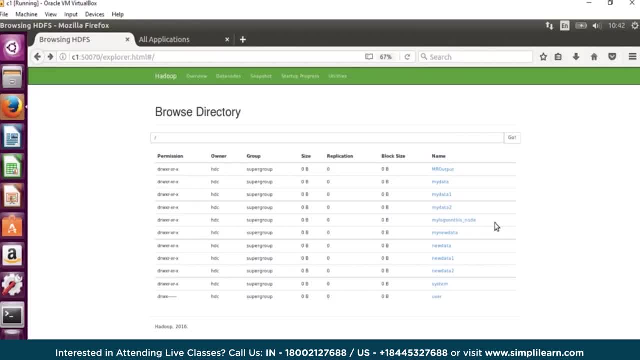 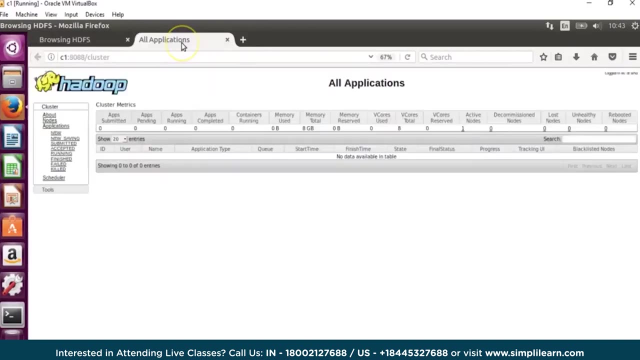 then obviously you will have to ask the admin or you will have to give the user permission to read and write from SDFS. So this is the directory which I've created, which will contain my output once the MapReduce job finishes, and this is my cluster file system, If you look on this UI. 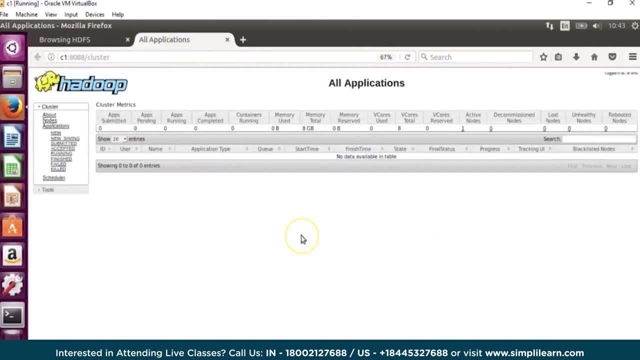 this shows me about my yarn, which is available for taking care of my any processing. It, as of now, shows that I have total of 8 GB memory and I have 8 V cores. Now that can be depending on what configuration we have set or how many nodes are available. 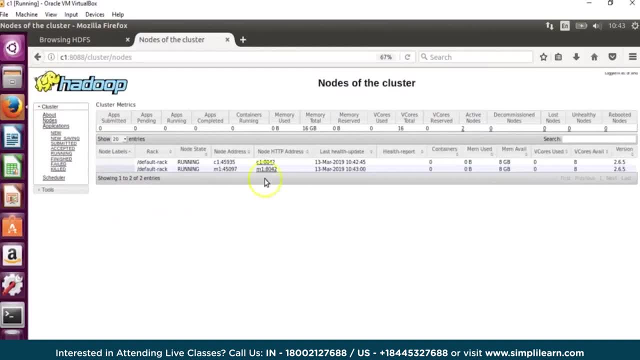 We can look at nodes which are available, and that shows me. I have two node managers running. each has 8 GB memory and 8 V cores. Now, that's not true, actually, but then we have not set the configurations for node managers and that's why it takes the default properties. 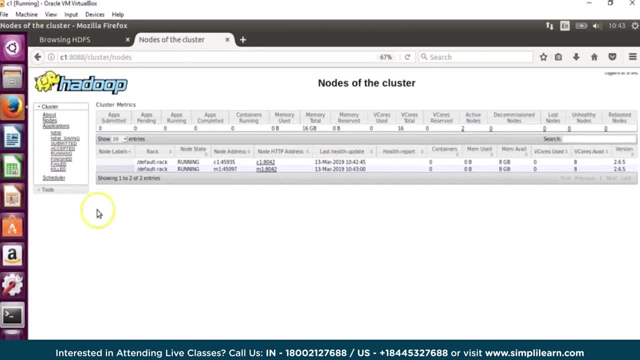 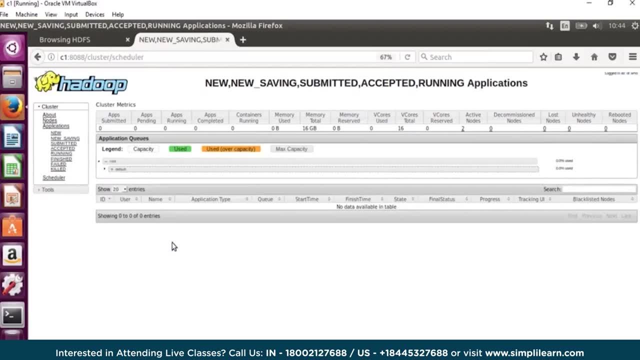 that is, 8 GB RAM and 8 V cores. Now this is my yarn UI. We can also look at scheduler, which basically shows me the different queues, if they have been configured, where you will have to run the jobs. We'll discuss about all these in later in detail. Now let's go back to our terminal and 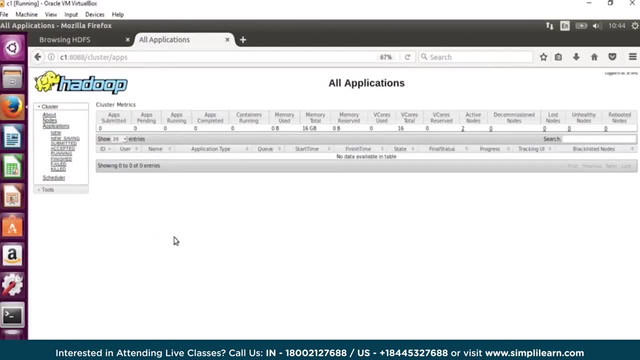 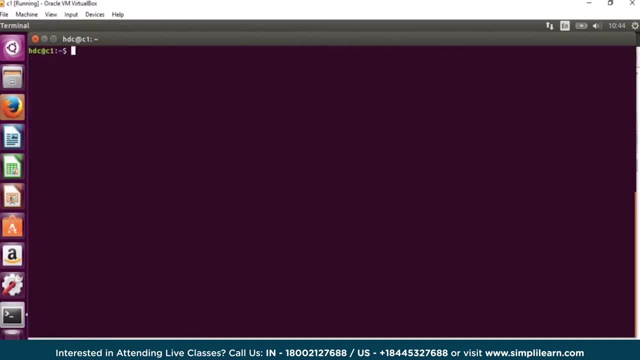 let's see where we can find some sample applications which we can run on the cluster. So once I go to the terminal I can well submit the MapReduce job from any terminal. Now here, I know that my Hadoop related directory is here and within Hadoop you have various directories We have discussed 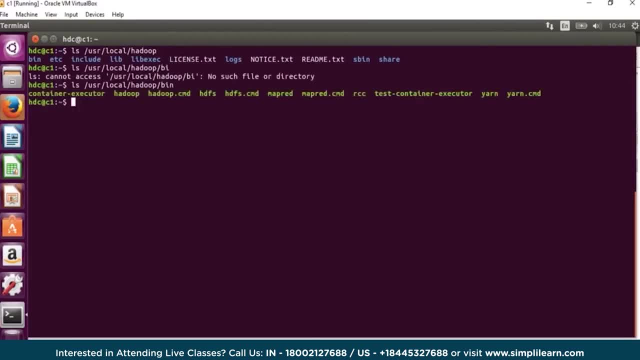 that in binaries you have the commands which you can run. In Sbin you basically have the startup scripts and here you also notice there is a share directory in the end. If you look in the share directory you would find Hadoop, and within Hadoop you have various sub directories in which we will 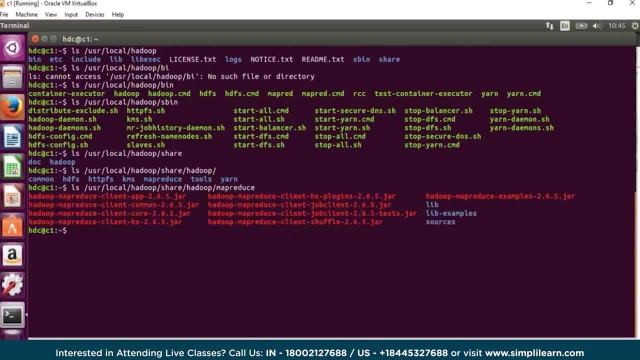 look for MapReduce Now. this MapReduce directory has some sample jar files which we can use to run a MapReduce on the cluster. Similarly, if you are working on a Cloudera cluster, you would have to go into opt cloudera parcel cdh slash lib and in that you 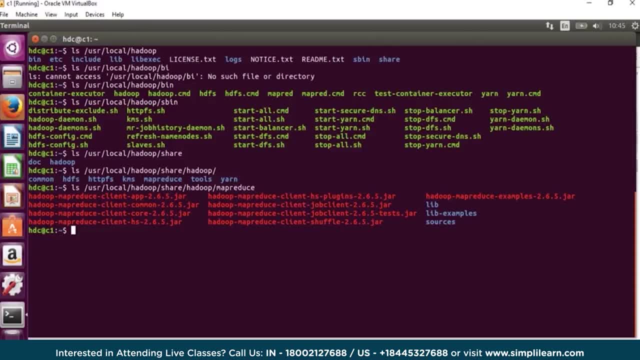 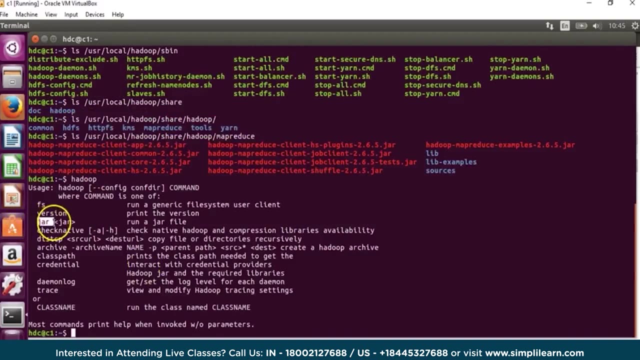 would have directories for HDFS MapReduce or HDFS yarn where you can still find the same jars. It is basically a package which contains your multiple applications. Now how do we run a MapReduce? We have an option called jar which can be used to run a jar file Now at any point of time, if you would. 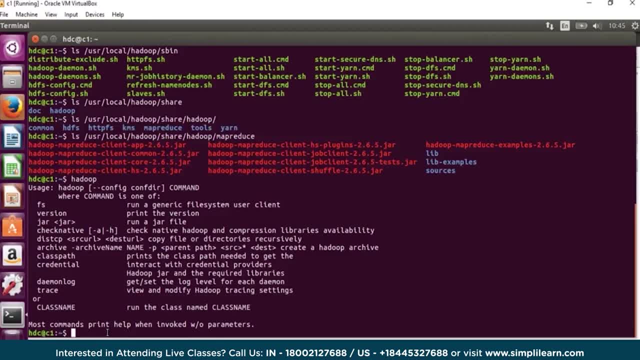 want to see what are the different classes which are available in a particular jar. you could always do a jar minus xvf, For example, I could say jar xvf and I could say user local Hadoop, share, Hadoop, MapReduce and then list down your jar file. So I'll say: 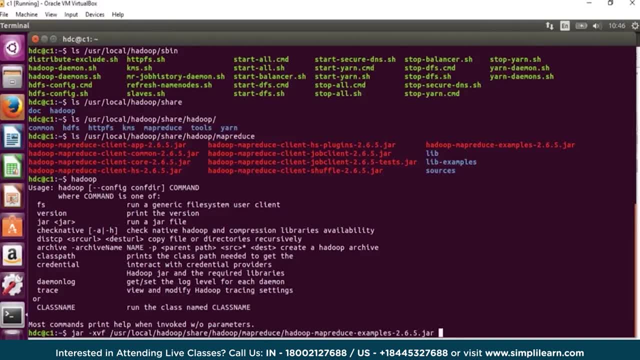 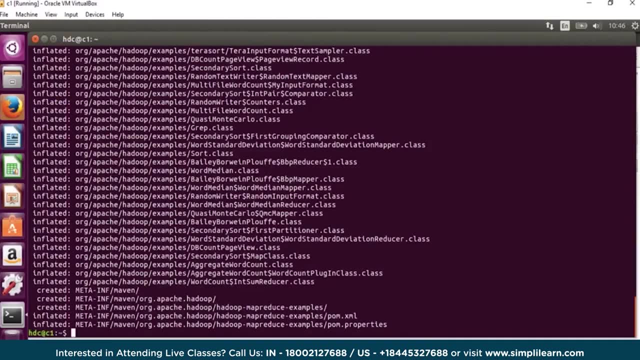 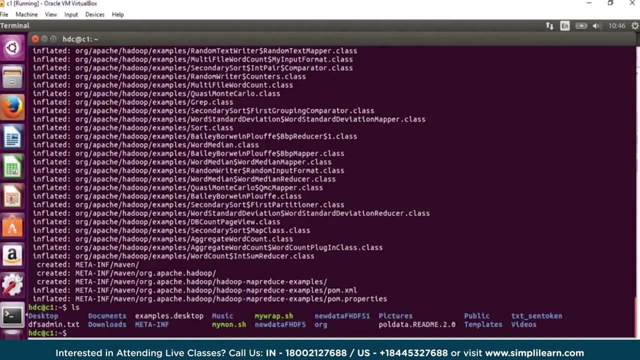 Hadoop, MapReduce examples. and if I do this, this should basically unpack it to show me what classes are available within this particular jar. and it has done this. It has created a meta file and it has created a org directory. We can see that by doing a ls and here if you look in ls org, since 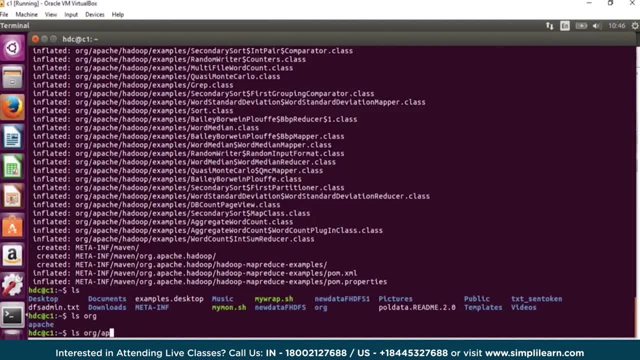 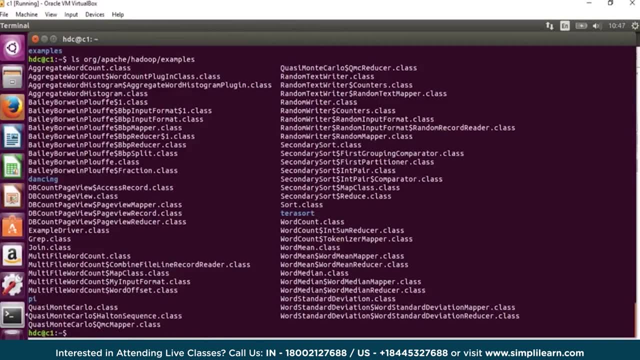 I ran the command from a phone directory. I can look into org patchy Hadoop examples, which shows me the classes which I have and those classes which I have and those classes which I have contain which mapper or reducer classes. So it might not be just mapper and reducer but you can. 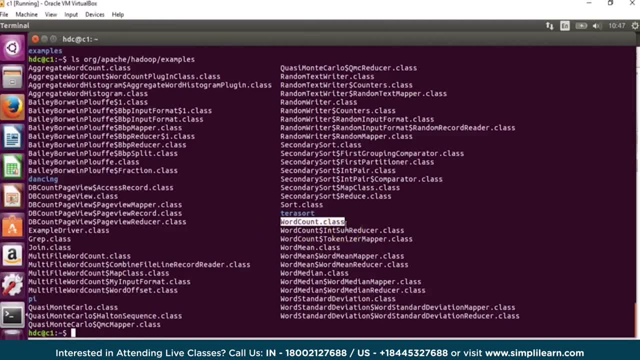 always have a look. So, for example, I am targeting to use word count program which does a word count on files and gives me a list of words and how many times they occur in a particular file or in set of files, and this shows me that what are the classes which belong to word count. So we have a int sum. 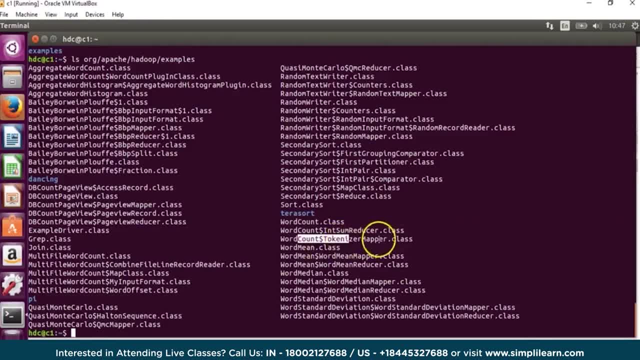 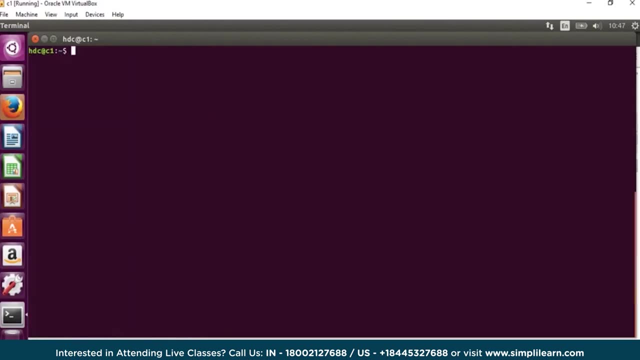 reducer. So this is my reducer class. I have tokenizer mapper. that is my mapper class, right, And basically this is what is used. These classes are used if you run a word count. Now there are many other programs which are part of this jar file and we can expand and see that. So I can say: 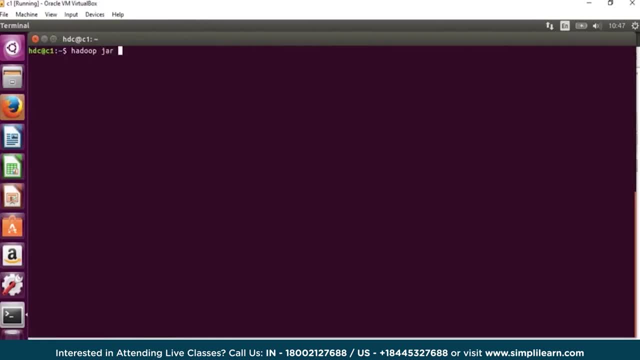 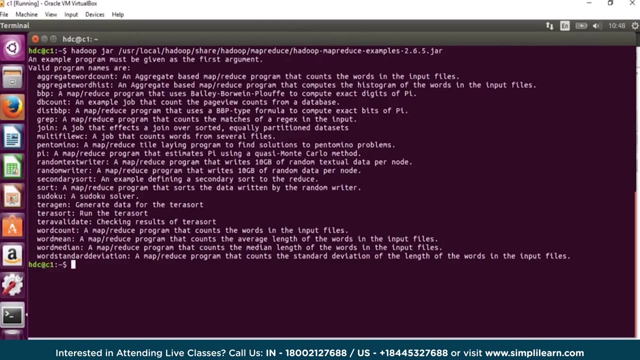 Hadoop jar and give your path. So I'll say: Hadoop jar user: local Hadoop. share Hadoop map: reduce Hadoop map. reduce examples and if I hit on enter, that will show me what are the inbuilt classes which are already available Now. these are certain things which we can use Now. there are other jar files also. For example, I can: 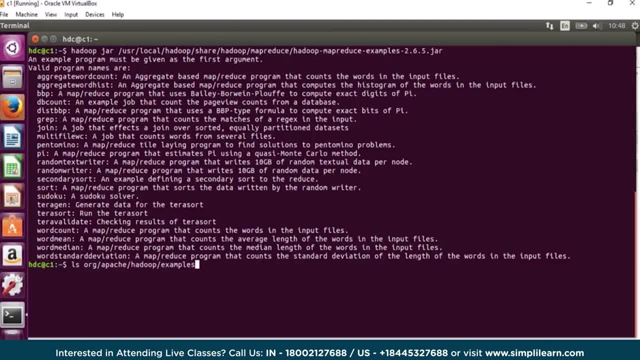 look at Hadoop, and here we can look at the jar files which we have in this particular path. So this is one Hadoop map reduce examples which you can use. You can always look in other jar files, like you can look for Hadoop map reduce client, job, client, and then you can look at the test one. So that is also. 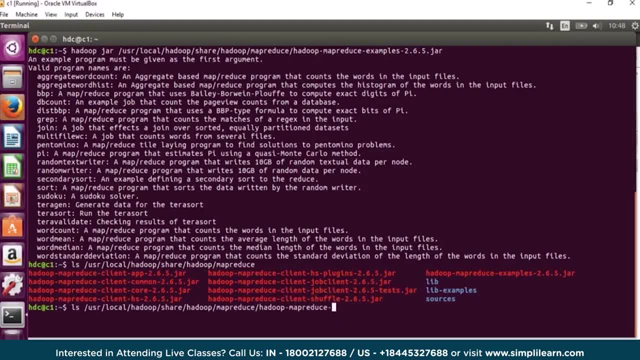 an interesting one So you can always look into it. Hadoop map: reduce client, job, client and then you have something ending with this. So if I would have tried this one using my Hadoop jar command- So in my previous example when we did this, it was showing: 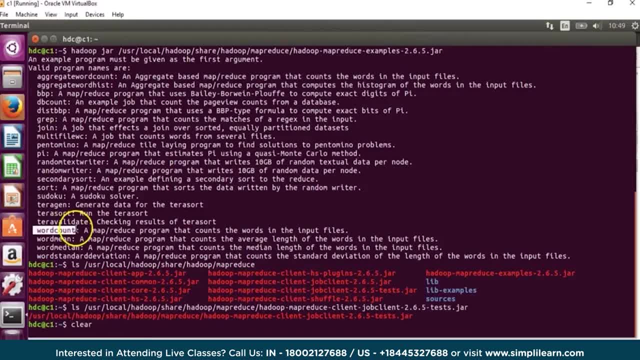 me all the classes which are available, and that already has a word count. Now there are other good programs which you can try, like TerraGen to generate dummy data, TerraSort to check your sorting performance and so on, and TerraValidate to validate the results. Similarly, we can also 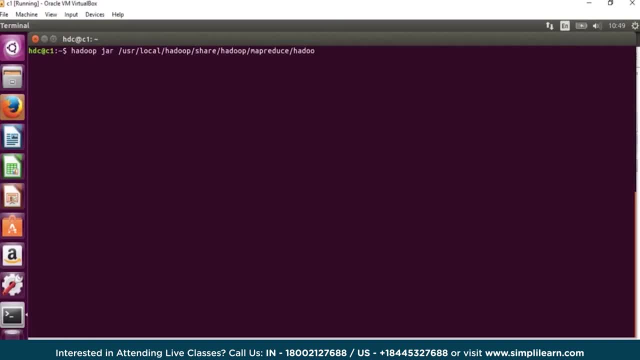 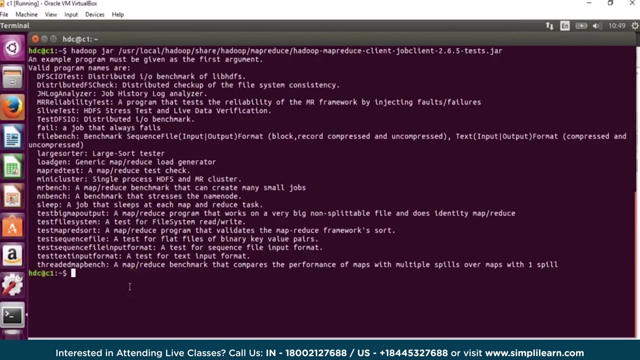 do a Hadoop jar, as I said on Hadoop map reduce- I think that was client- and then we have job client and then test jar. Now this has a lot of other classes which can be used or programs which can be used for doing a stress testing or checking your cluster status and so on. One of them: 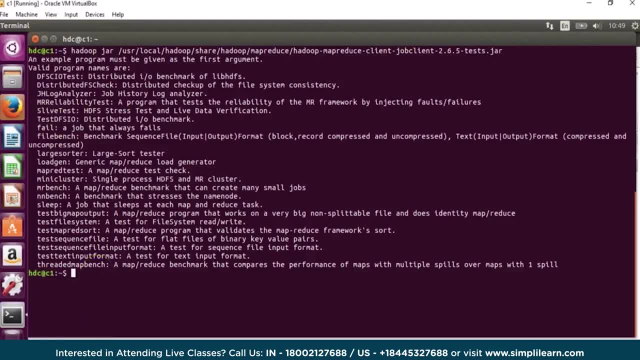 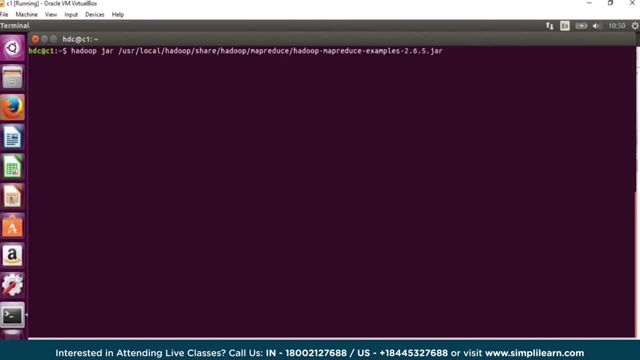 interesting one is test the FSIO. But let's not get into all the details. in first instance Let's run a map. reduce Hadoop work is running now as standard. Let's see what we are getting now. I just want to show that. 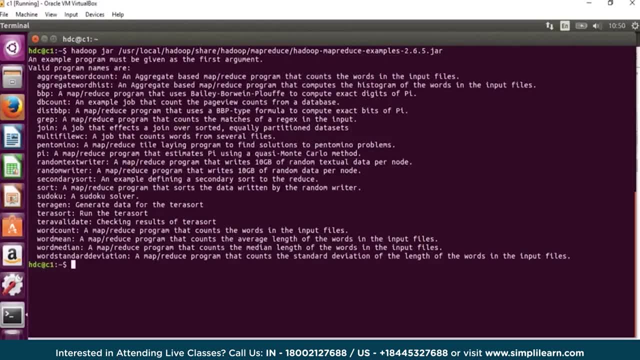 you actually need to give Hadoop jar and then my jar file and if I hit on enter it would say it needs the input and output. It needs which class you want to run. So for example, I would say word count and again if I hit on enter it tells me that you need to give me some input and output to. 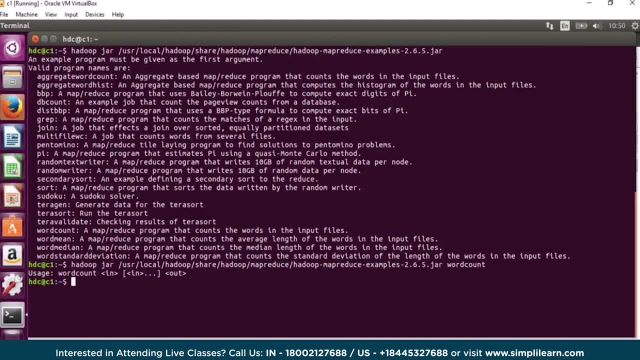 process And obviously this processing will be happening on cluster. that is our yarn processing framework, unless and until you would want to run this job in a local mode in a local mode, but let's first try how it runs on the cluster. so how do we do that? now, here i can. 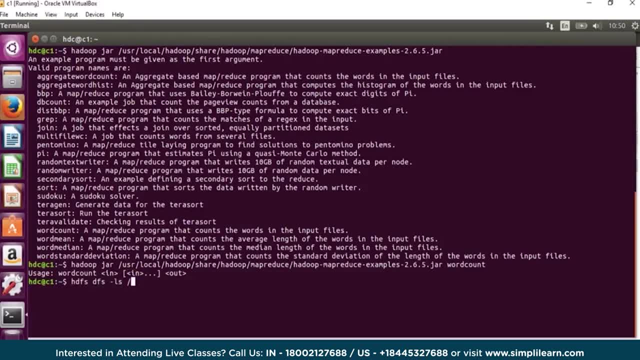 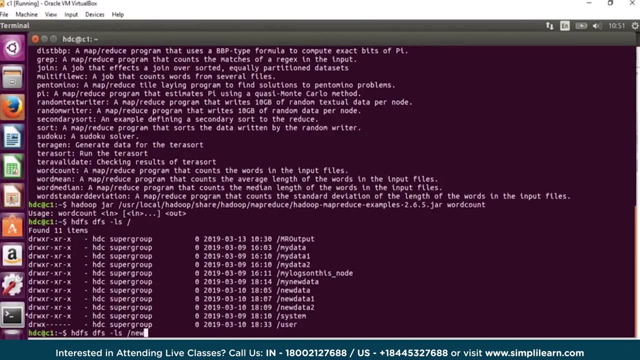 do a hdfs ls slash command to see what i have on my hdfs now through my ui. i was already showing you that we have set of files and directories which we can use to process. now we can take up one single file. so, for example, if i pick up new data and i can look into the files here, what we 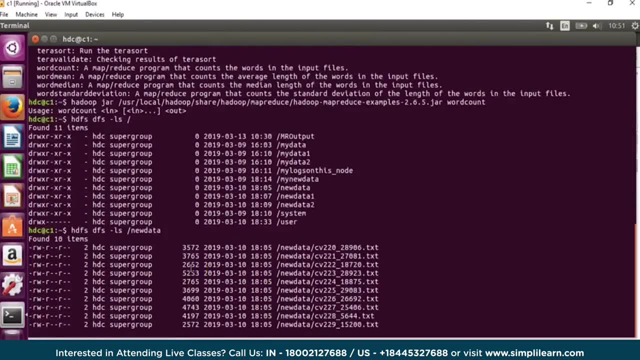 have and we can basically run a map reduce on a single file or multiple files. so let's take this file, whatever that contains, and i would like to do a word count so that i get a list of words and their occurrence in this file. so let me just copy this now. i also need my output to be written and 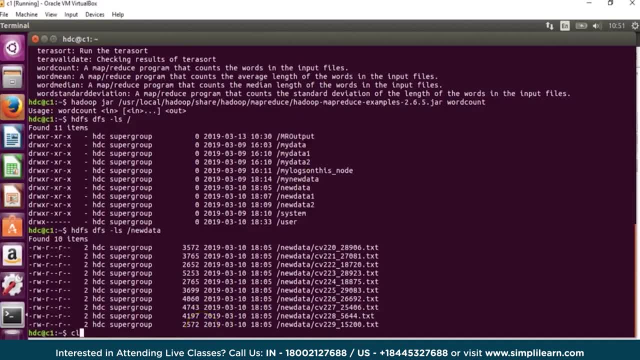 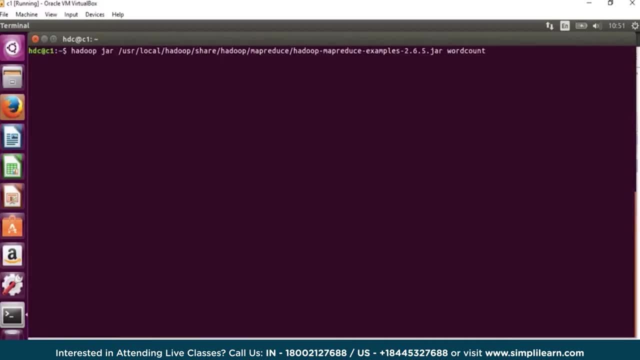 that will be written here. so here, if i want to run a map reduce, i can say hadoop, which we can pull out from history, so hadoop, jar word count. now i need to give my input so that will be new data and then i will give this file which we just 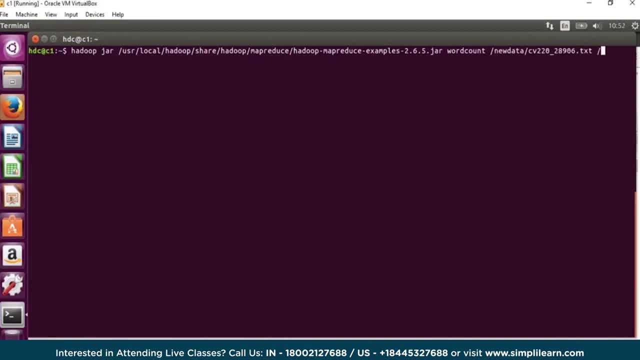 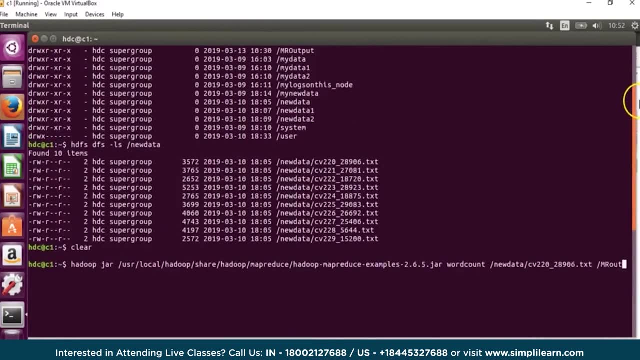 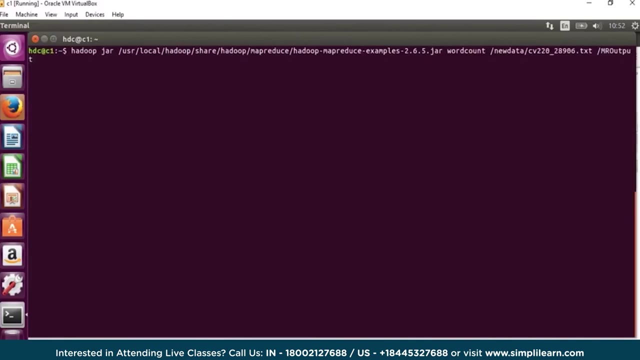 copied. now i am going to run the word count on you on a single file and i will basically have my output, which will be stored in this directory, the directory which i have created already, mr output. so let's do this output, and this is fair enough. now you can give many other properties. 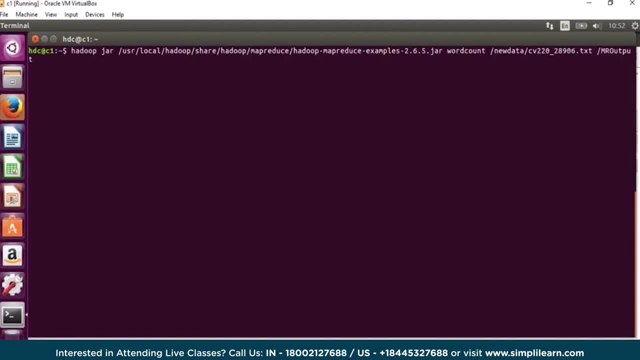 you can specify how many map jobs you want to run, how many reduce jobs you want to run, do you want your output to be compressed, do you want your output to be merged, or many other properties can be defined when you are specifying word count and then you can pass in an argument to pass properties from the command line which will 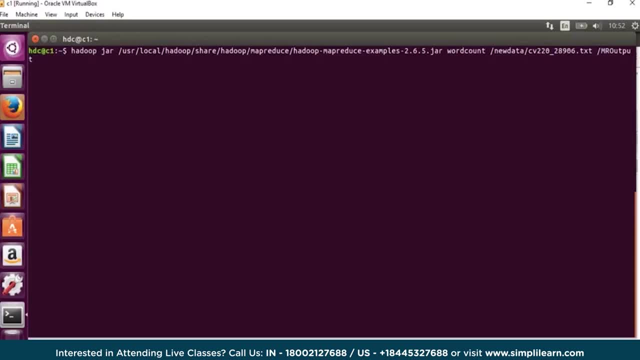 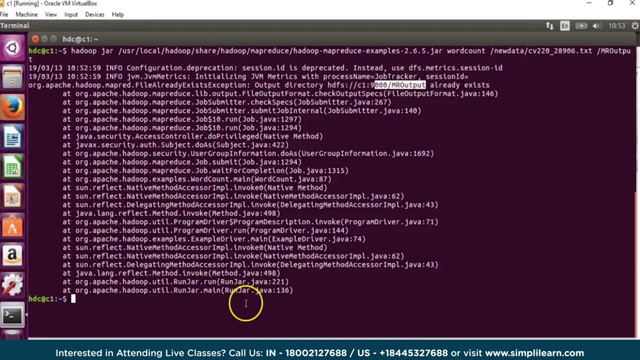 affect your output now once i go ahead and submit this. this is basically running a simple inbuilt map reduce job on our hadoop cluster. now, obviously, internally it will be looking for name node. now we have some issue here and it says the output already exists. what does that mean? so it basically means 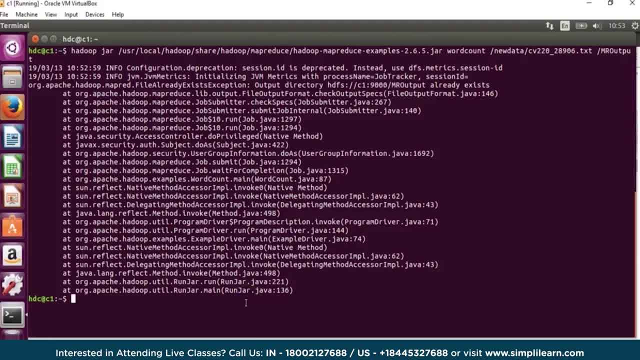 that hadoop will create an output for you. you just need to give a name, but then you don't need to create it. so let's give, let's append the output with number one, and then let's go ahead and run this. so i've submitted this command. now. this can also be run in background, if you would want to run. 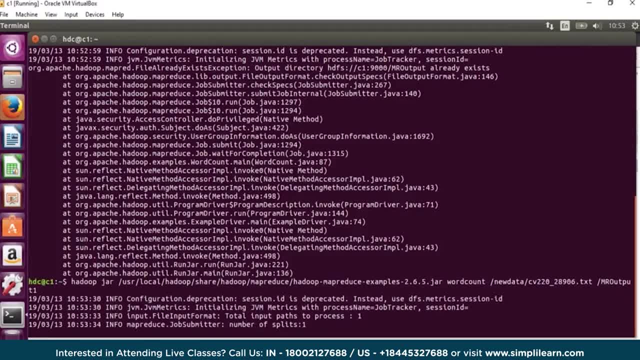 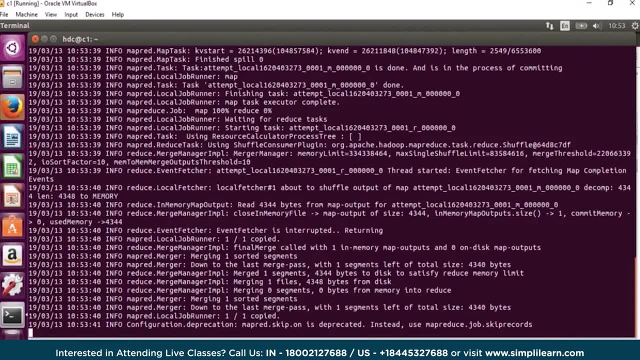 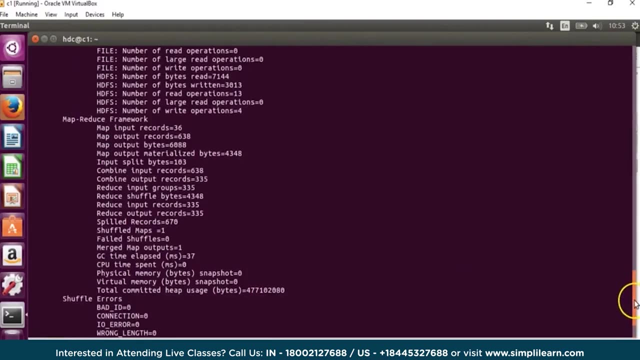 multiple jobs on your cluster at the same time, so it takes total input paths to processes one. so that is, there is only one right on which your job has to work. now it will internally try to contact your resource manager and basically this is done. so here we can have a look and we can see some counters here. now what I 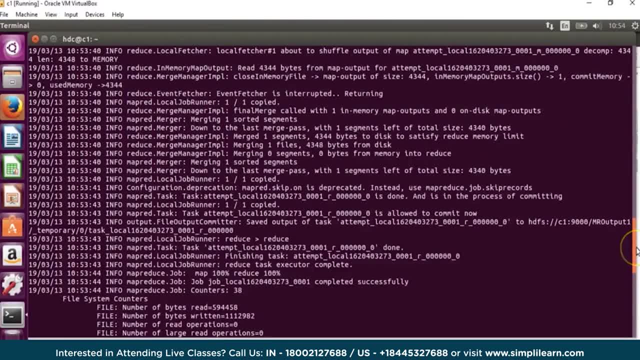 also see is for some property which it is missing. it has run the job but it has run in a local mode. it has run in a local mode so although we have submitted so, this might be related to my yarn settings and we can check that. so if I do a 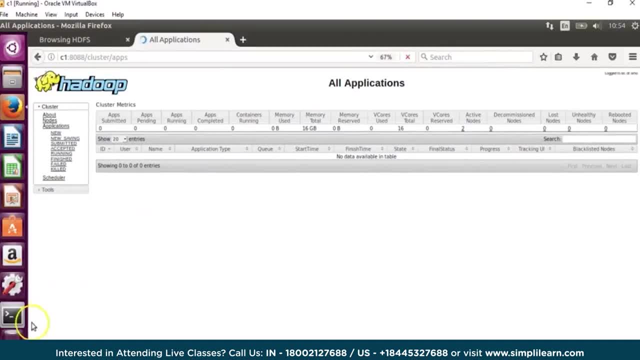 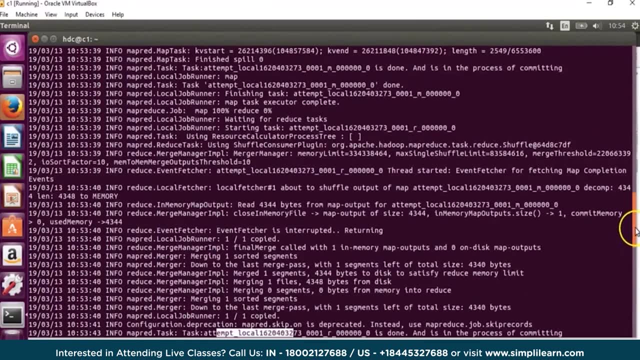 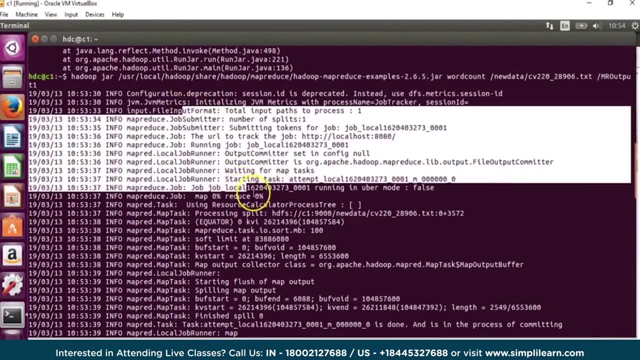 refresh when I have run my application. it has completed. it would have created an output, but the only thing is it did not interact with your yarn. it did not interact with your resource manager. we can check those properties and here, if we look into the job, it basically tells me that 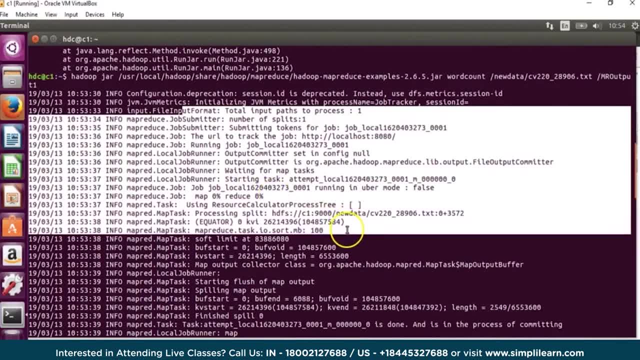 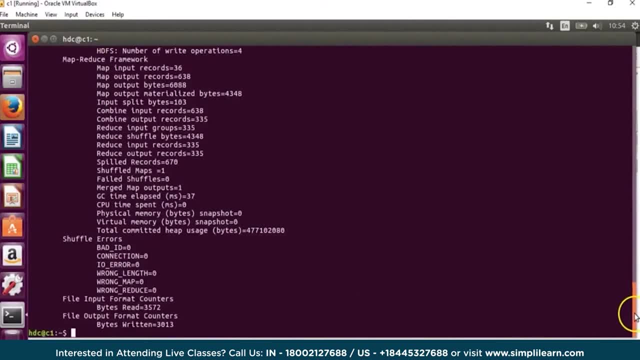 it went for mapping and reducing, it would have created an output. it worked on my file, but then it ran in a local mode. it ran in a local mode. so map reduce, remember, is a programming model. right now, if you run it on yarn, you get the facilities of running it on a cluster where 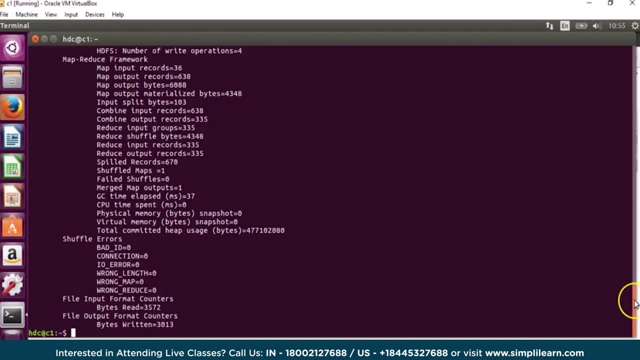 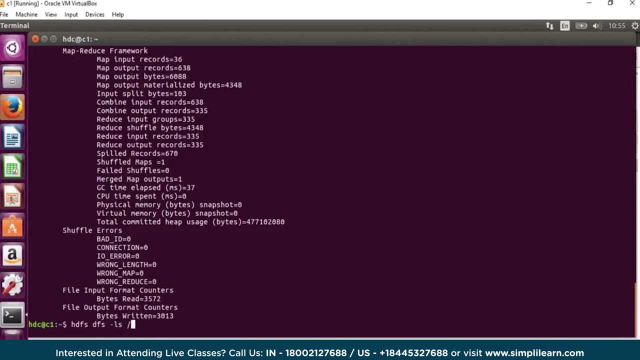 yarn takes care of resource management. if you don't run it on yarn and run it on a local mode, it will use your machine's RAM and CPU cores for processing, but then we can quickly look at the output and then we can also try running this on yarn. so if I look into my HDFS and if I look into 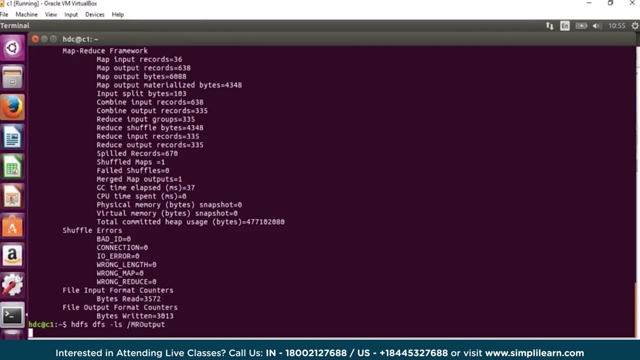 my output: M R output. that's the directory which was not used. actually, let's look into the other directory, which is ending with one, and that should show me the output created by this map reduce. although it ran in the local mode, it fetched an input file from your HDFS. 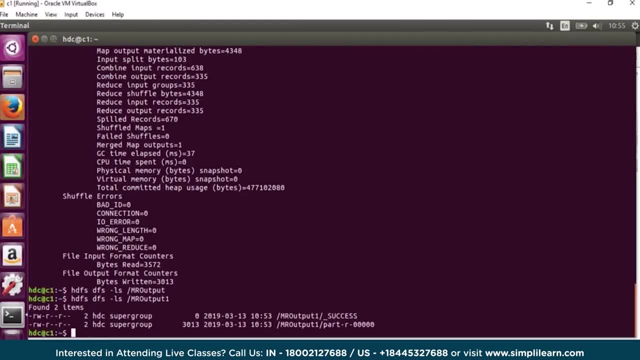 and it would have created output in HDFS. now that's my part file which is created and if you look at part minus R, minus these zeros, if you would have more than one reducer running, then you would have multiple such files created. we can look into this. what does this file contain which would 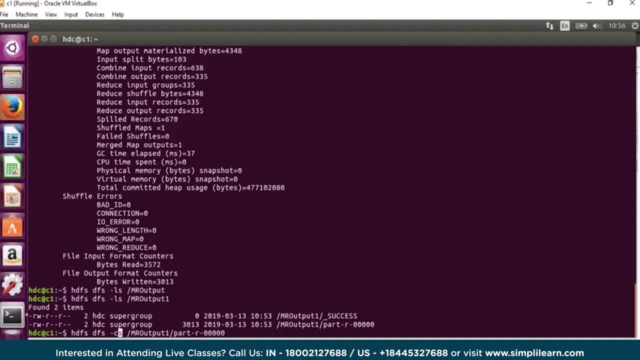 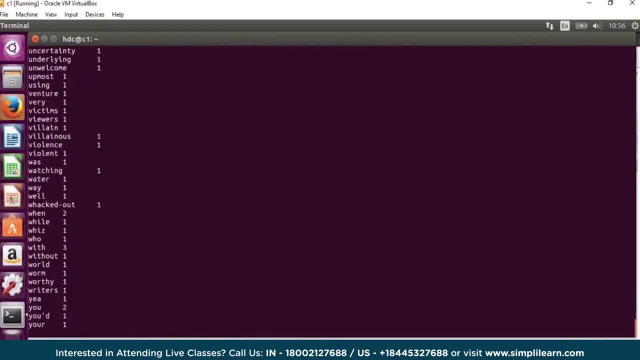 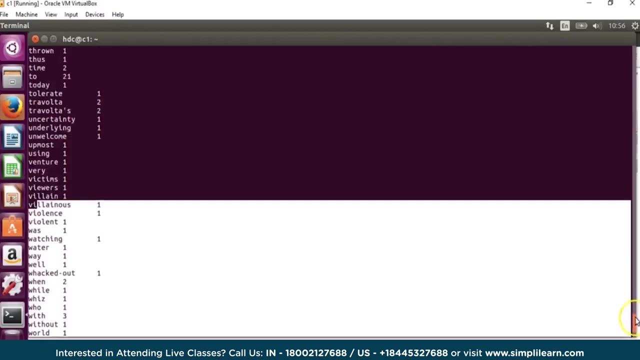 be my word count, and here I can say cat, which basically shows me what is the output created by my map reduce. let's have a look into this. so the file which we gave for processing has been broken down and now we have the list of words which occur in the file, plus a count of. 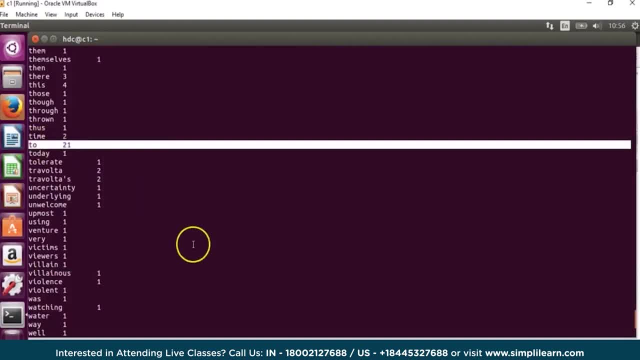 those words. so if there is some word which is in is more, then it shows me the count. so this is a list of my words and the count for that. so this is how we run a sample map reduce job. I will also show you how we can run it on. yeah, now let's run map reduce on yarn and 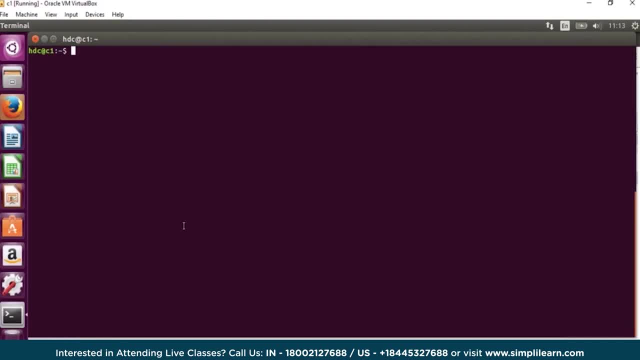 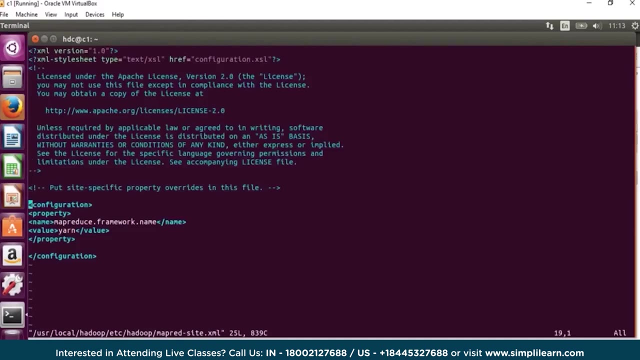 initially when we tried running a map reduce, it did not hit yarn but it ran in a local mode and that was because there was a property which had to be changed in map reduce hyphen site file. so basically, if you look into this file, the error was that I had given a property which says map. 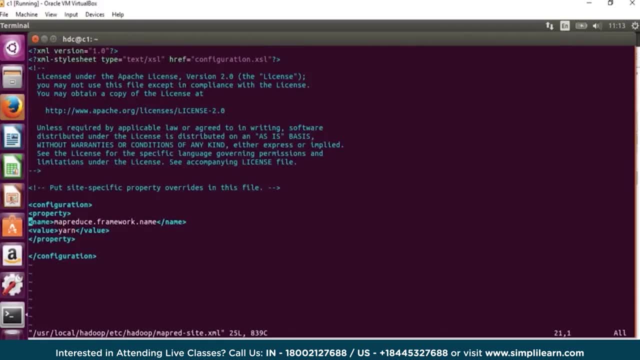 red dot framework dot name and that was not the right property name and that was ignored and that's why it ran in a local mode. so I changed the property to map reduce dot framework dot name, restarted my cluster and everything should be fine now and that map red. 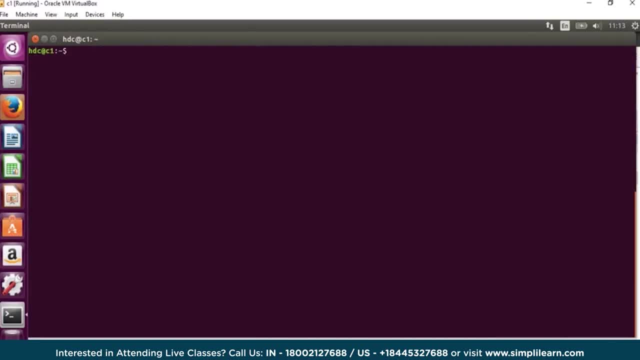 hyphen site file has also been copied across the nodes. now to run a map reduce on a Hadoop cluster so that it uses yarn and yarn takes care of resource allocation on one or multiple machines. so I'm just changing the output here and now I will submit this job, which should first connect. 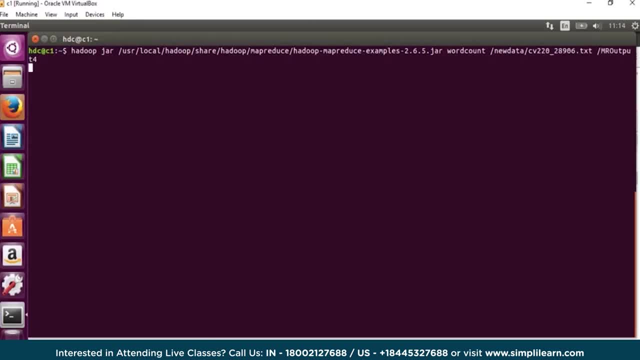 to the resource manager, and if it connects to the resource manager, that means our job will be run using yarn on the cluster rather than in a local mode. so now we have to wait for this application to internally connect to resource manager and once it starts there we can always go back to. 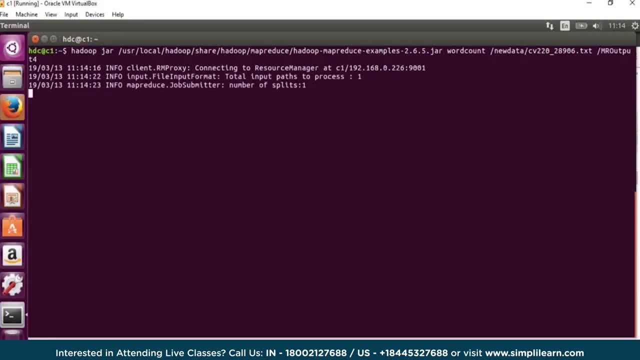 the web UI and check if our application has reached yarn. so it shows me that there is one input part to be processed. that's my job ID. that's my application ID, which you can even monitor status from the command line. now, here, the job has been submitted. so let's go back here and 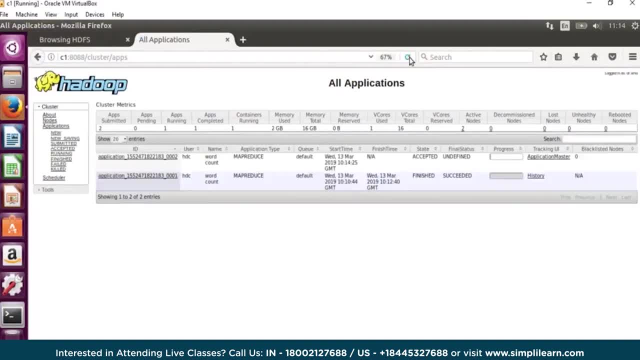 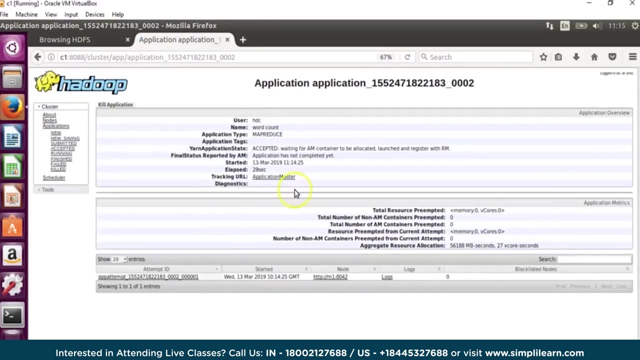 just do a refresh on my yarn UI, which should show me the new application which is submitted. it tells me that it is in accepted state. application master has already started and if you click on this link, it will also give you more details of how many map and reduce tasks would run. so as of now, it 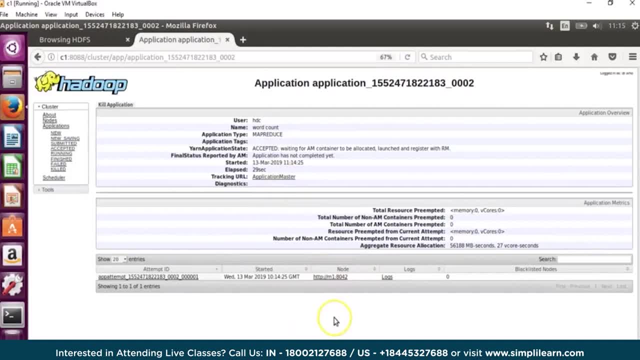 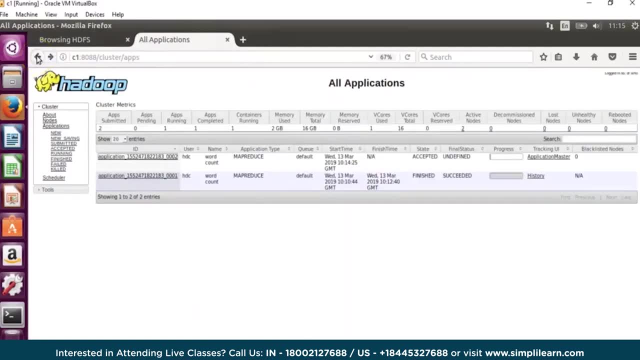 says the application master is running, it would be using this node, which is M1. we can always look into the logs. we can see. then there is a one task attempt which is being made and now, if I go back to my terminal, I will see that it is waiting to get some resources from. 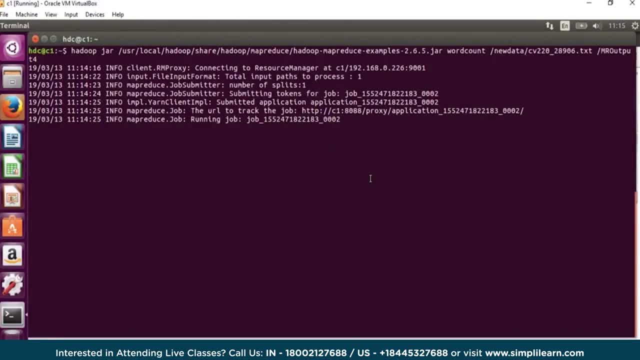 the cluster and once it gets the resources it will first start with the mapping phase. where the mapper function runs, it does the map tasks one or multiple, depending on the splits. so right now we have one file and one split, so we will have just one map task running and once the mapping 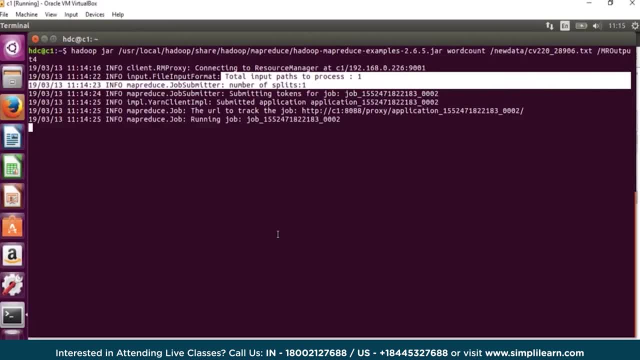 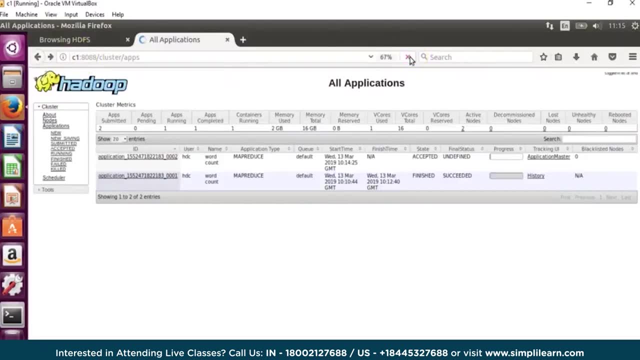 phase completes, then it will get into reducing, which will finally give me my output so we can be toggling through these sessions. so here I can just do a refresh to see what is happening with my application. is it proceeding? is it still waiting for resource manager to allocate some resources now just 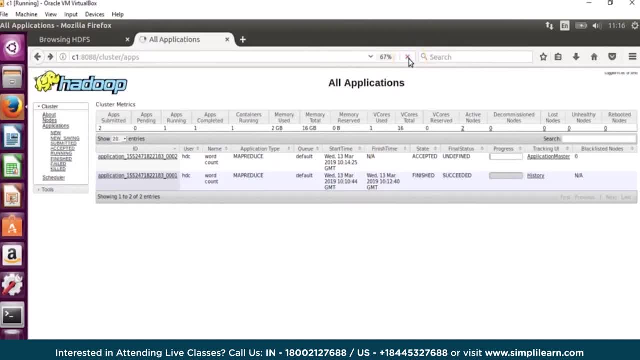 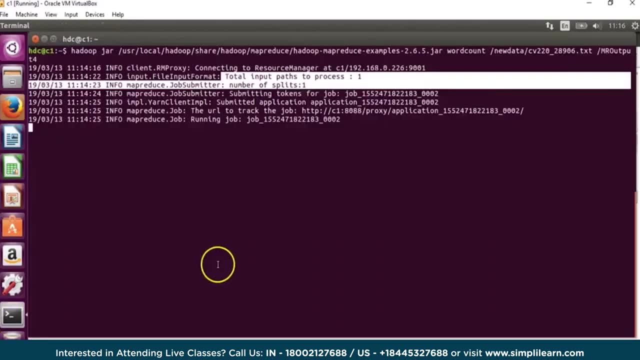 couple of minutes back I tested this application on yarn and we can see that my first application completed successfully and here we will have to give some time so that yarn can allocate the resources. now. if the resources were used by some other application, they will have to be freed up. 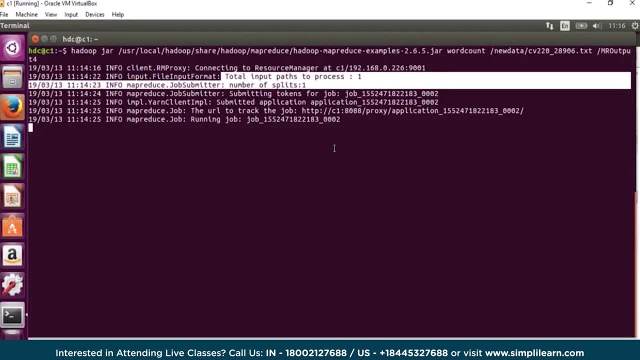 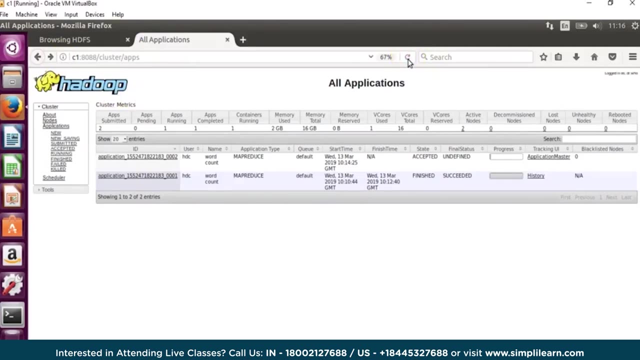 now, internally, yarn takes care of all that which we will learn more detail in yarn or you might have already followed the yarn based session now here. we will have to just give it some more time and let's see if my application proceeds with the resources what yarn can allocate to it sometimes. 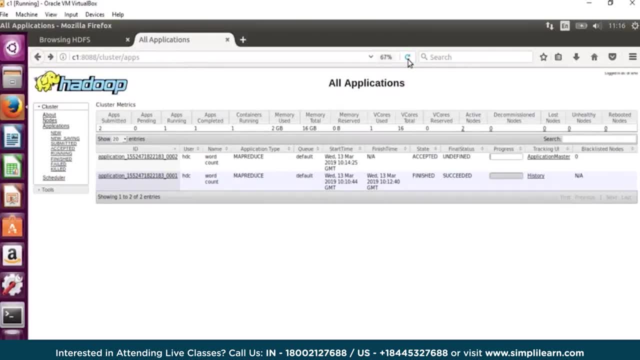 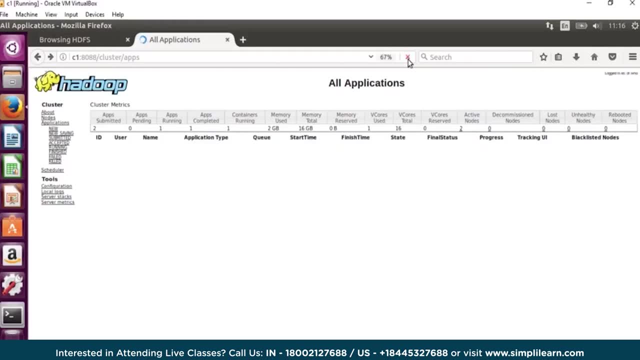 you can also see a slowness in what web UI shows up- and that can be used for other applications as well- be related to the amount of memory you have allocated to your notes. now for apache we can have less amount of memory and we can still run the cluster and, as i said, the memory which shows. 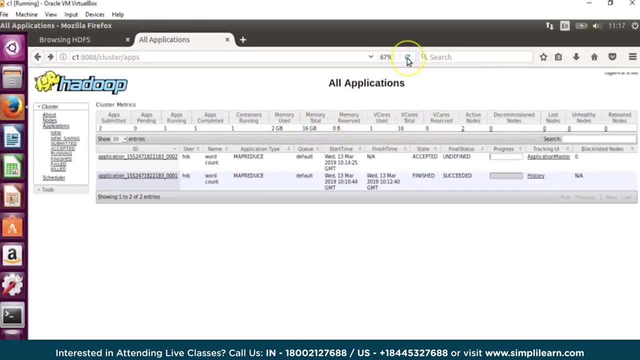 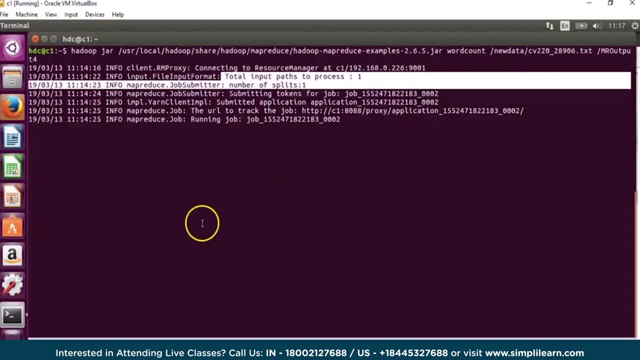 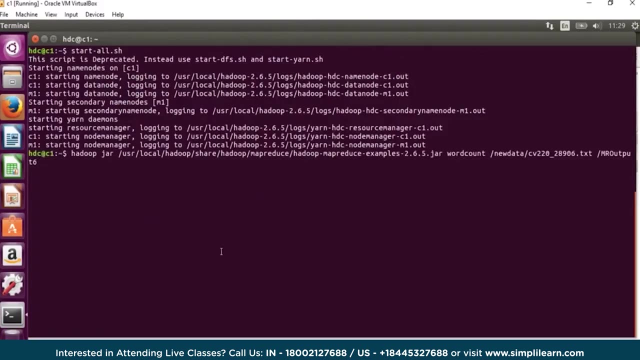 up here. 16 gb and 16 cores is not the true one. those are the default settings, right? but then my yarn should be able to facilitate running of this application. let's just give it couple of seconds and then let's look into the output. here again, i had to make some changes in the settings because 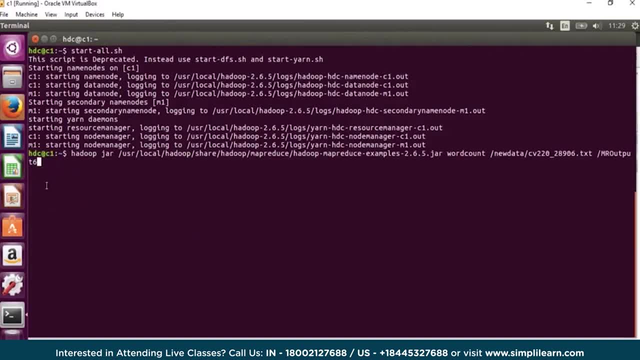 our application was not getting enough resources and then basically i restarted my cluster. now let's submit the application again to the cluster, which first should contact the resource manager and then basically the map and reduce process should start. so here i have submitted an application, it is connecting to the resource manager and then basically it will start. 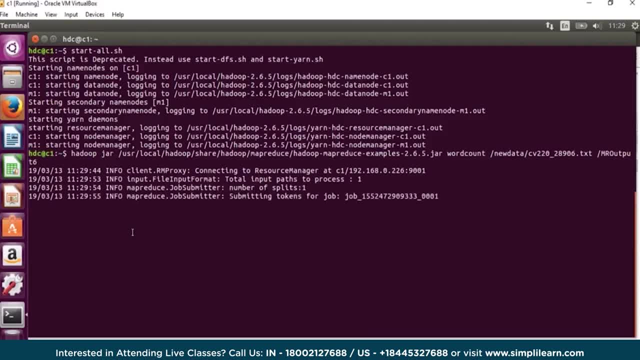 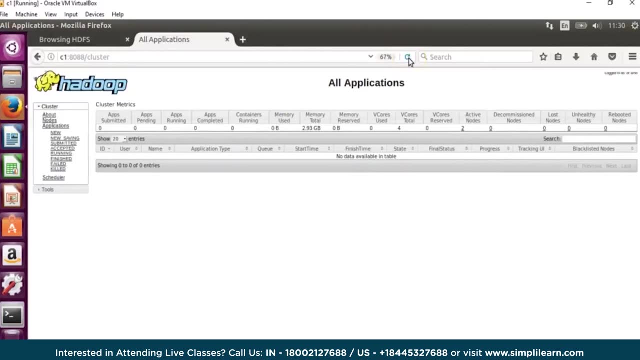 internally an app master. that is application master. it is looking for the number of splits, which is one. it's getting the application i d and it basically then starts running the job. it also gives you a tracking url to look at the output. and now we should go back and look at our yarn ui. if our application shows up here and we 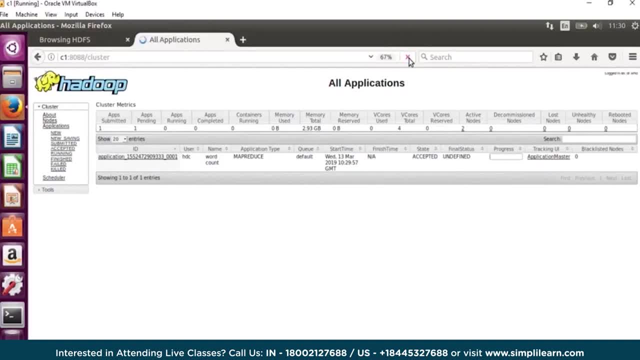 will have to give it a couple of seconds when it can get the final status change to running, and that's where my application will be getting resources. now, if you closely notice, here i have allocated specific amount of memory, that is, gb for node manager on every node, and i have basically given two cores each, which my machines 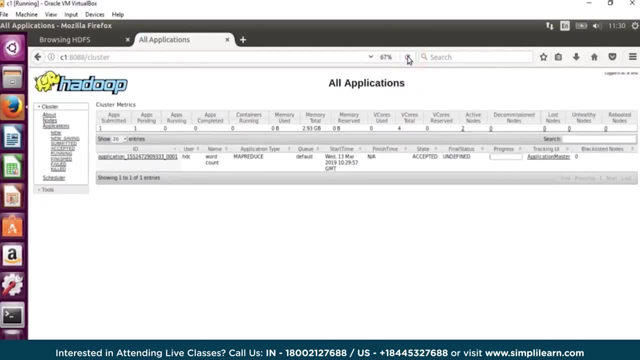 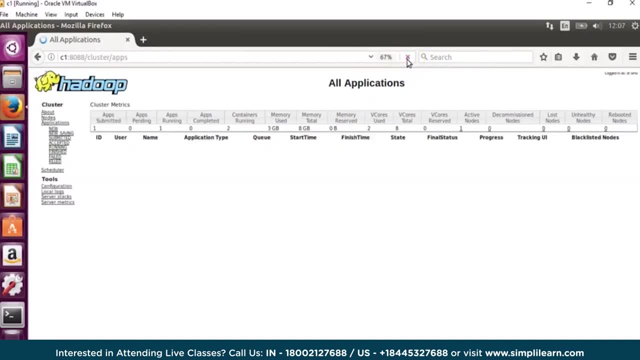 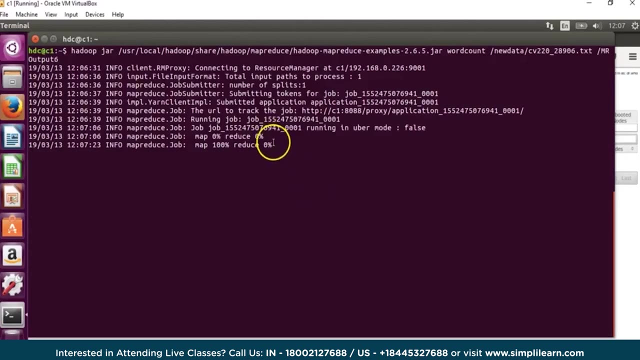 also have, and my yarn should be utilizing these resources rather than going for default. now the application has started moving and we can see the progress bar here, which basically will show what is happening, and if we go back to the terminal it will show that first it went. 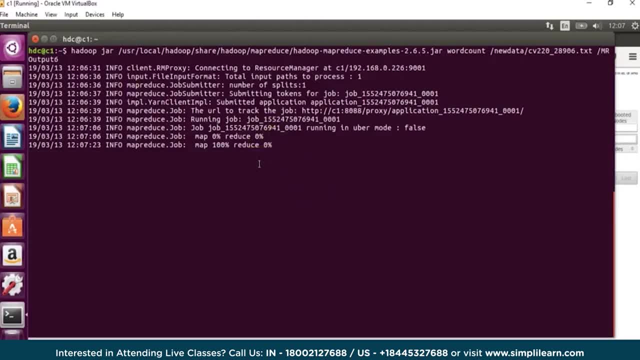 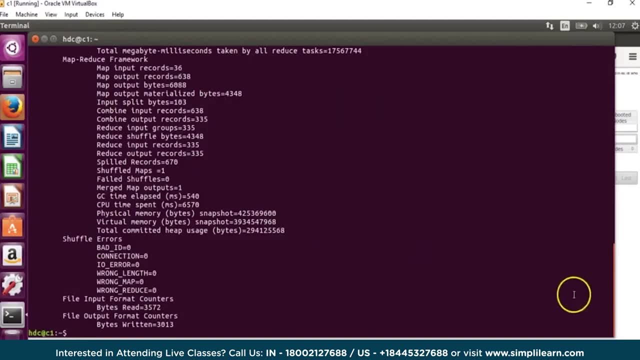 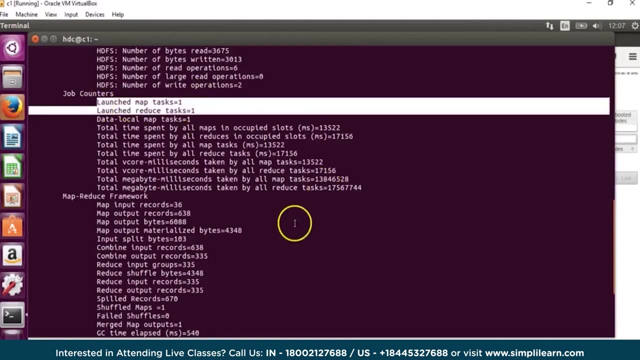 in deciding map and reduce, it goes for map. once the mapping phase complete, then the reducing phase will come into existence. and here my job has completed, so now it has basically used. we can always look at how many map and reduce tasks were run. it shows me that there was one map and one reduced task. now, with the number of map tasks depends on. 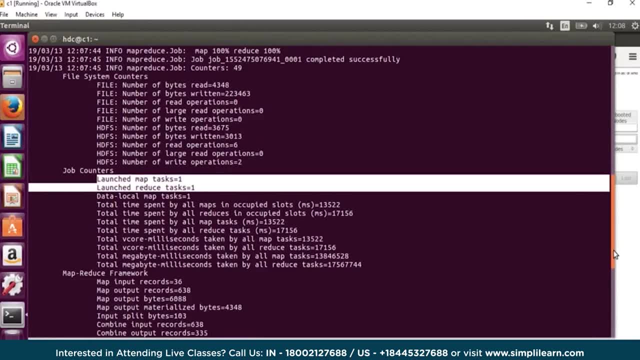 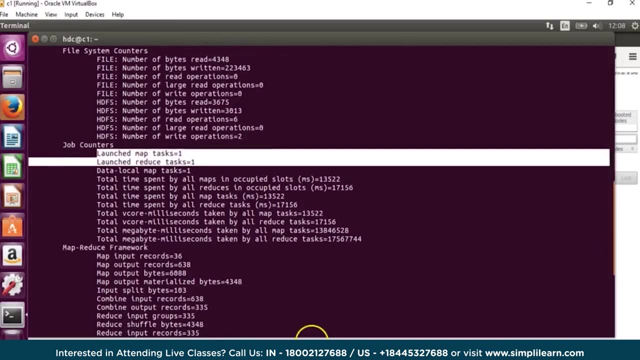 the number of splits, and we had just one file which is less than 128 mb. so that was one split to be processed and reduced task is internally decided by the reducer or depending on what kind of property has been set in hadoop config files. now it also tells me how many input records. 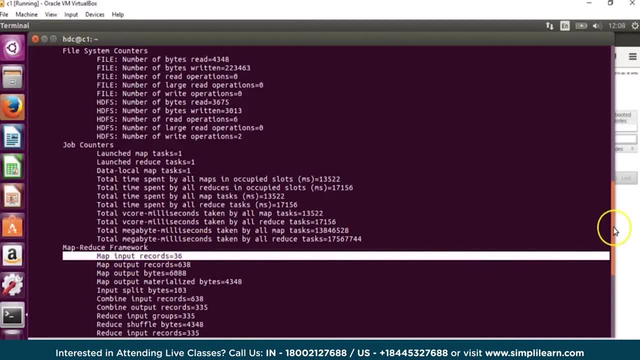 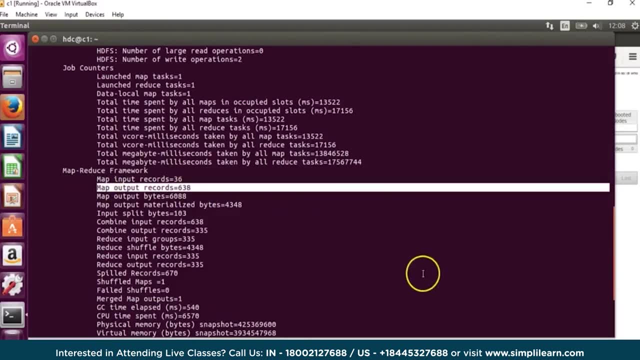 were read, which basically means these were the number of lines in the file. it tells me output records, which gives me the number of total words in the file- now there might be duplicates- and that which is processed by internal combiner: further processing or forwarding that information to. 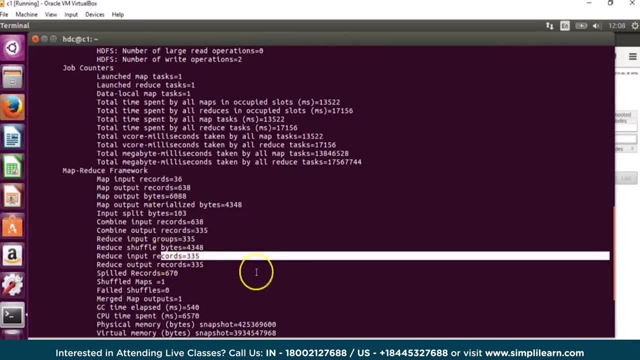 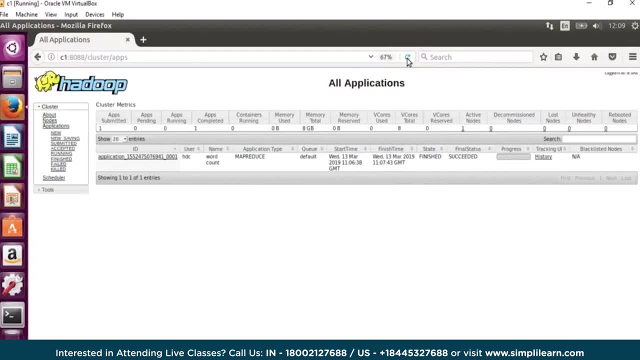 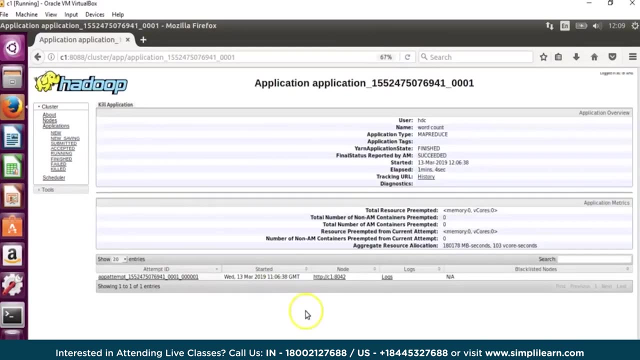 reducer and basically reducer works on 335 records, gives us a list of words and their count. now, if i do a refresh here, this would obviously show my application is completed. it says succeeded. you can always click on the application to look for more information. it tells me where it ran. now we do not have a history server running as of now. 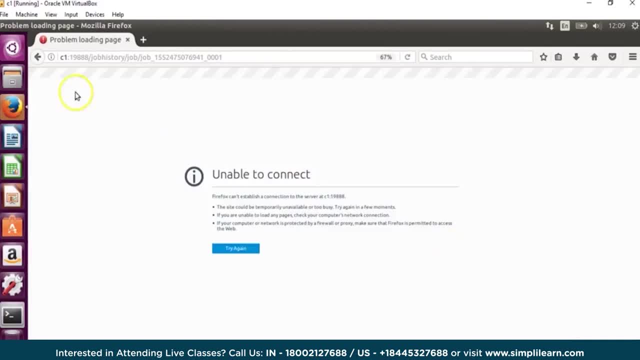 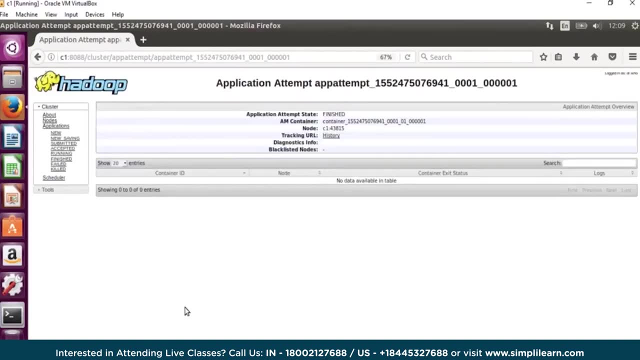 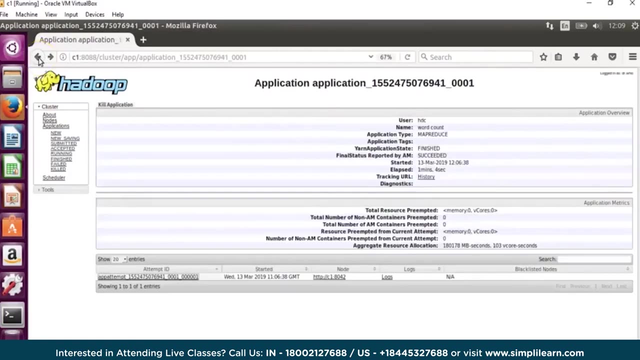 otherwise we can always access more information. so this leads to history server, where all your applications are stored. but i can click on this attempt tasks and this will basically show me the history url, or you can always look into the logs. so this is how you can submit a sample application which is inbuilt, which is 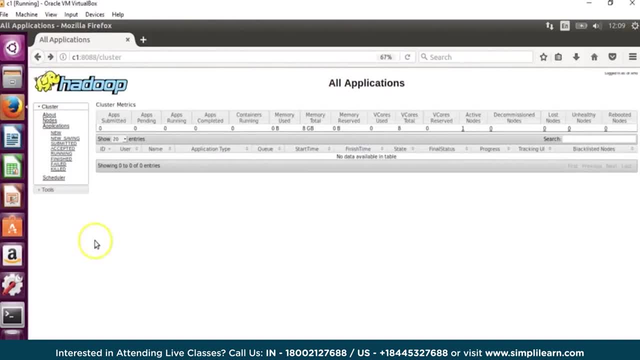 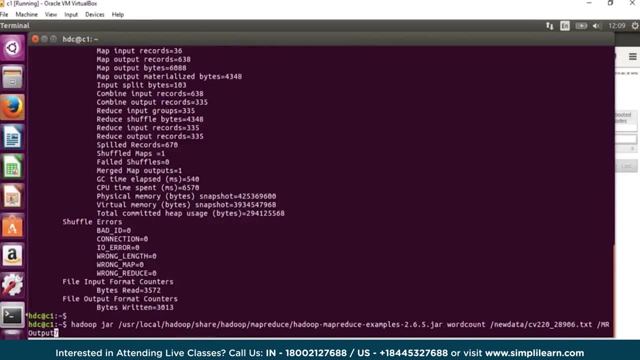 available in the jar on your hadoop cluster and that will utilize your cluster to run. now you could always, as i said, when you are running a particular job, remember to change the output directory and if you would not want it to be processing a single individual file, you could. 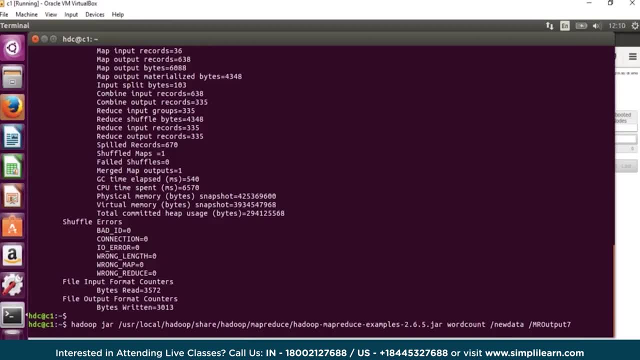 also point it to a directory. that basically means it will have multiple files and depending on the file sizes there would be multiple splits and according to that, multiple map tasks will be selected. so if i click on this, this would submit my second application to the cluster, which should first 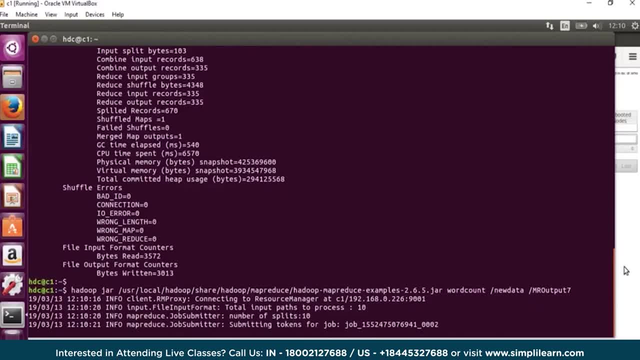 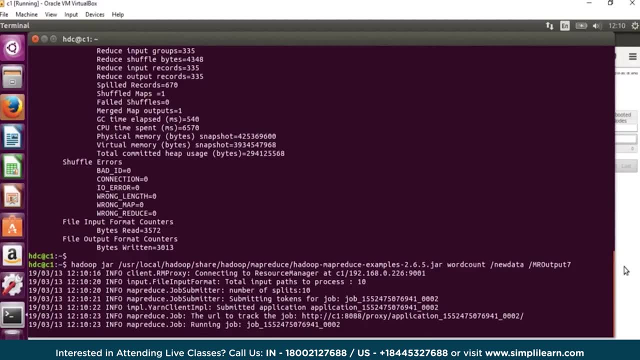 connect to resource manager, then resource manager has to start an application master. now here we are targeting 10 splits. now you have to sometimes give couple of seconds in your machines so that the resources which were used are internally already freed up, so that your cluster can pick it up and 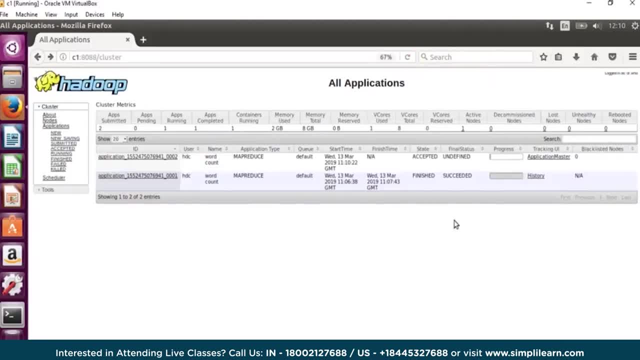 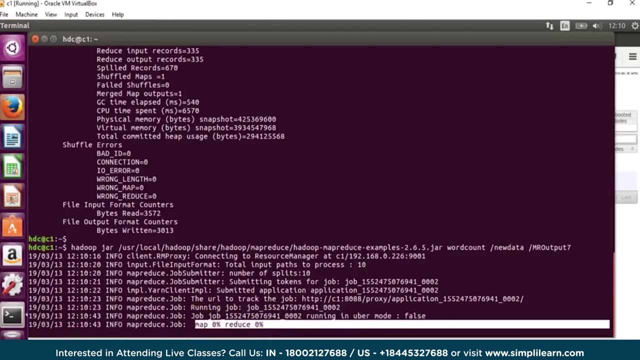 then your yarn can take care of resources. so right now my application is in undefined status, but then as soon as my yarn provides it the resources, we will have the application running on our yarn cluster. so it has already started. if you see it is going further, then it would launch 10 map tasks. 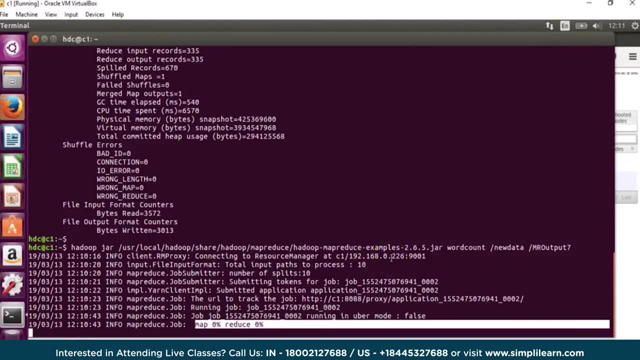 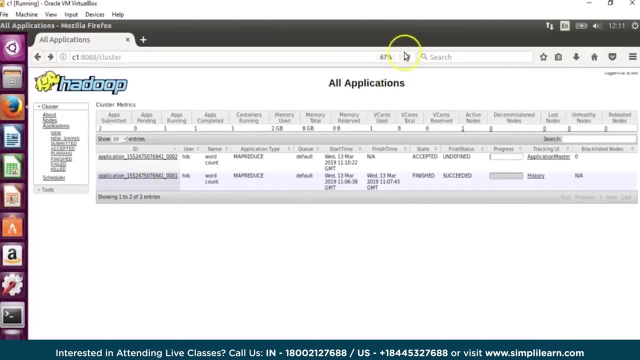 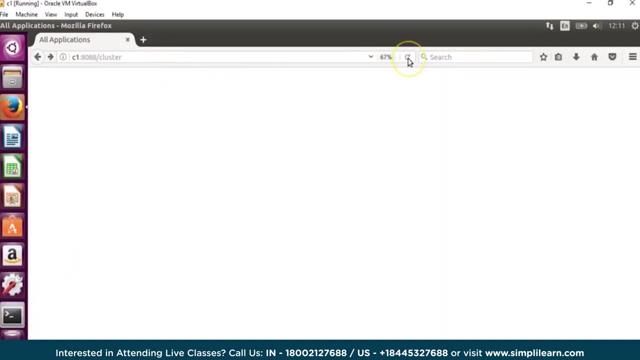 and it would. the number of reduced tasks would be decided on either the way your data is or based on the properties which have been set at your cluster level. let's just do a quick refresh here on my yarn ui to show me the progress. also take care that when you are 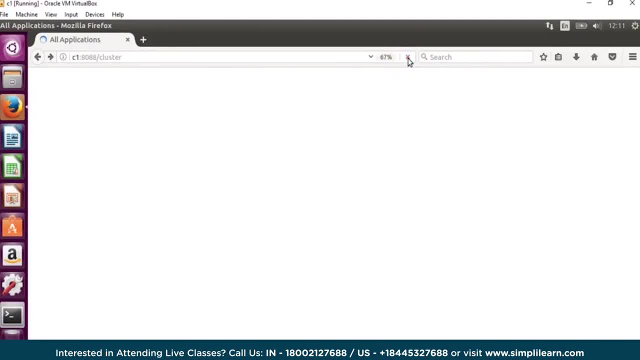 submitting your application, you need to have the output directory mentioned. however, do not create it. hadoop will create that for you. now, this is how you run a map reduce without specifying properties, but then you can specify more properties. you can look into what are the things which can be changed for your mapper and reducer, or basically having a combiner class which can do a. 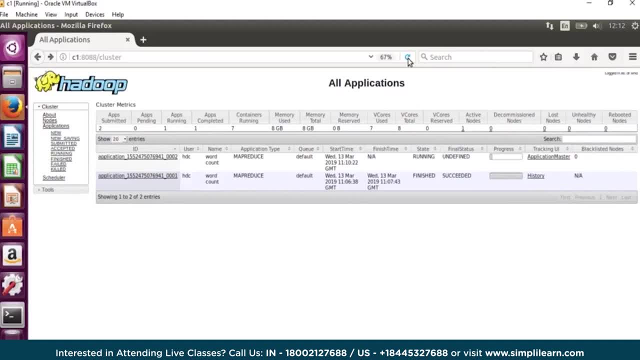 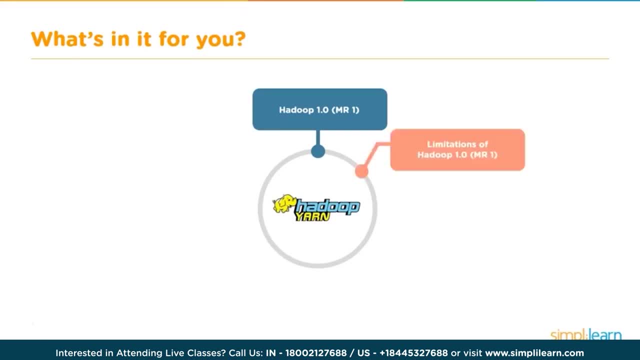 map reducing and all those things can be done. so we will learn about that in the later sessions. now we will compare hadoop version one, that is, with map reduce version one. we will understand and learn about the limitations of hadoop version one. what is the need of yarn? what is yarn? what kind? 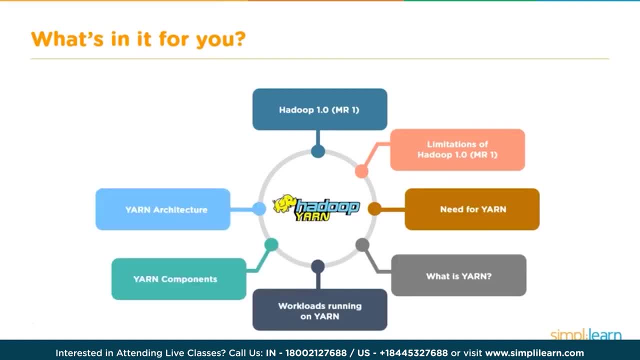 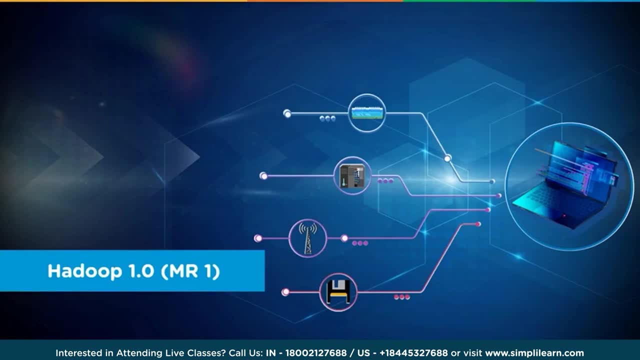 of workloads can be running on yarn: what are yarn components, what is yarn architecture and finally, we will see a demo on yarn. so hadoop version one or map reduce version one. well, that's outdated now and nobody is using hadoop version one, but it would be good to understand. 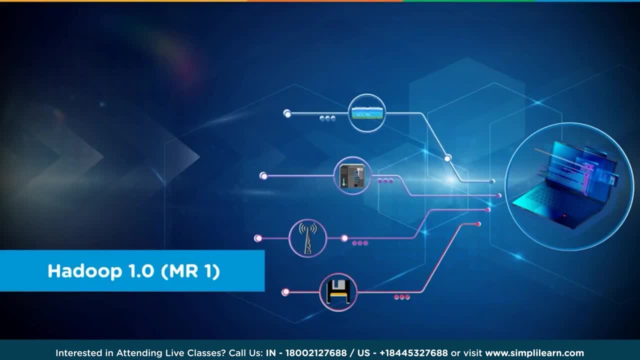 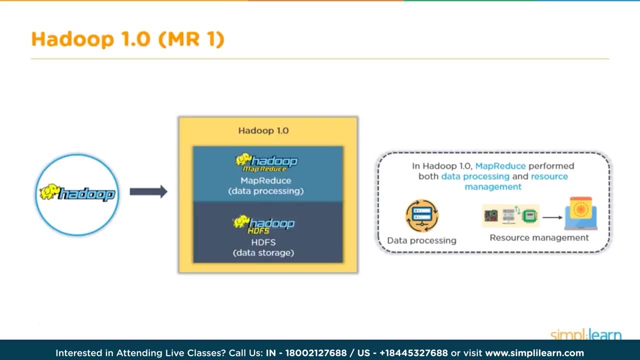 what was in hadoop version one and what were the limitations of hadoop version one, which brought in the thought for the future processing layer. that is yarn. now, when we talk about hadoop, we already know that hadoop is a framework and hadoop has two layers. one is your storage layer. 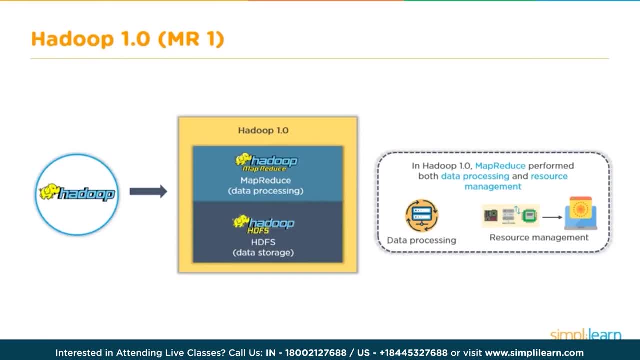 that is, your sdfs hadoop distributed file system, which allows for distributed storage and processing, which allows fault tolerance by inbuilt replication and which basically allows you to store huge amount of data across multiple commodity machines. when we talk about processing, we know that map reduce is the oldest and the most mature. 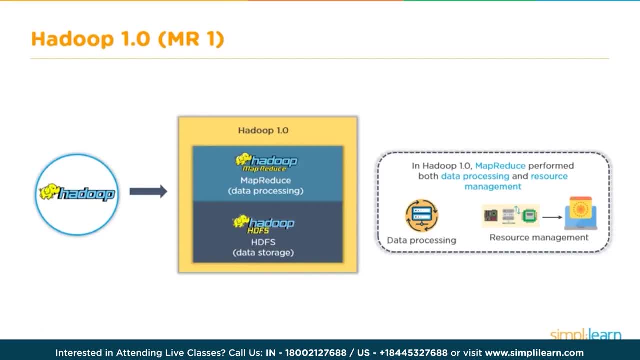 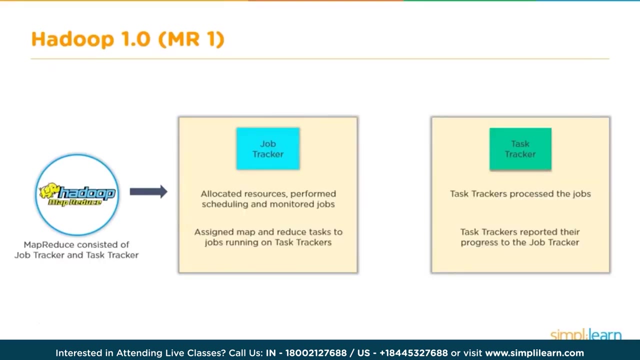 processing programming model which basically takes care of your data processing on your distributed file system. so in hadoop version one, map reduce performed both data processing and resource management and that's how it was problematic. in map reduce we had basically, when we talk about the processing layer, we had the master, which was called job tracker, and then you. 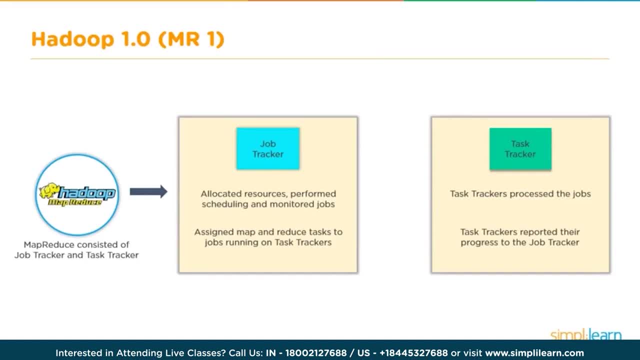 had the slaves, which were the task trackers. so your job tracker was taking care of allocating resources. it was performing scheduling and even monitoring the jobs. it basically was taking care of assigning, map and reduce tasks to the jobs. running on hadoop version one, task trackers and task trackers which were co-located with data nodes were responsible. 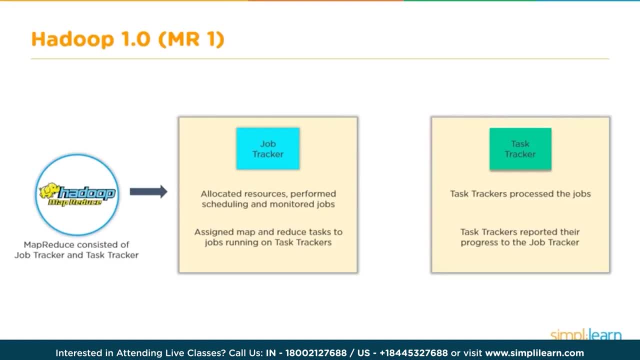 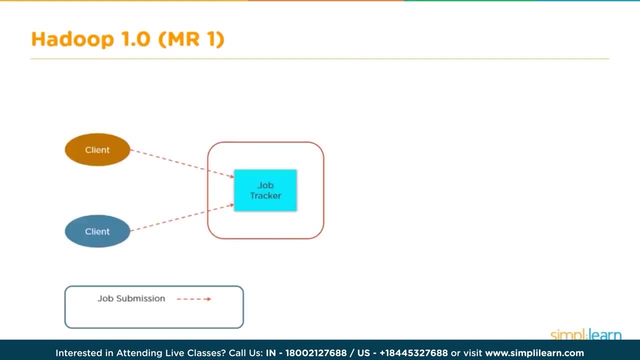 for processing the jobs. so task trackers were the slaves for the processing layer which reported their progress to the job tracker. so this is what was happening in hadoop version one. now when we talk about hadoop version one, we would have say client machines or an api or an application which 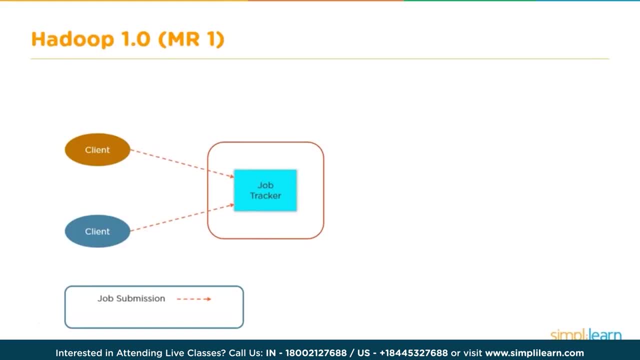 basically submits the job to the master, that is, job tracker. now, obviously we cannot forget that there would be an involvement from name node which basically tells which are the machines or which are the data nodes where the data is already stored. now, once the job submission happens to the job tracker, 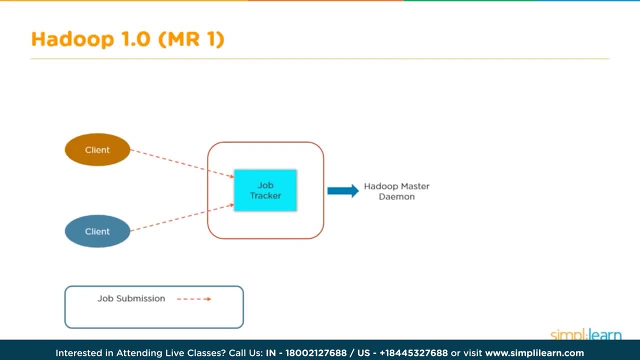 job tracker being the master daemon for taking care of your processing request and also resource management. job scheduling would then be interacting with your multiple task trackers, which would be running on multiple machines. so each machine would have a task tracker running and that task tracker, which is a processing slave, would be co-located with the data nodes. now we 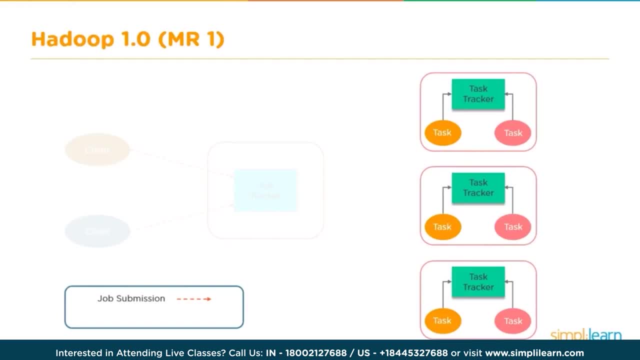 know that in case of hadoop, you have the concept of moving the processing to wherever the data is stored, rather than moving the data to the processing layer. so we would have task trackers which would be running on multiple machines and these task trackers would be responsible for handling the tasks. what are these tasks? these are the application, which is broken down into small 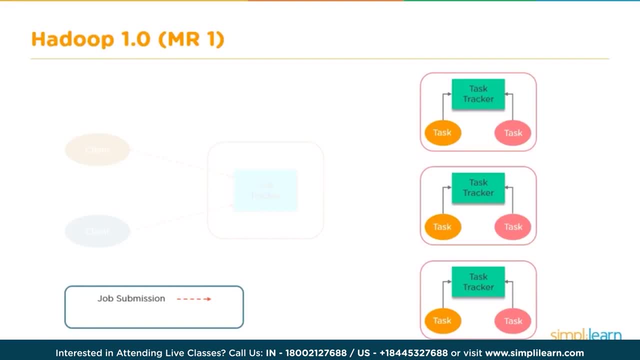 tasks which would work on the data which is respectively stored on that particular node. now, these were your slave daemons, right? so your job tracker was not only tracking the resources, so your task trackers were sending heartbeats, they were sending in packets and information to the job tracker, which would then be knowing how many resources and when we talk about resources. 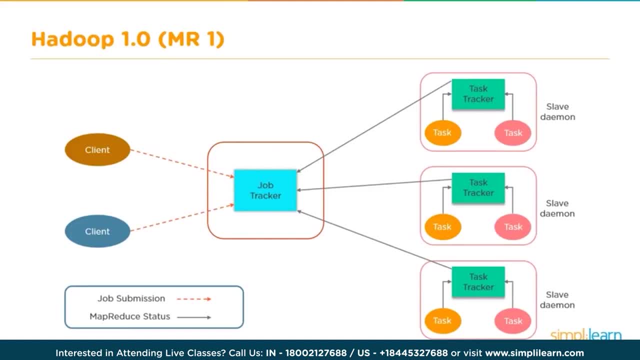 we are talking about the cpu cores. we are talking about the ram, which is the cpu core, which is the ram which would be available on every node. so task trackers would be sending in their resource information to job tracker and your job tracker would be already aware of what amount of resources. 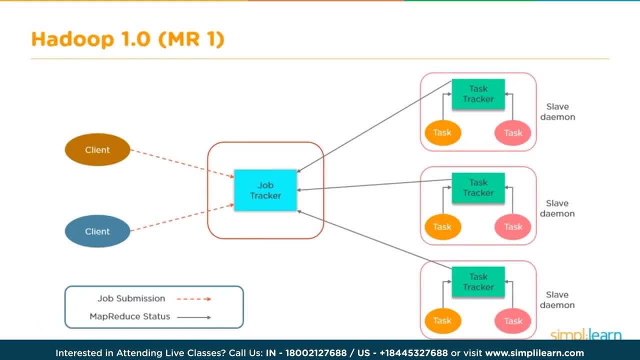 are available on a particular node? how loaded a particular node is? what kind of work could be given to the task tracker? so job tracker was taking care of resource management and it was also breaking the application into tasks and doing the job scheduling part. assign different tasks to these slave demons, that is, your task trackers. so job tracker was eventually overburdened. 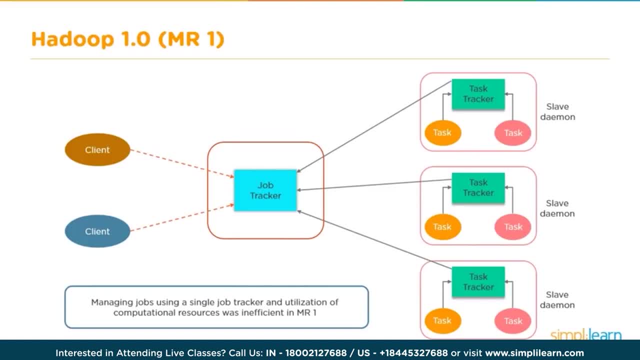 right because it was managing jobs. it was tracking the resources from multiple task trackers and basically it was taking care of job scheduling. so job tracker would be overburdened and in a case if job tracker would fail then it would affect the overall processing. so if the master is killed, if 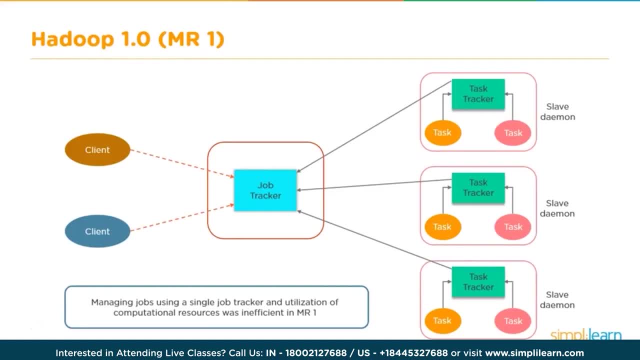 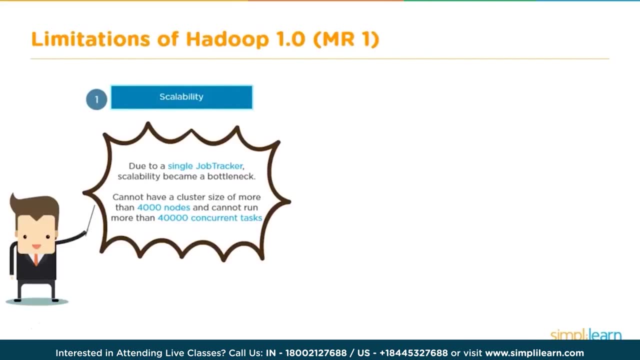 the master demand dies, then the processing cannot proceed. now, this was one of the limitations of hadoop version one. so when you talk about scalability- that is, the capability to scale due to a single job tracker, scalability would be hitting a bottleneck. you cannot have a cluster size of more than 4000 nodes and cannot run more than. 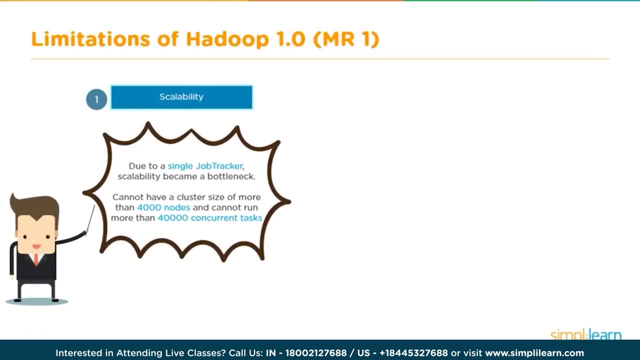 40 000 concurrent tasks. now, that's just a number. we could always look into the individual resources which each machine was having and then we can come up with an appropriate number. however, with a single tracker, there was no horizontal scalability for the processing layer, because we had single. 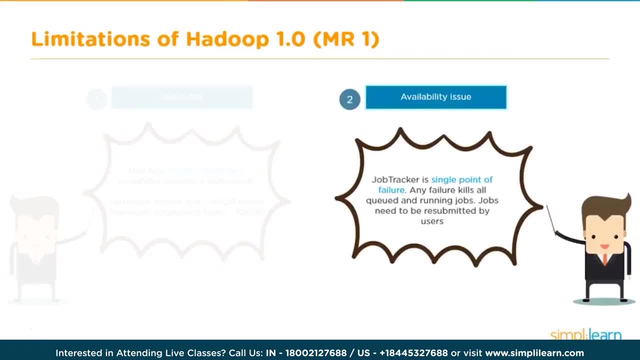 processing master. now, when we talk about availability, job tracker, as i mentioned, would be a single point of failure. now, any failure kills all the queued and running jobs and jobs would have to be resubmitted. now why would we want that in a distributed platform, in a cluster which has 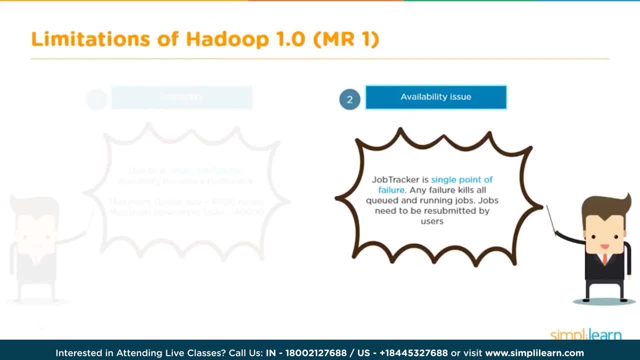 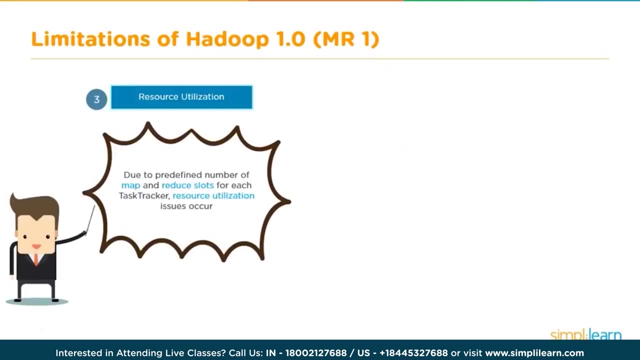 hundreds and thousands of machines. we would want a processing layer which can handle huge amount of processing, which could be more scalable, which could be more available and could handle different kind of workloads when it comes to resource utilization, now, if you would have a predefined number of map and reduce slots for each task tracker, you would have issues which would relate 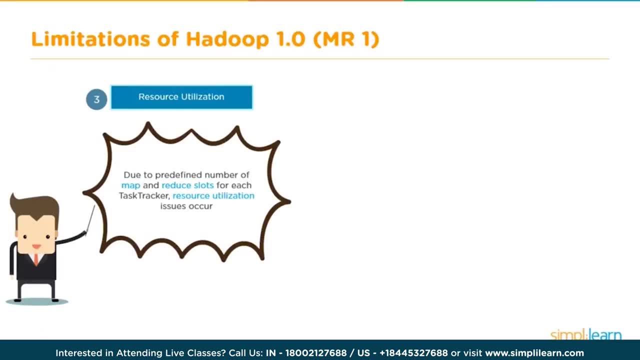 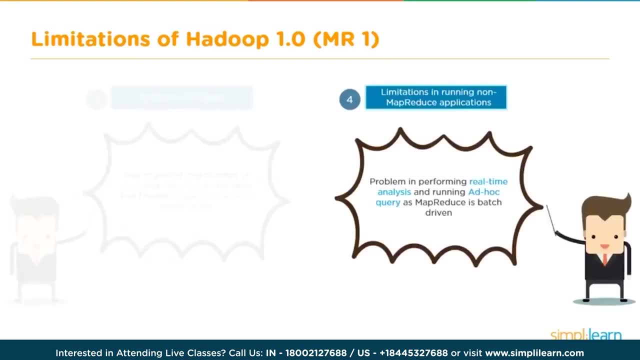 to resource utilization and that again is putting a burden on the master which is tracking these resources, which has to assign jobs, which can run on multiple machines in parallel. so limitations in running non-map reduce applications. now that was one more limitation of hadoop version 1 and 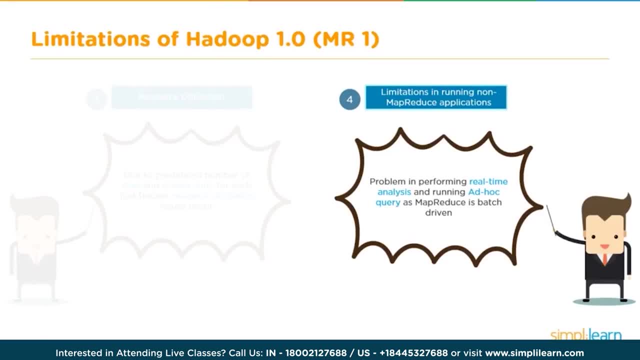 map reduce. that. the only kind of processing you could do is map reduce and map reduce programming model. although it is good, it is oldest, it has matured over a period of time, but then it is very rigid. you will have to go for mapping and reducing approach and that was the only kind of processing. 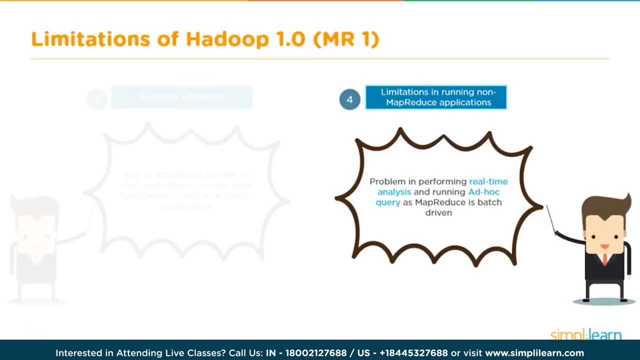 which could be done in hadoop version 1.. so when it comes to doing a real-time analysis or doing ad-hoc query, or doing a graph-based processing or massive parallel processing, there were limitations because that could not be done in hadoop version 1, which was having. 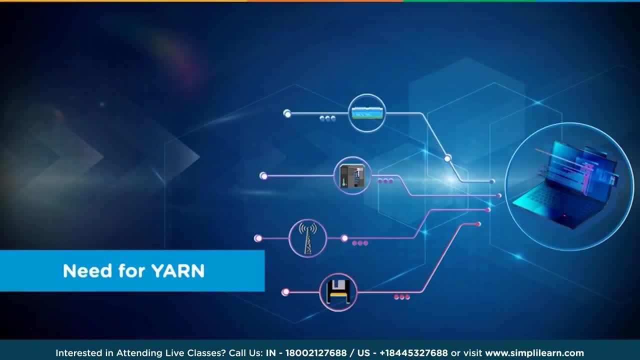 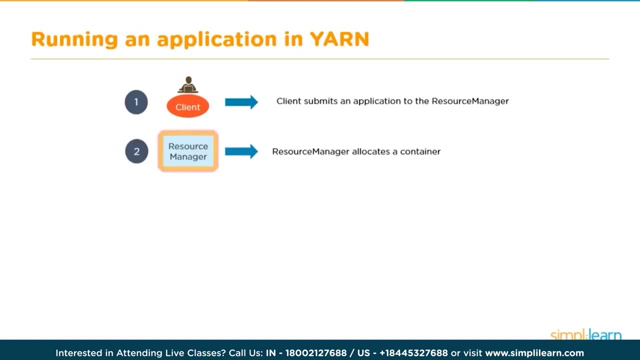 map, reduce version 1 as the processing component. now that brings us to the execution. so your client submits an application to resource manager, resource manager allocates a container, or i would say this is at a high level, right. resource manager is negotiating the resources. and apparently, who is negotiating the resources? it is your applications manager who is. 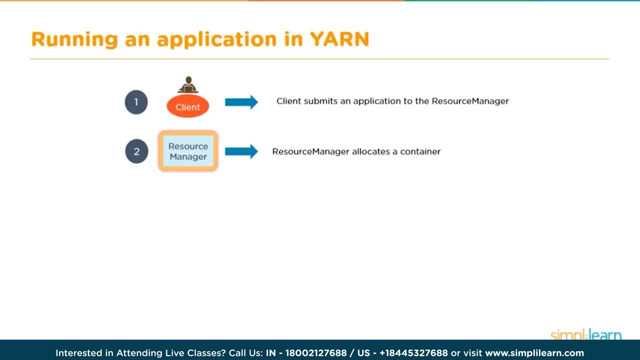 granting this request. it is node manager and that's how we can say: resource manager allocates a container. application master basically contacts the related node manager because it needs to use the containers. node manager is the one which launches the container or basically gives those resources within which an application can run. an application master itself will then accommodate. 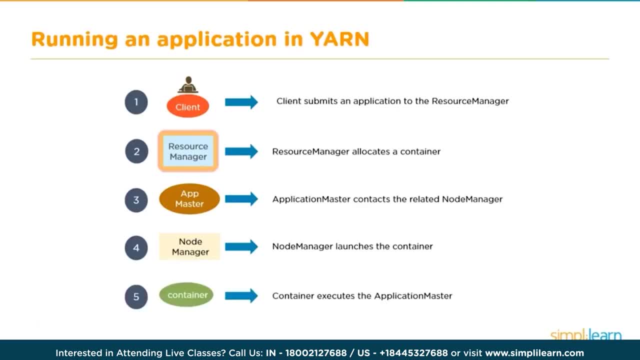 itself in one of the containers, then use other containers for the processing And it is within these containers the actual execution happens. Now that could be a map task, that could be a reduce task, that could be a Spark executor taking care of Spark tasks. 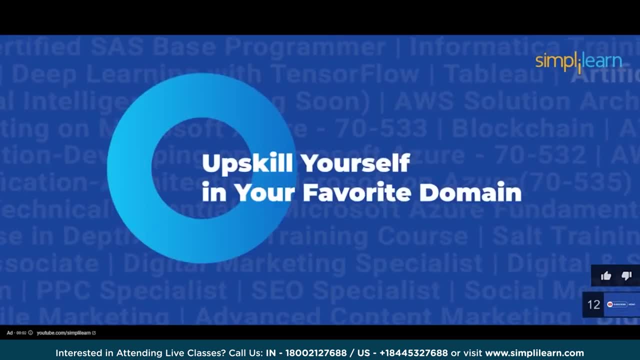 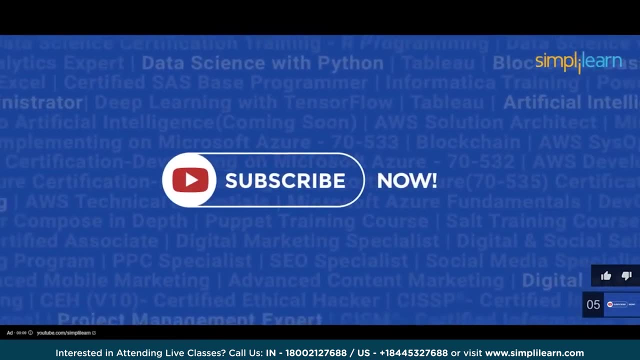 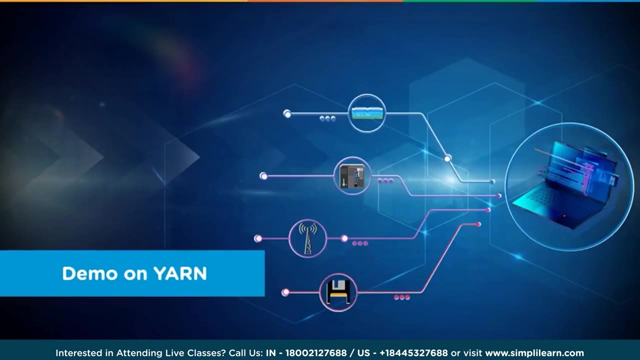 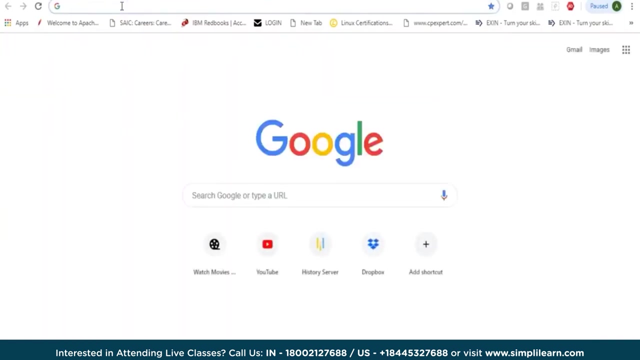 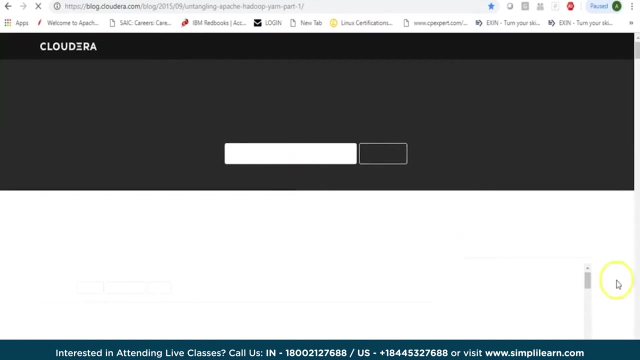 and many other processing. So before we look into the demo on how YARN works, I would suggest looking into one of the blogs from Cloudera- So you can just look for YARN Untangling- and this is really a good blog which basically talks about the overall functionality. 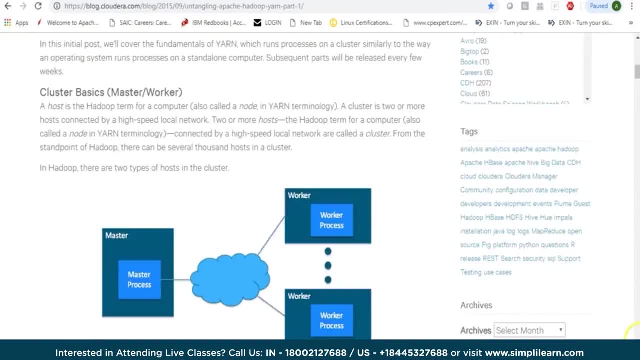 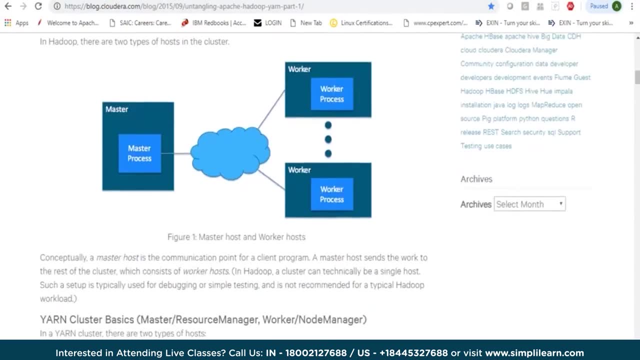 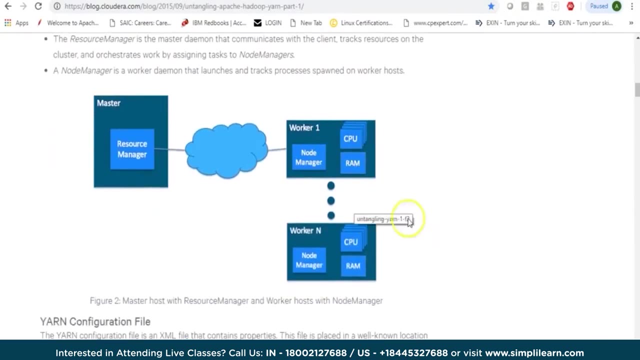 which I explained just now. So, as we mentioned here, so you basically have the master process, you have the worker process, which basically takes care of your processing, your resource manager being the master and node manager being the slave. This also talks about the resources. 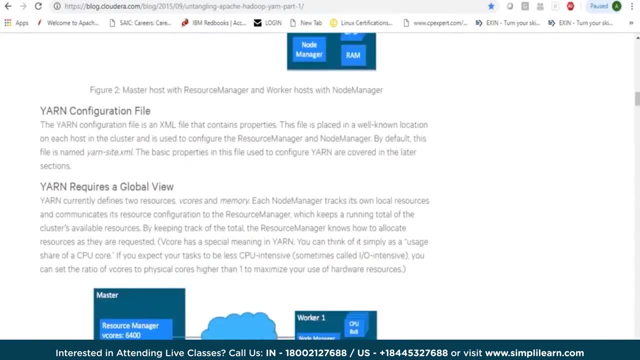 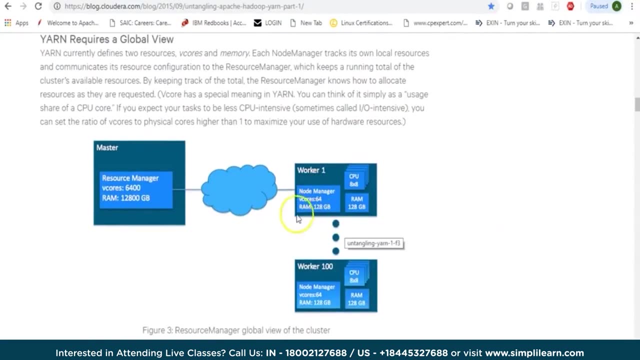 which each node manager has. It talks about the YARN configuration file where you give all these properties. It basically shows you node manager which reports the amount of resources it has to resource manager. Now remember, if worker node shows eight into eight CPU cores and 128 GB RAM. 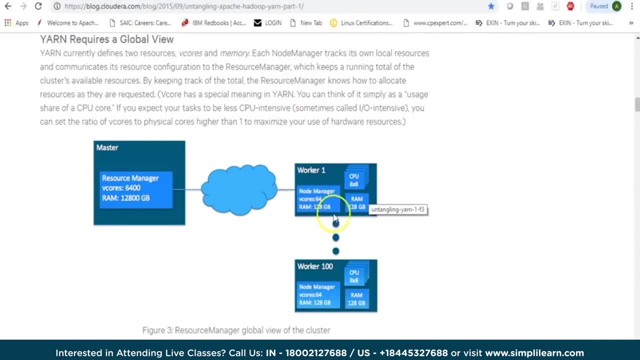 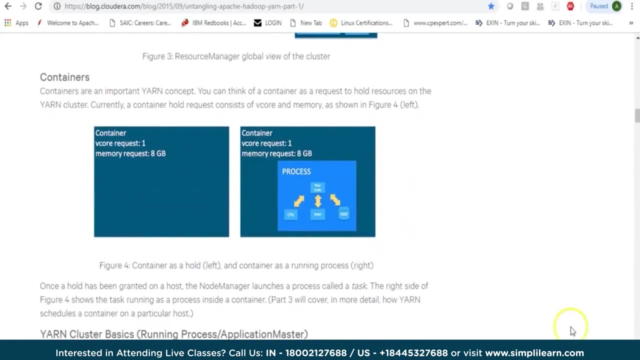 and if your node manager says 64 V cores and RAM 128 GB, then that's not the total capacity of your node. It is some portion of your node which is allocated to node manager. Now, once your node manager reports that your resource manager is requesting for containers, 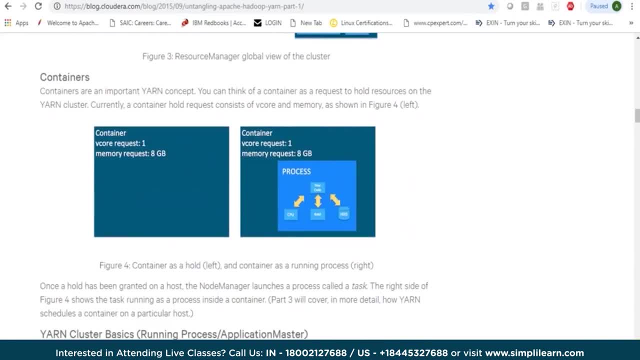 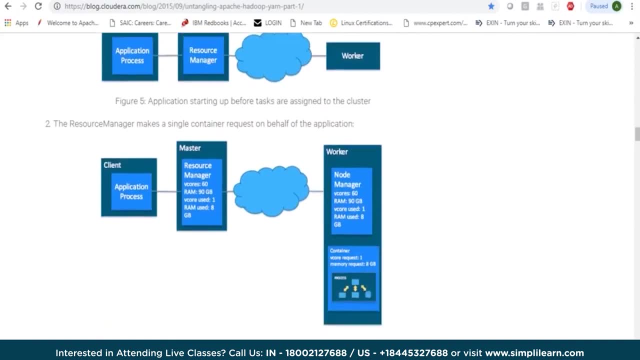 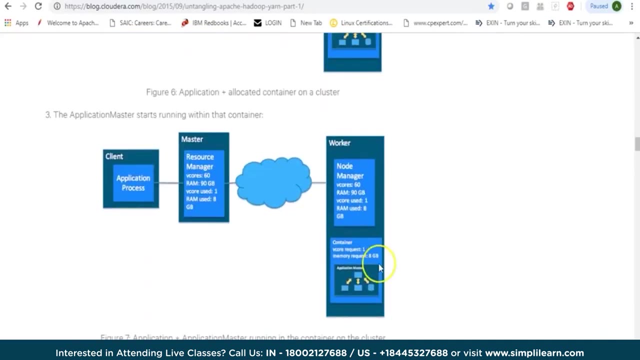 based on the application. What is a container? It is basically a logical name given to a combination of V core and RAM. It is within this container where you would have basically the process running. So once your application starts and once node manager is guaranteed these containers. 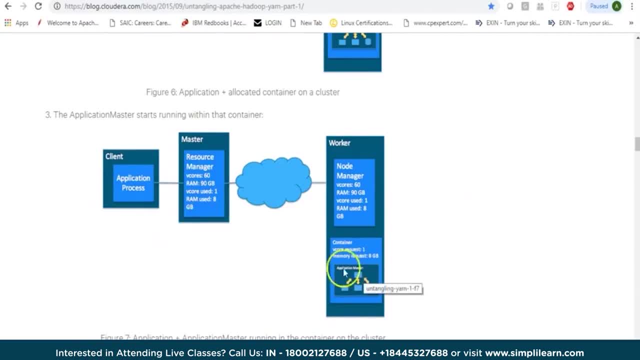 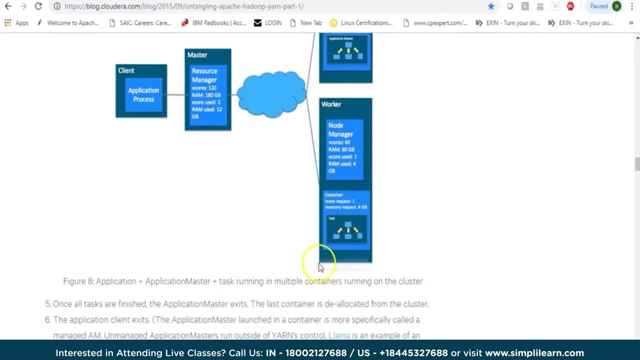 your application or your resource manager has basically already started an application master within the container, And what does that application master do? It uses the other containers where the tasks would run. So this is a very good blog which you can refer to, And this also talks about MapReduce. 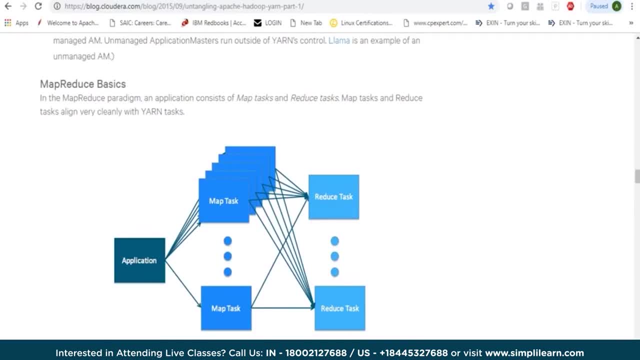 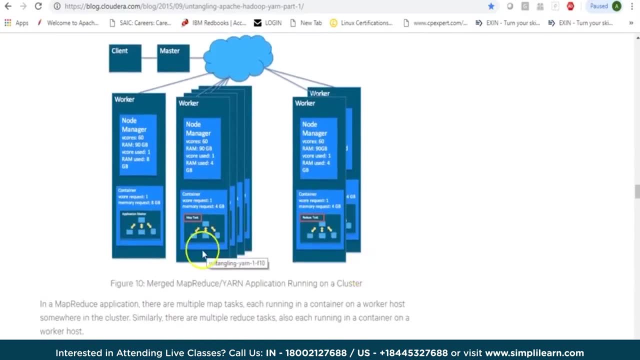 If you have already followed the MapReduce tutorials in past, then you would know about the different kind of tasks. that is, Map and Reduce, And these Map and Reduce tasks could be running within the container in one or multiple. As I said, it could be Map task. 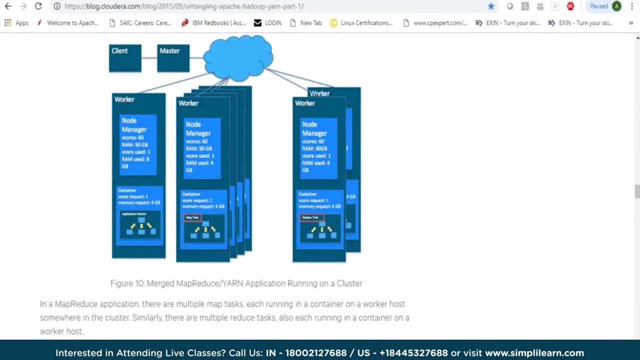 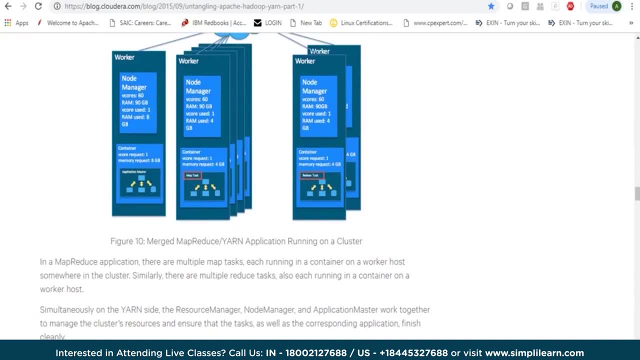 it could be Reduce task. it could be a Spark based task which would be running within the container Now, once the task finishes, basically that resources can be freed up So the container is released and the resources are given back to YARN so that it can take care of further processing. If you'll further look in this blog, you can also look into the part two of it, where you talk mainly about configuration settings. You can always look into this, which talks about why and how much resources are allocated to the node manager. It basically talks about your operating system overhead. 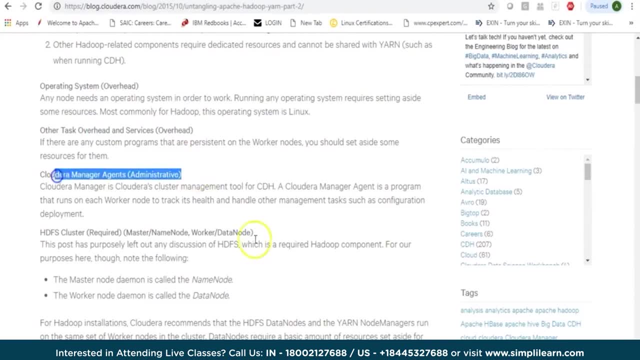 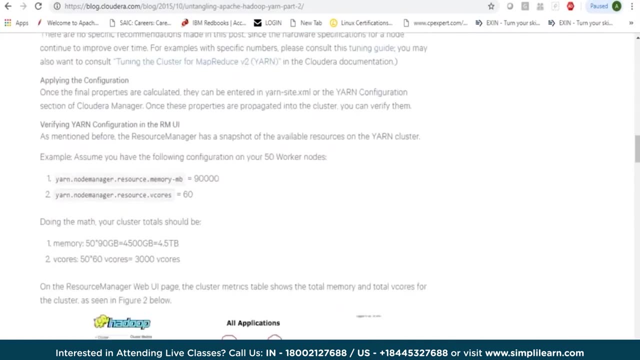 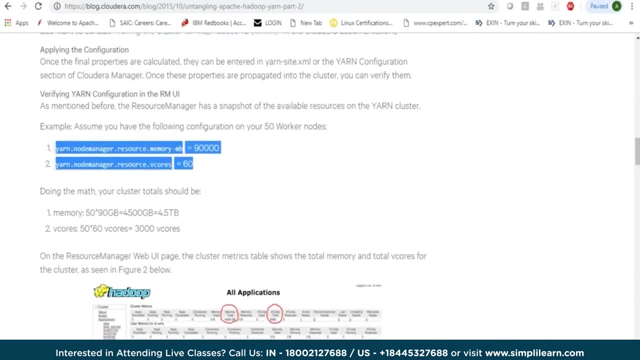 It talks about other services. It talks about CloudAdr, Hotendworks related services running and other processes which might be running, And based on that, some portion of RAM and CPU cores would be allocated to node managers. So that's how it would be done in the YARN-site file. 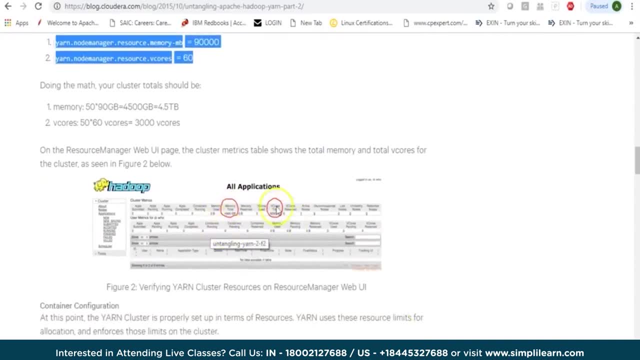 And this basically shows you what is the total amount of memory and CPU cores which is allocated. So that's how it is allocated to node manager. Then within every machine where you have a node manager running on every machine in the YARN-site file. 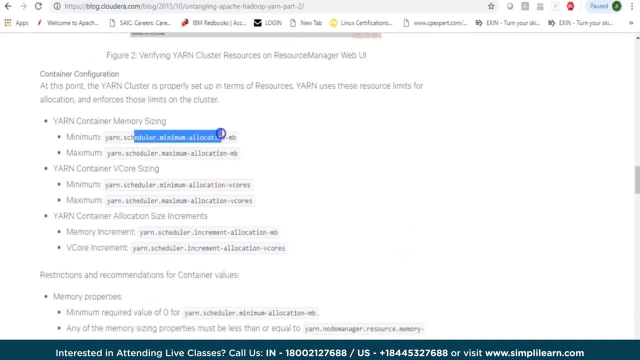 you would have such properties, which would say: what is the minimum container size? What is the maximum container size in terms of RAM, What is the minimum for CPU cores, What is the maximum for CPU cores And what is the incremental size in where RAM and CPU cores can increment? 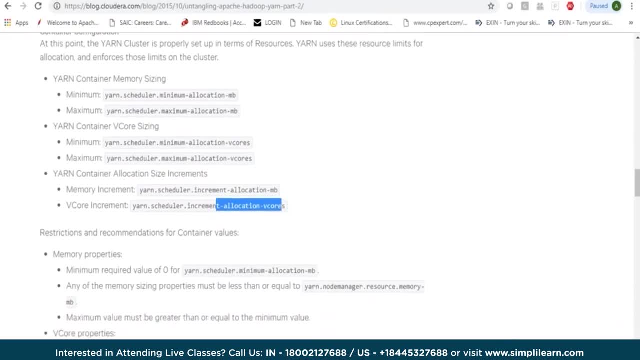 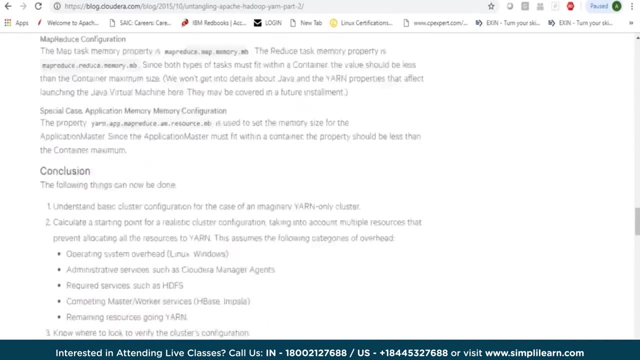 So these are some of the properties which defined how containers are allocated for your application request. So have a look at this and this could be a good information which talks about different properties. Now you can look further- which talks about scheduling. 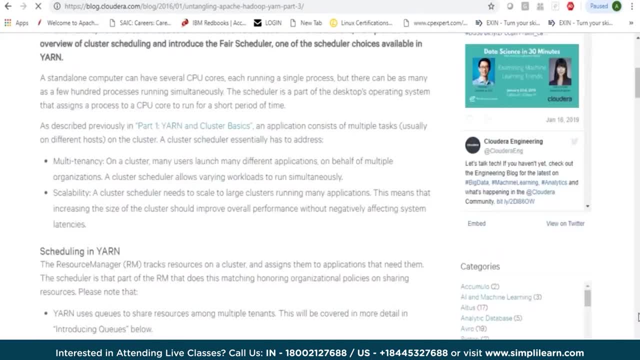 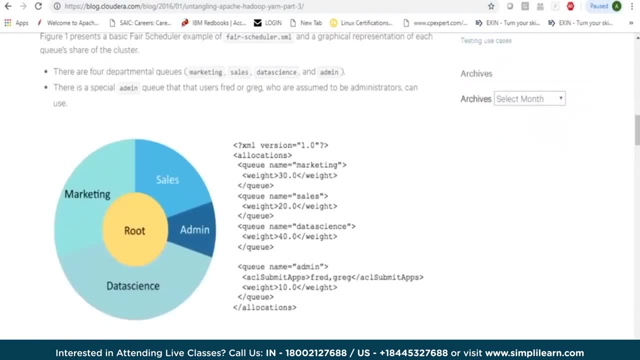 If you look in this particular blog which also talks about scheduling, where it talks about scheduling in YARN, which talks about fair scheduler, or you basically having different queues in which allocations can be done, You also have different ways in which queues can be managed. 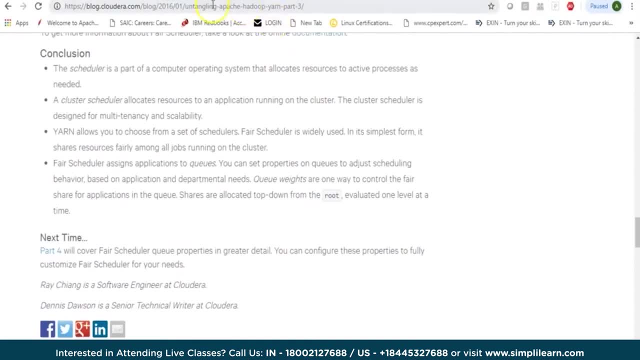 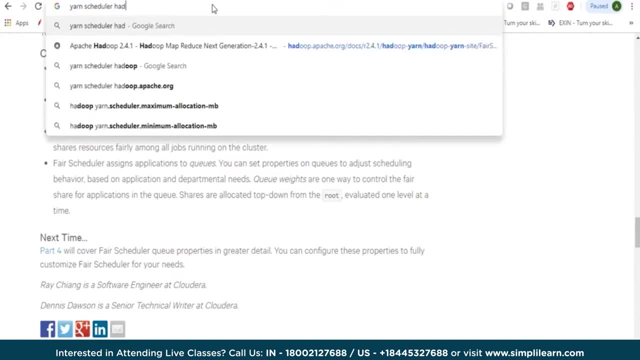 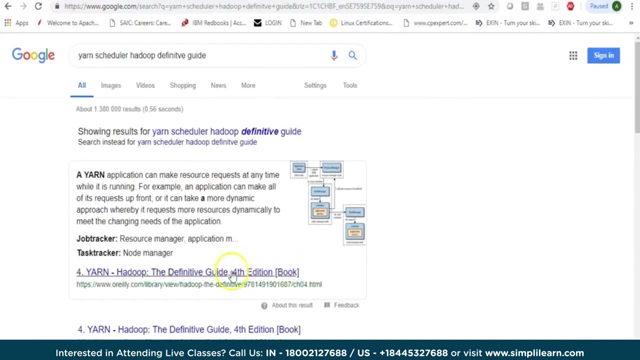 and different schedulers can be done, So you can always look at this series of blog. You can also be checking for YARN schedulers and then search for Hadoop Definitive Guide, and that could give you some information on how it looks when you look for Hadoop Definitive Guide. 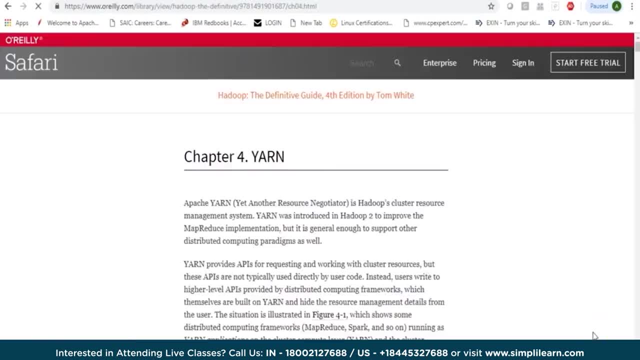 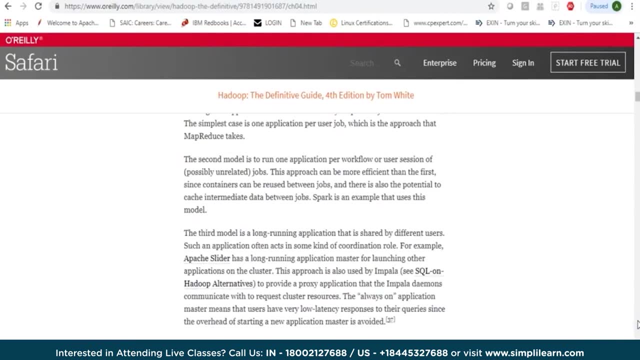 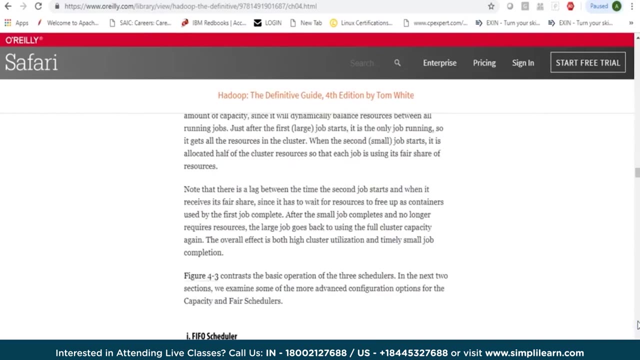 So if you look into this book which talks about the different resources, as I mentioned, so you could have a FIFO scheduler that is first in, first out, which basically means if a long running application is submitted to the cluster, all of the small running applications will have to wait. 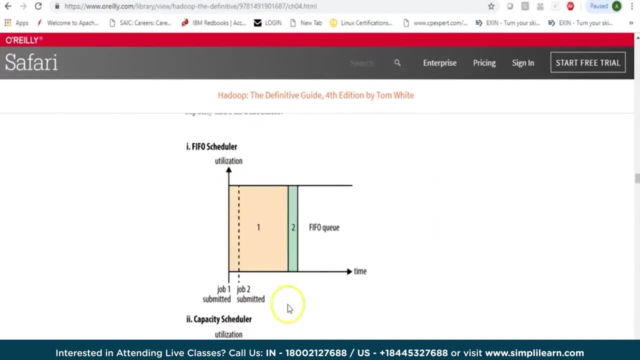 There is no other way, but that would not be a preferred option. if you look in FIFO scheduler, If you look for capacity scheduler, it basically means that you could have different queues created and those queues would have resources allocated, So then you could have a production queue. 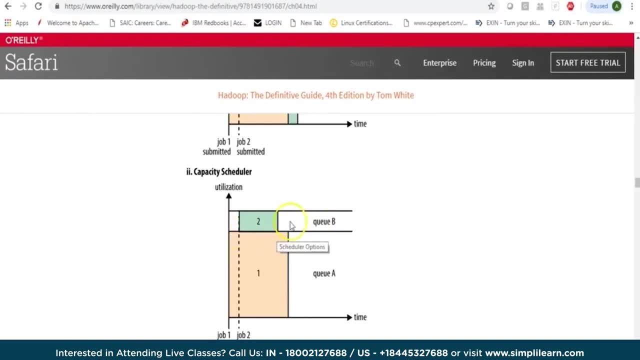 where production jobs are running in a particular queue which has fixed amount of resources allocated. you could have a development queue where development jobs are running and both of them are running in parallel. You could then also look into fair scheduler, which basically means again. 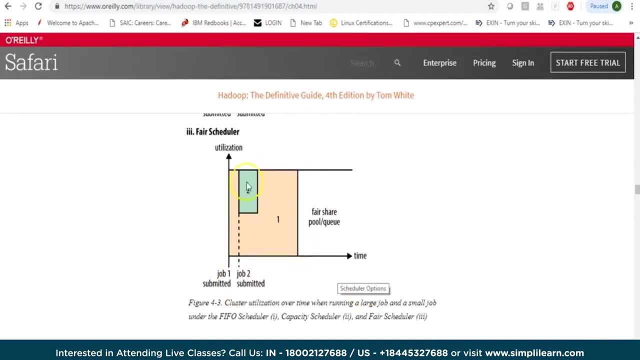 multiple applications could be running on the cluster. however, they would have a fair share. So when I say fair share in brief, what it means is if I had given 50% of resources to a queue for production and 50% of resources for a queue of development. 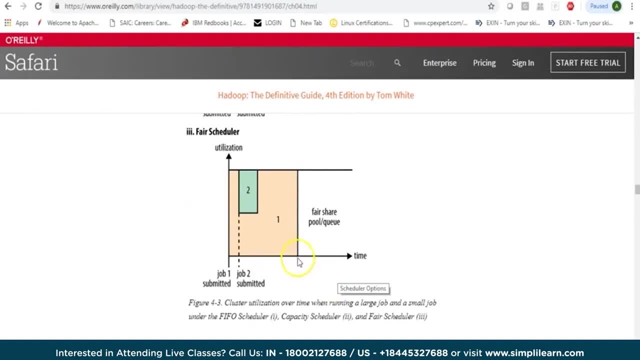 and if both of them are running in parallel, then they would have access to 50% of cluster resources. However, if one of the queue is unutilized, then second queue can utilize all cluster resources. So look into the fair scheduling part. 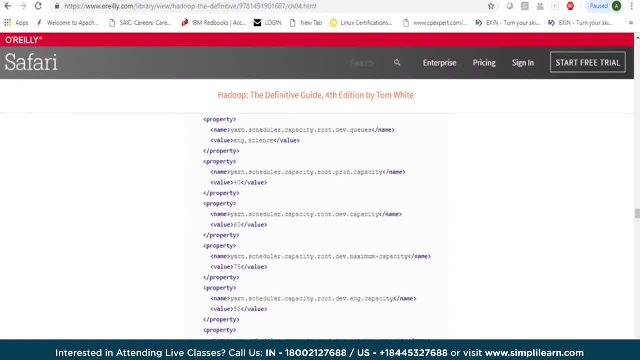 It also shows you about how allocations can be given, and you can learn more about schedulers and how queues can be used for managing multiple applications. Now we will spend some time in looking into few ways, or a few quick ways, to manage multiple applications. 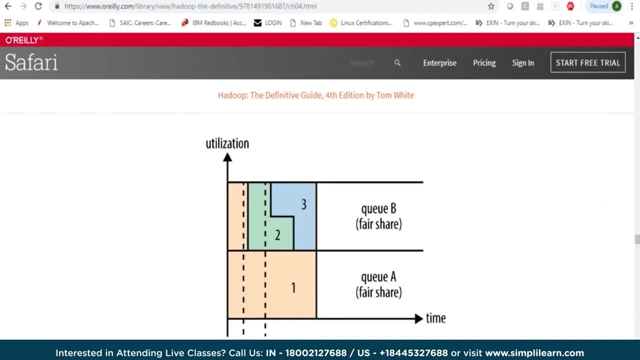 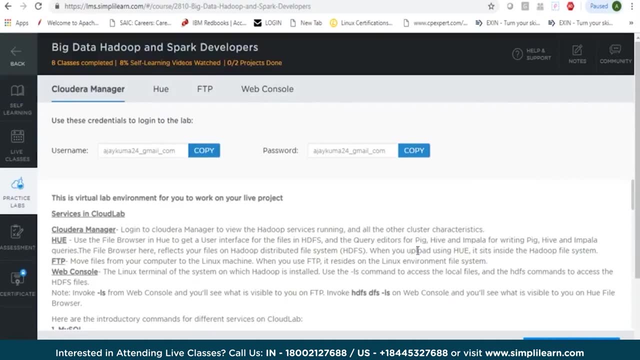 Now we will spend some time in looking into few ways, or a few quick ways, in interacting with YARN in the form of a demo To understand and learn on how YARN works. we can look into a particular cluster. Now here we have a designated cluster which can be used. 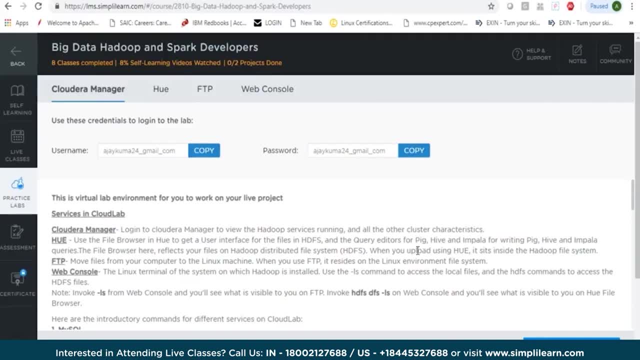 You could be using the similar kind of commands on your Apache-based cluster or a Cloudera Quickstart VM if you already have, or if you have a Cloudera or a Hortonworks cluster running. There are different ways in which we can interact with YARN. 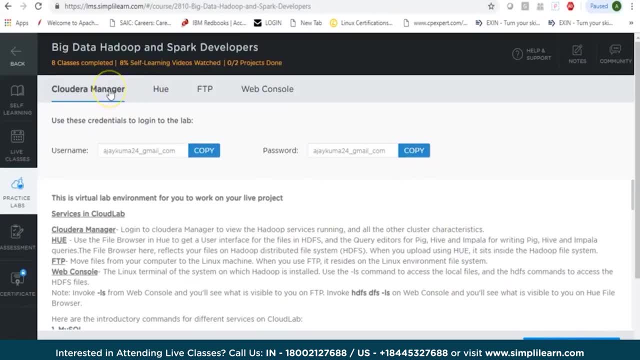 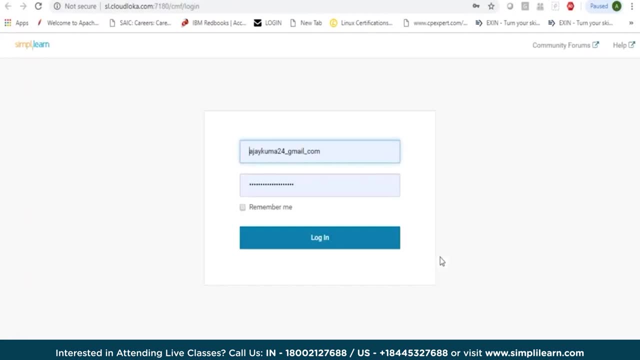 and we can look at the information. One is basically looking into the admin console. So if I would look into Cloudera Manager, which is basically an admin console for a Cloudera's distribution of Hadoop, Similarly you could have a Hortonworks cluster. 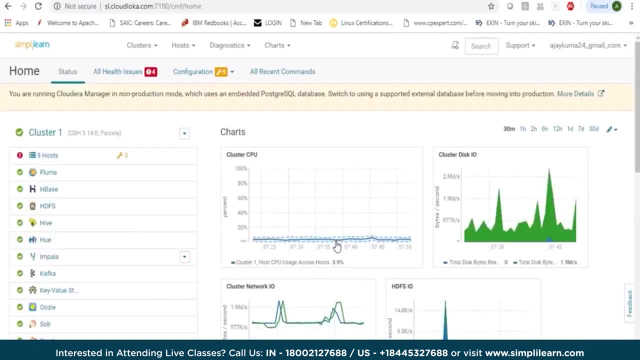 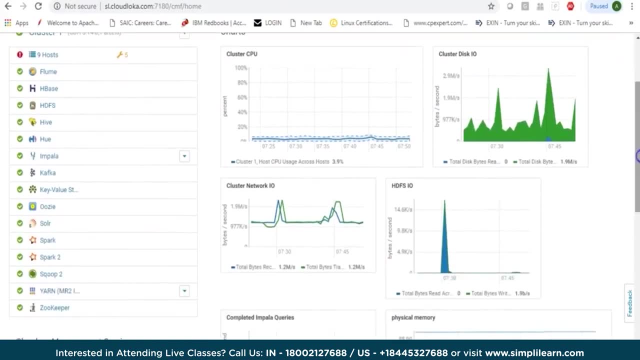 then access to the admin console. So if you have even read access for your cluster and if you have the admin console, then you can search for YARN as a service, which is running. You can click on YARN as a service and that's it. 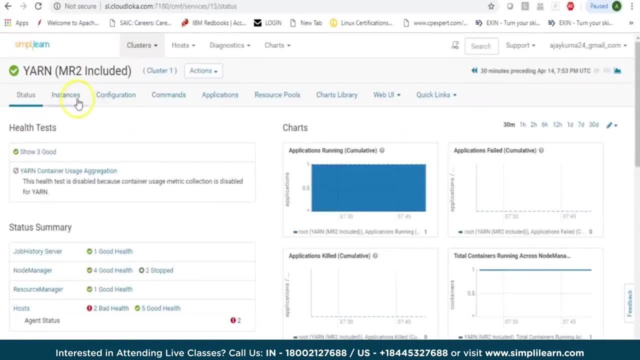 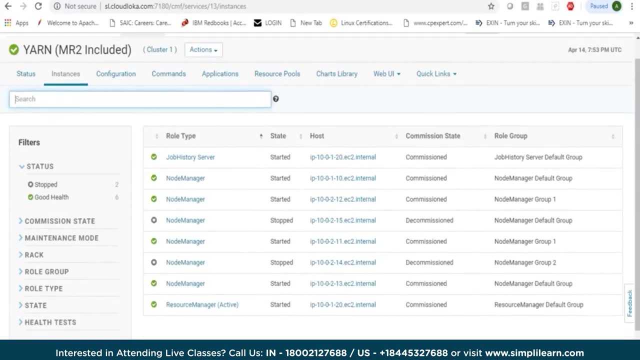 You can click on YARN as a service and that's it, And that gives you different tabs. So you have the instances, which tells basically what are the different roles for your YARN service running. So we have here multiple node managers. 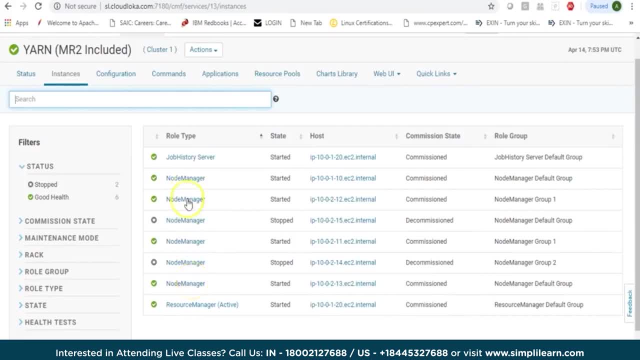 Now some of them show in stop status, but that's nothing to worry. So we have three and six node managers. We have resource manager, which is one, but then that can also be in a high availability where you can have active and standby. 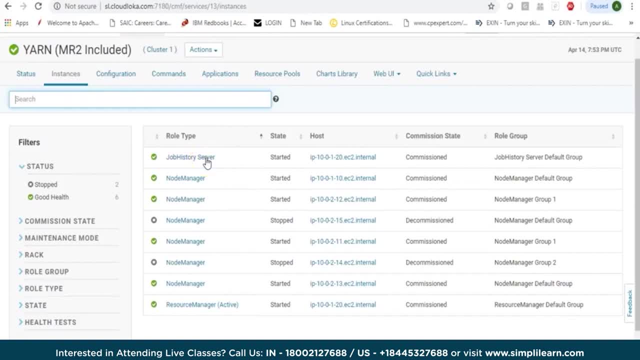 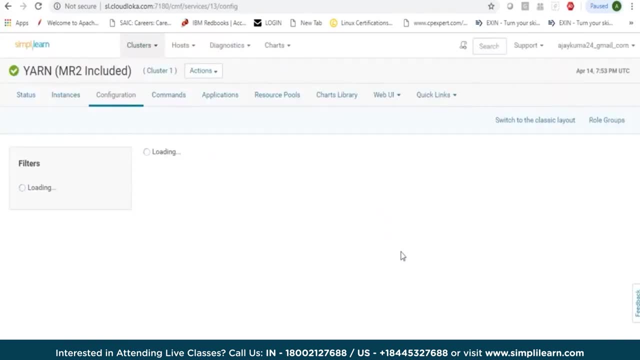 You also have a job history server which would show you the applications once they have completed. Now you can look at the YARN configurations And, as I was explaining, you can always look for the properties which are related to the allocation. So you can here search, for course. 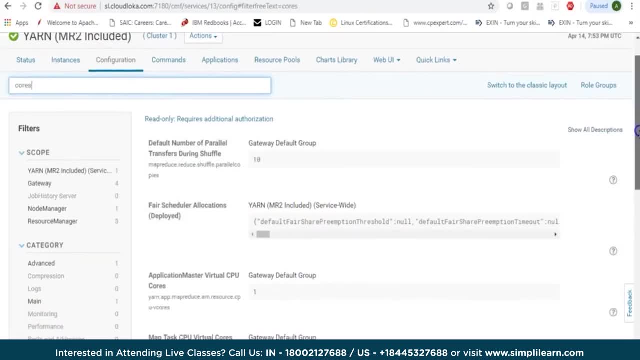 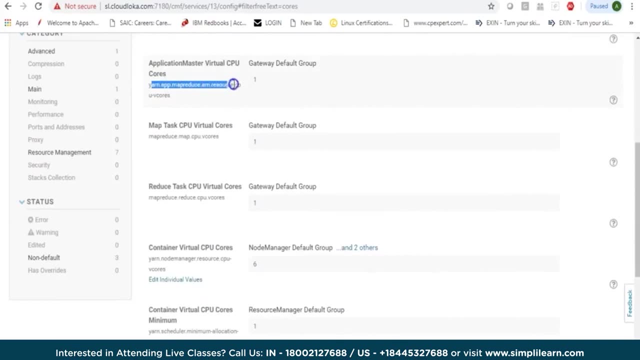 and that should show you the properties which talk about the allocations. So here, if we see, we can be looking for YARN app. MapReduce application master resource, CPU course. What is the CPU course allocation? This is allocated for MapReduce, MapTask, ReduceTask. 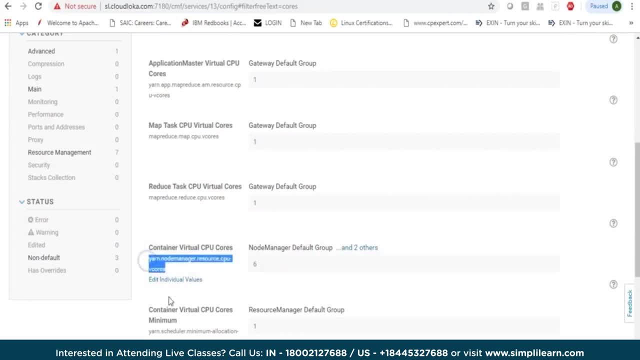 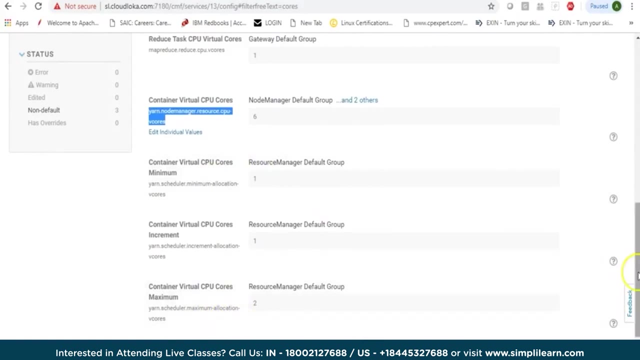 You can be looking at YARN node manager resource CPU course, which basically says every node manager on every node would be allocated with six CPU course And the container sizing is with minimum allocation of one CPU core and the maximum could be two CPU cores. 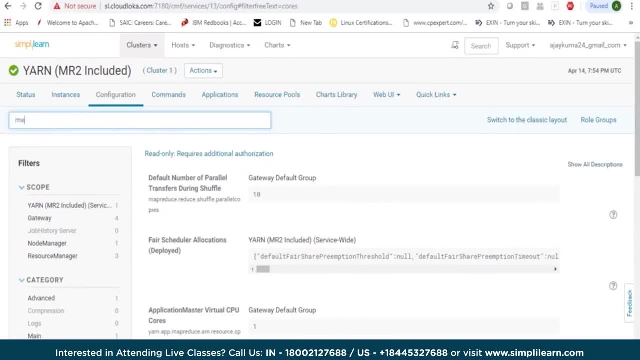 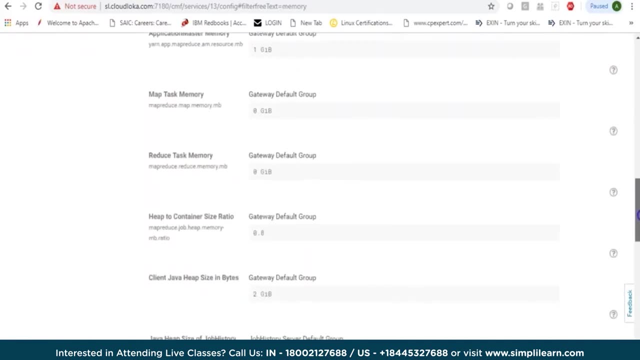 Similarly, you could also be searching for memory allocation, And here you could then scroll down to see what kind of CPU cores are allocated for each node manager, And you can see that this kind of memory allocation has been done for the node manager. 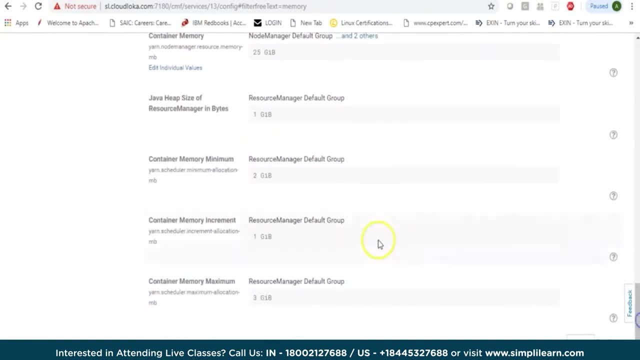 So, if we look further, it should give me information of node manager which basically says here that the container minimum allocation is 2 GB, the maximum is 3 GB And we can look at node manager which has been given 25 GB per node. 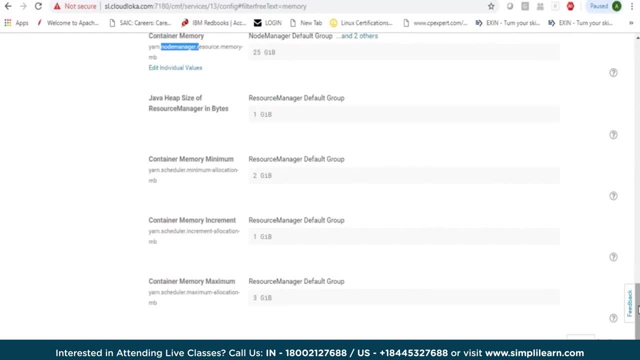 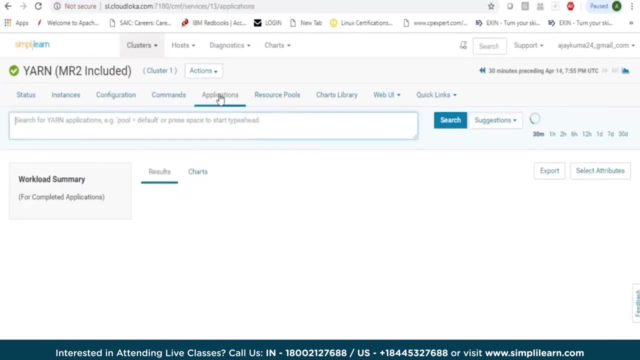 So it's a combination of this memory and CPU cores which is allocated to every node manager. Now we can always look into Applications tab. That would show us different applications which are submitted on YARN, For example. right now we see there. 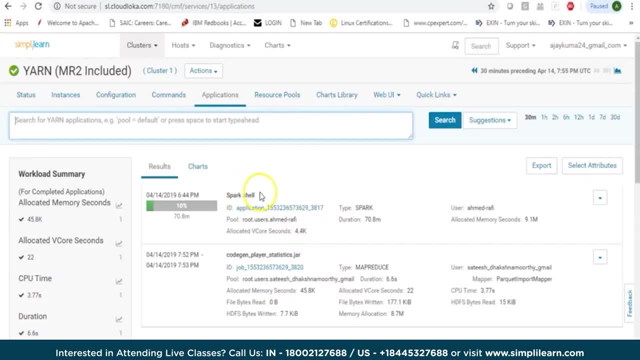 is a Spark application running, which is basically a user who is using Spark Shell, which has triggered a application on Spark and that is running on YARN. You can look at different applications workload information. You can always do a search based on the number of days. 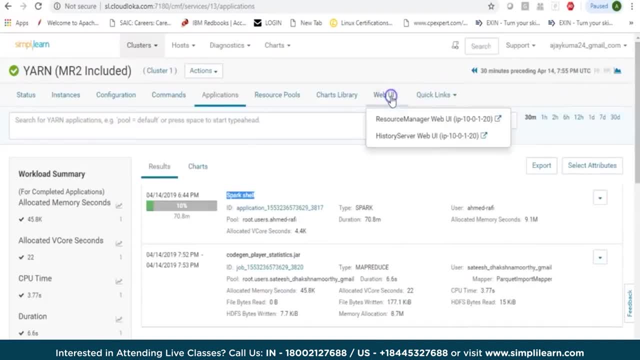 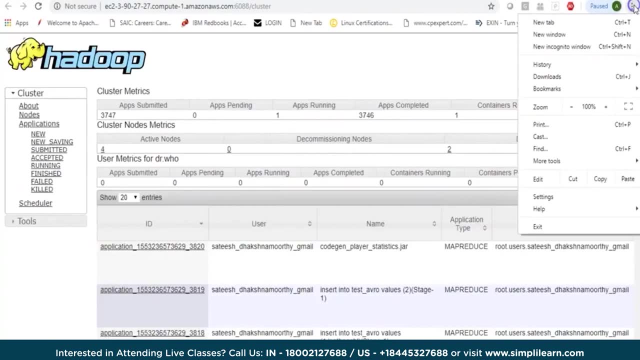 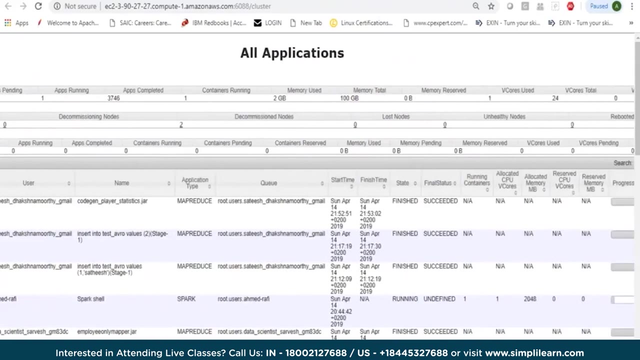 how many applications have run And so on. You can always go to the web UI and you can be searching for the resource manager web UI And if you have access to that, it will give you overall information of your cluster. So this basically says that here we have 100 GB memory. 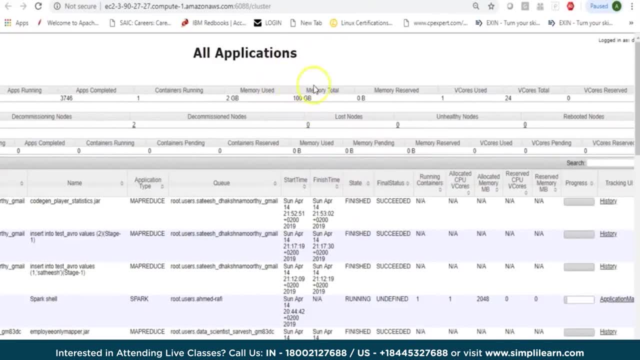 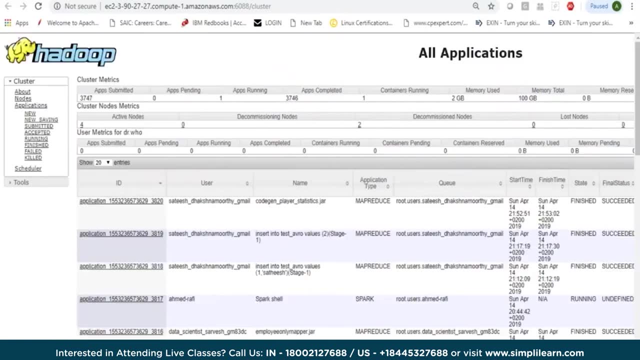 allocated, So that could be say 25 GB per node, And if we have 4 node managers running and we have 24 cores, which is 6 cores per node, If we look further here into node manager I could get more information. 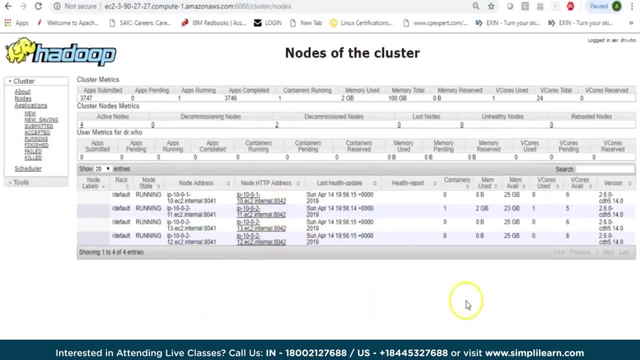 So this tells me that I have 4 node managers running, and node managers basically have 25 GB memory allocated per node and 6 cores out of which some portion is being utilized. We can always look at the scheduler here, which can give us information. what kind of scheduler? 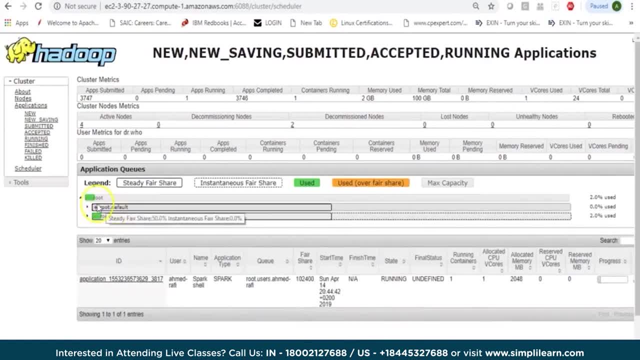 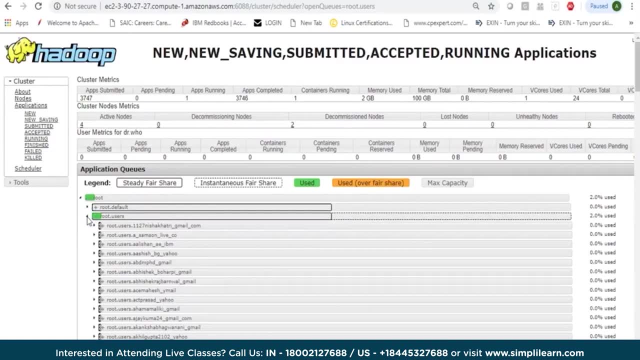 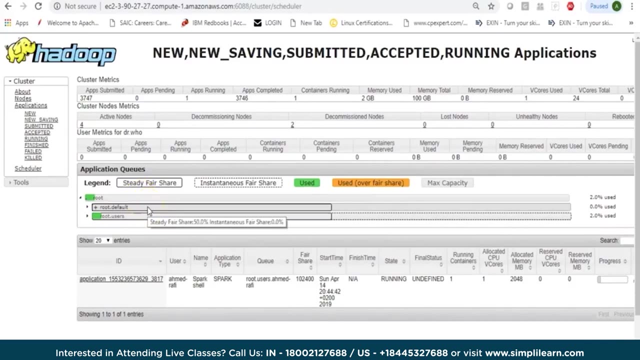 has been allocated. So we basically see that there is just a root queue and within root you have default queue and you have basically users queue based on different users. We can always scroll here and that can give us information, if it is a fair share. 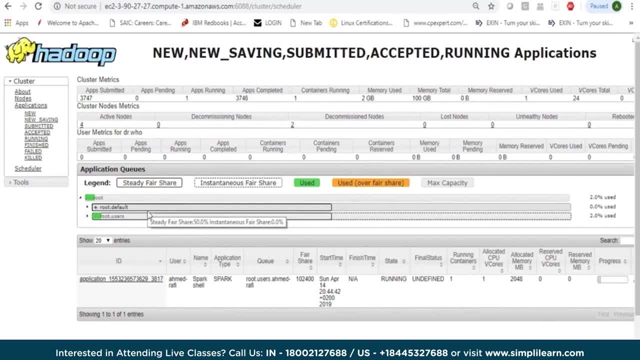 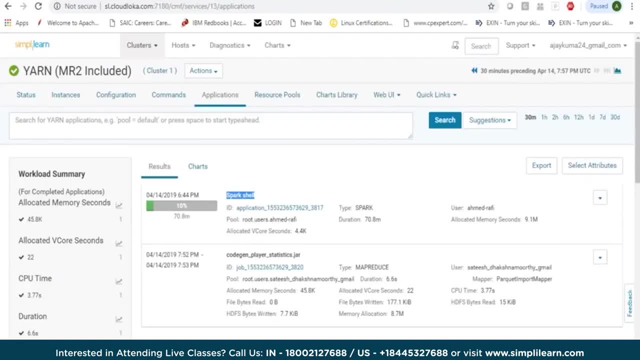 So here we see that my root dot default has 50% of resources and the other queue also has 50% of resources, which also gives me an idea that a fair scheduler is being used. We can always confirm that if we are using a fair scheduler. 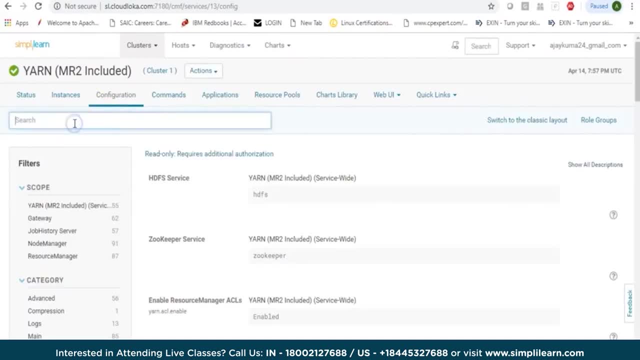 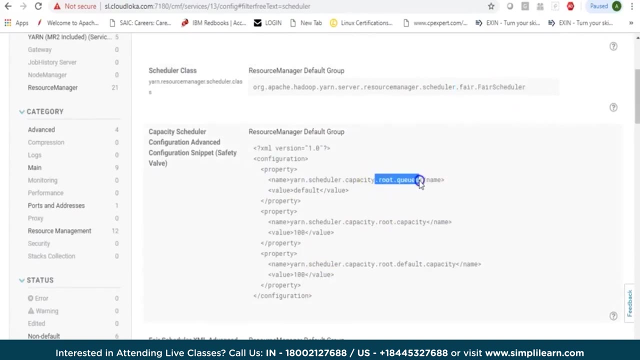 or a capacity scheduler which takes care of allocation. So search for scheduler And that should give you some understanding of what kind of scheduler is being used and what are the allocations given for that particular scheduler. So here we have fair scheduler. It shows me you have under root, you have the root queue. 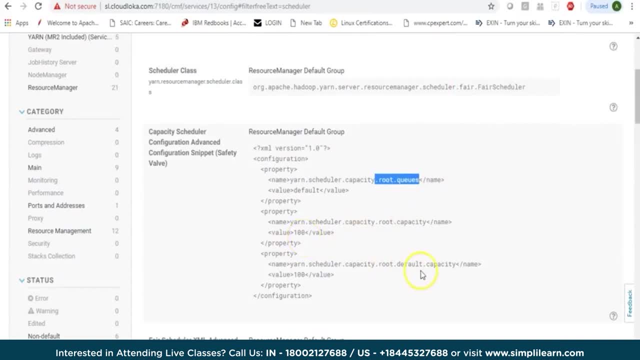 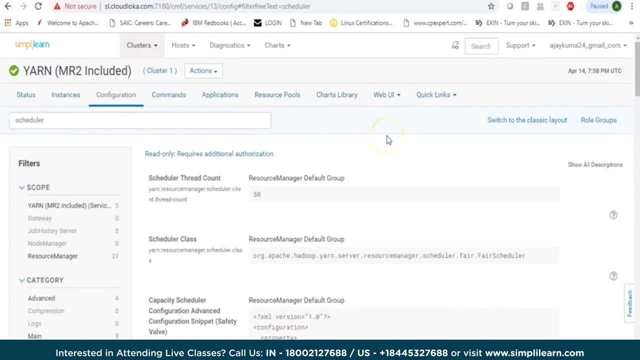 which has been given 100% capacity, and then you have within that default, which also takes 100%. So this is how you can understand about YARN. by looking into the YARN web UI, You can be looking into the configurations, You can look at applications. 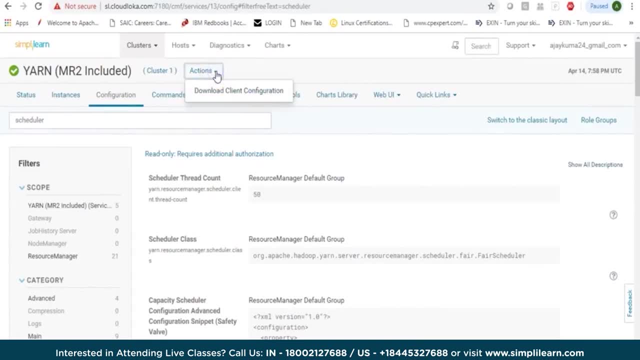 You can always look at different actions. Now, since we do not have admin access, the only information we have is to download the client configuration. We can always look at the history server, which can give us information of all the applications which have successfully completed. 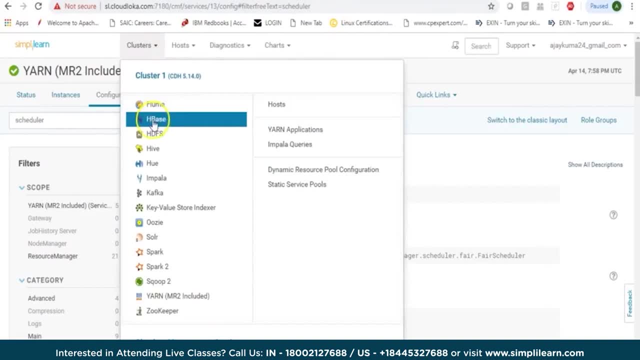 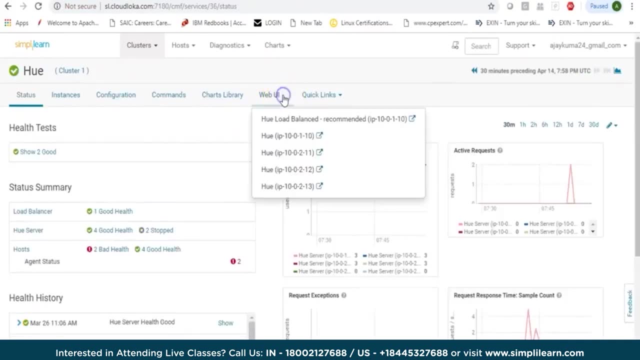 Now, this is from your YARN UI. What I can also do is I can be going into Hue, which is the web interface, and your web interface also basically allows you to look into the jobs, So you can click on Hue web UI. 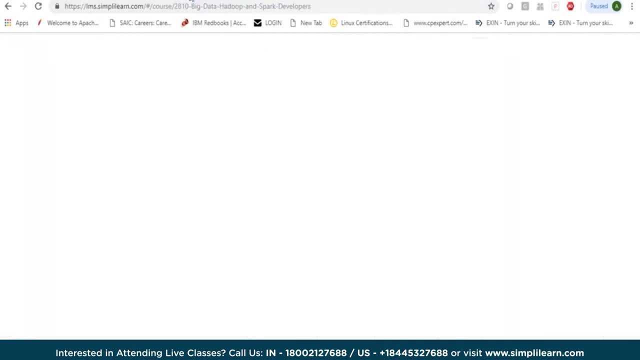 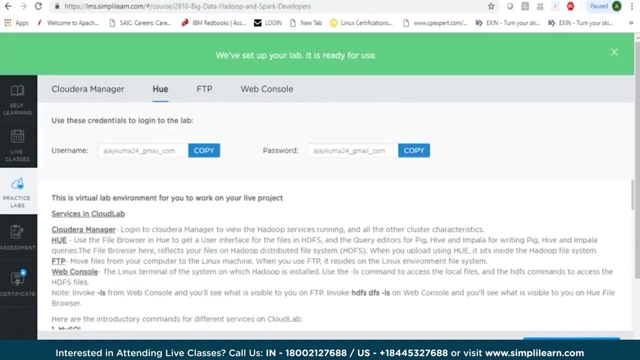 and if you have access to that, it should show up or you should have a way to get to your Hue, which is a graphical user interface. mainly comes with your cloud error. You can also configure that with Apache. Hortonworks has a different way of giving you the web UI access. 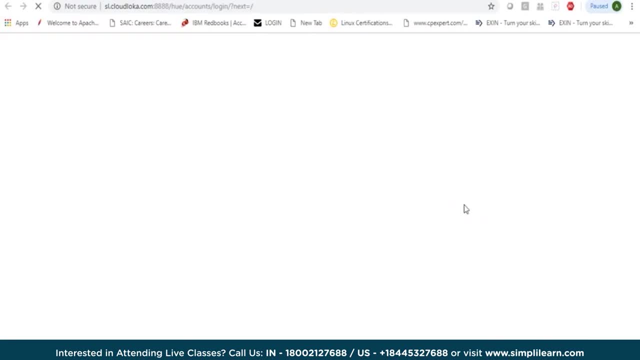 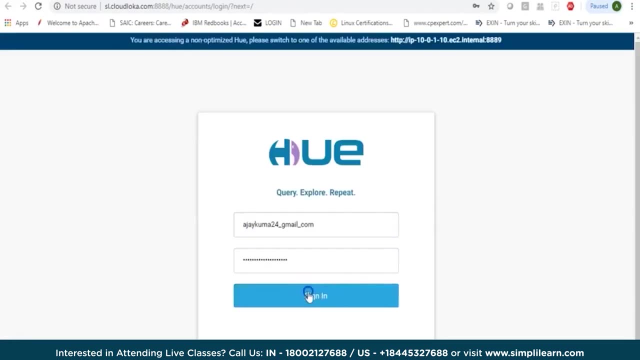 You can click and get into Hue and that is also one way where you can look at YARN. You can look at the jobs which are running, if there are some issues with it, and these are your web interfaces. So either you look from YARN web UI. 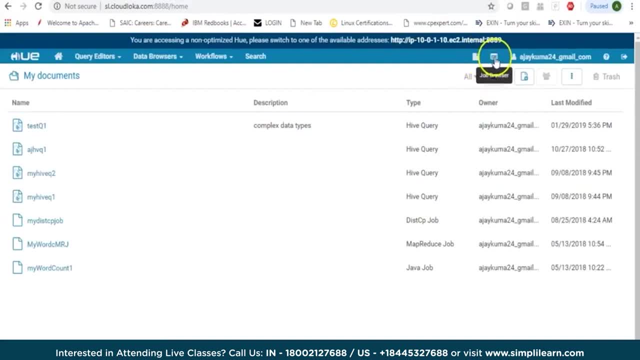 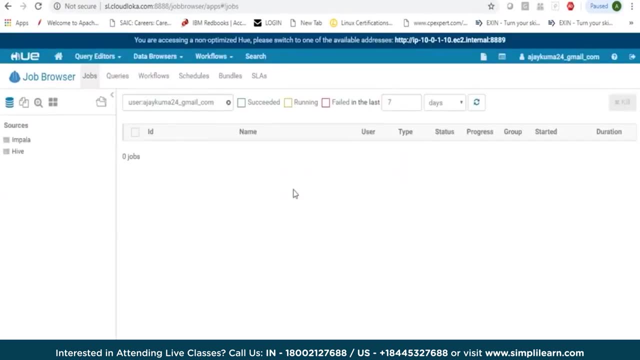 or here in Hue, you have something called a job browser which can also give you information of your different applications which might have run. So here I can just remove this one, which would basically give me a list of all the different kinds of jobs or workloads which were run. 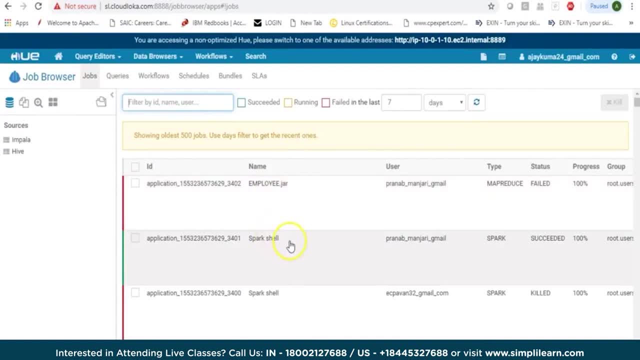 So either it was a Spark-based application, or it was a MapReduce, or it was coming from Apache. So here I have a list of all the applications and it says this was a MapReduce, this was a Spark, something was skilled. 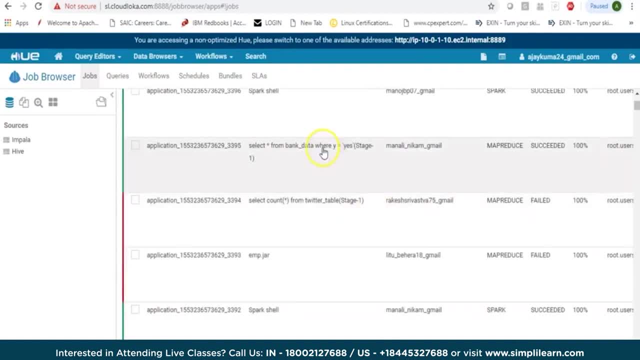 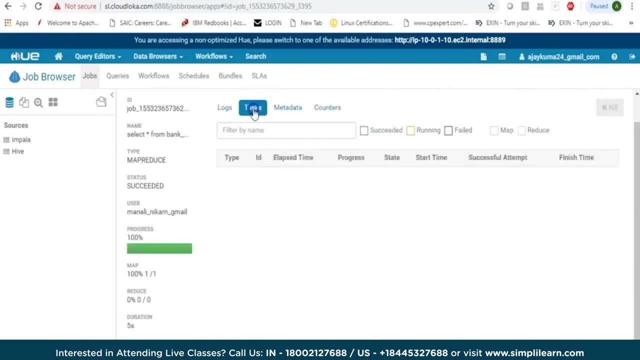 something was successful and this was basically probably a Hive query which triggered a MapReduce job. You can click on the application and that tells you how many tasks were run for it, So there was a map task which ran for it. You can get into the metadata information. 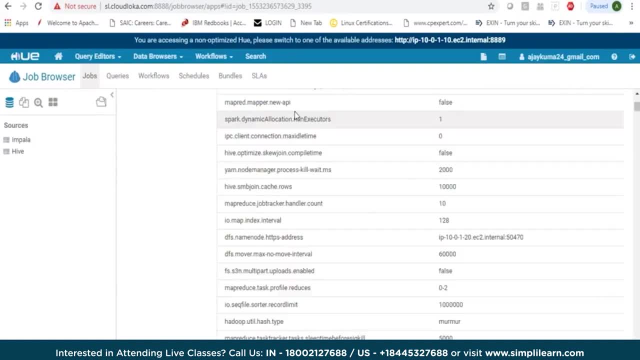 which obviously you can also look from the YARN UI to look into your application, Which can give you a detailed information of: if it was a MapReduce, how many map and reduce tasks were run, what were the different counters. If it was a Spark application, 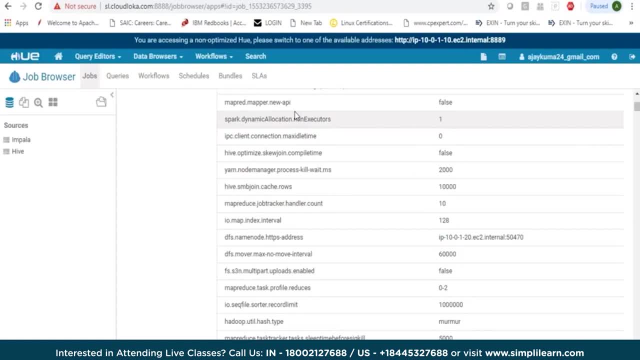 it can let you follow through Spark history server or job history server So you can always use the web UI to look into the jobs. You can be finding a lot of useful information here. You can also be looking at how many resources were used. 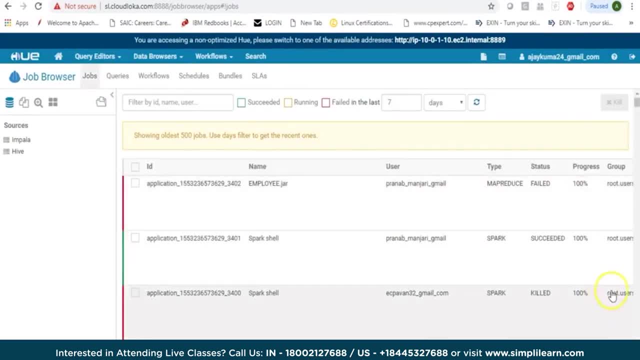 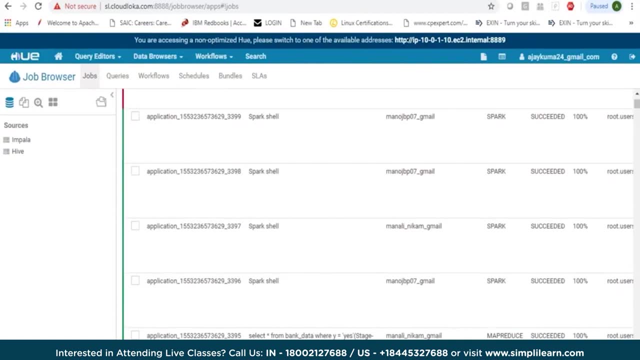 and what happened to the job. was it successful, did it fail? and what was the job status Now, apart from web UI, which always you might not have access to. So in a particular cluster, in a production cluster, there might be restrictions. 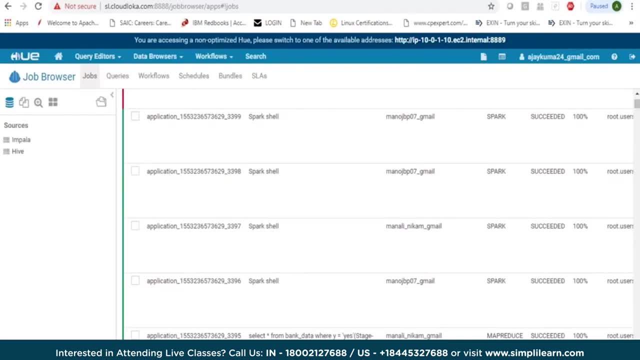 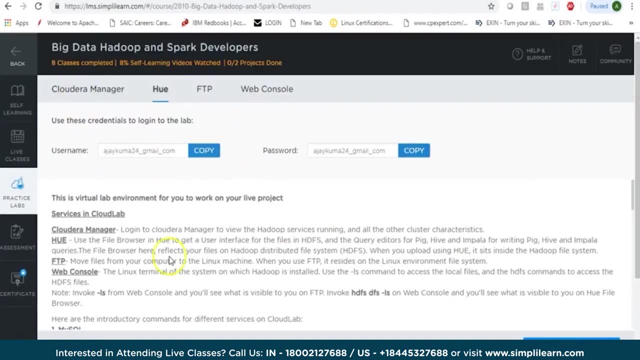 and the organization might not have access- given to all the users- to graphical user interface. like you, Or might be you would not have access to the cloud data manager or admin console because probably organization is managing multiple clusters using this admin console. So the one way 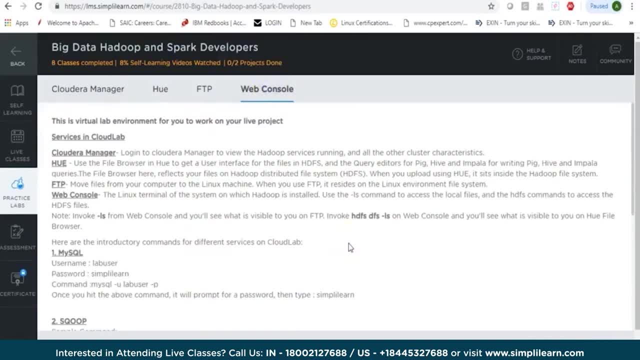 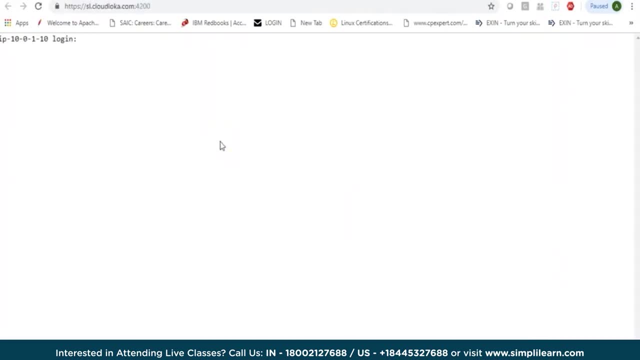 which you would have access is your web console or basically your edge node or client machine, from where you can connect to the cluster and then you can be working. So let's log in here and now. here we can give different commands. So this is the command line. 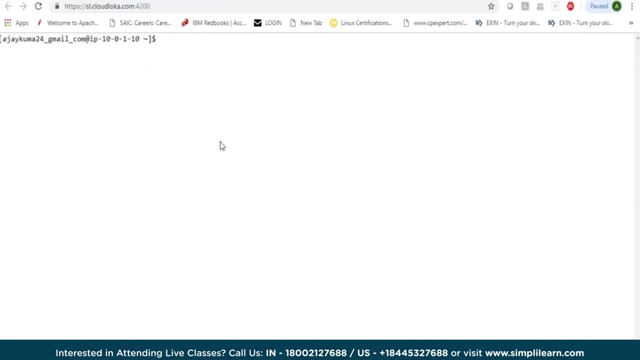 from where you can have access to different details. You can always check by just typing in MapRed, which gives you different options where you can look at the MapReduce related jobs. you can look at different queues, if there are queues configured. you can look at the history server. 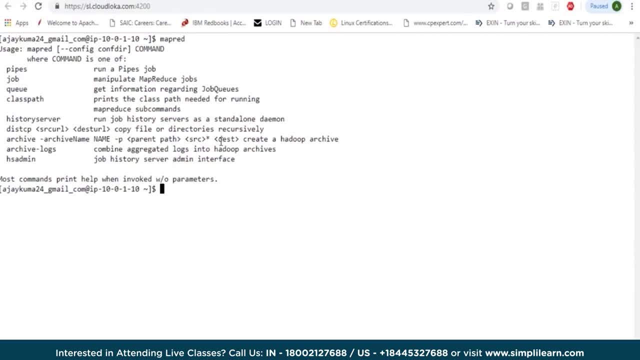 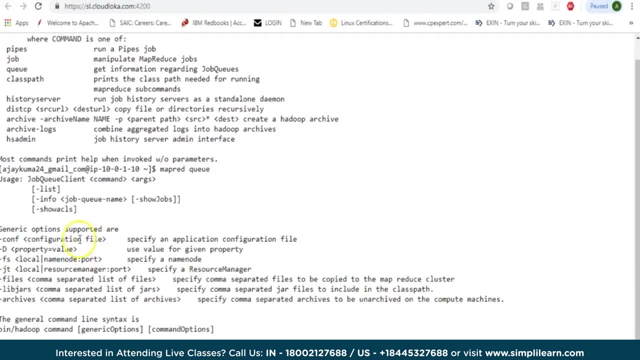 or you can also be doing some admin stuff, provided you have access. So, for example, if I just say MapRed and queue here, this basically gives me an option. says: what would you want to do? Would you want to list all the queues? 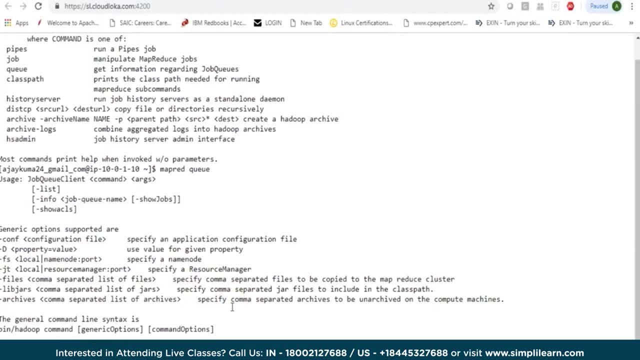 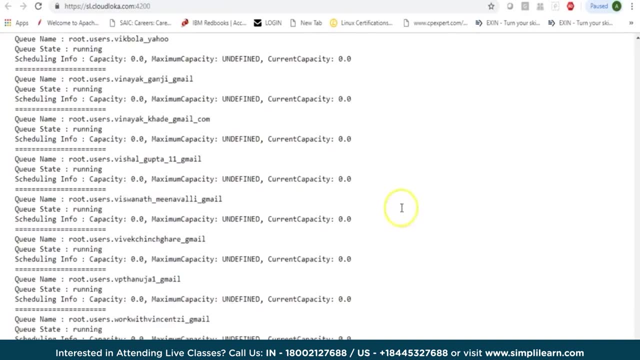 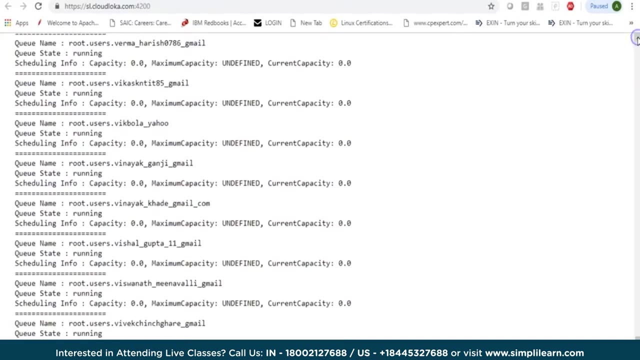 Do you want information on a particular queue? So let's try a list, and that should give you different queues which were being used. Now here we know that per user, a queue dynamically gets created, which is under rootusers, and that gives me what is the status of the queue. 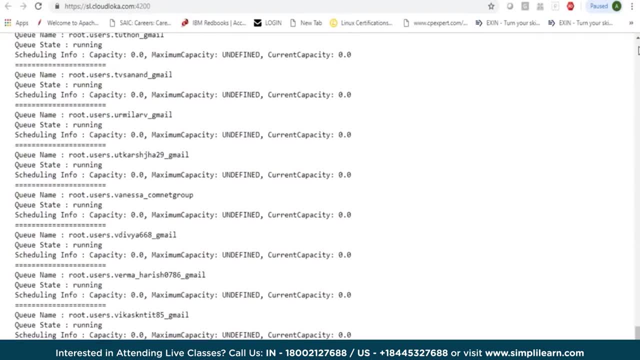 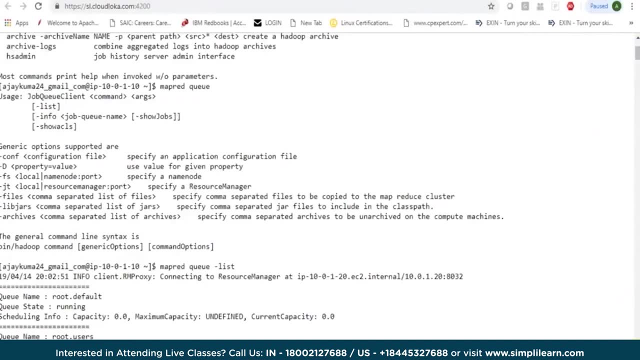 What is the capacity? Has there been any kind of maximum capacity or capping done? So we get to see a huge list of queues which dynamically get configured in this environment, and then you also look at your rootdefault. I could have also picked up. 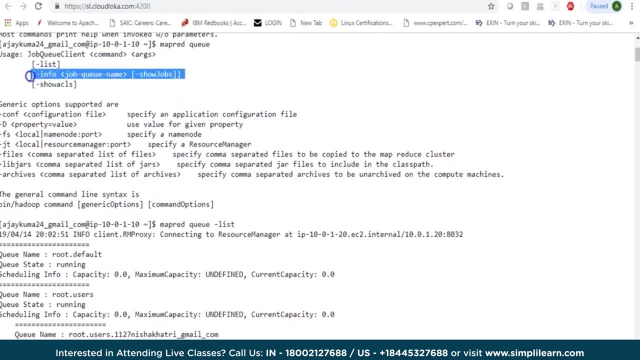 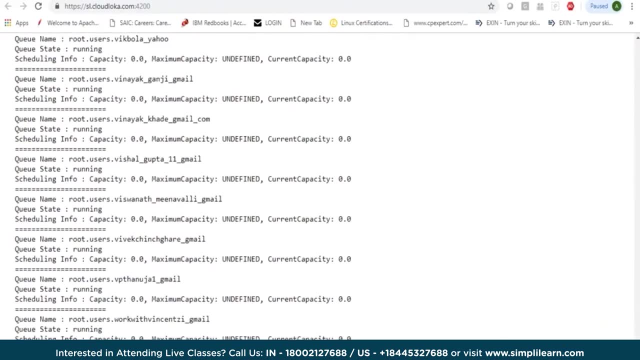 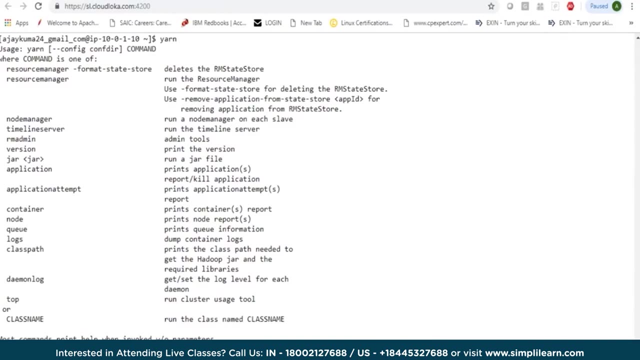 one particular queue and I could have said: show me the jobs. So I could do that. Now here we can also give a yarn command. So let me just clear the screen and I will say yarn, and that shows me different options. So, apart from your web interface, 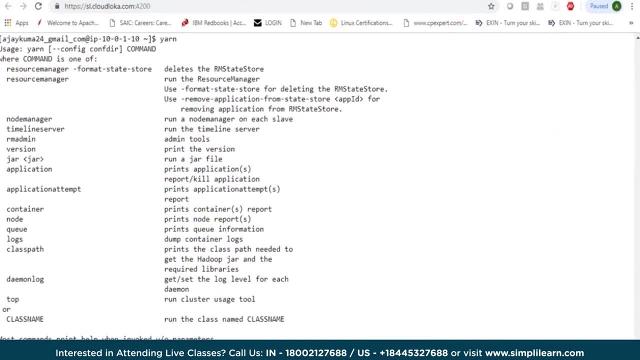 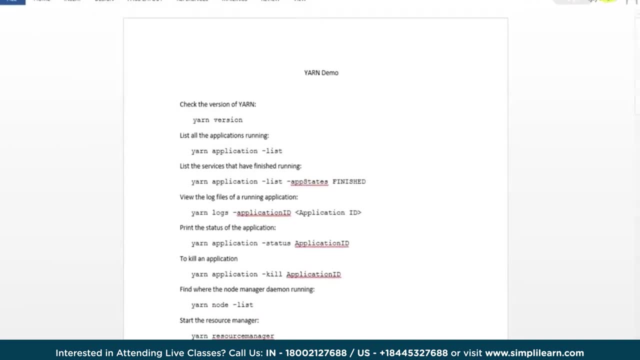 something like web UI. apart from your yarns web UI, you could also be looking for information using yarn commands here. So these are some list of commands which we can check. Now you can just type in yarn and version if you would want to see the version. 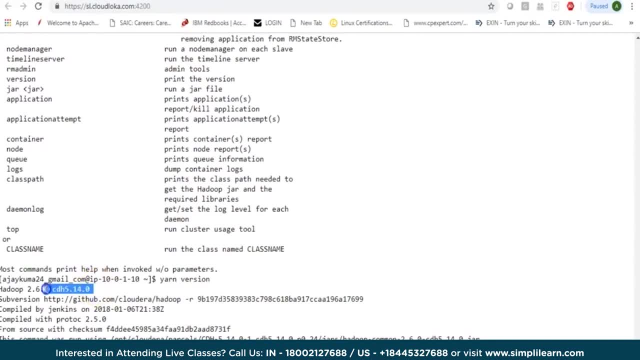 which basically gives you information of what is the Hadoop version being used and what is the vendor specific distribution version. So here we see: we are working on Cloudera's distribution 5.14, which is internally using Hadoop 2.6.. 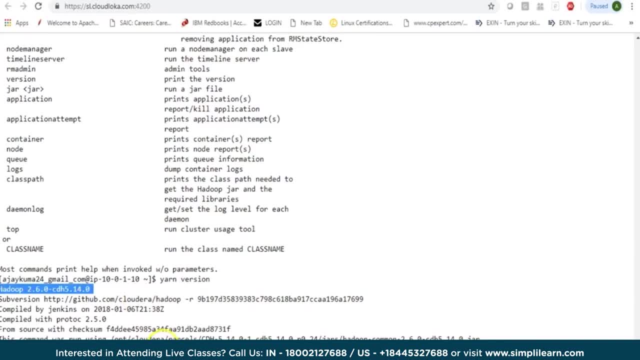 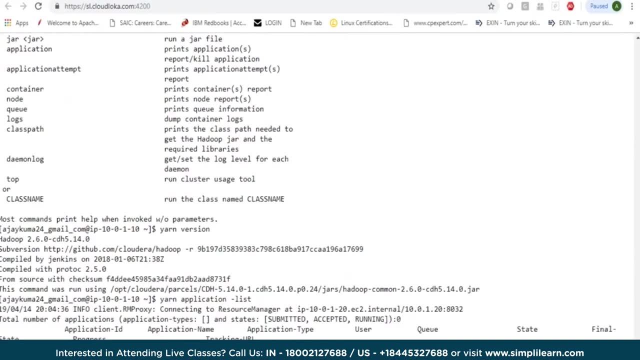 Now, similarly, you can be doing a yarn application list. So if you give this, that could be an exhaustive list of all the applications which are running or applications which have completed. So here we don't see any applications because right now probably there are no applications. 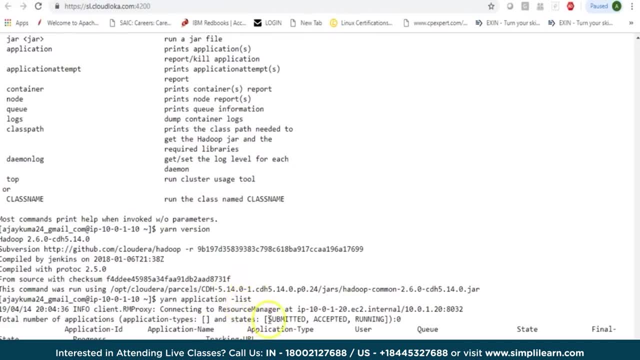 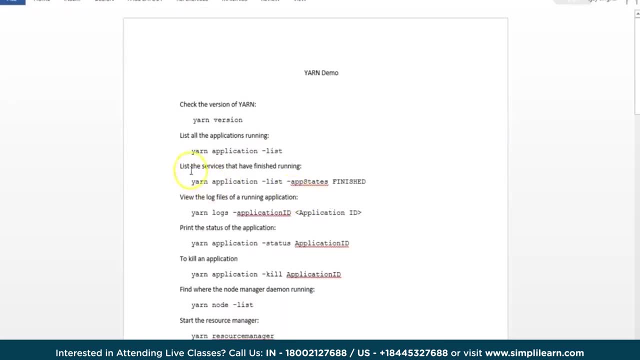 which are running. It also shows you you could be pulling out different status, such as submitted, accepted or running. Now you could also say: I would want to see the services that have finished running. So I could say: yarn application list and app states as finished. 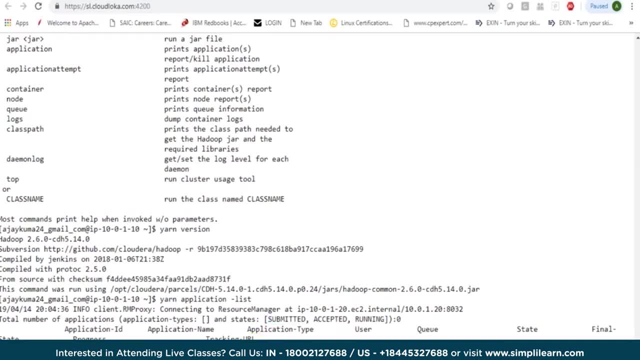 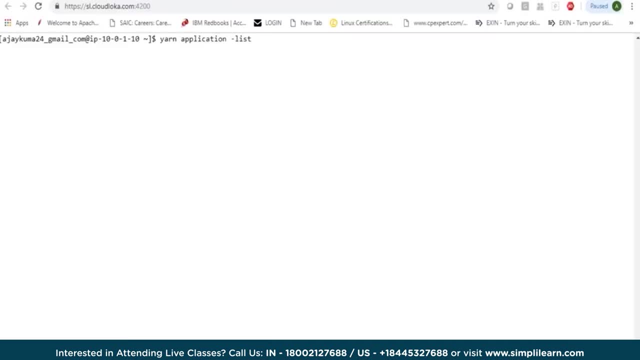 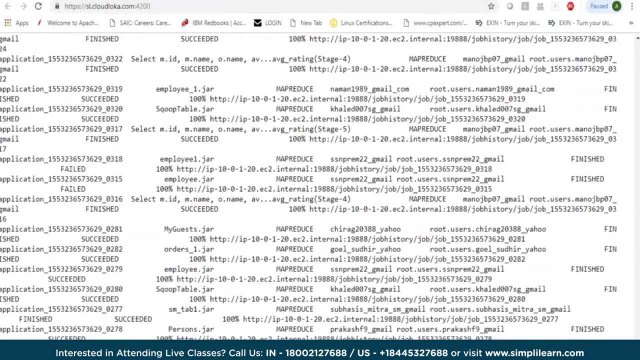 So here we could be using our command So I could say: yarn, application list, and then I would want to see the app states which gives me the applications which have finished, and we would want to list all the applications which finished. Now that might be applications. 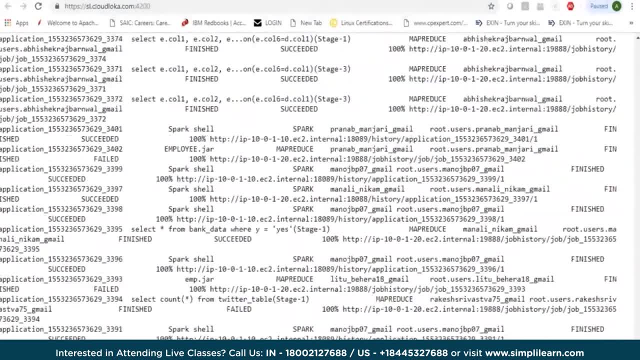 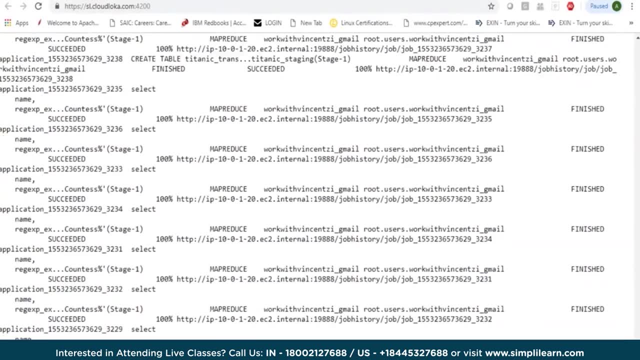 which succeeded right, And there is a huge list of application which is coming in from the history server, which is basically showing you the huge list of applications which have completed. So this is one way, and then you could also be searching for one particular application. 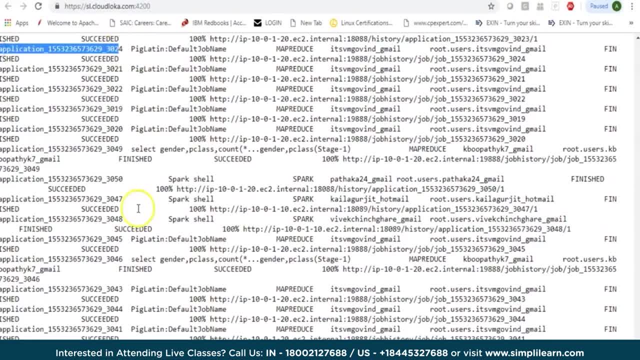 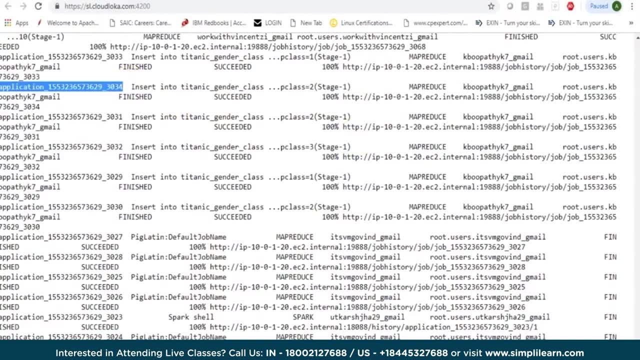 If you would want to search a particular application, if you have the application ID, you could always be doing a grep. That's a simple way I could say: basically, let's pick up this one, and if I would want to search for this, if I would want more details on this, 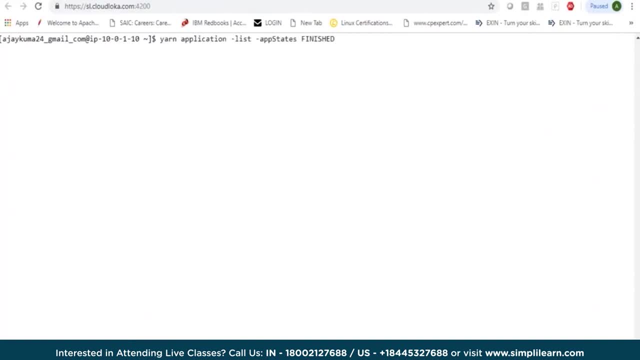 I could obviously do that by calling in my previous command and you could do a grep. if that's what you want to do And if you would want to search, is there any application which is in the list of my applications that shows my application? I could pull out more information. 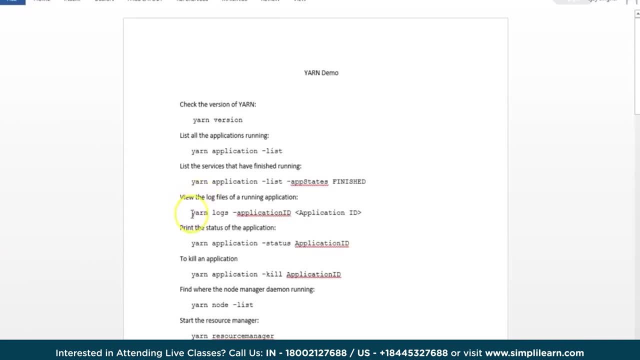 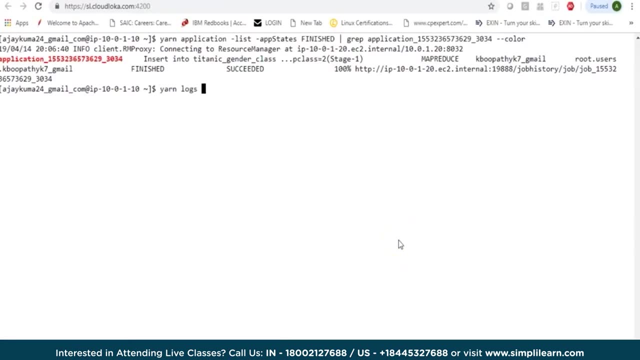 about my application. So I could look at the log files for a particular application by giving the application ID. So I could say: yarn logs. Now that's an option and every time, anytime you have a doubt, just hit enter. It will always give you options. 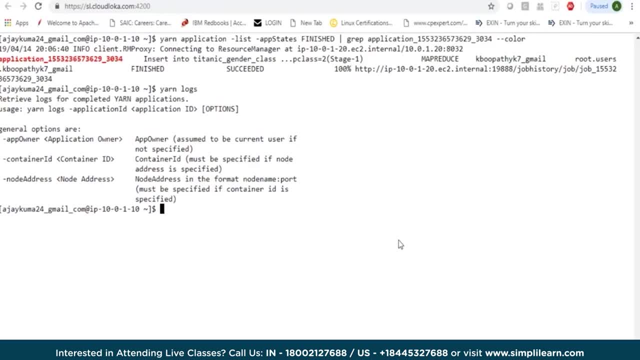 what you need to give with a particular command. So I can say yarn logs application ID. Now we copied an application ID and we could just give it here. We could give other options like app owner or if you would want to get into the container. 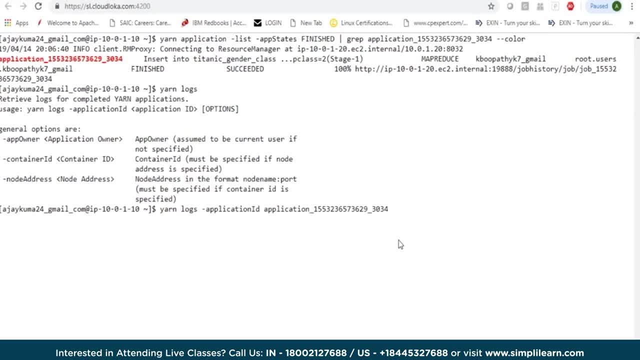 details or if you would want to check on a particular node. Now here I'm giving yarn logs and then I'm pointing it to an application ID and it says the log aggregation has not completed. Might be this was an application which was triggered based on. 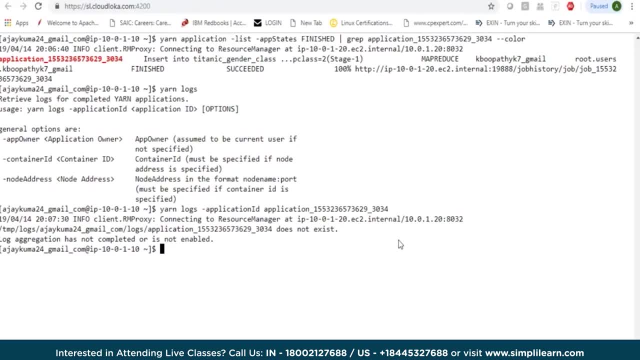 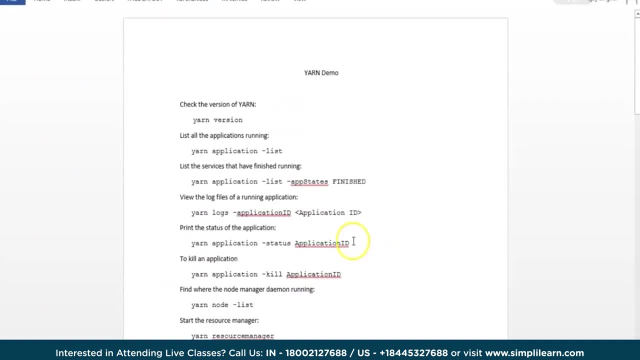 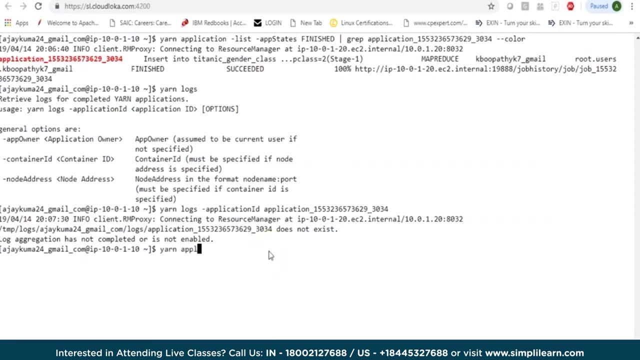 a particular interactive shell or based on a particular query. So there is no log existing for this particular application. You can always look at the status of an application. You can kill an application, So here you can be saying yarn, yarn, application, and then what would you want to do? 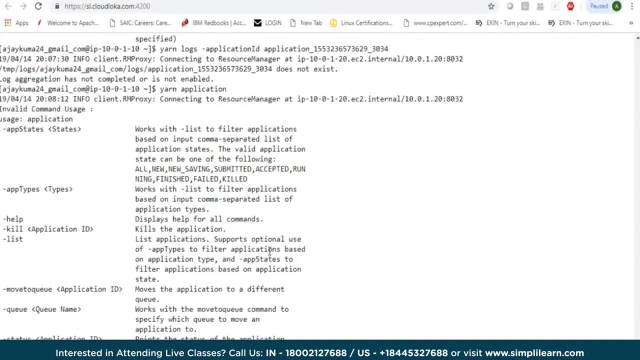 with an application, Hit an enter. It shows you the different options. So we just tried app states. You could always look at the last one which says status, and then for my status I could be giving my application ID, So that tells me what is the status of this application. 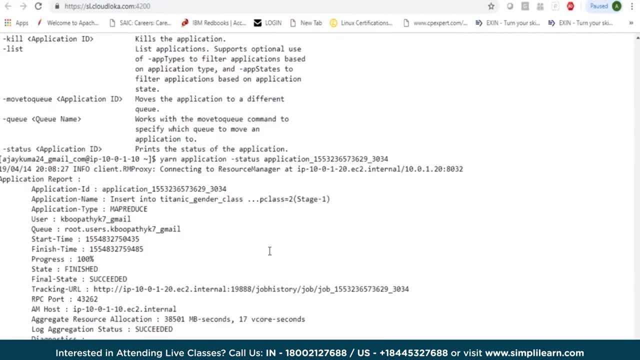 It connects to the resource manager. It tells me what's the application ID, what kind of application it was, who ran it, which was the queue, where the job was running, what was the start and end time. what is the progress? 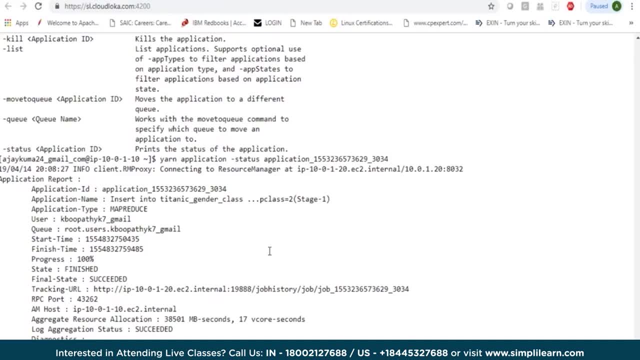 the status of it, if it is finished or if it has succeeded, and then it basically gives me also an information of where the application master was running. It gives me the information where you can find this job details in history server if you are interested in looking into. 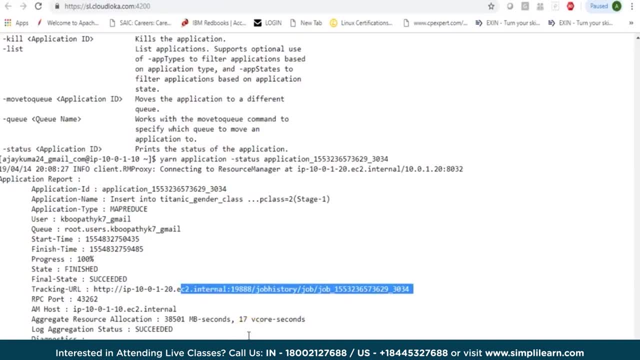 It also gives you an aggregate resource allocation which tells how much you have which GB memory and how many core seconds it used. So this is basically looking out at the application details. Now I could kill an application if the application was already running. I could always do a yarn application. 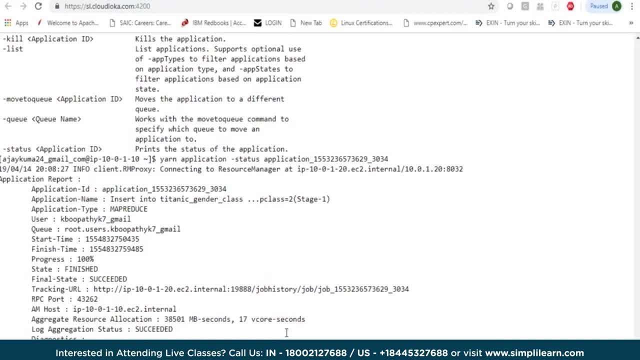 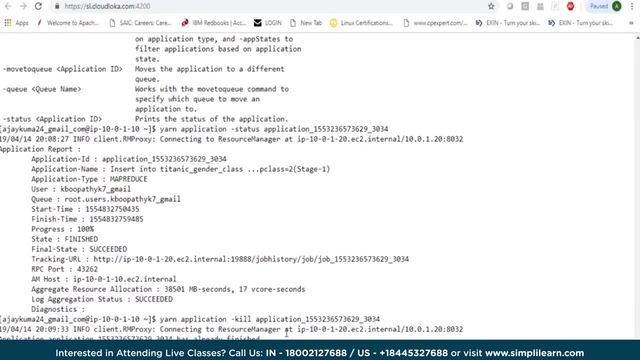 minus kill and then I could be giving my application. Now I could try killing this, however, it would say the application is already finished. If I had an application running and if my application was already given an application ID by resource manager, I could just kill it. 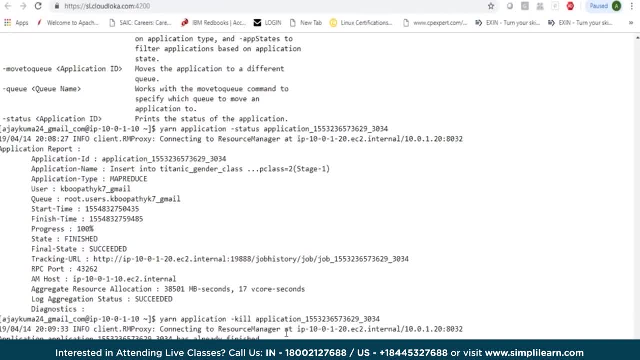 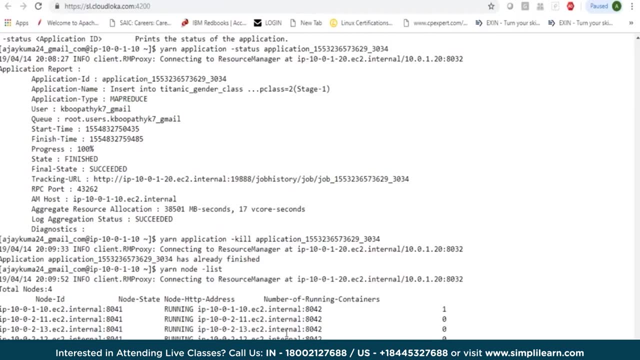 I can also say yarn node list, which would give me a list of the node managers. Now, this is what we were looking from, the yarn web UI, and we were pulling out the information so we can get this kind of information from your command line. Always remember. 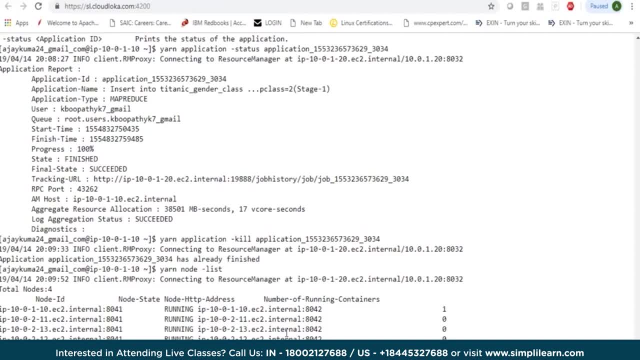 and always try to be well accustomed with the command line so you can do various things from the command line. and then, obviously, you have the web UIs, which can help you with a graphical interface easily able to access things. Now you could be also starting the resource manager. 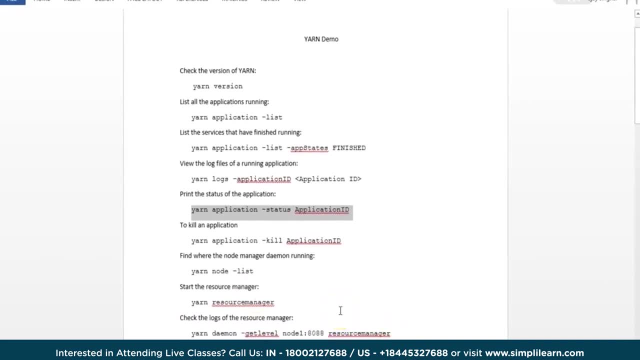 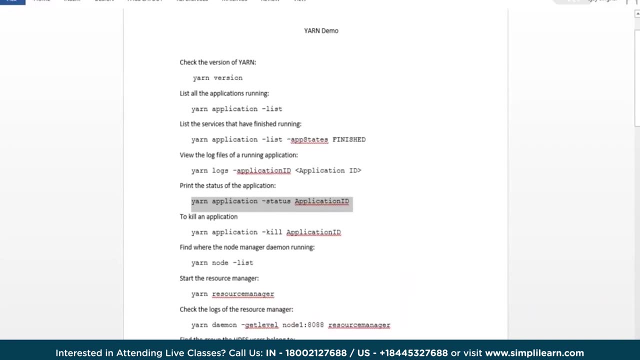 which we would not be doing here because we are already running in a cluster. So you could give a yarn resource manager. You could get the logs of resource manager, if you would want, by giving yarn daemon. So we can try that. So you can say yarn. 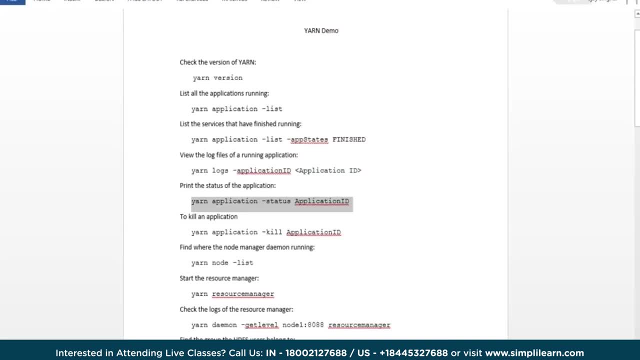 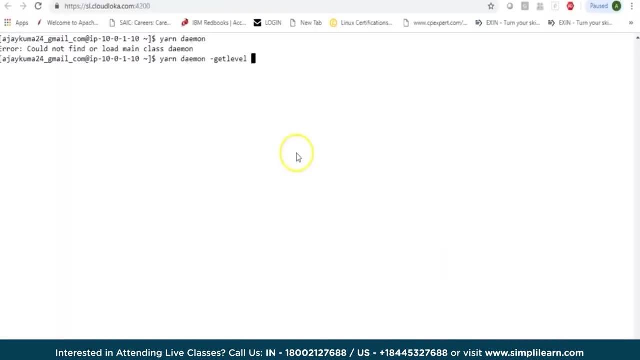 and then daemon, So it says it does not find the daemon. So you can give something like this: get level. and here I will have to give the node and the IP address where you want to check the logs of resource manager. So you could be giving this. 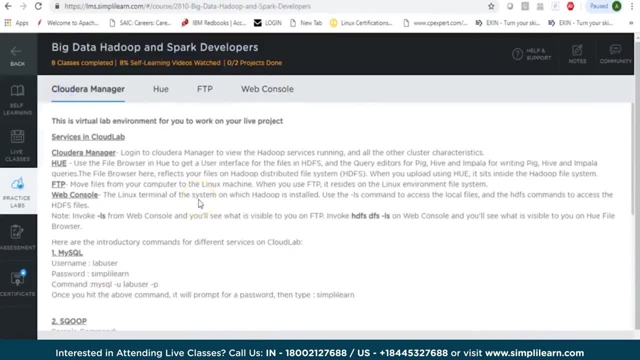 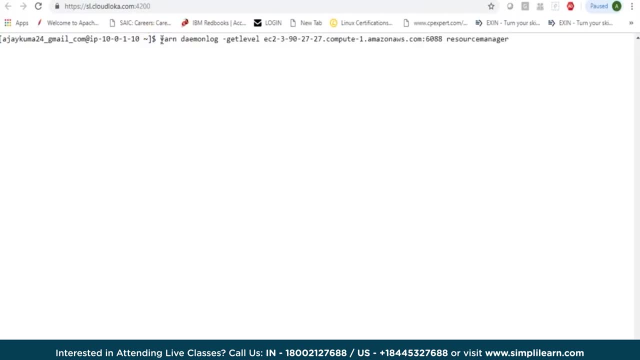 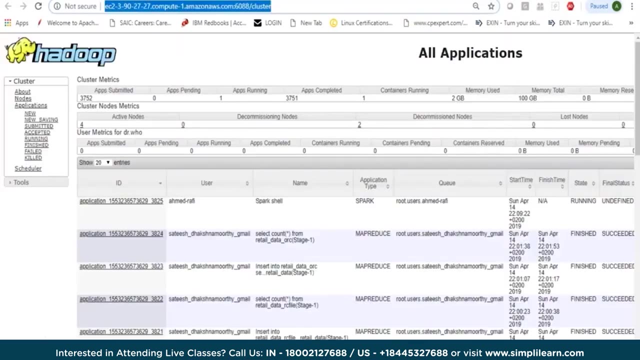 for which we will have to then get into cloud data manager to look into the nodes and the IP address. You could be giving a command, something like this, which basically gives you the level of the log which you have, and I got this resource manager address from the web UI. 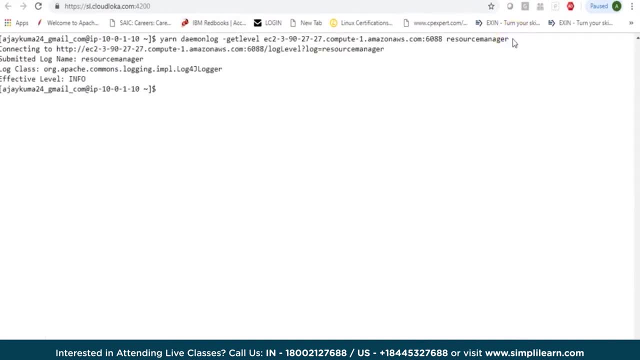 Now I can be giving in this command to look into the daemon log and it basically says you would want to look at the resource manager related log and you have the log4j which is being used for logging The kind of level which has been set as info. 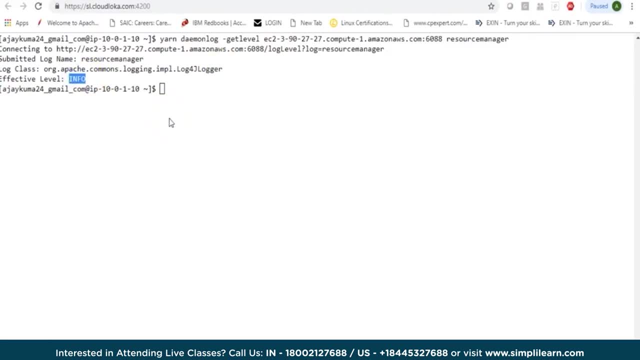 which can again be changed in the way you are logging the information. Now you can try any other commands, also from yarn, For example looking at the yarn rmedmin. So you can always do a yarn rmedmin and this basically gives you a lot of other information. 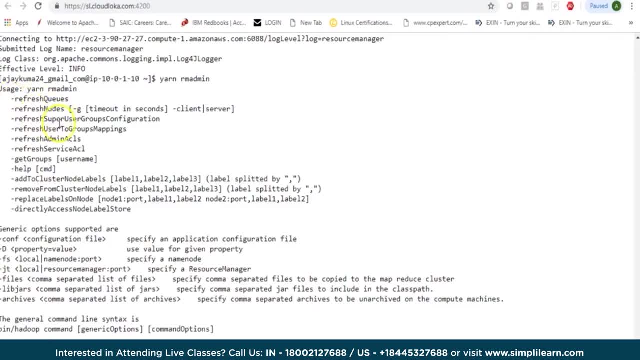 like refreshing the queues or refreshing the nodes or basically looking at the admin, ACLs or getting groups, So you could always get group names for a particular user. Now we could search for a particular user, such as yarn or HDFS itself. So I could just say here: 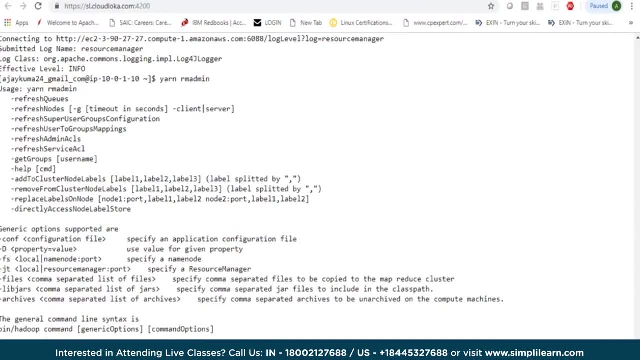 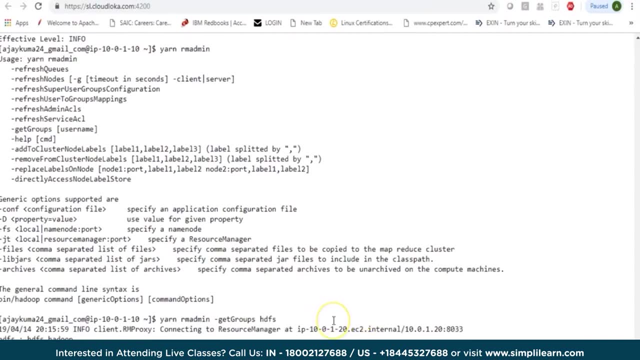 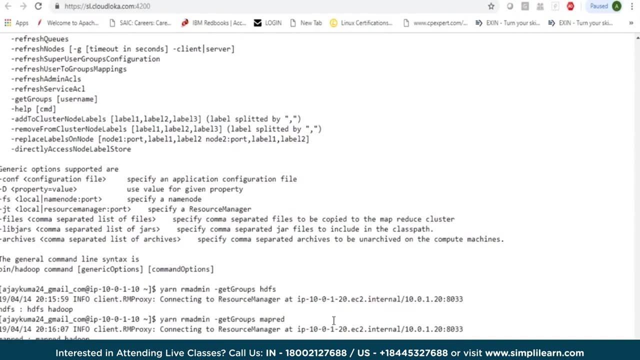 I would want get groups and then I could be searching for, say username HDFS. So that is it. This tells me HDFS belongs to a Hadoop group. Similarly you could search for, say, MapRed, or you could search for yarn. So these are service related users. 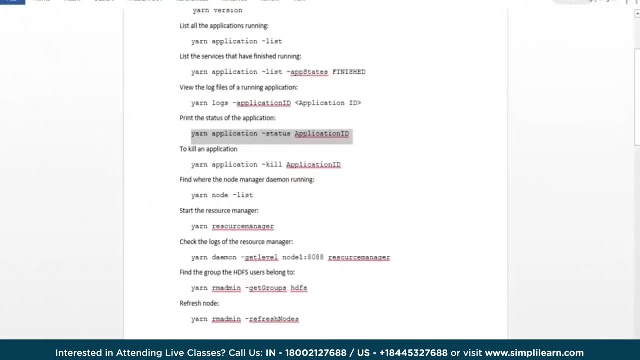 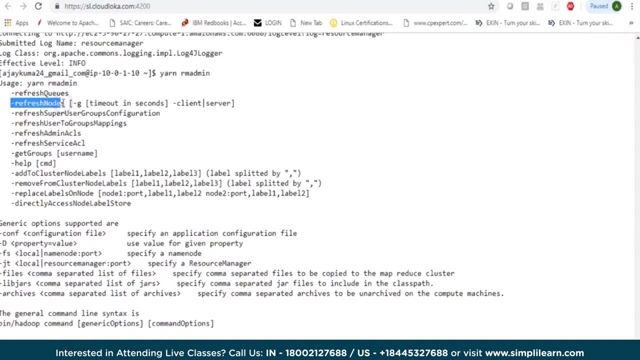 which automatically get created and you can pull out information related to these. You can always do a refresh nodes kind of command, and that is mainly done internally. This can be useful when you are doing commissioning, decommissioning, But then in case of cloud error, 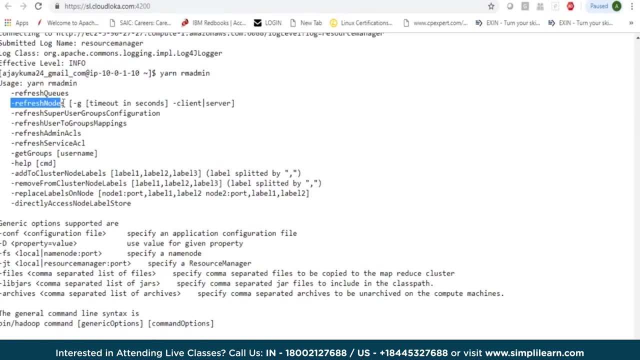 or Hortonworks kind of cluster. you would not be able to manually giving this command, because if you are doing a commissioning decommissioning from an admin console and if you are an administrator, then you could just restart the services which are affected and that will take care of this. 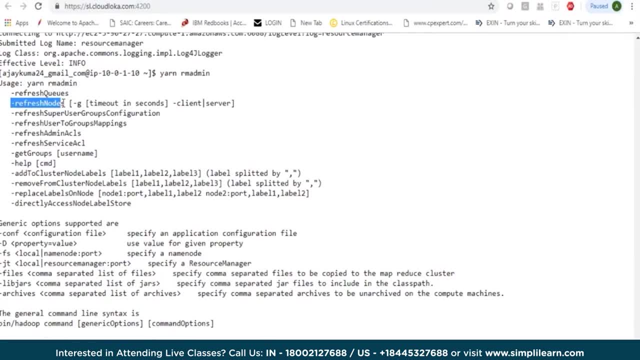 But if you were working in an Apache cluster and if you were doing commissioning decommissioning, then you would be using in two commands: Refresh nodes, and basically that's for refreshing the nodes which should not be used for processing, And similarly you could have a command: 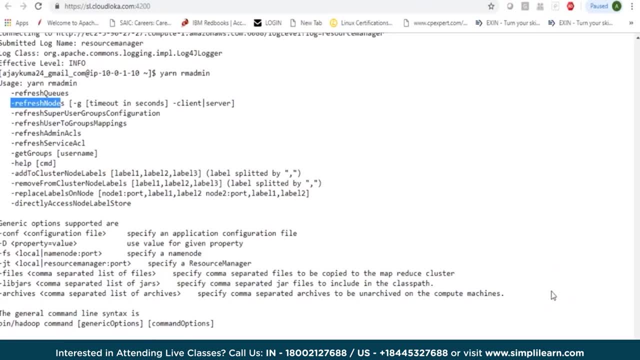 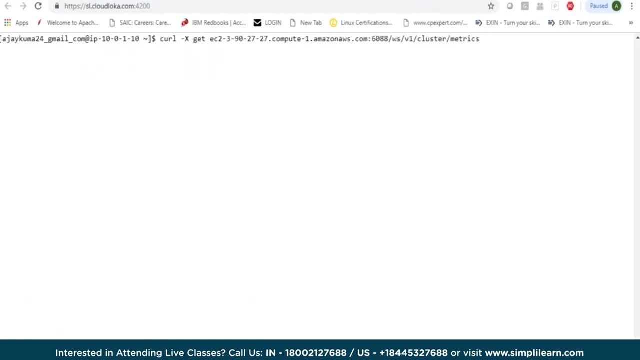 refresh nodes, which comes with SDFS. So these are different options which you can use with your yarn on the command line. You could also be using curl commands to get more information about your clusters by giving curl minus x and then basically pointing out to your resource manager. 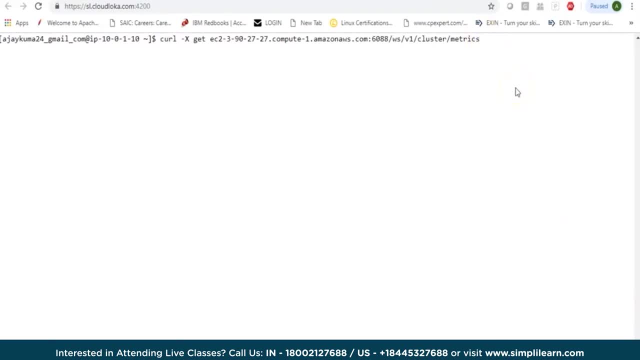 web UI address. Now here I would like to print out the cluster related metrics, and I could just simply do this, which basically gives me a high level information of how many applications were submitted, how many are pending, what is the reserved resources, what is the available amount. 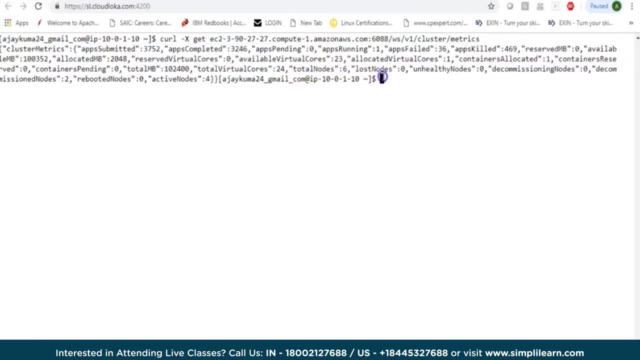 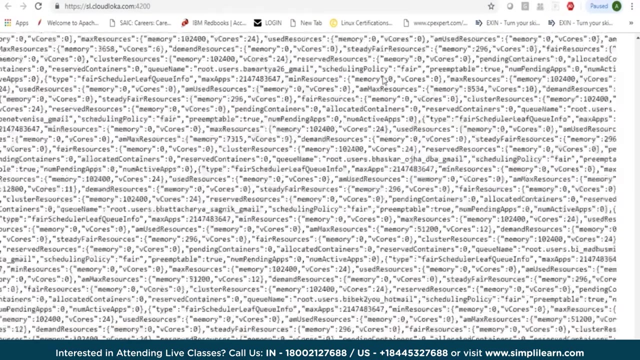 of memory or CPU cores and all the information. Similarly, you can be using the same curl commands to get more information, like scheduler information. So you would just replace the metrics with scheduler and you could get the information of the different queues. Now that's a huge list. 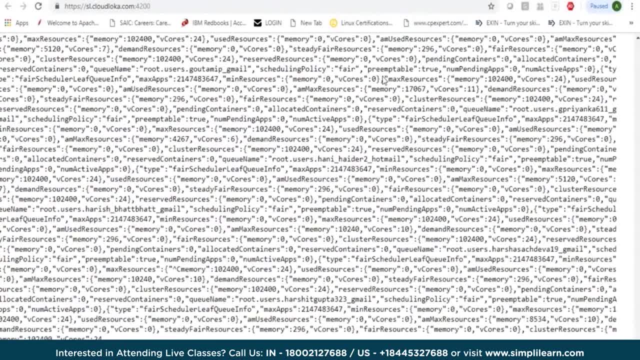 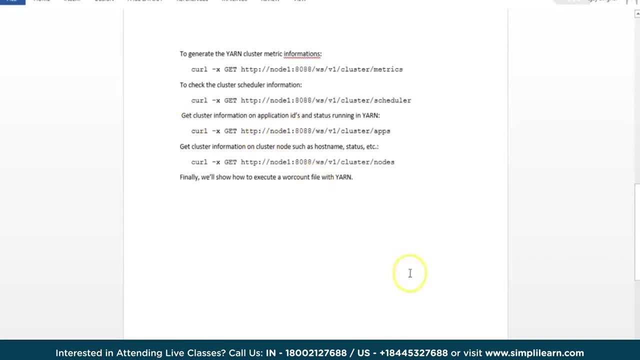 We can cancel this and that would give me a list of all the queues which are allocated and what are the resources allocated for each queue. You could also get cluster information and application IDs and status running of applications running in yarn. So you would have to replace. 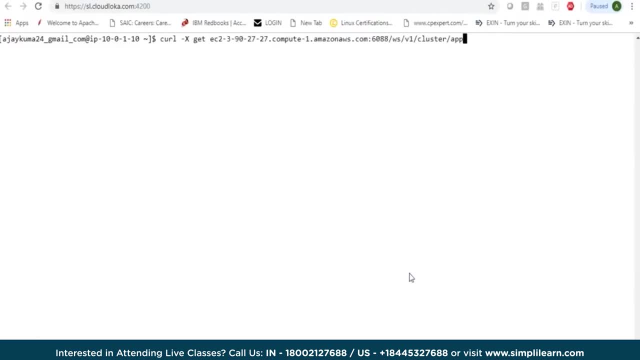 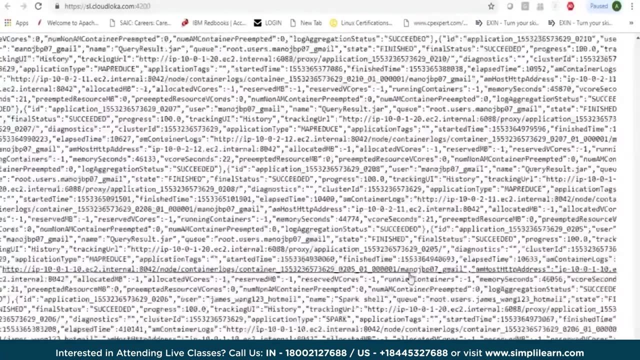 the last bit of it and you would say I would want to look at the applications and that gives me a huge list of applications. Then you can do a grip and you can be filtering out specific queries and specific application related information. Similarly, you can be looking: 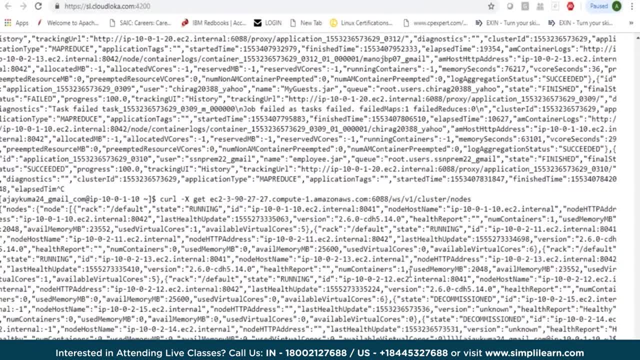 at the nodes So you can always be looking at node specific information which gives you how many nodes you have. But this could be mainly used when you have an application which wants to, or a web application which wants to use a curl command and would want to get information. 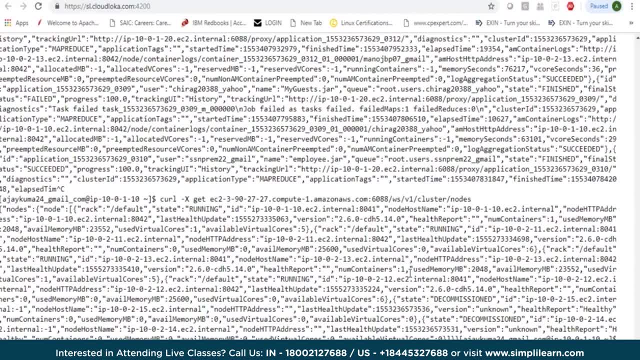 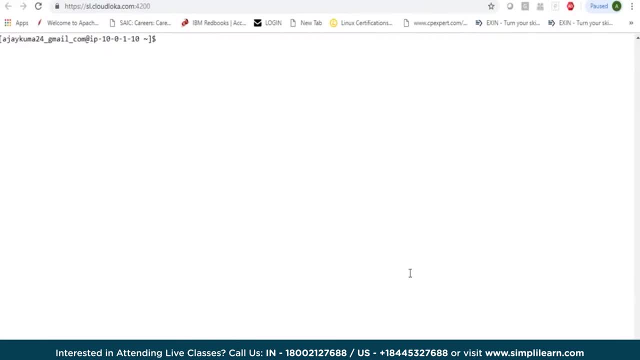 about your cluster from an HTTP interface. Now, when it comes to application, we can basically try running a simple or a sample map reduced job, which could then be triggered on yarn and it would use the resources. Now I can look at my application here and I can be looking into 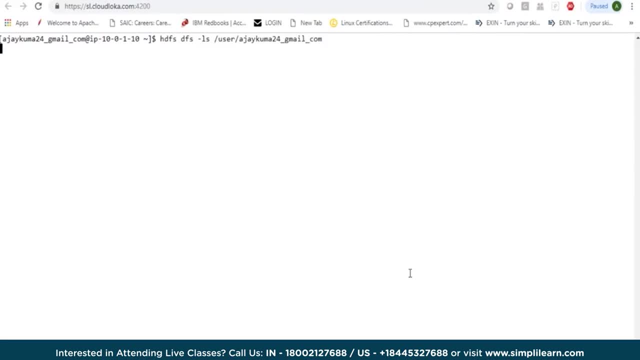 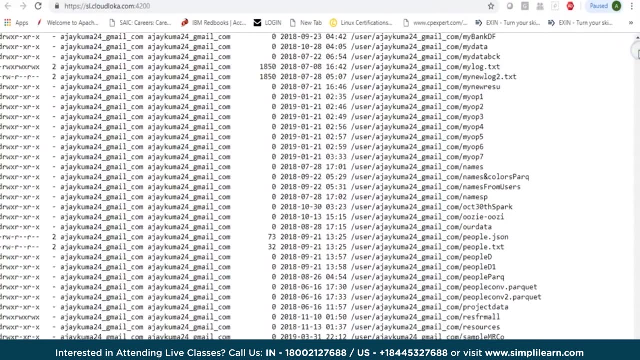 my specific directory, which is this one which should have a lot of files and directories which we have here. Now I could pick up one of these and I could be using a simple example to do some processing. Let's take up this file. So there is a file. 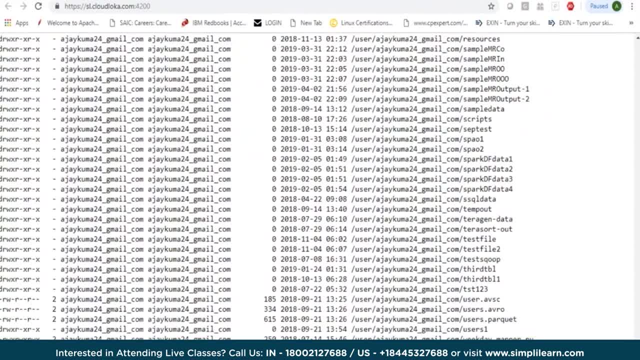 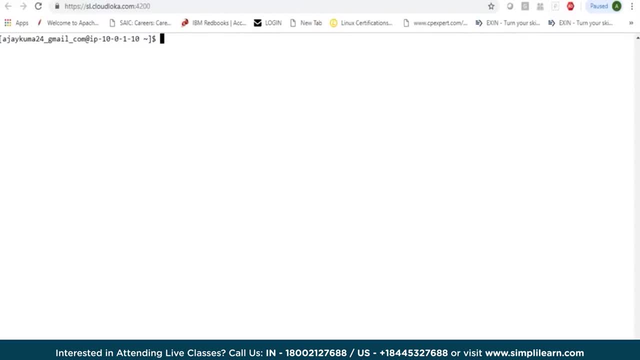 and I could run a simple word count. or I could be running a hive query which triggers a map reduced job. I could even run a spark application which would then show that the application is running on the cluster. So, for example, if I would say spark to shell, 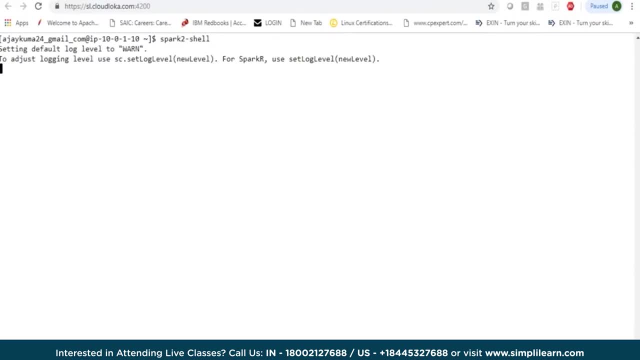 now, I know that this is an interactive way of working with spark, but this internally triggers a spark submit and this runs an application. So here, when you do a spark to shell, by default it will contact yarn, so it gets an application ID. It is running on yarn. 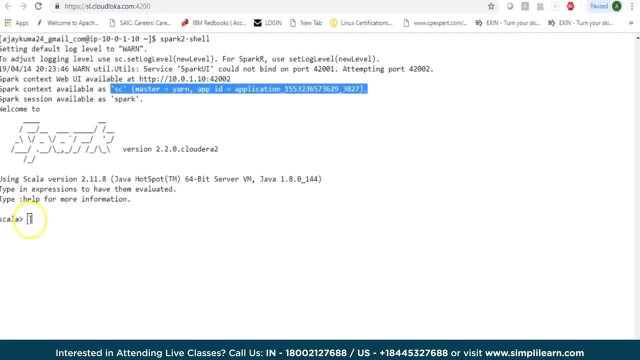 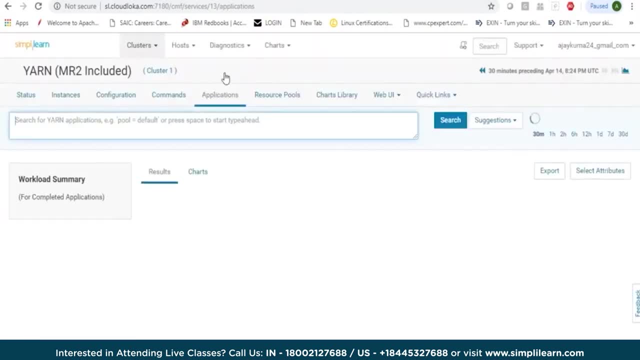 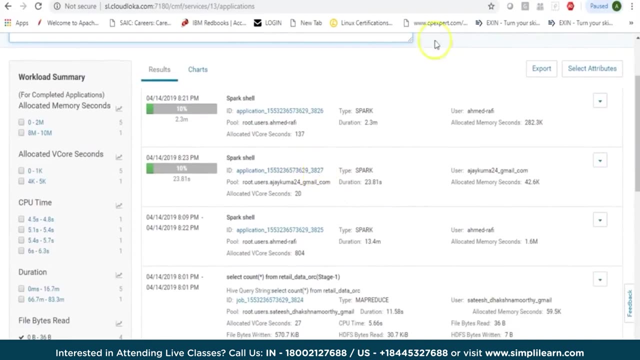 with the master being yarn, and now I have access to the interactive way of working with spark. Now, if I go and look into applications, I should be able to see my application, which has been started here, and it shows up here. So this is my application. 3827. 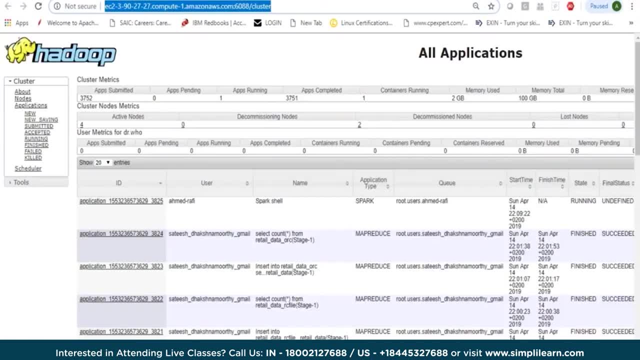 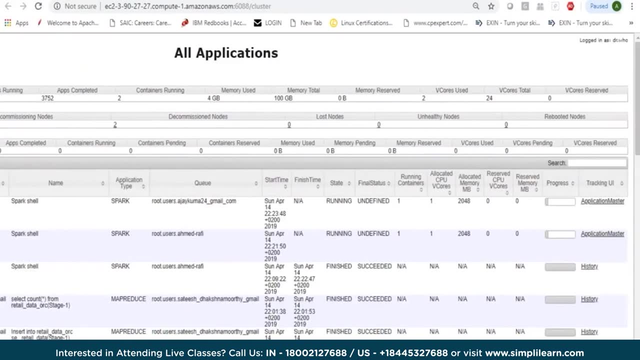 which has been started on yarn and as of now we can also look into the yarn UI. and that shows me the application which has been started, which basically has one running container which has one CPU core allocated 2GB RAM, and it's in progress. 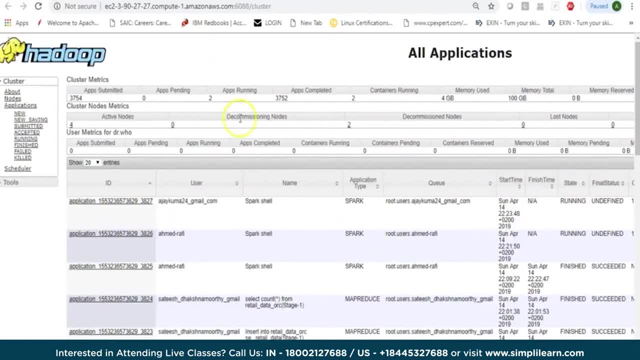 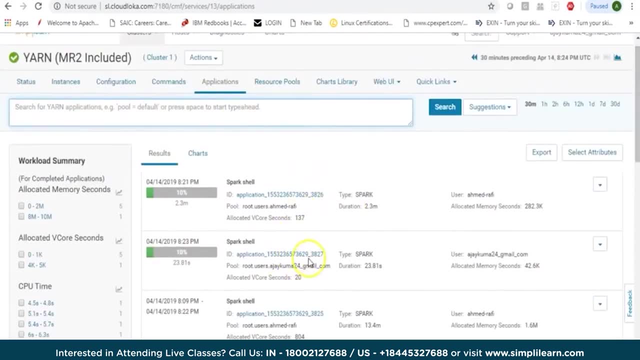 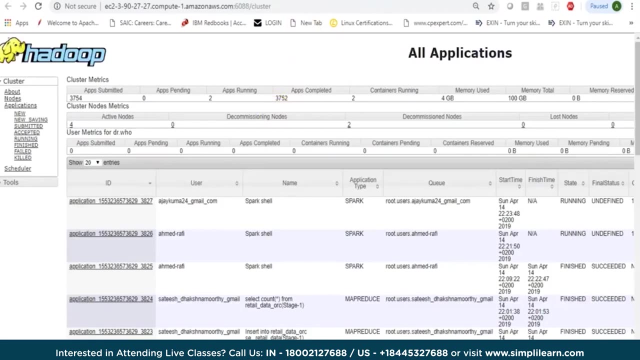 although we are not doing anything there. So we can always look at our application from the yarn UI or, as I mentioned, from your applications tab within yarn services, which gives us the information, and you can even click on this application to follow and see more information. but you should be given access to that. 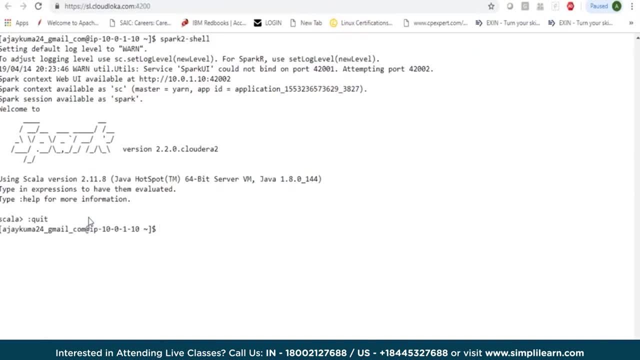 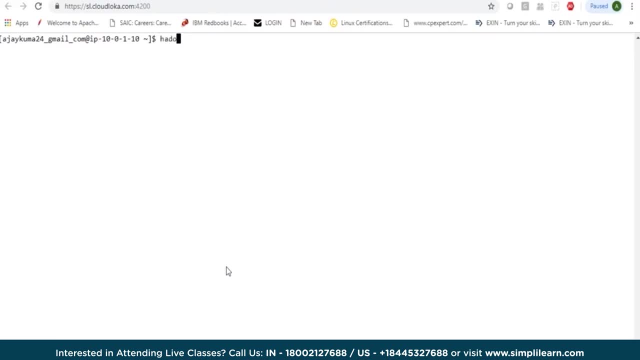 Now, this is just a simple application which I triggered using spark shell. Similarly, I can basically be running a MapReduce. Now, to run a MapReduce, I can say hadoop jar, and that basically needs a class. so we can look for the default path. 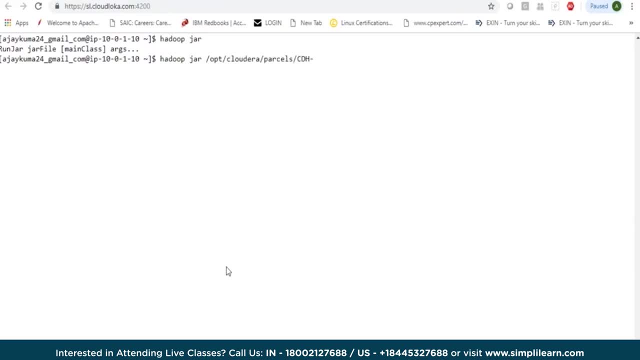 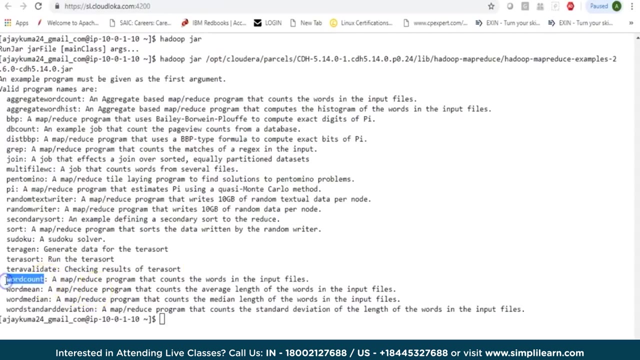 which is opt, cloudera parcels, cdh, lib, hadoop, MapReduce- hadoop MapReduce examples. and then we can look at this particular jar file and if I hit on enter, it shows me the different classes which are part of this jar. and here I would like to use word count. 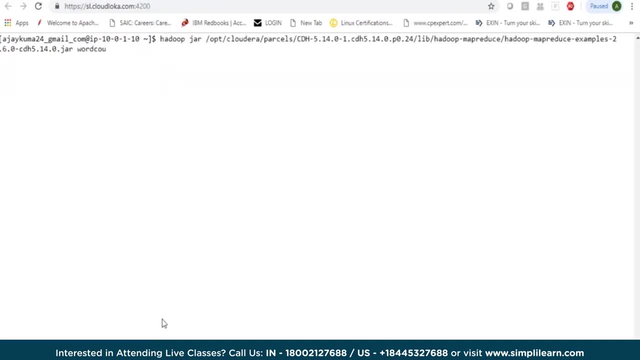 so I could just give this. I could say: word count now, remember, I could run the job in a particular queue by giving in an argument here. so I could say "-d MapRedjobqueuename, and then I can point my job to a particular queue. I can even give different arguments. 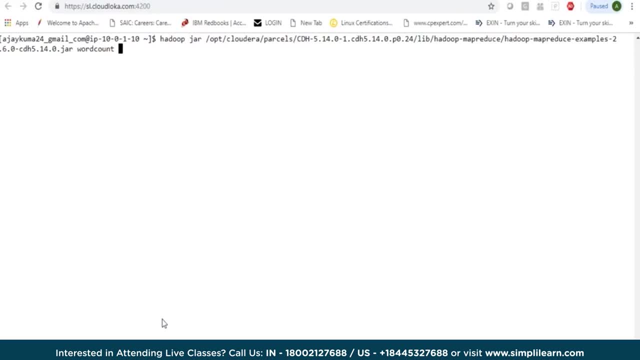 in saying I would want my MapReduce output to be compressed, or I want it to be stored in a particular directory, and so on. so here I have the word count and then basically what I can be doing is I can be pointing it to a particular input path. 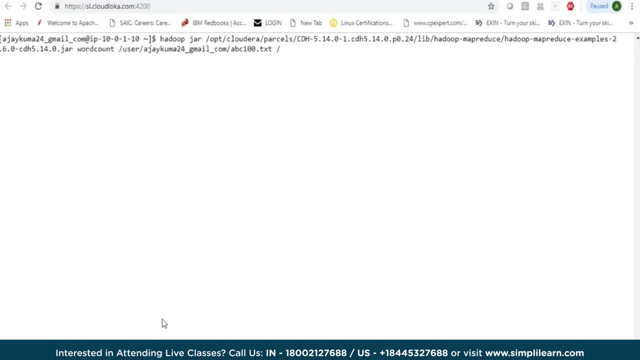 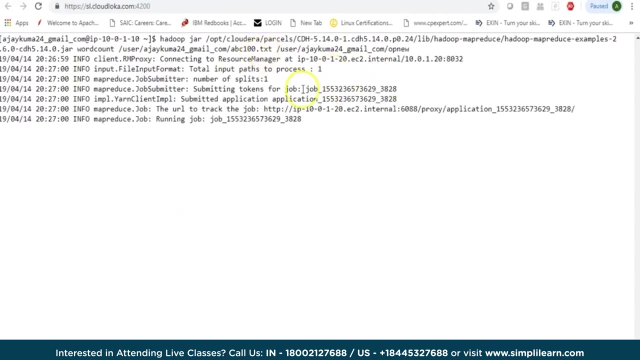 and then I can have my output which can be getting stored here again a directory which we need to choose, and I will say output new and I can submit my job. now, once I have submitted my job, it connects to resource manager. it basically gets a job ID. 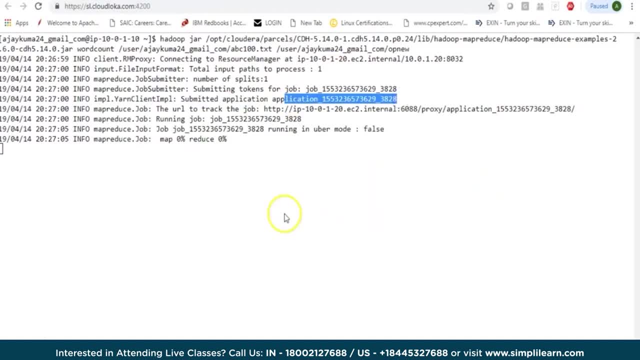 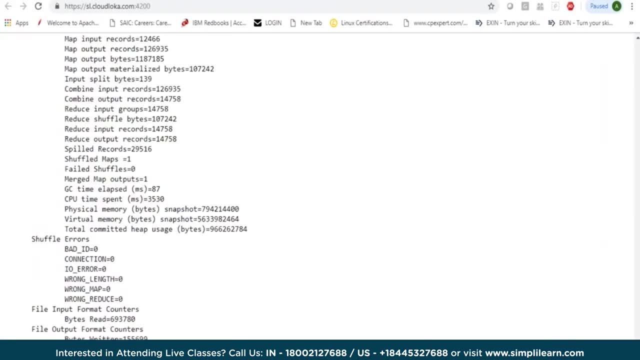 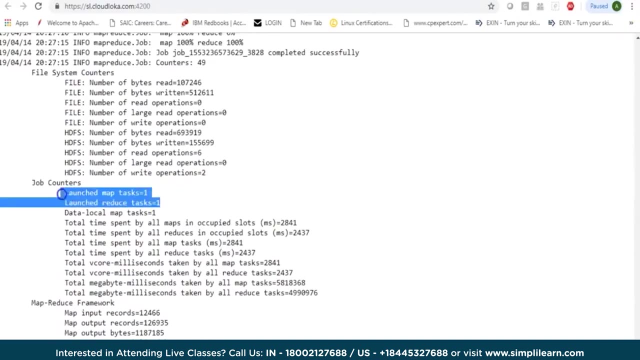 it gets an application ID. it shows you from where you can track your application. you can always go to the yarn UI and you can be looking at your application and the resources it is using. so my application was not a big one and it has already completed. it triggered one map task. 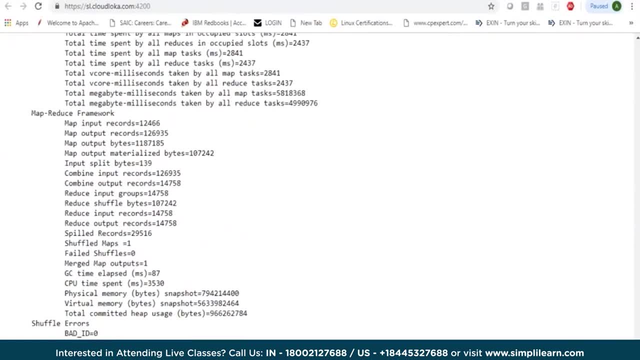 it launched one reduce task- it was working on around 12,466 records- where you have then the output of map, which is these many number of output records, which was then taken by a combiner and finally by a reducer, which basically gives you the output. so this is my yarn application, which has completed. 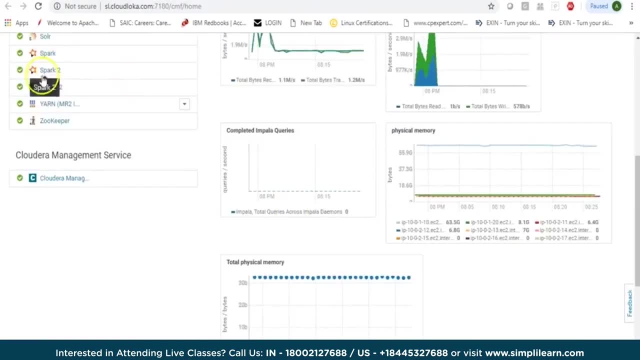 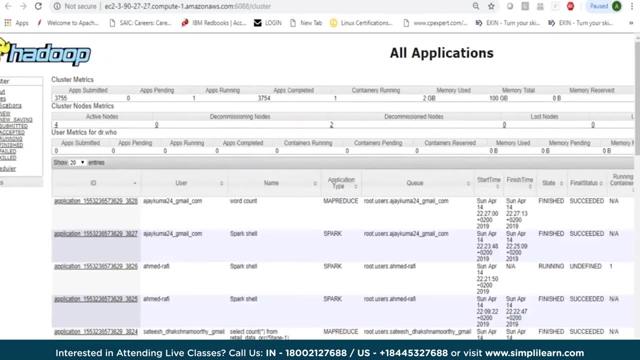 now I could be looking into the yarn UI and if my job has completed, you might not see your application here. so as of now it shows up here the word count which I ran. it also shows me my previous park shell job. it shows me my application is completed. 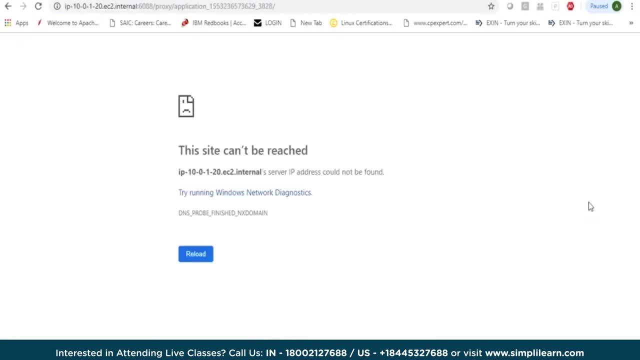 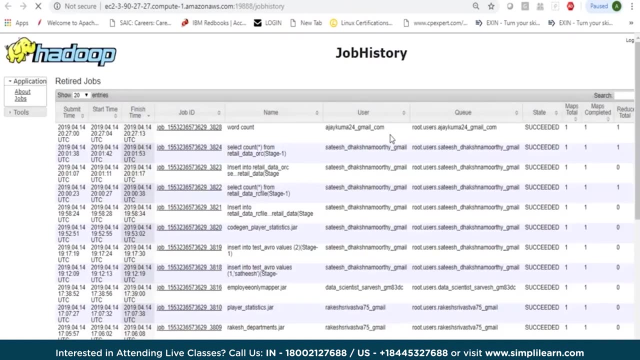 and if you would want further information on this, you can click and go to the history server if you have been given access to it, or directly go to the history server web UI where your application shows up. it shows how many map and reduce tasks it was running. 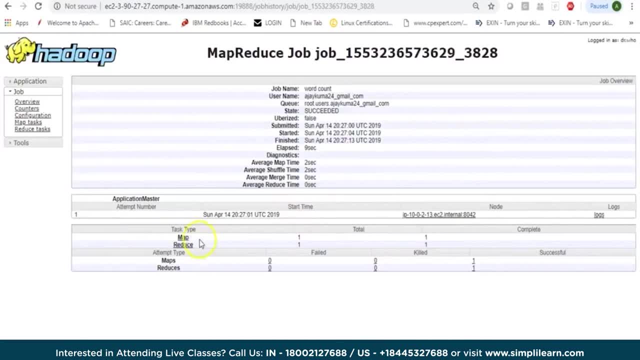 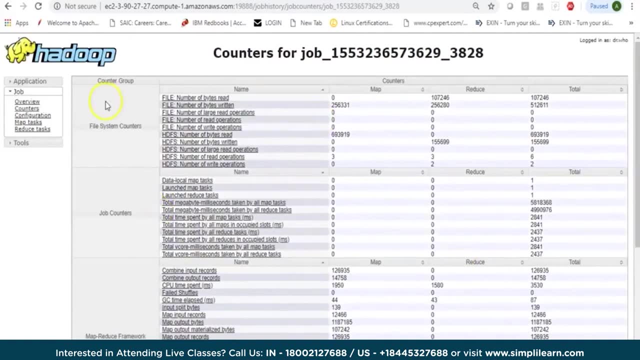 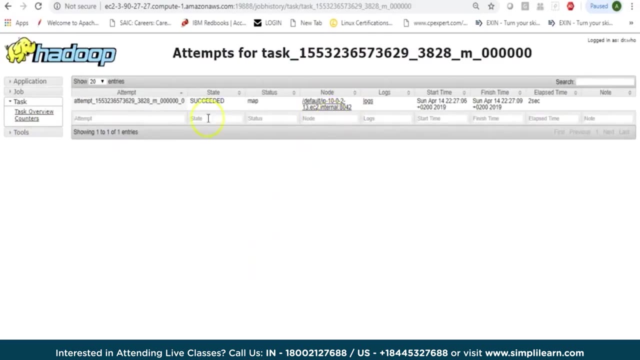 you can click on this particular application which basically gives you information of your map and reduce tasks. you can look at different counters for your application. you can always look at map specific tasks. you can always look into one particular task, what it did, on which node it was running. 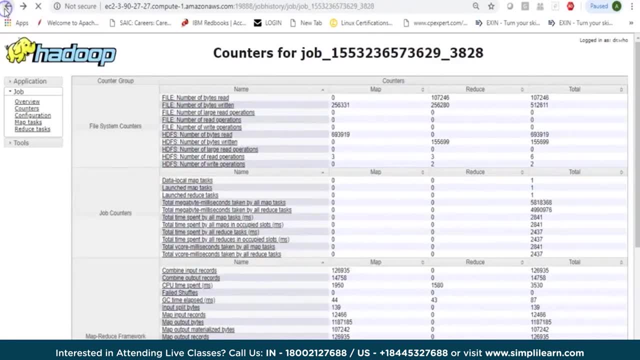 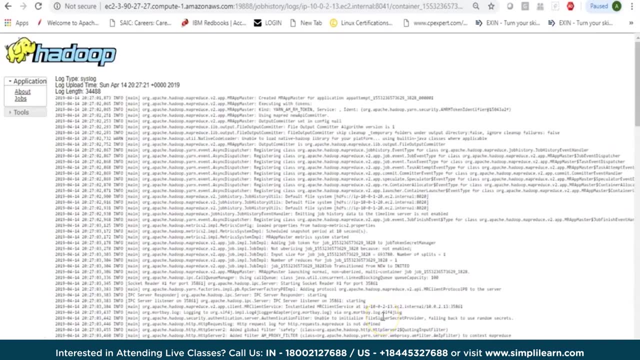 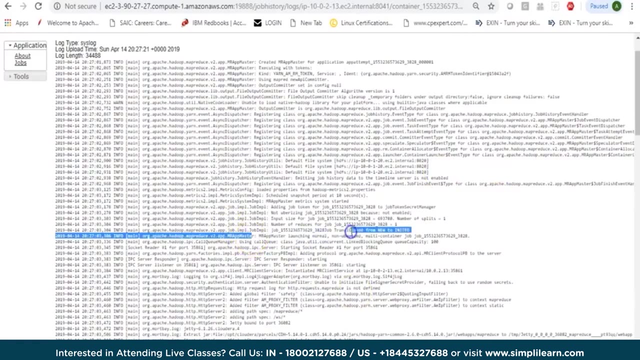 or you can be looking at the complete application log. so you can always click on the logs and here you have. click here for full log, which gives you the information, and you can always look for your application, which can give you information of app master being launched. or you could have search for the word container. 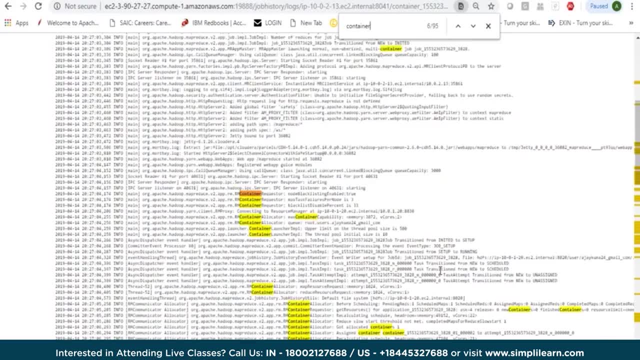 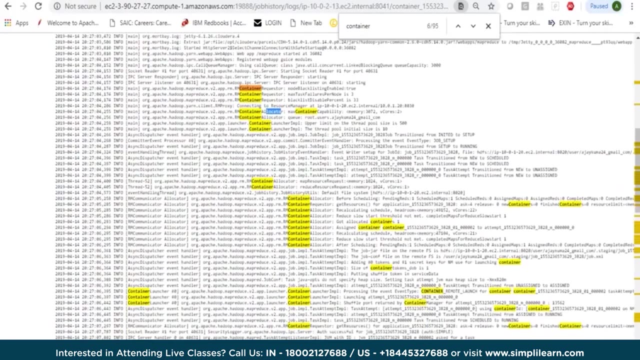 so you could see a job which needs one or multiple containers and then you could say container is being requested, then you could see container is being allocated, then you can see what is the container size and then basically your task moves from initializing to running in the container. 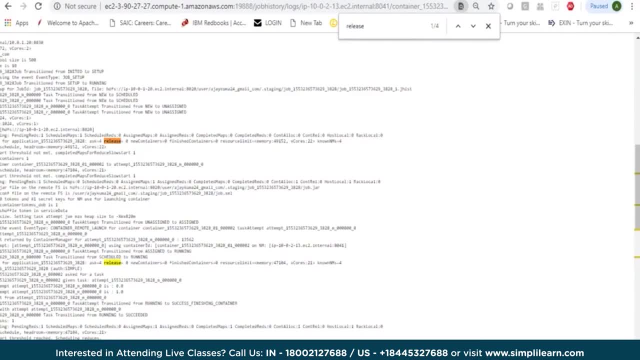 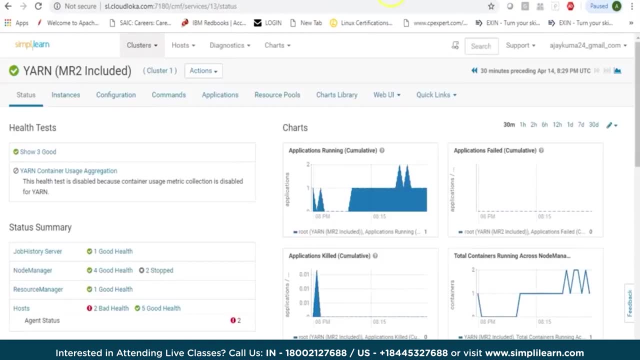 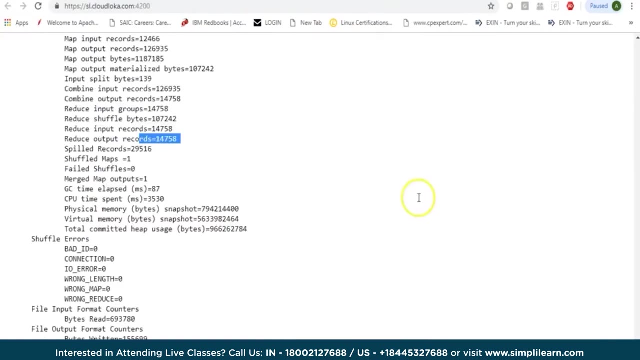 and finally, you can even search for release, which will tell you that the container was released. so you can always look into the log for more information. so this is how you can interact with yarn. this is how you can interact with your command line to look for more information. 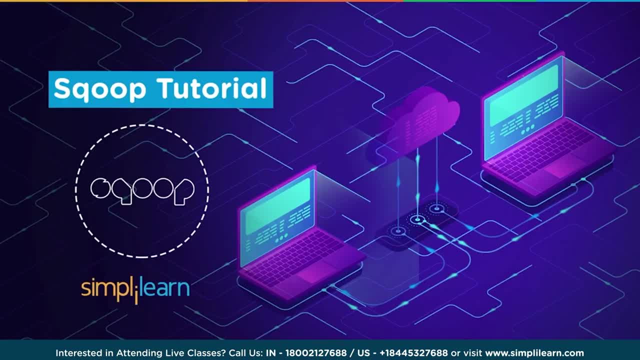 or using your yarn web UI. My name is Richard Kirschner and I'm with the Simply Learn team. that's wwwsimplylearncom. Get Certified, Get Ahead. Today we're going to dive in on Scoop, one of the many features of the Hadoop ecosystem. 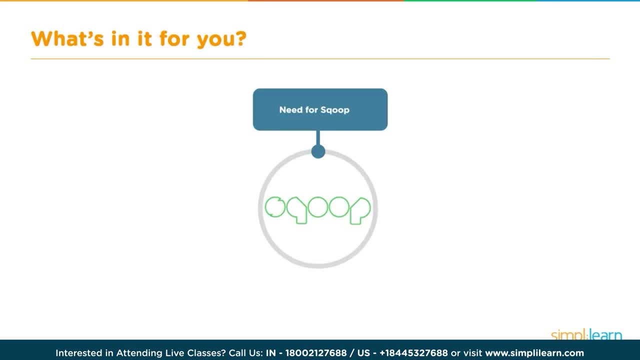 for the Hadoop file system. What's in it for you? Today, we're going to cover the need for Scoop. What is Scoop? Scoop features, Scoop architecture, Scoop interface, Scoop import, Scoop export, Scoop processing, and then, finally, we'll have a little hands-on demo on Scoop. 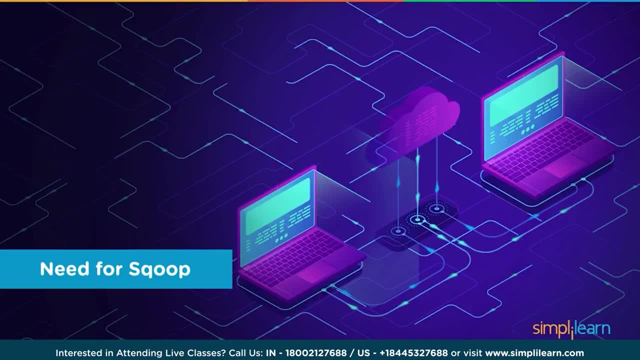 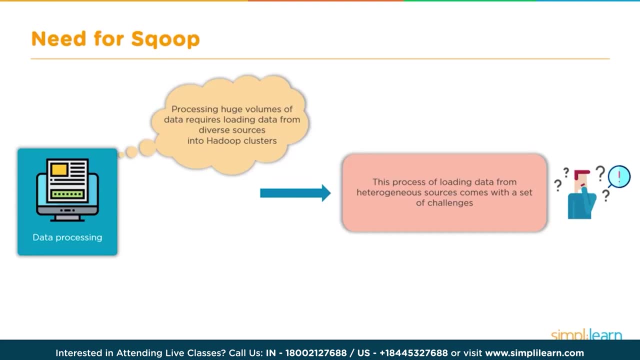 so you can see what it looks like. So where does the need for Scoop come in in our big data Hadoop file system? Processing huge volumes of data requires loading data from diverse sources into Hadoop cluster. You can see, here we have our data processing. 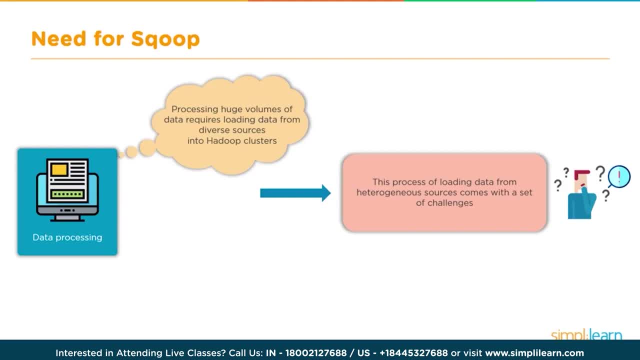 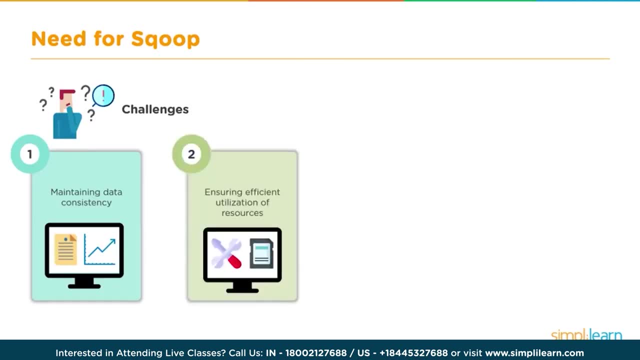 and this process of loading data from the heterogeneous sources comes with a set of challenges. So what are the challenges? Maintaining data consistency. Ensuring efficient utilization of resources, Especially when you're talking about big data. We can certainly use up the resources when importing terabytes and petabytes of data. 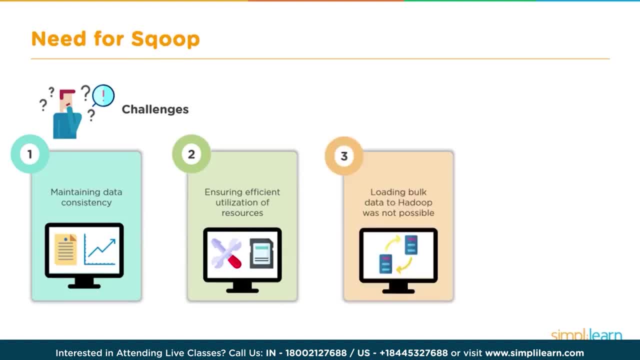 over the course of time, Loading bulk data to Hadoop was not possible. It was one of the big challenges that came up when they first had the Hadoop file system going, And loading data using script was very slow. In other words, you'd write a script. 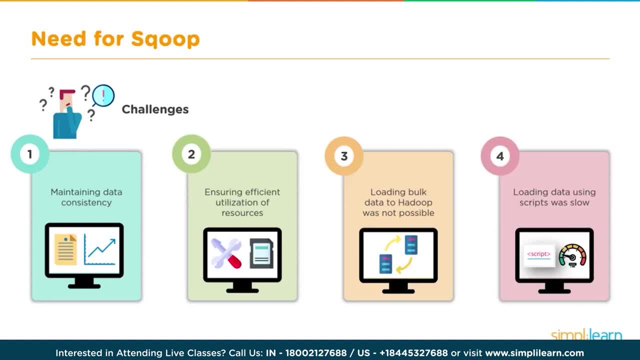 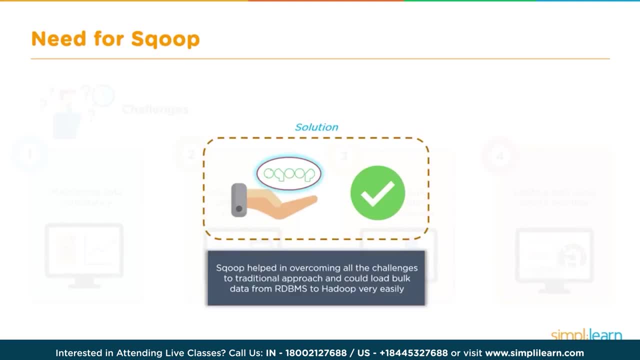 in whatever language you were in, and then it would very slowly load each piece and parse it in. So the solution Scoop Scoop helped in overcoming all the challenges to traditional approach and could lead bulk data from RDBMS to Hadoop very easily. So think your enterprise server. 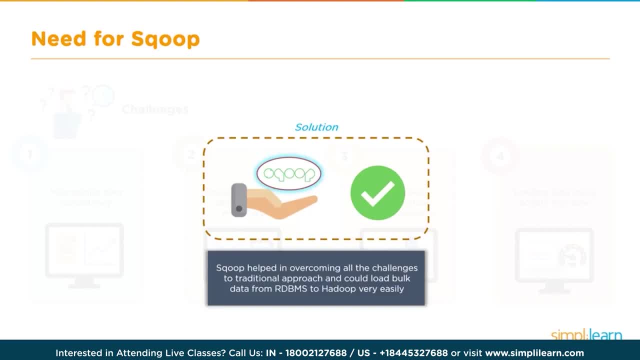 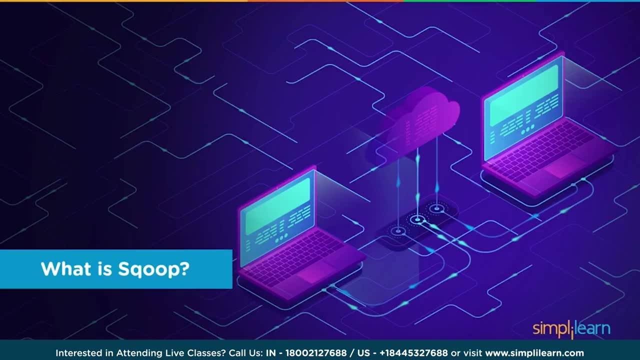 you want to take the from MySQL or your SQL and you want to bring that data into your Hadoop warehouse, your data filing system, and that's where Scoop comes in. So what exactly is Scoop? Scoop is a tool used to transfer bulk of data. 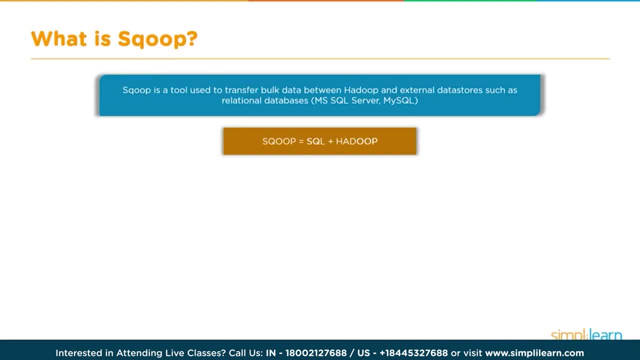 between Hadoop and external data stores such as relational databases and MySQL Server or the Microsoft SQL Server or MySQL Server or SQL Plus Hadoop. and you can see, here we have our RDBMS, all the data we have stored on there, and then your Scoop is the middle ground. 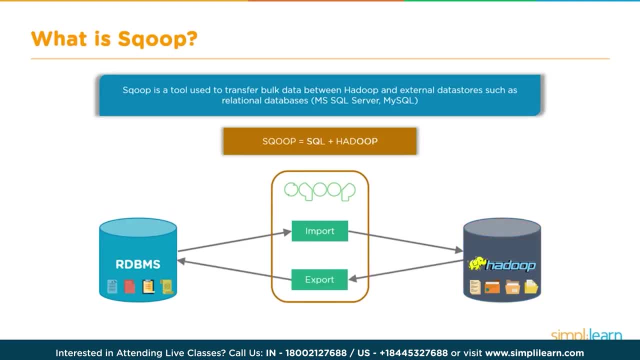 and brings the import into the Hadoop file system. It also is one of the features that goes out and grabs the data from Hadoop and exports it back out into an RDBMS. Let's take a look at Scoop Features. Scoop features has parallel import and export. 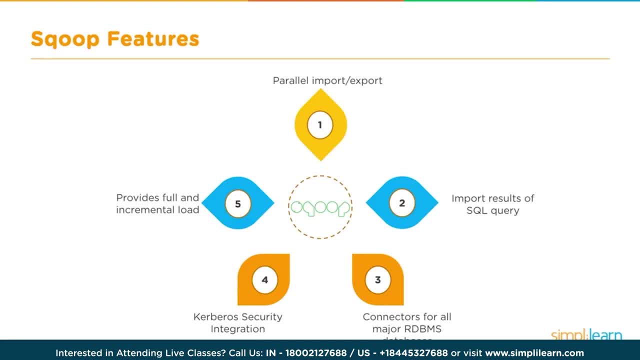 It has import results of SQL query connectors for all major RDBMS databases. Kerberos security integration provides full and incremental load. so we look at parallel import and export. scoop uses yarn- yet another resource negotiator framework, to import and export data. this provides fault tolerance on a top of 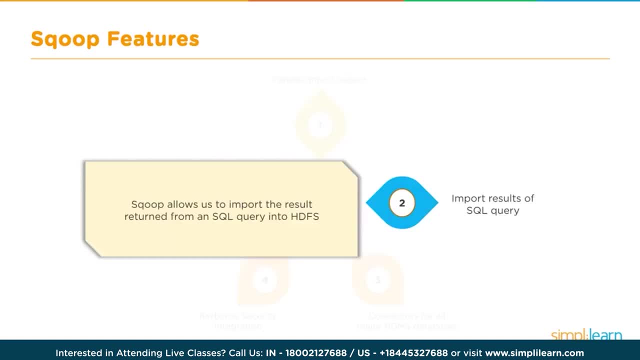 parallelism. scoop allows us to import the result return from an SQL carry into the Hadoop file system or the HDFS and you can see here where the import results of SQL query come in. scoop provides connectors for multiple relational database management system. our DBMS is databases such as mysql and. 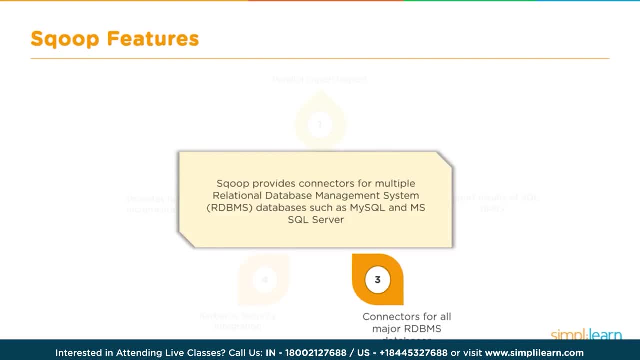 Microsoft SQL Server and has connectors for all major our DBMS databases. scoop supports Kerberos computer network authentication protocol that allows nodes communicating over a non secure network to prove their identity to one another in a secure manner. scoop can load the whole table or parts of the 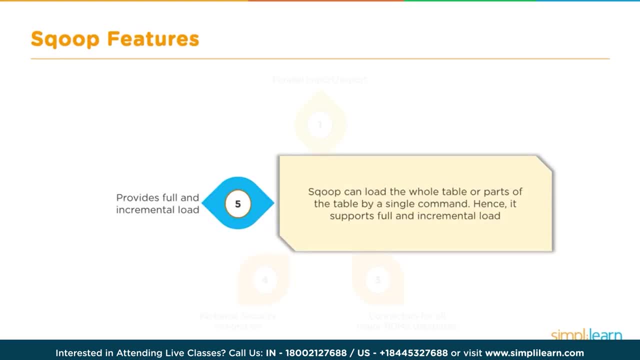 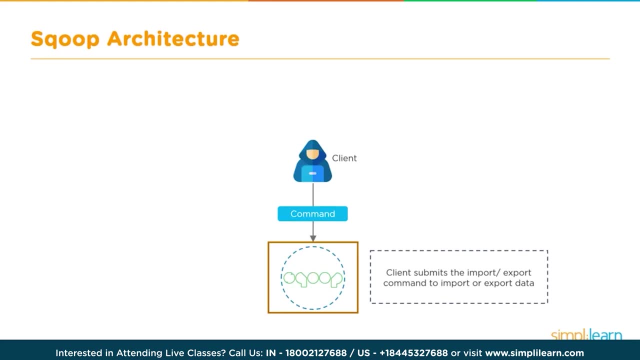 table by a single command. hence it supports full and incremental load. let's dig a little deeper into the scoop. architecture: we have our client, in this case a hooded wizard, behind his laptop. you never know who's going to be accessing the Hadoop cluster and the 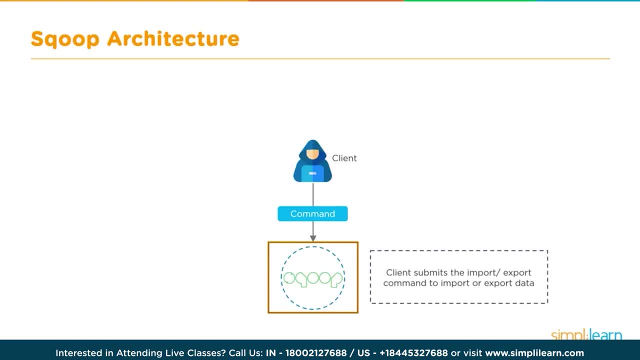 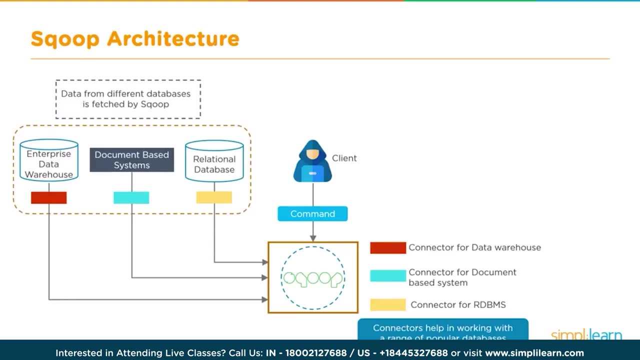 client comes in and sends their command, which goes into scoop. the client submits the import- export command to import or export data. data from different databases is fetched by scoop and so we have enter enterprise data warehouse document based systems. you have connect connector for your data warehouse a. 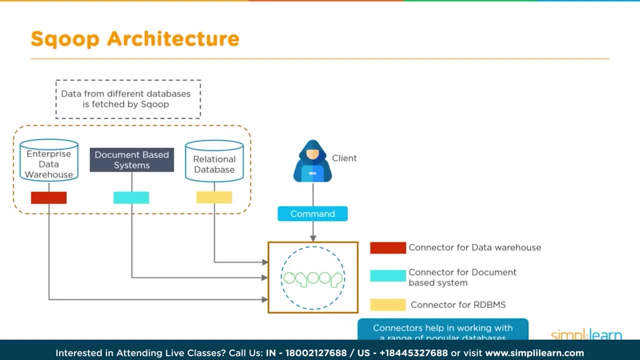 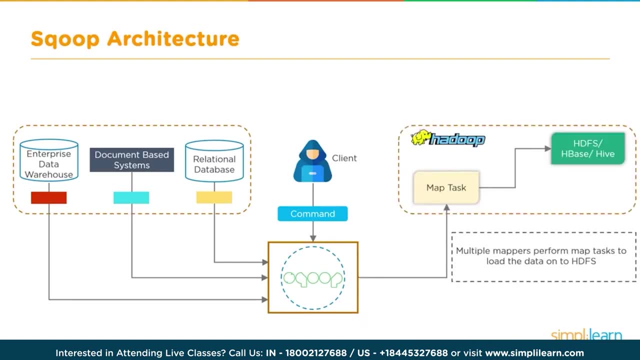 connector for document based systems which reaches out to the Hadoop cluster and you can access the Hadoop cluster, those two entities and we have our connector for the rdbms. so connectors help in working with a range of popular databases. multiple mappers perform map tasks to load the data onto hdfs. 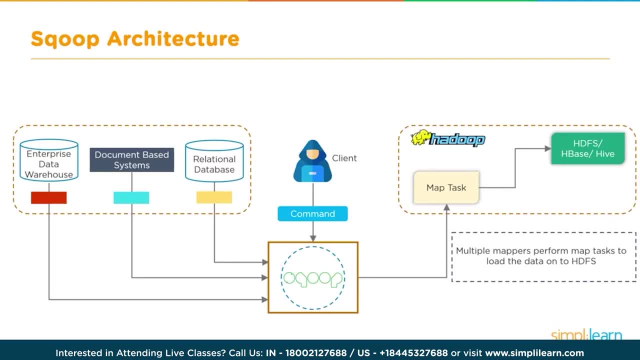 the hadoop file system and you can see here we have the map task. if you remember from hadoop, hadoop is based on map reduce, because we're not reducing the data, we're just mapping it over. it only accesses the mappers and it opens up multiple mappers to do parallel processing. and you can see. 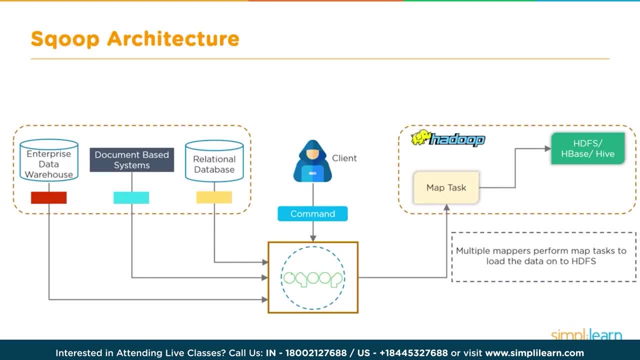 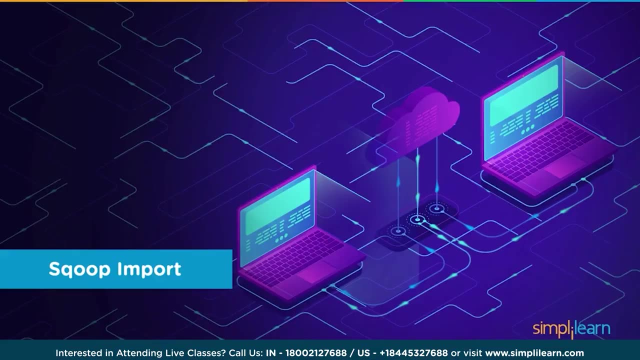 here. the hdfs hbase hive is where the target is for this particular one. similarly, multiple map tests will export the data from hdfs onto rdbms using scoop export command. so just like you can import it, you can now export it using the multiple map routines, scoop import. so here we have. 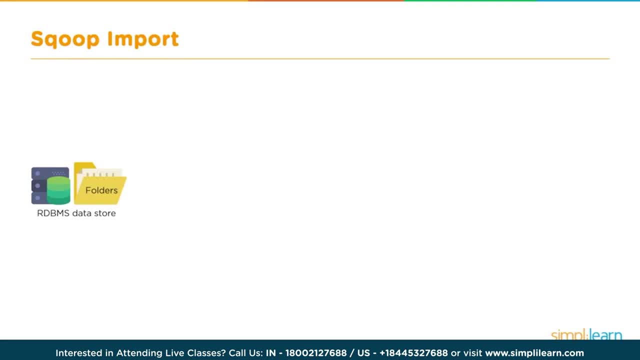 our rdbms data store and we have the folders on there. so maybe it's your company's database, maybe it's an archive at google with all the searches going on, whatever it is. usually you think with scoop, you think it's going to be an archive or something like that, and then you can import it. 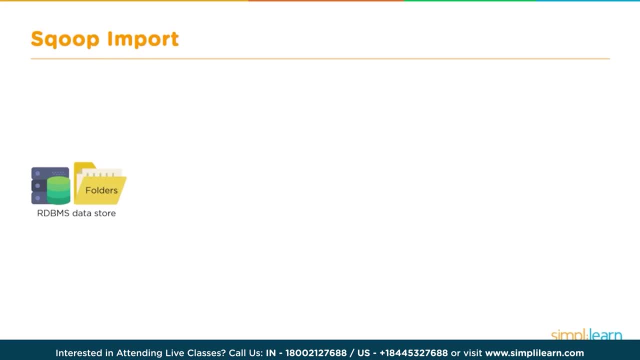 in any type of way. you just import it in any type of way. you think sql, you think my sql server or microsoft sql server, that kind of setup. so it gathers the metadata and you see the scoop. import so introspect database to gather metadata, primary key information, and then it submits. so you can. 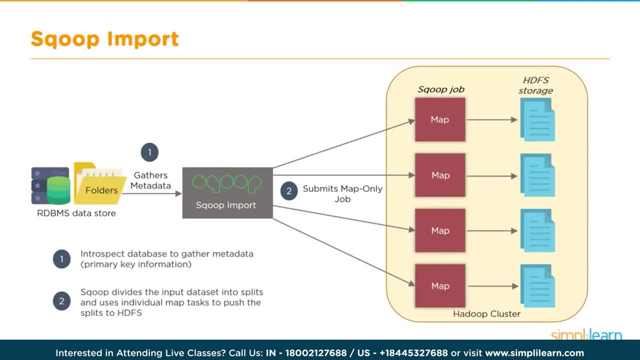 see submits map only job. remember we talked about map reduce. it only needs the map side of it, because we're not reducing the data, we're just mapping it over. scoop divides the input data set into splits and uses individual map tests to push the splits into hdfs. 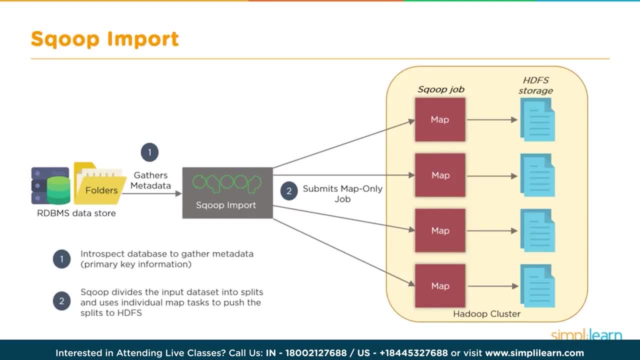 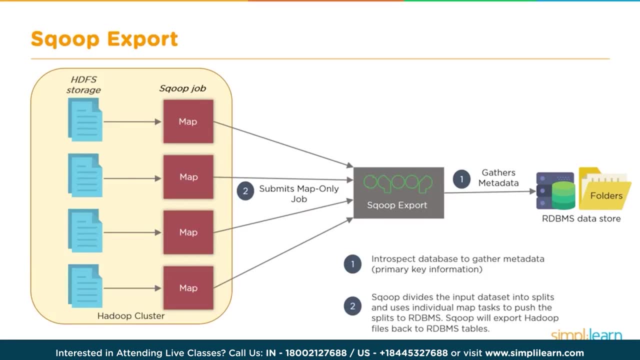 So right into the Hadoop file system And you can see down on the right is kind of a small depiction of a Hadoop cluster And then you have scoop export. So we're gonna go the other direction And with the other direction 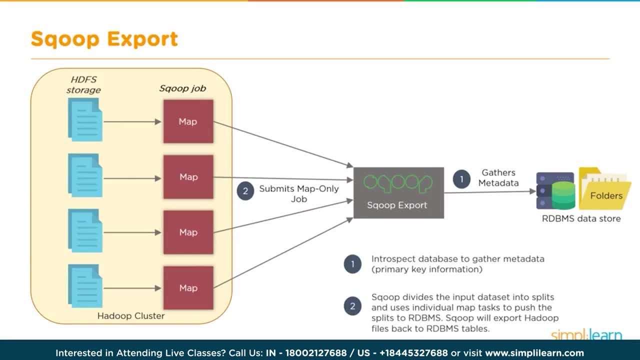 you have your Hadoop file system storage, which is your Hadoop cluster. You have your scoop job and each one of those clusters then gets a map Mapper comes out to each one of the computers that has data on it. So the first step is you've gotta gather the metadata. 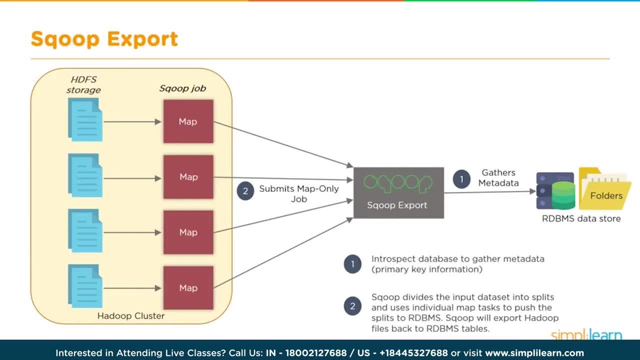 So step one: you gather the metadata. Step two: submits map only job Introspect database to gather metadata, primary key information. Scoop divides the input data set into splits and uses individual map tests to push the splits to RDBMS. 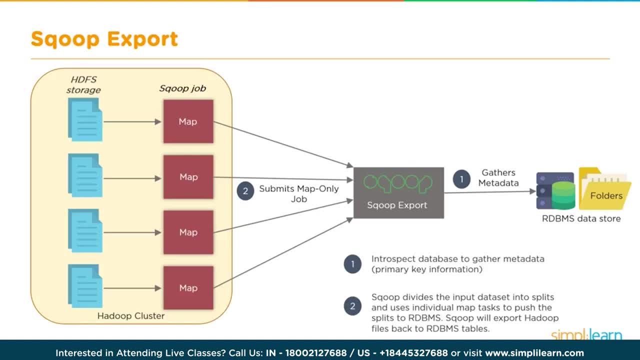 Scoop will export Hadoop files back to RDBMS tables, And you can think of this in a number of different manners. One of them would be if you're restoring a backup from the Hadoop file system into your enterprise machines. There's certainly many others. 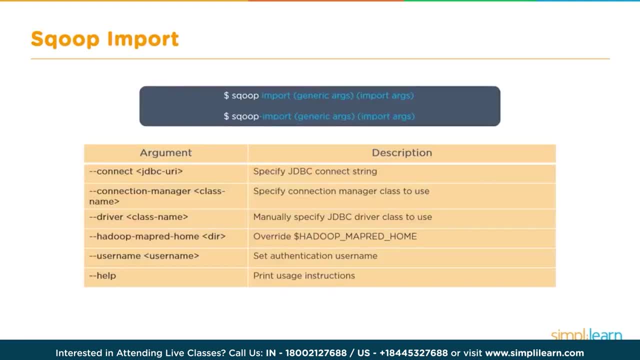 as far as exploring data and data science. So as we dig a little deeper into the scope input, we have our connect, our JDBC and our URL, So specify the JDBC connect string Connecting manager. we specify the connection manager class to use. 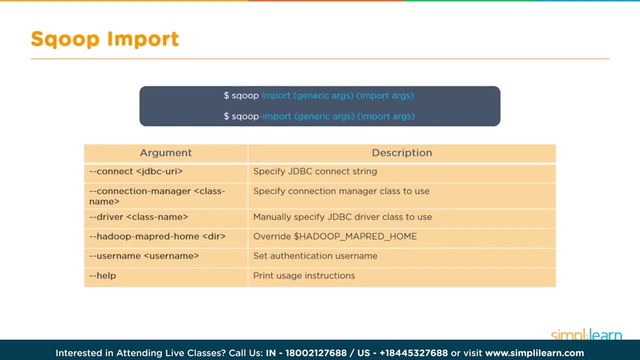 You can see here driver with the class name. manually specify the JDBC driver class to use Hadoop map. reduce home directory. Override Hadoop mapped home User name, set authentication user name and, of course, help print uses instructions And with the export. 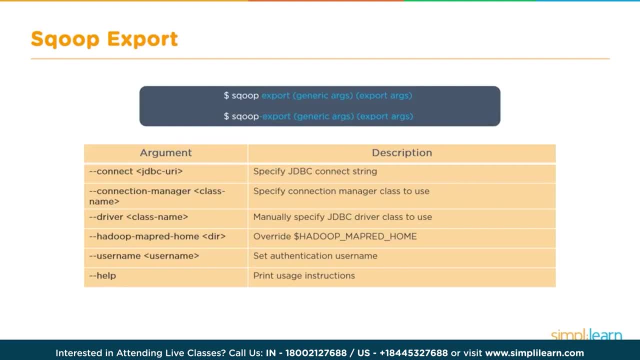 you'll see that we can specify the JDBC connect string, specify the connection manager class to use manually. specify JDBC driver class to use. We do have to let it know. to override the Hadoop map, reduce home, And that's true on both of these. 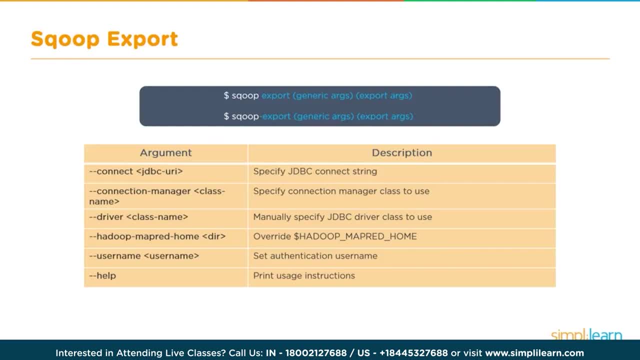 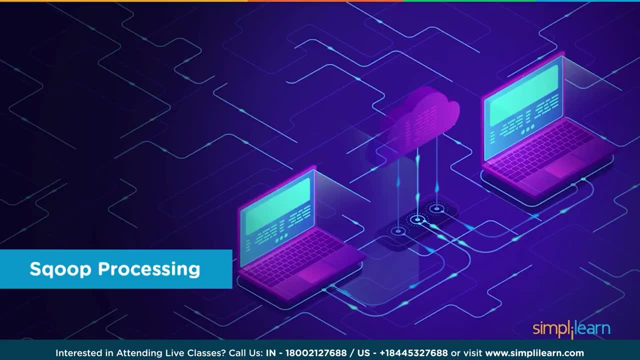 And set authentication user name And finally you can print out all your help setup So you can see the format for Scoop is pretty straightforward, both import and export. So let's continue on our path and look at Scoop processing and what the computer goes through for that. 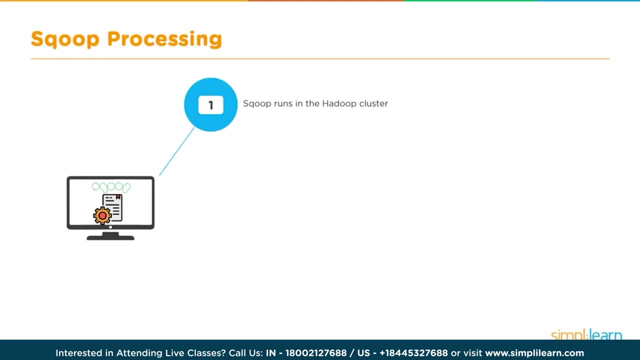 And we talk about Scoop processing. First Scoop runs in the Hadoop cluster. It imports data from the RDBMS, the NoSQL database, to the Hadoop file system. So remember, it might not be importing the data from a RDBMS, it might actually be coming from a NoSQL. 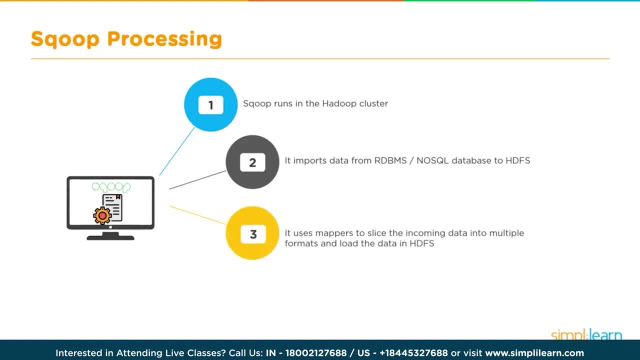 and there's many out there. It uses mappers to slice the incoming data into multiple formats and load the data into HDFS. It exports data back into an RDBMS, while making sure that the schema of the data in the database is maintained. 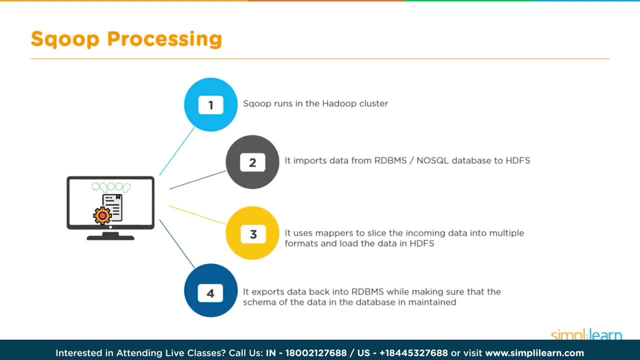 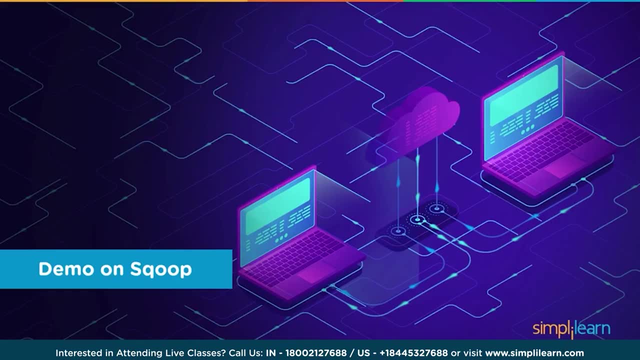 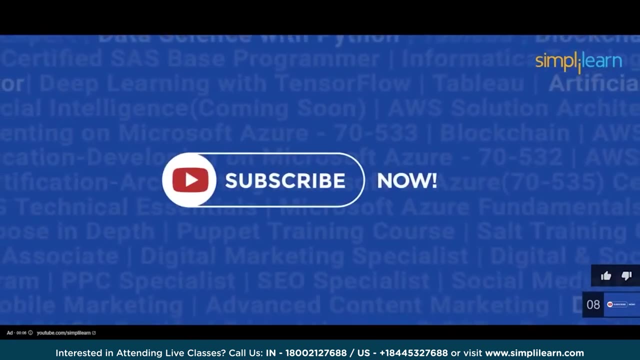 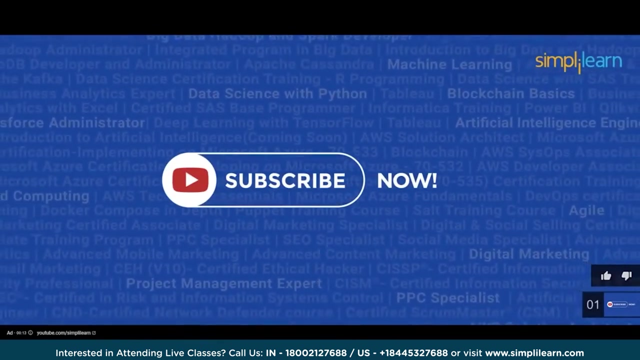 So now that we've looked at the basic commands in our Scoop and the Scoop processing- or at least the basics as far as theory is concerned- let's just jump in and take a look at a demo on Scoop. For this demo, I'm going to use our Cloudera Quick. 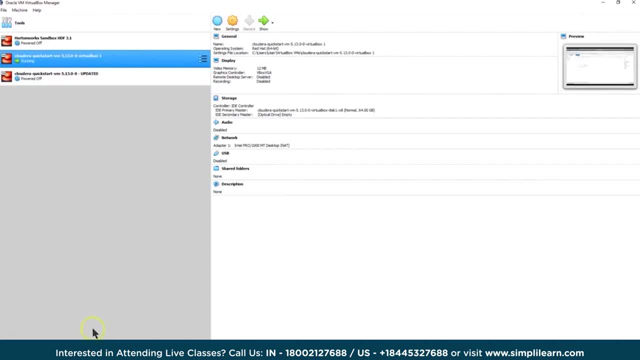 Start. If you've been watching our other demos we've done, you'll see that we've been using that pretty consistently. Certainly this will work in any of your Horton Sandbox, which is also a single node testing machine. Cloudera is one of them. 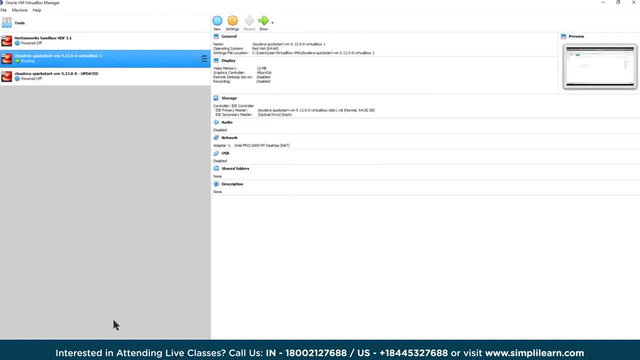 There's a Docker version instead of VirtualBox, And you can also set up your own Hadoop cluster Plan a little extra time. If you're not an admin, it's actually a pretty significant endeavor For an admin if you've been adminning Linux machines. 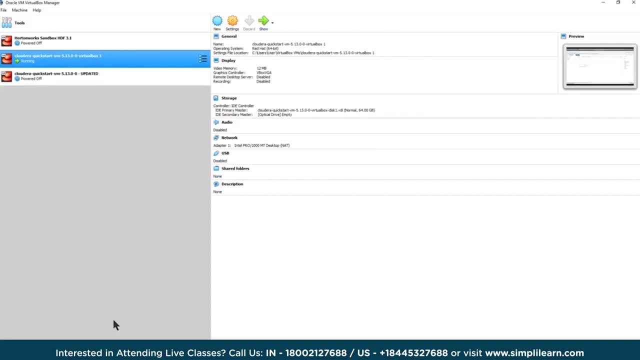 for a very long time, and you know a lot of the commands. I find it for most admins. it takes them about two to four hours the first time they go in and create a virtual machine and set up their own Hadoop. In this case, though, when you're just 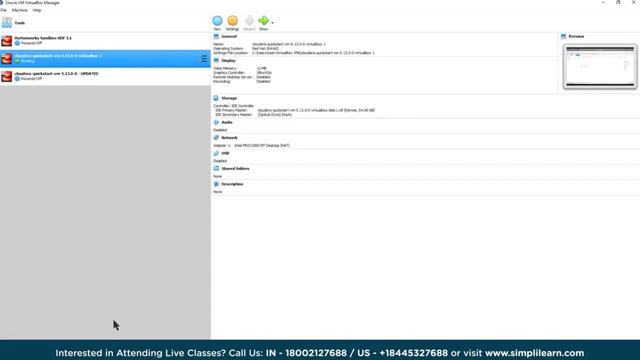 learning and getting set up. best to start with Cloudera. Cloudera also includes an installed version of MySQL. That way you don't have to reinstall the SQL version for importing data from and to Once you're in the Cloudera Quick Start. 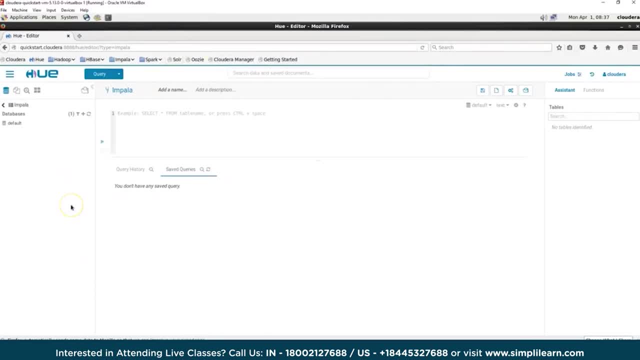 you'll see it opens a nice CentOS Linux interface And it has a desktop setup on there. This is really nice for learning. so you're not just looking at command lines And from in here it should open up by default to Hue. If not, you can click on Hue. 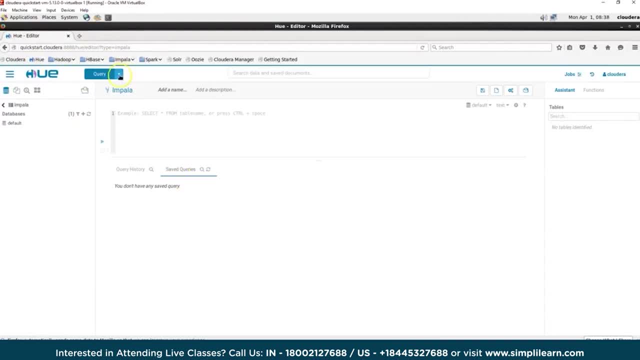 Hue's kind of a fun little web-based interface. Under Hue I can go under Query, I can pick an editor And we'll go right down to Scoop. So now I'm just going to load the Scoop editor in our Hue. 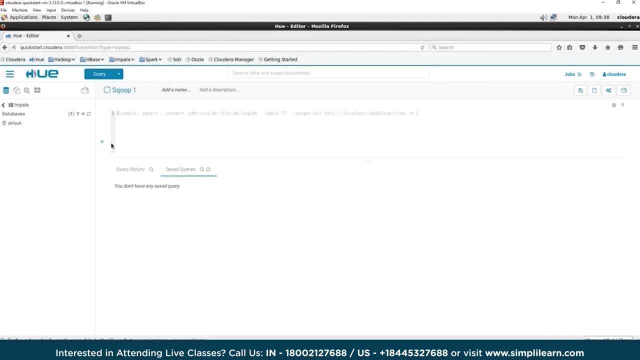 Now I'm going to switch over and do this all in command line. I just want to show that you can actually do this in Hue through the web-based interface. The reason I like to do the command line is specifically on my computer. it runs much quicker. 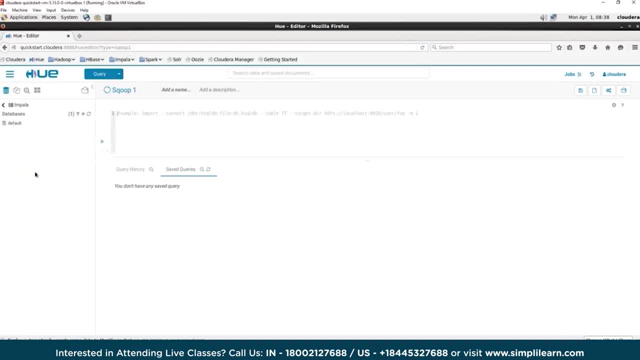 Or if I do the command line here and I run it, it tends to have an extra lag or an added layer in it. So for this we're going to go ahead and open our command line. The second reason I do this is we're 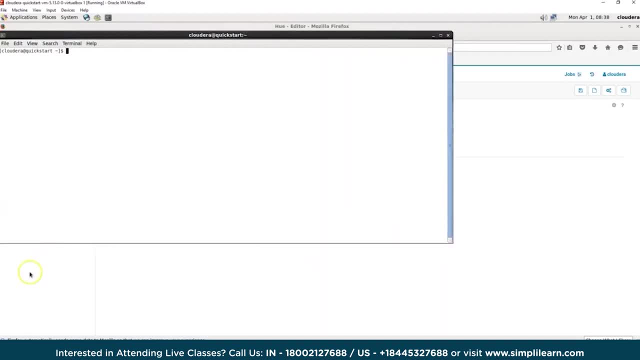 going to need to go ahead and edit our MySQL so we have something to scoop in. Otherwise I don't have anything going in there And of course we zoom in. We'll zoom in this and increase the size of our screen. So for this demo, our hands-on, I'm 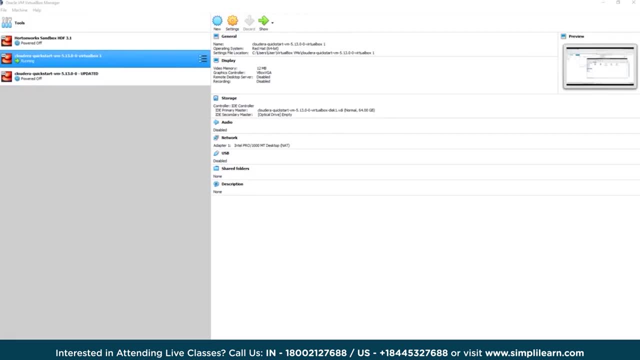 going to use Oracle VirtualBox Manager and the Cloudera Quick Start. If you're not familiar with this, we do have another tutorial we put out And you can send a note in the YouTube video below and let our team know and they'll send you a link. 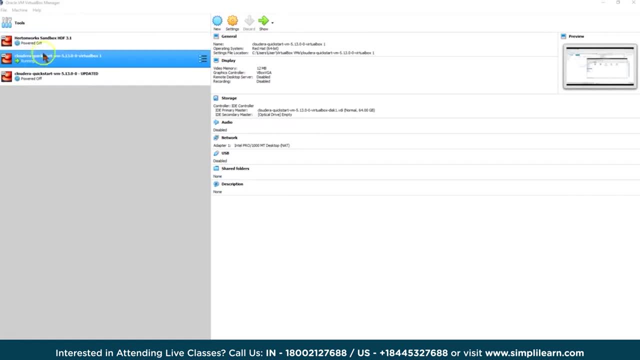 Or come visit wwwsimplylearncom. Now. this creates a Linux box on my Windows computer, So we're going to be in Linux And it'll be the Cloudera version with Scoop. It will also be using MySQL- MySQL Server. 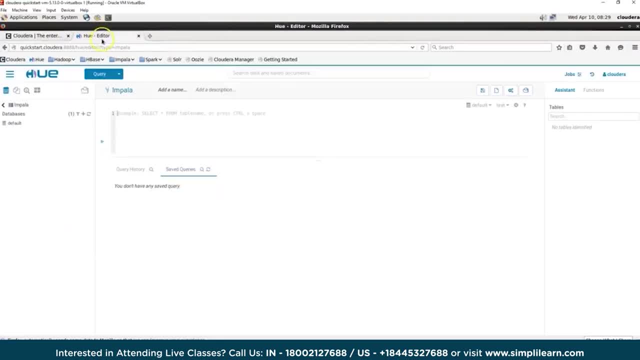 Once inside the Cloudera VirtualBox we'll go under the Hue Editor. Now we're going to do everything in Terminal Window, But I just want you to be aware that under the Hue Editor you can go under Query Editor. 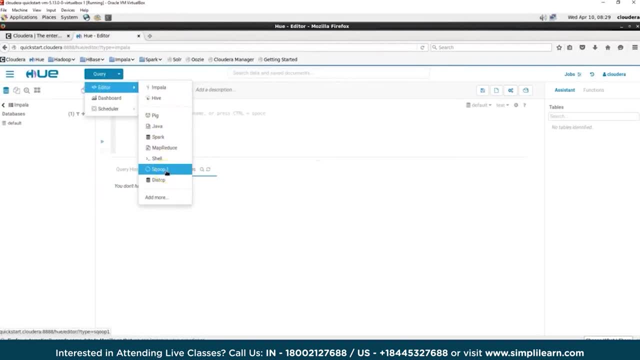 And you'll see as we come down here. here's our Scoop on this, So you can run your Scoop from in here. Now, before we do this, we have to do a little exploration in MySQL or MySQL Server. That way we know what data is coming in. 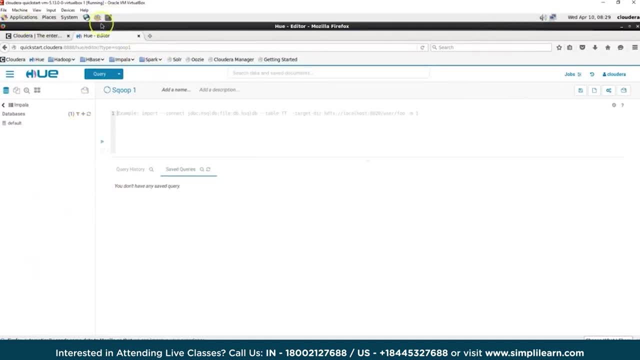 So let me go ahead and open up a Terminal Window In Cloudera. you have a Terminal Window at the top here that you can just click on and open it up, And let me just go ahead and zoom in on here. Go View and Zoom In. 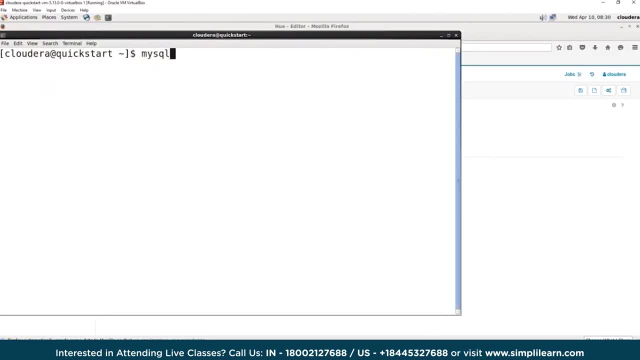 Now to get into MySQL Server, you simply type in MySQL And that's it, And this part will depend on your setup. Now the Cloudera Quick Start comes up, that the username is Root and the password is Cloudera. 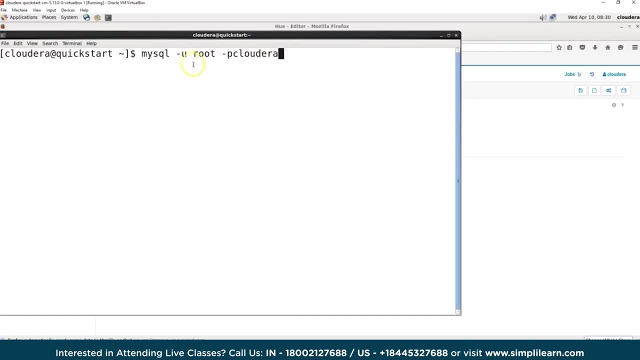 Kind of a strange quirk is that you can put a space between the minus U and the root, but not between the minus P and the Cloudera. Usually you'd put in a minus capital P and then it prompts you for your password on here. 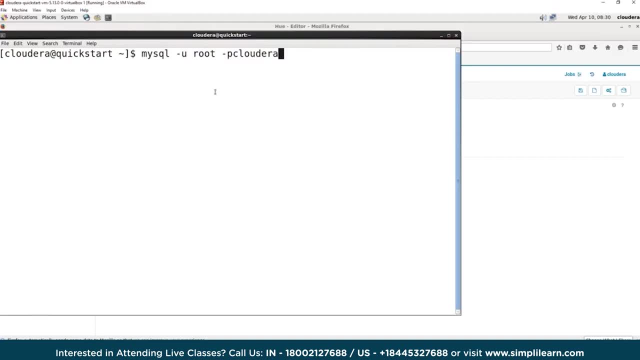 For this demo. I don't worry too much about you knowing the password on that, So we'll just go right into MySQL Server, since this is the standard password for this: Quick Start. And you can see we're now into MySQL And we're going to do just a couple of quick commands in here. 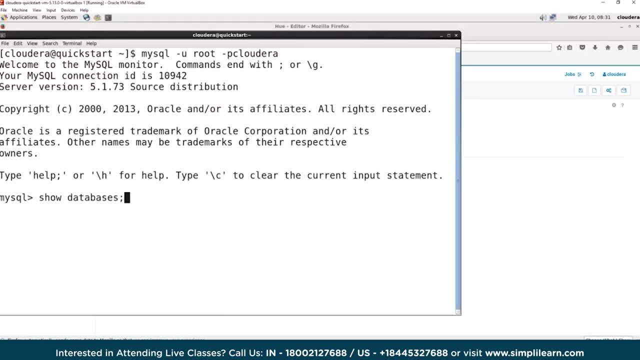 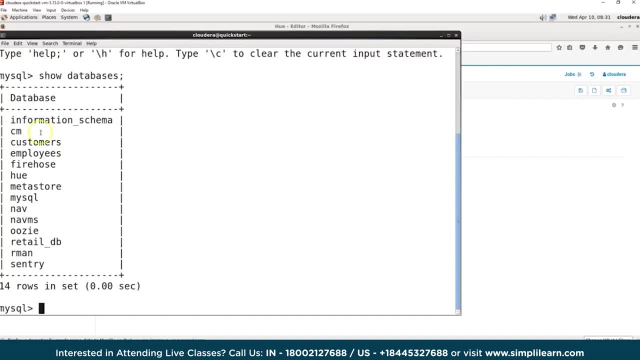 There's Show Databases And you follow by the semicolon. That's standard in most of these shell commands. So it knows it's the end of your shell command And you'll see in here in the Quick Start: Cloudera, Quick Start. 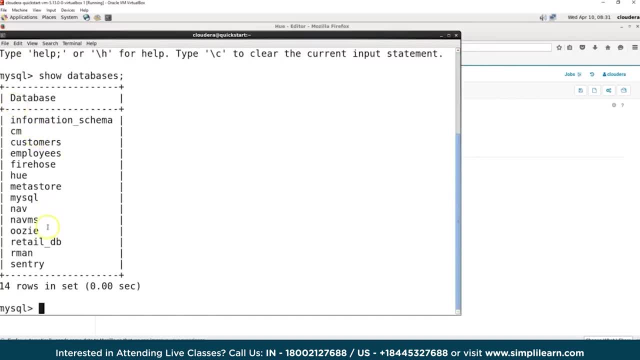 the MySQL comes with a standard set of databases. These are just some of these have to do with the Uzi, which is the Uzi part of Hadoop, where others of these- like Customers and Employees and stuff like that- those are just for demo purposes. 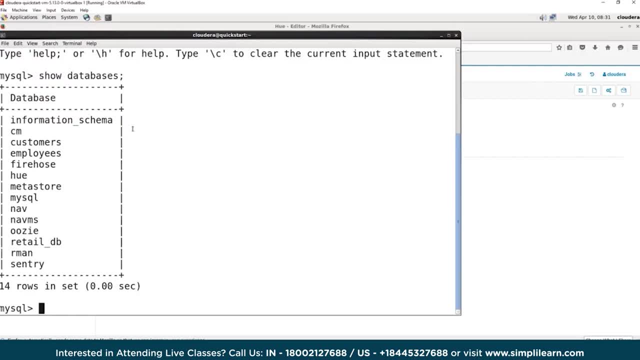 They come as a standard setup in there so that people going in for the first time have a database to play with, which is really good for us. so we don't have to recreate those databases And you will see on the list here we have a Retail underscore DB. 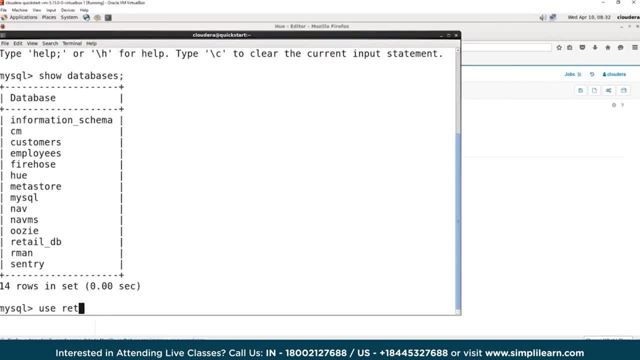 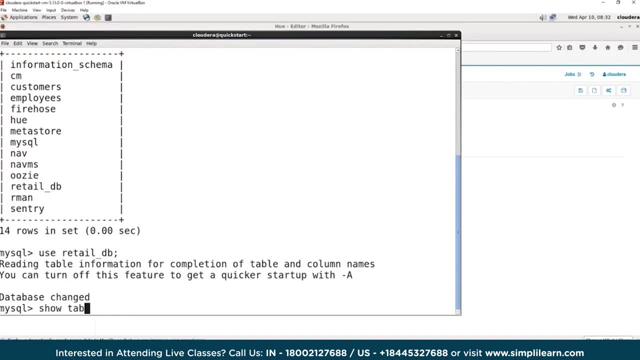 And then we can simply do Use Retail underscore DB. This will set that as a default in MySQL. And then we want to go ahead and show the tables, And if we show the tables you can see under the database the Retail DB database. 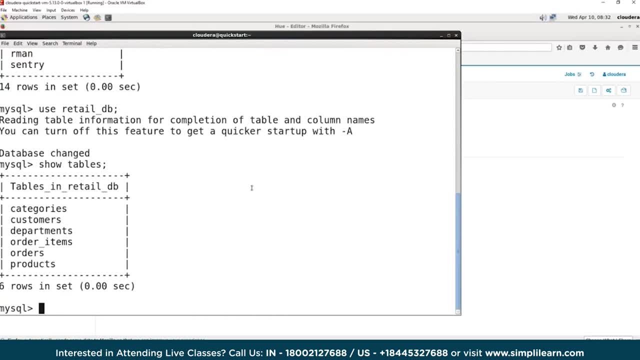 we have Categories, Customers, Departments, Order Items, Orders, Products. So there's a number of tables in here And we're going to go ahead and just use a standard SQL command. And if you did our Hive language, you'll note. remember it's the same for HQL. also on this, 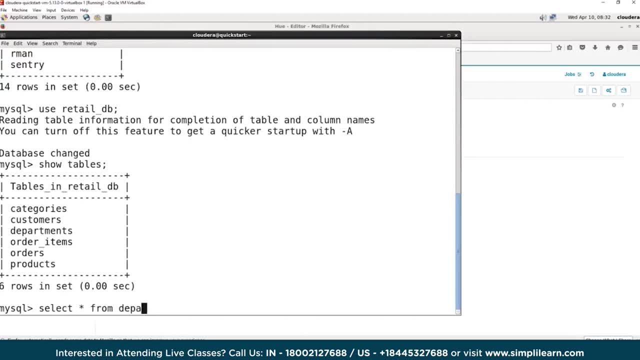 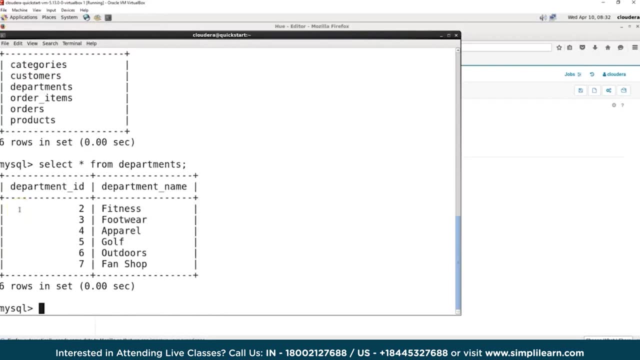 We're just going to select star everything from Departments. So there's our Departments table And we're going to list everything on the Departments table And you'll see we have six lines in here and it has a Department ID and a Department Name. 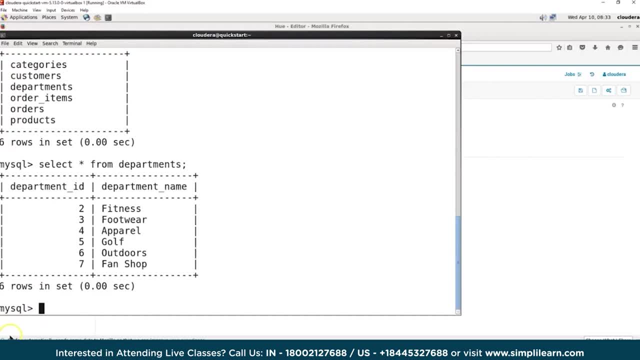 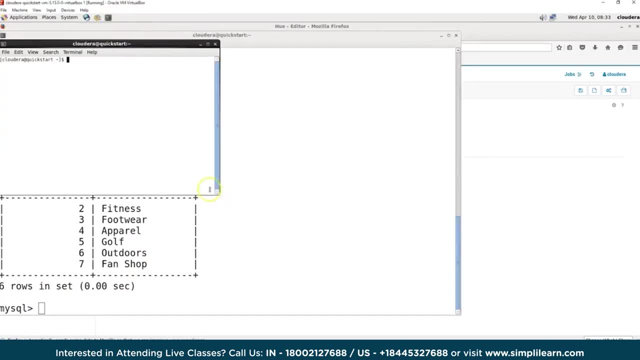 Two for Fitness, three for Footwear, so on and so forth. Now, at this point I can just go ahead and exit, But it's kind of nice to have this data up here so we can look at it and flip back and forth between the screens. 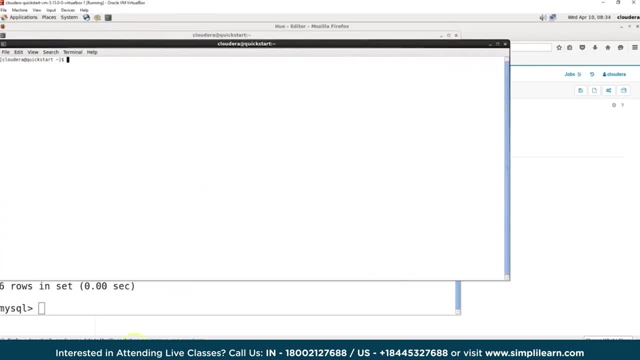 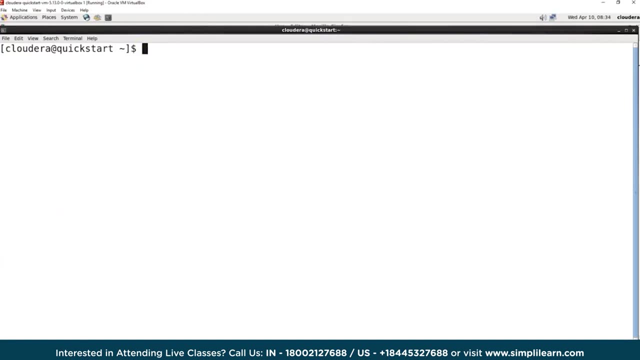 So I'm going to open up another terminal window And we'll go ahead and zoom in on this also. And it isn't too important for this particular setup, but it's always kind of fun to know what setup you're working with. What is your host name? 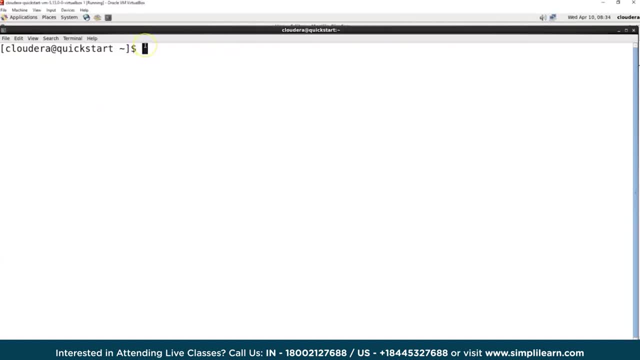 And so we'll go ahead and just type that in. This is a Linux command and it's a host name Minus F, And you see we're on Quick Start Cloudera. No surprise there. Now this next command is going to be a little bit longer. 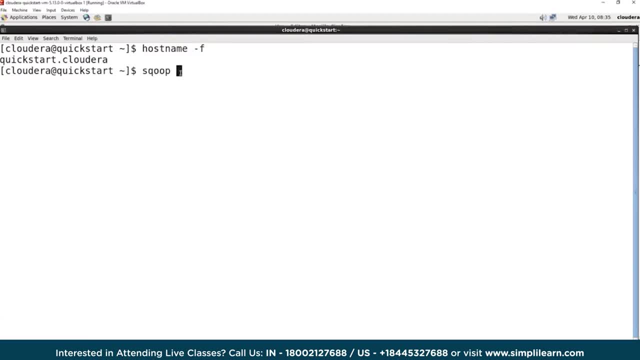 because we're going to be doing our first Scoop command And I'm going to do two of them. We're going to list Databases and list Tables. This is going to take just a moment to get through this because there's a bunch of stuff going on here. 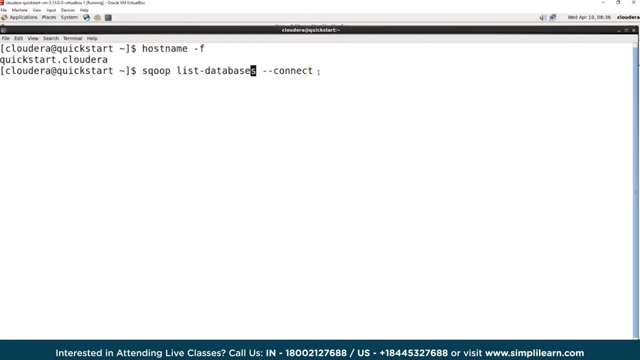 So we have Scoop, we have List Databases, we have Connect And under the Connect command, we need to let it know how we're connecting. We're going to use the JDBC. This is a very standard one: JDBC- MySQL. 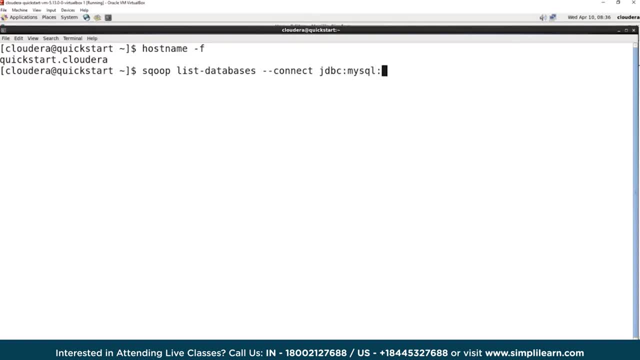 So you'll see that if you're doing an SQL database, that's how you start it off with, And then the next part. this is where you have to go look it up. It's however it was created. So if your admin created a MySQL server, 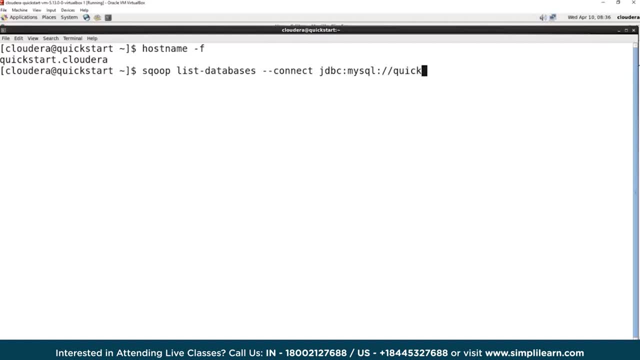 with a certain setup. that's what you have to go by And you'll see that usually they list this as Local Host, So you'll see something like Local Host. sometimes. There's a lot of different formats, But the most common is either Local Host. 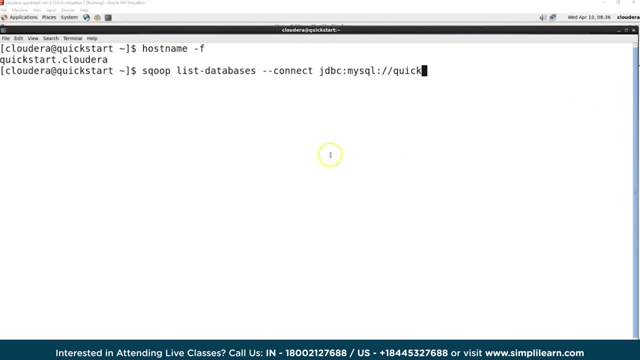 or the actual connection. So in this case we want to go ahead and do Quick Start 3306.. And so Quick Start is the name of the Local Host database and how it's hosted on here And when you set up the Quick Start for Hadoop. 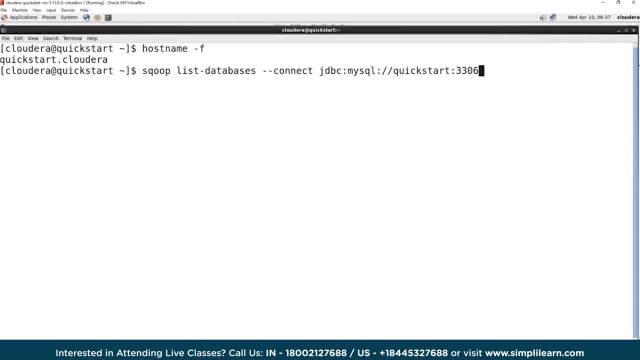 under Cloudera. it's port 3306 is where that's coming in, So that's where all that's coming from, And so there's our path for that. And then we have to put in our password. We type in the type password. 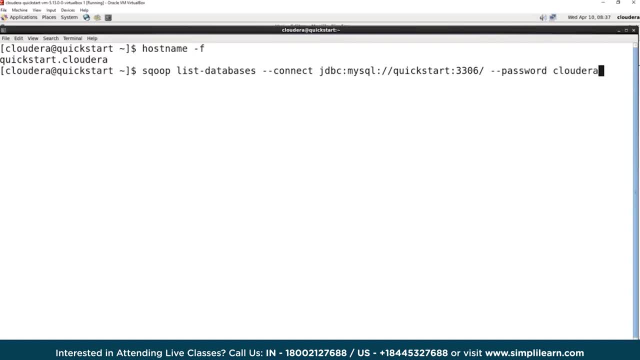 If you look it up, password on the Cloudera Quick Start is Cloudera And we have to also let it know the username And again, if you're doing this, you'd probably put in a minus capital. You can actually just do it for a prompt for the password. 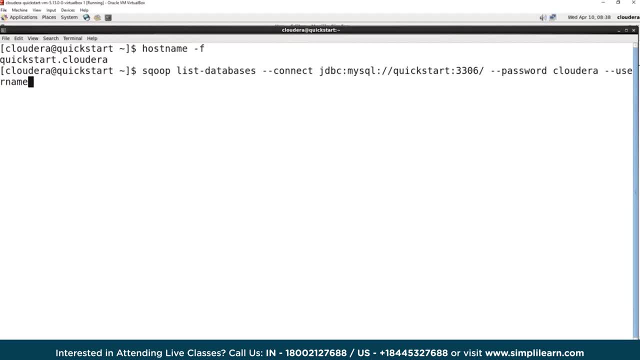 So if you leave that out, it'll prompt you, But for this it doesn't really matter. I don't care. if you see my password, It's the default one for Cloudera, Quick Start, And then the username on here is simply root. 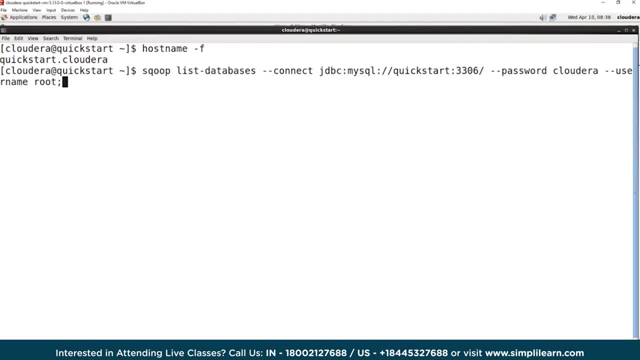 And then we're going to put our semicolon at the end And so we have here our full setup. Then we go ahead and list the databases And you'll see you might get some warnings on here. I haven't run the updates on the Quick Start. 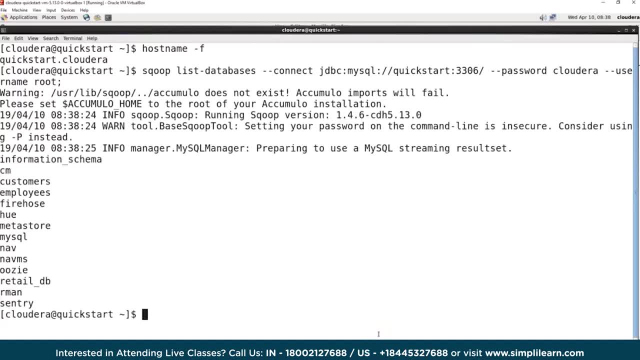 I suggest you're not running the updates either, if you're doing this for the first time, because it'll do some reformatting on there And it quickly pops up and you can see. here's all of the tables we went in there. And if we go back to the previous window, 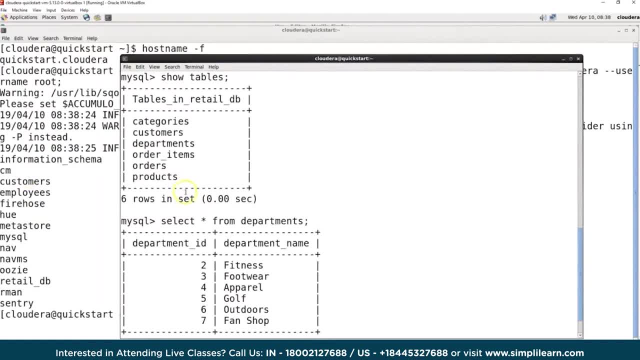 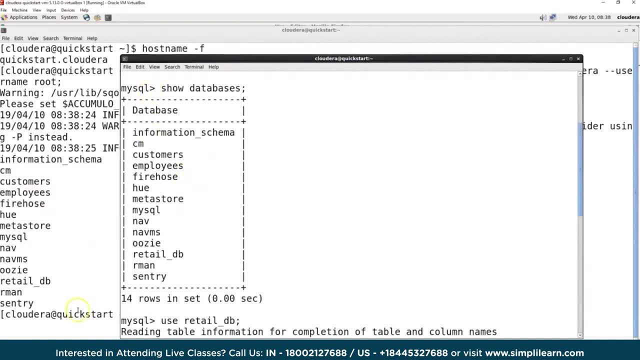 we should see that these tables match. So here we come in and here we have our databases And you can see back up here where we had the CM, customers, employees and so on. So the databases match. And then we want to go ahead and list the tables. 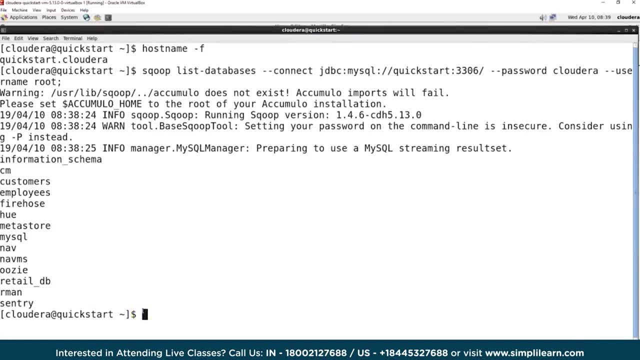 for a specific database, So let's go ahead and do that. I'm a very lazy typist So I'll put the up arrow in And you can see here: scoop list databases. We're just going to go back and change this from databases to list tables. 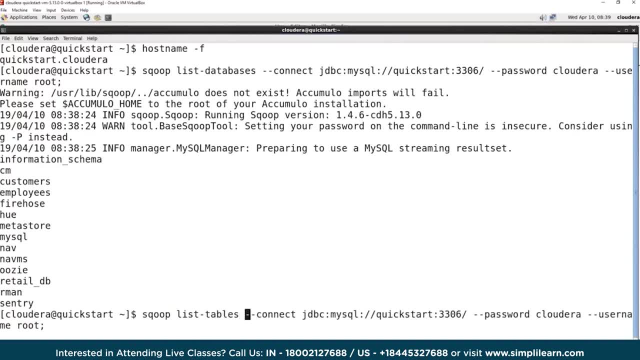 So we want to list the tables in here. Same connection, So most of the connection is the same, except we need to know which tables we're listing. An interesting fact is you can create a table without being under a database, So if you left this blank, it will show the open tables. 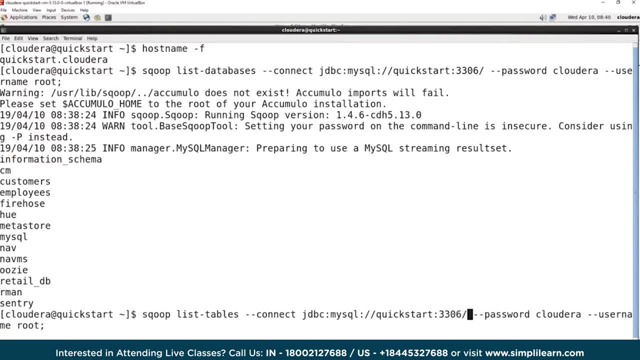 that aren't connected directly to a database or under a database. But what we want to do is, right past this last slash on the 3306, we want to put that retail underscore DB, because that's the database we're going to be working with. 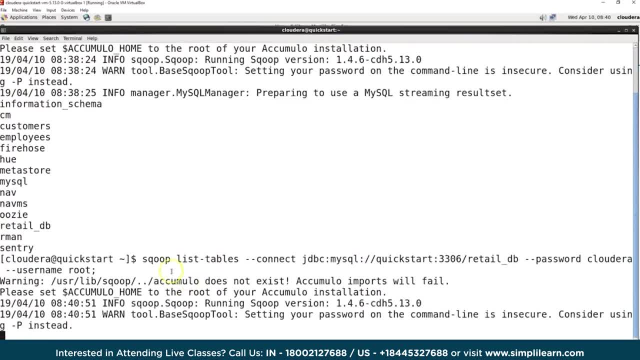 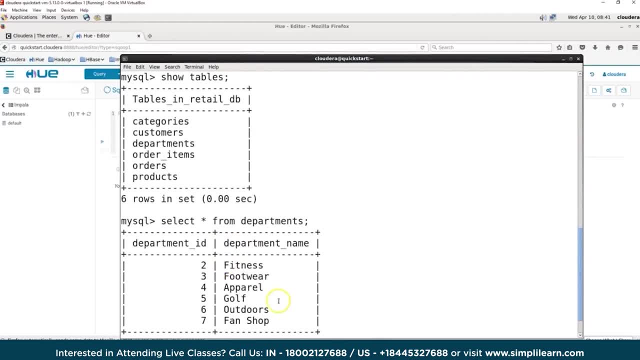 And this will go in there and show the tables listed under that database. And here we go. We got categories, customers, departments, order items and products. If we flip back here real quick, there it is the same thing we had. 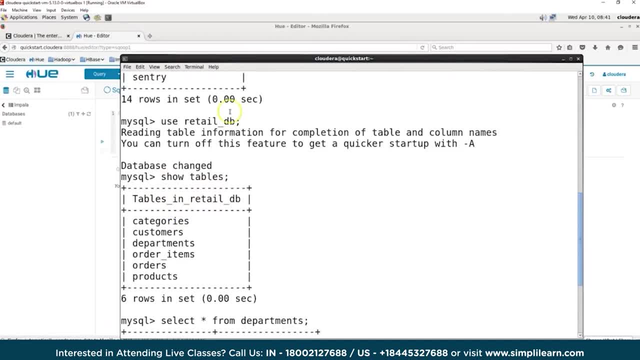 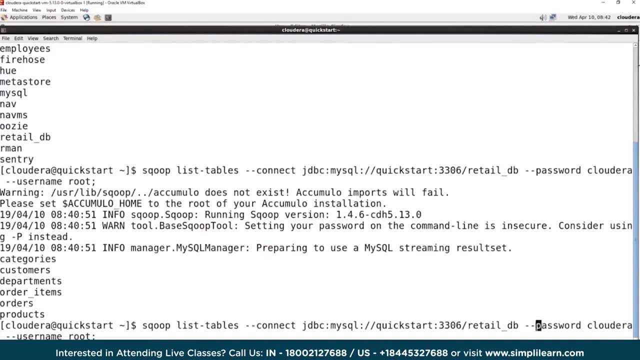 We had categories, customers, departments, order items and so on, And so let's go ahead and run our first import command, And again, I'm that lazy typer. so we're going to do scoop And instead of list tables. 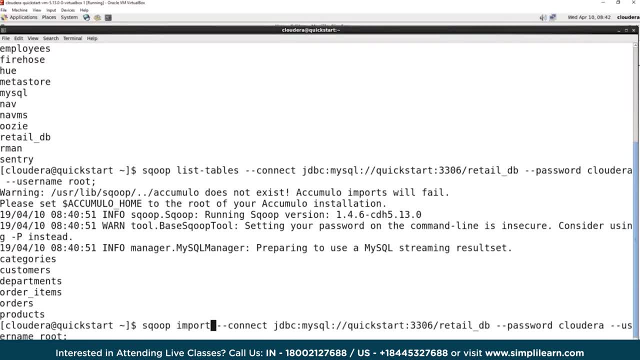 we want to go ahead and import. So there's our import command. And so once we have our import command in there, then we need to tell it exactly what we're going to import. So everything else is the same. We're importing from the retail DB, so we keep that. 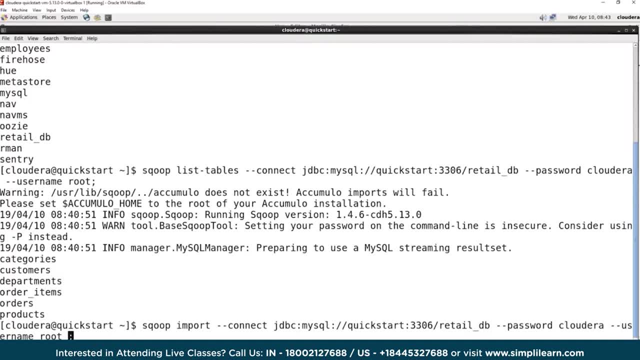 And then at the very end we're going to tag on dash dash table That tells us we can tell it what table we're importing from And we're going to import departments There we go. So this is pretty straightforward, because what's nice about this? 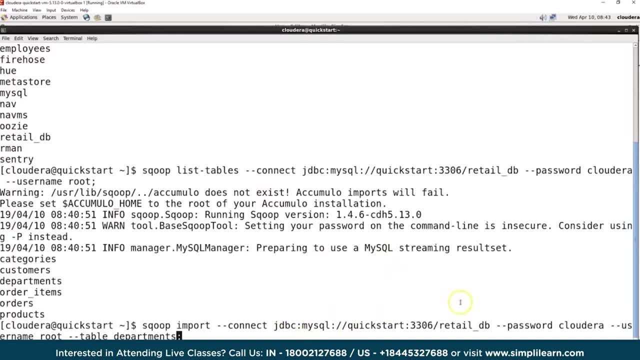 is. you can see the commands are the same. I got the same connection. I change it for whatever database I'm in. Then I come in here. Our password and the username are going to be the same. That's all under the MySQL server setup. 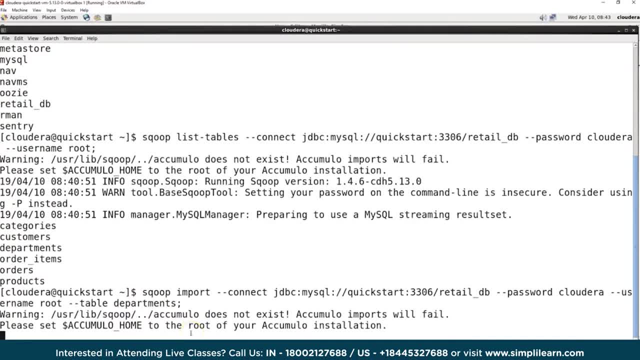 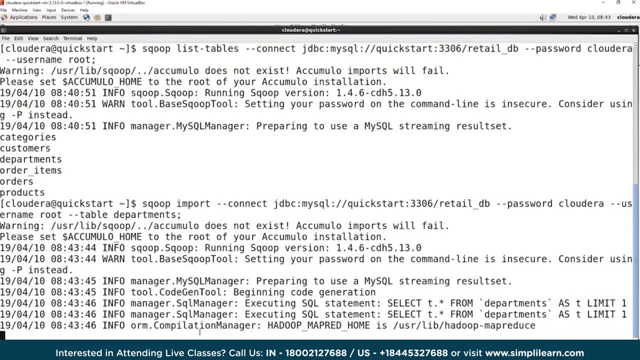 And then we let it know what table we're entering in. We run this And this is going to actually go through the mapper process in Hadoop. So this is a mapping process. It takes the data and it maps it up to different parts. 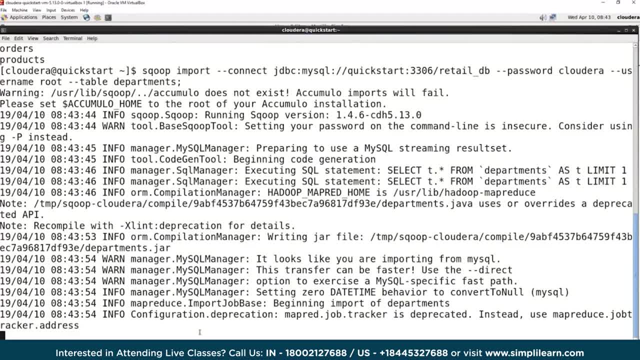 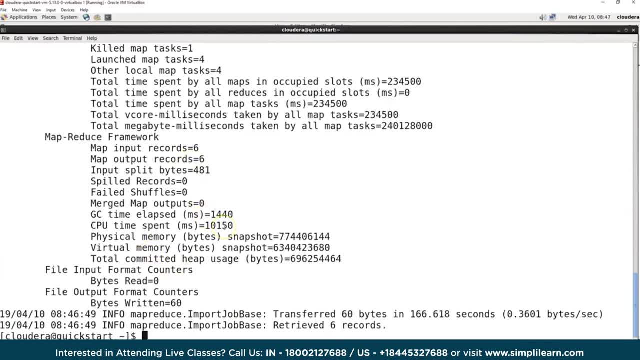 in the setup in Hadoop on there and then saves that data into the Hadoop file system- And it does take it a moment to zip through- Which I kind of skipped over for you, Since it is running a. you know it's designed to run across a cluster. 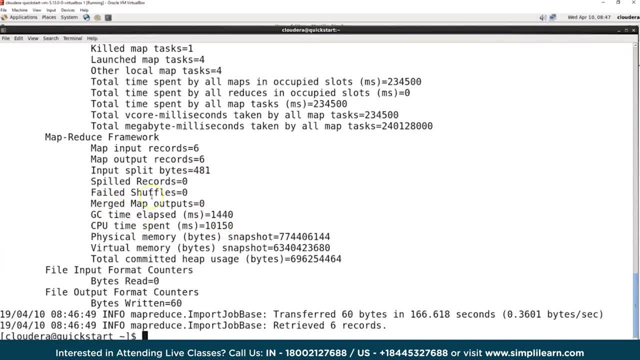 not on a single node. So when you're running on a single node it's going to run slow, even if you dedicate a couple cores to it. I think I put dedicated four cores to this one And so you can see right down here. 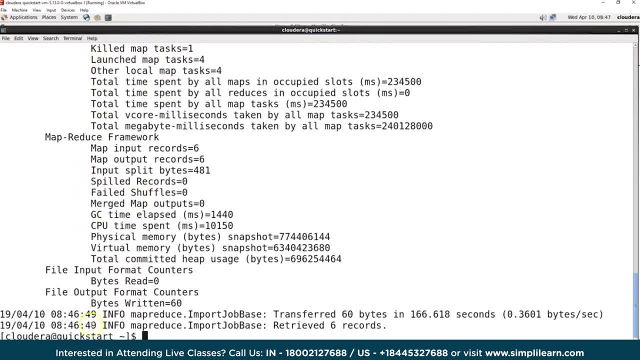 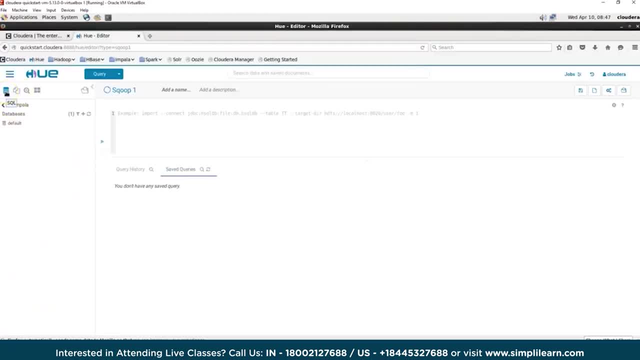 we get to the end. It's now mapped in that information And then we can go in here, We can go under, we can flip back to our Hue, And under Hue, on the top, I have there's databases, And the second icon over is your Hadoop file system. 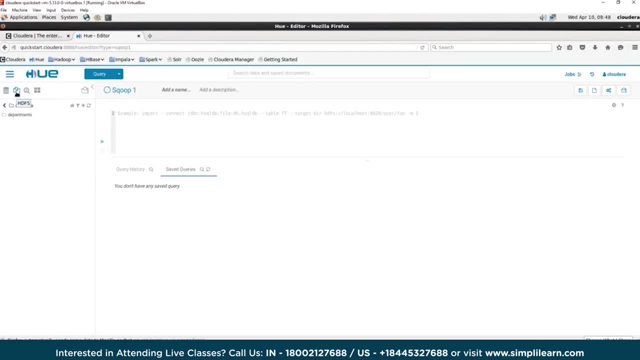 And we can go in here and look at the Hadoop file system And you'll see it show up underneath our documents. There it is departments, Cloudera departments, And you can see there's always a delay when I'm working in Hue. 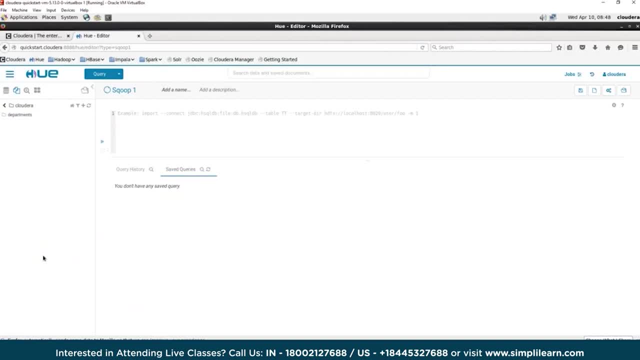 which I don't like, And that's the quick start issue. That's not necessarily running it on a server. When I'm running it on a server, you pretty much have to run through some kind of server interface. I still prefer the terminal window. 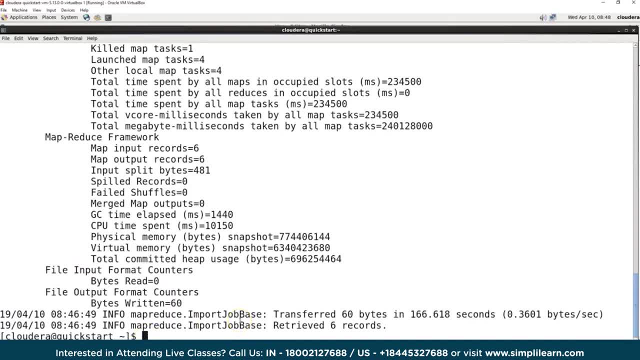 It still runs a lot quicker. But we'll flip back on over here to the command line And we can do the Hadoop type in the Hadoop FS and then list minus LS, And if we run this you'll see underneath our Hadoop file system. 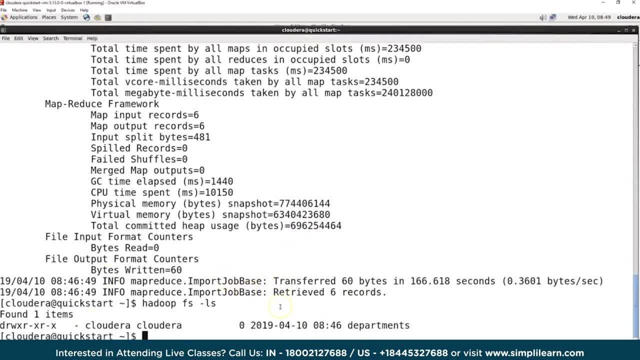 there is our departments, which has been added in, And we can also do Hadoop FS And this is kind of interesting For those who've gone through the Hadoop file system. everything you'll recognize this on here. I'm going to list the contents of departments. 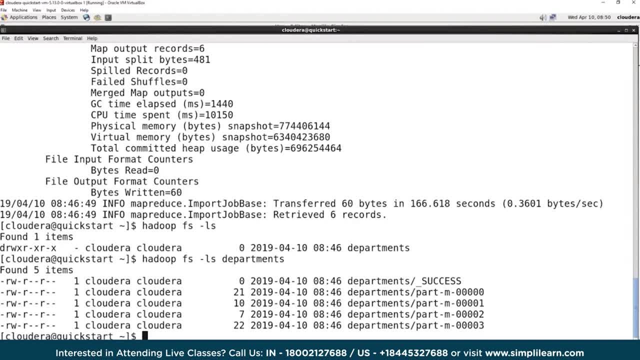 And you'll see, underneath departments we have part M000,, 001,, 002, 003.. And so this is interesting, because this is how Hadoop saves these files. This is in the file system. This is not in Hive, So we didn't directly import this into Hive. 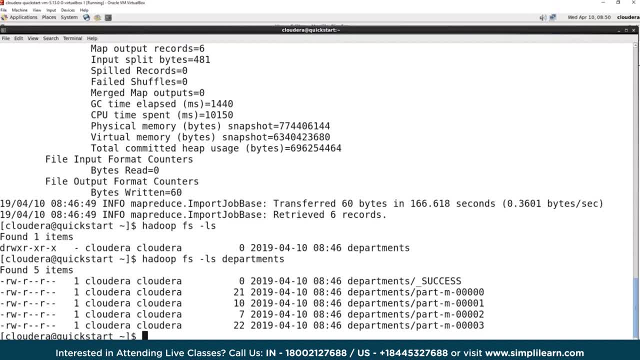 We put this in the Hadoop file system. Depending on what you're doing, you would then write the schema for Hive to look at the Hadoop file system. Certainly visit our Hive tutorial for more information on Hive specific So you can see in here. 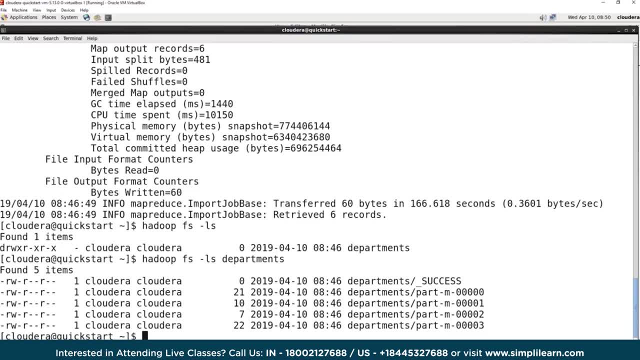 are different files that it forms that are part of departments, And we can do something like this: We can look at the contents of one of these files- FS minus LS, or a number of the files- And we'll simply do the full path. 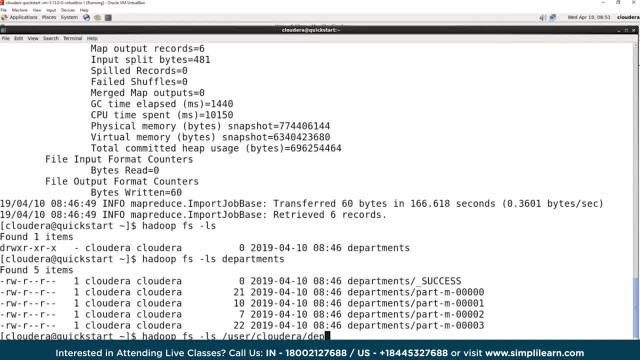 which is user Cloudera, And then we already know. the next one is departments, And then after departments we're going to put slash part star, So this is going to say anything that has part in it. So we have part dash, M000, and so on. 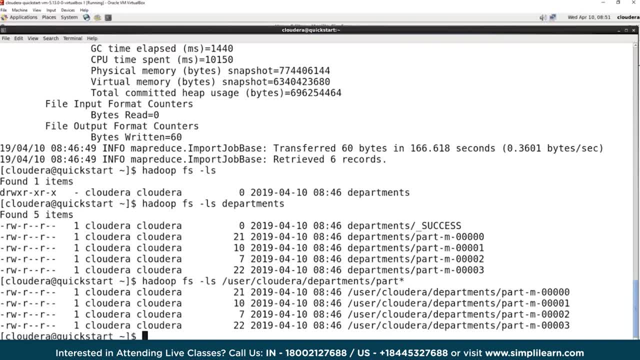 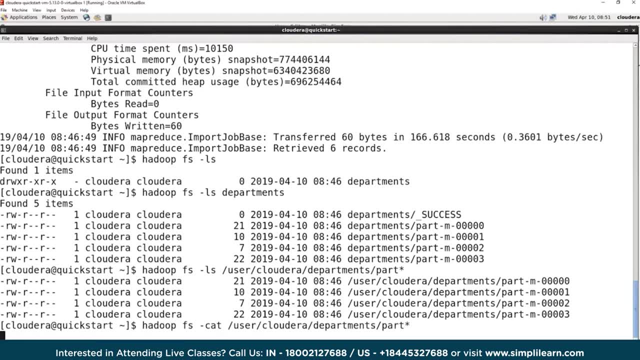 We can go ahead and cat use that cat command or that list command to bring those up, And then we can use the cat command to actually display the contents. And that's a Linux command, Hadoop Linux command to cat catinate. 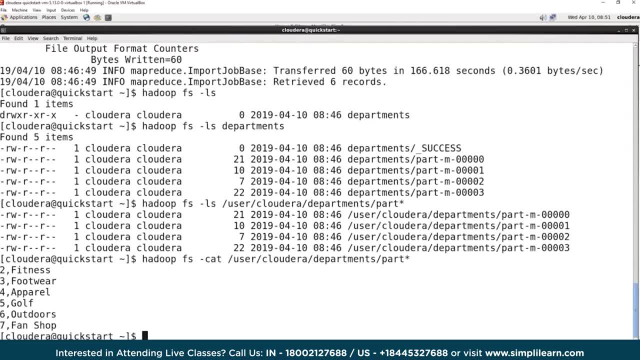 Not to be confused with catatonic catastrophic. There's a lot of cat got your tongue And we see here fitness footwear apparel. That should look really familiar because that's what we had in our MySQL server When we went in here. 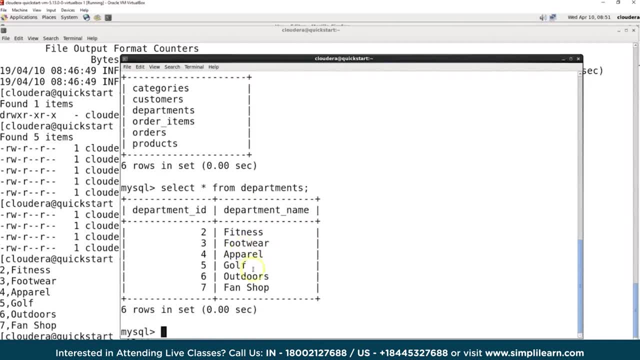 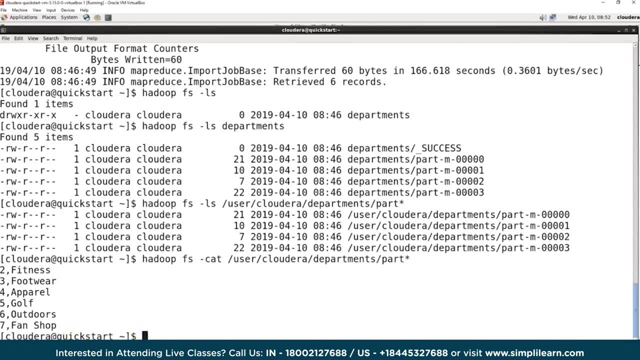 we did a select all on here. There it is Fitness, footwear, apparel, golf, outdoors and fan shop, And then, of course, it's really important let's look back on over here to be able to tell it. 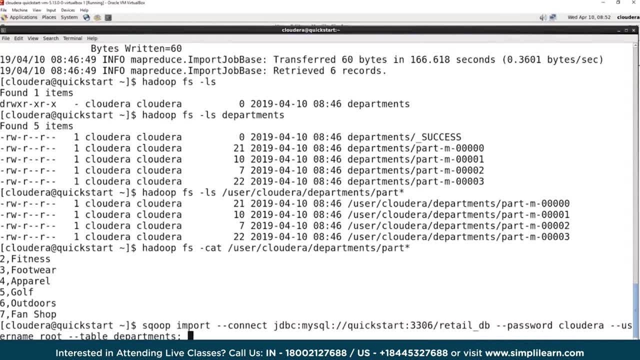 where to put the data. So we go back to our import command. So here's our scoop: import: We have our connect, We have the DB underneath our connection, our MySQL server. We have our password, our username, the table going where it's going to. 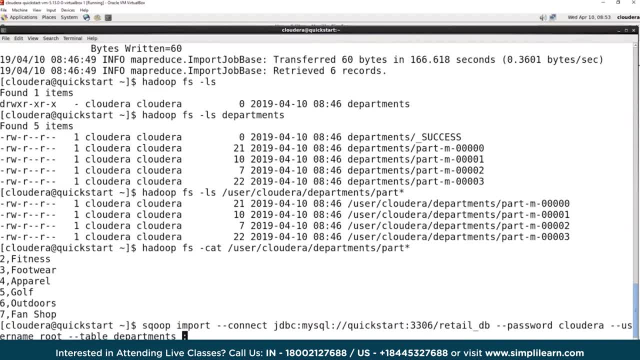 I mean the table where it's coming from, And then we can add a target on here. We can put in target dash directory And you do have to put the full path. That's a Hadoop thing. It's a good practice to be in. 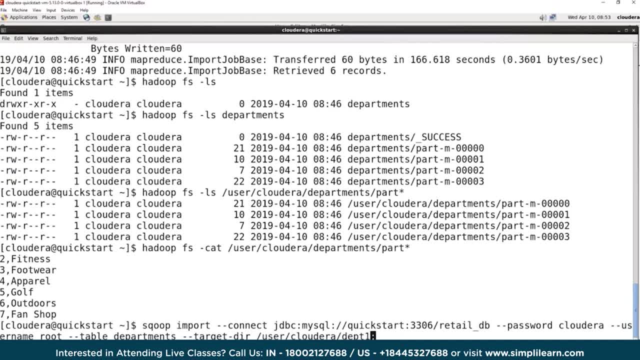 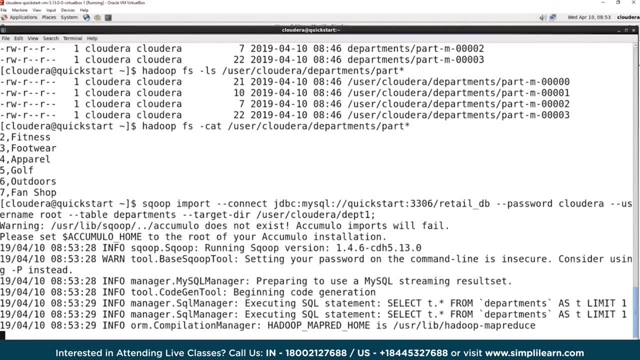 And we're going to add it to department. We'll just do department one, And so here we now add a target Target directory in here And user cloud era department one. And this will take just a moment before, So I'll go ahead and skip over the process. 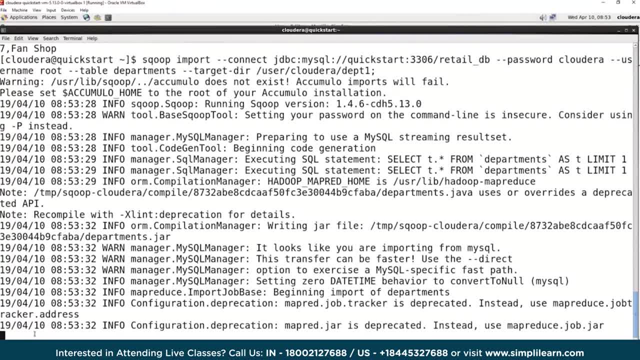 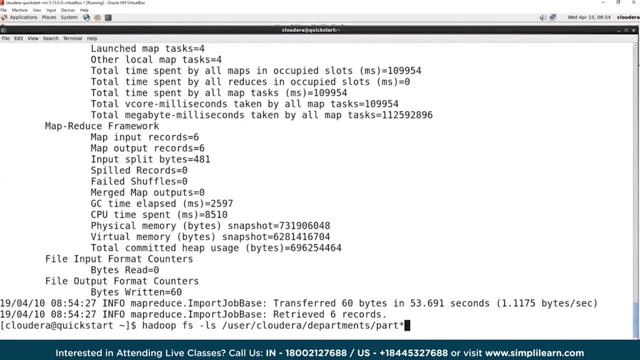 since it's going to run very slowly. It's only running on, like I said, a couple cores And it's also on a single node And now we can do the Hadoop. Let's just do the up arrow File system list. 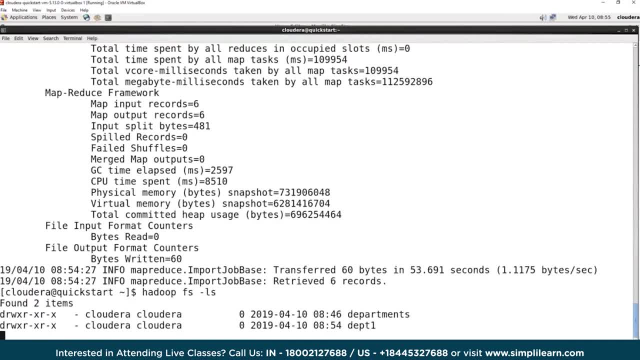 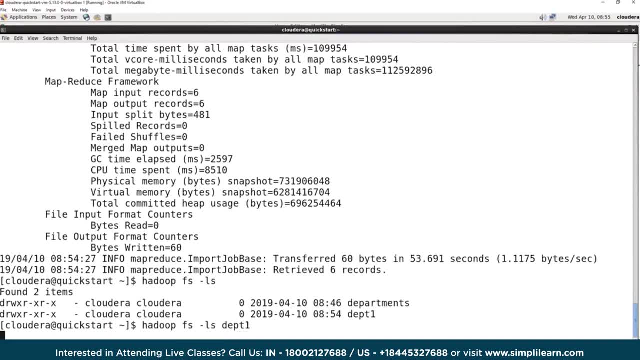 We want just straight list And when we do the Hadoop file system minus LS or list, you'll see that we now have department one And we can of course do list department one And you can see we have the files inside department one. 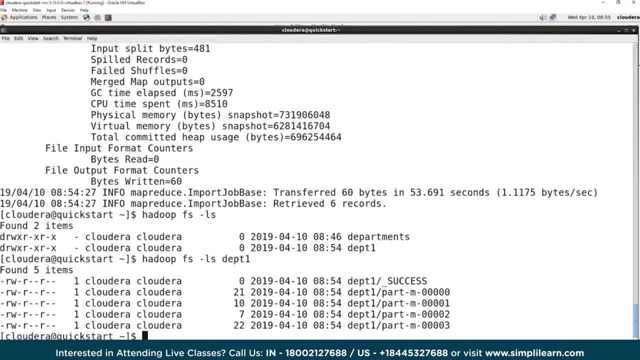 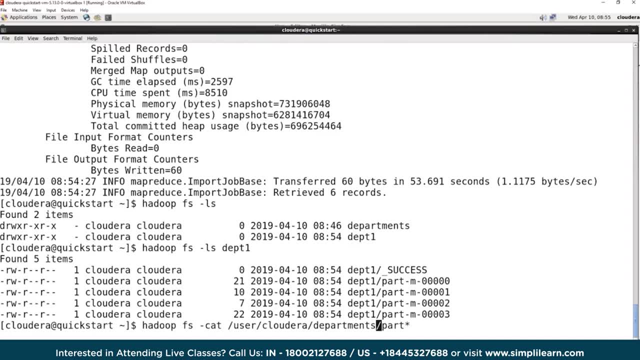 And they mirrored what we saw before, with the same files in there And the part M, O 00, and so on. If we want to look at them, it would be the same thing we did before with the cat, Except instead of departments. 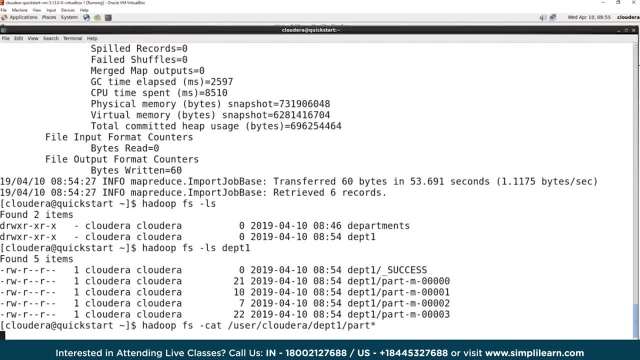 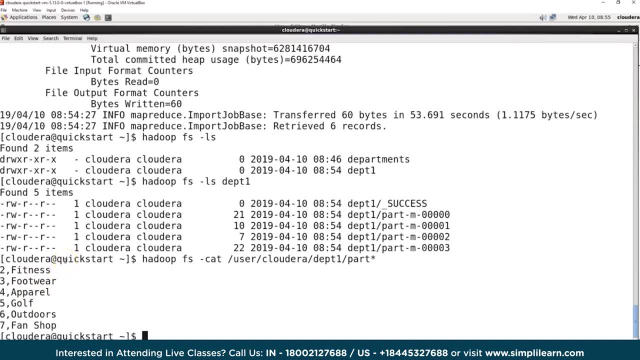 we'd be department one. There we go, And then that's going to come up with the same data we had before. Now, one of the important things when you're importing data- and it's always a question to ask- is: do you filter the data? 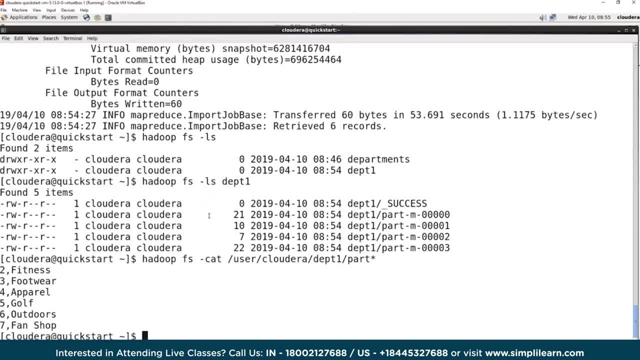 before it comes in? Do we want to filter this data as it comes in? so we're not storing everything in our file system? You would think: Hadoop, big data, put it all in there. I know from experience that putting it all in there 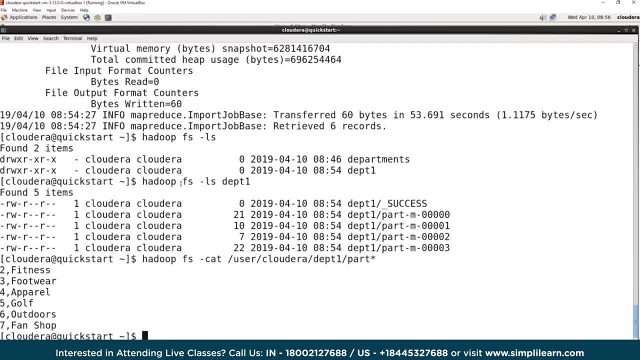 can turn a couple hundred terabytes into a petabyte very rapidly, And suddenly you're having to really add on to that data store and you're storing duplicate data sometimes. So you really need to be able to filter your data out, And so let's go ahead. 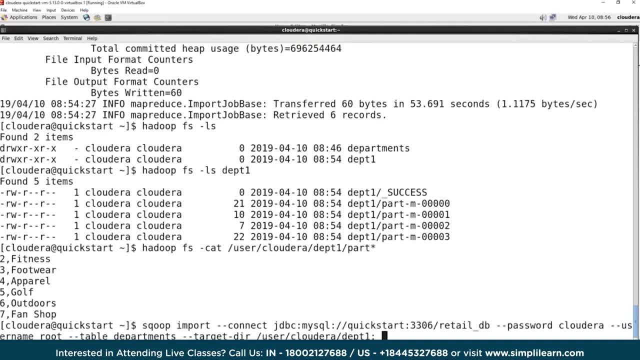 and use our up arrow to go to our last import, since it's still a lot the same stuff. So we have all of our commands under import. We have the command to add the target. We're going to change this to department two. 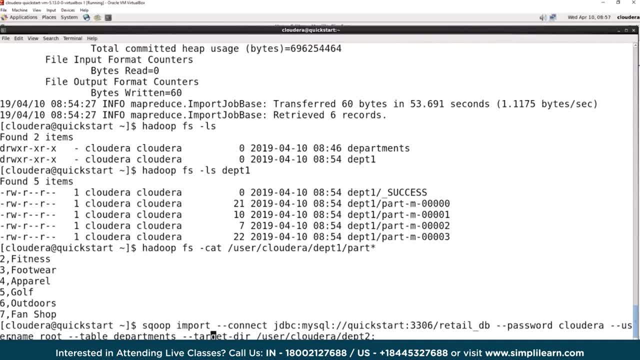 So we're going to create a new directory for this one, And then, after departments, there's another command that we didn't really slide in here and that's our mapping, And I'll show you what this looks like in a minute. So we're going to put M3 in there. 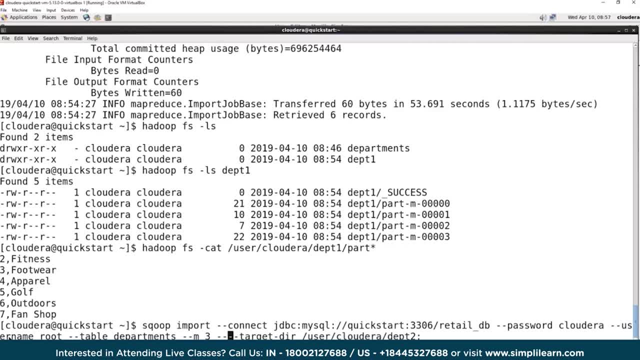 That doesn't have nothing to do with the filtering. I'll show you that in a second though, what that's for. And we just want to put in where. So where and what is the where In this case? we want to know. 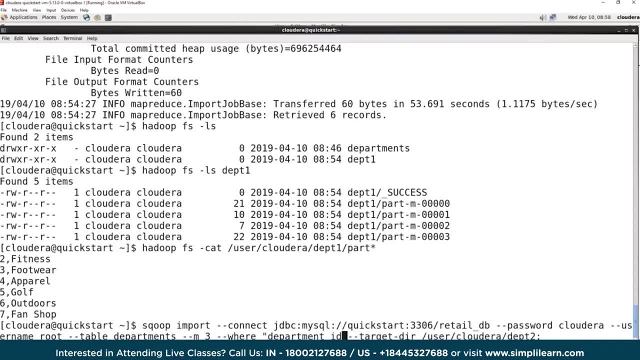 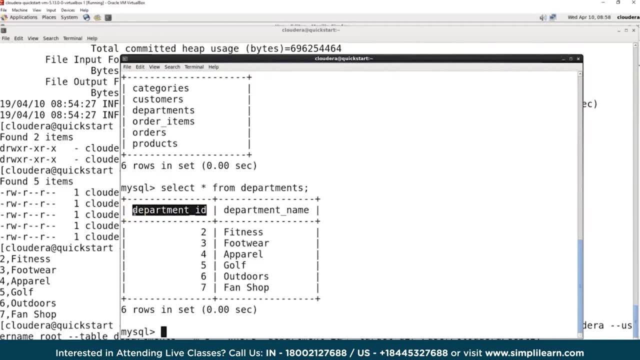 where department ID and if you want to know where that came from, we can find that if we flip back on over here, we have department underscore ID. So this is where that's coming from. That's just the name of the column on here. 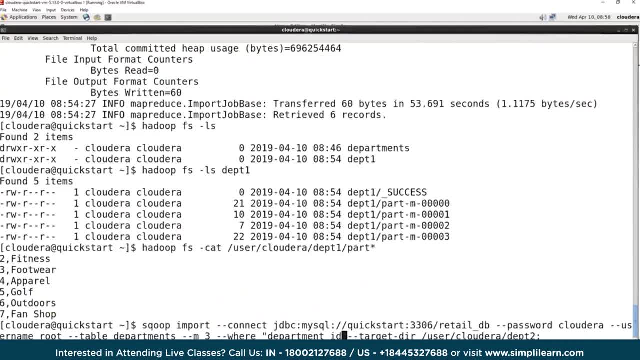 So we come in here to department. ID is greater than four, Simple logic. there You can see where you'd use that for: maybe creating buckets for ages, you know age from 10 to 15, 20 to 30. You might be looking for. 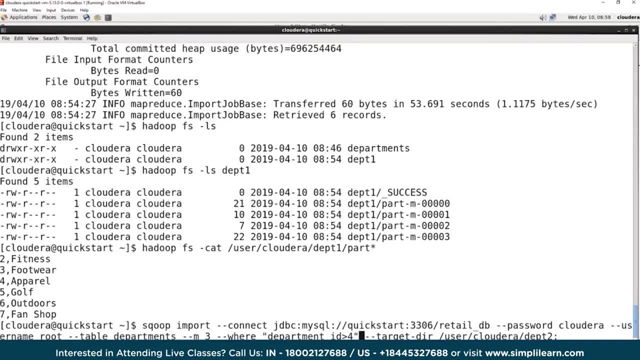 I mean, there's all kinds of reasons why you could use the where command on here And filter information out. Maybe you're doing word counting and you want to know words that are used less than 100 times. You want to get rid of the. 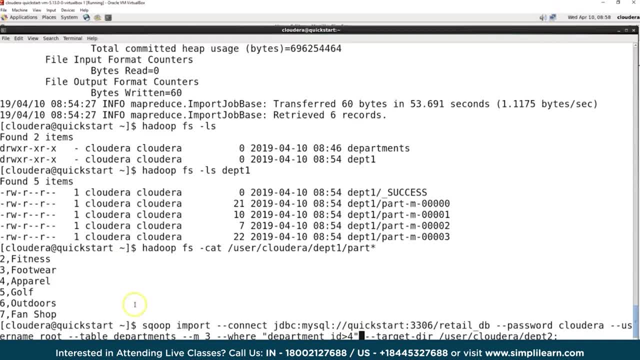 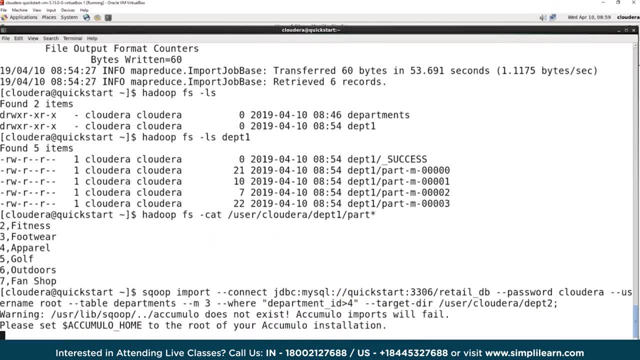 and is, and, and, and all the stuff that's used over and over again. So we'll go ahead and put the where and then department ID is greater than four, We'll go ahead and hit enter on here And this will create. 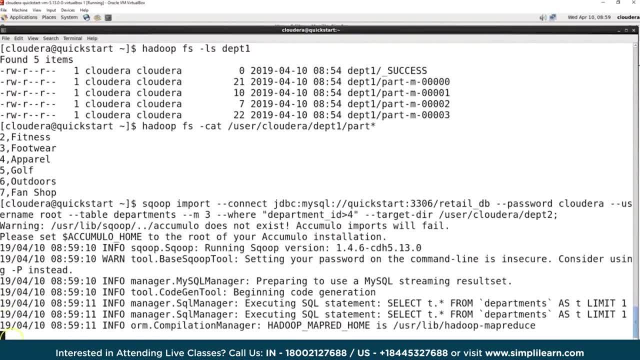 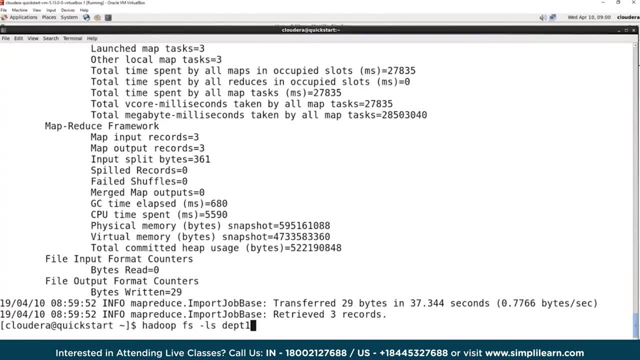 our department two setup on this And I'll go ahead and skip over some of the runtime. Again, it runs really slow on a single node. Real quick page through our commands. Let's see, here we go, Our list, and we should see underneath. 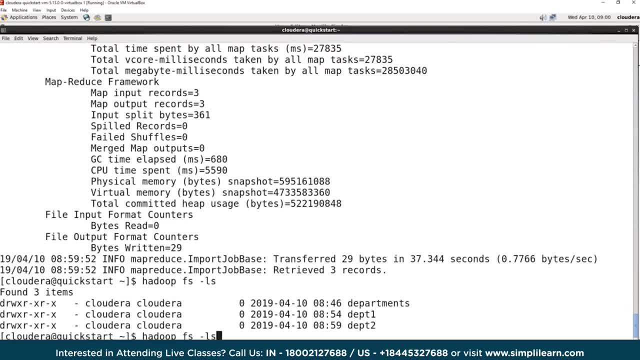 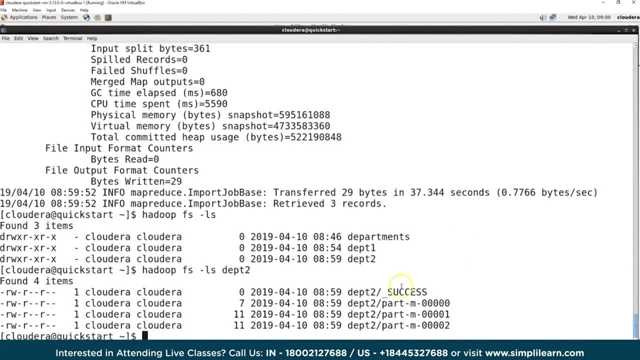 the list, the department two, on here now, And there it is Department two, And then I can go ahead and do list department two. You'll see the contents in here And you'll see that there is only three maps And it could be that the data 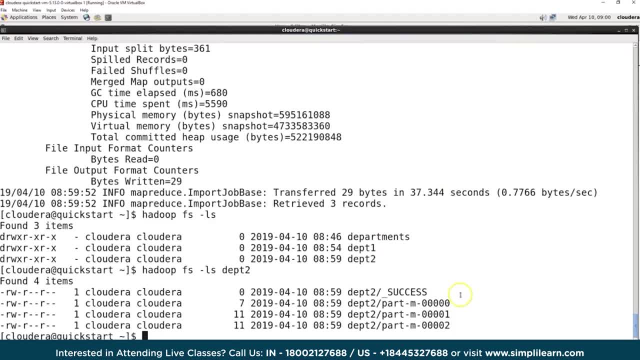 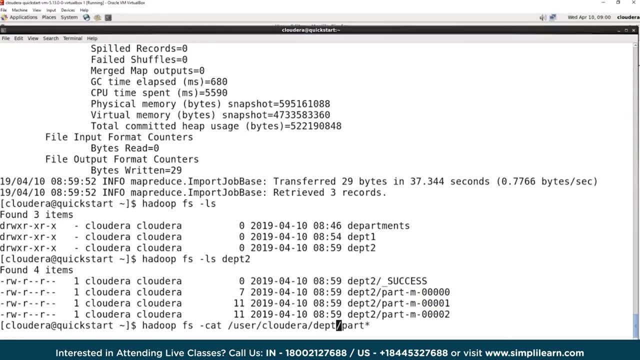 created three maps, But remember, I set it up to only use three mappers, So there's zero, one and two, And we can go ahead and do a cat on there. Remember, this is department two, So we want to look at. 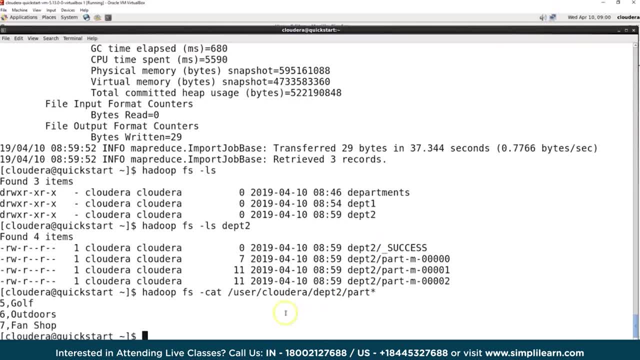 all the contents of these three different files. And there it is. It's greater than four. So we have: golf is five, outdoor is six, fan shop is seven. So we've effectively filtered out our data and just storing the data we want on our file system. 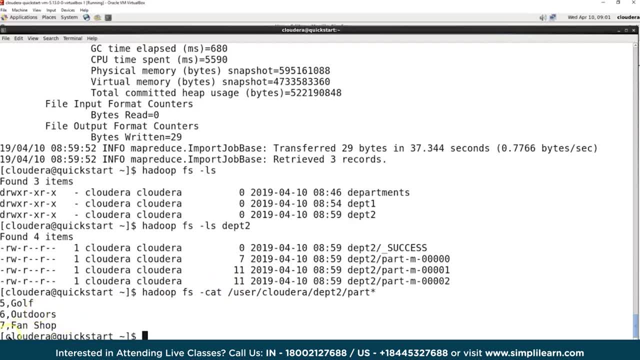 So if you're going to store data on here, the next stage is to export the data. Remember, a lot of times you have MySQL Server and we're continually dumping that data into our long-term storage and access the Hadoop file system. But what happens when you? 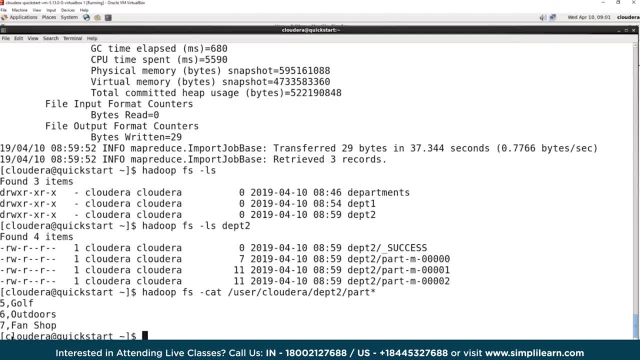 need to pull that data out and restore a database, Or maybe you have. you just merged with a new company- a favorite topic- merging company and merging databases- That's listed under nightmare, and how many different names for company can you have? 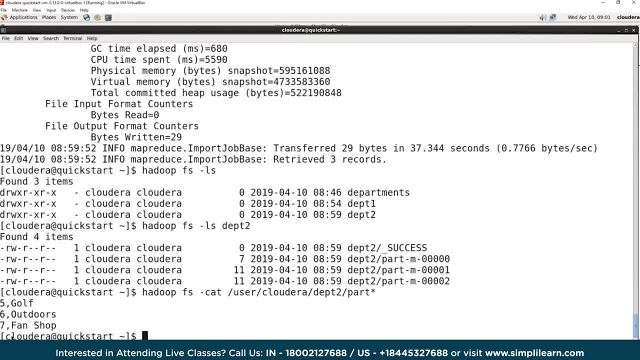 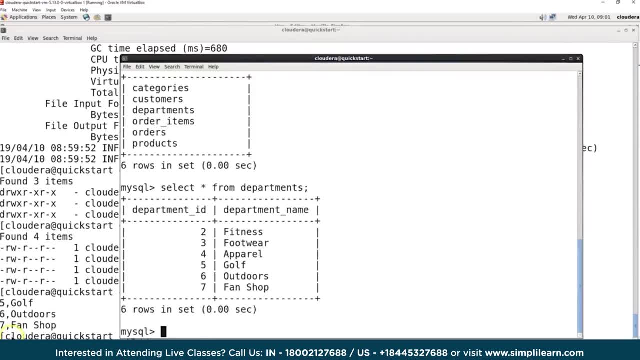 So you can see where being able to export is also equally important. And let's go ahead and do that And I'm going to flip back over to MySQL Server here And we'll need to go ahead and create our database we're going to export into 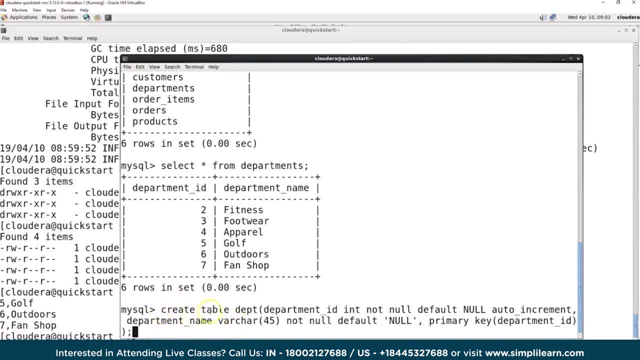 Now I'm not going to go too much in detail on this command. We're simply creating a table and the table's going to have. it's pretty much the same table we already have in here from departments, But in this case we're going to create. 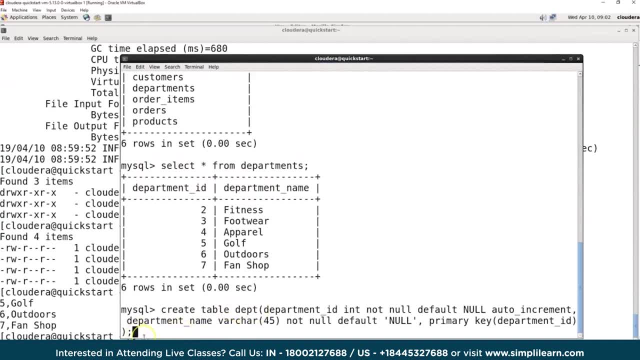 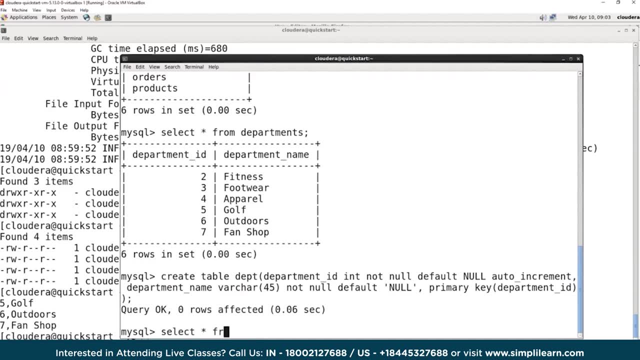 a table called DEPT. So it's the same setup but it's just going to. we're just giving it a different name, a different schema, And so we've done that and we'll go ahead and do a select star from DEPT. 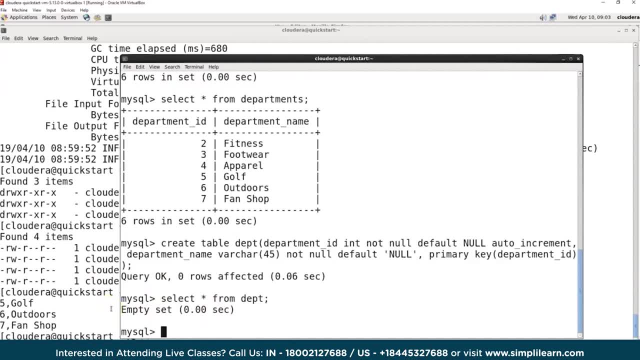 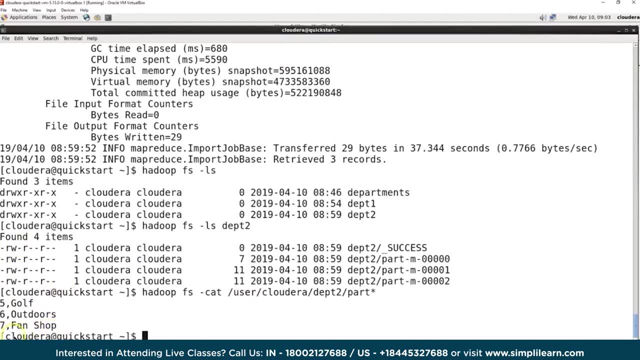 There we go And it's empty. That's what we expect: A new database, a new data table- and it's empty in there. So now we need to go ahead and export our data that we just filtered out into there. So let's flip back. 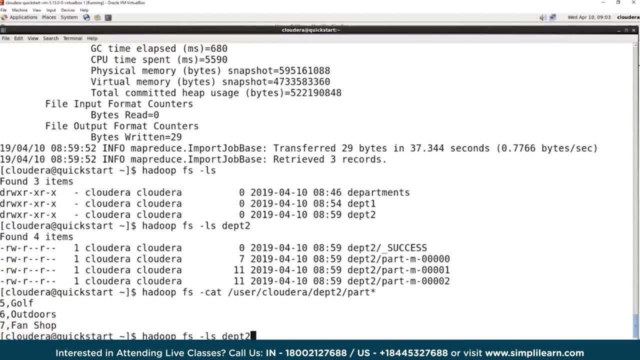 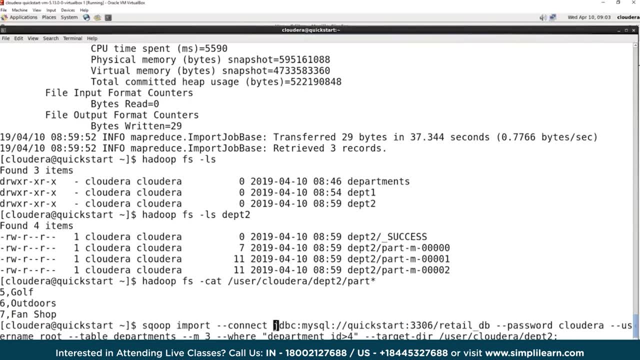 on over here to our scoop setup, which is just our Linux terminal window, And let's go back up to one of our commands: Scoop import. In this case, instead of import, we're going to take the scoop and we're going to export. 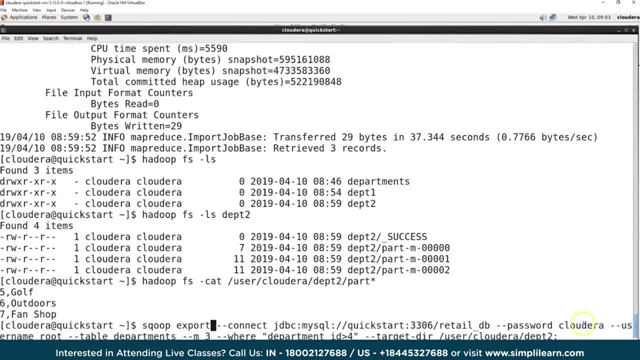 So we're going to just change that Export And the connection is going to remain the same. So same connect, same database. We're also we're still doing the retail DB. We have the same password, so none of that changes. 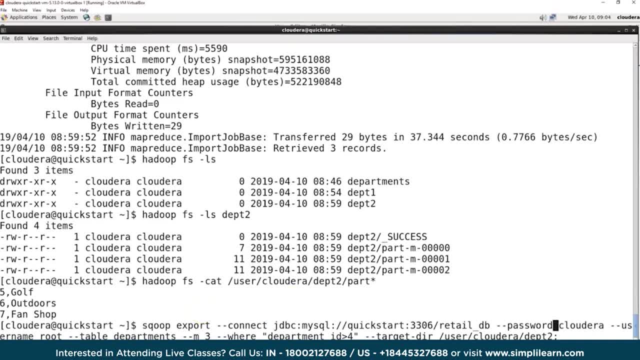 The big change here is going to be the table Instead of departments. remember, we changed it and gave it a new name, And so we want to change it here also: DEPT, So department We're not going to, don't worry about. 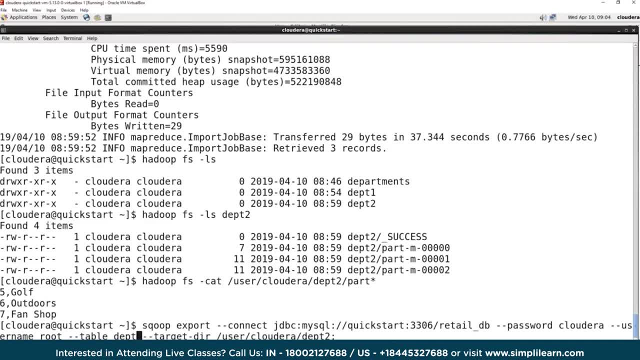 the mapper count and the where was part of our import. There we go. And then, finally, it needs to know where to export from. So instead of target directory, we have an export directory. That's where it's coming from, Still user. 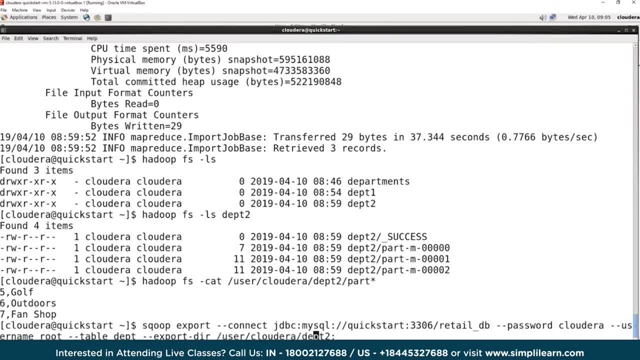 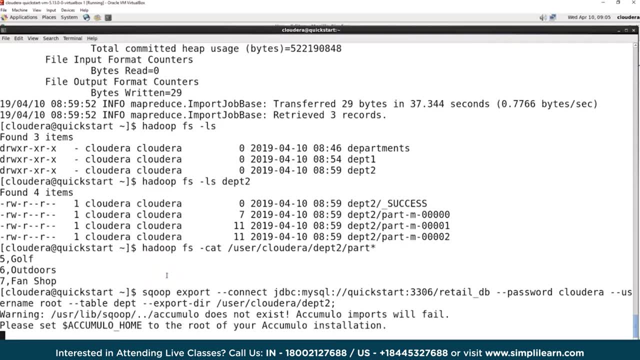 Cloudera, and we'll keep it as department too, Just so you can see how that data is coming back that we filtered in And let's go ahead and run this. It'll take it just a moment to go through its steps. 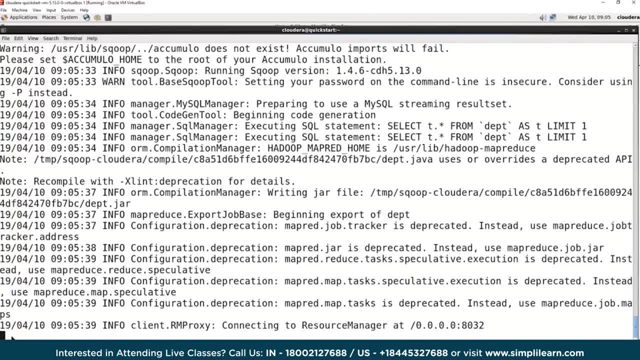 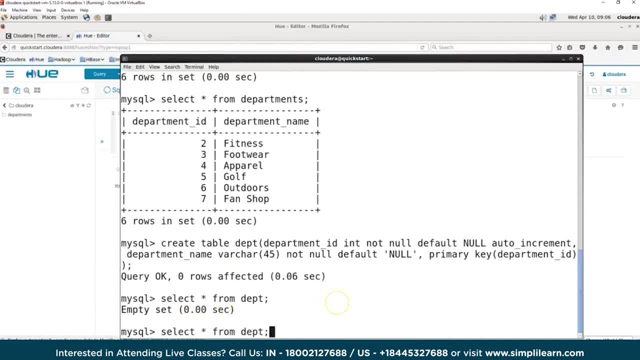 And again, because it's slow, I'm just going to go over here so you don't have to sit through it, And once we've wrapped up our export we'll flip back on over here to MySQL. Use the up arrow And this time we're going. 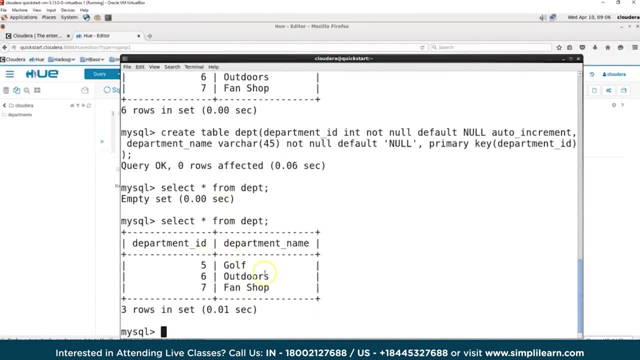 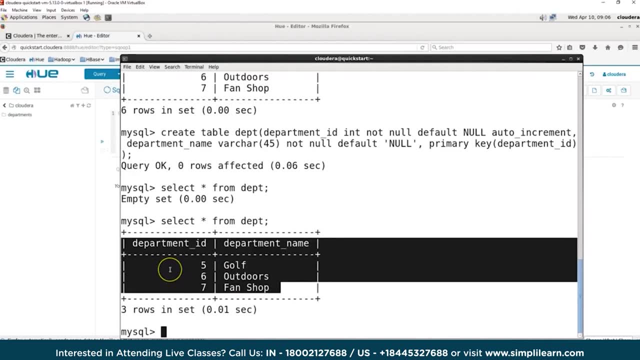 to select star from department And we can see that. there it is. It exported the golf outdoors and fan shop, And you can imagine also that you might have to use the where command in your export also. So there's a lot of mixing. 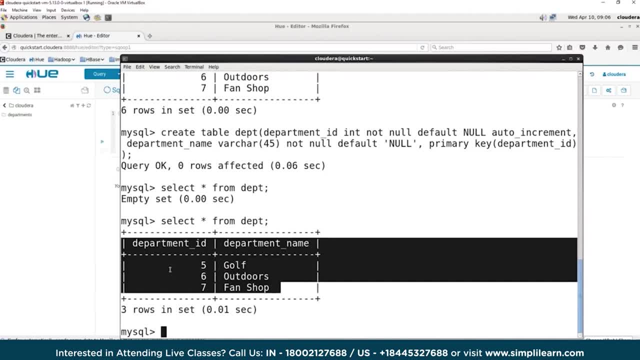 The command line for scoop is pretty straightforward. You're changing the different variables in there. whether you're creating a table listing a table listing databases, It's a great tool for bringing your data into the Hadoop file system and exporting it. 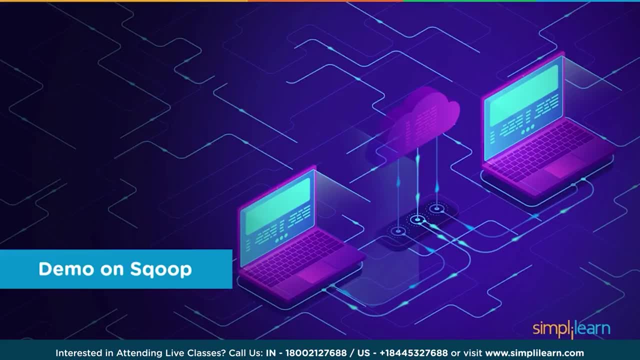 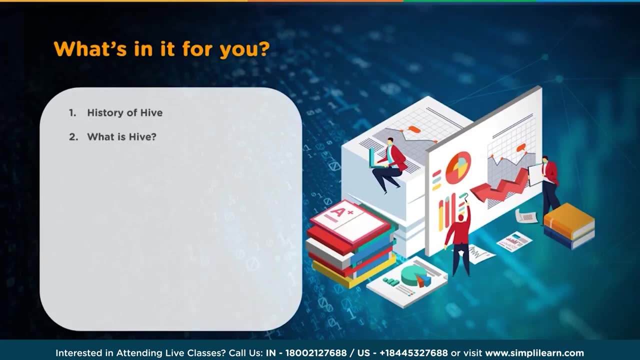 So, now that we've wrapped up our demo on scoop and gone through a lot of basic commands, that wraps it up for us today. First, we're going to start with the history of Hive. What is Hive? Architecture of Hive, Data flow in Hive. 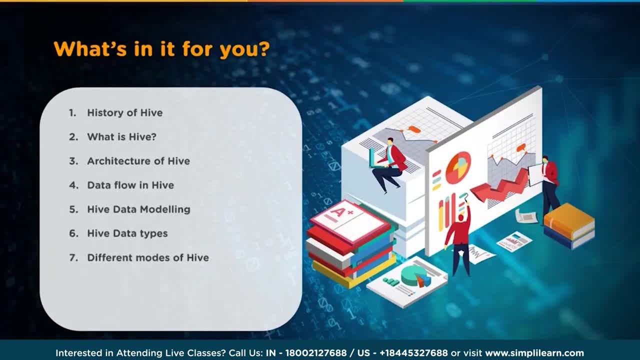 Hive data modeling, Hive data types, Different modes of Hive And difference between Hive and RDBMS. Finally, we're going to look into the features of Hive and do a quick hands-on demo on Hive in the Cloudera Hadoop file system. 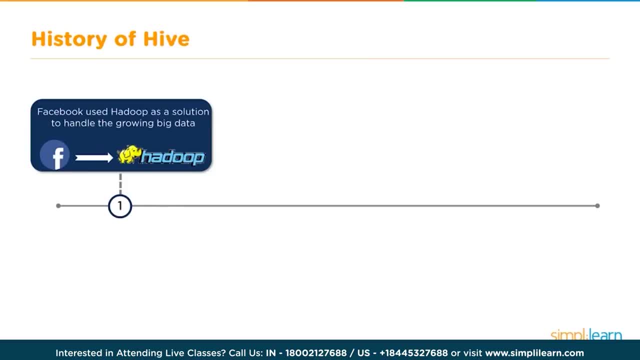 Let's dive in with a brief history of Hive. So the history of Hive begins with Facebook. Facebook began using Hadoop as a solution to handle the growing big data, And we're not talking about a data that fits on one or two or even five computers. 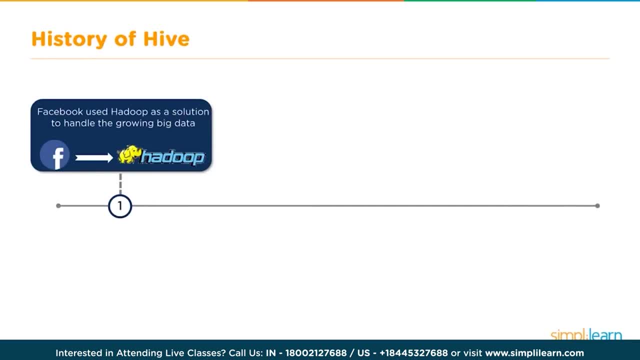 We're talking data that fits on. if you've looked at any of our other Hadoop tutorials, you'll know we're talking about very big data and data pools, And Facebook certainly has a lot of data it tracks. As we know, the Hadoop uses MapReduce. 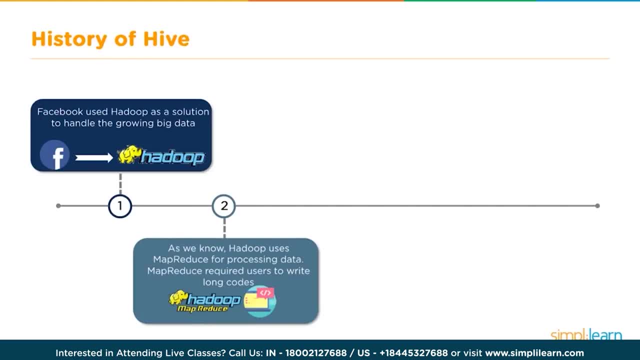 for processing data. MapReduce required users to write long codes, And so you'd have these really extensive Java codes, very complicated for the average person to use. Not all users reversed in Java and other coding languages. This proved to be a disadvantage for them. 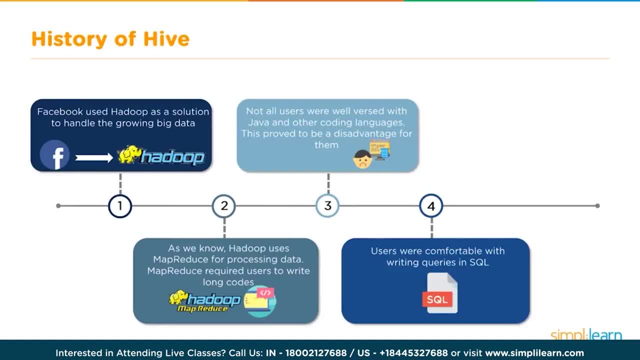 Users were comfortable with writing queries in SQL. SQL has been around for a long time, the standard SQL query language. Hive was developed with the vision to incorporate the concepts of data and the concepts of tables, columns, just like SQL. So why Hive? 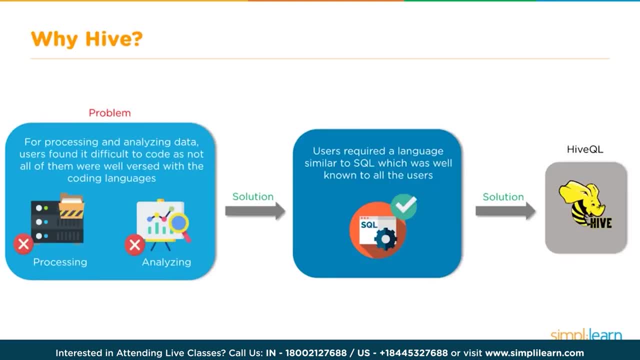 Well, the problem was for processing and analyzing data. users found it difficult to code, as not all of them were well versed with the coding languages. You have your processing, you have your analyzing, And so the solution was required: a language similar to SQL. 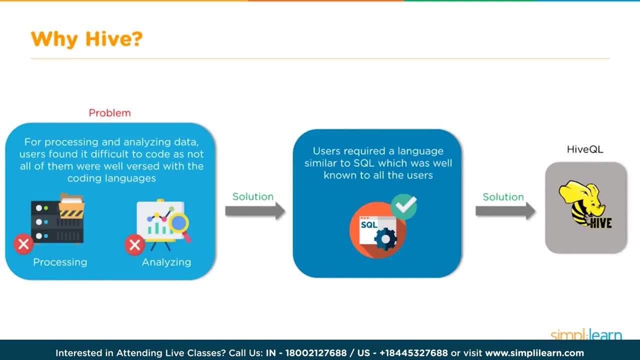 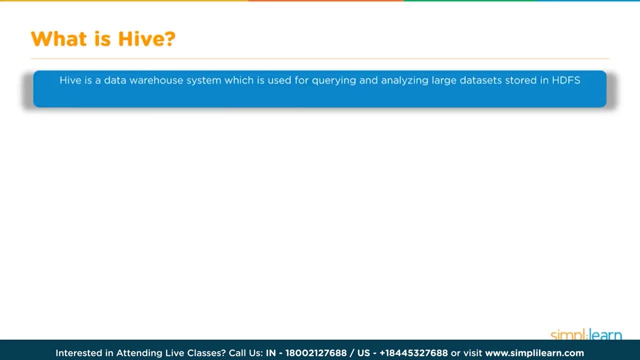 which was well known to all the users, And thus the Hive or HQL language evolved. What is Hive? Hive is a data warehouse system which is used for querying and analyzing data and analyzing large data sets stored in the HDFS or the Hadoop file system. 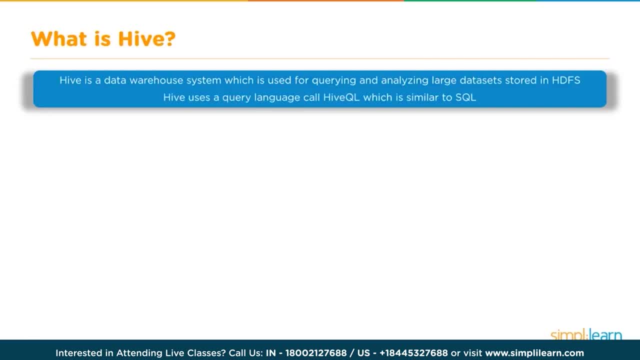 Hive uses a query language that we call HiveQL or HQL, which is similar to SQL. So if we take our user, the user sends out their Hive queries and then that is converted into a MapReduce tasks and then accesses the Hadoop MapReduce system. 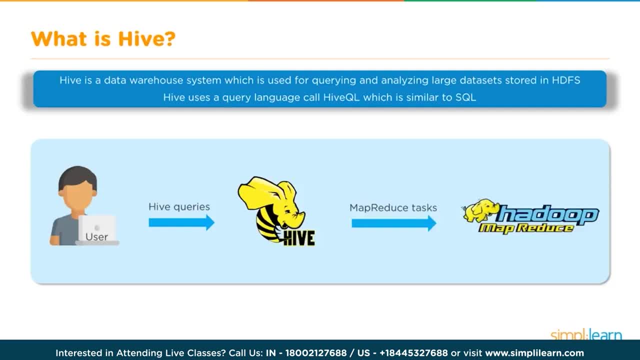 Let's take a look at the architecture of Hive. Architecture of Hive. We have the Hive client, So that could be the programmer, or maybe it's the manager who knows enough about the Hive. So let's take a look at the architecture of Hive. 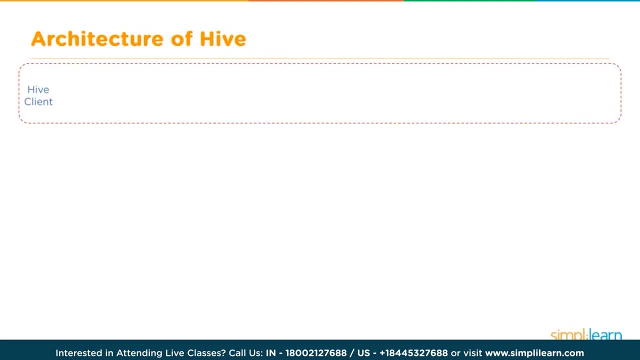 Architecture of Hive. We have the Hive client, So that could be the programmer, or maybe it's the manager who knows enough SQL to do a basic query to look up the data they need. The Hive client supports different types of client applications in different languages. 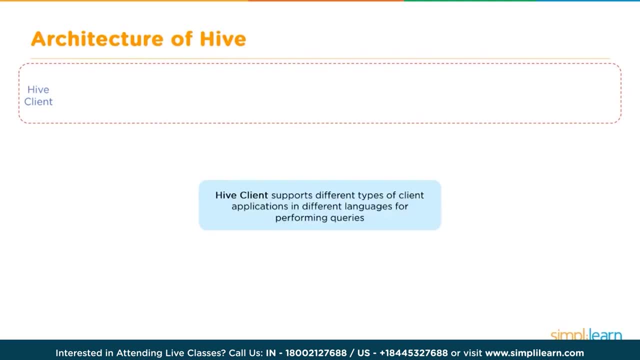 for performing queries, And so we have our Thrift application in the Hive Thrift client. Thrift is a software framework. Hive server is based on Thrift so it can serve the request from all programming language that support Thrift. And then we have our JDBC application. 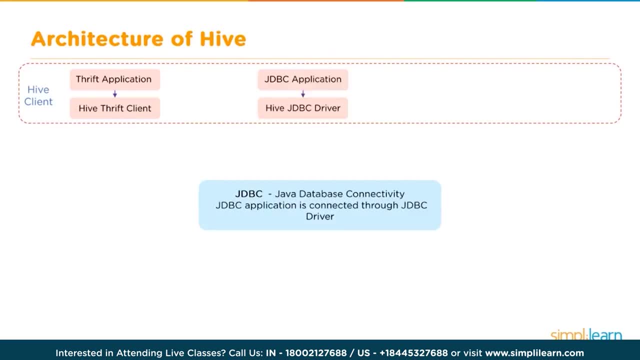 and the Hive JDBC driver. JDBC is a software framework that is based on Thrift, So it can serve the request from all programming language that support Thrift. And then we have the ODBC, Java Database Connectivity. JDBC application is connected through the JDBC driver. 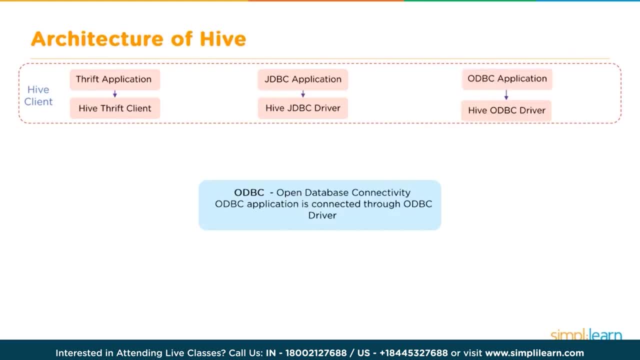 And then you have the ODBC application or the Hive ODBC driver, The ODBC or Open Database Connectivity. the ODBC application is connected through the ODBC driver. With the growing development of all of our different scripting languages- Python, C++, Spark, Java. 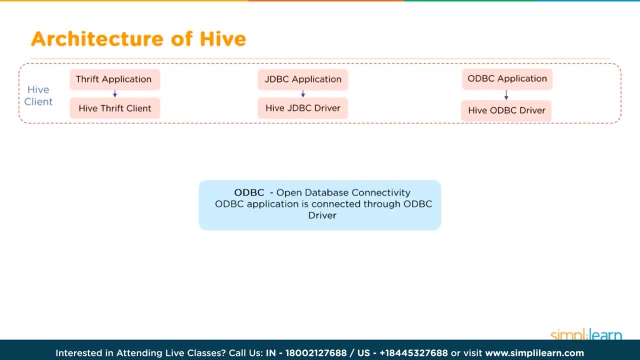 you can find just about any connection in any of the main scripting languages, And so we have our Hive services. As we look at deeper into the architecture, Hive supports various services, So you have your Hive server, basically your Thrift application or your Hive Thrift client. 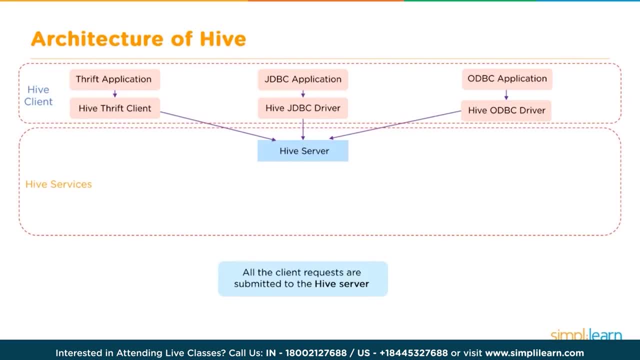 or your JDBC or your Hive JDBC driver, your ODBC application or your Hive ODBC driver. They all connect into the Hive server And you have your Hive web interface. You also have your CLI. Now the Hive web interface is a GUI is provided. 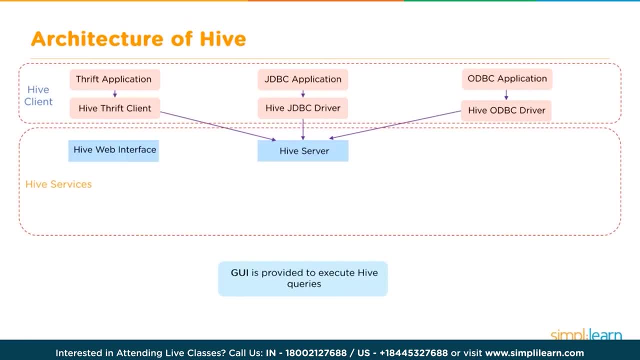 to execute Hive queries, And we'll actually be using that later on today. So you can see kind of what that looks like and get a feel for what that means. Commands are executed directly in CLI And then the CLI is a direct terminal window. 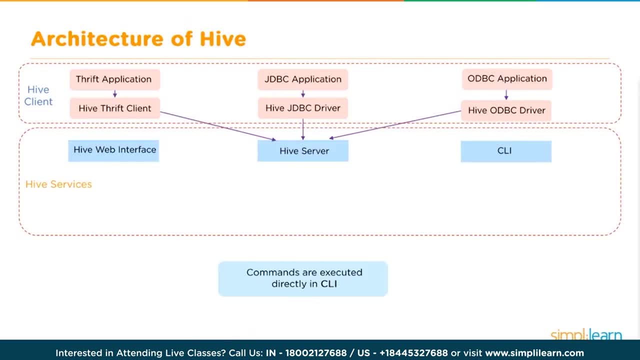 And I'll also show you that too, so you can see how those two different interfaces work. These then push the code into the Hive driver. Hive driver is responsible for all the queries submitted, So everything goes through that driver. Let's take a closer look. 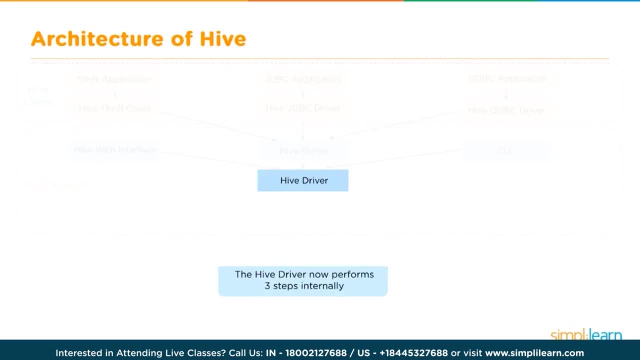 at the Hive driver. The Hive driver now performs three steps internally. One is a compiler. Hive driver passes query to compiler, where it is checked and analyzed. Then the optimizer kicks in and the optimized logical plan in the form of a graph of MapReduce. 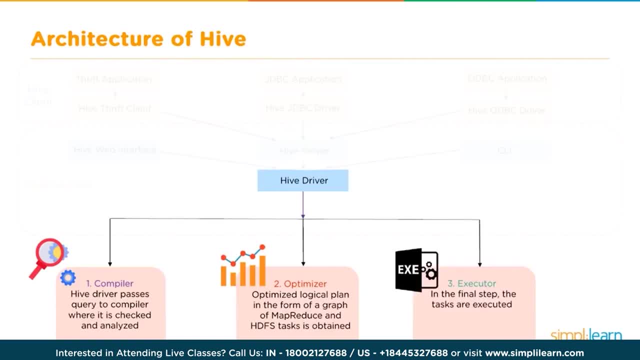 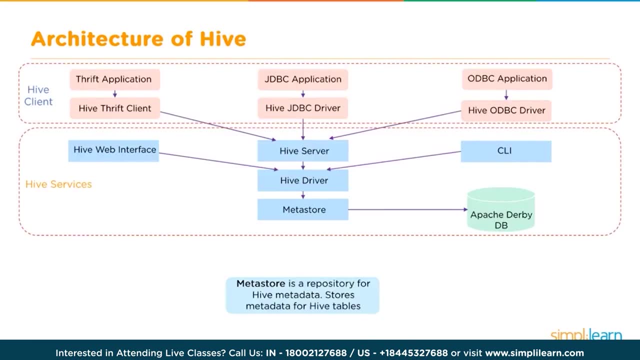 and HDFS tasks is obtained And then finally in the executor, in the final step, the tasks are executed. When we look at the architecture, we also have to note the metastore. Metastore is a repository for Hive metadata. It stores metadata for Hive tables. 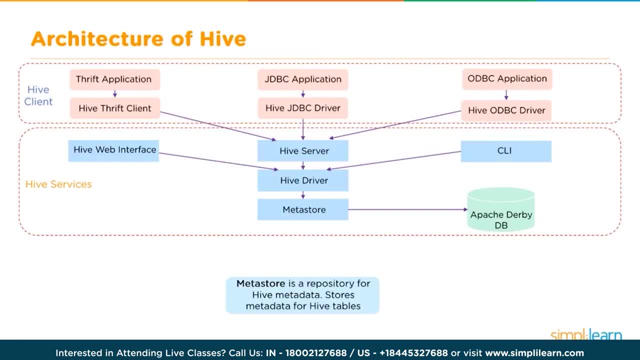 And you can think of this as your schema. and where is it located? And it's stored on the Apache, Derby DB. Processing and resource management is all handled by the MapReduce V1.. You'll see MapReduce V2, the Yarn and the Tez. 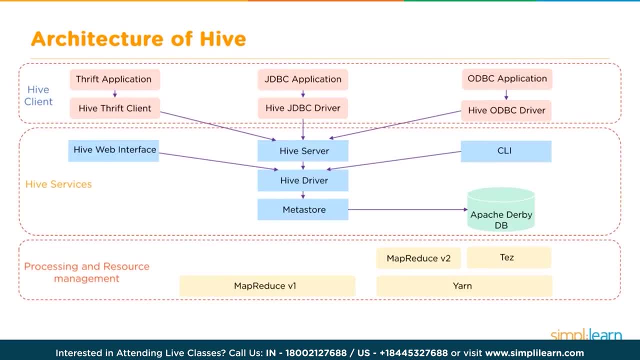 These are all different ways of managing these resources, depending on what version of Hadoop you're in. Hive uses MapReduce framework to process queries, And then we have our distributed storage, which is the HDFS, And if you looked at our Hadoop tutorials, 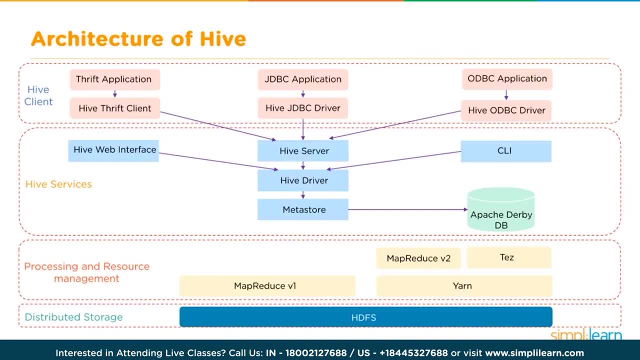 you'll know that these are on commodity machines and are linearly scalable. That means they're very easy and very affordable. A lot of time, when you're talking about big data, you're talking about a tenth of the price of storing it on enterprise computers. 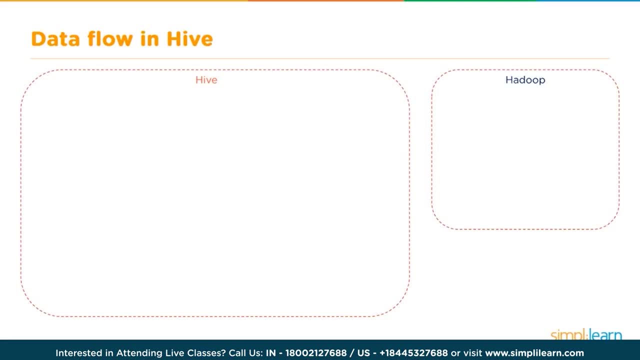 And then we look at the data flow in Hive. So in our data flow in Hive we have our Hive and the Hadoop system, And underneath the user interface or the UI, we have our driver, our compiler, our execution engine and our metastore. 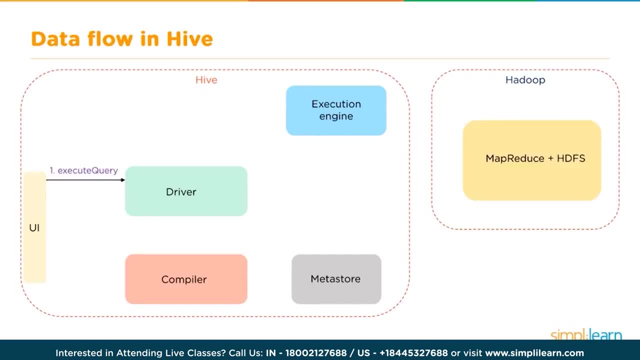 That all goes into the MapReduce and the Hadoop file system. So when we execute a query, you can see it coming in here. it goes into the driver. step one, Step two: we get a plan. What are we going to do? It refers to the query execution. 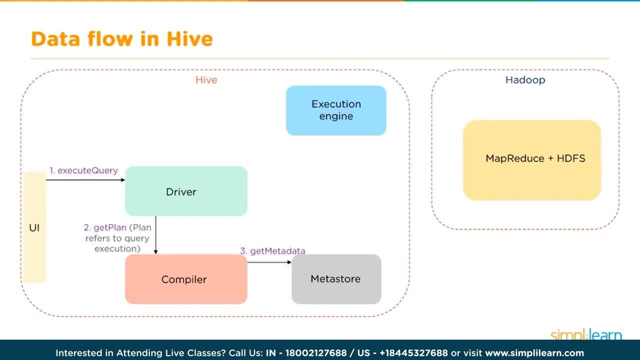 Then we go to the metadata. It's like, well, what kind of metadata are we actually looking at? Where is this data located? What is the schema on it? Then it comes back with the metadata into the compiler. Then the compiler takes all that information. 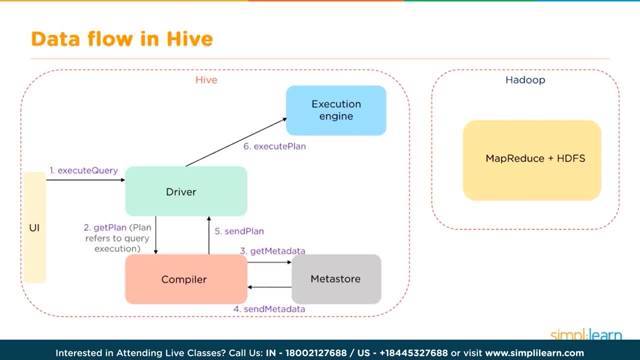 and the send plan returns it to the driver. The driver then sends the execute plan to the execution engine Once it's in the execution engine. the execution engine acts as a bridge between Hive and Hadoop to process the query And that's going into your MapReduce. 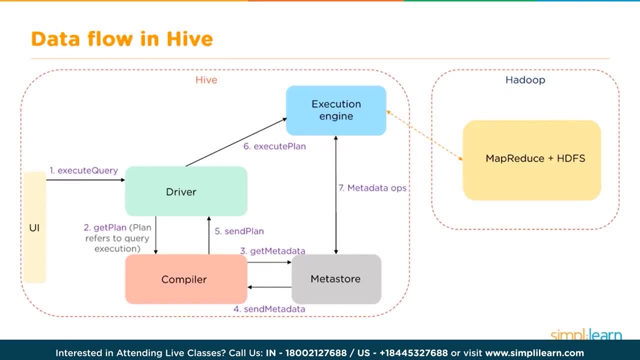 and your Hadoop file system or your HDFS, And then we come back with the metadata operations. It goes back into the metastore to update or let it know what's going on, Which also goes to the between. it's a communication between the execution engine and the metastore. 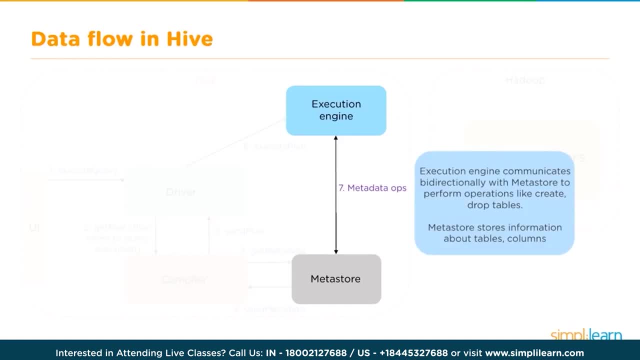 Execution engine communications is bidirectionally with the metastore to perform operations like create drop tables. Metastore stores information about tables and columns. So again, we're talking about the schema of your database And once we have that, we have a bidirectional. 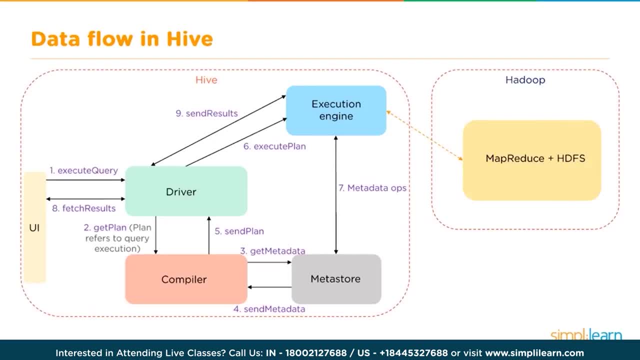 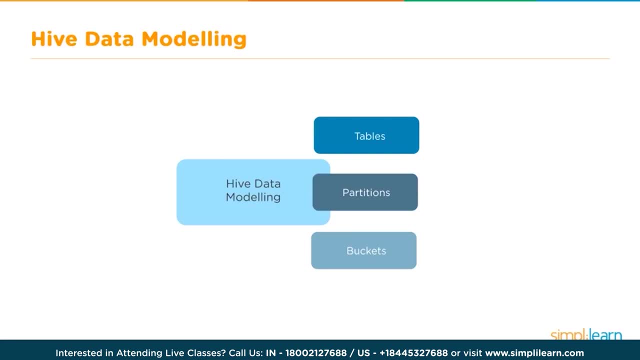 send results communication back into the driver And then we have the fetch results which goes back to the client. So let's take a little bit. look at the Hive data modeling. Hive data modeling. So you have your Hive data modeling, You have your tables. 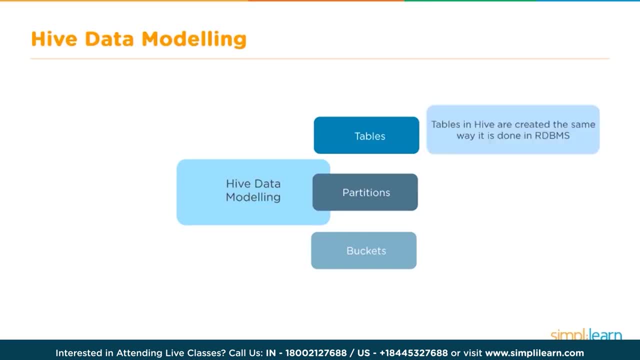 You have your partitions And you have buckets. The tables in Hive are created the same way it is done in RDBMS. So when you're looking at your original SQL Server or MySQL Server, where you might have enterprise equipment and a lot of people pulling and moving stuff off of there, 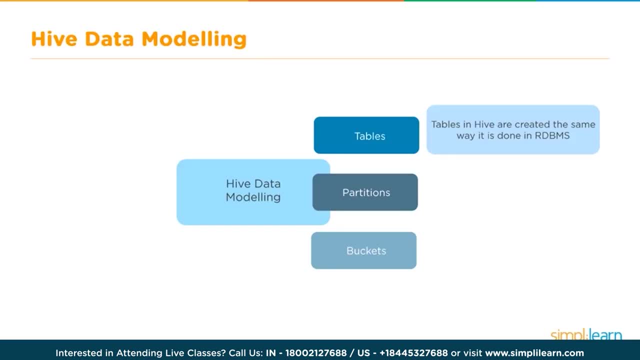 The tables are going to look very similar And this makes it very easy to take that information. and let's say you need to keep current information but you need to store all of your years of transactions back into the Hadoop Hive So you match those. 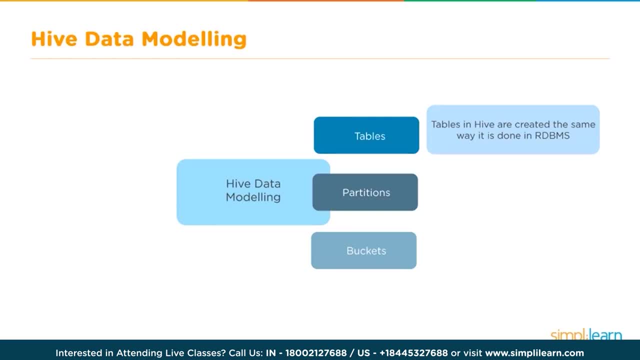 Those all kind of look the same, The tables are the same, Your databases look very similar And you can easily import them back And store them into the Hive system Partitions. Here tables are organized into partitions for grouping same type of data. 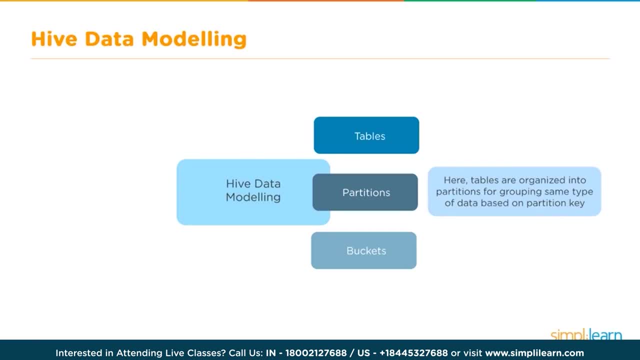 based on partition key. This can become very important for speeding up the process of doing queries. So if you're looking at dates as far as like your employment dates of employees, if that's what you're tracking, You might add a partition there, because that might be one of the key things. 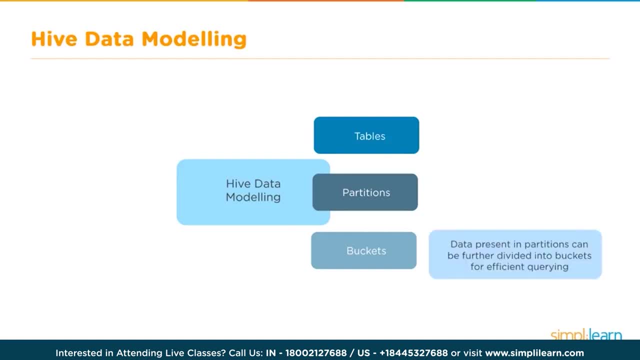 that you're always looking up as far as employees are concerned. And finally, we have buckets. Data present in partitions can be further divided into buckets for efficient querying. Again, there's that efficiency At this level. a lot of times you're working with the programmer. 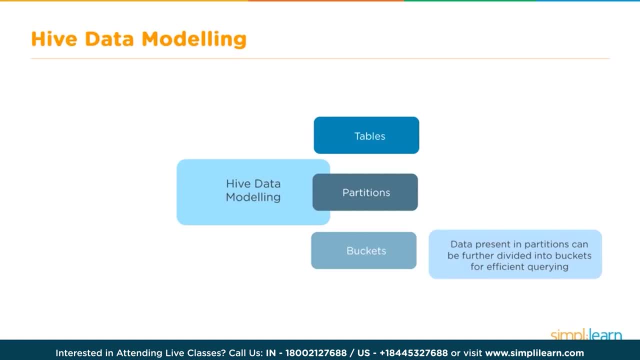 and the admin of your Hadoop file system to maximize the efficiency of that file system. So it's usually a two person job and we're talking about Hive data modeling. You want to make sure that they work together and you're maximizing your resources. 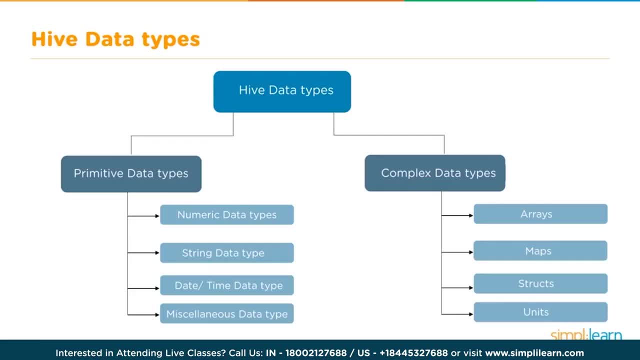 Hive data types. So we're talking about Hive data types. We have our primitive data types And our complex data types. A lot of this will look familiar because it mirrors a lot of stuff in SQL. In our primitive data types we have the numerical data types. 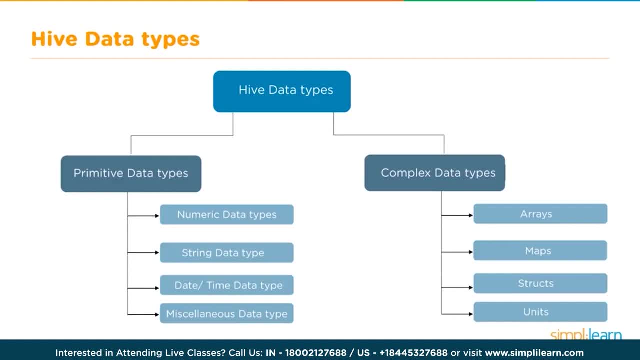 String data type, Date time data type And miscellaneous data type, And these should be very. they're kind of self explanatory. but just in case, Numerical data is your floats, your integers, your short integers- All of that numerical data comes in as a number. 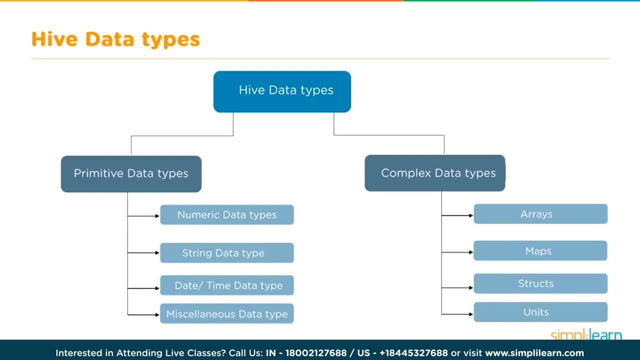 A string, of course, is characters and numbers, And then you have your date time stamp, And then we have kind of a general way of pulling your own created data types in there. That's your miscellaneous data type, And we have complex data types. 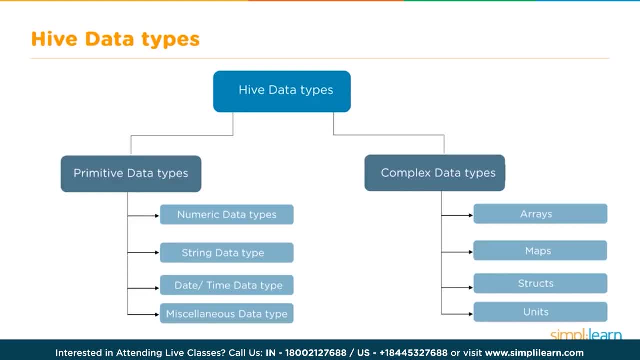 So you can store arrays, You can store maps, You can store structures And even units in there, As we dig into Hive data types and we have the primitive data types and the complex data types. So we look at primitive data types and we're looking at numeric data types. 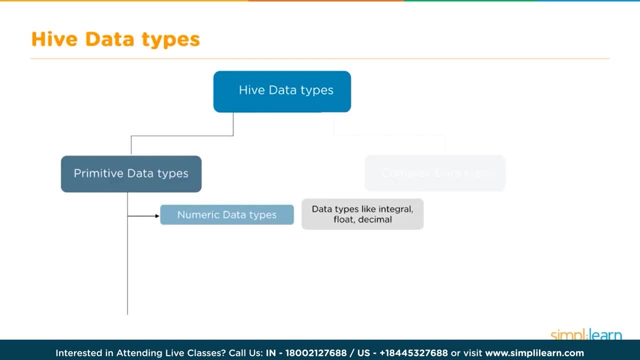 Data types like an integer, a float, a decimal. Those are all stored as numbers in the Hive data system. A string data type Data types like characters and strings. You store the name of the person you're working with. You know John Doe. the city, Memphis. 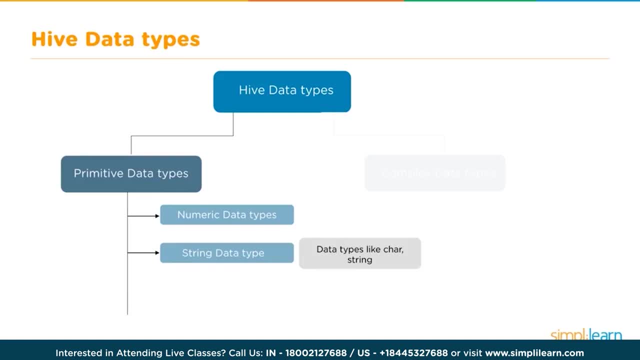 the state Tennessee, Maybe it's Boulder, Colorado, USA, Or maybe it's Hyperbad India. That's all going to be string. It's stored as a string character And, of course, we have our date time data type, Data types like time stamp, date interval. 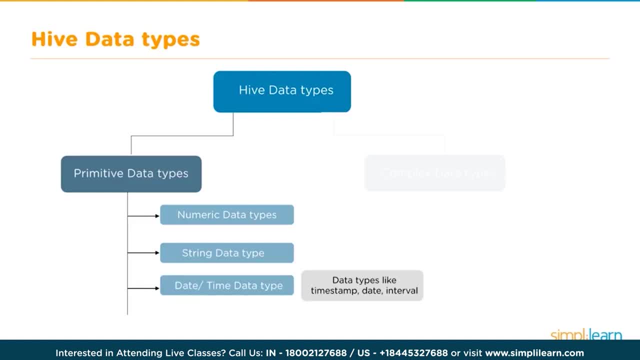 Those are very common as far as tracking sales, Anything like that, So you can just think if you can type a stamp of time on it. Or maybe you're dealing with a race and you want to know the interval. How long did the person take to complete? 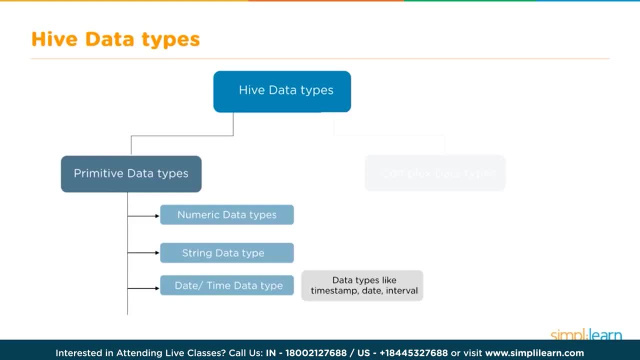 whatever task it was. All of that is date, time data type, And then we talk miscellaneous data type. These are like boolean and binary, And when you get into boolean and binary you can actually almost create anything in there. Put your yes- no's. 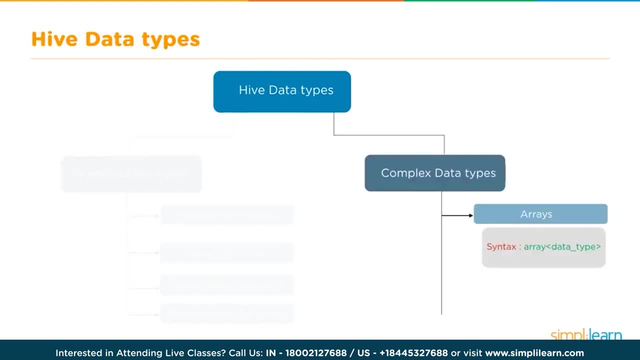 Zero one. Now let's take a look at complex data types a little closer. We have arrays, So your syntax is of data type and it's an array, And you can just think of an array as a collection of same entities: One, two, three, four. 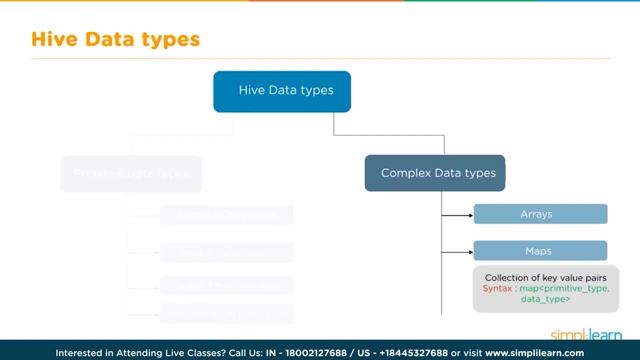 If they're all numbers, Then you have maps. This is a collection of key value pairs. So understanding maps is so central to Hadoop. So when we store maps you have a key, which is a set. You can only have one key per mapped value. 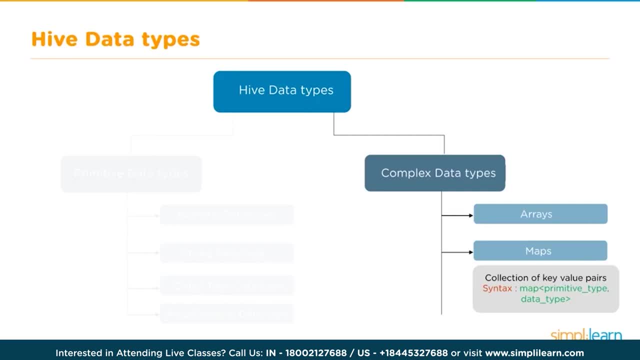 And so in Hadoop, of course you collect the same keys and you can add them all up or do something with all the contents of the same key. But this is our map as a primitive type, data type And our collection of key value pairs. 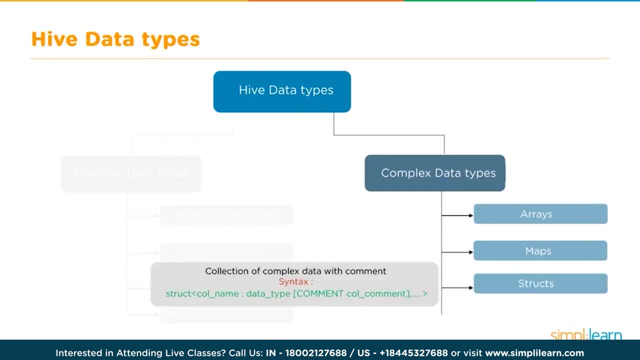 And then collection of complex data with comment, So we can have a structure where you have column name, data type, comment, column comment. So you can get very complicated structures in here with your collection of data and your comment and setup. And then we have units. 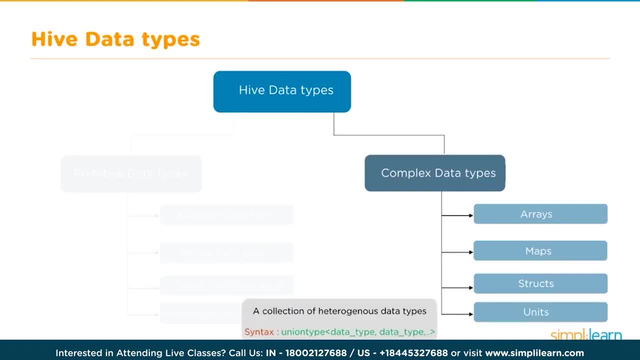 And this is a collection of heterogeneous data types. So the syntax for this is union type, data type, data type and so on. So it's all going to be the same, A little bit different than the arrays, where you can actually mix and match. 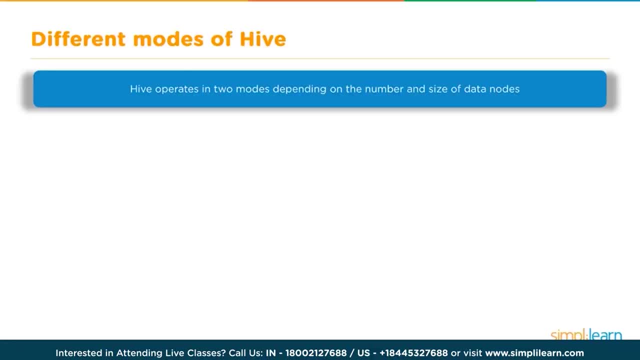 Different modes of Hive. Hive operates in two modes depending on the number and size of data nodes. We have our local mode and our map reduce mode. When we talk about the local mode, it is used when Hadoop is having one data node and the data is small. 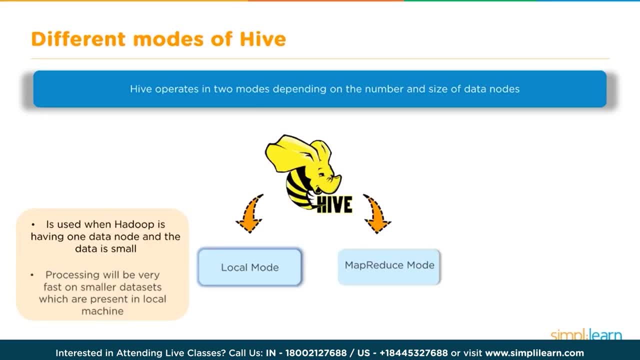 Processing will be very fast on the smaller data sets which are present in local machine. And this might be that you have a local file of stuff you're uploading into the Hive and you need to do some processes in there. you can go ahead and run those Hive processes. 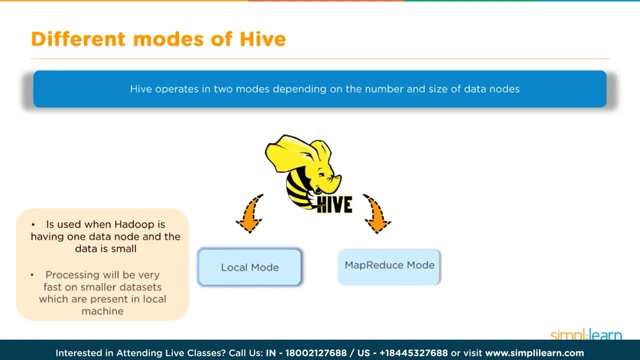 and queries on it. Usually you don't see much in the way of a single node Hadoop system. If you're going to do that, you might as well just use like an SQL database or even a Java SQLite or something. Python is SQLite. 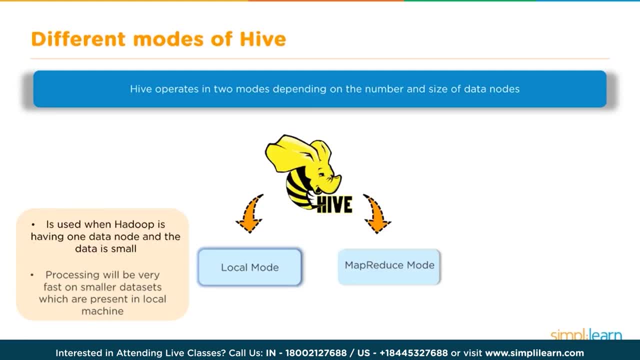 So you don't really see a lot of single node Hadoop databases. But you do see the local mode in Hive where you're working with a small amount of data that's going to be integrated into the larger database, And then we have the map reduce mode. 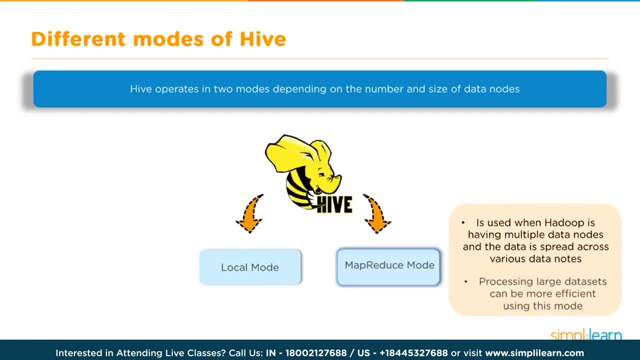 This is used when Hadoop is having multiple data nodes and the data is spread across various data nodes. Processing large data sets can be more efficient using this mode, And this you can think of, instead of it being one, two, three or even five computers. 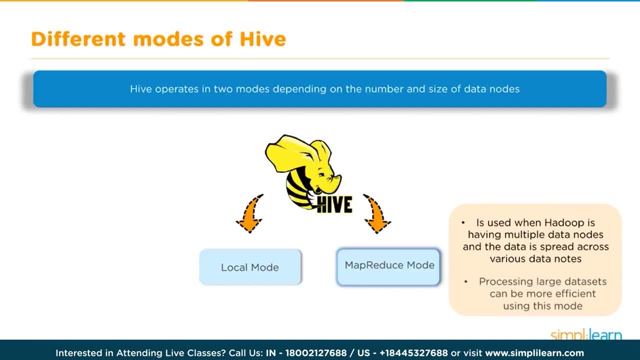 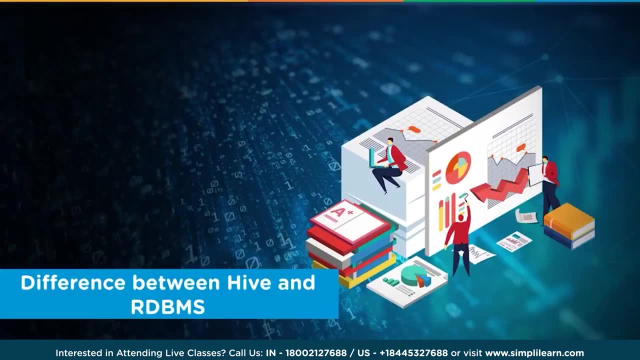 we're usually talking with the Hadoop file system. we're looking at ten computers, Fifteen, a hundred, where this data is spread across all those different Hadoop nodes. Difference between Hive and RDBMS: Remember, RDBMS stands for the Relational Database Management System. 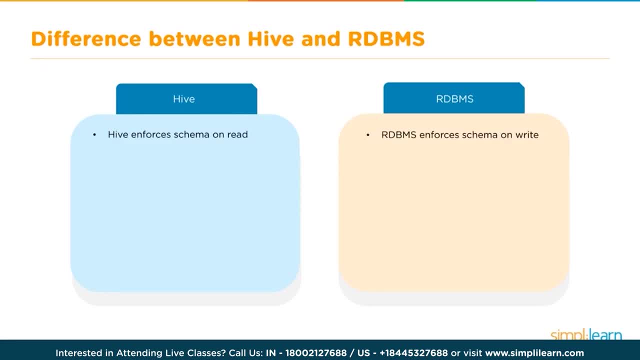 Let's take a look at the difference between Hive and the RDBMS. With Hive, Hive enforces schema on read And it's very important that whatever is coming in, that's when Hive is looking at it and making sure that it fits the model. 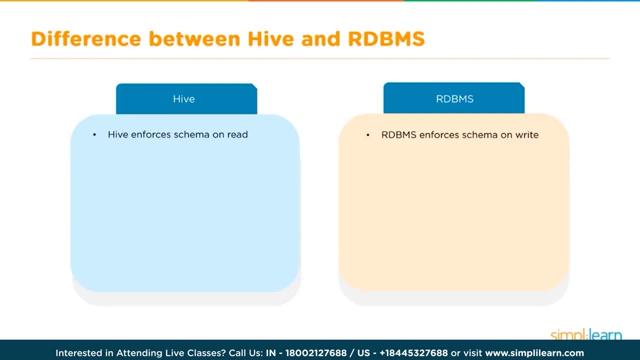 The RDBMS enforces a schema when it actually writes the data into the database. So it's read the data and then, once it starts to write it, that's where it's going to give you the error or tell you something is incorrect about your scheme. 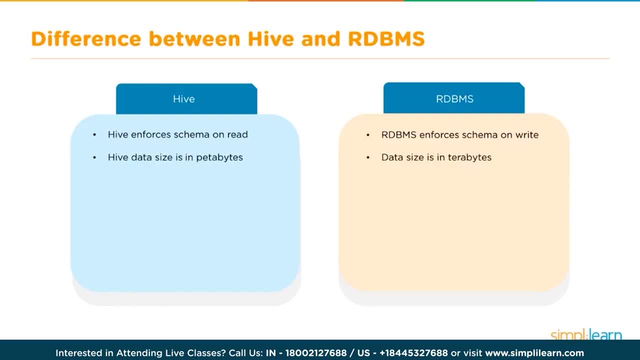 Hive. data size is in petabytes. That is hard to imagine. When we're looking at your personal computer on your desk, maybe you have ten terabytes. if it's a high-end computer, We're talking petabytes, So that's hundreds of computers grouped together. 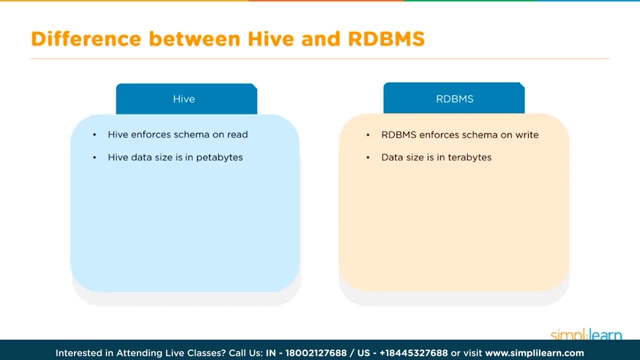 With RDBMS, data size is in terabytes. Very rarely do you see an RDBMS system that's spread over more than five computers, And there's a lot of reasons for that. With the RDBMS, it actually has a high-end amount of writes to the hard drive. 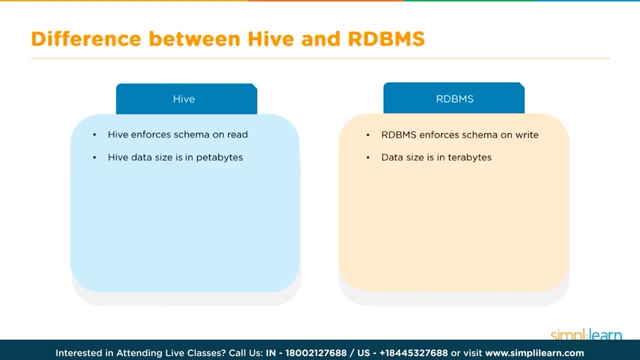 There's a lot more going on there. You're writing and pulling stuff, So you really don't want to get too big with an RDBMS and you're going to have a lot of problems With Hive. you can take it as big as you want. 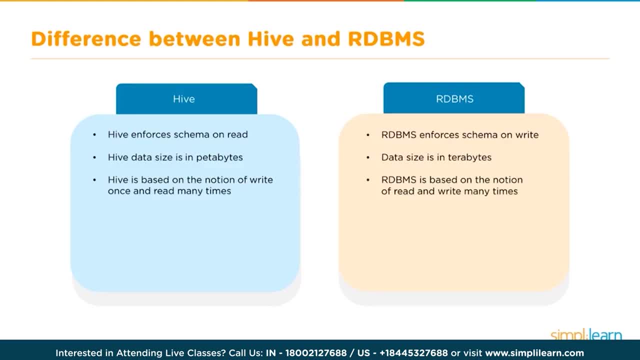 Hive is based on the notion of write once and read many times. This is so important. They call it WRM, which is write W once O read R many times M They refer to it as WRM, and that's true. 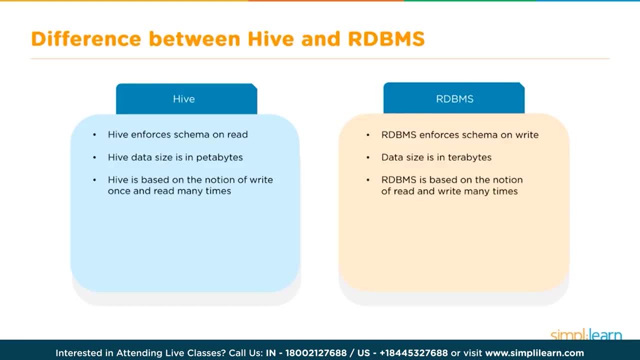 of a lot of your Hadoop setup. It's altered a little bit but in general we're looking at archiving data that you want to do data analysis on. We're looking at pulling all of that stuff off your RDBMS from years and years. 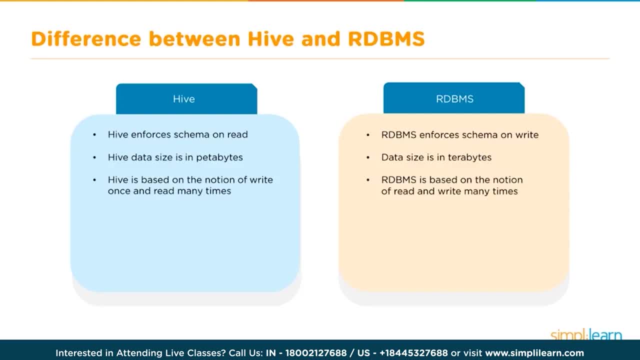 of business or whatever your company does, or scientific research, and putting that into a huge data pool so that you can now do queries on it and get that information out of it. With the RDBMS, it's based on the notion of read and write. many times 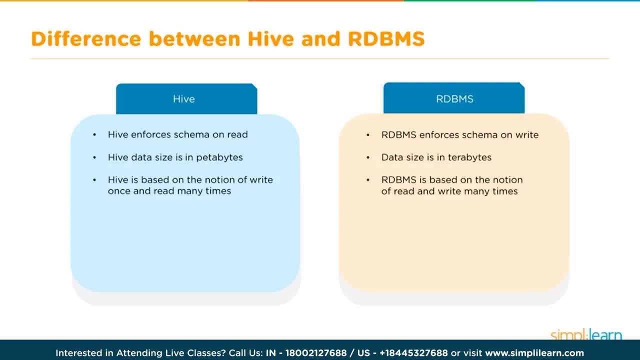 So you're continually updating this database. You're continually bringing up new stuff, new sales. the account changes because they have a different licensing now, whatever software you're selling all that kind of stuff where the data is continually fluctuating, And then Hive resembles a traditional database. 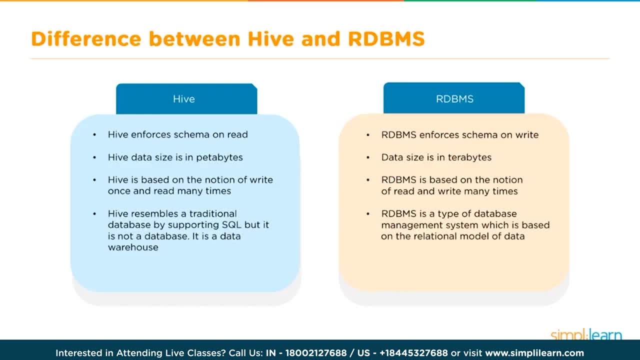 supporting SQL. but it is not a database, It is a data warehouse. This is very important and it goes with all the other stuff we've talked about, that we're not looking at a database but a data warehouse to store the data and still have fast and easy access. 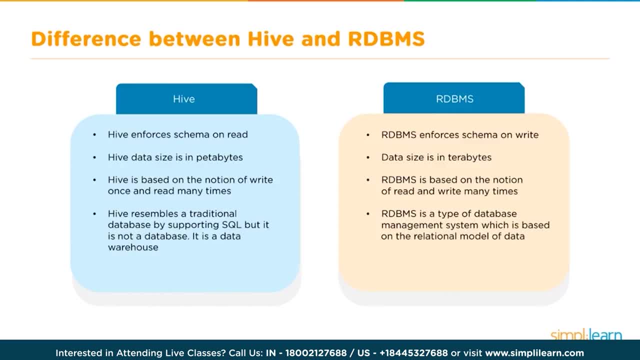 to it for doing queries. You can think of Twitter and Facebook. They have so many posts that are archived back historically. Those posts aren't going to change. They made the post, they're posted, they're there and they're in their database. 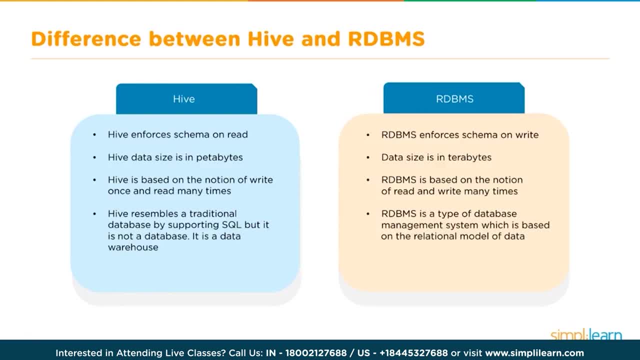 but they have to store it in a warehouse. They want to pull it back up With the RDBMS. it's a type of database management system which is based on the relational model of data And then, with Hive, easily scalable at a low cost. 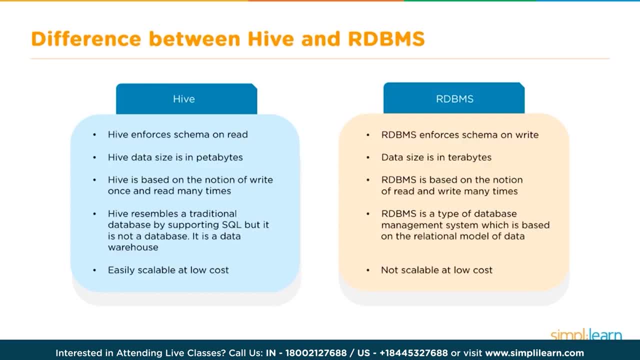 Again, we're talking maybe $1,000 per terabyte. The RDBMS is not scalable at a low cost. When you first start on the lower end, you're talking about 10,000 per terabyte of data, including all the backup on the models. 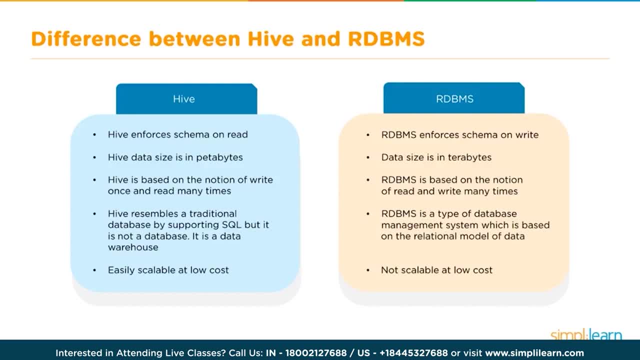 and all the added necessities to support it. As you scale it up, you have to scale those computers and hardware up, So you might start off with a basic server and then you upgrade to a Sun computer to run it And you spend tens of thousands of dollars. 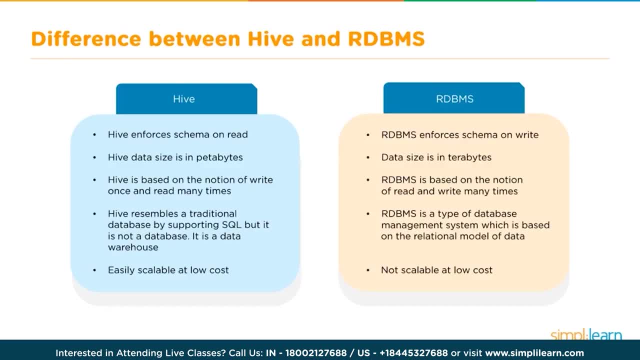 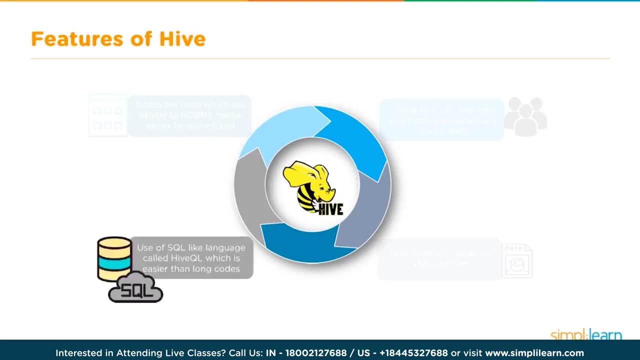 for that hardware upgrade. With Hive, you just put another computer into your Hadoop file system. So let's look at some of the features of Hive. When we're looking at the features of Hive, we're talking about the use of SQL-like language. 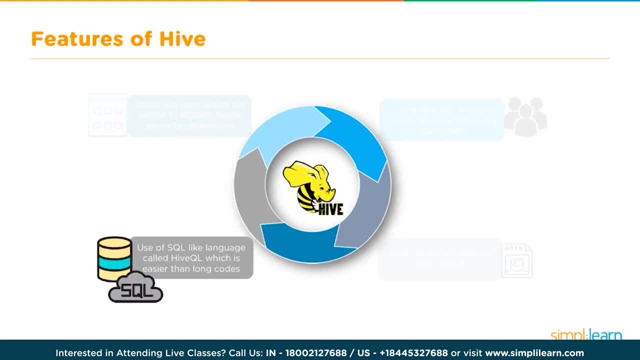 called HiveQL. A lot of times you'll see that as HQL, which is easier than long codes. This is nice if you're working with your shareholders. You come to them and you say, hey, you can do a basic SQL query on here. 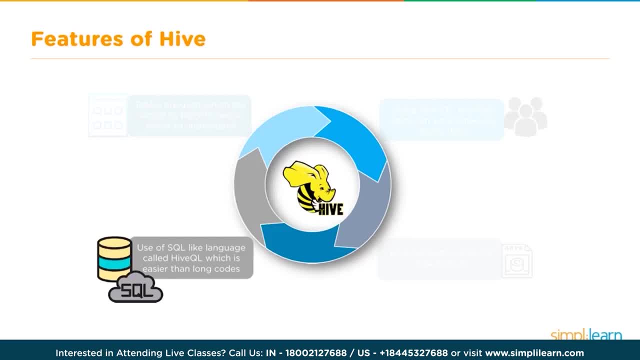 and pull up the information you need. This way you don't have to have your programmers jump in every time they want to look up something in the database. They actually now can easily do that if they're not skilled in programming and script writing. 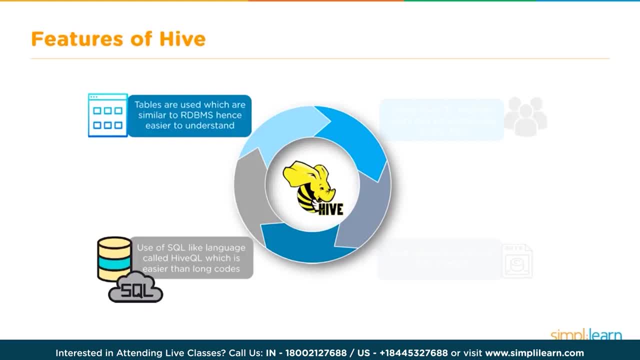 Tables are used which are similar to the RDBMS, hence easier to understand, And one of the things I like about this is when I'm bringing tables in from a MySQL server or SQL server. there's almost a direct reflection between the two. 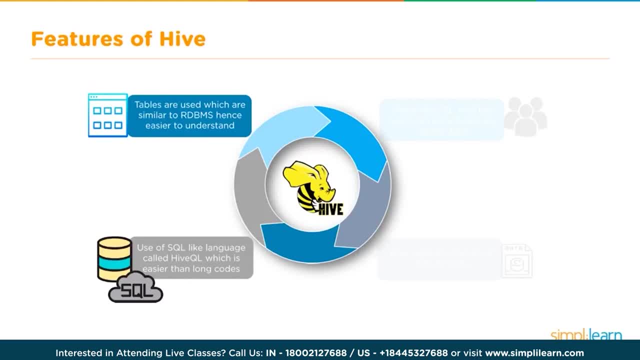 So when you're looking at one which is the data which is continually changing, and then you're going into the archive database, it's not this huge jump where you have to learn a whole new language. You mirror that same schema into the HDFS. 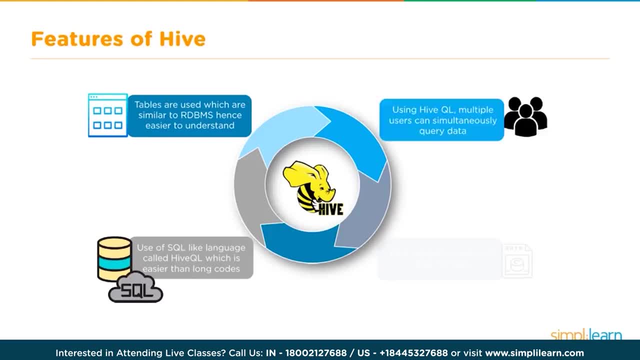 into the Hive, making it very easy to go between the two, And then, using HiveQL, multiple users can simultaneously query data. So again, you can have multiple clients in there and they send in their query. That's also true with the RDBMS. 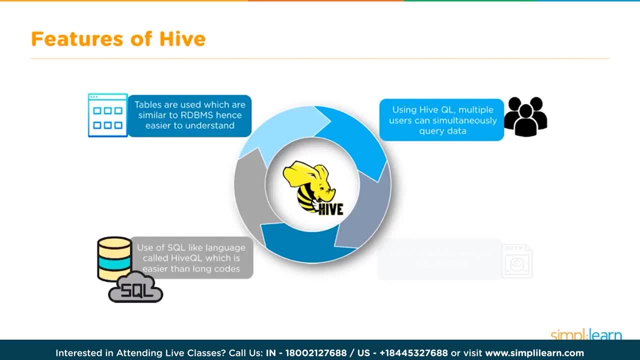 which kind of queues them up because it's running so fast you don't notice the lag time. Well, you get that also with the HQL. As you add more computers in the query can go very quickly, depending on how many computers and how much resources each machine has. 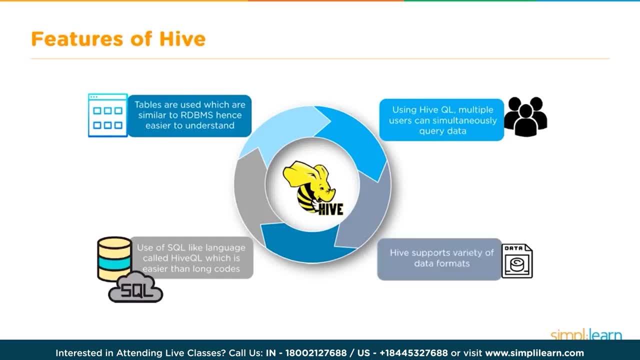 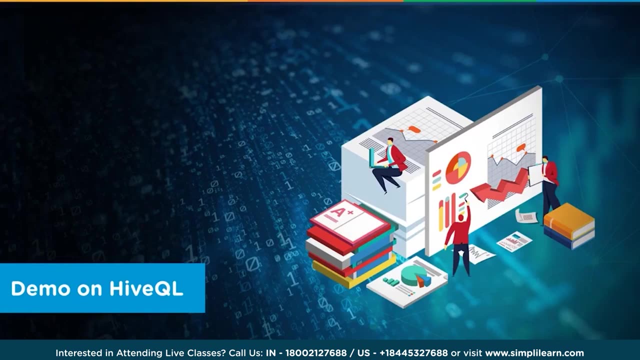 to pull the information, And Hive supports a variety of data types. So with Hive it's designed to be on the Hadoop system, which you can put almost anything into the Hadoop file system. So with all that, let's take a look at a demo on HiveQL or HQL. 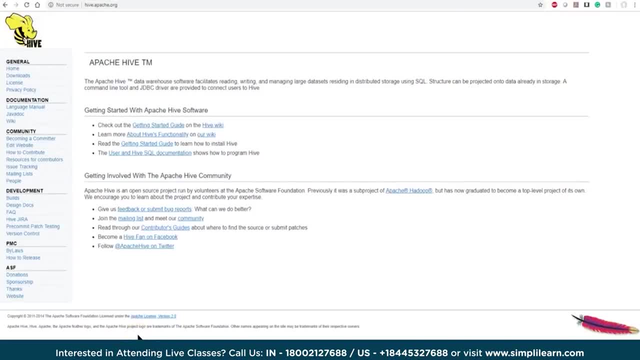 Before I dive into this, let's take a look at the hands-on demo. Let's take a look at the website hiveapacheorg. That's the main website, since Apache- It's an Apache open source software. This is the main software or the main site for the build. 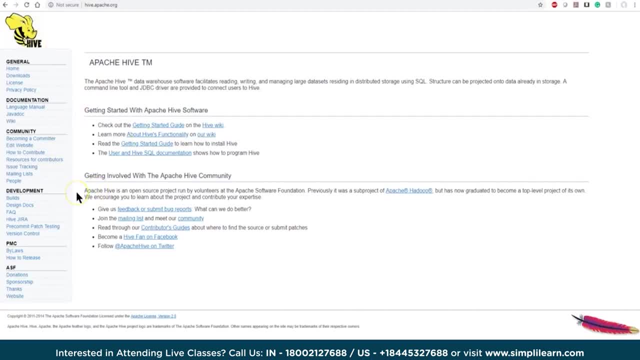 And if you go in here you'll see that they're slowly migrating Hive into Beehive. And so if you see Beehive versus Hive, note that Beehive is the new releases coming out. That's all it is. It reflects a lot of the same functionality of Hive. 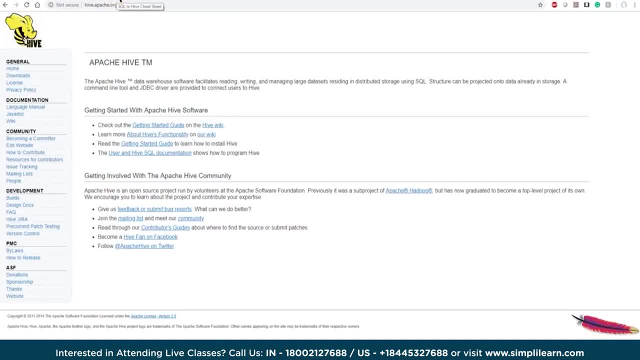 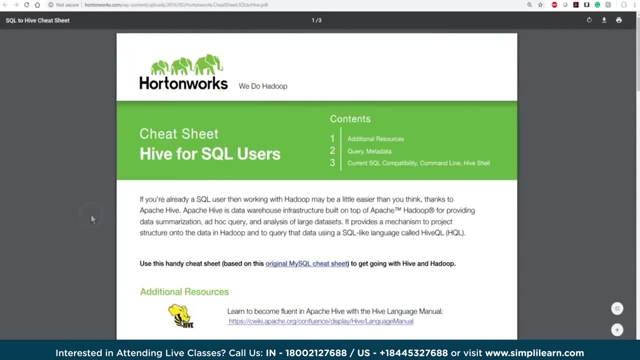 It's the same thing. And then we like to pull up this kind of documentation on commands, And for this I'm actually going to go to Hortonworks Hive cheat sheet, And that's because Hortonworks and Cloudera are two of the most common used builds for Hadoop. 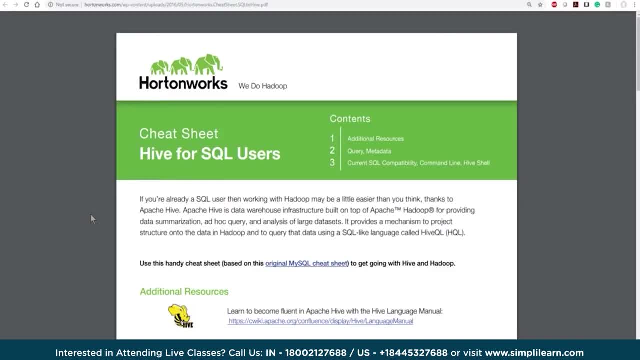 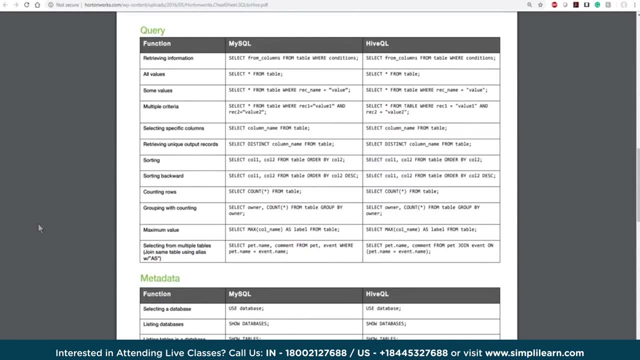 and for which include Hive and all the different tools in there, And so Hortonworks has a pretty good PDF. you can download cheat sheet on there. I believe Cloudera does too, But we'll go ahead and just look at the Horton one, because it's the one that comes up really good. 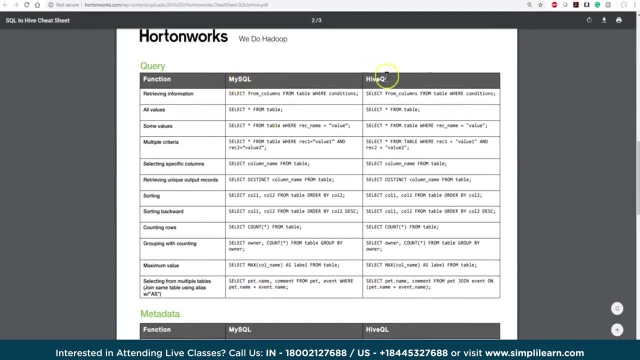 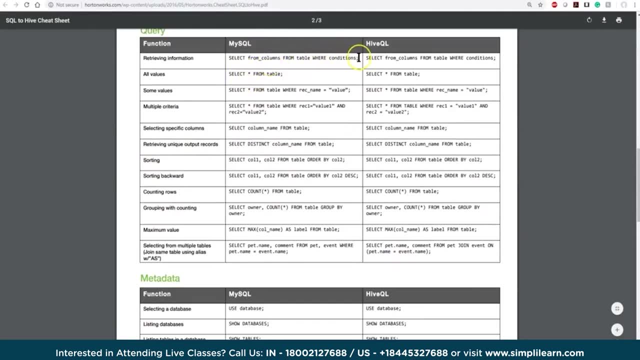 And you can see when we look at the query language it compares MySQL Server to HiveQL or HQL And you can see the basic select. We select from columns, from table where conditions exist. You know most basic command on there And they have different things you can do with it. 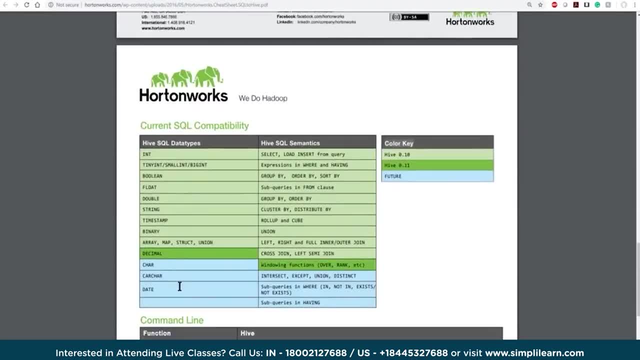 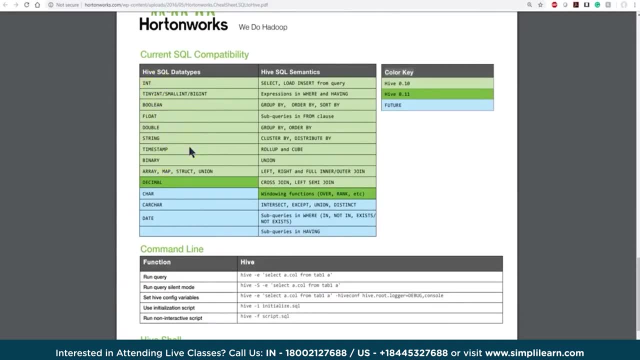 just like you do with your SQL, And if you scroll down you'll see data types. So here's your integer, your flow, your binary double string timestamp and all the different data types. you can use Some different semantics, different keys, features, functions. 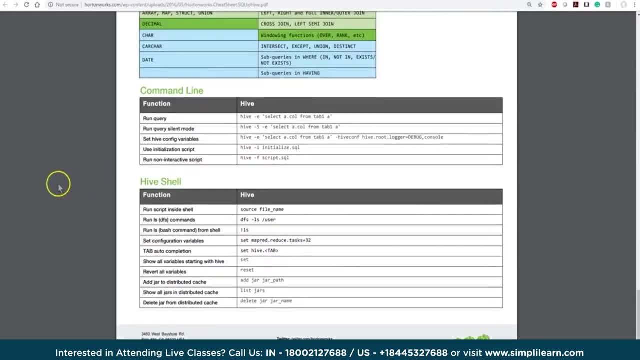 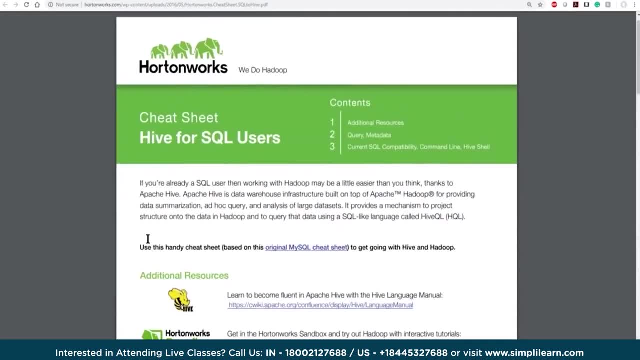 for running a Hive query command line setup and of course the Hive shell setup in here. So you can see right here, if we loop through it, it has a lot of your basic stuff in it. We're basically looking at SQL across a Horton database. 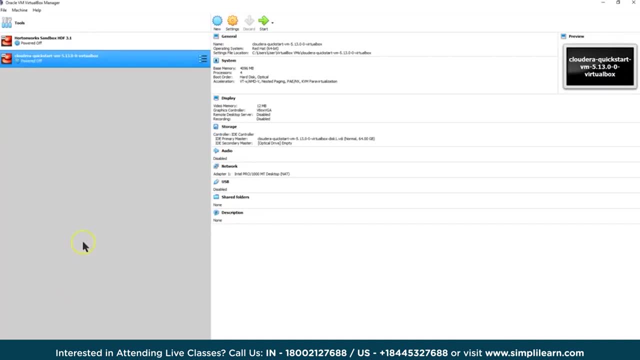 We're going to go ahead and run our Hadoop cluster Hive demo And I'm going to go ahead and use the Cloudera quick start And this is in the virtual box. So again, we have an Oracle virtual box which is open source. 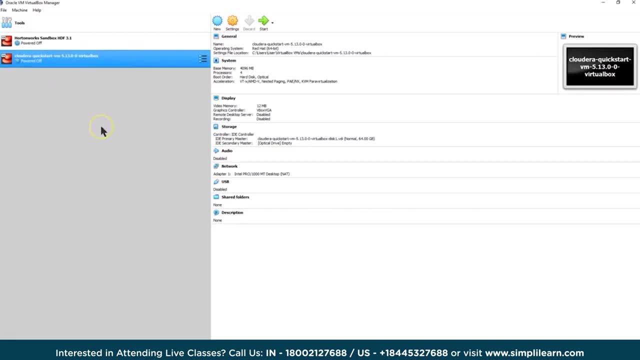 And then we have our Cloudera, And then we have our Cloudera quick start, which is the Hadoop setup on a single node. Now, obviously, Hadoop and Hive are designed to run across a cluster of computers, So when we talk about a single node, 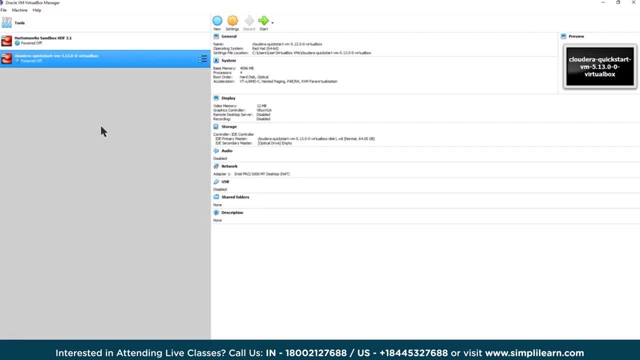 it's for education, testing, that kind of thing, And if you have a chance you can always go back and look at our demo we had on setting up a Hadoop system in a single cluster. Just set a note down below in the YouTube video. 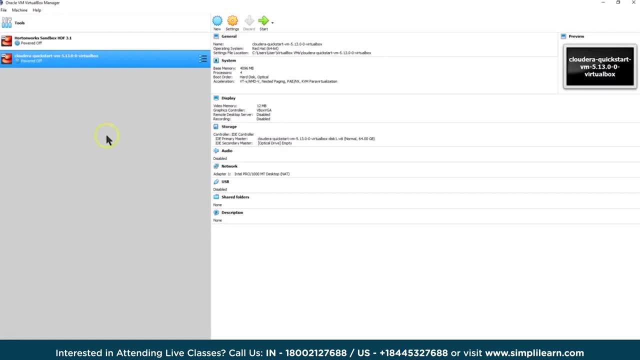 And our team will get in contact with you and send you that link if you don't already have it, Or you can contact us at the wwwscanadacom Now in here. it's always important to note that you do need on your computer. 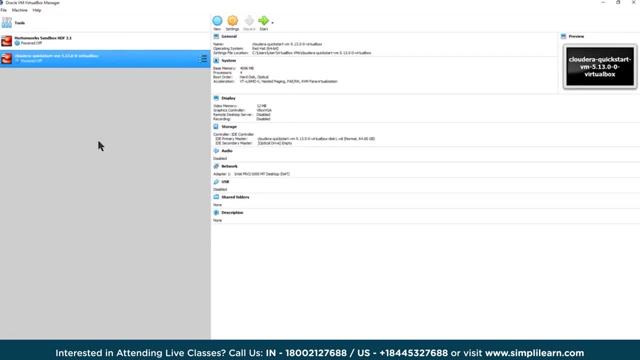 if you're running on Windows- because I'm on a Windows machine- you're going to need probably about 12 gigabytes to actually run this. It used to be. you could buy with a lot less, but as things have evolved they take up more and more resources. 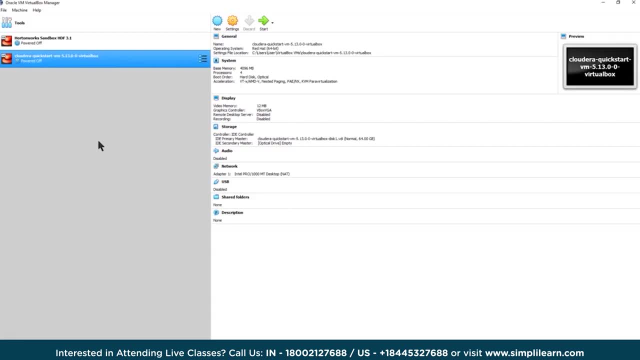 And you need the professional version If you have the home version. I was able to get that to run, but boy did it take a lot of extra work to get the home version to. let me use the virtual setup on there And we'll simply click on the Cloudera Quick Start. 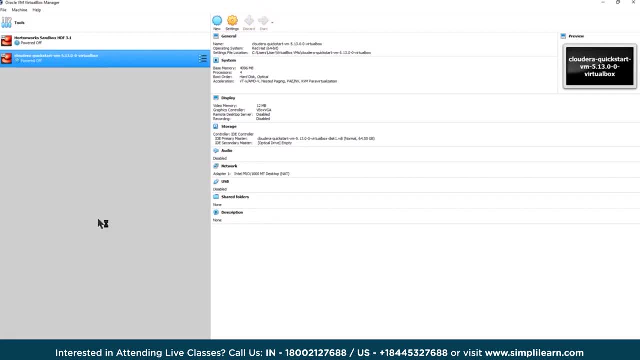 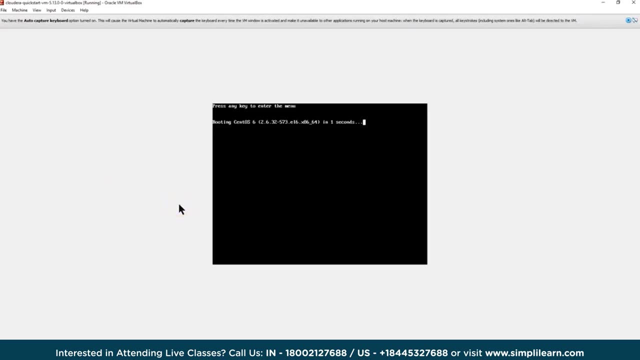 and I'm going to go ahead and just start that up, And this is starting up our Linux. So we have our Windows 10,, which is the computer I'm on, and then I have the VirtualBox, which is going to have a Linux operating system in it. 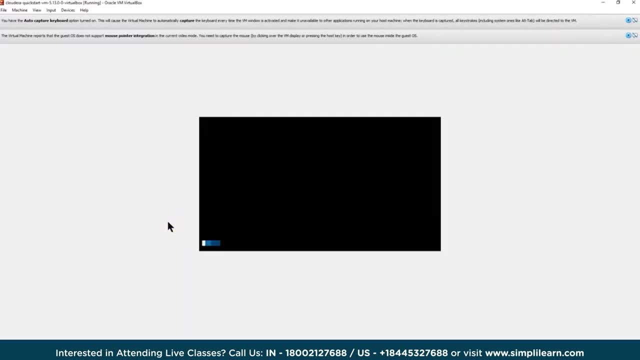 And we'll skip ahead, so you don't have to watch the whole install. Something interesting to know about the Cloudera is that it's running on Linux CentOS and, for whatever reason, I've always had to click on it and hit the Escape button for it to spin up. 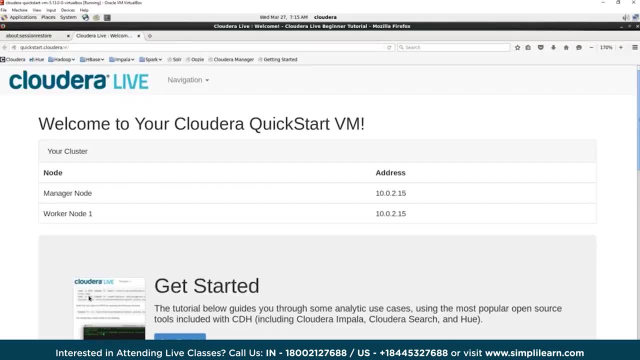 And then you'll see the DOS coming up. Now that our Cloudera is spun up on our virtual machine with the Linux on, we can see here we have our. it uses the Thunderbird browser on here by default and automatically opens up. 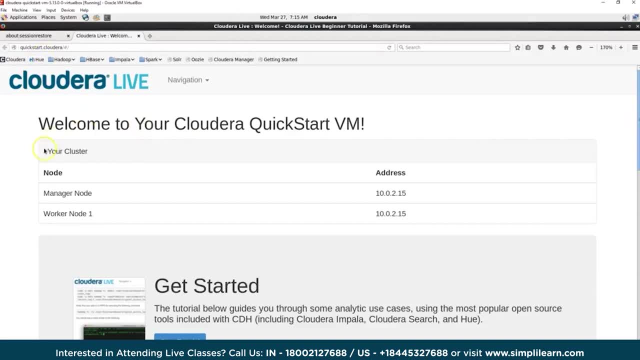 a number of different tabs for us. And a quick note, because I mentioned the restrictions on getting setup on your own computer. if you have a home edition computer and you're worried about setting it up on there, you can also go in there and spin up a one month free service. 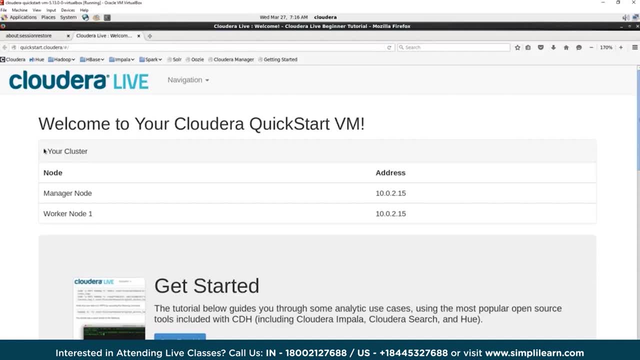 on Amazon Web Service to play with this. So there's other options. You're not stuck with just doing it on the quick start menu. You can spin this up in many other ways. Now, the first thing we want to note is that we've come in here into Cloudera. 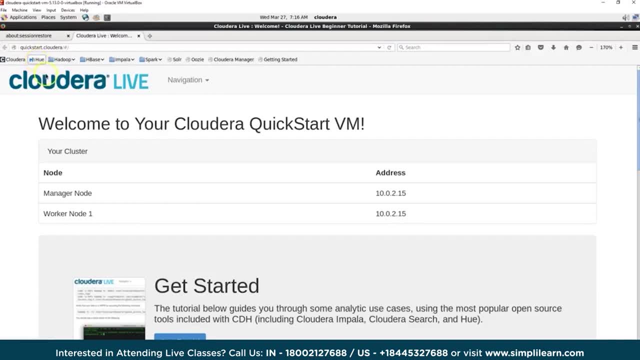 and I'm going to access this in two ways. The first one is we're going to use Hue And I'm going to open up Hue and it'll take it a moment to load from the setup on here And Hue is nice. 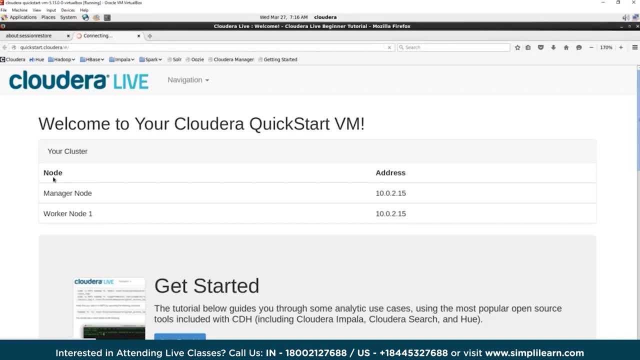 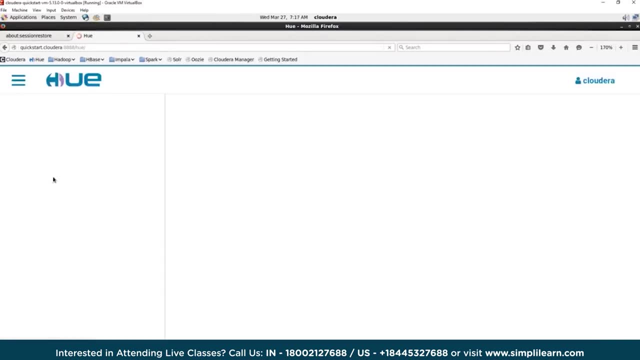 if I go in and use Hue as an editor into Hive or into the Hadoop setup, usually I'm doing it as a from an admin side: a lot more information, a lot of visuals, less to do with actually diving in there and just executing code. 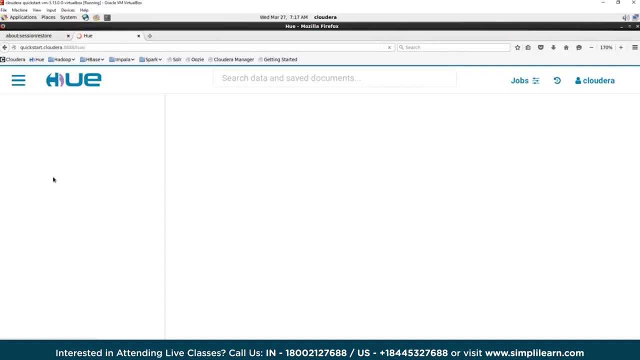 And you can also write this code into files and scripts and there's other things you can other ways. you can upload it into Hive, But today we're going to look at the command lines and we'll upload it into Hue and then we'll go into and actually do our work. 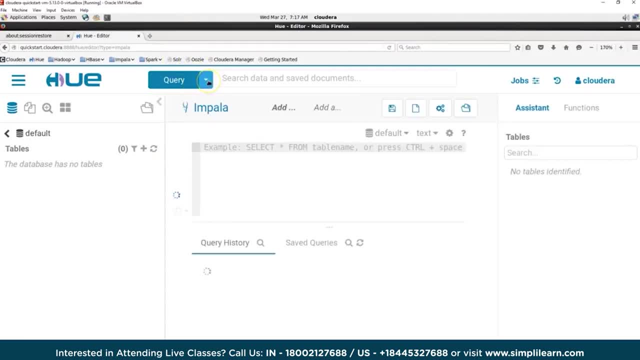 in a terminal window under the Hive shell. Now in the Hue browser window, if you go under query and click on the pull down menu and then you go under editor, click on Hive and this will open up our query down here and now it has a nice little B that shows our Hive going. 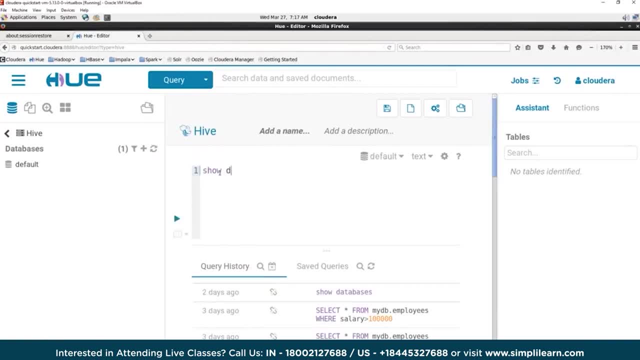 and we can go something very simple down here like show databases, And we follow it with a semi-colon, And that's the standard in Hive is. you always add our punctuation at the end there And I'll go ahead and run this and the query will show up underneath. 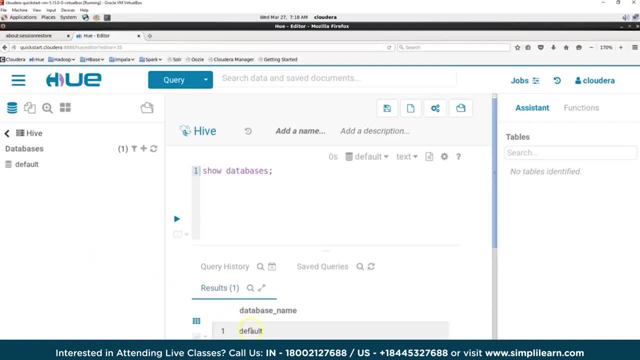 And you'll see down here, since this is a new quick start I just put on here. you'll see it has the default down here for the databases. I haven't actually created any databases on here. And then there's a lot of other like 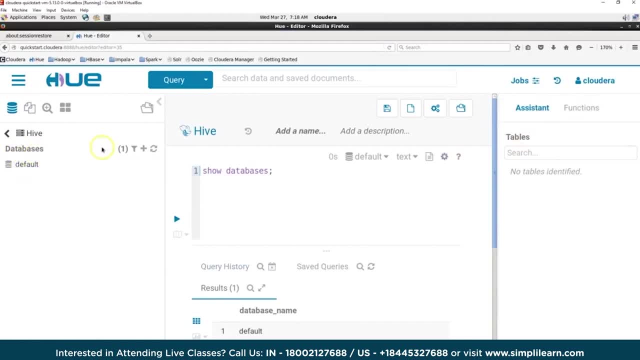 assistant function tables your databases up here. There's all kinds of things you can look at through Hue as far as a bigger picture. The downside of this is it always seems to lag For me. whenever I'm doing this, I always seem to run slow. 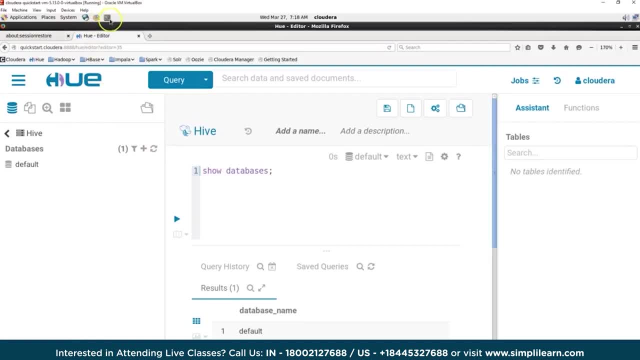 So if you're in Cloudera, you can open up a terminal window. They actually have an icon at the top. You can also go under applications and under applications, system tools and terminal. Either one will work. So this is the terminal window. 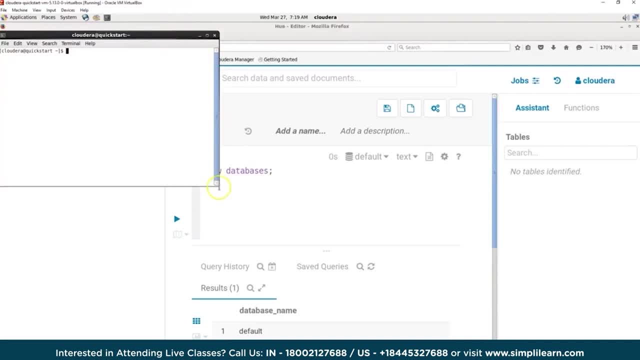 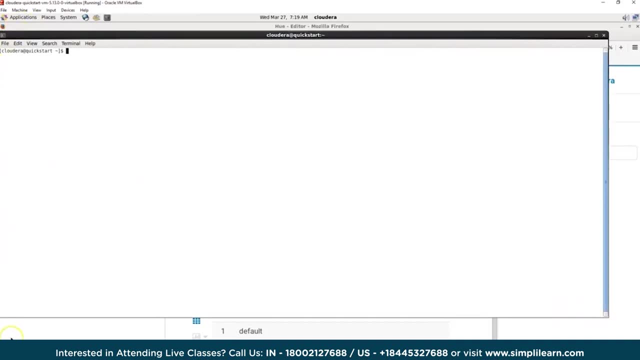 And this terminal window is now running underneath our Linux. So this is a Linux terminal window on our virtual machine which is resting on our regular Windows 10 machine, And we'll go ahead and zoom this in so you can see the text better on your own video. 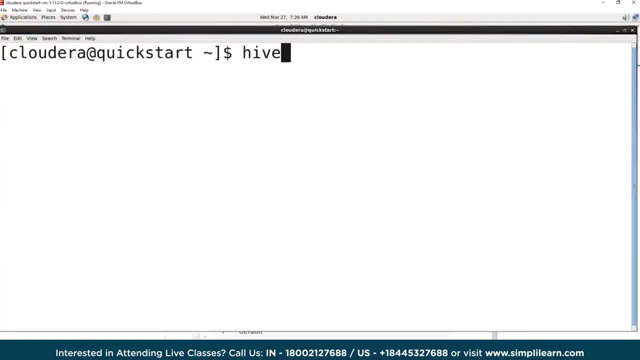 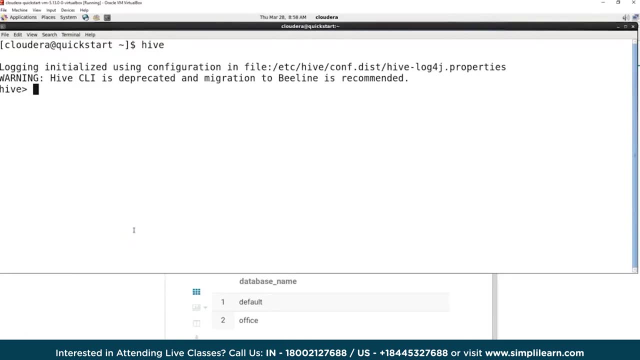 And I simply just clicked on view and zoom in And then all we have to do is type in Hive And this will open up the shell on here And it takes it just a moment to load. When starting up Hive, I also want to note that 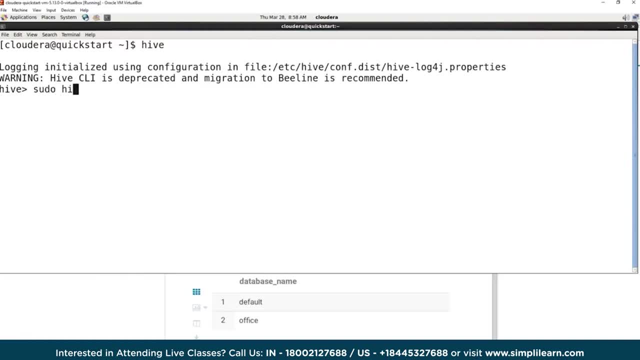 if you're running your writes on the computer, you're running your action. you might have to do sudo hive and put in your password and username. Most computers are usually set up with the Hive login. Again, it just depends on how you're accessing. 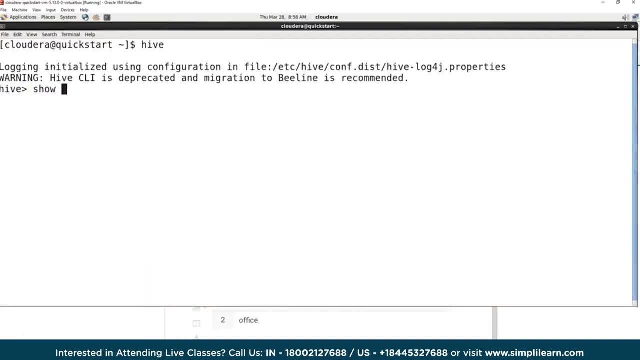 the Linux system and the Hive shell. Once we're in here, we can go ahead and do a simple HQL command- Show databases- And if we do that, we'll see here that we don't have any databases. So we can go ahead and create a database. 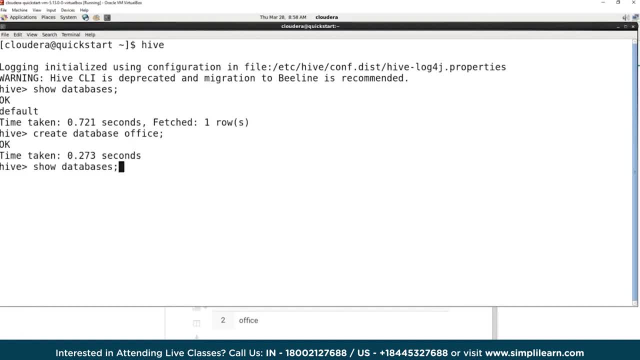 And we'll just call it Office for this moment. Now, if I do show up arrow, up arrow is a hotkey that works in both Linux and in Hive, So I can go back and page through all the commands I've typed in. 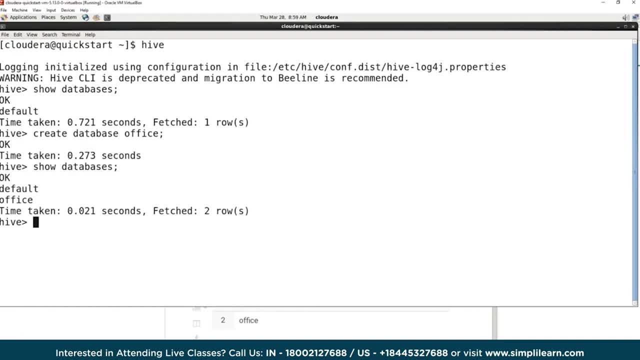 And we can see now that I have my. there's, of course, the default database and then there's the Office database. So now we've created a database. It's pretty quick and easy And we can go ahead and drop the database. We can do drop database office. 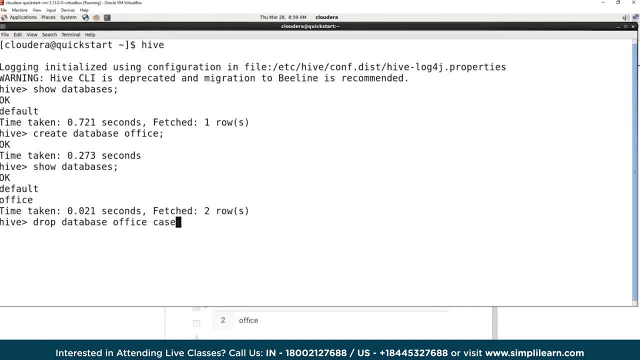 Now this will work on this database because it's empty. If your database was not empty, you would have to do cascade, And we can do that on the database itself. Now, if we do show database and we'll go ahead and recreate our database, 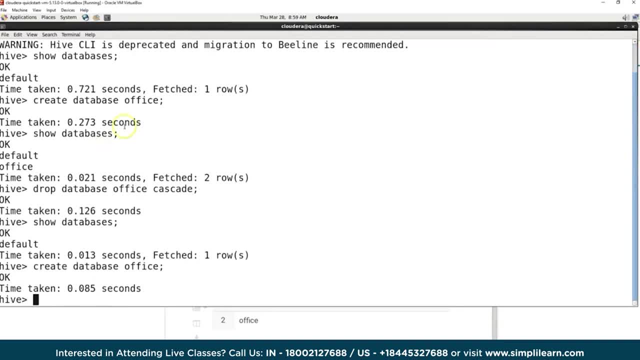 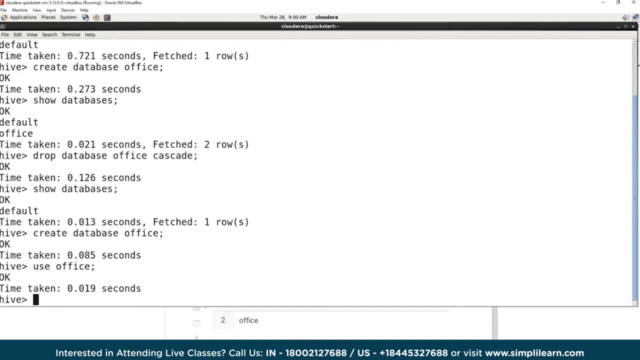 because we're going to use the Office database for the rest of this hands-on demo. A really handy command, now set with the SQL or HQL, is to use Office And what that does is that sets Office as the default database. So, instead of having to reference the database, 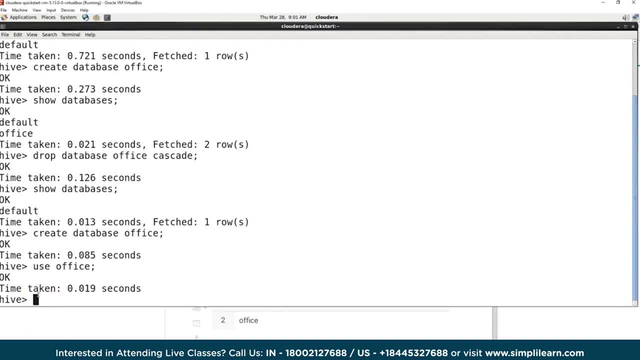 every time we work with a table, it now automatically assumes that's the database being used for what we're working on. The difference is you put the database name period table And I'll show you in just a minute what that looks like and how that's different. 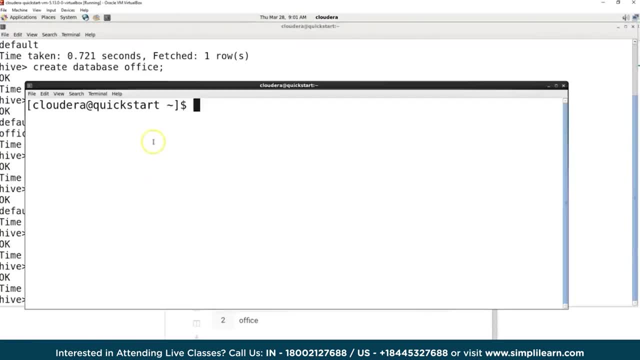 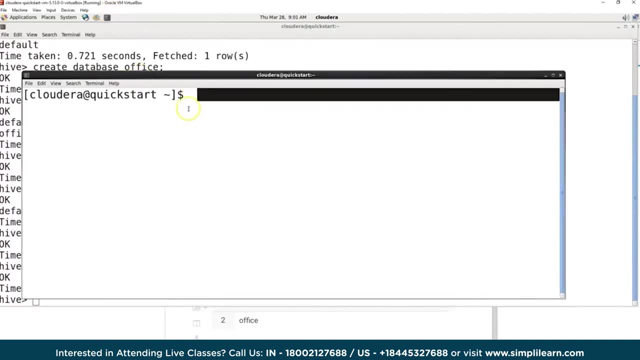 If we're going to have a table and a database, we should probably load some data into it. So let me go ahead and switch gears here and open up a terminal window. You can just open another terminal window and it'll open up right on top of the one. 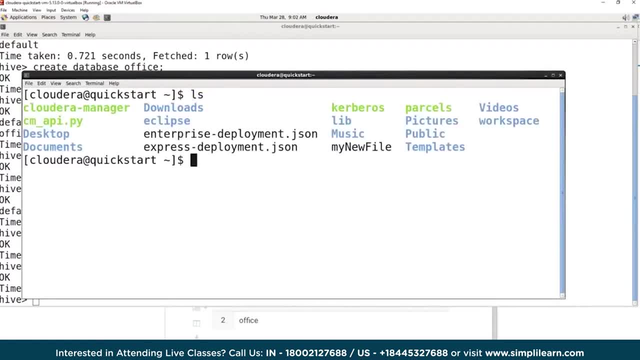 that you have Hive Shell running in, And when we're in this terminal window first, we're going to go ahead and just do a list, which is, of course, a Linux command. We can do documents, We can list in documents And we're actually going to be looking at. 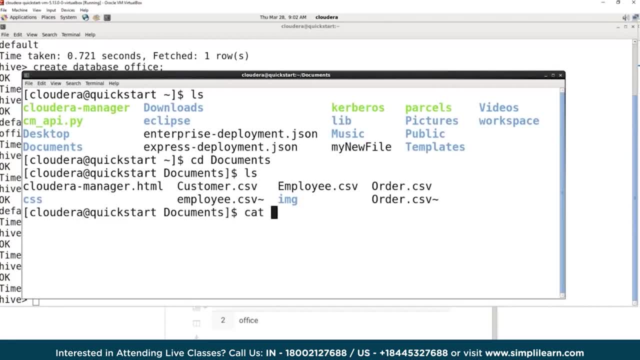 employeecsv. A Linux command is the cat. You can use this actually to combine documents. There's all kinds of things that cat does, But if we want to just display the contents of our employeecsv file, we can simply do cat employeecsv. 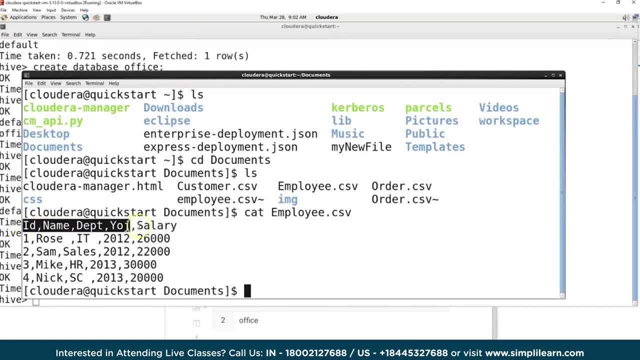 And when we're looking at this, we want to know a couple things. One: there's a line at the top, So the very first thing we notice is that we have a header line. The second thing we notice is that the data is comma separated. 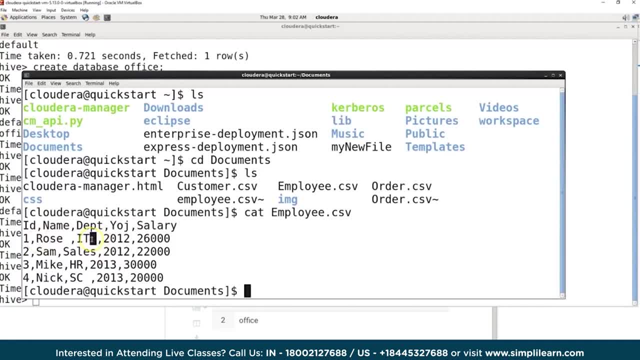 And in this particular case you'll see a space here. Generally, with these you've got to be real careful. with spaces. There's all kinds of things you've got to watch out for because it can cause issues. These spaces won't, because these are all. 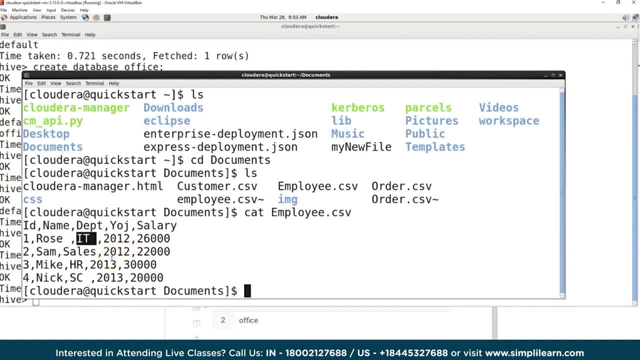 strings that the space is connected to. If this was a space next to the integer, you would get a null value that comes into the database without doing something extra in there. Now, with most of Hadoop that's important to know that you're writing the data once. 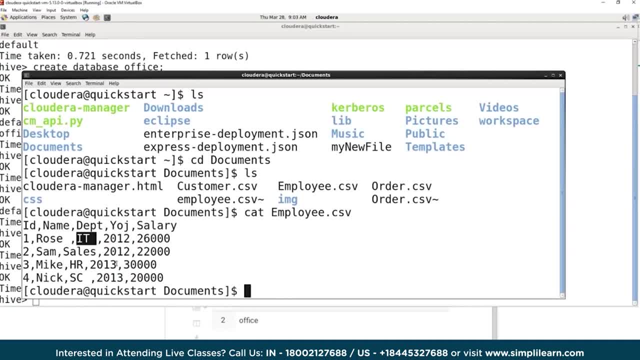 so you don't have to do almost all your Hadoop things coming in. So you really want to process the data before it gets into the database And for those of you who have studied data transformation, that's the etl, where you extract, transfer. 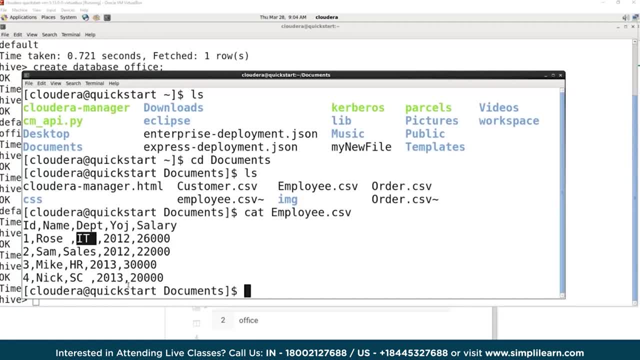 form and then load the data. So you really want to extract and transform before putting it into the hive. Then you load it into the hive with the transformed data And of course we also want to note the schema. We have an integer, string, string. 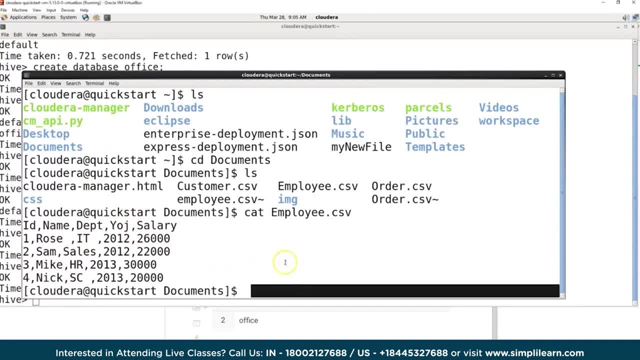 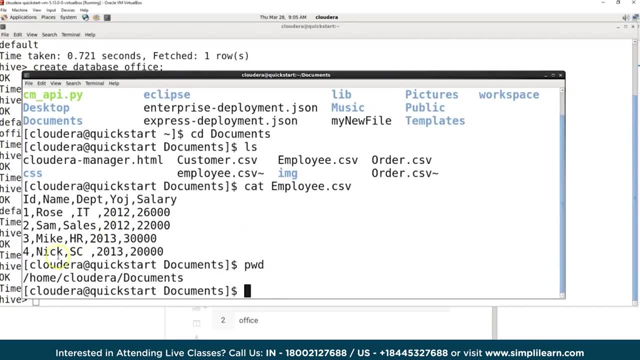 integer, integer. That's the way the data is set up. The last thing that you're going to want to look up is the source. Since we're doing local uploads, we want to know what the path is. We have the whole path. 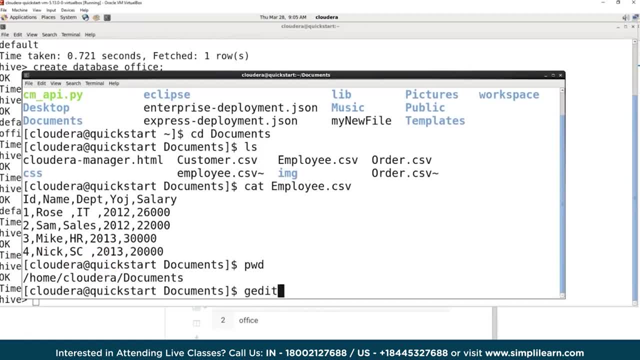 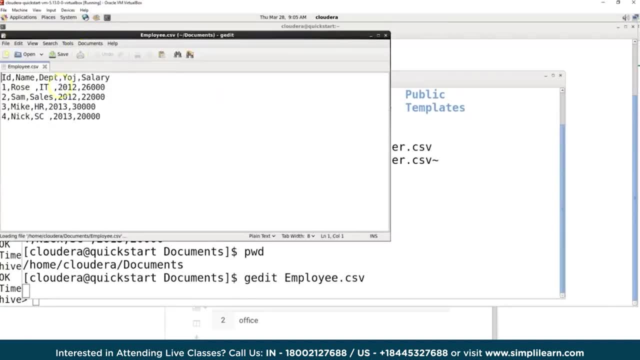 In this case it's home slash, Cloudera slash documents, And these are just text documents we're working with right now. We're not doing anything fancy, So we can do a simple git edit employee dot csv and you'll see it comes up here. 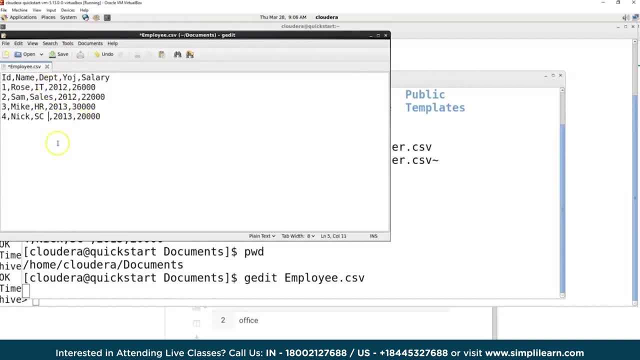 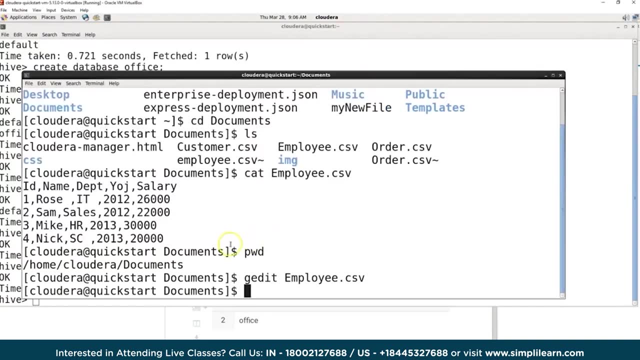 It's just a text document so I can easily remove these added spaces. There we go, And so now it has the new setup in there. We've edited it. The git edit is usually one of the defaults that loads into Linux, So any text editor will do. 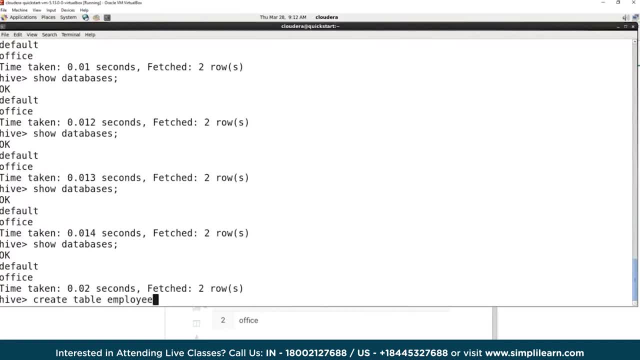 Back to the hive shell. So let's go ahead and create a table employee, And what I want you to note here is I did not put the semicolon on the end here. Semicolon tells it to execute that line. So this is kind of nice if you're. 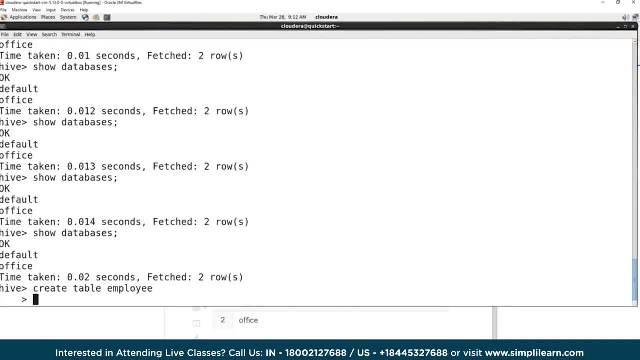 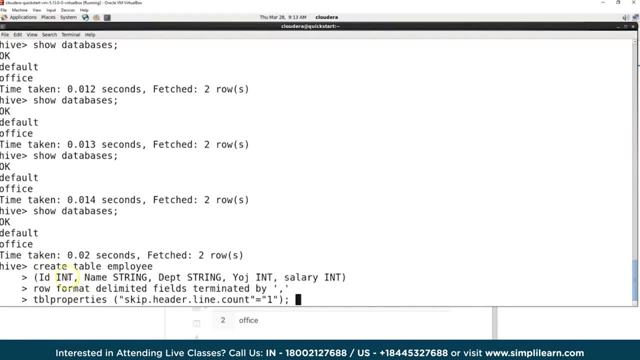 you can actually just paste it in if you have it written on another sheet And you can see right here where I have create table employee, So I can just follow my commands at once. Now, just so I don't have any typo errors, I went ahead and just pasted the next three lines in: 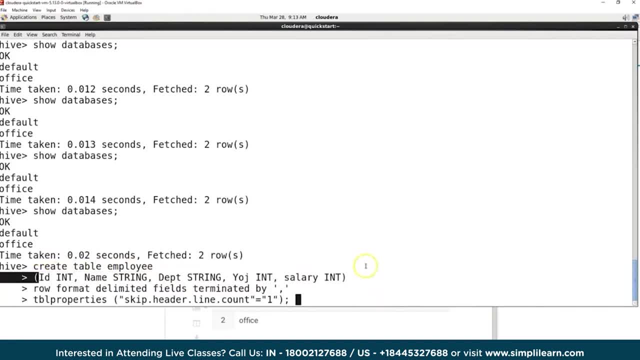 And the next one is our schema. If you remember correctly from the other side, we had the different values in here, which was id name, department, year of joining and salary, And the id is an integer name, is a string, department, string. 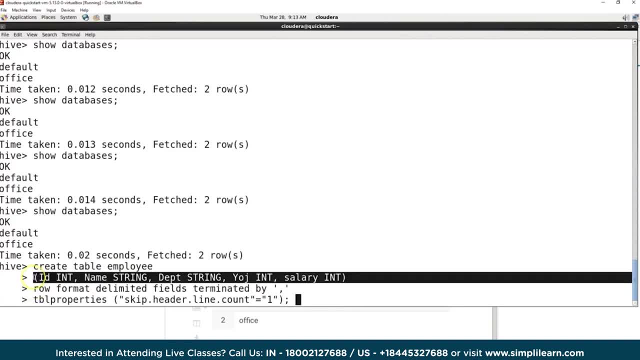 year of joining, salary is an integer And they're in brackets. We put closed brackets around them And you could do this all as one line. And you could do this all as one line And this is important because the default is tabs. 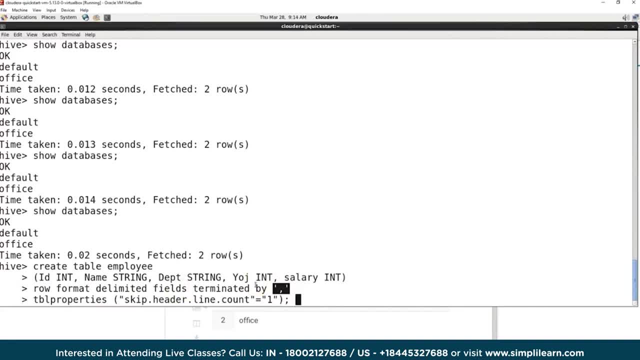 So if I do it now, it won't find any terminated fields, So you'll get a bunch of null values loaded into your table. And then, finally, our table properties. we want to skip the header line. count equals one. Now, this is a lot of work for uploading. 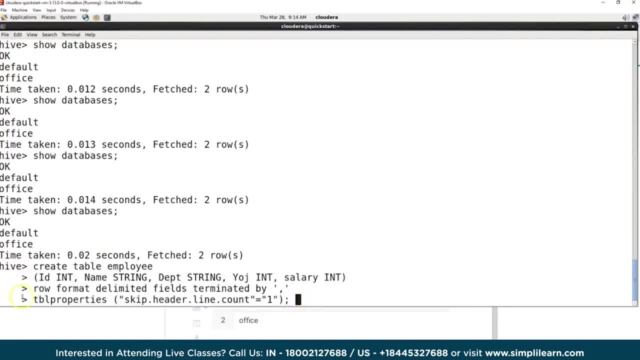 a single file. It's kind of goofy, when you're uploading a single file, that you have to put all this in here. But keep in mind Hive and Hadoop is designed for writing many files into the database. You write them all in there and then 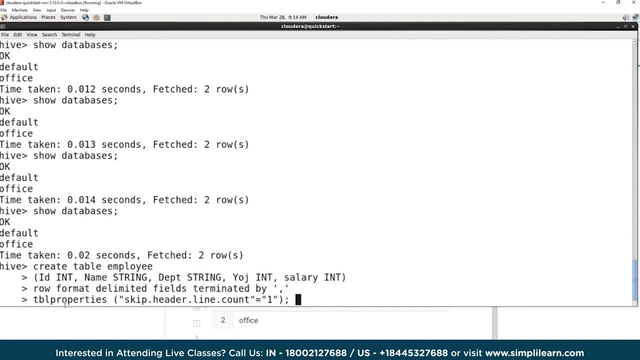 they're saved. It's an archive, It's a data warehouse, And then you're able to do all your queries on them. So a lot of times we're not looking at just the one file coming up, We're loading hundreds of files. 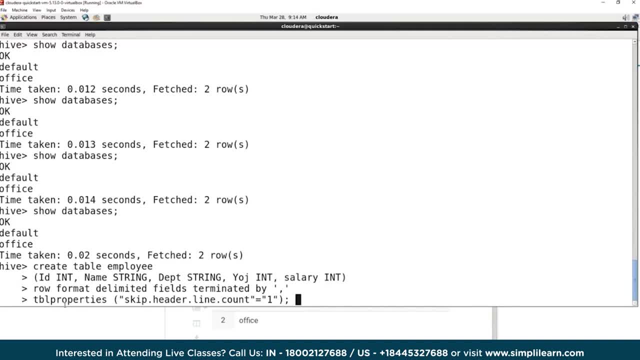 You have your reports coming off of your main database. All those reports are being loaded. You have your log files. All this different data is being dumped into Hadoop and, in this case, Hive on top of Hadoop, And so we need to let it know. 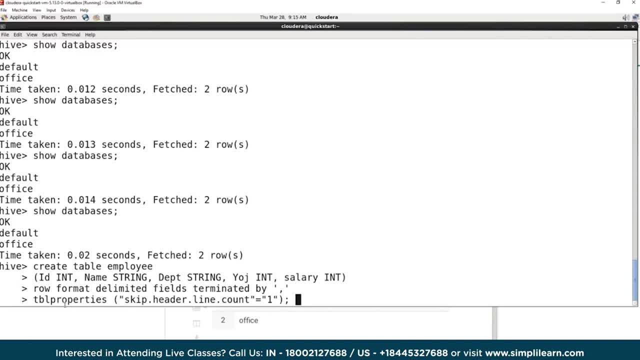 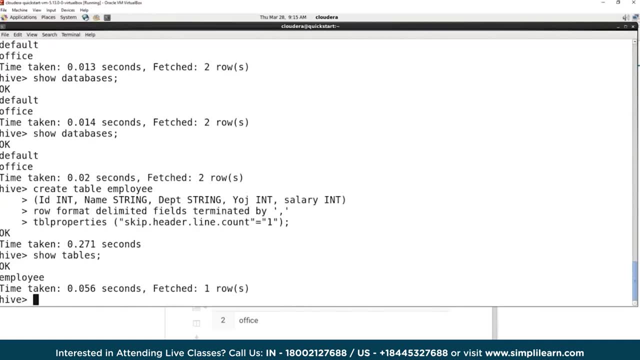 hey, how do I handle these files coming in? And then we have the semicolon at the end to go ahead and run this line. And so we'll go ahead and run that. And now, if we do a show tables, you can see there's our employee on there. 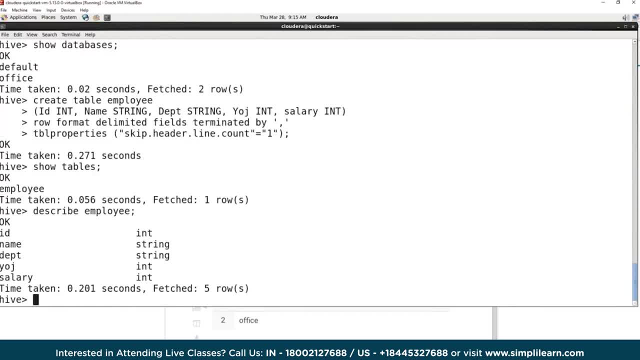 We can also describe. If we do describe employee, you can see that we have our ID integer, name string, department string, year of joining integer and salary integer. And then finally, let's just do a select star from employee. Very basic SQL and HQL command. 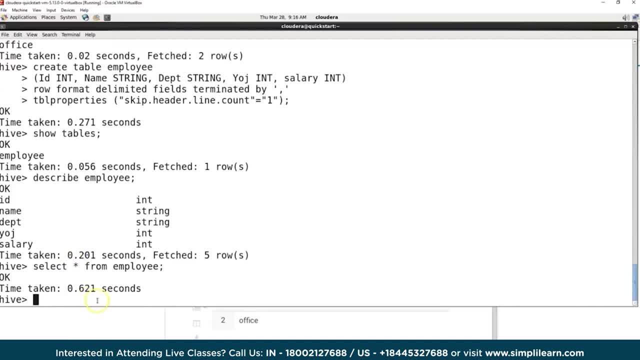 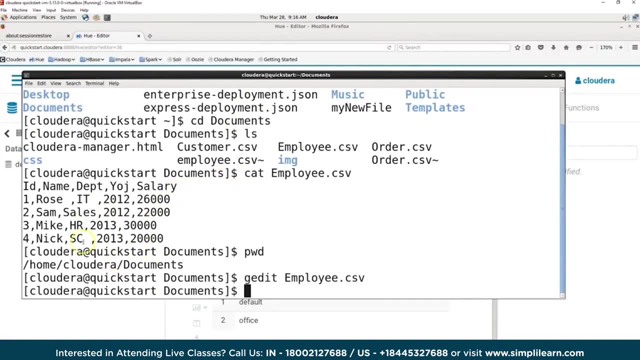 Selecting data. It's going to come up and we haven't put anything in it. as we expect. There's no data in it. So if we flip back to our Linux terminal window, you can see where we did the cat employee dot csv. 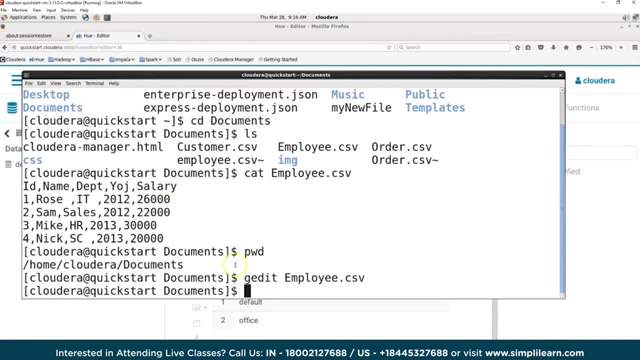 And you can see all the data we expect to come into it And we also did our PWD And right here you see the path. You need that full path. when you are loading data, You know you can do a browse and if I did it right now with just 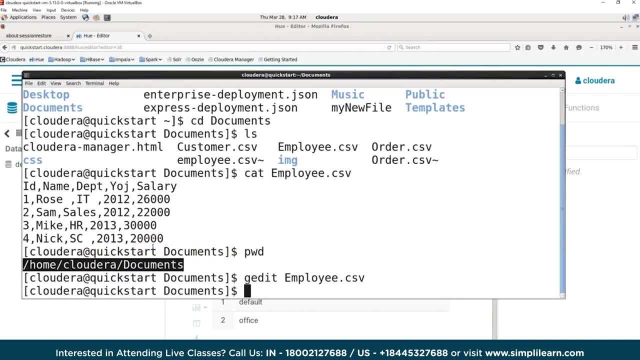 the employee dot csv as a name, it will work. But that is a really bad habit Because you don't know what else is going on in the computer. You want to do the full path almost in all your data loads, So let's go ahead and flip back over here. 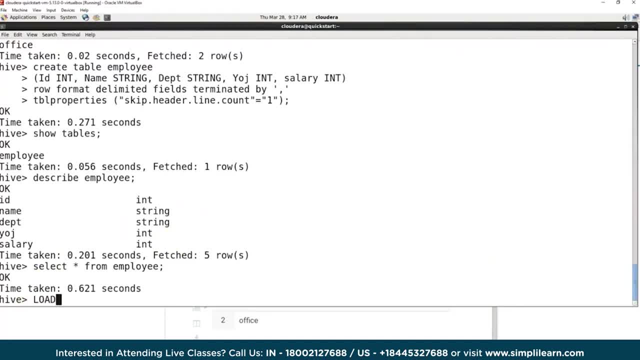 to our hive shell we are working in And the command for this is load data. So that says hey, we are loading data. That's a hive command, HQL, And we want local data. So you have to put down local And path. So now it needs to know where the path is. 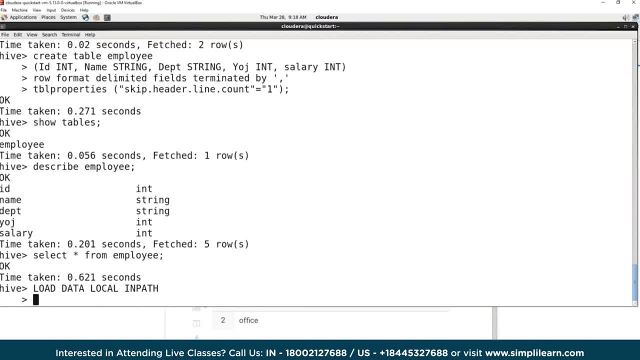 Now to make this more legible, I'm just going to go ahead and hit enter And then we will just paste the full path in there which I have stored over on the side. So it will be a good prepared demo. And you will see, here we have home cloud era documents. 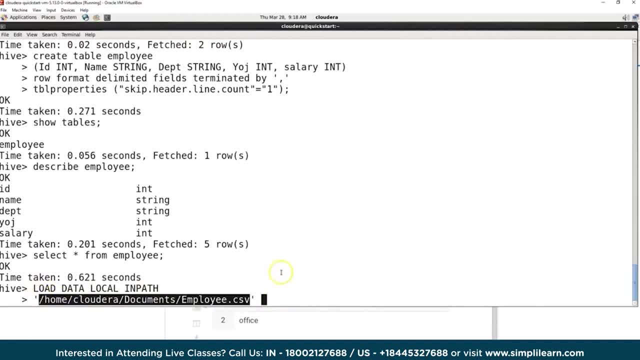 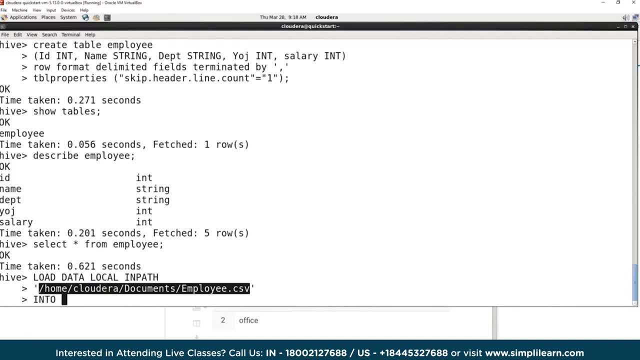 employee dot csv. So it is the whole path for this text document in here And we go ahead and hit enter in there And then we have to let it know where the data is going. So now we have a source and we need a destination. 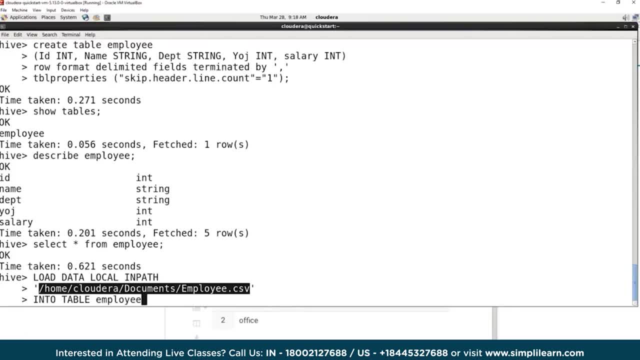 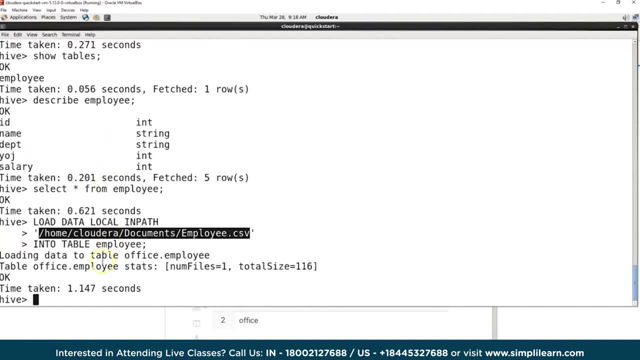 And it is going to go into the table and we will just call it employee. We will just match the table in there And, because I want it to execute, we put the semicolon on the end. It goes ahead and executes all three lines. 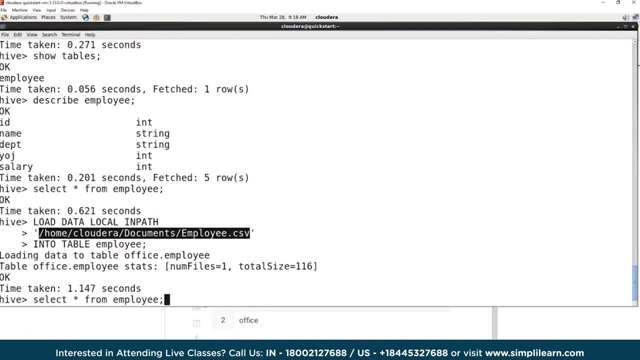 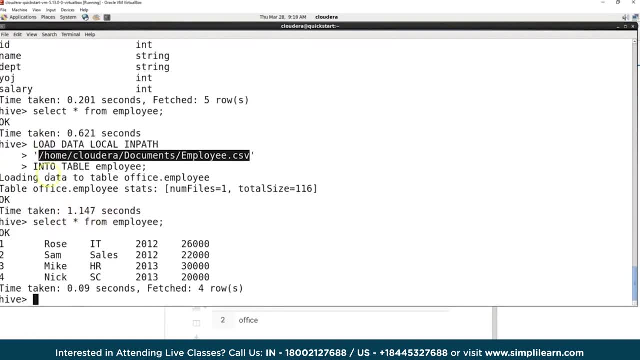 Now, if we go back, Select star from employee Just using the up error to page through my different commands I have already typed in. You can see right here we have as we expect. we have Rose, Sam, Mike and Nick And we have all their information. 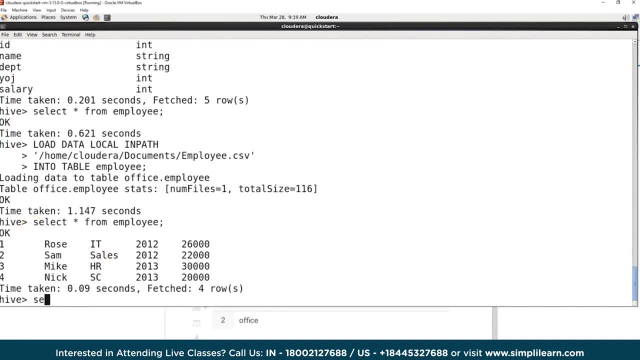 showing in our four rows. And then let's go ahead and do select and count. Just look at a couple of these different select options you can do. We are going to count everything from employee. Now, this is kind of interesting because the first one 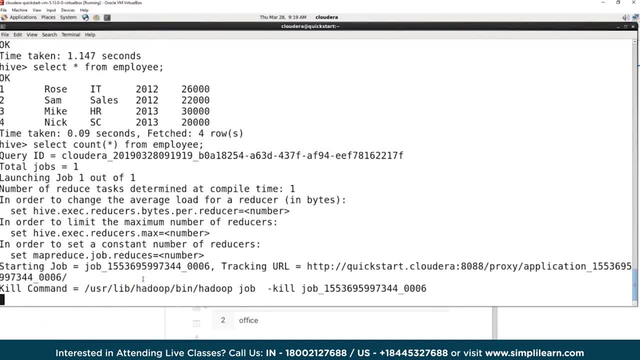 just pops up with a basic select, Because it doesn't need to go through the full map reduce phase. But when you start doing a count it does go through the full map reduce. setup in the Hive and Hadoop. And because I am doing this, 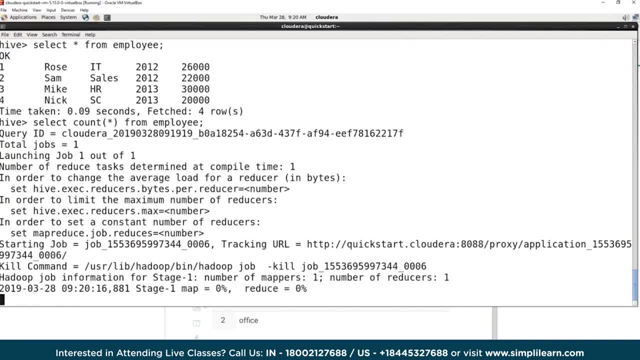 demo on a single node: Cloudera VirtualBox on top of a Windows 10. all the benefits of running it on a cluster are gone and instead it is now going through all those added layers, so it takes longer to run. Like I said, when you do a single node. 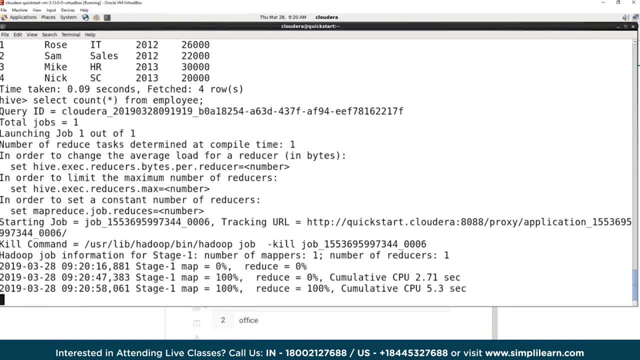 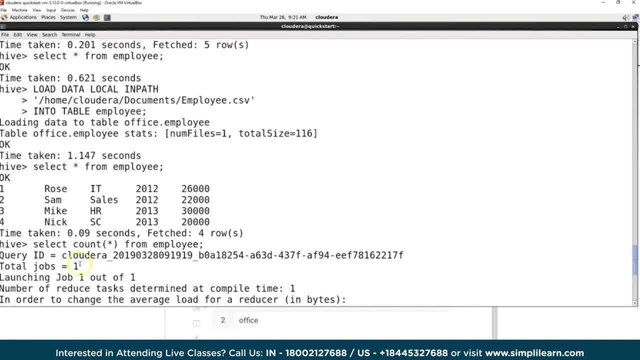 as I said earlier, it doesn't do any good as an actual distribution because you are only running it on one computer and then you have added all these different layers to run it And we see it comes up with four. and that is what we expect. We have four rows. 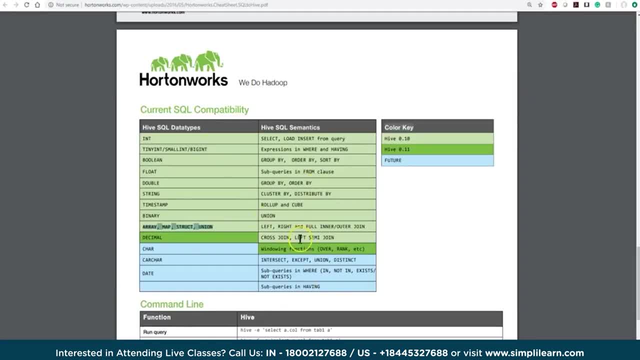 we expect four at the end And if you remember from our cheat sheet which we brought up here from Horton's, it is a pretty good one. There are all these different commands we can do. We will look at one more command where we do what they call. 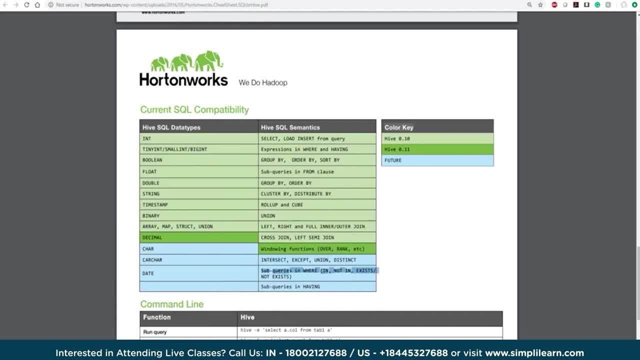 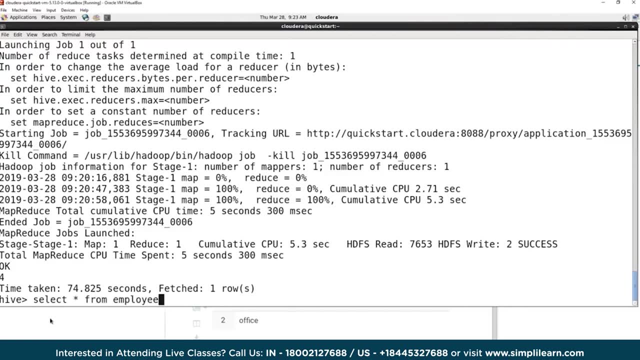 sub queries right down here, Because that is really common to do, a lot of sub queries, And so we will do select star or all different columns from employee. Now, if we weren't using the office database, it would look like this: from office dot: employee, And either one will work. 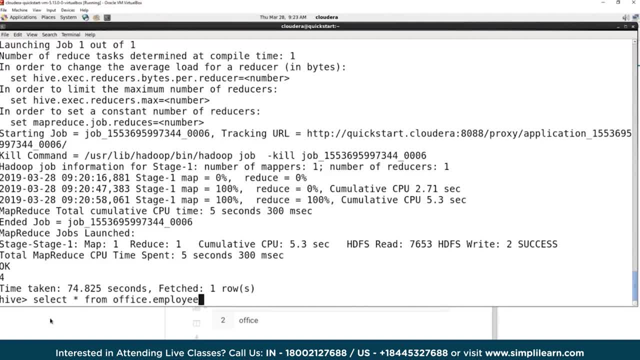 on this particular one, because we have office set as a default on there. So, from office employee and then the command where creates a subset, and in this case we want to know where the salary is greater than 25,000.. There we go And of course we end with our 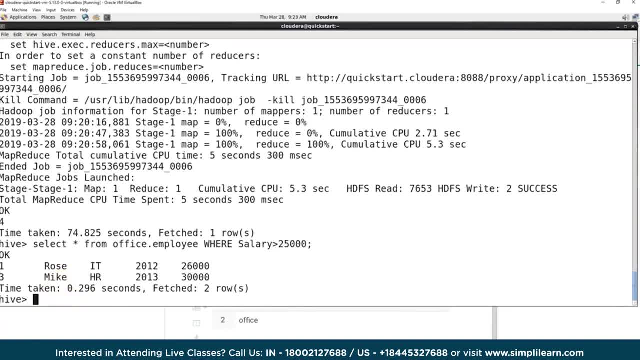 semicolon And if we run this query, you can see it pops up and there is our salary and we can see some people top earners. We have Rose in IT and Mike in HR. Kudos to them. Of course, they are fictitional. We don't actually have a Rose. 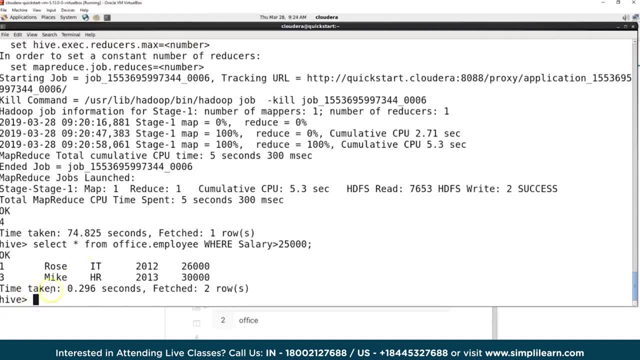 and a Mike in those positions- Or maybe we do So. finally, what we want to go ahead and do is we are done with this table. Now, remember, you are dealing with a data warehouse, so you usually don't do a lot of dropping of tables and 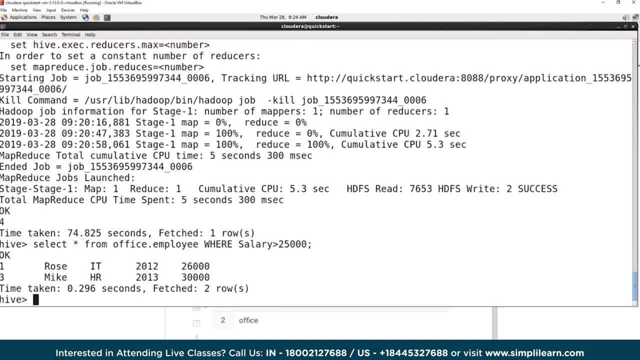 databases, But we are going to go ahead and drop this table here. Before we drop it, one more quick note is: we can change it. So what we are going to do is we are going to alter table office employee And we want to go ahead and rename it. 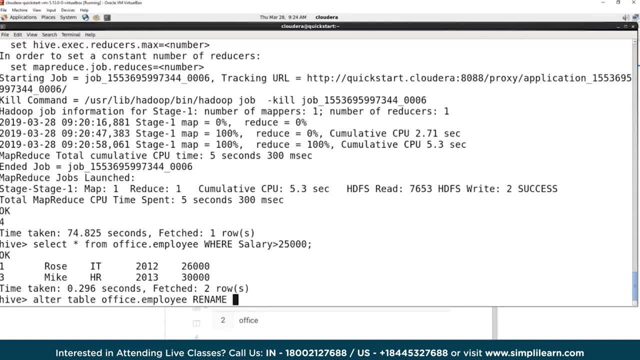 There are some other commands you can do in here, but rename is pretty common And we are going to rename it to and it is going to stay in office and it turns out one of our shareholders really doesn't like the word employee. He wants employees plural. 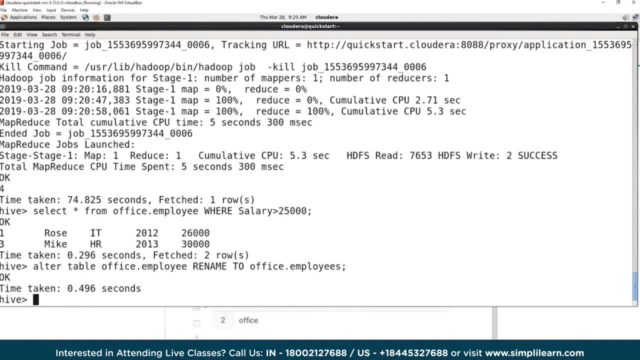 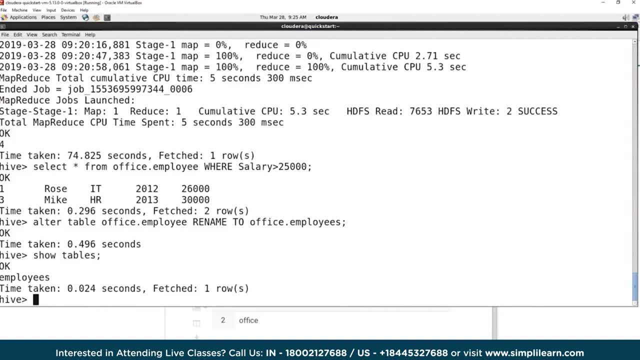 It is a big deal to him. So let's go ahead and change that name for the table. It is that easy because it is just changing the metadata on there. And now, if we do show tables, you will see we now have employees, not employee. 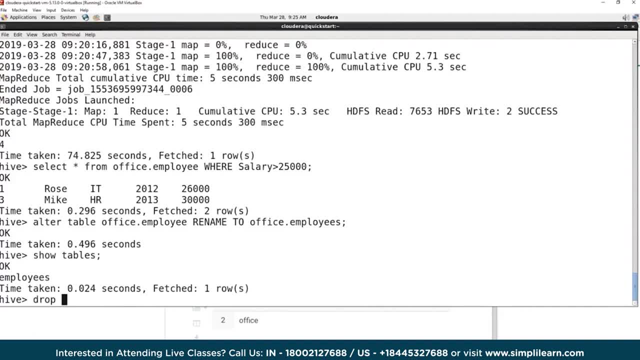 And then at this point maybe we are doing some house cleaning because this is all practice, So we are going to go ahead and drop table and we will drop table employees because we changed the name in there. So if we did employee it would just give us an error. 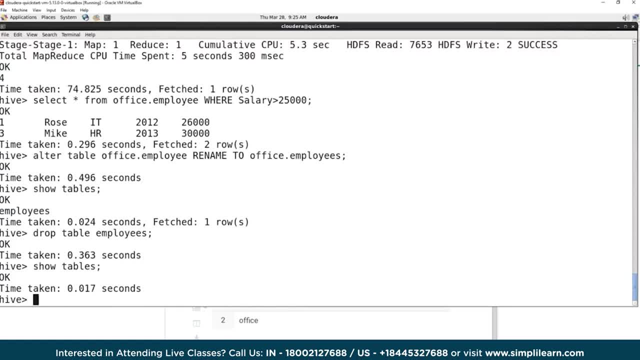 And now, if we do show tables, you will see all the tables are gone. Now the next thing we want to go ahead and take a look at and we are going to walk back through the loading of data just real quick, because we are going to load two. 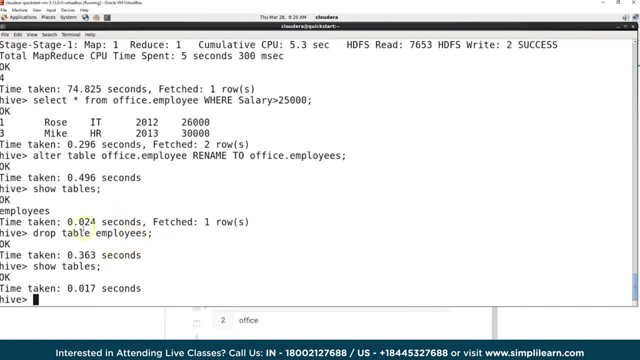 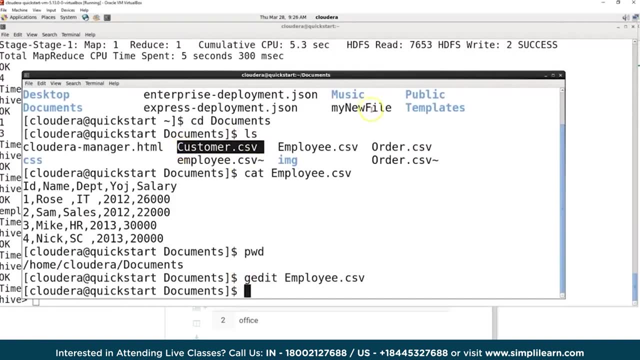 tables in here And let me just float back to our terminal window so we can see what those tables are that we are loading So up here we have. we have a customer file and we have an order file. We want to go ahead and put the customers and the orders 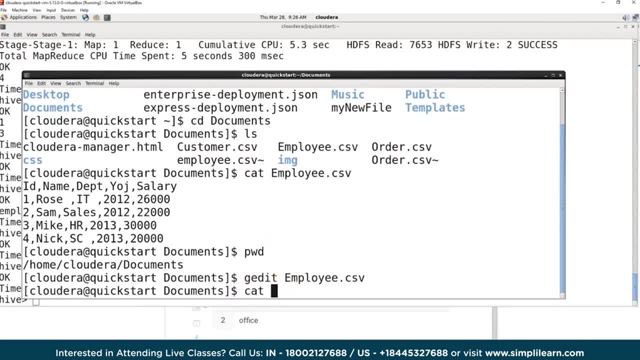 into here. So those are the two we are doing, And, of course, it is always nice to see what you are working with. So let's do our cat customercsv. we could always do gedit, but we don't really need to edit these, We just want to take a look at. 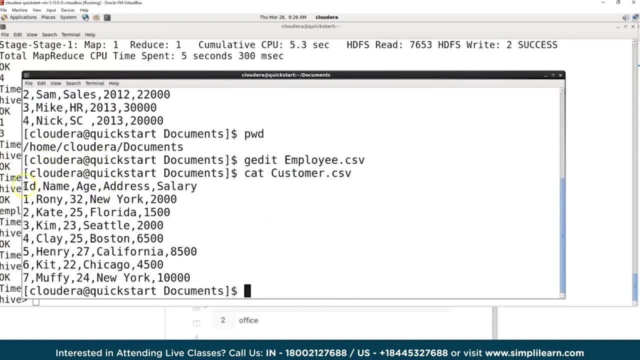 the data in customer. And important in here is again, we have a header, so we have to skip a line, comma separated. Nothing odd with the data. We have our schema which is integer, string, integer, string, integer. So you know you would want to take that. 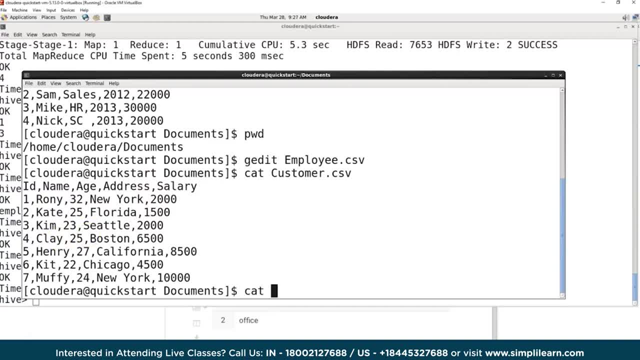 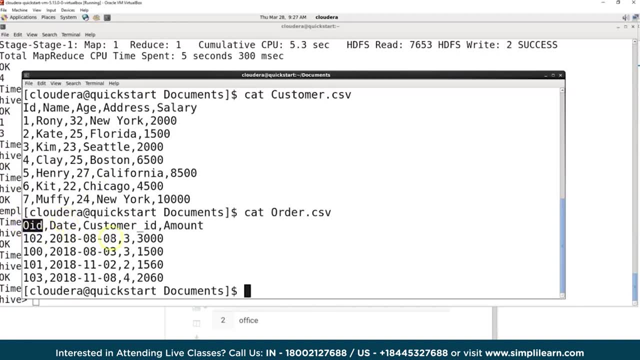 note that down or flip back and forth when you are doing it. And then let's go ahead and do cat ordercsv and we can see we have oid, which I am guessing is the order id. We have a date. Oh, something new. We have done integers and strings, but we haven't done. 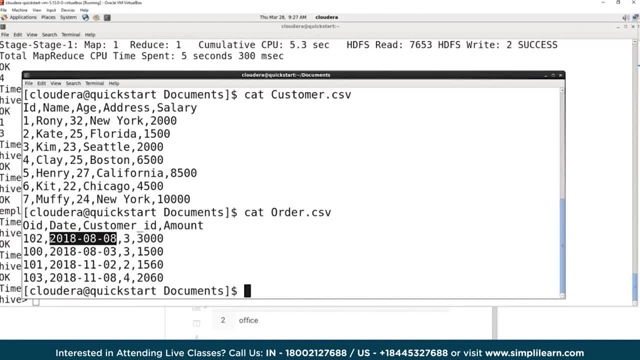 date When you are importing new and you never worked with the date. date is always one of the more trickier fields to port in, And that is true of just about any scripting language I have worked with. All of them have their own idea of how date is supposed. 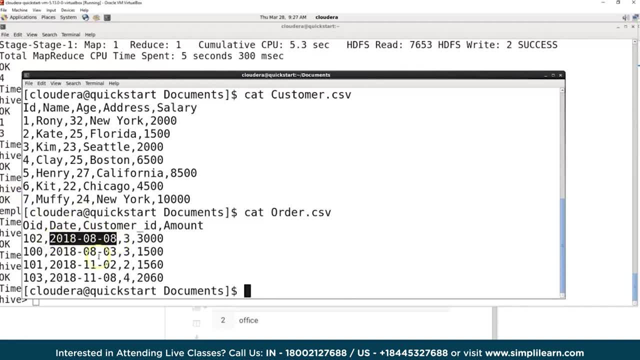 to be formatted what the default is. This particular format, where it is year and it has all four digits dash month, two digits dash day, is the standard import for the hive. So you will have to look up and see what the different formats are If you are going to do a different format. 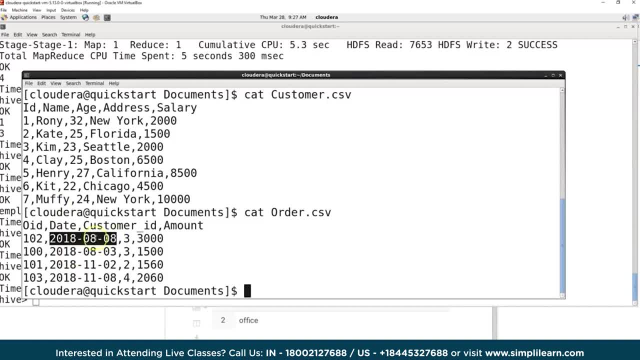 in there coming in or you are not able to preprocess the data, But this would be a preprocessing of the data thing coming in, If you remember correctly from our etl, which is e, just in case you weren't able to hear me last time. 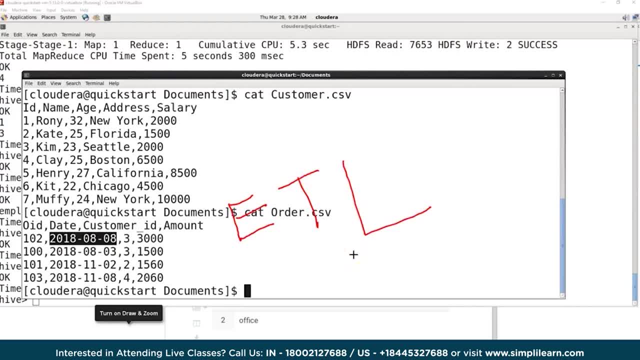 etl, which stands for extract, transform then load. So you want to make sure you are transforming this data before it gets into here, And so we are going to go ahead and bring both this data in here, And really we are doing this so we can show you. 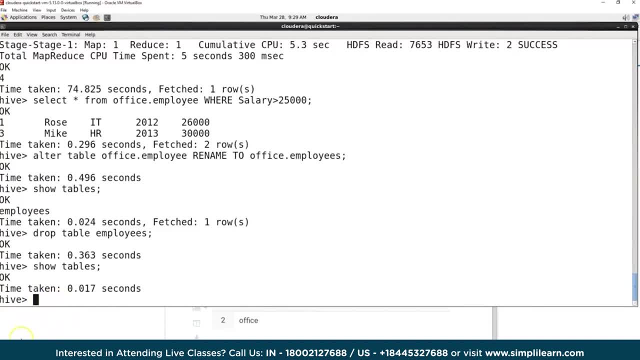 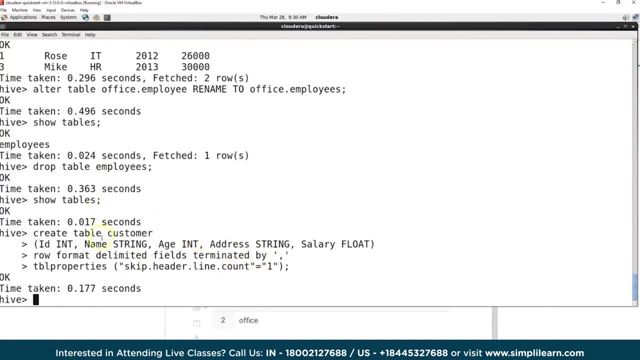 the basic join. There is, if you remember from our setup, merge, join- all kinds of different things you can do, But joining different data sets is so common, So it is really important to know how to do this. We need to go ahead and bring in these two data sets. 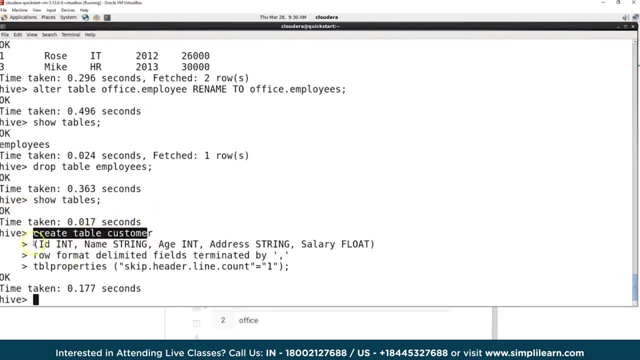 And you can see where I just created a table: customer. Here is our scheme, The integer: name, age, address, salary. Here is our, delimited by commas, and our table properties. where we skip a line. Well, let's go ahead and load the data first, And then we will do that. 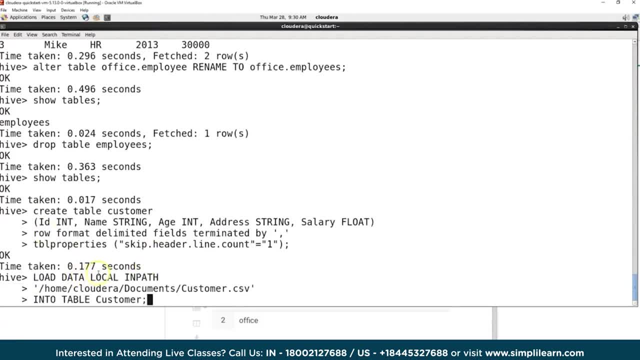 with our order And let's go ahead and put that in here, And I have got it split into three lines so you can see it easily. We have got load data local in path. So we know we are loading data, We know it is local and we have the path. Here is. 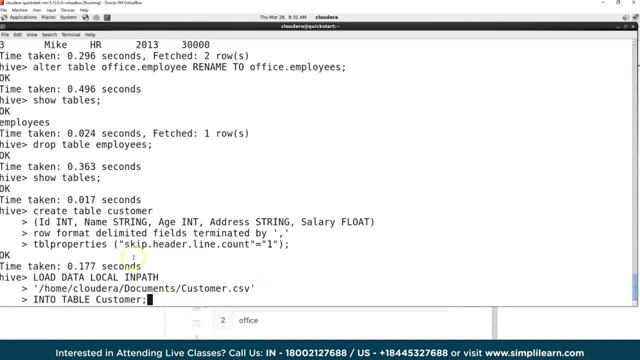 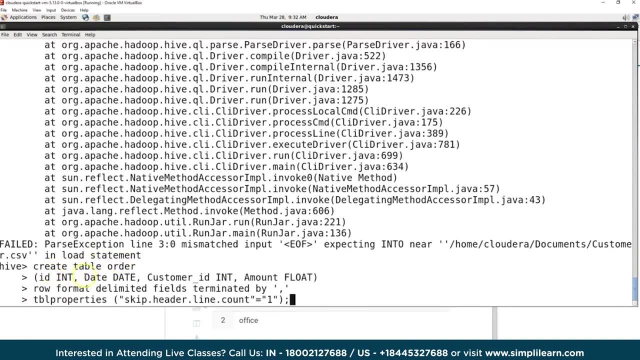 the complete path, for oops, this is supposed to be order. csv Grabbed the wrong one. Of course it is going to give me errors, because you can't recreate the same table on there, And here we go: Create table. Here is our integer. 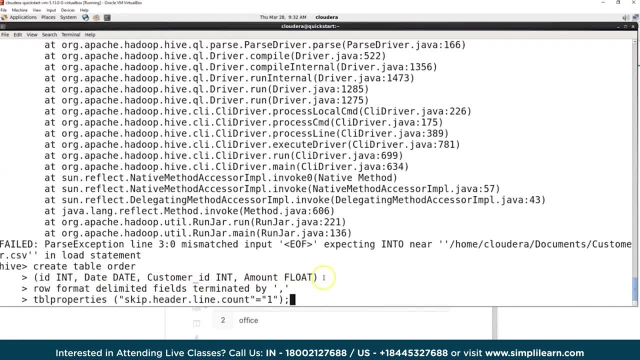 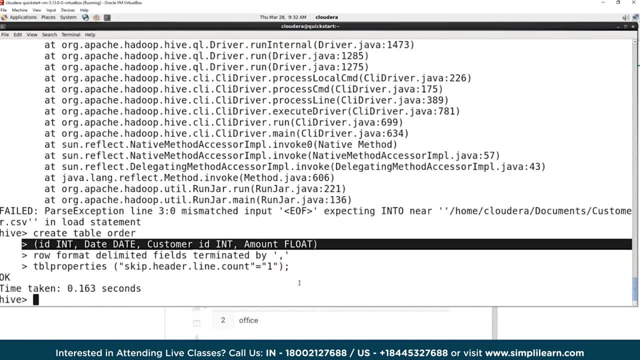 date customer, the basic set up that we had coming in here for our schema: row format, commas, table properties, skip header line And then finally, let's load the data into our order table. Load data local in path: home cloud data documents. 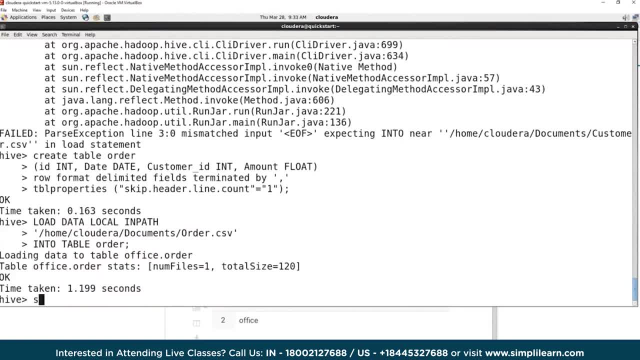 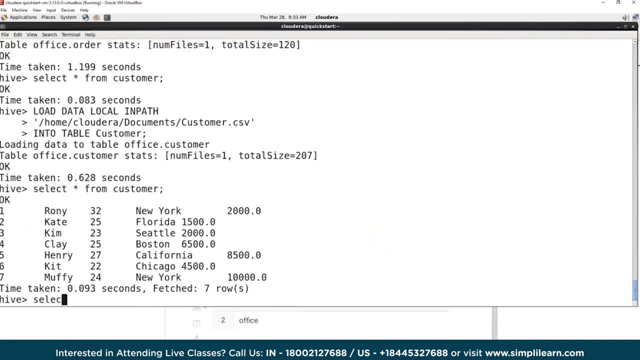 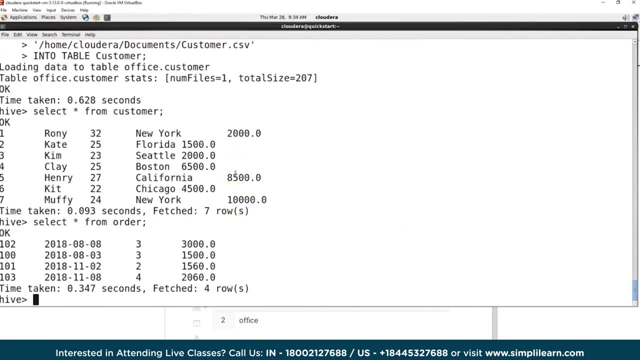 ordercsv into table order. Now, if we did everything right, we should be able to do select star from customer And you can see we have all seven customers. and then we can do select star from order And we have four orders. So this is just like a quick frame. 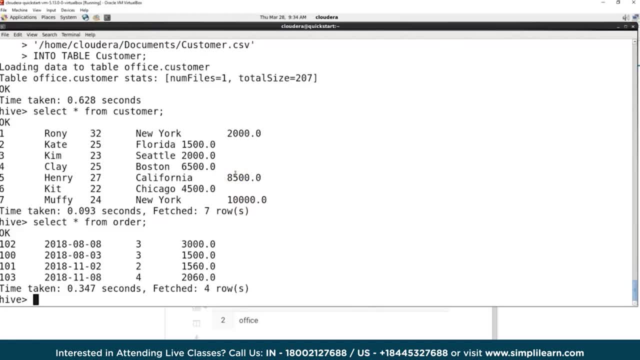 A lot of times when you have your customer databases in business, you have thousands of customers from years and years and some of them close their business, they change names, all kinds of things happen. So what we want to do is we want to go ahead and find 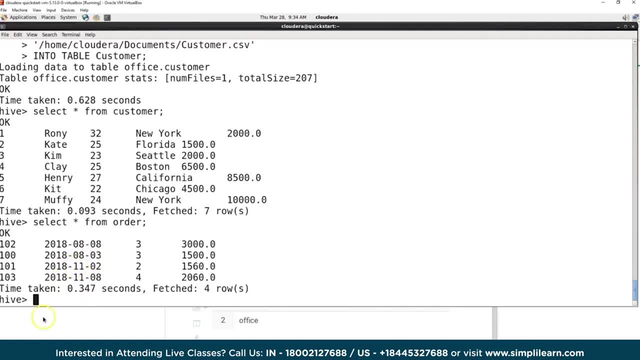 just the information connected to these orders and who is connected to them. So let's go ahead and do select, because we are going to display this information. So select, and this is kind of interesting. We are going to do cid and I am going to 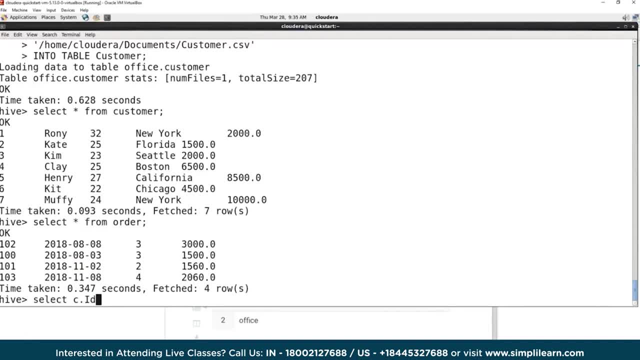 define c as customer, As a customer table, in just a minute. Then we are going to do cname and again we are going to define the c cage. So this means from the customer we want to know their id, their name, their age and then 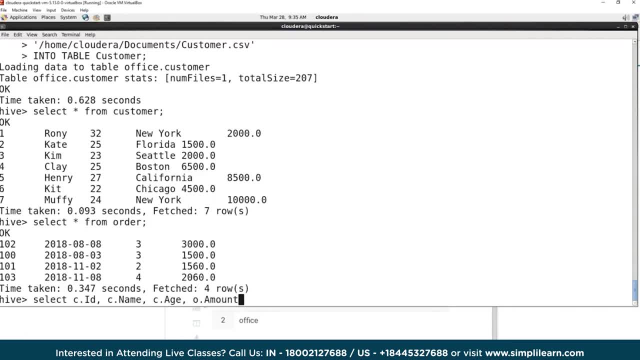 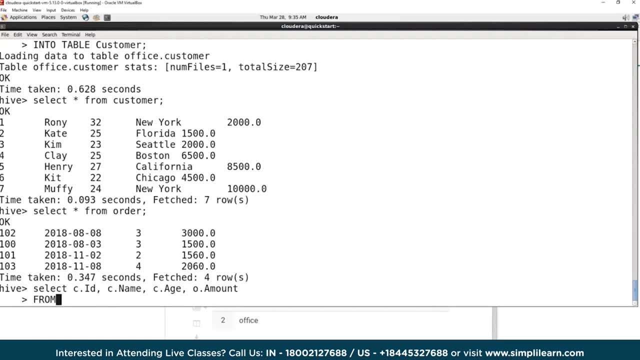 you know, I would also like to know the order amount. So let's do o for dot amount And then this is where we need to go ahead and define what we are doing And I will go ahead and utilize from customer. So we are going to take the customer table in here. 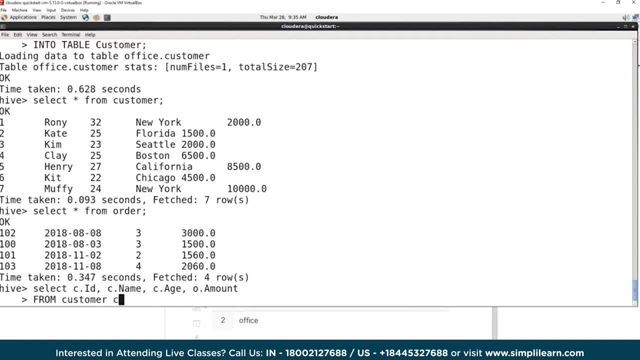 and we are going to name it c. That is where the c comes from. So that is the customer table c, and we want to join order as o. That is where our o comes from. So the oamount is what we are joining in there. And then we want to do this: 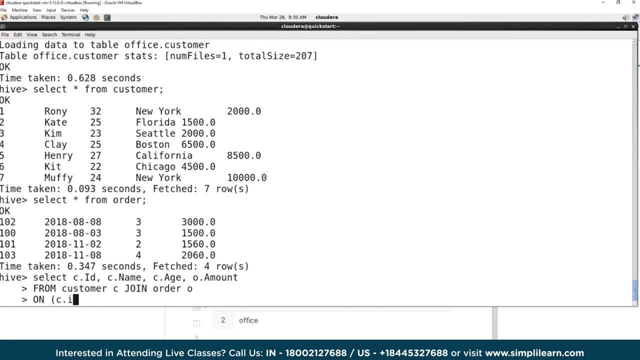 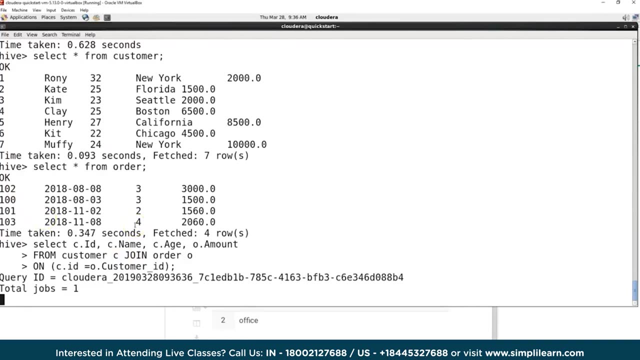 on. We have to tell it how to connect the two tables. Cid equals o customer underscore id. So now we know how they are joined. And now remember, we have seven customers in here, We have four orders and as it processes, we should get a return of four. 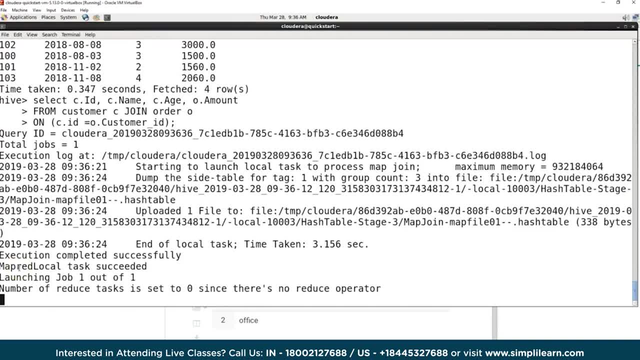 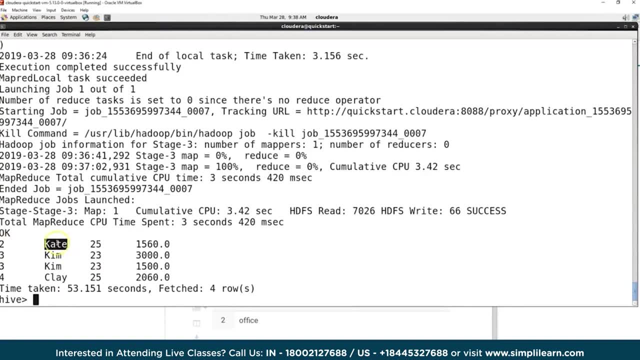 different names joined together, And they are joined based on, of course, the orders on there, And, once we are done, we now have the order number, the person who made the order, their age and the amount of the order which came from the order table. So you have your different. 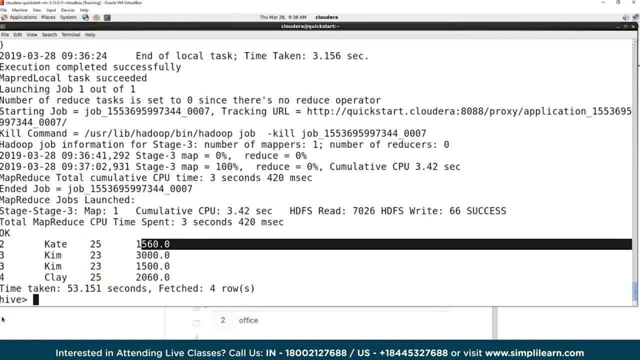 information And you can see how the join works here. Very common use of tables and hql and sql. And let's do one more thing with our database and then I will show you a couple other Hive commands And let's go ahead and do a drop. 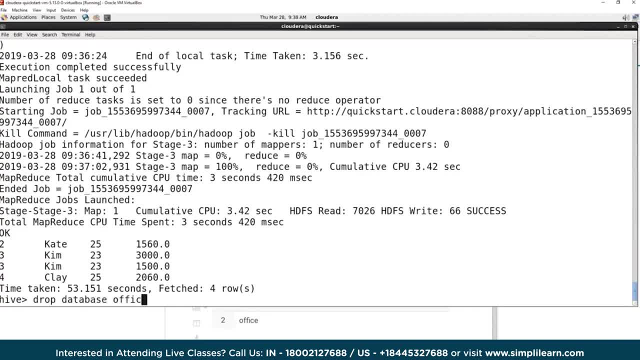 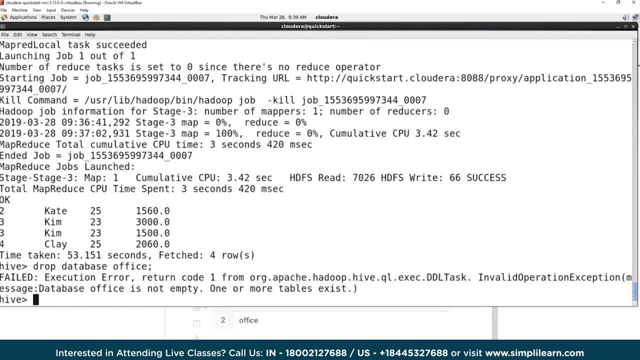 and we are going to drop database office And if you are looking at this and you remember from earlier, this will give me an error And let's just see what that looks like. It says: fail to execute exception: one or more tables exist. So if you remember from before, 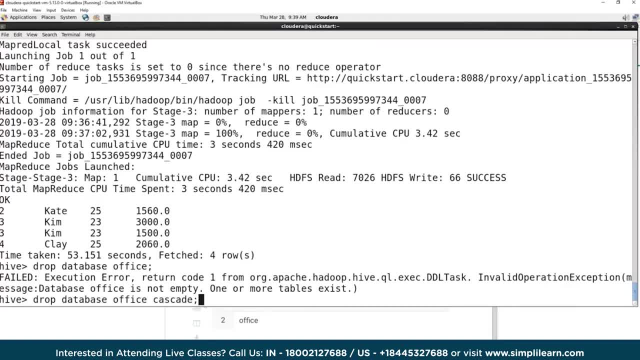 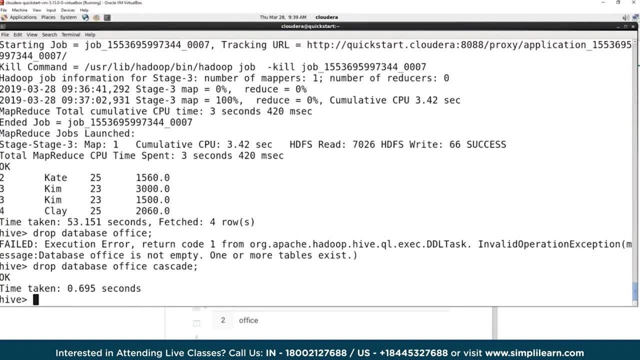 you can't just drop a database unless you tell it to cascade. That lets it know. I don't care how many tables are in it, let's get rid of it. And in Hadoop, since it's an instance, a warehouse, a data warehouse, usually don't do a lot of dropping. 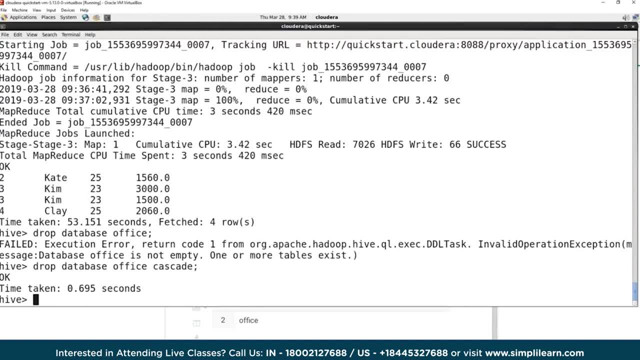 Maybe at the beginning when you are developing the schemas and you realize you messed up, you might drop some stuff. But down the road you are really just adding commodity machines to take up so you can store more stuff on it. So you usually don't do a lot of database dropping. 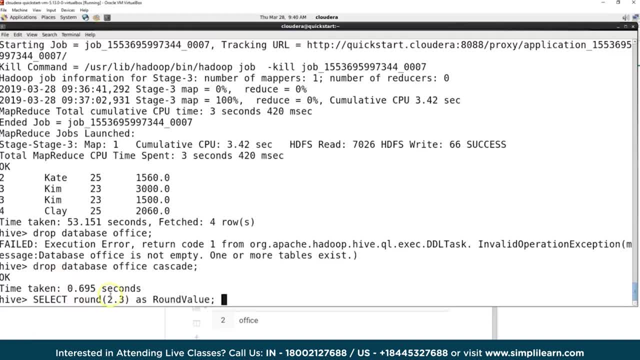 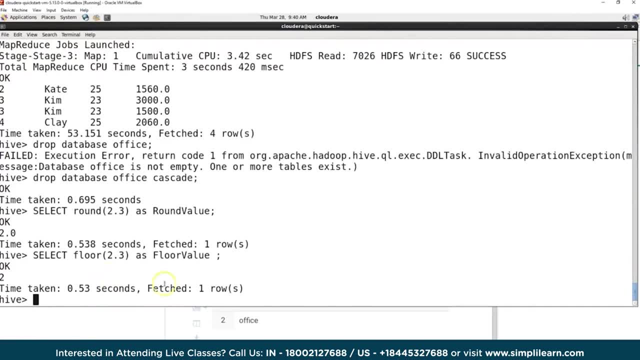 And some other fun commands. to know is: you can do select round 2.3 as round value. You can do a round off in Hive. We can do as floor value, which is going to give us 2.. So it turns it into an integer. 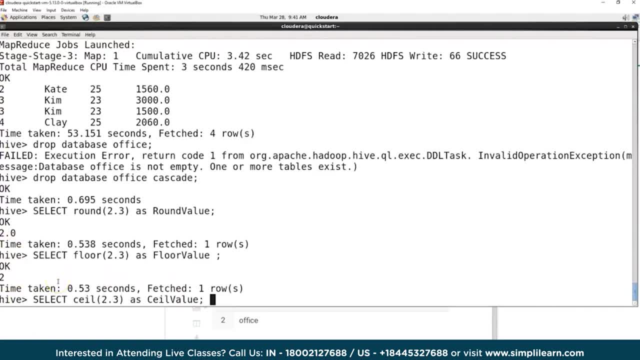 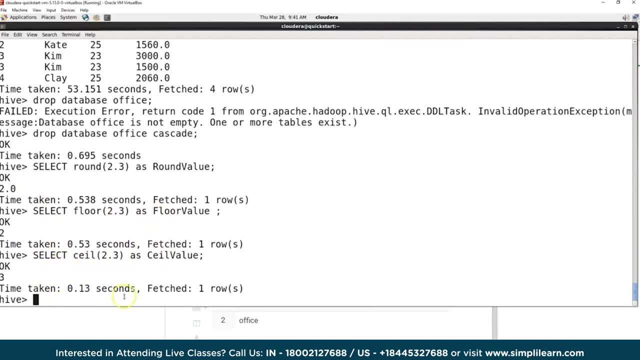 which is a float. It goes down, basically truncates it, but it goes down, and we can also do ceiling, which is going to round it up. So we are looking for the next integer above. There is a few commands we didn't show in here. 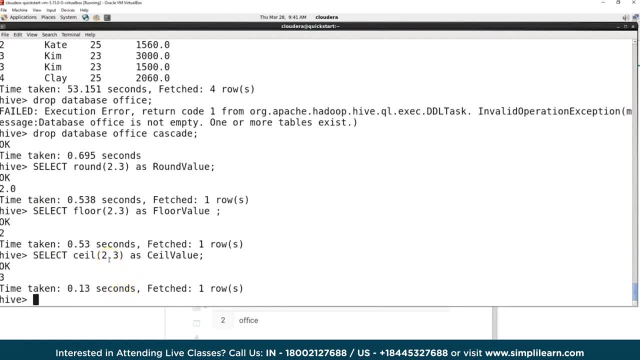 because we are on a single node. As an admin, to help speediate the process, you usually add in partitions for the data in buckets. You can't do that on a single node because when you add a partition, it partitions it across separate nodes But beyond. 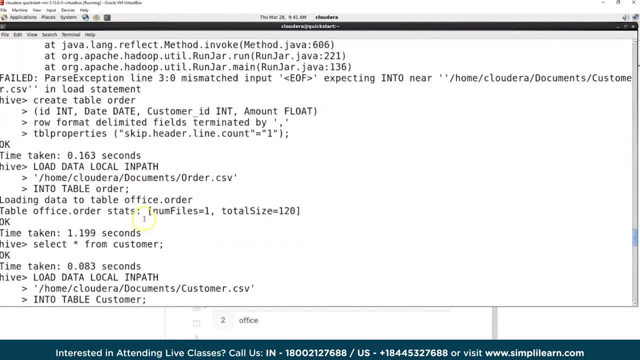 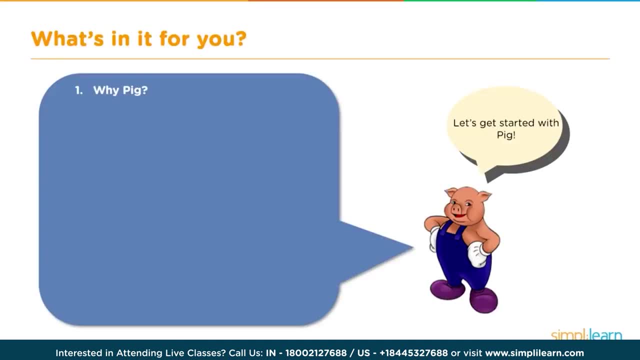 that you can see that it is very straight forward. We have SQL coming in and all your basic queries that are in SQL are very similar to HQL. Let's get started with PIG. Why PIG? What is PIG? MapReduce vs. 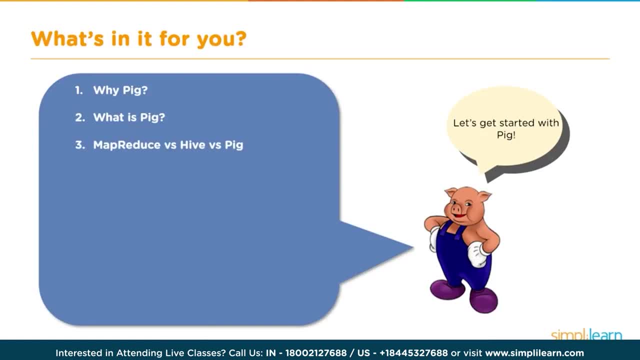 Hive vs PIG. Hopefully you have had a chance to do our Hive tutorial and our MapReduce tutorial. If you haven't, send a note over to SimplyLearn and we will follow up with a link to you. We will look at PIG architecture. 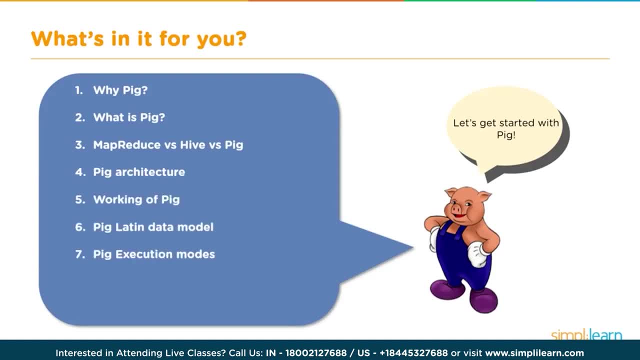 working of PIG, PIG- Latin data model, PIG execution modes, a use case, Twitter and features of PIG. And then we will tag on a short demo so you can see PIG in action. So why PIG? As we all know, Hadoop uses 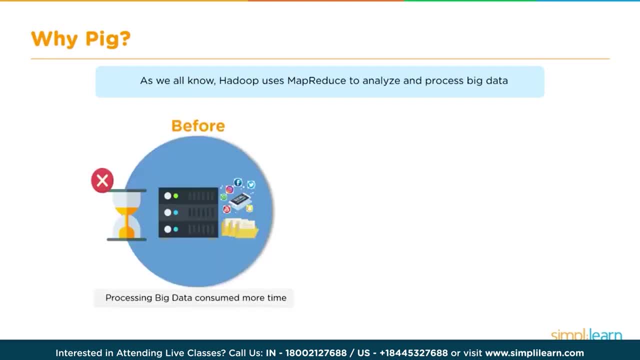 MapReduce to analyze and process big data. Processing big data consumed more time, So before we had the Hadoop system, they would have to spend a lot of money on a huge set of computers and enterprise machines. So we introduced the Hadoop MapReduce And so afterwards, 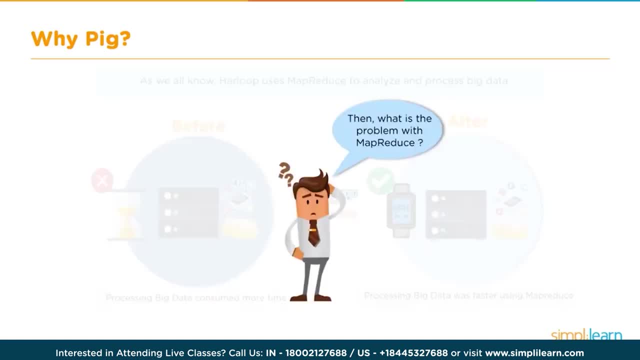 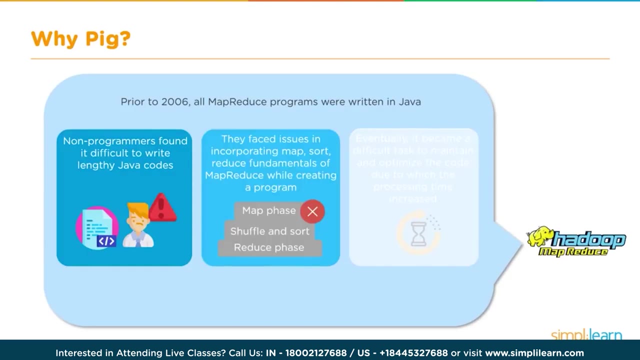 processing big data was faster using MapReduce, Then what is the problem with MapReduce? Prior to 2006,, all MapReduce programs were written in Java. Non-programmers found it difficult to write lengthy Java codes. They faced issues in incorporating map sort reduce to fundamentals. 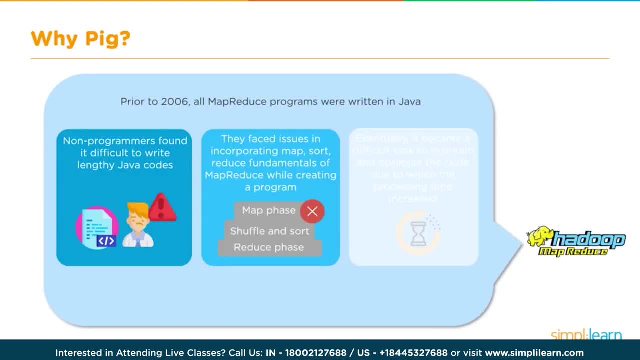 of MapReduce while creating a program. You can see here map phase, shuffle and sort reduce phase. Eventually it became a difficult task to maintain and optimize a code, due to which the processing time increased. You can imagine a manager trying to go in there and needing a simple. 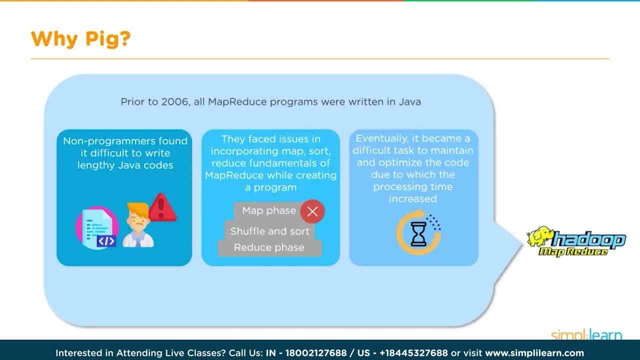 query to find out data and he has to go talk to the programmers anytime he wants anything, So that was a big problem. Not everybody wants to have an on-call programmer for every manager on their team. Yahoo faced problems to process and analyze large datasets using Java as the codes. 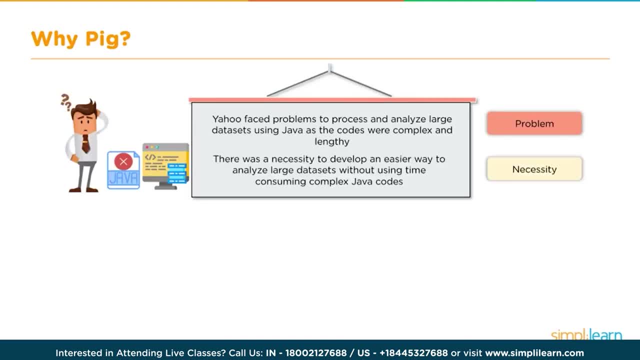 were complex and lengthy. There was a necessity to develop an easier way to analyze large datasets without using time-consuming, complex Java modes and codes and scripts and all that fun stuff. Apache Pig was developed by Yahoo. It was developed with the vision to analyze and 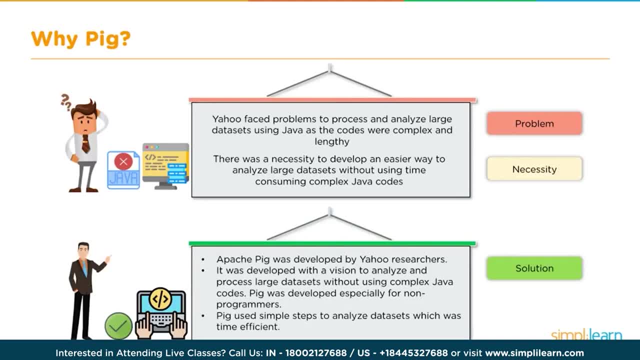 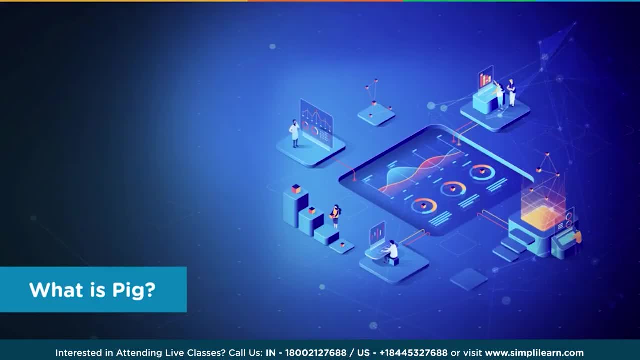 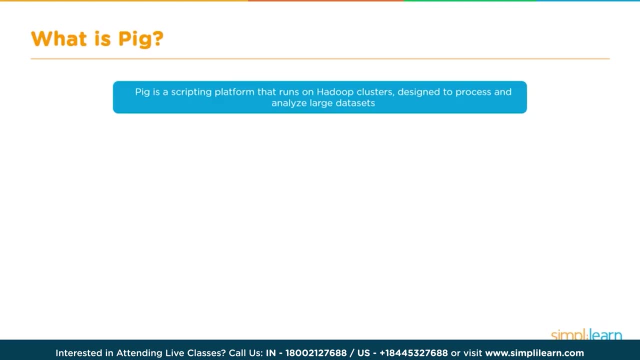 process large datasets without using complex Java codes. Pig was developed especially for non-programmers. Pig used simple steps to analyze datasets, which was time efficient. So what exactly is Pig? Pig is a scripting platform that runs on Hadoop clusters, designed to process and analyze. 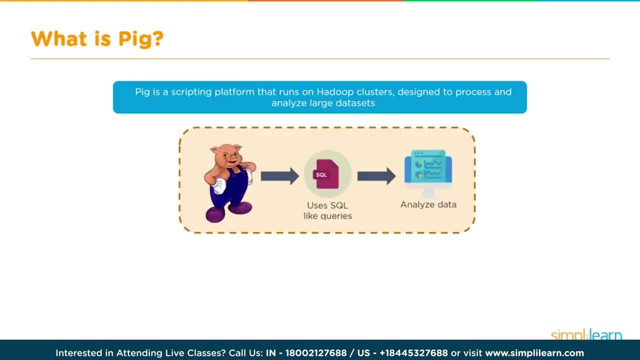 large datasets. And so you have your Pig, which uses SQL-like queries. They're definitely not SQL, but some of them resemble SQL queries- And then we use that to analyze our data. Pig operates on various types of data, like structured, semi-structured. 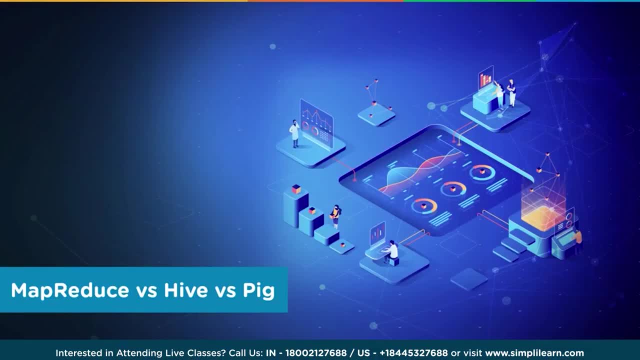 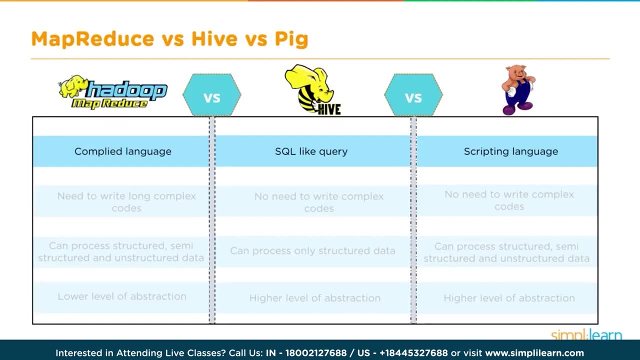 and unstructured data. Let's take a closer look at MapReduce versus Hive versus Pig. So we start with a compiled language, your MapReduce, And we have Hive, which is your SQL like query, And then we have Pig, which is a scripting language. 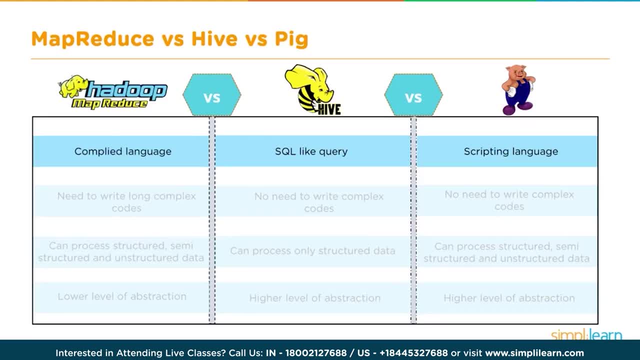 It has some similarities to SQL, but it has a lot of its own stuff. Remember: SQL, like query, which is what Hive is based off- looks for structured data, And so we get into scripting languages like Pig. now we're dealing more with structured, semi-structured and even unstructured. 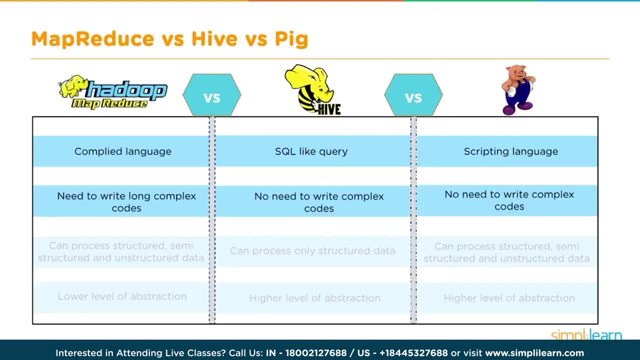 data. With a Hadoop MapReduce, we have a need to write long, complex codes. With Hive, no need to write complex codes. You could just put it in a simple SQL query or HQL, HiveQL And in Pig- no need to write complex codes. 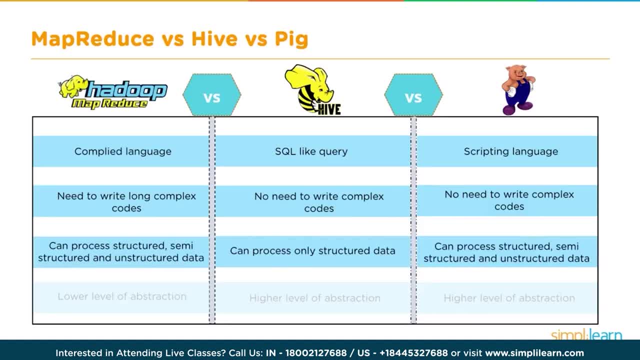 as we have Pig Latin Now remember- in the MapReduce. it can produce structured, semi-structured and unstructured data And, as I mentioned before, Hive can process only structured data. Think rows and columns, Where Pig can process structured, semi-structured. 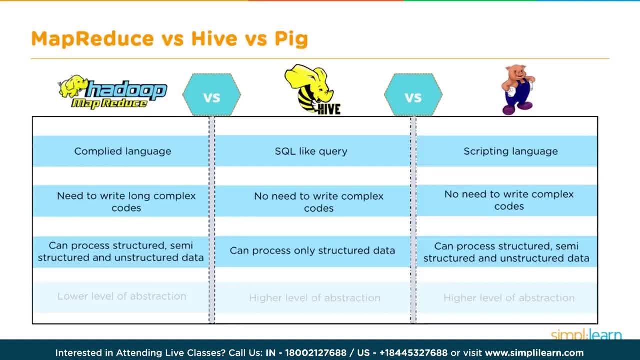 and unstructured data. You can think of structured data as rows and columns, Semi-structured as your HTML XML documents that you have on your web pages, And unstructured could be anything from groups of documents and written format. Twitter Tweets. 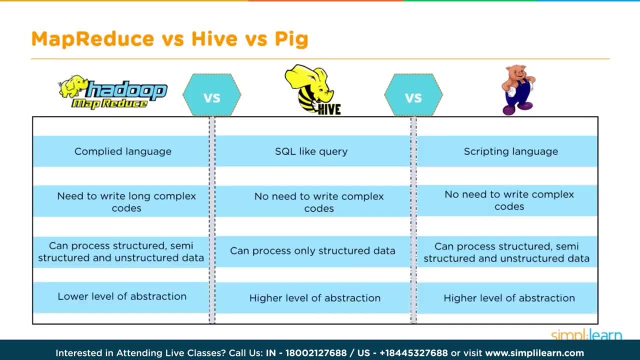 any of those things come in as very unstructured data And with our Hadoop MapReduce we have a lower level of abstraction. With both Hive and Pig we have a higher level of abstraction, So it's much more easy for someone to use without having to dive in deep. 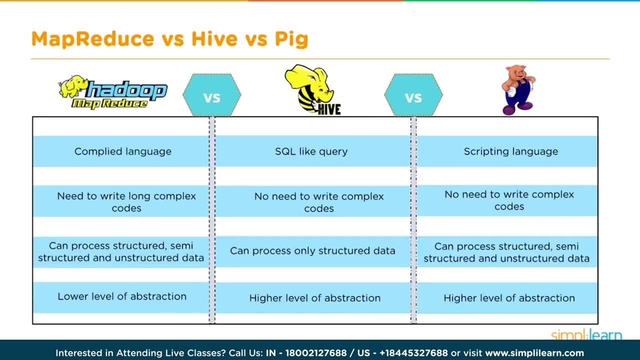 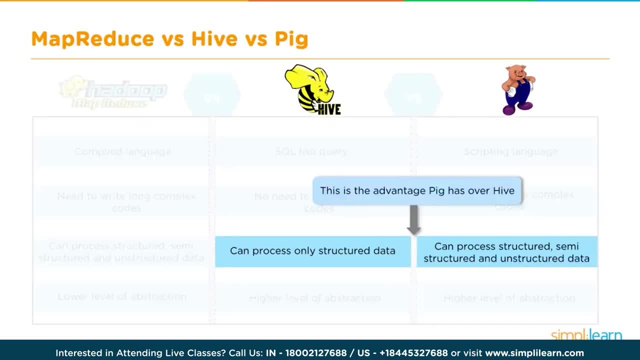 And write a very lengthy MapReduce code And those MapReduce codes can take 70, 80 lines of code, when you can do the same thing in one or two lines with Hive or Pig. This is the advantage Pig has over Hive: It can process only. 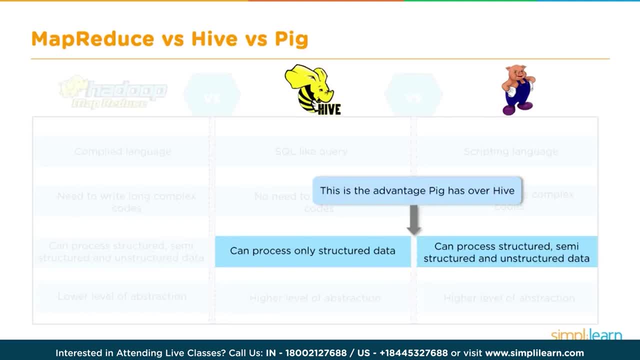 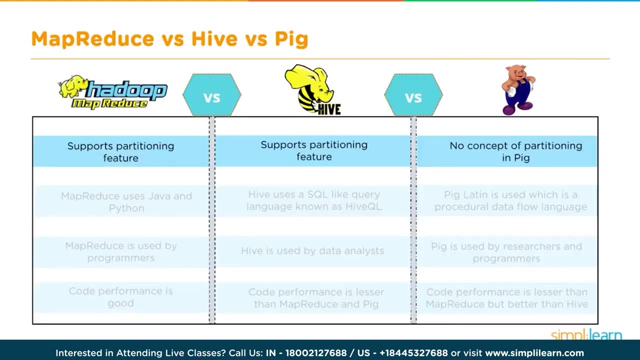 structured data in Hive, while in Pig it can process structured, semi-structured and unstructured data. Some other features to note that separates the different query languages is when we look at Map and Reduce. MapReduce supports partitioning features, as does Hive Pig. 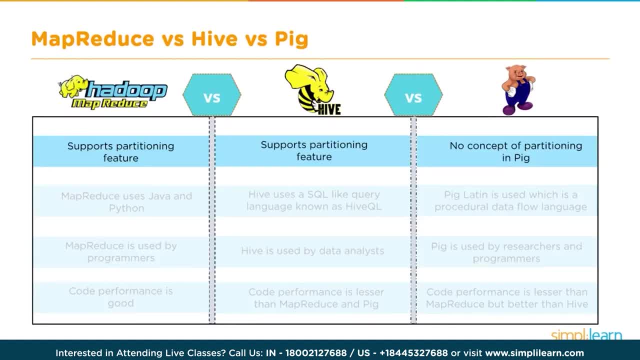 no concept of partitioning in Pig, so it doesn't support your partitioning feature. Your partitioning features allow you to partition the data in such a way that it can be queried quicker. You're not able to do that in Pig MapReduce. 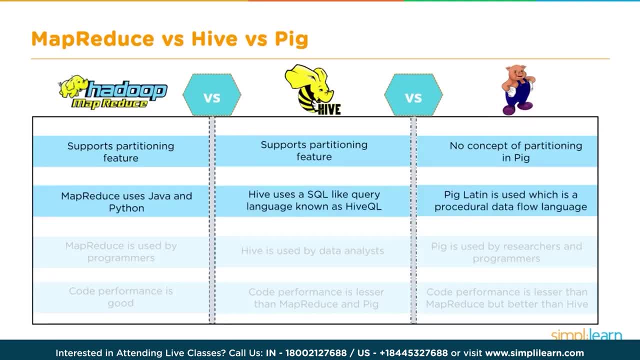 uses Java and Python, while Hive uses an SQL-like query language known as HiveQL or HQL. Pig Latin is used, which is a procedural data flow language. MapReduce is used by programmers. pretty much is straightforward on Java. Hive is used by data analysts. 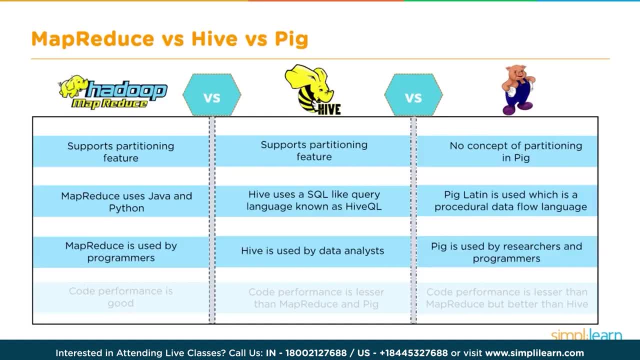 Pig is used by researchers and programmers. Certainly there's a lot of mix between all three. Programmers have been known to go in and use Hive for a quick query and anybody's been able to use Pig for a quick query or research Under Map and Reduce. 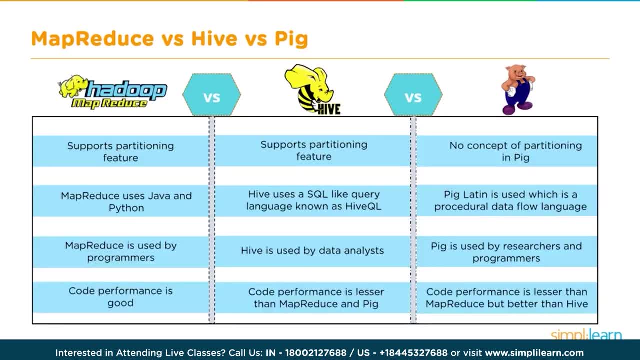 code performance is really good. Under Hive code performance is lesser than Map and Reduce and Pig. Under Pig code performance is lesser than MapReduce, but better than Hive. So if we're going to look at speed and time, the MapReduce is going. 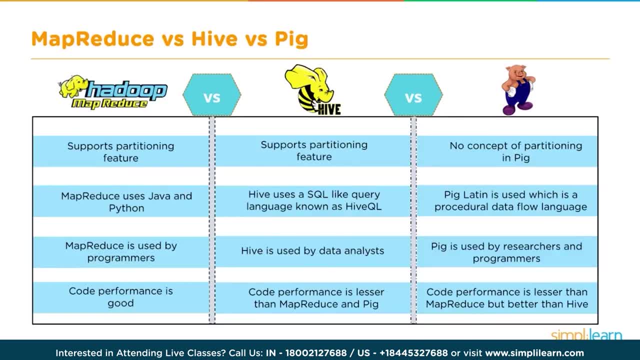 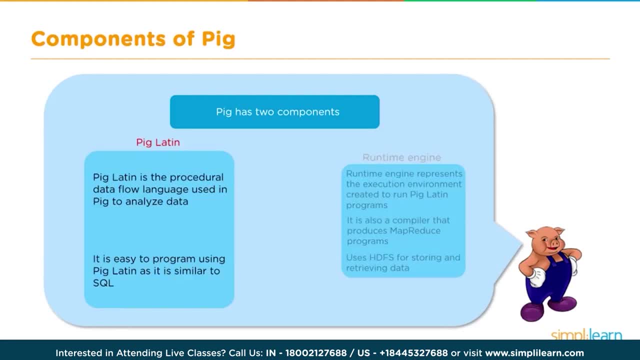 to be the fastest performance on all of those where Pig will have the second and Hive follows in the back. Let's look at components of Pig. Pig has two main components. We have Pig Latin. Pig Latin is the procedural data flow language used. 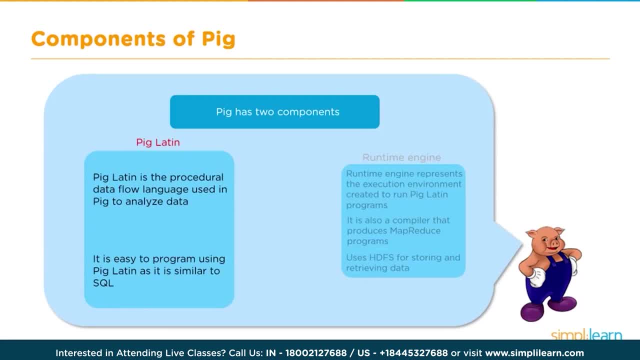 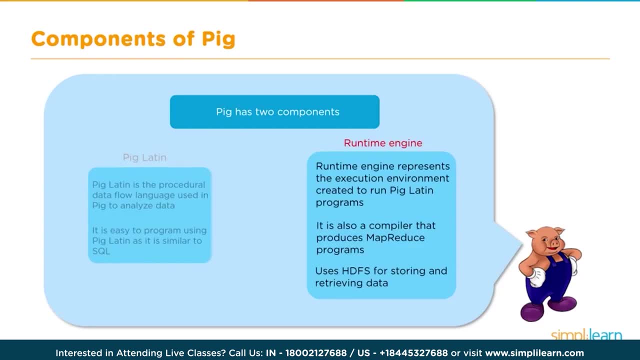 in Pig to analyze data. It is easy to program using Pig Latin. It is similar to SQL. And then we have the Runtime Engine. Runtime Engine represents the execution environment created to run Pig Latin programs. It is also a compiler that produces MapReduce programs. 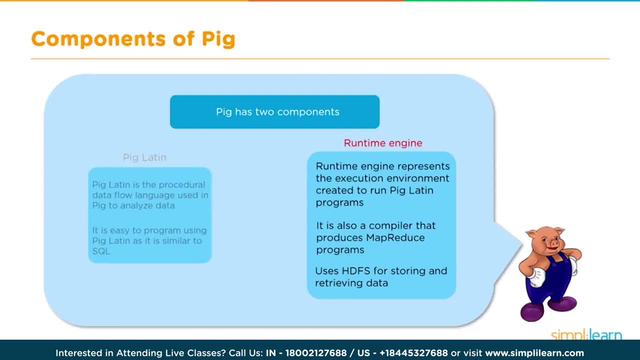 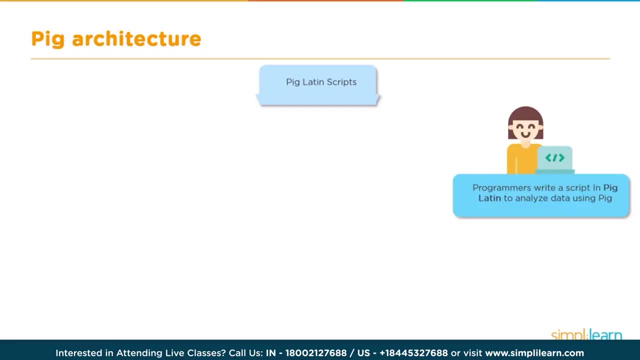 It uses HDFS or your Hadoop file system for storing and retrieving data. And as we dig deeper into Pig architecture, we'll see that we have Pig Latin scripts. Programmers write a script in Pig Latin to analyze data using Pig. Then you have the. 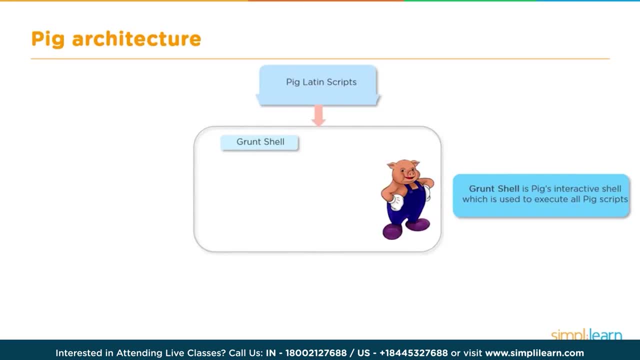 Grunt shell- And it actually says Grunt when we start it up and we'll show you that here in a little bit- which goes into the Pig server, And this is where we have our parser. Parser checks the syntax of the Pig script After checking. 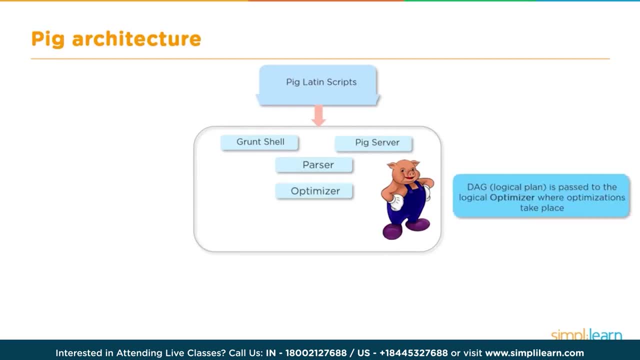 the output will be a DAG directed acylic graph, And then we have an optimizer which optimizes after your DAG. your logical plan is passed to the logical optimizer where an optimization takes place. Finally, the compiler converts the DAG into MapReduce. 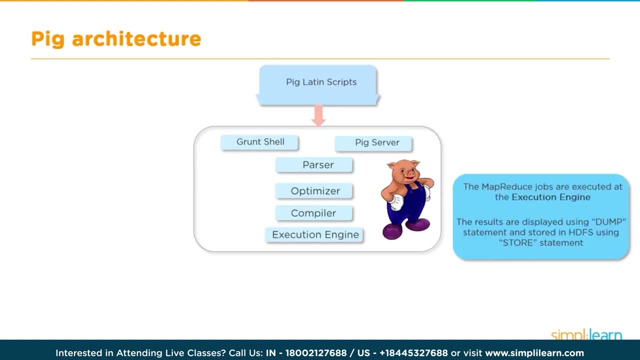 jobs, And then that is executed on the MapReduce under the execution engine. The results are displayed using dump statement and stored in HDFS using store statement. And again we'll show you that The kind of end you always want to execute. 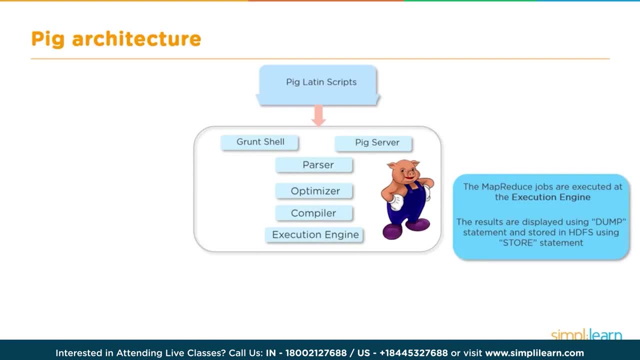 everything once you've created it, and so dump is kind of our execution statement And you can see right here, as we were talking about earlier, once we get to the execution engine and it's coded into MapReduce, then the MapReduce processes it onto the. 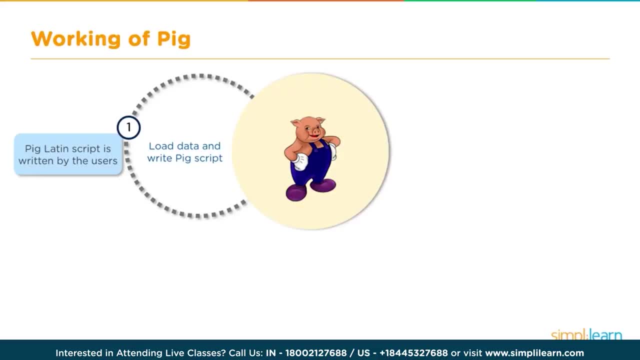 HDFS Working of Pig Pig Latin script is written by the users. So you have load data and write pig script and pig operations. So when we look at the working of pig pig Latin script is written by the users. There's step one: we load. 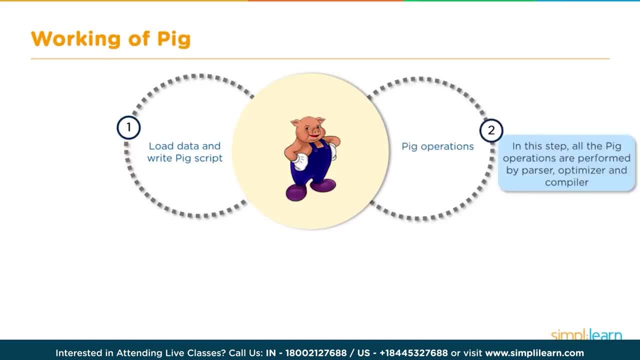 data and write pig script. And step two: in this step all the pig operations are performed by parser, optimizer and compiler. So we go into the pig operations And then we get to step three: execution of the plan. In this stage the results are shown. 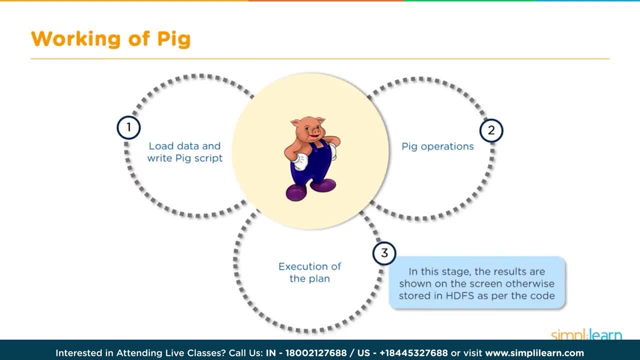 on the screen, otherwise stored in the HDFS, as per the code. So it might be: you have a small amount of data, you're reducing it to and you want to put that on the screen, Or you might be converting a huge amount of data which you want to put back into. 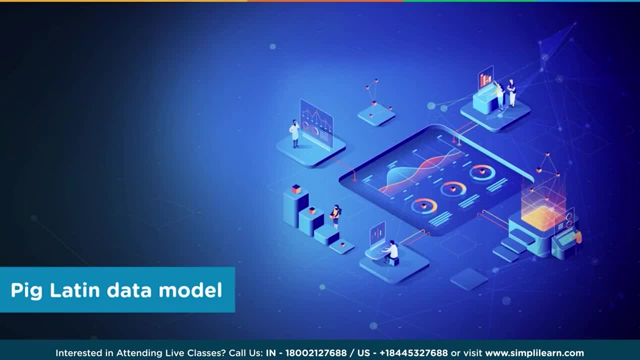 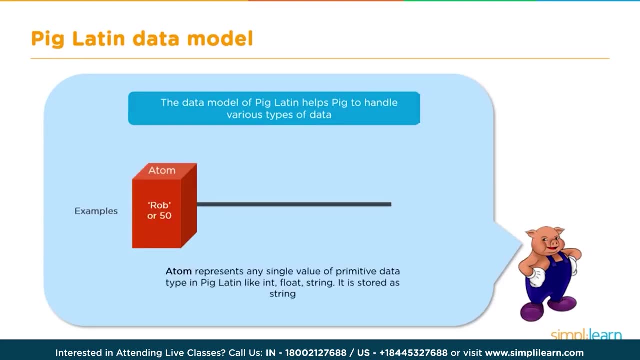 the Hadoop file system for other use. Let's take a look at the pig Latin data model. The data model of pig Latin helps pig to handle various types of data. For example, we have Adam, Rob or 50. Adam represents any single value of primitive. 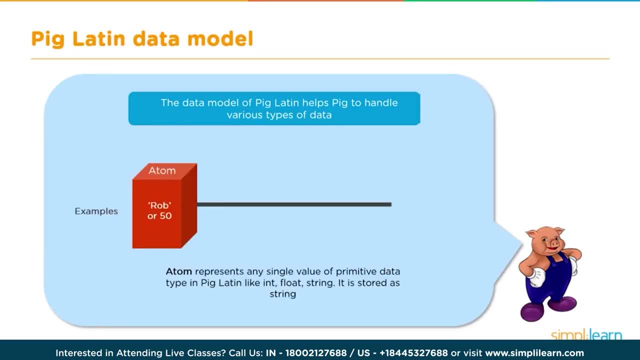 data type in pig Latin, like integer float string, It is stored as a string Tuple, so we go from our Adam, which is our most basic thing. So if you look at just Rob or just 50,, that's an. 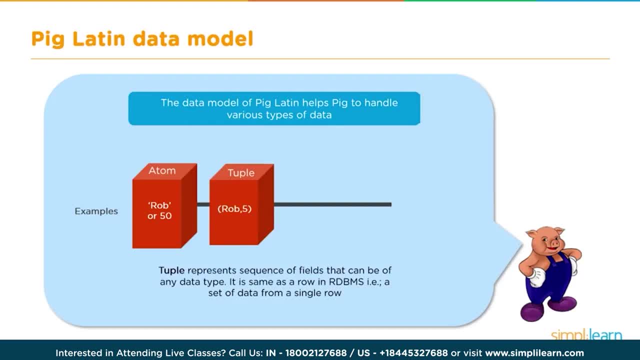 Adam. That's our most basic object we have in pig Latin. Then you have a tuple. Tuple represents sequence of fields that can be of any data type. It is the same as a row in RDBMS, For example, a set of data from a single row. 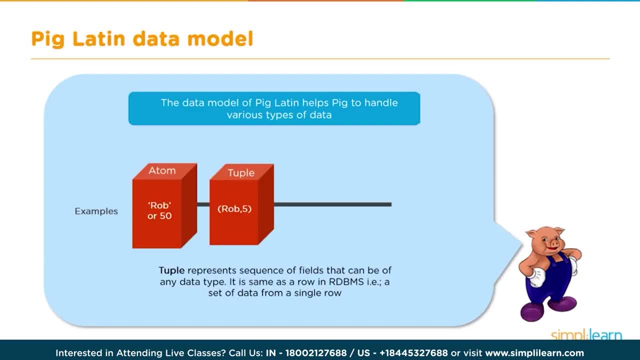 And you can see here we have Rob 5.. And you can imagine with many of our other examples we've used, you might have the ID number, the name where they live, their age, their date of starting the job. That would all be one row and stored as 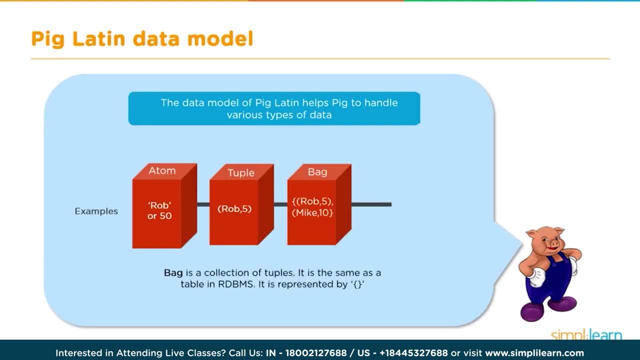 a tuple And then we create a bag. A bag is a collection of tuples. It is the same as a table in RDBMS and is represented by brackets And you can see, here we have our table with Rob 5, Mike 10.. 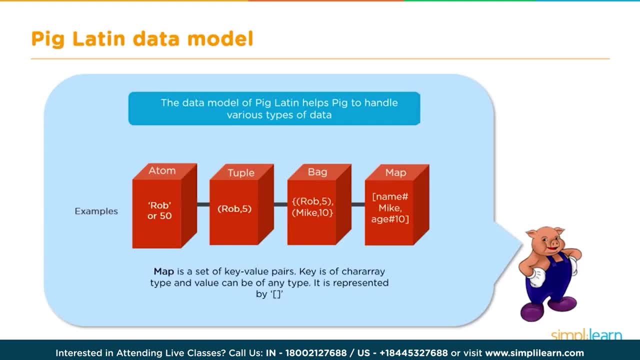 And we also have a map. A map is a set of key-value pairs. Key is of character, array, type, and a value can be of any type. It is represented by the brackets, And so we have name and age, where the key value is Mike and 10.. 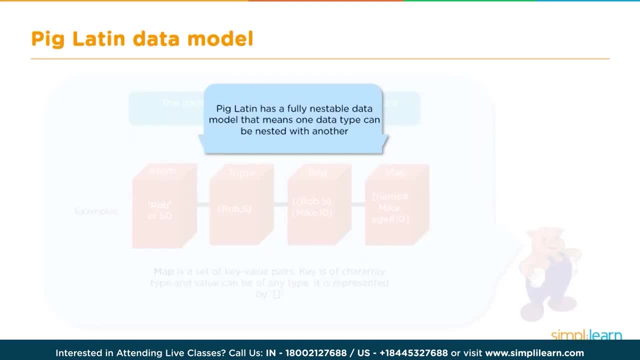 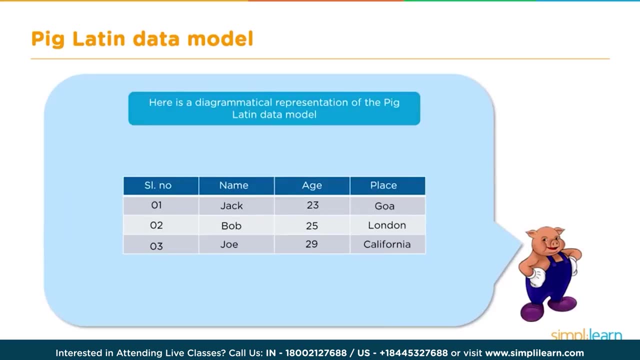 Pig Latin has a fully nestable data model. That means one data type can be nested within another. Here's a diagram representation of Pig Latin data model And in this particular example we have basically an ID number, a name, an age. 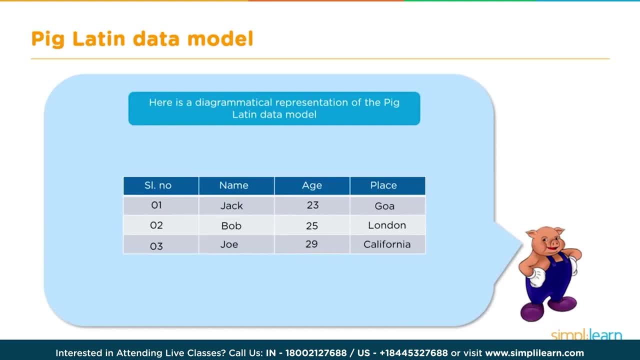 and a place And we break this apart and we look at this model from Pig Latin perspective. We start with our field And, if you remember, a field contains basically an atom. It is one particular data type And the atom is stored as a string. 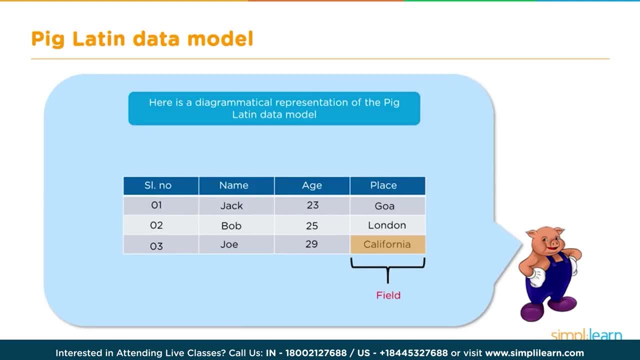 which then converts it into either an integer number or character string. Next, we have our tuple, And in this case you can see that it represents a row. So our tuple would be 3, Joe 29,, California. And finally, we have our bag. 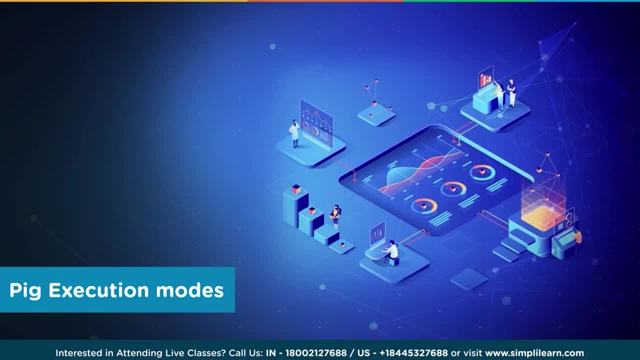 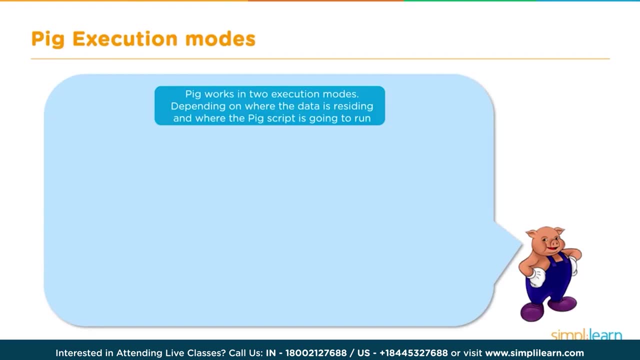 which contains three rows in it. in this particular example, Let's take a quick look at pig execution modes. Pig works in two execution modes, depending on where the data is residing and where the pig script is going to run. We have local mode Here the pig engine takes 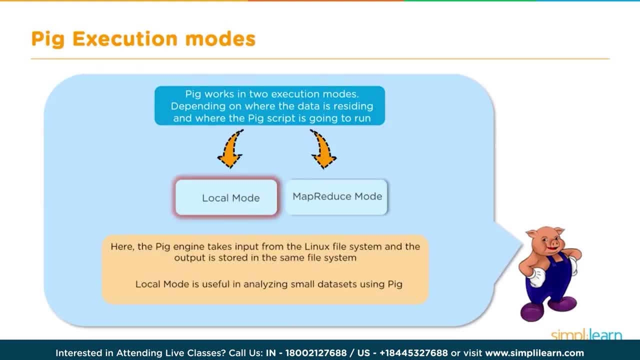 input from the Linux file system and the output is stored in the same file system- Local mode. Local mode is useful in analyzing small data sets using Pig, And we have the MapReduce mode Here. the pig engine directly interacts and executes in HDFS. 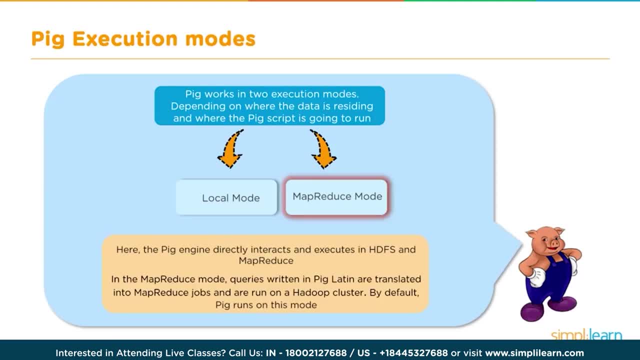 and MapReduce. In the MapReduce mode, queries written in Pig Latin are translated into MapReduce jobs and are run on a Hadoop cluster. By default, Pig runs in this mode. There are three modes in Pig, depending on how a Pig Latin. 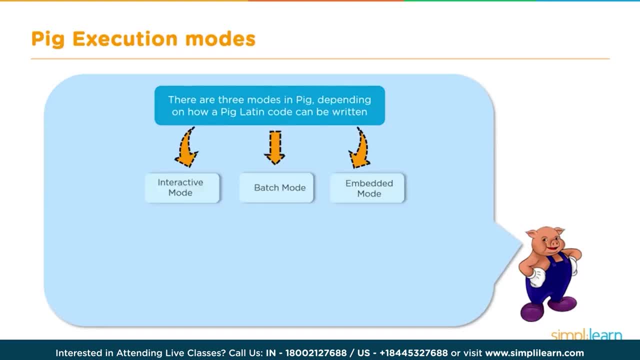 code can be written. We have our interactive mode, batch mode and embedded mode. The interactive mode means coding and executing the script line by line. When we do our example, we'll be in the interactive mode. In batch mode, all scripts are coded in a file. 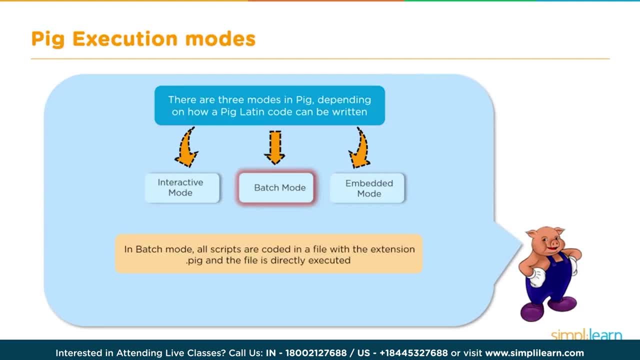 with the extension pig, and the file is directly executed. And then there's embedded mode. Pig lets its users define their own functions, UDFSs, in a programming language such as Java. So let's take a look and see how this works in a 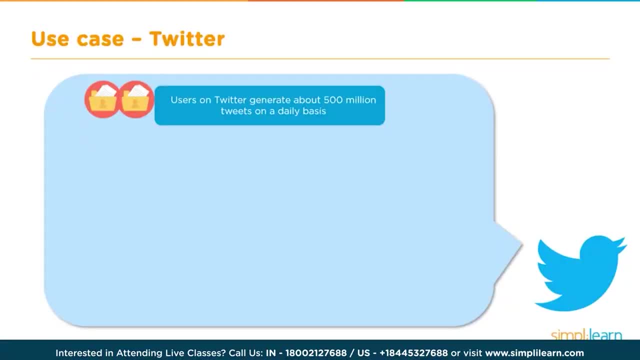 use case. In this case, use case Twitter. Users on Twitter generate about 500 million tweets on a daily basis. The Hadoop MapReduce was used to process and analyze this data. Analyzing the number of tweets created by a user in the tweet table was done using MapReduce. 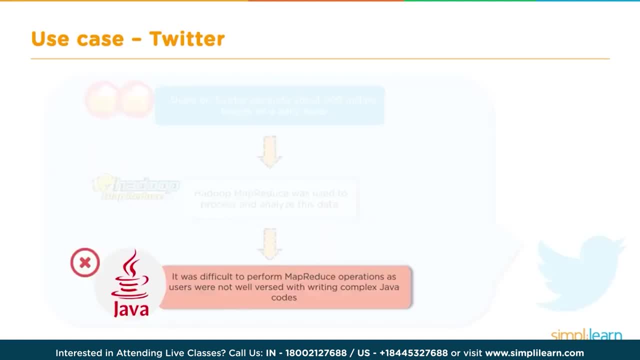 in Java programming language And you can see the problem. It was difficult to perform MapReduce operations as users were not well versed with written, complex Java codes. So Twitter used Apache Pig to overcome these problems, And let's see how. Let's start with the problem statement. 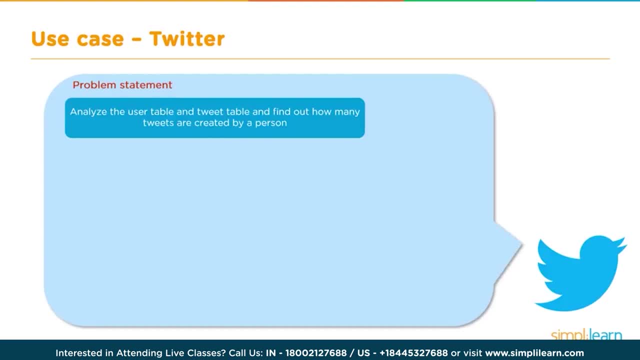 Analyze the user table and tweet and find out how many tweets are created by a person. And here you can see we have a user table. We have Alice, Tim and John with their ID numbers One, two, three And we have a tweet table In the tweet table. 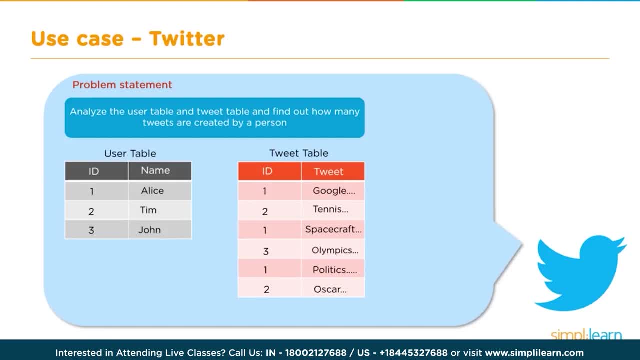 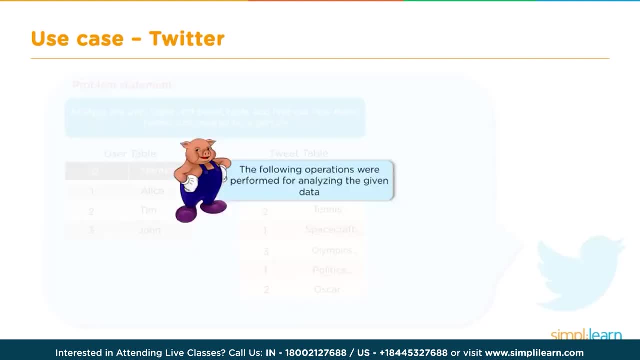 you have the ID of the user and then what they tweeted. Google was a good, whatever it was: tennis, dot dot dot, spacecraft, Olympics, politics, whatever they're tweeting about. The following operations were performed for analyzing given data: First, the Twitter. 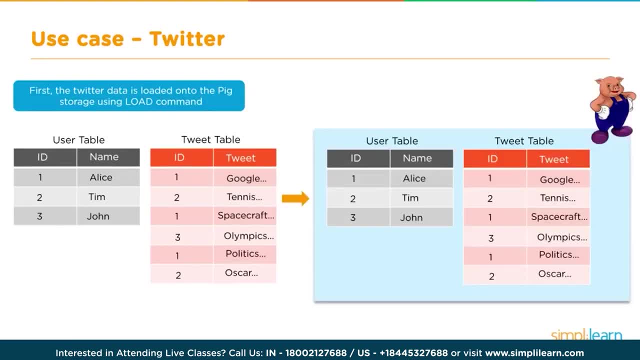 data is loaded into the pig storage using load command And you can see here we have our data coming in and the Nesco is going into pig storage And this data is probably on an enterprise computer. So this is actually active Twitter's going on and then it goes into Hadoop. 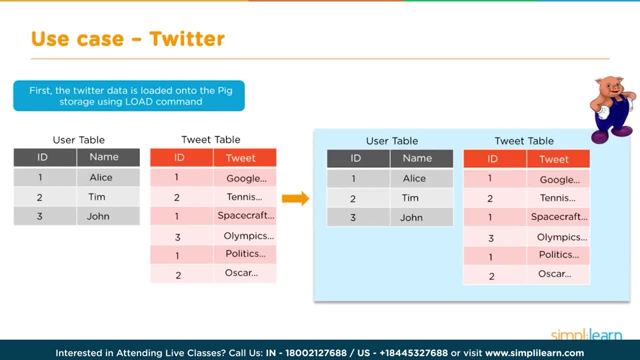 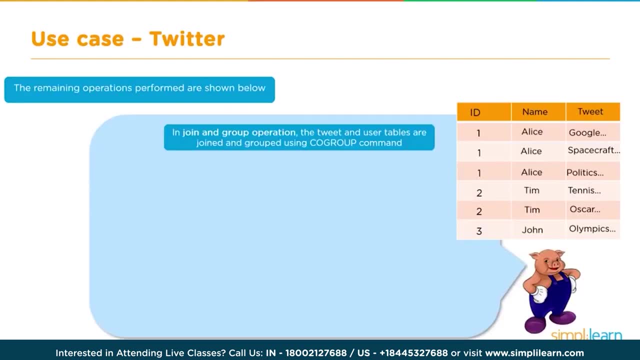 file system. Remember, the Hadoop file system is a data warehouse for storing data, And so the first step is we want to go ahead and load it into the pig storage, into our data storage system. The remaining operations performed are shown below In join. 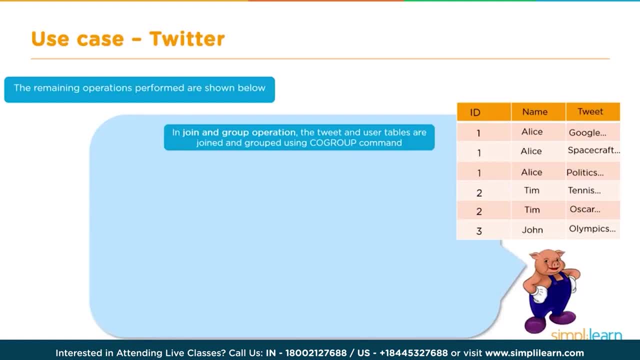 and group operation. the tweet and user tables are joined and grouped using co-group command And you can see here where we add a whole column when we go from user names and tweet to the ID linked directly to the name. So Alice was user one, Tim was. 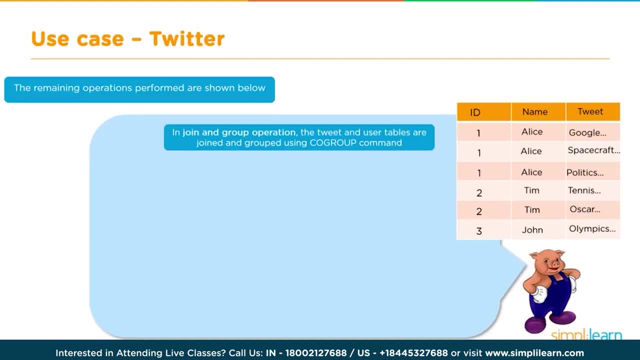 two and John three, And so now they're listed with their actual tweet. The next operation is the aggregation. The tweets are counted according to the names. The command used is count. So it's very straight forward. We just want to count how many tweets. 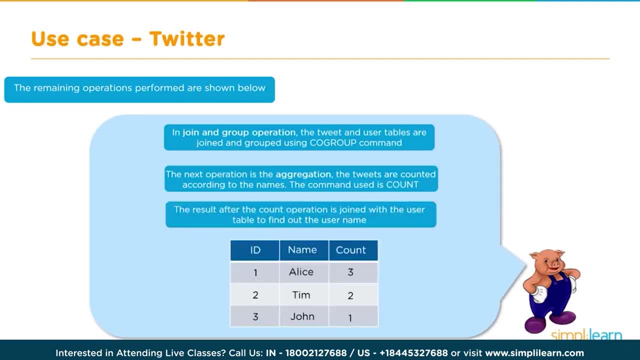 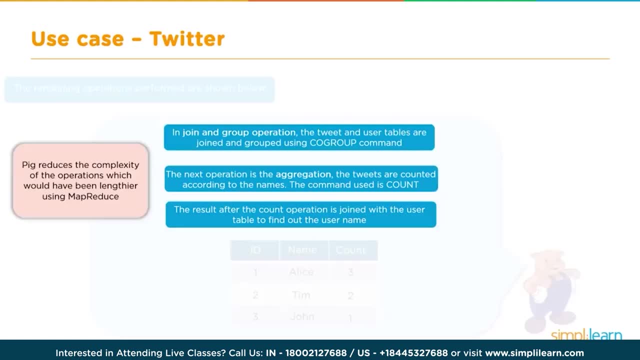 each user is doing And finally the result after the count operation is joined with the user table to find out the user name, And you can see here where Alice had three, Tim two and John one Pig reduces the complexity of the operations which would have been. 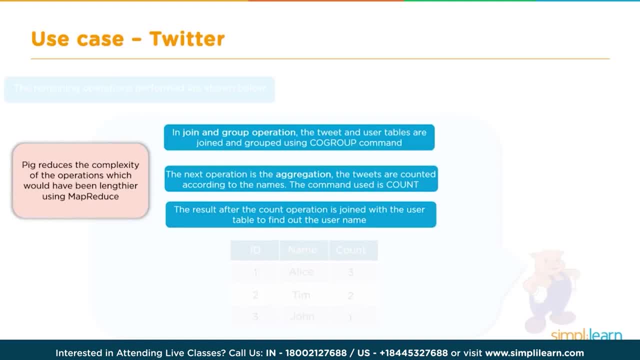 lengthy using MapReduce. In join and group operation, the tweet and user tables are joined and grouped using co-group command. The next operation is the aggregation. The tweets are counted according to the names. The command used is count. The result after the count. 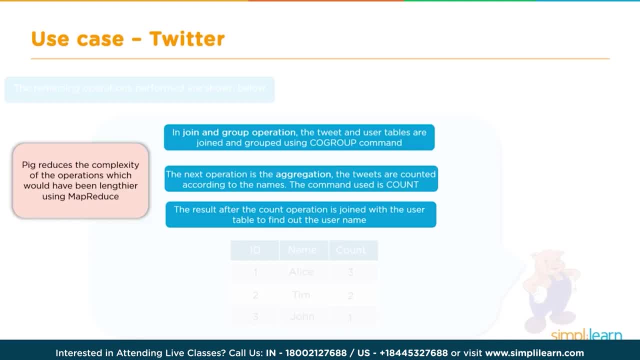 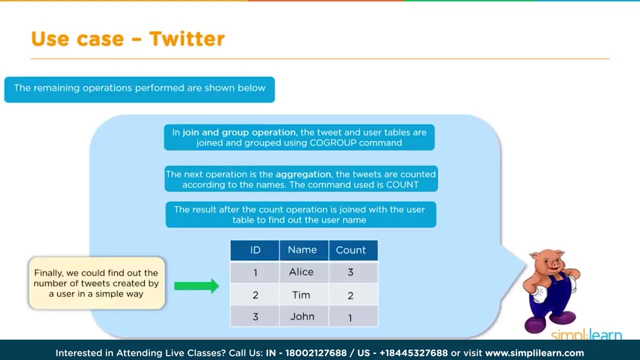 operation is joined with the user table to find out the user name And you can see we're talking about three lines of script versus a MapReduce code of about 80 lines. Finally, we could find out the number of tweets created by a user. 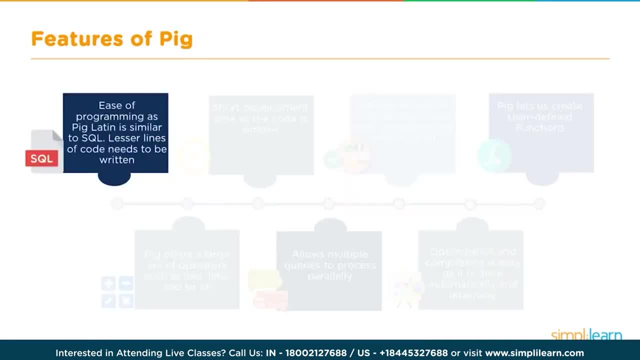 in a simple way. So let's go quickly over some of the features of Pig that we already went through. most of these, First, ease of programming. as Pig Latin is similar to SQL, Lesser lines of code need to be written. Short development time, as the code is. 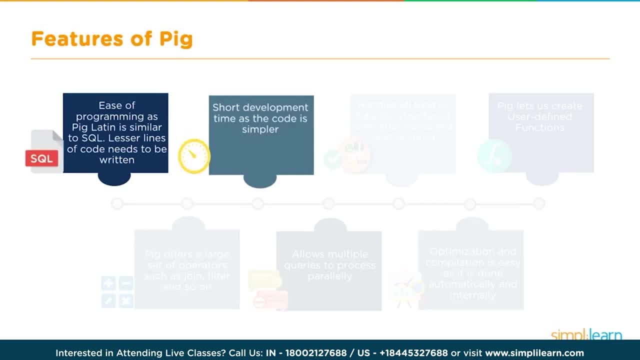 simpler So we can get our queries out rather quickly instead of having to have a programmer spend hours on. it Handles all kind of data, like structured, semi-structured and unstructured. Pig lets us create user defined functions. Pig offers a large set of operators, such as join. 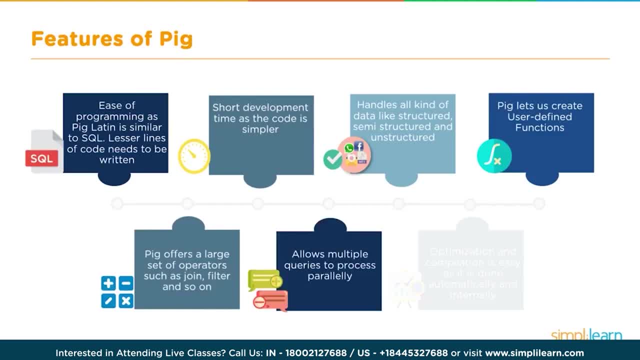 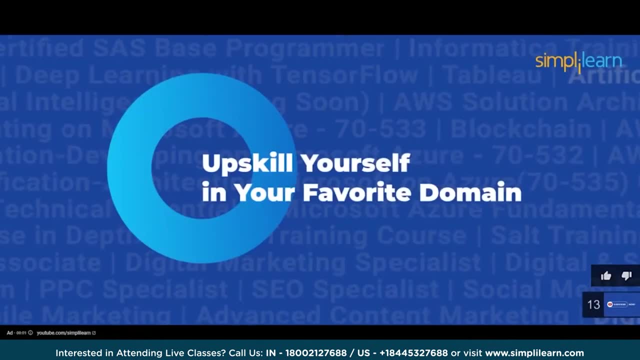 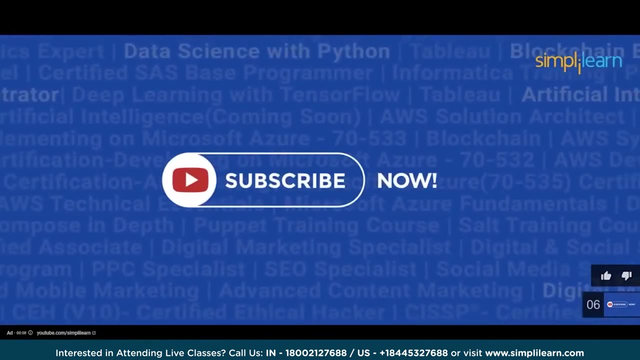 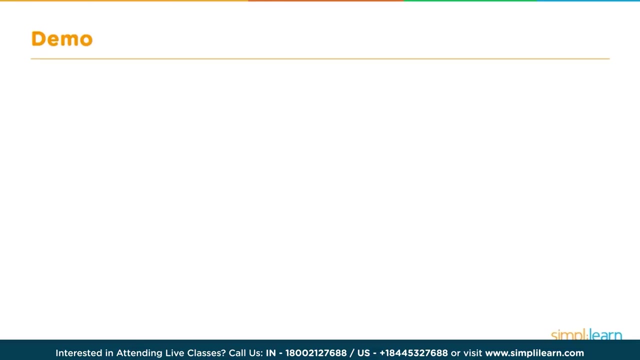 filter and so on. It allows for multiple queries to process, unparallel, And optimization and compilation is easy, as it is done automatically and internally. So enough theory, Let's dive in and show you a quick demo on some of the commands you can do and pick. 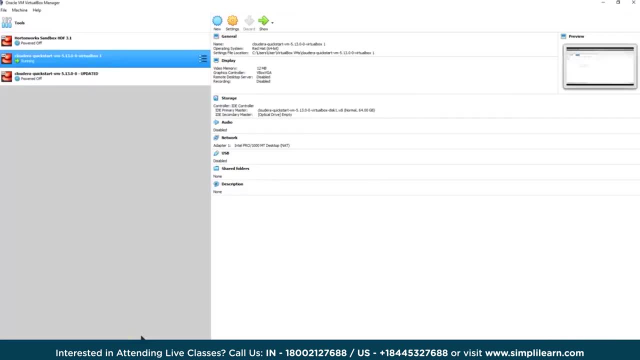 Today's setup will continue as we have in the last three demos, to go ahead and use Cloudera Quickstart, And we'll be doing this in VirtualBox. We do have a tutorial in setting that up. You can send a note to our Simply Learn team and they can. 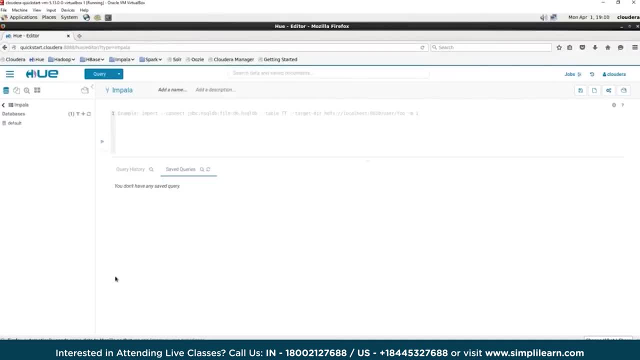 get that link to you Once your Cloudera Quickstart has spun up. and remember, this is VirtualBox. We've created a virtual machine and this virtual machine is CentOS Linux. Once it's spun up, you'll be in a full Linux system. 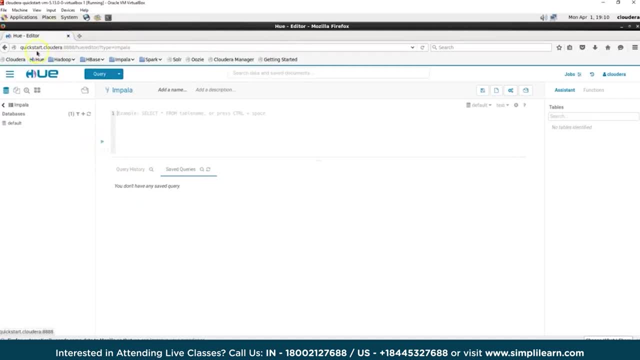 here And, as you can see, we have Thunderbird Browser, which opens up to the Hadoop Basic System Browser, And we can go underneath the hue where it comes up by default. If you click on the pull-down menu and go under Editor, you can see there's. 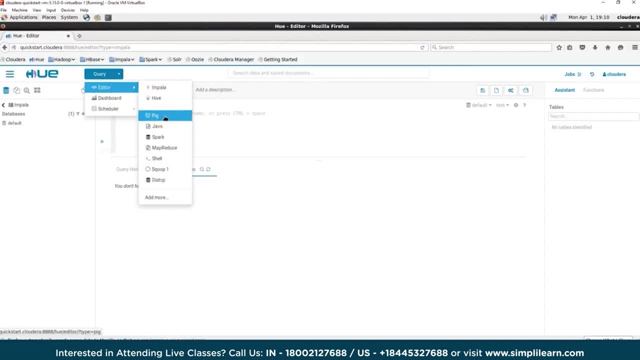 our Impala, our Hive Pig, along with a bunch of other query languages you can use And we're going under Pig And then, once you're in Pig, we can go ahead and use our command line here and just click that little. 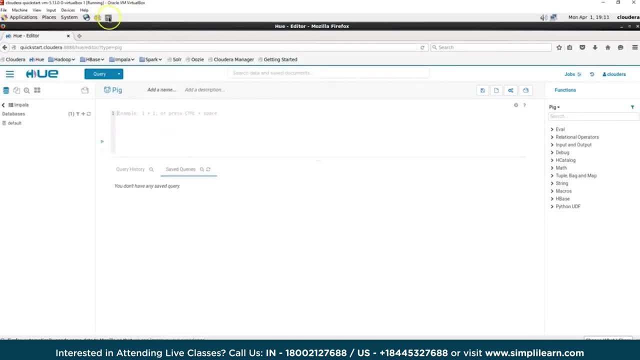 blue button to start it up and running. We will actually be working in Terminal Window And so if you were in the Cloudera Quickstart, you can open up the Terminal Window up top, or if you're in your own setup and you're logged in. 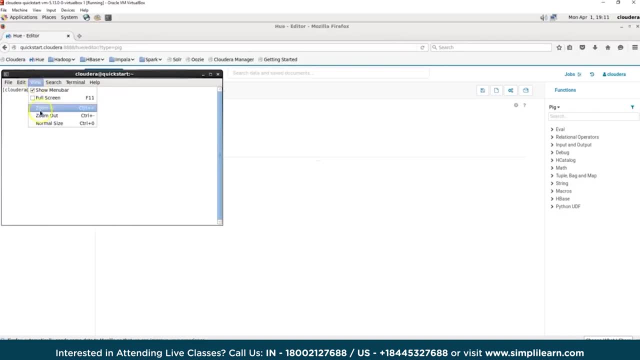 you can easily use all of your commands here in Terminal Window And we'll zoom in. that way you get a nice view of what's going on There. we go Now for our first command. we're going to go ahead and do a Hadoop command and import. 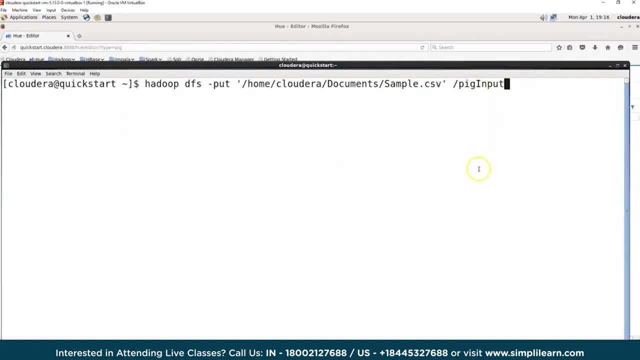 some data into the Hadoop system, in this case a Pig input. And let's just take a look at this. We have Hadoop Now let's just know it's going to be a Hadoop command, It's going to be a DFS. There's actually four variations. 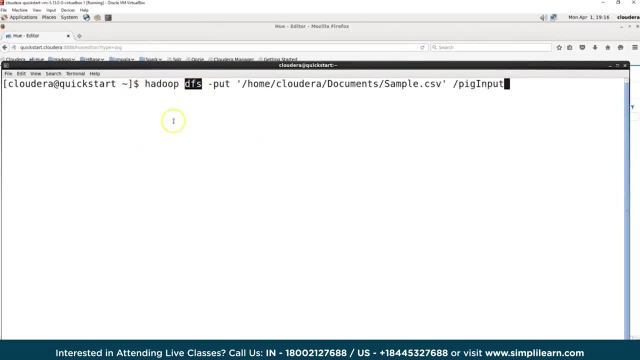 of DFS. So if you have HDFS or whatever, that's fine. All four of them used to be different setups underneath different things, and now they all do the same thing, And we want to put this file, which in this case is: 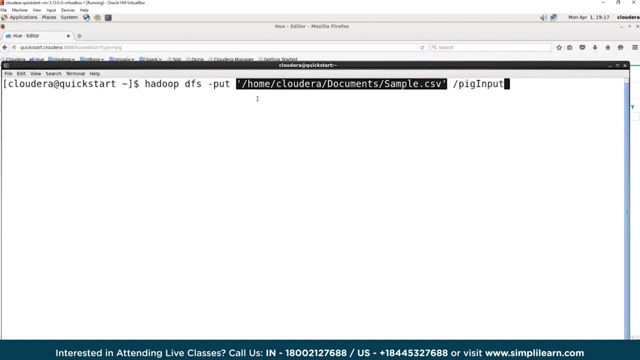 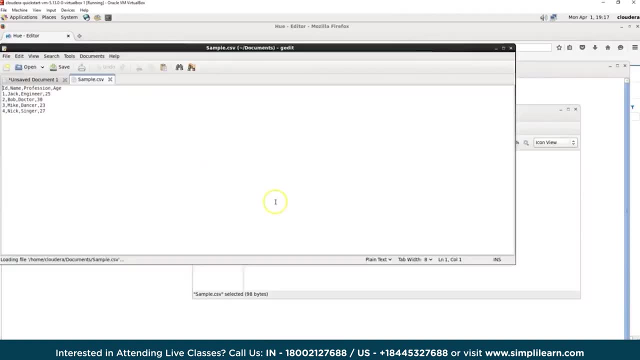 under Home, Cloudera Documents and Sample, And we just want to take that and put it into the Pig input And let's take a look at that file. If I go into my document browsers and open this up, you'll see it's got a simple. 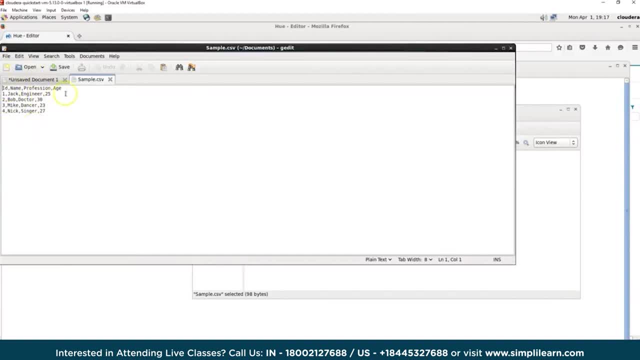 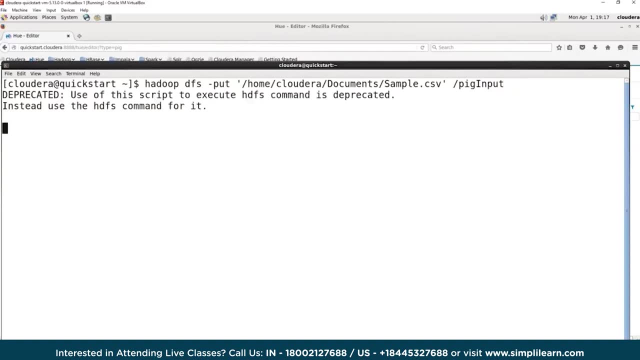 ID Name, Profession and Age. We have 1, Jack Engineer 25. And that was in one of our earlier things we had in there, And so let's go ahead and hit enter and execute this, And now we've. 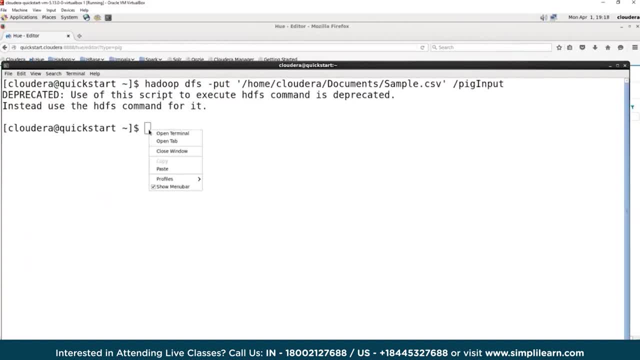 uploaded that data and it's gone into our Pig input. And then a lot of the Hadoop commands mimic the Linux commands And so you'll see we have cat as one of our commands Or it has a hyphen before it. So we execute that with Hadoop DFS. 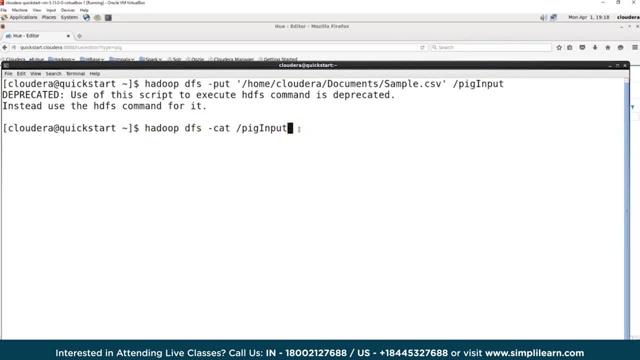 hyphen: cat slash pig input, because that's what we called it. That's where we put our sample CSV and we execute this. You can see from our Hadoop system it's going to go in and pull that up And sure enough, it pulls out. 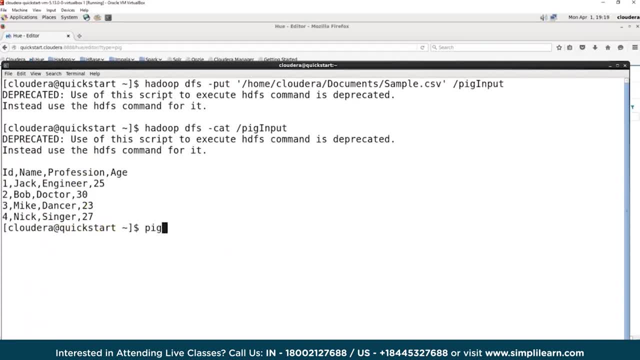 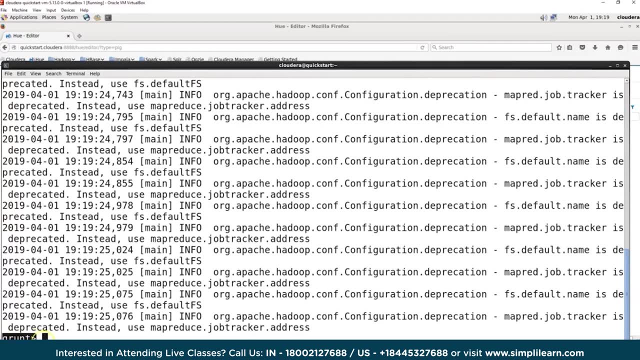 the data file we just put in there And then we can simply enter the pig latin or pig editor mode by typing in pig And we can see here. by our grunt- I told you that's how it was going to tell you you were in pig latin. 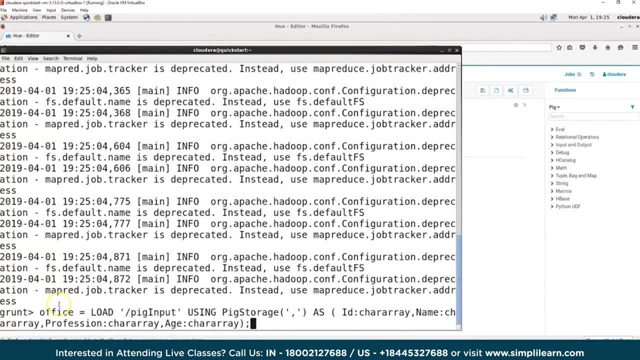 There's our grunt command line. So we are now in the pig shell, And then we'll go ahead and put our load command in here, And the way this works is I'm going to have office equals load, And here's my load. In this case it's going to be pig. 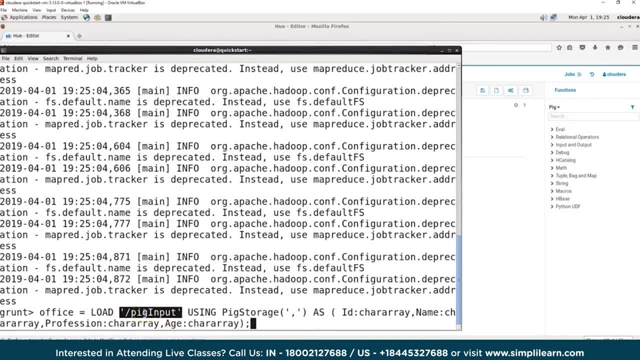 input. We have that in single brackets. You remember that's where the data is in the Hadoop file system, where we dumped it into there. We're going to be using pig storage. Our data was separated as with a comma, So there's our comma separator. 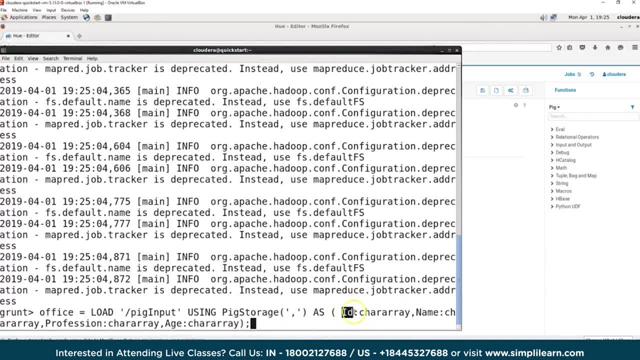 And then we have as- And in this case we have an ID character array, name character array, profession character array and age character array, And we're just going to do them all as character arrays, just to keep this simple for this one. 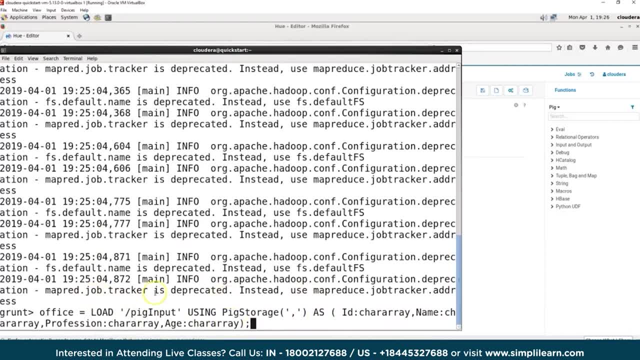 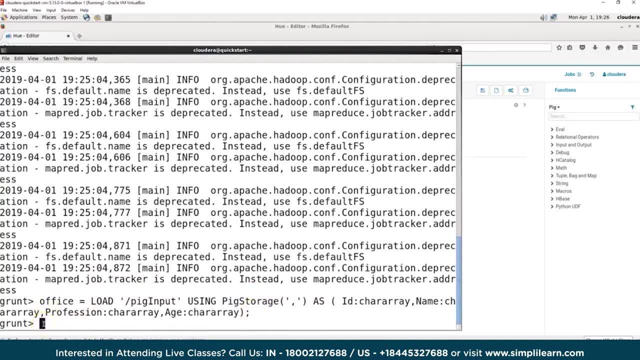 And then when I hit put this all in here, you can see that's our full command line going in And we have our semicolon at the end. So when I hit enter, it's now set office up, But it hasn't actually done anything. 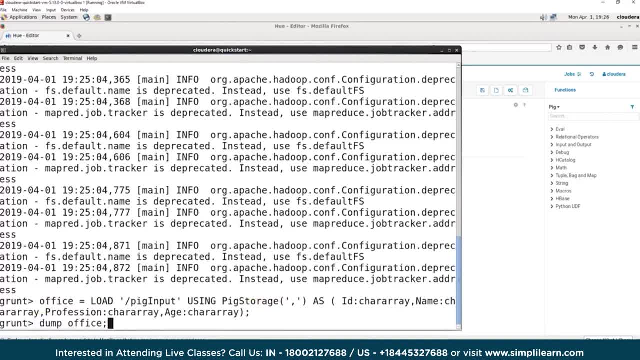 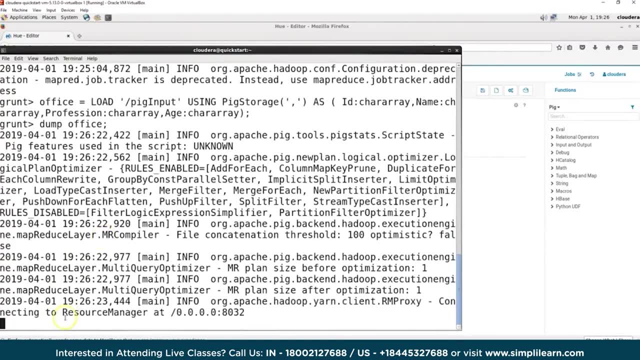 yet It doesn't do anything until we do dump office. So there's our command to execute whatever we've loaded or whatever setup we have in here And we run that. You can see it go through the different languages And this is going through the MapReduce, Remember. 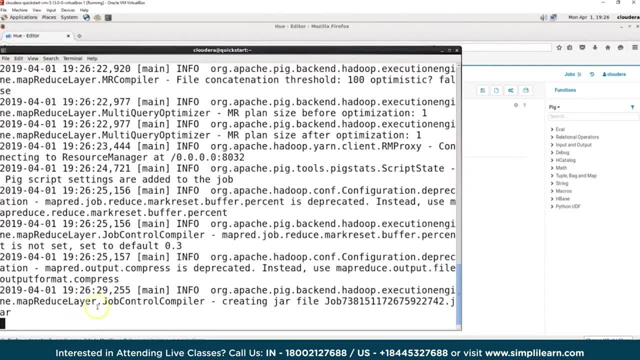 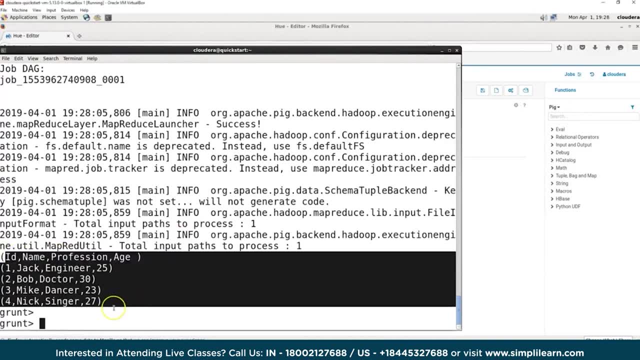 we're not doing this locally, We're doing this on the Hadoop setup And once we've finished our dump, you can see we have ID name, profession, age and all the information that we just dumped into our pick. We can now do, let's say, 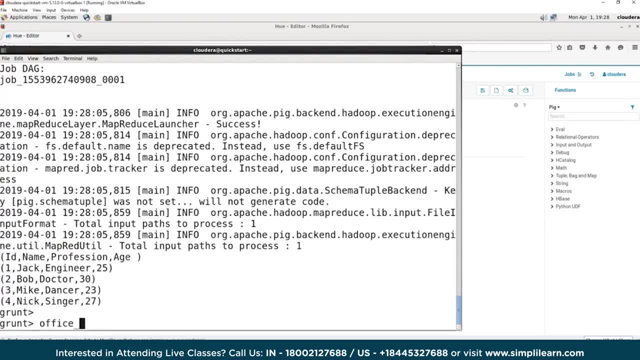 oh, let's say we have a request just for- we'll keep it simple in here, but just for the name and age, And so we can go office. We'll call it each as our variable Underscore each And we'll say: 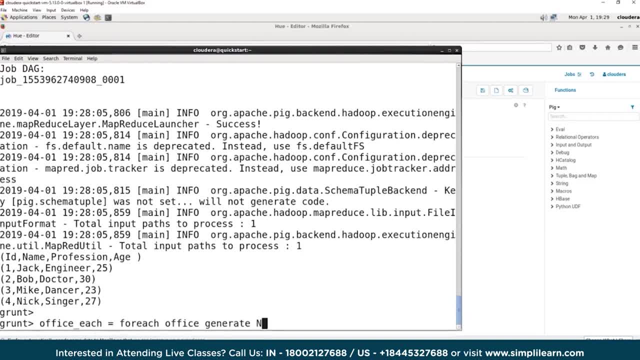 for each office, generate name, comma, age And for each means that we're going to do this for each row And if you're thinking MapReduce, you know that this is a map function Because it's mapping each row and generating name and age on here. 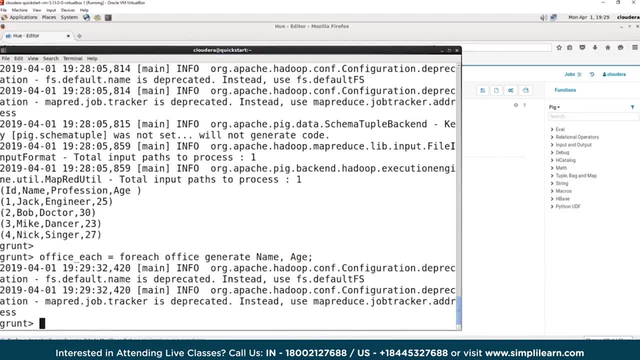 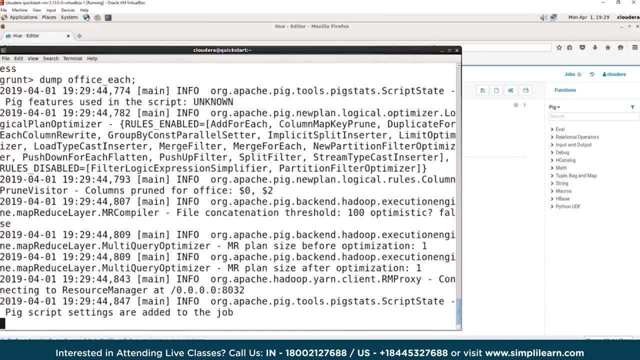 And of course, we want to go ahead and close it with a semicolon And then, once we've created our query or the command line in here, let's go ahead and dump office underscore each in with our semicolon And this will go through our MapReduce. 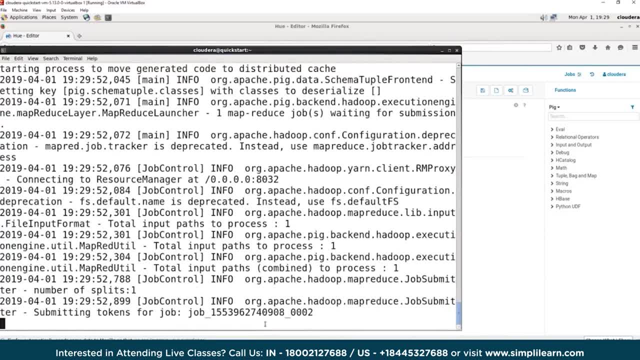 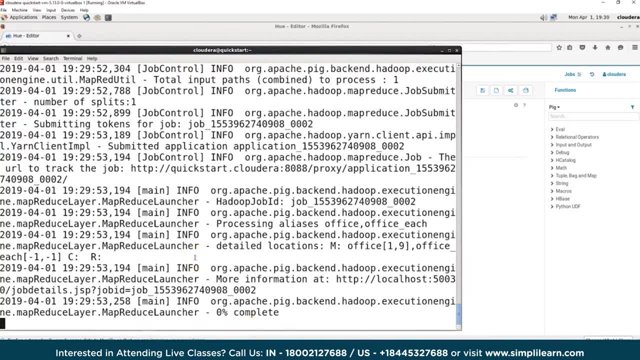 setup on here, And if we were on a large cluster, the same processing time would happen. In fact, it's really slow because I have multiple things on this computer and this particular virtual box is only using a quarter of my processor. It's only. 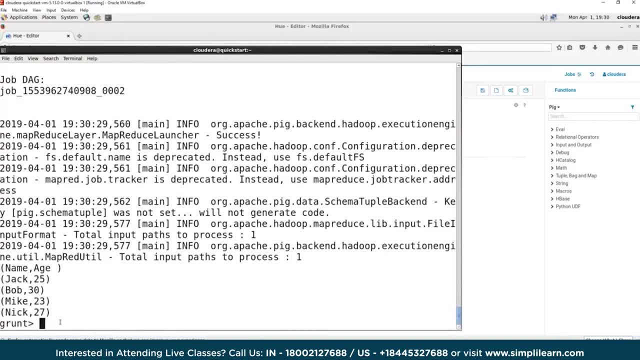 dedicated to this And you can see here. there it is name and age, And it also included the top row, since we didn't delete that out of there or tell it not to, And that's fine for this example, But you need to be aware of those things when you're processing. 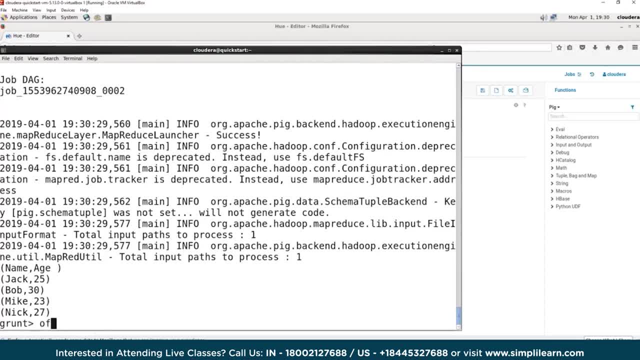 a significantly large amount of data or any data, And we can also do office and we'll call this DSC for descending. So maybe the boss comes to you and says, hey, can we order office by ID descending, And of course your boss, you've. 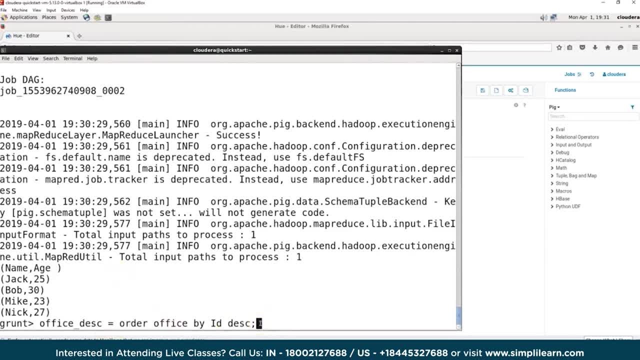 taught them how to your shareholder. sounds a little derogatory when I say: boss, You've talked to the shareholder and you said: and you've taught them a little bit of pig Latin, and they know that they can now create office description And we can order office by ID. 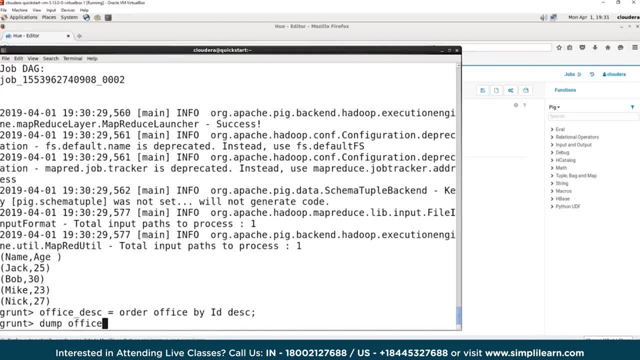 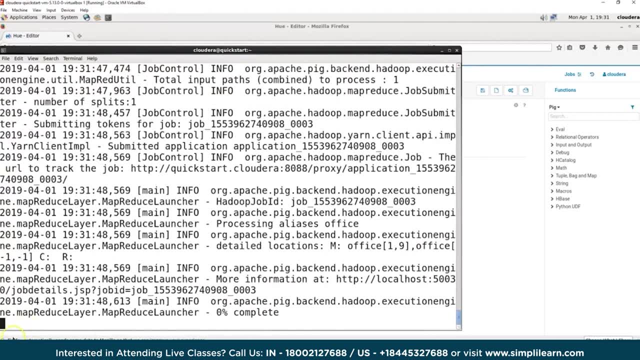 description. And of course, once we do that, we have to dump office underscore description so that it'll actually execute. And there it goes into our MapReduce. It'll take just a moment for it to come up because again, I'm running on only a quarter of my. 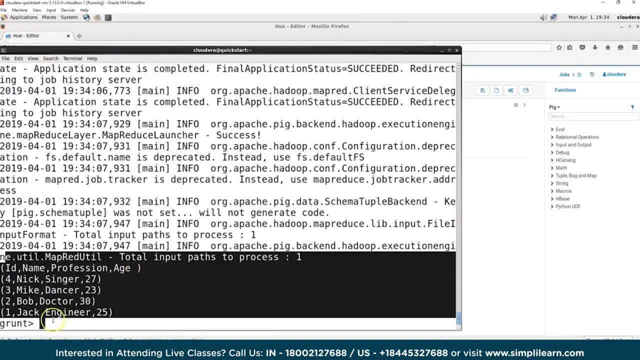 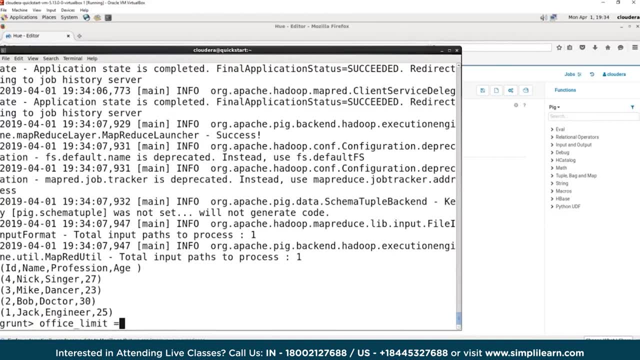 processor And you can see. we now have our IDs, in descending order, returned. Let's also look at- and this is so important with any time you're dealing with big data. Let's create office with a limit, And you can, of course, do any of this instead. 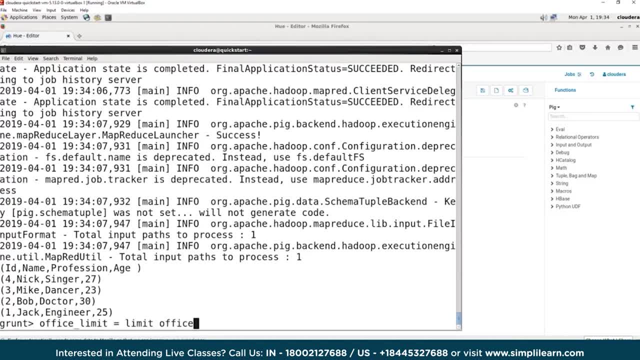 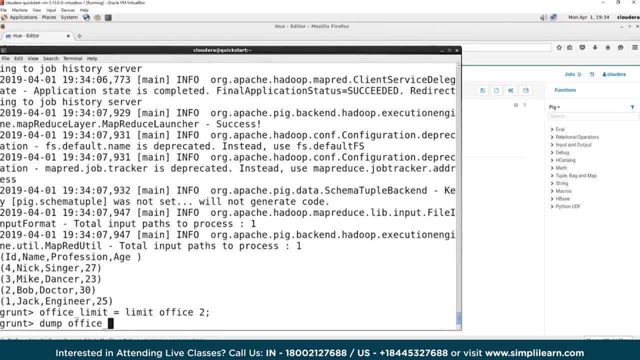 of with office. we could do this with office descending so you get just the top two IDs on there. But we're going to limit just to two And of course, to execute that we have to dump office underscore limit And you can just think of dumping your garbage. 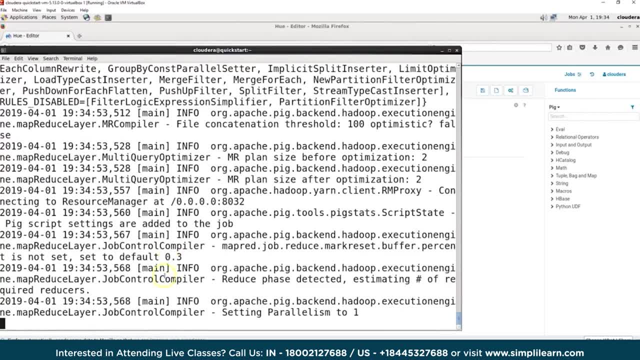 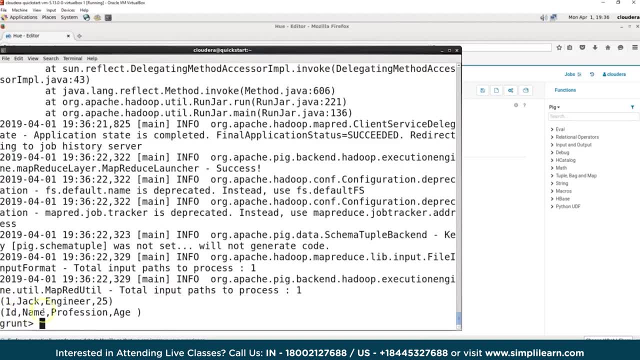 into the pig pen for the pig to eat. There we go, Dump office limit two And that's going to just limit our office to the top two. And for our output we get our first row which had our ID name, profession and 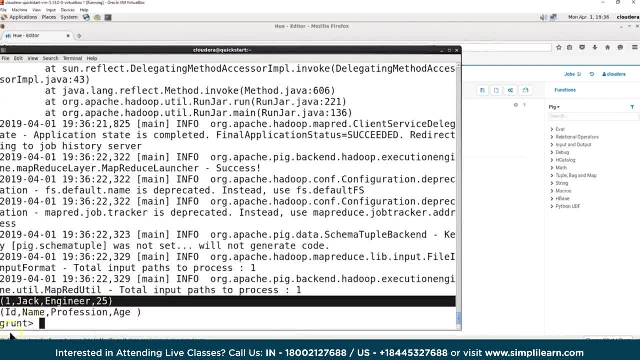 age, And our second row, which is Jack, who's an engineer. Now let's do a filter. We'll call it office underscore filter. You guessed it: Equals. filter office by profession: equals. And keep note, this is similar to how Python does it with the double equal signs for equal. 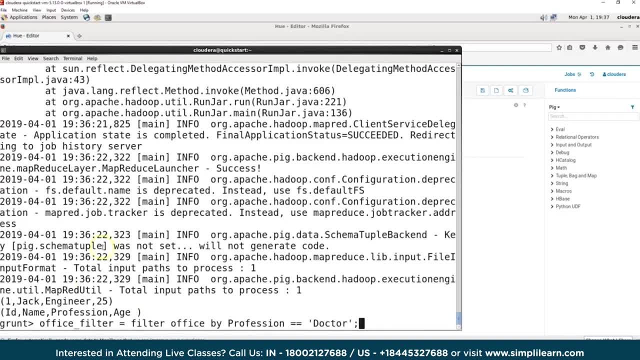 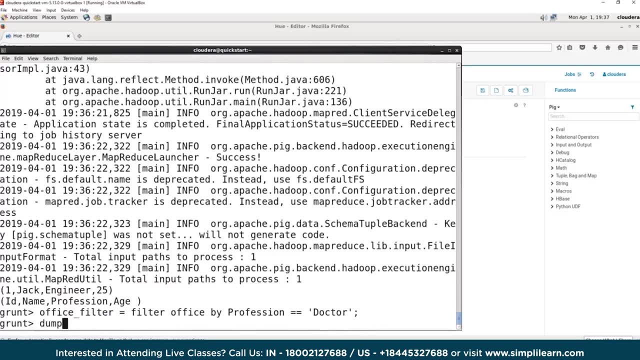 for doing a true false statement. So for your logic statement, remember to use two equal signs in pig And we're going to say it equals doctor. So we want to find out how many doctors do we have on our list And we'll go ahead and do our dump. We're dumping. 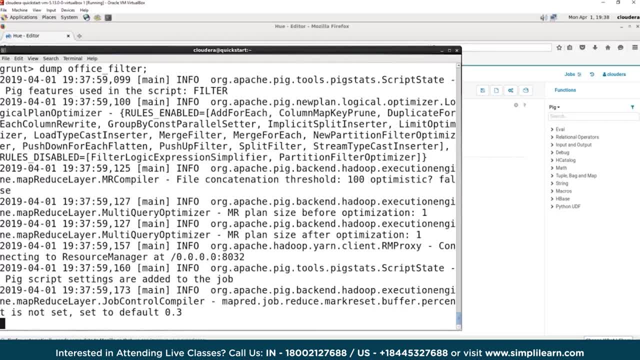 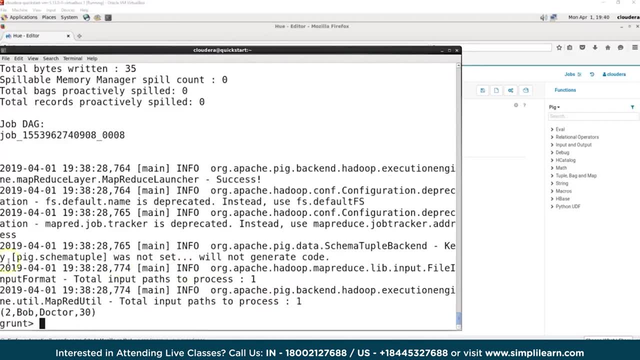 all our garbage into the pig pen And we're letting pig take over And see what it can find out. And see who's a doctor on our list And we find employee ID number two: Bob is a doctor, 30 years old. For this next section, 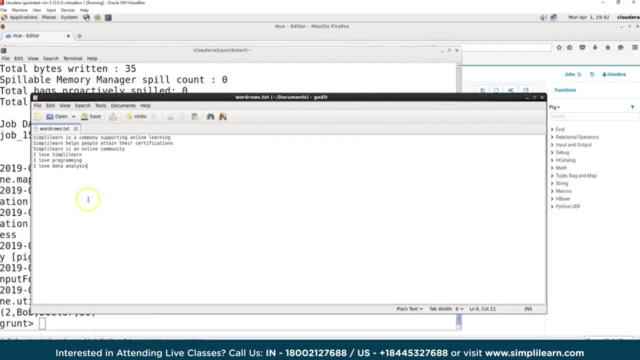 we're going to cover something we see a lot nowadays in data analysis And that's word counting: Tokenization. That is one of the next big steps as we move forward In our data analysis: where we go from, say, stock market analysis of highs and lows and all the 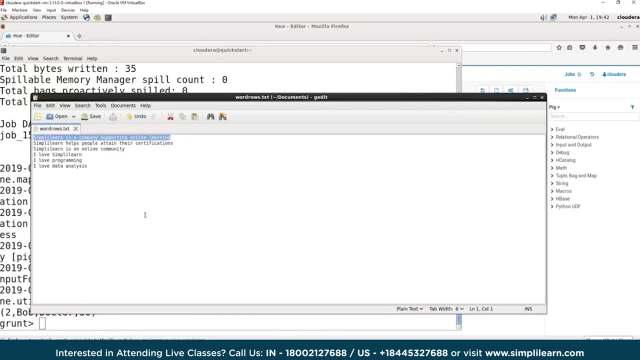 numbers to what are people saying about companies on Twitter? What are they saying on the web pages and on Facebook. Suddenly, you need to start counting words and finding out how many words are totaled, How many are in the first part of the document, And so on. 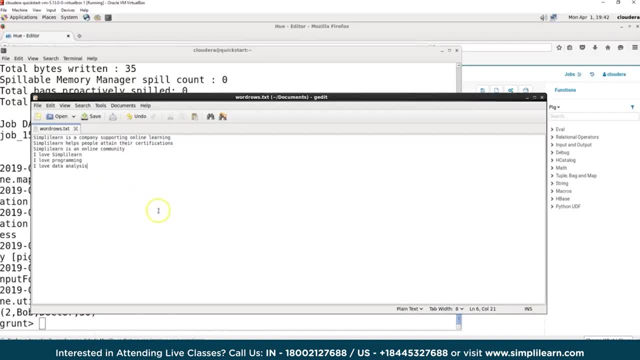 We're going to cover a very basic word count example And in this case I've created a document called word rows dot text And you can see here we have. SimpliLearn is a company supporting online learning. SimpliLearn helps people attain their certifications. 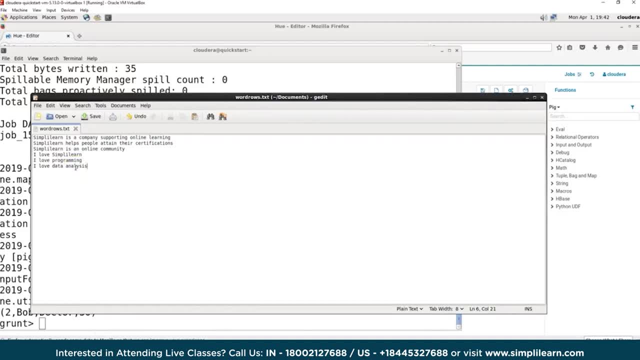 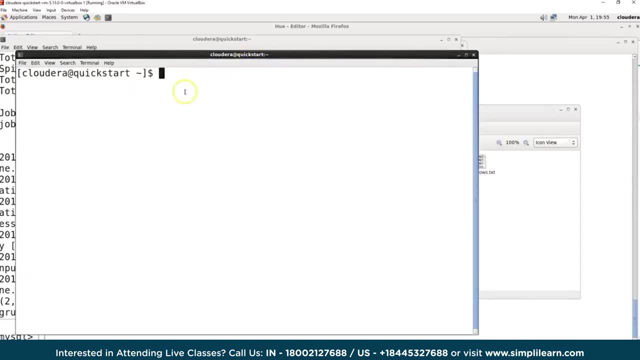 SimpliLearn is an online community. I love SimpliLearn, I love programming, I love data analysis, And I went and saved this into my documents folder so we could use it. And let me go ahead and open up a new terminal window for our word count. 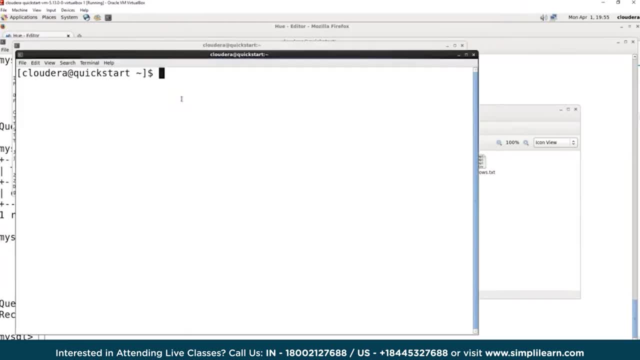 Let me go ahead and close the old one. So we're going to go in here and instead of doing this as pig, we're going to do pig minus x local, And what I'm doing is I'm telling the pig to start the pig shell. 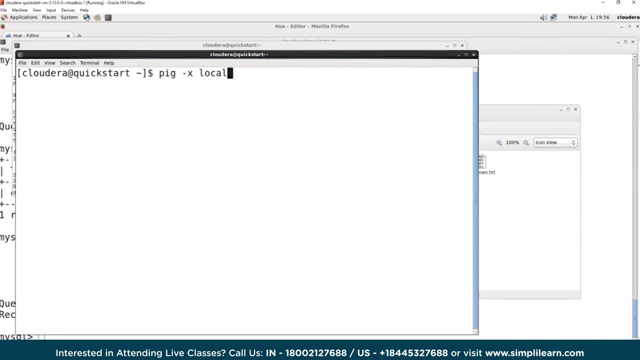 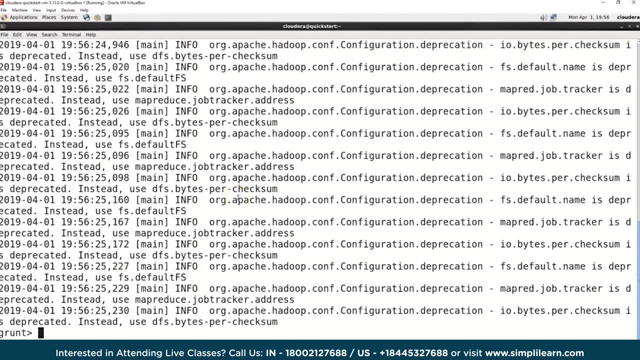 but we're going to be looking at files local to our virtual box or this CentOS machine And let me go ahead and hit enter on there. Just maximize this up. There we go And it will load pig up and it's going to look just the same. 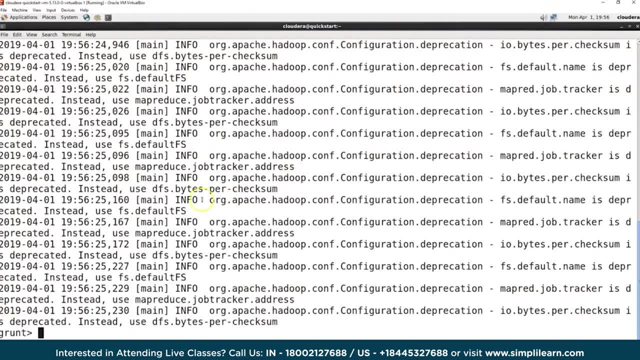 as the pig we were doing- which was defaulted to HADOOP system, To our HDFS. This is now defaulted to the local system. Now we're going to create lines and we're going to load it straight from the file. Remember last time we took 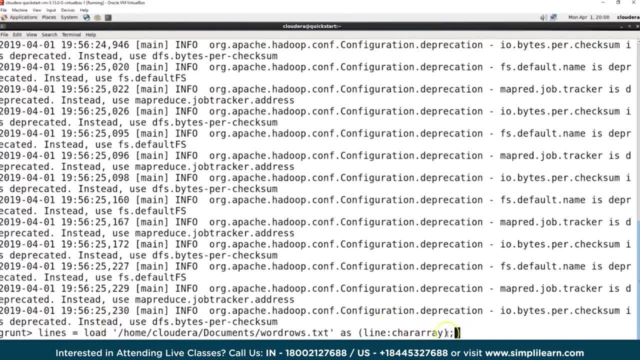 the HDFS and loaded it into there and then loaded it into the pig. Since we've gone the local, we're just going to run a local script. We have lines equals: load home, The actual full path home, Cloudera documents And I. 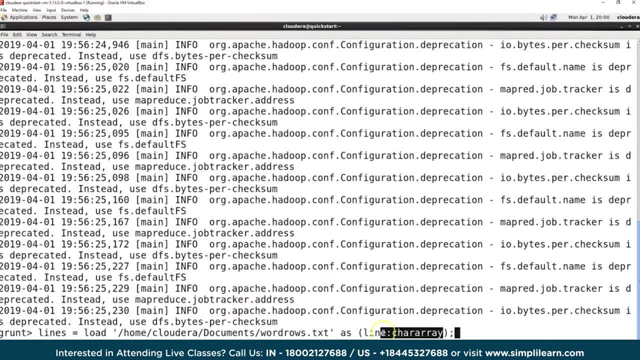 called it word rows, dot text, And as line, as a character array. So each line- And I've actually you can change this- to read each document, I certainly have done a lot of document analysis And then you go through and do word. 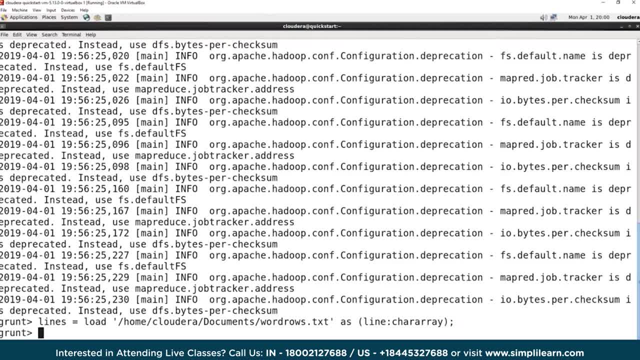 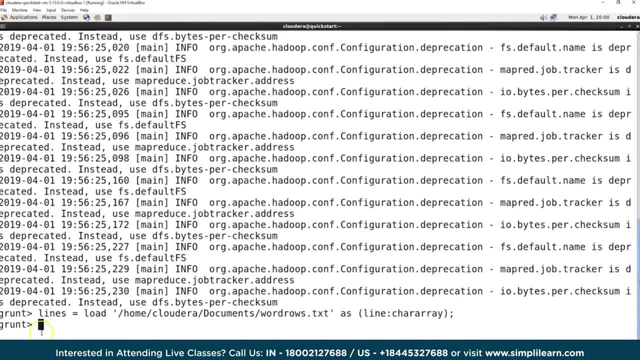 counts and different kind of counts in there. So once we go ahead and create our line, instead of doing the dump, we're going to go ahead and start entering all of our different setups. So we're going to go through each of our steps we want to go through. 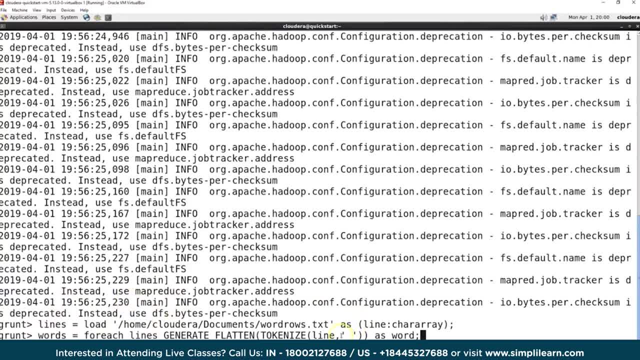 And let's just take a look at this next one, Because the load is straight forward. We're loading from this particular file. Since we're local, it's loading it directly from here instead of going into the Hadoop file system. And it says as: 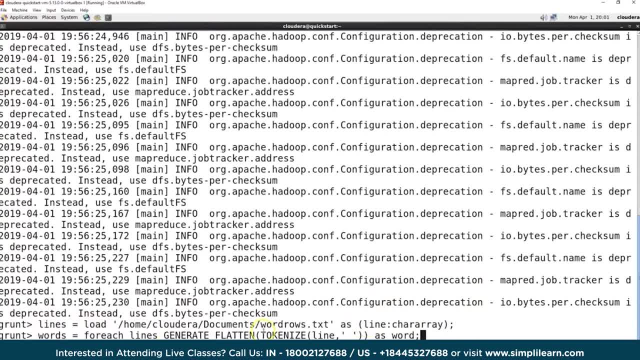 and then each line is read as a character array. Now we're going to do words equal for each of the lines, generate flat, tokenize line space as word. Now there's a lot of ways to do this. This is: if you're a programmer, you're just splitting the line up by 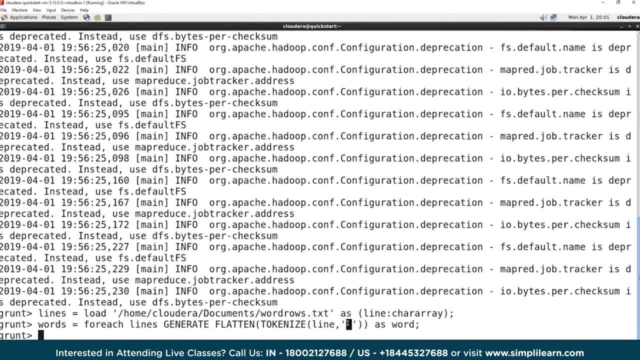 spaces. There's actual ways to do tokenize it. You gotta look for periods, capitalization. There's all kinds of other things you play with with this, But for the most basic word count we're just going to separate it by spaces. The flatten takes the line. 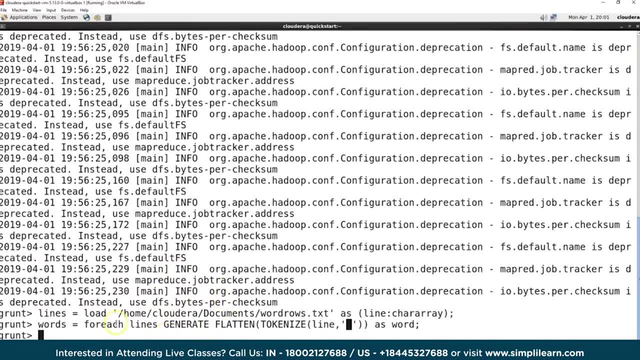 and just creates a. it flattens each of the words out. So this is: we're just going to generate a bunch of words for each line And then each of those words is, as a word, A little confusing in there, but if you really think about it, we're just going down each line. 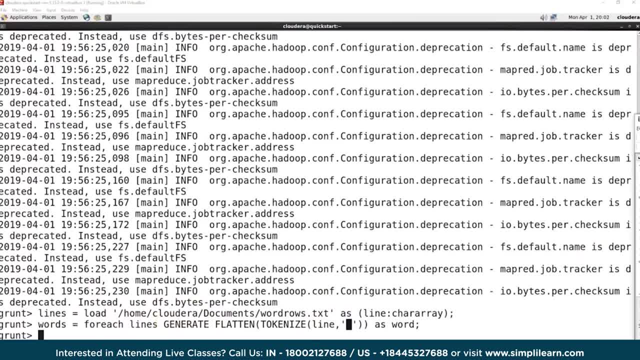 separating it out and we're generating a list of words. One thing to know is the default for tokenize. You can just do tokenize line without the space in there. If you do that, it'll automatically tokenize it by space. You can do either one And then we're going to do group. 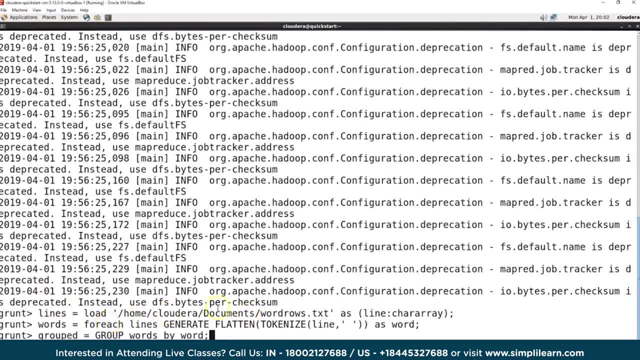 We're going to group it by words. So we're going to group words by word. So, when we split it up, each token is a word and it's a list of words, And so we're going to group equals, group words by words. So we're going to group all. 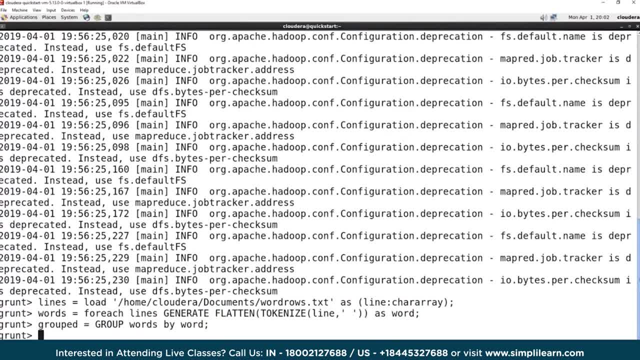 the same words together, And if we're going to group them, then we want to go ahead and count them, And so, for count, we'll go ahead and create a word count variable, And here's our for each. So for each grouped, grouped is our line where we group all. 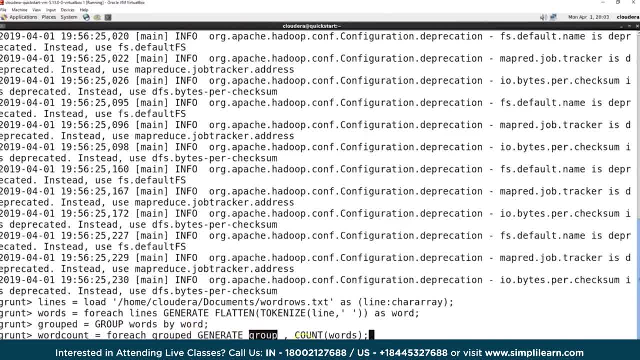 the words in the line that are similar, We're going to generate a group And then we're going to count the words For each grouped. So for each line where we group the words together, we're going to generate a group, and that's. 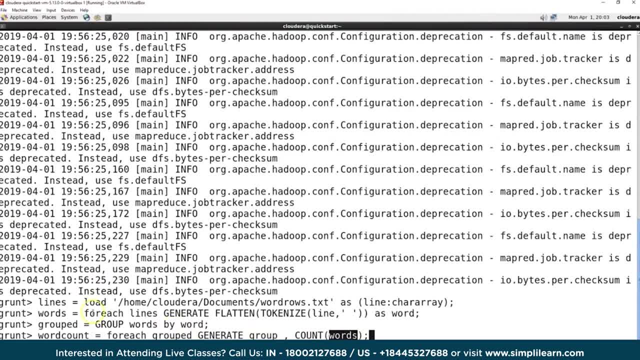 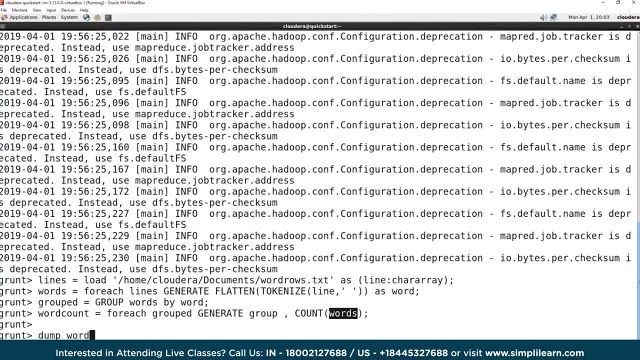 going to count the words. We want to know the word count in each of those And that comes back in our word count. And finally, we want to take this and we want to go ahead and dump word count. And this is a little bit more. 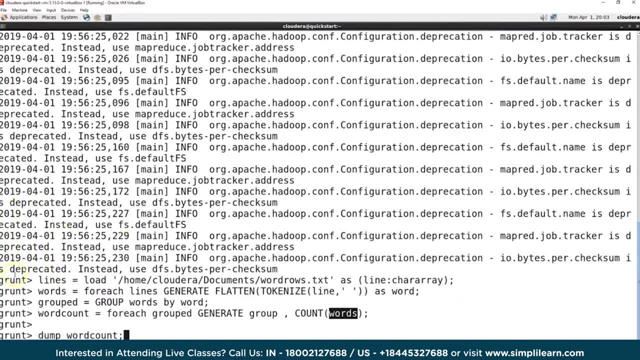 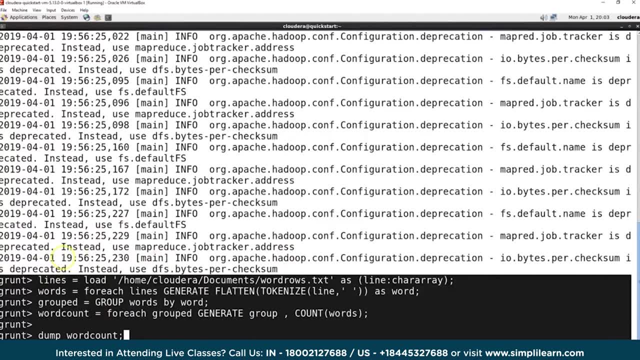 what you see when you start looking at grunt scripts. You'll see right here these lines. right here We have each of the steps you take to get there. So we load our file For each of our lines we're going to generate and tokenize it into. 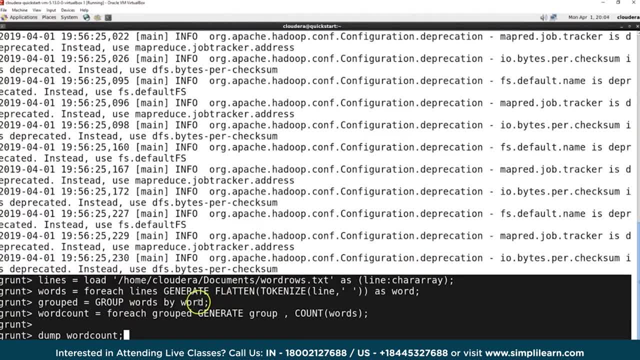 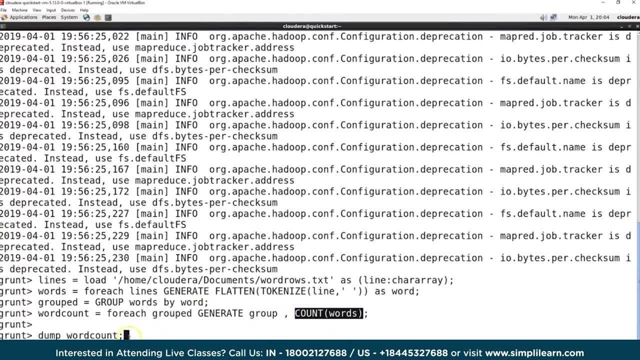 words. Then we're going to take the words and we're going to group them by same words For each grouped. we're going to generate a group and we're just going to count the words. So we're going to summarize all the words in here And let's go ahead and do. 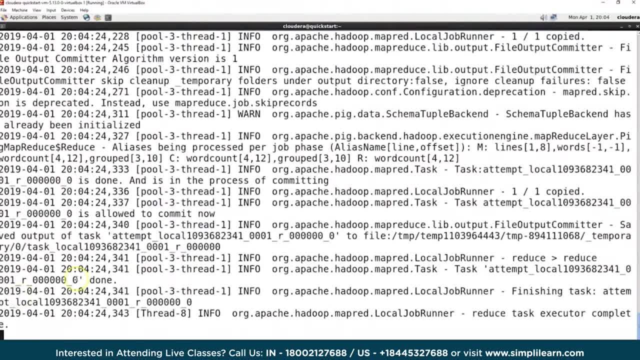 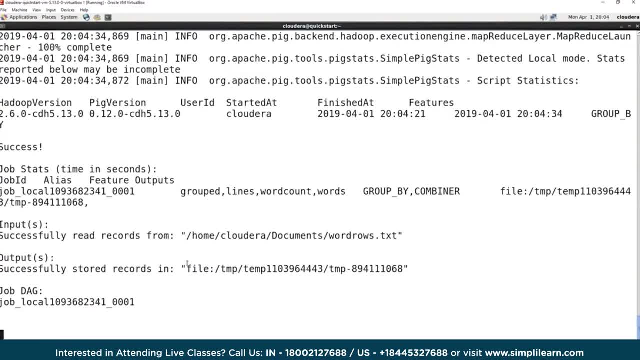 our dump word count, which actually executes all this And it goes through our MapReduce. It's actually a local runner. You'll see down here. you start seeing where they still have MapReduce, but it's a special runner. We're mapping it. That's a part of each. 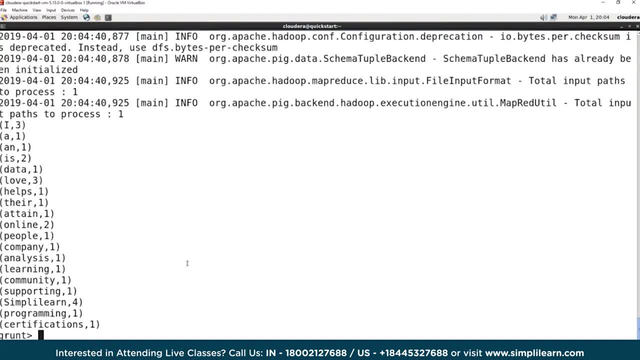 row being counted and grouped, And then when we do the word count, that's the reducer. The reducer creates these keys And you can see I is used three times: A came up once, N came up once Is too. Continue on down here to attain. 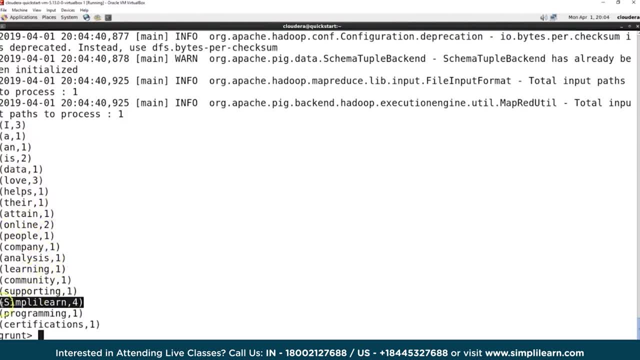 online people company analysis, Simply learn. they took the top rating with four Certification. So all these things are then counted in the how many words are used And in data analysis. this is probably the very beginnings of data analysis where you might look at it and say, oh, they mentioned. 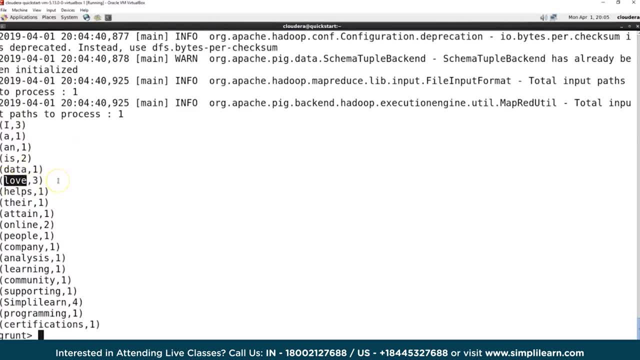 love three times. So whatever's going on in this post, it's about love And what do they love? And then you might attach that to the different objects in here So you can see that Pig Latin is fairly easy to use. There's nothing really, you know it might. 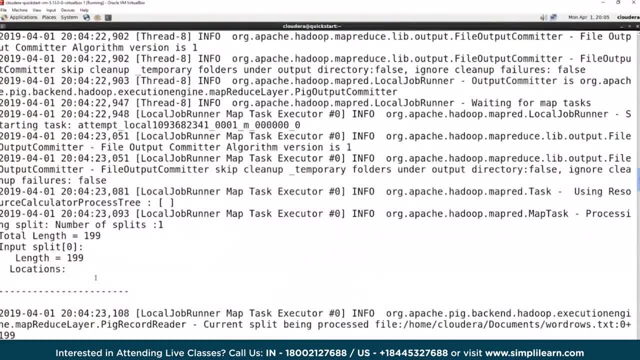 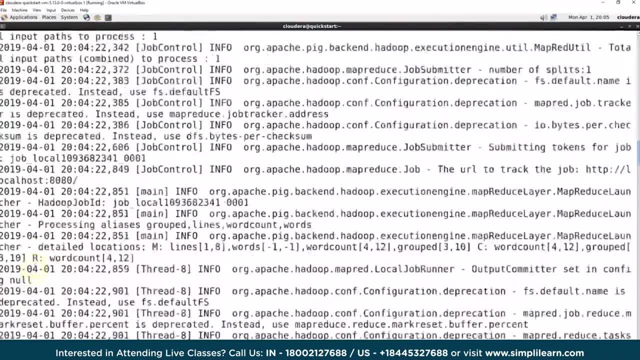 take a little bit to learn the script, depending on how good your memory is. As I get older, my memory leaks a little bit more, so I don't memorize it as much. But that was pretty straight forward. The script we put in there And then it goes through the full map. 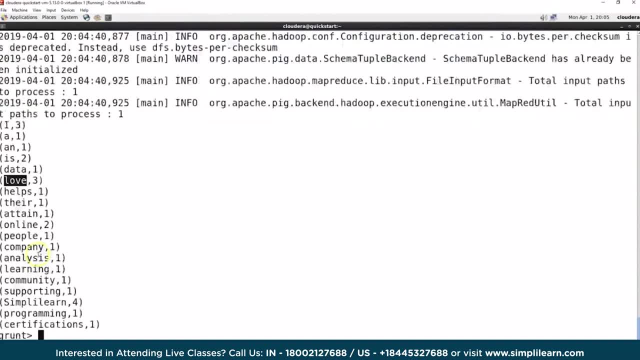 reduce, localize, run Comes out and, like I said, it's very easy to use. That's why people like Pig Latin is because it's intuitive. One of the things I like about Pig Latin is when I'm troubleshooting, When we're troubleshooting. a lot of times you're 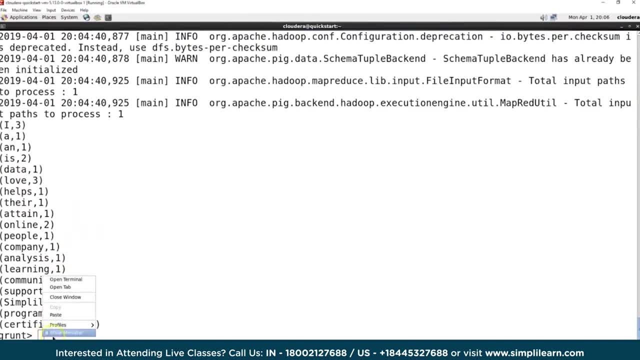 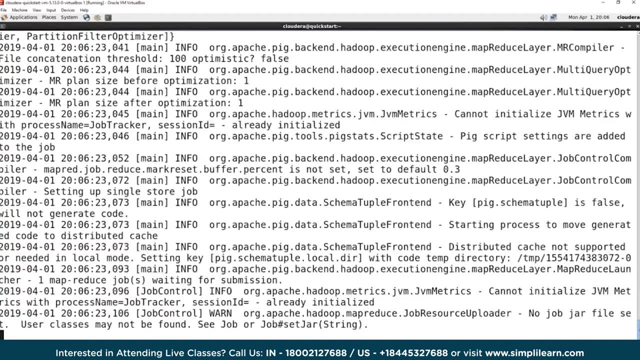 working with a small amount of data and you start doing one line at a time, And so I can go lines equal load and there's my loaded text And maybe I'll just dump lines And then it's going to run, It's going to. 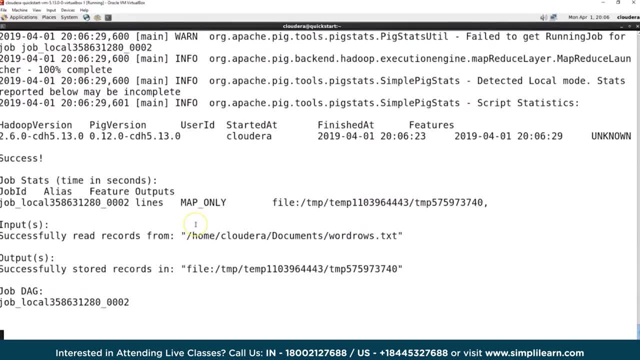 show me all the lines that I'm working on in this small amount of data And that way I can test that If I got an error on there that said, oh, this isn't working, Maybe it'll be like: oh my gosh, I'm in map reduce or I'm in. 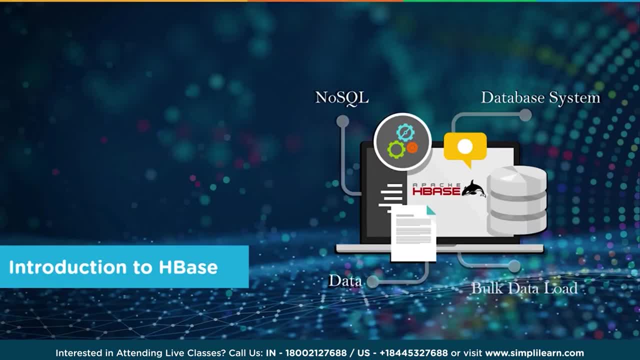 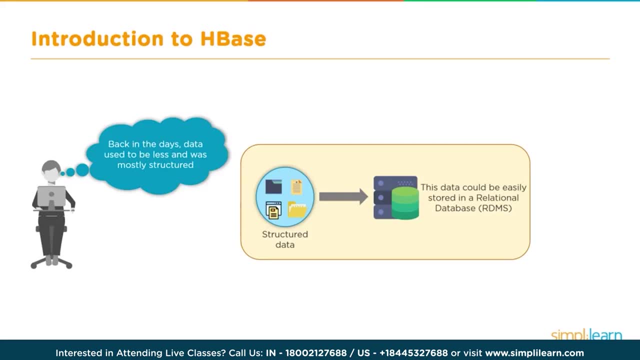 the basic grunt shell instead of the local path grunt. Let's start with an introduction to HBase. Back in the days, data used to be less and was mostly structured, And you see we have structured data here. We usually had it like in a 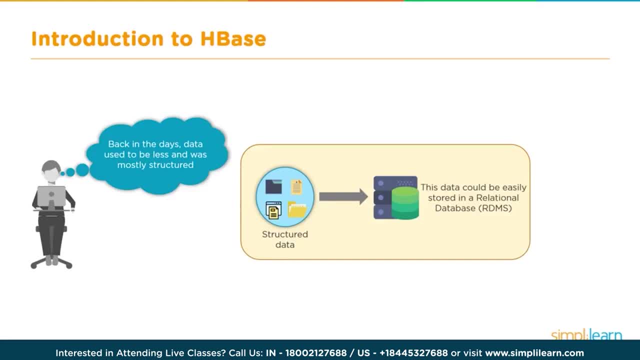 database where you had every field was exactly the correct length. So if you had a name field, it was exactly 32 characters. Remember the old access database in Microsoft? The files were small. If we had hundreds of people in one database, that was considered big data. 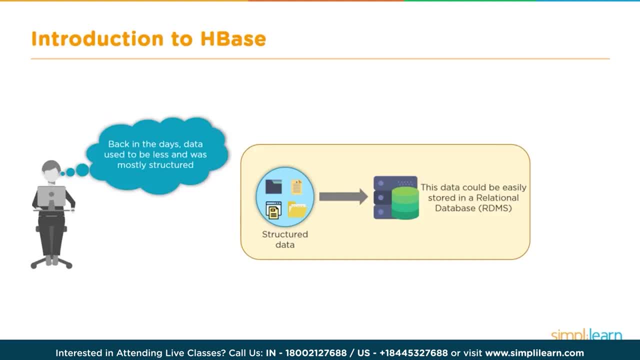 This data could be easily stored in relational database or RDBMS. When we talk about relational database, you might think of Oracle, You might think of SQL, Microsoft, SQL, MySQL. All of these have evolved even from back then to do a lot more today than they did. 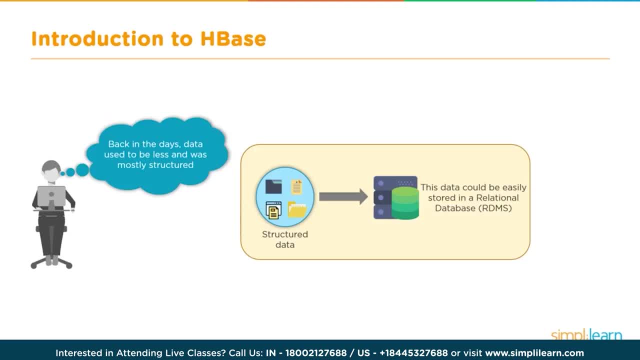 But they still fall short in a lot of ways, And they're all examples of an RDMS or relationship database. Then internet evolved and huge volumes of structured and semi-structured data got generated, And you can see here, with the semi structured data, we have email. 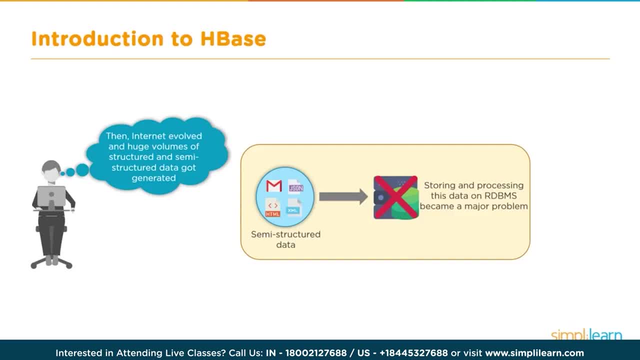 If you look at my spam folder, you know what we're talking about: All the HTML pages, XML, which a lot of times is displayed on our HTML and help desk pages, JSON. All of this really has just even in the last. each year it almost doubles from the 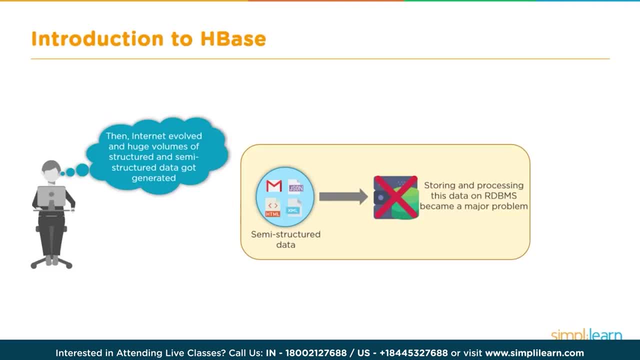 year before, how much of this is generated. So storing and processing this data on an RDBMS has become a major problem, And so the solution is: we use Apache HBase. Apache HBase was the solution for this. Let's take a look at the. 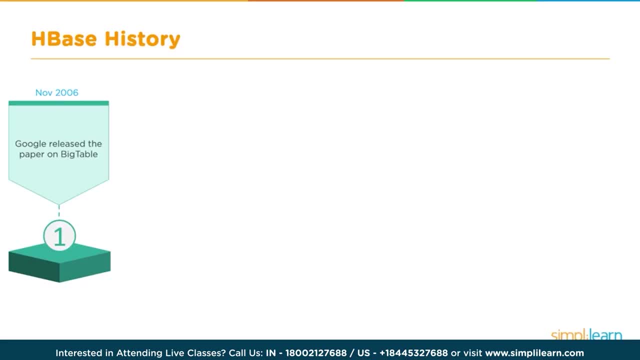 history, The HBase history. When we look at the HBase history, we're going to start back in 2006, November, Google released the paper on Bigtable And then in 2017, just a few months later, HBase prototype was created as a 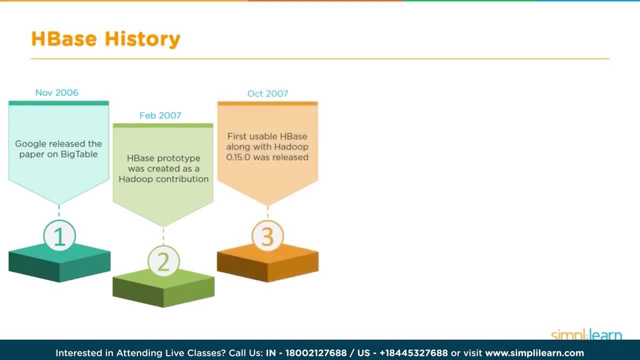 Hadoop contribution. Later on in the year 2007, in October, first usable HBase along with the Hadoop 0.15 was released, And then, in January of 2008, HBase became the subproject of Hadoop, And later on that year, in October- all the way. 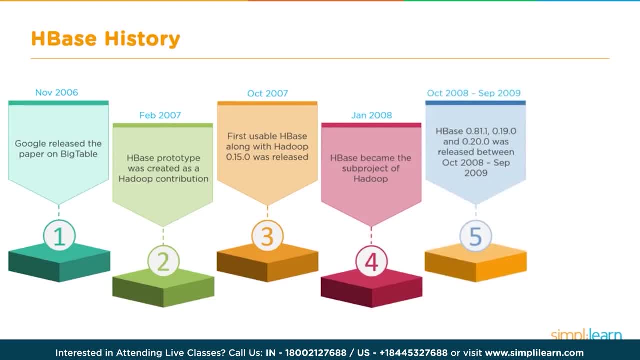 into September the next year, HBase was released the 0.81 version, the 0.19 version and 0.20.. And finally, in May of 2010, HBase became Apache top level project. And so you can see in the course of about. 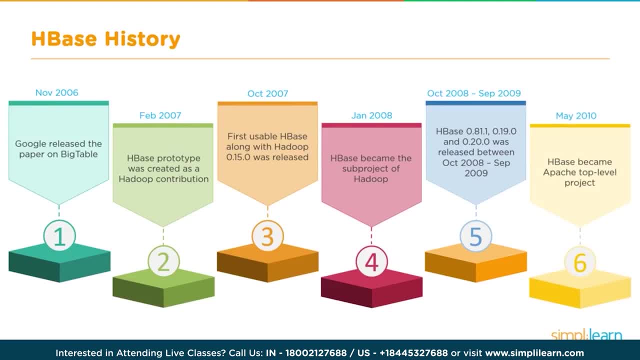 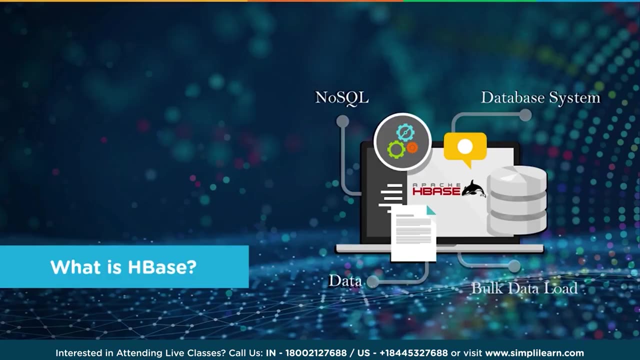 four years. HBase started off as just an idea on paper and has evolved all the way till 2010 as a solid project under the Apache And since 2010 it's continued to evolve and grow as a major source for storing data in semi-structured data. So what is? 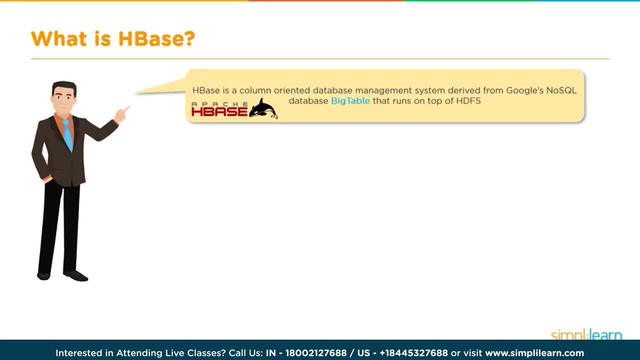 HBase. HBase is a column oriented database management system derived from Google's NoSQL database Bigtable that runs on top of the Hadoop file system or the HDFS. It's an open source project that is horizontally scalable, and that's very important to understand. 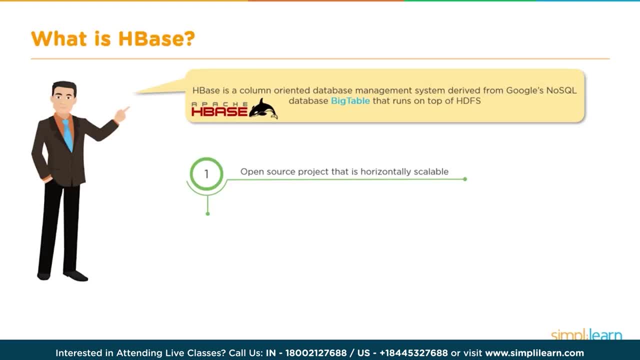 that you don't have to buy a bunch of huge, expensive computers. you're expanding it by continually adding commodity machines And so it's a linear cost expansion as opposed to being exponential. NoSQL database written in Java, which permits faster querying, So Java is the back end for 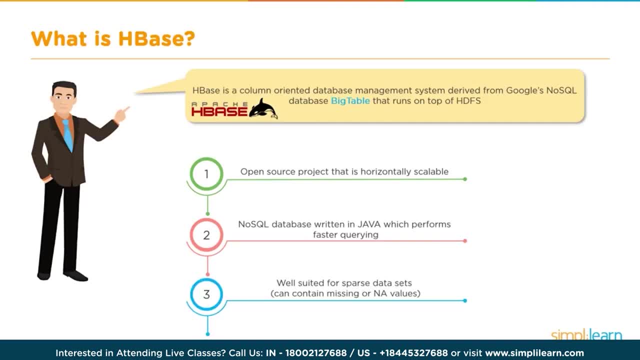 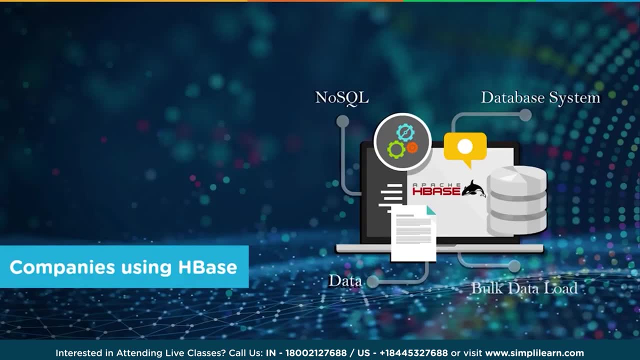 the HBase setup And it's well suited for sparse data sets, So it can contain missing or NA values, and this doesn't boggle it down like it would another database Companies using HBase, So let's take a look and see who is using this. 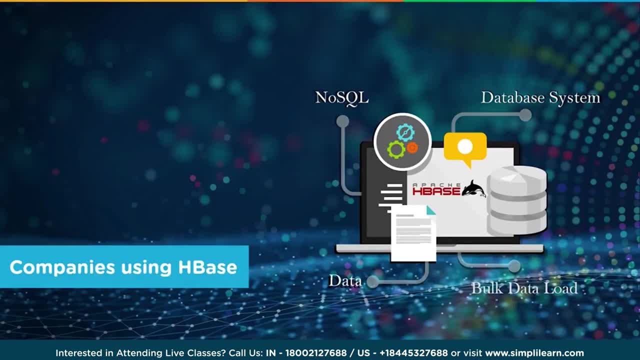 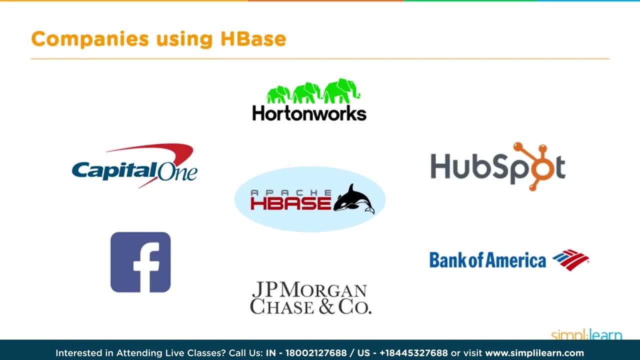 NoSQL database for their servers and for storing their data. And we have Hortonworks, which isn't a surprise because they're one of the Cloudera Hortonworks. They are behind Hadoop and one of the big developments and backing of it, And, of course, Apache HBase. 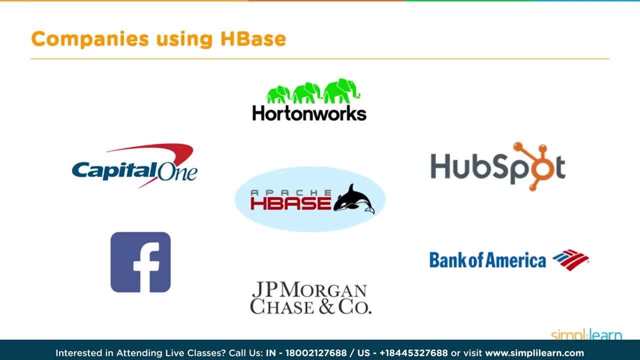 is the open source behind it And we have Capital One as bank. you also see Bank of America where they're collecting information on people and tracking it, So their information might be very sparse. They might have one bank way back when they collected information as far as the person's 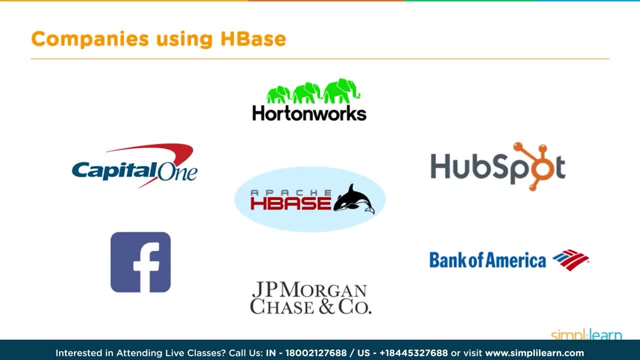 family and what their income for the whole family is and their personal income, And maybe another one doesn't collect the family income, As he started saying. where you have data that is very difficult to store, where it's missing a bunch of data, Hubspot is using it- Facebook. 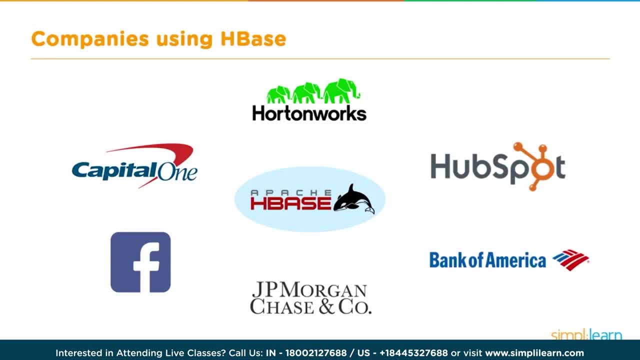 certainly all of your Facebook, Twitter, most of your social medias are using it, And then, of course, there's JPMorgan Chase and company, another bank that uses the HBase as their data warehouse for NOS SQL. Let's take a look at an HBase use case. 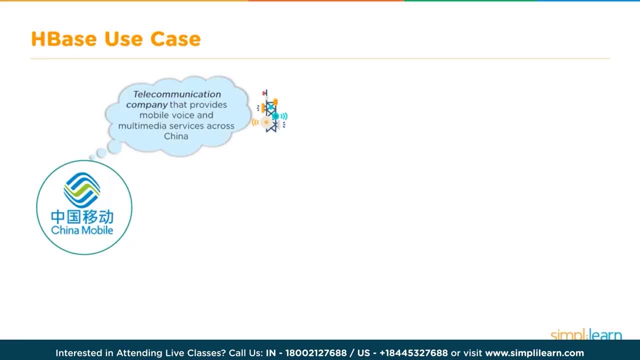 so we can dig a little bit more into it to see how it functions. Telecommunication company that provides mobile voice and multimedia services across China, The China Mobile And China Mobile. they generate billions of call detailed records, or CDR, And so these CDRs. 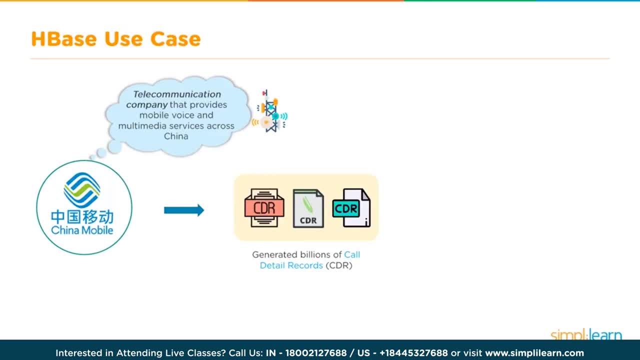 and all these records of these calls and how long they are and different aspects of the call, maybe the tower they're broadcasted from. all of that is being recorded so they can track it. A traditional database systems were unable to scale up to the vast volumes of data and provide. 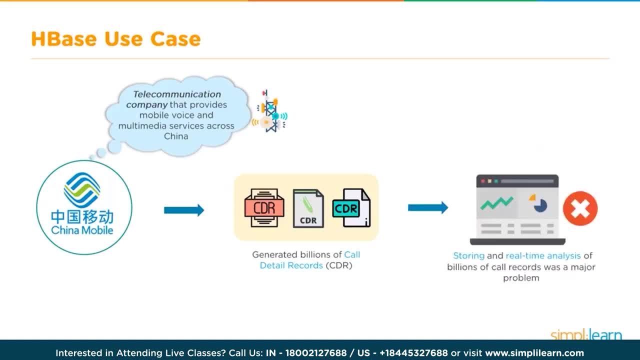 a cost effective solution- No good. So storing in real time analysis of billions of call records was a major problem for this company Solution, Apache HBase. HBase stores billions of rows of detailed call records. HBase performs fast processing of records using 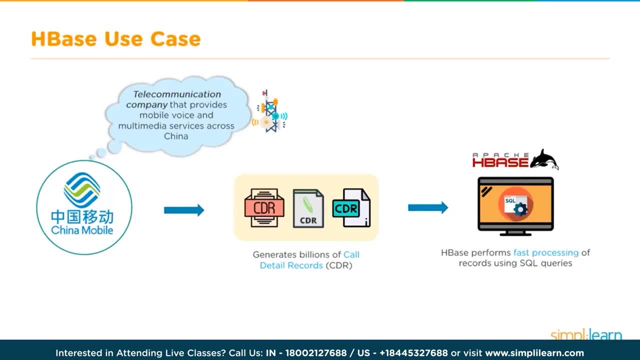 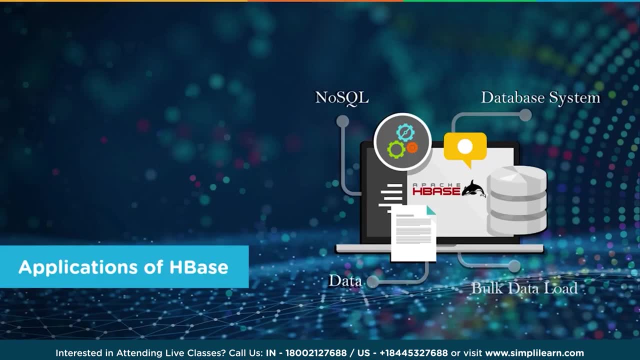 SQL queries. So you can mix your SQL and no SQL queries And usually just say no SQL queries because of the way the query works. Applications of HBase. One of them would be in the medical industry. HBase is used for storing genome sequences. 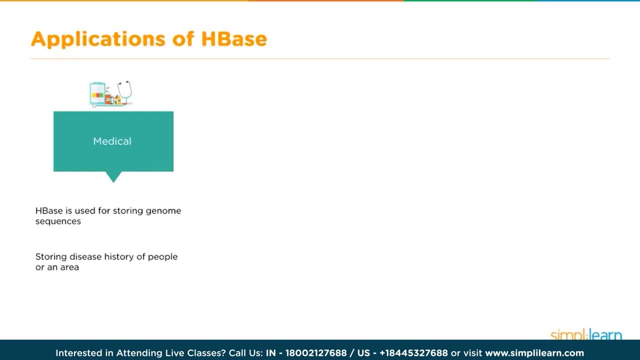 Storing disease history of people of an area, And you can imagine how sparse that is. as far as both of those A genome sequence might be only have pieces to it that each person is unique or is unique to different people, And the same thing with disease. You really 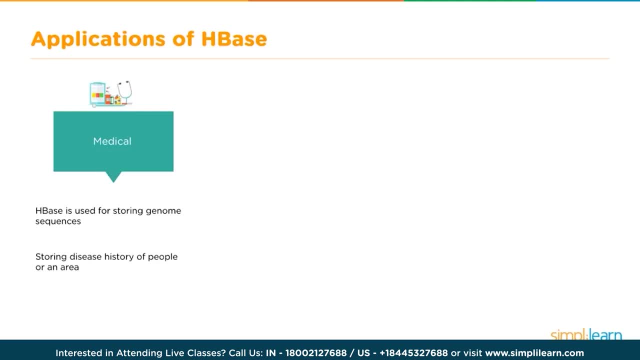 don't need a column for every possible disease a person could get. You just want to know what those diseases, those people have had to deal with in that area. E-commerce HBase is used for storing logs about customer search history, Performs analytics and target advertisement. 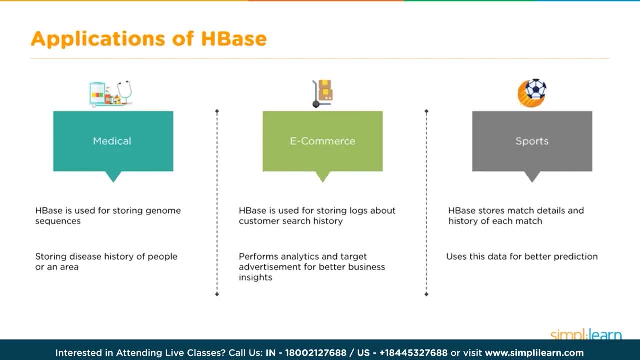 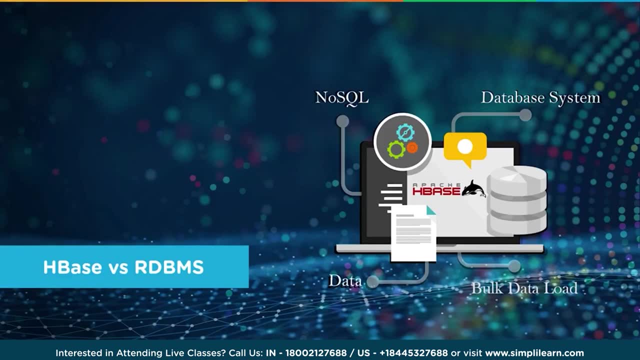 for better business insights. Sports HBase stores match details and the history of each match, Uses this data for better prediction. So when we look at HBase, we all want to know what's the difference between HBase versus RDBMS, That is, a relational database. 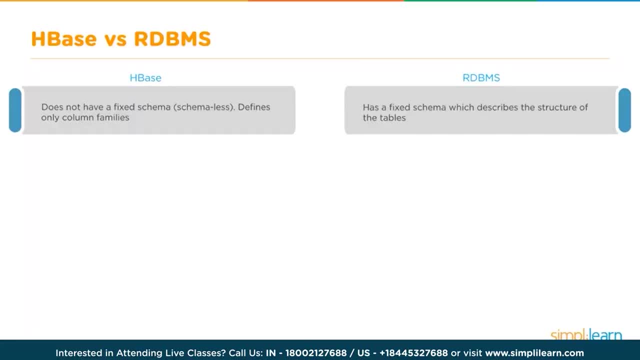 management system HBase versus RDBMS. So the HBase does not have a fixed schema. It's schemaless. It defines only column families, And we'll show you what that means later on. RDBMS has a fixed schema which describes the structure of the tables. 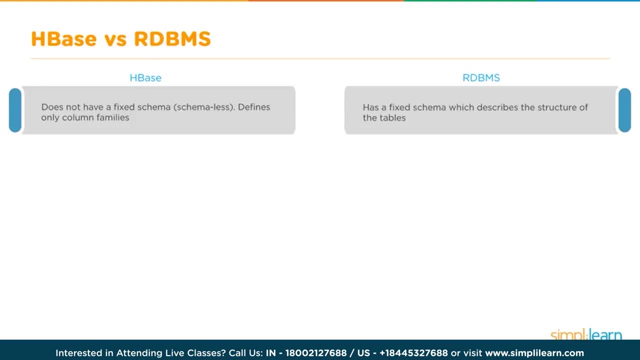 And you can think of this as you have a row and you have columns And each column is a very specific structure: How much data can go in there and what it does With the HBase. it works well with structured and semi-structured data. 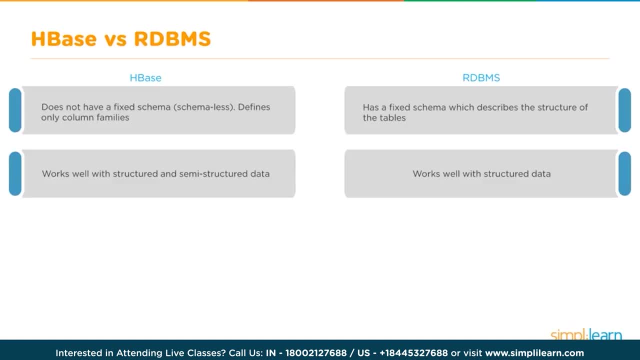 With the RDBMS it works only well with structured data. With the HBase it can have denormalization data. It can contain missing or null values. With the RDBMS it can store only normalized data. Now you can still store a null. 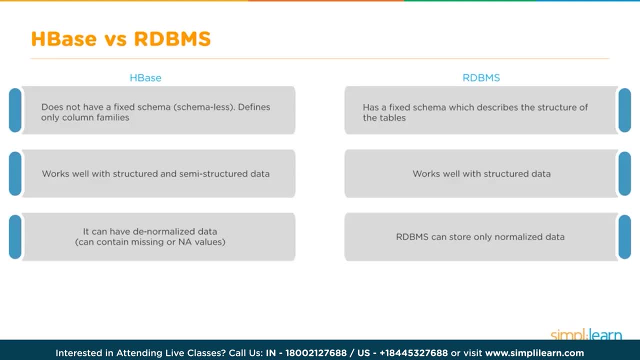 value in the RDBMS, but it still takes up the same space as if you're storing a regular value in many cases- And it also for the HBase- is built for wide tables. It can be scaled horizontally, For instance, if you were doing 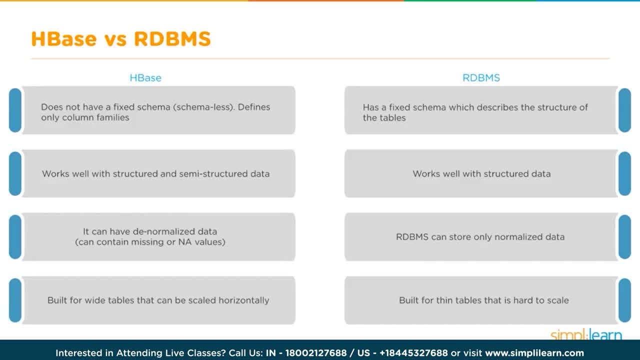 a tokenizer of words and word clusters, you might have 1.4 million different words that you're pulling up and then you have a combination of words. So with an RDBMS it's built for thin tables that are hard to scale. You don't want to store 1.4 million. 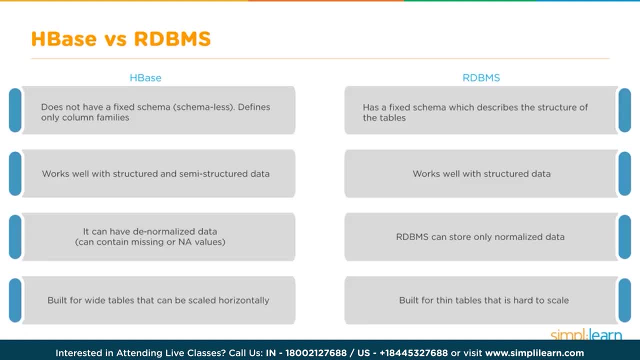 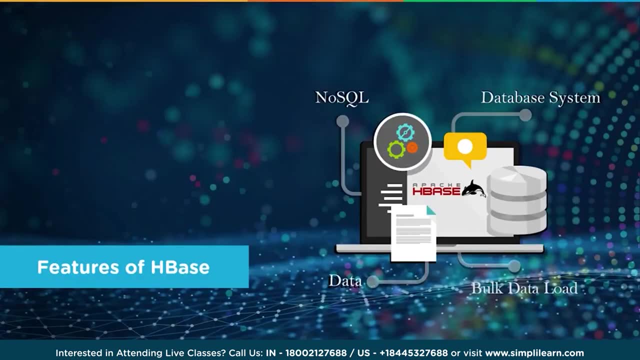 columns in your SQL, It's going to crash and it's going to be very hard to do searches With the HBase. it only stores that data, which is part of whatever row you're working on. Let's look at some of the features of the HBase. It's scalable. 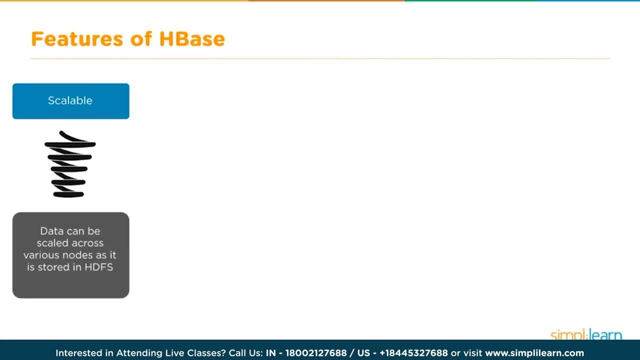 Data can be scaled across various nodes as it is stored in the HDFS, And I always think about this. it's a linear add-on. For each terabyte of data, I'm adding on roughly a thousand dollars in commodity computing With an enterprise machine. 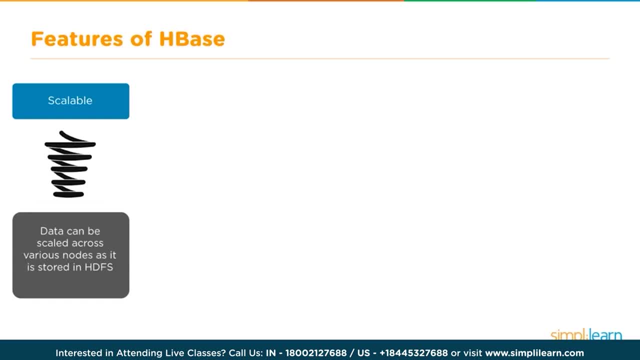 we're looking at about 10,000 at the lower end for each terabyte of data, And that includes all your backup and redundancy. So it's a big difference. It's like a tenth of the cost to store it across the HBase. 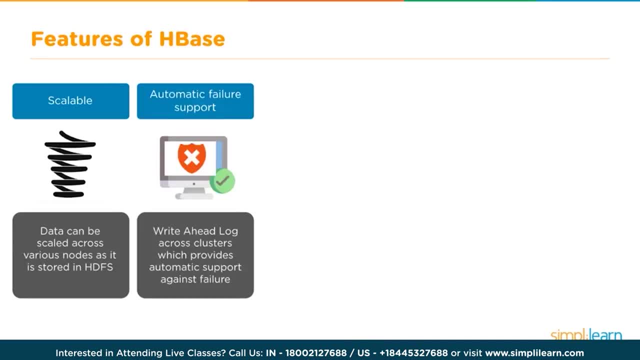 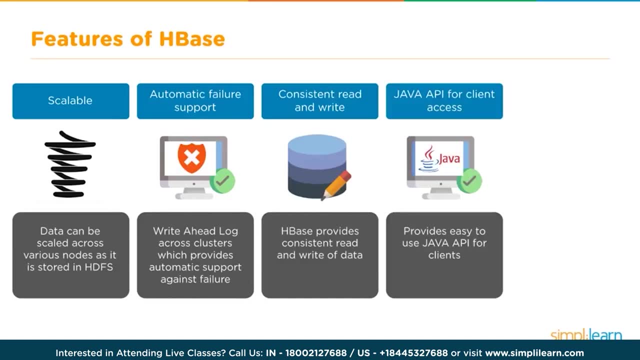 It has automatic failure support. Write ahead, log across clusters, which provides automatic support against failure. Consistent read and write HBase provides consistent read and write of the data. It's a Java API for client access. Provides easy to use Java API for clients. 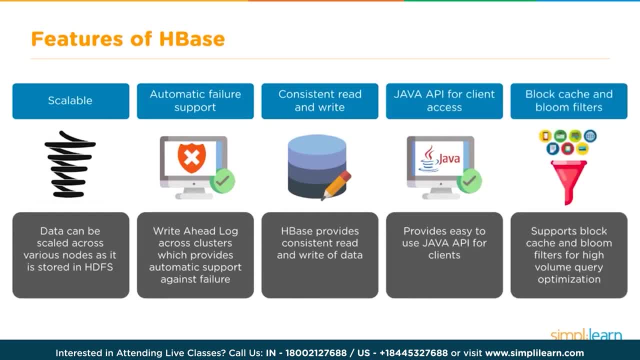 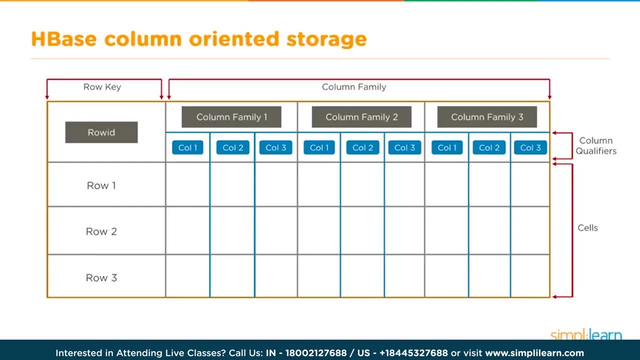 Block cache and bloom filters. So the HBase supports block caching and bloom filters for high volume query optimization. Let's dig a little deeper into the HBase storage- HBase column oriented storage- And I told you we're going to look into this to see. 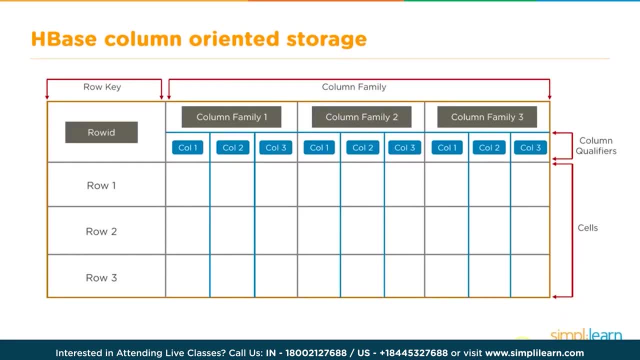 how it stores the data, And here you can see you have a row key, And this is really one of the important references is each row has to have its own key or your row ID. And then you have your column family And in here you can see we have 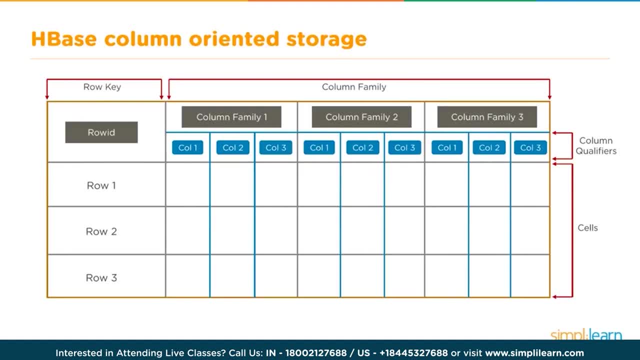 column family 1,, column family 2, column family 3.. And you have your column qualifiers. So you can have in column family 1, you can have three columns in there And there might not be any data in that. So when you go into column, 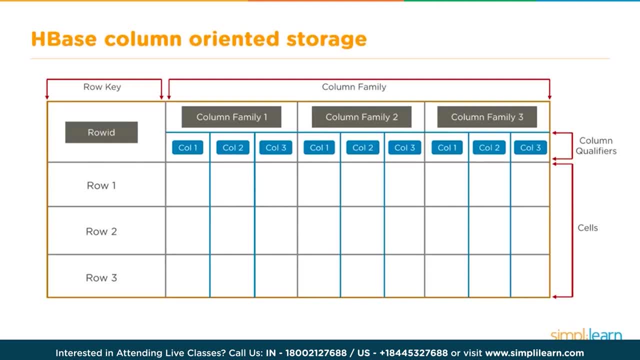 family 1 and do a query for every column that contains a certain thing. that row might not have anything in there and not be queried Where. in column family 2, maybe you have column 1 filled out and column 3 filled out, And so on and so forth. 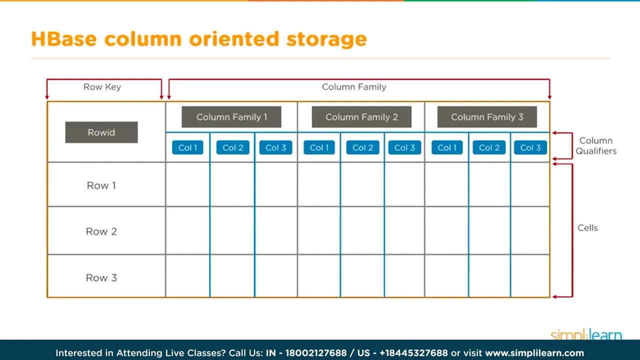 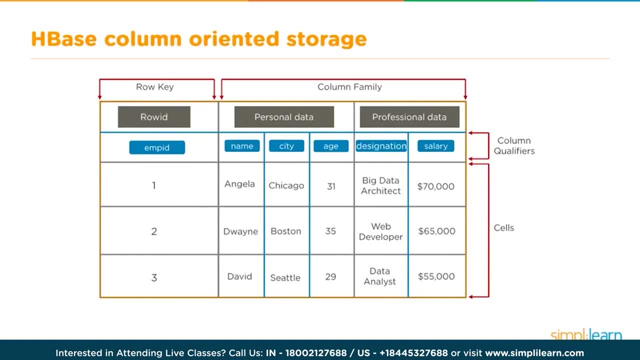 And then each cell is connected to the row where the data is actually stored. Let's take a look at this and what it looks like when you fill the data in. So in here we have a row key with a row ID And we have our employee ID 123.. 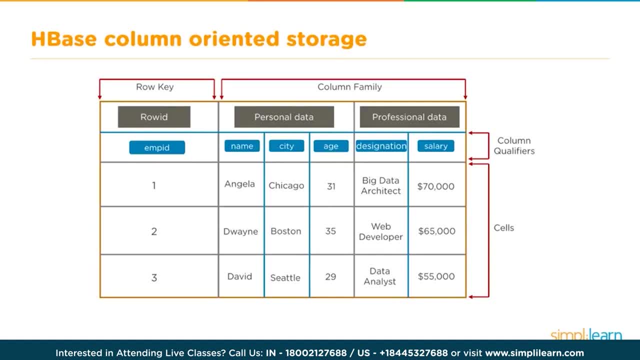 That's pretty straight forward. You probably would even have that on an SQL server, And then you have your column family. This is where it starts really separating out. Your column family might have personal data And under personal data you would have name, city, age. 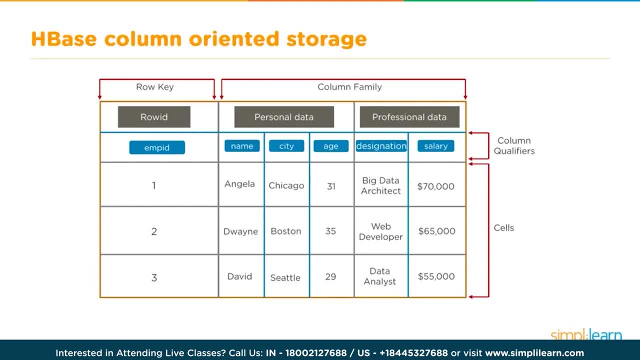 You might have a lot more than just that. You might have number of children, You might have degree, All those kinds of different things that go under personal data, And some of them might be missing. You might only have the name and the age of an employee. 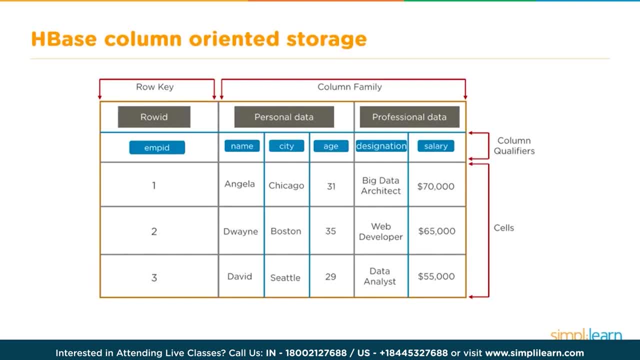 You might only have the name, the city and how many children, And not the age, And so you can see with the personal data. you can now collect a large variety of data and store it in the HBase very easily, And then maybe you have a family. 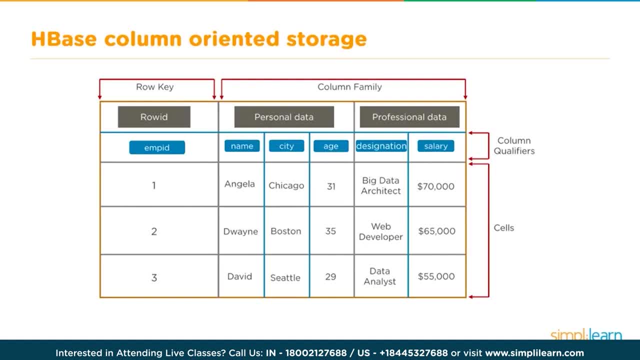 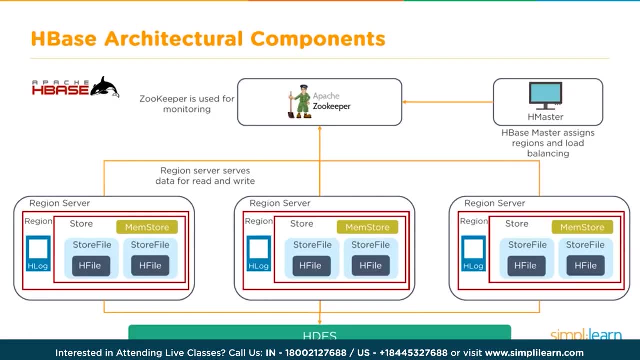 of professional data, Your designation, your salary, all the stuff that the employee is doing for you in that company. Let's dig a little deeper into the HBase architecture And so you can see here what looks to be a complicated chart. It's not as complicated. 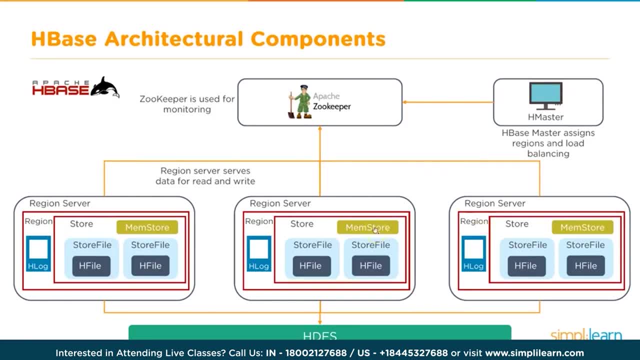 as you think, From the Apache HBase. we have the zookeeper, which is used for monitoring what's going on, And you have your HMaster. This is the HBase master that assigns regions and load balancing And then underneath the region or the 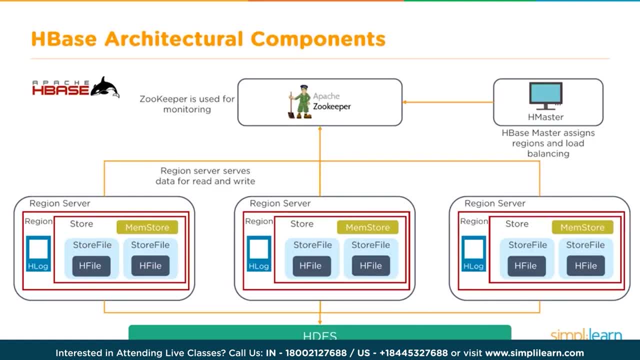 HBase master. then under the HMaster or HBase master, you have your read- your server serves data for read and write- And the region server, which is all your different computers you have in your Hadoop cluster. you'll have a region, an HLog, you'll have a. 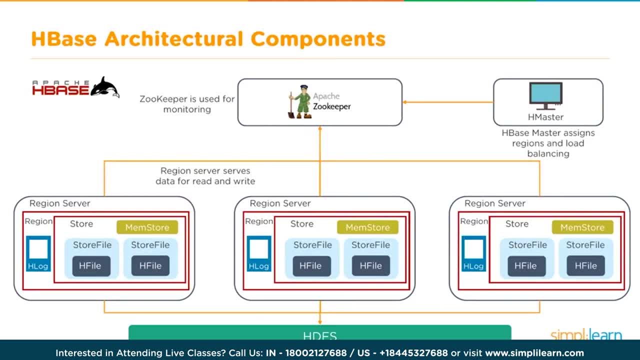 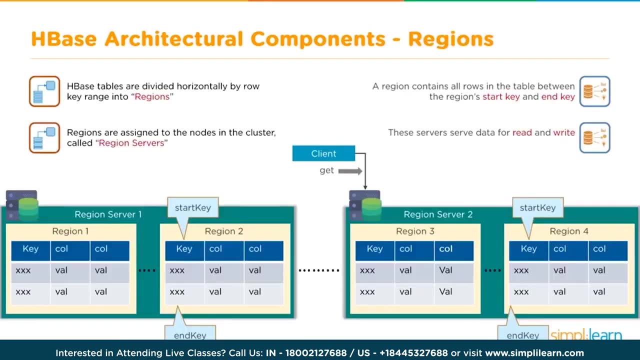 store, memory store, and then you have your different files for HFile that are stored on there And those are separated across the different computers And that's all part of the HDFS storage system. So when we look at the architectural components or regions and we're 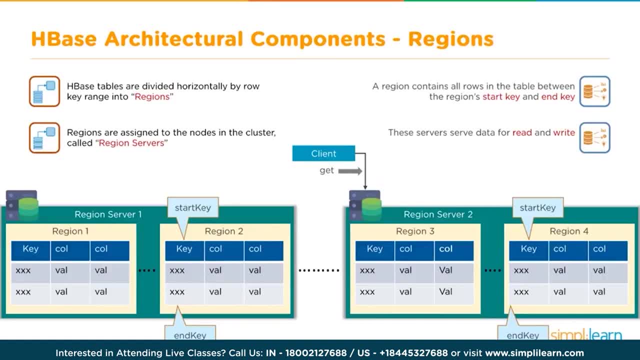 drilling down a little bit, HBase tables are divided horizontally by a row, So you have a key range into regions. So each of those IDs you might have IDs 1 to 20,, 21 to 50, or whatever they are- Regions are. 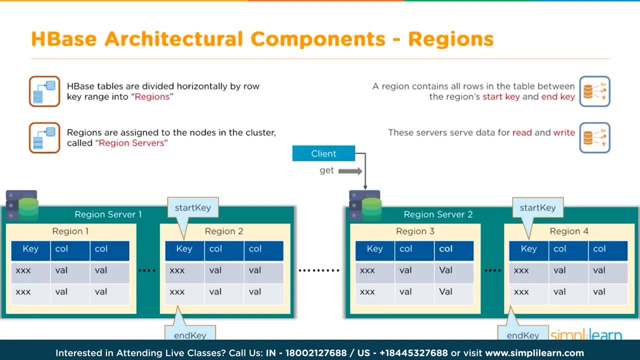 assigned to the nodes in the cluster called region servers. A region contains all rows in the table between the region start key and the end key, Again 1 to 10,, 11 to 20, and so forth. These servers serve data for read and write. 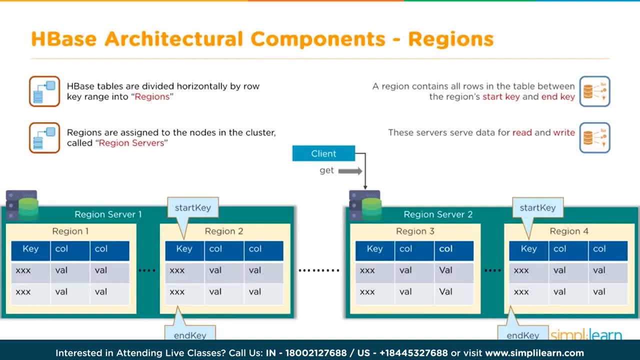 And you can see, here we have the client and the get and the get sends it out and it finds out where that start, if it's between which start keys and end keys, and then it pulls the data from that different region server. 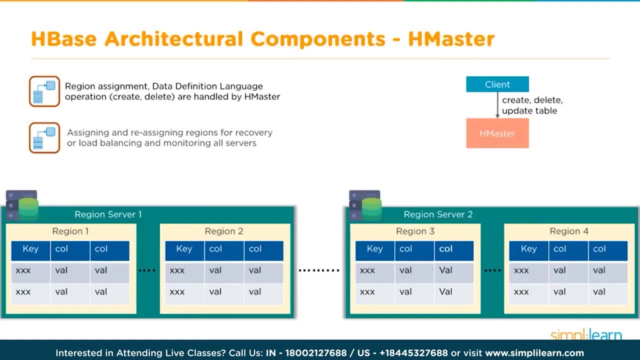 And so the region, sign, data, definition, language, operation, create, delete are handled by the HMaster. So the HMaster is telling it: what are we doing with this data? what's going out there, Assigning and reassigning regions for recovery or load? 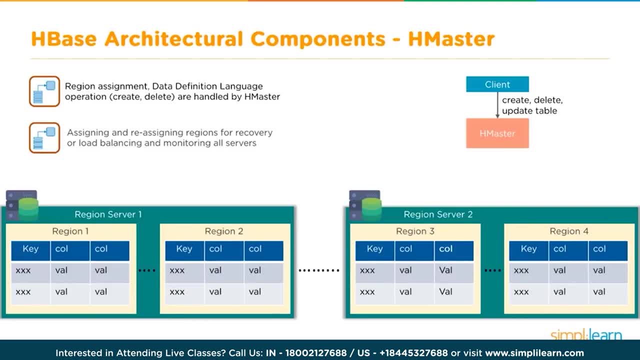 balancing and monitoring all servers. So that's also part of it. So you know if your IDs, if you have 500 IDs across 3 servers, you're not going to put 400 IDs on server 1 and 100 on the. 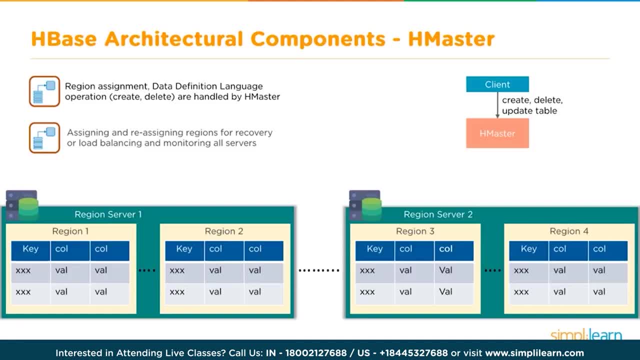 server 2 and leave region 3 and region 4 empty. You're going to split that up And that's all handled by the HMaster And you can see here: it monitors region servers. assigns regions to region servers. assigns regions to region servers. 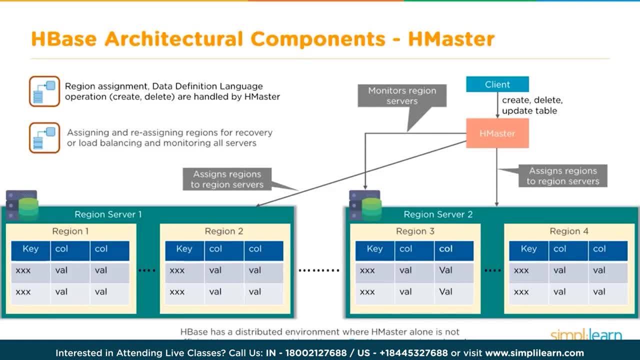 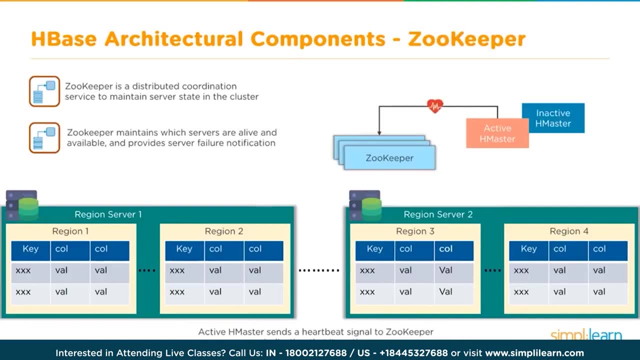 and so forth and so forth. HBase has a distributed environment where HMaster alone is not sufficient to manage everything. Hence ZooKeeper was introduced. It works with HMaster, So you have an active HMaster which sends a heartbeat signal to ZooKeeper. 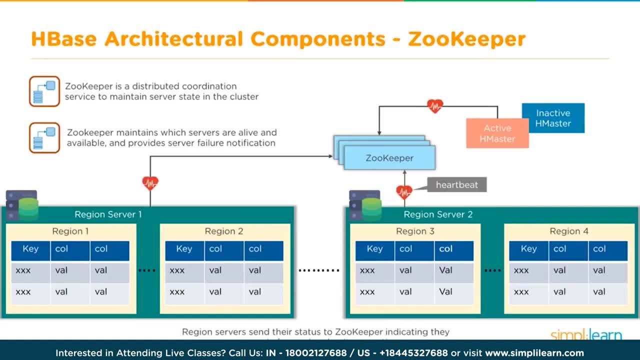 indicating that it's active. And the ZooKeeper also has a heartbeat to the region servers, So the region servers send their status to ZooKeeper, indicating they are ready for read and write operation. Inactive server acts as a backup If the active HMaster fails. 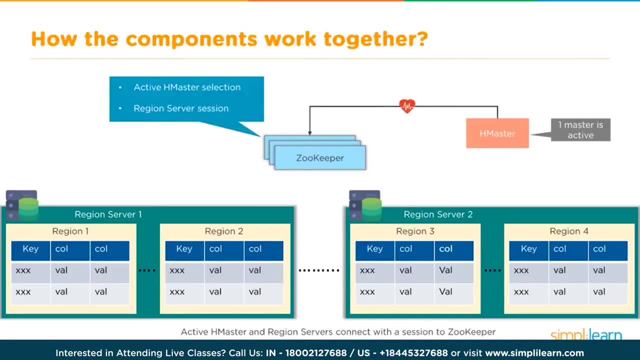 it will come to the rescue. Active HMaster and region servers connect with a session to ZooKeeper So you can see your active HMaster selection region server session. They're all looking at the ZooKeeper keeping that pulse. An active HMaster and region server connects. 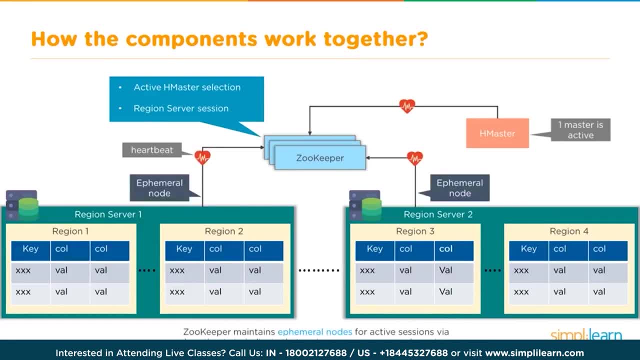 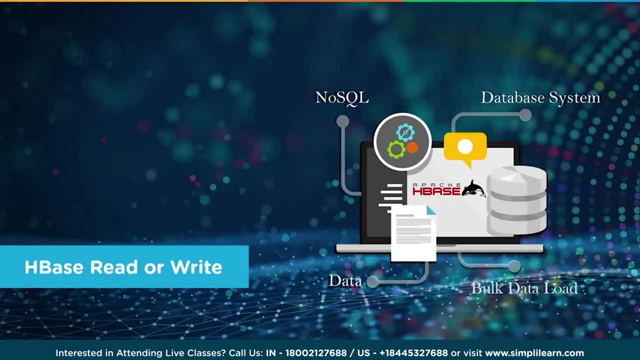 with a session to the ZooKeeper, And you can see here where we have ephemeral nodes for active sessions via heartbeats to indicate that the region servers are up and running. So let's take a look at HBase. read or write going on. There's a special HBase. 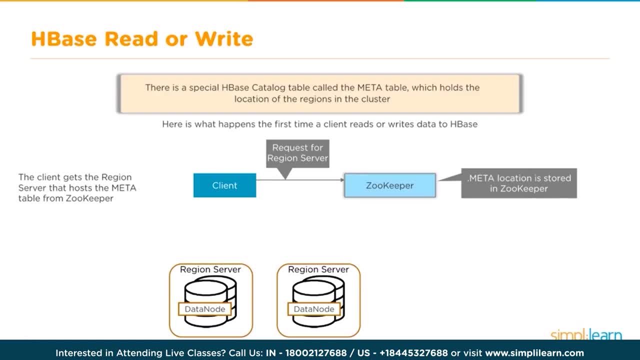 catalog table, called the meta table, which holds the location of the regions in the cluster. Here's what happens: the first time a client reads or writes data to HBase, The client gets the region server, the host, the meta table from ZooKeeper And you can see right here: 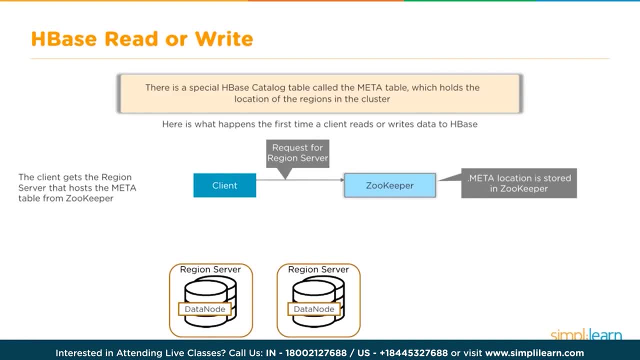 the client has a request for your region server and goes, hey, ZooKeeper, can you handle this? The ZooKeeper takes a look at it and goes, ah, meta location is stored in ZooKeeper, So it looks at its meta data on there. And then the meta data: 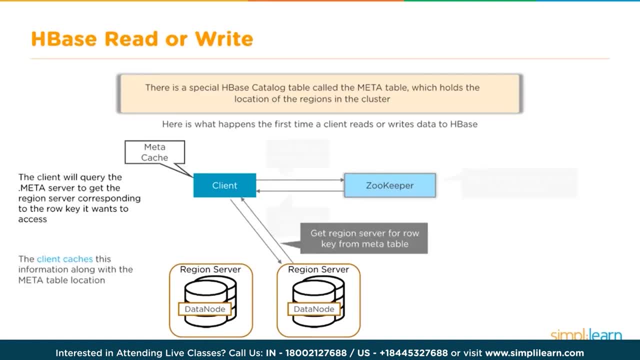 table location is sent back to the client. The client will query the meta server to get the region server corresponding to the row key if it wants to access. The client caches this information along with the meta table location And you can see here the client going back and forth to 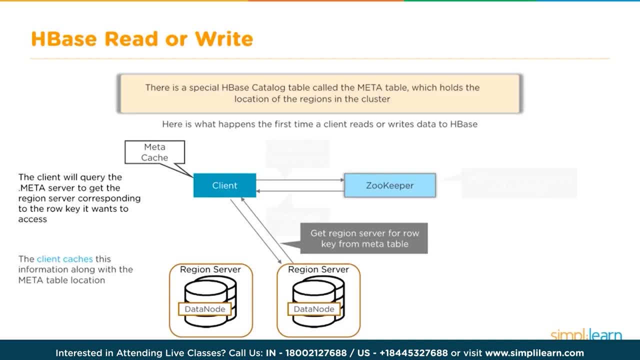 the region server with the information And it might be going across multiple region servers, depending on what you're querying. So we get the region server for row key from the meta table. That's where that row key comes in and says, hey, this is where we're going with this. 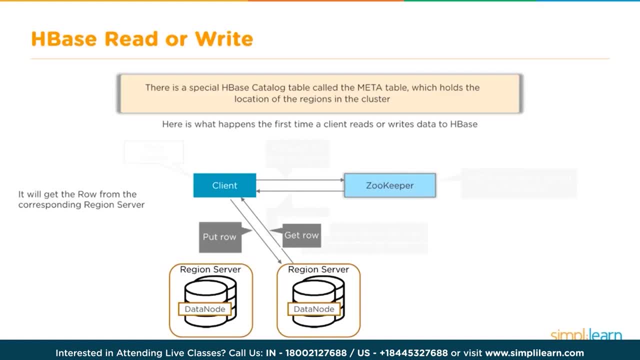 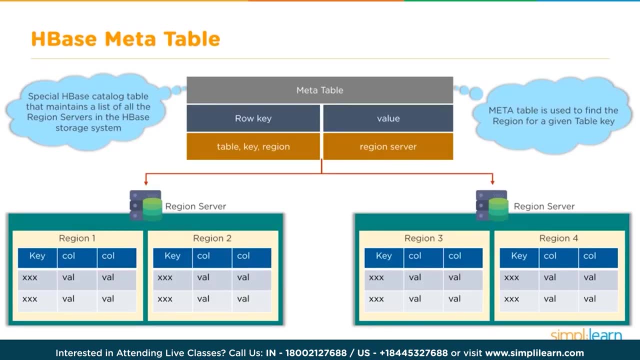 And so once it gets the row key from the corresponding region server, we can now put row or get row from that region server. Let's take a look at the HBase meta table, Special HBase catalog table that maintains a list of all the region servers. 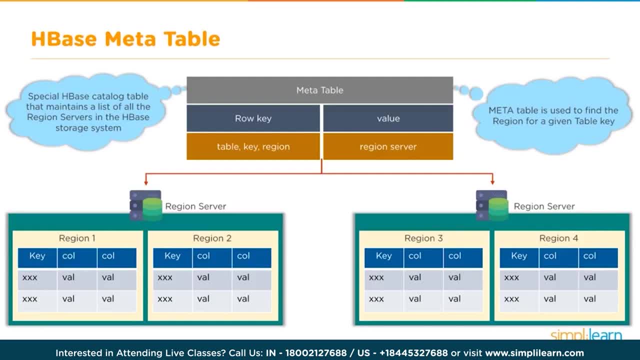 in the HBase storage system. So you see, here we have the meta table, We have a row key and a value table key, region, region server. So the meta table is used to find the region for the given table key And you can see. 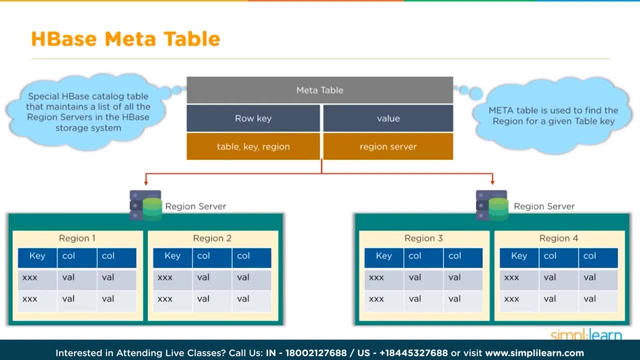 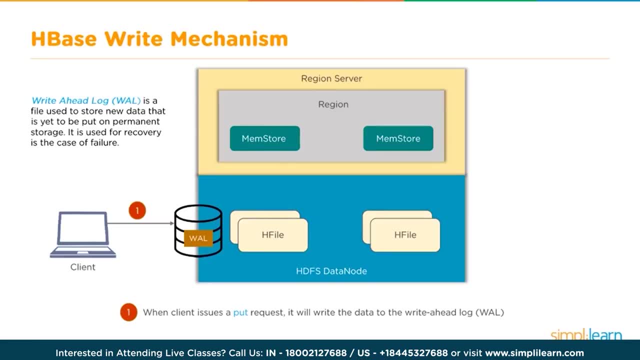 down here our meta table comes in and it's going to figure out where it's going with the region server And we look a little closer at the write mechanism. in HBase We have write ahead log or wall as you abbreviate it, Kind of a way to remember. 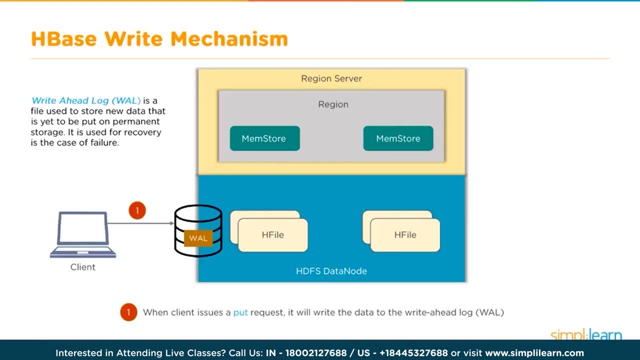 wall is write ahead log. It's a file used to store new data that is yet to be put on permanent storage. It is used for recovery in the case of failure, So you can see here where the client comes in and it literally puts the new data coming in into. 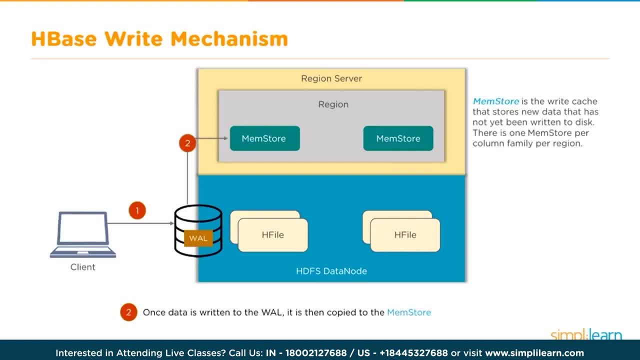 this kind of temporary storage or the wall on there Once it's gone into the wall. then the memory store memstore is the write cache that stores the new data that has not yet been written to disk. There is one memstore per column, family, per. 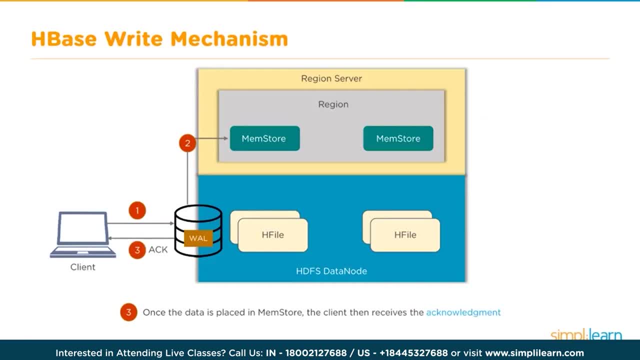 region. And once we've done that, we have three ACK. Once the data is placed in memstore, the client then receives the acknowledgement. When the memstore reaches the threshold, it dumps or commits the data into HFile. As you can see right here, we've taken 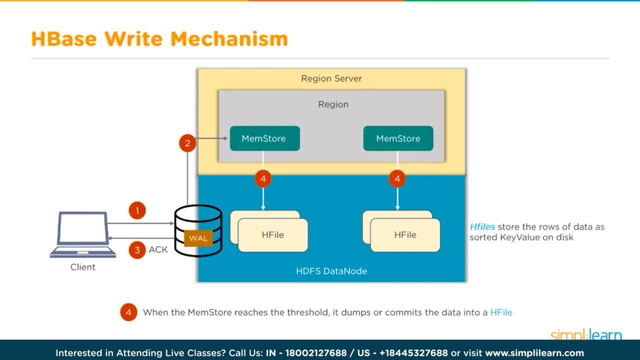 our. it's gone into the wall. The wall then sorts it into the different memory stores, And then the memory stores it says, hey, we've reached, we're ready to dump that into our HFiles. And then it moves it into the. 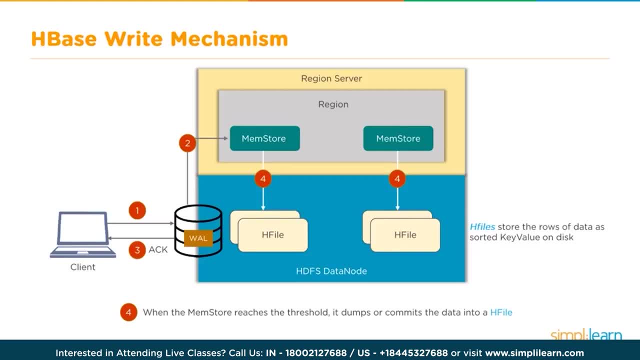 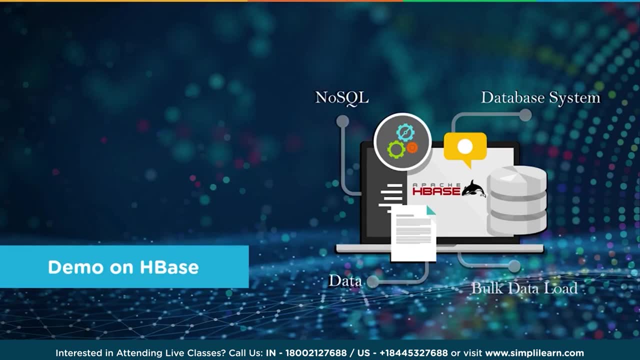 HFiles. HFiles store the rows of data as stored key value on disk. So here we've done a lot of theory. Let's dive in and just take a look and see what some of these commands look like and what happens in our HBase. 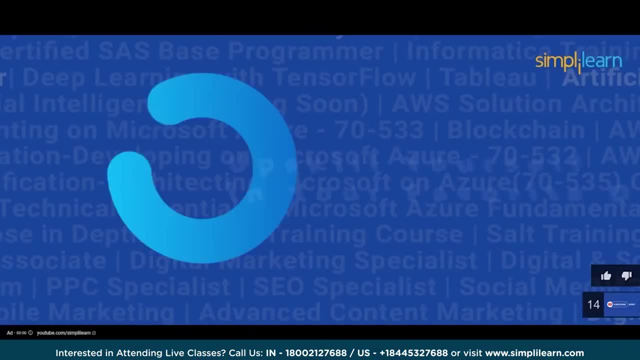 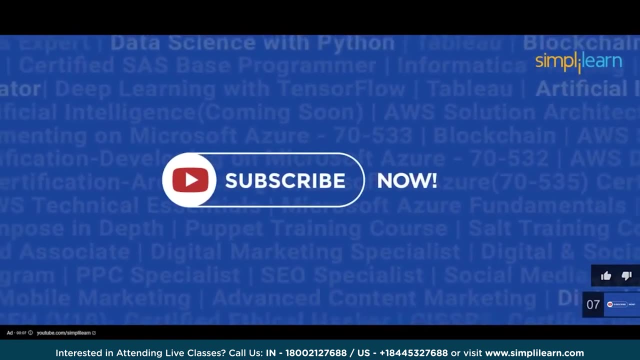 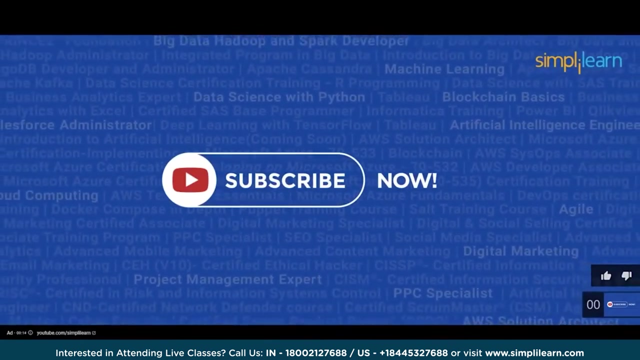 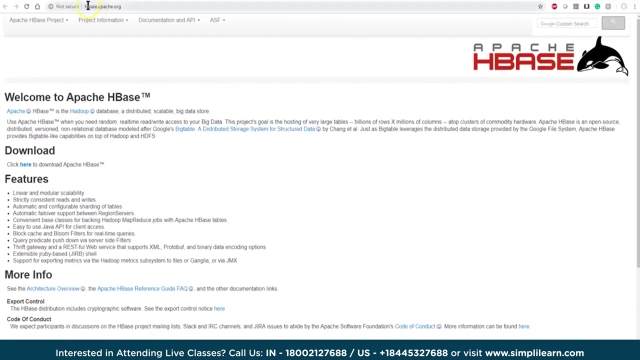 when we're manipulating a no SQL setup. So if you're learning a new setup, it's always good to start with. where is this coming from? It's open source by Apache And you can go to hbaseapacheorg And you'll see that. 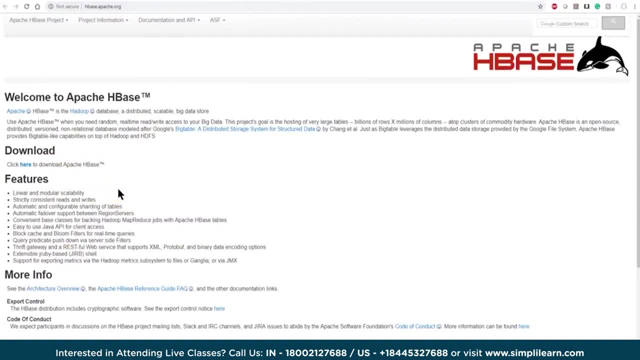 it has a lot of information. You can actually download the HBase separate from the Hadoop, although most people just install the Hadoop because it's bundled with it And if you go in here you'll find a reference guide And so you can. 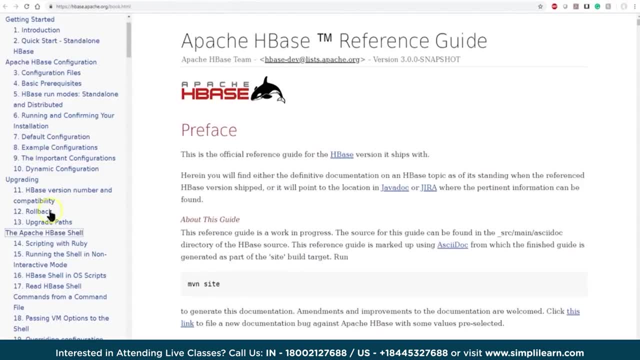 go through the Apache reference guide And there's a number of things to look at, but we're going to be going through Apache HBase shell. That's what we're going to be working with And there's a lot of other interfaces on the setup And you can look up a lot of. 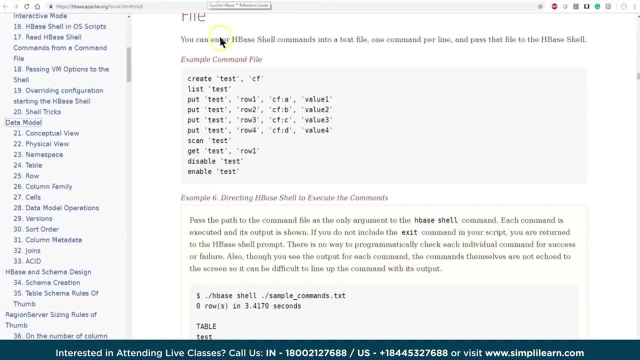 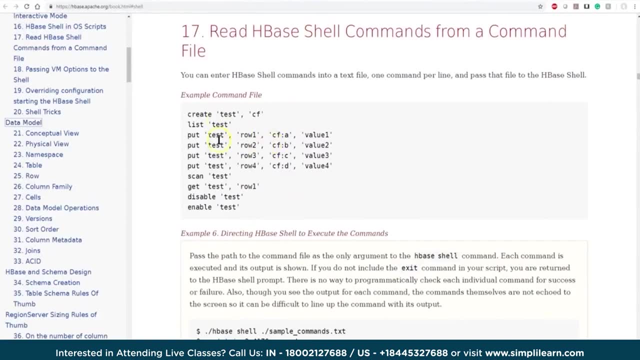 the different commands on here. So we go into the Apache HBase reference guide and we can go down to read HBase shell commands from a command file. You can see here where it gives you different options of formats for putting the data in and listing the data. 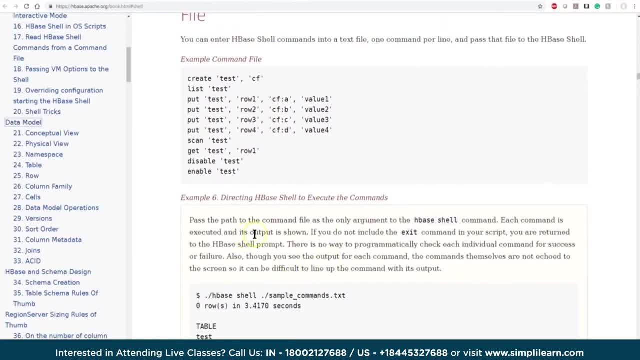 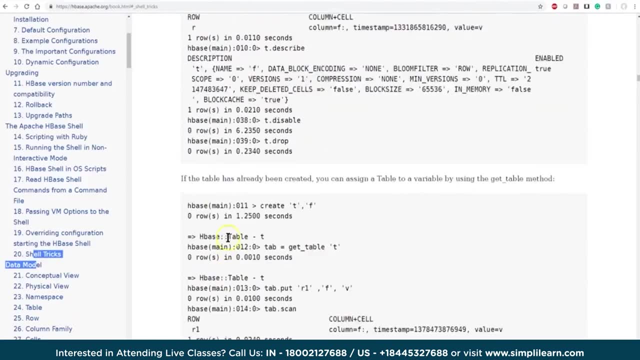 Certainly, you can also create files and scripts to do this too, But we're going to look at the basics. We're going to go through this on a basic HBase shell. And one last thing to look at is, of course, if you continue down, the 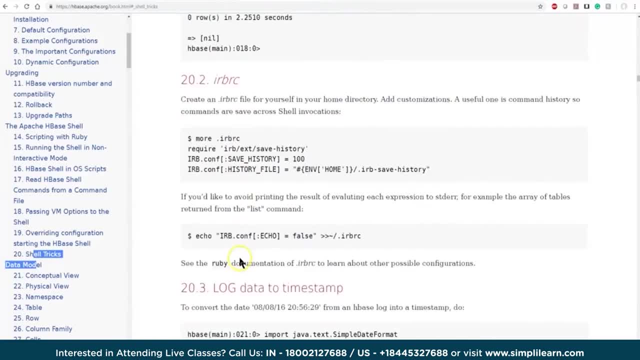 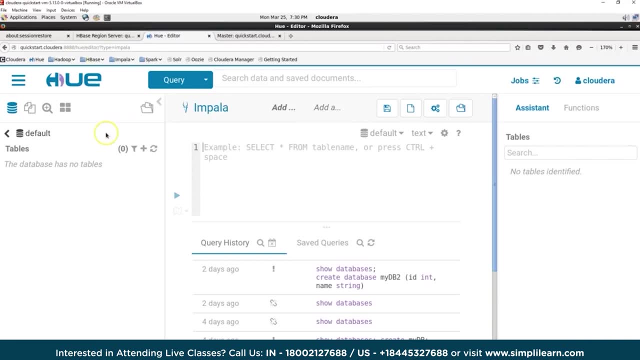 setup. you can see here where they have more detail as far as how to create and how to get to your data on your HBase. Now I will be working in a VirtualBox And this is by Oracle. You can download the Oracle VirtualBox. You can put a note in. 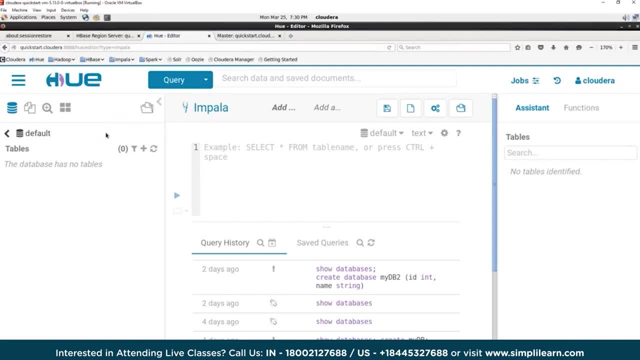 below for the YouTube, as we did have a previous session on setting up virtual setup to run your Hadoop system in there. I'm using the Cloudera QuickStart installed in here. There's Horton's. You can also use the Amazon Web Service. There's a number of options for. 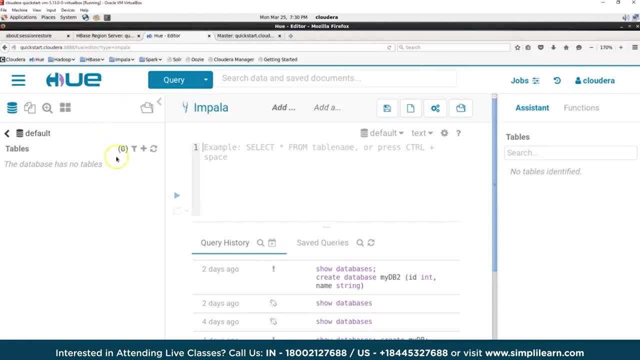 trying this out. In this case we have Cloudera on the Oracle VirtualBox. The VirtualBox has Linux CentOS installed on it, And then the Hadoop has all the different Hadoop flavors, including HBase, And I bring this up because my computer is a. 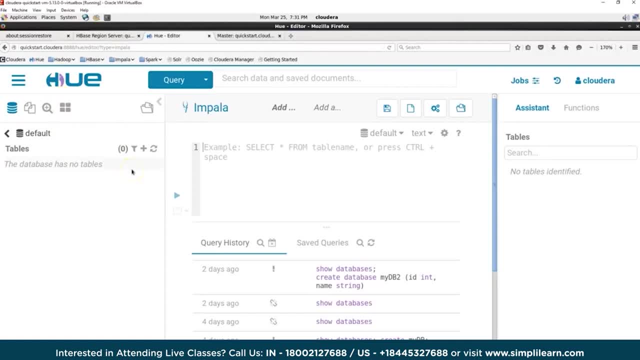 Windows 10.. The operating system of the VirtualBox is Linux And we're looking at the HBase data warehouse And so we have three very different entities all running on my computer And that can be confusing if it's the first time in and working with this kind of setup. 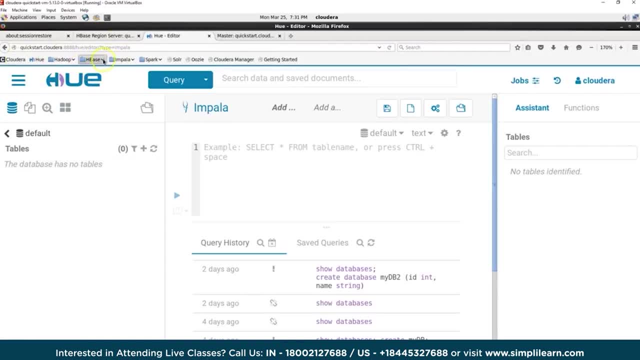 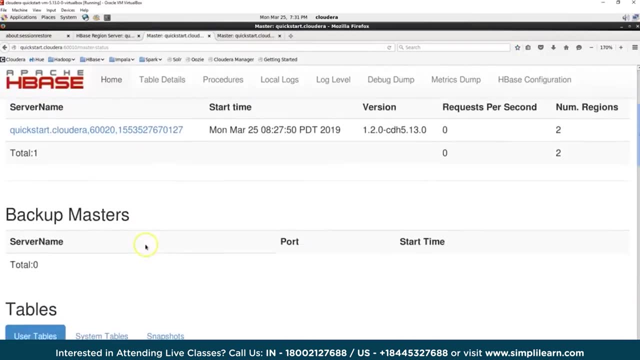 Now you'll notice in our Cloudera setup they actually have some HBase monitoring. So I can go underneath here and click on HBase and Master And it will tell me what's going on with my region servers. It will tell me what's going on with 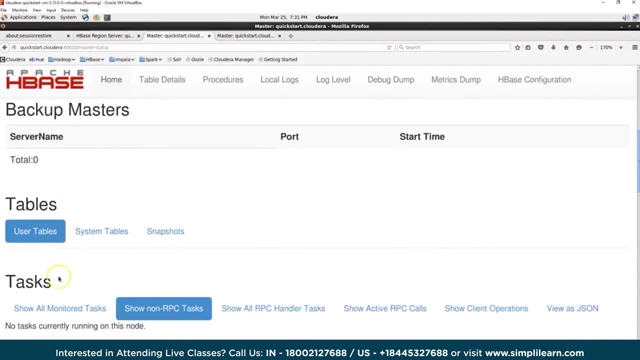 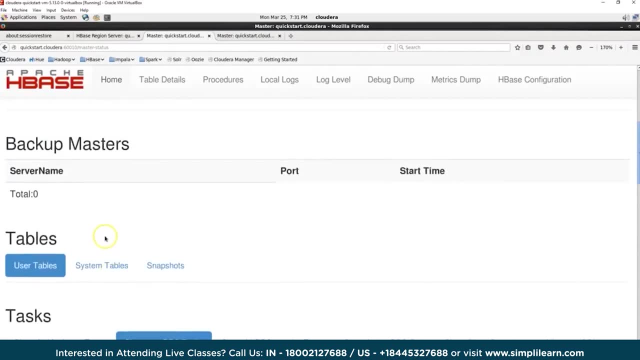 our backup Tables. Right now I don't have any user tables because we haven't created any, And this is only a single node and a single HBase, Tor, So you're not going to expect anything too extensive in here. since this is for practice and education and 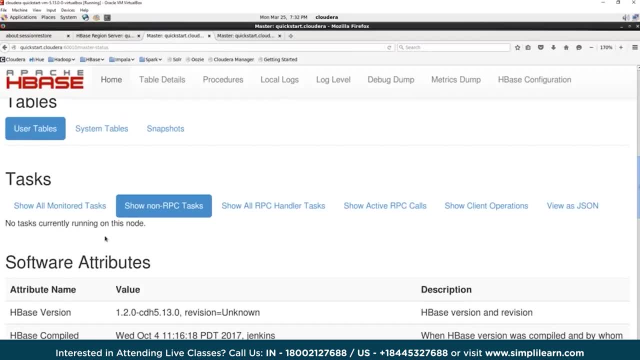 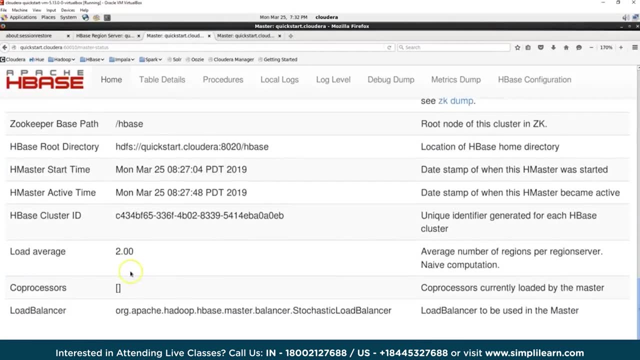 perhaps testing out the package you're working on. It's not for really. You can deploy Cloudera, of course, But when you talk about a quick start or a single node setup, that's what it's really for. So we can go through all the different HBase and you'll see all kinds. 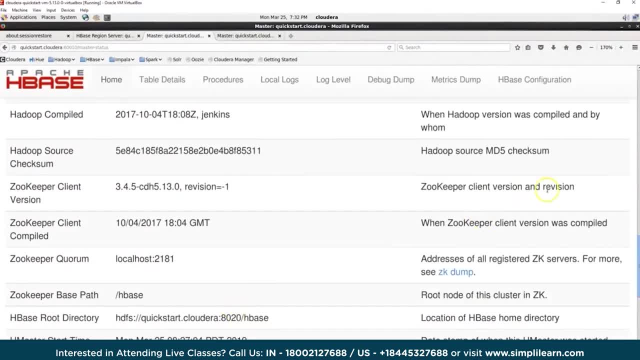 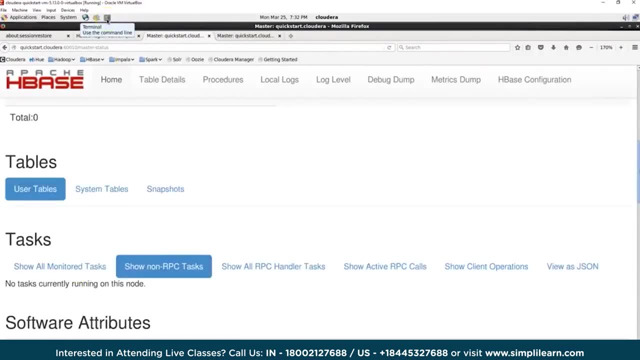 of different information with Zookeeper- if you saw it flash by down here What version we're working in, since Zookeeper is part of the HBase setup. Where we want to go is we want to open up a terminal window, And in Cloudera it happens to be. 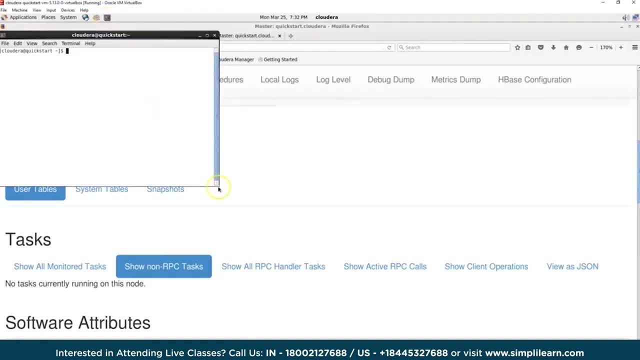 up at the top, And when you click on here you'll see your Cloudera terminal window open. And let me just expand this so we have a nice full screen, And then I'm also going to zoom in. That way I have a nice. 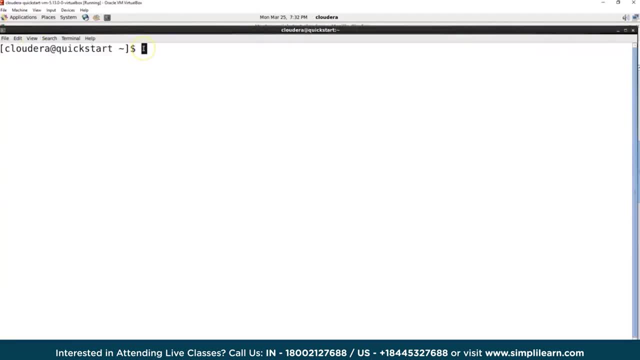 big picture and you can see what I'm typing and what's going on. And to open up your HBase shell, simply type HBase shell to get in And hit enter And you'll see. it takes just a moment to load And we'll be in our 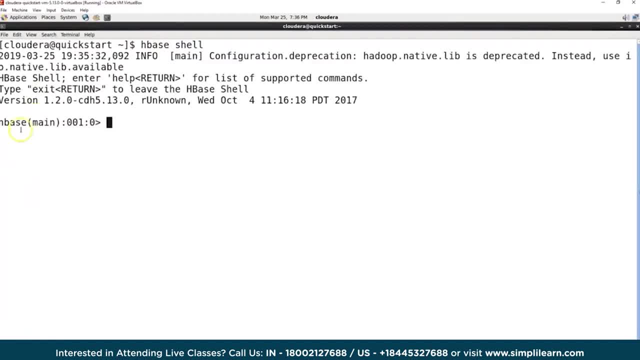 HBase shell for doing HBase commands. Once we've gotten into our HBase shell, you'll see you'll have the HBase prompt information ahead of it. We can do something simple like list, And this is going to list whatever tables we have. 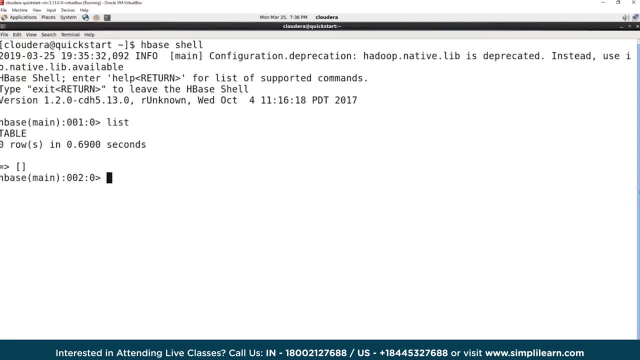 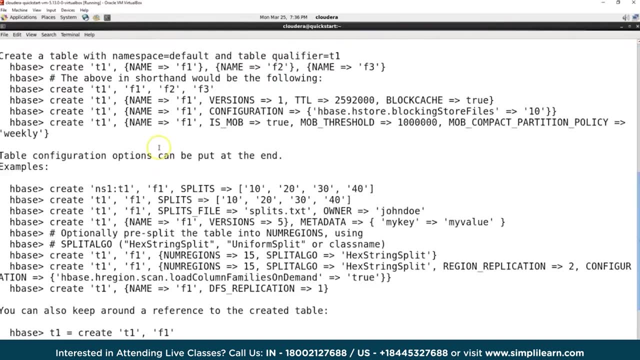 And it so happens that there's a base table that comes with HBase. Now we can go ahead and create, And I'm going to type in: just create. What's nice about this is it's going to throw me kind of a. it's going to say, hey, there's no, just 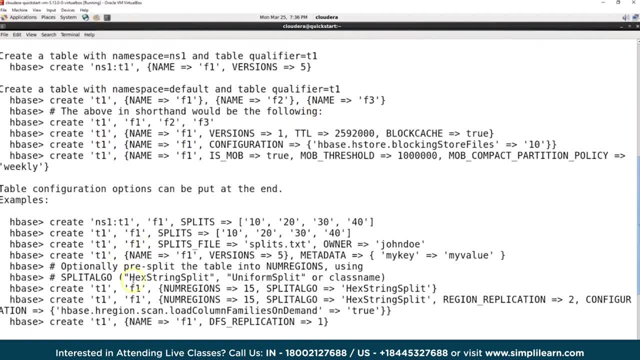 straight create, But it does come up and tell me all these different formats we can use for create, So we can create our table and one of our families. You can add splits, names, versions, all kinds of things you can do with this. But let's just start with a very 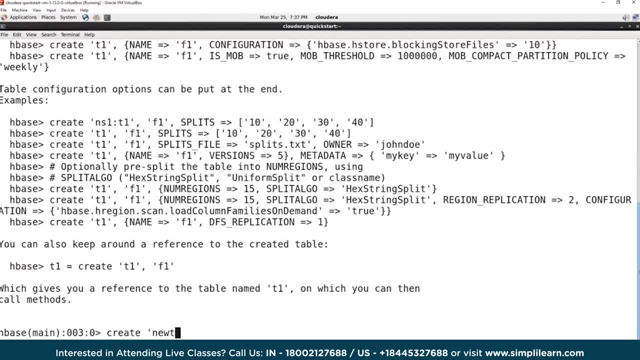 basic one on here And let's go ahead and create and we'll call it new table, Let's just call it new TBL for table, New table. And then we also want to do, let's do- knowledge. So let's take a look at this. I'm creating a new. 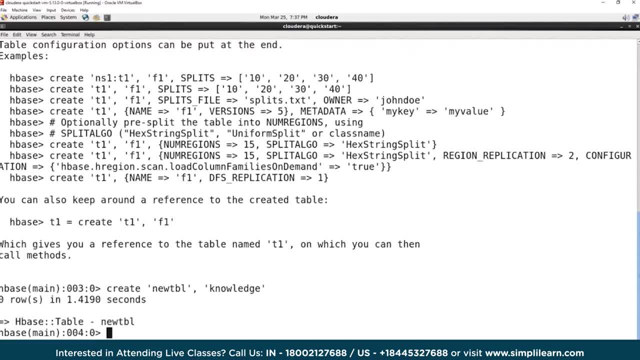 table and it's going to have a family of knowledge in it. And let me hit enter, It's going to come up and it's going to take it a second to go ahead and create it. Now we have our new table in here, So if I go list, you'll. 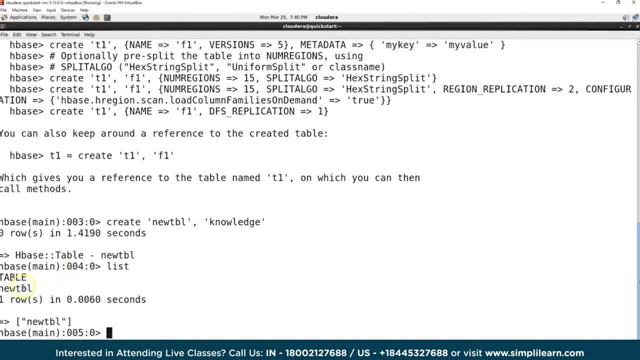 now see table and new table. So you can now see that we have the new table and, of course, the default table That's set up in here And we can do something like describe, We can describe, and then we're going to do new TBL, And when we describe it, 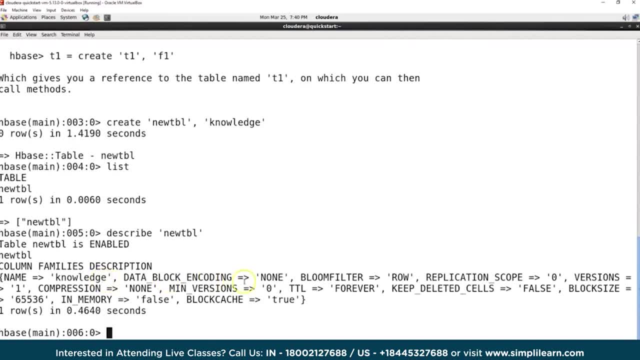 it's going to come up. It's going to say: hey name, I have knowledge. data block encoding none. bloom filter, row replication, scope, version, All the different information you need. New minimum version: zero, forever deleted cells: false. 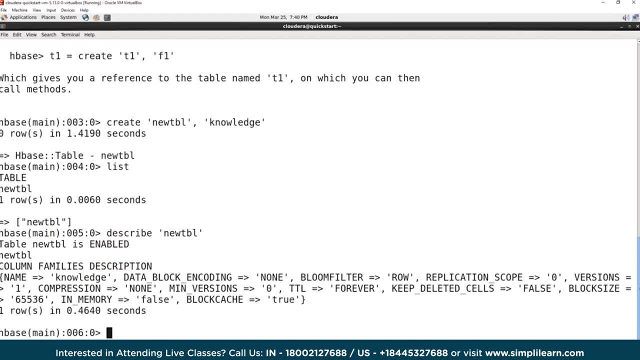 block size in memory And you can look this stuff up on Apacheorg to really track it down. One of the things that's important to note is versions, So you have your different versions of the data that's stored, And that's always important to understand. 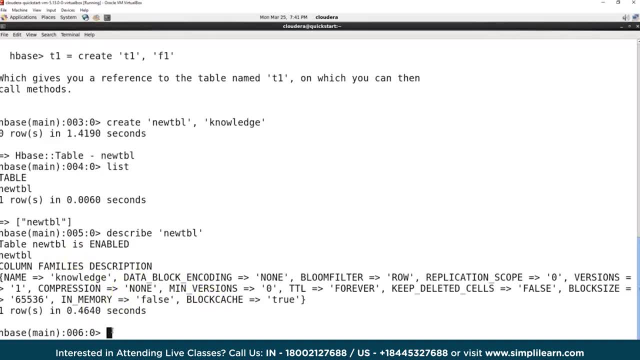 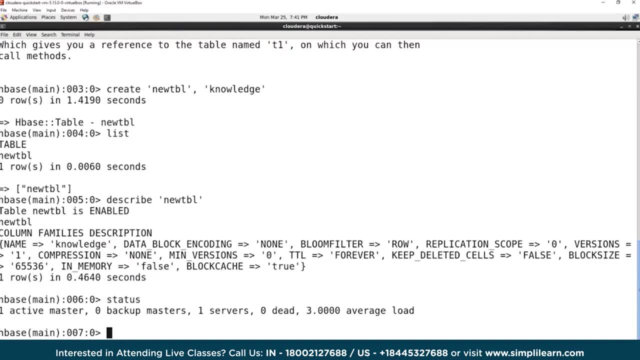 that We might talk about that a little bit later on. And then we have to describe it. We can also do a status. The status says I have one active master going on. That's our HBase as a whole. We can do status. 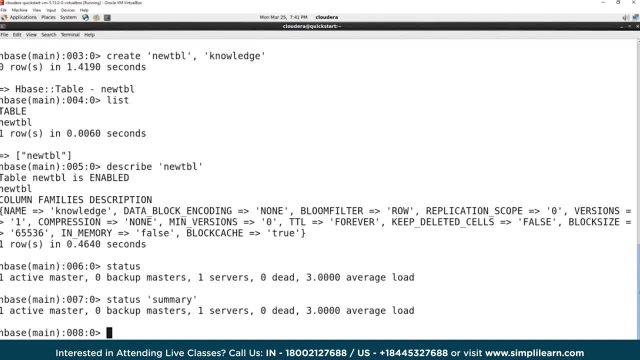 summary, And it should do the same thing as status. So we got the same thing coming up And now that we've created it, let's go ahead and put something in it. So we're going to put new TBL and then we want row one. You know what, before I even do? 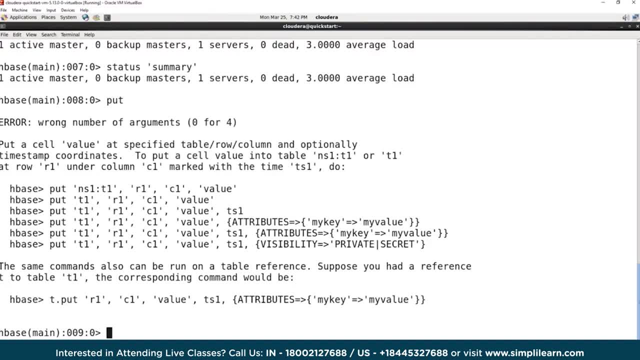 this. let's just type in put And you can see. when I type in put, it gives us like a lot of different options of how it works and different ways of formatting our data as it goes in, And all of them usually begin with the new. 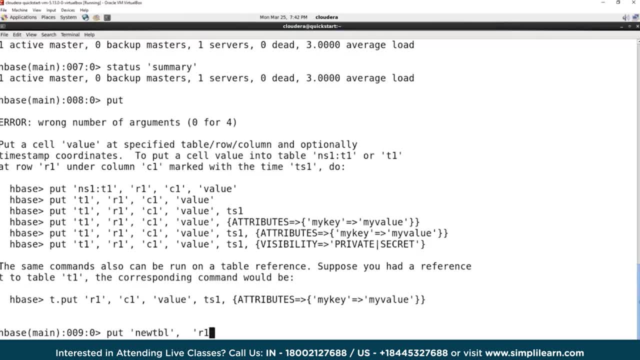 table New TBL, Then we have- in this case we'll call it row one, And then we'll have knowledge. Remember, we created knowledge already And we'll do knowledge sports. And then, in knowledge and sports, we're going to set that equal to. 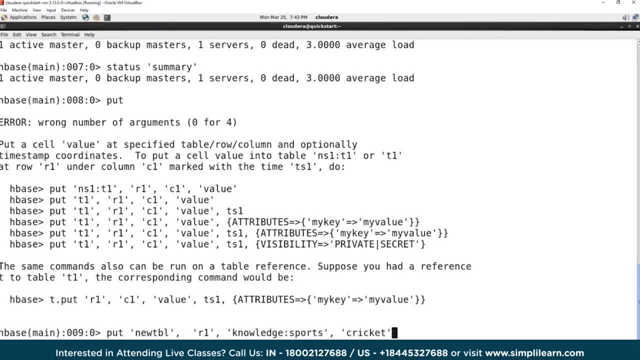 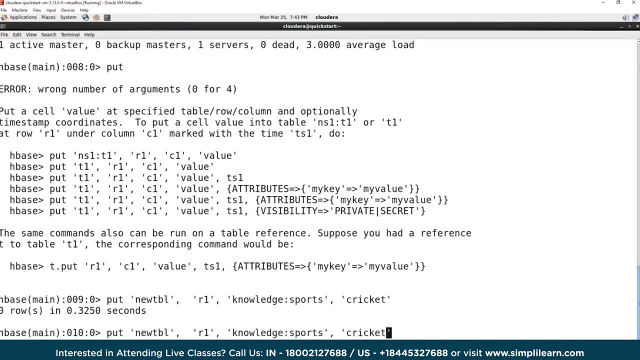 cricket. So we're going to put underneath this our knowledge setup. We have a thing called sports in there And we'll see what this looks like in just a second. Let's go ahead and put in. we'll do a couple of these, Let's see. let's do another. 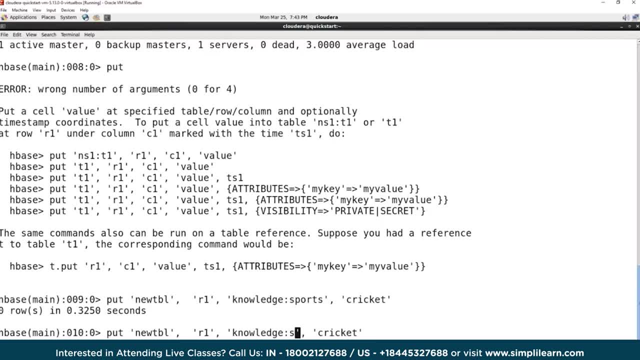 row one, and this time, instead of sports, let's do science. This person not only. we have row one which is both knowledgeable in cricket and also in chemistry. So it's a chemist who plays cricket in row one, And let's see if we have, let's do another row. 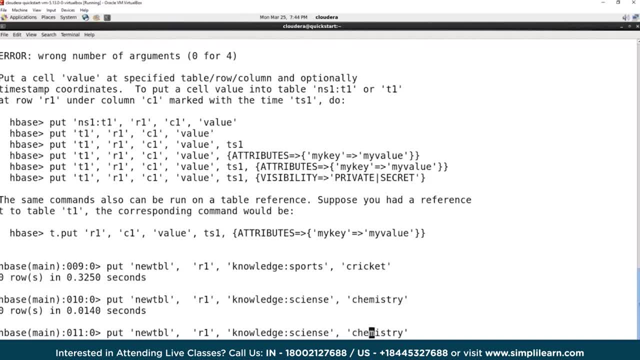 one just to keep it going. And we'll do science. In this case, let's do physics, Not only in chemistry, but also physicists. I have quite a joy in physics myself. So here we go. We have row one, There we go, And then let's. 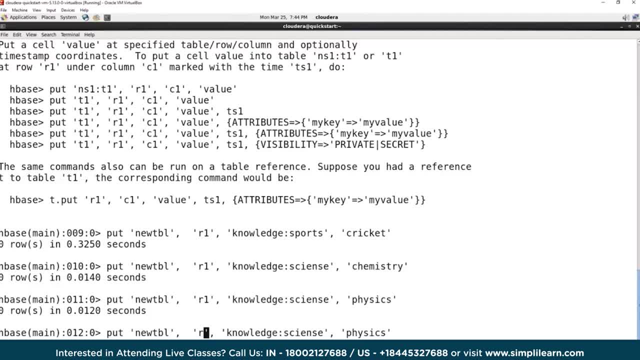 do row two. Let's see what that looks like when we start putting in row two. And in row two this person is: has knowledge in economics. This is a master of business and how, or maybe it's global economics, Maybe it's just for. 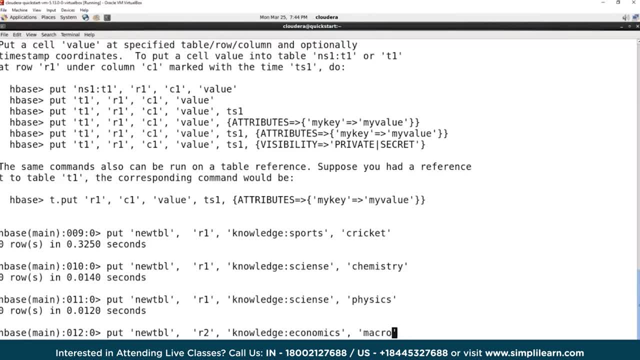 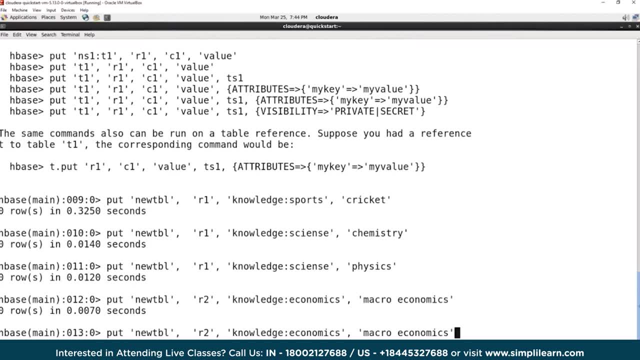 the business and how it fits in with the country's economics, And we'll call it macroeconomics. So I guess it is for the whole country there. So we have knowledge, economics, macroeconomics, And then let's just do one more. We'll keep it as. 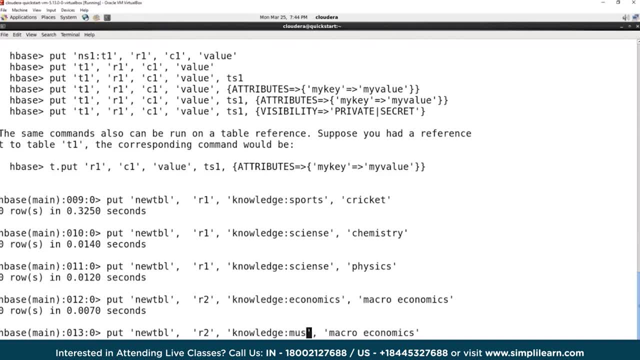 row two, And this time our economist is also a musician, So we'll put music. And they happen to have knowledge and they enjoy. oh, let's do pop music. They're into the current pop music going on. So we've loaded our database. 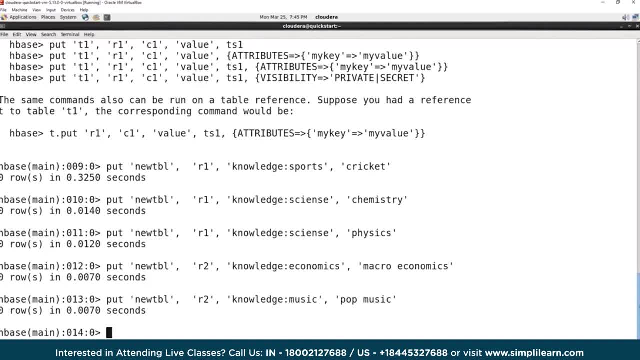 And you'll see, we have two rows, Row one and row two, in here, And what we can do is we can list the contents of our database by simply doing scan, Scan and then let's just do scan by itself. so you can see how that. 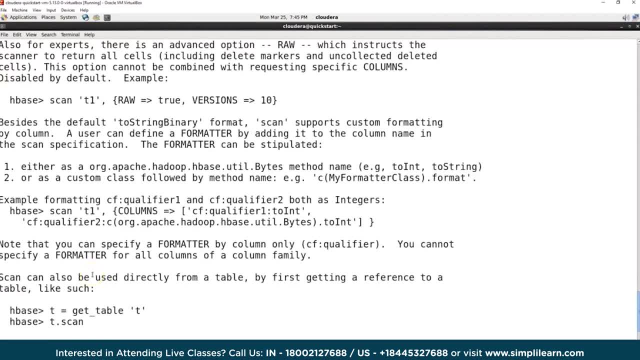 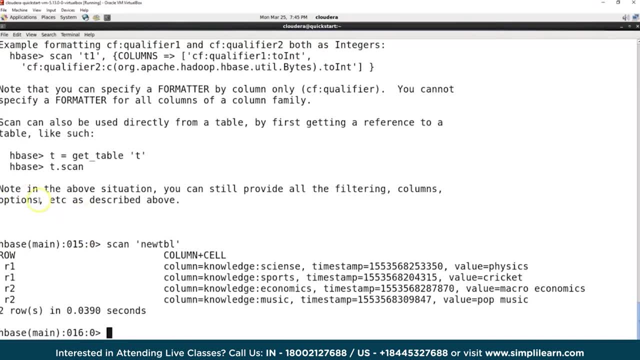 looks. You can always just type in there and it tells you all the different setups you can do with scan and how it works. In this case we want to do scan new TBL And in our scan new TBL we have row one row one row. 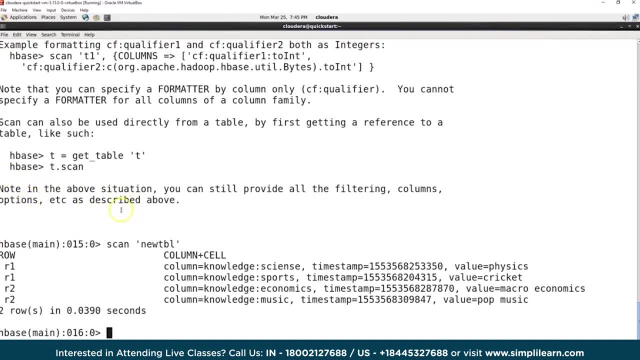 two. row two And you'll see. row one has a column called knowledge, science, time step, value, crickets, Value physics, So it has information as to when it was created, when the time stamp is. Row one also has knowledge sports and a value of cricket, So we have 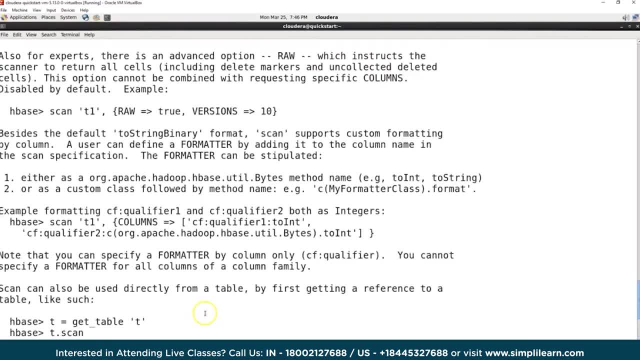 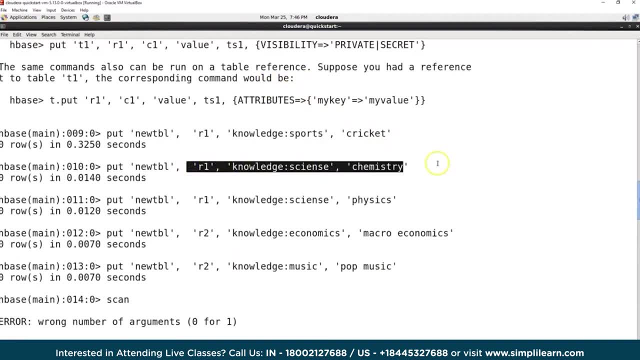 sports and science. And this is interesting because, if you remember, up here we also gave it originally. we told it to come in here and have chemistry. We had science, chemistry and science, physics, And we come down here. I don't see the chemistry. Why? 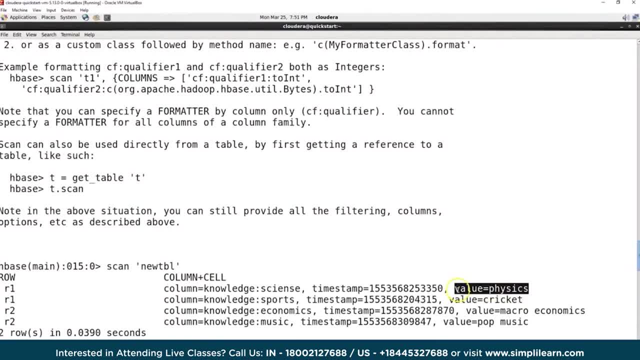 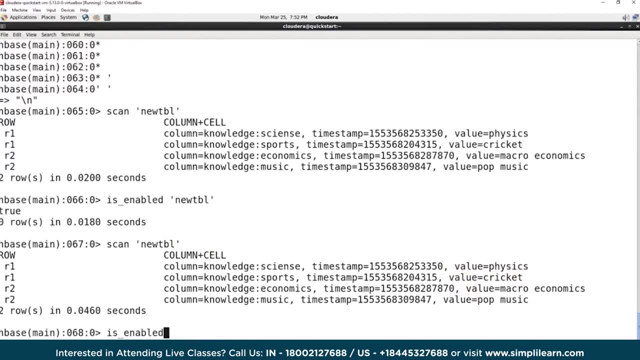 Because we've now replaced chemistry with physics, So the new value is physics. on here, Let me go ahead and clear it down a little bit, And in this we're going to ask, the question is enabled: new table. When I hit enter in here, you're going to see: 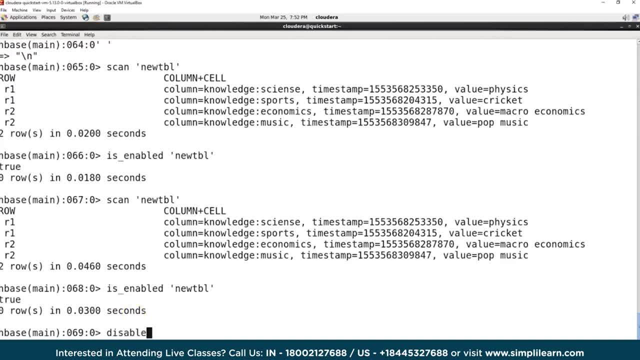 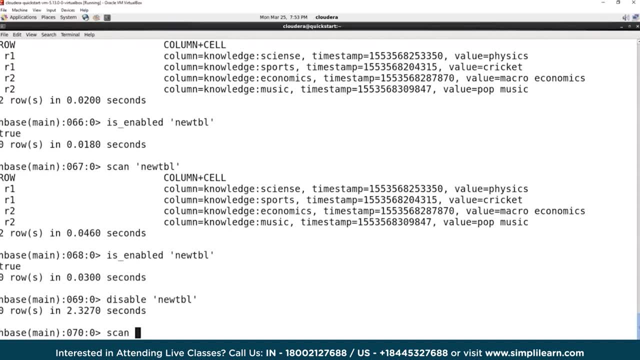 it comes out true, And then we'll go ahead and disable it. Let's go ahead and disable new table. Make sure I have our quotes around it. And now that we've disabled it, what happens when we do the scan? When we do the scan new? 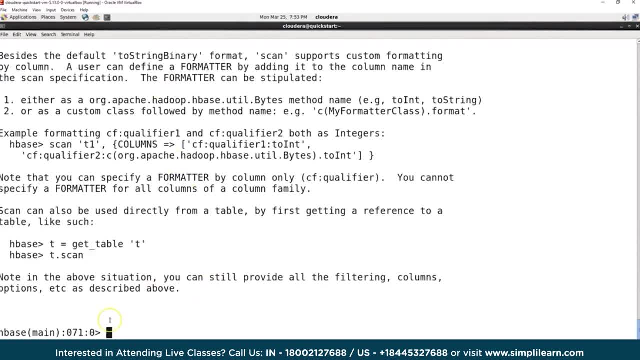 table. I hit enter, you're going to see that we get an error coming up. So once it's disabled, you can't do anything with it until we re-enable it. Now, before we enable the table, let's do an alteration on it. 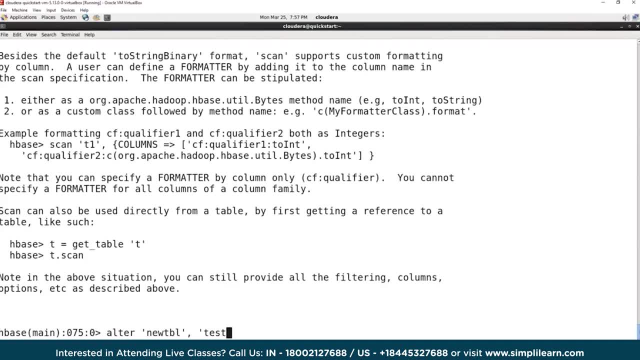 Here's our new table And this should look a little familiar because it's very similar to create. We'll call this test info, We'll hit enter in there, It'll take just a moment for updating And then we want to go ahead and. 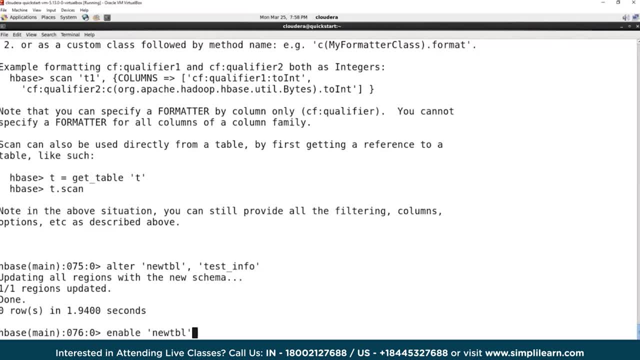 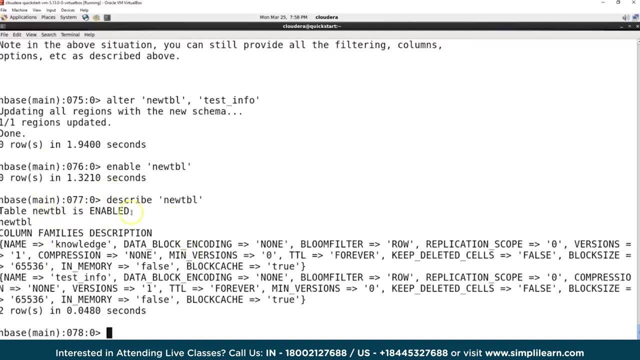 enable it. So let's go ahead and enable our new table, So it's back up and running And then we want to describe, Describe new table And we come in here. you'll now see we have name, knowledge And under there, 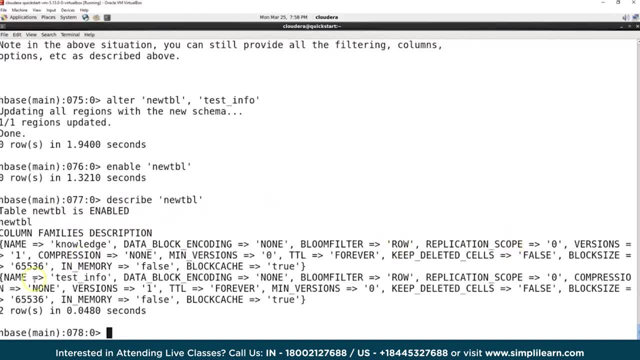 we have our data encoding and all the information under knowledge, And then we also have down below test info. So now we have the name test info And all the information concerning the test info on here And we'll simply enable it. New table. So now. 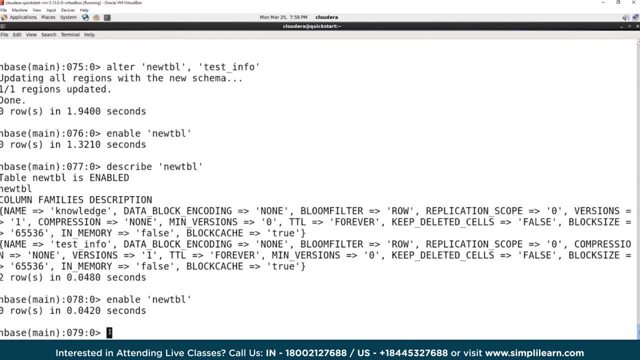 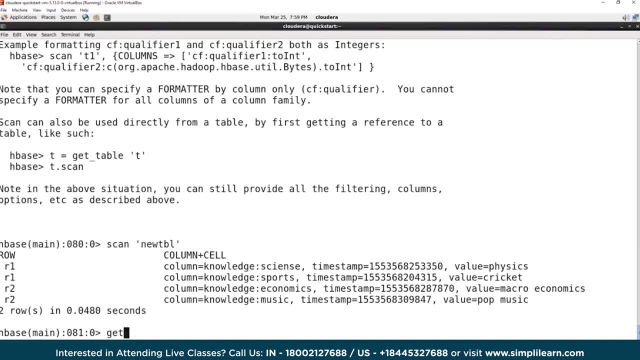 it's enabled. Oops, I already did that. I guess we'll enable it twice. And so let's start looking at. well, we had scan new table And you can see here where it brings up the information like this: But what if we want to go ahead and get? 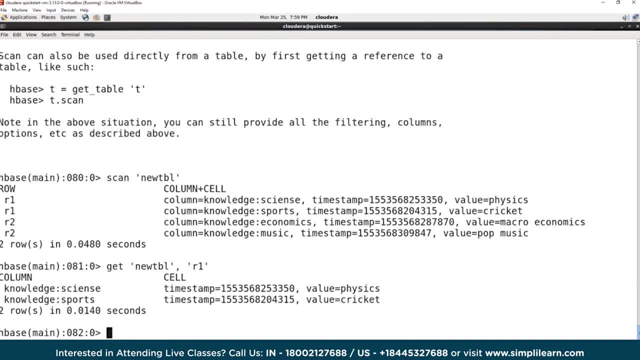 a row, So we'll do r1.. And when we do hbase r1, you can see we have knowledge science and it has a timestamp Value physics. And we have knowledge sports and it has a timestamp on it And value cricket. And then let's see what happens. 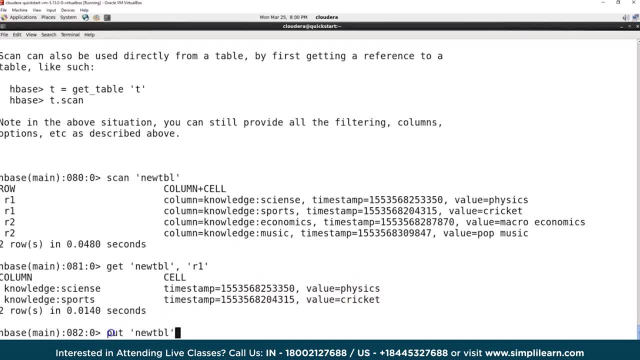 when we put into our new table, And in here we want row 1. And if you can guess from earlier, because we did something similar- We're going to do knowledge economics And then it's going to be a sort of- I think it was what- macro economics. 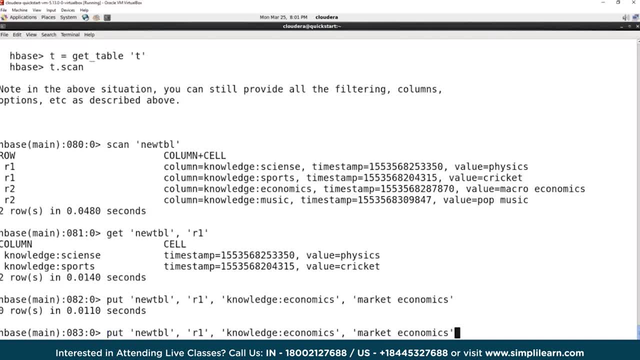 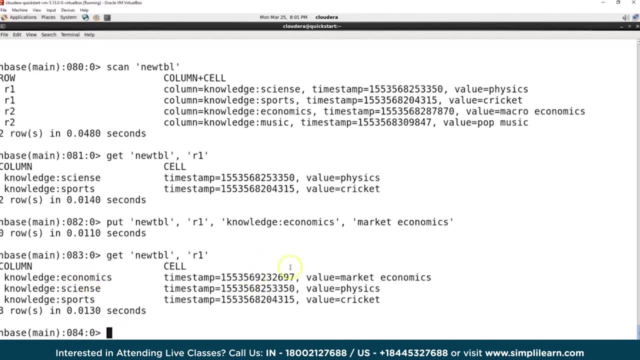 It's now market economics And we'll go back and do our git command And now see what it looks like And we can see here where we have knowledge economics- It has a timestamp Value- market economics, Physics and cricket, And this is because we have 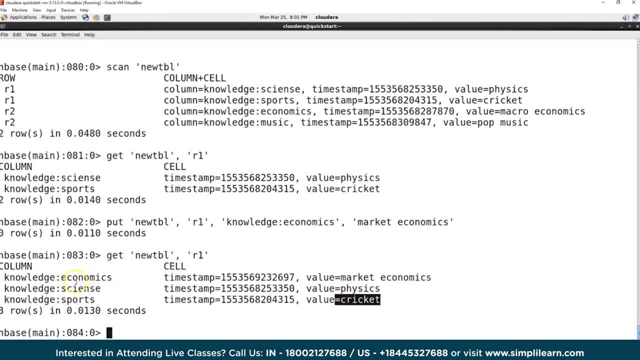 economics, science and sports. Those are the three different columns that we have, And then each one has different information in it, And so if you manage to go through all these commands and look at basics on here, You'll now have the ability. 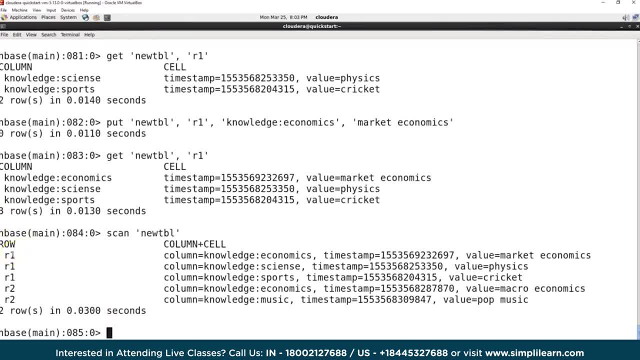 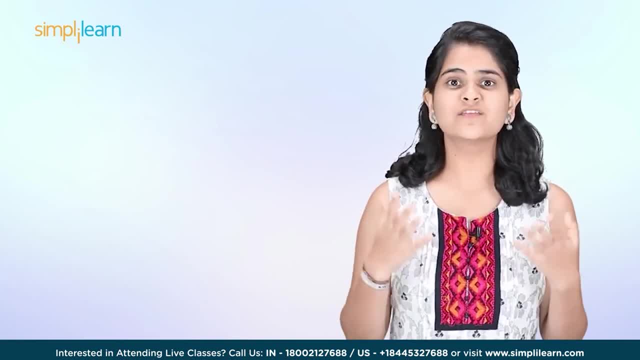 to create a very basic HBase setup- No SQL setup- Based on your columns and your rows. Thank you, guys. Now that we're done with Hadoop ecosystem, we have Shruti, who will take us to big data applications. Before we move on to the applications, 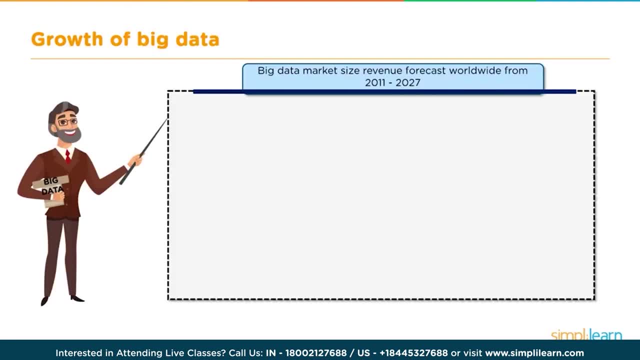 let's have a quick look at the big data market revenue forecast worldwide from 2011 to 2027.. So here's a graph in which the Y axis represents the revenue in billion US dollars and the X axis represents the years As it is seen clearly from: 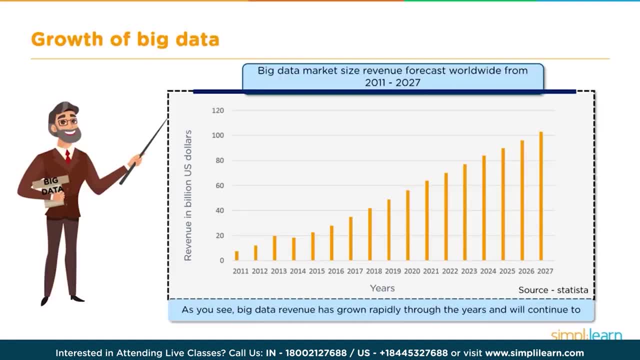 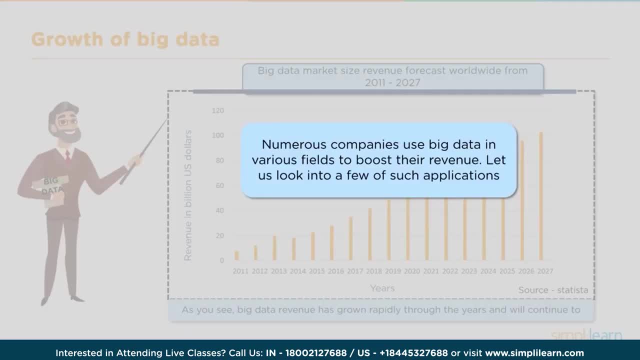 the graph. big data has grown until 2019.. And statistics predict that this growth will continue even in the future. This growth is made possible as numerous companies use big data in various domains to boost their revenue. We will look into few of such applications. 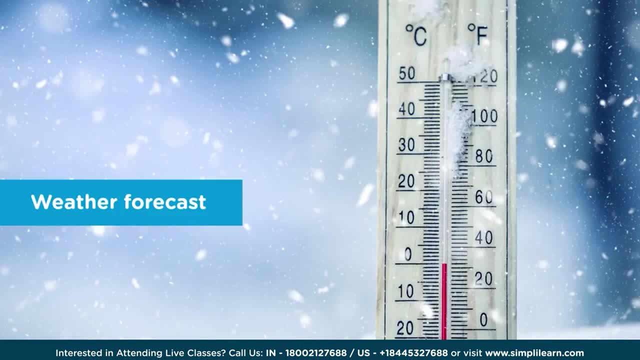 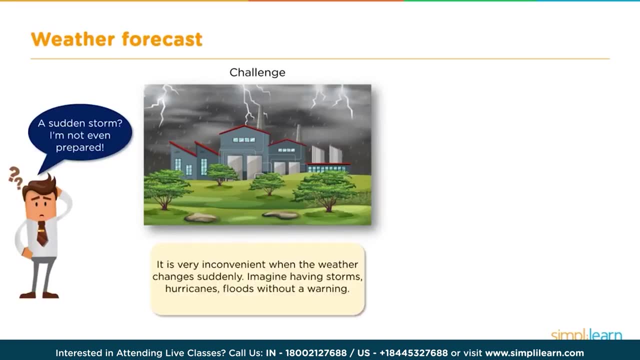 The first big data application we will look into is weather forecast. Imagine there is a sudden storm and you're not even prepared. That would be a terrifying situation, isn't it? Dealing with any calamities, such as hurricanes, storms, floods, would be very inconvenient if we are. 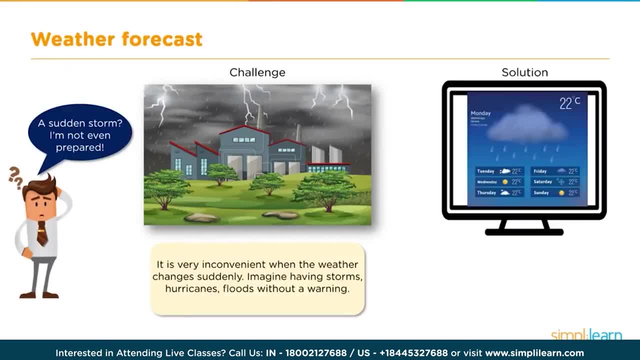 caught off guard. The solution is to have a tool that predicts the weather of the coming days well in advance. This tool needs to be accurate, and to make such a tool, big data is used. So how does big data help here? Well, it allows us to. 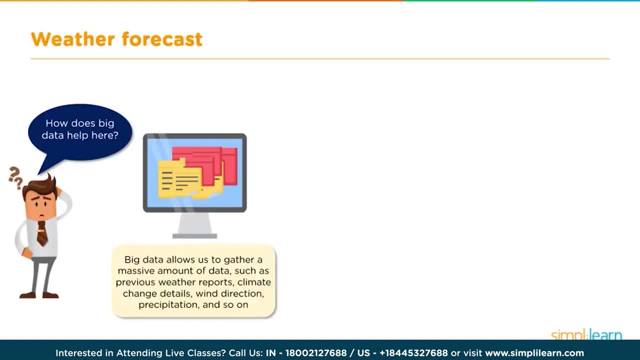 gather all the information required to predict the weather, Information such as the climate change details, wind direction, precipitation, previous weather reports and so on. After all this data is collected, it becomes easier for us to spot a trend and identify what's going. 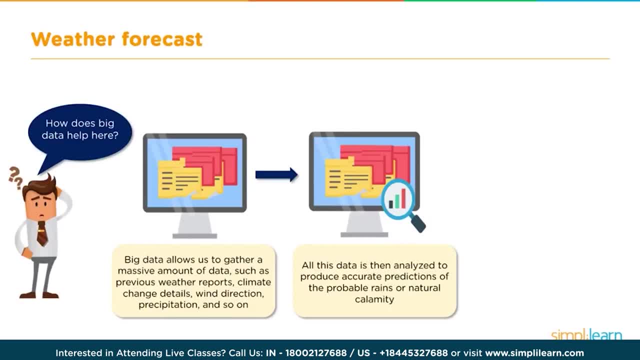 to happen next by analyzing all of this big data. A weather prediction engine works on this analysis. It predicts the weather of every region across the world for any given time. By using such a tool, we can be well prepared to face any climate change. 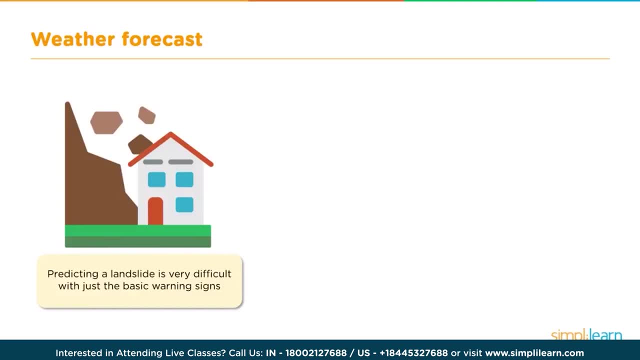 or any natural calamity. Let's take an example of a landslide and try to understand how big data is used to tackle such a situation. Predicting a landslide is very difficult with just the basic warning signs. Lack of this prediction can cause a huge damage. 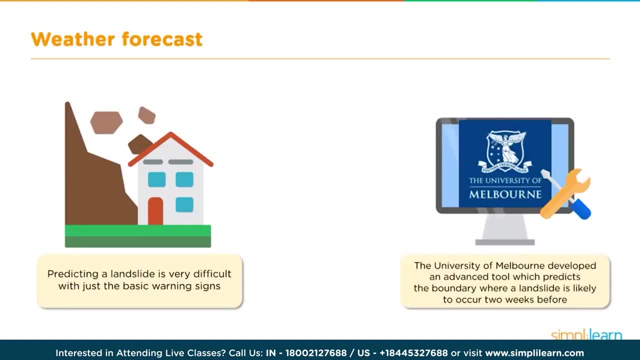 to life and property. This challenge was studied by the University of Melbourne and they developed a tool which is capable of predicting a landslide. This tool predicts the boundary where a landslide is likely to occur two weeks before. This magical tool works on both big data and applied mathematics. 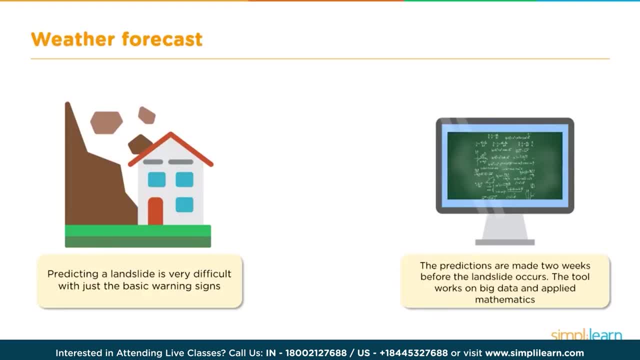 An accurate prediction like this, which is made two weeks before, can save lives and help in relocating people in that particular region. It also gives us an insight into the magnitude of the upcoming destruction. This is how big data is used in weather forecast and in predicting. 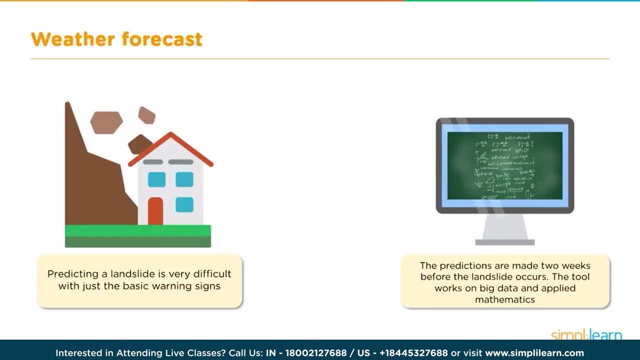 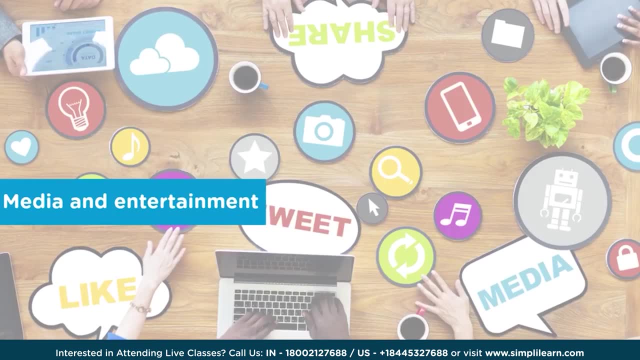 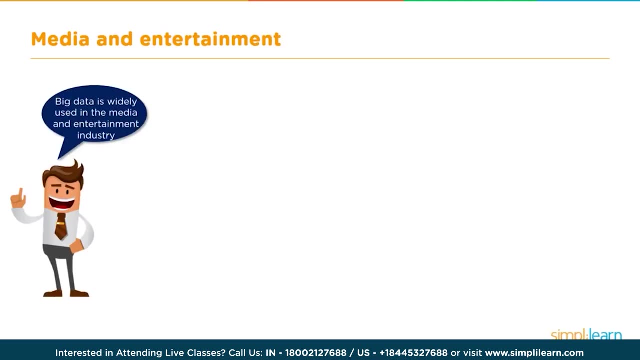 any natural calamities across the world. Let us now move on to our next application, that is, big data application in the field of media and entertainment. The media and the entertainment industry is a massive one. Leveraging big data here can produce sky high results and boost the revenue for. 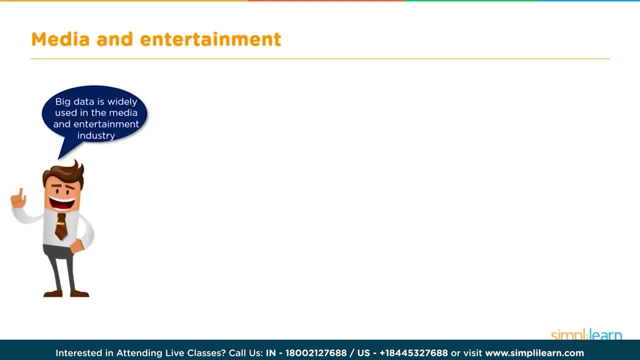 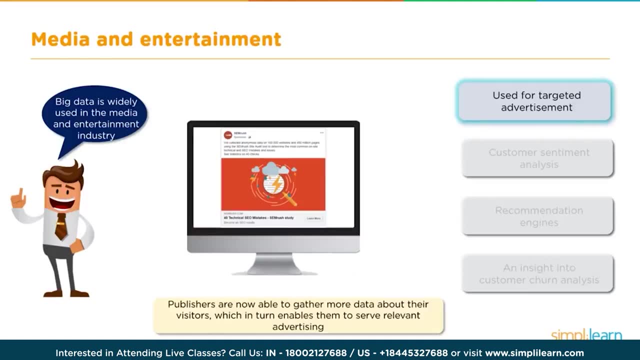 any company. Let us see the different ways in which big data is used in this industry. Have you ever noticed that you come across relevant advertisements in your social media sites and in your mailboxes? Well, this is done by analyzing all your data, such as your previous browsing. 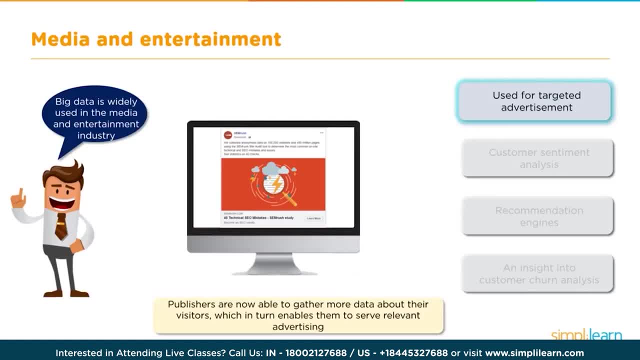 history and your purchase data. Publishers then display what you like in the form of ads, which will in turn catch your interest in looking into it. Next up is customer sentiment analysis. Customers are very important for a company. The happier the customer, the greater the company's. 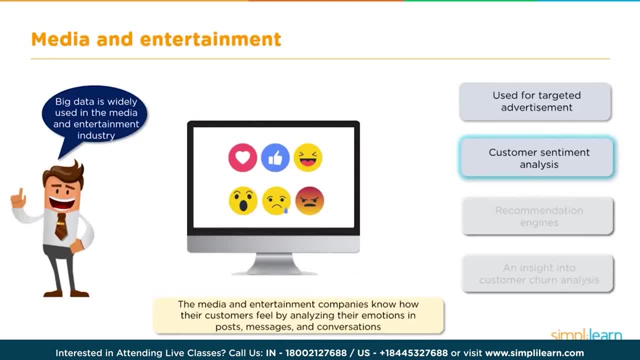 revenue. Big data helps in gathering all the emotions of a customer, through their posts, messages, conversations, etc. These emotions are then analyzed to arrive at a conclusion regarding the customer's satisfaction. If the customer is unhappy, the company strives to do better the next time and provides. 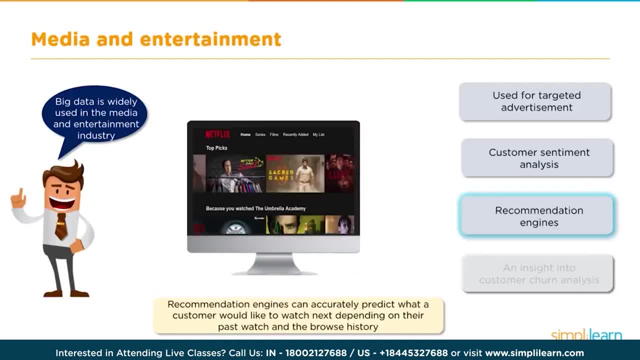 their customers a better experience. While purchasing an item from an e-commerce site or while watching videos on an entertainment site, you might have noticed a segment which says most recommended list for you. This list is a personalized list which is made available to you by analyzing all 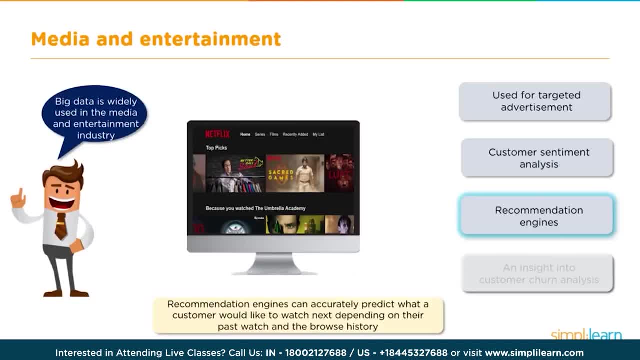 the data such as your previous watch history, your subscriptions, your likes and so on. Recommendation engine is a tool that filters and analyzes all this data and provides you with a list that you would most likely buy. By doing so, the site is able to. 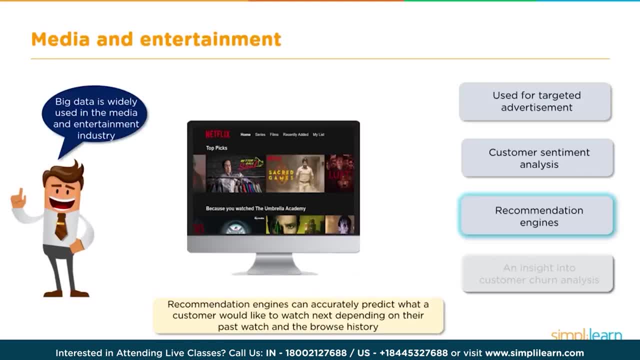 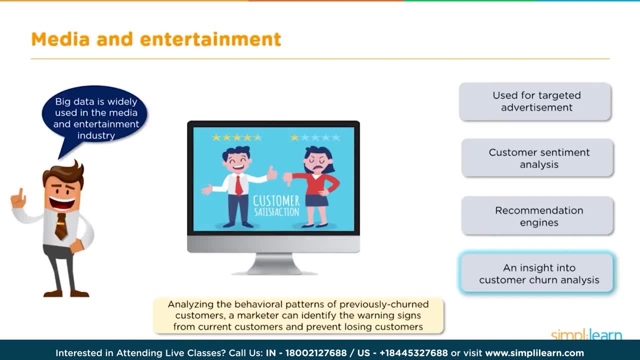 retain and engage its customer for a longer time. Next is customer churn analysis. In simple words, customer churn happens when a customer stops their subscription with a service. Predicting and preventing this is of paramount importance to any organization By analyzing the behavioral patterns of previously. 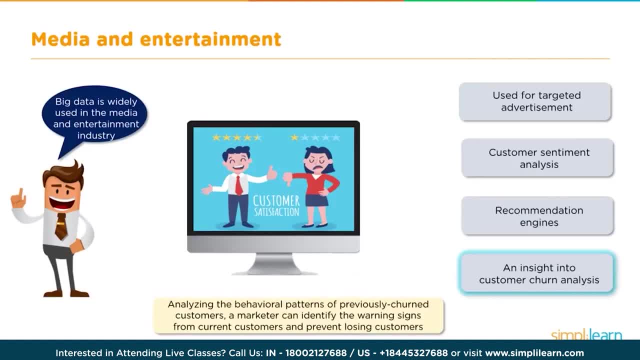 churned customers. an organization can identify which of their current customers are likely to be churned By analyzing the behavioral patterns of previously churned customers. an organization can identify which of their customers are likely to be churned By analyzing all of this data, the 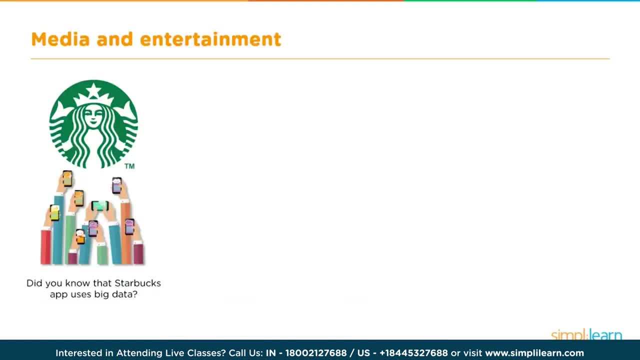 organization can then implement effective programs for customer retention. Let us now look into an use case of Starbucks. Big data is effectively used by the Starbucks app. 17 million users use this app and you can imagine how much data they generate- Data in the form of their 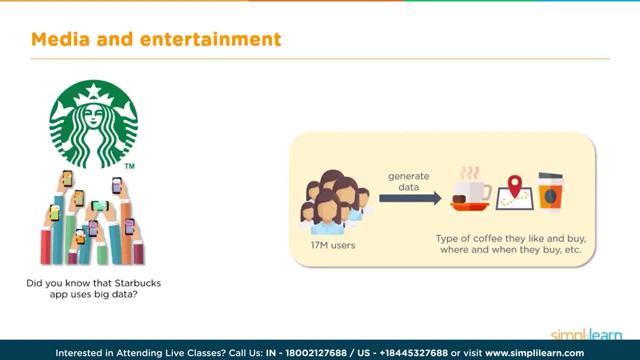 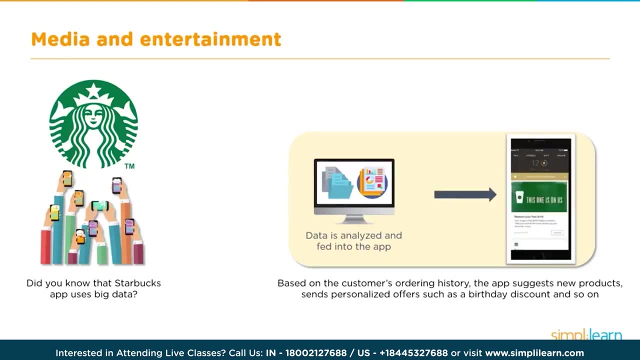 coffee buying habits, the store they visit and to the time they purchase. All of this data is fed into the app. So when a customer buys a coffee, the customer enters a new Starbucks location, the system analyzes all their data and they are provided with their 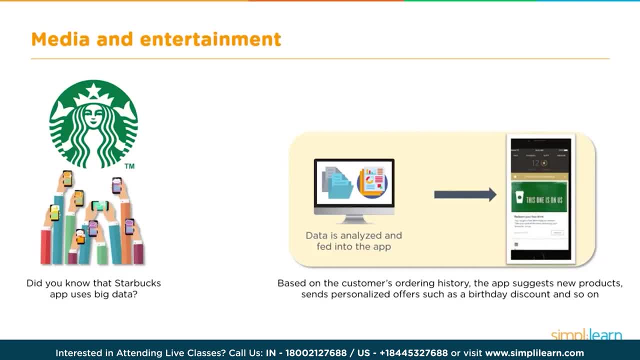 preferred order. This app also suggests new products to the customer. In addition to this, they also provide personalized offer and discounts on special occasions. Moving on to our next sector, which is health care, It is one of the most important sectors. Big data is widely used here to save. 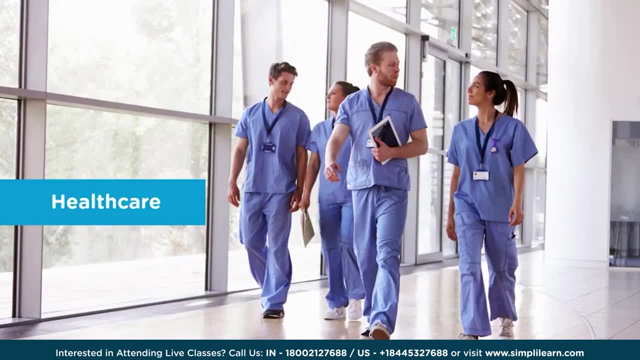 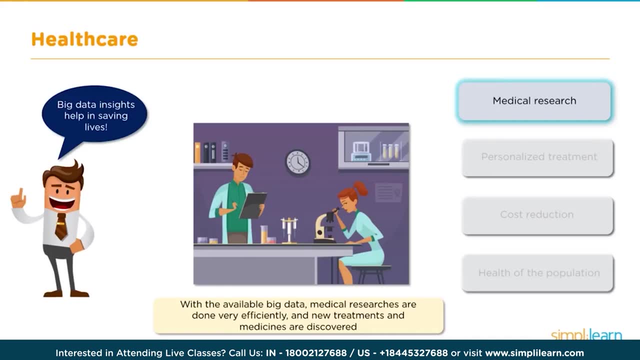 lives, With all the available big data. medical care is one of the most important sectors With all the available big data. medical researches are done very effectively. They are performed accurately by analyzing all the previous medical histories, and new treatments and medicines are. 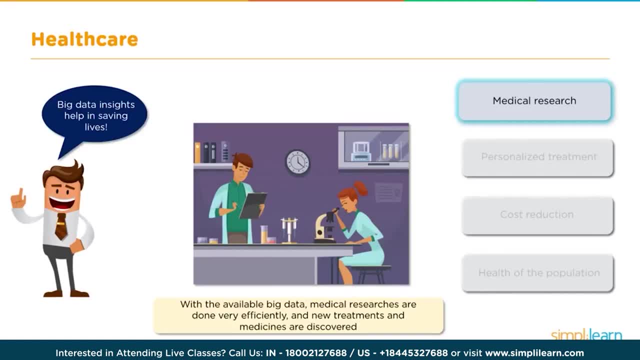 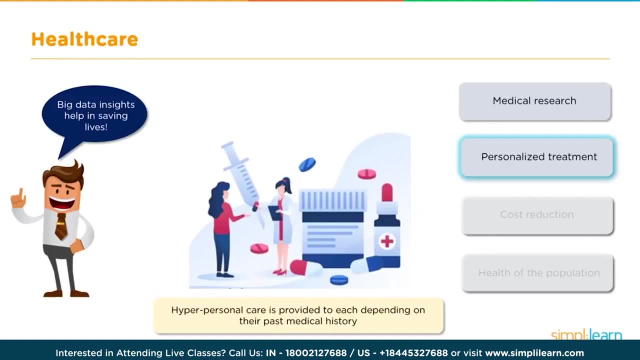 discovered, Cure can be found out even for few of the incurable diseases. There are cases when one medication need not be effective for every patient. Hence personal care is very important. Personal care is provided to each patient depending on their past medical history. 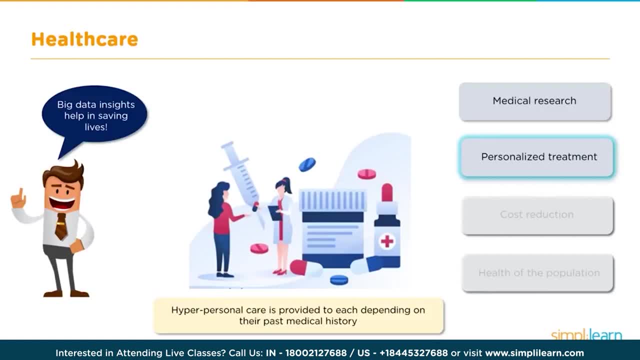 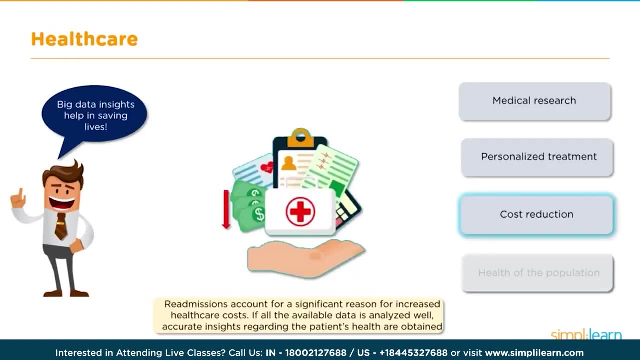 An individual's medical history, along with their body parameters, are analyzed and personal attention is given to each of them. As we all know, medical treatments are not very pocket friendly. Every time a medical treatment is taken, the amount increases. This can be reduced if 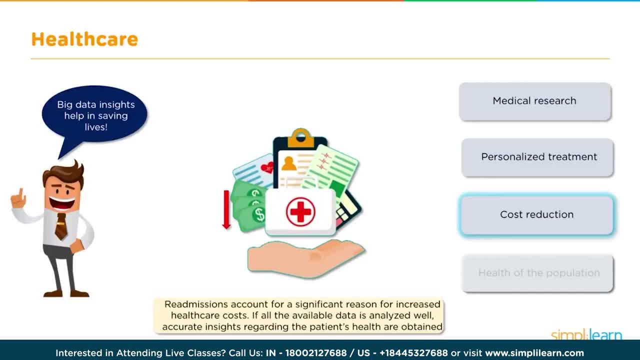 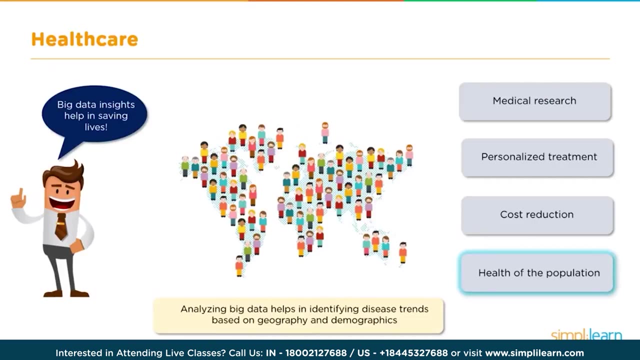 readmissions are brought down. Analyzing all the data precisely will deliver a long term efficient result, which will in turn prevent a patient's readmission. frequently, With globalization came an ease in the ease for infectious diseases to spread widely, Based on geography and demographics. 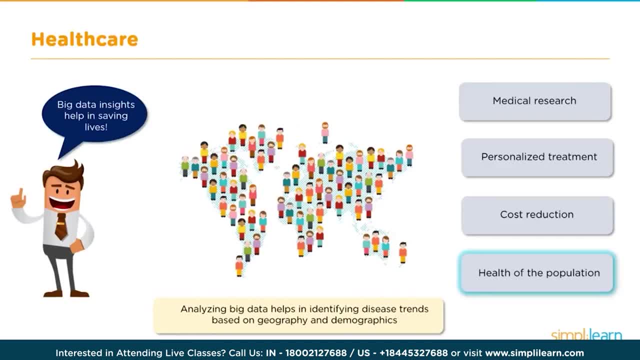 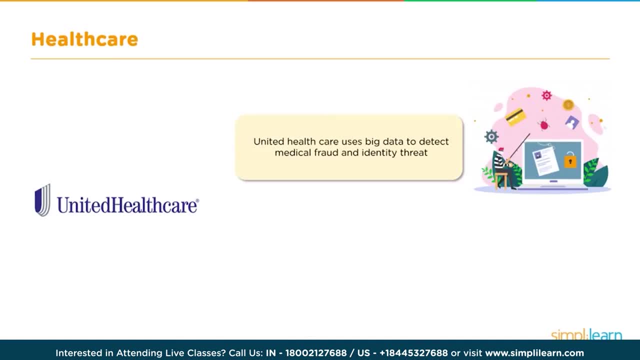 big data helps in predicting where an outbreak of epidemic viruses are most likely to occur. An American healthcare company, United Healthcare, uses big data to detect any online medical fraud activities, such as payment of unauthorized benefits, intentional misrepresentation of data and so on. The healthcare company runs. 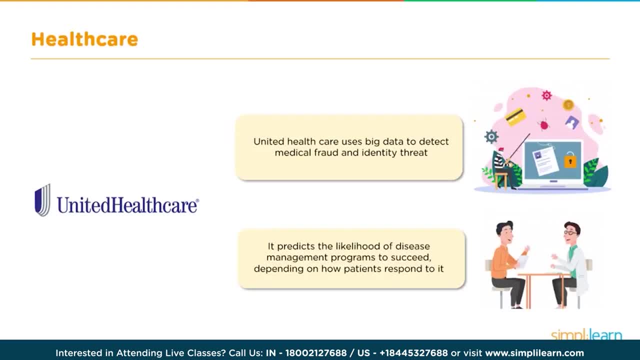 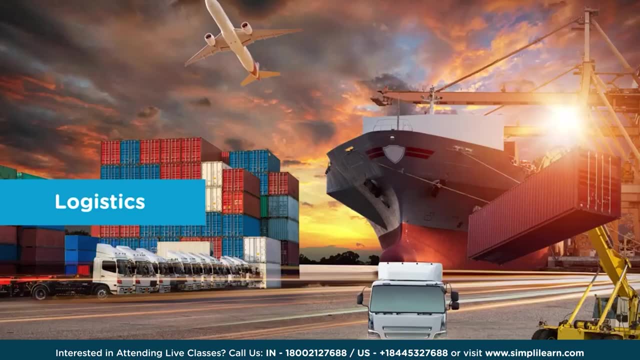 disease management program. The success rates of these programs are predicted using big data, depending on how patients respond to it. The next sector we will look into is logistics. Logistics looks into the process of transportation and storage of goods, The movement of a product from its supplier to a consumer. 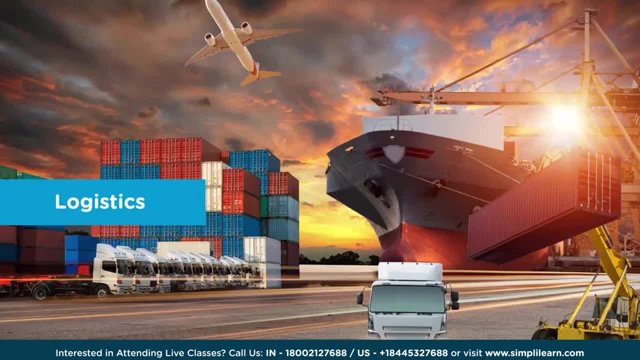 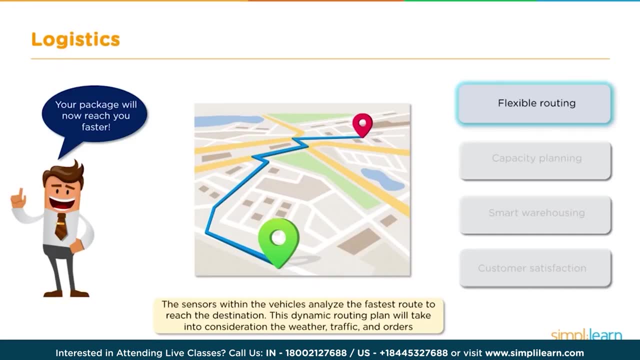 is very important. Big data is used to make this process faster and efficient. The most important factor in logistics is the time taken for the products to reach their destination. To achieve minimum time, sensors within the vehicle analyze the fastest route. This analysis is based 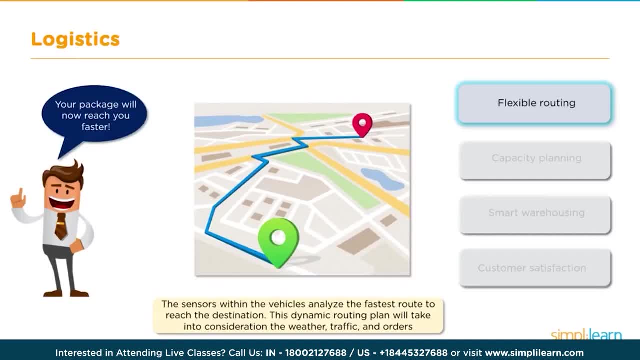 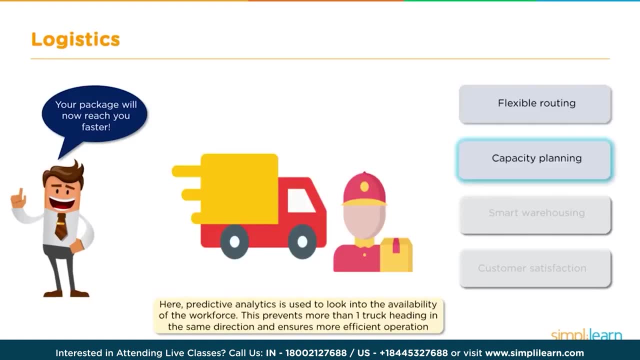 on various data, such as the weather, traffic, the list of orders and so on. By doing so, the fastest route is obtained and the delivery time is reduced. Capacity planning is another factor which needs to be taken into consideration. Details regarding the workforce and the 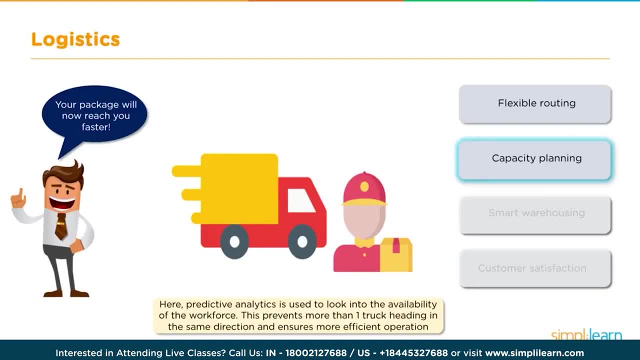 number of vehicles are analyzed regularly and each vehicle is allocated a different route. This is done as there is no need for many trucks to travel in the same direction, which will be pointless. Depending on the analysis of the available workforce and resources, this decision is taken. Big data analytics. 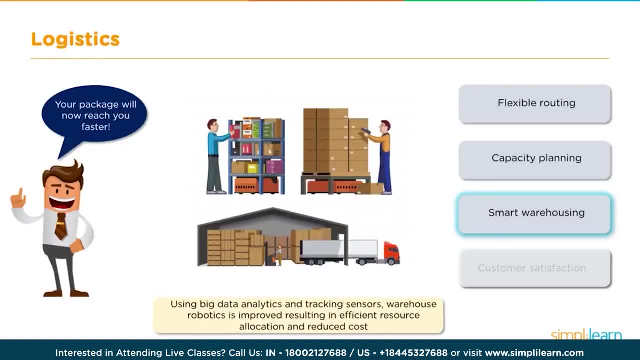 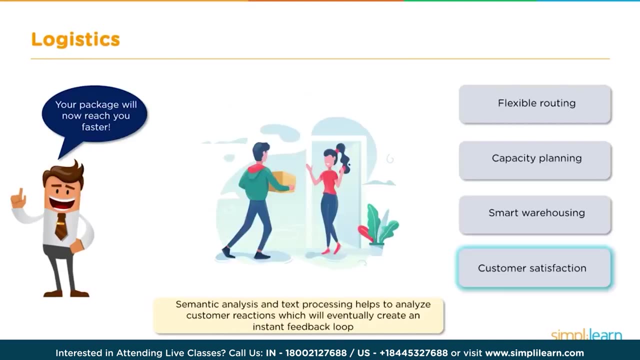 also finds its use in managing warehouses efficiently. This analysis, along with tracking sensors, provide information regarding the under utilized space, which results in efficient resource allocation and eventually reduces the cost. Customer satisfaction is important in logistics, just like it is in any other sector. Customer reactions are 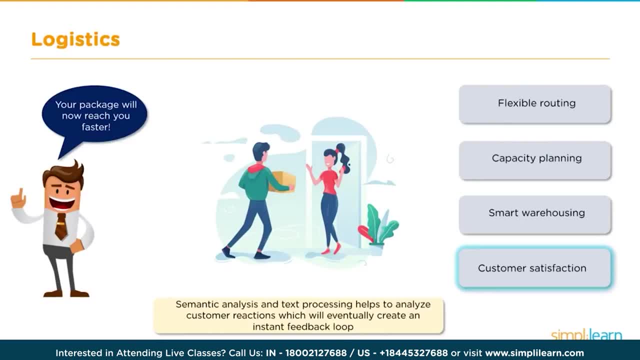 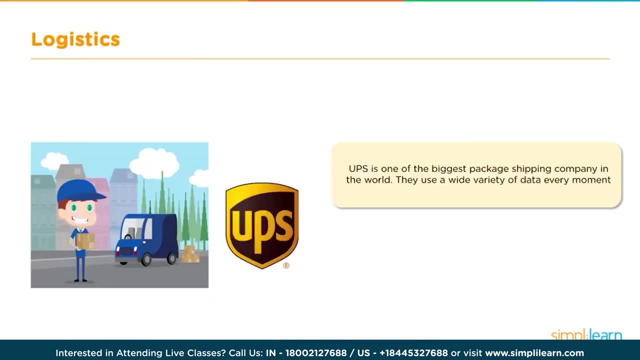 analyzed from the available data, which will eventually create an instant feedback loop. A happy customer will always help the company gain more customers. Let us now look into a use case of UPS. As you know, UPS is one of the biggest shipping company in the world. They have a 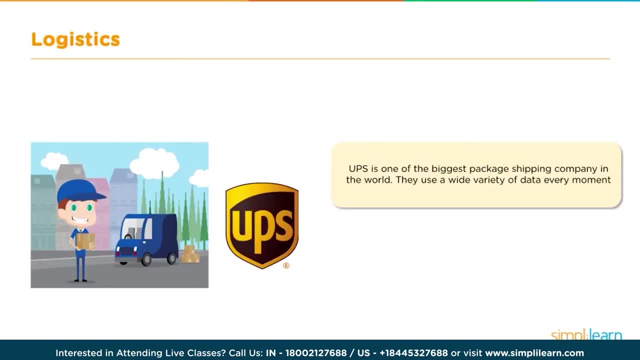 huge customer database and they work on data every minute. UPS uses big data to gather different kinds of data regarding the weather, the traffic jams, the geography, the locations and so on. After collecting all this data, they analyze it to discover the best and 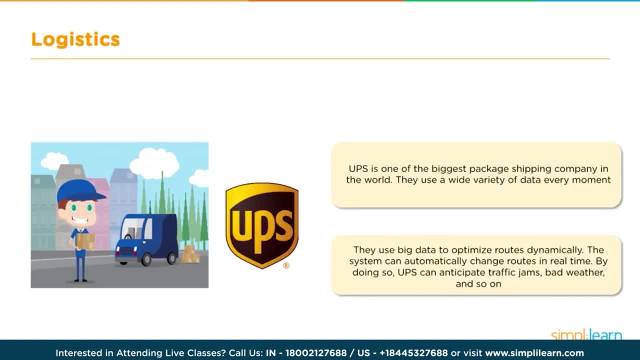 the fastest route to the destination. In addition to this, they also use big data to change the routes in real time. This is how efficiently UPS leverages big data. Next up, we have a very interesting sector. that is, the travel and tourism sector. 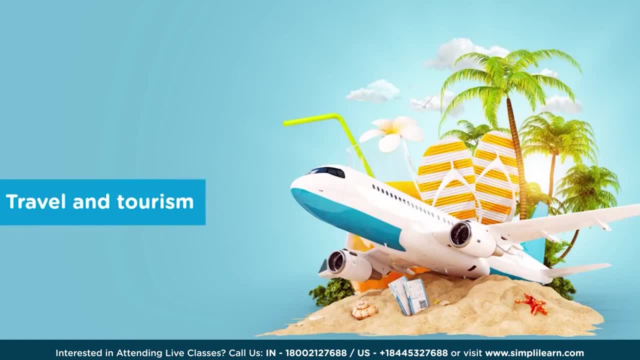 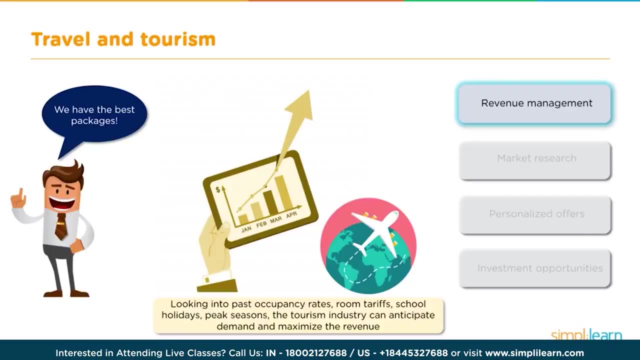 The global tourism market is expected to grow in the near future. Big data is used in various ways in this sector. Let us look into a few of them. Hotels can increase their revenue by adjusting the room tariffs depending on the peak seasons, such as holiday. 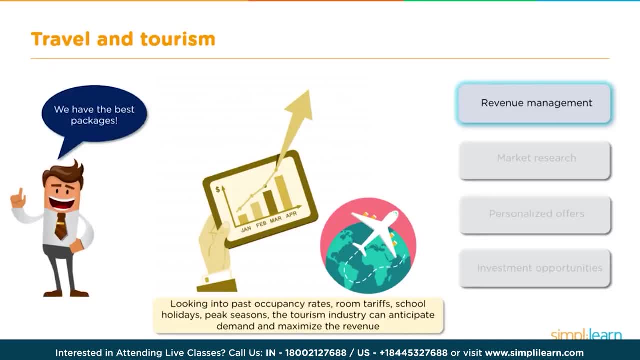 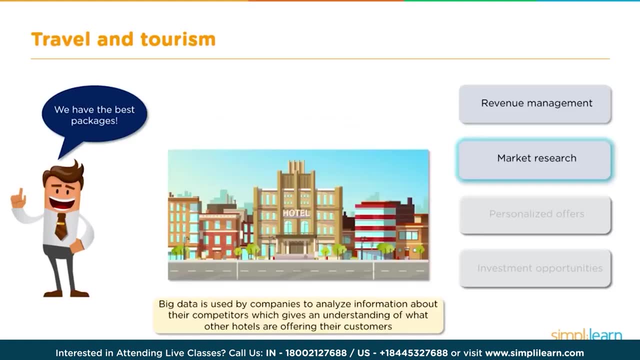 seasons, festive seasons and so on. The tourism industry uses all of this data to anticipate the demand and maximize their revenue. Big data is also used by resorts and hotels to analyze various details regarding their competitors. This analysis result helps them to incorporate all the good. 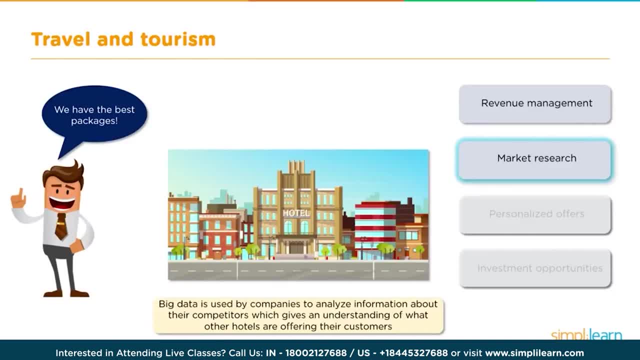 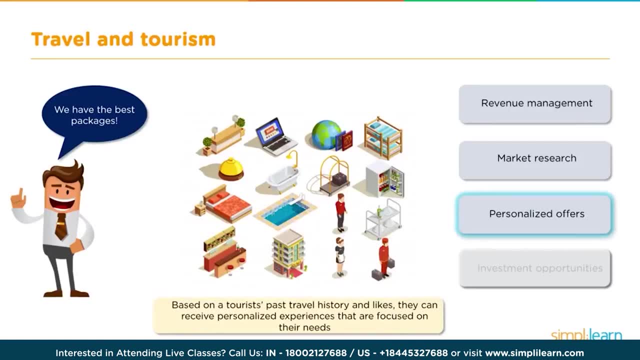 facilities their competitors are providing, And by doing so the hotel is able to flourish further. A customer always comes back if they are offered good packages which are more than just the basic ones. Looking into a customer's past travel history, likes and preferences- hotels. 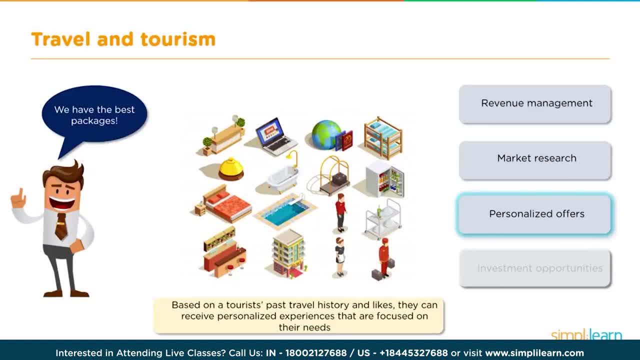 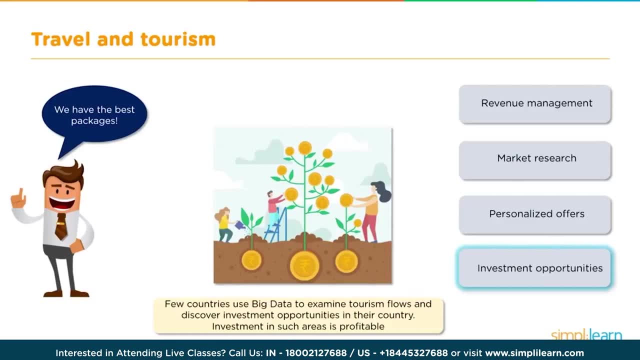 can provide its customers with personal ized experiences which will interest them highly. Investing in an area which could be the hub of tourism is very wise. Few countries use big data to examine the tourism activities in their country, and this, in turn, helps them discover new and 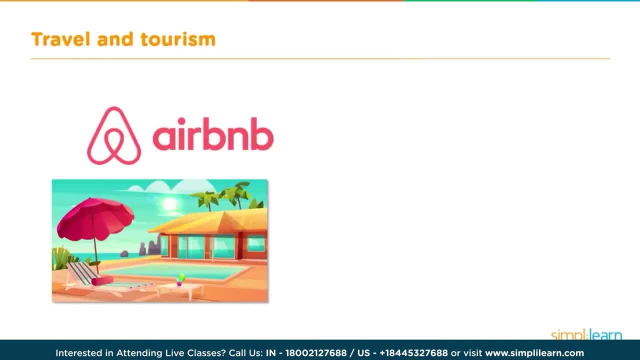 fruitful investment opportunities. Let us look into one of the best online homestay networks- Airbnb- and see how big data is used by them. Airbnb undoubtedly provides its customers with the best accommodation across the world. Big data is used by it to analyze the different kinds of available. 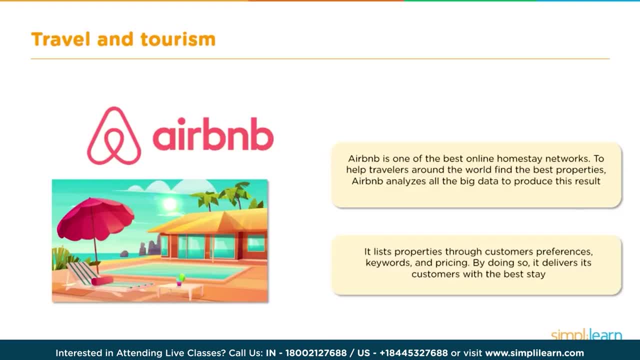 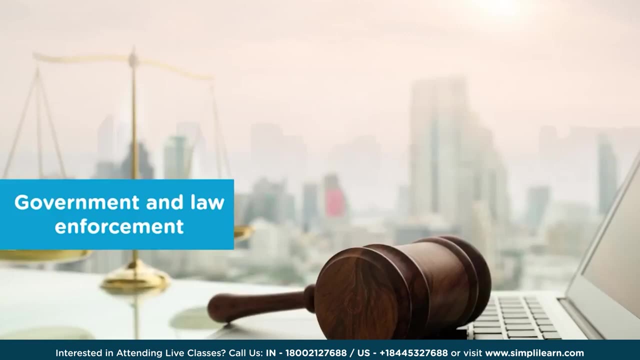 properties Depending on the customer's preferences, the pricing, the keywords, previous customers ratings and experiences. Airbnb filters out the best result. Big data works its magic yet again. Now we will move on to our final sector, which is the government and law. 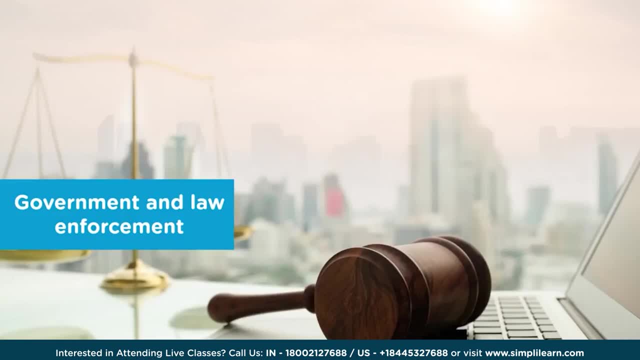 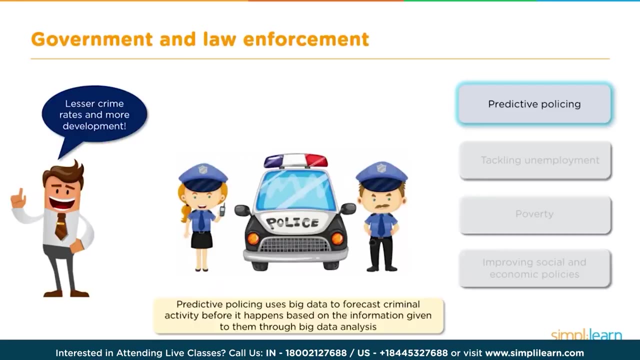 enforcement sector. Maintaining law and order is of utmost importance to any government. It is a huge task by itself. Big data plays an active role here, and in addition to this, it also helps governments bring in new policies and schemes for the welfare of its citizens. The police- 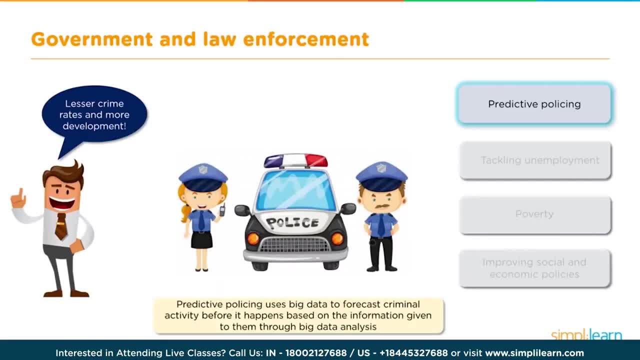 department is able to predict criminal activities way before it happens by analyzing big data information such as the previous crime records in a particular region, the safety aspect in that region, and so on. By analyzing these factors, they are able to predict any activity which breaks the law and 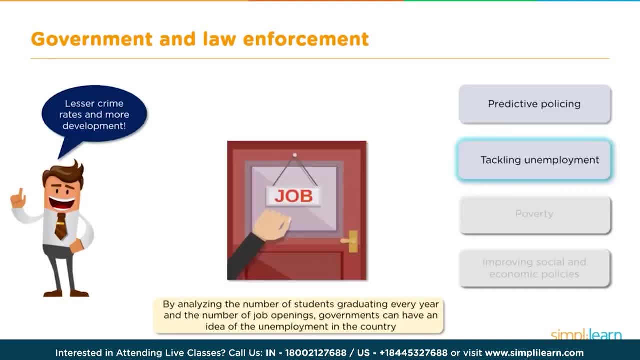 order of the region. Governments are able to tackle unemployment to a great extent by using big data. By analyzing the number of students graduating every year to the number of relevant job openings, the government can have an idea of the unemployment rate in the country and then take 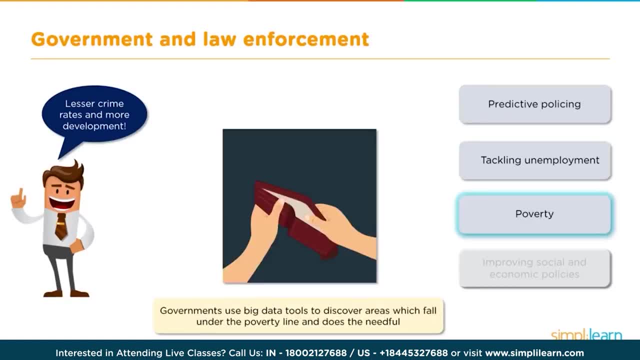 necessary measures to tackle it. Our next factor is poverty. In large countries it is difficult to analyze which area requires attention and development. Big data analytics makes it easier for governments to discover such areas. Poverty gradually decreases once these areas begin to develop. Governments have to always 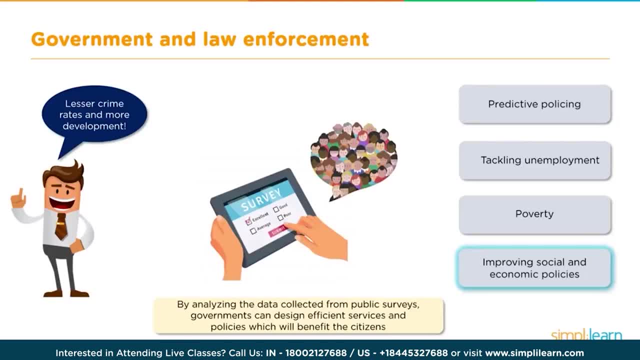 be on the lookout for better development. A public survey voices the opinion of a country's citizens. Analyzing all the data collected from such surveys can help governments build better policies and services, which will benefit its citizens. Let us now move on to our next topic. 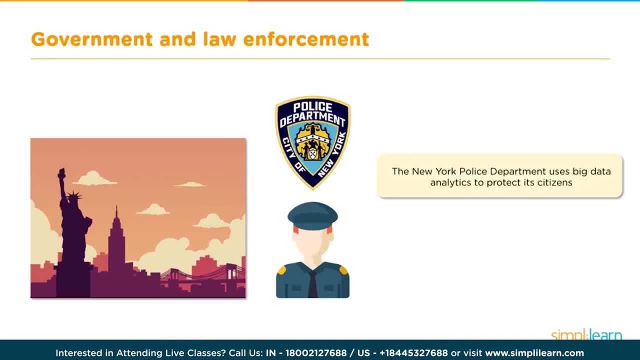 Did you know that the New York Police Department uses big data analytics to protect its citizens? The department prevents and identifies crimes by analyzing a huge amount of data, which includes fingerprints, certain emails and records from previous police investigations, and so on. After analyzing all of this data, 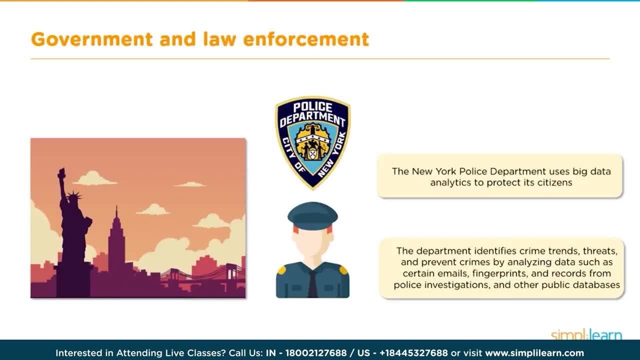 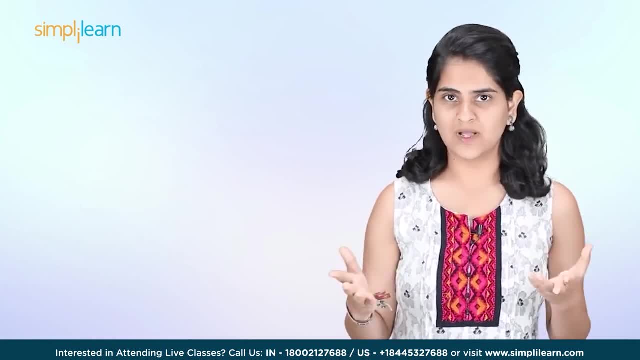 meaningful insights are drawn from it which will help the police in taking the required preventive measures against crimes. Thank you, Shruti. Let us now have a look at the next data processing framework, Spark. We have our instructor, Ajay, who will take us. 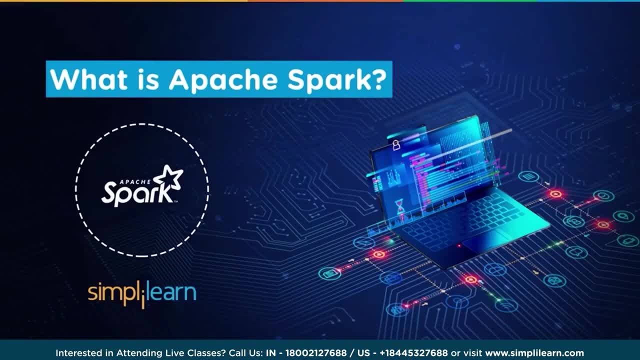 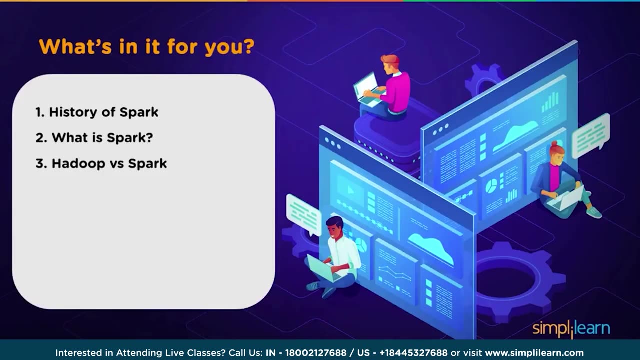 through Apache Spark its installation. Welcome to this tutorial on Apache Spark, one of the most in-demand technologies and processing frameworks in the big data world, And here we will learn on Apache Spark. history of Spark. what is Spark? Hadoop- which? 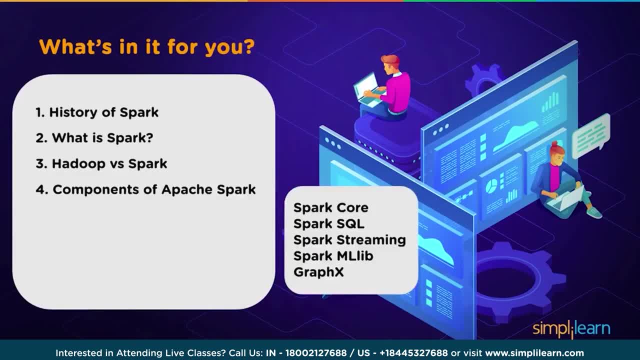 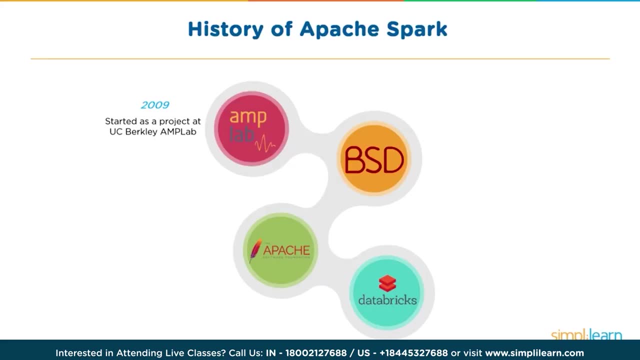 is a framework. again, Wes Spark components of Apache, Spark, that is, Spark Core, Spark, SQL, Spark Streaming, Spark MLlib and Graphics. Then we will learn on Spark architecture, applications of Spark Spark use cases. So let's begin with understanding. 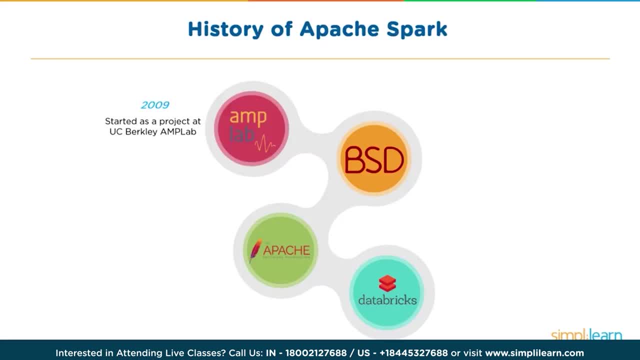 about history of Apache Spark. It all started in 2009 as a project at UC Berkeley AMP Labs by Matej Zahiria. In 2010, it was open sourced under a BSD license. In 2013, Spark became an Apache top level project and 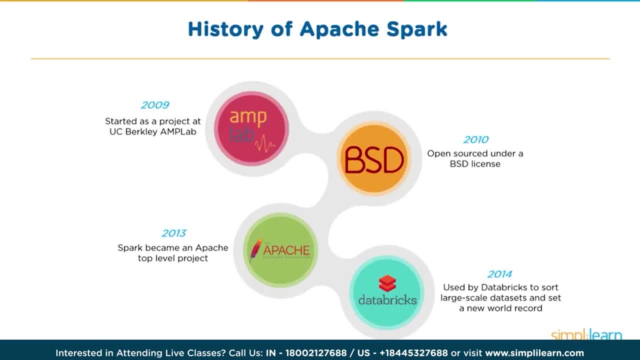 in 2014, used by Databricks to sort large scale data sets, and it set a new world record. So that's how Apache Spark started, and today it is one of the most in-demand processing framework- or I would say in-memory computing framework- which is used across the 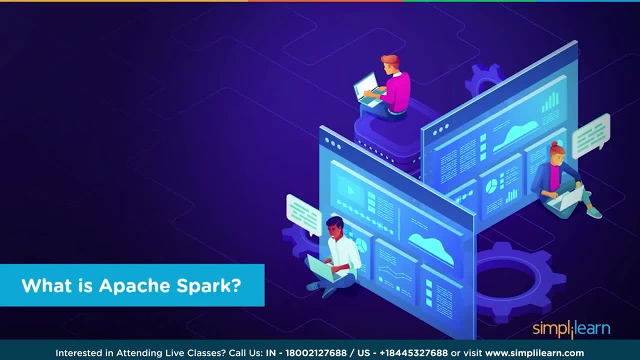 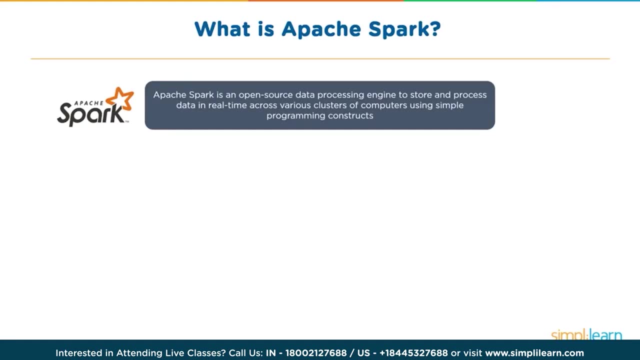 big data industry. So what is Apache Spark? Let's learn about this. Apache Spark is a open source in-memory computing framework, or you could say data processing engine, which is used to process data in batch and also in real time across various cluster computers, and it has 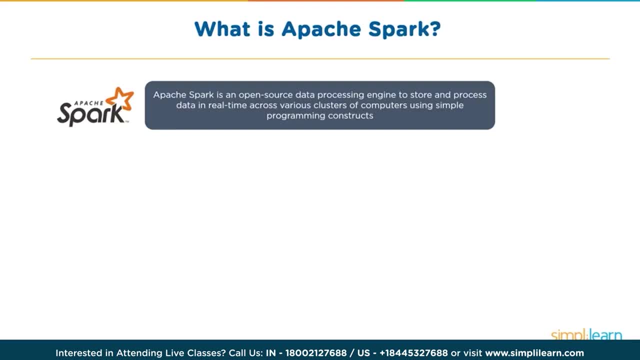 a very simple programming language behind the scenes, that is Scala which is used, although if users would want to work on Spark, they can work with Python, they can work with Scala, they can work with Java and so on- Even R, for that matter. So 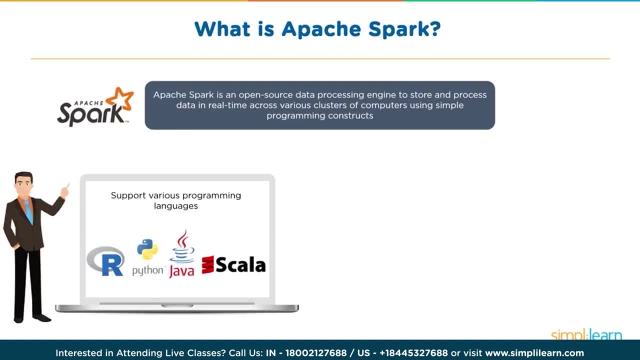 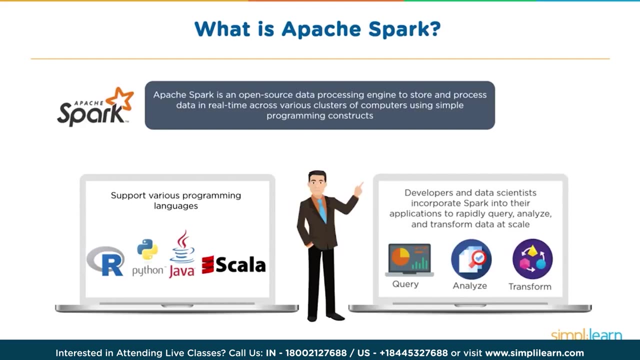 it supports all these programming languages and that's one of the reasons that it is called Polyglot, wherein you have good set of libraries and support from all the programming languages, and developers and data scientists incorporate Spark into their applications or build Spark based applications to process, analyze, 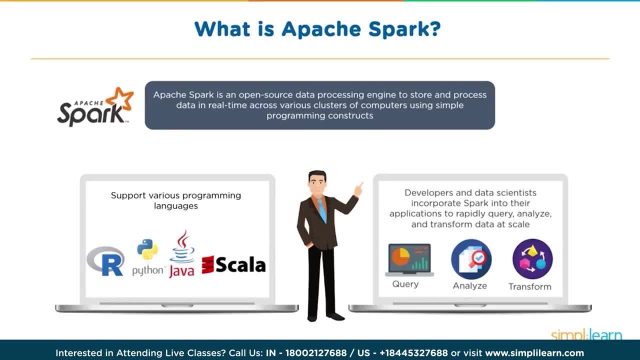 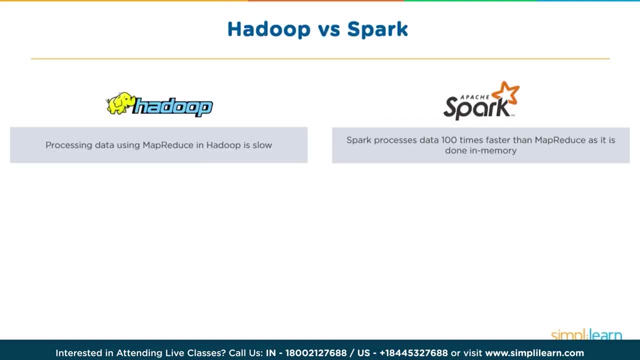 query and transform data at a very large scale. So these are key features of Apache Spark. Now, if you compare Hadoop West Spark, we know that Hadoop is a framework and it basically has MapReduce, which comes with Hadoop, for processing data. However, processing 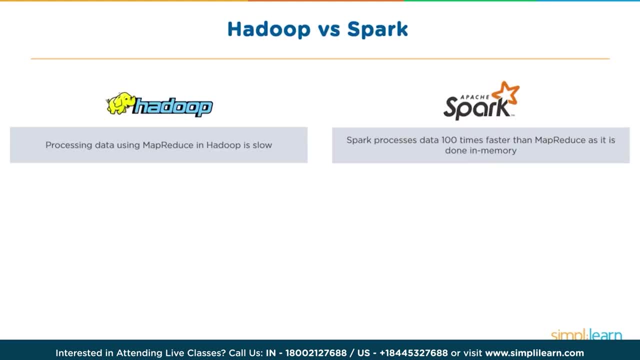 data using MapReduce in Hadoop is quite slow because it is a batch oriented operation and it is time consuming. If you talk about Spark, Spark can process the same data 100 times faster than MapReduce, as it is a in-memory computing framework. Well, 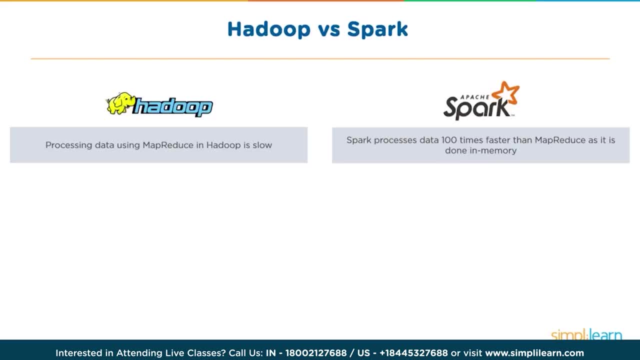 there can always be conflicting ideas, saying: what if my Spark application is not really efficiently coded and my MapReduce application has been very efficiently coded? Well then it's a different case. However, normally, if you talk about code which is efficiently written for MapReduce or for Spark based, 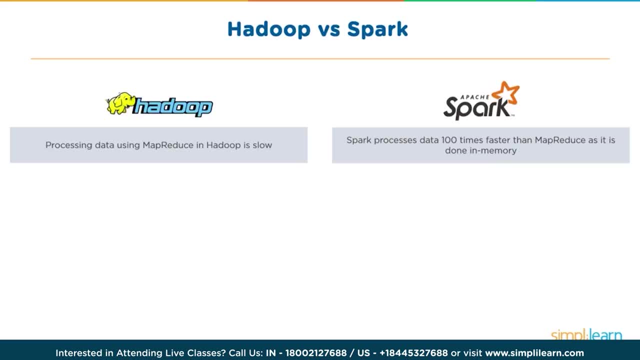 processing. Spark will win the battle by doing almost 100 times faster than MapReduce. So, as I mentioned, Hadoop performs batch processing and that is one of the paradigms of MapReduce programming model, which involves mapping and reducing, and that's quite rigid, So it performs. 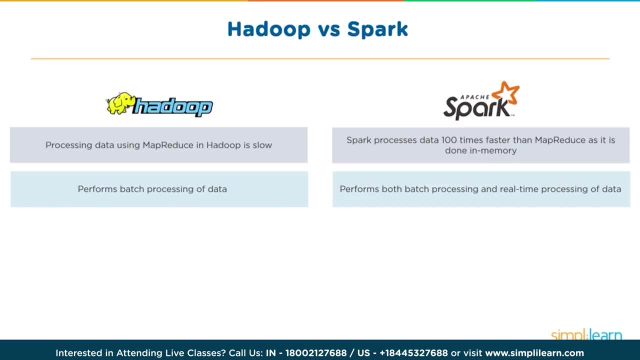 batch processing, the intermittent data is written to SDFS and written read back from SDFS, and that makes Hadoop's MapReduce processing slower. In case of Spark, it can perform both batch and real time processing. However, lot of use cases are based on 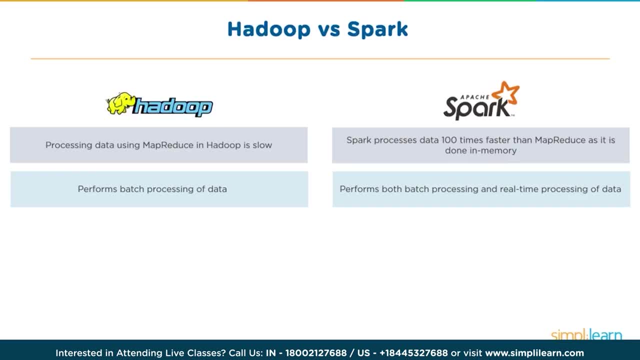 real time processing. Take an example of Macy's, take an example of retail giant such as Walmart, and there are many use cases who would prefer to do real time processing or I would say, near real time processing. So when we say real time or near real, 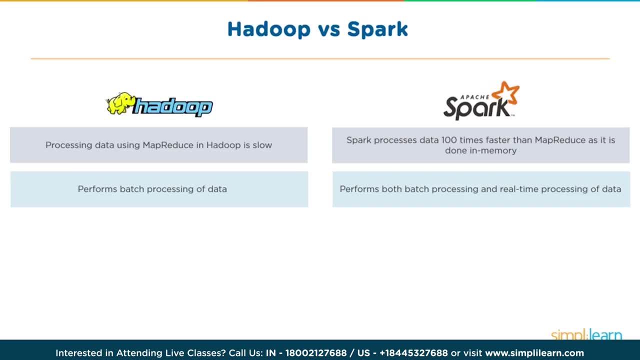 time it is about processing the data as it comes in, or you are talking about streaming kind of data. Now Hadoop, or Hadoop's MapReduce, obviously was started to be written in Java. Now you could also write it in Scala or in Python. However, 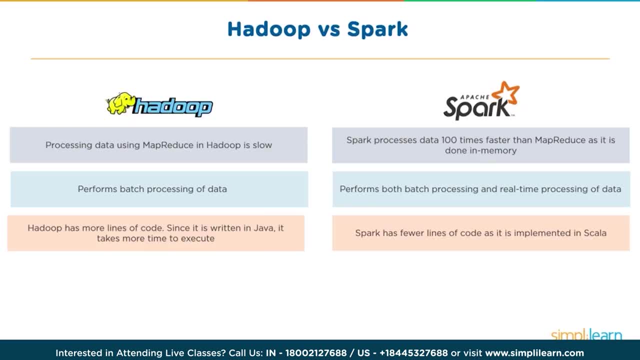 if you talk about MapReduce, it will have more lines of code, since it is written in Java, and it will take more times to execute. You have to manage the dependencies, you have to do the right declarations, you have to create your mapper and reducer. 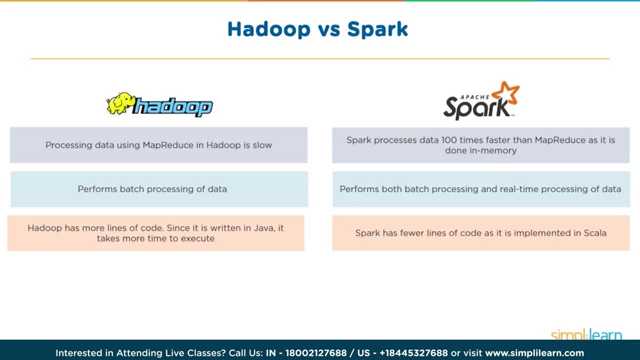 and driver classes. However, if you compare Spark, it has few lines of code, as it is implemented in Scala, and Scala is a statically typed, dynamically inferred language. It's very, very concise and the benefit is it has features from both functional programming and object oriented language. 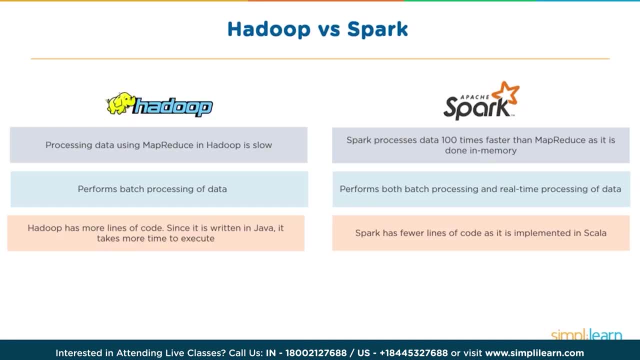 And in case of Scala, whatever code is written, that is converted into byte codes and then it runs in the JVM. Now Hadoop supports Kerberos authentication. There are different kind of authentication mechanisms. Kerberos is one of the well known ones and it can really get difficult to manage. 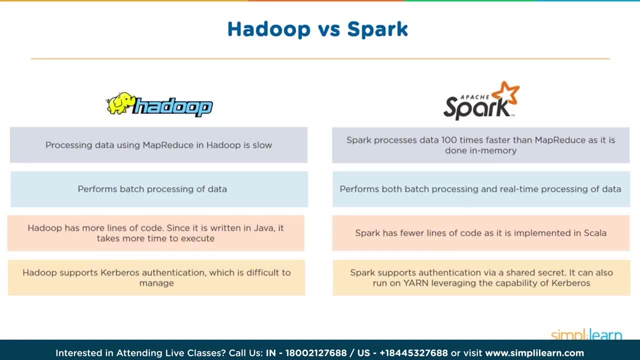 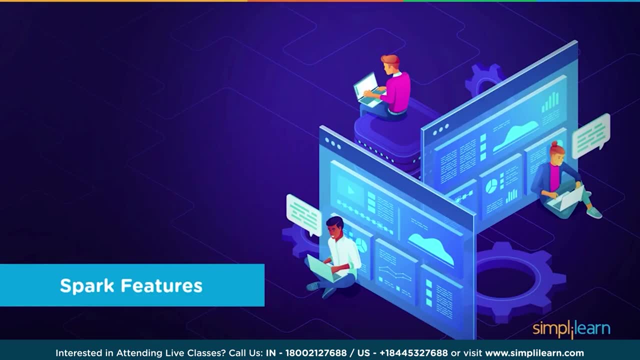 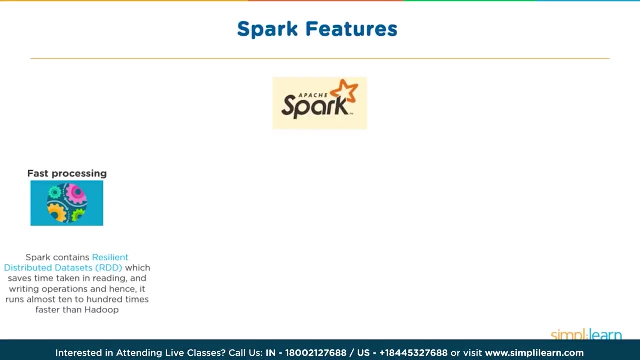 Now Spark supports authentication via a shared secret. It can also run on YARN, leveraging the capability of Kerberos. So what are Spark features which really makes it useful? Spark is a unique or in demand processing framework. When we talk about Spark features, one of the key 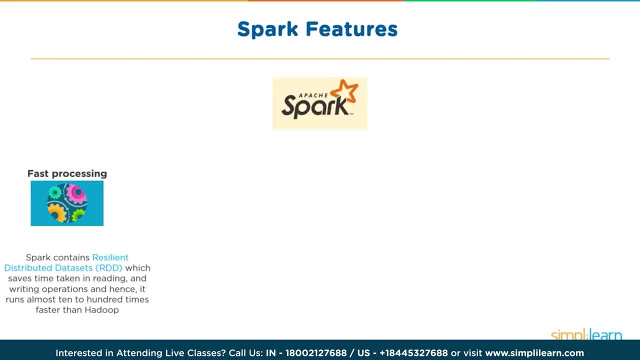 features is fast processing. So Spark contains resilient distributed data sets. So RDDs are the building blocks for Spark And we will learn more about RDDs later. So Spark contains RDDs, which saves huge time taken in reading and writing operations. So it can 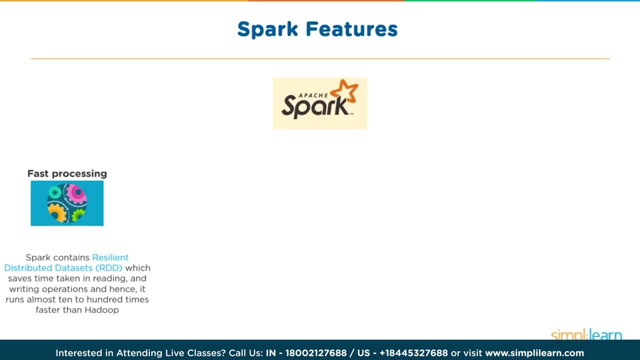 be 100 times, or you can say 10 to 100 times faster than RDDs When we say in memory computing. here I would like to make a note that there is a difference between caching and in memory computing. Think about it: Caching is mainly. 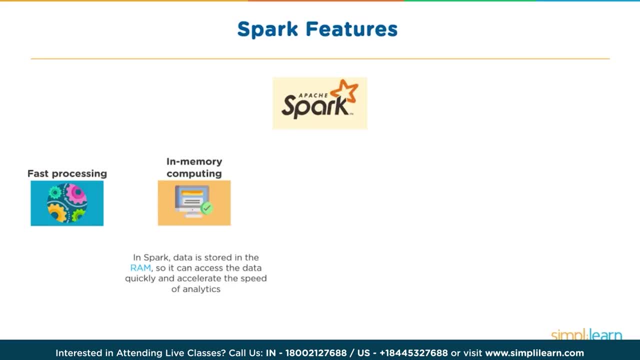 to support read ahead mechanism, where you have your data preloaded so that it can benefit further queries. However, when we say in memory computing, we are talking about lazy valuation. We are talking about data being loaded into memory only and only when a specific kind of action. 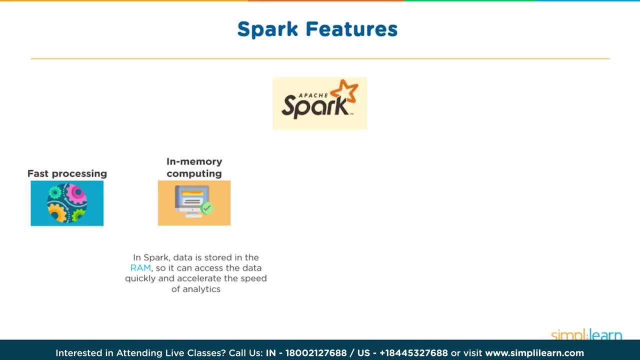 is invoked, So data is stored in RAM. So here we can say: RAM is not only used for processing, but it can also be used for storage, And we can again decide whether we would want that RAM to be used for persistence or just for computing, So it can access. 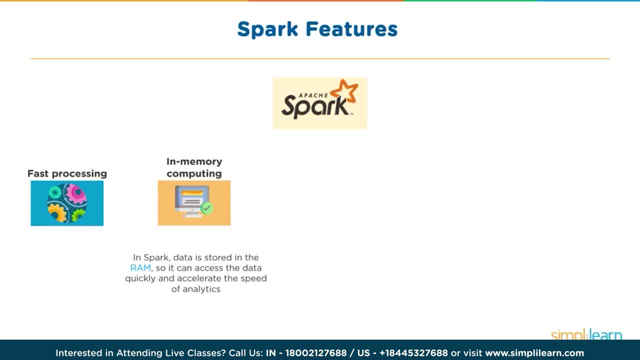 the data quickly and accelerate the speed of analytics. Now, Spark is quite flexible. It supports multiple languages, as I already mentioned, and it allows the developers to write applications in Java, Scala, R or Python. It's quite fault tolerant, So Spark contains these. 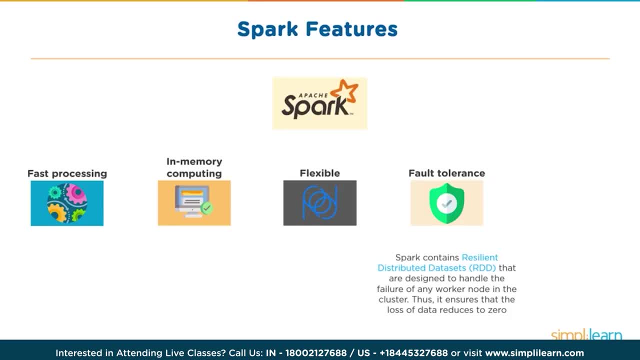 RDDs, or you could say execution logic, or you could say temporary data sets, which initially do not have any data loaded, and the data will be loaded into RDDs only when execution is happening. So these can be fault tolerant, as these RDDs are distributed across. 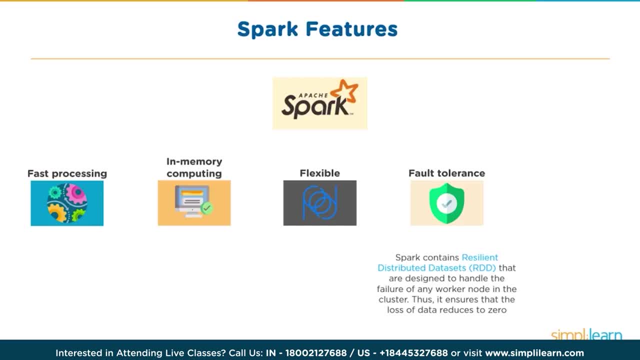 multiple nodes. So failure of one worker node in the cluster will really not affect the RDD because that portion can be recomputed. So it ensures loss of data. It ensures that there is no data loss and it is absolutely fault tolerant. It is for better analytics. so 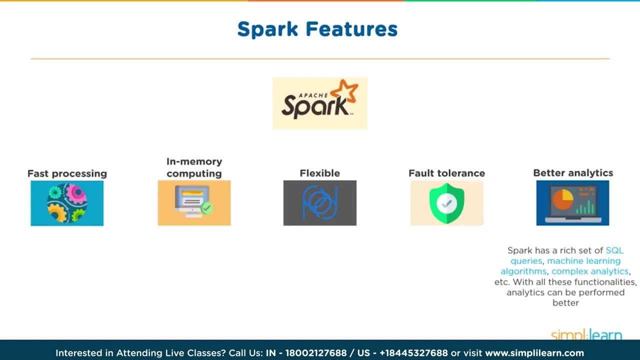 Spark has rich set of SQL queries, machine learning algorithms, complex analytics, all of this supported by various Spark components which we will learn in coming slides. With all these functionalities, analytics can be performed better in terms of Spark. So these are some of the key features of 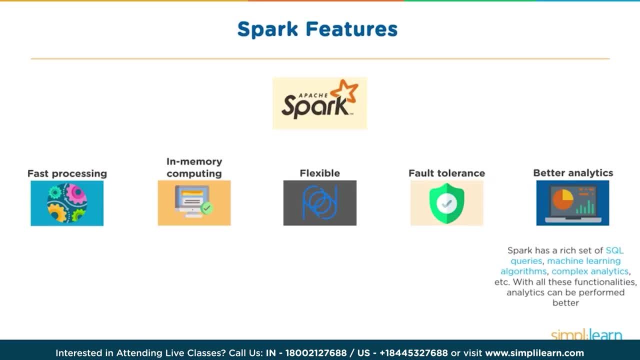 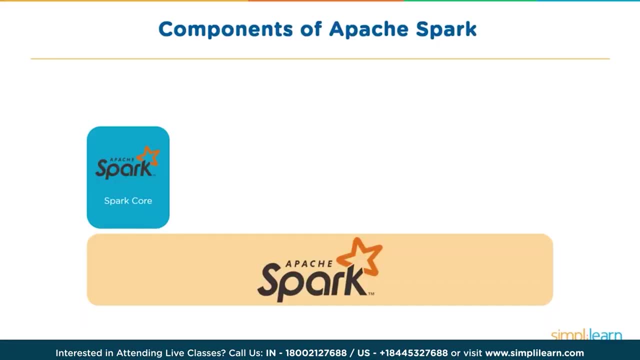 Spark. However, there are many more features which are related to different components of Spark and we will learn about them. So what are these components of Spark which I am talking about? Spark core, So this is the core component which basically has RDDs, which has a core engine. 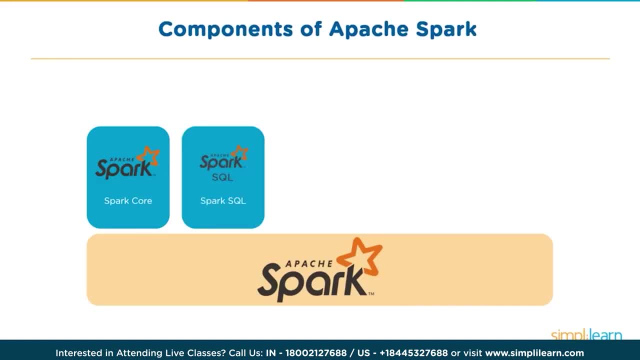 which takes care of your processing. Now you also have Spark SQL, So people who would be interested in working on structured data or data which can be structurized would want to prefer using Spark SQL, and Spark SQL internally has components or features like data frames and data. 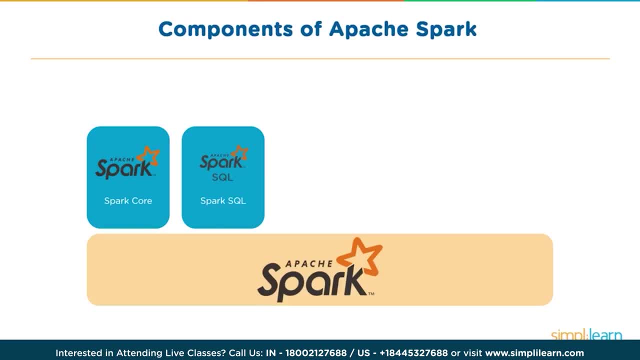 sets which can be used to process your structured data in a much, much faster way. You have Spark streaming. Now that's again an important component of Spark, which allows you to create your Spark streaming applications, which not only works on data which is being streamed in or data which is 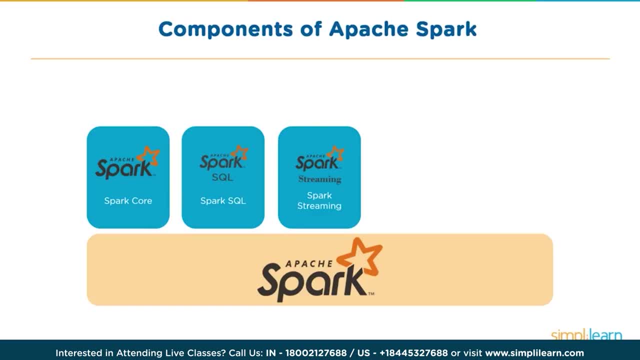 constantly getting generated, but you would also- or you could also- transform the data. You could analyze or process the data as it comes in in smaller chunks. You have Spark's MLlib Now. this is basically a set of libraries which allows developers or data scientists to build their 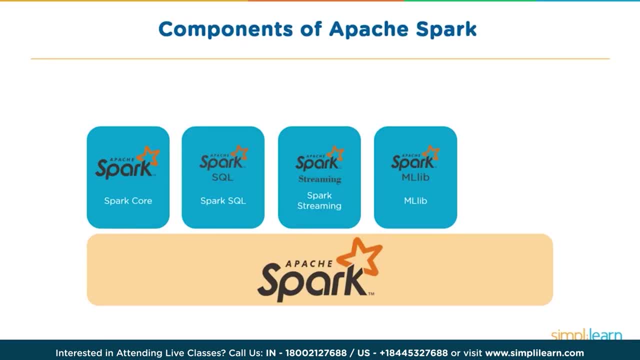 machine learning algorithms so that they can do predictive analytics or prescriptive, descriptive, preemptive analytics, or they could build their recommendation systems or bigger, smarter machine learning algorithms using these libraries, And then you have graphics. So think about organizations like LinkedIn or, say, Twitter, where 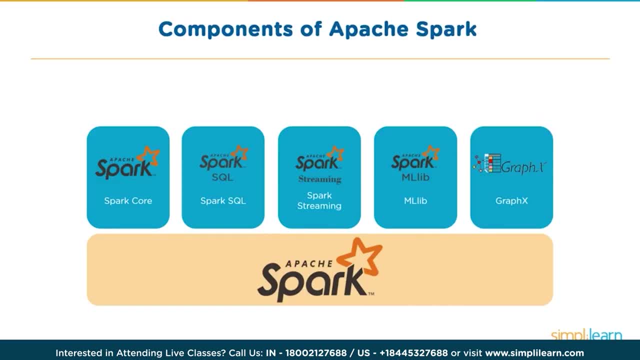 you have data which naturally has a network kind of flow, So data which could be represented in the form of graphs. Now, here, when I talk about graphs, I'm not talking about pie charts or bar charts, but I'm talking about network related data, that is, data which can be networked. 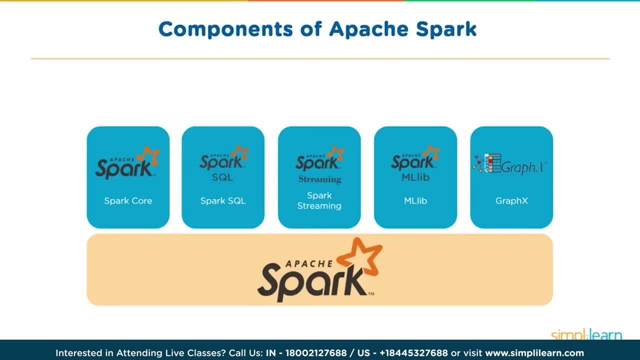 together which can have some kind of relationship. Think about Facebook, think about LinkedIn, where you have one person connected to other person or one company connected to other company. So if we have our data which can be represented in the form of network graphs, then Spark has a component called graphics. 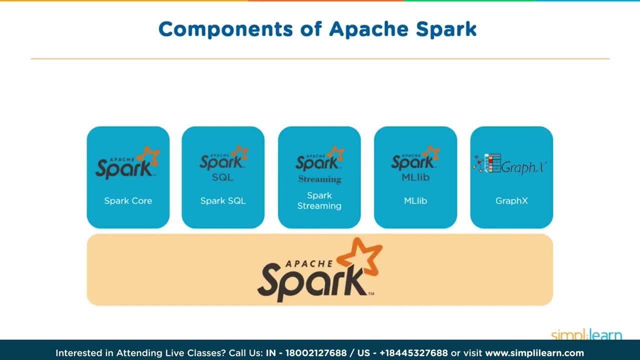 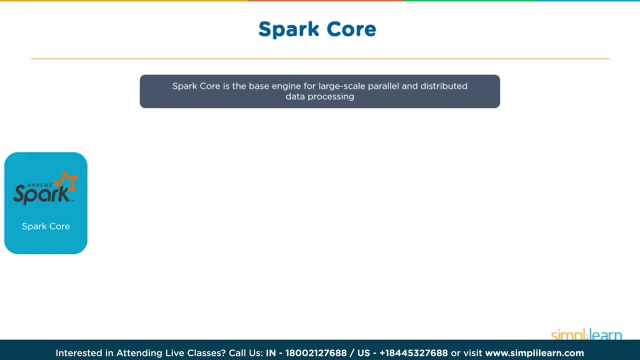 which allows you to do graph based processing. So these are some of the components of Apache: Spark, Spark Core, Spark SQL, Spark Streaming, Spark MLlib and Graphics. So to learn more about components of Spark, let's learn here about Spark Core. Now this is the base. 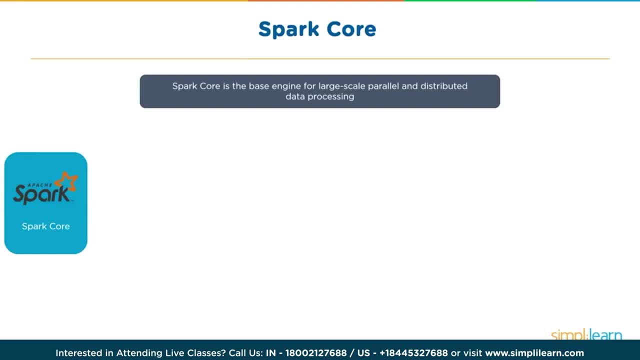 engine, and this is used for large scale parallel and distributed data processing. So when you work with Spark at least- and the minimum you would work with- is Spark Core, which has RDDs as the building blocks of your Spark, So it is responsible for your memory management. your fault. 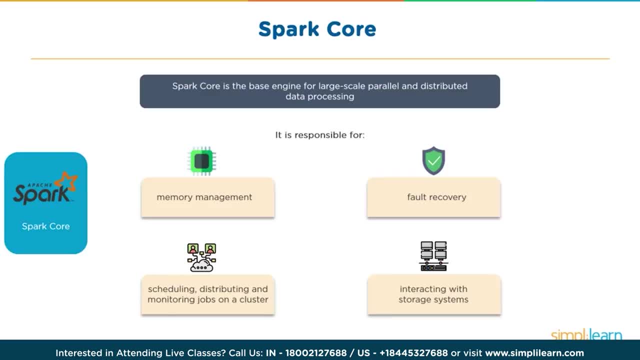 recovery, scheduling, distributing and monitoring jobs on a cluster and interacting with storage systems. So here I would like to make a key point: that Spark by itself does not have its own storage. It relies on storage. Now that storage could be your SDFS, that is, Hadoop's. 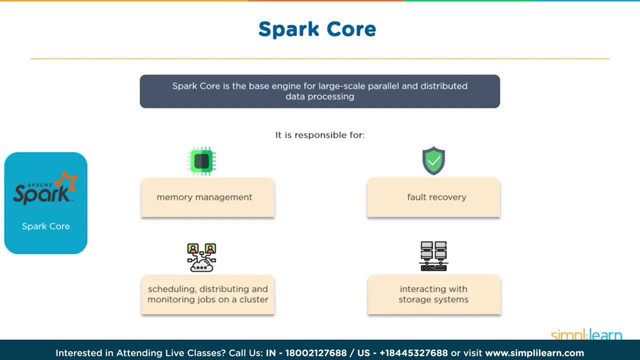 distributed file system. It could be a database like NoSQL database, such as HBase, or it could be any other database, say RDBMS, from where you could connect your Spark and then fetch the data, extract the data, process it, analyze it. 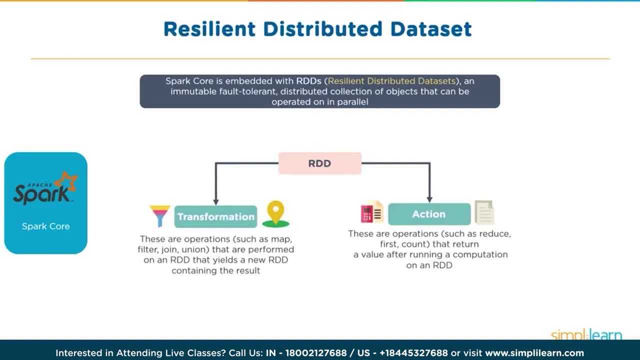 So let's learn a little bit about your RDDs- resilient distributed data sets. Now, Spark Core, which is the base engine, or the core engine, is embedded with the building blocks of Spark, which is nothing but your resilient distributed data set. So, as the name says, it is resilient, so it is. 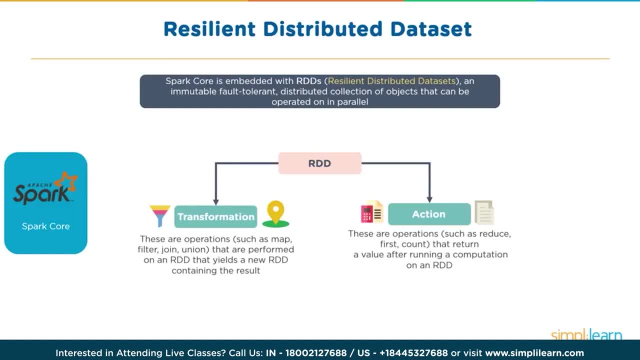 existing for a shorter period of time. distributed, So it is distributed across nodes and it is a data set where the data will be loaded or where the data will be existing for processing. So it is immutable, fault tolerant. distributed collection of objects. So that's what your RDD is. 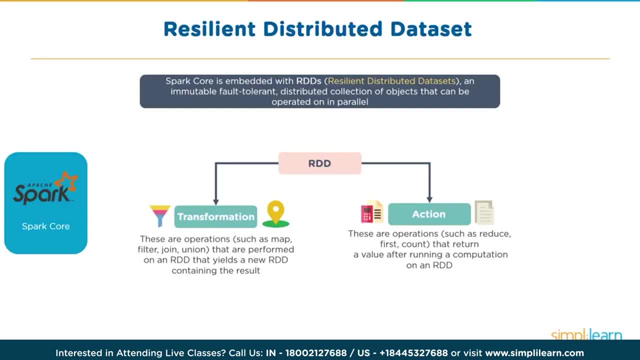 And there are mainly two operations which can be performed on an RDD. Now, to take an example of this, say, I want to process a particular file. Now here I could write a simple code in Scala and that would basically mean something like this: So if I say val, 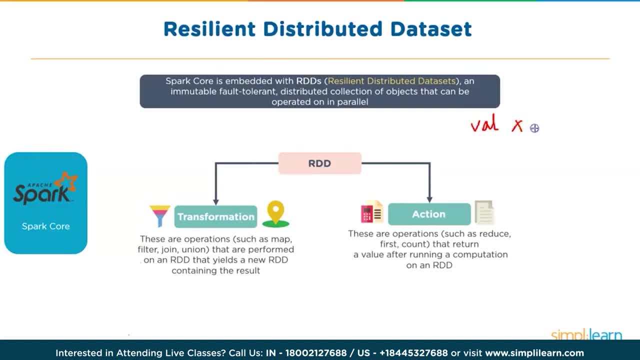 which is to declare a variable. I would say val x, and then I could use what we call a Spark Context, which is basically the most important entry point of your application. So then I could use a method of Spark Context, for example, that is text file, and then I could point it to. 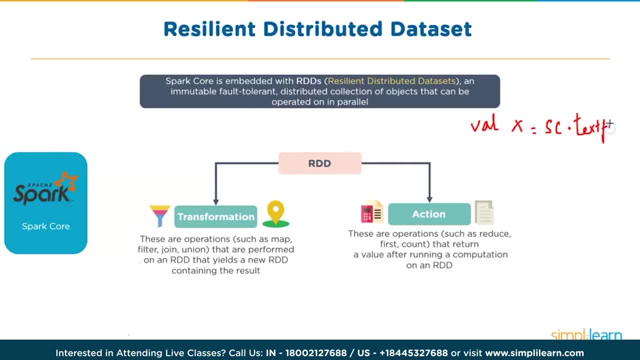 a particular file. So this is just a method of your Spark Context, and Spark Context is the entry point of your application. Now, here I could just give a path in this method. So what does this step do? It does not do any valuation. 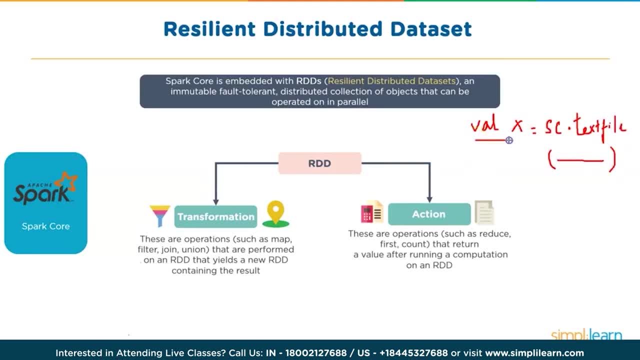 So when I say val x, I am creating an immutable variable and to that variable I am assigning a file. Now what this step does is it actually creates a RDD resilient distributed data set. So we can imagine this as a simple execution logic, a empty data. 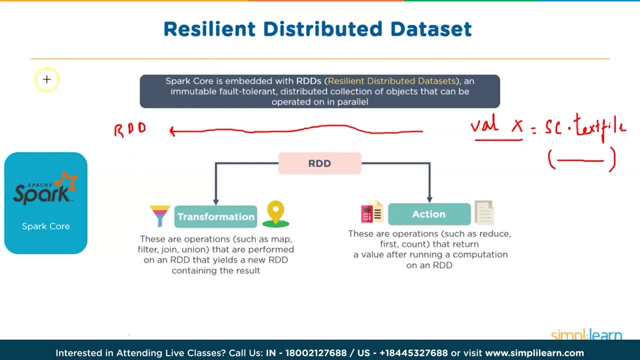 set which is created in memory of your node. So if I would say I have multiple nodes in which my data is split and stored, imagining that your yarn, your Spark is working with Hadoop, So I have Hadoop which is using, say, two nodes. 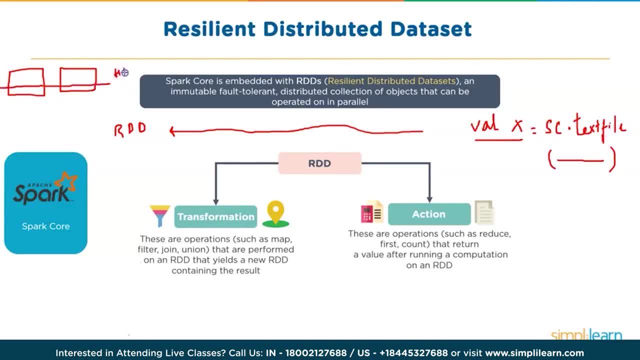 and this is my distributed file system, HDFS, which basically means my file is written to HDFS and it also means that the file related blocks are stored in the underlying disk of these machines. So when I say val x equals sc dot text file, that is using a method. 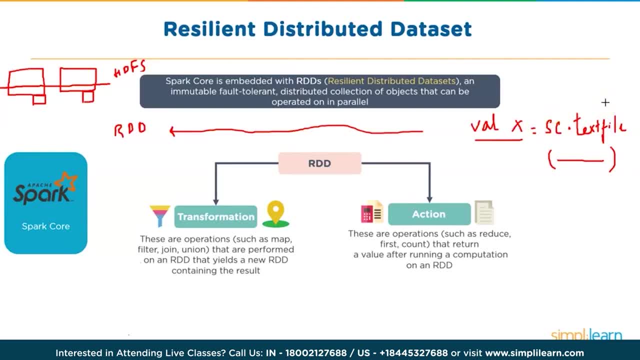 of Spark context. Now there are various other methods, like whole text files, parallelize and so on. This step will create an RDD, So you can imagine this as a logical data set which is created in memory across these nodes, because these nodes have the data. However, 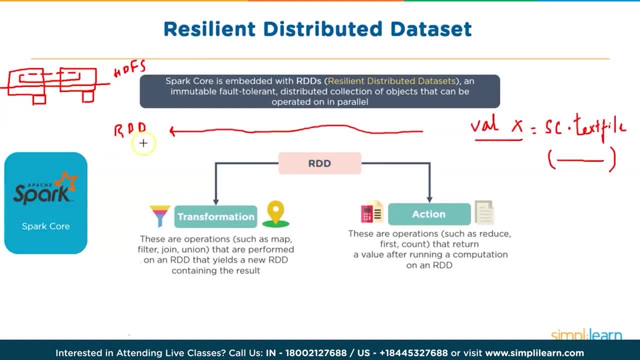 no data is loaded here. So this is the first RDD and, I can say, first step in what we call as a DAG, A DAG which will have series of steps which will get executed at later stage. Now, later I could do further processing on this, I could say val. 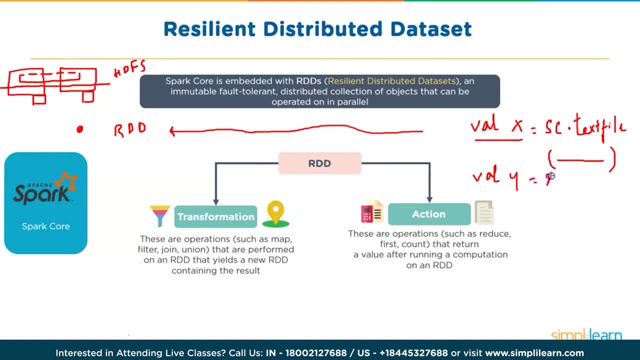 y, and then I could do something on x, so I could say x dot map and I would want to apply a function to every record or every element in this file and I could give a logic here: x dot map. now this second step is again creating an RDD. 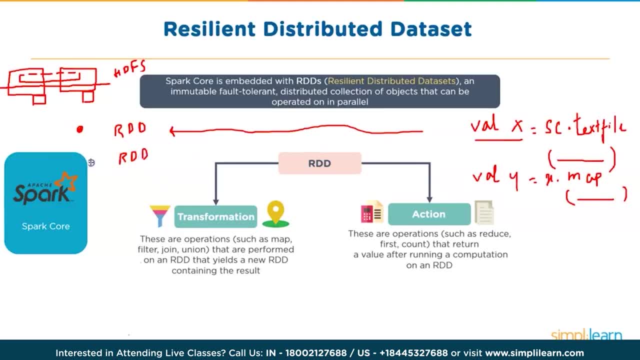 a resilient distributed data set. you can say: second step in my DAG, okay, and here you have a external RDD, one more RDD created which depends on the first RDD. So my first RDD becomes the base RDD or parent RDD, and the resultant RDD becomes the child RDD. Then we can. 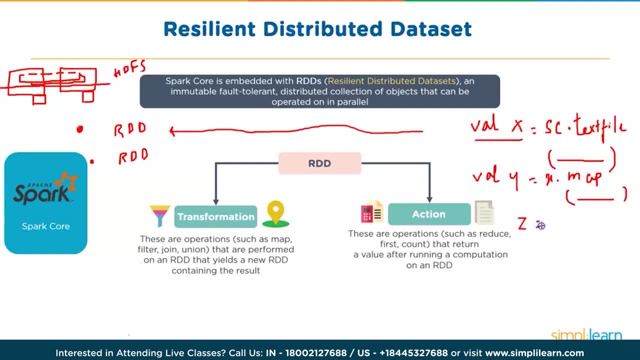 go further and we could say val z and I would say: okay, now I would want to do some filter on y. So this filter, which I am doing here and then I could give a logic, might be. I am searching for a word, I am searching for some pattern. 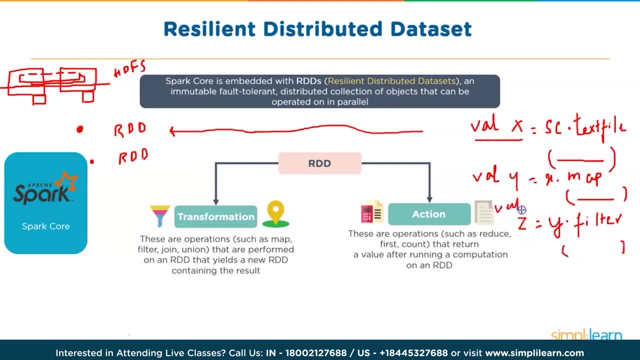 so I could say: val z equals y dot filter, which again creates one more RDD, a resilient distributed data set in memory, and a. you can say: this is nothing but one more step in the DAG. so this is my DAG, which is a series of steps which will be executed. 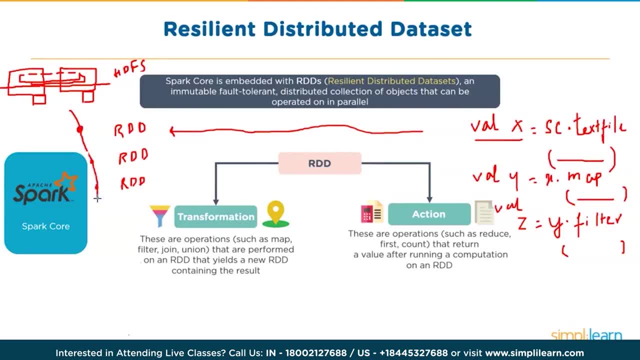 now here. when does the execution happen? when the data get? when will the data get loaded into these RDDs? so all of this, that is, using a method, using a transformation like map, using a transformation like filter or flat map or anything else, these are your transformations. so the 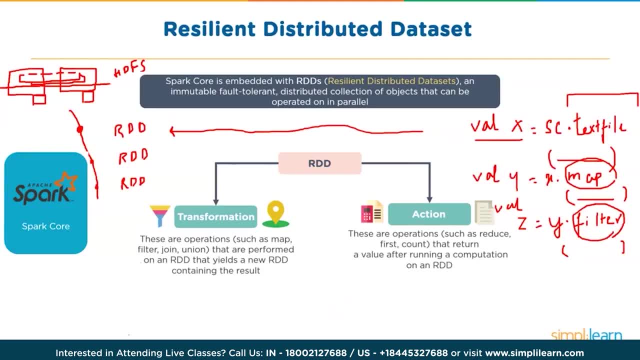 operations such as map filter, join, union and many others will only create RDDs, which basically means it is only creating execution logic. no data is evaluated, no operation is happening right now, only and only when you invoke an action that is. might be you want to print some result. might be. 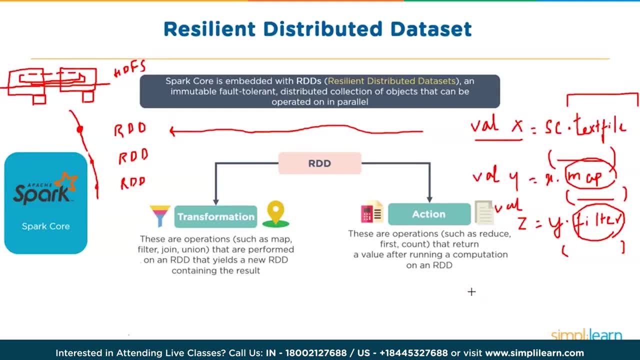 you want to take some elements and see that might be, you want to do a count. so those are actions which will actually trigger the execution of this DAG right from the beginning. so if I here say z dot count, where I would want to just count the number of words which I am, 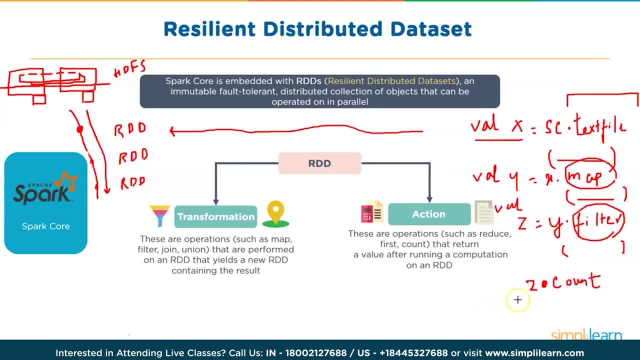 filtering. this is an action which is invoked and this will trigger the execution of DAG right from the beginning. so this is what happens in a spark. now, if I do a z dot count again, it will start the whole execution of DAG again, right from the beginning. so my z dot count second. 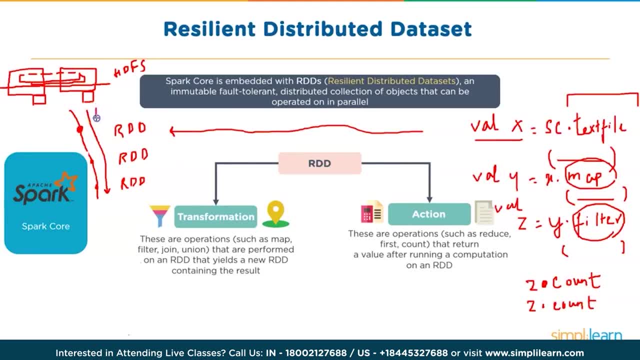 time an action is invoked again, the data will be loaded in the first RDD, then you will have map, then you will have filter and finally you will have result. so this is the core concept of your RDDs and this is how RDD works. so mainly in spark there are 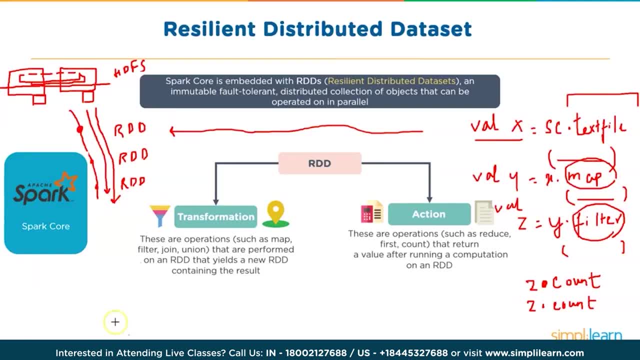 two kind of operations: one is your transformations and one is your actions. transformations, or using a method of spark context, will always and always create an RDD, or you could say, a step in the DAG. actions are something which will invoke the execution, which will invoke the execution from the first RDD. 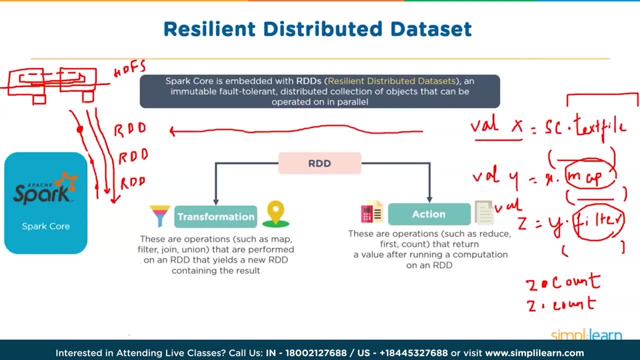 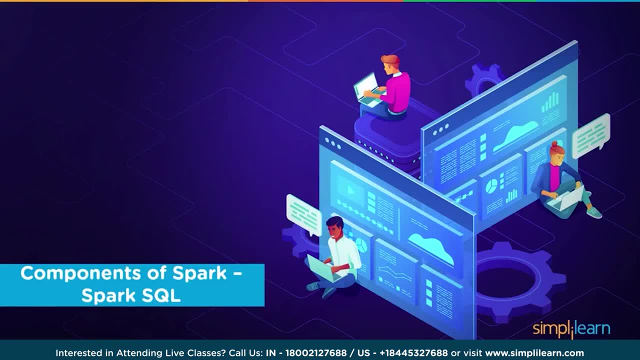 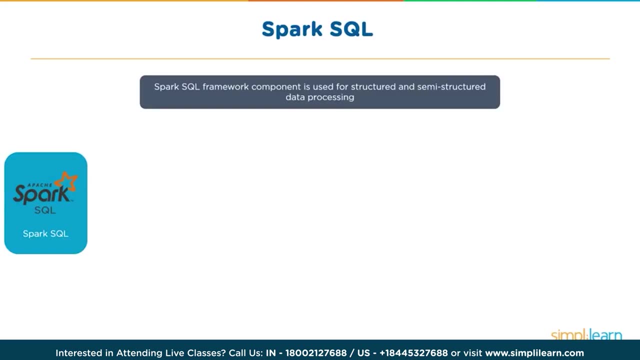 till the last RDD where you can get your result. so this is how your RDDs work. now, when we talk about components of spark, lets learn a little bit about spark SQL. so spark SQL is a component type processing framework which is used for structured and semi structured data processing. 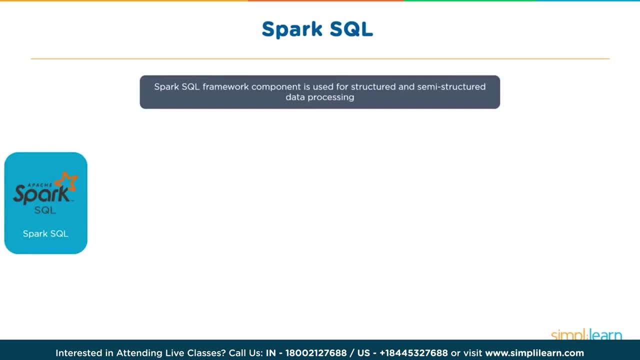 so usually people might have their structured data stored in RDBMS or in files where data is structured with particular delimiters and has a structure. and if one wants to process this structured data, if one wants to use spark to do in memory processing and work on this, 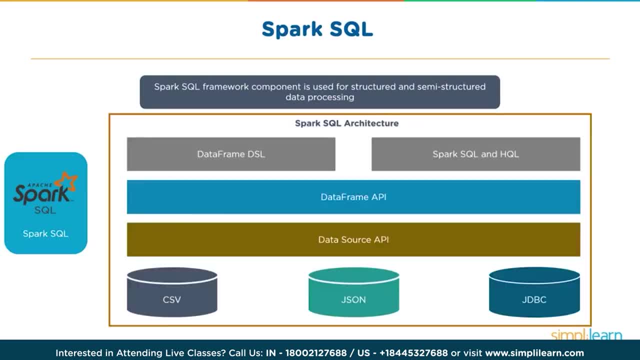 structured data. they would prefer to use spark SQL. so you can work on different data formats, say CSV, JSON. you can even work on smarter formats like Avro Parquet, even your binary files or sequence files. you could have your data coming in from RDBMS, which can then 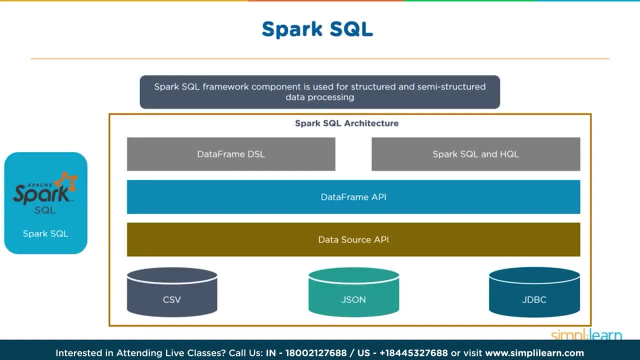 be extracted using a JDBC connection. so, at the bottom level, when you talk about spark SQL, it has a data source API which basically allows you to get the data in whichever format it is. now spark SQL has something called as data frame API. so what are data frames? 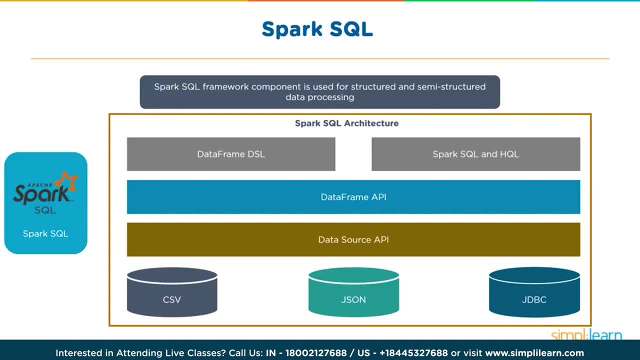 data frames. in short, you can visualize or imagine as rows and columns, or if your data can be represented in the form of rows and columns with some column headings. so data frame API allows you to create data frames. so, like my previous example, when you work on a file, when you want to process it, 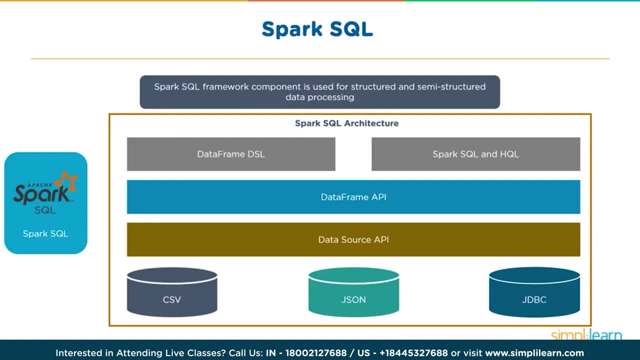 you would convert that into an RDD using a method of spark context or by doing some transformations. so, in the similar way, when you use data frames or when you want to use spark SQL, you would use spark context, which is SQL context, or hive context or spark which. 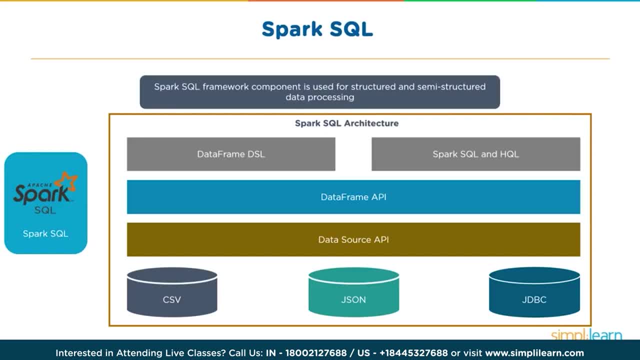 allows you to work with data frames. so, like in my earlier example, we were saying: val x equals sc dot text file. now, in case of data frames, instead of sc you would be using, say, spark dot something. so spark context is available for your data frames API to be used. 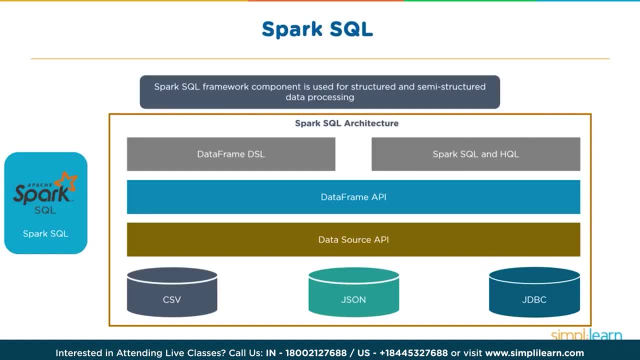 in older versions, like spark 1.6 and so on, we were using hive context or SQL context. so if you were working with spark 1.6, you would be saying val x equals sql context dot. here we would be using spark dot. so data frame API basically allows you to create: 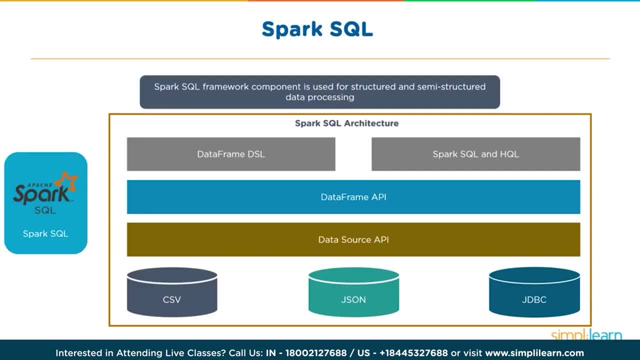 data frames out of your structured data, which also lets spark know that data is already in a particular structure. it follows a format and, based on that, your sparks backend DAG scheduler, right. so when I say about DAG, I talk about your sequence of steps, so spark is already aware of 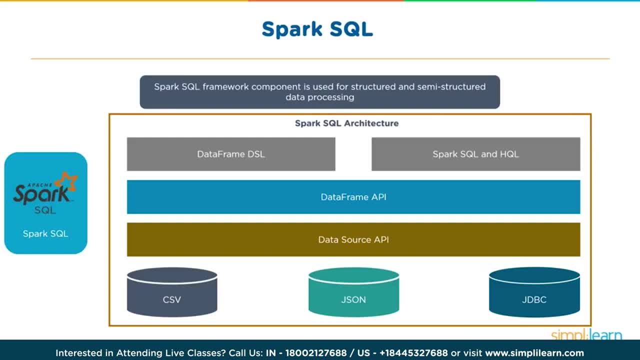 what are the different steps involved in your application? so your data frame API basically allows you to create data frames out of your data and data frames- when I say, I'm talking about rows and columns with some headings, and then you have your data frame DSL language or you can use spark. 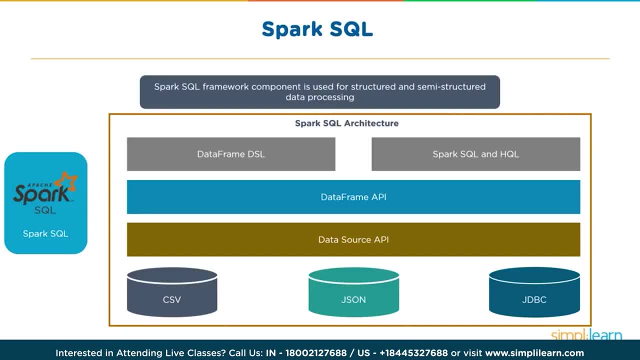 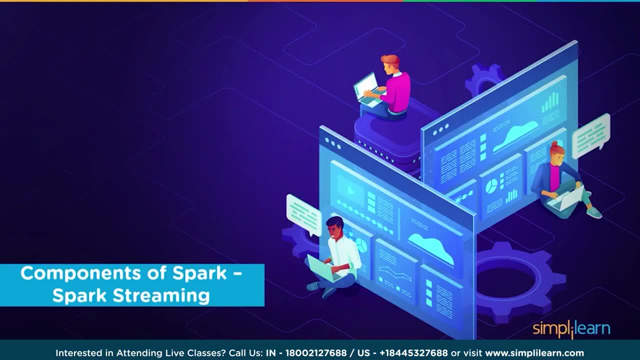 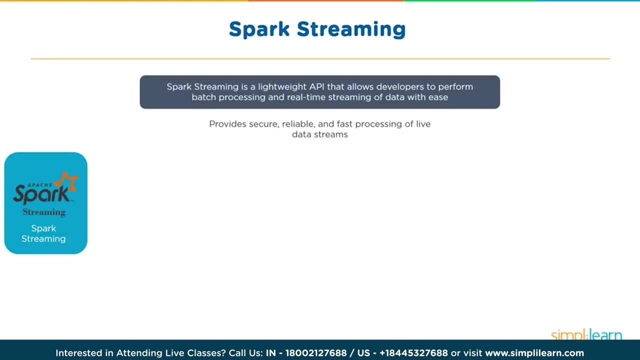 SQL or hive query language. any of these options can be used to work with your data frames. so to learn more about data frames, follow in the next sessions. when you talk about spark streaming now, this is very interesting for organizations who would want to work on streaming data. imagine. 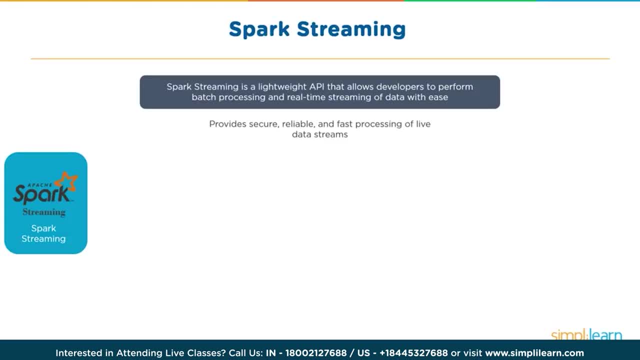 a store like Macy's where they would want to have machine learning algorithms. now, what would these machine learning algorithms do? suppose you have lot of customers walking in the store and they are searching for particular product or particular item, so there could be cameras placed in the store, and this is being already. 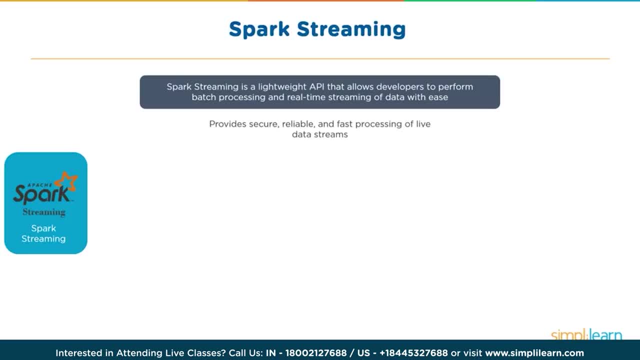 done. there are cameras placed in the store which will keep monitoring in which corner of the store there are more customers. now, once camera captures this information, this information can be streamed in to be processed by algorithms, and those algorithms will see which product or which series of product. 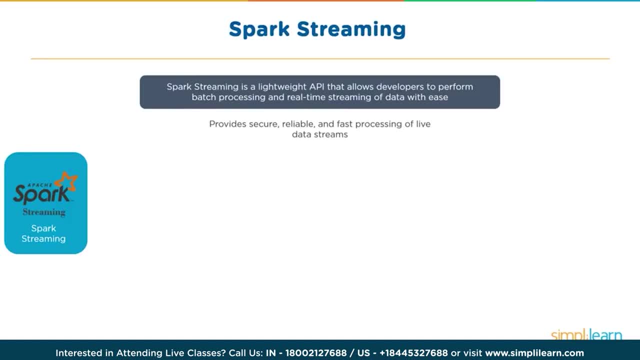 customers might be interested in and if this algorithm in real time can process based on the number of customers, based on the available product in the store, it can come up with a attractive alternative price so that which the price can be displayed on the screen and probably customers would. 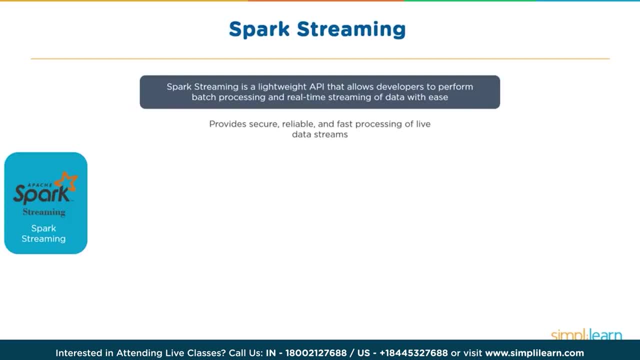 buy the product. now, this is a real time processing, where the data comes in, algorithms work on it, do some computation and give out some result, and which can then result in customers buying a particular product. so the whole essence of this machine learning and real time processing will 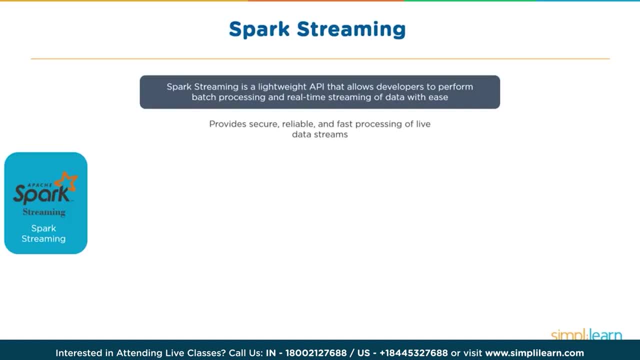 really hold good if and when customers are in the store. or this could relate to even a online shopping portal where there might be machine learning algorithms which might be doing real time processing based on the clicks which customer is doing, based on the clicks, based on customer history. 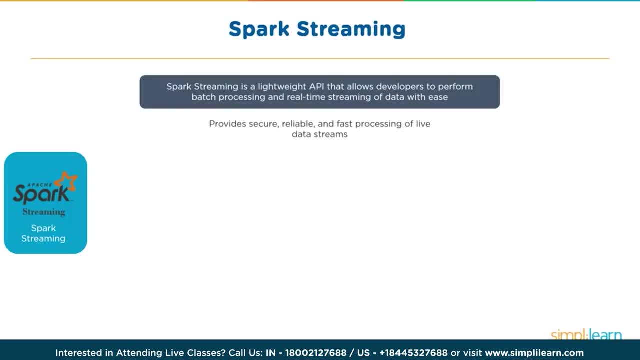 based on customer behavior. algorithms can come up with recommendation of products or better, altered price so that the sale happens now. in this case, we would be seeing the essence of real time processing only in a fixed or in a particular duration of time, and this also means that you should have something. 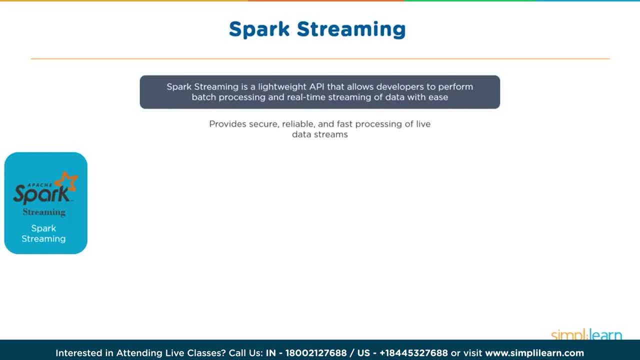 which can process the data as it comes in. so spark streaming is a lightweight API that allows developers to perform batch processing and also real time streaming and processing of data, so it provides secure, reliable, fast processing of live data streams. so what happens here in spark streaming in brief? 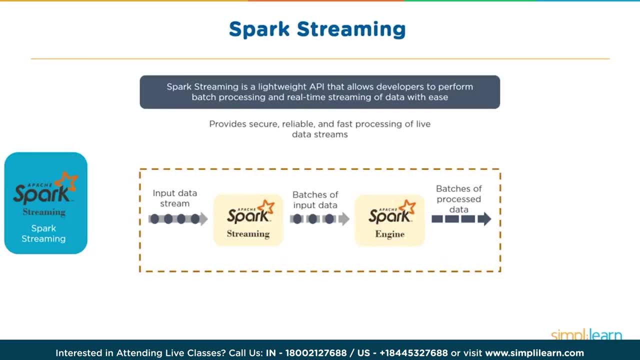 so you have a input data stream. now that data stream could be a file which is constantly getting appended. it could be some kind of metrics, it could be some kind of events based on the clicks which customers are doing or based on the products which they are choosing in a store. this input data, 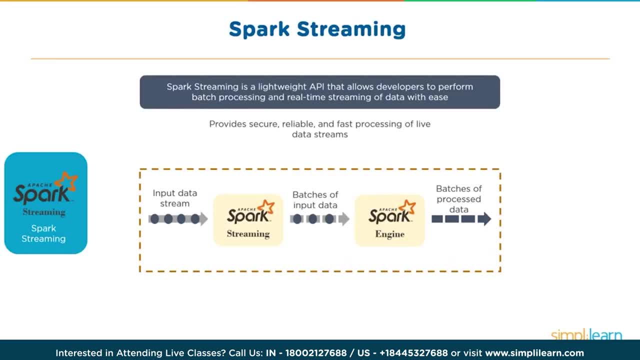 stream is then pushed in through a spark streaming application. now spark streaming application will broke, break this content into smaller streams, what we call as discriticized streams, or batches of smaller data on which processing can happen in frames, so you could say: process my file every five seconds. 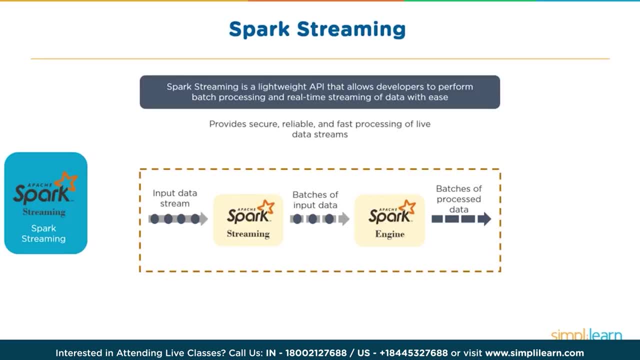 for the latest data which has come in. now there are also some windows based options like. when I say windows, I mean a window of past three events. window of past three events, each event being of five seconds. so your batches of smaller data is processed by spark engine. 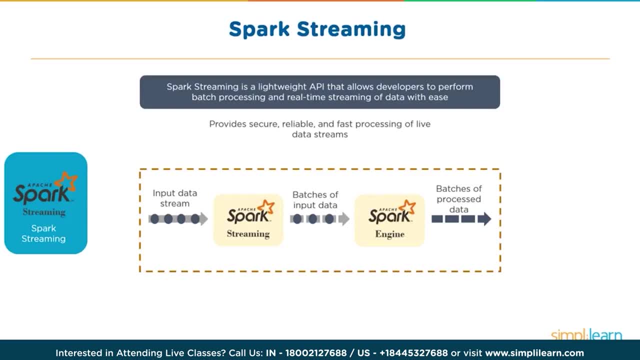 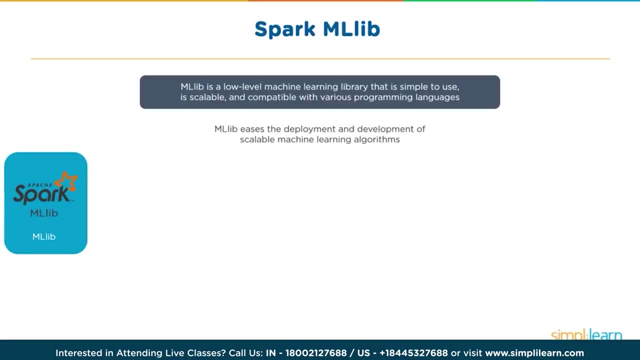 and this process. data can then be stored or can be used for further processing. so that's what spark streaming does. when you talk about ML lib, it's a low level machine learning library that is simple to use, scalable and compatible with various programming languages. now hadoop also has some libraries. 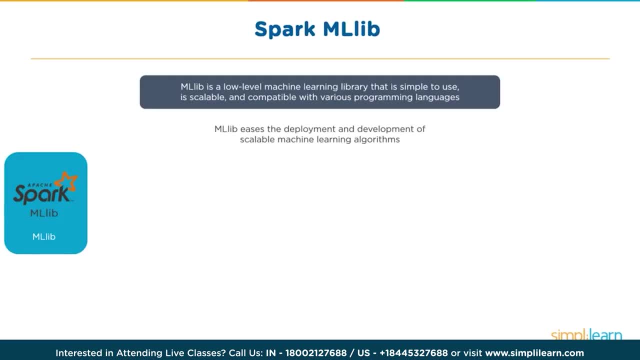 like you have apache mahout, which can be used for machine learning algorithms. however, in terms of spark, we are talking about machine learning algorithms which can be built using ML libs libraries, and then spark can be used for processing. so ML lib eases the deployment and development. 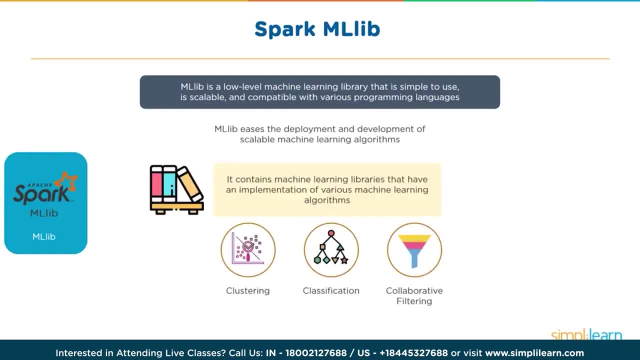 of scalable machine learning algorithms. I mean think about your clustering techniques. so think about your classification: where you would want to classify the data, where you would want to do supervised or unsupervised learning. think about collaborative filtering and many other data science related techniques or techniques which are required to build your recommendation. 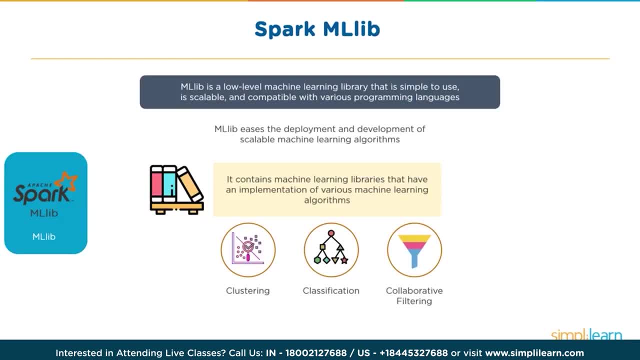 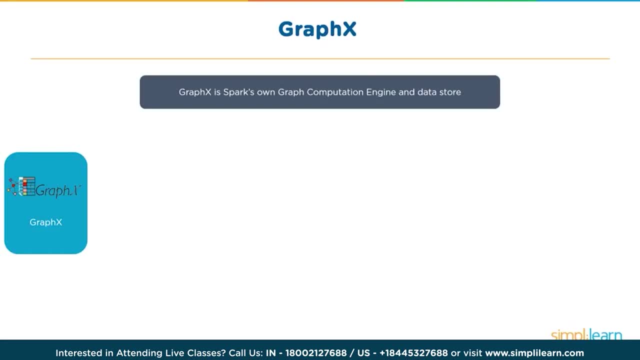 engines or machine learning algorithms can be built using sparks ML. lib. graphics is sparks own graph computation engine. so this is mainly if you are interested in doing a graph based processing. think about Facebook, think about LinkedIn, where you can have your data which can be stored, and that data 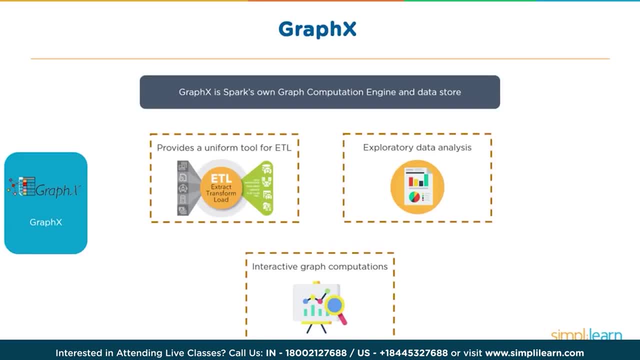 has some kind of network connections, or you could say it is well networked. I could say X is connected to Y, Y is connected to Z, Z is connected to A. so X, Y, Z, A, all of these are in terms of graph, terminologies we call as vertices. 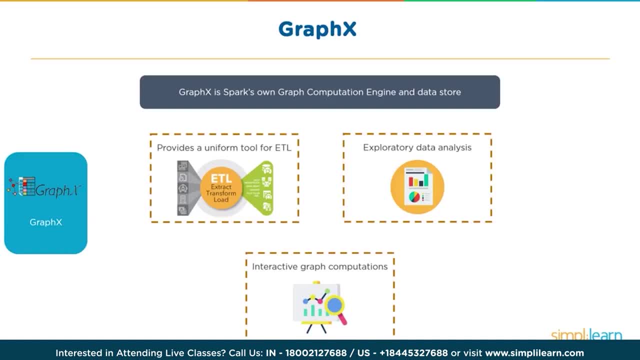 or vertex, which are basically being connected, and the connection between these are called edges. so I could say A is friend to B, so A and B are vertices and friend, a relation between them is the edge. now, if I have my data which can be represented in the form of graphs, if I would 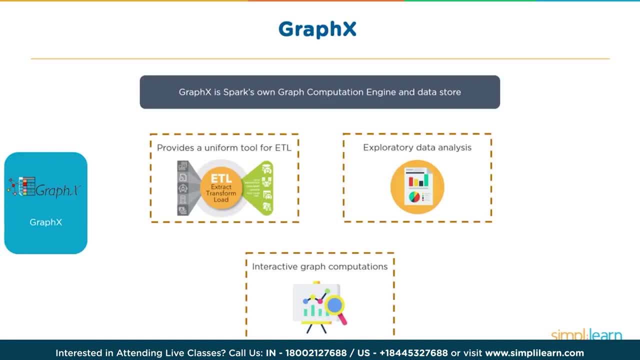 want to do a processing in such way. this could be not only for social media. it could be for your network devices, it could be a cloud platform. it could be about different applications which are connected in a particular environment. so if you have data which can be represented in the form of, 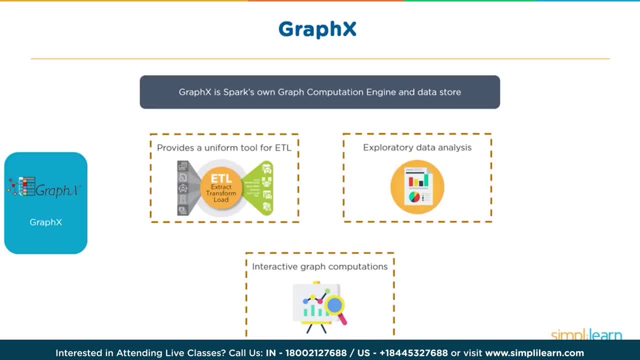 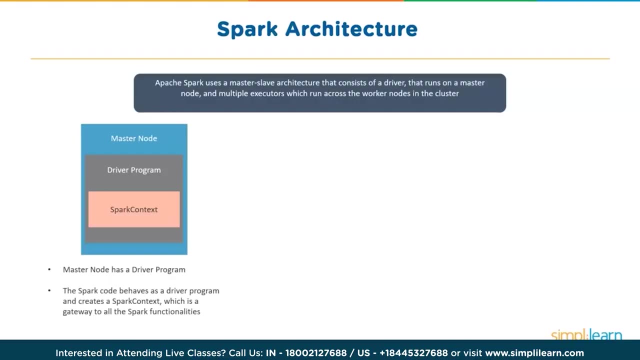 graph, then graphics can be used to do ETL, that is, extraction, transformation, load, to do your data analysis and also do interactive graph computation. so graphics is quite powerful. now, when you talk about spark, your spark can work with your different clustering technologies. so it can work with a. 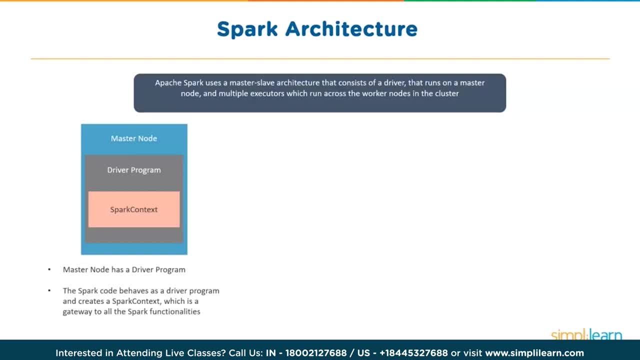 Apache mesos. that's how spark came in, where it was initially, to prove the credibility of Apache mesos. spark can work with yarn, which is usually you will see in different working environments. spark can also work as standalone, that means without Hadoop. spark can have its own setup with master. 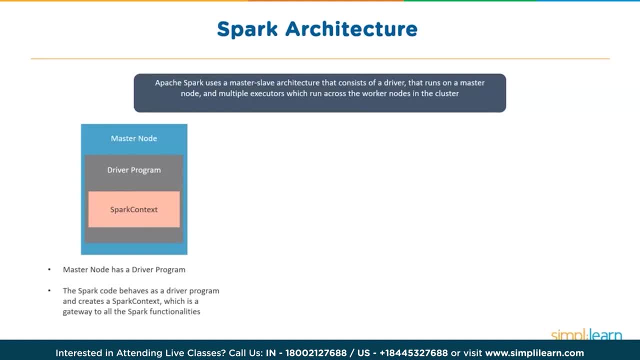 and worker processes. so usually, or you can say technically, spark uses a master slave architecture. now, that consists of a driver program that can run on a master node. it can also run on a client node. it depends on how you have configured or what your application is. and then 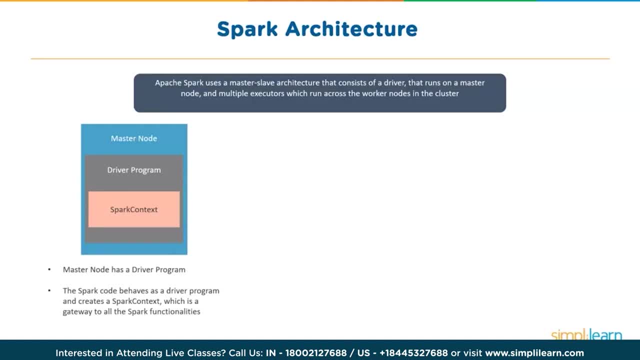 you have multiple executors which can run on worker nodes. so your master node has a driver program and this driver program internally has the spark context. so your spark, every spark application, will have a driver program and that driver program has a inbuilt or internally used spark context which 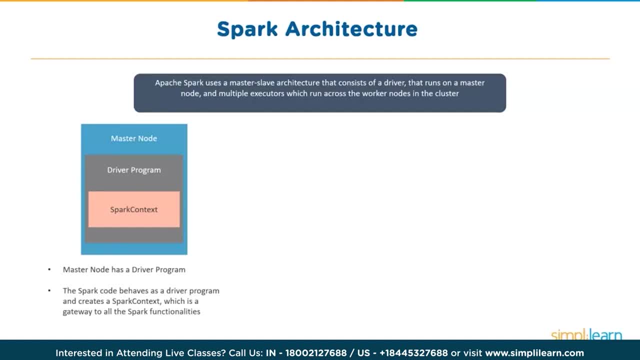 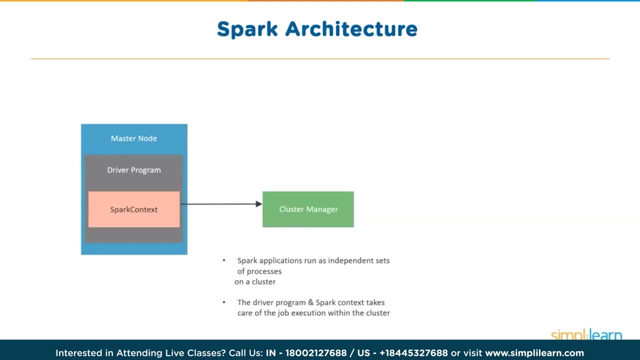 is basically your entry point of application for any spark functionality. so your driver or your driver program interacts with your cluster manager. now, when I say interacts with cluster manager, so you have your spark context, which is the entry point that takes your application request to the cluster manager. now, as I said, 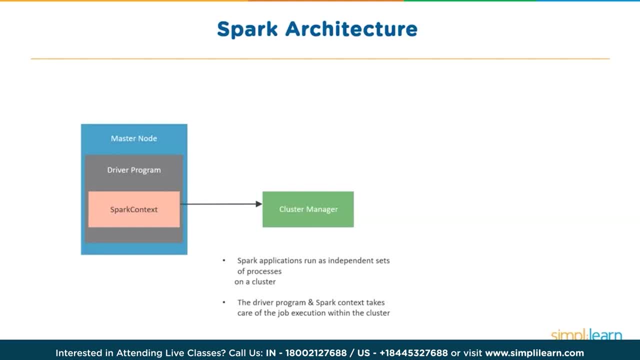 your cluster manager could be say: Apache mesos, it could be yarn, it could be spark standalone master itself. so your cluster manager, in terms of yarn, is your resource manager. so your spark application internally runs as series or set of tasks and processes your driver program wherever that is run. 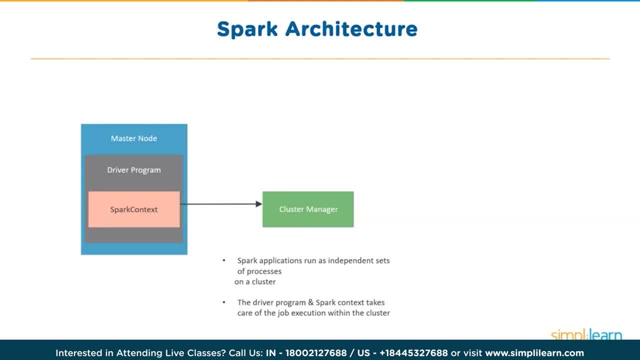 will have a spark context and spark context will take care of your application execution. how does that do it? spark context will talk to cluster manager. so your cluster manager could be yarn and in terms of tasks, you can say cluster manager for yarn would be resource manager. so at high, 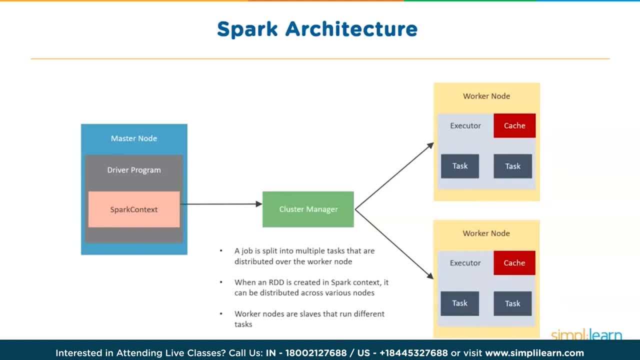 level we can say a job is split into multiple tasks and those tasks will be distributed over the slave nodes or worker nodes. so whenever you do some kind of transformation or you use a method of spark, context and RDD is created and this RDD is distributed across multiple nodes, as I explained. 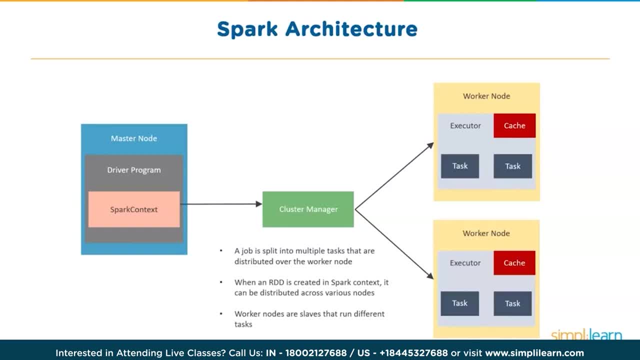 earlier worker nodes are the slaves that run different tasks. so this is how a spark architecture looks like. now we can learn more about spark architecture and its interaction with yarn. so usually what happens when your spark context interacts with the cluster manager? so in terms of yarn, I could say resource manager. 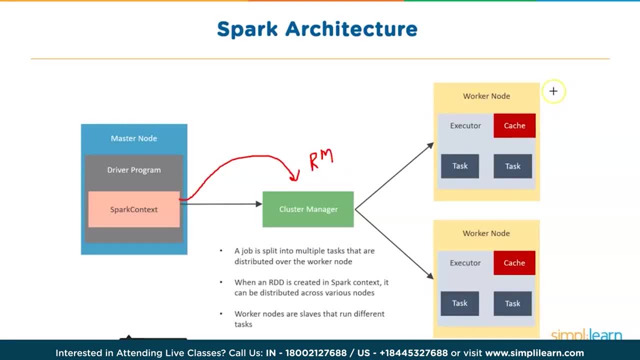 now we already know about yarn. so you would have say node managers running on multiple machines and each machine has some RAM and CPU cores allocated for your node manager. on the same machine you have the data nodes running which obviously are there to have the Hadoop related data. so whenever the 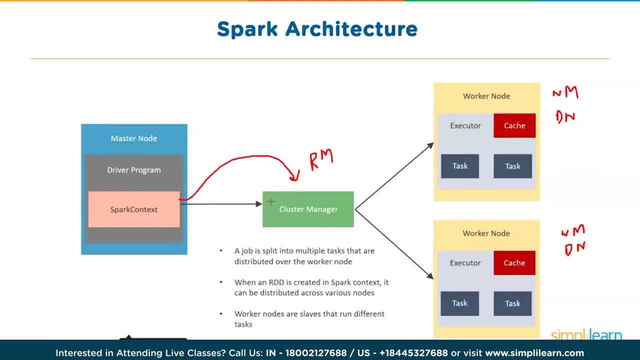 application wants to process the data. your application, via spark context, contacts the cluster managers. that is resource manager. now what does resource manager do? resource manager makes a request, so resource manager makes request to the node manager of the machines, wherever the relevant data resides. asking for containers? so your resource manager is 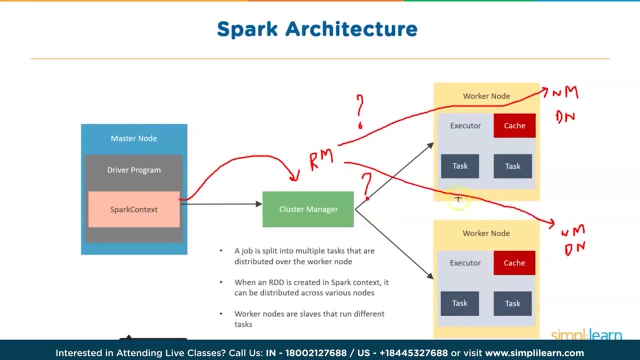 negotiating or asking for containers from node manager saying, hey, can I have a container of one GB RAM and one CPU core, can I have a container of one GB RAM and one CPU core? and your node manager, based on the kind of processing it is doing, will approve. 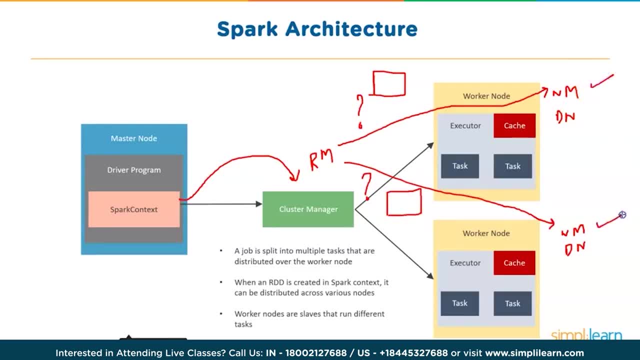 or deny it. so node manager would say: fine, I can give you the container. and once this container is allocated or approved by node manager, resource manager will basically start an extra piece of code called appmaster. so appmaster is responsible for execution of your applications, whether those are spark applications or 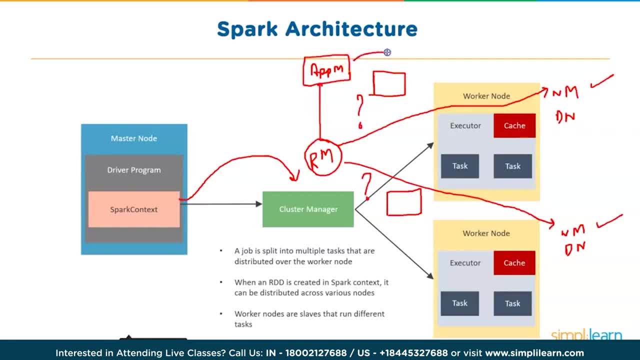 MapReduce. so your application master, which is a piece of code, will run in one of the containers, that is, it will use the RAM and CPU core and then it will use the other containers which were allocated by node manager to run the tasks. so it is within this container which 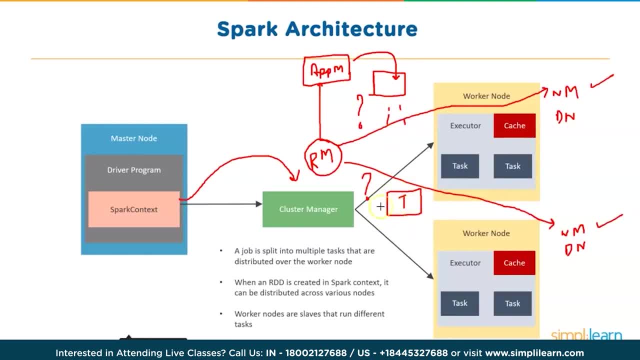 can take care of execution. so what is a container? a combination of RAM and CPU core. so it is within this container we will have a executor process which would run, and this executor process is taking care of your application related tasks. so that's how overall spark works. 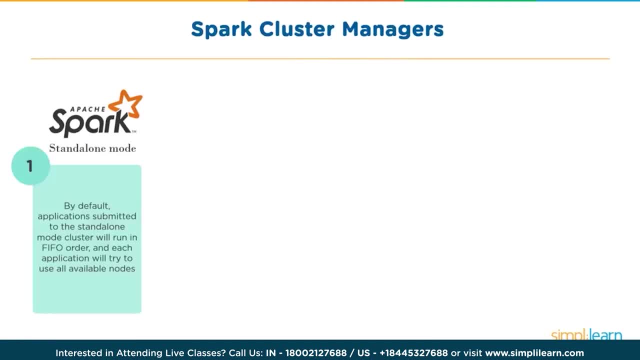 in integration with yarn. now let's learn about this. spark cluster managers. as I said, spark can work in a standalone mode, so that is without Hadoop. so by default, application submitted to spark standalone mode cluster will run in FIFO order and each application will try to use all. 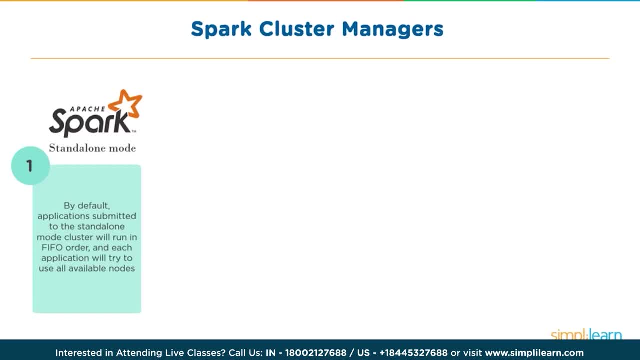 the available nodes. so you could have a spark standalone cluster, which basically means you could have multiple nodes. on one of the nodes you would have the master process running and on the other nodes you would have the spark worker processes running. so here we would not have any. 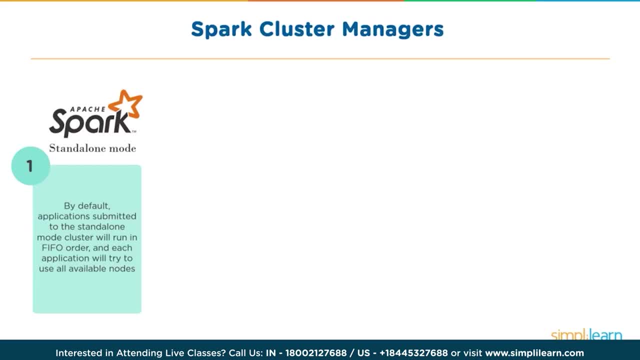 distributed file system because spark is standalone and it will rely on an external storage to get the data, or probably the file system of the nodes where the data is stored, and processing will happen across the nodes where your worker processes are running. you could have spark working with. 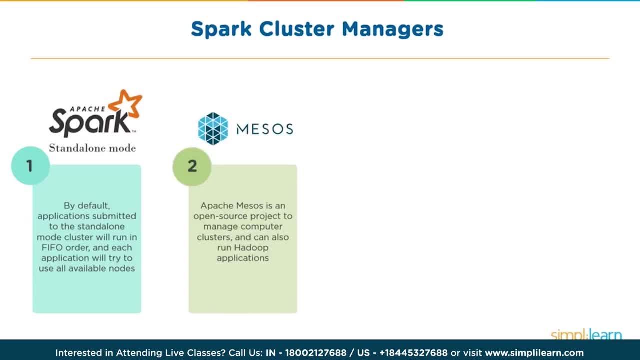 apache mesos. now, as I said, apache mesos is an open source project to manage your computer clusters and can also run Hadoop applications. apache mesos was introduced earlier and spark came in and has existence. to prove the credibility of apache mesos, you can have spark working with Hadoop's. 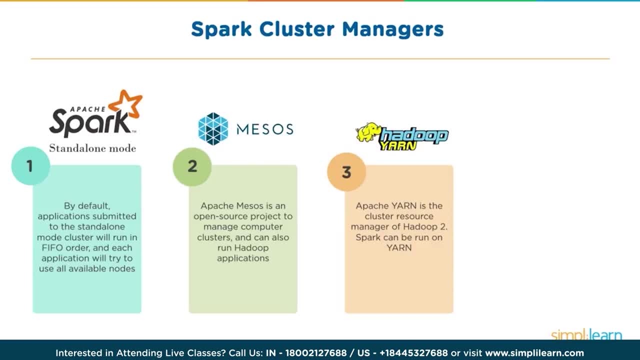 yarn. this is something which widely you will see in different working environments. so yarn, which takes care of your processing and can take care of different processing frameworks, also supports spark. you could have kubernetes now. that is something which is making a lot of news in today's world. it is an open source. 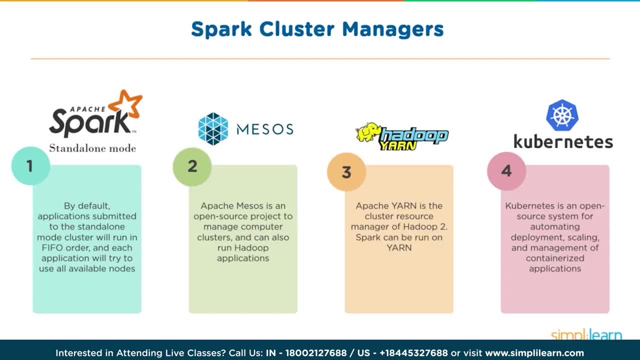 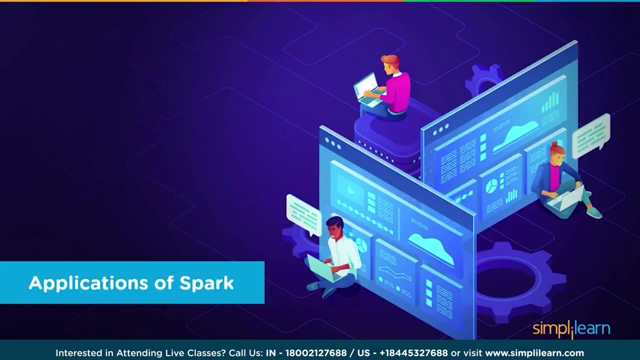 system for automating deployment, scaling and management of containerized applications, so where you could have multiple docker based images which can be connecting to each other. so spark also works with kubernetes. now let's look at some applications of spark. so jpmorgan chase and company uses spark to. 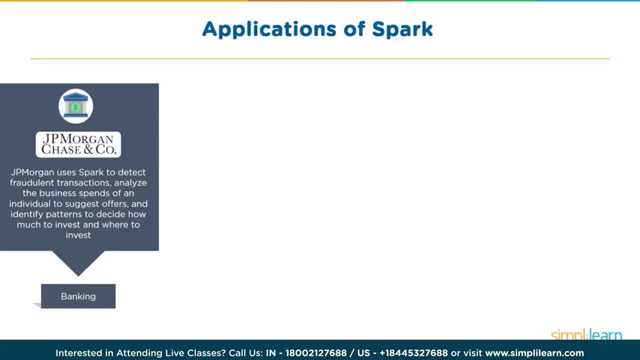 detect fraudulent transactions, analyze the business spends of an individual to suggest offers and identify patterns to decide how much to invest and where to invest. so this is one of the examples of banking. lot of banking environments are using spark due to its real time processing capabilities and in memory faster. 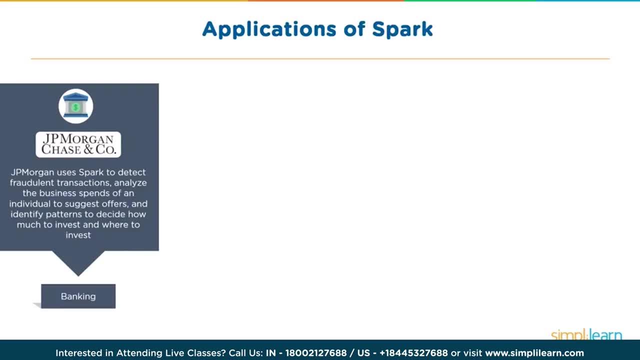 processing where they could be working on fraud detection or credit analysis or pattern identification and many other use cases. alibaba group that uses also spark to analyze large data sets of data, such as real time transaction details. now that might be based online or in the stores. looking at the browsing history: 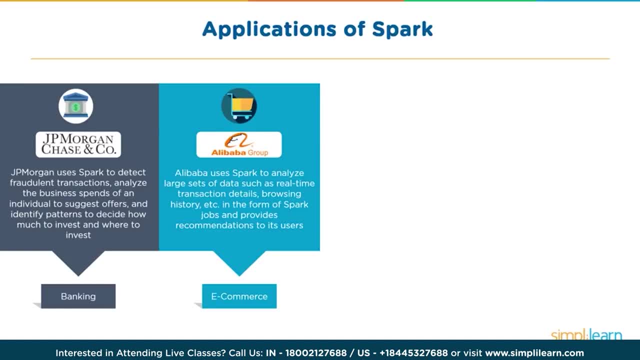 in the form of spark jobs and then provides recommendations to its users. so alibaba group is using spark in its e-commerce domain. you have iqvia now. this is a leading healthcare company that uses spark to analyze patients data, identify possible health issues and diagnose it based on their medical history. 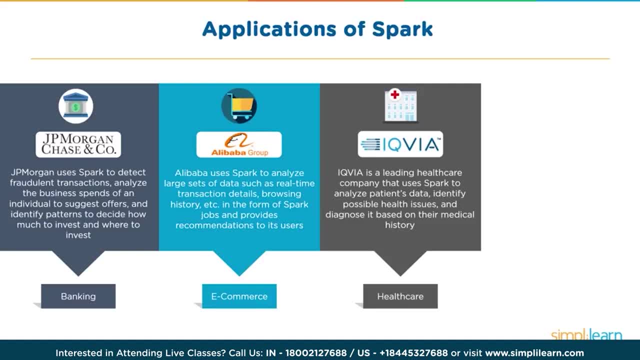 so there is lot of work happening in healthcare industry, where real time processing is finding lot of importance, and real time and faster processing is what is required. so healthcare industry and iqvia is also using spark. you have netflix, which is known, and you have riot games, so entertainment. 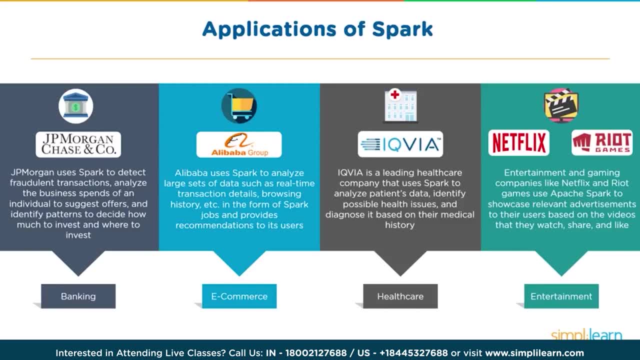 and gaming companies like netflix and riot games use apache spark to showcase relevant advertisements to their users based on the videos that they have watched, shared or liked. so these are few domains which find use cases of spark. that is banking, e-commerce, healthcare, entertainment, and then there are many more which 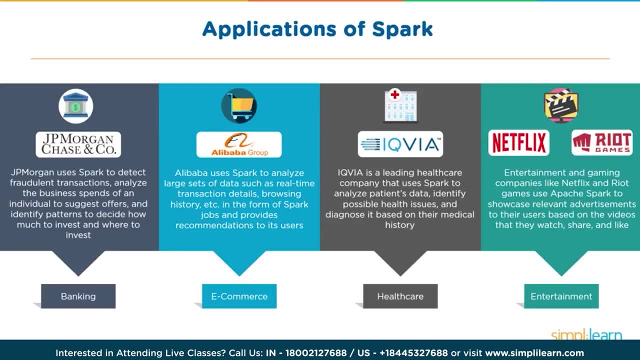 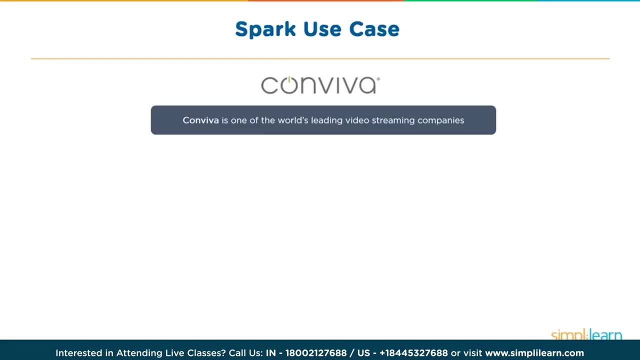 are using spark in their day to day activities for real time in memory, faster processing. now let's discuss about spark's use case and let's talk about conviva, which is world's leading video streaming companies. so video streaming is a challenge. now, if you talk about youtube, which has 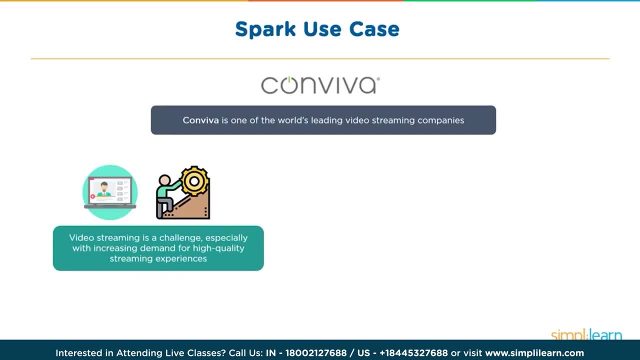 data. you could always read about it. so youtube has data which is worth watching 10 years. so there is huge amount of data where people are uploading their videos or companies are doing advertisements and this videos are streamed in or can be watched by users. so video streaming. 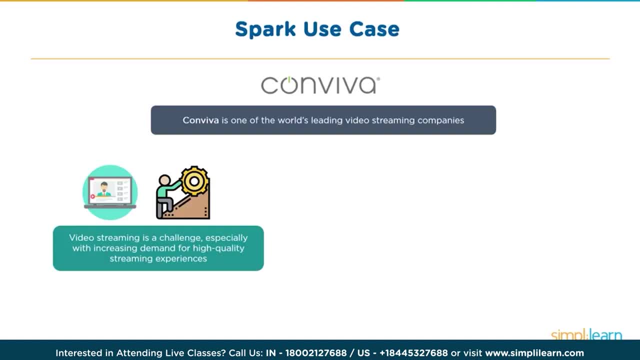 is a challenge, and especially with increasing demand for high quality streaming experiences. conviva collects data about video streaming quality to give their customers visibility into the end user experience. they are delivering. now how do they do it? apache spark again. using apache spark, conviva delivers a better. 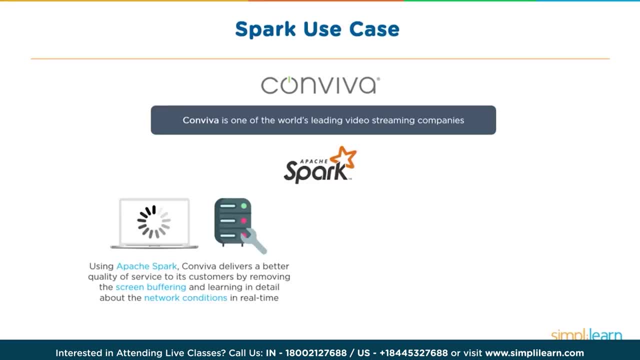 quality of service to its customers by removing the screen buffering and learning in detail about network conditions in real time. this information is then stored in the video player to manage live video traffic coming in from 4 billion video feeds every month. to ensure maximum retention, now using apache spark. 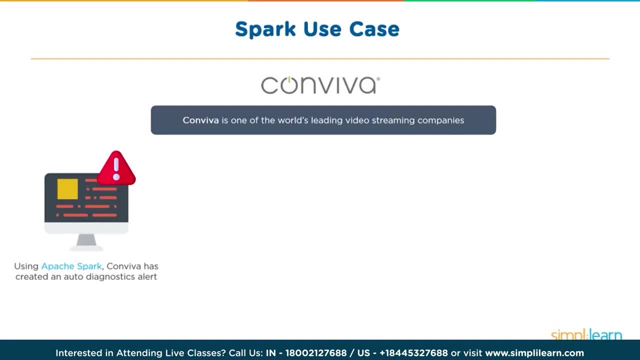 conviva has created an auto diagnostics alert. it automatically detects anomalies along the video streaming pipeline and diagnoses the root cause of the issue. now this really makes it one of the leading video streaming companies based on auto diagnostic alerts. it reduces waiting time before the video starts. it avoids buffering. 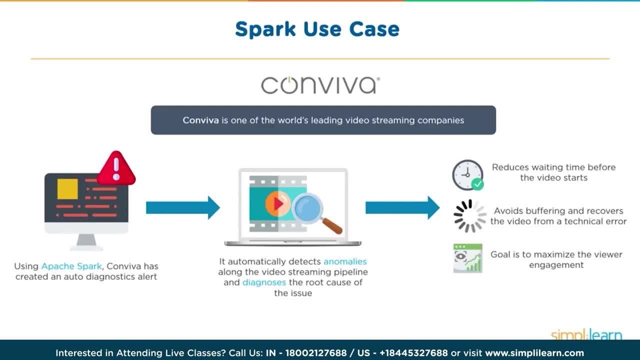 and recovers the video from a technical error, and the whole goal is to maximize the viewer engagement. so this is spark's use case, where conviva is using spark in different ways to stay ahead in video streaming related deliveries. so let's have a quick demo on setting up spark. 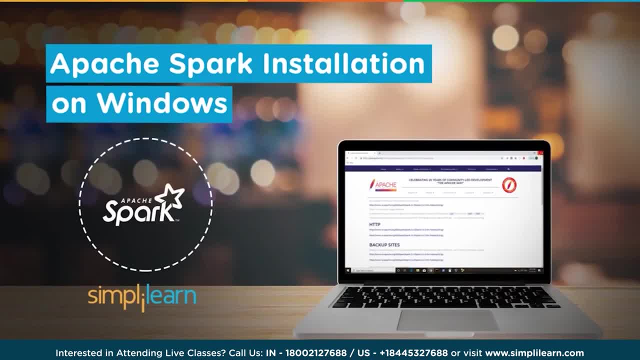 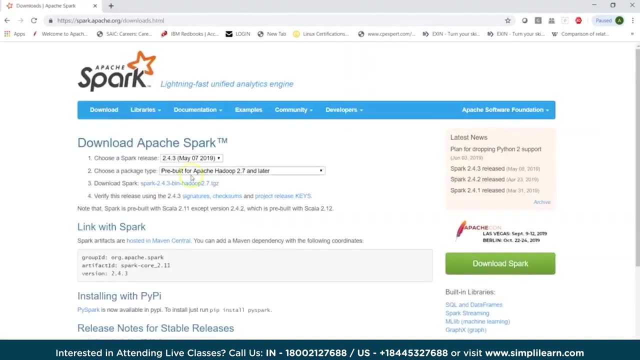 on windows and trying out the spark's interactive way of working. for this first thing is you will have to download spark. now you can just go to google and type spark download and once you click on this link it shows you a spark release, a package type, which says: 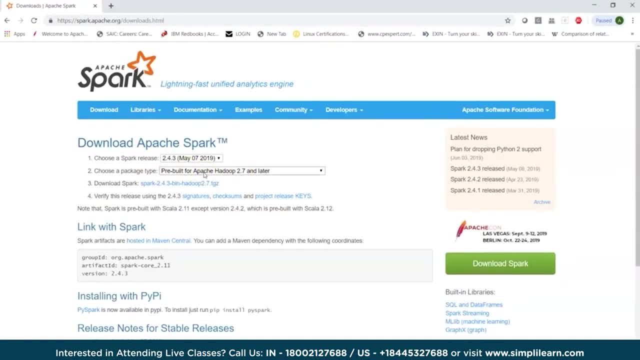 prebuilt. so we will have to get a prebuilt apache hadoop related spark. so here i will choose, say, spark 2.4.3, and i will choose prebuilt for apache 2.6, and then i can just click and download on this spark 2.4.3. 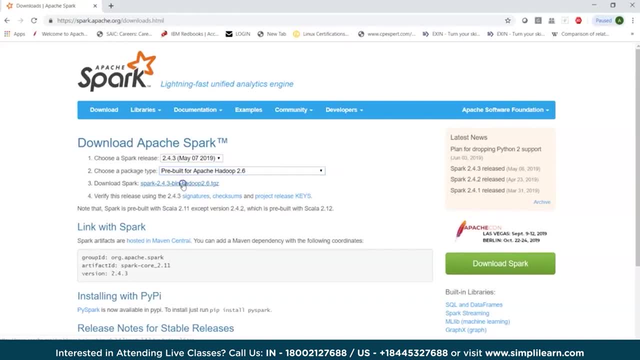 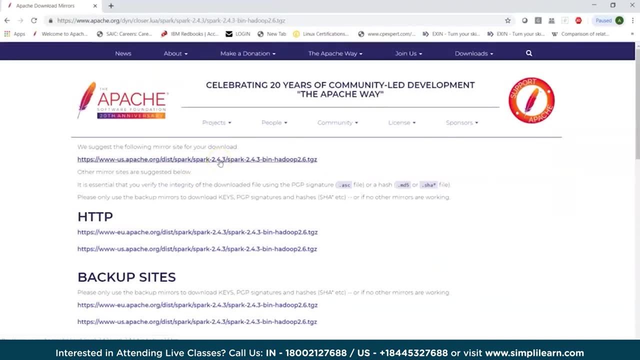 bin hadoop 2.6 tar file. once you click on this link takes you to the mirror site and you can just click on this link and download spark 2.4.3. once this is done, which i have already downloaded here, i can go to my. 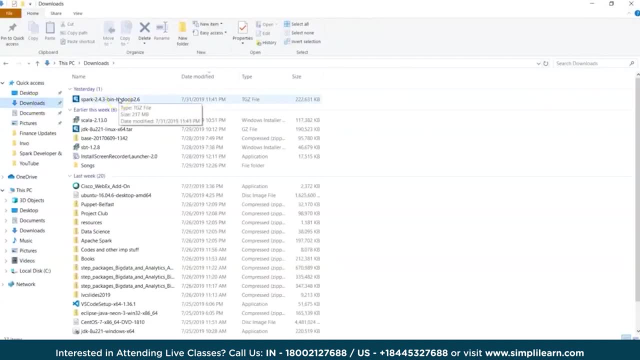 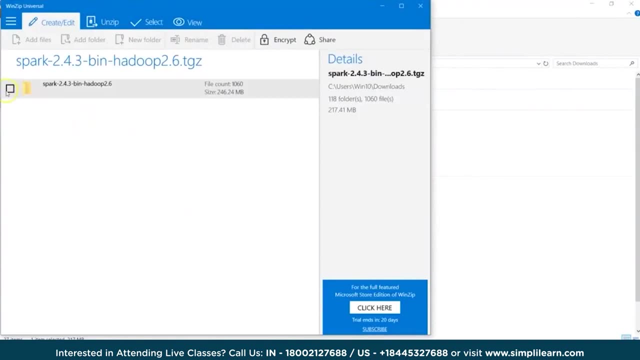 downloads and it shows that i have a tar file. now we will have to untar it or unzip it. so i can click on this link and i already have winzip which allows me to unzip spark 2.4.3. i can choose a location so i can say: 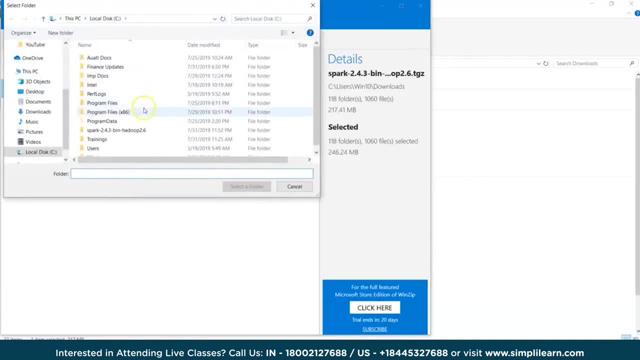 unzip. click on unzip, choose local, and then i can choose one of my folders. so i have already unzipped it here, and that's how my spark 2.4.4 directly exists here. 2.4.4, i'm sorry. now let's go. 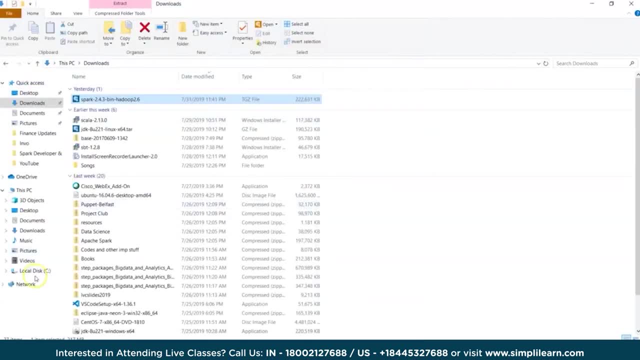 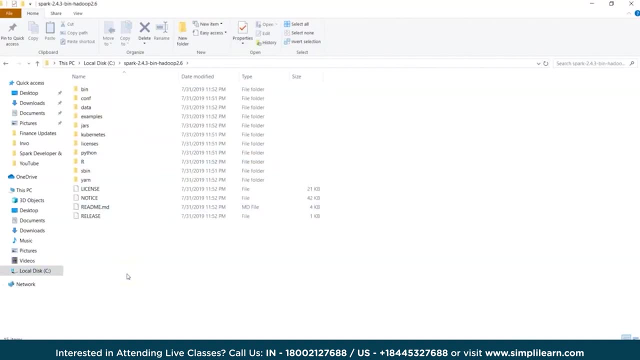 and look into this directory and what it contains so i can click on c drive and then spark 2.4.3 and this has the folders which are required for us to use spark. if you look in bin, we have different applications and commands which we can use. 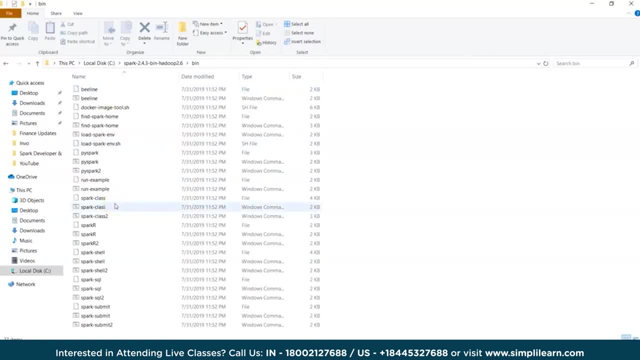 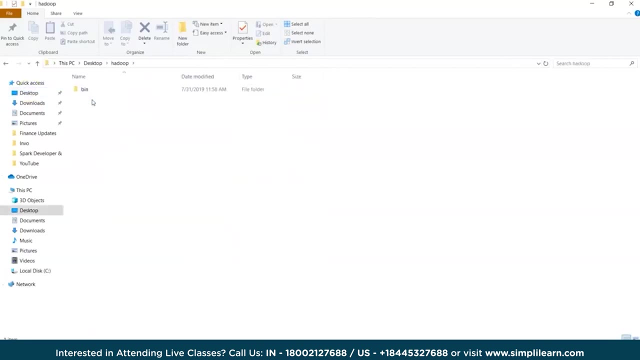 and if you also see, i would have added one of the utilities here either. we can have the win utils, because spark will need hadoop and we are planning to use spark on windows. so what we need is this. so i have in my desktop a hadoop directory. 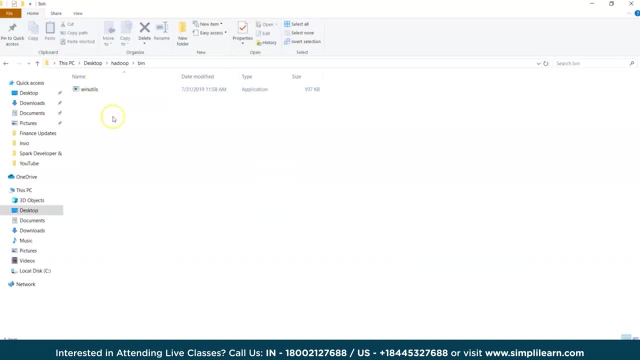 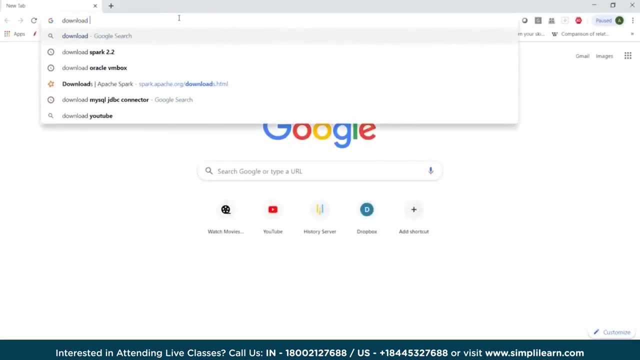 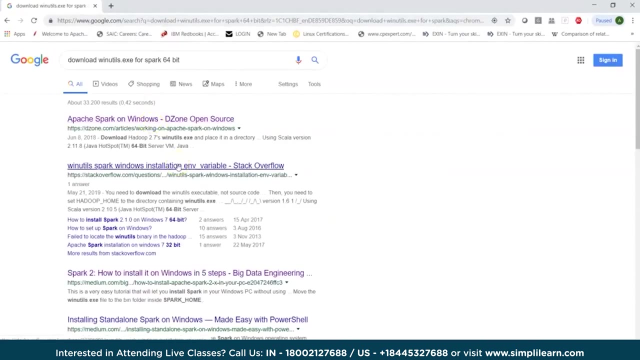 which has a bin folder, and here i have downloaded a win utils executable file which you can always search on internet and you can say download win utils exe for spark 64 bit and then you can find the link from where you can download this. for example, we can click on: 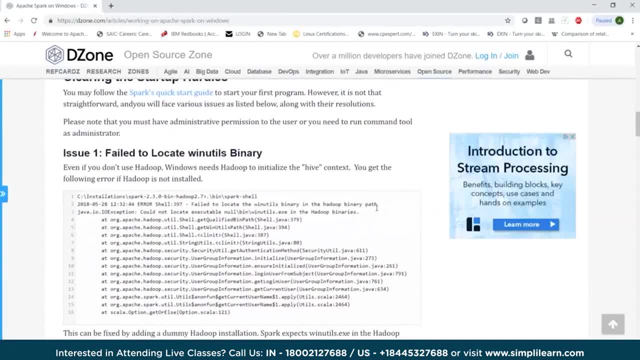 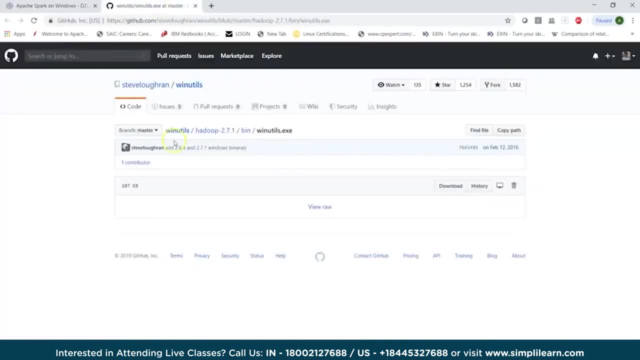 this and here we can search for win utils. so here we have the link. i can open this link in a different tab and this basically shows me win utils for hadoop 2.7.1. similarly you can search for hadoop 2.6 and you. 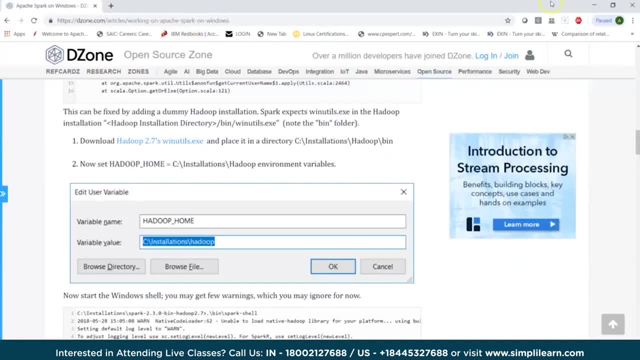 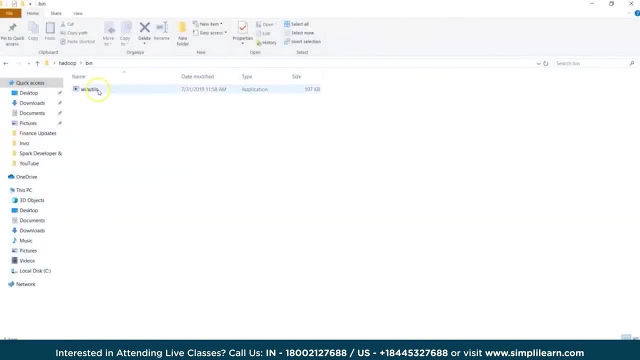 can download. however, 2.7 will also work fine. now i have downloaded win utils exe and that's in this hadoop folder within bin. i have this, so we need two things here. one is spark, which is untarred and in a particular location, and then 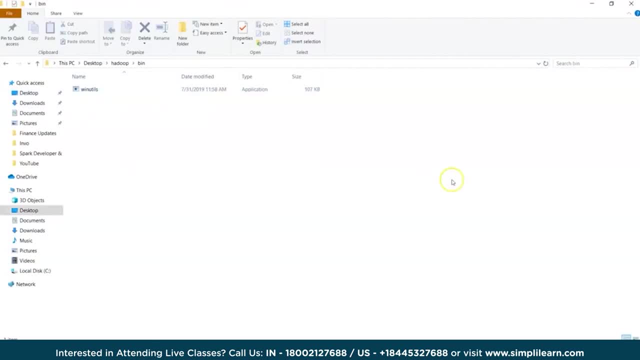 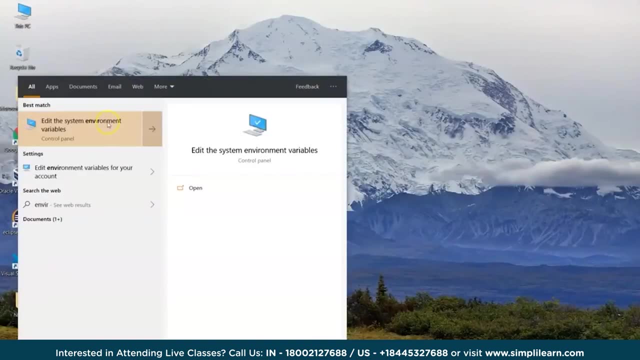 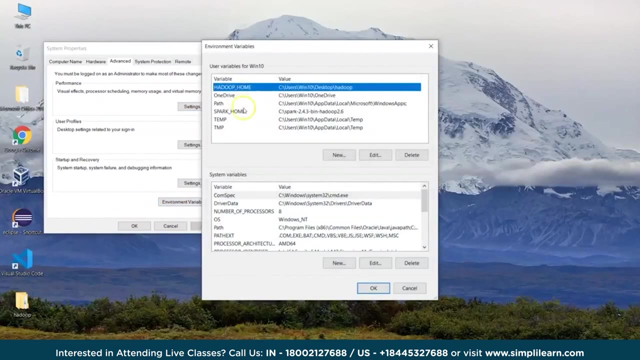 your hadoop, which has bin, and this has win utils. now, once you have these things, you can set your environment variables by just typing envir. go to your edit system, environment variables, click on environment variables and here, if you see, i have added two variables, so you can just click on new. 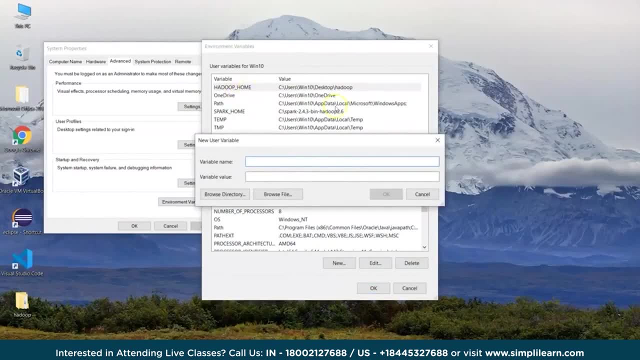 and then you can give your variable name as hadoop underscore home and then you can give the path where you have your hadoop directory that contains bin and that contains win utils exe. i also have added spark home, which points to my spark directory. now, once you have this, you 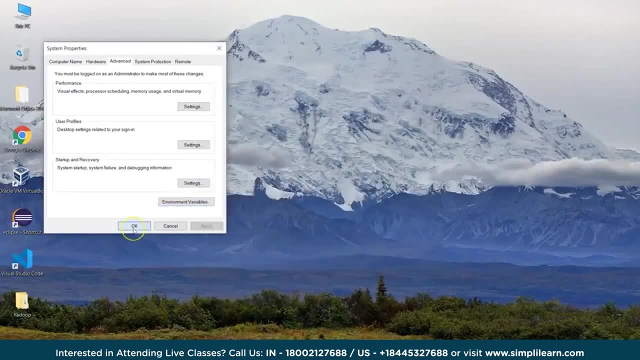 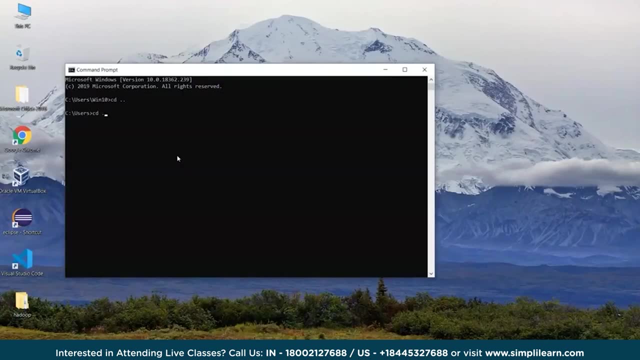 are ready to use your spark on windows in local mode. once this is done, i can open up my command prompt, and here i need to go to my spark directory. i can just say cd, spark, .4.3, and then i can do a dir slash p. 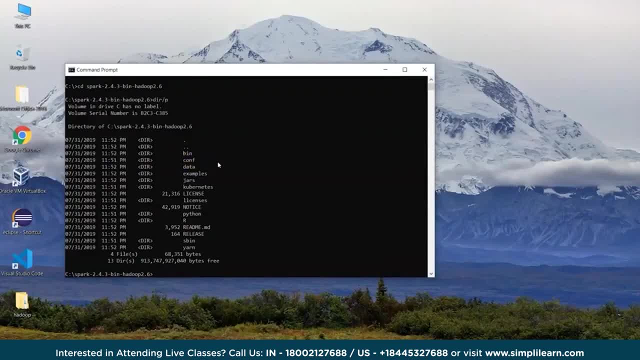 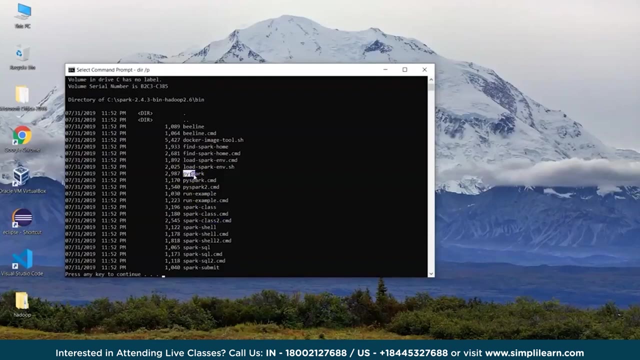 which shows me the folders where we have bin. so to execute spark, we can look into what our bin has, and it has different programs, such as you have spark shell to work with scala and in an interactive way of working with spark. you can also use py spark, which allows you to use 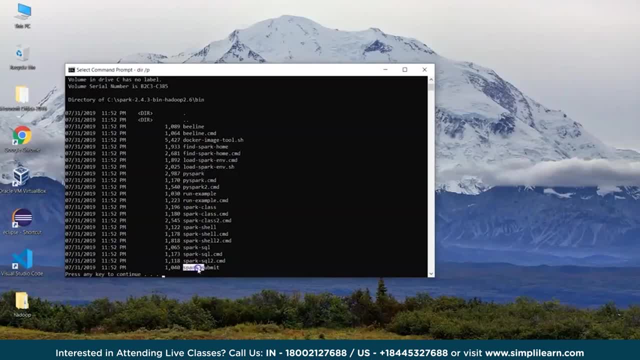 python to work with spark and you also have spark submit if you have packaged your application in a jar file to submit it on a cluster. so in this case we would be using spark in a local mode. so let's use spark shell and test it. so i can just say spark. 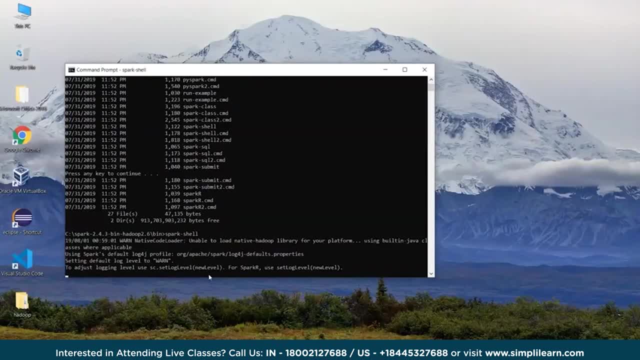 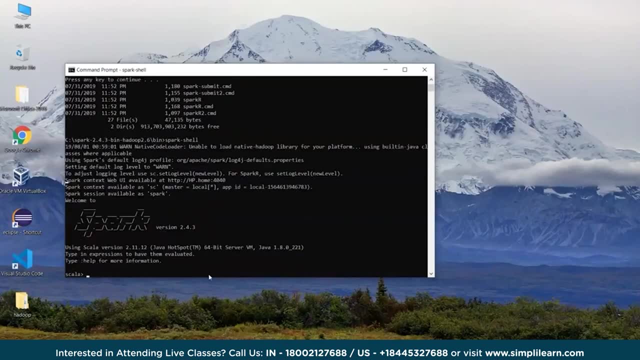 shell in this way to start my spark in an interactive way. now, based on the path which you have set for your win utils exe and spark shell, you should be able to use spark. so it says: welcome to spark version 2.4.3 it. 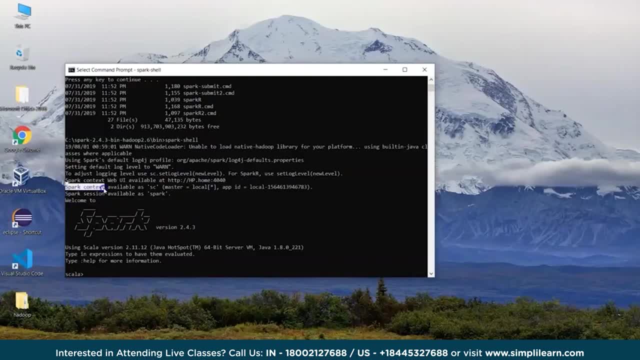 also shows that spark context, which is the entry point of your application, is available as sc, wherein it is connecting to master as local and it has an application id. it also shows you a spark ui which you can look at and it says spark session is available as spark. so if 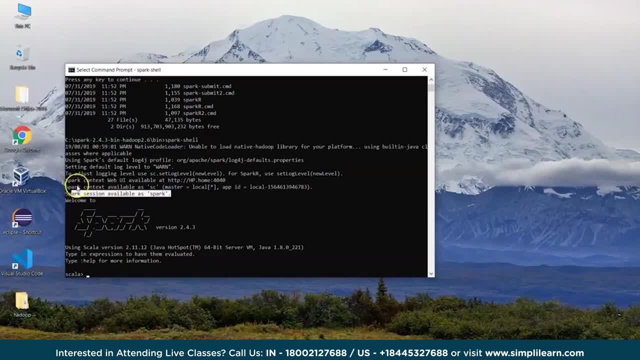 you are interested in working with spark core, that is, with rdd's, we would be using spark context, and if you are interested in working with spark sql, that is, data frames and data sets, then we can be using spark session. so let's try it out so we can declare. 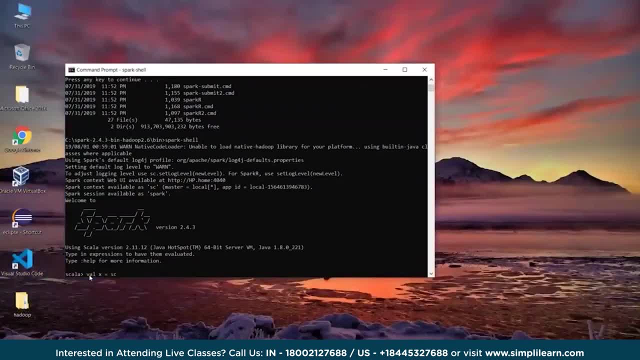 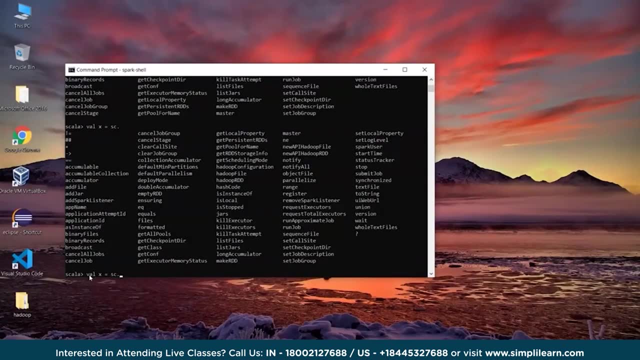 a variable that is a immutable variable, and now i will use spark context with a method of spark context, so i could just do a tab to see what are the available options within your spark context, and here we can use one of them to read a file. so i will use 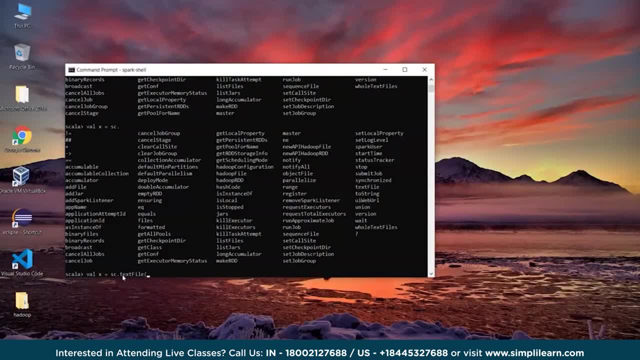 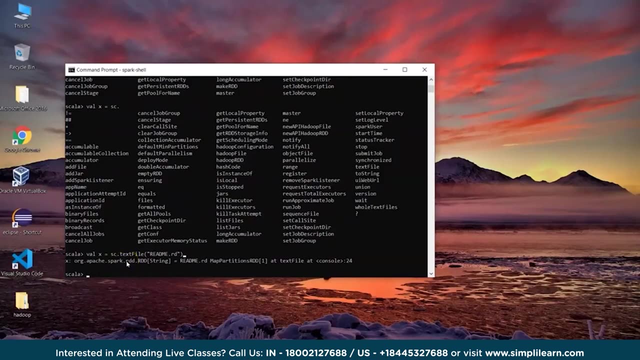 sctxt file and then i need to point to a file. so i already know that in my spark directory i have a file called readmerd and this is the method of spark context: if i enter, it will create a rdd. now, as i have explained about rdd's, 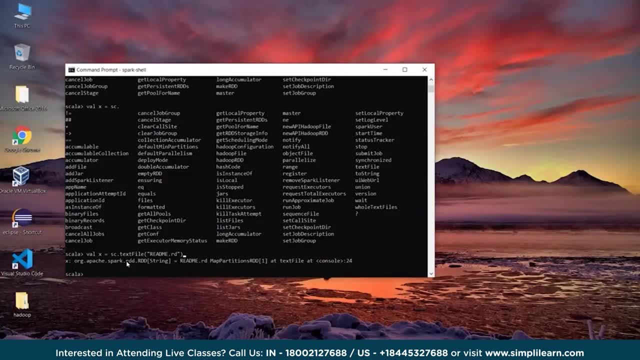 these are resilient distributed data sets. there is no evaluation happening right now, so even if this file does not exist, i would still have an rdd created. now i can go further and do some more transformations on this, so i could say val y and then i could say take x. 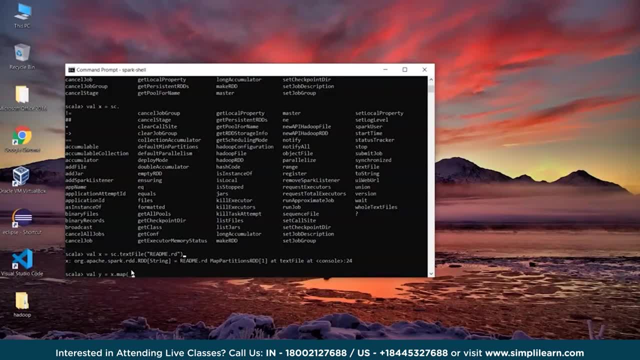 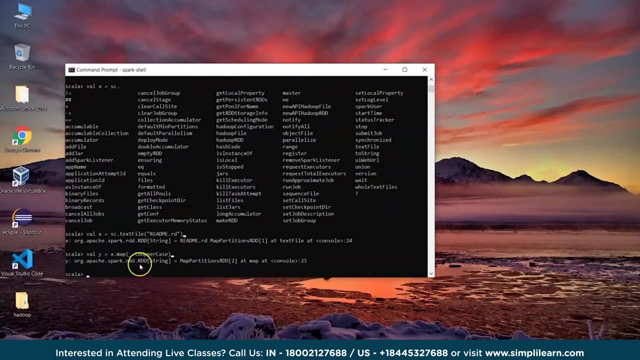 i would like to do a map transformation on it and i would use two uppercase. now this is a inbuilt function where i would want to convert the content of this file into uppercase. when i hit on enter, it again creates an rdd, and this rdd is: 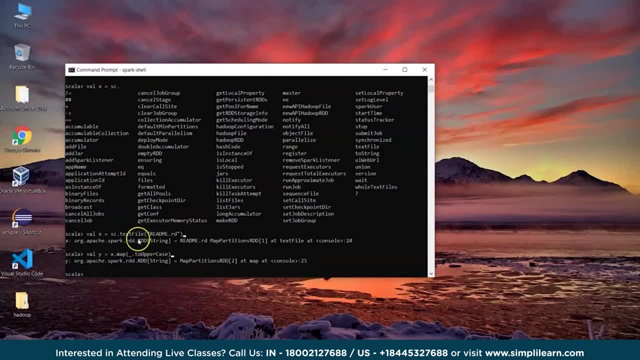 basically a child rdd of the parent rdd created by text file. remember, here we don't have any evaluation happening or any execution happening. it has just transformation which will lead to creation of further rdd's. now we can invoke an action to see the result and 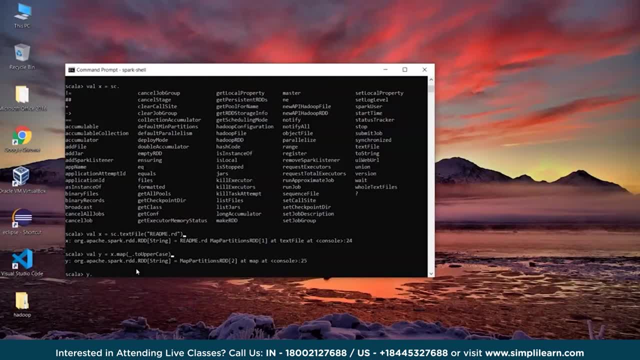 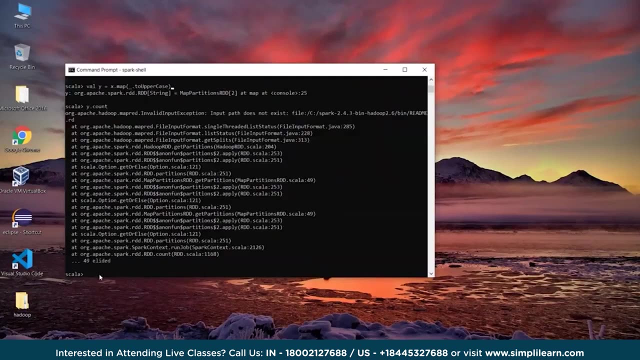 whenever you invoke an action it will trigger the execution of your DAG starting from your first rdd till the last transformation you did before invoking an action. so i could just say count to see how many lines it has. and once i do this it says input path does not. 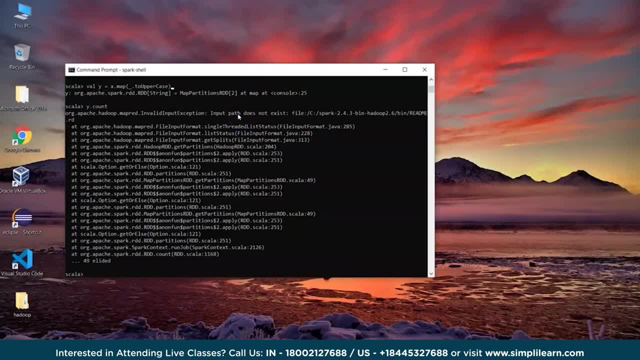 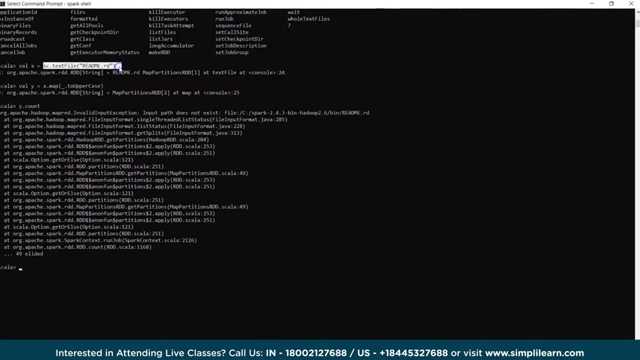 exist. it is not able to find a file in this location. so this clearly explains that there was no evaluation happening when we did this, when we tried to read a file, and neither when we did a map transformation only and only when we invoked an action it tried to search for. 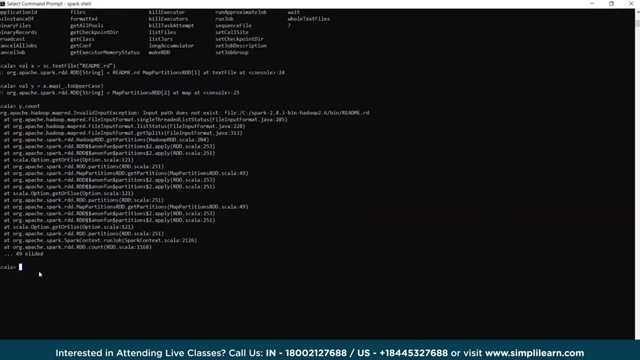 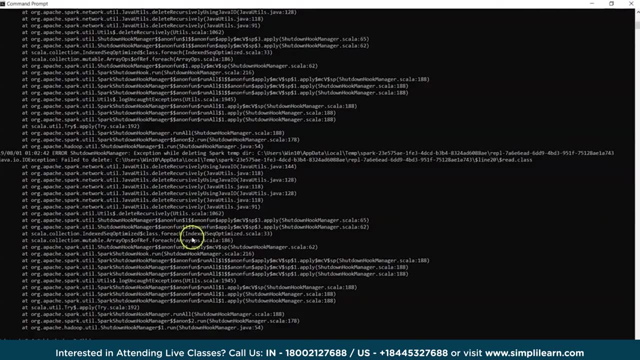 file in this location. so let's quit this and check if the file exists. to quit, you can just do a ctrl d or you could do a colon: quit now here if you see some messages like this which says unable to delete temporary file. so that's a known issue. 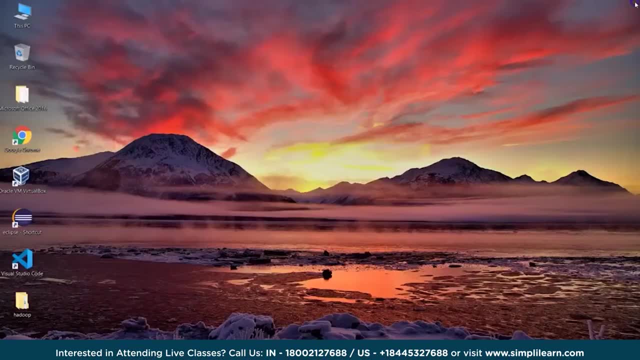 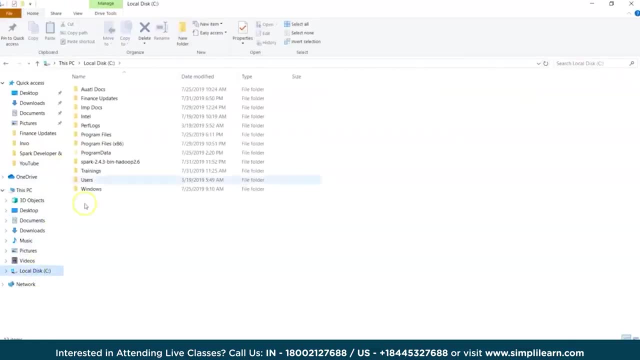 we can fix that, but my spark is working fine. now let's go and check if the file exists. so i will go in here and then i will look in my spark directory to see if the file exists. so this is the file: readme dot md. however, i had done readme dot. 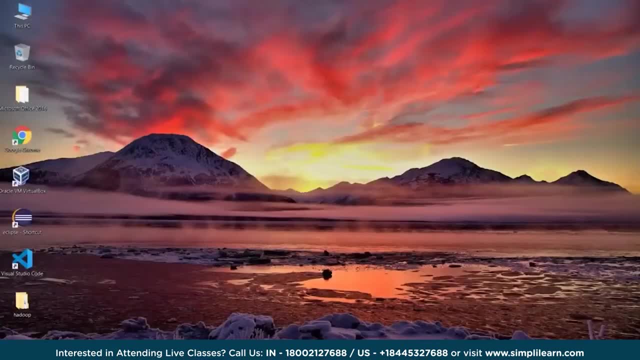 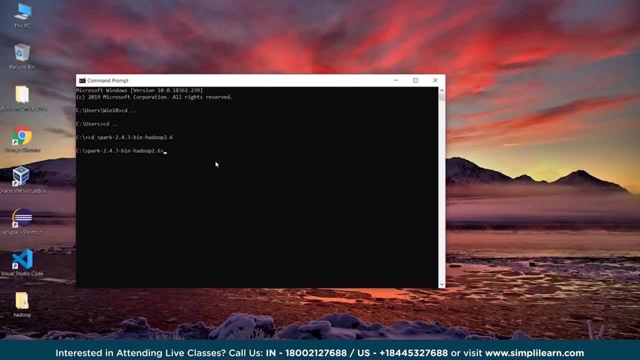 rd. so let's do it again and let's test if our spark shell works fine, so we can go into the spark directory by just doing this, and then either i could be going into bin directory and then start spark shell, or some people prefer to do it this way, wherein you: 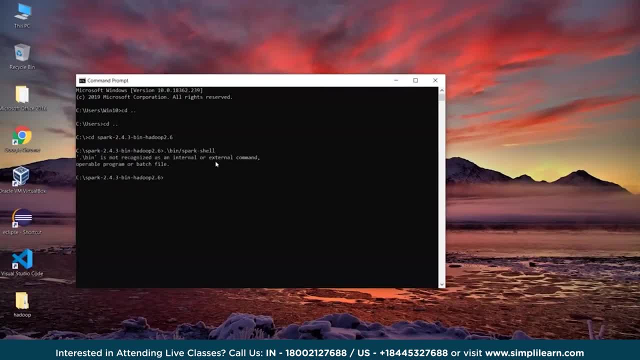 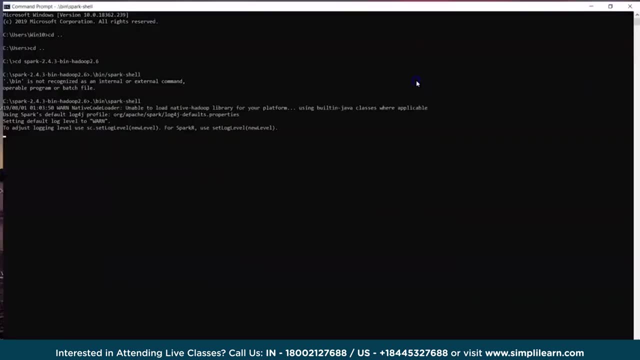 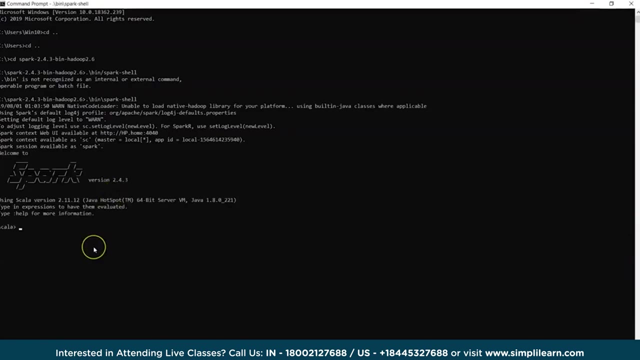 can say bin spark shell, and that should start your spark shell, but there was a error in the slash, so let's do it this way and this will start your spark shell- an interactive way of working with your spark and using spark context or spark. now, once we have 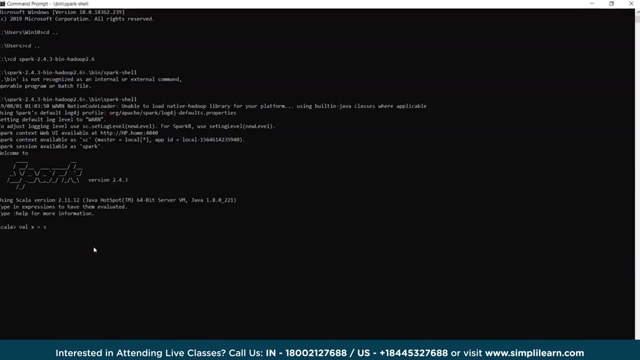 done this. i can again say val x and i can say sc, which is spark context, which is already initialized when you start your spark shell. i can say text file, and i would want to read a file which is readme dot md. now we know that this file exists. however, 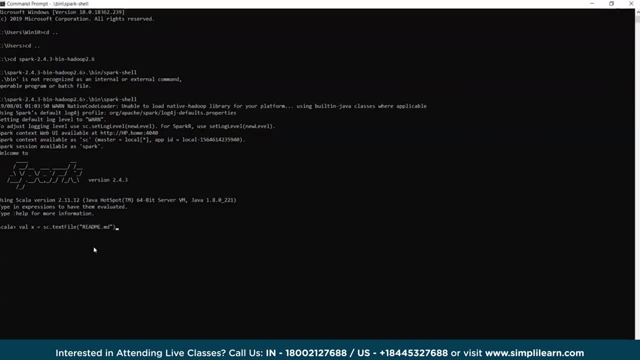 the checking of the file existing or not. that means an evaluation does not happen when you do a transformation or when you use a method of spark context. it just creates an rdd. click on this and this has created an rdd of string. now we can do. 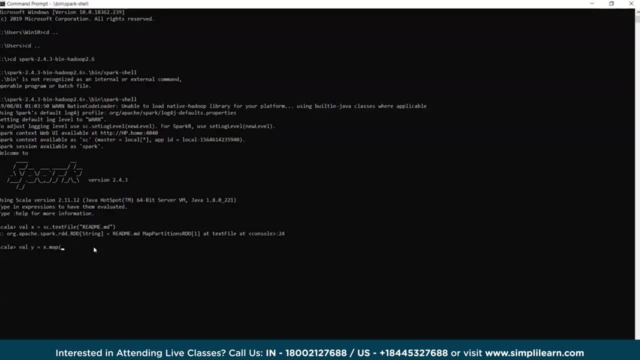 further transformation on x by saying map, and then i can say: i would want to convert the content into upper case, and that's also done. now, finally, let's invoke an action which will trigger the execution of my tag which contains these rdds. so i could just say y and i could say 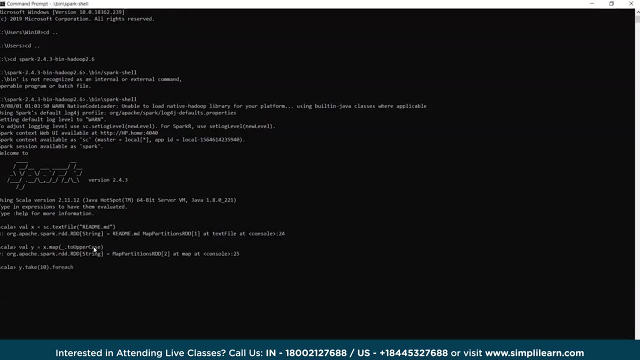 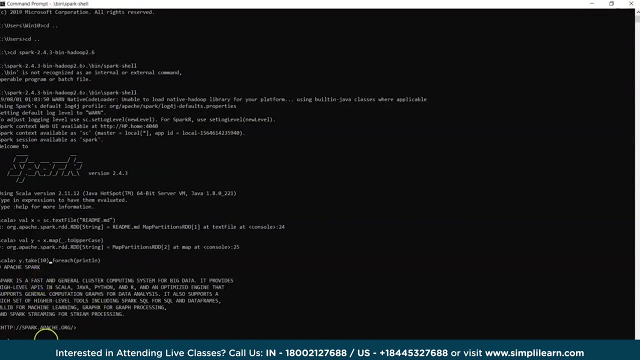 take 10 and i could say, for each print, ln, and this should be able to invoke an action and it shows me the result from the file which is converted into upper case. remember, if i do a y dot count, which is another action, it will trigger the execution of tag right. 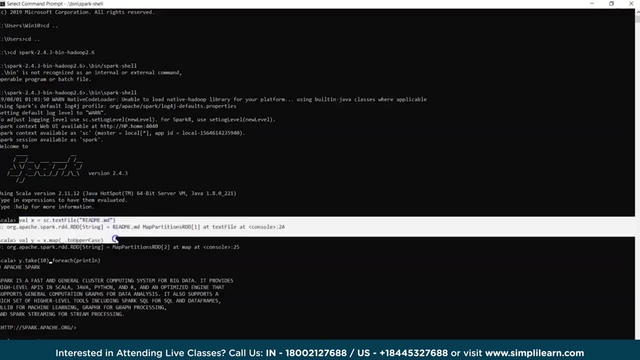 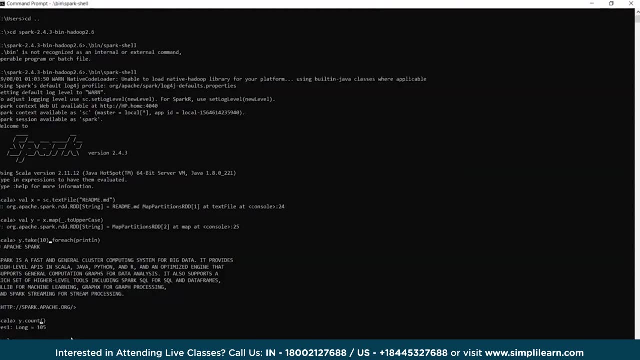 from the beginning, where the first rdd was created. the transformation will be done and then it will show me the count of lines which exist as a result of this. so we can do this, and this says me that there are 105 lines. this is a simple example of 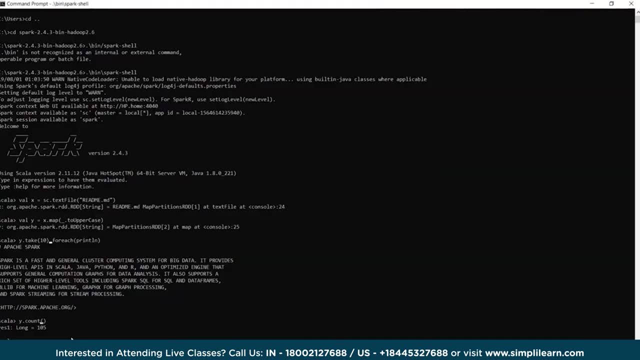 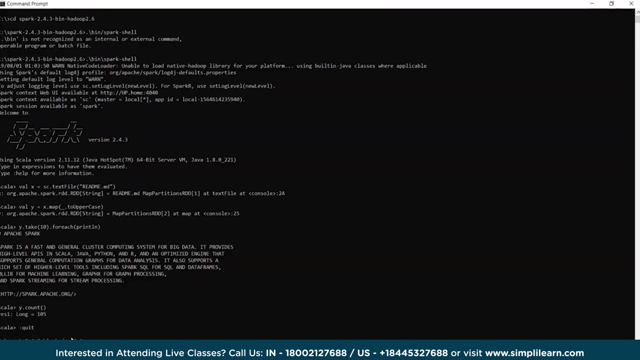 using spark shell and using spark in an interactive way on your windows machine. now to quit, we can always do a colon quit or we could do a control d and that basically takes you out of your spark shell. similarly, we can work on py spark by just saying dot slash. 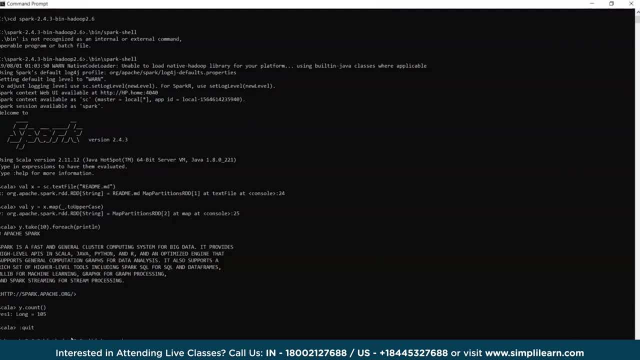 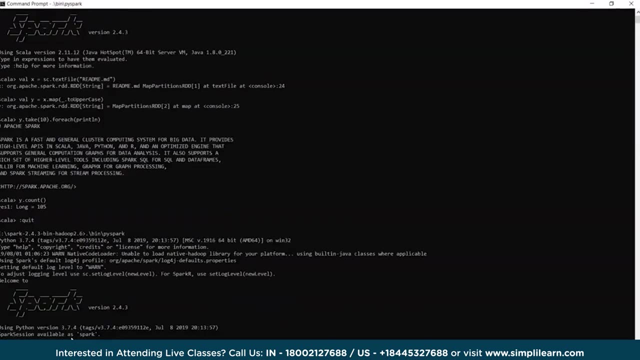 bin slash, py, spark, and that's python's way of working with spark, which brings your python shell. it starts the spark context which is available as sc, and if you are interested in working on data frames or data sets using spark sql, then we would be using spark. now, here i can. 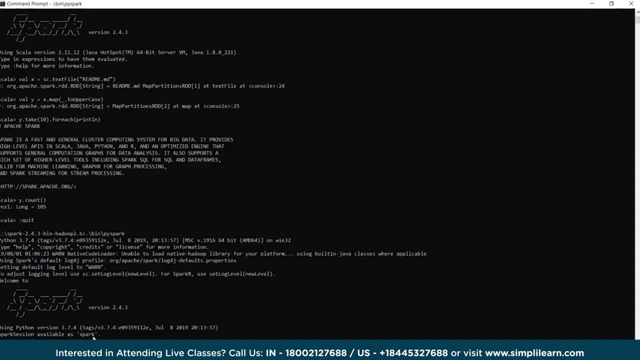 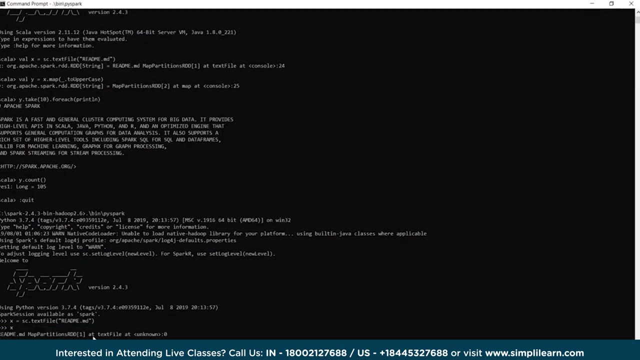 just declare a variable x and i can just do sc dot text file, like what we did using scala. we can be referring to the same file, readme dot md- and this has created an rdd. you can just type in x and that shows the rdd which. 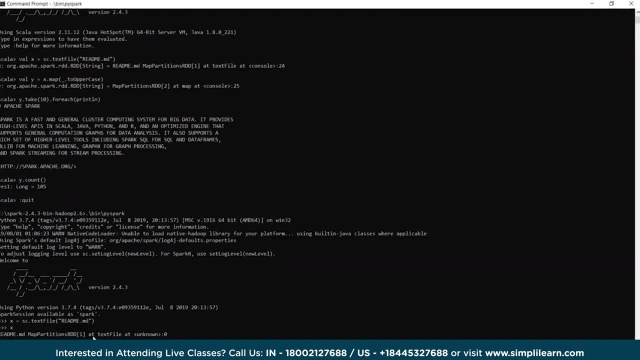 was created. you can then further do some transformation on it using x dot map, and then i could say: i would want to convert this to uppercase. now, in case of python, you would normally use lambda if you would want to do any kind of transformation. so i would say lambda x. 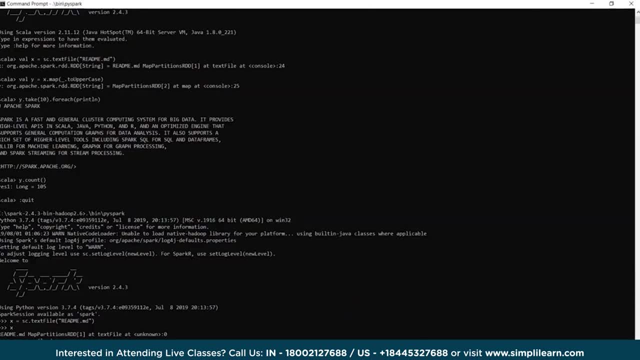 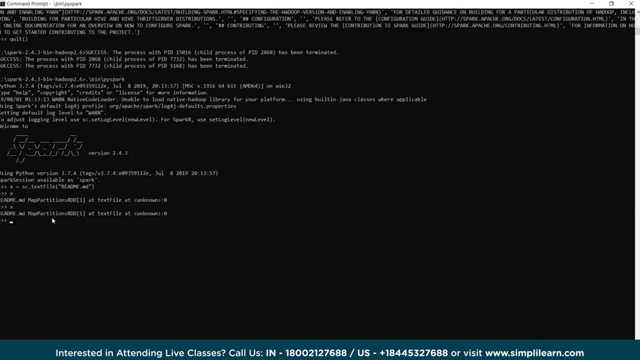 and then i would want to convert this to uppercase, so here we can check if my rdd was correctly created and, as i was saying, we can then do some transformation on it. so i can say again: y equals. and then i would want to do some transformation on x. 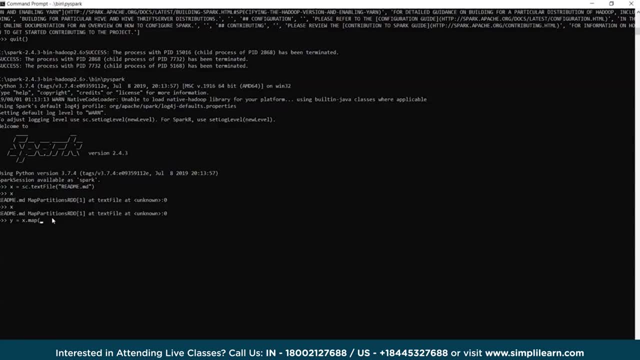 i would say x dot map. so in case of python, as i explained, whenever we want to use an anonymous function or we want to do some transformation, then we can pass in the function to the transformation. so here i can say lambda and then i can just say line or 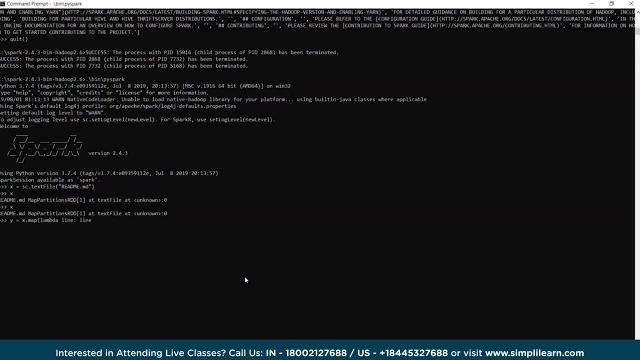 i could say x or a, whatever that is, and i could say line. i would use a inbuilt function that is upper, which should convert the content of x to uppercase. now, remember, we are just doing some transformations here, so if i click on y again and enter, 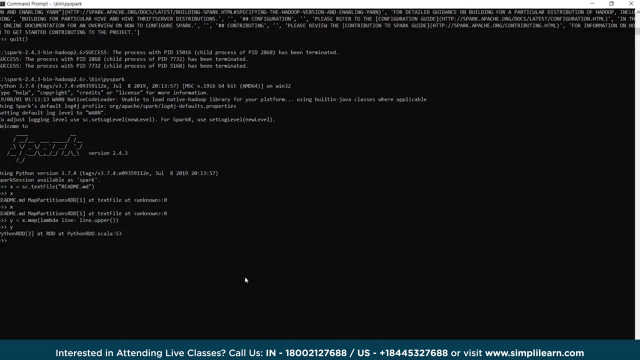 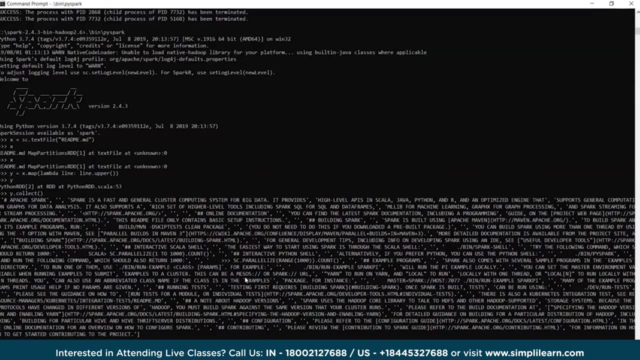 sorry, if i enter y, it will show me that that has created an rdd. to see the content, i can just say y, dot collect, and that should show me the content of first few lines which is converted in uppercase. so this clearly shows that we can even use python. 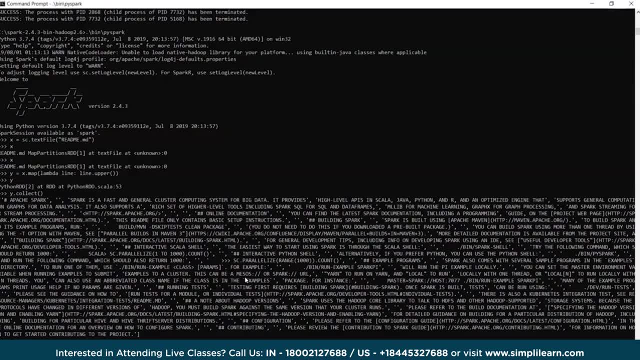 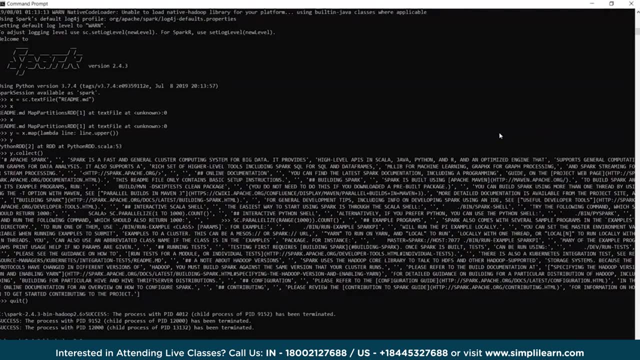 to work with spark by using py spark. now to quit this, we can just say quit and that should take you out of your py spark shell. so this is how you work on spark shell or py spark on your windows machine. so this has a local spark setting. 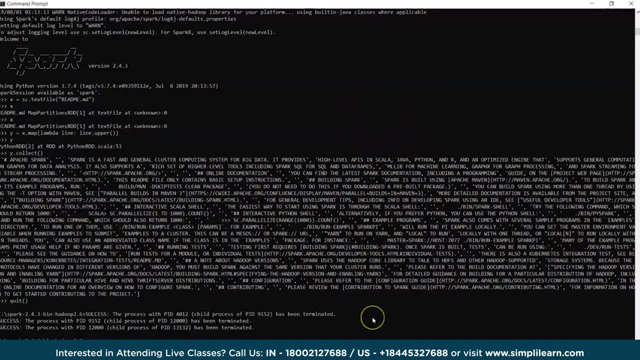 setup, or basically spark running in a local mode and you could be using the interactive way of working with spark. now, if we have packaged our application in a jar file, then i could be using spark submit to submit my application. how do we do that for this we? 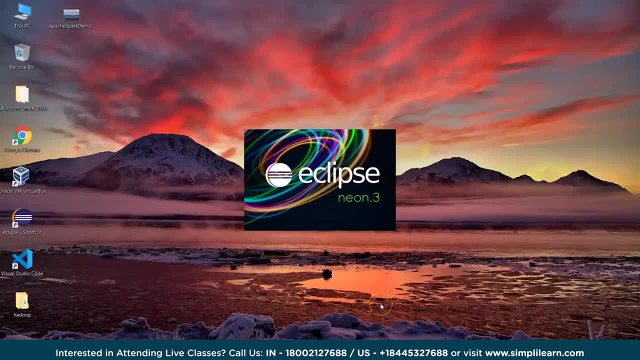 can basically bring up one of our ids. so in my case, i'm using eclipse and i can get into my eclipse. now there are two options here. one: we can be writing code in your ide. that is eclipse. we can be compiling the code based on the spark related. 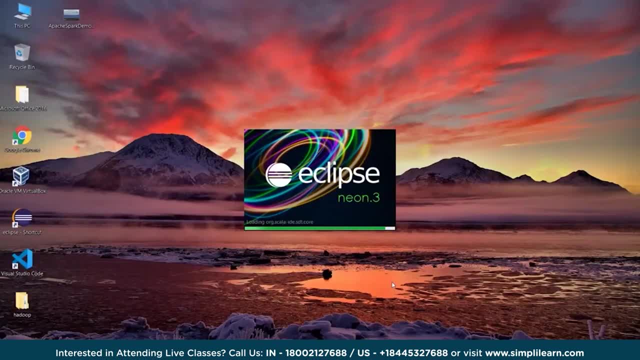 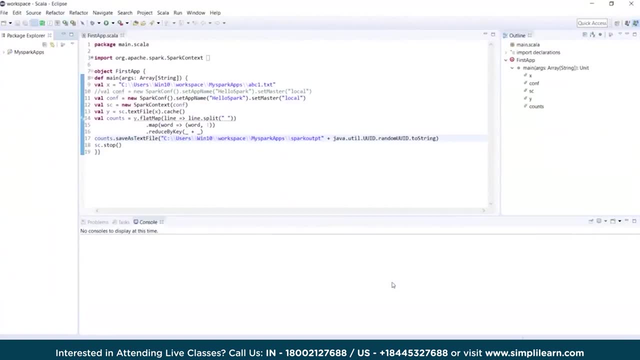 jars and then we can run our application from ide, which would interact with your spark. that's one way. the second way is we can use packaging tools like sbt to package our application as jar and then push the jar to your local spark or a hadoop based spark and then 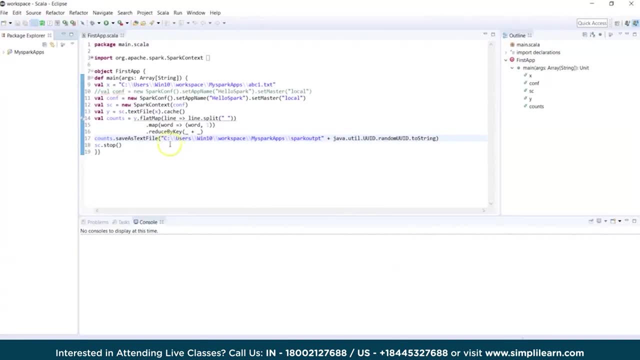 run it using spark submit. now this is a simple sample application for which i have set up certain things here. the first thing is, when you have downloaded eclipse for all the people who are new, they might have to add the scala plugin now if you see here in my eclipse it. 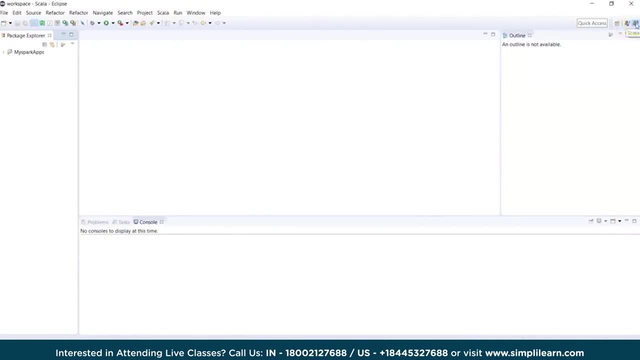 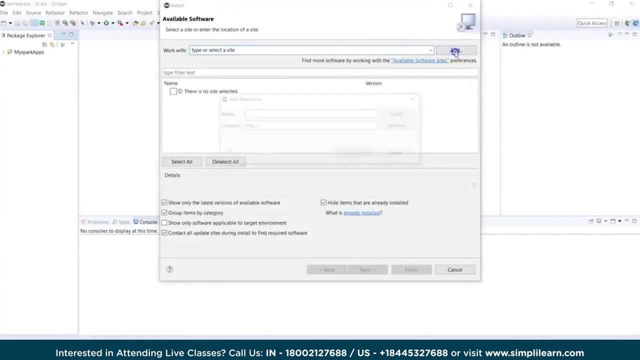 shows up java perspective and it shows scala perspective. now, how did i get this? you can click on help and you can say install new software and here you can say add, you can say scala ide, and then you will have to give a link from where you can get the. 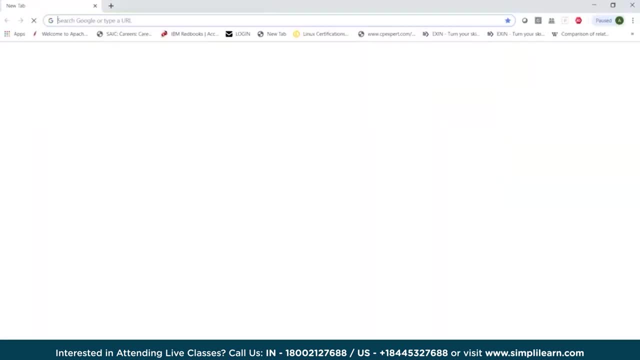 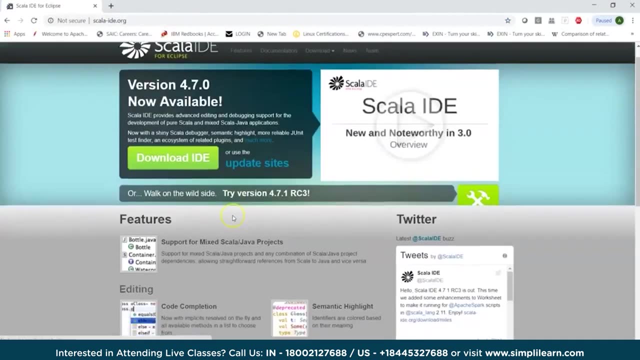 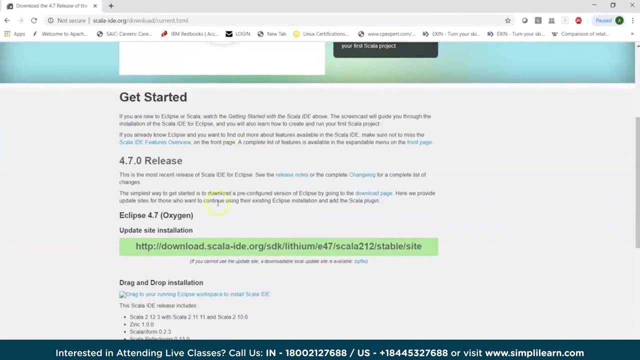 scala ide. how do i get that? so i can go to my browser and i can say scala ide dot org. and once you go to this link, just scroll down, click on stable and that shows you different releases for your different ides. now for eclipse. although this shows, 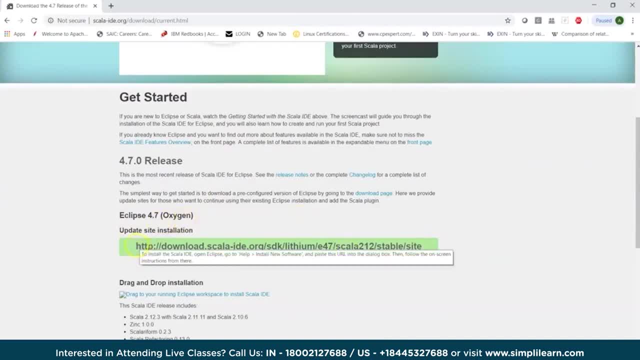 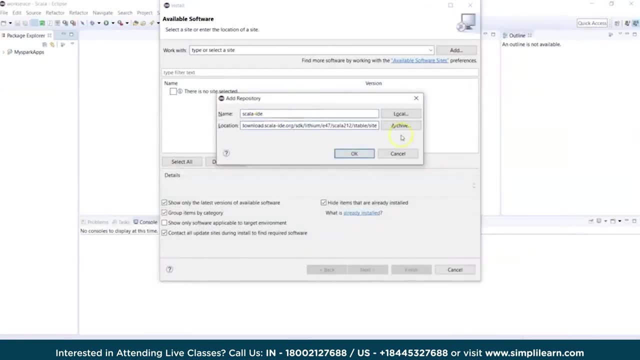 for oxygen and i have eclipse neon. but that works fine. you can just copy this link and here, once you have copied the link, give the location here and you can say: okay, now, once you do that, it shows you different options from where you can choose scala ide for eclipse. now, in my case, 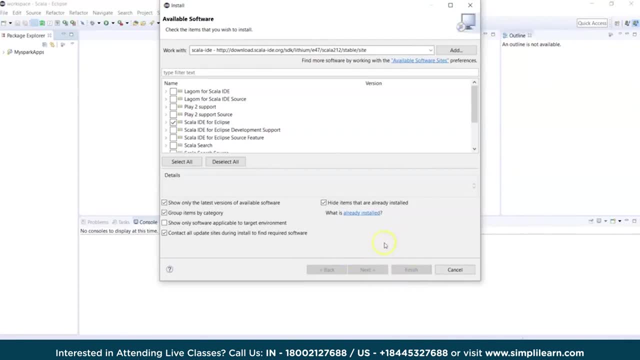 it is already installed, so these options don't show up. however, if you do not have this option, for example, let's choose something else. say, i will say scala search, and once i do this, next gets activated. so scala ide is already installed in my case, so i can. 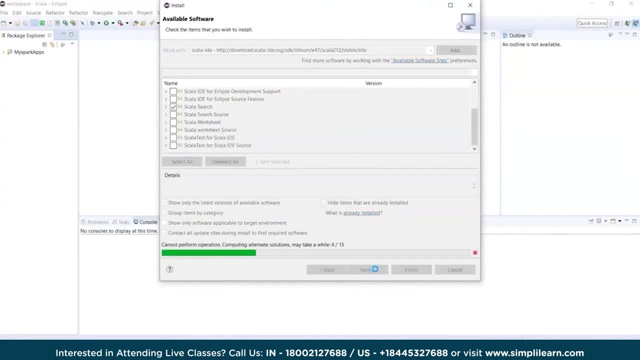 click on next and this should basically get scala search plugin also, which can be added to my eclipse. now, once this is done, you will be prompted to restart your eclipse and then you should have your scala perspective. so for now i'll just cancel this, because i already 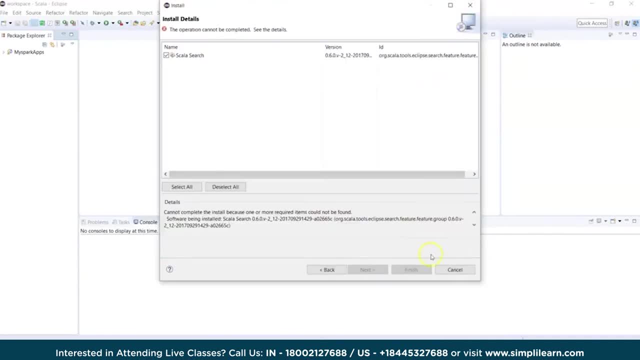 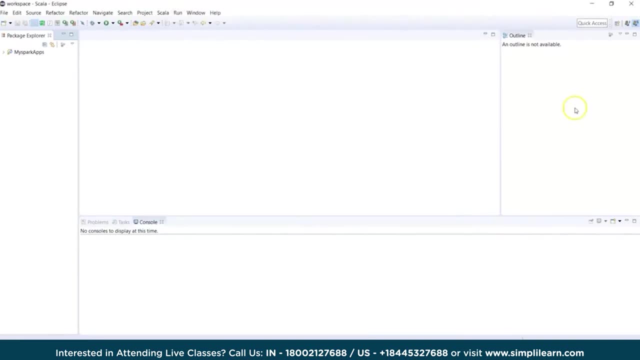 have my scala ide dot eclipse. so this is done. i'll just do a cancel here now. once you have your scala ide or scala plugin added to your ide, you can always click on this icon. here and here you can just click. double click on scala, that will open up. 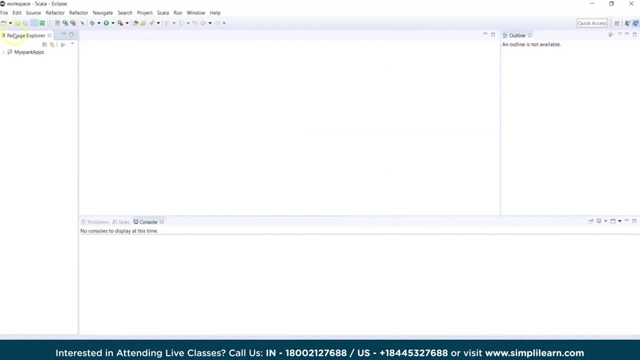 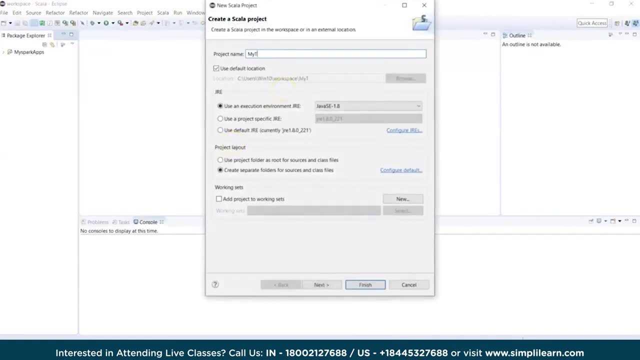 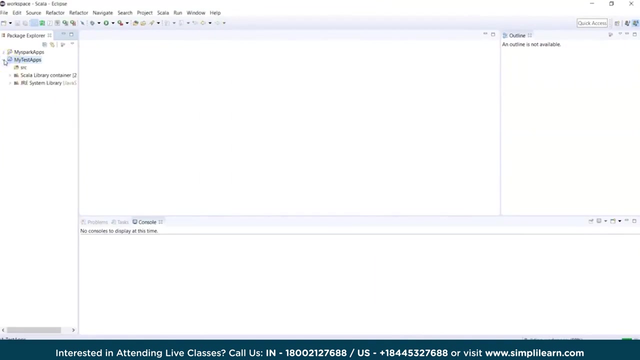 scala perspective. so that's the first thing. then you can always click on file new and create a scala project. for example, i could say my test apps and then i can just say finish, so it has added a project. now what we need to do is we need 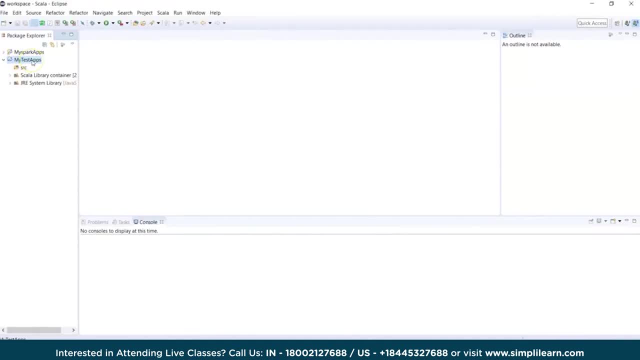 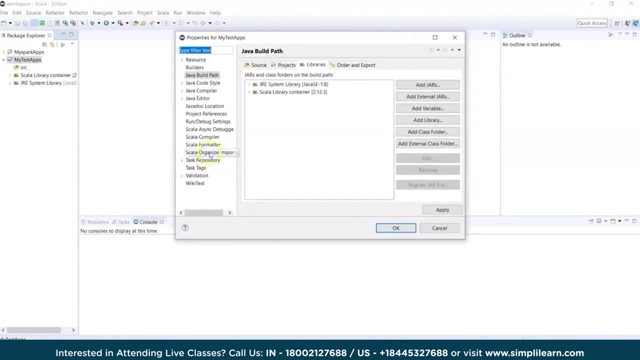 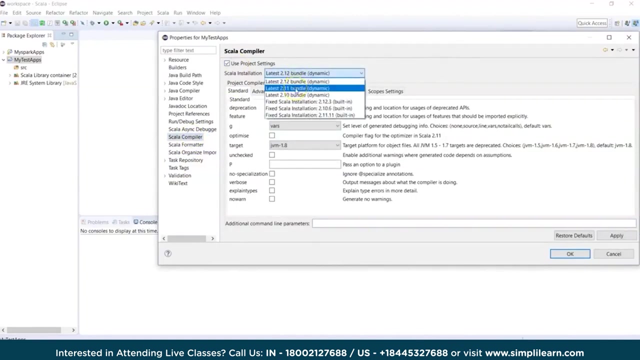 to make sure that our setup is fine. so first thing i would suggest is click on this, go to your build path and here click on configure build path. so where it says scala compiler, it would be good to choose for your project settings. instead of 2.12, go for 2.11. 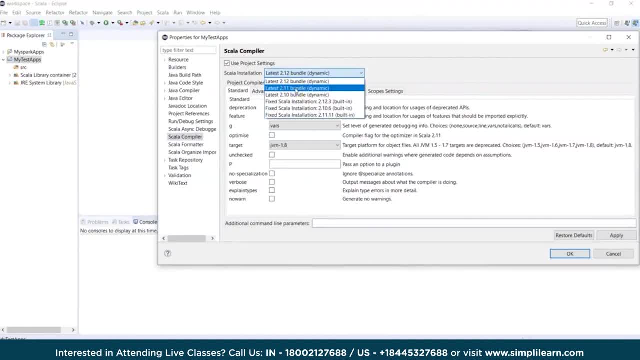 so sometimes you might have problems with scala 2.12, which might not be able to compile for your scala 2.11. so use latest 2.11 bundle and then you can say apply. it says compiler settings have changed. a full rebuild is required for changes to take effect. 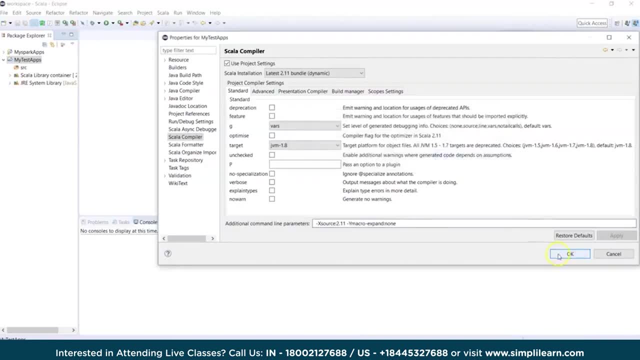 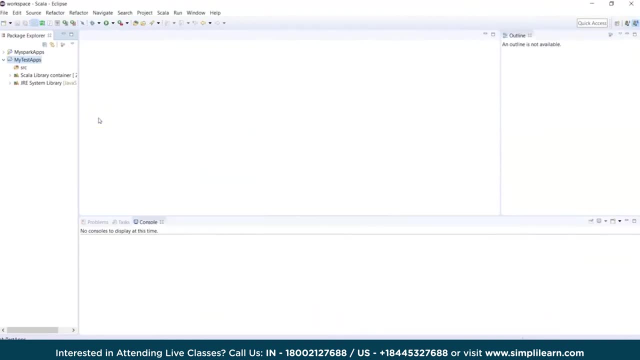 shall all projects be clean? now we can say ok and we can say ok. so this will build your workspace to use scala 2.11 bundle now, once that is done, second thing what we need is: we would want to write our code and we would want our 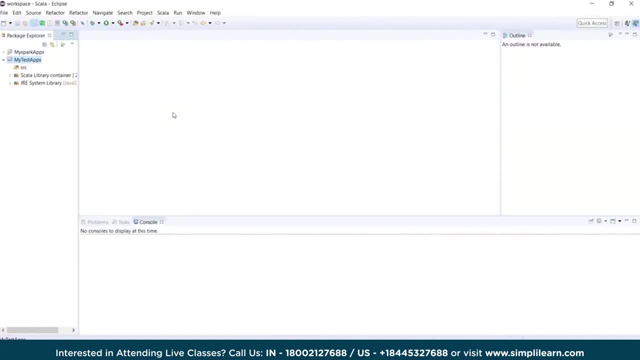 code to compile for that. as i said, if we want to write our code using an ide and then run it from our ide rather than using a build tool like maven or svt, i can just add the spark related jars to my build path, so i can right click. 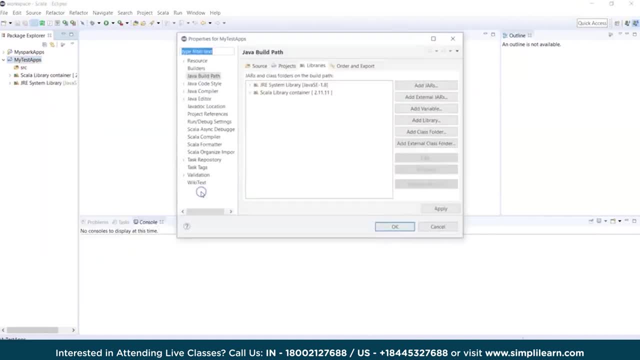 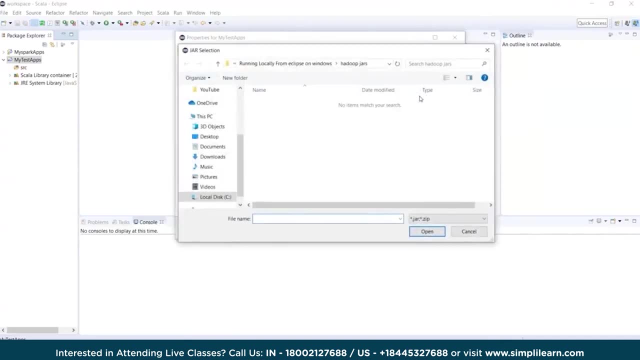 here i can say build path and i can click on configure build path. and here, where it says libraries, i can say add external jars. now this needs my spark related jars. now where do i find it? so remember, we have downloaded spark, so you can even find it there. so 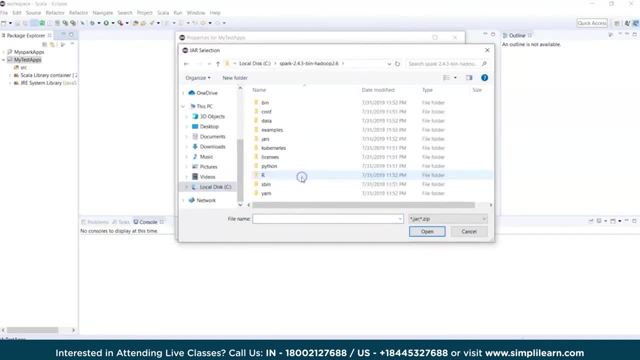 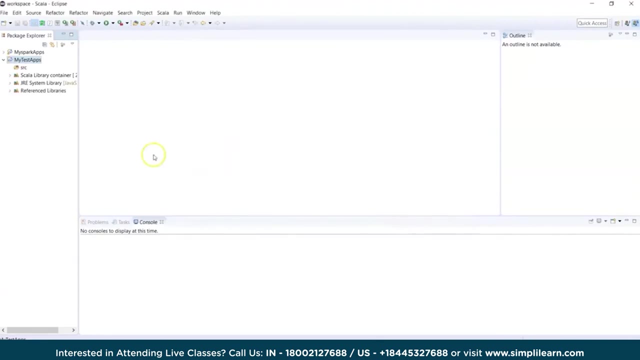 you can click on wherever your spark is and then you can click for jars, which shows you all spark related jars. you can just do a control a and just add it to your build path, say apply, and then just say ok. so once this is done, you have already added the. 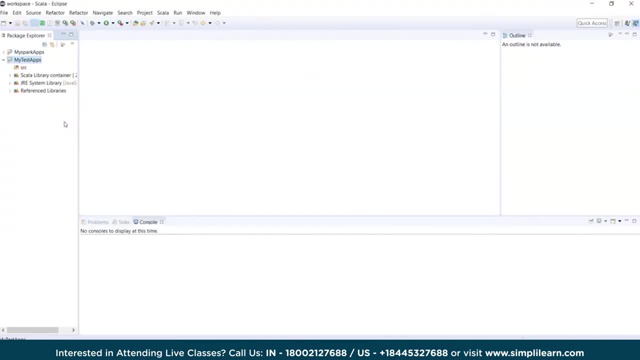 spark related jars, which might be good enough for you to write an application. once this is done, we need to basically go ahead and write our code. now, how do i do that? i can just click on source and i can say new and then i can say package. 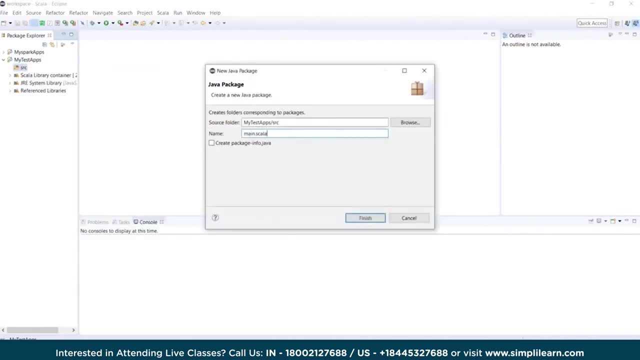 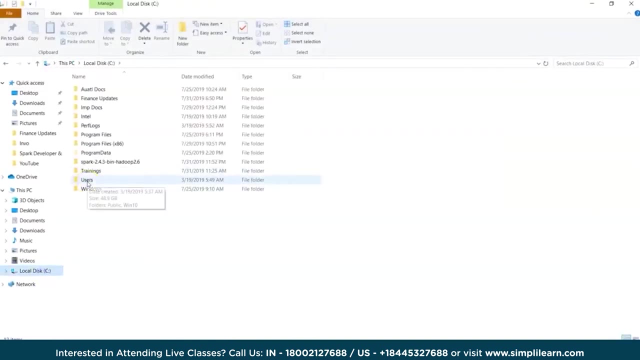 and here you can say main dot scala. click on finish and that has created main dot scala. so that would be source slash- main slash scala in the folders. we can always check that. so i can go to c drive. i can look in users, win 10 and then look in my workspace. 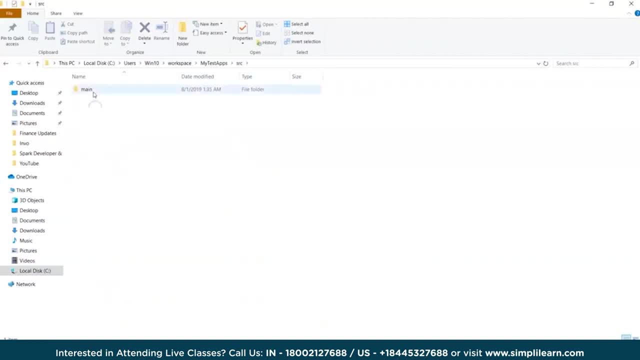 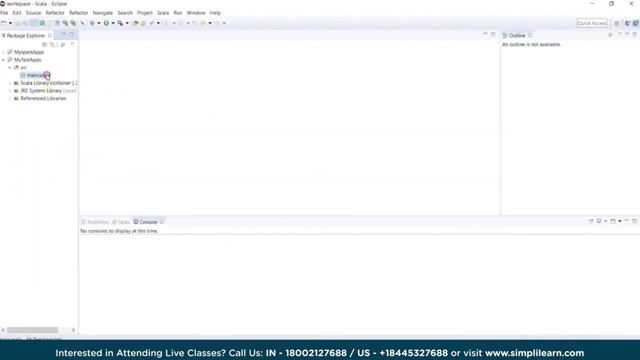 for my project and if you see, in source we have main and we have scala. now this is where we will be writing our code. so for this then i can just right click and i can say new and i can just create an object and i can give it a name, so we can say test. 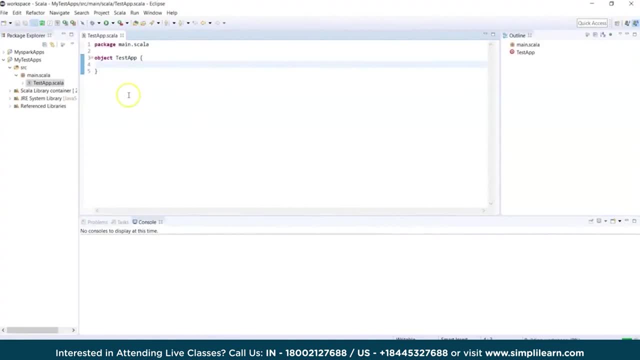 app and then we can say finish. so in case of scala and spark, we need to create an object and then we need to define main class here. once that is done, we also need to import some packages and we need to initialize the spark context. now for that you. 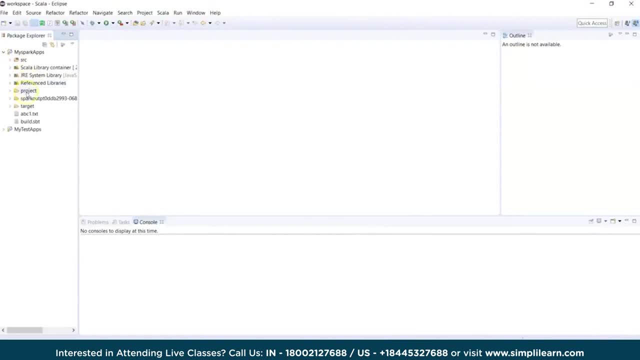 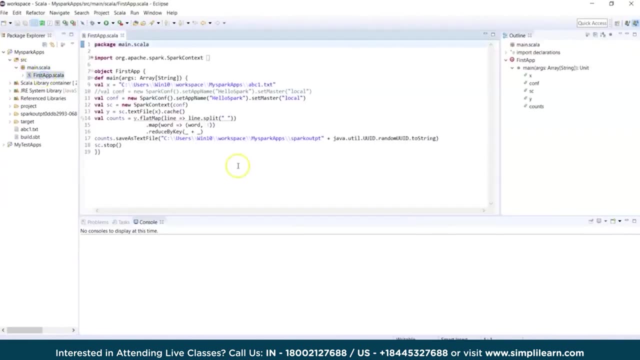 can take an example here. so i have already written the code and i can look in source main scala and i have created an app called first app dot scala. now here we have the package name. we are importing some packages which are required for us to initialize spark. 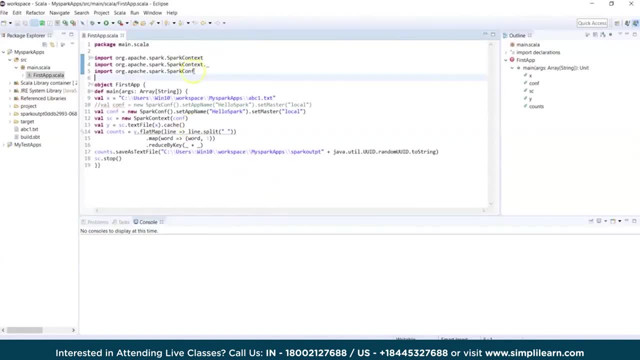 context and spark configuration. so it is spark context, spark conf, and here is my object. and for a particular project, at least one of your object or one of your application needs to be the main. so we define the main here by saying def main, args and array of string. then 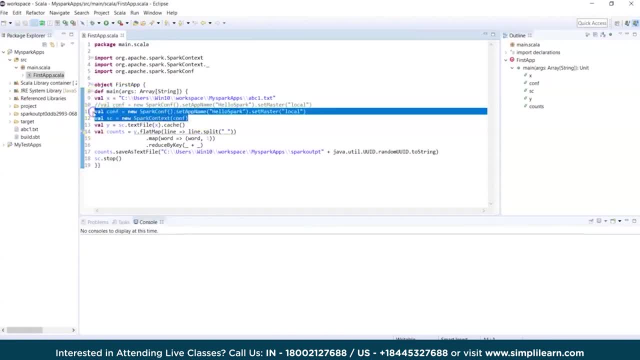 we need to basically define our spark context. so i am creating a configuration object here and then i say new spark conf. i am setting my application name to hello spark and then- this is very important if you intend to run your spark application either using spark- submit or. 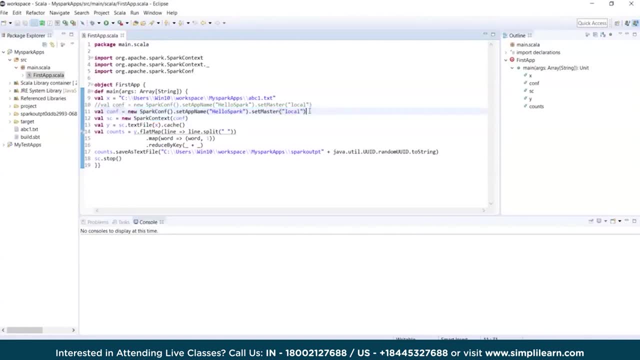 from your id, you need to specify your master as local. now that could be given with one thread or multiple threads. so this is my configuration and then i initialize my spark context pointing to my configuration. so this is the most important part here. now, if you see this, 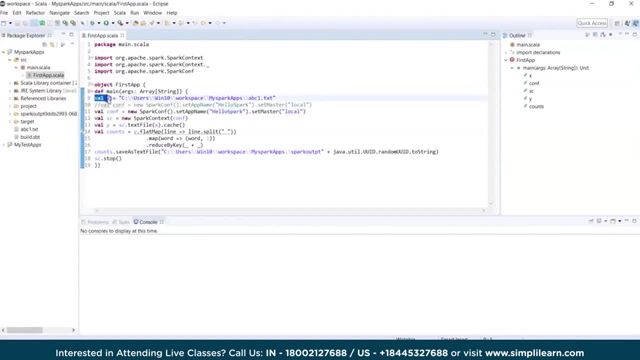 is something which i showed you in the command line. so i am doing a val x and i am pointing it to a file in my project directory which is abc1.txt. so this is just to make sure that you are giving a windows path and you are. 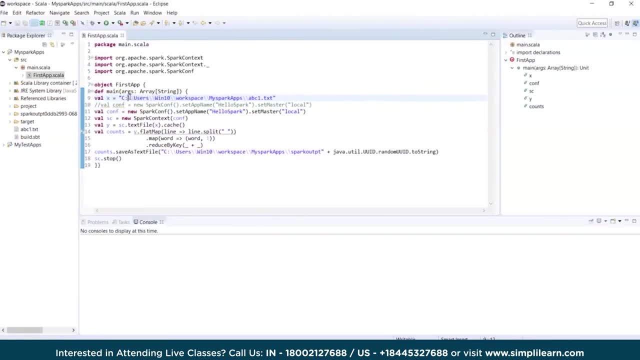 giving the right escape characters now, if it would be. if you intend to run this application on a hadoop based cluster, then you will have to give the path of the file accordingly, which we can see later. so here i have val x. i am pointing it to a file which i have created. 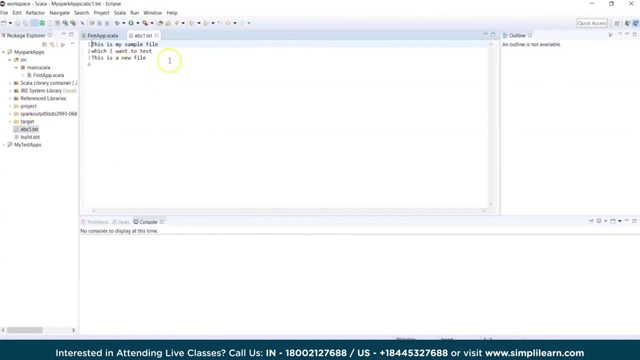 here and this just contains three lines. this is my sample file which i want to test. this is a new file. now here i have created a variable called x. further i would say val y and i would use spark context method text file, like what we did in interactive way, and i am 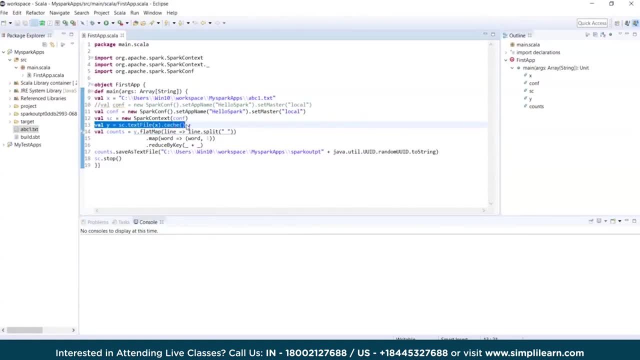 pointing it to x. i am also using some extra features like caching, so that i can cache the rdd which gets created. further, i create a variable called counts and then i do a flat map transformation on y where i would split the content based on space. i would do a map. 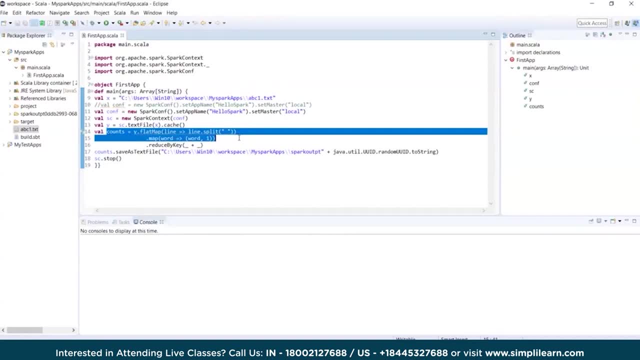 transformation, where i would get every word from the file and map it with number one, and finally, i do a reduce by key operation. once this is done, i do a saves as text file. now i could do a collect, i could do a take, i could do a count and i could also. 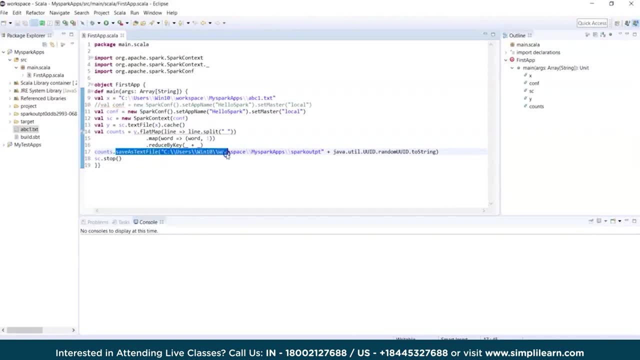 do a save as text file, where i would want my output to be saved in this location. plus, i am using a java utility to append a random number to my output directory. finally, i do a spark context top. so this is my application and if you see here my application, 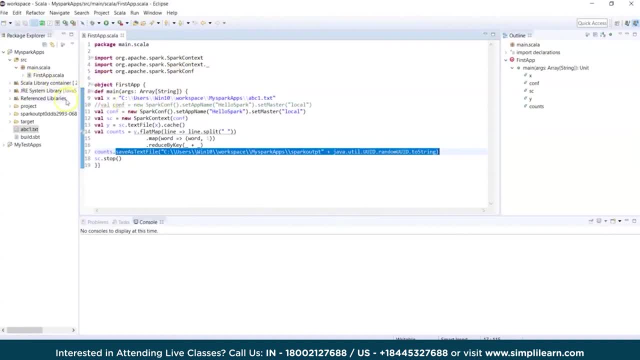 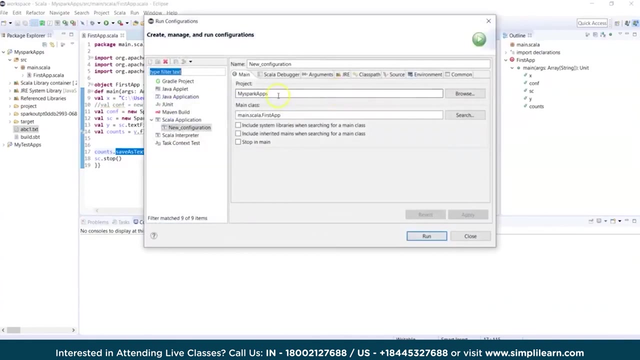 completely compiles, because i have already added the relevant jar files in the build path. now, once this application is done, we need to run this. but before doing that, we need to look into our run configurations. so you can click on run configurations, and here i am giving my project name, i am specifying 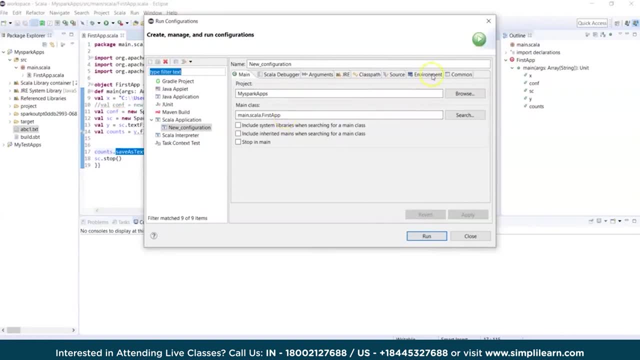 my main class, which is first app. then you can straight away go to environment, and here i am giving my project name. i have added two variables. one is spark underscore, local underscore, ip, which points to this machine's local host, and then i have said hadoop underscore. 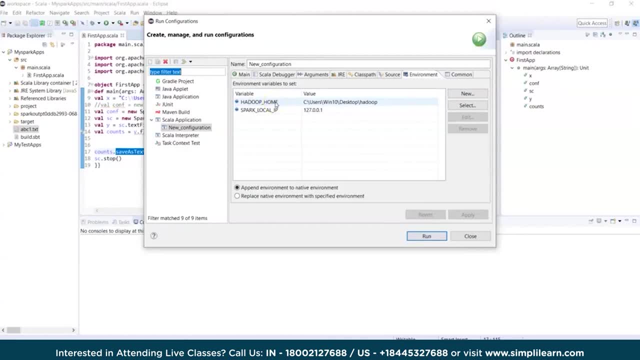 home, because spark, even when you are running locally, would want if hadoop is existing. so we can just set hadoop underscore home. and i am pointing it to my desktop hadoop directory, which contains bin folder, and that bin folder contains a winutilsexe. once this is done, we are fine and 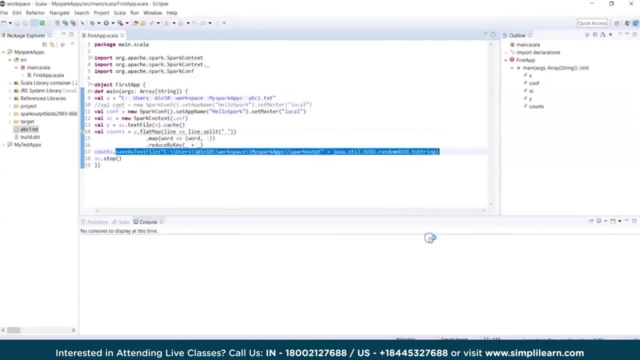 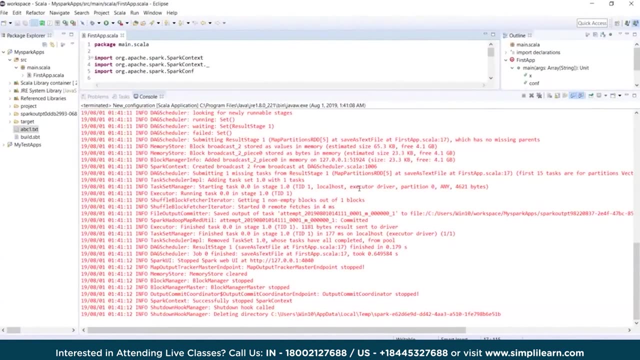 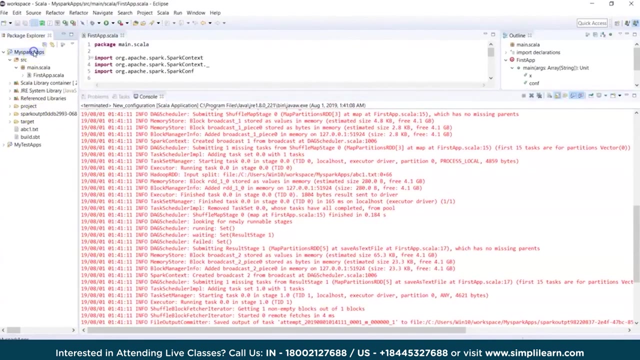 then i can test my application by just clicking on run. now this should trigger my application on my windows machine. using my ide, i didn't have to package this as jar, and here my application is completed, which should have created one additional directory here so i can click. 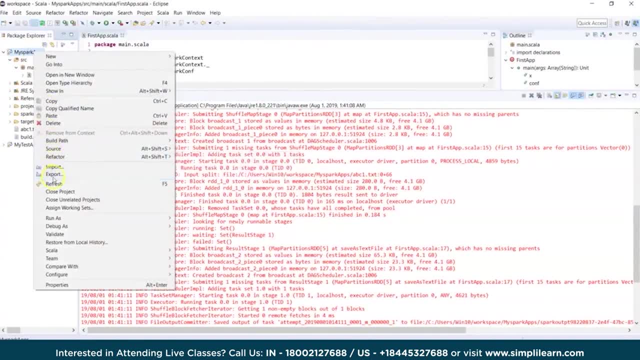 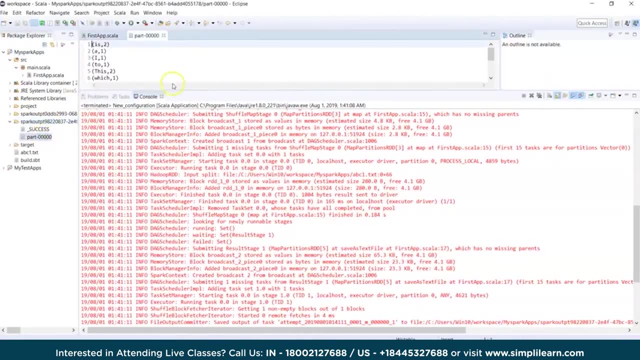 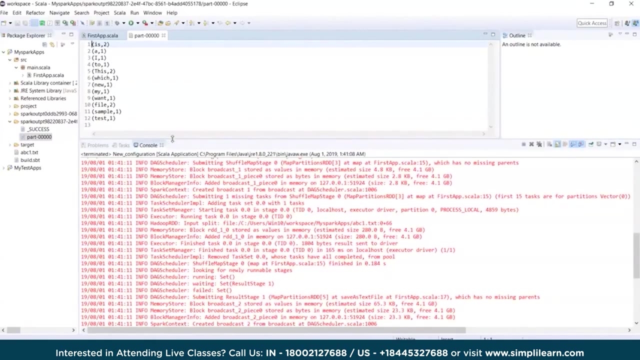 on this. i can right click and i can try doing a refresh, and here you see, a new output is created. we can look into this. it has a part file which shows my word count. so this is a simple example of setting up your ide and running your applications from. 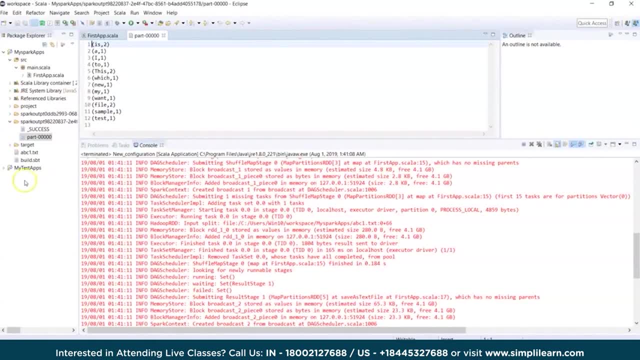 ide on a local spark. now, what you also see is a build file here. what is that for? so, in case you would want to create a project and you would want to package the application as a jar file and then run it on the cluster using spark, submit now in that case. 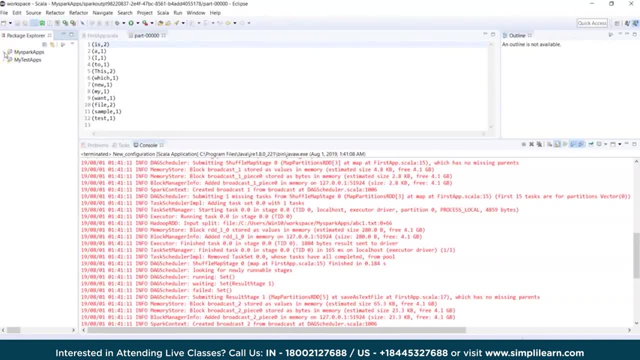 we can avoid adding the jars to my build path, but what i would need is i would need build dot sbt file within my project folder. remember, if you intend to package your application as a jar and then run it on a cluster or on a local setup. 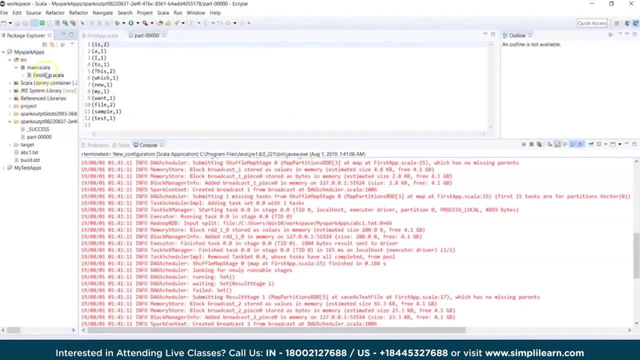 you would not need the build related jars. however, if the build related jars which are already here will not cause any harm, let them be there now. we have a build dot sbt file also, which is existing in my project folder. now, just for this run, i can in. 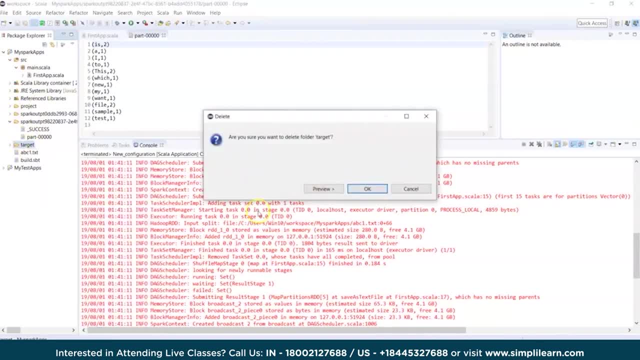 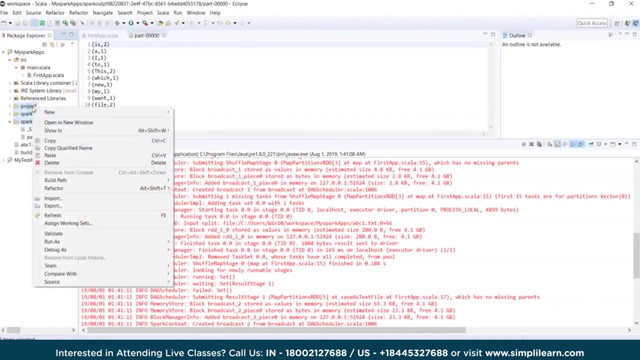 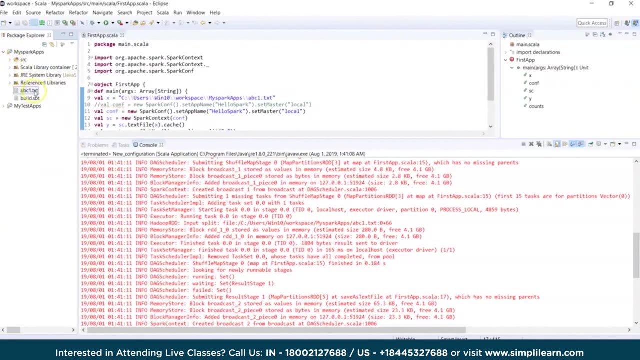 fact delete this target directory. it will be anyways recreated and, if you would want, we can also clean up these. just to avoid the confusion, i will delete these now. i just have my project folder and i have the libraries, i have abc1.txt and i have a. 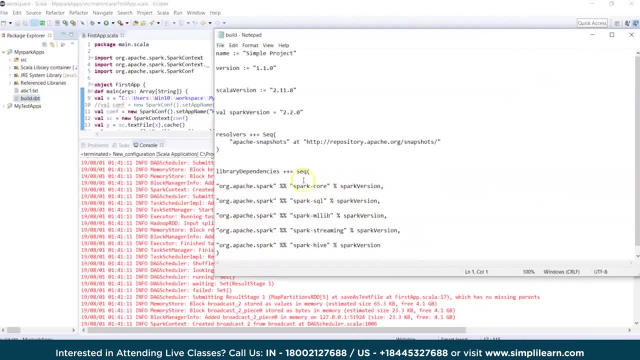 build dot sbt file. what does that contain? so this basically has a name. i am giving a version which will be appended to my jar. i am saying the scala version which i am using, which is 2.11.8, and i am saying spark version, which is: 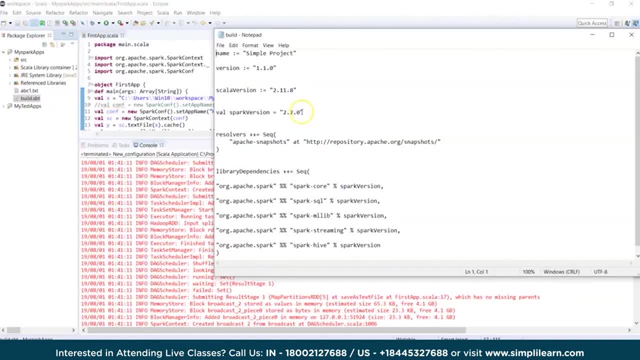 2.2.0. you can replace these with the version which you intend to use. other than that, we are pointing to the different spark components and the relevant dependency related jars which your sbt can get for you. so i have given spark core, spark sql ml. 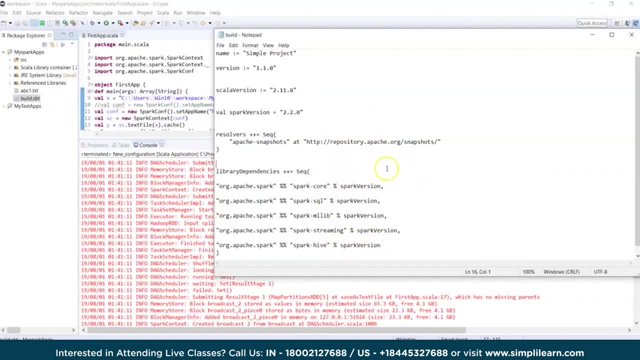 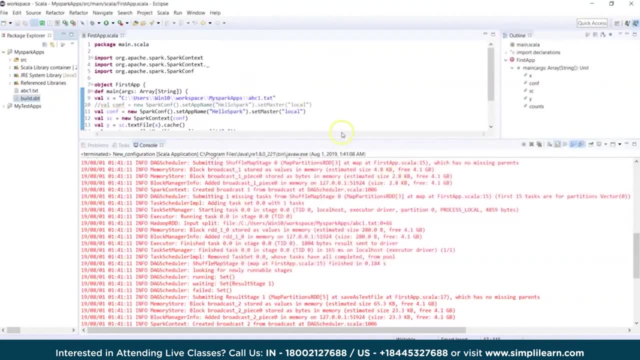 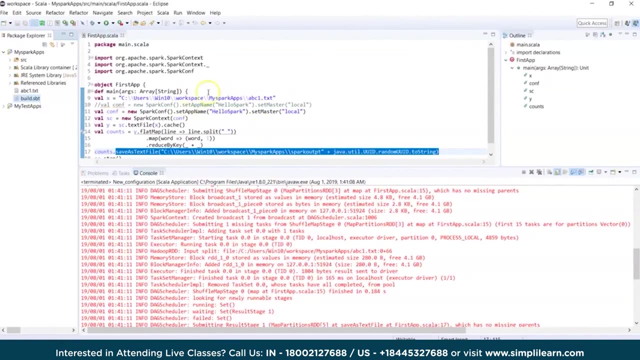 lib: spark streaming and spark hive, which will be then fetched from the repository. so this is my build dot sbt file, which exists in my project folder. we have our code written. we have our build dot sbt file, which is already existing in my project folder, my code. 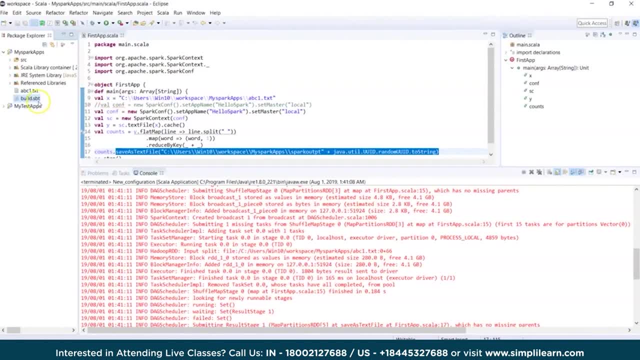 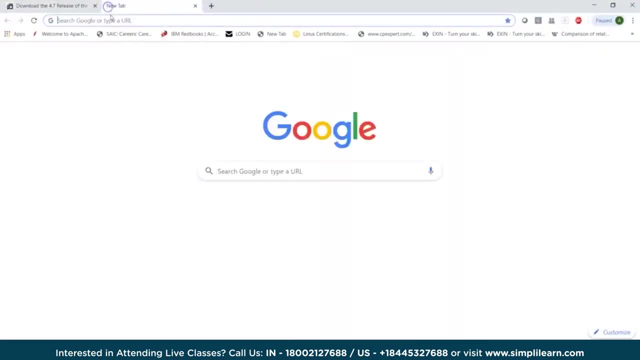 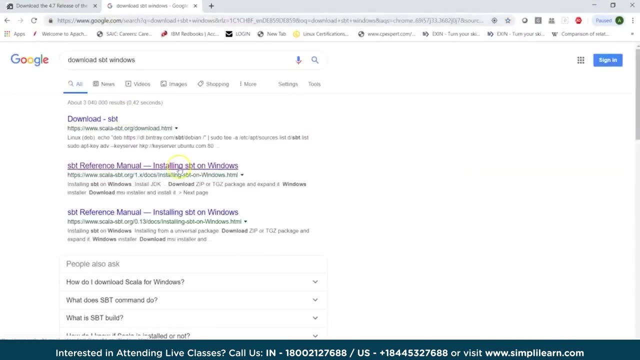 is already fine. now we need to use sbt to package my applications into jar, for which you will have to download sbt. so you can just say download sbt windows and that should take you to the installing sbt on windows page. now, here you can just download the msi installer. 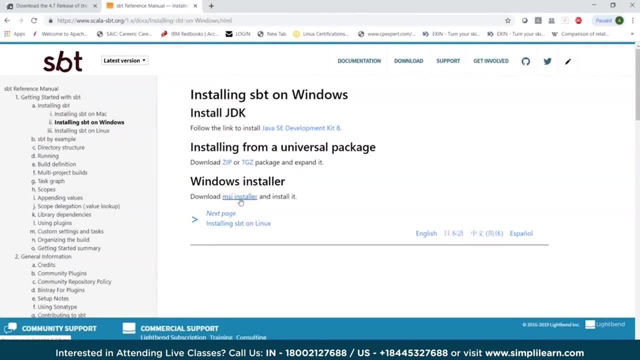 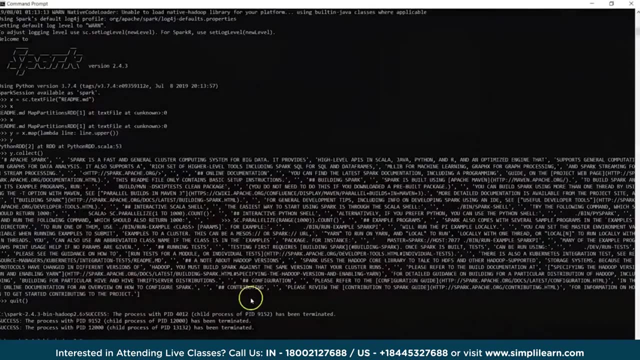 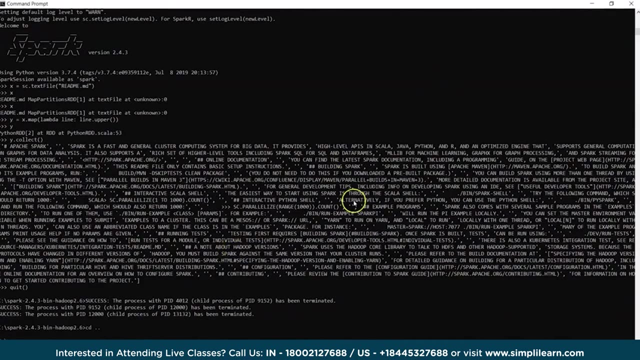 and run through the installer, which will basically install sbt on your machine. now i have already done that, so my build file is ready. my code is ready. all i need to do is now use sbt. so what i can do is from my command line: i. 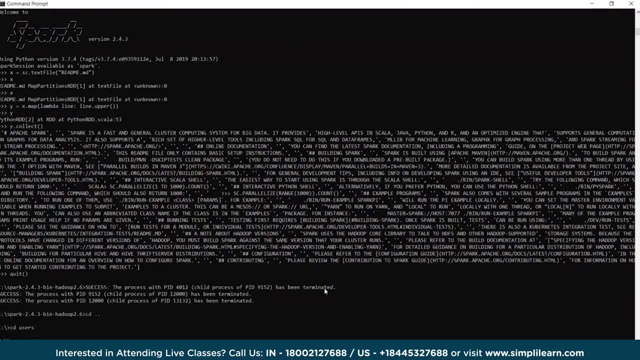 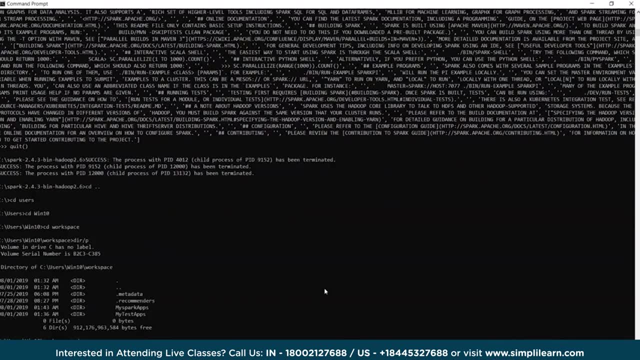 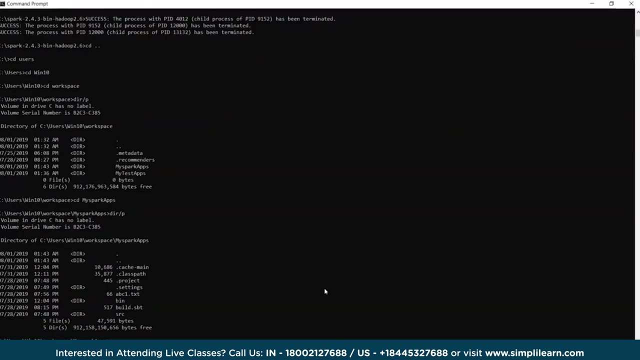 can just say cd and i will go into users, i'll go into win 10 and i'll go into my workspace now, here i can see for my projects and i can go into my spark apps. now, once i'm in my project folder, we can double check that it has a. 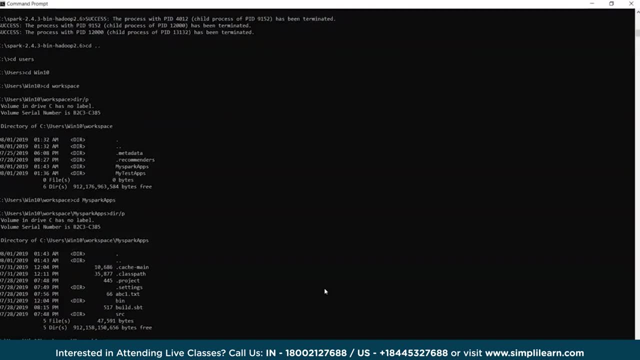 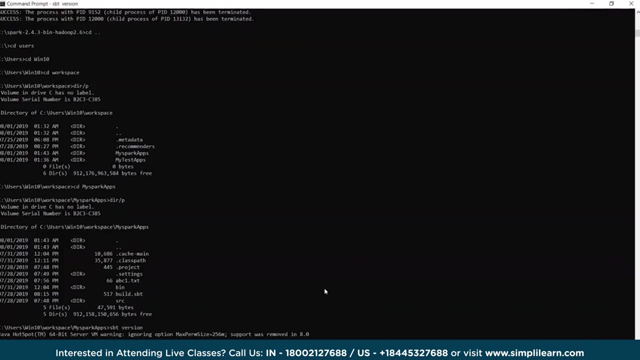 build dot sbt, which is fine. sbt is already installed on this machine and i can just say sbt. if you would want to check, you can always do sbt version to check if you have sbt. and this command is also done once you install. 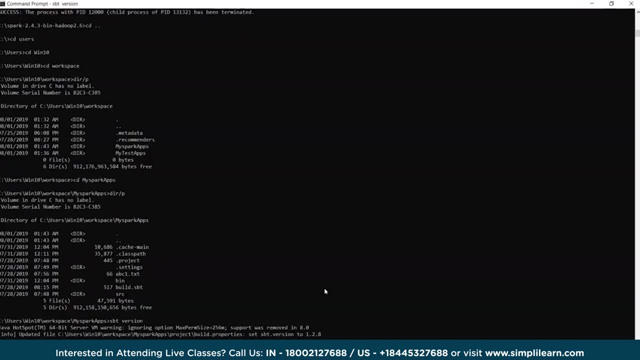 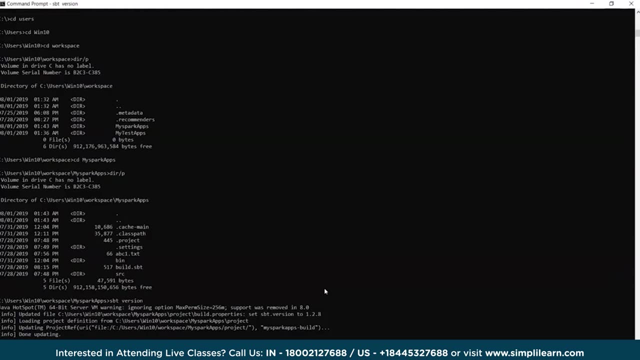 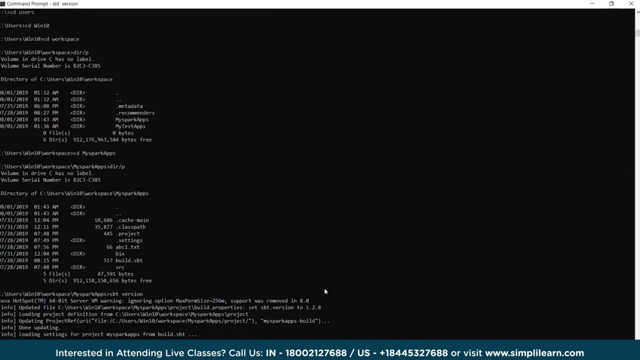 sbt for the first time. you can always do sbt version and before displaying it was displaying sbt's version. it will try to fix all your dependencies. it will try to get all the relevant dependencies. so this is just to check that sbt is installed on my machine. as i said, 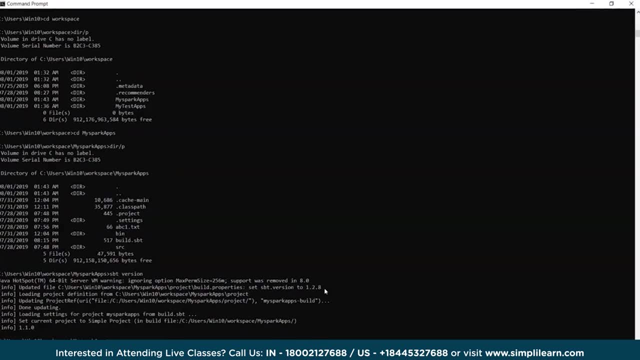 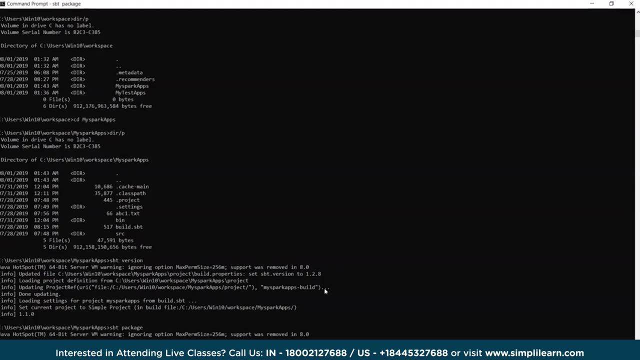 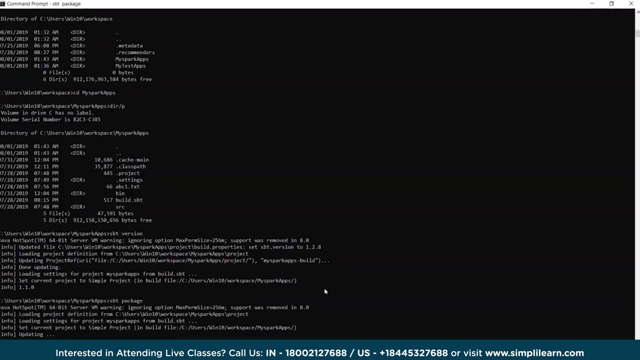 my code is already ready. i have a build dot sbt file and i can just say sbt package, which then will refer to build dot sbt, will look for your code in source main scala and then, if everything is fine, it will package it as jar. 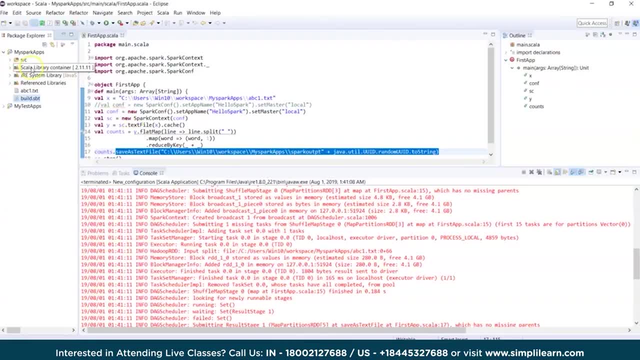 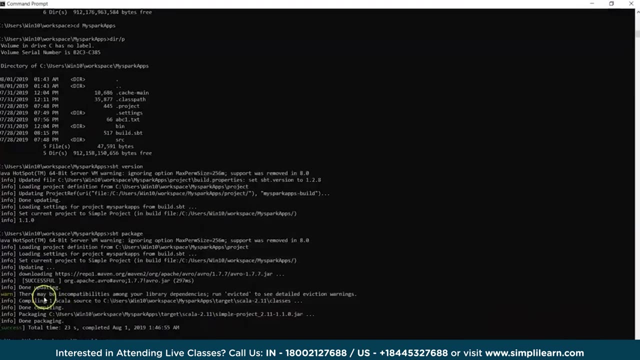 and it will create folders within your project folder. we can click on this. we can try doing a refresh to see now, if you see here the project was again created. a target folder is created within scala 2.11. i will have my jar created so we can see that. 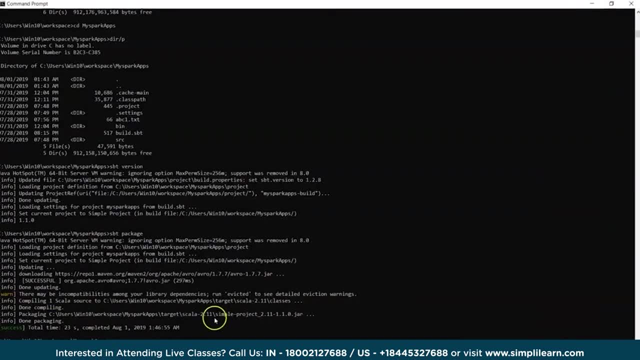 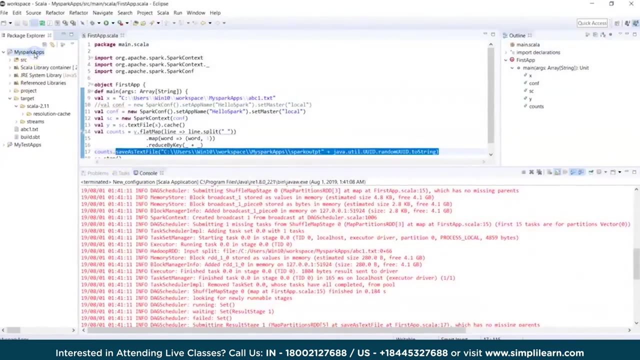 my sbt was fine. it has packaged the code and it has created a jar file as simple project 2.11-1, which can be used to run on the cluster or in a local mode. let's check in eclipse. i will click on this and 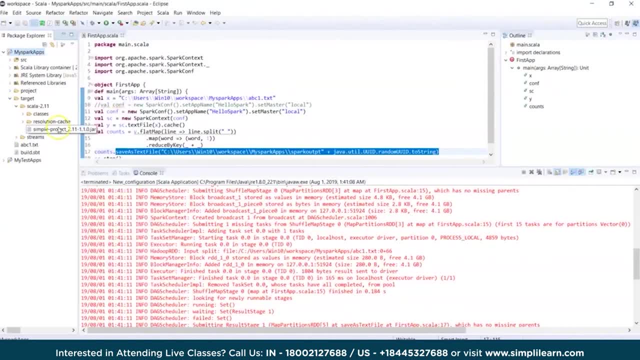 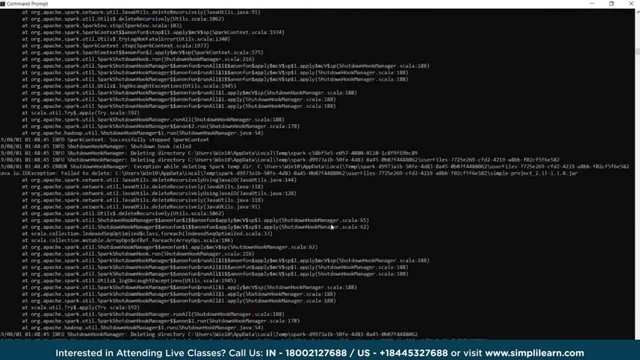 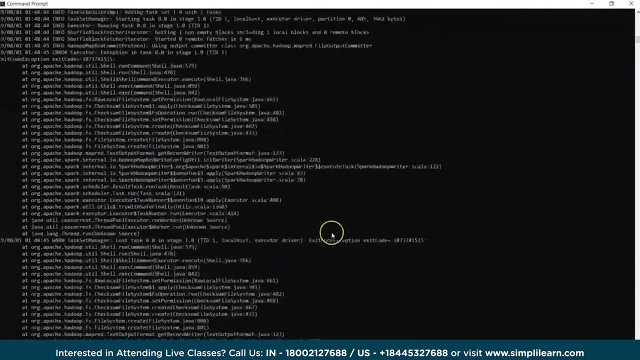 i will just do a refresh and i see my jar is already existing, which basically means then we can do a spark submit. so this is where we see that i am already running a spark submit command. now this might show up some error messages, but we can see how. 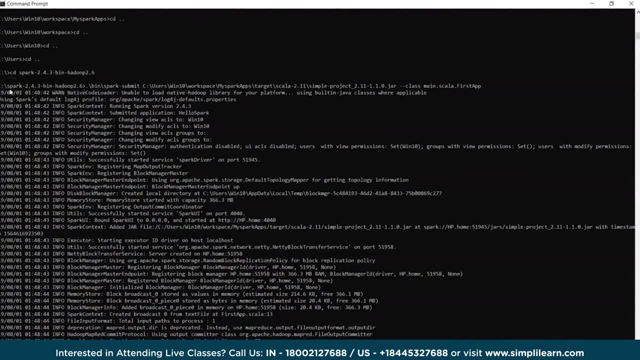 we did this. so, if you see here, once my packaging was done, i went into my spark folder, i did a bin slash, spark submit, i mentioned my jar file and then i said my class main dot, scala dot, first app. so this is my app and this is how i am using spark. 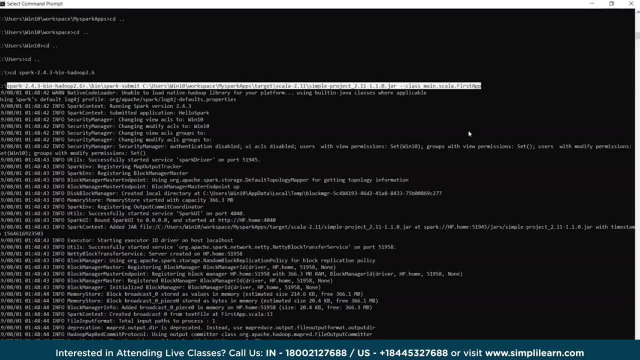 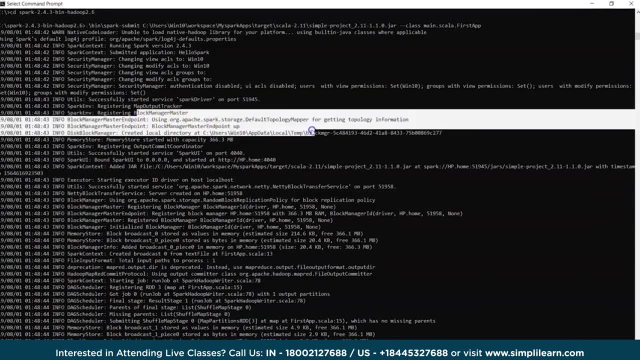 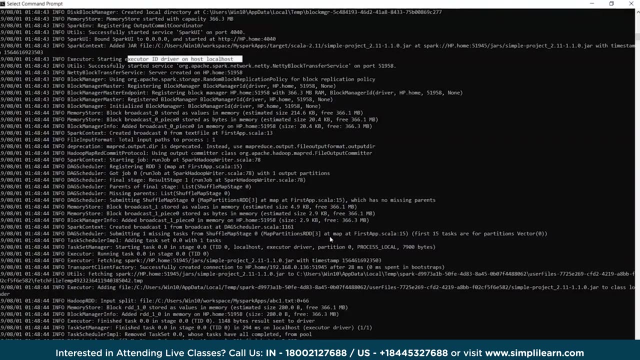 submit, to submit an application which is running in local mode so we can see further. if it starts processing, so here it says created local directory, then it starts an executor on local host, it goes for execution and then if we see further, we could also see it will add our jar to. 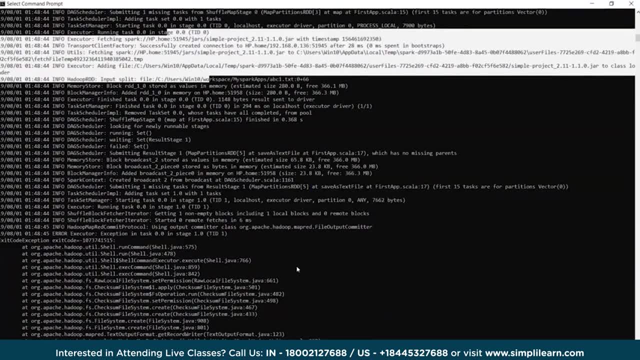 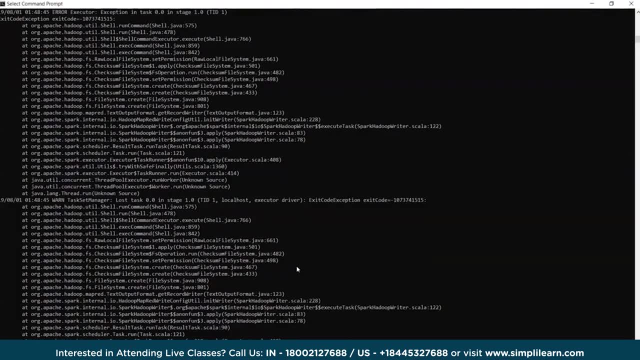 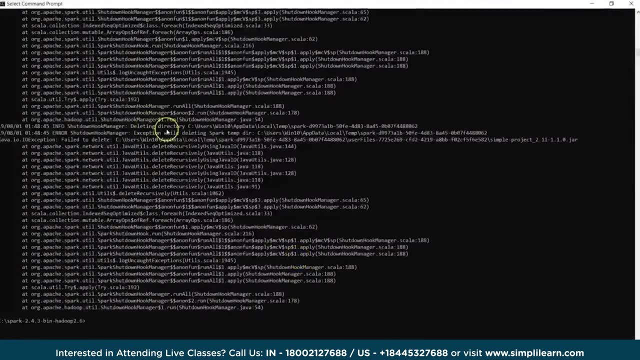 the class path and then, finally, it should be doing the execution now if there is any error message that might be related to your file not being deleted or if there is any problem with executor, so we can basically come back and check here if there was any specific error. 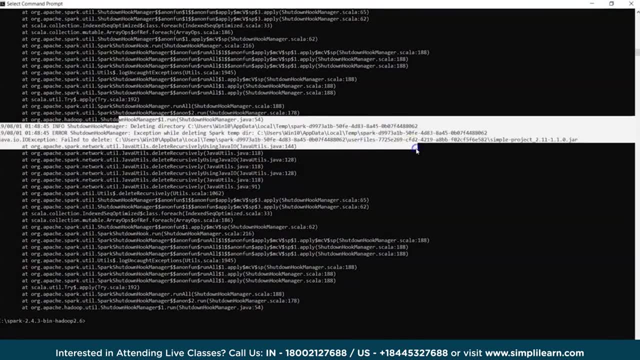 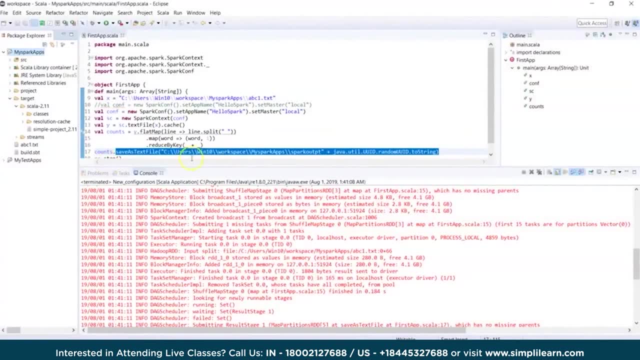 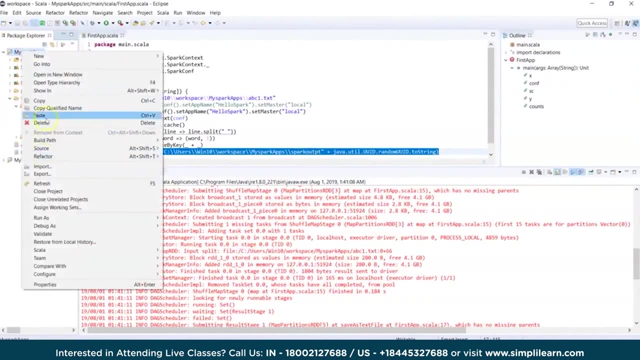 so it. the error was that it tries to delete temp directory but it does not have the permissions. so we have not done that. but as per my application, it should be creating a output in this folder as spark out. so let's click on this and see i'll do a refresh. 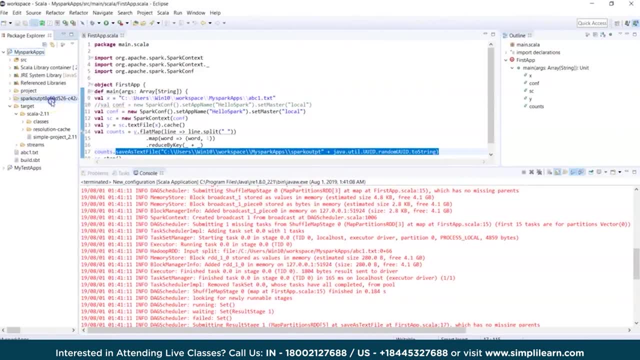 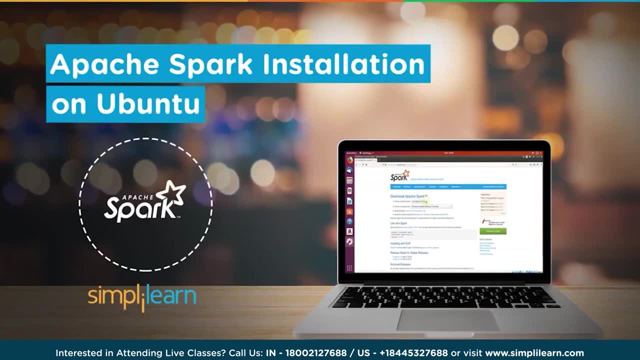 right and, if you see, a new spark output has been created. previous sessions we have seen how we can set up spark on windows or set up our spark related ide so that we can run our applications on windows. now, here we have a quick demo on setting up spark as a. 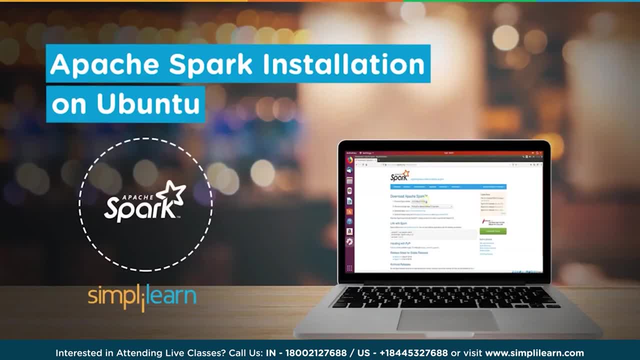 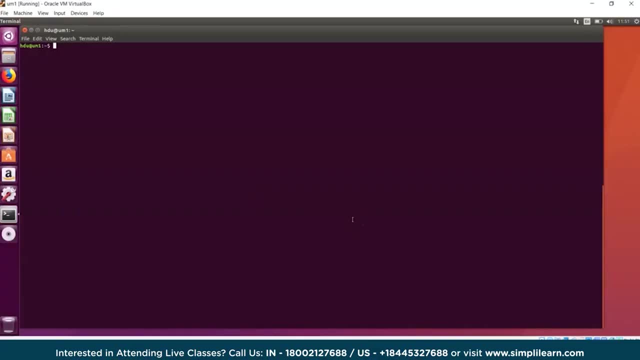 standalone cluster on ubuntu machines and then trying out spark way of working, for which we need at least two machines. and here i have ubuntu machines set up, um1 and um2, just to give insights on how my machines look. so if i look in my pc host, i 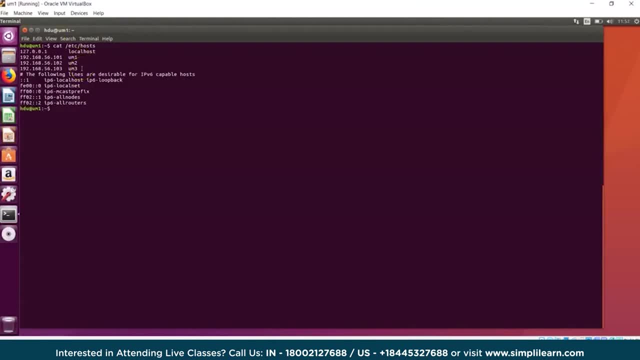 have the ip address of multiple machines, so i can ping one machine to other machine by just doing a ping um2, and that should work fine. similarly, i have also set up ssh access for these machines. both of the machines have hdu as the user and i can just 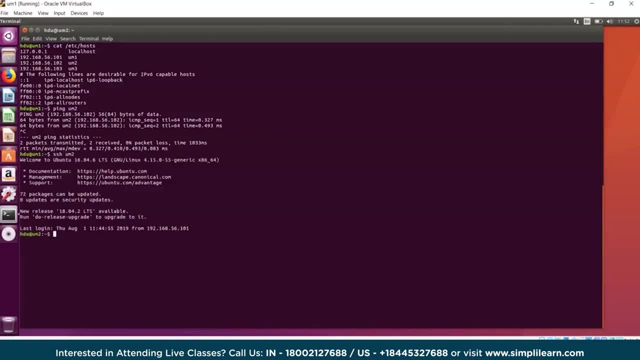 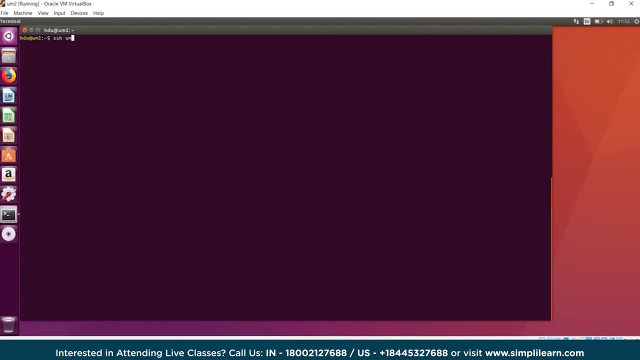 do a ssh um2, and that logs me into the second machine without a password. similarly, i can check the same thing from my second machine by doing a ssh um1, and that works fine too. so we need two machines which can ping each other. firewall disabled, able to ssh. 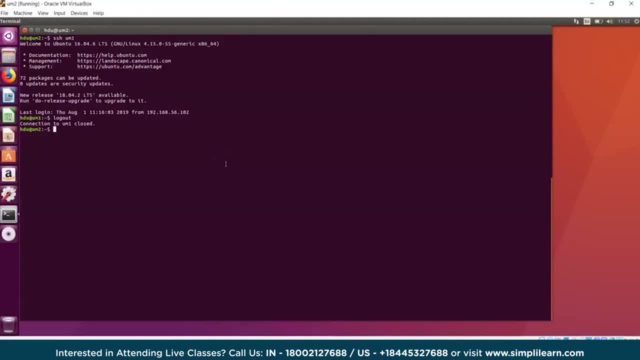 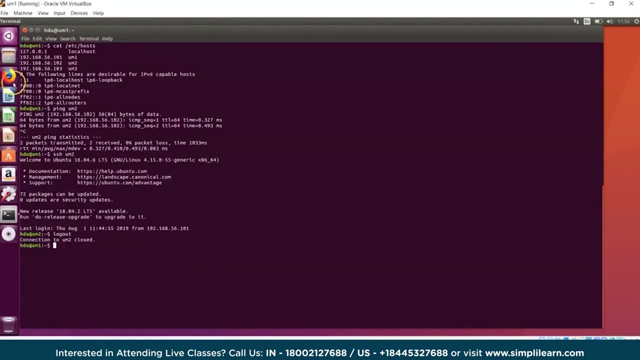 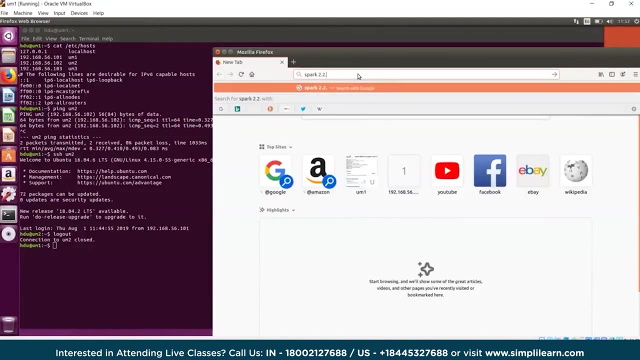 each other so that we can set up a standalone cluster of spark. how do we do it? so? first thing is, we will have to download the spark related tar file. now i can just go to google and i can type in spark 2.2.1. 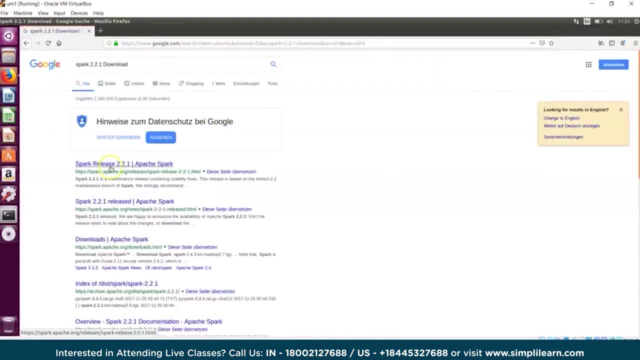 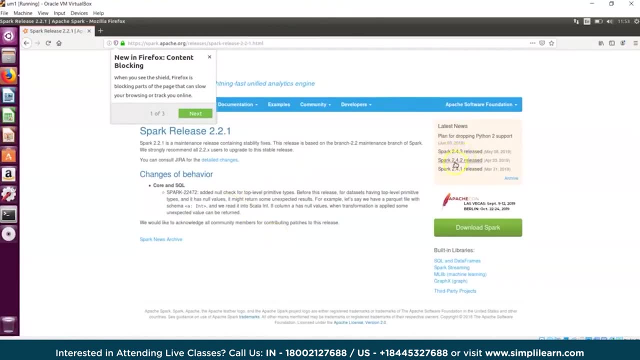 download. now that's what i'm interested in, and this takes you to spark release 2.2.1. however, here it shows you the latest release is 2.4 and then 2.4.2. so what we can do is we can go. 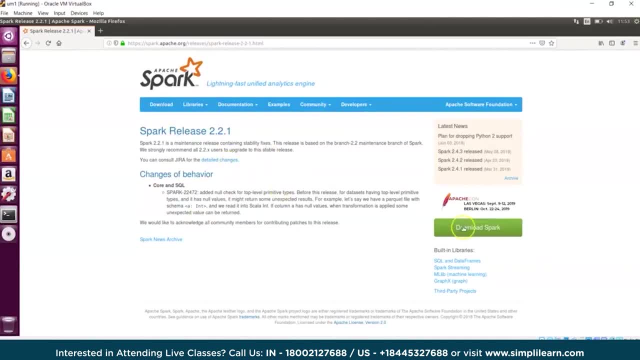 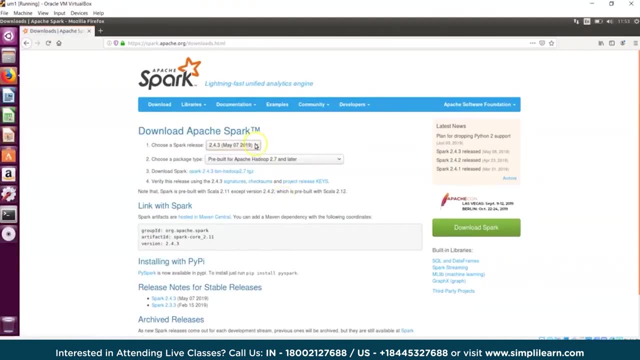 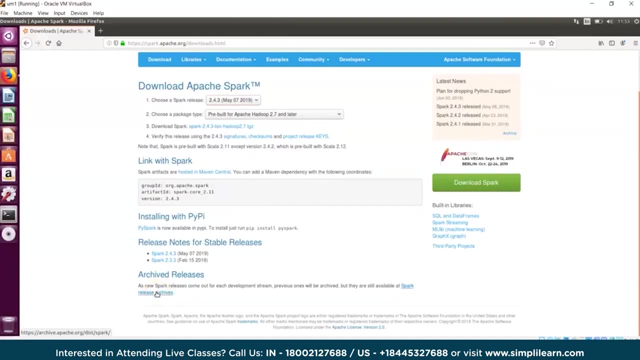 to archives, so i can basically look at existing versions. now here i can click on download and this shows me a spark release and also prebuilt for apache hadoop. now what we can also do is we can go to these archives for an older, stable version. i click on this and 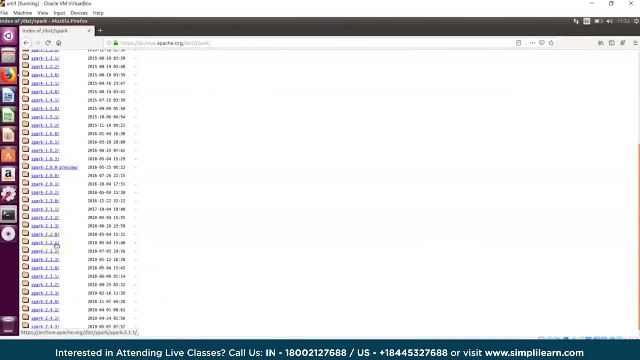 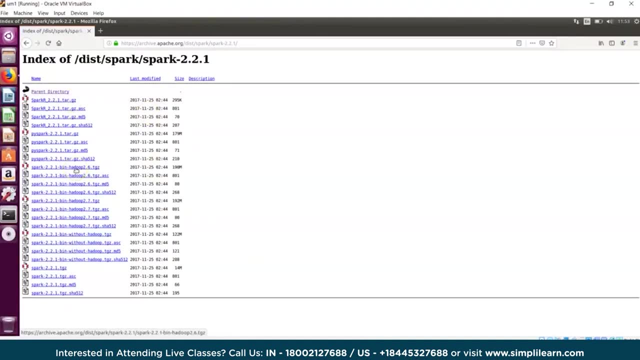 here i have spark 2.2.1. now i can click on this and we can either install something which is not already built or we can download this one, which is spark 2.2.1. bin hadoop 2.6.tgz. 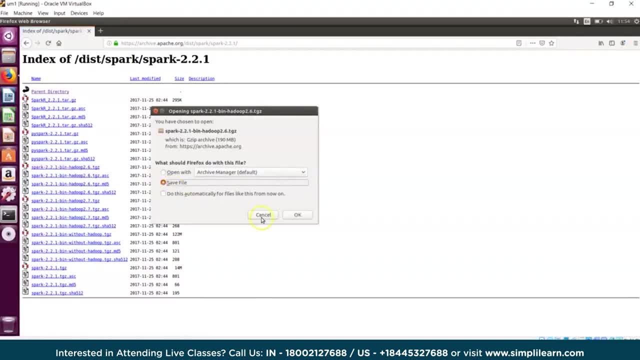 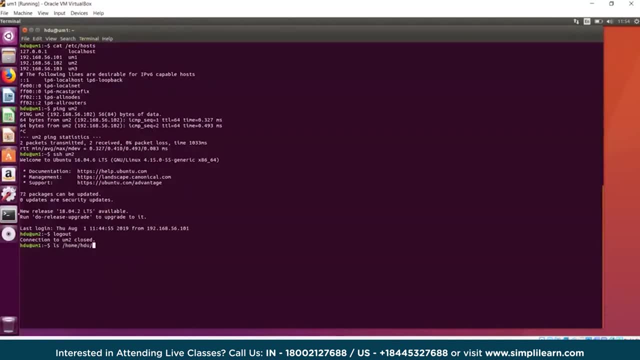 so you click on this link and then save this file, which i have already done. and here, if you see, in my machine i have home hdu downloads which has my different packages which i have downloaded. also, if you notice, i have downloaded jdk8, so you can check on my machines. 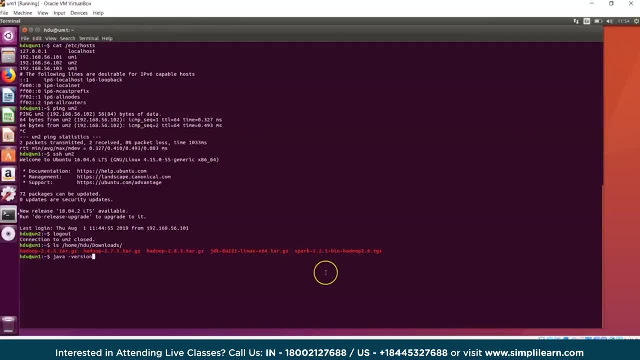 so, apart from machines being able to ping each other and being able to do a ssh, we also need machines to have java, which is already installed once this is done. now i have my spark related package, so i go into user local directory and then you can give a command here. that is. 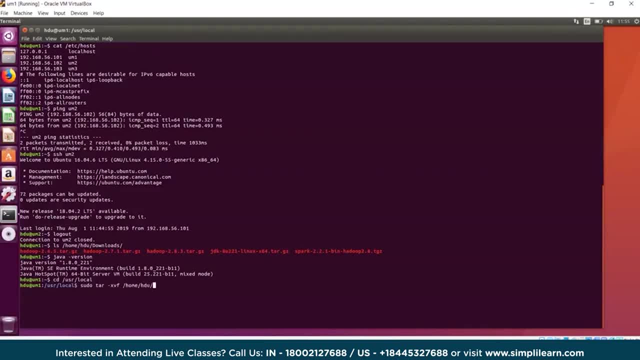 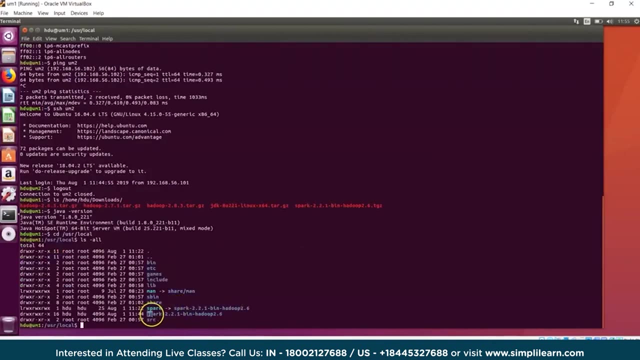 sudo tar xvf home hdu downloads and then give your spark package. now, once you do this, this will untar the spark directory and create a directory in my user local location. if you see here, this is the directory which is created, but you also see that there is a spark. 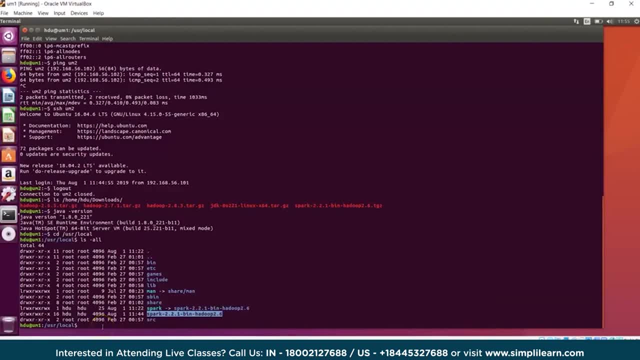 link which is pointing to spark. now that is because if you would want to work on a newer version of spark, you could just do the same thing for newer version and then make your link pointing to the newer version of spark. how do you create a link? you can just say sudo. 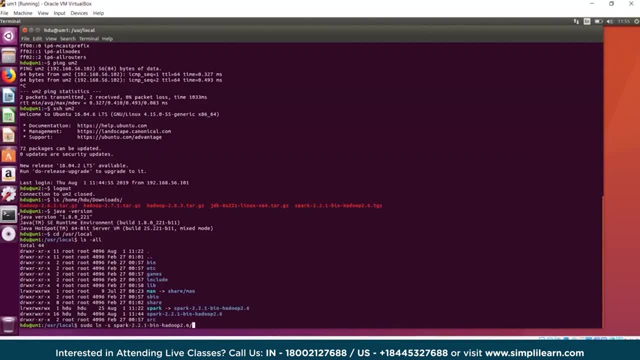 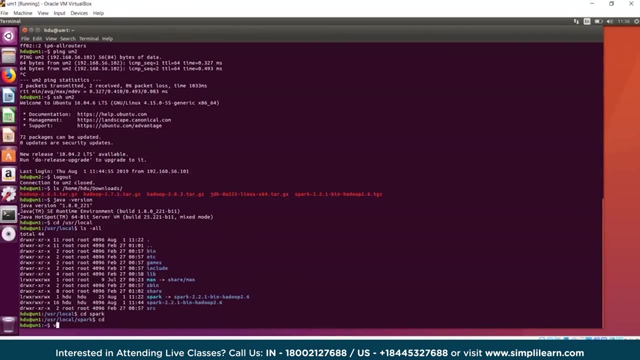 ln minus s. you can give your spark directory and then you can create a link. so i have already created a link and my spark path will then become this: now, what do we do with this? once we have done this, once we have created a link, we can go into the bash. 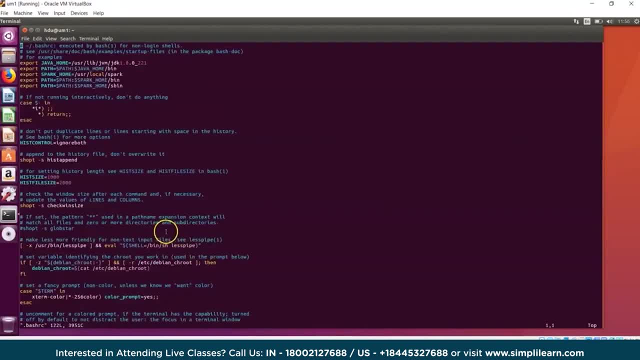 file of my user and, if you carefully see, here i have given my java path so that i can execute java related commands, and i have also added my spark related path here which says user local spark. so in case you would be changing your spark version to a latest. 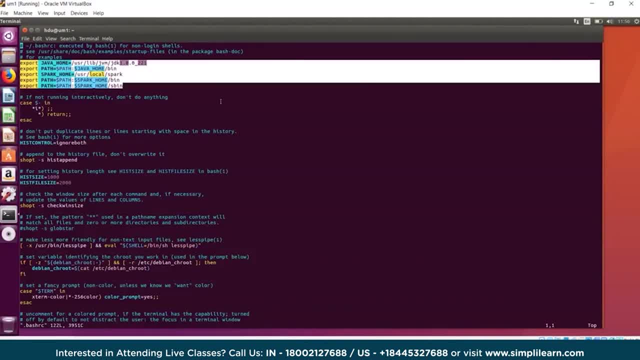 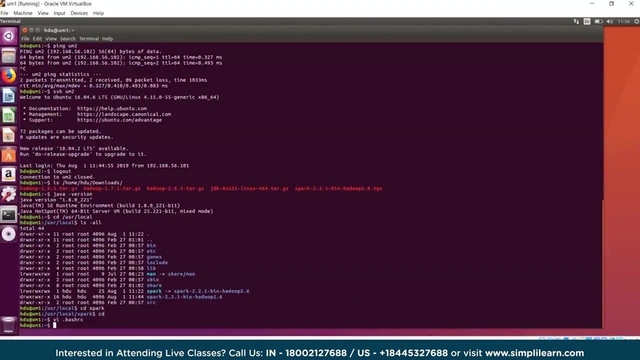 one. you will not have to change things in your bash file. only thing you will have to do is unlink the existing spark link and create a new link to your newer version. so this is done on this machine and now i can basically be using spark now before. 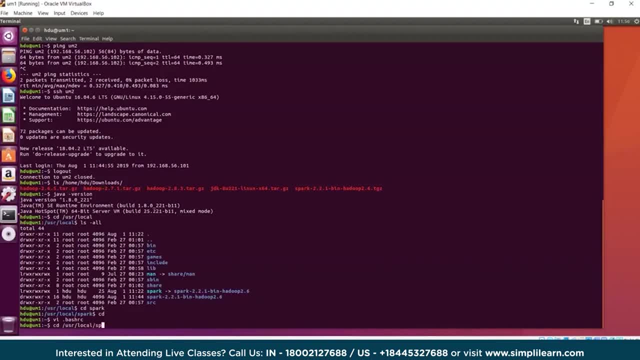 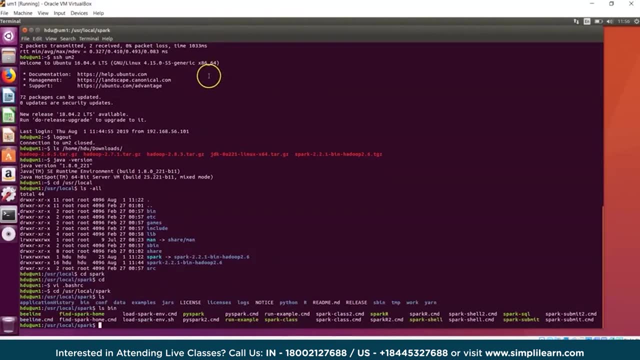 doing that, we can go into user local spark and this has different directories. so if you look in bin, these has the binaries, programs like your py spark, your spark shell, spark sql and spark submit, which we will see how we can use here. if you look in sbin, it has other. 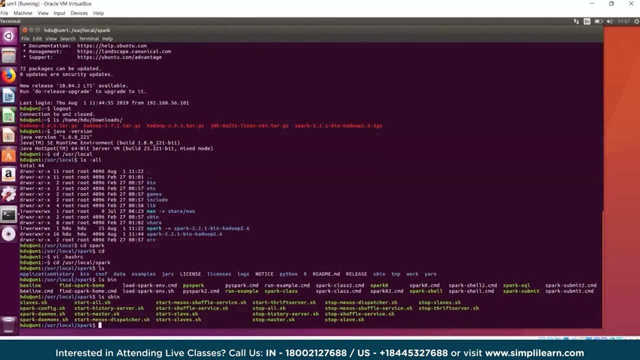 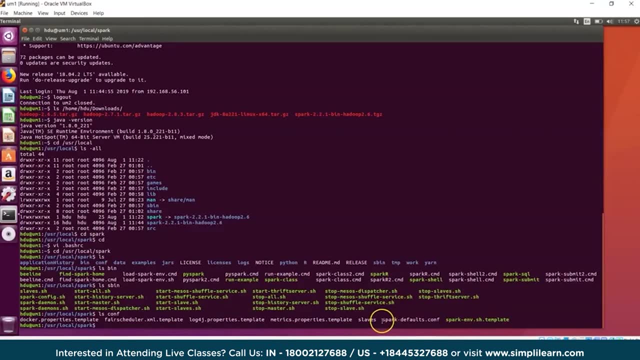 startup scripts to start your history server or to start your master or worker processes. if you look in conf, this has your config directories. now here by default, you might see spark minus default dot conf- dot template. i have renamed that to dot conf. slaves template has been renamed to: 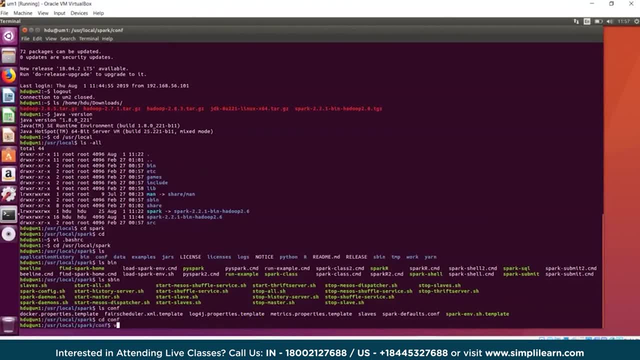 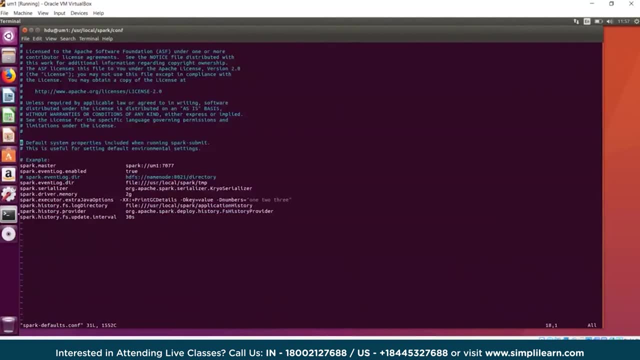 slaves. so let's look into this so i can go into conf and then i will look in spark default conf now here, based on our setup now here, we intend to set up a spark standalone cluster that is without hadoop, but i would want to have a spark. 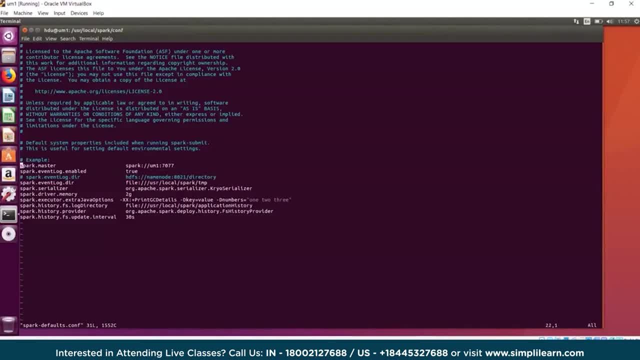 standalone distributed cluster so i have uncommented this property. it says spark dot master and i say spark and i also mentioned that my master will run on this machine, which is um1. spark event log dot enabled is true because we would want to track the events i have. 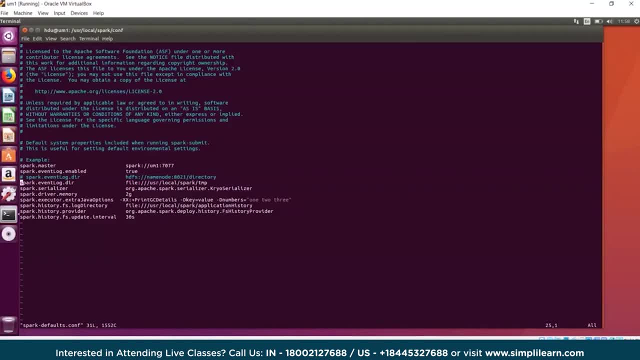 mentioned a directory, so this is a local directory in user local spark and we will have to create it. it talks about the default serializer. it talks about the driver memory, which was, by default, 5 gigabyte. i have reduced it to 2 gigabyte based on my 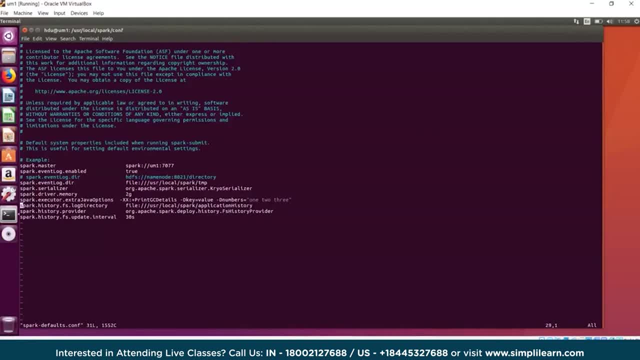 machine configuration you have java options and then if you intend to run a history server so that whenever your spark applications complete you will have your application stored in history server. i have given the log directory, which is user local spark and then application history, and this also needs to be created. 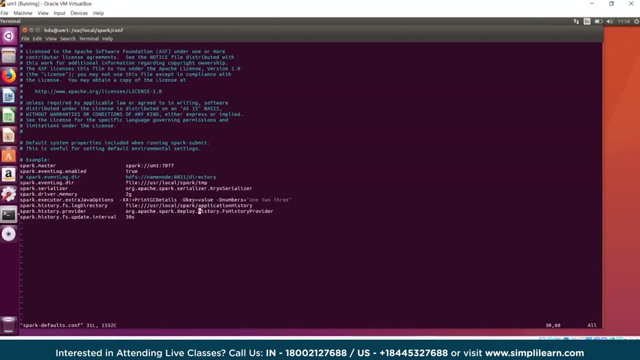 we have spark history provider for the class which takes care of history server and the update interval of looking for your application. so this is what we have in our spark default and if you look in slaves, i have given the machines where i would want my worker processes. 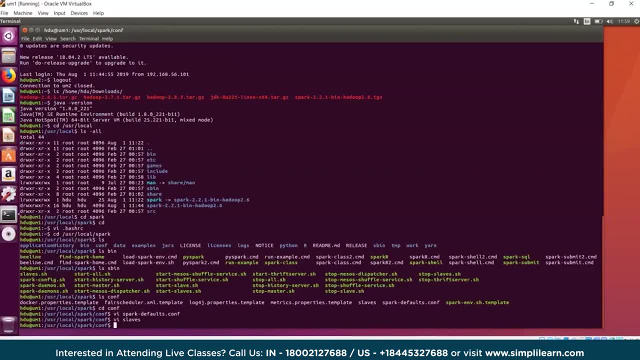 to run. so that is um1 and um2. now, once you have made your changes in your spark default conf and slaves file, what you can simply do is scp, assuming that whatever was done on this machine- that is, untiring your spark directory, creating a link, updating 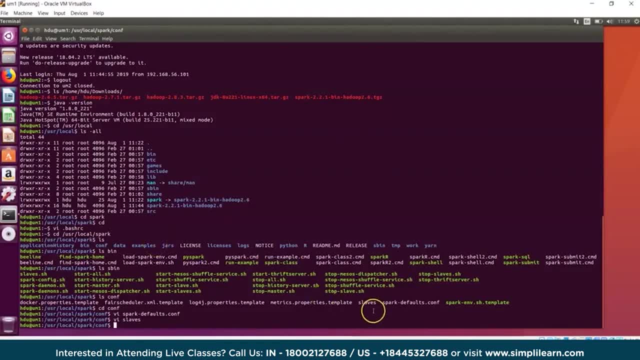 your bash rc and renaming your config files. same steps need to be done on the second machine, and your second machine would also be prepared to be used for your spark cluster. so once you have both the machines which can ping each other, which can ssh each other, both of the 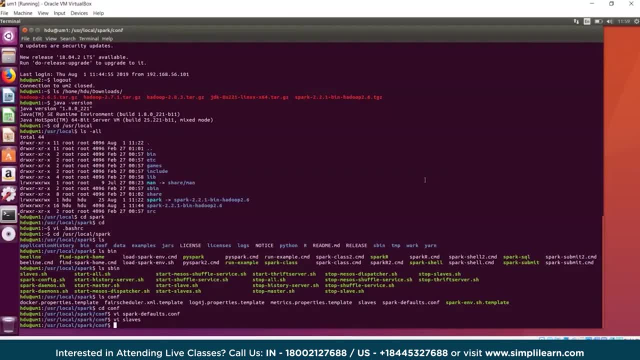 machines have java. both of the machines have the same spark version downloaded and the basic setup done. i can just easily copy the spark related config from here into my other machine, that is sdu um2, and then i can give a path which is user local spark conf and in this way, 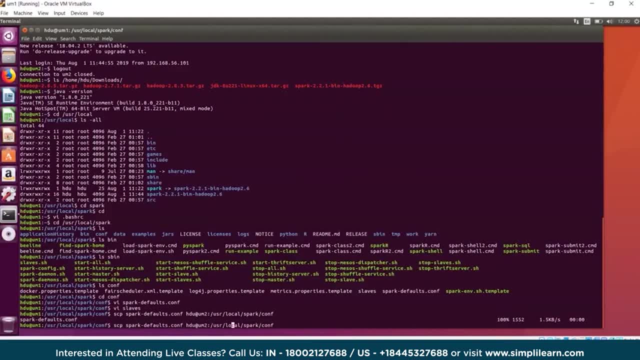 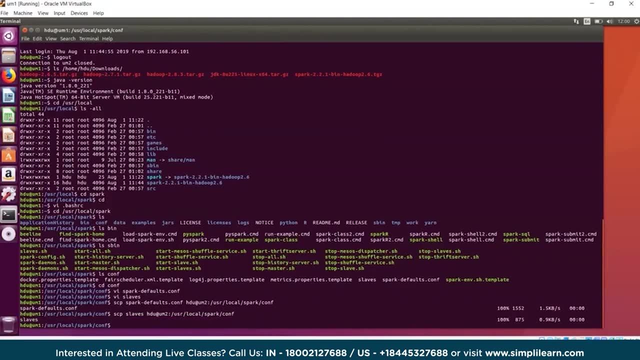 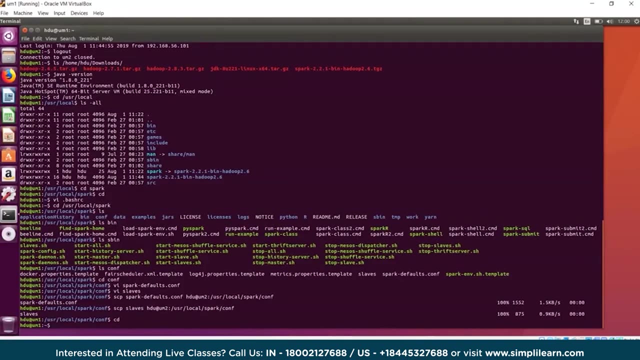 i don't need to edit my config files again and similarly, i can even copy the slaves file. this is all we need to basically have our spark standalone cluster. now, since we have updated our bash rc, we can give our spark command from anywhere we have set up our config files. 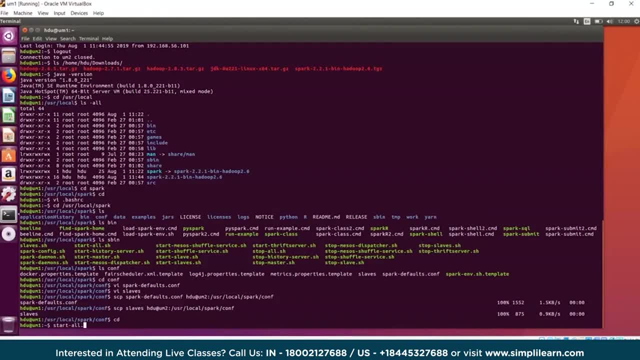 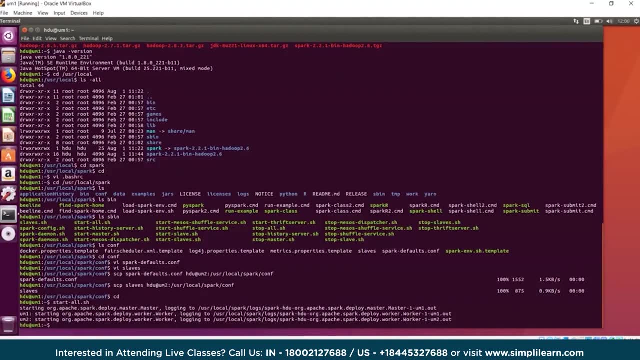 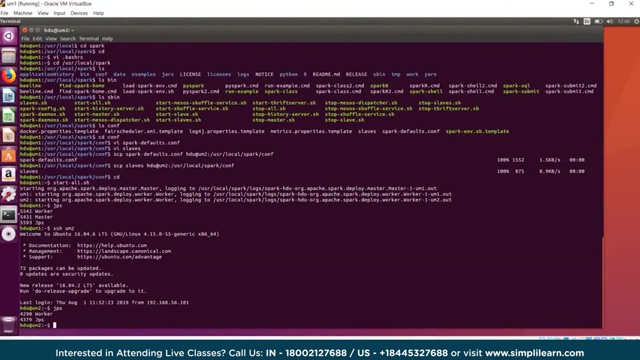 so i can just do a start minus all dot sh and that, based on my config files, based on the directories which are mentioned, it will start my master process and my worker process on both the machines. so here we have a spark standalone cluster which has two workers. 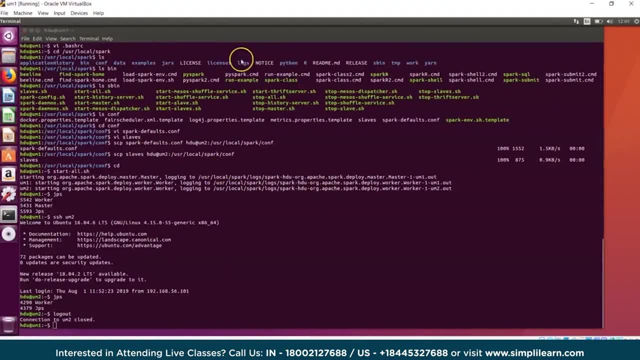 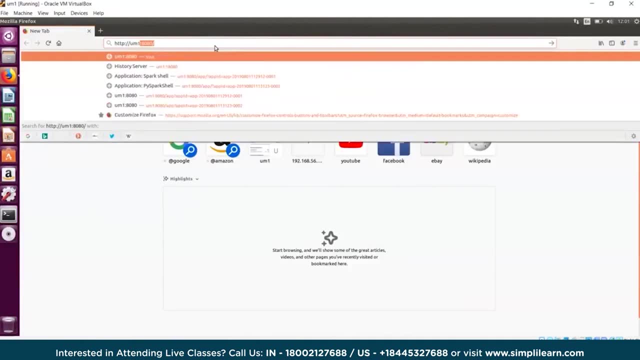 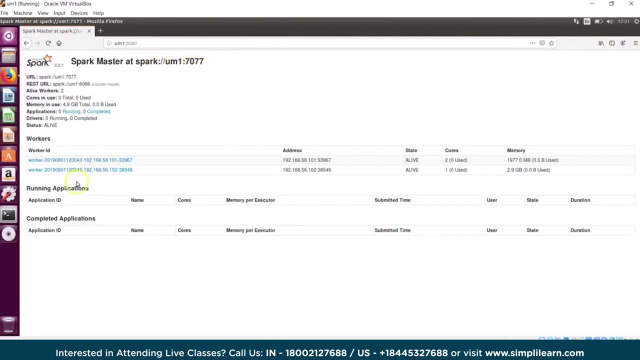 and one master. now we can always go to the browser interface and we can check for the spark ui, which should be available, by typing in http: slash, slash, my master, and then the port is 8080. so this shows that i have a spark master running. i have two worker processes. 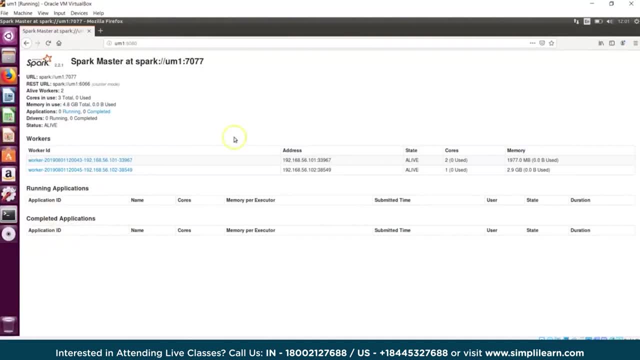 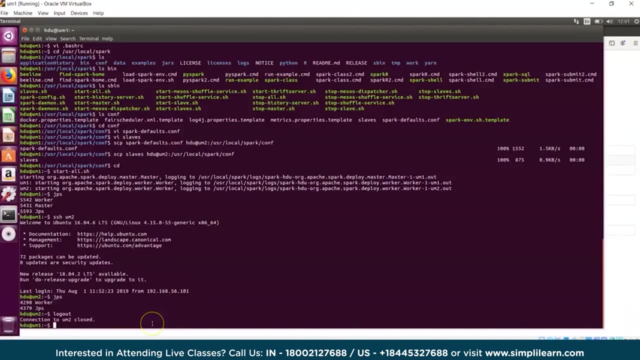 right now there are no applications which are running, but my spark ui is already available. when we start using spark, either by spark shell or py spark or even spark submit, we will see our applications getting populated here. additionally, we can also start the start history server by just. 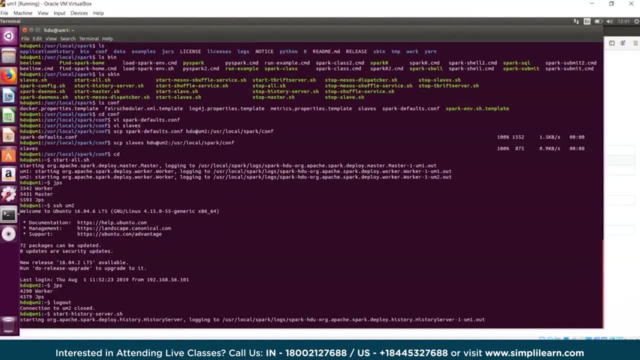 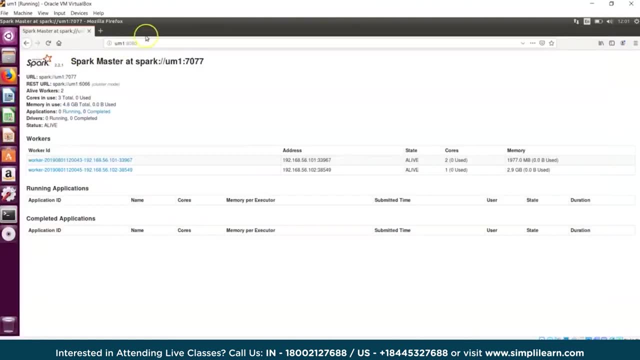 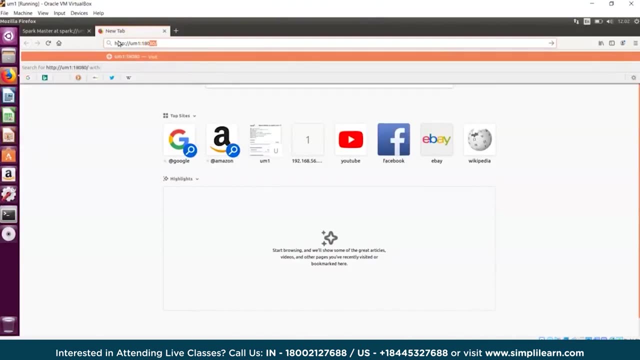 saying start history server dot sh and that will start my history server. once this is done, we have a history server also running and we can go back. and then we can again pull out the history server user interface by giving in the port, which is default, 18080. 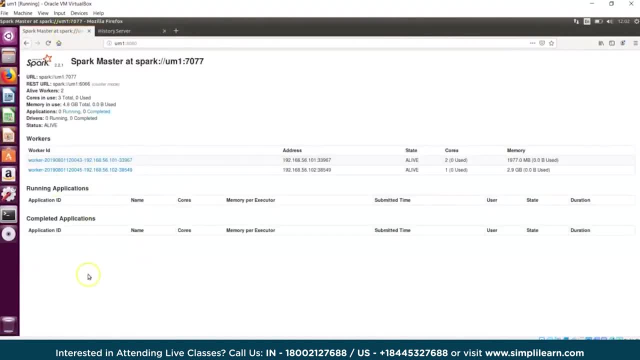 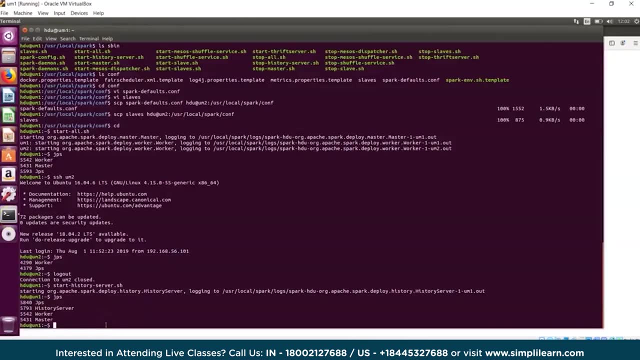 so i have a spark standalone cluster with one master, two workers and also a history server which is running. once we have this, we can try working with spark, either with spark shell or py spark or, if you have packaged your application as a jar using sbt or maven, you could also. 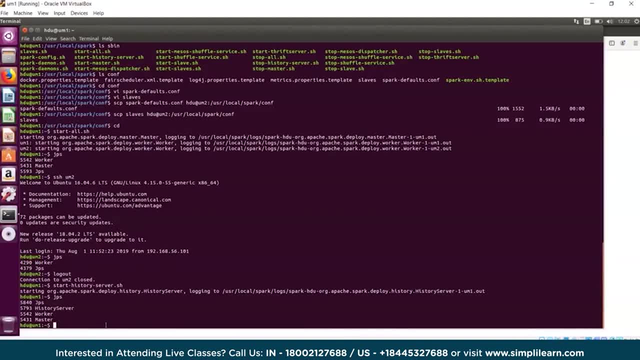 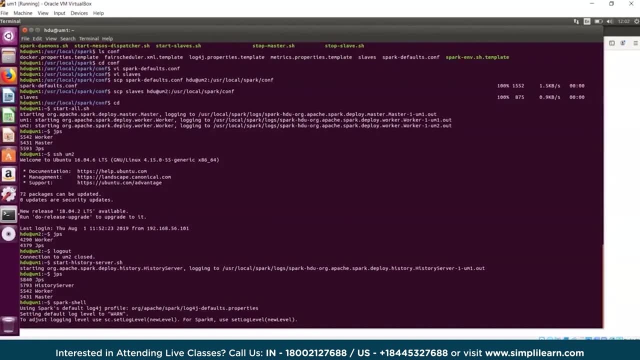 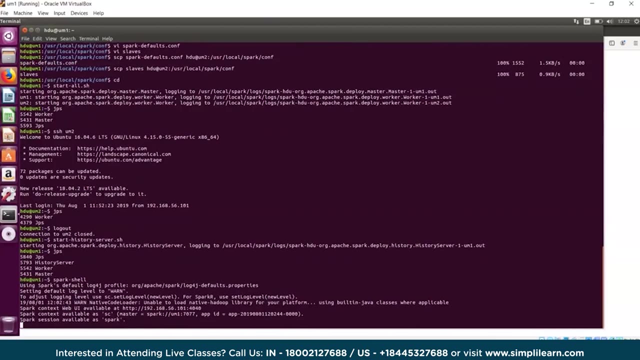 use spark submit. additionally, you could also use spark sql. so to work with spark, i would just say spark shell on one of my machines, both my machines which have worker processes running. we can start our spark shell on any of these machines. remember, here our spark will rely. 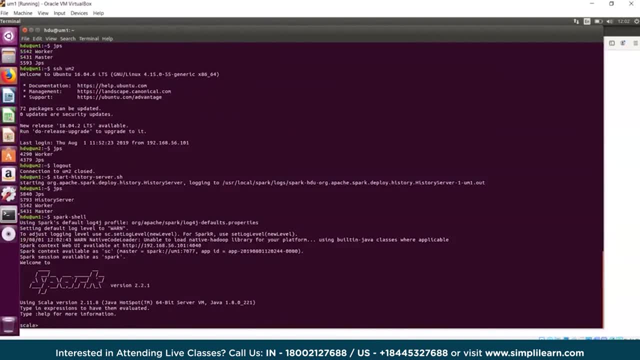 on the storage of these machines. that is the file system, because it does not have any hadoop or distributed file system. we have started our spark shell and that shows spark context, which is available as sc. spark session is available as spark, so to work with spark core and. 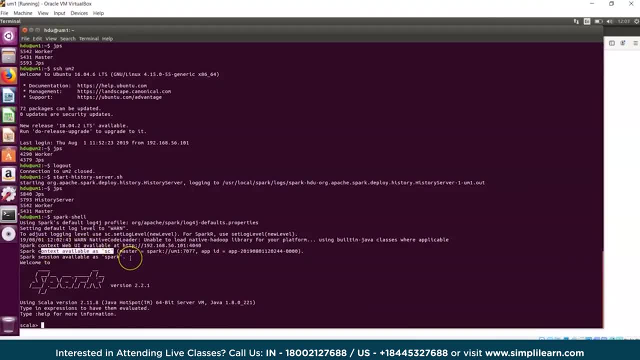 rdds, we would be using spark context and if you intend to work with spark sql- that is, data frames and data sets- you can be using spark. let's try a quick, simple example. so i'll say val x, sc, dot text file, and now i would want to point it to a file. 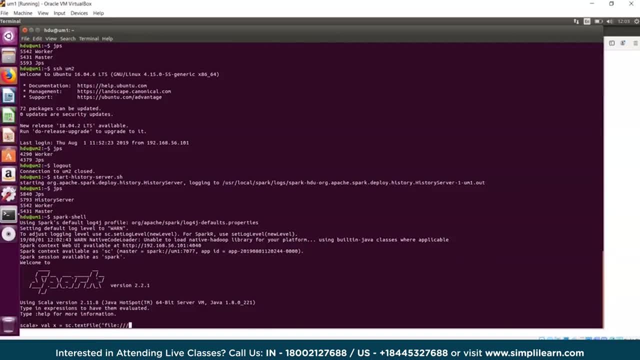 so i will say the complete path. remember, i am giving the spark command from my home directory, so i will have to say user local spark and then i can point to a file which is existing here and this is what i would want to use to do some processing. we are using the. 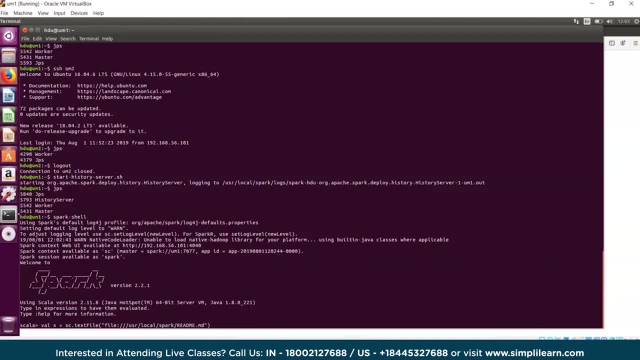 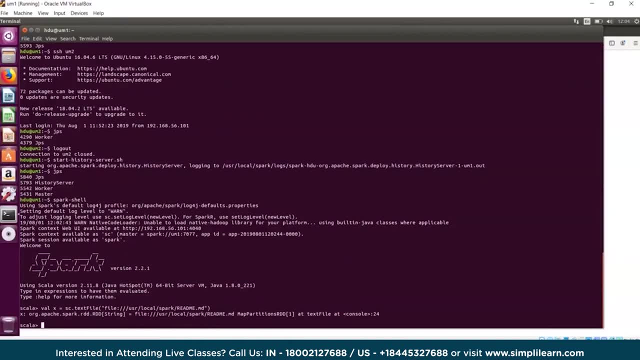 first step here, wherein we are using a method of spark context, which will not relate in any evaluation and it will just create an rdt. now we are using the scalars way, so let's create one more variable and then we can do some transformation on it. 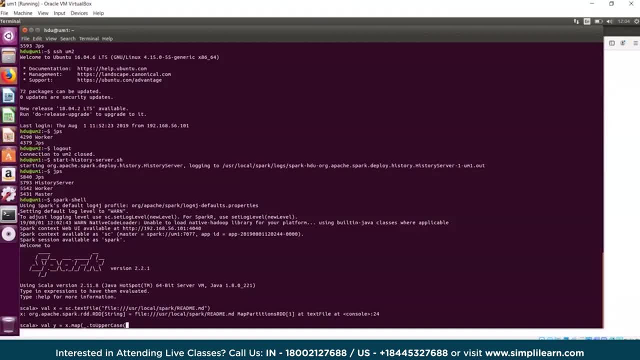 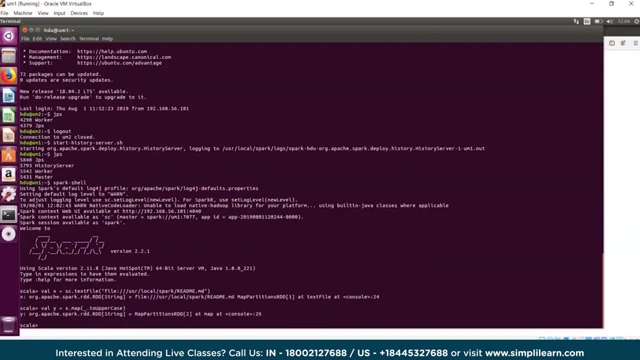 by saying: to upper case. i would just want to convert the content into upper case, and this is again a transformation, so that will just create an rdt. once this is done, we can invoke an action to basically see some results. so i could just simply do a collect. 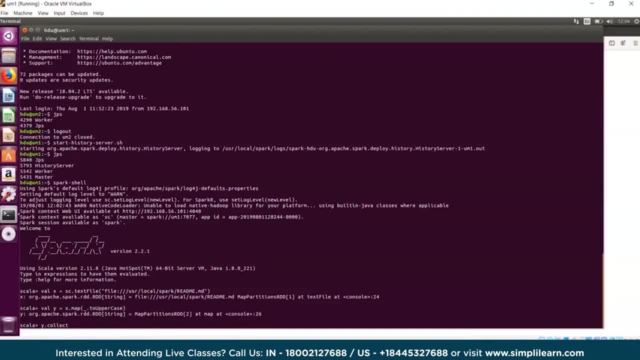 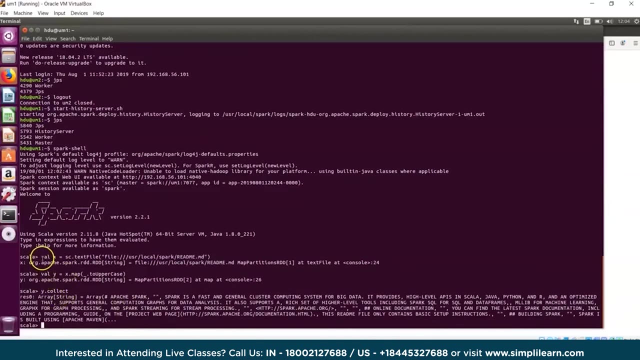 which is an action, and this action will trigger the execution of dag, which starts from the farthest rdt. that is the first step, where your file is loaded into rdt. now, once we do this, we should be able to see our result, and that, basically, is execution of dag. 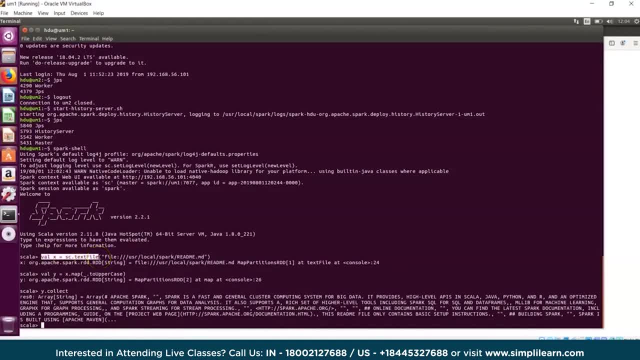 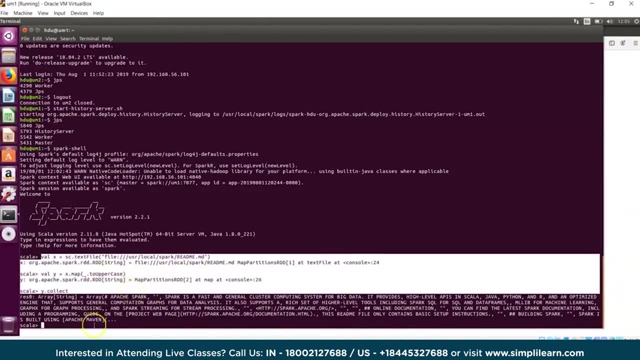 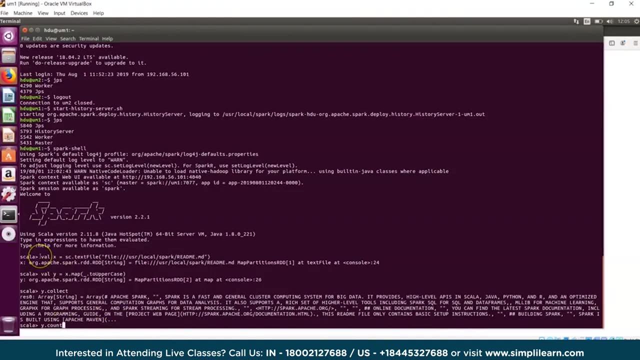 so, from the time we have used a text file, which is a method of spark context, to we did a transformation and till we invoked an action, becomes my one job. now, if i would do y dot count, which is again a different action, this will trigger the execution of dag. 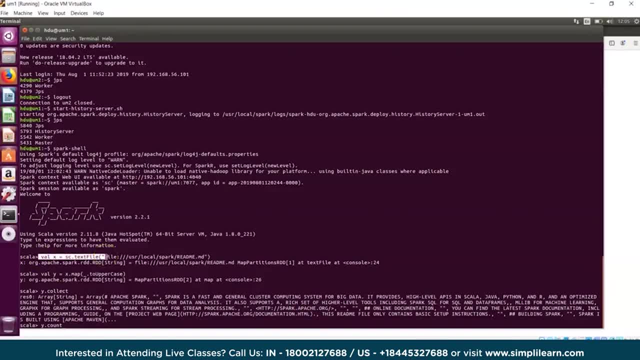 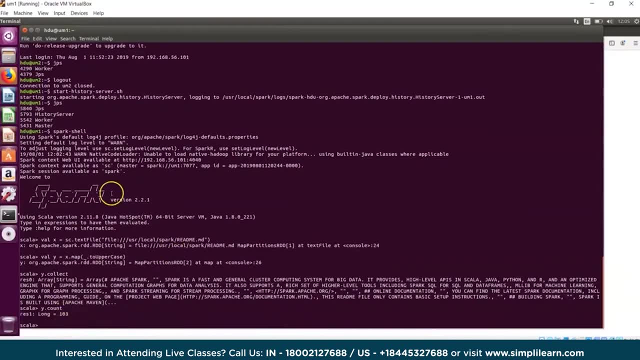 right from the beginning. that is c dot text file where the data will again be loaded in rdd. a map transformation will happen and then you will have a count. now we can always see this in the spark ui by just going in here and just doing a refresh. 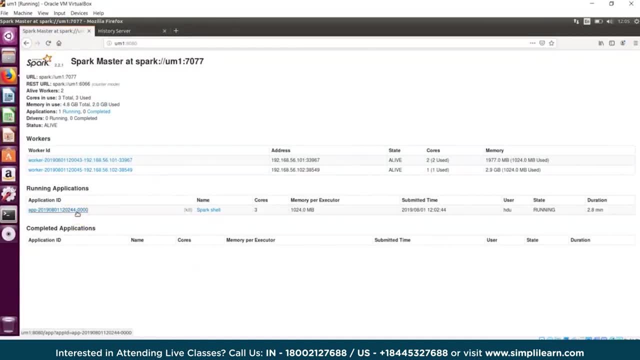 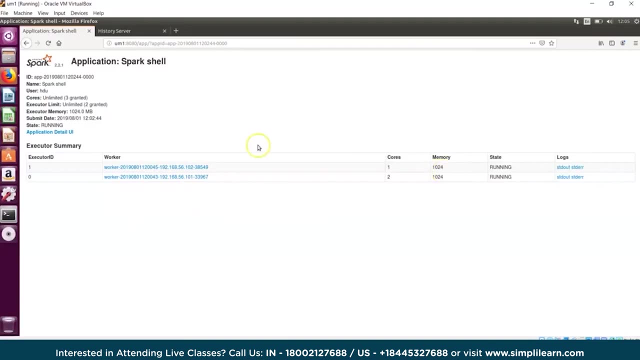 so that will show me that there is an application which is running via spark shell. it has utilized three cores, it has utilized memory per executor one gigabyte, and we can click on this application which shows that it used both the workers, one core and one gb on. 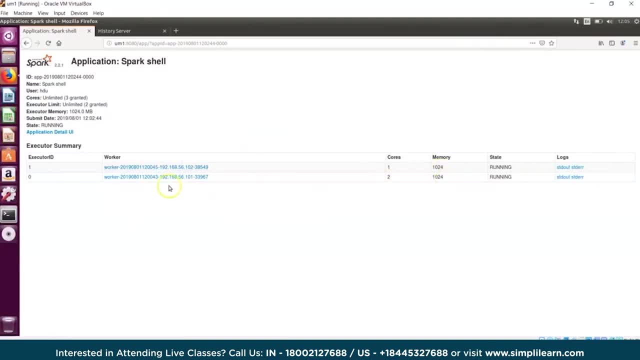 this worker and two cores and memory. on this worker i can click on application detail ui, wherein i can see what are the actions i invoked. we also see the number of tasks which are run, and that is because every rdd which is created by default is having 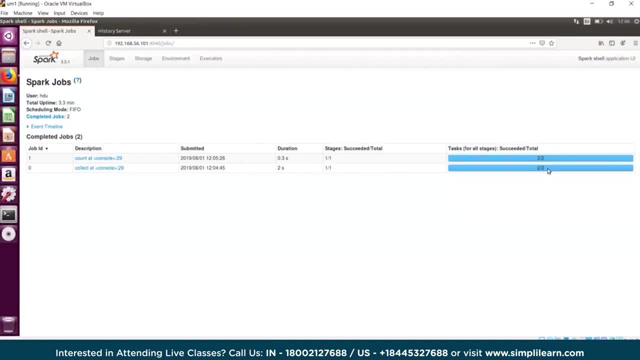 two partitions and for each partition you would have one task. well, we can change the partitions and many more things can be done, but that you can learn in later sessions. here we have two jobs: one ended with collect and one ended with count. now i can click on collect and. 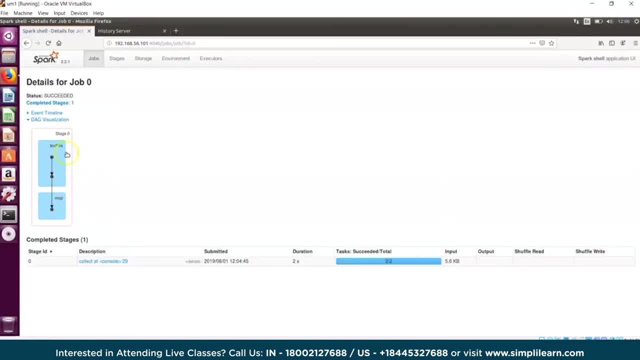 i can see the dag visualization which tells me we started a text file, we did a map and finally we did a collect. it shows that everything was done in state zero. that is just one stage. i can click on count and that again shows me the dag visualization. 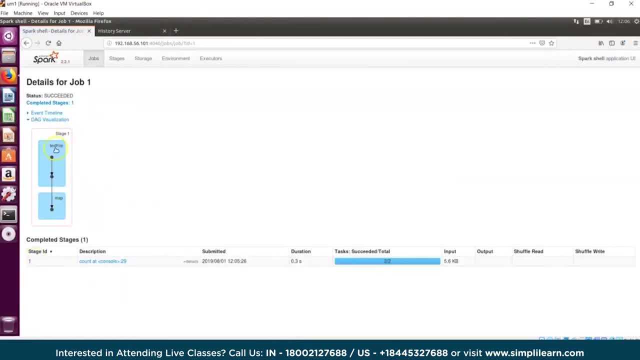 which is a different stage, a different job id, which started with text file map and then we did a count. if you would want to see more details, you can always use these tabs to look at different stages within your application. if you were doing some caching, looking at environment variables, 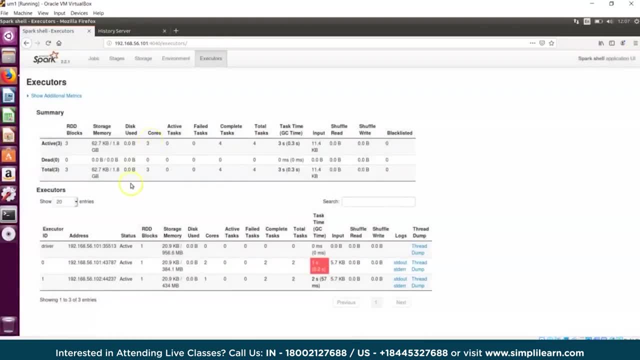 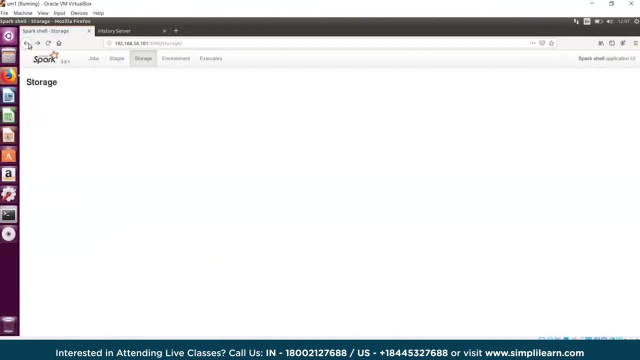 and also to see how many executors were used, including the one for the driver, on which nodes these executors ran, how many cores, how many tasks were run, was there any shuffling involved, and so on. so this is how i have used spark shell. that is an interactive way. 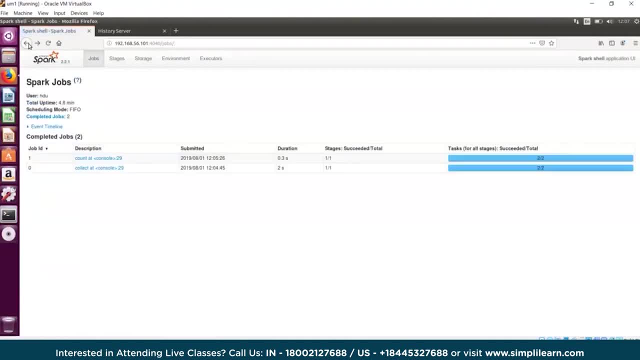 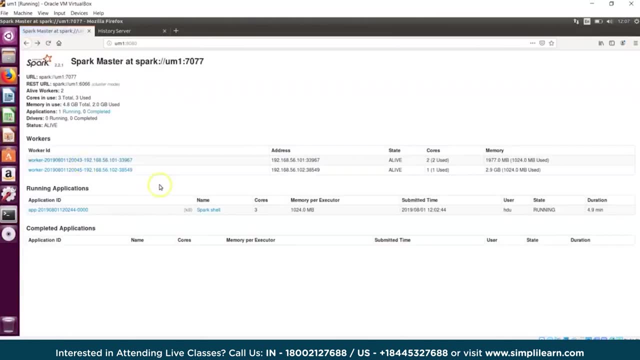 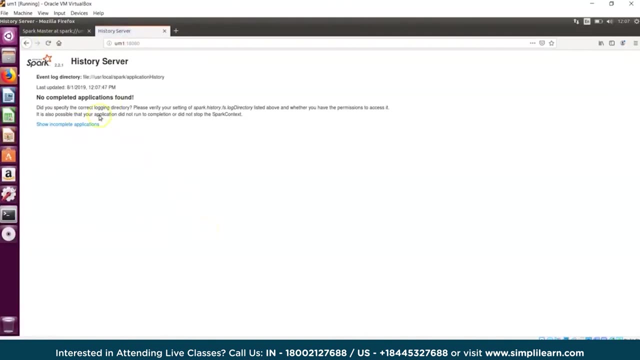 of running my application and since we have a spark ui, we can always look at applications when they have run and we can always drill down and know more details. now, since my application is completed, i can do a refresh on history server, but that does not show anything, because when we 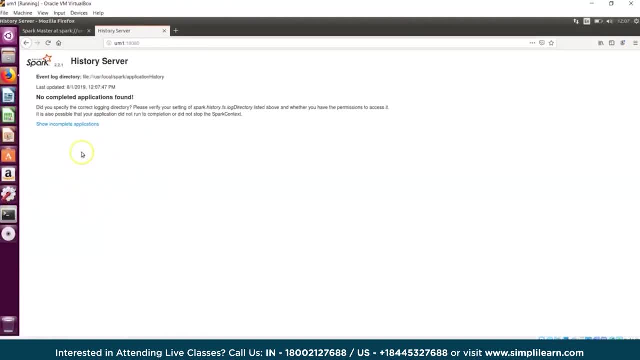 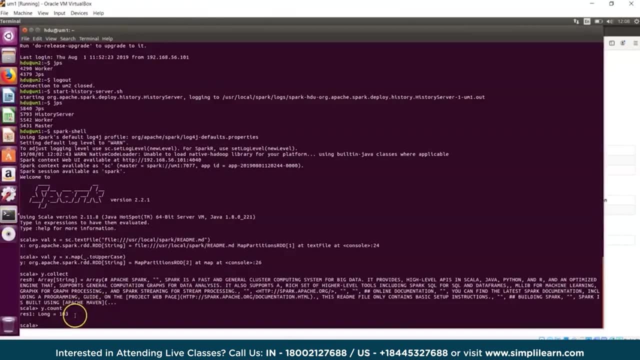 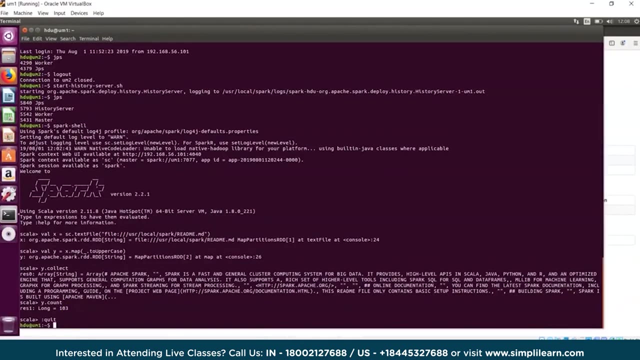 started a spark shell. it started an application and that application is still in running status, if you see here under running applications. so this is how we use spark shell on a standalone spark cluster. now we can just do a colon quit and that takes me out of spark shell. similarly, 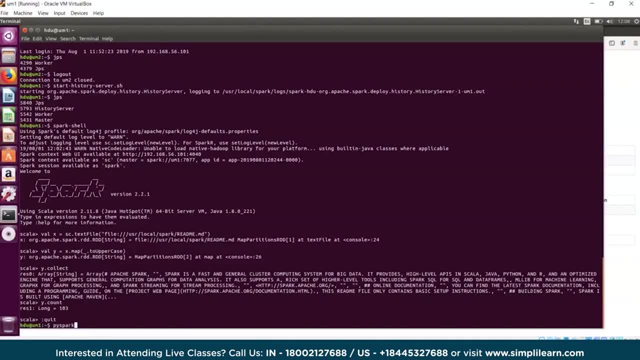 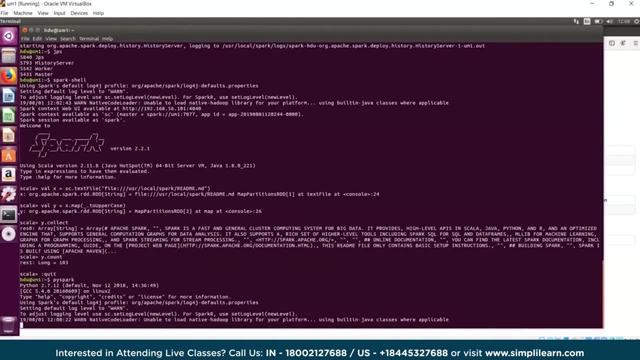 if i would want to work on pi spark- that is python's way of working with spark- i can just type in pi spark, which should bring my python shell, and then i can continue working with spark and again go back and look at my ui while my pi. 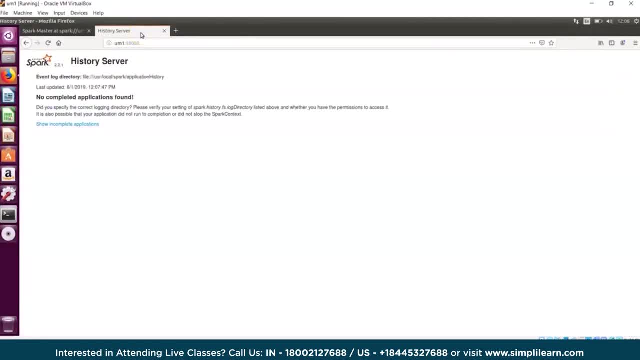 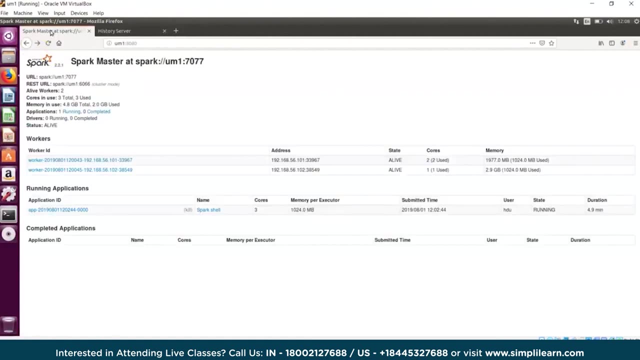 spark comes up, i can go here. since i quit my spark shell, i can just do a refresh to see if my application is yet coming up in history server. it might take some time and you can always go back and look at incomplete applications or wait till your application is populated in. 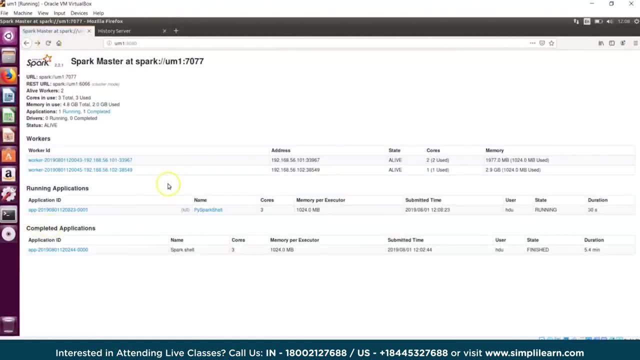 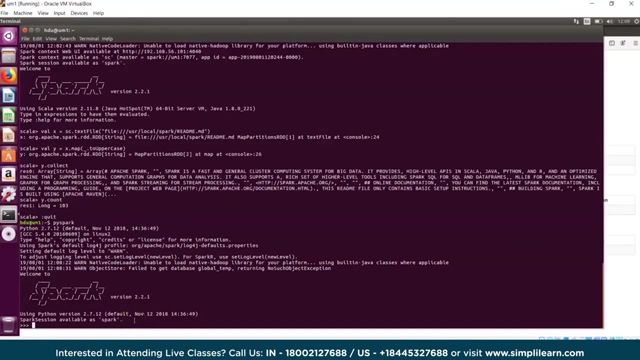 history server. now, if i do a refresh here on spark ui, it says this application was completed. it says finished and then now we have started pi spark, so it has started a new application, pi spark shell, and that is in running status. we can come back here, and now we have our python's. 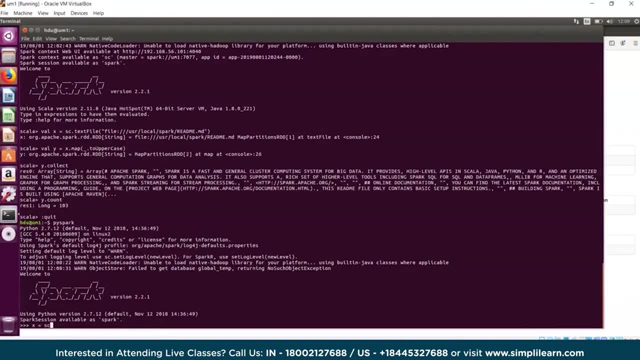 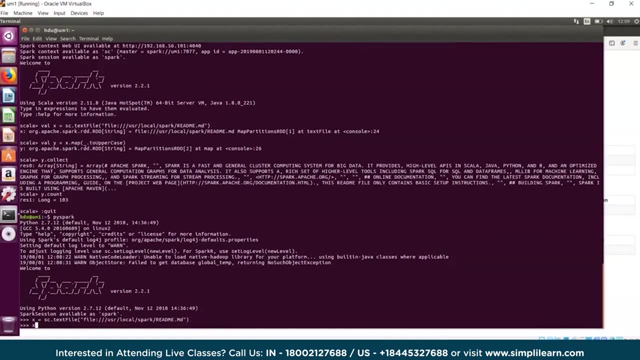 way so i can do the same thing which i did in scala using sc dot text file. i will point it to a file which exists in user local spark. read me: dot md. so that's the file which i'm interested in now. this would have created an rdt which we can confirm. 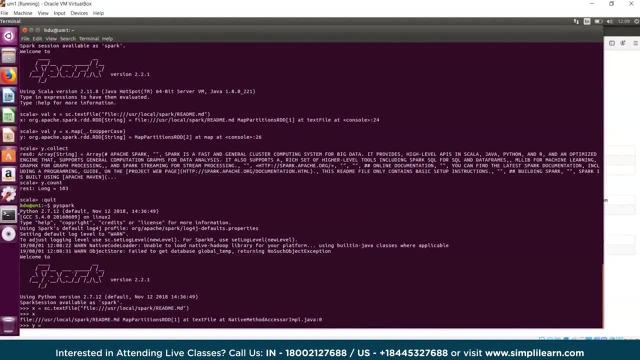 by just typing in x. now i can create a different variable and i can say: i would want to do a transformation of map. now, in case of python, when you use anonymous functions or when you want to apply some functions to your transformations, you use lambda functions. so we say: 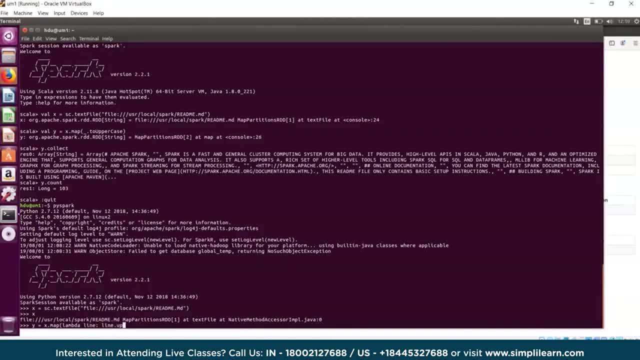 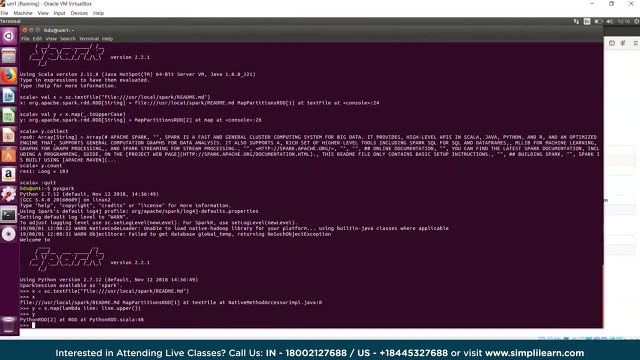 lambda line and then i would say what i want to do to the line. i will say: i will use a inbuilt uppercase upper function which should convert my content into uppercase, but as of now this is a transformation, so it only creates an rdt to see the result. 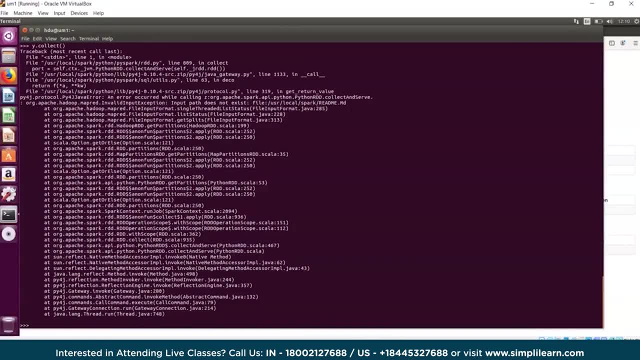 i can do a y dot collect and that should bring up my result now in case, if it says the file does not exist, that is because there was a typo here and we can repeat this step. so let's bring up here again x and i can give the right. 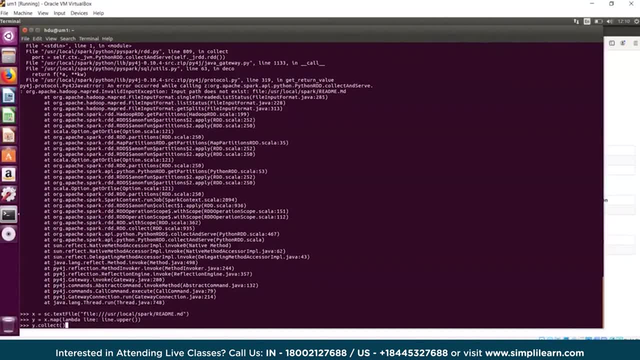 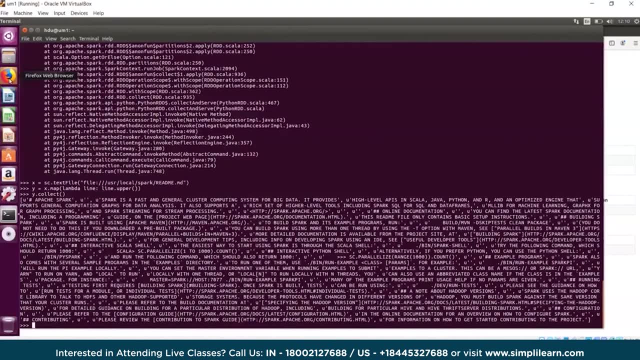 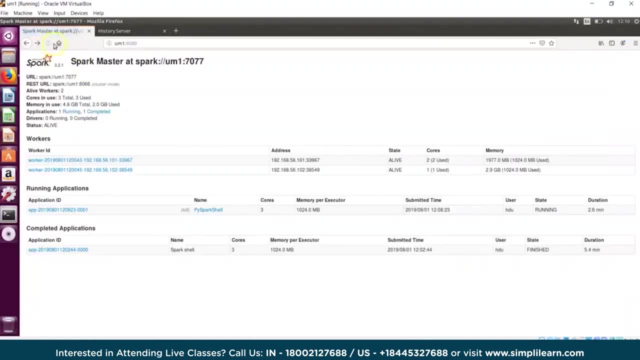 name of the file, i can do a transformation and finally i can see the result. so this is using py spark on a standalone spark cluster which is working without hadoop, which has two worker nodes and one master node. we can always come and do a refresh here to. 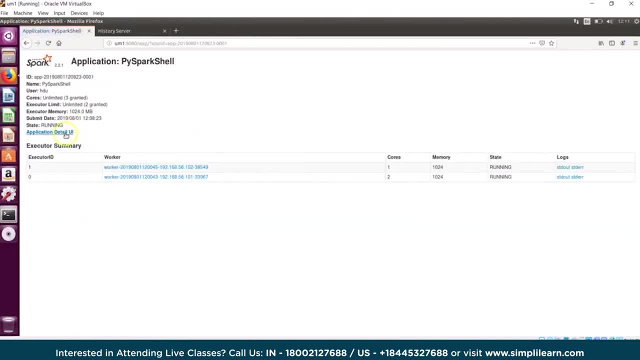 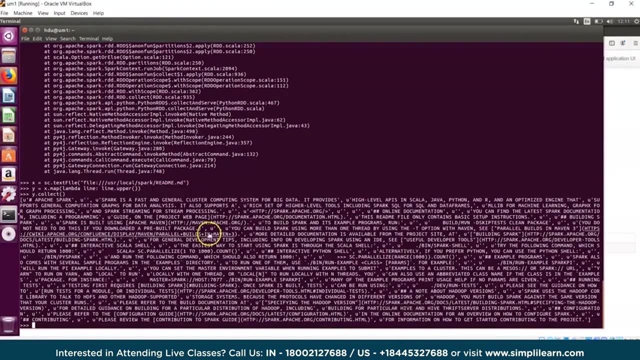 look at more details. so we have our application. we can click on this again, similarly, like we did for scala application detail ui. i see my application ended at collect. it ran two tasks and i can look at my that. so this is how we can use spark shell. 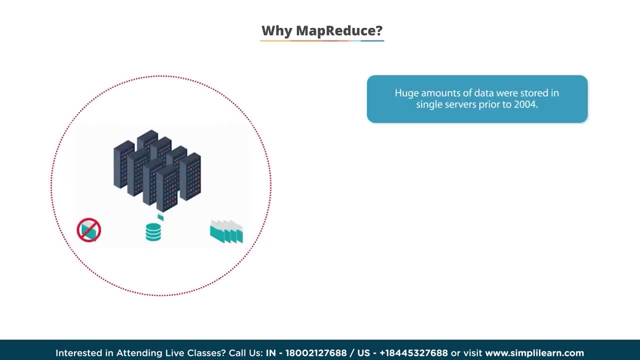 or py spark. logical integration of the search results and analysis of the data was a nightmare, not to mention the massive efforts and expenses that were involved. the threat of data loss, challenge of data backup and reduced scalability resulted in the issue snowballing into a crisis of sorts to 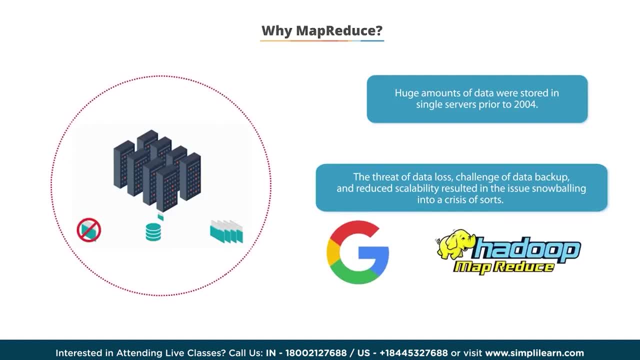 counter this, google introduced map reduce in december of 2004, and the analysis of data sets was done in less than 10 minutes rather than 8 to 10 days. queries could run simultaneously on multiple servers and search results could be logically integrated and data could be analyzed in real time. 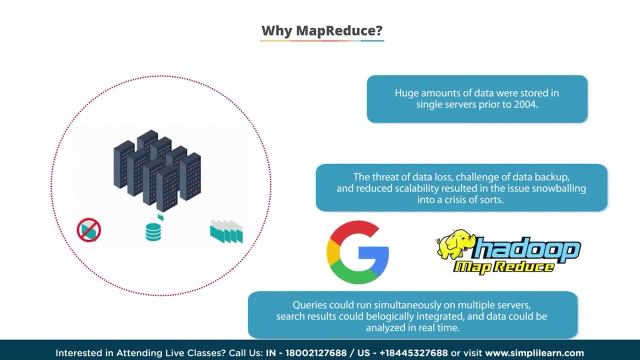 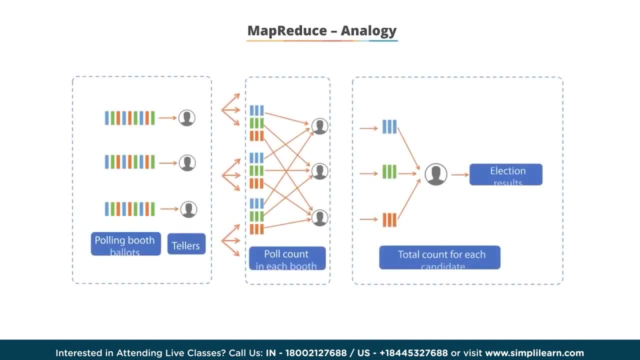 the usps of map reduce are its fault tolerance and scale availability. let's look at a map reduce analogy. the map reduce steps listed here represent manual vote counting after an election. as an analogy, in step one, each polling booth ballot papers are counted by a teller. this is a pre. 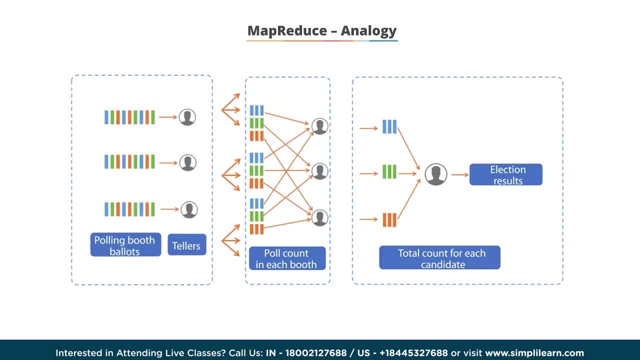 map reduce step called input splitting. in step two, tellers of all booths count the ballot papers in parallel. as multiple tellers are working on a single job, the execution time will be faster. this is called the map method. in step three, the ballot count of each booth under the 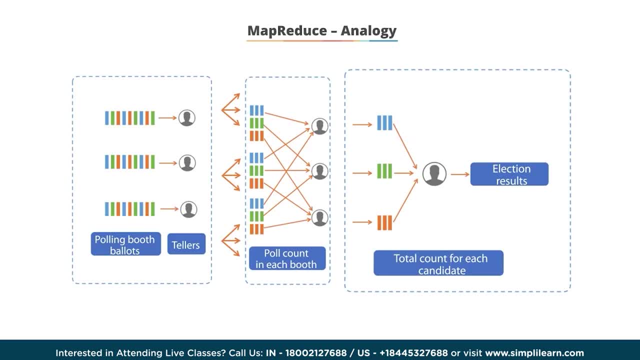 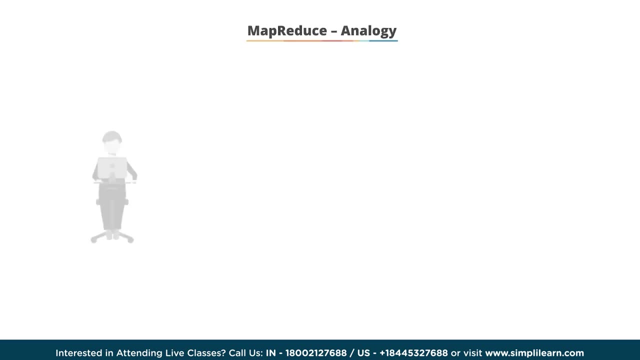 assembly and parliament seat positions is found and the total count for the candidates is generated. this is known as the reduce method. thus, map and reduce help to execute the job quicker than an individual counter. the map- reduce- analogy vote counting is an example to understand the use of 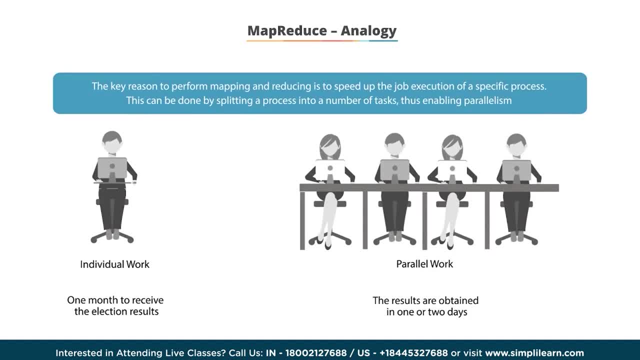 map reduce. the key reason to perform mapping and then reducing is to speed up the job execution of a specific process. this can be done by splitting a process into a number of tasks, thus enabling parallelism. if one person counts all of the ballot papers and waits for others to finish the 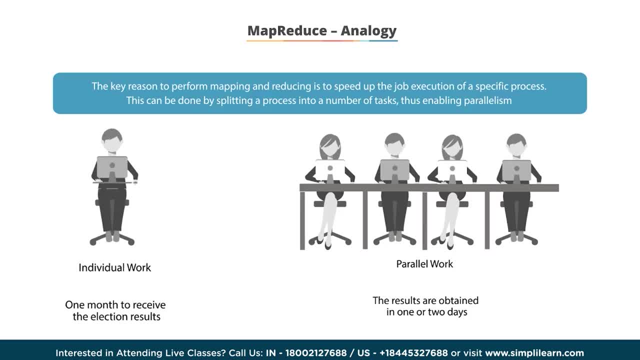 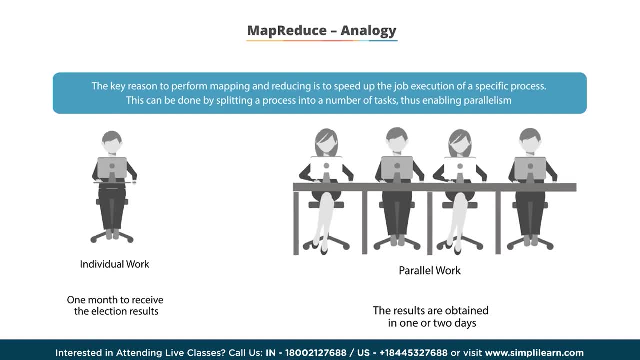 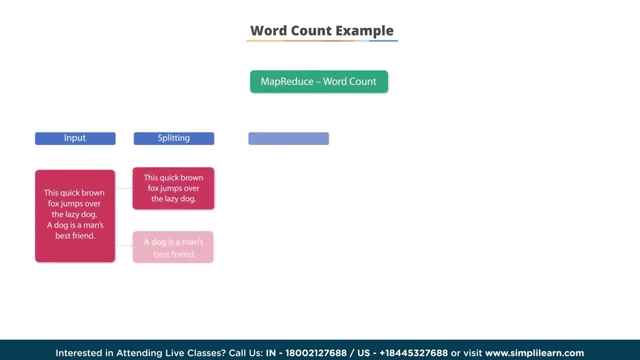 ballot count. it could take a month to receive the election results. when many people count the ballot papers simultaneously, the results are obtained in one or two days. this is how map reduce works. let's look at a word count example. in this screen, the map reduce operation is explained using a real 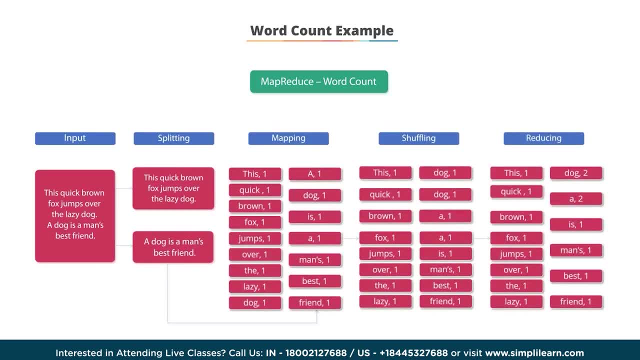 time problem. the job is to perform a word count of the given paragraph. on the left, the sentence in input says: the quick brown fox jumps over a lazy dog and a dog is a man's best friend. we will then take this sentence through the corresponding steps of splitting mapping. 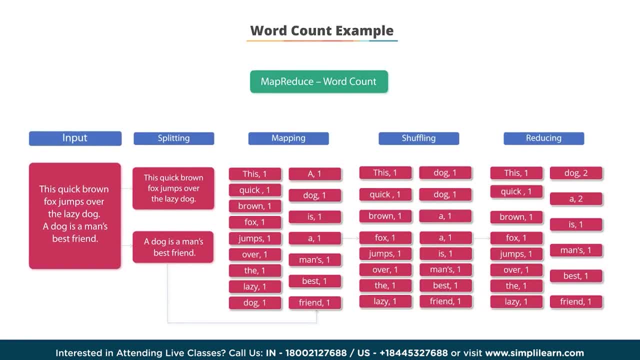 shuffling and reducing. the map reduce process then begins with the input phase, which refers to providing data for which the map reduce process is to be performed. the sentence used is as input here. the next step is the splitting phase, which refers to converting a job submitted by the client into a number. 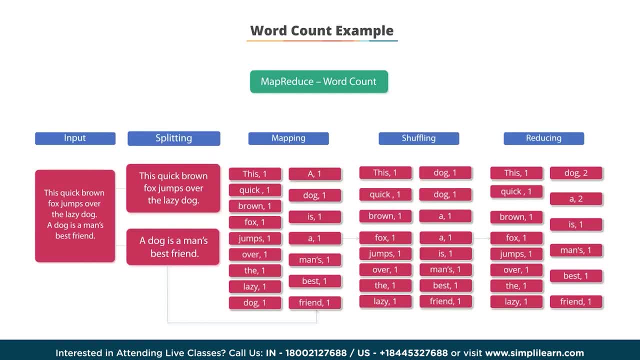 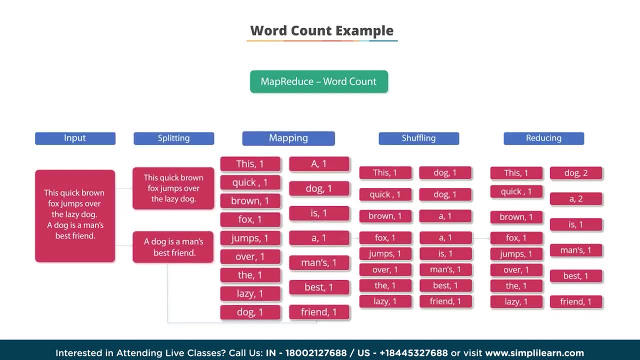 of tasks. in this example, the job is to split into two tasks, one for each sentence. then the mapping phase refers to generating a key value pair for the input. since this example is about counting words, the sentence is now split into words by using the substring method to generate. 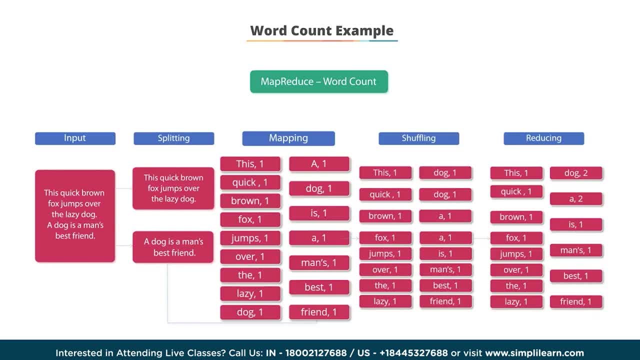 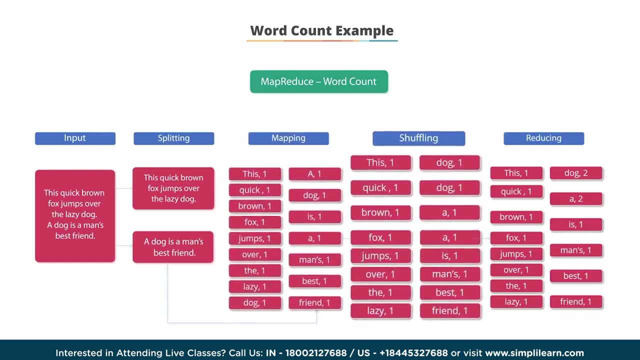 words from lines. the mapping phase will ensure that the words generated are each converted into keys and a default value of one is allotted to each key or each word in the sentence. in the next step, the shuffling phase, refers to sorting the data based on those keys. 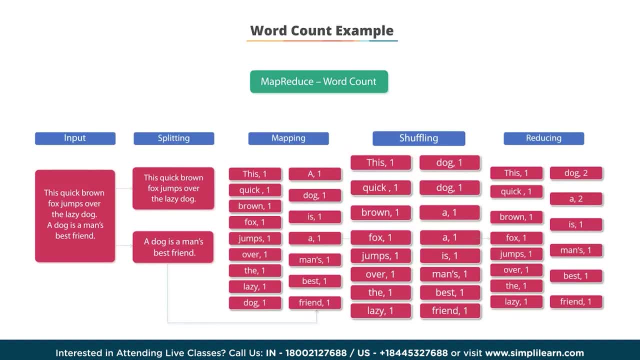 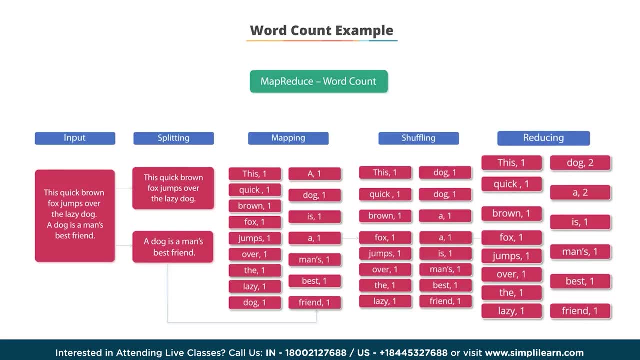 as shown on screen, the words sorted into ascending order. the last phase is the reducing phase. in this phase the data is reduced based on the repeated keys by incrementing the value of each key. where there's a duplicate word, the word dog and the letter a are repeated. 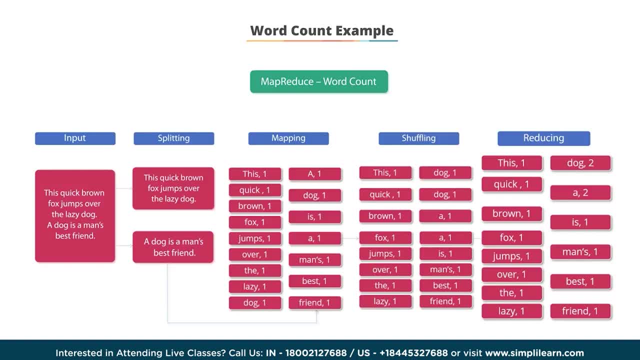 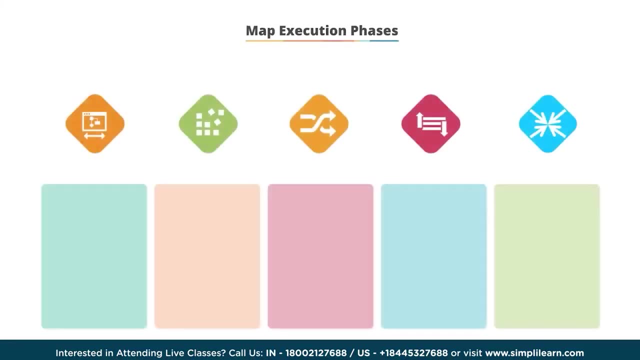 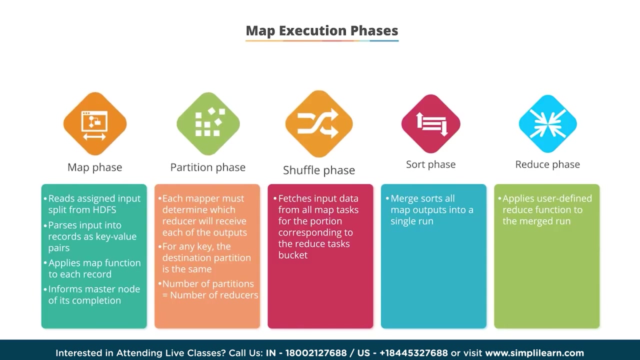 therefore, the reducer will delete the key and increase the value depending on the number of occurrences of the key. this is how the map reduce operation is performed. map execution phases. map execution consists of five phases: the mapping phase, the partition phase, the shuffle phase, the sort phase and the reduce. 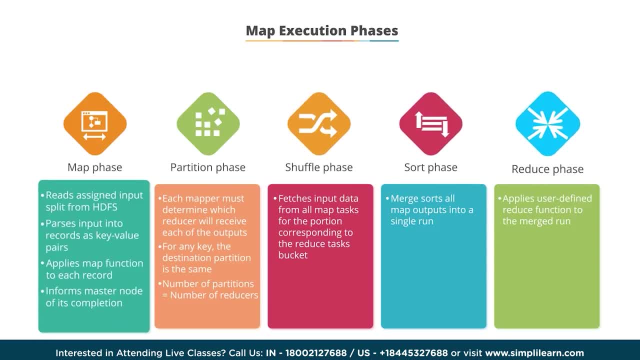 phase, the assigned input split is read from hdfs, where a split could be a file block by default. furthermore, input is parsed into records as key value pairs. the map function is applied to each record to return zero or more new records. these intermediate outputs are stored in the local file system as a 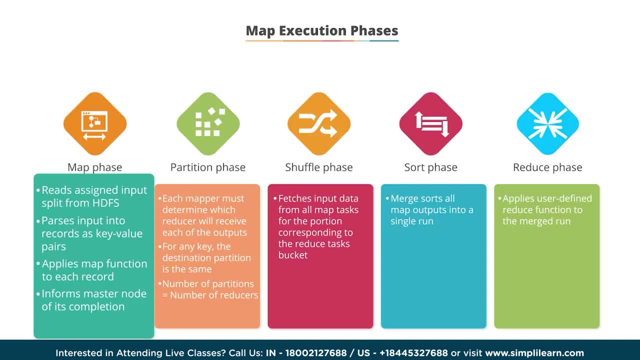 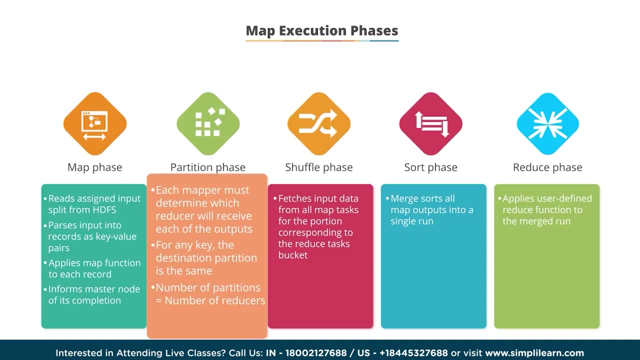 file. they are sorted first by bucket number and then by a key. at the end of the map phase, information is sent to the master node after its completion in the partition phase. each mapper must determine which reducer will receive each output for any key, regardless of which mapper instance generated it. 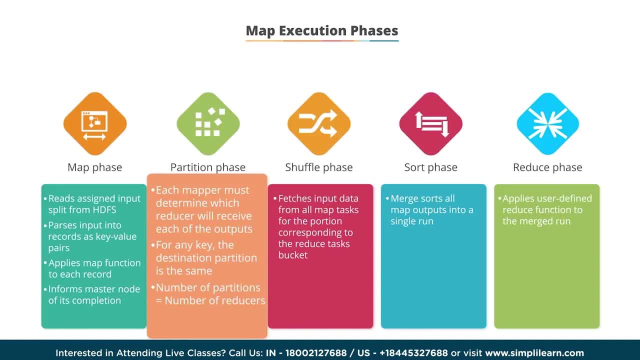 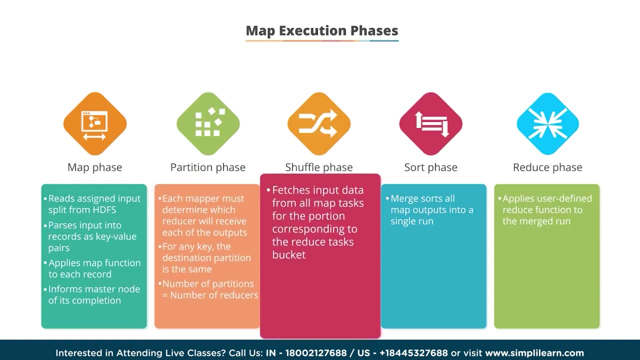 the destination partition is the same, so for a single word, that word would always go to the same destination partition. note that the number of partitions will be equal to the number of reducers. in the shuffle phase, input data is fetched from all map tasks for the portion corresponding to the reduced tasks. 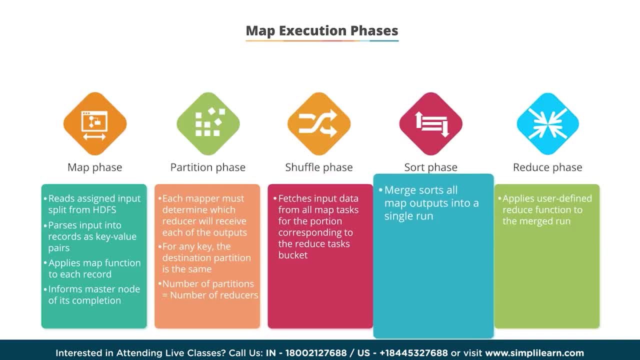 bucket. in the sort phase, a merge sort of all map outputs occurs in a single run. and finally, in the reduce phase, a user defined reduce function is applied to the merged run. the arguments are a key and the corresponding list of values. the output is written to a file. 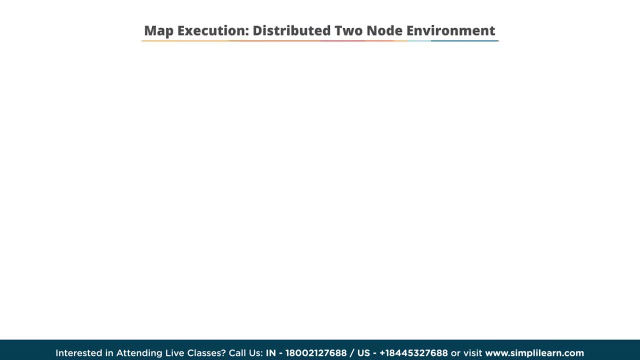 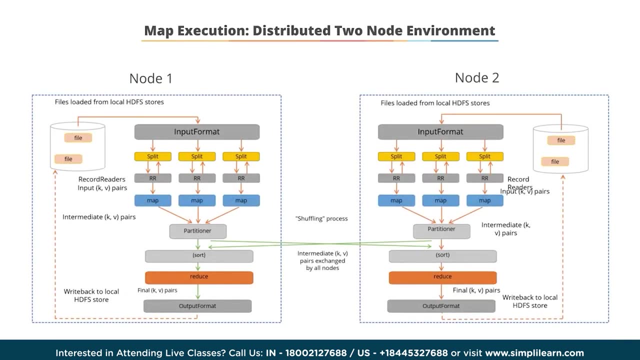 in hdfs map execution in a distributed two node environment. the mappers on each of the nodes are assigned to each input split a box based on the input format. the record reader reads the split as a key value pair. the map function is applied to each record to then return. 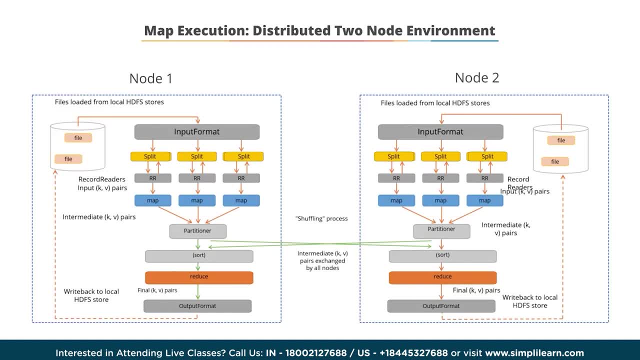 zero or more new records. these intermediate outputs are stored in the local file system. thereafter, a partitioner assigns the records to the reducer. in the shuffling phase, the intermediate key value pairs are exchanged by all nodes. the key value pairs are then sorted by applying the key and 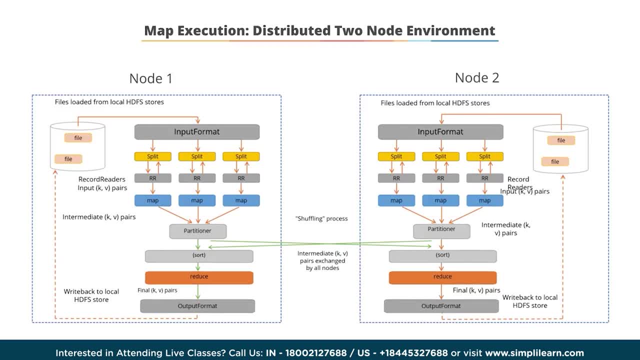 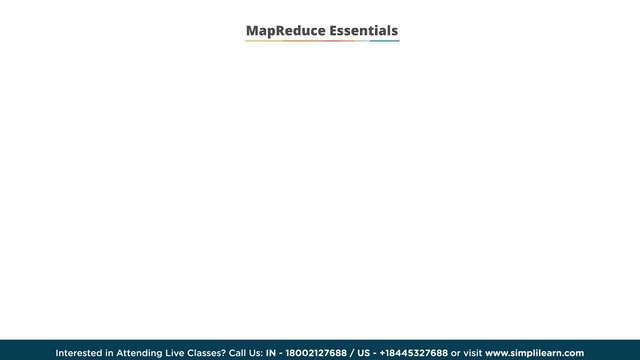 reduce function again. the output is stored in hdfs based on the specified output file format. the essentials of each map reduce phase are shown on the screen. the job input is specified in key value pairs. each job consists of two stages. first, a user defined map function is 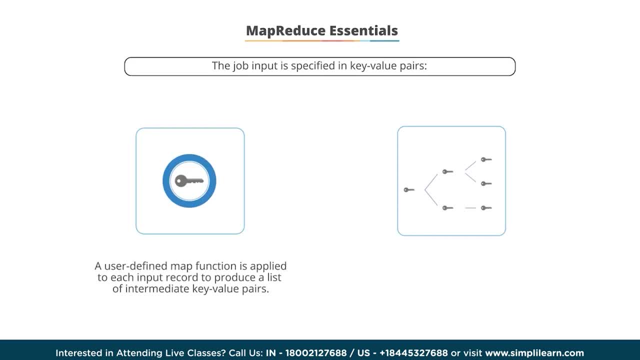 applied to each input record to produce a list of intermediate key value pairs. second, a user defined reduce function is called once for each distinct key in the map output. then the list of intermediate values associated with that key is passed. the essentials of each map reduce phase are as follows. 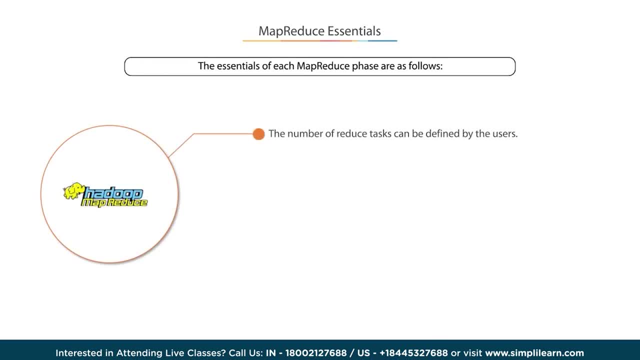 first, the number of reduced tasks can be defined by the users. second, each reduced task is assigned a set or record groups, that is, intermediate records corresponding to a group of keys. third, for each group, a user defined reduce function is applied to the recorded values and for the reduced tasks, are read. 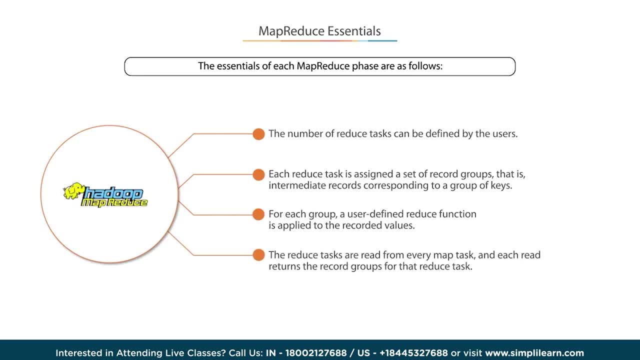 from every map task and each read returns the record groups for that reduced task. reduced phase cannot start until all mappers have finished processing. so combining your output is important step once all the tasks are completed. map reduce job. a job is a map reduce program that causes. 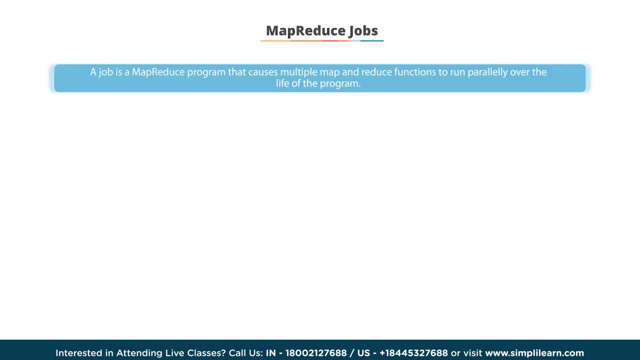 multiple map and reduce functions to run parallelly over the life of the program. many copies of map and many copies of reduce functions are worked for parallel processing across the input data set. a task is a map or reduce function executed on a subset of this data. with this understanding of job, 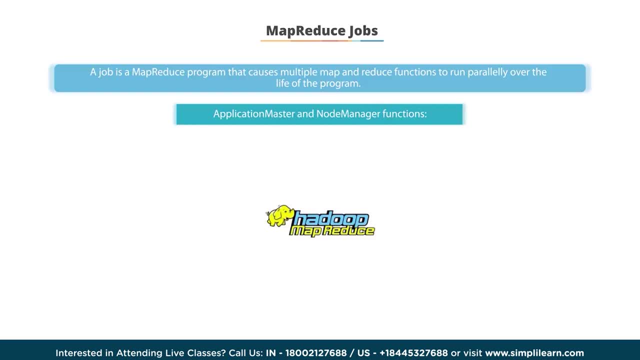 and task. the application master and node manager functions become easier to comprehend. first, the application master is responsible for the execution of a single application or map reduce job. it defines the job request into tasks and assigns those tasks to node managers running on one or more slave nodes. the 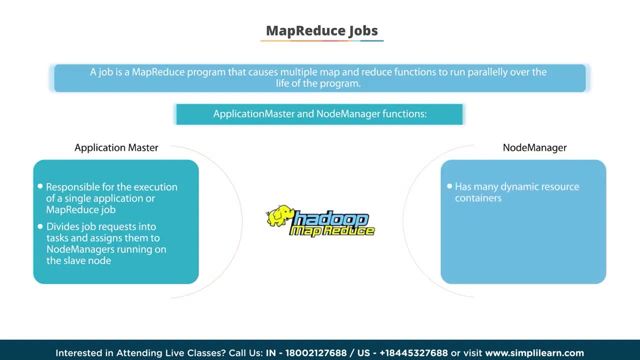 node manager has a number of dynamically created resource containers. the size of a container depends on the amount of resources it contains, such as memory, cpu disk and network io. it executes map and reduce tasks by launching these containers when instructed to by: the map reduce application master map reduce and associated. 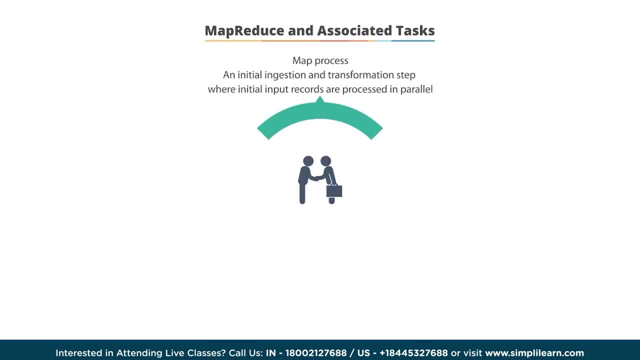 tasks. the map process is an initial step to process individual input records in parallel. the reduced process is all about summating the output with a defined goal as coded in the business logic. the node manager keeps track of individual map tasks and can run in parallel. a map job runs as a part of a 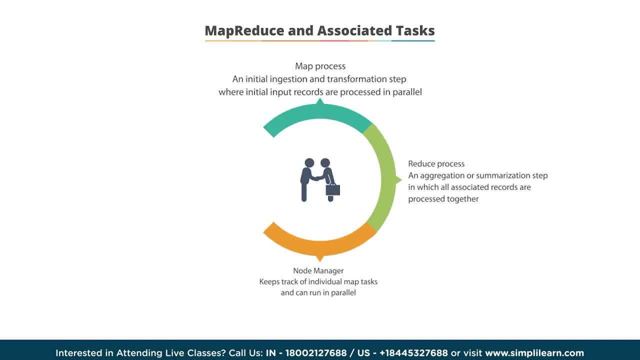 container execution by node manager on a particular container and runs in parallel. in parallel, a particular data node within a cluster. the application master keeps track of a map- reduce job, the hadoop map- reduce job work interaction. initially, a hadoop map reduce job is submitted by a client. 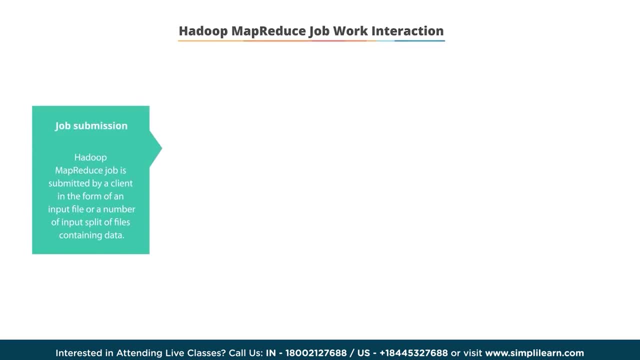 in the form of an input file or a number of input splits of files, each containing data. the map reduce application master will then distribute the input split to separate node managers. the map reduce application master then coordinates with those node managers. the map reduce application master will now 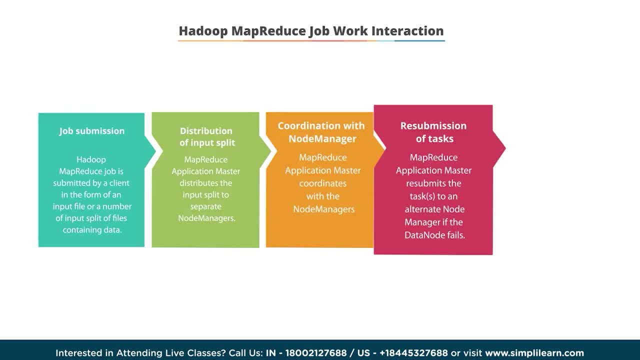 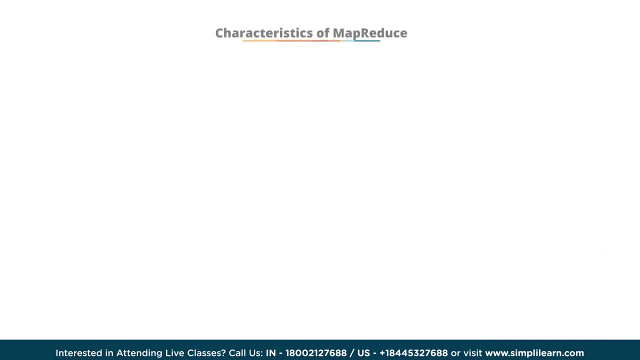 resubmit the task to an alternate node manager if that data node should fail. the resource manager gathers the final output and informs the client of success or failure status. let's look at the characteristics of map reduce. map reduce is designed to handle very large-scale data in the range of 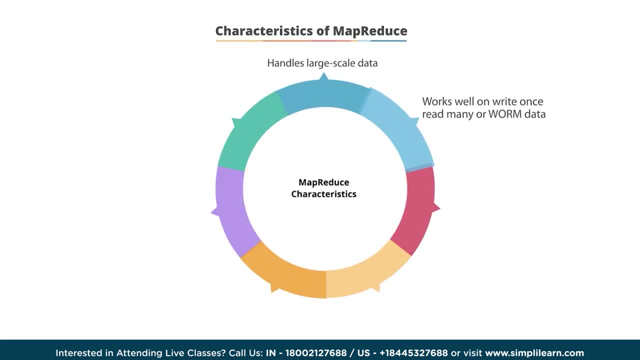 petabytes and exabytes. it works well on write once and read many data sets, also known as worm data map. reduce allows parallelism without mutexes. the map and reduce operations are performed by the same processor. those operations are provisioned near the data as data locality is preferred. 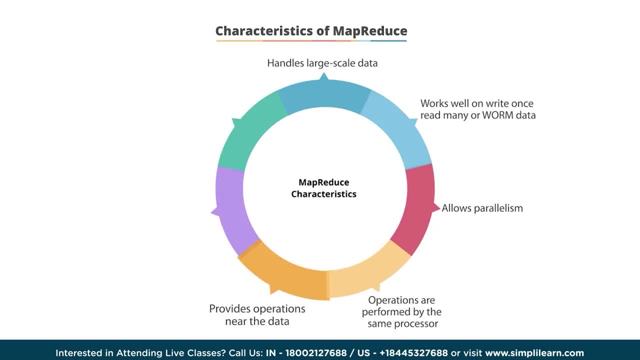 in other words, we will move the application to the data and not the other way around. commodity hardware and storage is leveraged in map reduce to keep things cost effective, and the runtime takes care of splitting and moving data for operations. some of the real-time uses of map. 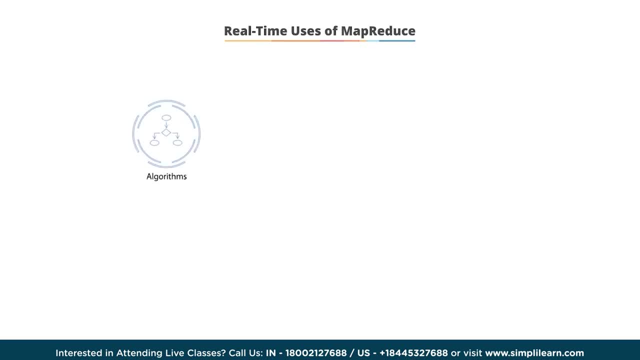 reduce are as follows: simple algorithms, such as grep text indexing and reverse indexing, such things as data intensive computing, which would include sorting large and small sets of data, stream data and structured data. data mining operations, such as bayesian classification, which you'll study later. and search engine operations, such as 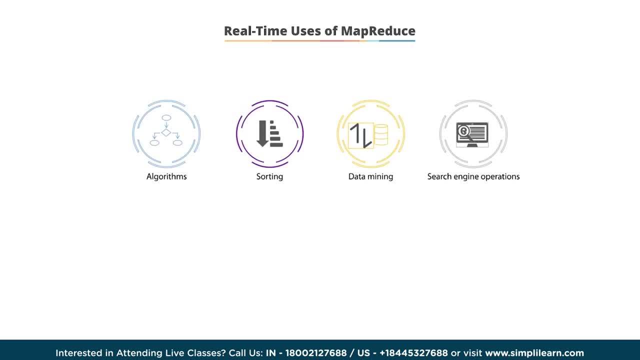 keyword indices, ad rendering and page ranking. enterprise analytic analytics to ensure the business is operating smoothly and with the best decision making data available. gaussian analysis for locating extraterrestrial objects in astronomy, which uses very large data sets. and semantic web and web 3.0 indices and operations, such as: 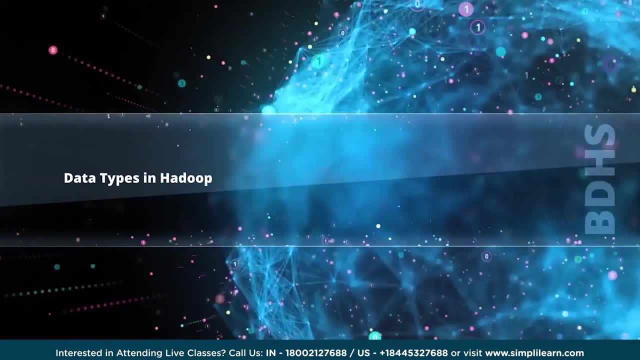 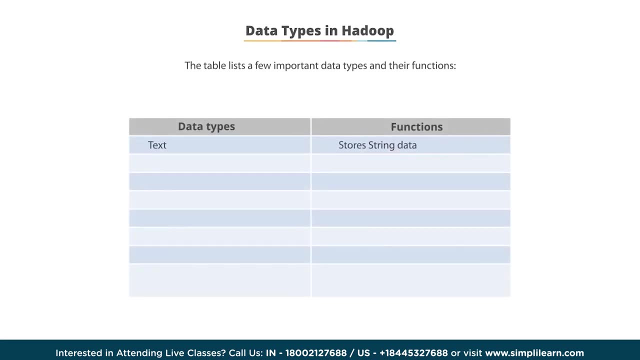 data types in hadoop. data types in hadoop. the first data type is text. the function of this data type is stored to string data. the int writable data type stores integer data. long writable, as the name suggests, stores long data. similarly, other data types are float writable for storing float data. 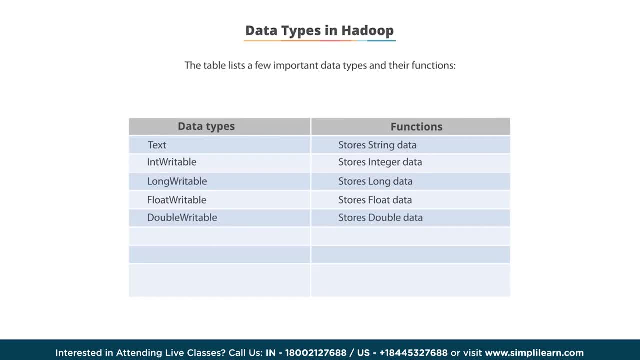 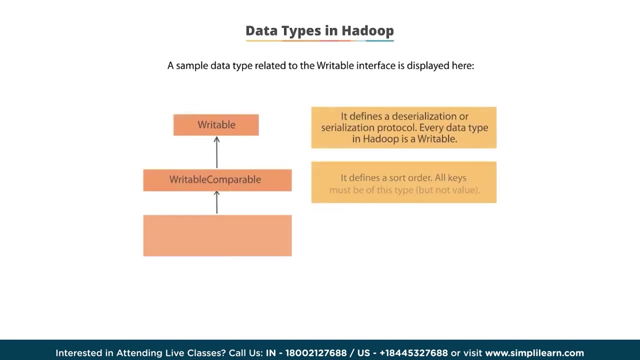 and double writable for storing double data. there is also boolean writable for storing multiple and byte writable data types. null writable is a placeholder when a value is not needed. this illustration here shows a sample data type that you can create on your own. this data type will need you to implement. 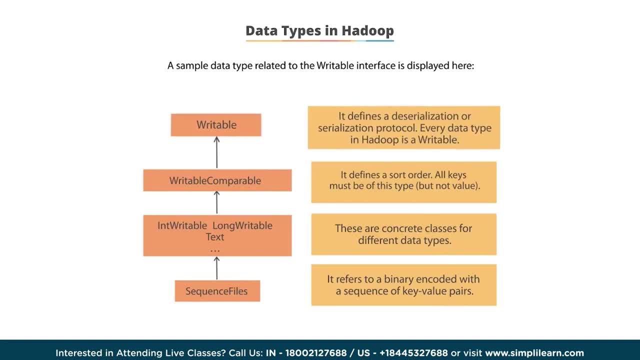 a writable interface. as you can see, writable will define a deserialization or serialization protocol. every data type in hadoop is a writable. writable, comparable, will define your sort order. all keys must be of this type, but not value. then int, writable and long writable and the various concrete classes. 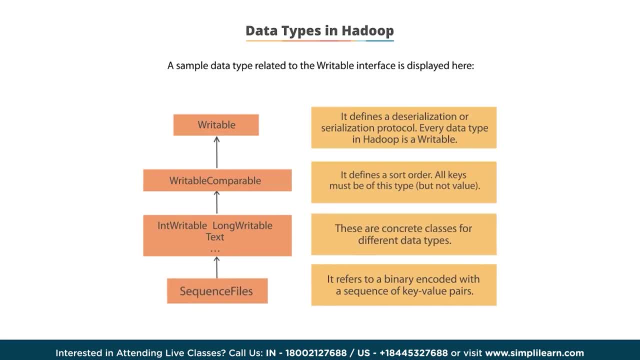 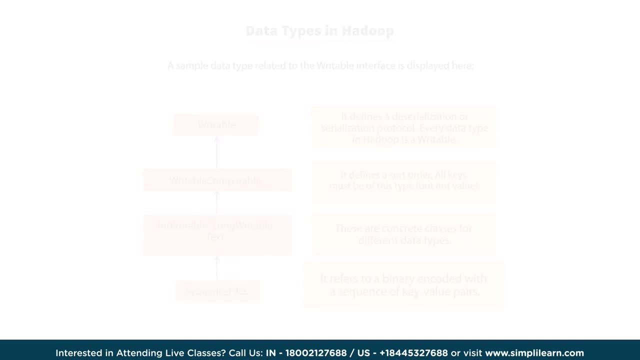 that you'll define for your different data types. lastly, sequence files refers to a binary encoded with a sequence of key value pairs. input format in mapproduce. mapproduce can specify how its input is to be read by defining an input format. the table lists some of the 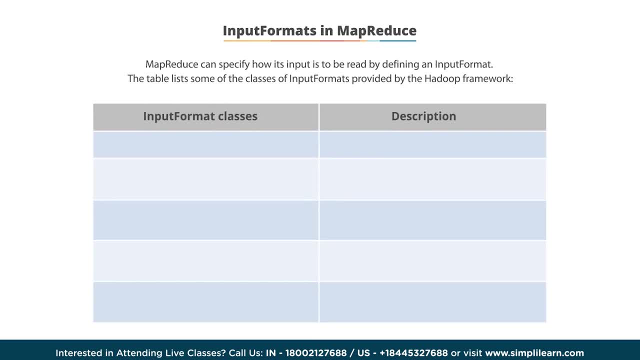 classes of input formats provided by the hadoop framework. let's look at each of them. the first class is key value text input format, which is used to create a single key value pair per line text input format is used to create a program that considers a key as the line number. 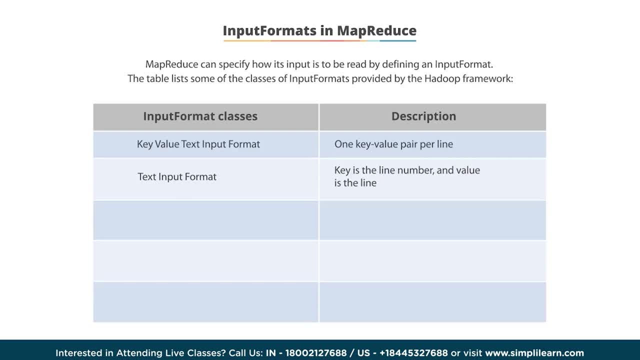 and a value as the line itself. nline input format is similar to text input format, except that there are n number of lines that make an input split. multi file input format is used to implement an input format that aggregates multiple files into one split format to be implemented. 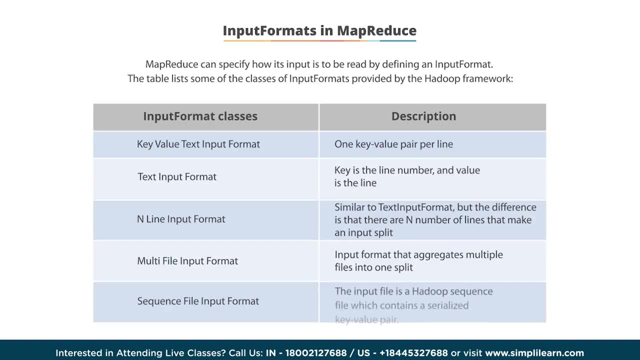 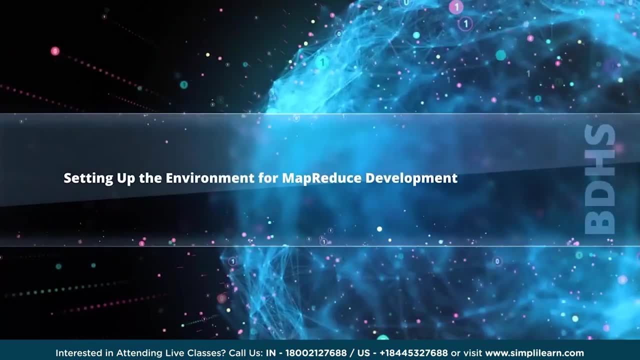 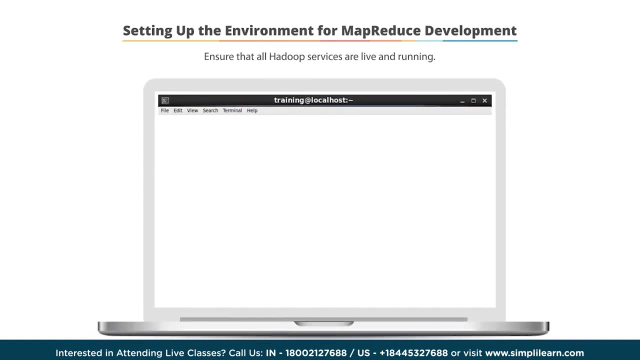 the input file must be a hadoop sequence file which contains serialized key value pairs. we set the environment for mapproduce development. first. let's ensure that all hadoop services are live and running. this can be verified in two steps. first, use the command jps. 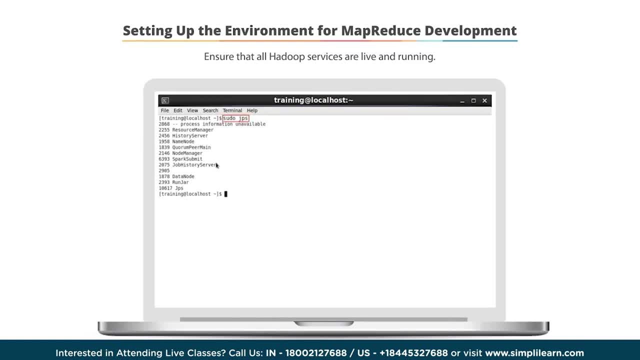 as shown- type: sudo, jps- and then look for all five services that you need: node, data node, node manager, resource manager and secondary name node. maybe additional services that are used by a hadoop cluster, but these are the ones that we require as core services. next look: 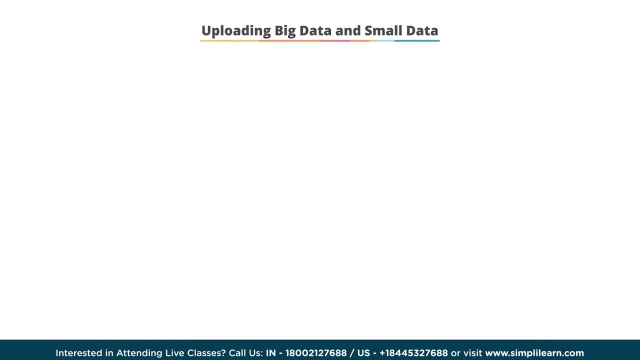 let's look at uploading big data and small data. the command to upload any data, big or small, from the local file system to hdfs is hadoop fs copy from local and then the source file address and the destination file address. now let's look at the steps of. 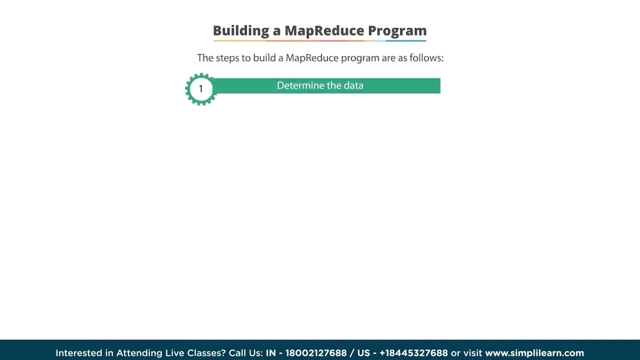 building a mapproduce program, first determine if the data can be made parallel and solved by using mapproduce. for example, you need to analyze whether the data is write once, read many or worm type data in nature. then design and implement a solution as a mapper and then 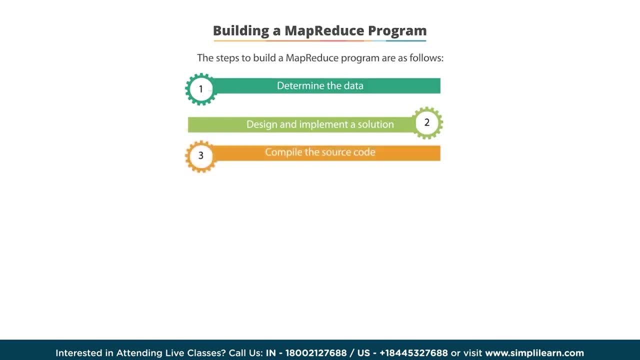 reducer class within your code. compile the source code with hadoop core and package the code as a jar executable. configure the application job as the number of mapper and reducer tasks and to the number of input and output streams, then load the data or use it on previously available data and 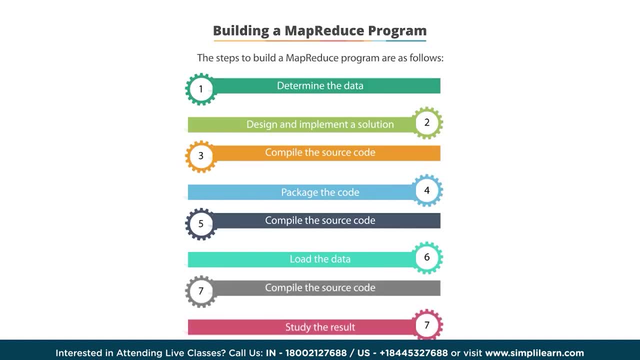 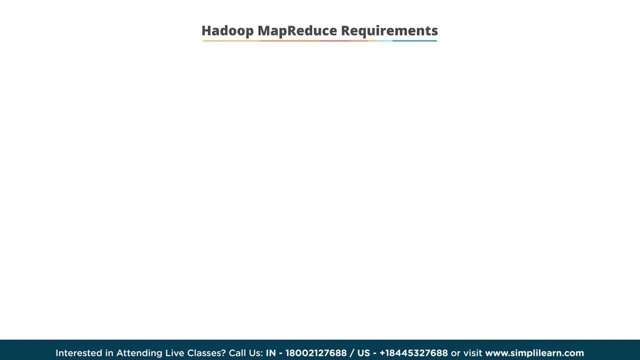 then launch and monitor the job. you can then study the results and repeat any of the previous steps as needed. the hadoop mapproduce requirements. the user or developer is required to set up the framework with the following parameters: the locations of the job input in the. 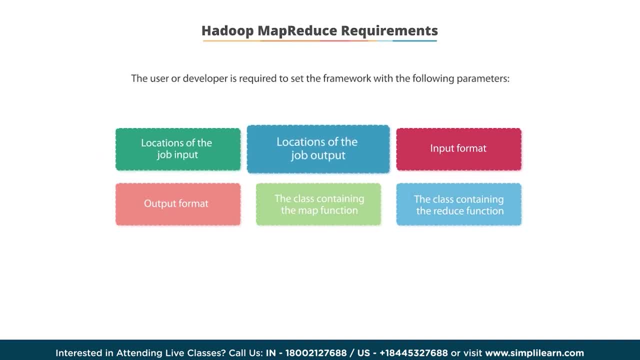 distributed file system. the location of the job output in the distributed file system. the input format to use. the output format to use. define a class containing the map function and then a separate class containing the reduce function, which is optional. if a job does not need a reduce function, there is no need. 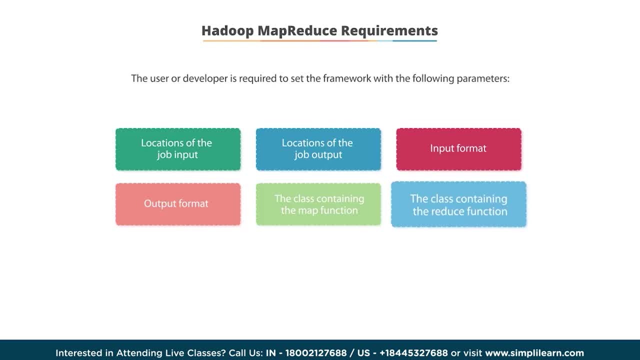 to specify a reducer class in your code. the framework will partition the input schedule and execute map tasks across the cluster if requested. it will sort the results of the map task and it will execute the reduced tasks with the map output. the final output will be moved to the output. 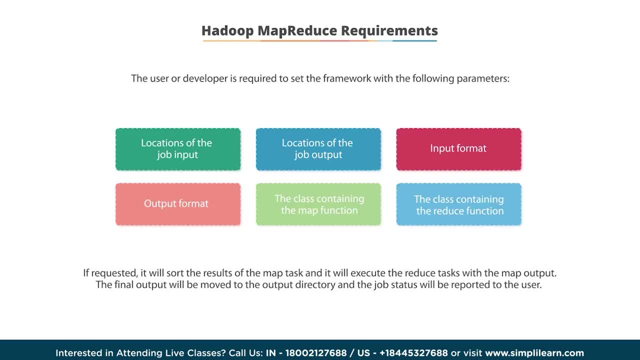 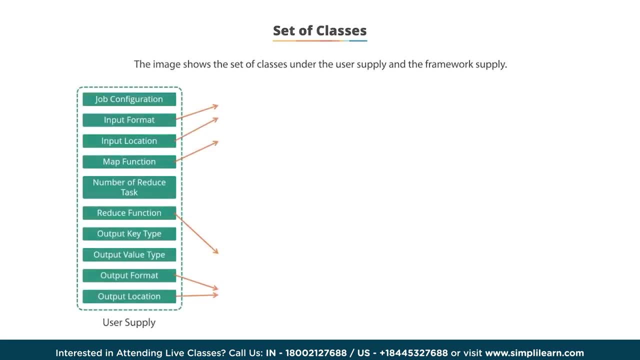 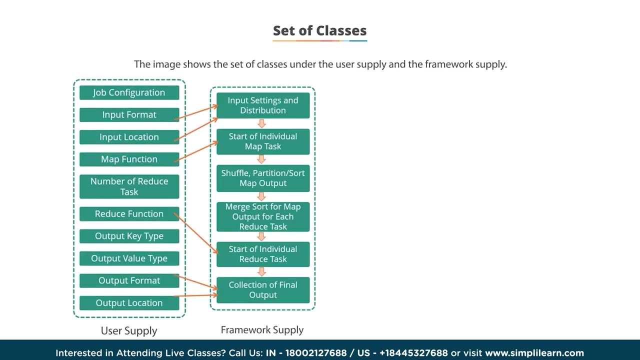 directory and the job status then reported to the user set of classes. this image shows the set of classes under the user supply and the framework supply. the user supply reverts to the set of java classes and the methods provided to a java developer for developing hadoop map. reduce applications. 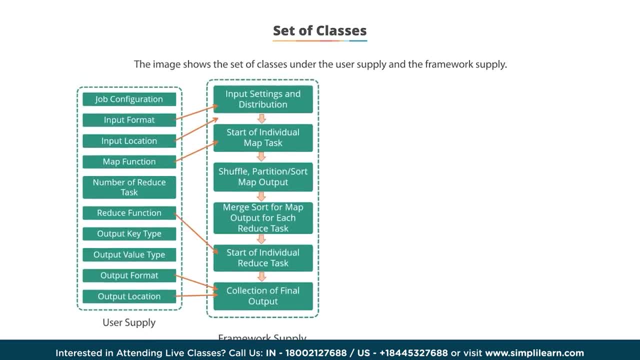 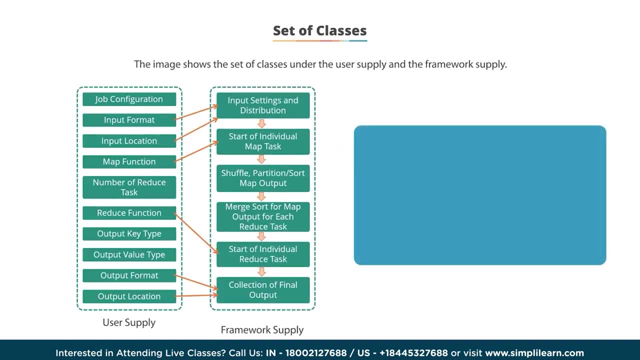 the framework supply refers to defining the workflow of a job which is followed by all hadoop services. as shown in the image, the user provides the input location and the input format as required by the program logic. once the resource manager accepts the input, a specific job is divided into tasks by the 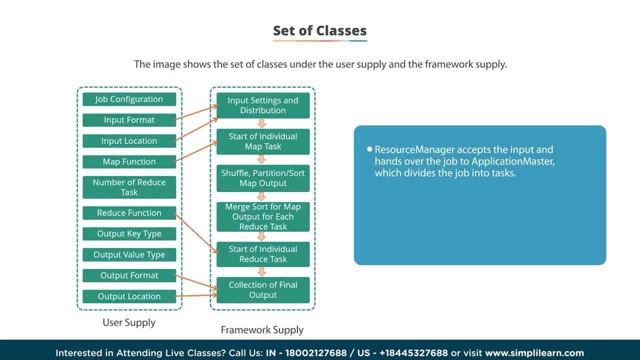 application master. each task is then assigned to an individual node manager. once the assignment is complete, the node manager will start the map task. it performs shuffling, partitioning and sorting for individual map outputs. once the sorting is complete, the reducer starts the merging process. this is also called the reduce. 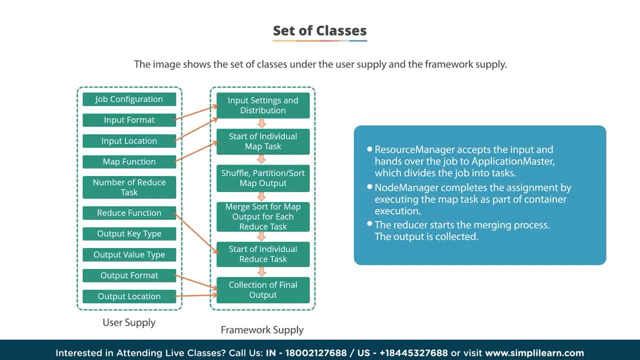 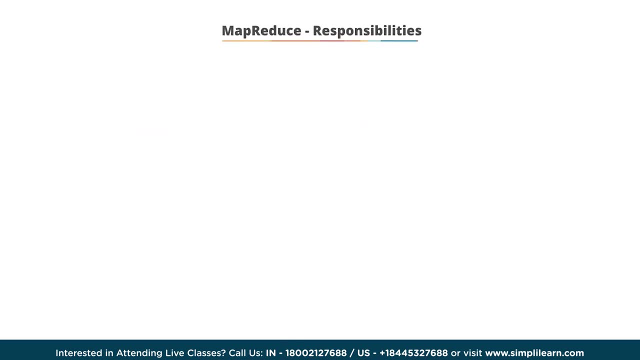 task. the final step is collecting the output, which is performed once across all the individual tasks once they're completed. this reduction is based on programming logic. let's look at map reduce responsibilities. the basic user or developer responsibilities of map reduce are: one: setting up the job. two: 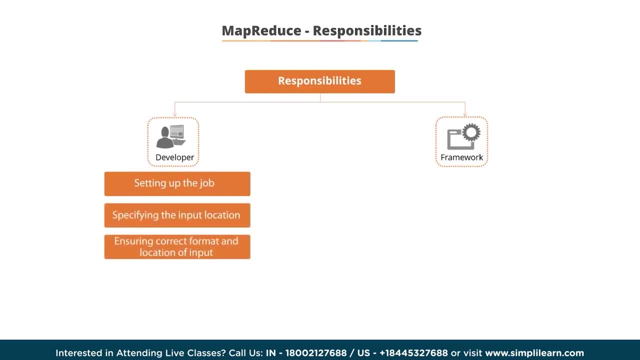 specifying the input location. and three, ensuring that the input is in the expected format and location. the framework responsibilities of map reduce are: distributing jobs among the application master and node manager, nodes of the cluster running the map operation, then performing the shuffling and sorting operations. next are the optional 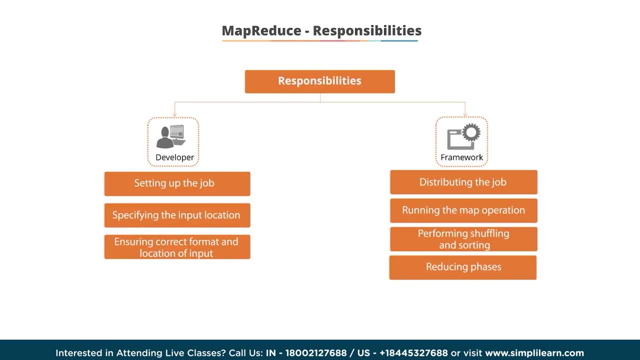 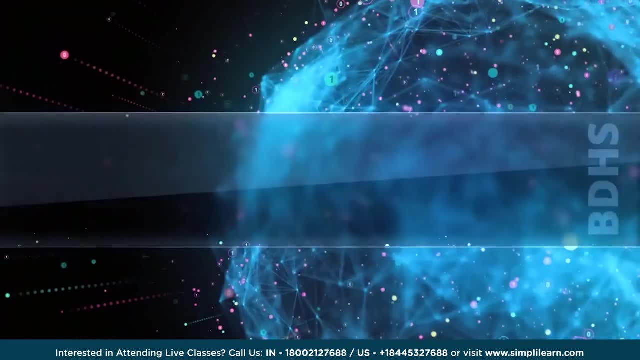 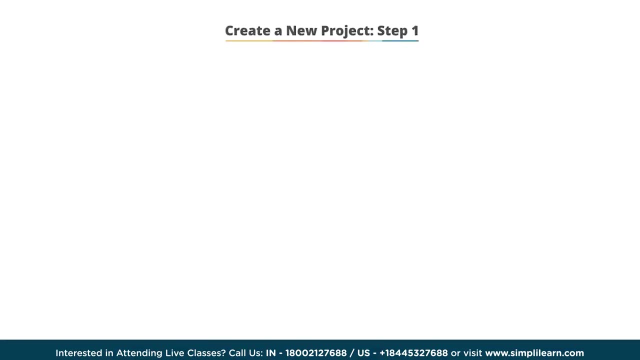 reducing phases and finally placing the output in the output directory and informing the user of the job completion status. create a new project- the. let's see how we would create a new project. first, make sure eclipse is installed on your system. once it's installed, you can create a new project. 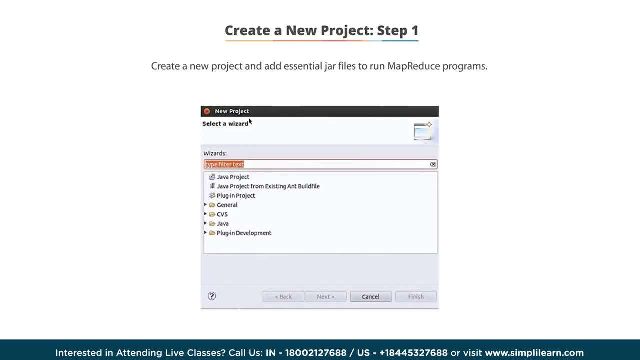 and add the essential jar files to run a map. reduce program. then to create a new project, click the file menu, select new project or alternatively press control n to start the wizard of a new eclipse project. the screen shows a new project and select wizard options for the 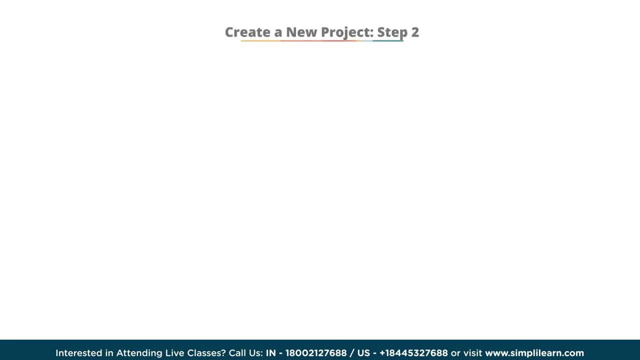 first step. in step number two, you would select a java project from the list, then click the next button to continue. step three: the newly created project has to have a name. in this case, we'll type the project name as word count and click the next button to continue. 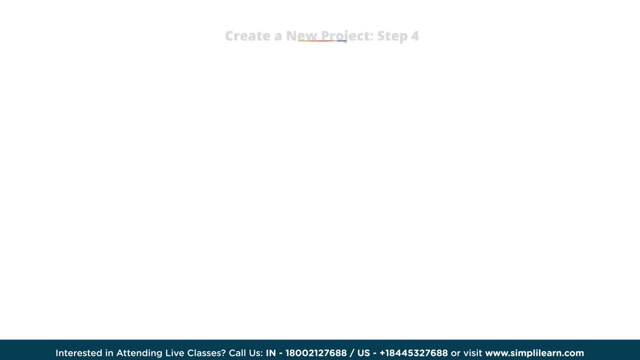 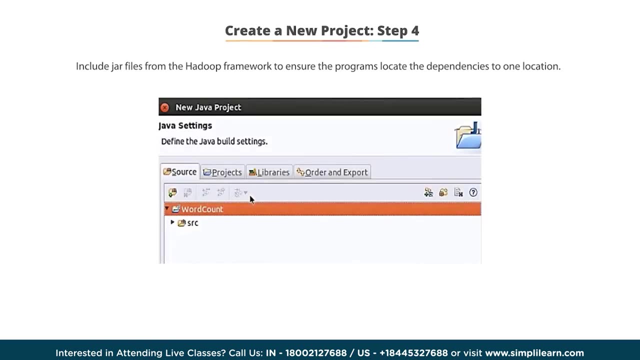 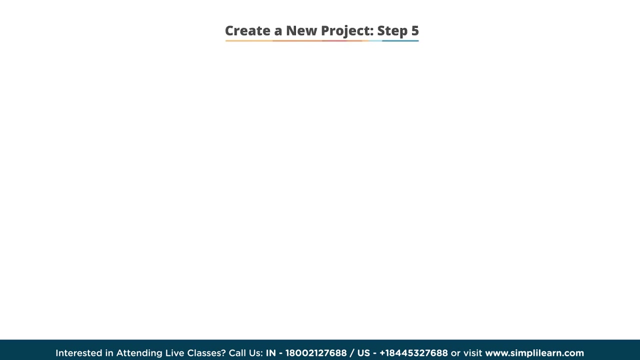 in step number four, we'll create a new project. in step four of your new project, you will now include jar files from the hadoop framework to ensure that the programs locate the dependencies to one location. and in step number five, you will add the essential jar files. 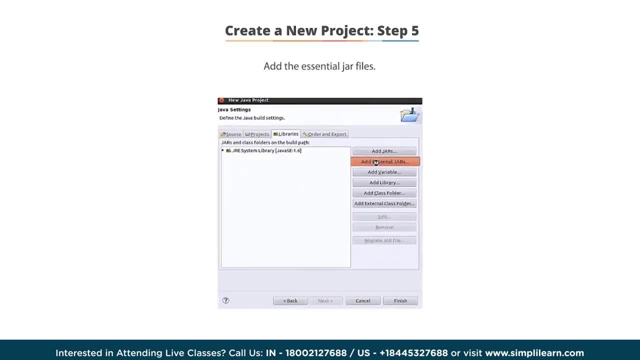 to locate these, go to the libraries tab and click the add external jars button to add the essential jar files. after adding the jar files, click the finish button to complete the project successfully. next we'll check the hadoop environment to ensure we have map reduce. it is important to check whether 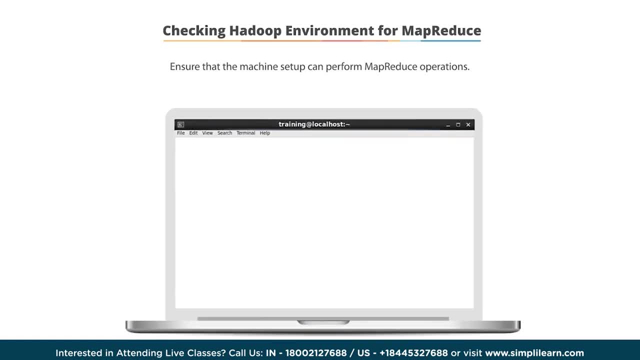 the machine setup can perform map reduce operations. to verify this, use the example jar files that are deployed by a hadoop installation. this can be run by running the command shown on the stream. before executing this command, ensure that the words dot txt file resides in the data slash first location. 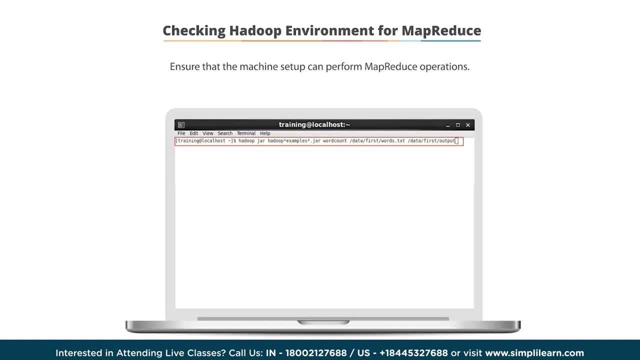 in the on screen example you see the hadoop jar command being executed. passing it, the hadoop examples: dot jar file set word count and then data slash. first slash words dot txt as the input and data slash first slash output as the selected output. advanced map reduce. 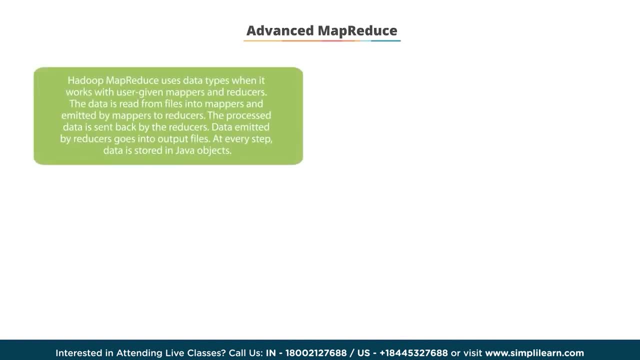 hadoop map reduce uses data types to work with user given mappers and user given reducers. the data is read from files into the mapper and emitted by mappers to the reducers. the processed data is sent back by the reducers. data emitted by reducers goes into output files at. 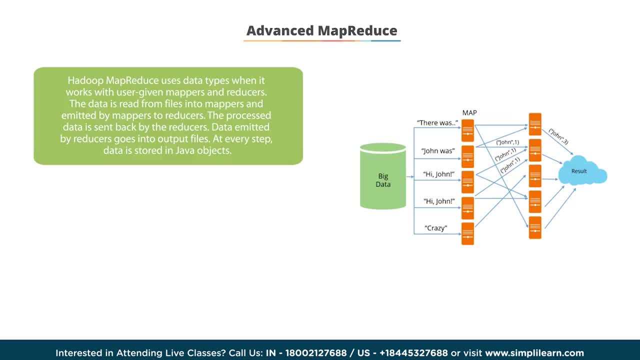 every step data is stored in java objects. let's now understand the writable data types in advanced map reduce. in the hadoop environment, all input and output objects across the network must obey the writable interface which allows hadoop to read and write data in a serialized form for transmission. 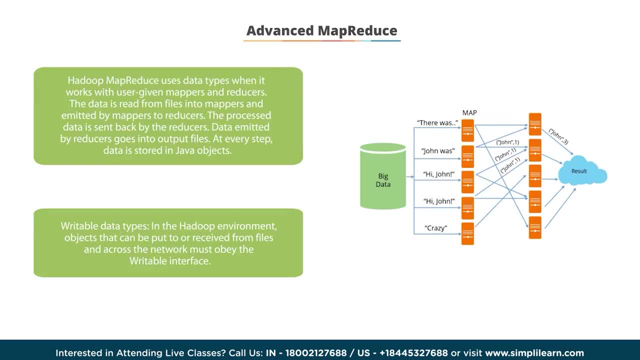 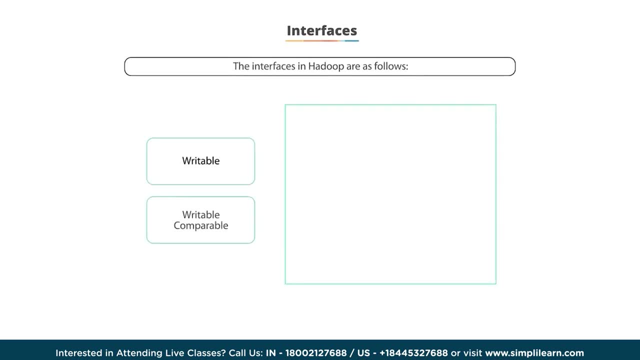 let's look at hadoop interfaces in some more detail. the interfaces in hadoop are writable and writable- comparable, as you've already seen. a writable interface allows hadoop to read and write data in a serialized form for transmission. a writable interface consists of two methods: read and write fields. 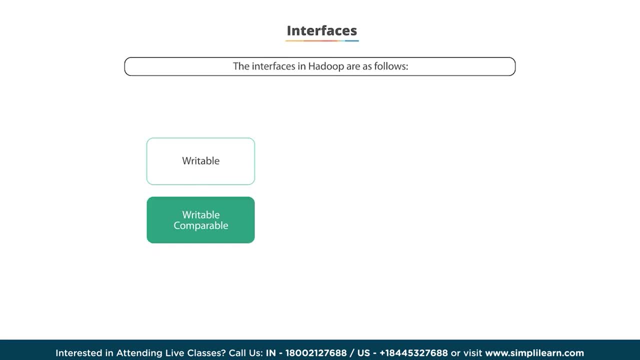 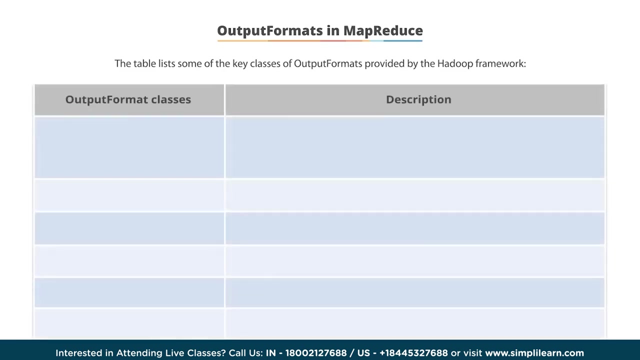 a writable comparable interface extends the writable interface so that the data can be used as a key and not as a value, as shown here. the writable comparable implements two methods: compareTo and hashCode output formats in mapper. now that you've completed the input formats in mapper, let's look into the classes for the. 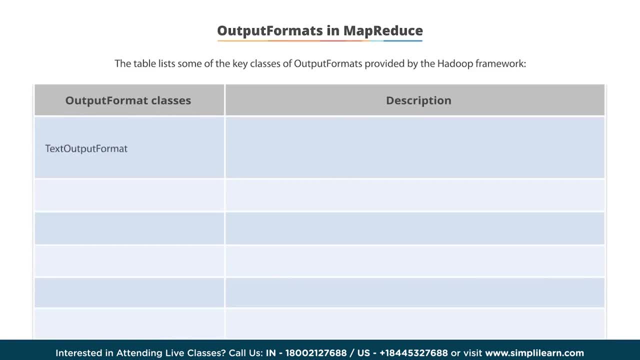 MapReduce output format. the first class is default output format, which is text output format. it writes records as lines of text. each key value pair is separated by a tab character. this can be customized by using the MapReduce text output format dot separator property. the corresponding input format is key value. 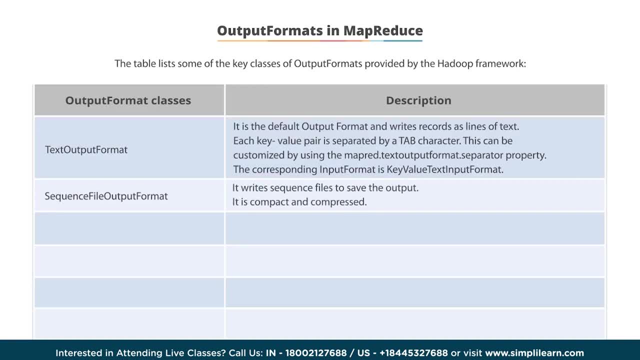 text input format. sequence file output format writes sequence files to save on output space. this represents a very compact and compressed version of normal data blocks. sequence file, as binary output format, is responsible for writing key value pairs that are in raw binary format into a sequential file container. 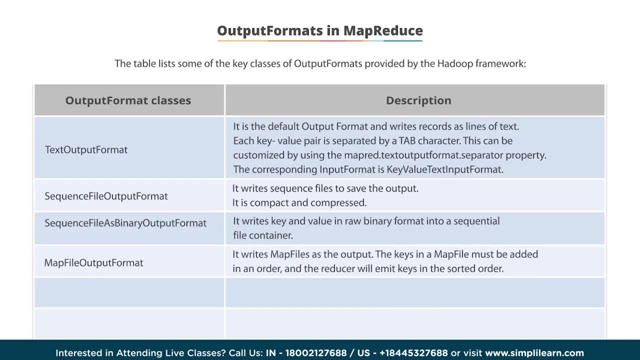 and map file output format writes map files as the output. the keys in a map file are added in a specific order. the reducer then emits keys in that sorted order. multiple text output format writes data to multiple files whose names are derived from the output keys and values. 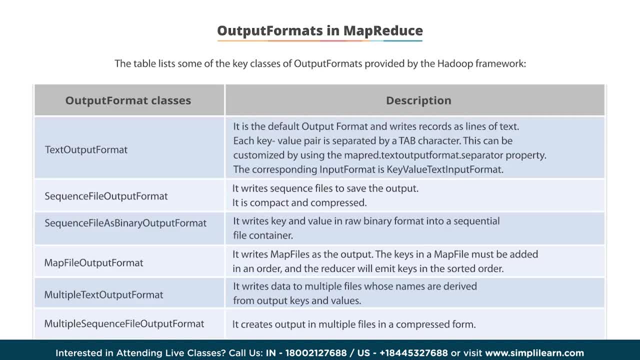 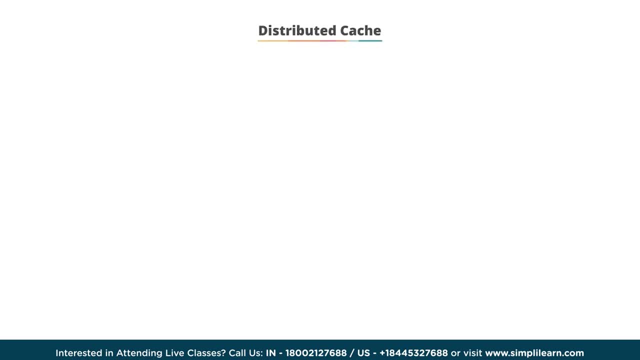 sequence file output format creates output in multiple files in a compressed form. let's look at distributed caching. a distributed cache is a Hadoop feature to cache files that are needed by the applications. a distributed cache will help boost efficiency when a map or reduced task needs access. 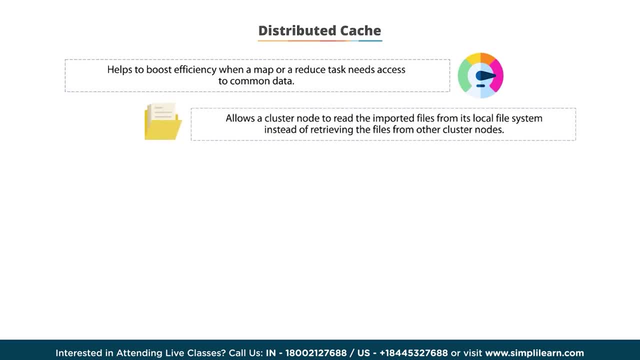 to common data. it allows a cluster node to read the imported files from its local file system instead of retrieving the files from other cluster nodes in the environment. it allows both single files and archives such as zip and targz. it copies files only to slave nodes. if there are no slave nodes, 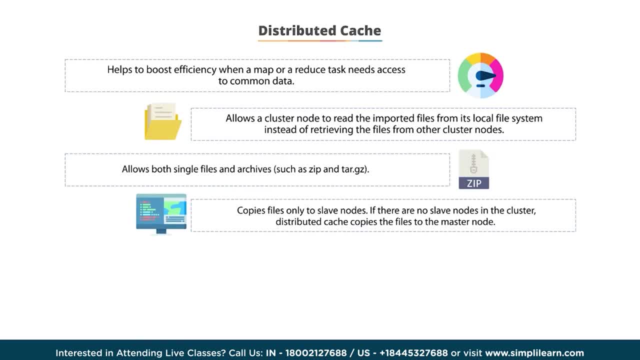 in the cluster, then distributed cache copies the files to the master node. it allows access to the cached files from mapper or reducer applications to make sure that the current working directory is added into the application path and allows referencing of the cached files as though they were present in the current working. 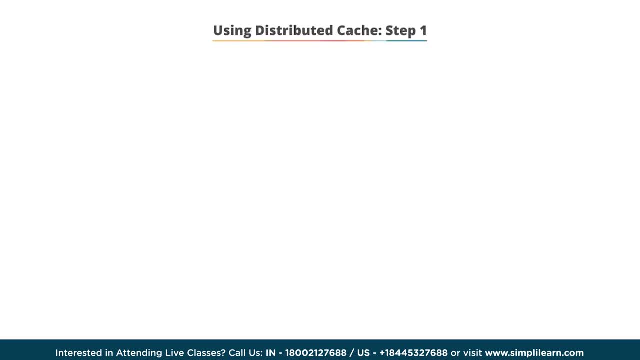 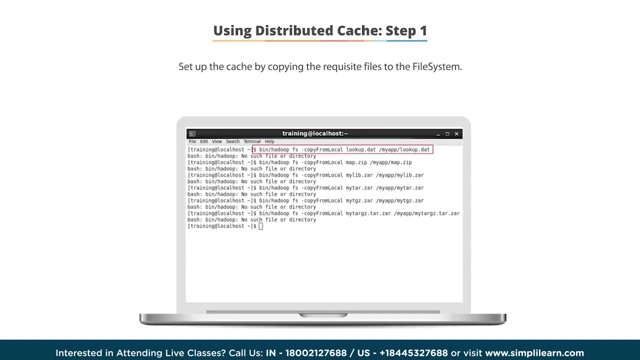 directory, vastly speeding up access using distributed cache. step one first set up the cache by copying the requisite files to the file system as shown here. here we see a bin slash Hadoop FS command using a dash copy from local of the file lookup dot dat to HDFS. 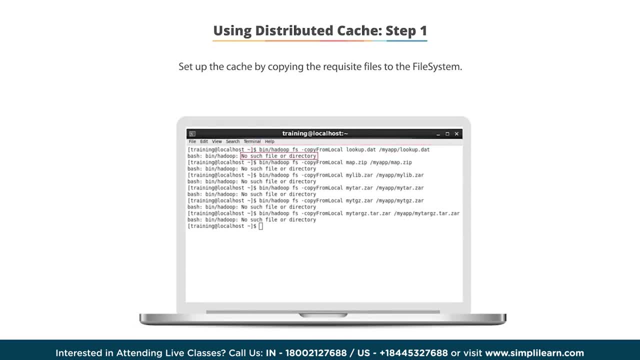 myapp slash lookup dot dat. this shows us that there is currently no file or directory of that name. the Hadoop FS copy from local remember will take a file from your local file system and place it in the target directory within the HDFS file system using distributed cache. 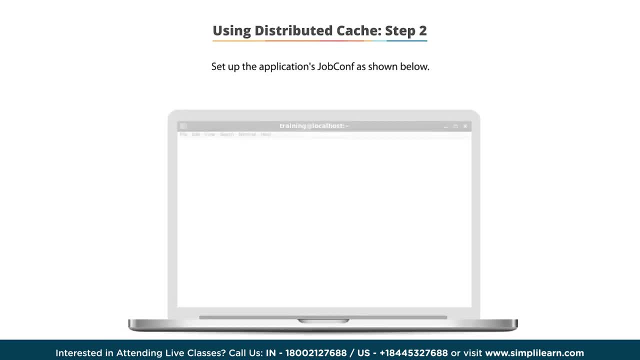 step two: set the application job conf as shown in the example. in this case, we are setting up a new instance of job. by creating a new instance of job conf, we then will call a distributed cache, add cache file method and create a new URI specifying the location, in this case myapp. 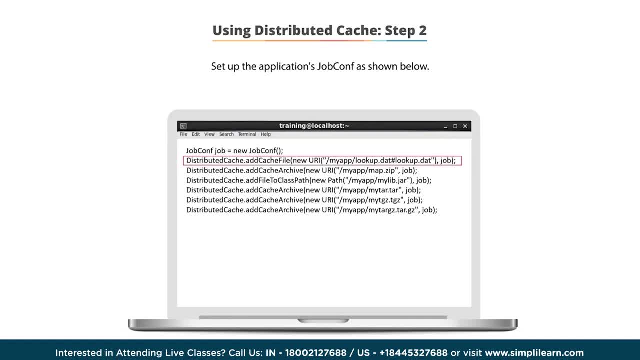 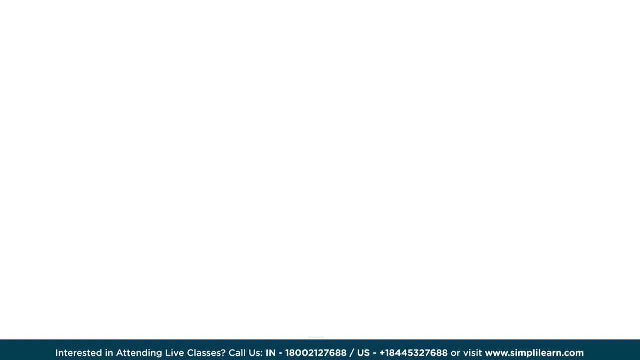 lookup dot dat with the file name of lookup dot dat. in the same way, each of the different commands here shows you creating a cache entry for zip files, jar files, tar files, tgz and gz files. in step three of setting up your distributed cache, you will use the cache files in the 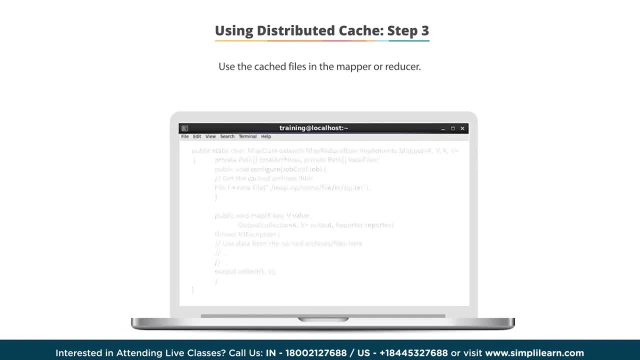 mapper or reducer class that you create. once the private path and configure information is in your program, you simply declare an instance of file called f, specifying the new file along with the parameter of dot, map, dot, zip, slash- some file in zip dot text. this will map your. 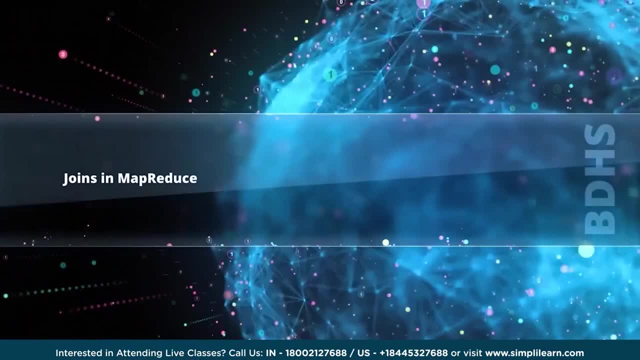 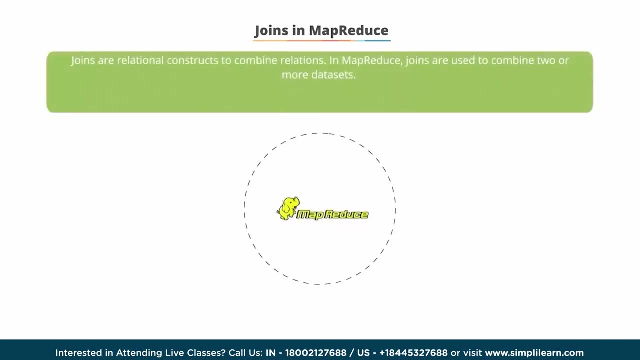 file into the distributed cache. joins in mapper reduce joins are relational constructs that can be used to combine. relations in mapper reduce joins are applicable in situations where you have two or more data sets you want to combine. a join is performed either in the map phase or later on. 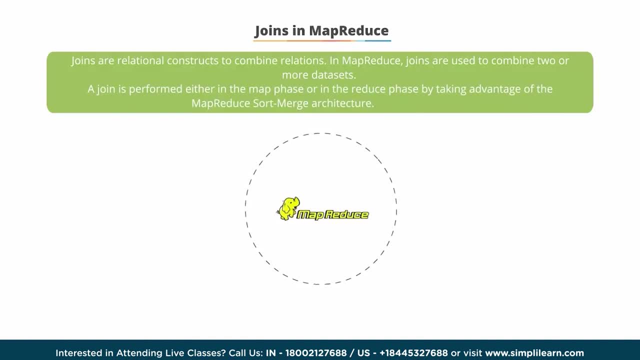 in the reduce phase by taking advantage of the mapper reduce sort, merge architecture. the various join patterns available in mapper reduce are reduced side join, replicated join, composite join and cartesian product. a reduced side join is used for joining two or more large data sets with the same foreign key, with any. 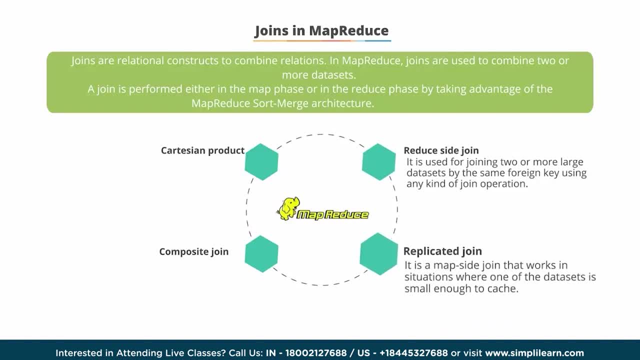 kind of join operation. a replicated join is a map side join that works in situations where one of the data sets is small enough to cache. that's vastly improving its performance. a composite join is a map side join used on very large formatted input data sets sorted and partitioned. 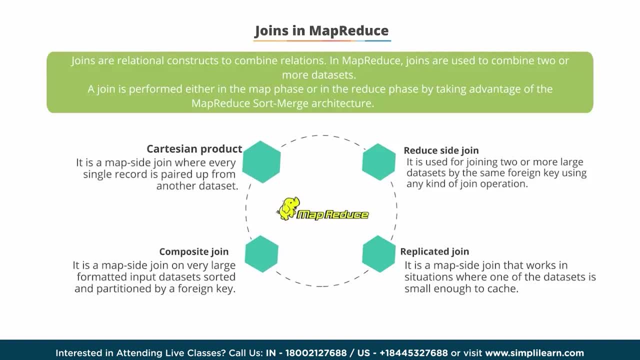 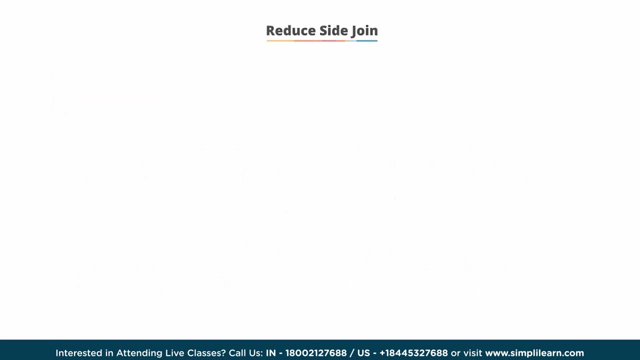 by a foreign key. and lastly, a cartesian product is a map side join where every single record paired up with another full data set. this style of join typically takes a significantly longer period of time to execute. a reduced side join works in the following ways: the mapper first prepares. 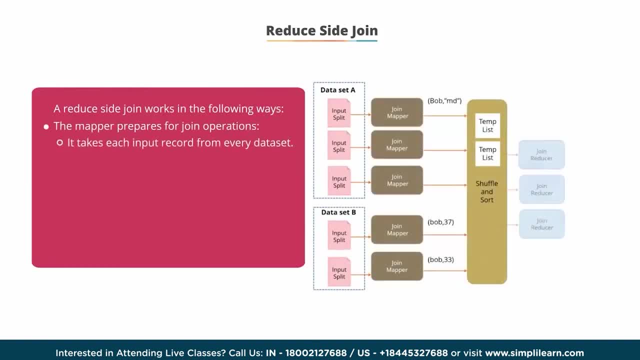 for join operations. it takes each input record from every data set and emits a foreign key record pair. the reducer then performs a join operation, where it collects the values of each input group into temporary lists. the temporary lists are then iterated over and the records from both sets are now joined. 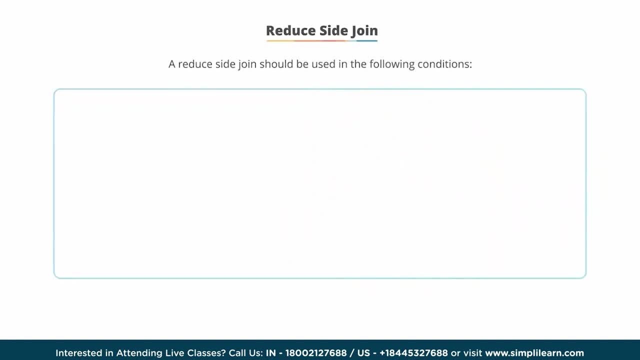 a reduced side. join should be used in the following conditions: when multiple large data sets are being joined by a foreign key, or when flexibility is needed to execute any join operation, or when a large amount of network bandwidth is available, as we'll be moving data across the network and also 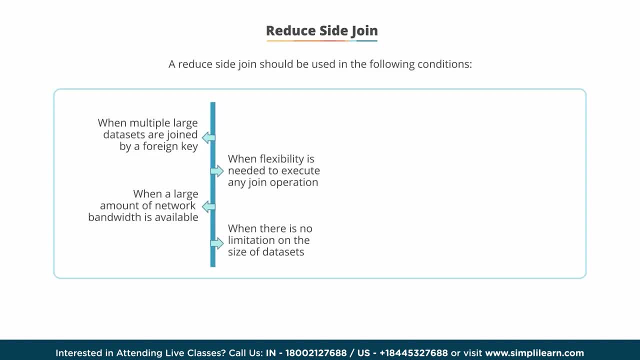 when there is no limitation on the size of data sets. the sequel analogy of a reduced side join is given on the screen. in the output of a reduced side join, the number of part files equals the number of reduced tasks. so if you have 10 reduced tasks, 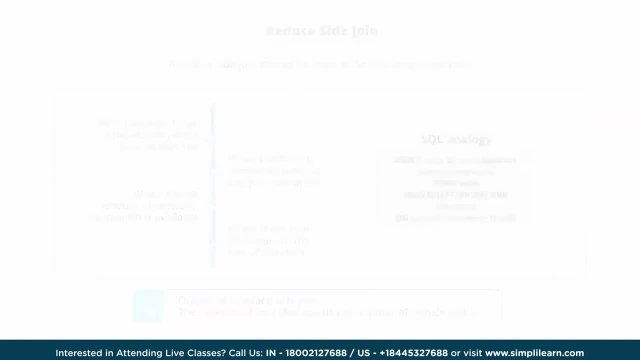 you will have 10 separate part files, replicated joins. a replicated join is a map only pattern, in other words does not use the reduce phase, and works as follows: it reads all files from the distributed cache and then stores them in in memory lookup tables. the mapper processes each record. 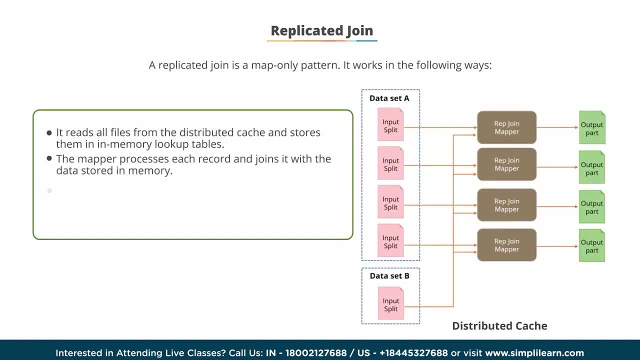 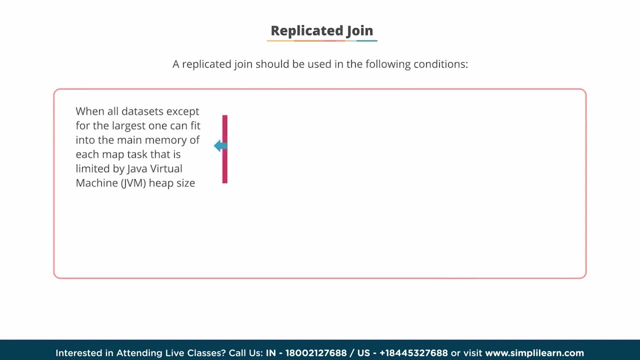 and joins it with the data stored in memory. there is no data shuffled to the reduce phase. the mapper gives the final output part. this type of join is typically very quick. replicated join should be used when all data sets except for the largest one can fit into the main memory of each map. 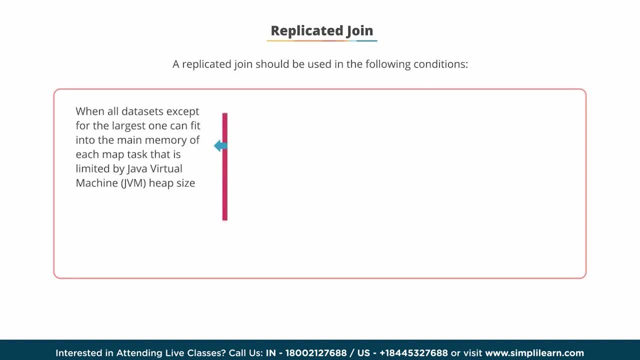 task that is limited by the size of your java virtual machine or jvm heap size. when there is a need for an inner join or a left outer join, with the large input data set being the left part of the operation, a sql analogy of this type replicated join. 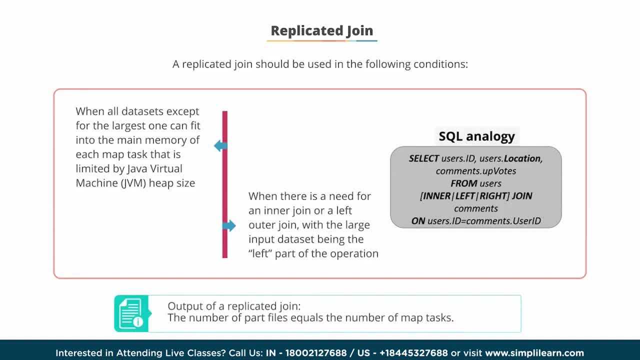 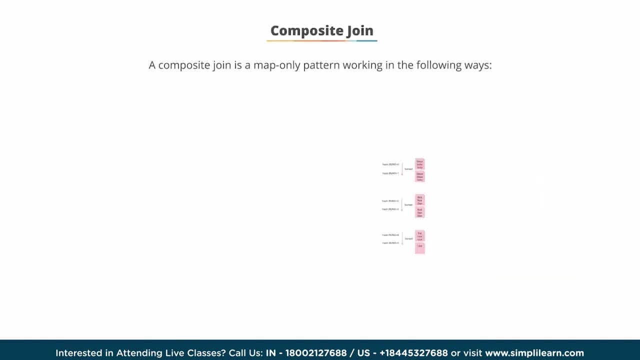 is given on the screen in the output of a replicated join, the number of part files equal the number of map tasks and again, as this is using memory as one side of the join, it is typically much faster. a composite join is a map only pattern working in the following: 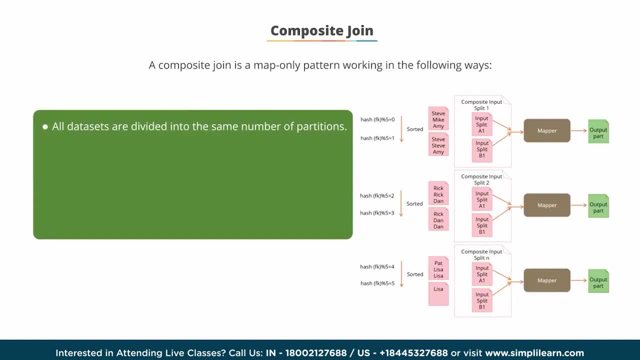 ways, all data sets are divided into the same number of partitions. each partition of data set is sorted by a foreign key and all the foreign keys reside in the associated partition of each data set. two values are retrieved from the input tuple associated with each data set, based on the foreign key and the 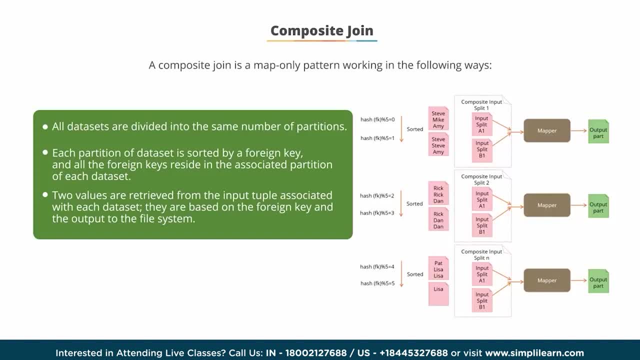 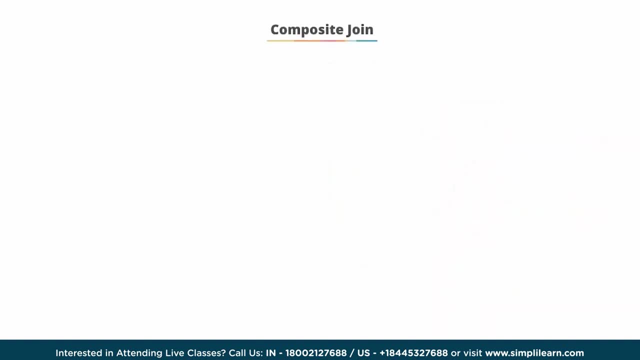 output to the file system. this type of join is typically very lengthy and, depending on the size of your data sets, can run for a very long time. the composite join should be used when all data sets are sufficiently large and when there is a need for an inner join. 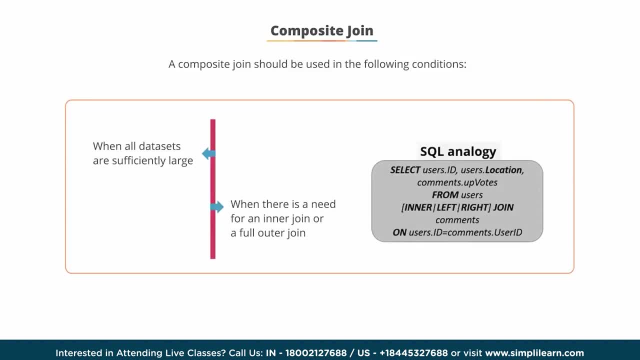 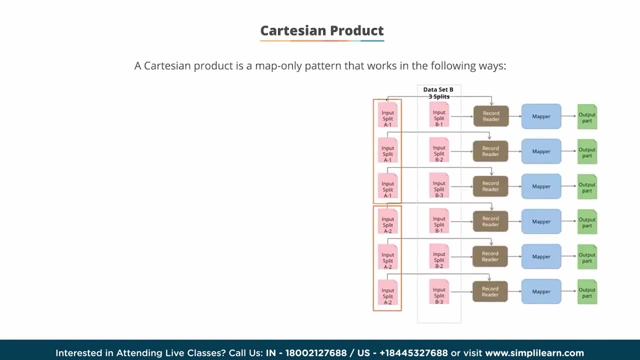 or a full outer join. a sql analogy of a composite join is displayed on the screen. in the output of a composite join, the number of part files equal the number of map tasks. the cartesian product. a cartesian product is a map only pattern that works in the following ways: 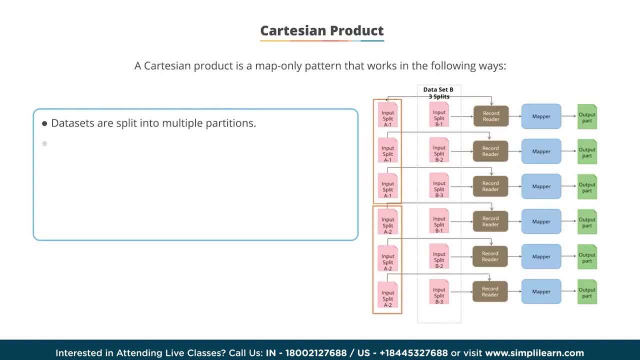 data sets are split into multiple partitions. each partition is fed to one or more mappers. for example, in the image shown here, split a dash one and split a dash two are fed to three mappers each. a record reader will read every record of input splits associated with the mapper. 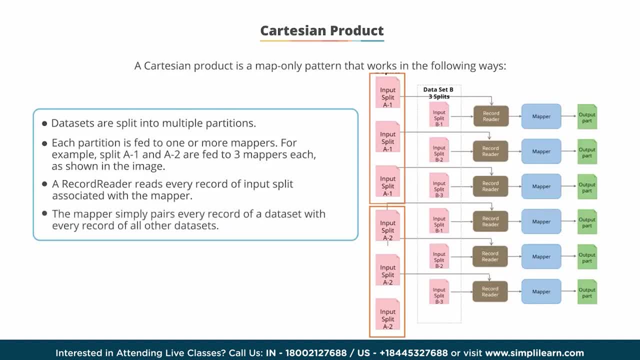 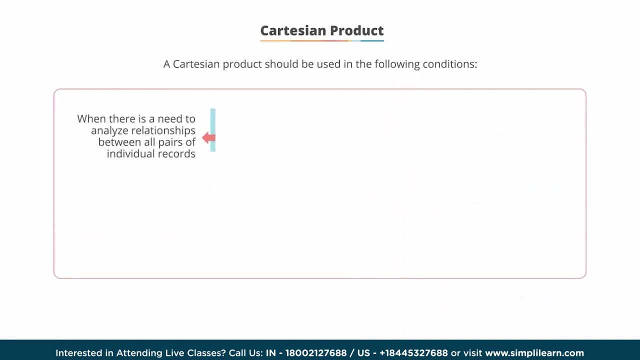 and the mapper simply pairs every record of a data set with every record of all other data sets. the cartesian product should be used when there is a need to analyze relationships between all pairs of individual records and when there are no constraints on the execution time, as these can take a long. 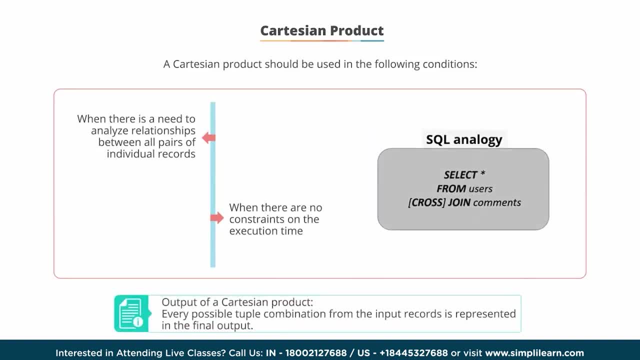 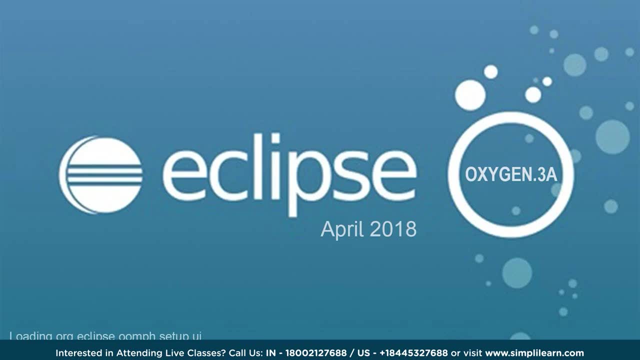 time in the output of a cartesian product, every possible tuple combination from the input records is represented. now i have set up some code in eclipse which can be either tested on your windows machine by running it in a local mode or packaging your code in cdr transferring it to your cluster. 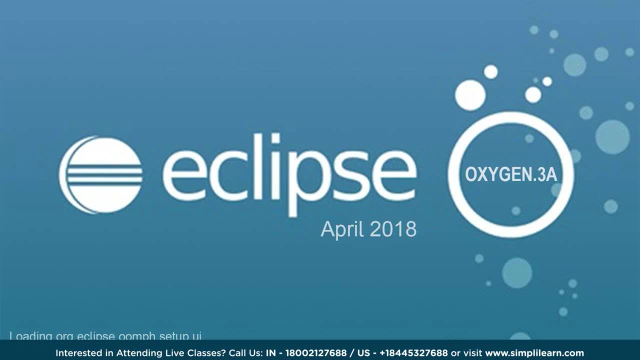 and then basically running it on your cluster nodes. so we'll see both of these examples. now let's assume and let's understand about a problem. say, for example, we have a telecom based company which would want to process its data. say it would want to find out the 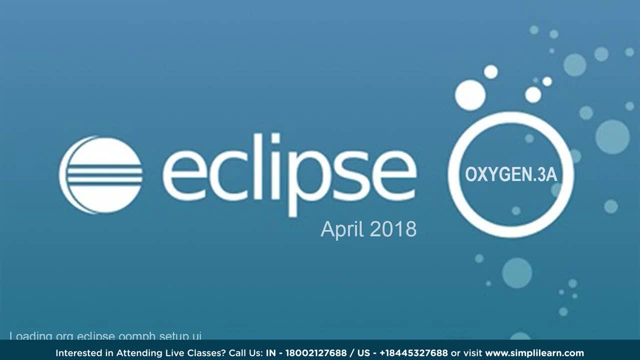 number of subscribers and the kind of calls they are making. or, for example, let's imagine a online website or a music website where users listen to various tracks, the data gets collected and then basically, it has to be processed. so imagine you have a company which is hosting music online. 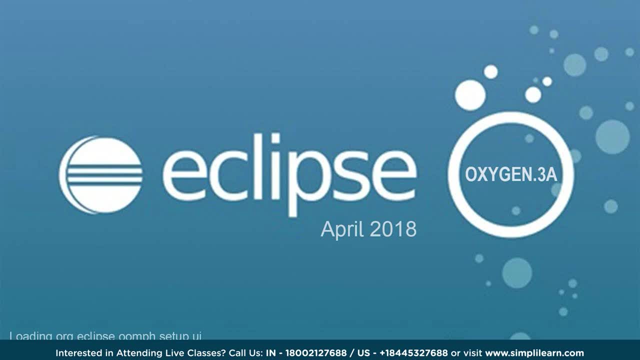 and you have users who either are subscribers or basically create their accounts, listen to different tracks and then basically use these services. now what if i would want to process such data, for example, if i would want to find out what is the number of unique listeners or number of times the track was? 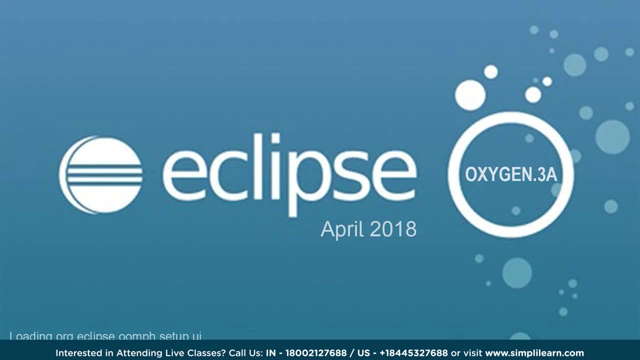 shared with other users, or number of times the track was listened to on the radio, or in total, or even was skipped on the radio. now, in that case, i would want to process the data to find out information. so we will solve this kind of problem using the map. reduce programming model. 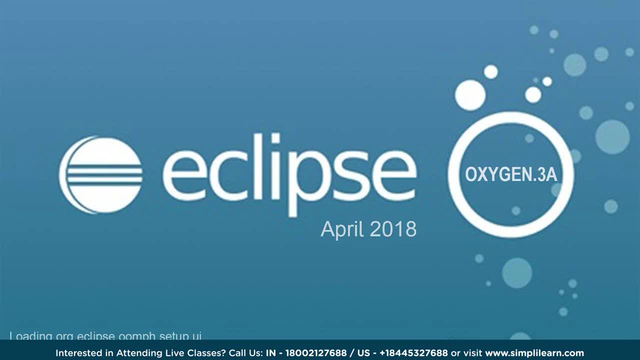 the map reduce approach which, as i explained earlier, goes for mapping and then for, goes for reducing, and in between it has different phases, that is, shuffling and sorting. you have your partitioner phase, you have a mini reducer, which is your combiner phase, although all of these intermittent. 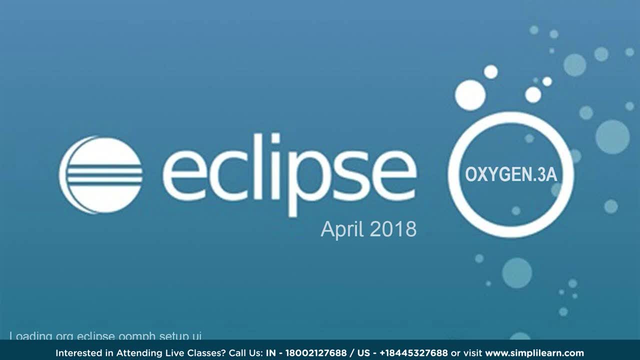 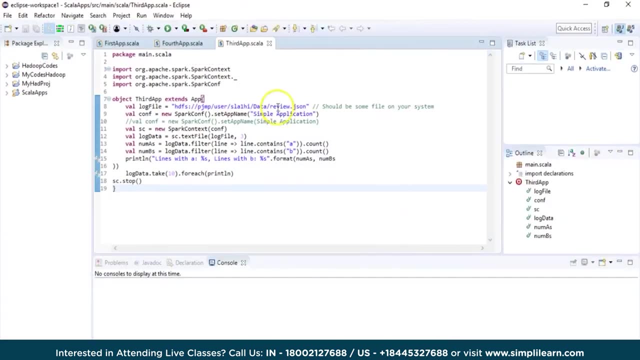 phases are taken care by the framework itself. the developer, or the person who is developing the solution, is responsible to work on the mapper function and the reducer function. now for that, we can basically be writing our code to process this data by giving a mapper and a reducer function data. 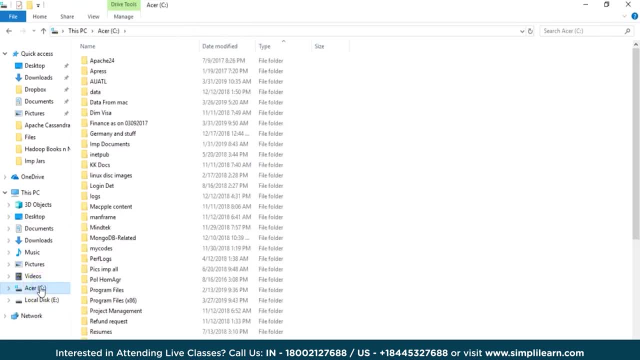 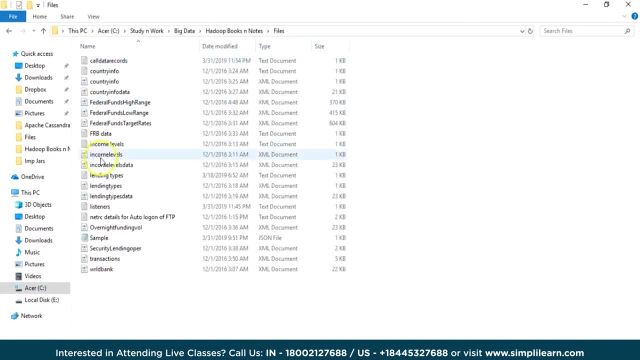 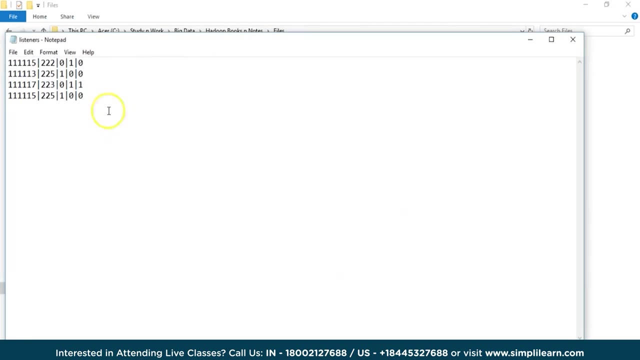 we can look into example and say, for example, let me pull out some data here. let's look in, say, some files i have and, for example, in this case it would be this kind of data: now that magnitude could be anything right now. here i have the data. 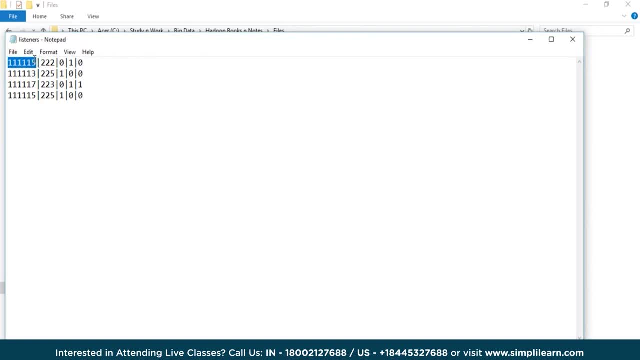 which the first column talks as the user id or the membership id. the second is the track id you have, then your if the track was shared online. the fourth one is number of times the track was listened to in total, and the fifth one is if a particular track was skipped. now, 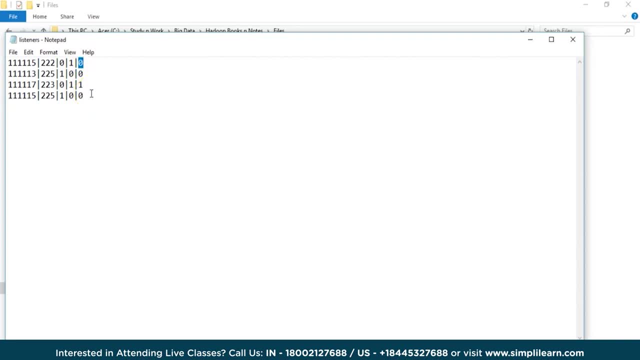 i could have this data in huge numbers and then i could be processing it, but we will take a simple, small example to understand how mapper reduce does this. so this is a file which i have already uploaded on the cluster and which will be as my input file. now let's 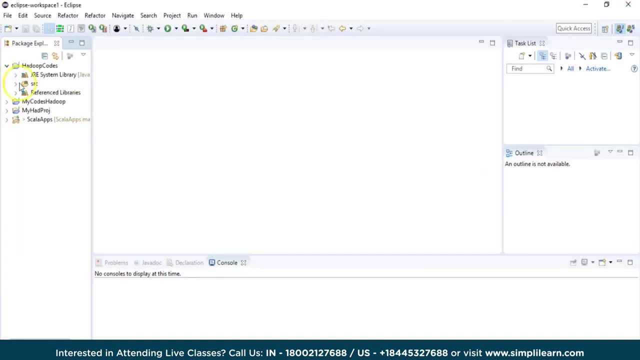 look at the code. so what we would need is, for this kind of processing, we would first need to understand the data. now, here, the first column, as i said, is user id and second one is track id, which can then be used to basically process the data. we need to write a mapper class. 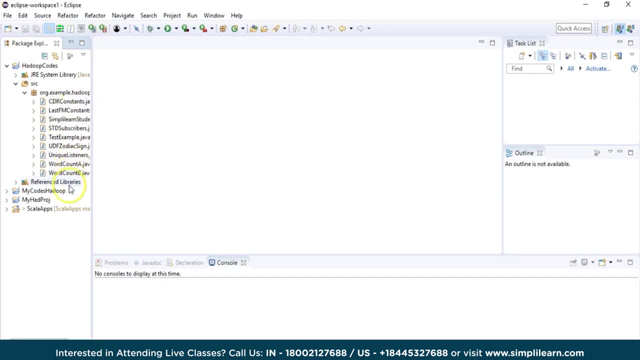 which would emit the track id from this data. so i have it here and let me also open up a constant class for this, which is here. so, as i mentioned, we will have to write a mapper class which would emit track id from the data and user ids. 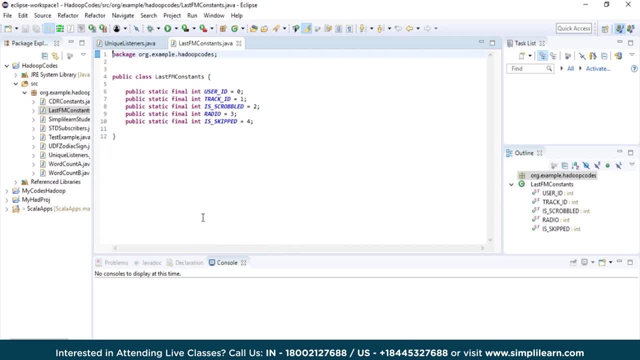 with some intermediate key value pairs. now that is what your mapping phase does. it works on the input splits, it basically does the mapping and it gives you a list of data elements which are nothing but your intermediate key value pairs. to explain it in a simple way, i would say: 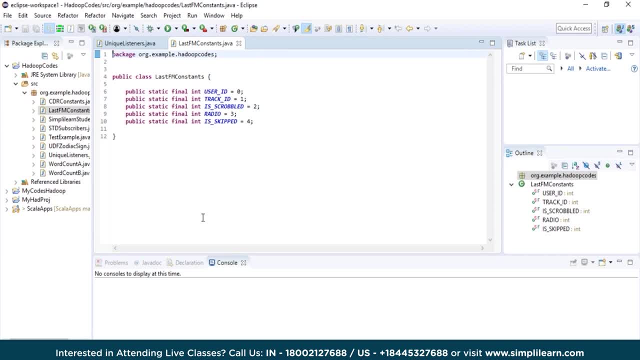 just let's work on this data sequence. so let's create a constant class, as shown here. so this is my package. now i create a class called last fm- constants, and then i am here declaring some variables with some constant values for each of the field which i just showed in. 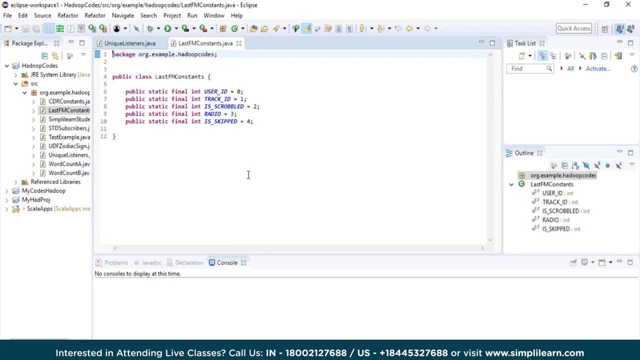 the file. you have user id, you have track id. you have is scrabbled or shared radio and is skipped. now these are my constant, which will be used while i process. then we will have to work on a mapper class which could or which would immediate emit. 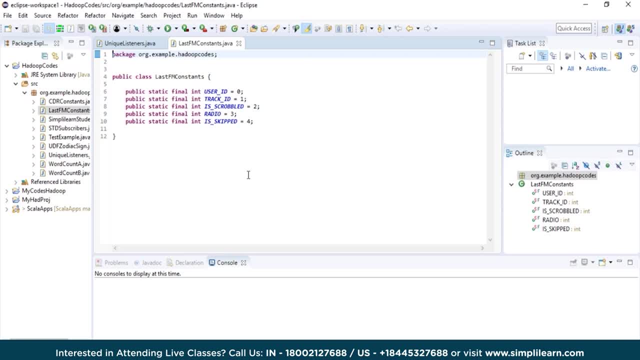 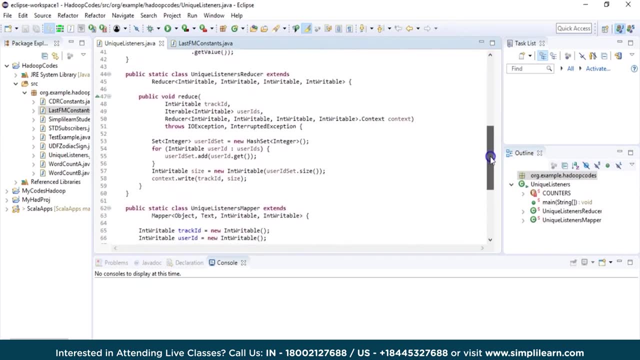 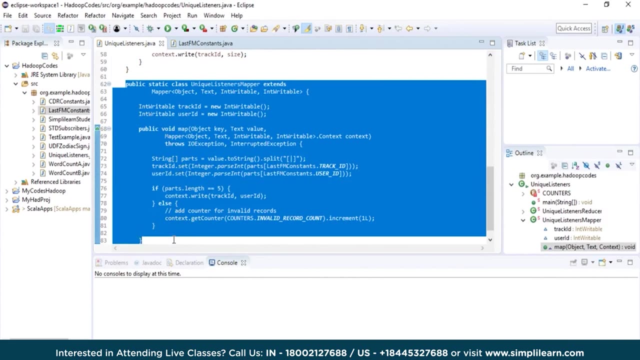 intermediate key value pair pairs, that is, your track id and user id. now how do we do that? so here is an example. so we basically would have a mapper class as it's seen here. this is my mapper class, which will be used to process or do the mapping phase. now. 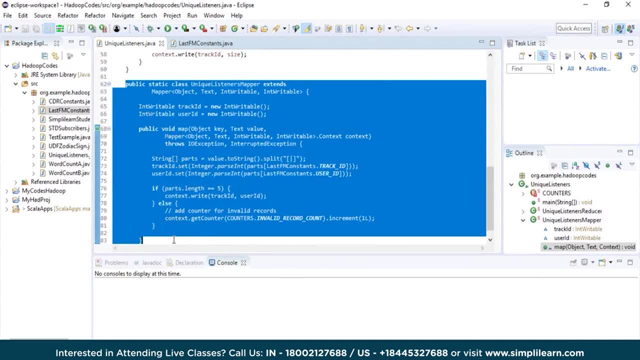 here we have the class name, which is unique listener, and unique listeners mapper, which extends the mapper class. that means i would have to import the relevant packages for my code, which i have done on the top here. then i have variables, that is, track id, user id, which. 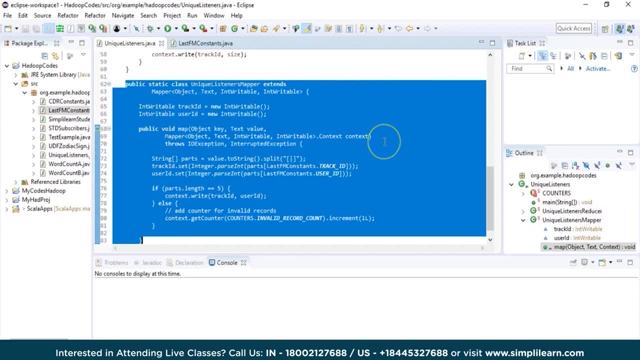 use int writable. so hadoop has its own data types, say int writable long, writable, boolean writable, which are similar to what you have in java as int boolean long. but these data types which are used by hadoop are basically an implementation of writable and writable comparable interfaces. 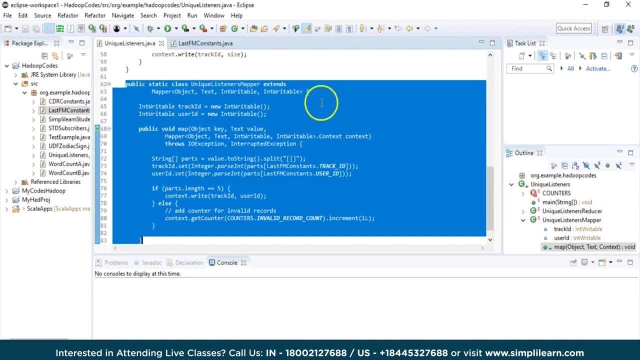 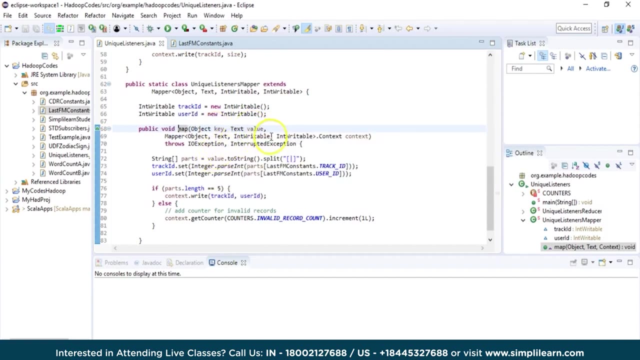 so those are two interfaces which are then responsible for these classes which we are using as data types in our code. here we start our map task, which would then consider key, which is an object value, as in text, and then you have your data types. that is int writable. 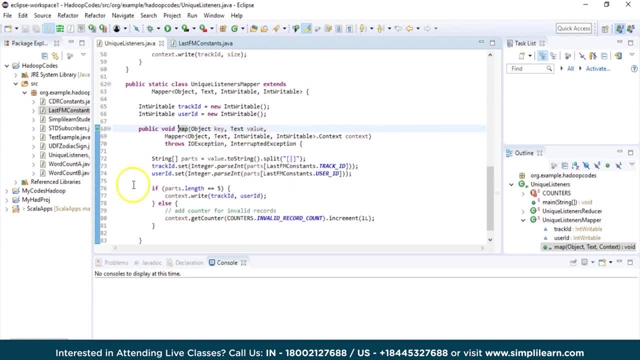 text and object. we are also handling exception, and then what we do is we work on the file so we would split it based on the delimiter. now, in my case, the delimiter is a pipe. then what we do is we set for the track id using our constants. that is what we have. 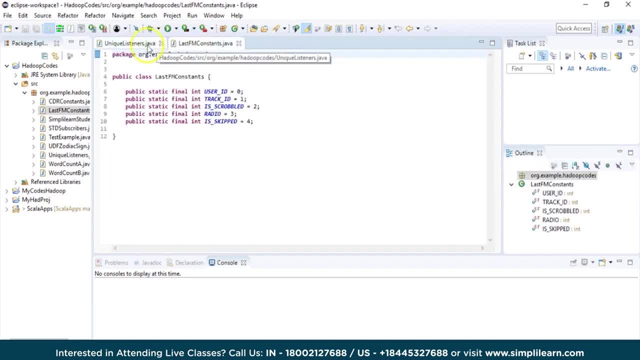 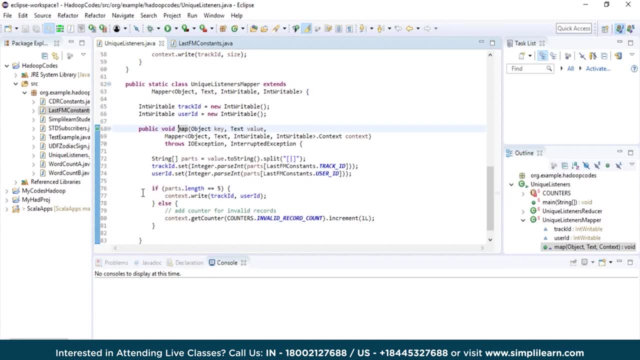 seen here, which is for your user id, track id and so on. and we do the same thing, we for our user id. we look into the values and then we basically emit out just the track id and user id. that would be my intermediate key value pairs. now, 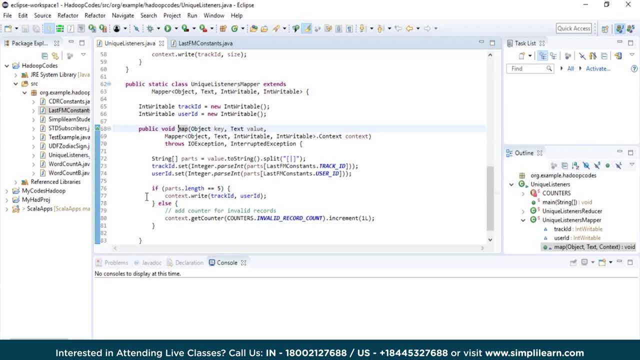 here i am also using a counter named invalid record count. now that is mainly to count if there are any invalid record which do not exist in the file in an expected format. now you know we don't do this in case of invalid records. if we don't do this, what would happen? 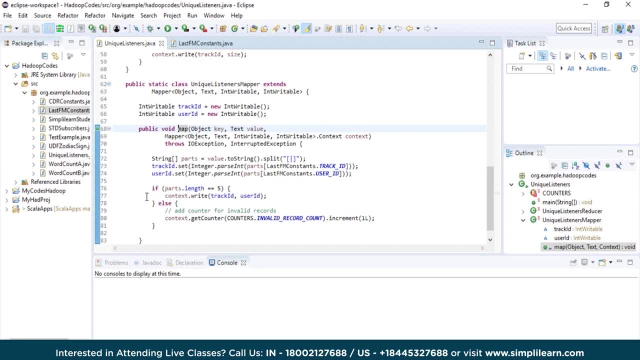 if we had invalid records in our file then our program might fail and that is the reason i am using counters, dot invalid record, dot count, and i am going to use it for my mapper, once we have our mapper written, which basically will look into the file and 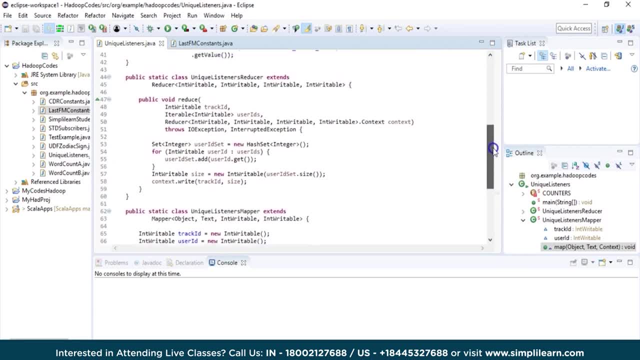 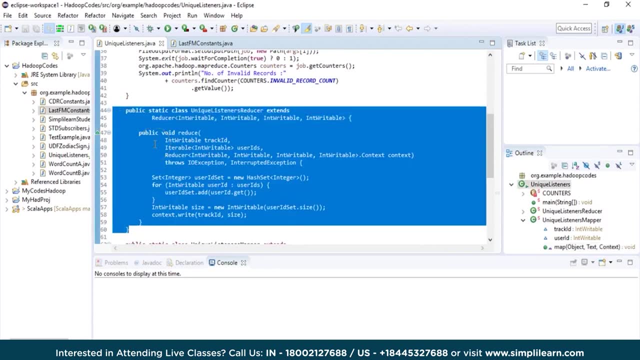 emit the track id and user id, then i would write my reducer class. now this is how my reducer class looks, where i am saying public static class, unique listener reducer, which extends reducer class, and then the data types which it would need so int writable for the values. 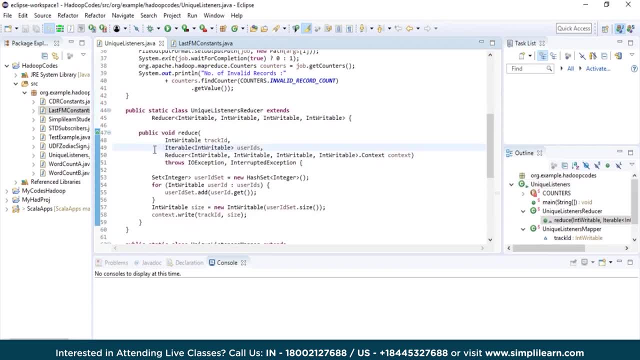 which it works on. so our reduce task will work on track id and this reducer class is to aggregate the results. so we cannot directly use some reducer, as the records we are getting are not unique. the records might be duplicates. it might be the same user with the same. 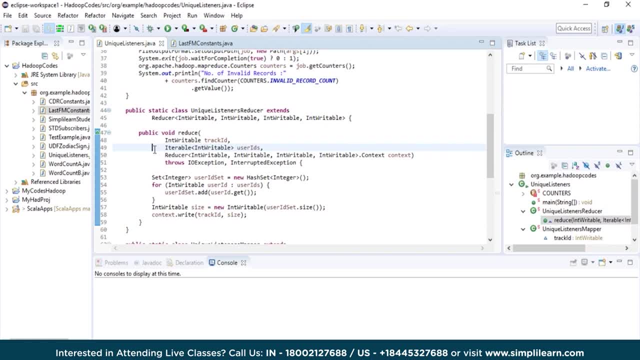 membership id, listening to a different track or sharing it, and we cannot be just using a generic reducer. so here we work on the reducer and this is how my code would look. so what my reducer does, it basically would help me in solving the problem, such as basically: 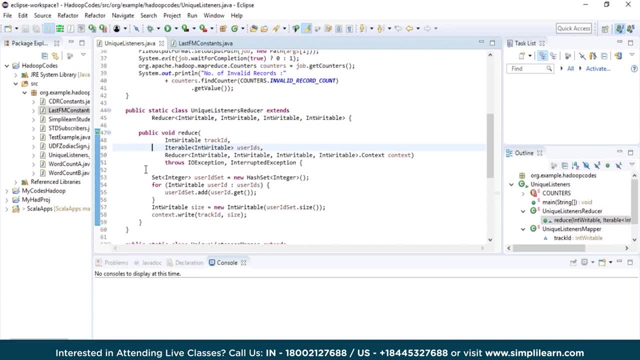 aggregating and counting the number of tracks which were shared or listened to, or over all the number of tracks, and then you have your tracks which were skipped. one of the main task of your reducer class is on working on the intermediate data which is created by your mapper. or you can say: 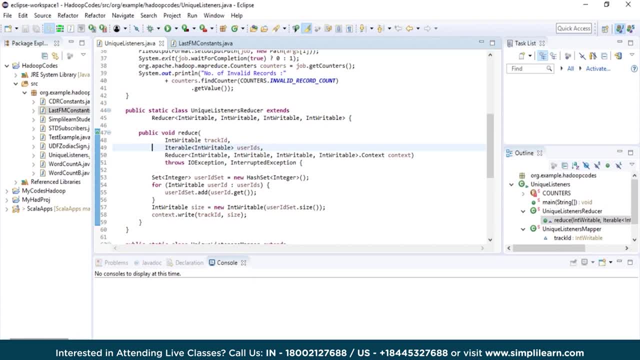 multiple map tasks, which would be running on multiple splits on one or multiple nodes, and your reducers work is to aggregate the result based on the keys here we are using set to eliminate duplicate user ids. now, once we have written our reducer class, which basically works on the 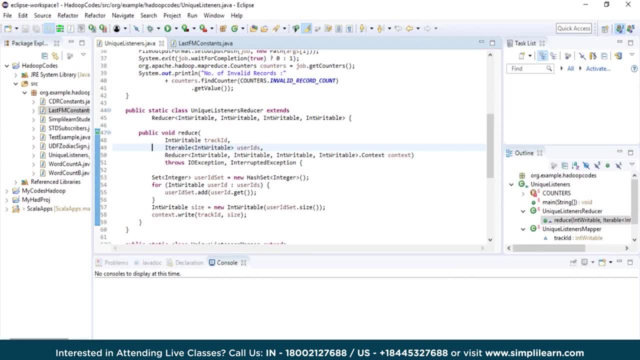 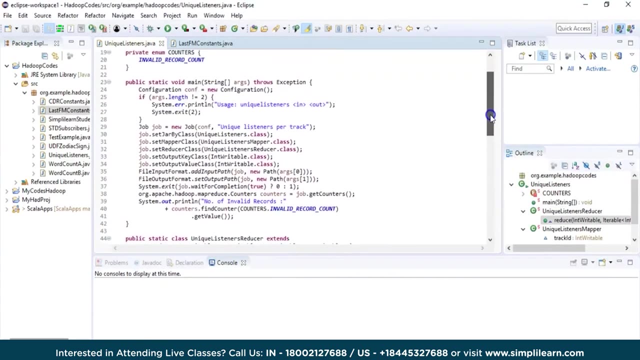 user id set. it eliminates the duplicate user ids and then it basically gives me a count of the track ids in an aggregated way. to solve my use case, once i have done that, i also need a driver class which basically tells about my overall code. so here we are having a 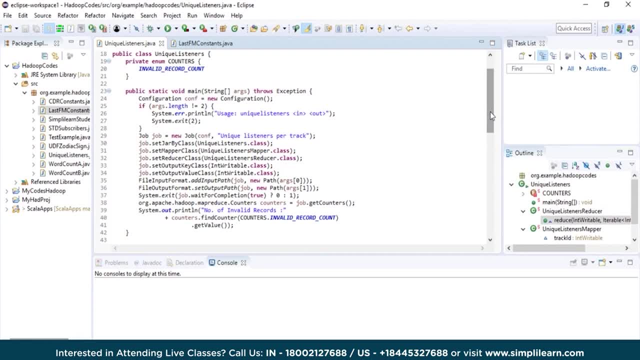 job configuration where i say my name of the job could be unique listeners per track. i am setting the jar by class, calling it as unique listeners. that's my class. i'm mentioning my mapper, i'm mentioning my reducer. now, if you notice, i'm not using a combiner class. 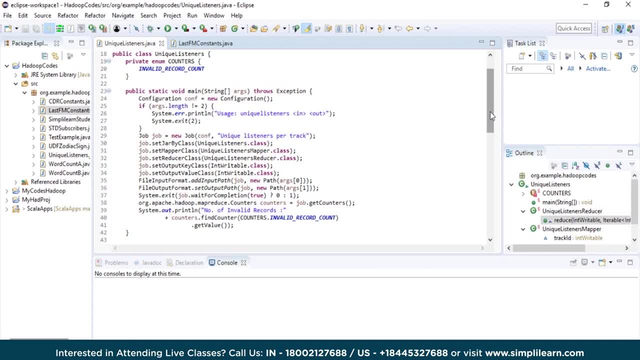 for this use case, we would not need that. so combiner class is a mini reducer which basically helps in reducing the data or aggregating the data before it reaches the reducer class. i am also talking about the key, which would be using int writable, and then the value, which would also be 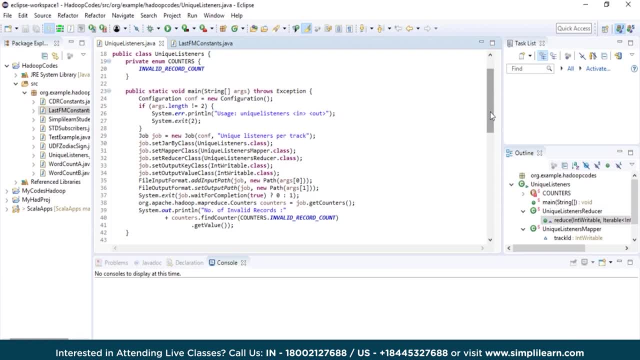 int writable, as all my values are in numeric. if i had my key in something else or if i had names instead of user id, then i could have used text class. i also specify what would be my input and output path, which will be specified as an argument. 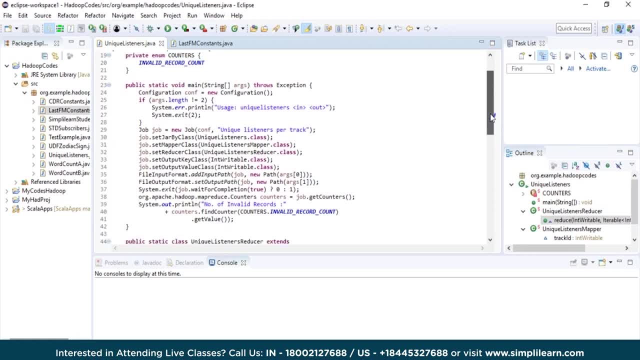 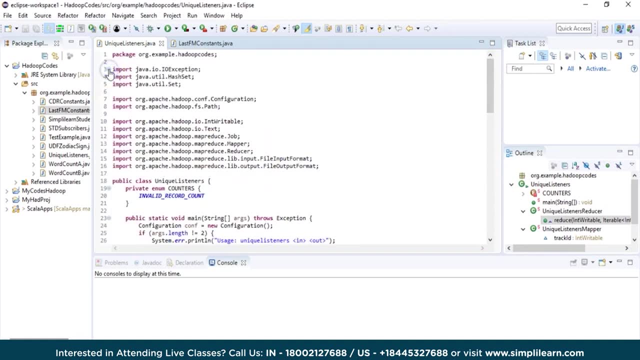 and then, basically, i am printing out number of invalid records. so this is my mapper use program to work on solving our business use case. also, notice, i am using the relevant packages which are being used in the code and for these packages and for my this code to compile, we 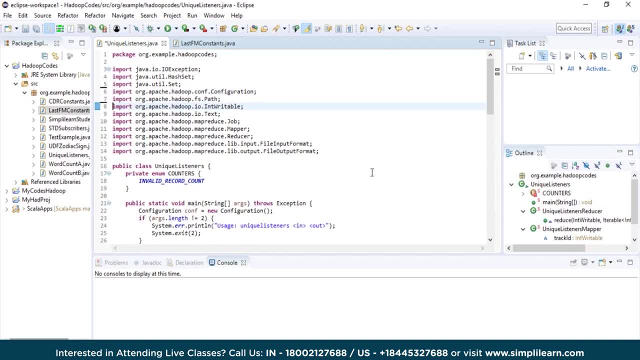 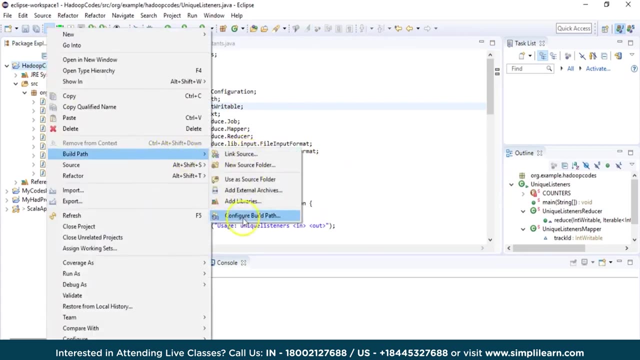 need to make sure that we have added the right dependencies. now you could have created your code with pom and, using maven or based on the classes, what you are using, you can always add the jars, the relevant jars, to the build path. so here we can look at the build path. what i have. 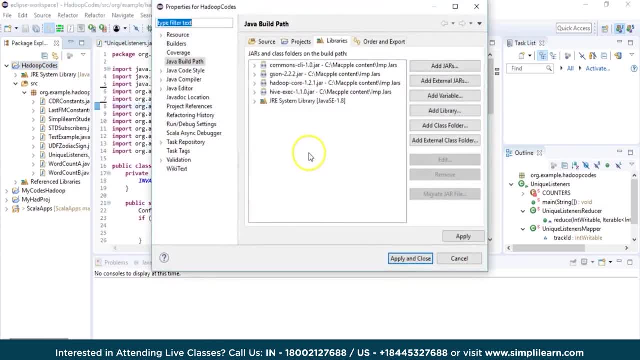 and we can see what jars i have used. so the main ones are your commons. i have hadoop core now you can ignore hive or json json which i have here. those are for different applications. so the main is common, cli and hadoop core, depending on what you are using. 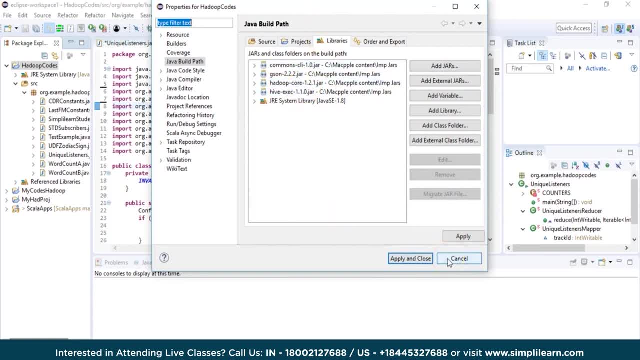 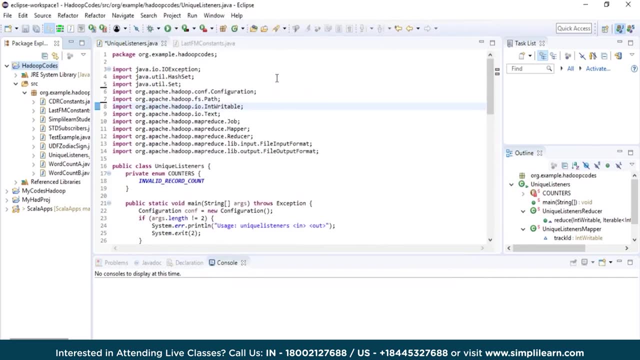 within your application, so that has to be added to your build path also. we are having the java 1.8 now. if i wanted to run this application or test it on my local machine, i could have also set up the configurations. however, it is preferred to run the. 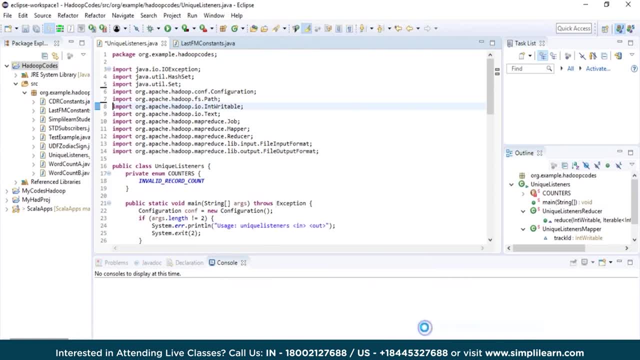 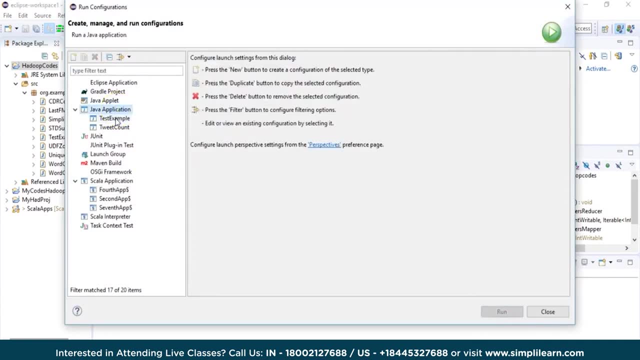 code on a yarn based cluster. if you would want to try to run it on windows, then you can always go to the run configuration. you can basically specify your application which you would want to run. you can then say what is your class name. you can be passing in your arguments here. 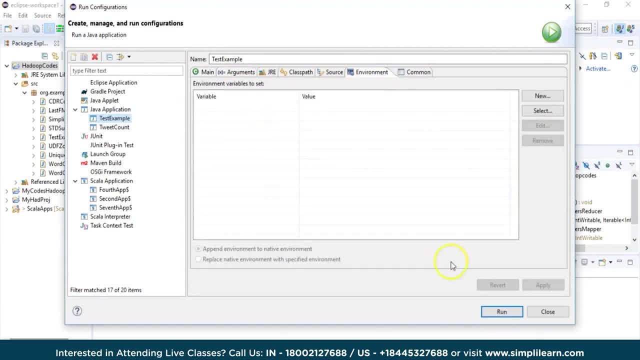 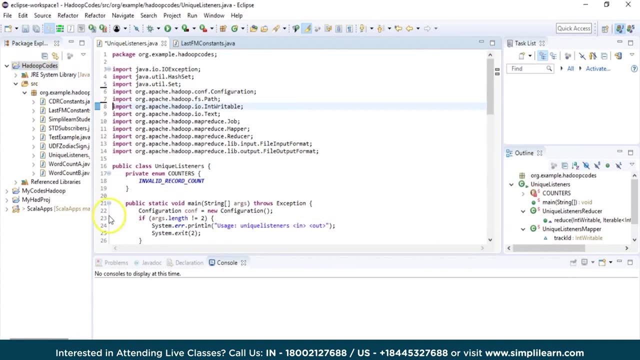 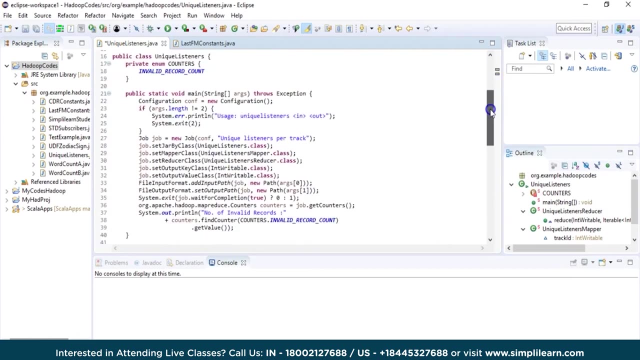 and in your environment. you can specify hadoop as a local ip. however, i suggest package it as jar and run it on a cluster. so what you could do is you could select your class. now my unique listeners dot java class is also getting the constants from last fm constants. 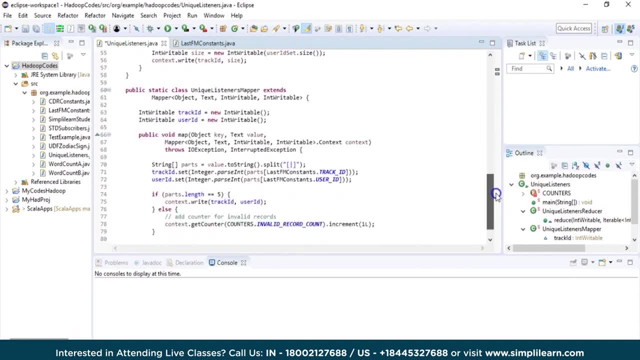 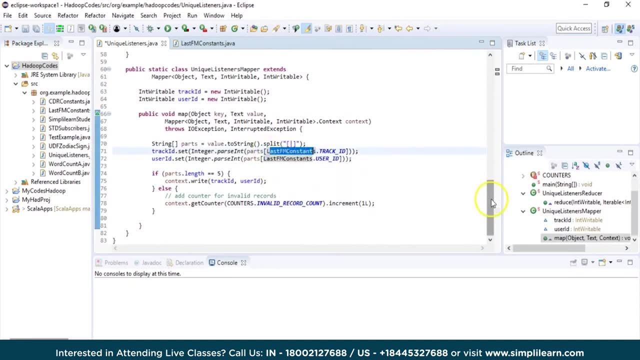 so both of them belong to the same project and i'm using that here for my mapper and for my reducer. so in mapper i refer to last fm constants, where i've given constant values for all of these fields. once you have your code ready, you can always package. 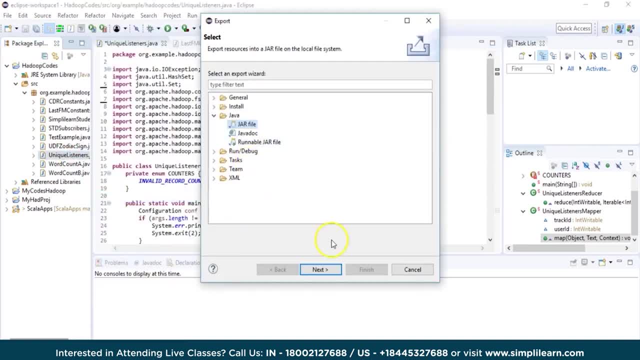 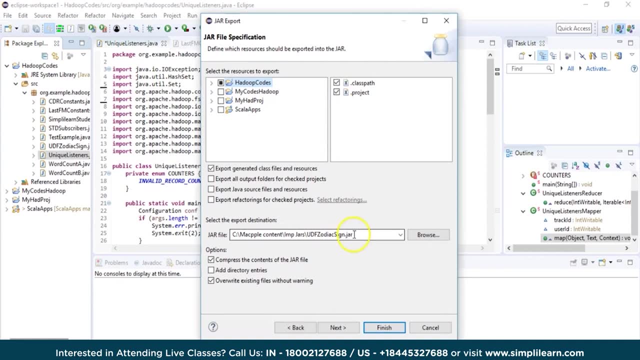 it as jar by saying export and select the jar option in java, click on next and then you can select your project and give it a name. so i have. i'm pointing into a different jar file, but i can do a browse. i have already packaged it as jar and you can see. 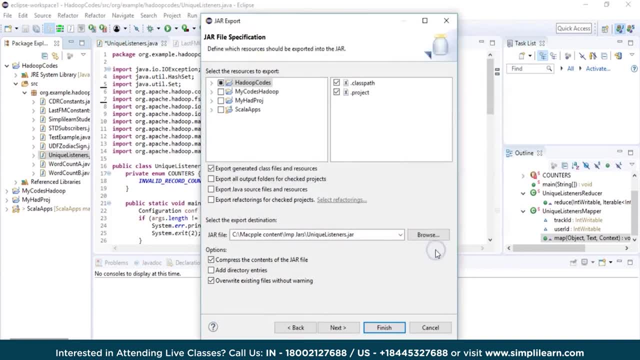 i have a jar here, so i can select this. i can say save, and that would be my jar. if i'm making some changes, it will anyways overwrite it. once you have your jar ready, what you need to do is place it on your cluster. now. i have already done that. 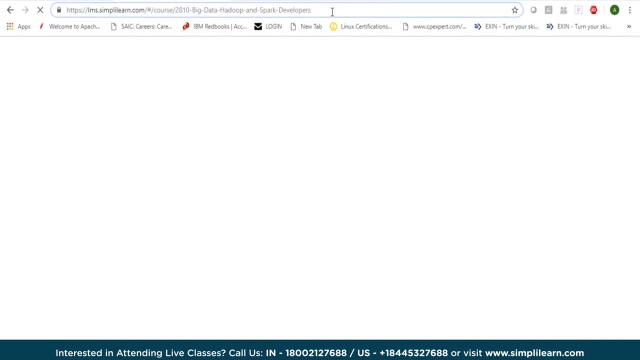 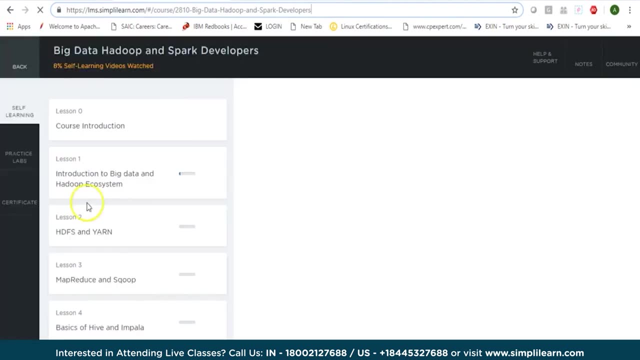 i have a cluster here. let me bring it up, and what we can do is you can use different ways. you can have a apache cluster, you could have a cloud era cluster wherein you need to place. so let me get into this now. here i'm using a already set up lab. 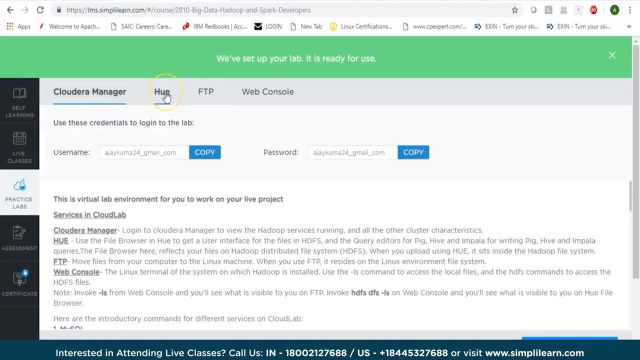 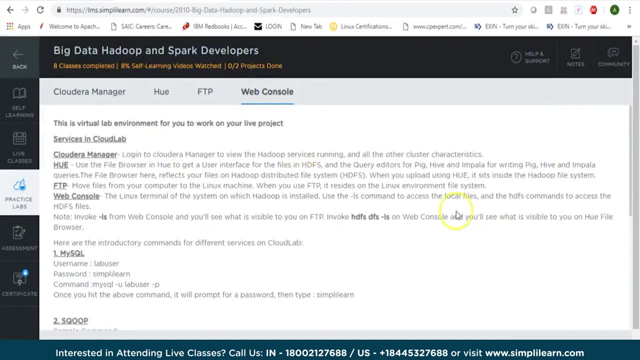 environment. you can be doing an ftp. you can upload your code using hue. i have done an ftp from my local machine and uploaded it to the cluster. i could click on web console, which basically gives me a console to try out things. you could, as i said, you 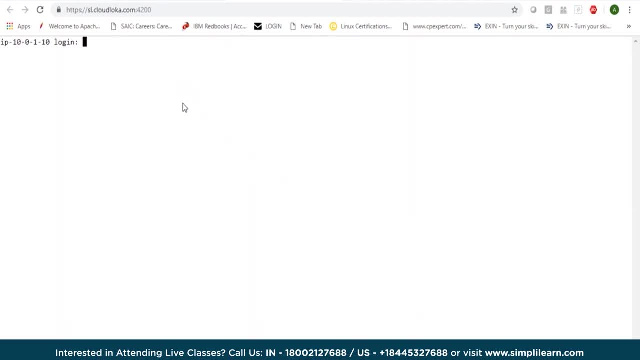 need the jar and then you need to push your jar to your cluster. let me log in here, and once i'm logged in, i am on a edge node which allows me to connect to a cluster which is cloud eras based, and now i can check on my hdfs. 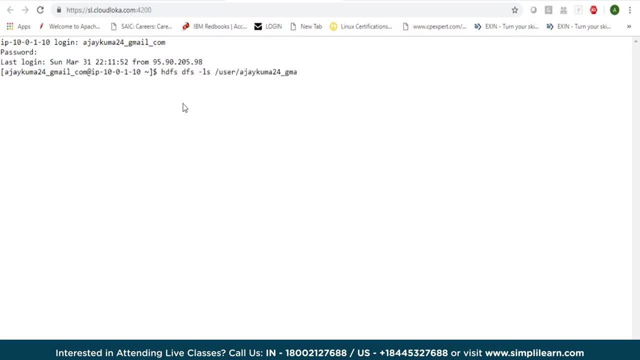 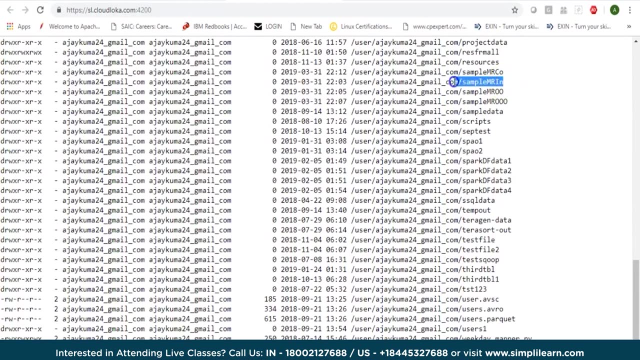 path in my user directory i should have multiple files and directories and in one of the directories i have placed in this file so we can look in here, which is sample, mr in, and that's my directory where i have the input so i can look in sample, mr in. 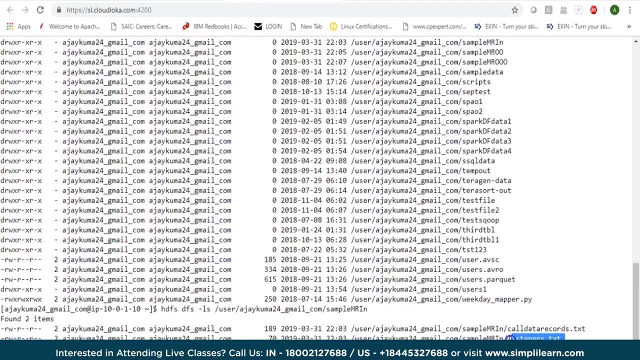 and the same file which i showed in the beginning- i have uploaded it here- which is the listeners file, which we can even check, so i can say listeners dot txt and i can even do a cat. so this is the file which is already existing here, which has the content. 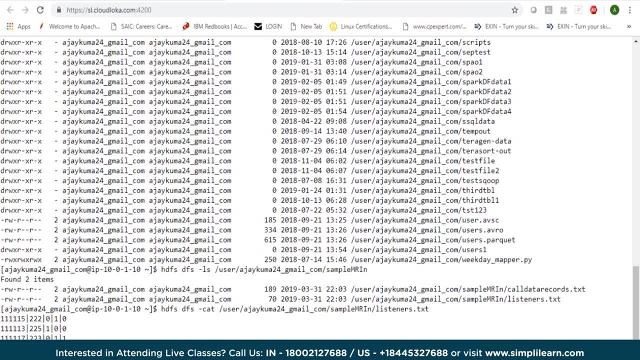 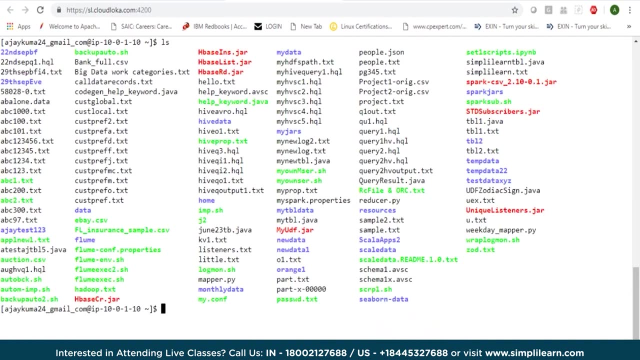 which we spoke about, although not huge content, but it is more than enough for us to test our code and obviously we can upload huge data and then have the same MapReduce program helping us in answering our questions. we also need the jar file, and the jar file should be here. 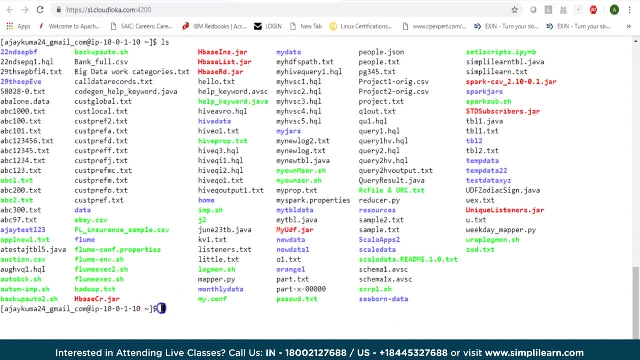 which i have uploaded. so i need to run this now to run your MapReduce. you can say hadoop jar. you will give your jar name, which is this one. now i need to give my package name with my class name. so i will say org. example: hadoop. 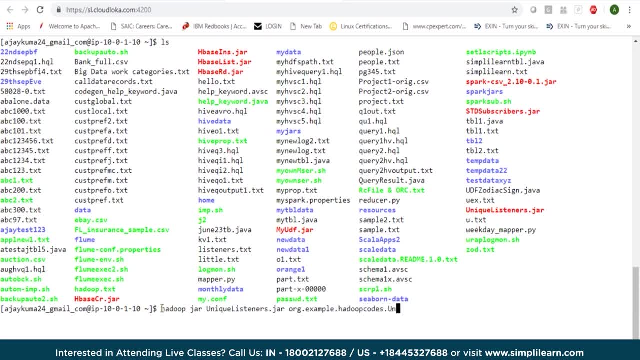 codes and then i need to give my class, which is unique listeners. now if i hit enter here it will ask me to give an input and output, as my code says to pass in the arguments. so we will pass in the arguments here. so i will say my directory where i 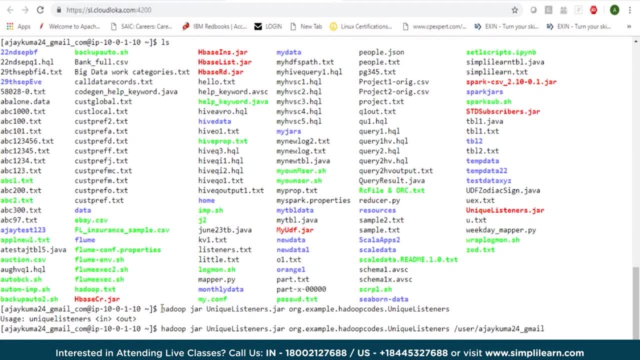 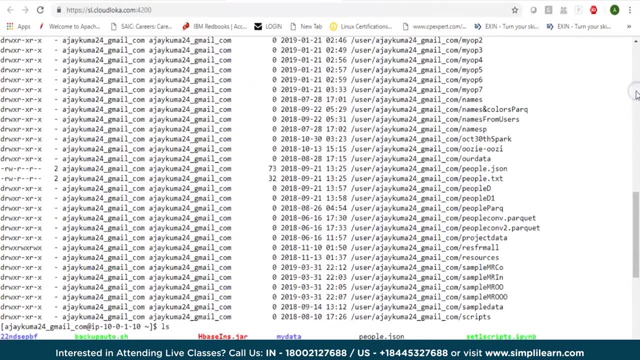 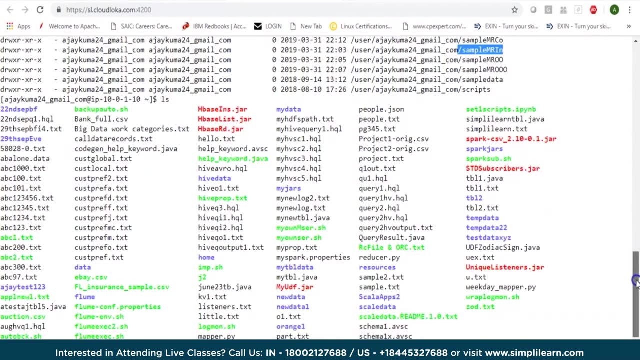 have the data now. i could be picking up one file or multiple files to process this. so i will say just one file which is here and that's my file, which is sample mr in. that is what i want to use. so i will say sample mr in and i need to. 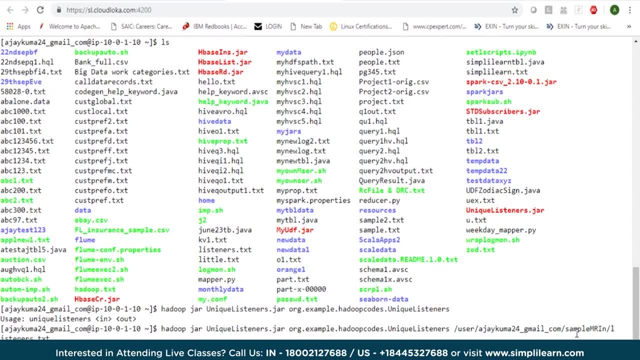 give my file name, so i can say listenerstxt, and then i can give an output which will get created when you run your map reduce. so i can say sample, mr, and then i can say output one and this is the directory which will get created, which will have my output. now you can run. 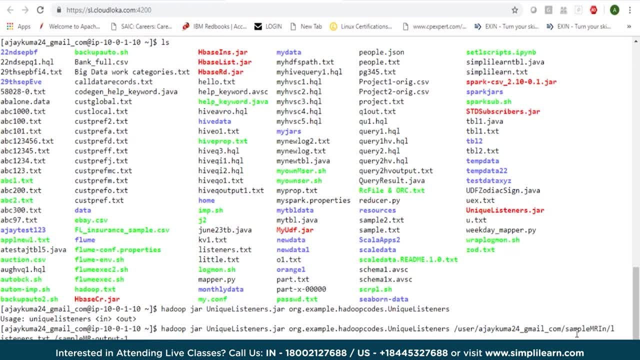 this job. in this way, you can even run it in a local mode. by specifying arguments on the command line, you can give different kind of properties. if you want your map reduce jobs output to be in a compressed format, you can do all that. so let's run this. 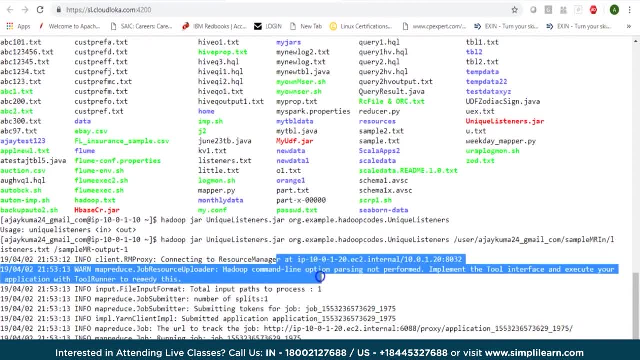 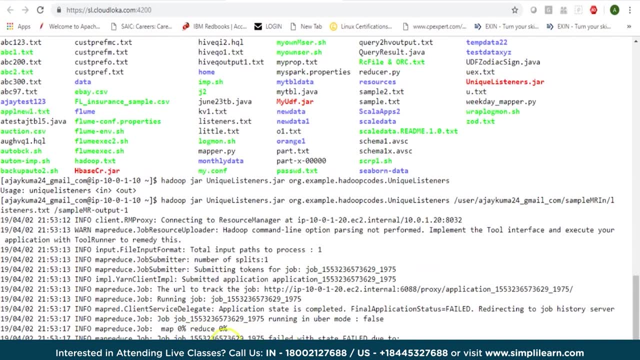 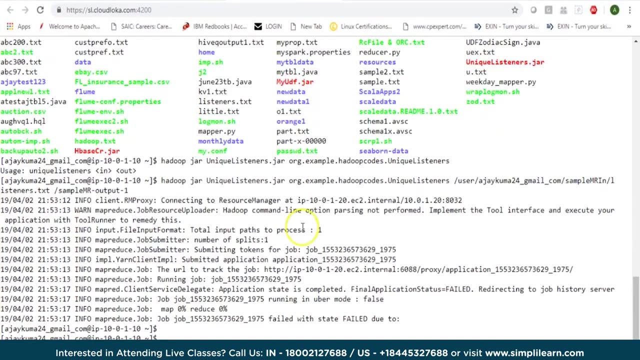 and this should connect to the resource manager. the job is processing one input file. it will start with the mapping phase first. now it looks that the job has failed due to some reason. let's have a look. i just looked into the job and i realized why it failed. the main reason was: 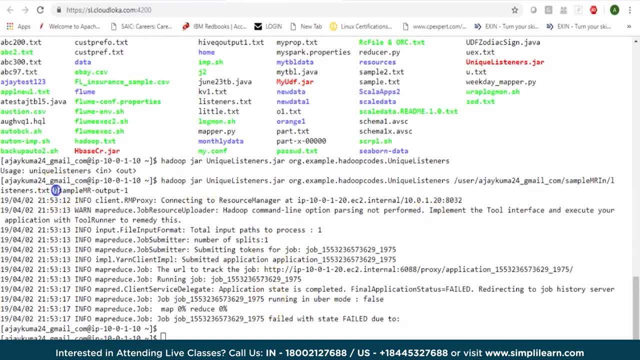 i was trying to write an output in the directory to which i don't have access. i need to have access to write the output in a directory to which my user id has permissions. for this we will have to submit the job again with the right path where it can write the. 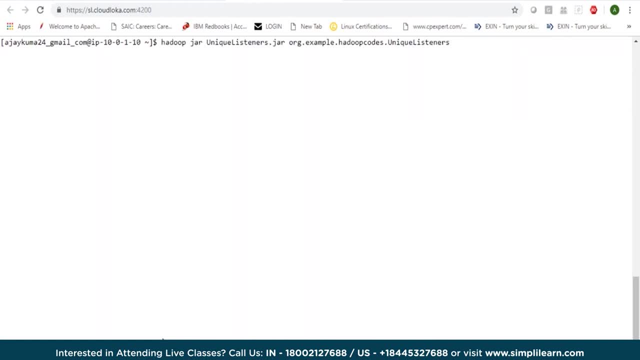 output. so we can do this. this is my class, i need input, so i'll say: and then we can say: sample: mr in and i'm looking for listeners, dot txt, and i need to give an output, which should be in this path, and then we can say: 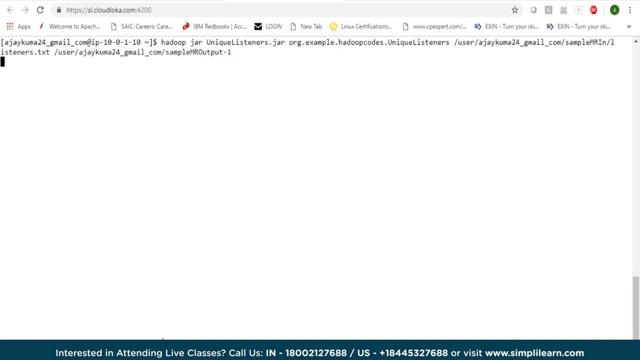 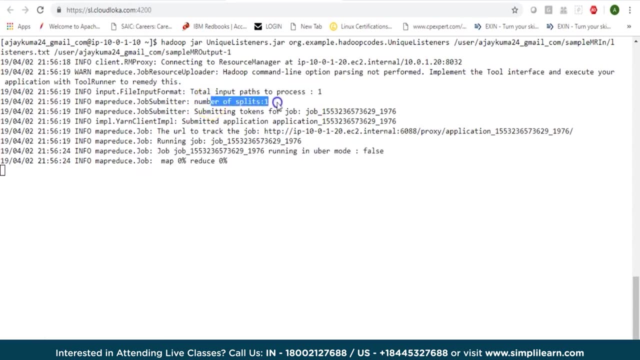 sample, mr, output one and then submit the job. now, once i have submitted the job, as i said, it has one input part to process. it is working on one split because the file which we are trying to work on is smaller than the block size. it goes for the mapping. 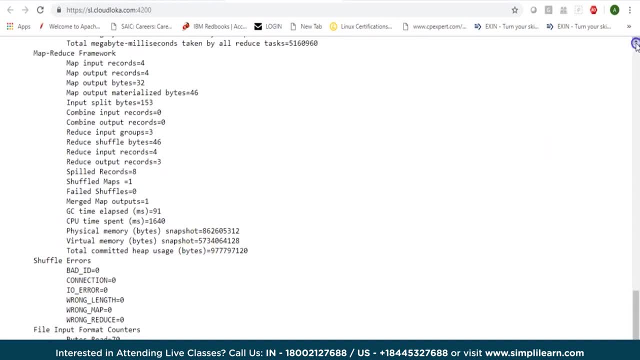 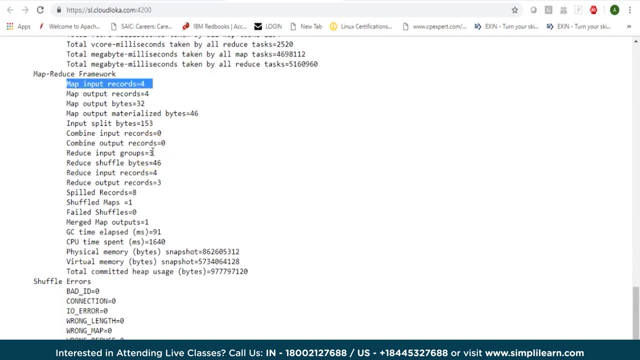 phase. and then it goes for reducing, and it's done so. if you carefully look at the map: reduce output. here it says the number of outputs it had to process was just four. so every line by default is considered as a record and we had totally four lines the output. 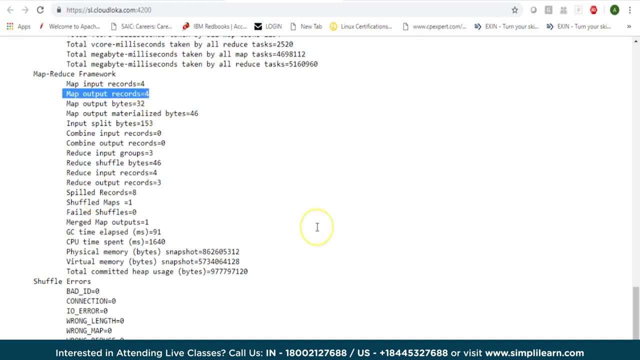 is basically working on again giving you four records right, because we are doing a split based on the delimiter. then this would become an input to combiner if we had a combiner class, but we don't use that, so the output from your map goes to the reduce. 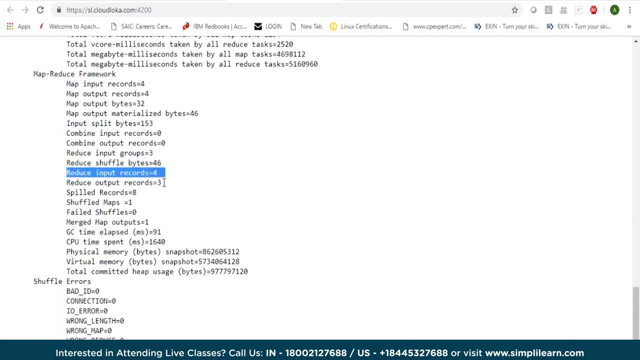 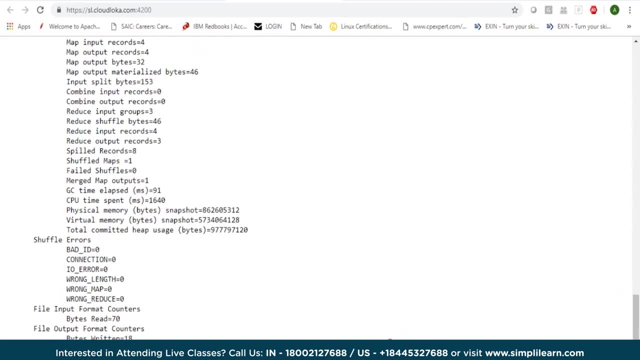 which will basically work on the input records and create output records. now we can have a look at this, the output of this job, which is stored in HDFS, and i can either be giving a complete path or i can just mention the directory which i used and that. 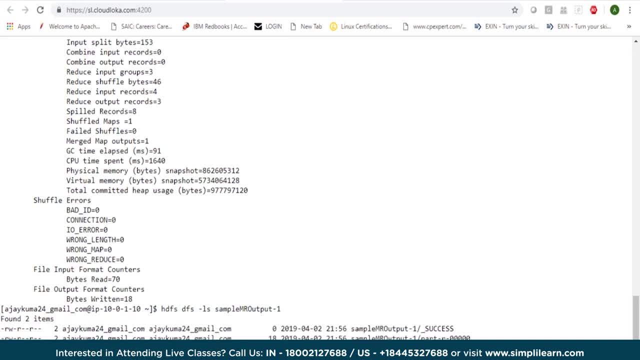 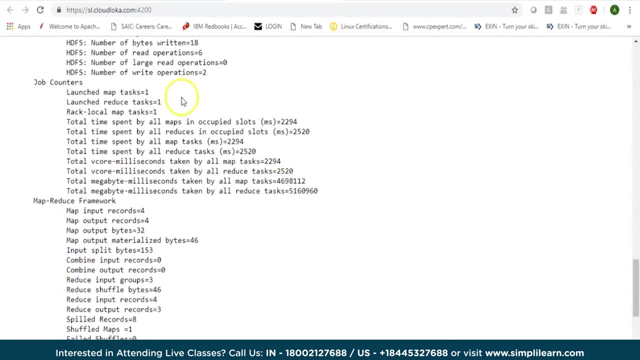 should by default take me to the directory which should have my output. now, based on how many reduce tasks were used, you will have number of part files which show up here. so we have one map and one reduce task that could have controlled or that could have been controlled by. 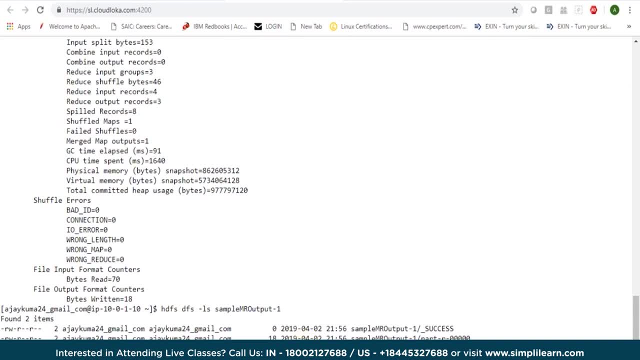 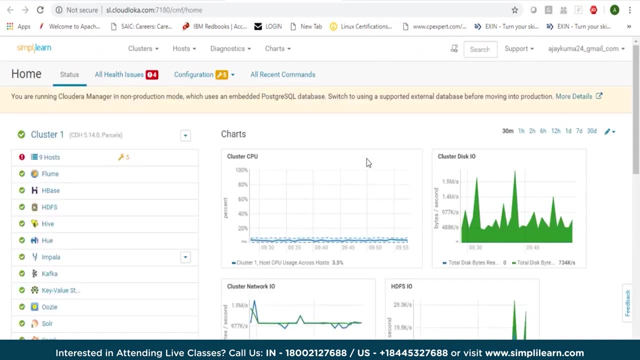 giving things on the command line. so here i have run it in a yarn mode where yarn was used to allocate resources for my applications, and we can always check that on the yarn UI or also by going to say cloud error manager, if that is available. if you are not using cloud error, 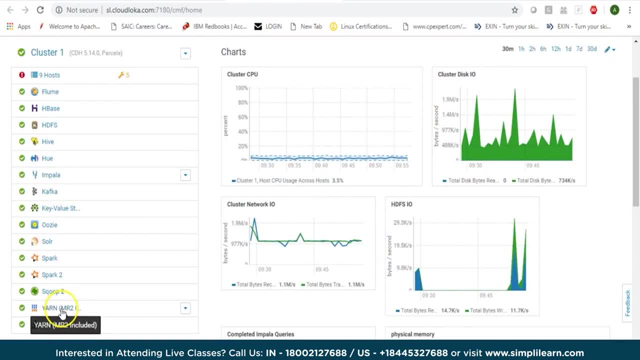 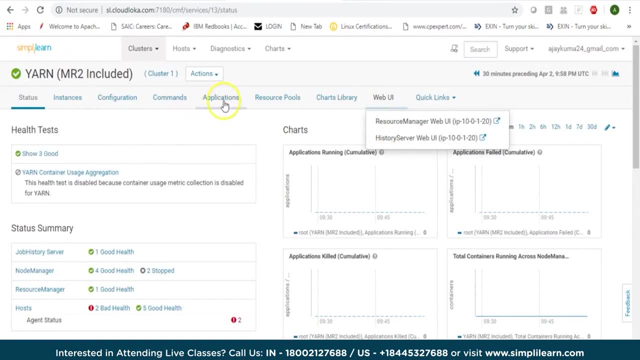 cluster, then you can always, in apache cluster, go to your yarn and you can go into the UI wherever your resource manager is running. so that is one option. or if you have a cloud error cluster, you can look in applications, which will show all the applications which were recently. 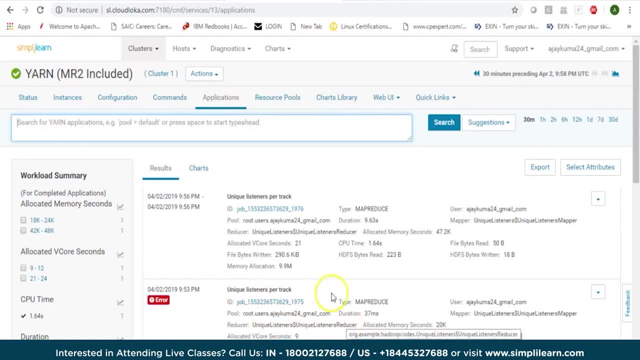 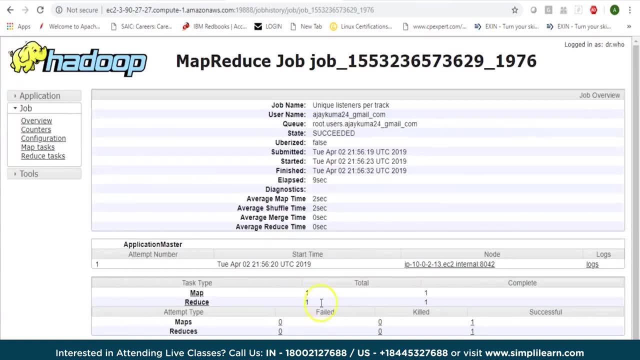 run. so this was the thing which failed earlier because of permissions, and this is the one which succeeded. now i have a job id which can always take me to the yarn UI, the history server, where i see how many map and jobs were run and for further information. 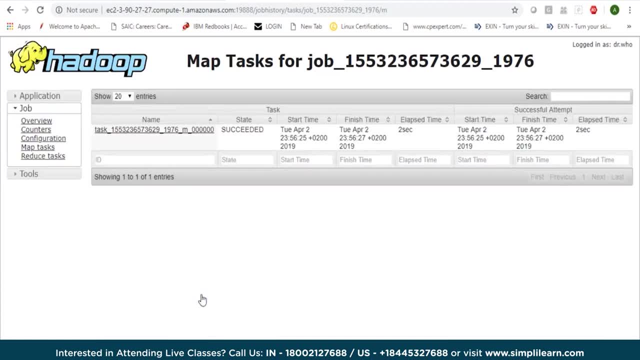 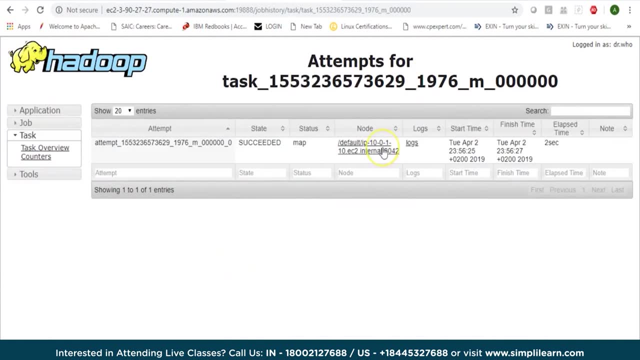 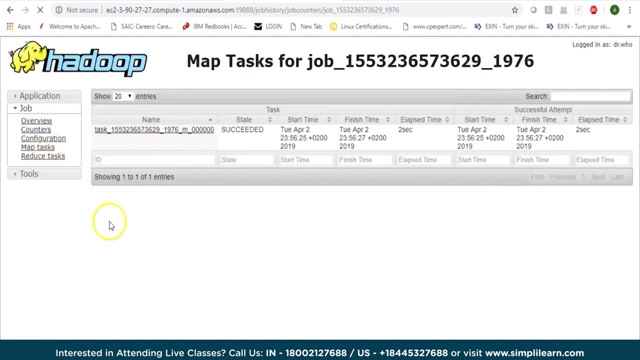 you can always go and look into the map and reduce tasks. so this was a map task which ran within a container which was allocated by your yarn, and we can also look on the node and logs what really happened. you can also look into the reduce task. you can also look at the counters. 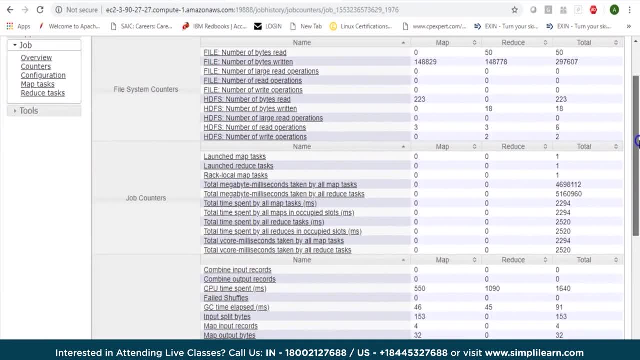 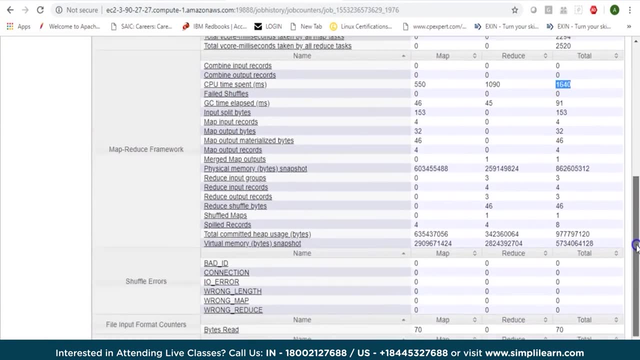 which we were seeing on the command line on how many map and reduce task, how many bytes were read, what was the garbage collection time, how much CPU time was spent in milliseconds. and you get all the counters here you can specifically be looking at counters for map or for reduce, so your 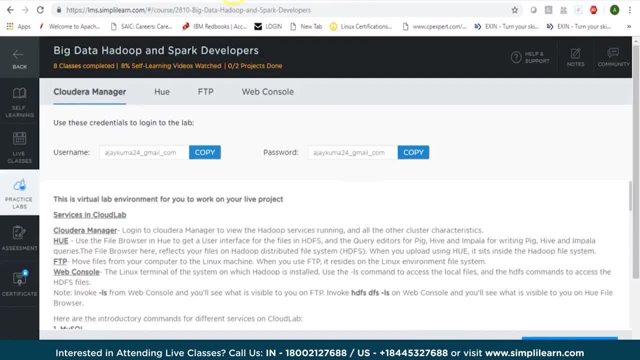 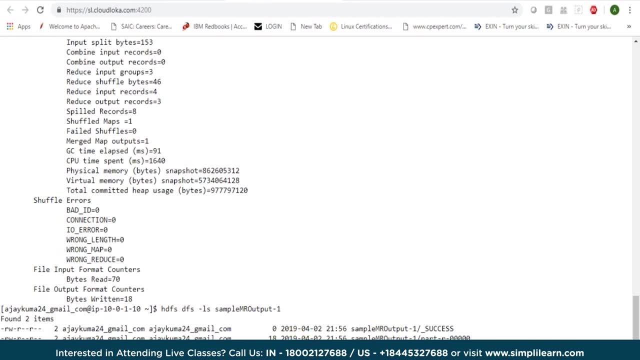 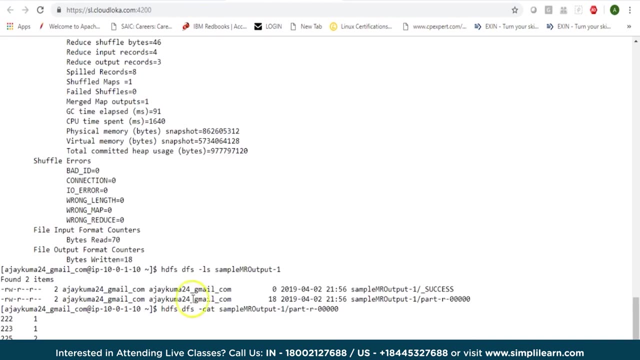 yarn UI helps you to look into for more information. now, if i go back to my console and i have the output file, i can basically look into it by selecting the output file and i can do a cat which basically will show me what is my output. so this is my map reduce. 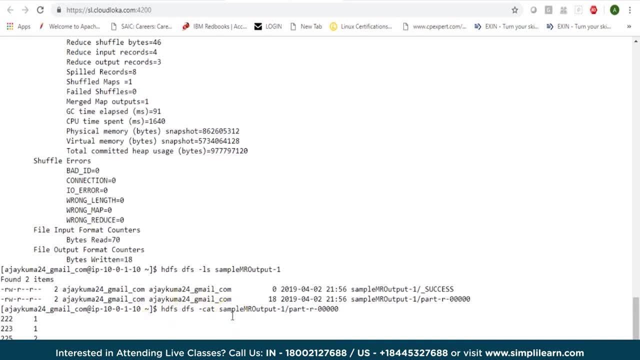 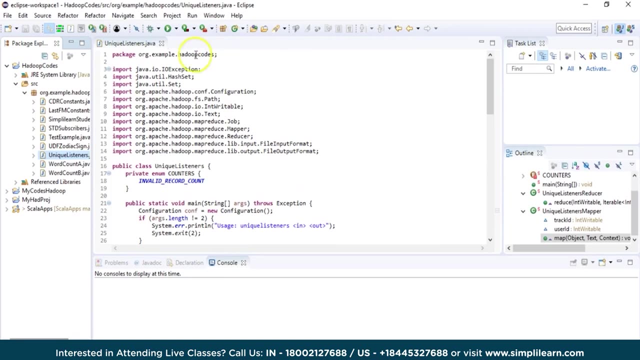 and basically what it has done has. it has aggregated and pulled out the information for your different listeners based on the data, what we have provided. let's look at one more example of using map reduce programming model to solve a real time business case or a problem. now the problem. 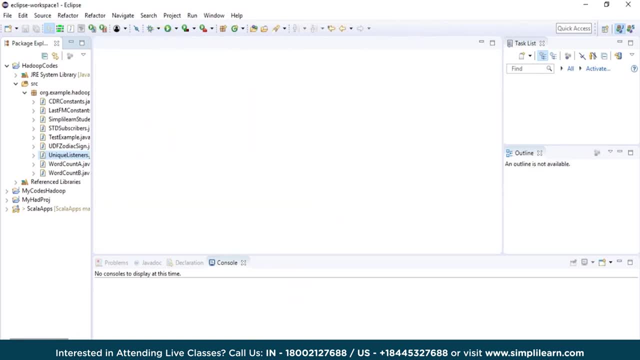 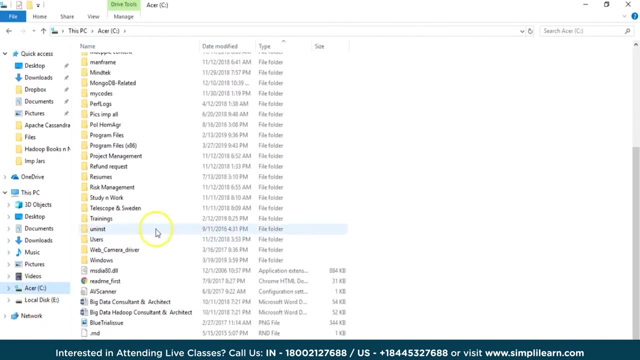 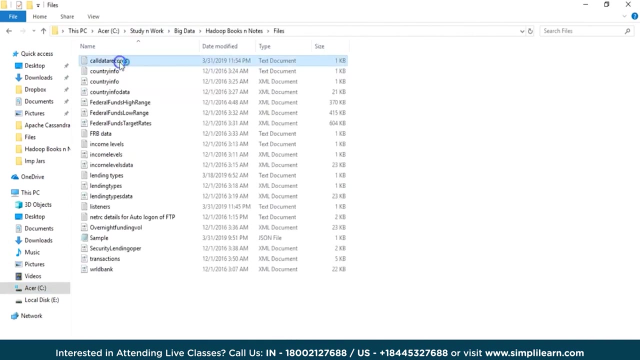 in hand is that we have some data collected from a telecom giant and basically we have some sample data here which lists the list of subscribers which are using the services. now, if i look into the file, i have call data records, which basically gives me information about the data. 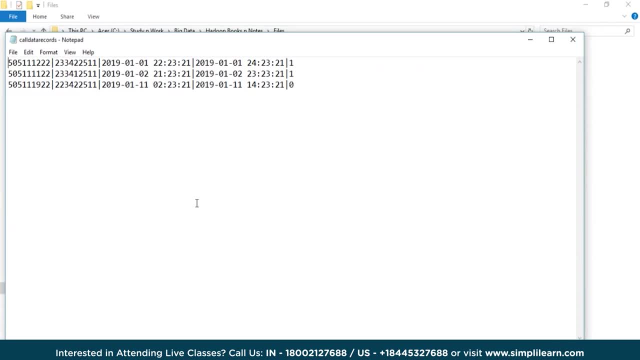 collected by a telecom company. so this telecom company keeps records of its subscribers and it calls this particular file as call data records. now, what does this call data records contain? it basically has a from phone number as the first field. it has the two phone number, that is. 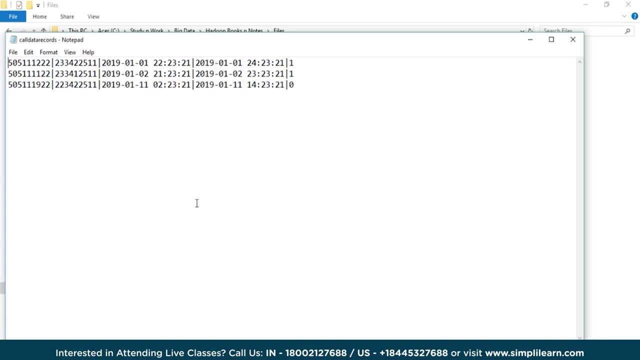 call being made to a particular number. then we have the call start time following a timestamp, you have a call end time and then we have, finally, if this call was a distance call or what we call as std call. now what we need to do is we need to use 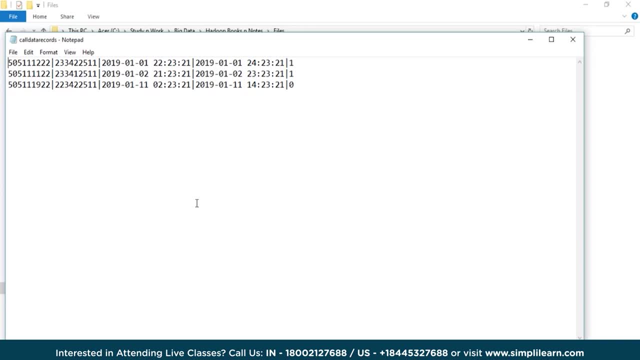 our knowledge of map reduce, we need to use the map reduce programming model and we need to come up with a code to find out all the phone numbers, for example, who were making more than 60 minutes of std calls. now, here, the flag one basically means it. 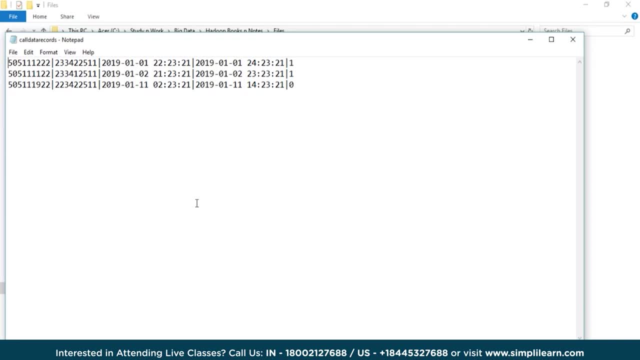 was an std call and zero means it was a local call. how do we do that? using map reduce. so this is again a problem where you would want to count through the data and you would want to aggregate the values to come up with result. so let's. 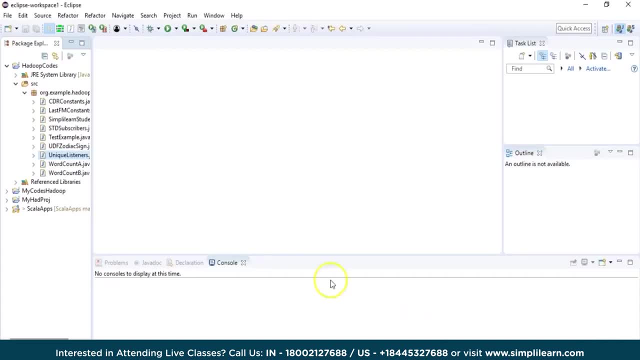 look at a sample code for this one. so here i have my eclipse and again, like a previous example, we are having a class which declares some constants for the fields. so you have phone number with zero, phone number with one call, start time, call end time and an std flag. 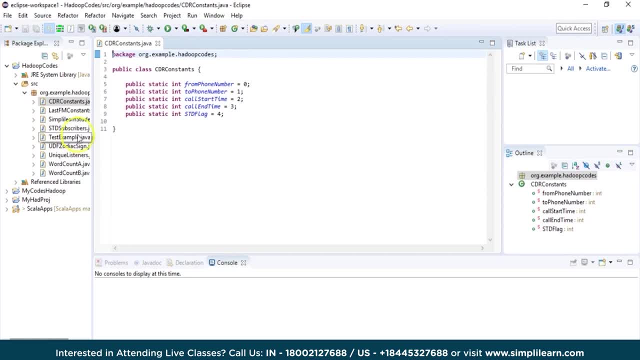 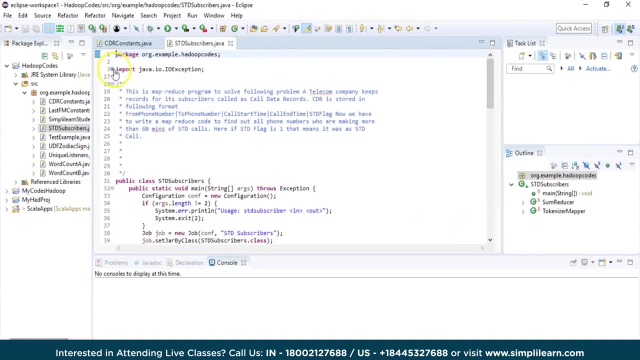 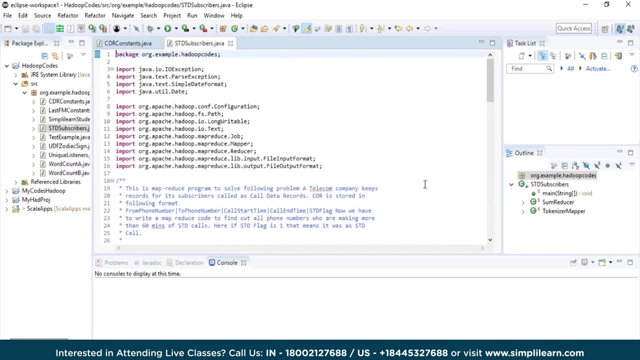 so these are the constants which i would be using in my code, and here is my main class which will use the map reduce, basically to solve this problem. now i'm importing the packages and, as i explained earlier, these packages are mainly to make sure that we can use the classes in our code. 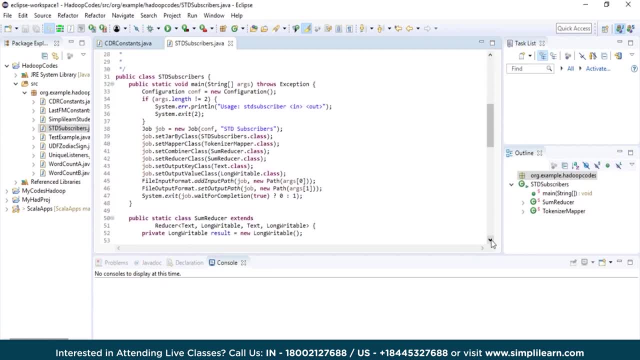 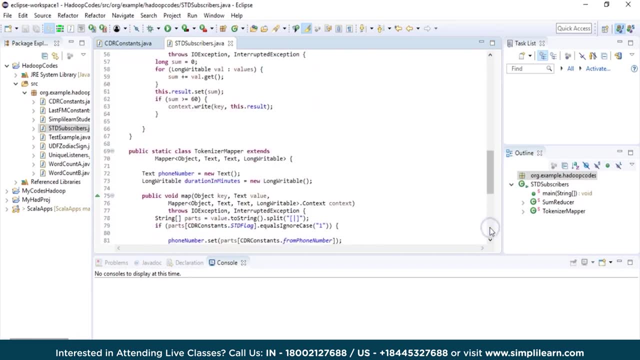 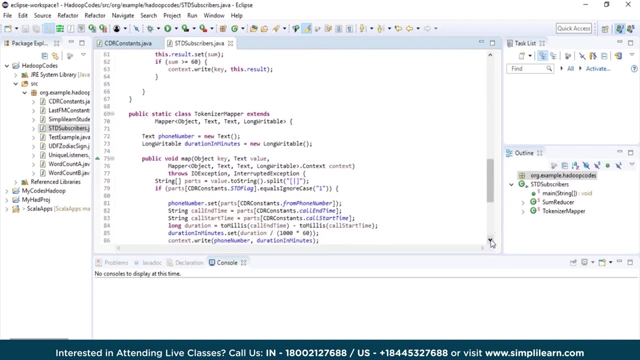 in the right way. so here now, the order of your driver class or your mapper and reducer does not matter, right? the first thing. what we need is we need a mapper which will do the map task. so here i'm creating a mapper which is tokenizer mapper and that extends. 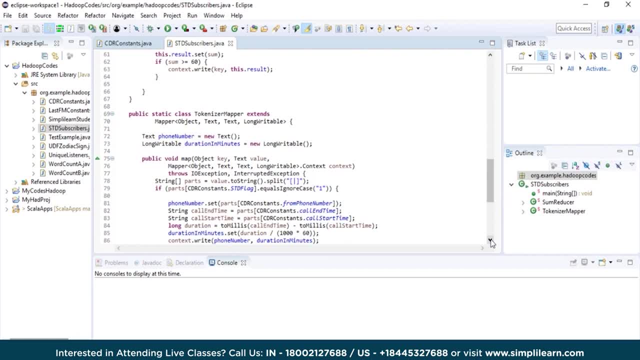 your mapper class. it accepts the data types, that is, object text and long writable, as explained earlier. these are your data types, which are hadoop specific, and data types like int, writable, long writable, boolean writable and many others depend on the writable and writable comparable interfaces. now here we. 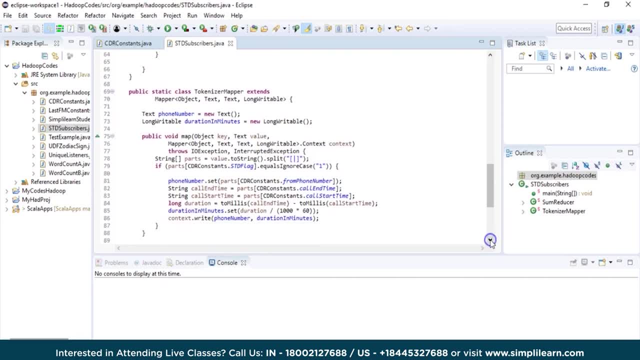 start with taking up our phone number. we basically also take duration in minutes. so these are the variables and i'm using the appropriate data type for those. then i start writing my map task. now what does my map task do? it basically works on the string which we have and it breaks. 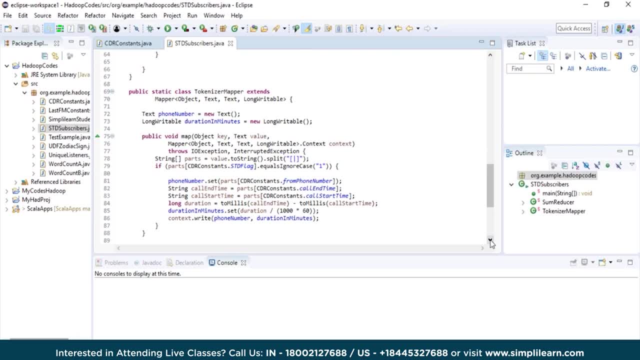 it into individual elements based on a delimiter. once that is done, then we are also checking if that particular string which we are looking for has a std flag, because we would want to find out how many customers, or how many of them, were making phone calls which were. 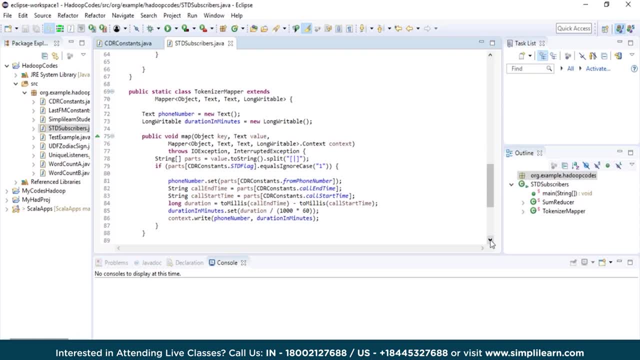 more than 60 minutes. and if these calls were std calls, then basically i work on the phone number and i set it using the cdr constants, for which we have already created a class using the phone number, call end time, call start time, and i also compute or calculate the long duration. 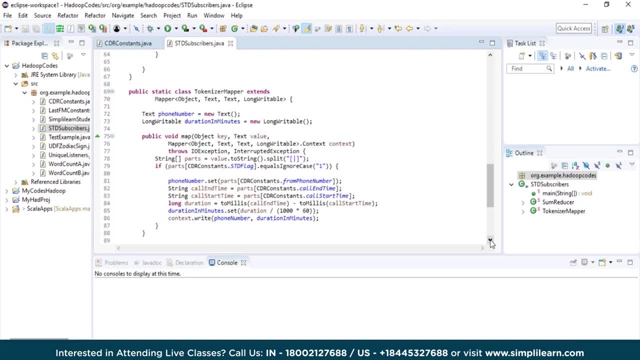 because we need to find out the calls which are more than 60 minutes. finally, we extract the phone numbers and the duration of the call made by a particular phone number. so this would be my mapper, giving an intermediate output which would then have to be sorted and shuffled, and then 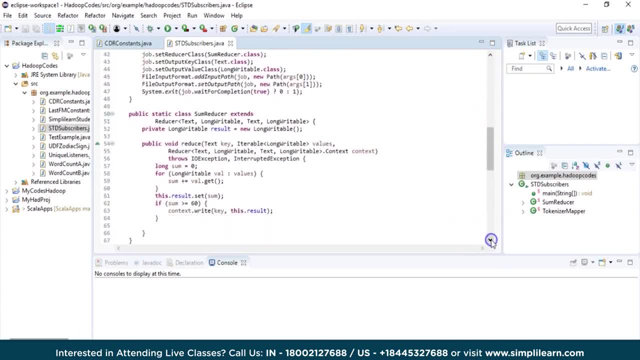 handed over to reducer. what does my reducer do? it uses the right data types. it basically starts with a sum as zero. it would look into all the keys and values and wherever it would find keys which are repeating and the duration is more than 60, it would give me. 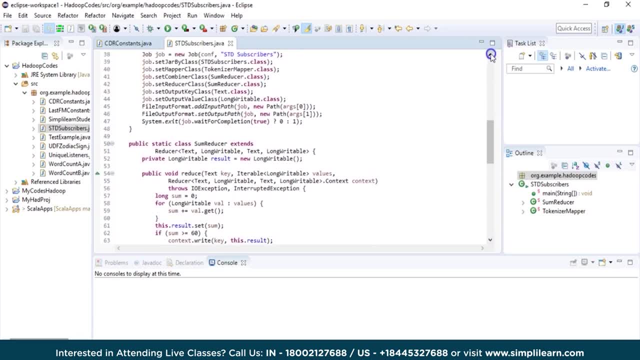 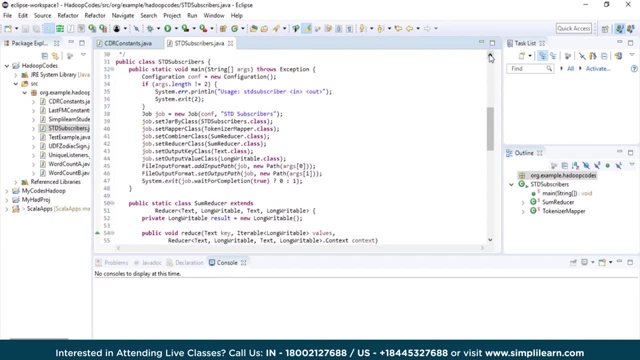 an aggregated result. this is my reducer. and finally, we have a driver, as i explained earlier, which has job configuration, your mapper reducer. and also we are using, just as an example, a combiner class which does not have a class of its own, but it is basically using the same. 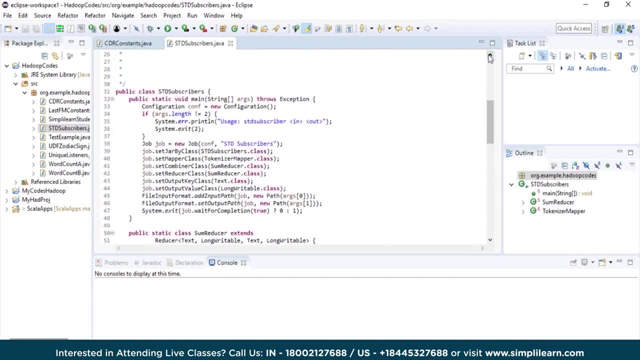 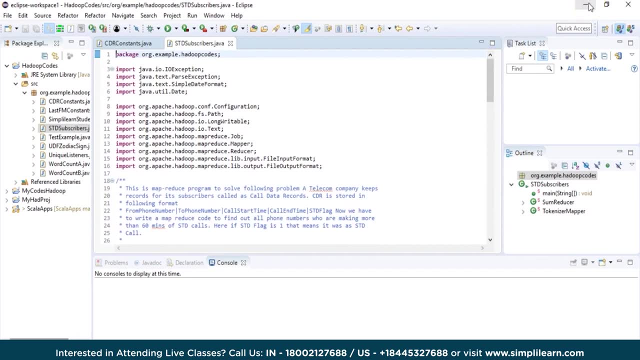 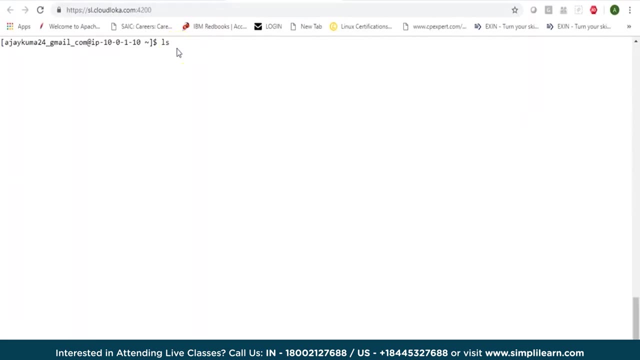 reducer class. once your code is ready, check if it compiles, check if you have all the dependencies met and package it as jar, transfer it to the cluster and run it with or on top of yarn. so what we can do is- i have already moved it here and we can look into- 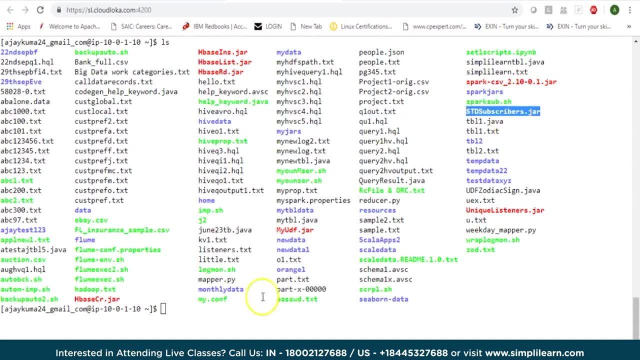 this machine. i already have my jar file, which basically also needs a input, which i have already pushed to my cluster so we can look in for the file which should be existing in sample mr in directory which is within my user and my name directory and i have the call data record. 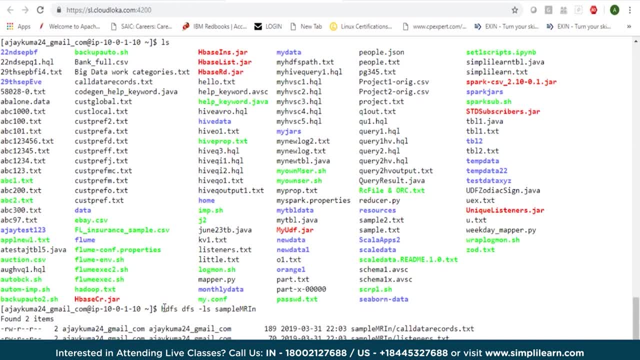 which basically shows the data which i was showing in the notepad file. now i can say hadoop jar and point it to my jar, which is std subscribers jar. we need to use the package, so i'll say org example: hadoop codes. that's my package and my class name. 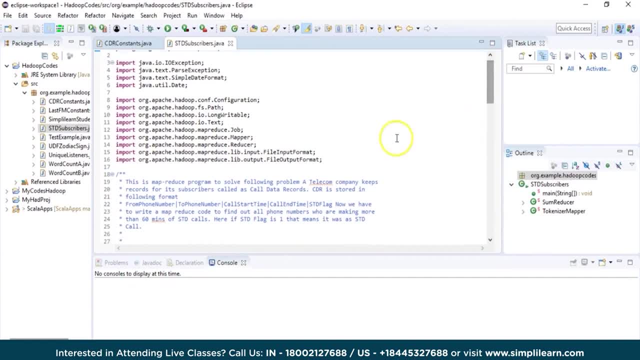 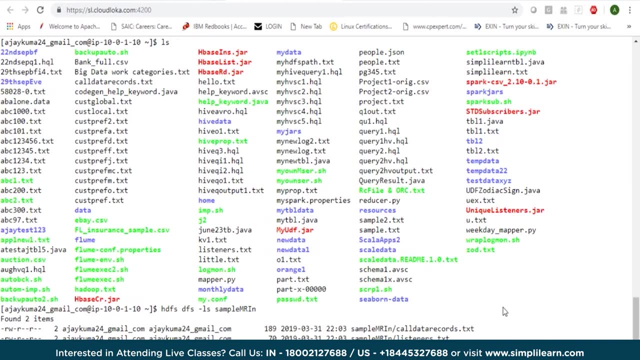 my class name is std subscribers, so i will say std subscribers, dot, and then you need to give your input. so we will say sample, mr in, and i will give in a particular file which is call data records, dot, txt, and then we can point it to an output directory. 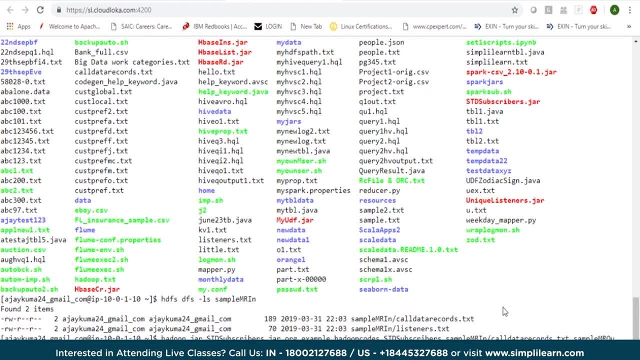 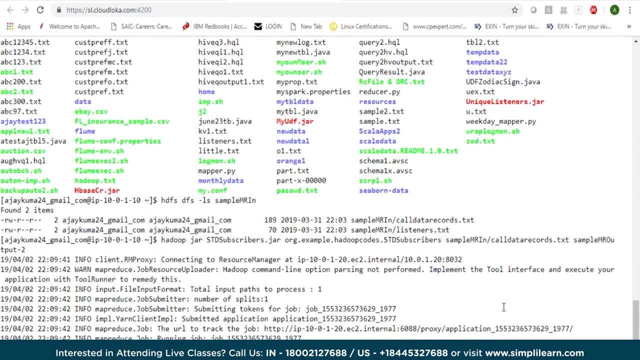 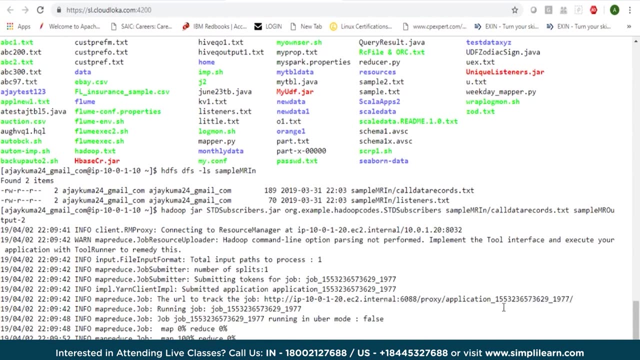 which will get created automatically. so i will say output two and that should have my result. and like we ran our first example, now i am again running it on one simple file. you can imagine this, as you can replace one single file with a directory which has multiple files. where might be the? 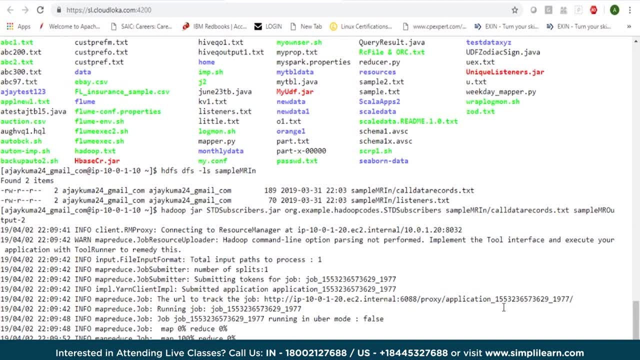 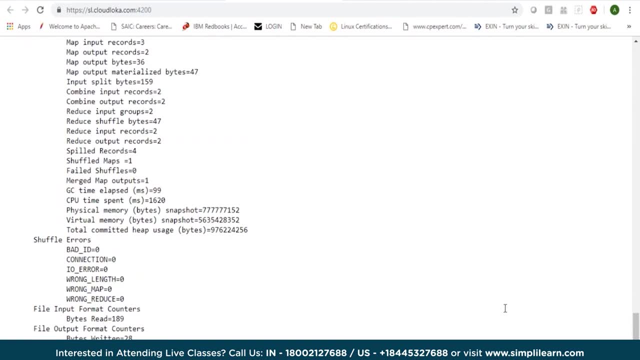 telecom company was already collecting data for couple of months and they would like to analyze this and you can run it in this way. so once this is done, we have our output, which can be seen by going into the directory saying sample mr output two and again this would have. 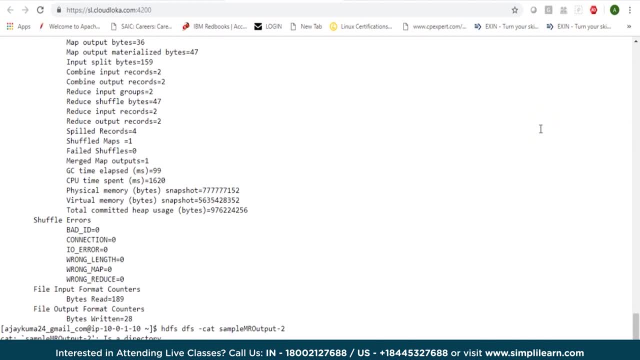 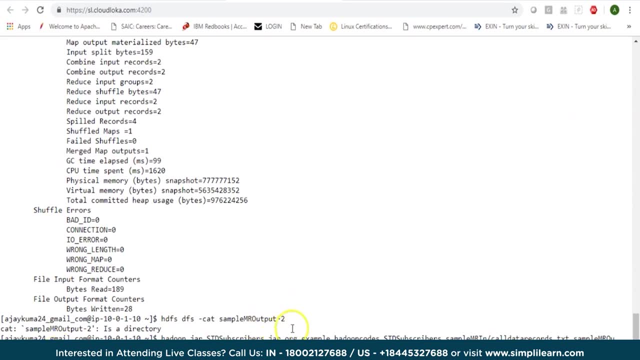 gone for one single reducer so we can look at whatever we gave as an output. so it was sample, mr. output two: and that is my directory. so since this is a directory, my cat command does not work on it. you need to give the file. so the command is by giving the. 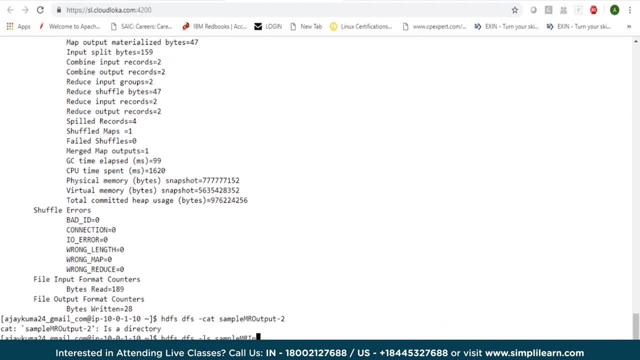 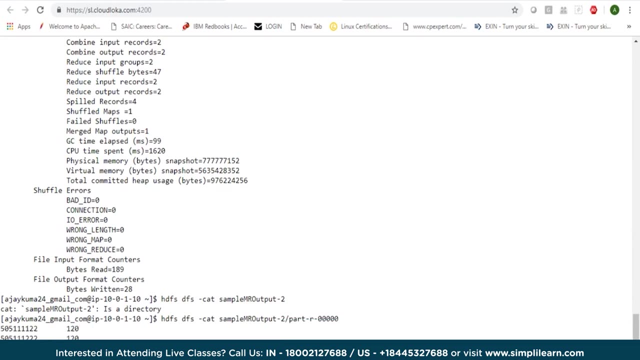 specific file, not by giving the directory, so it is cat sample: mr output: two slash part minus r, and then you can give five zeros and that should be my output, which should give me an information of which were the users or which were the phone numbers which made calls. 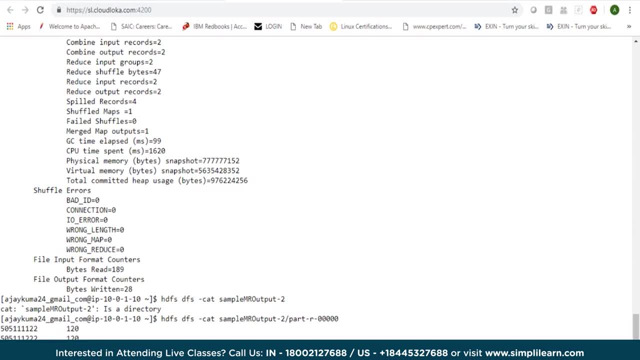 greater than 60 minutes and if these calls were std calls and what was the duration of the call. so this is how you can use MapReduce programming model to solve your real time business cases. always remember you have to code and create your mapper and reducer function and rest. 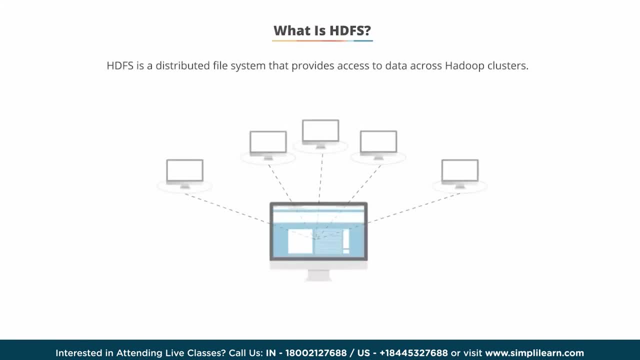 will be done by the framework. what is HDFS? HDFS is a distributed file system that provides access to data across Hadoop clusters. a cluster is a group of computers that work together. like other Hadoop related technologies, HDFS is a key tool that manages and 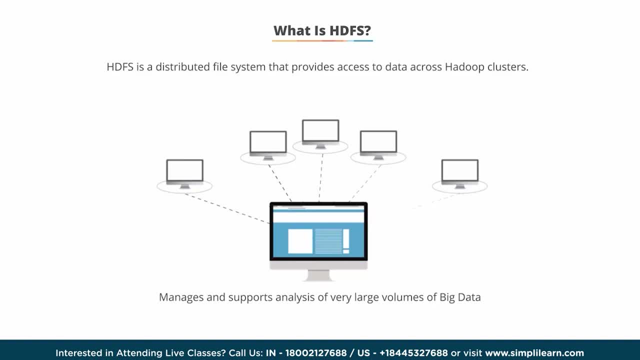 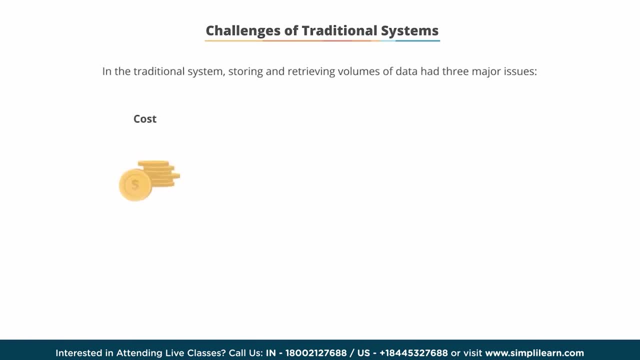 supports analysis of very large volumes- petabytes and even zettabytes- of data. some of the challenges of traditional systems are cost, speed and reliability. the traditional file system costs approximately ten thousand to fourteen thousand dollars per terabyte. searching and analyzing data was time consuming and expensive. also, 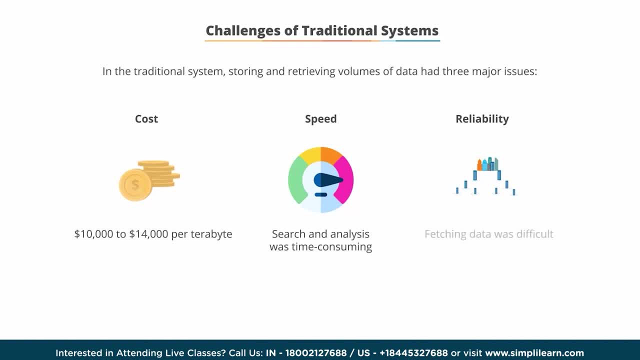 if search components were saved in different servers, fetching data was difficult. need for HDFS: HDFS resolves all the three major issues of the traditional file system. let's discuss how it does that one cost. HDFS is an open source software package, so it can be used with zero licensing. 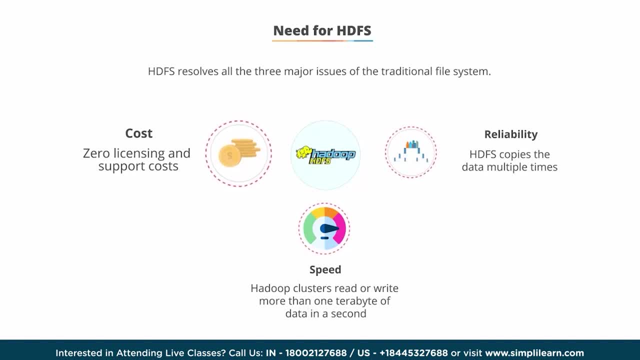 and support costs. it is designed to run on a regular computer speed. large Hadoop clusters can read or write more than a terabyte of data per second. a cluster comprises multiple systems logically interconnected in the same network. HDFS can easily deliver more than two gigabytes. 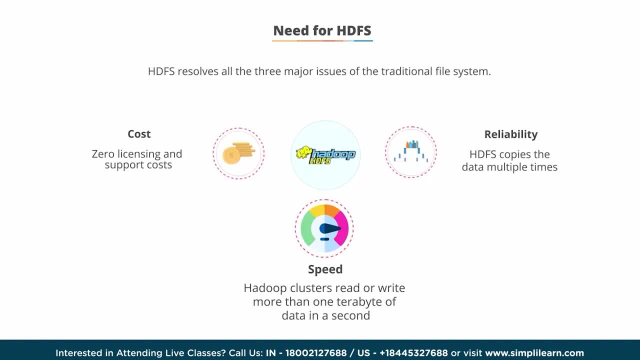 of data per second per computer to MapReduce, which is a data processing framework of Hadoop reliability. HDFS copies the data multiple times and distributes the copies to individual nodes. a node is a commodity server which is interconnected through a network device. HDFS then places at least 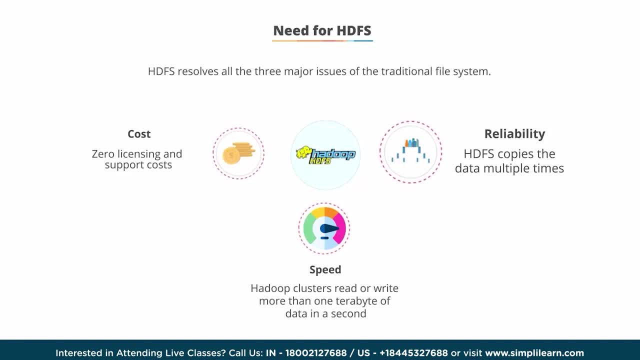 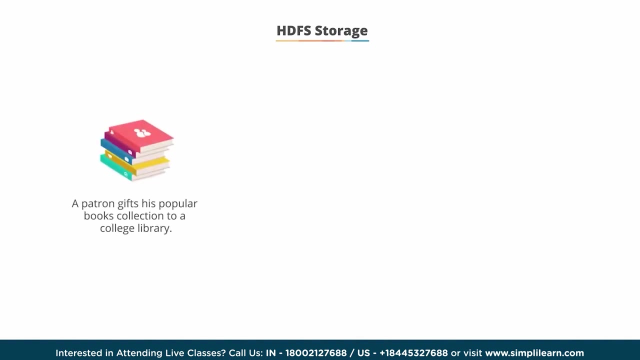 one copy of data on a different server. in case any of the data is deleted from any of the nodes, it can be found within the cluster. let's understand how HDFS stores files with an example: a librarian gifted a collection of popular books to a college library. 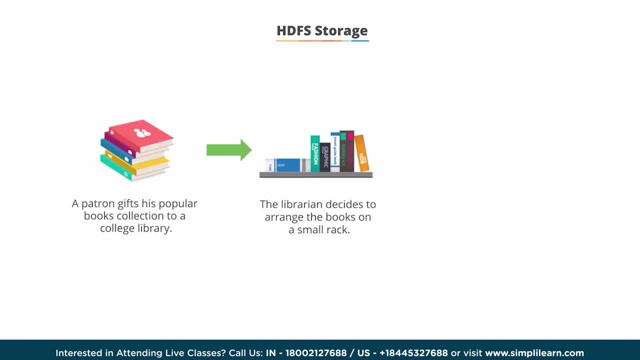 the librarian decided to arrange the books on a small rack and then distribute multiple copies of each book on other racks. this way, the students could easily pick a book from any of the racks. similarly, HDFS creates multiple copies of a data block. we see that a regular file system. 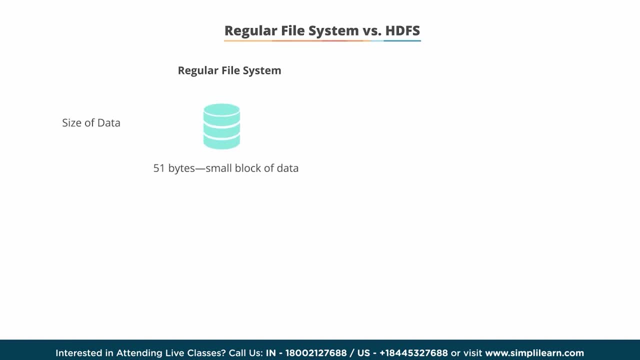 data size is 51 bytes- a small block of data, whereas HDFS, when it writes a block, is 128 megabytes, which is a large block of data. the small regular file system blocks suffer from disk IO problems, primarily because of multiple seek operations it takes to retrieve so many small blocks. 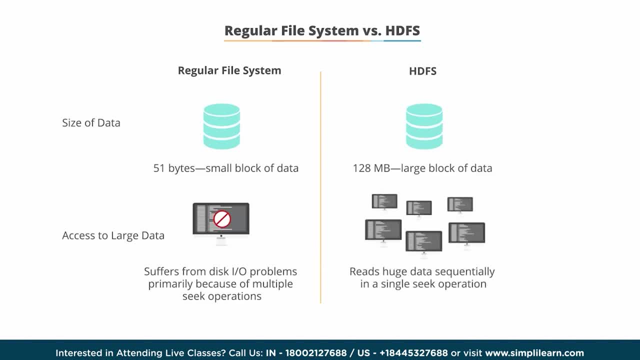 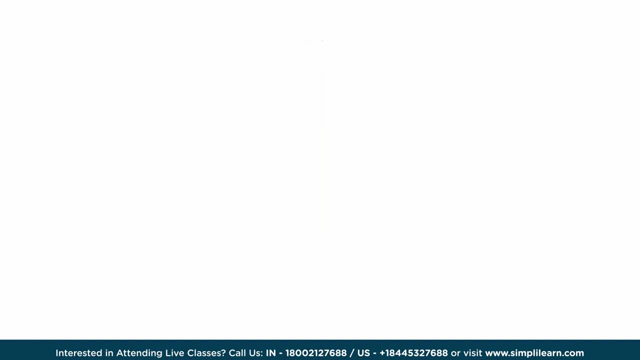 the HDFS file system has a very large block which requires many fewer reads and writes. so the reads huge data sequentially in a single seek operation, thus dramatically speeding up the read of the HDFS file system. HDFS storage. let's take a look at HDFS storage. 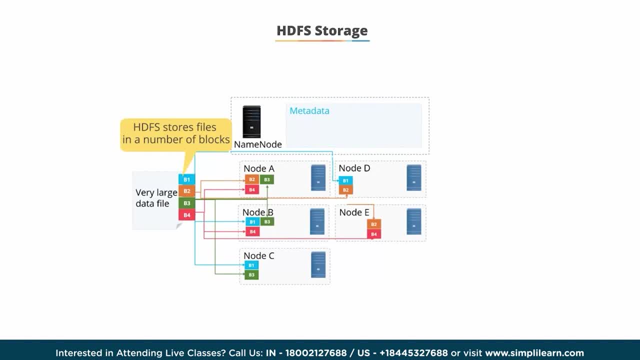 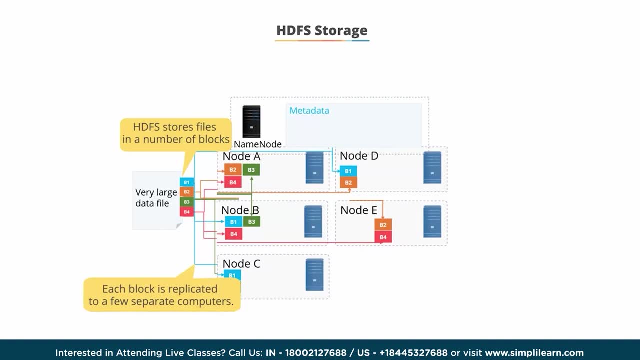 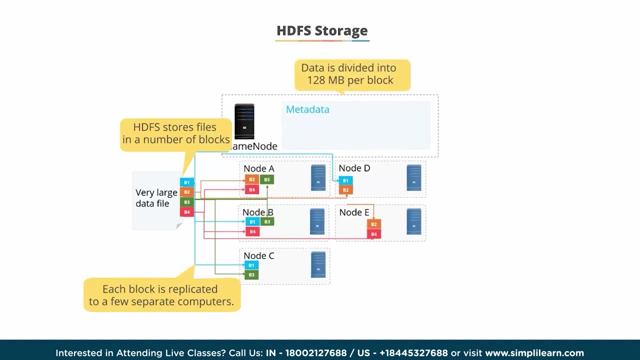 and how it works. HDFS stores files in a number of blocks. each block is replicated to a few separate computers. however, the count can be modified by the administrator. data is divided into 128 megabytes per block and then replicated across local disks of the cluster nodes. 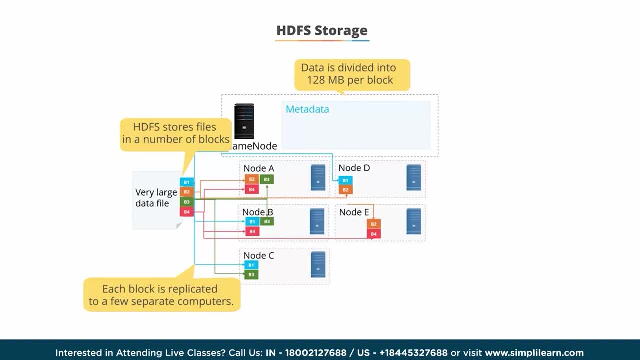 HDFS is a storage system for both input and output of MapReduce jobs. the metadata controls the physical location of a block and its replication within the cluster. the metadata is stored in something called a name node. so what are the characteristics of HDFS? we have fault tolerance. 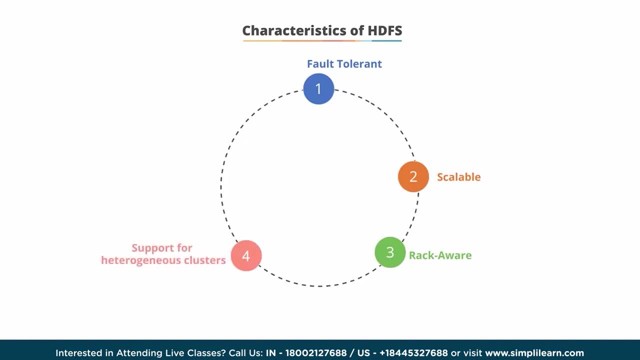 scalability, rack awareness, support for heterogeneous clusters and built for large data sets. so HDFS does provide this scalable, fault tolerant rackware storage designed to be deployed on commodity hardware. let's look at the first characteristic: fault tolerance. HDFS is designed with hardware failure in mind: data in a Hadoop cluster. 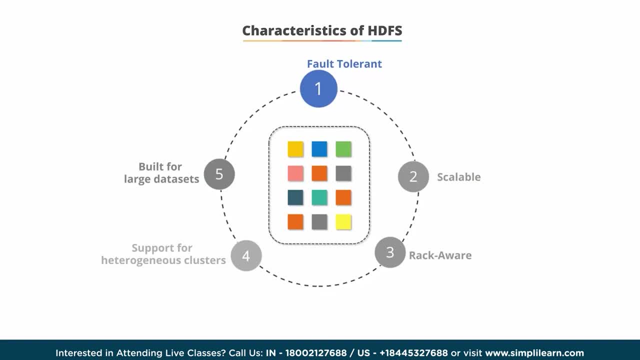 is called blocks. these are then duplicated and distributed throughout the cluster. since the data has been replicated, it is highly available and fault tolerant. the default replication factor is three. this can be changed upwards or downwards by an administrator. number two is scalability. when requirements increases, we can scale the existing cluster. 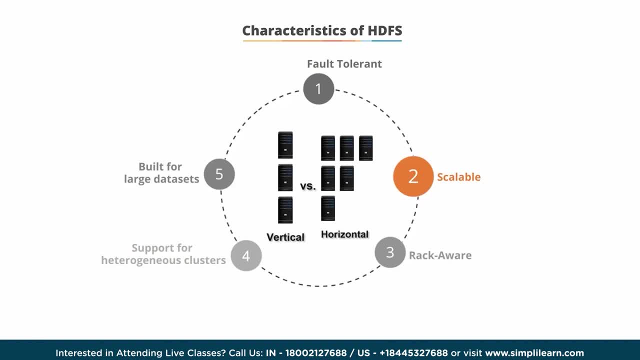 there are two scalability mechanisms available: one for larger hardware and horizontal, which provides an unlimited supply of computing added to the cluster. three is rack aware. a rack is a collection of machines, typically around 40 to 50, which are connected using the same network switch. if that entire network goes down. 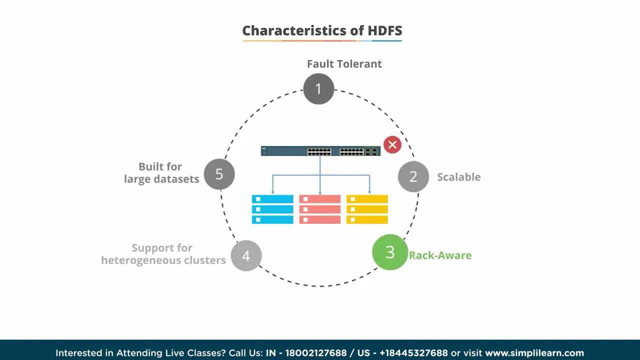 then all machines in that rack will be out of service. rack awareness is a concept introduced by Hadoop Cloud to address this issue. rack awareness achieves two things: one, by increasing the availability of a data block across multiple racks and two, better cluster performance by segmenting the read operations. 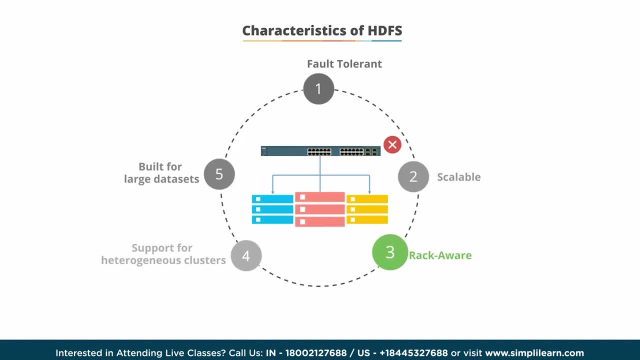 across multiple racks. communication between two data nodes on the same rack is more efficient than the same between two nodes on different racks, so information about the location of the cluster is stored in the name node. we'll be learning more about the name node, which holds our metadata. 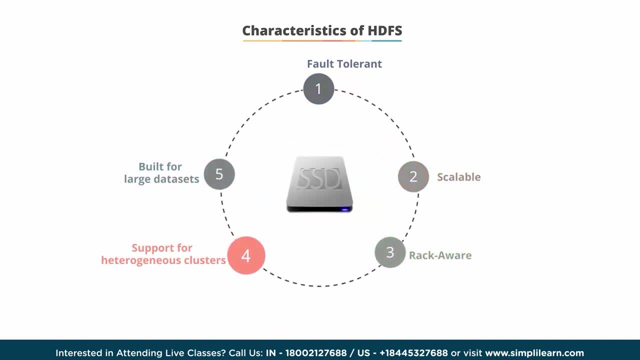 when we discuss the HDFS architecture before. HDS supports a variety of storage types to optimize data usage and lower costs. based on data usage frequency. you can configure each data directory with a storage type, such as SSDs for improved performance, archival storage for very dense and rarely accessed data. 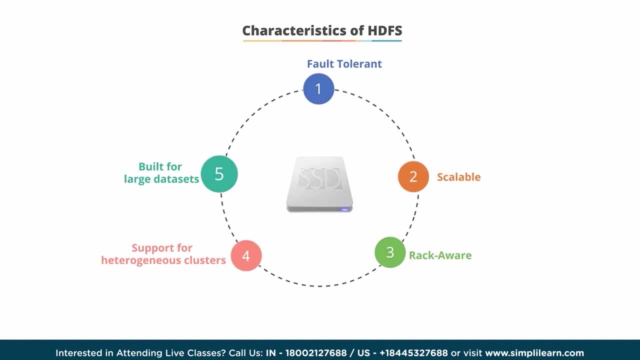 and so on. HDFS is meant to handle large files, ie in terabytes and petabytes of data. HDFS splits huge files into smaller chunks, known as data blocks, and requests for these blocks to go across a network and come without a lot of overhead. 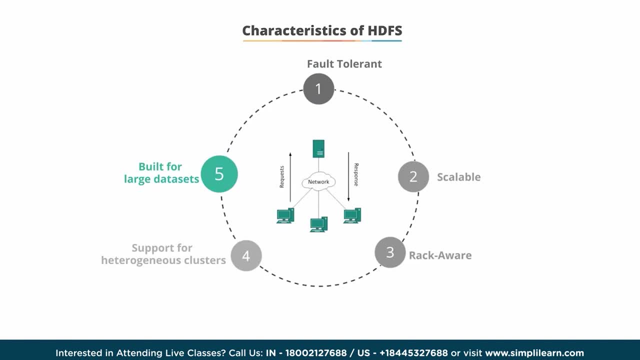 the size of the data block is very important concern in such scenarios. having a small block size can help you figure out where that block can be found, thereby increasing the network traffic, and having a very large block size can result in longer data processing times. to overcome both these scenarios, 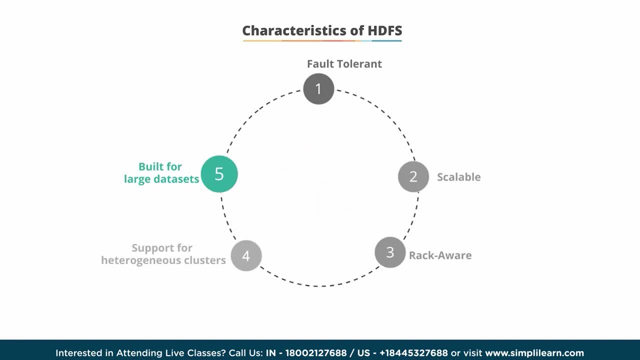 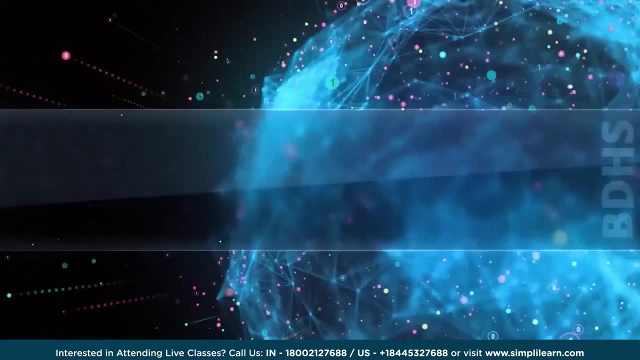 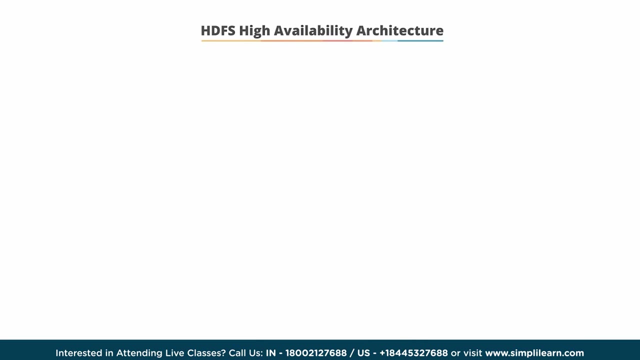 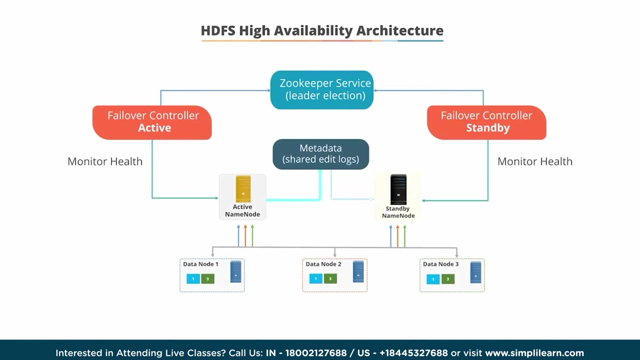 the default size of the HDFS block is 128 MB, which can also be configured up or down per your requirements. HDFS Architecture and Components: HDFS has a high availability architecture. broadly, HDFS has a master-slave architecture, so how does it work in a typical HA cluster? 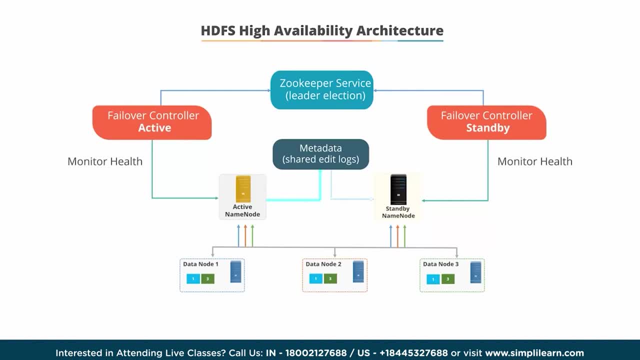 two or more separate machines are configured as name nodes. at any point in time, exactly one of the name nodes is in an active state and all the others are in a standby state. the active name node is responsible for all client operations in the cluster, while the standby 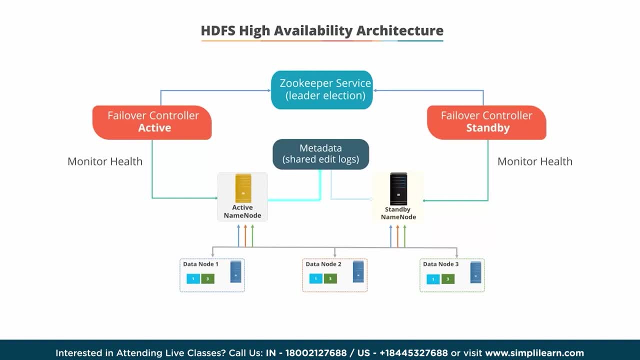 slave, maintaining enough state to provide a fast failover if necessary. the master node, that is, the name node, ensures that the data required for the operation is loaded and segregated into chunks of data blocks in slave nodes as data nodes. a data node serves read or write requests. 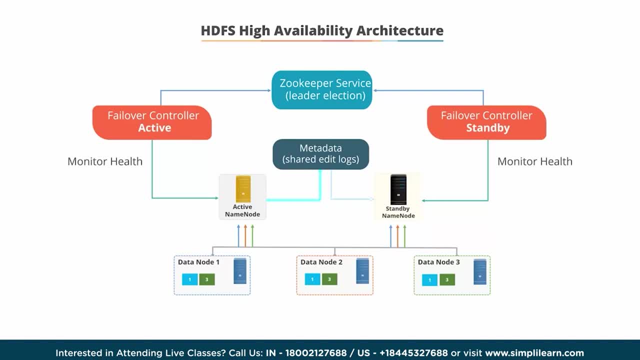 it also creates, deletes and replicates blocks based on the instructions from the name node. the active name node and the active name node keep in sync with each other through shared edit logs or metadata. the active name node updates the edit logs, which is the metadata information. 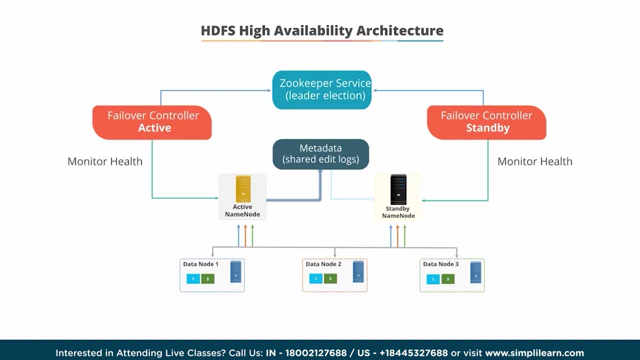 about the storage. this is done with namespace modifications like block locations, status of the name node and so on. the standby node reads the changes made to the edit logs in a consistent manner. in the event of a failover, the standby will ensure that it has read all the edits. 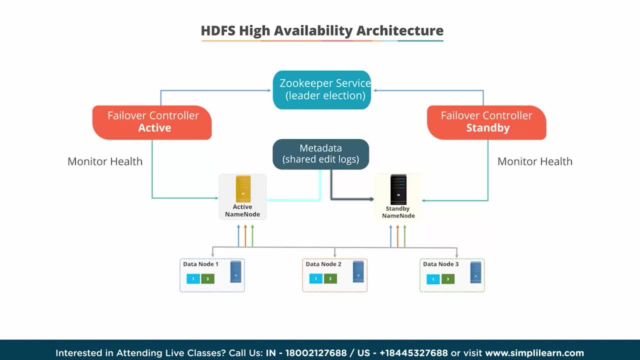 before promoting itself to the active state. note that this is a manual failover process which has to be performed by an admin. for an automatic failover, we will need to utilize services of Apache Zookeeper, which maintains small amounts of coordination data and a lot of data. 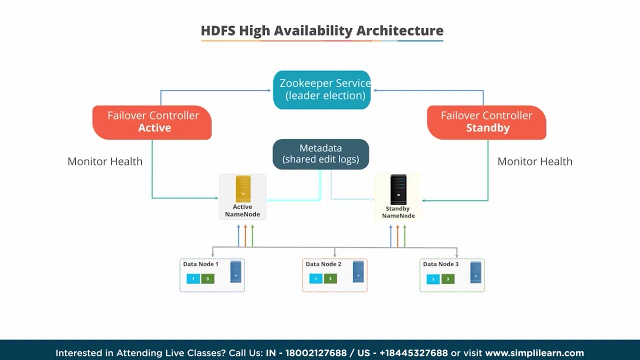 the health monitor, or ZKFC, keeps an open session with the active name node by periodically pinging it with a health check command. if the node has crashed, frozen or otherwise entered an unhealthy state, the health monitor will mark it as unhealthy and elect a new name node. 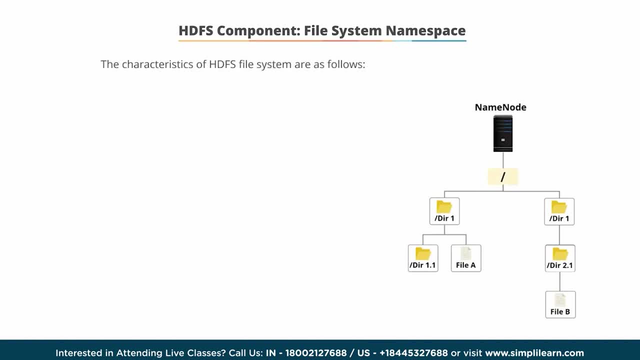 a key component of HTFS is the file system namespace itself. HTFS exposes a file system namespace and allows user data to be stored in files, much like we're used to in traditional operating systems. the HTFS does use a hierarchical file system that does include directories. 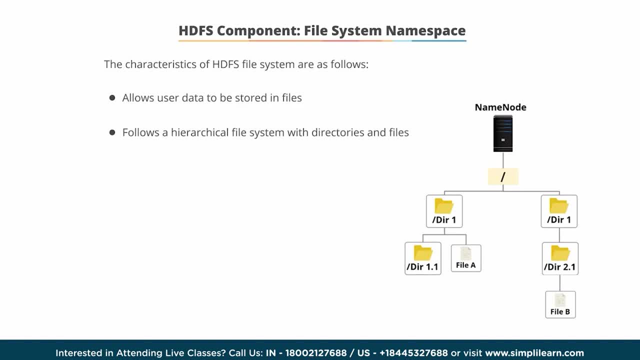 and files within those directories. the name node manages the file system namespace, allowing clients to work with files and directories. a file system supports operations like create, remove, move and name. the name node, apart from maintaining the file system namespace, records any change to metadata information, name node operation. 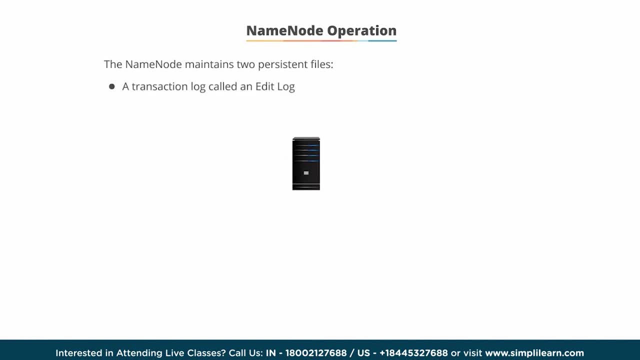 the name node maintains two persistent files: a transaction log called an edit log, and a namespace image called an FS image. the edit log records every change that occurs in a new file. the name node's local file system stores the edit log, the entire file system namespace, including mapping of blocks. 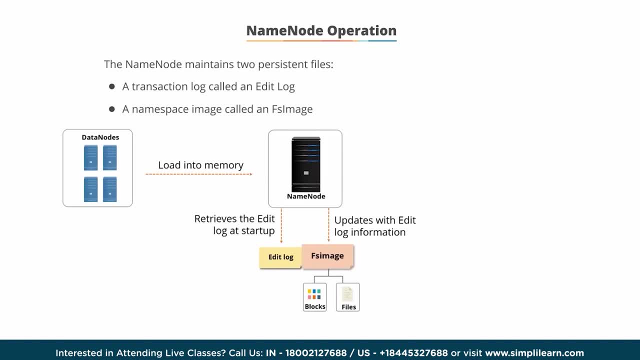 files and file system properties is stored in FS image. this is also stored in the name node's local file system. when new data nodes join a cluster, metadata loads the blocks that reside on a specific data node into its memory at startup. metadata then periodically loads the data at user defined 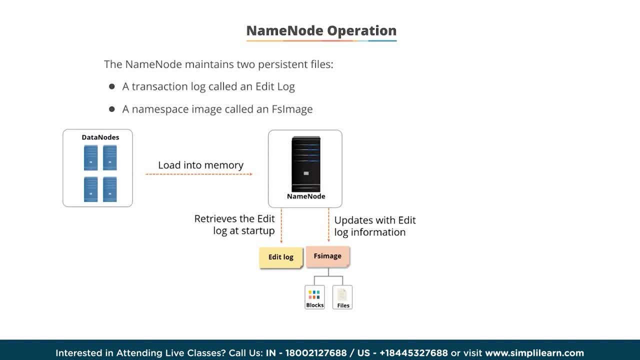 or default intervals. when the name node starts up, it retrieves the edit log and FS image from its local file system. it then updates the FS image with edit log information and stores a copy of the FS image on the file system as a checkpoint. the metadata size is limited. 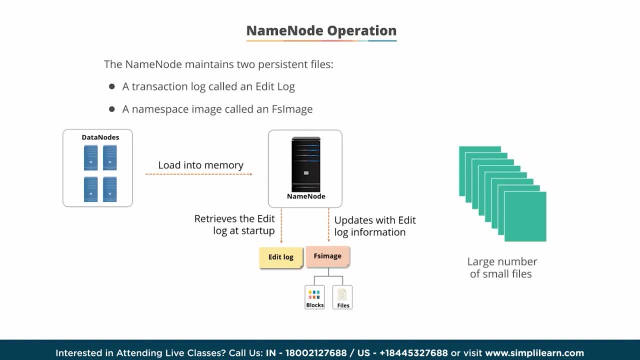 on the name node. a large number of small files would require more metadata than a small number of large files. hence the in-memory metadata management issue explains why HDFS favors a small number of large files. if a name node runs out of RAM, it will crash and the applications 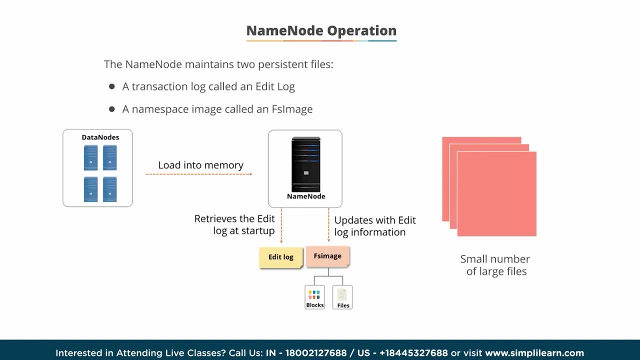 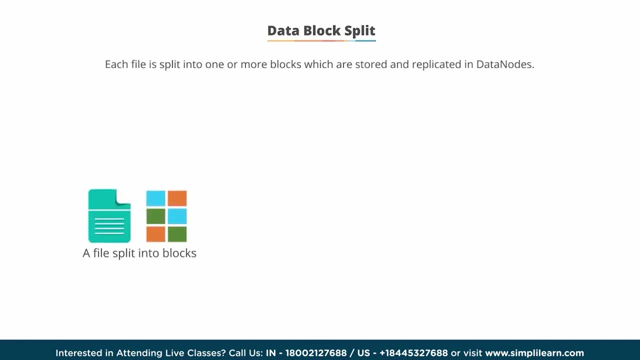 will not be able to use HDFS until the name node is operational again. data block splitting: each file is split into one or more blocks which are stored and replicated in data nodes. the data block split is an important process of the HDFS architecture, as discussed earlier. 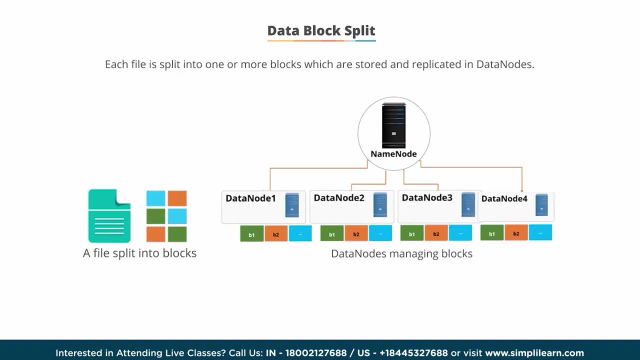 each file is split into one or more blocks, stored and replicated in data nodes. data nodes manage names and locations of file blocks. however, this potentially reduces the amount of parallelism that can be achieved, as the number of blocks per file decreases. each map task operates on one block. 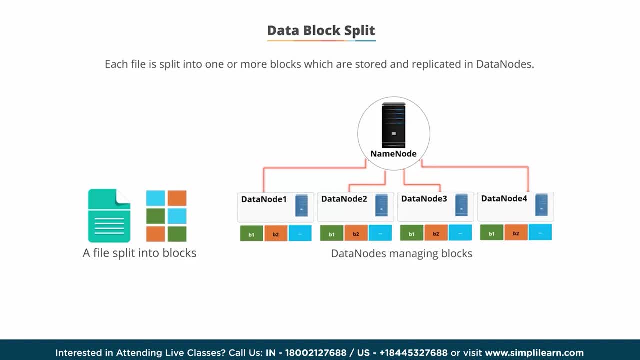 so if tasks are lesser than nodes in the cluster, the jobs will run slowly. however, this issue is smaller when the average map reduce job involves more files or larger individual files. let's look at some of the benefits of the data block approach. the data block approach provides. 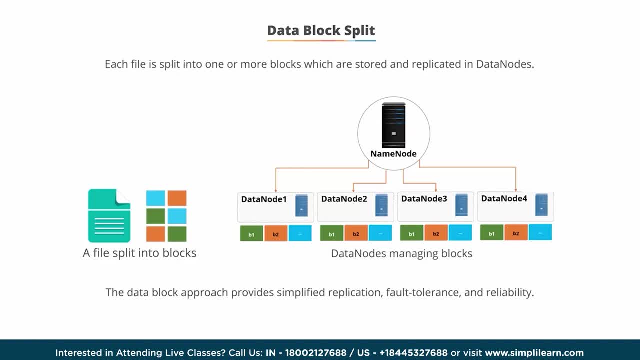 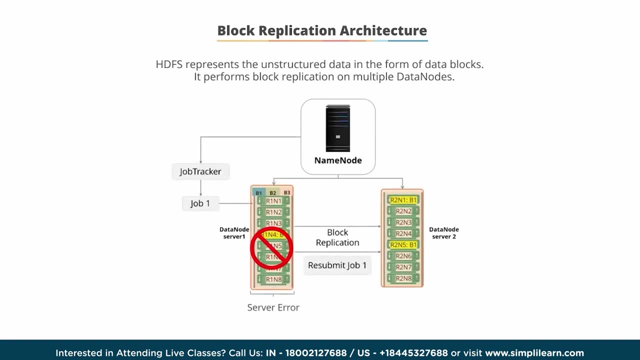 simplified replication, fault tolerance and reliability. it also helps by shielding users from storage subsystem details. the block replication architecture: block replication refers to creating copies of a block in multiple data nodes. usually the data is split into two parts, such as part dash zero and part dash one. HDFS performs block replication. 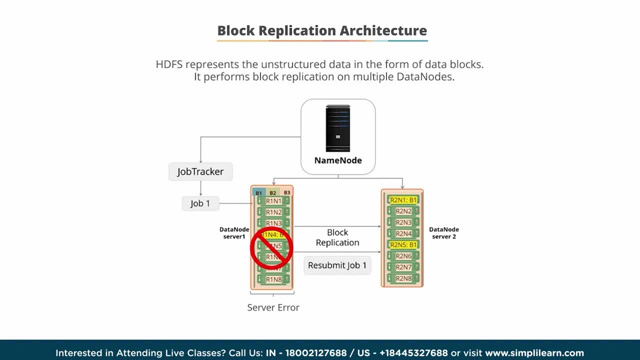 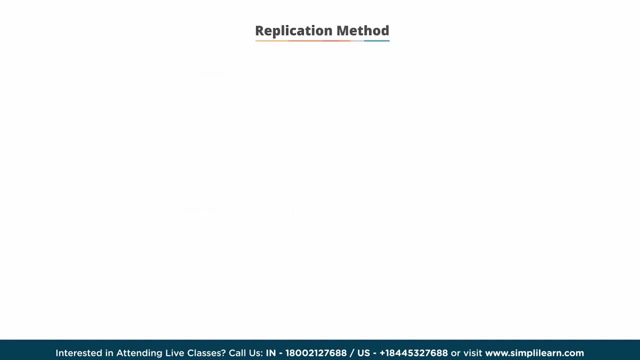 on multiple data nodes so that if an error exists on one of the data node servers, the job tracker service will resubmit the job to another data node server. the job tracker service is present in the name node server. let's now look at the replication method used. 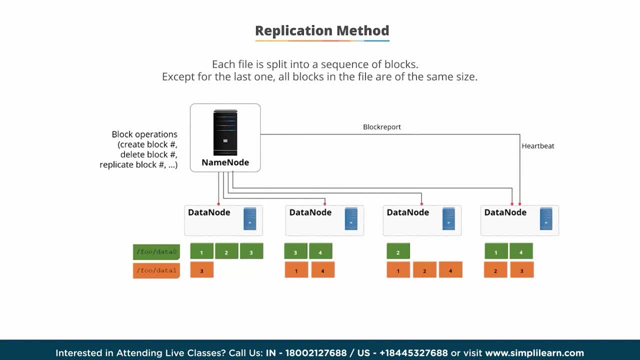 in the replication method in the sequence of blocks, all blocks except the last one in the file are of the same size. blocks are replicated for fault tolerance. the block replication factor is usually configured at the cluster level, but it can be configured at the file level. the name node receives. 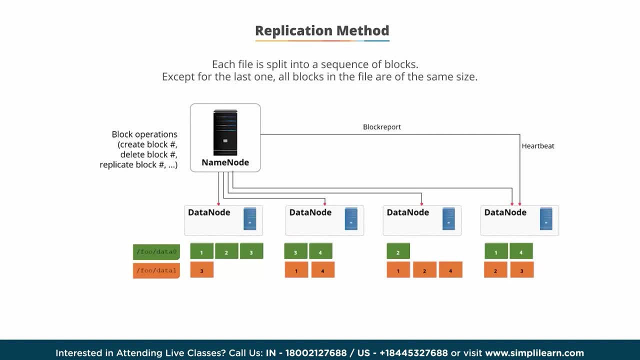 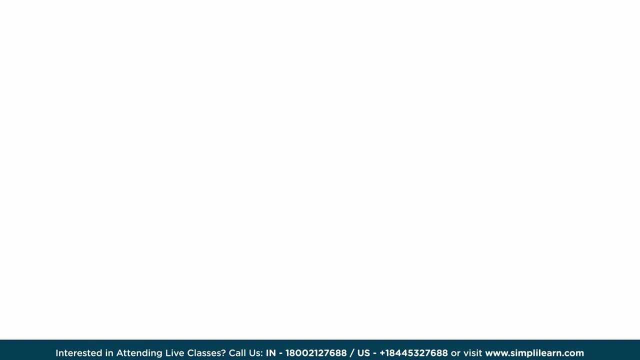 a heartbeat and a block report from each data node in the cluster. the heartbeat denotes that the data node is functioning properly. list the blocks on a data node. we also have a data replication topology. the topology of the replica is critical to ensure the reliability of HDFS. 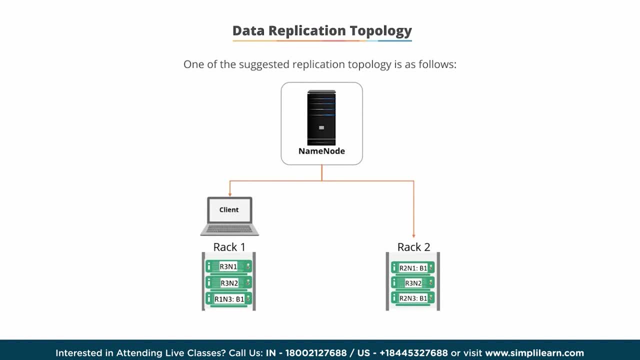 usually each data is replicated three times, where the suggested replication topology is as follows: one, place the first replica on the same node as that of the client. two, place the second replica on a different rack from that of the first replica. and three, place the third replica. 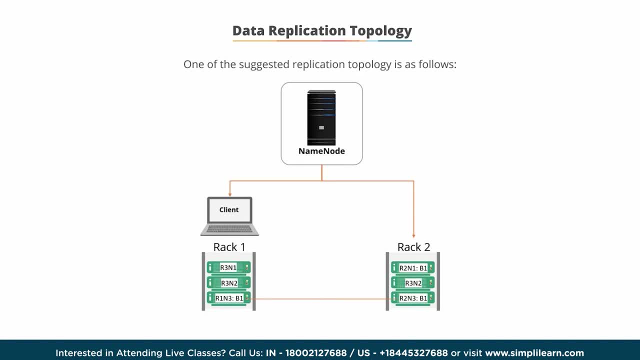 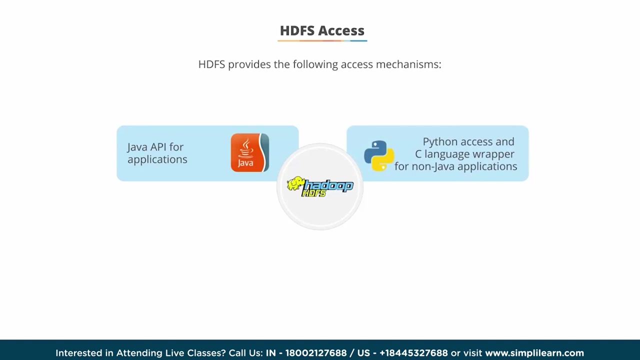 on the same rack as that of the second one, but on a different node. all of this achieves high accessibility and fault tolerance. HDFS access: HDFS provides various access mechanisms. a Java API can be used for applications on, and a C language wrapper for non-Java applications. 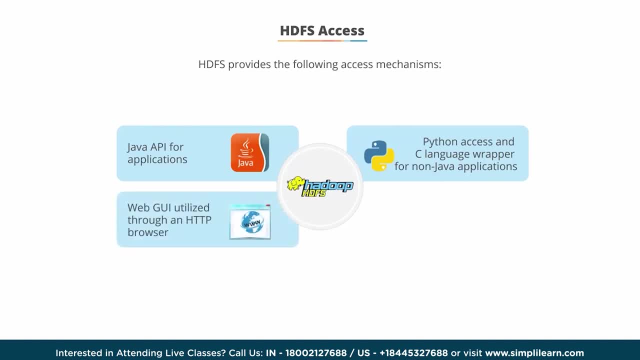 a web GUI can also be utilized through an HTTP browser, and an FS shell is available for executing commands at the file system level. on HDFS, let's look at the commands for HDFS in the command line interface. following are a few basic command lines of HDFS: 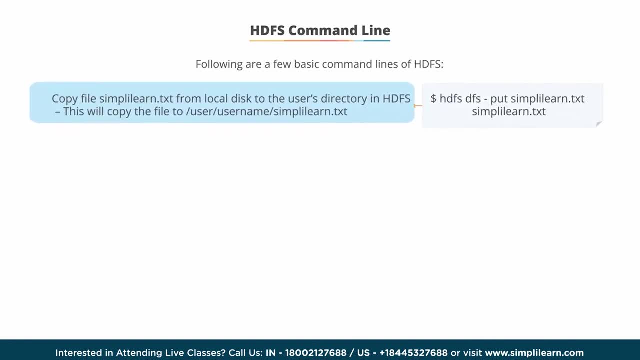 in order to copy the file simplylearntxt from the local disk to the user's directory, type the command line shown on the screen, and here you see the command hdfs, dfs-put simplylearntxt to simplylearntxt. this will take the file and copy it. 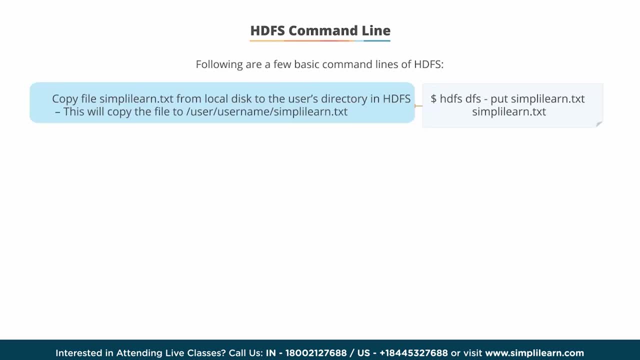 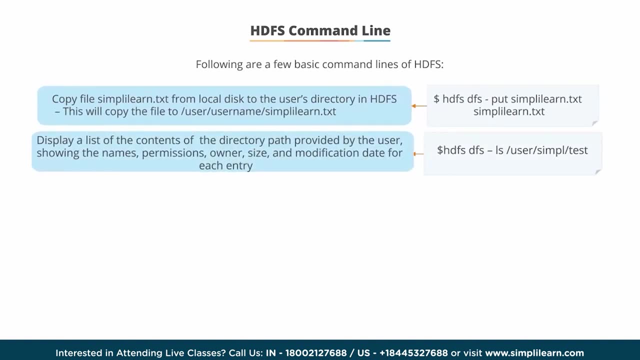 to slash: user slash- username, slash- simplylearntxt. to get a directory listing of the user's home directory. type the command line shown on the screen. in this case, we type in: hdfs, dfs, dash, ls. slash- user, slash- simple, slash test. in order to create a directory. 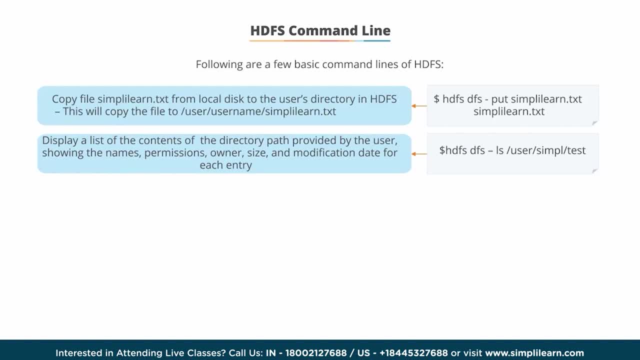 called testing under the user's home directory. type: hdfs, dfs, dash, mkdir, slash, user slash. simple slash test to delete the directory testing and all of its contents. type the command line: hdfs, dash, rm, dash, r, and testing. remember that when you are copying files, you are copying a file. 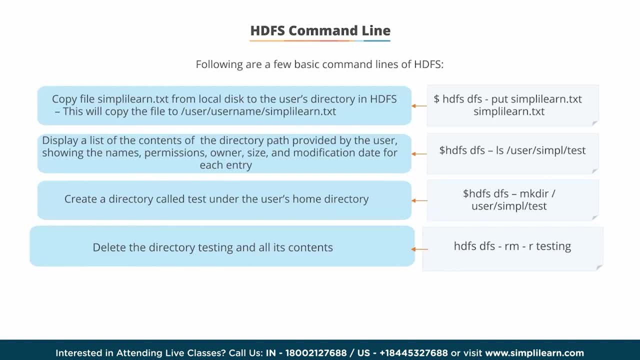 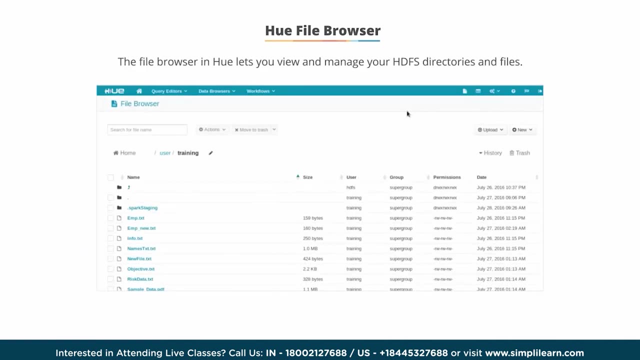 from your local file system into the hdfs storage cluster. the hdfs dfs command is what does this? let's look at the hue file browser. the file browser in hue lets you view and manage your hdfs directories and files. additionally, you can create, move, rename, modify upload. 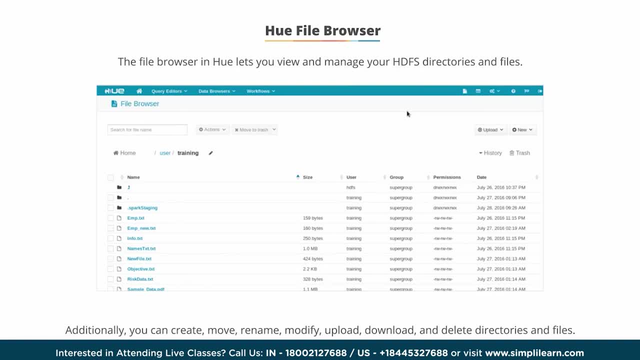 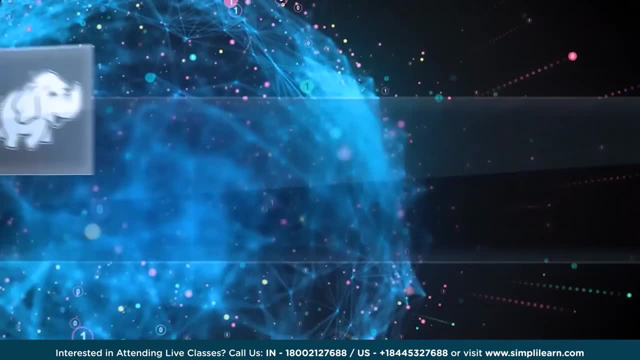 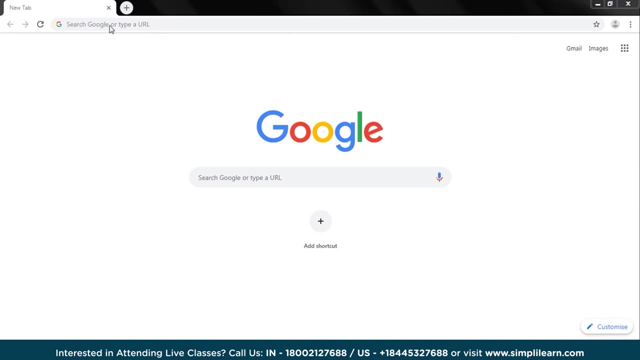 download and delete directories and files. you can also view the file contents all from within a convenient browser based utility. use of common hdfs commands. in this demo, you will learn how to use commonly used hdfs commands in simply learn cloud lab web console. so let's start. go to. 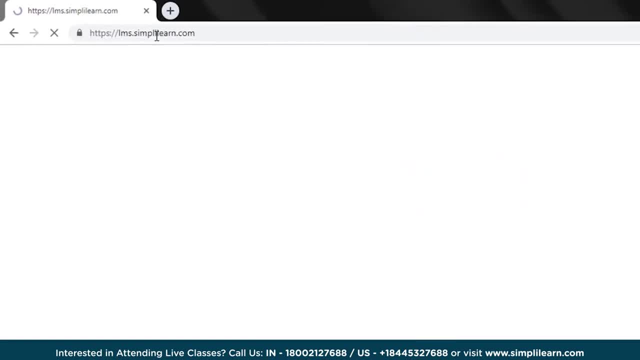 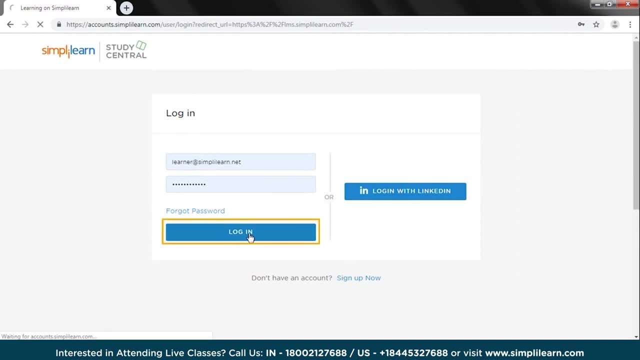 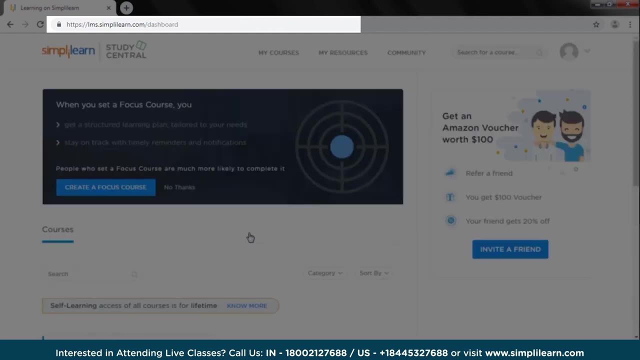 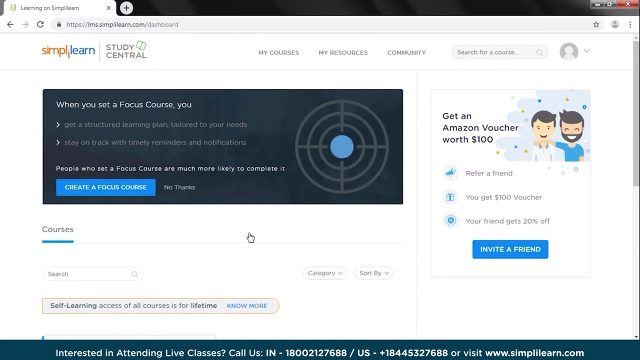 wwwsimplylearncom and click on login at the top right corner, it will navigate to tps colon slash slash lmssimplylearncom. on this page, enter your email id and password to login to your learner account. on successful login, you will be able to. 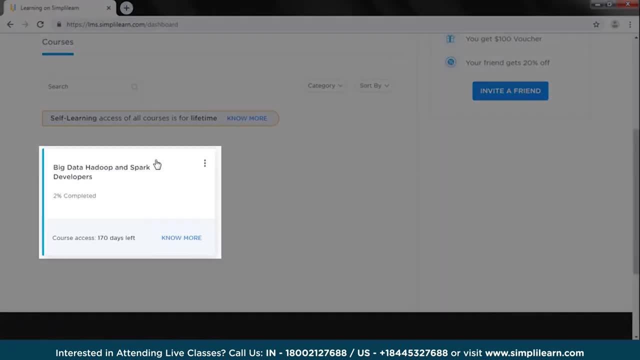 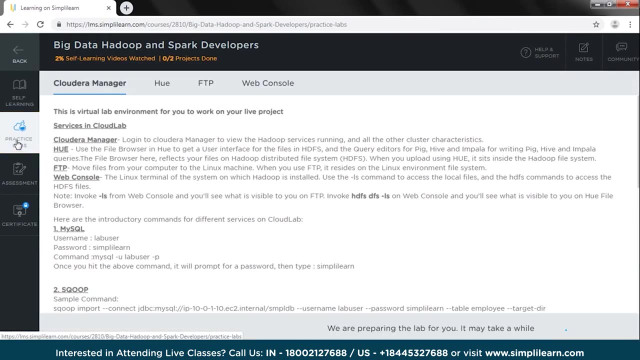 see a list of courses on the home page. click on the big data hadoop course to view its content and to access its practice lab. on clicking the practice lab tab, you will be able to see cloudera manager, hue, ftp and web console. click on web console and access the. 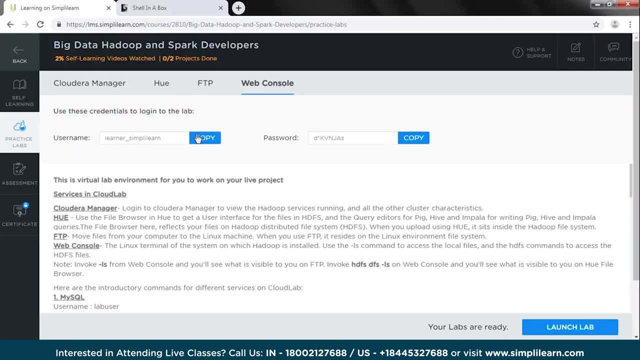 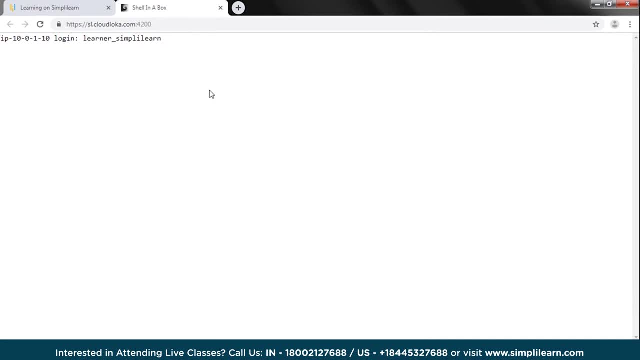 launch lab to use the linux terminal of the system on which hadoop is installed and to use various hdfs commands. you can log into the web console by simply clicking on the launch tab at the bottom right corner and copying and pasting the credentials from the 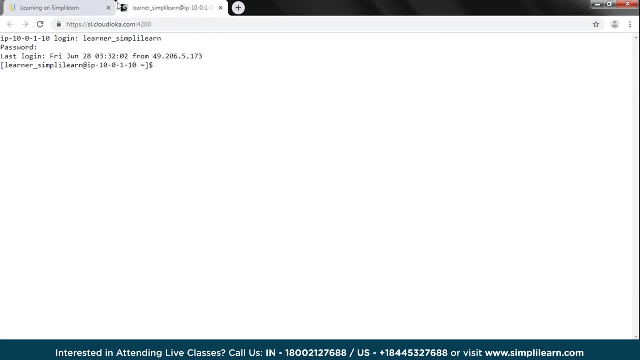 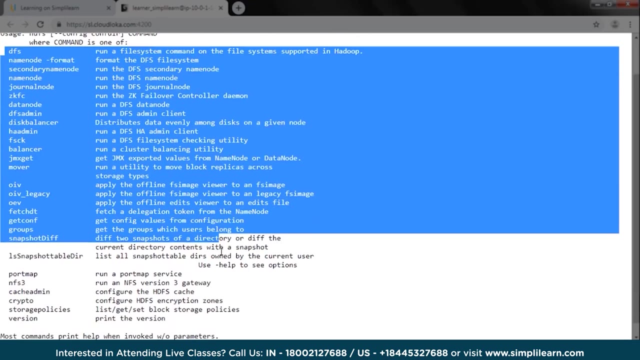 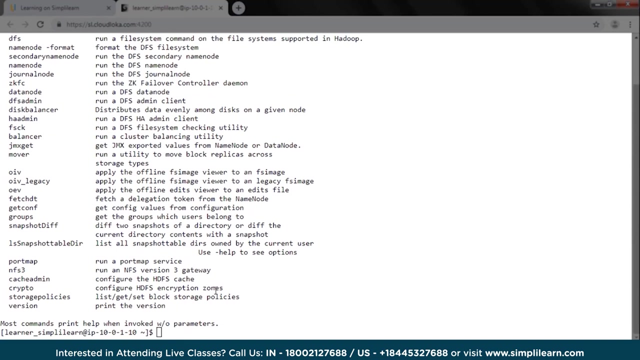 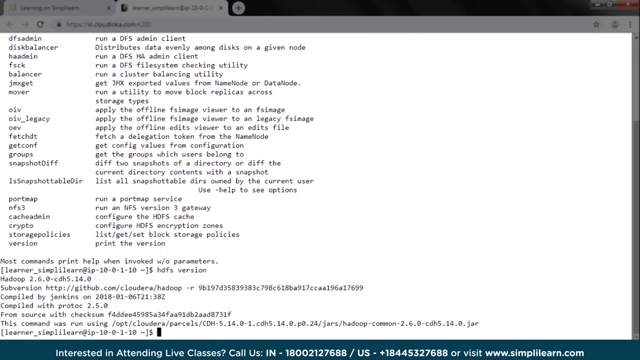 practice labs tab. now we will show you how to use common commands for hdfs. use hdfs help if you want to view the help content for common hdfs commands. use hdfs version to print the version of hadoop installed. then we have hdfs height. 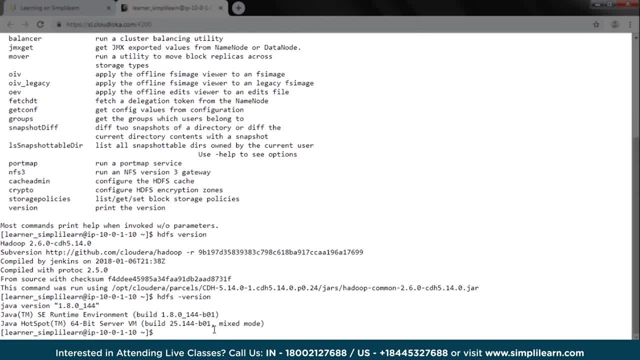 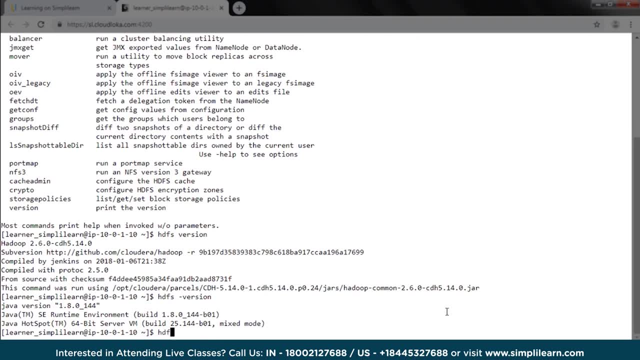 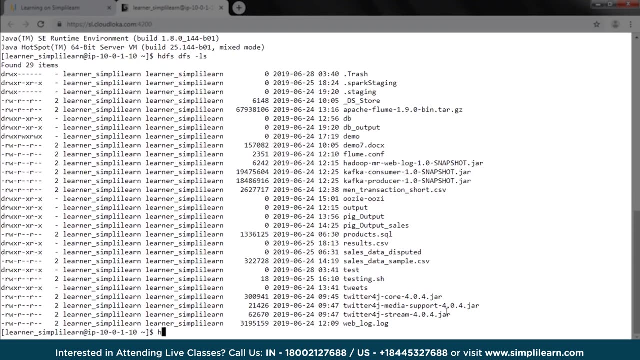 hyphen version which prints the version of Java and JVM. Use hdfs-dfs-ls to list home directory contents of the current user. Then we have hdfs-dfs-mkdir, followed by the directory name. Let's say demo1 is going to be used to create a new directory, demo1 in the current path. 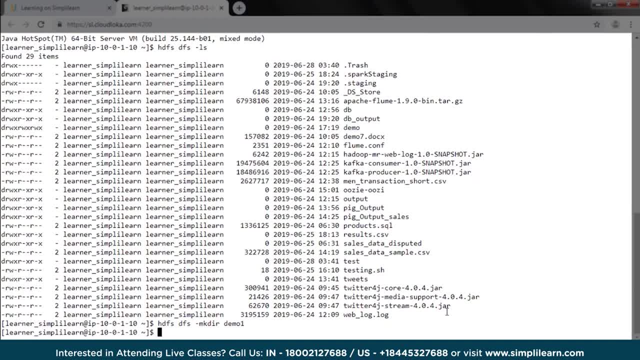 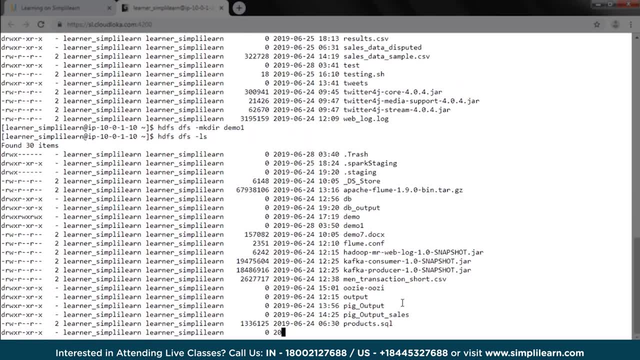 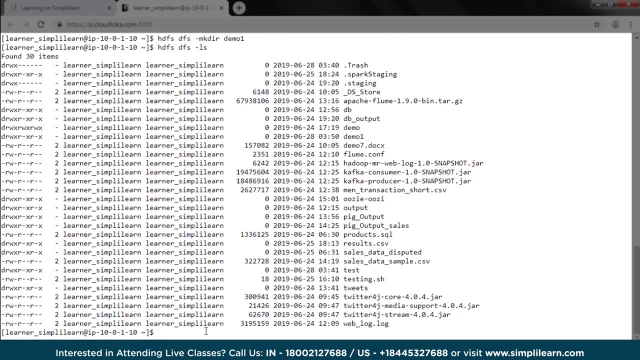 Now let's verify if the directory has been successfully created. Type hdfs-dfs-ls. It will show new directory demo1 has been created successfully. To remove directories we can use hdfs-dfs-rmr followed by the directory name. Let's say demo1, and then it will remove demo1 in the current path. 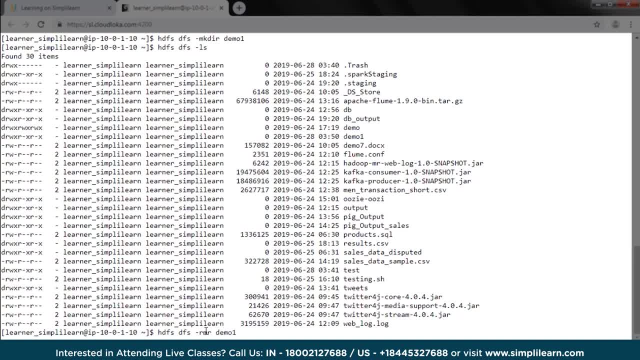 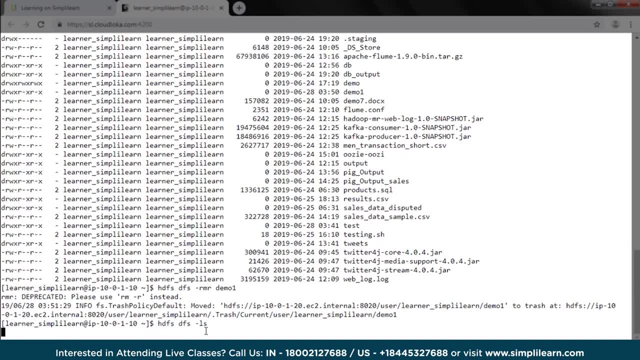 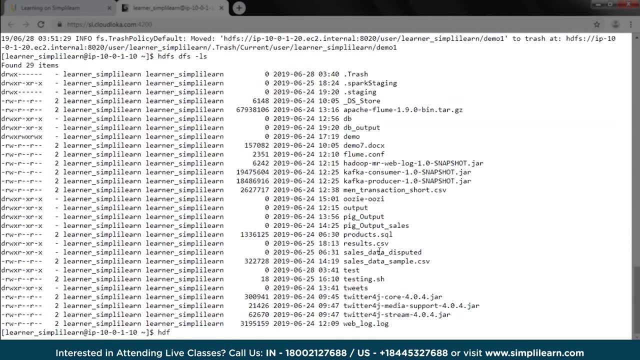 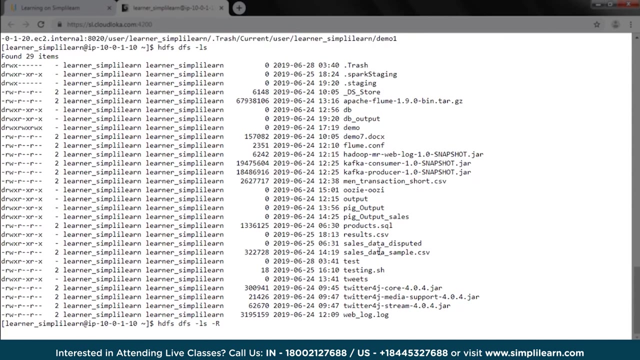 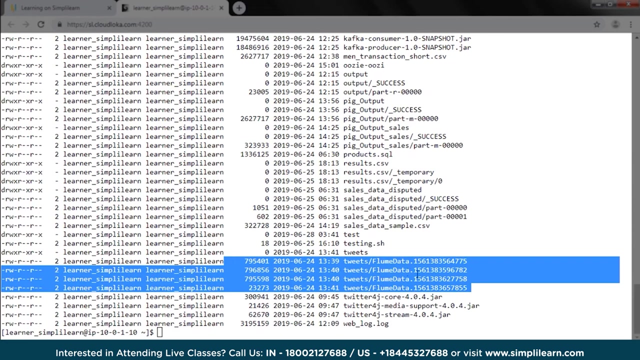 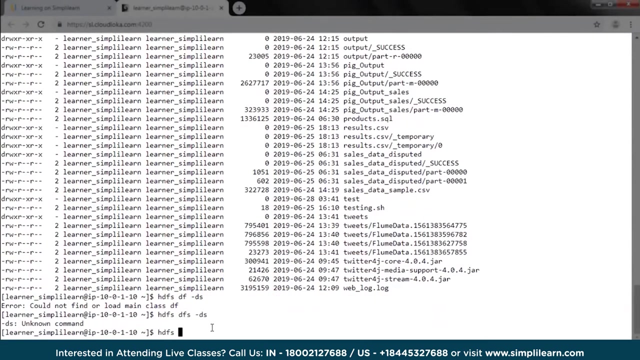 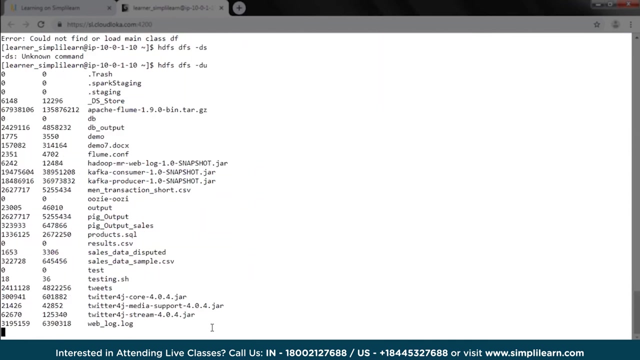 You can verify if it has been removed successfully by using hdfs-dfs-ls. Here you can see that demo1 has been removed successfully. Use hdfs-dfs-ls-R to recursively list subdirectories encountered in the current directory. Use hdfs-dfs-du to display sizes of files and directories contained in the given directory. 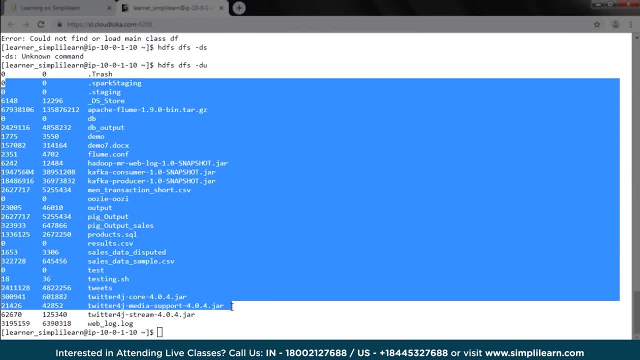 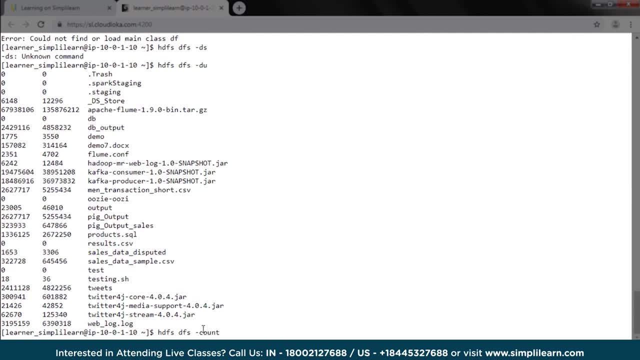 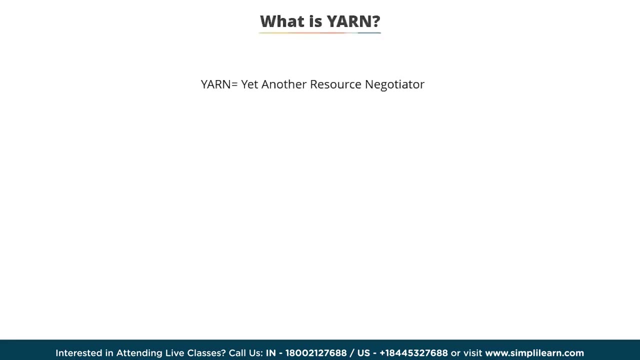 or the length of a file. in case it's just a file, Use hdfs-dfs-count directory name, let's say slash test, to count the number of files in the specified directory. YARN is the acronym for Yet Another Resource Negotiator. 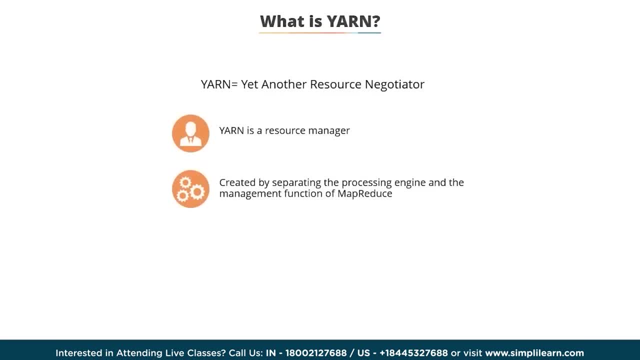 YARN is a resource manager created by separating the processing engine and the management function of MapReduce. It monitors and manages workloads, maintains a multi-tenant environment, manages the high availability features of Hadoop and implements security controls. Before 2012,. users could write MapReduce programs using scripting languages. 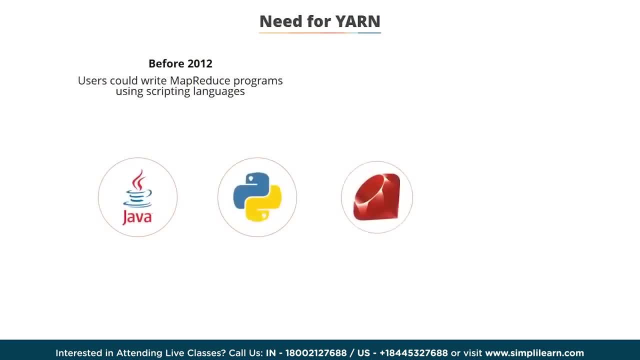 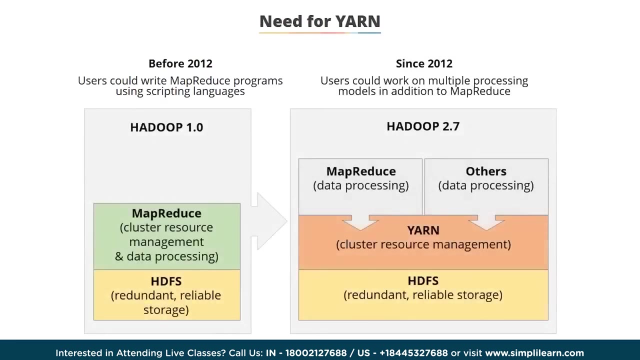 In 2012,. users could write MapReduce programs using scripting languages. They could also use PIG, a language used to transform data. No matter what language was used, its implementation depended on the MapReduce processing model. In May 2012,, during the release of Hadoop v2.0,, YARN was introduced. 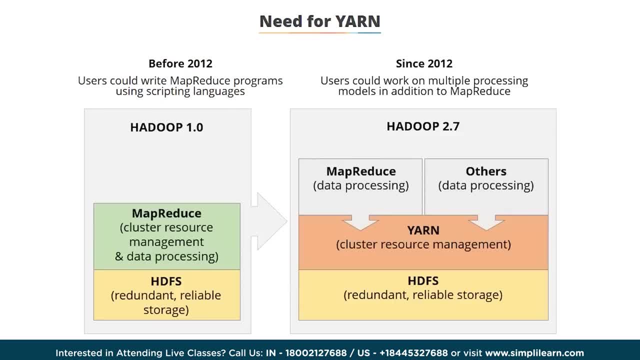 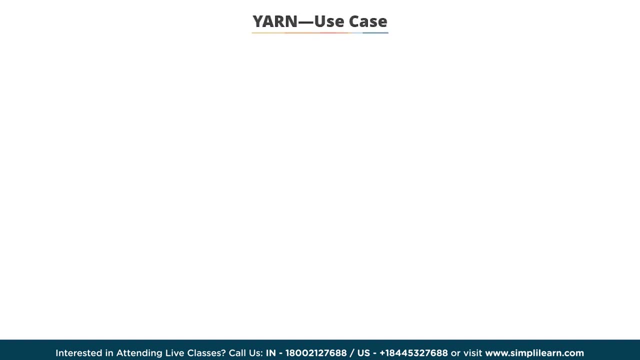 You are no longer limited to working with the MapReduce framework anymore, as YARN supports multiple processing models in addition to MapReduce, Such as Spark. Other features of YARN include significant performance improvement and a flexible execution engine. Now let's discuss YARN with the help of an example. 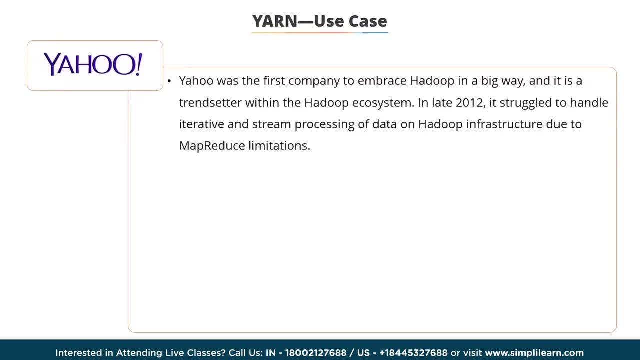 Yahoo was the first company to embrace Hadoop, and this became a trendsetter within the Hadoop ecosystem. In late 2012,, Yahoo struggled to handle iterative and stream processing of data on the Hadoop infrastructure due to MapReduce limitations. Both iterative and stream processing were important to Yahoo in facilitating its move. 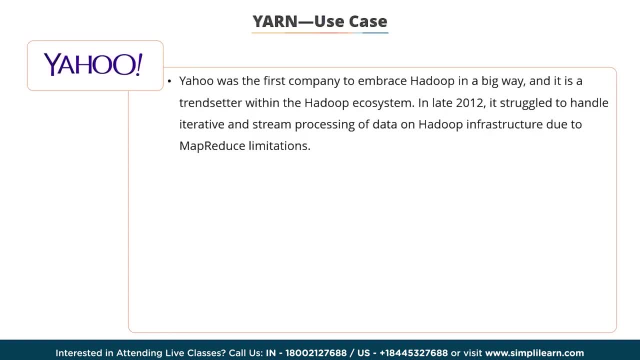 from batch computing to continuous computing. After implementing YARN in the first quarter of 2013,, Yahoo installed more than 30,000 production nodes on Spark for iterative processing, Storm for stream processing and Hadoop for batch processing, allowing it to handle more than 100 billion events such as clicks, impressions. 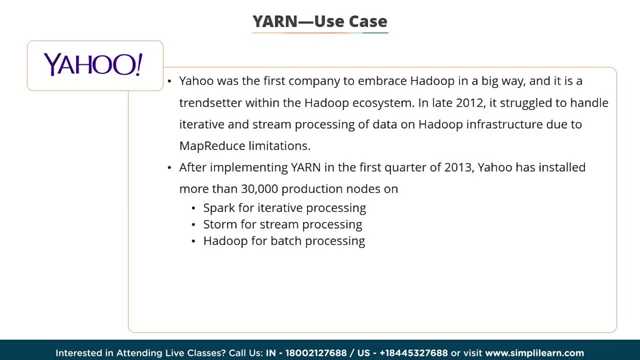 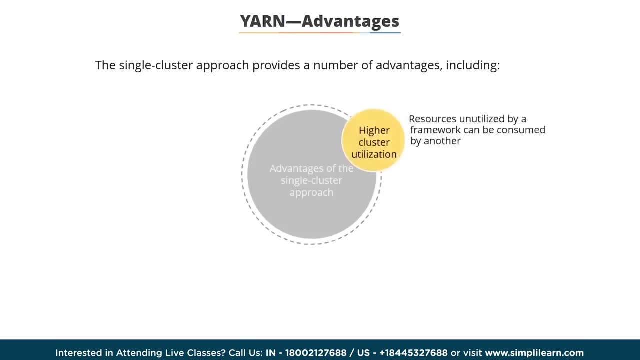 email content, metadata and more. This was possible only after YARN was introduced and multiple processing frameworks were implemented. The single-cluster approach provides a number of advantages, including Higher cluster utilization, where resources unutilized by a framework can be consumed. 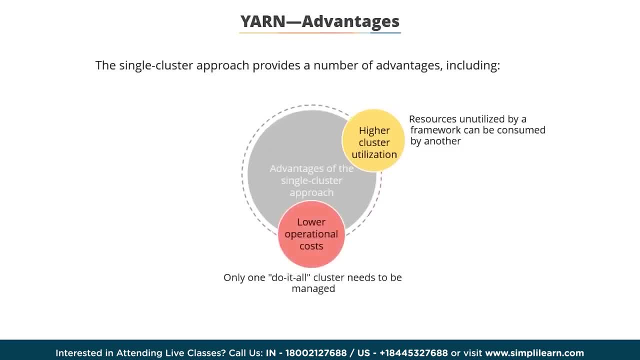 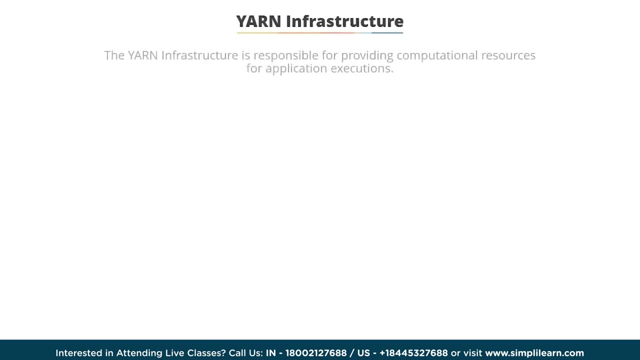 by another. Lower operational costs, because only one do-it-all cluster needs to be managed. Reduced data motion, As there's no need to move data between Hadoop, YARN and systems running on different clusters of computers. The YARN infrastructure is responsible, providing computational resources such as CPU or memory. 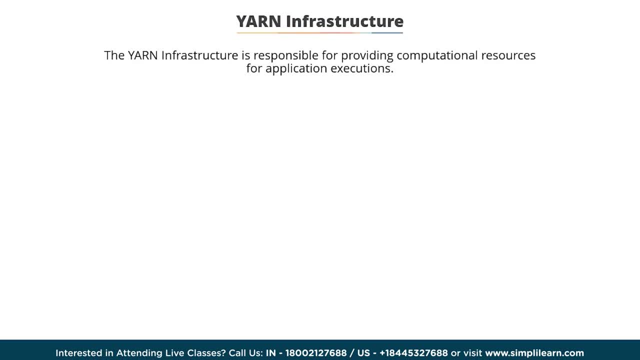 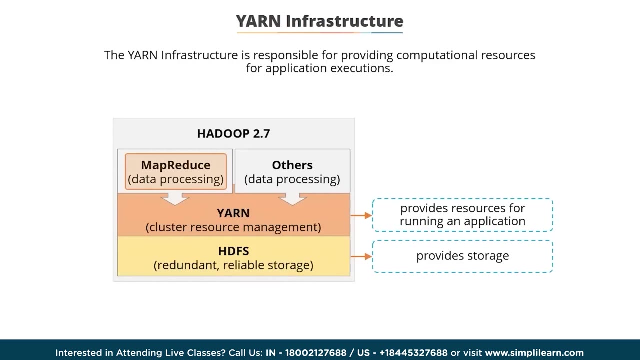 needed for application executions. YARN infrastructure and HDFS are completely independent. The former provides resources for running an application, while the latter provides storage. The MapReduce framework Is only one of the many possible frameworks that run on YARN. The fundamental idea of MapReduce version 2 is to split the two major functionalities. 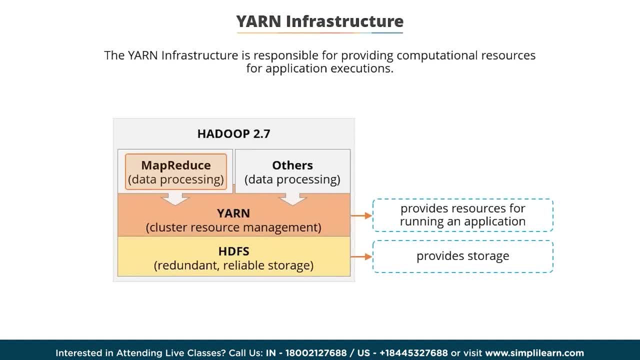 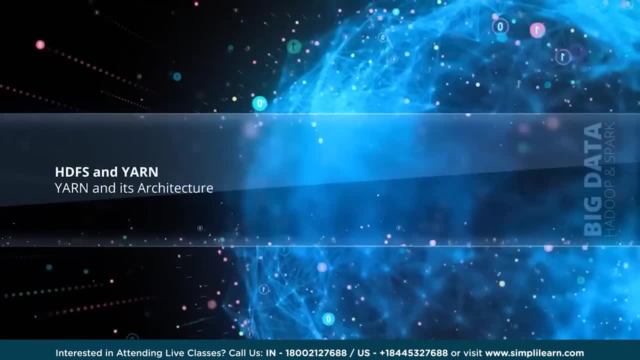 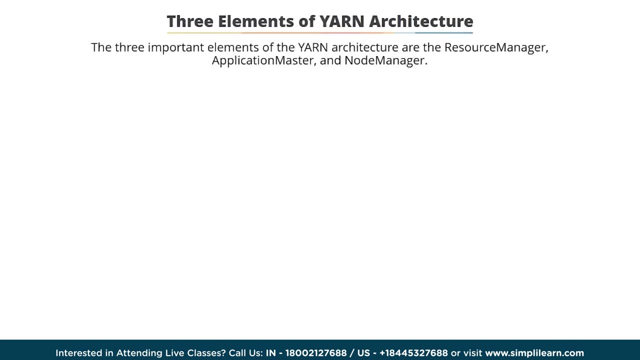 of resource management and job scheduling and monitoring into separate daemons. YARN and its architecture. In this topic we will discuss YARN and its architecture, Three elements of YARN architecture. The three important elements of the YARN architecture are Resource Manager, Application Master and Node Managers. 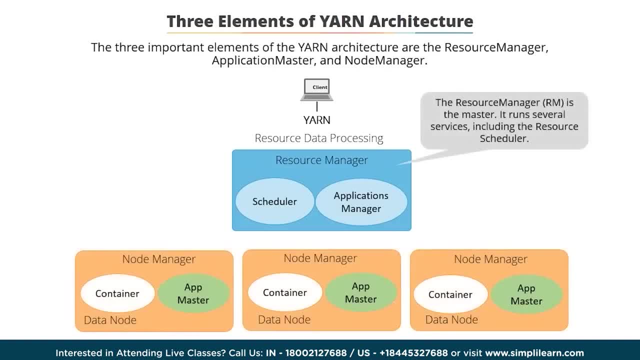 The Resource Manager, or RM, which is usually one per cluster, is the master server. Resource Manager knows the location of the data node and how many resources they have. This information is referred to as Rack Awareness. The RM runs several services, The most important of which is the Resource Scheduler. 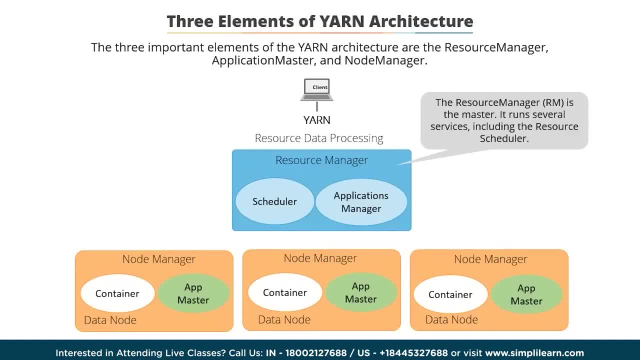 The Resource Scheduler is the resource scheduler That decides how to assign the resources. The Application Master is a framework-specific process that negotiates resources for a single application, That is, a single job or a directed acyclic graph of jobs, which runs in the first container. 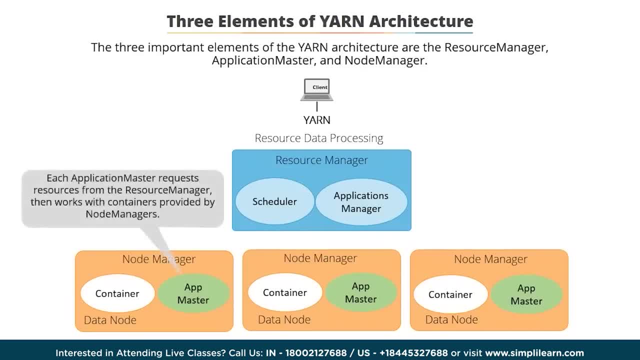 allocated for the purpose. Each Application Master requests resources from the Resource Manager and then works with the containers provided by Node Managers. The Node Managers can be many in one cluster. They are the slaves of the infrastructure. When it starts, it announces itself to the RM and periodically sends a heartbeat to the. 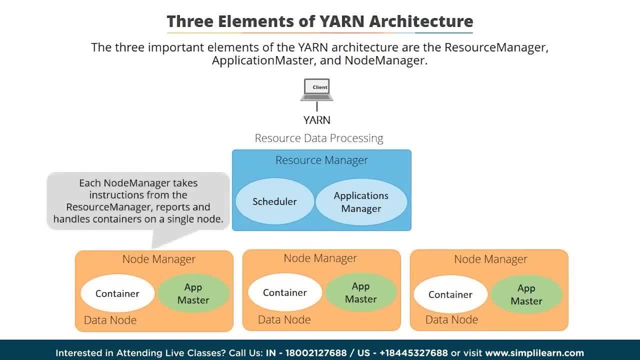 RM. Each Node Manager offers resources to the cluster. The resource capacity is the amount of memory and the number of vCores, short for virtual core. At runtime, the Resource Scheduler decides how to use this capacity. A container is a fraction of the node manager capacity and it is used by the client to 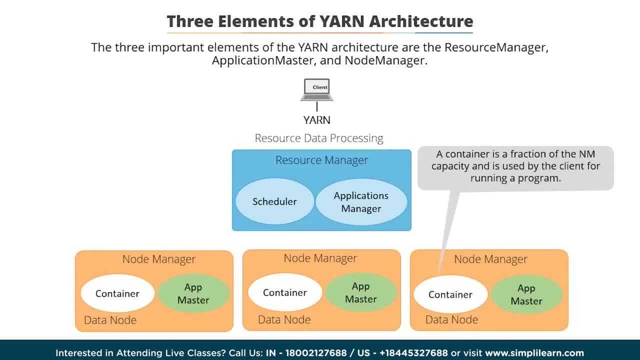 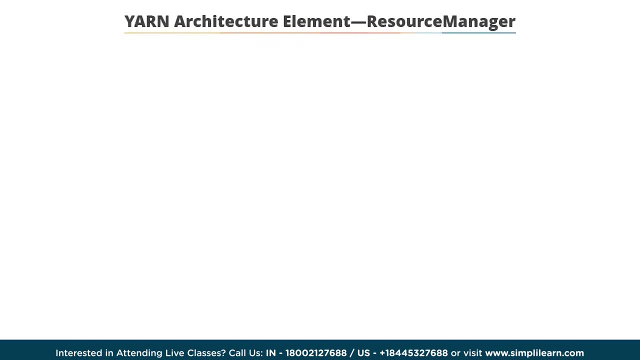 run a program. Each node manager takes instructions from the resource manager and reports and handles containers on a single node. In the next few screens you will see a detailed explanation of the three elements. The first element of YARN architecture is resource manager. 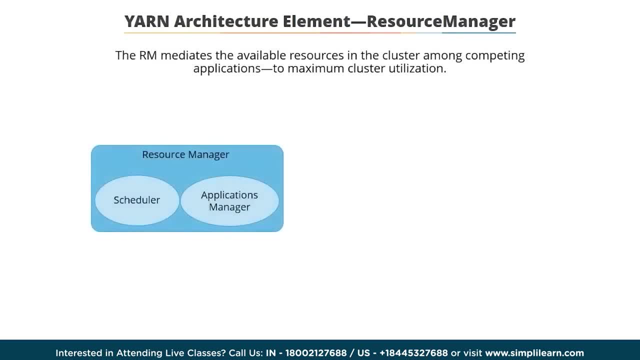 The RM mediates the available resources in the cluster among competing applications with the goal of maximum cluster utilization. It includes a pluggable scheduler called the YARN scheduler, which allows different policies for managing constraints, such as capacity, fairness and service level agreements. 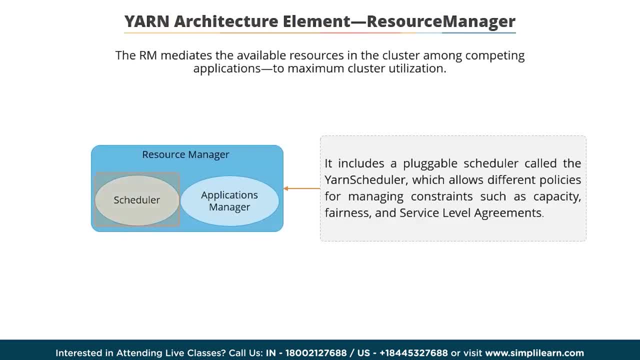 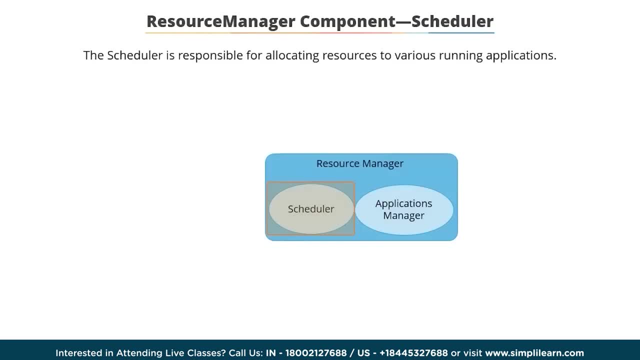 The resource manager has two main components: scheduler and applications manager. The scheduler is responsible for allocating resources. The scheduler is responsible for allocating resources to various running applications, depending on the common constraints of capacities, queues and so on. The scheduler does not monitor or track the status of the application. 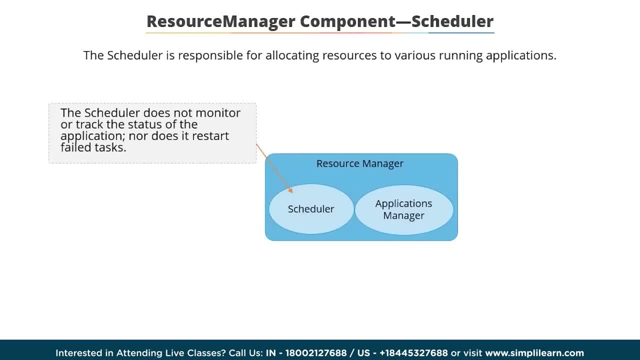 Also, it does not restart the tasks in case of any application or hardware failures. The scheduler performs its function based on the resource requirements of the applications. It does so based on the abstract notion of a resource container that incorporates elements such as memory, memory and memory. 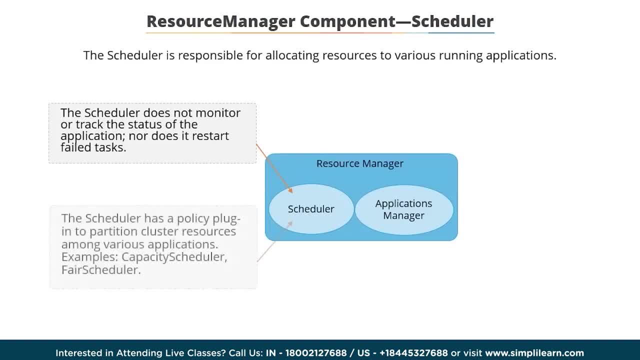 The scheduler is responsible for allocating resources to various running applications: CPU, disk and network. The scheduler has a policy plugin which is responsible for partitioning the cluster resources among various queues and applications. The current MapReduce schedulers, such as CapacityScheduler and the FAIR scheduler. 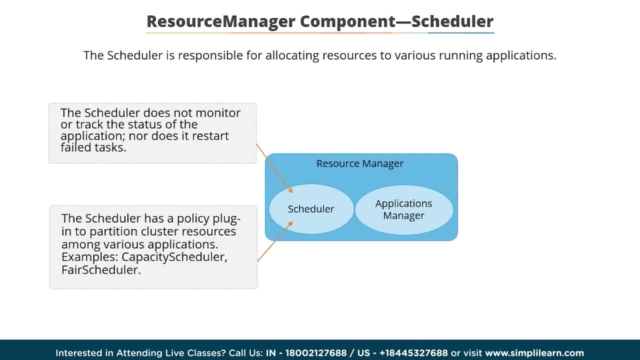 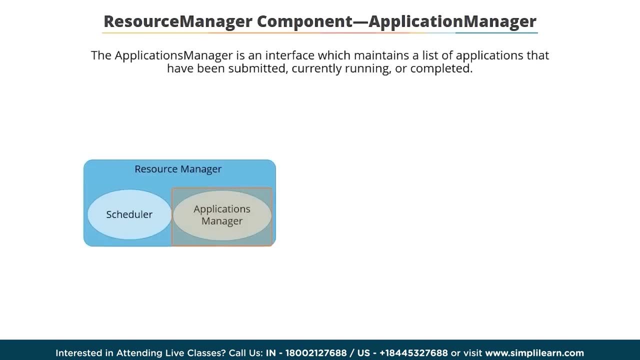 are some examples of the plugin. The CapacityScheduler supports hierarchical queues to enable a more predictable sharing of cluster resources. The applicational manager is an interface which maintains a list of applications that have been submitted, currently running or completed. The application manager is responsible for accepting job submissions, negotiating the 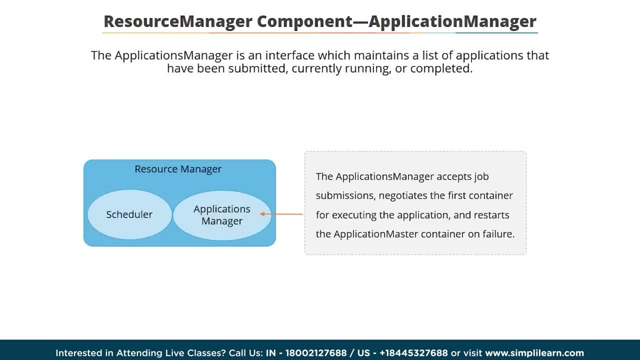 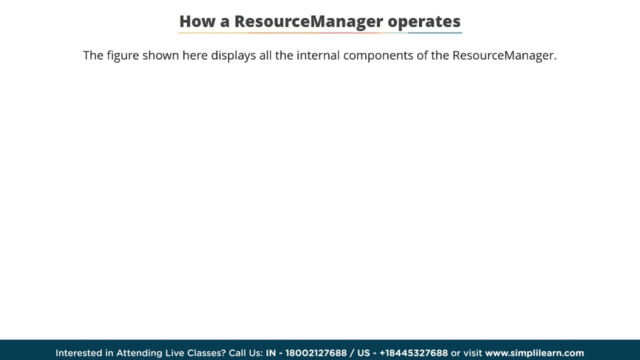 first container for executing the application-specific Application Master and restarting the Application Master container on failure. Let's discuss how each component of the resource manager work together. The resource manager is responsible for accessing the system and then executing the application. Manager communicates with the clients through an interface called the Client Service. A client can 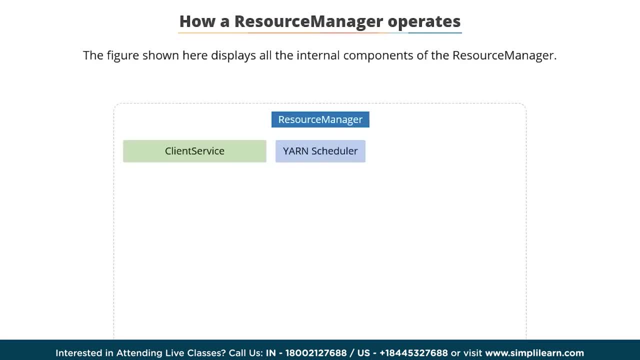 submit or terminate an application and gain information about the scheduling queue or cluster statistics through the Client Service. Administrative requests are served by a separate interface called the Admin Service, through which operators can get updated information about the cluster operation. In parallel, the Resource Tracker Service receives node heartbeats from 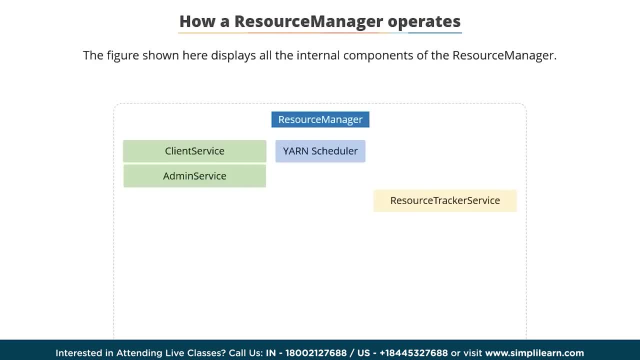 the Node Manager to track new or decommissioned nodes. The NM Liveliness Monitor and Nodes List Manager keep an updated status of which nodes are healthy so that the scheduler and the Resource Tracker Service can allocate work appropriately. The Application Master Service manages application. 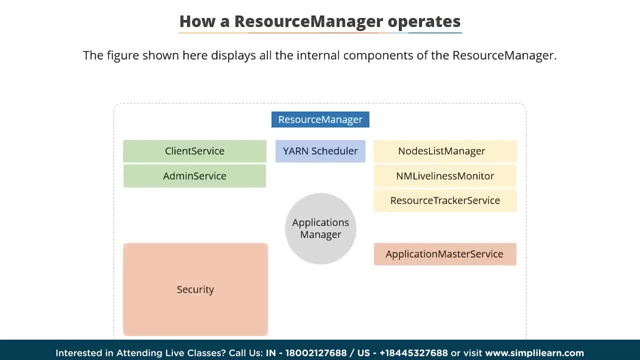 masters on all nodes, keeping the scheduler informed. The AM Liveliness Monitor keeps a list of application managers and their last heartbeat times to let the Resource Manager know what applications are healthy on the cluster. Any application master that does not send a heartbeat within a certain interval. 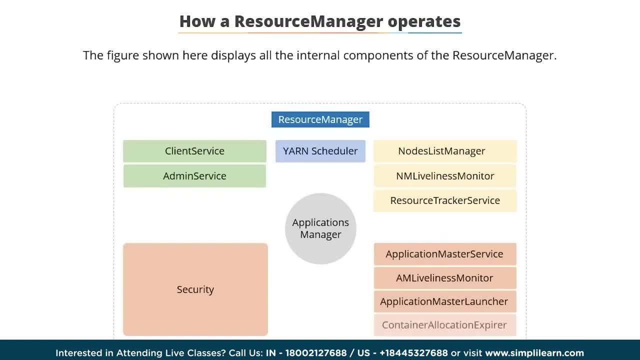 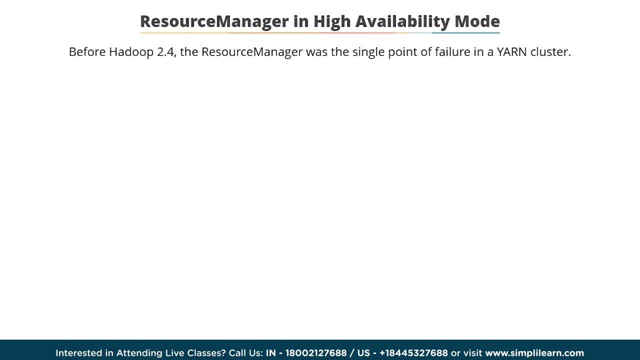 is marked as dead and rescheduled to run on a new container. Before Hadoop 2.4, the Resource Manager was the single point of failure in a YARN cluster. The High Availability, or HA, feature adds redundancy in the form of an Active Standby. 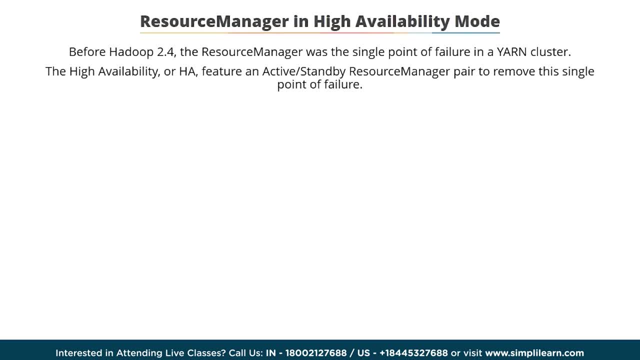 Resource Manager pair to remove the single point of failure. Resource Manager HA is realized through the Active Standby architecture. At any point of time, one of the RMs is active and one or more RMs are in Standby mode waiting to take over should anything happen to the active. The trigger to transition to active. 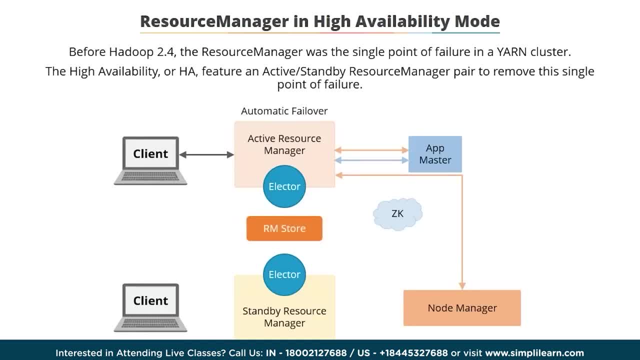 comes from either the admin through the command-line interface or through the integrated failover controller. The RMs have an option to embed the ZooKeeper-based Active Standby Elector to decide which RM should be active. When the active goes down or becomes unresponsive, another RM is automatically elected to be the active. 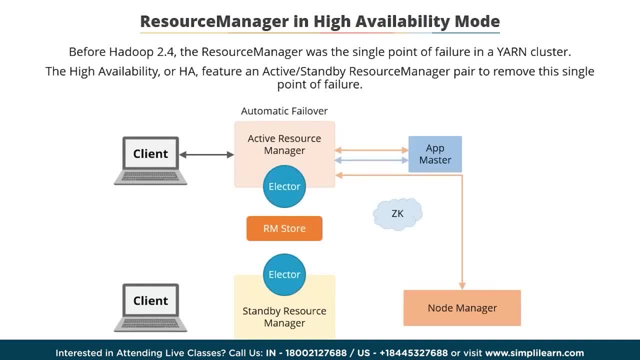 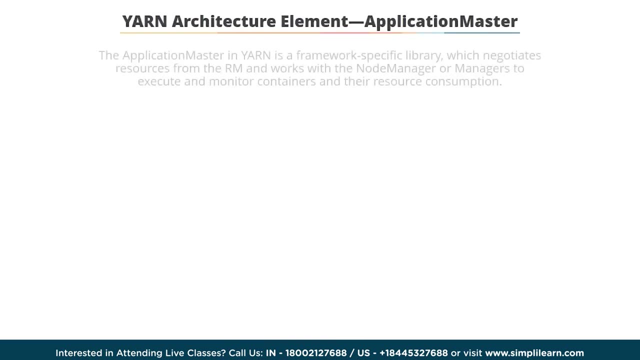 Note that there is no need to run a separate ZKFC daemon like in HDFS, because the Active Standby Elector embedded in RMs act as a failure detector and a leader elector. The second element of YARN architecture is the Application Master. 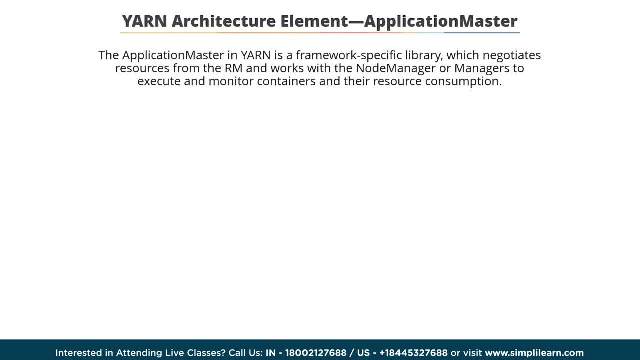 The Application Master in YARN is a framework-specific library which negotiates resources from the RM and works with the Node Manager or Managers to execute and monitor containers and their resource consumption. While an application is running, the Application Manager manages the application lifecycle: dynamic adjustments to resource consumption. 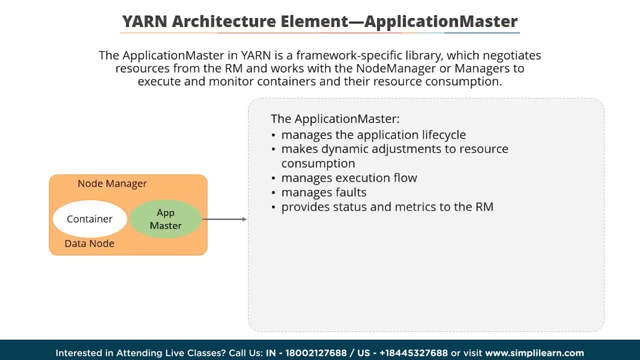 execution flow faults and it provides status and metrics. The Application Master is architected to support a specific framework and can be written in any language. It uses extensible communication protocols with the Resource Manager and the Node Manager. The Application Master can be customized to extend. 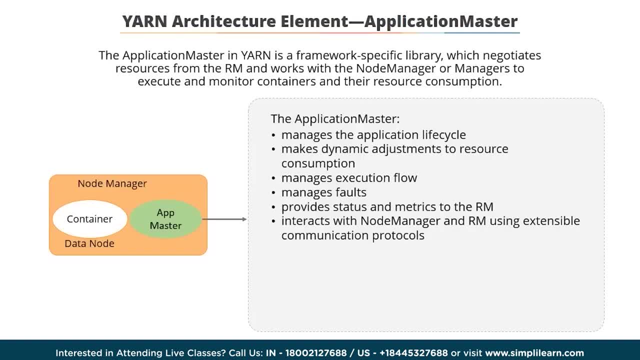 the framework or run any other code. Because of this, the Application Master is not considered trustworthy and is not run as a trusted service. In reality, every application has its own instance of an Application Master. However, it's feasible to implement an Application Master to manage a set. 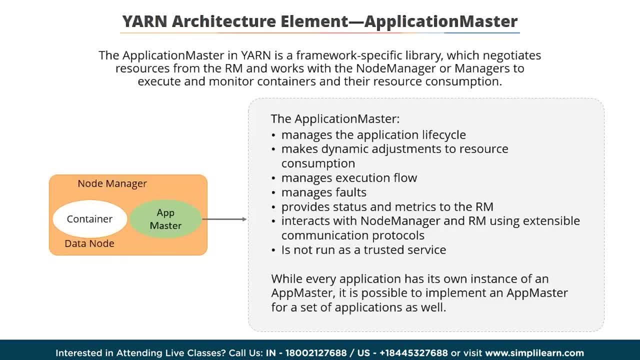 of applications, For example, an Application Master for PIG or HIVE to manage a set of maprenduced jobs driving manual. such asitter was a content manager for this application, making sure the service was laid out preferably in the background and are not Quantity Inter��을 access reused in the site. The 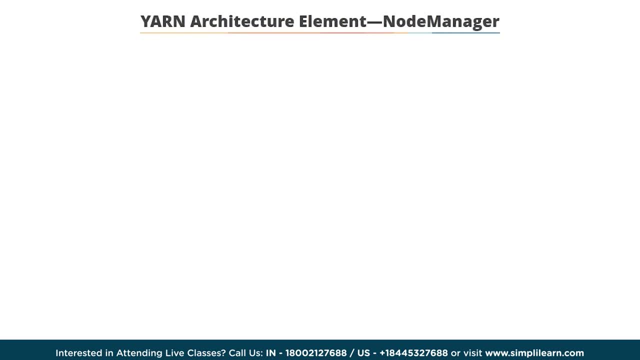 application management managementENS sixty non-The appreciated application 1994.モルタル monkey oin, 28 goals distance, or Iconic Air Department που neighbour第二boified. The third element of YARN architecture is the Node Manager When a container is leased to an application. 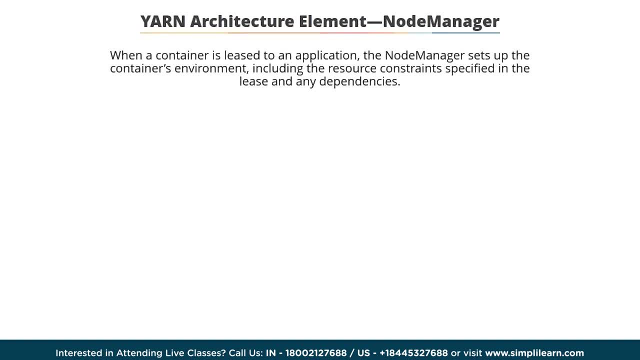 the Node Manager sets up the container's environment. The environment includes the resource constraints specified in the lease and any kind of dependencies such as data or executable files. The Node Manager monitors the health of the node, reporting to the Resource Manager when a hardware or software issue occurs. 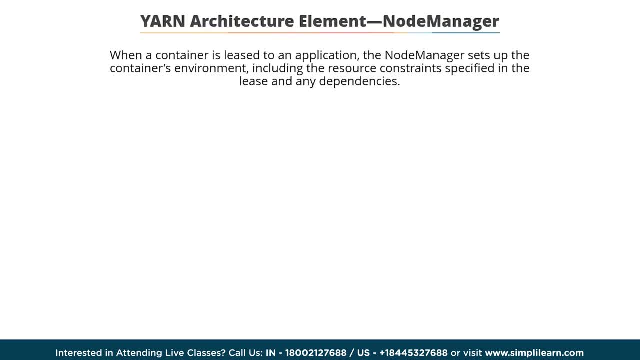 so that the scheduler can divert resource allocations to healthy nodes until the issue is resolved. The Node Manager also offers a number of services to containers running on the node, such as a log aggregation service. The Node Manager runs on each node and manages the activities. 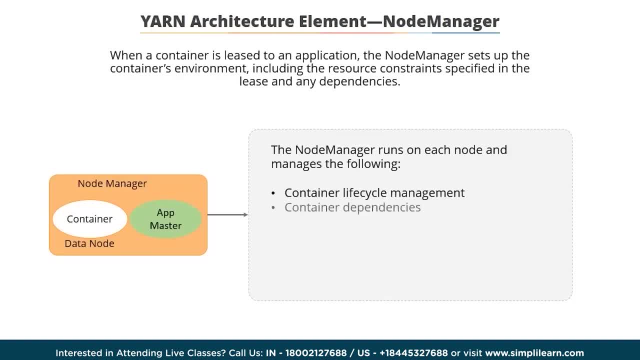 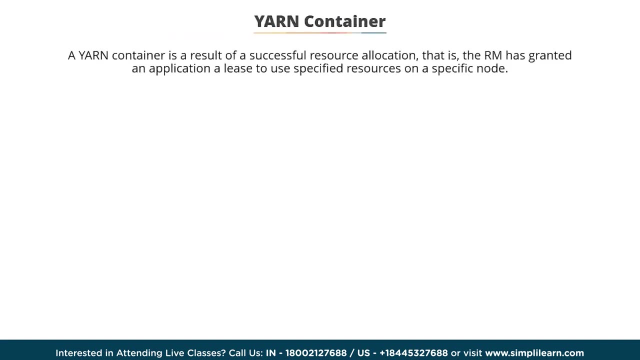 such as container lifecycle management, container dependencies, container leases. node and container resource usage node, health and log management and reports. node and container status to the Resource Manager. A YARN container is a collection of specific set of resources to use in certain amounts on a specific node. 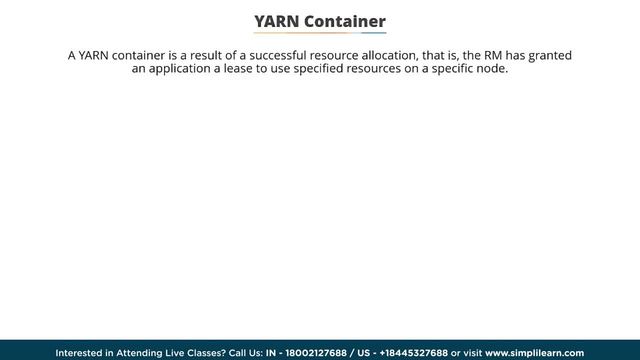 It is allocated by the Resource Manager on the basis of the application. The Application Manager presents the container to the Node Manager on the node where the container has been allocated, thereby granting access to the resources. Now let's discuss how to launch the container. 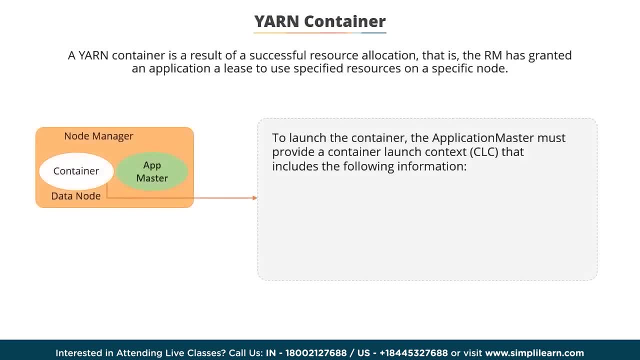 The Application Manager must provide a container launch context, or CLC. This includes information such as environment variables, dependencies on the requirement of data files or shared objects prior to the launch, security tokens and the command to create the process to launch the application. 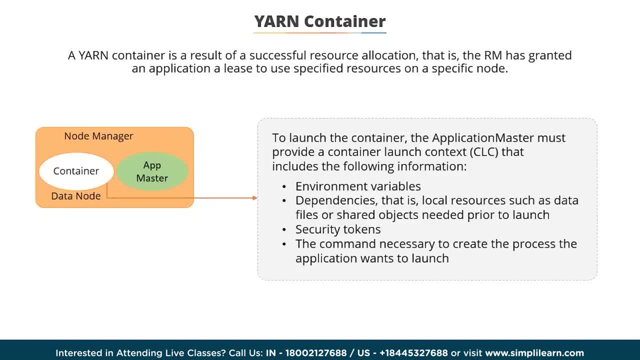 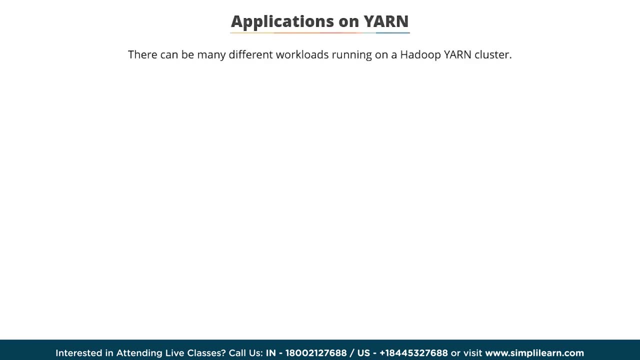 The CLC supports the Application Manager to use containers. This helps to run a variety of different kinds of work, from simple shell scripts applications to a virtual operating system. Owing to YARN's generic approach, a Hadoop YARN cluster runs various workloads. 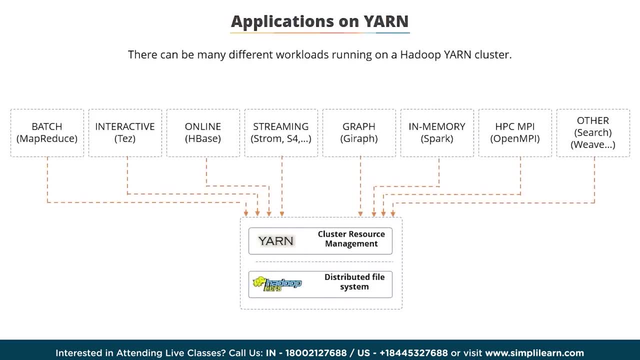 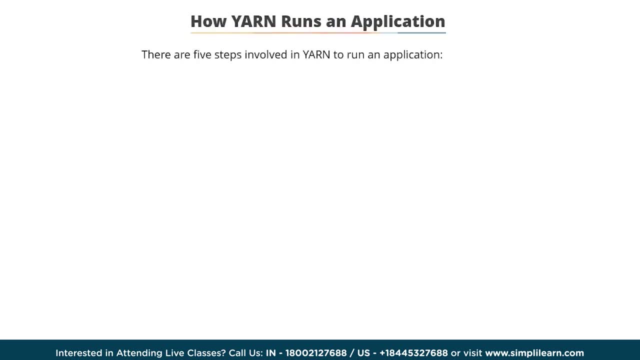 This means a single Hadoop cluster in your data center can run MapReduce, Storm, Spark, Impala and more Broadly. there are five steps involved in YARN to run an application. First, the client submits an application to the Resource Manager. 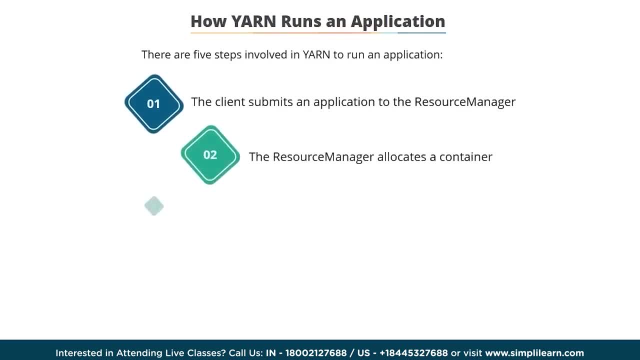 Then the Resource Manager allocates a container, Then the Application Master contacts the Related Node Manager, Then the Related Node Manager launches the container And finally, the container executes the Application Master. In the next few screens you will learn about each step in detail. 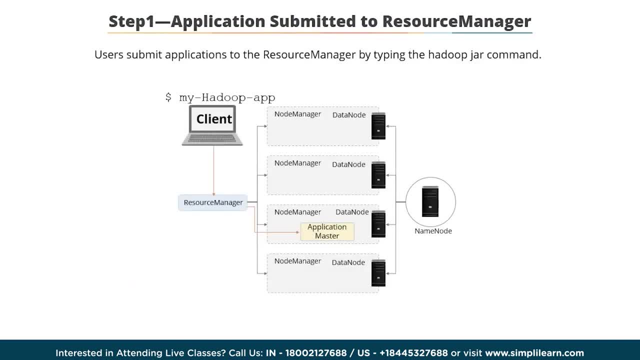 Users submit applications to the Resource Manager by typing the HadoopYARN command. The Resource Manager maintains the list of applications on the cluster and available resources on the Node Manager. The Resource Manager determines the next application that receives a portion of the cluster resource. 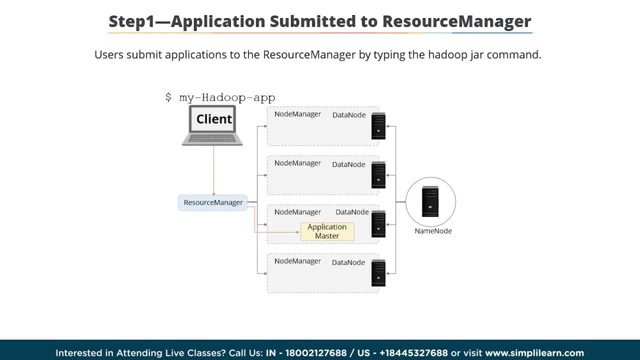 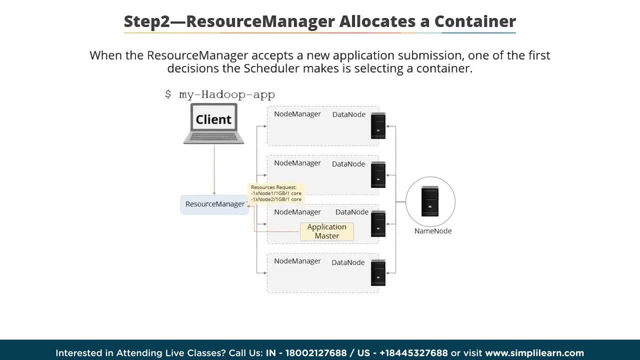 The decision is subject to many constraints, such as queue capacity, access control, lists and fairness. When the Resource Manager accepts a new application submission, one of the first decisions the scheduler makes is selecting a container. Then the Application Master is started and is responsible for the entire lifecycle. 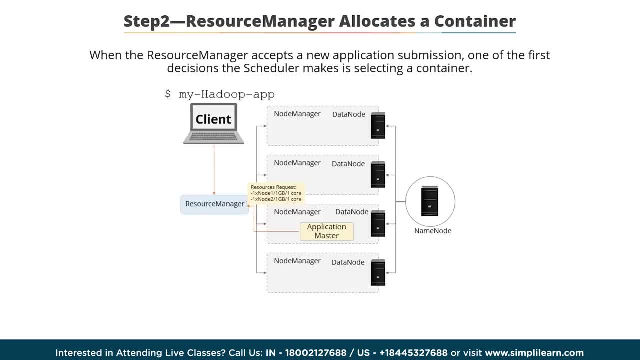 of that particular application. First, it sends resource requests to the resource manager to ask for containers to run the application's tasks. A resource request is simply a request for a number of containers that satisfy resource requirements, such as the following: Amount of resources expressed as megabytes of memory. 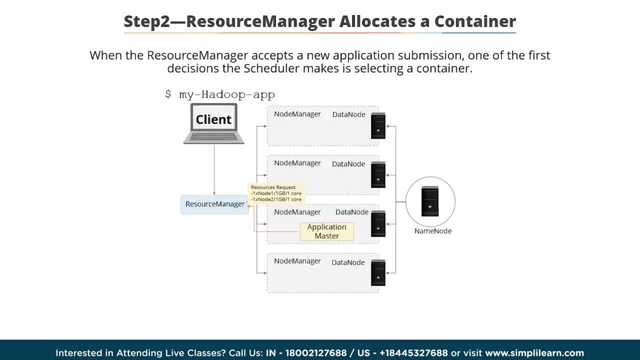 and CPU shares. Preferred location specified by host name or rack name. Priority within this application and not across multiple applications. The resource manager allocates a container by providing a container ID and a host name which satisfies the requirements of the application master. 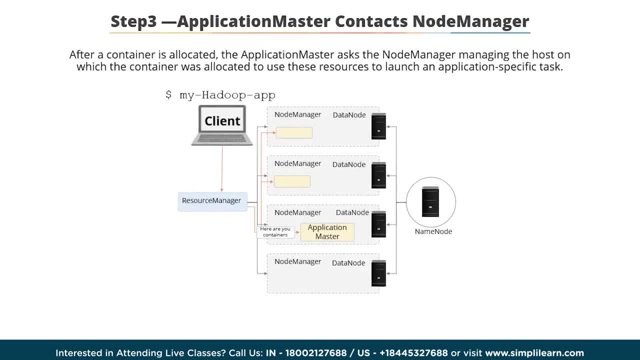 After a container is allocated, the application master asks the node manager managing the host on which the container was allocated to use these resources to launch an application service. The node manager has a specific task. This task can be any process written in any framework. 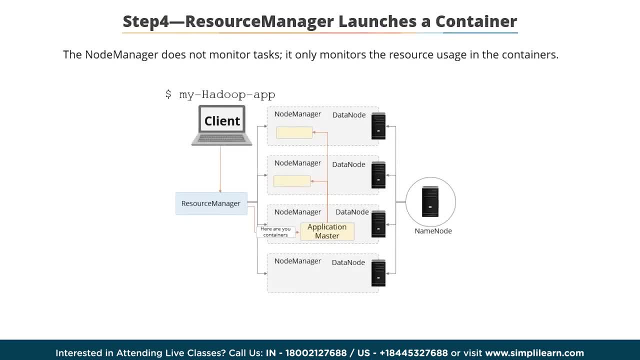 such as a MapReduce task. The node manager does not monitor tasks. It only monitors the resource usage in the containers. For example, it kills a container if it consumes more memory than initially allocated Throughout its life. the application master negotiates containers to launch all the tasks needed. 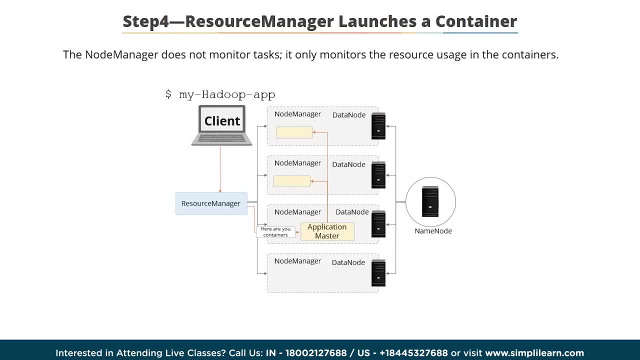 to complete its application. It also monitors the progress of an application and its tasks, restarts failed tasks in newly requested containers and reports progress back to the client that submitted the application. After the application is complete, the application master shuts itself and releases. 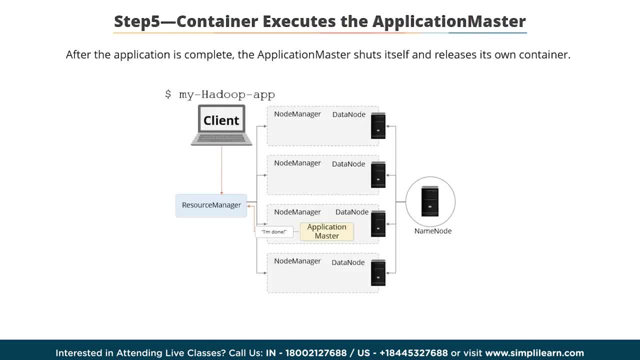 its own container. Though the resource manager does not monitor the tasks within an application, it checks the health of the application master. If the application master fails, it can be restarted by the new resource manager in a new container. Thus, the resource manager looks after the application master. 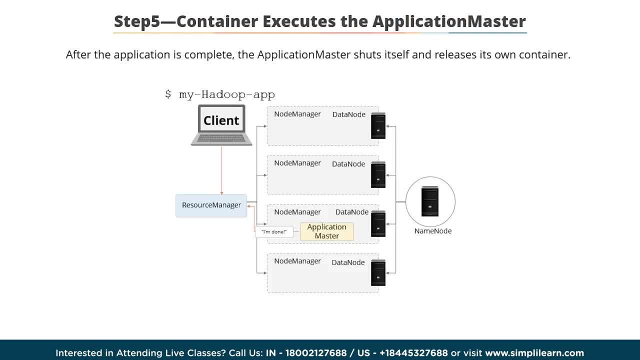 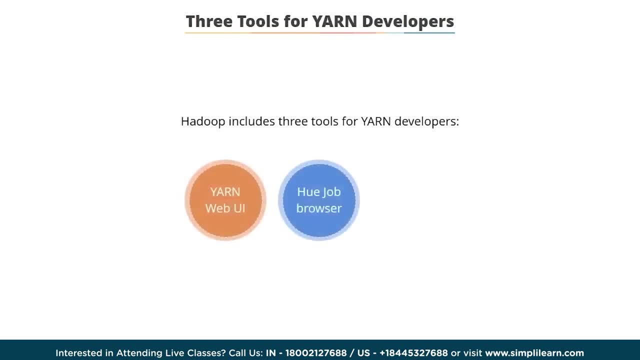 while the application master looks after the tasks. Hadoop includes three tools for YARN developers: YARN Web UI, Hue Job Browser. YARN Command Line. These tools enable developers to submit, monitor and manage jobs on the YARN cluster. 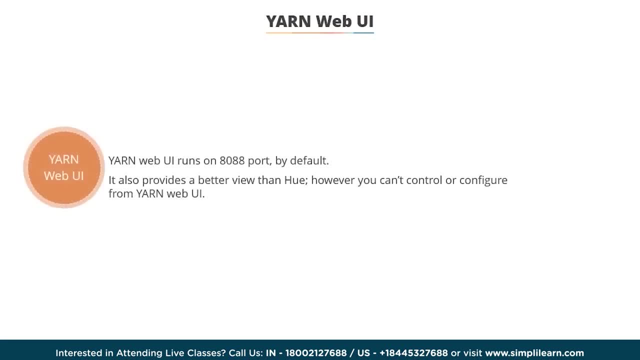 YARN Web UI, Hue Job Browser, YARN Command Line. These tools enable developers to submit, monitor and manage jobs on the YARN cluster. YARN Web UI runs on 8088 port by default. It also provides a better view than Hue. 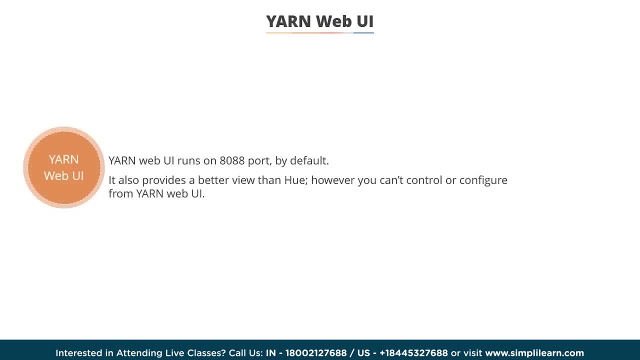 However, you can't control or configure from YARN Web UI. You will see a demonstration on YARN Web UI in the later screen. The Hue Job Browser allows you to monitor the status of a job, kill a running job and view logs. 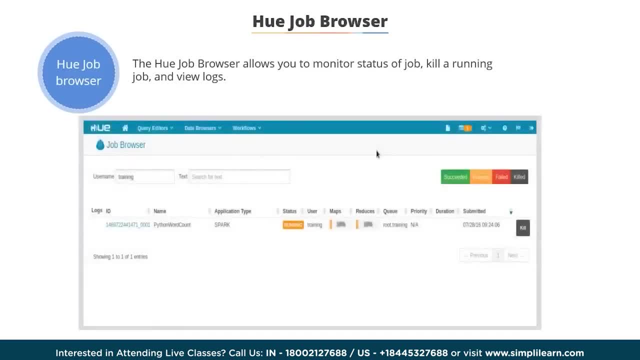 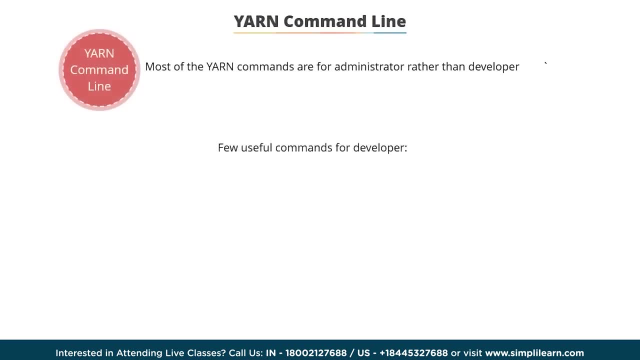 You will understand this by viewing a demonstration in the later screen. Most of the YARN commands are for the user. Most of the YARN commands are for the administrator rather than the developer. A few useful commands for developers are as follows: To list all commands of YARN, type, the command line shown on screen. 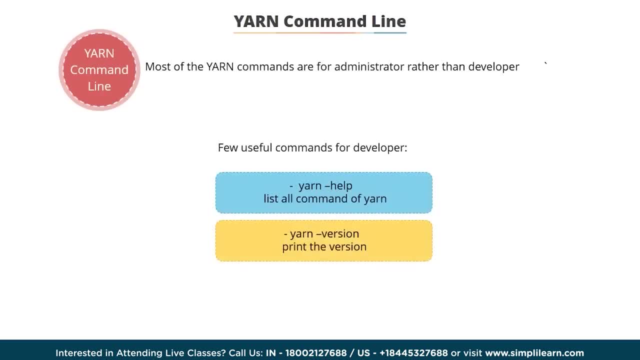 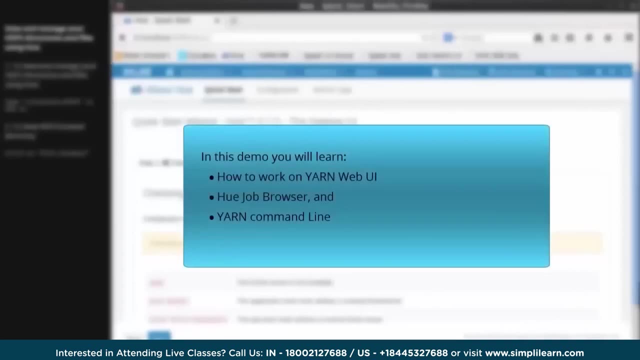 To print the version type: the command line shown on the screen. To view logs of a specified application ID type: the command line shown on your screen. Using YARN Web UI, Hue Job Browser and YARN Command Line, You will learn how to work on this demo. 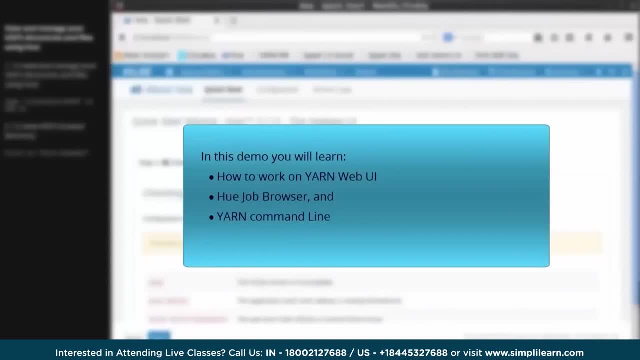 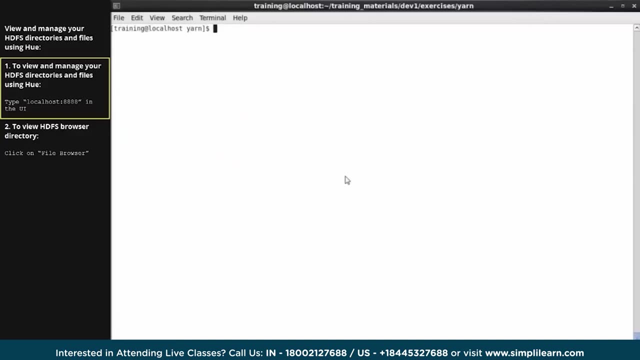 In this demo you will learn how to work on YARN Web UI, Hue Job Browser and YARN Command Line. Here is the demo. You will use the file wordcountpy, which is a Python file. This file will calculate the number of times each word appears. 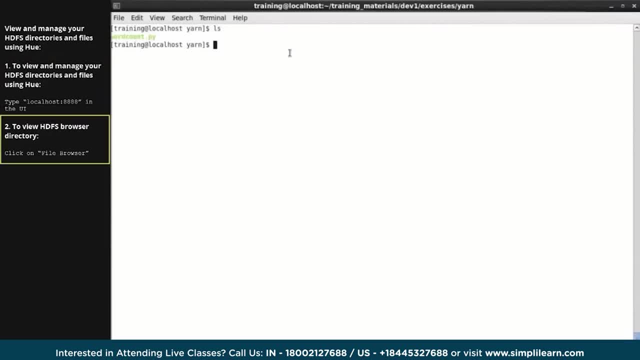 You will view how to execute this file with the help of YARN Type spark-submit. Let's define the master as yarn-client. The YARN file will input the information followed by the name of the Python file. You need each word count which is present in the word directory loudacre slash kb. 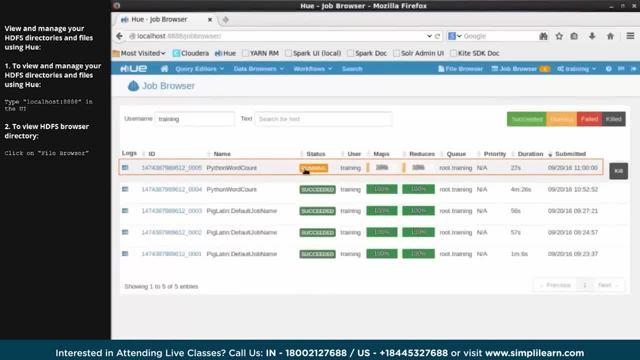 Click Job Browser. While the program is running on the terminal, let's see how the steps executing in YARN appear in Hue. You will notice the Python word count status as running. It will also show you the status of Map and Reducer. 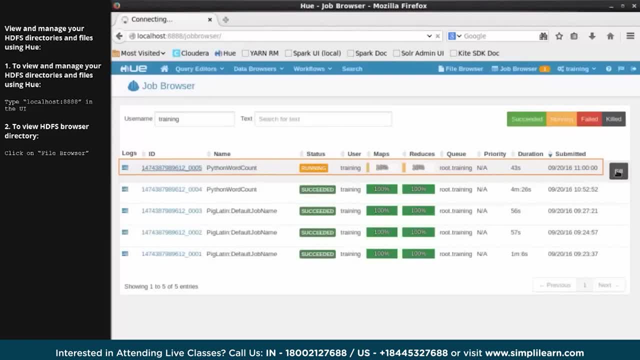 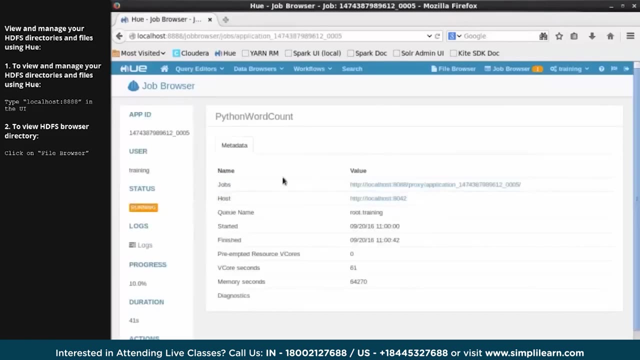 Click ID. You can also click on ID option to view more details of a job. You can also click on Kill option to end this job from UI. Once you enter the application, you can view the running metadata of that YARN. In this page you can also view the information, such as start time. 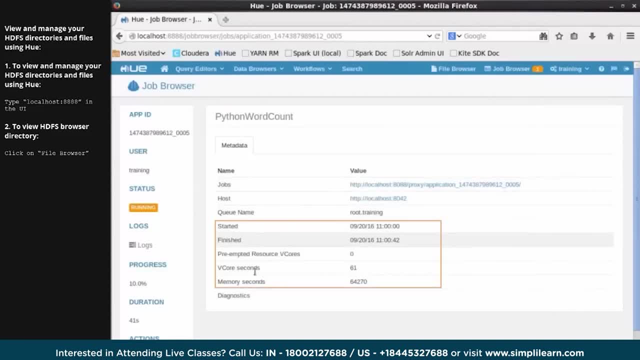 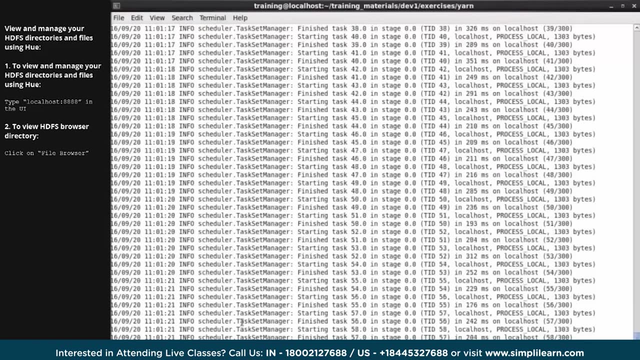 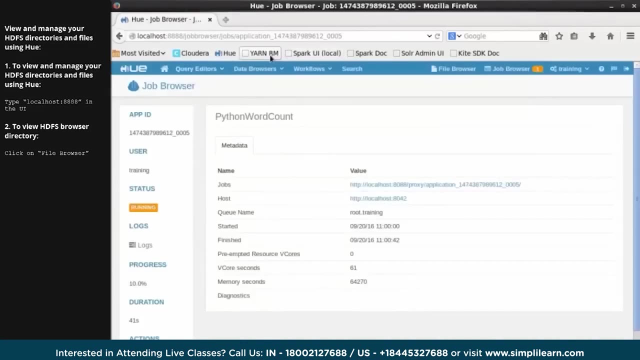 end time and the amount of memory per second that a running program consumes. Let's go back to the terminal. You can check similar details in Web User Interface, which you just viewed from YARN resources. You will need to navigate to the Azure Desktop Manager. 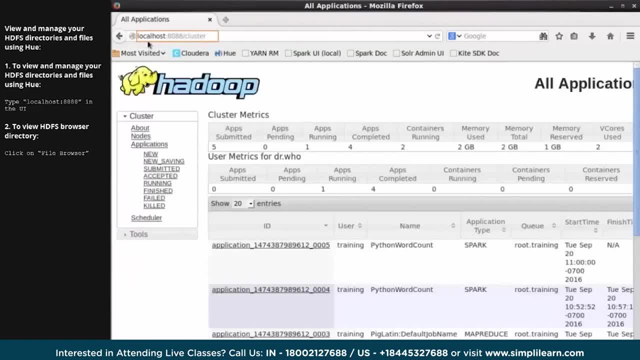 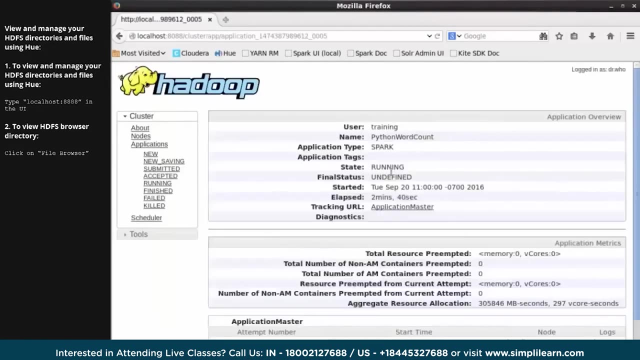 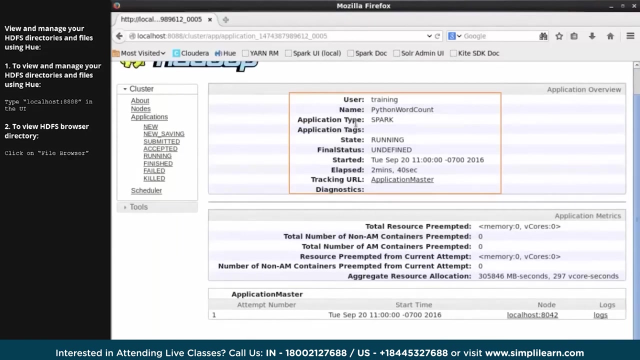 You need to navigate to localhost, colon 8088, slash cluster. You will again notice the running ID. Click this ID to view more details. You will be able to view information such as user name of the program, application type, current state of the running program. 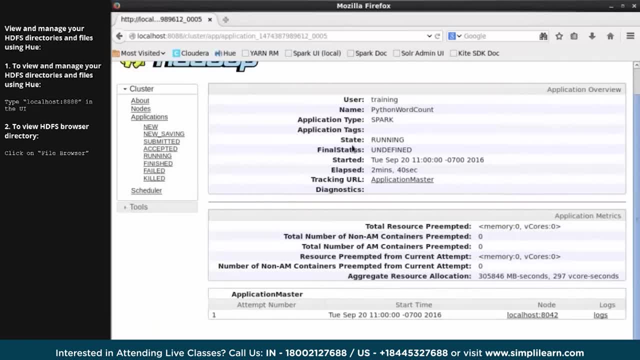 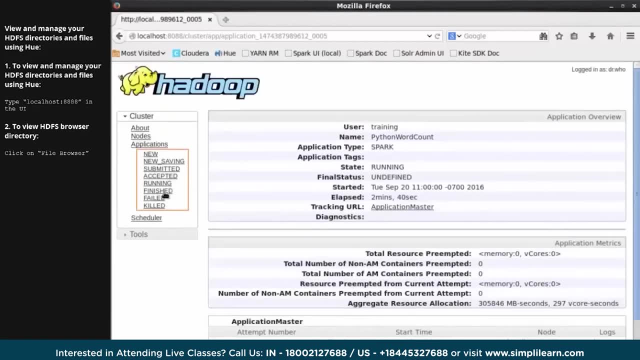 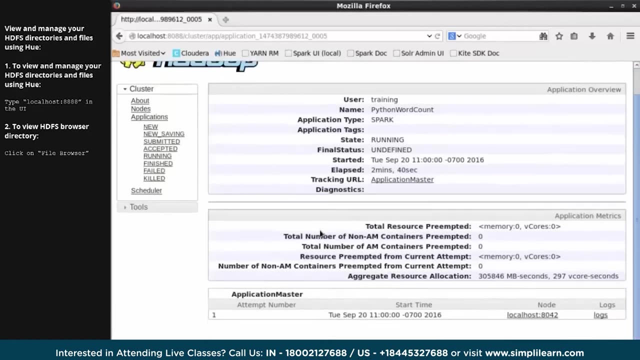 and a few additional information. You can also scroll through the accepted jobs, currently running jobs, finished jobs and a few more details. So this is another web UI page in which you can monitor your yarn progress. Once this program is complete, you can view the output in the terminal. 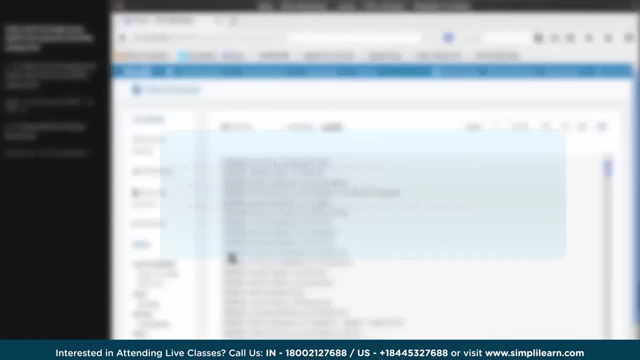 It displays the number of times each word appears. This brings you to the end of this demo. In this demo, you learned the steps to calculate the word count for a file. You have also learned the steps to monitor your yarn progress in a web user interface. 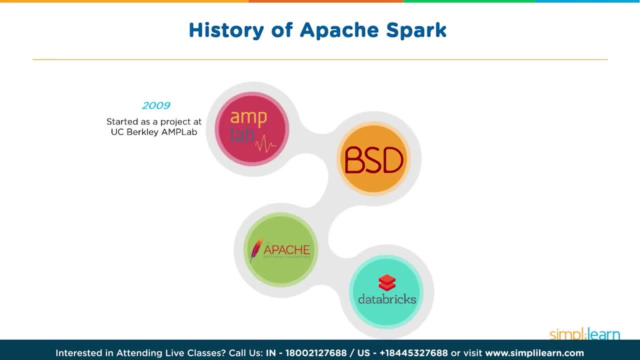 History of Apache Spark. It all started in 2009 as a project at UC Berkeley AMP Labs by Matej Zahiria. In 2010, it was open sourced under a BSD license. In 2013, Spark became an Apache top-level project. 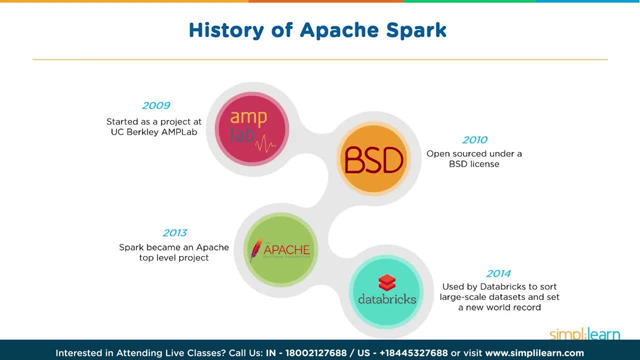 And in 2014, used by Databricks. In 2014,, Spark became the first large-scale database to sort large-scale datasets and it set a new world record. So that's how Apache Spark started, and today it is one of the most in-demand processing. 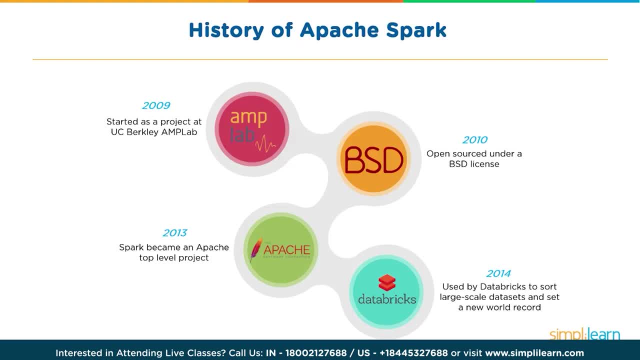 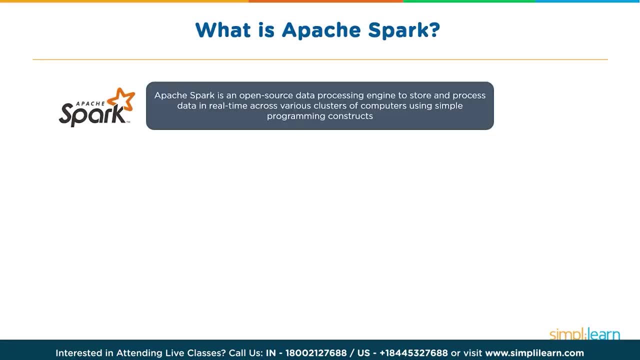 framework, or I would say in-memory computing framework, which is used across the big data industry. So what is Apache Spark? Let's learn about this. Apache Spark is an open-source in-memory computing framework, or you could say data processing engine, which is used to process data. 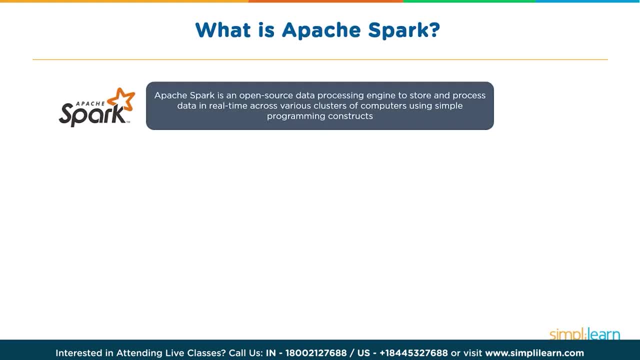 So what is Apache Spark? It is an open-source in-memory computing framework which is used to process data in batch and also in real-time across various cluster computers, And it has a very simple programming language behind the scenes. that is Scala, which is 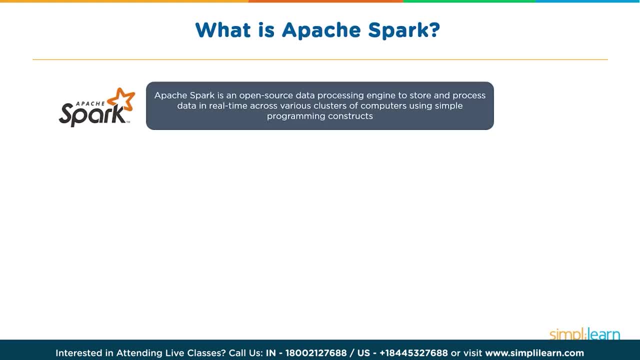 used, Although if users would want to work on Spark, they can work with Python, they can work with Scala, they can work with Java and so on, even R, for that matter. So it supports all these programming languages and that's one of the reasons that it is called. 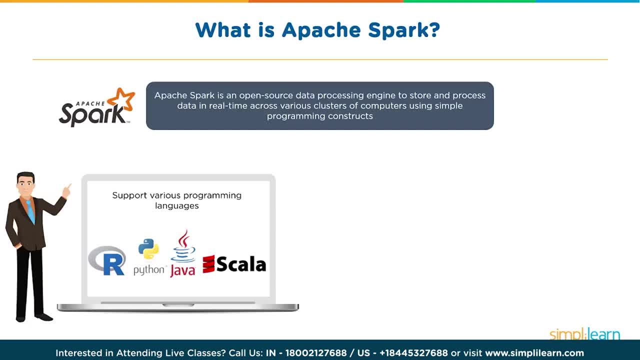 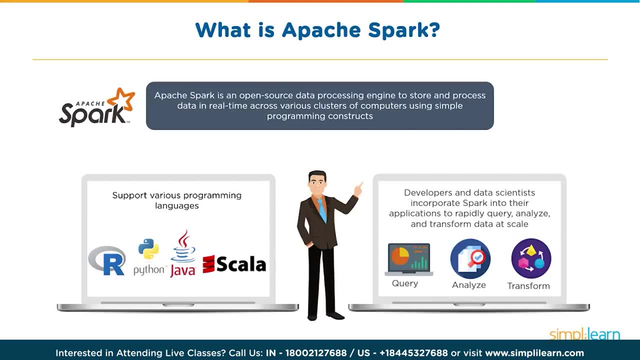 polyglot. You have good set of libraries and support from all the programming languages, And developers and data scientists incorporate Spark into their applications or build Spark-based applications to process, analyze, query and transform data at a very large scale. So these are key features of Apache Spark. 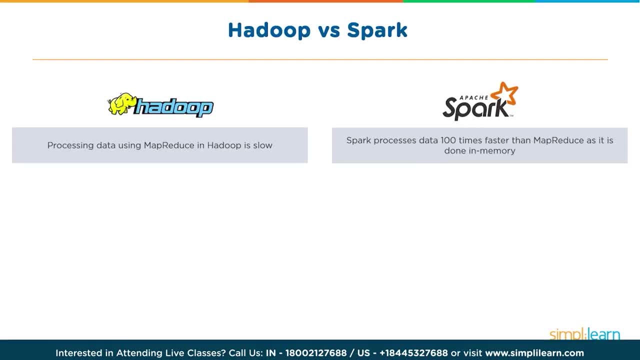 Now, if you compare Hadoop with Spark, we know that Hadoop is a framework And it basically has MapReduce, which comes with Hadoop, for processing data. However, processing data using MapReduce in Hadoop is quite slow because it is a batch-oriented. 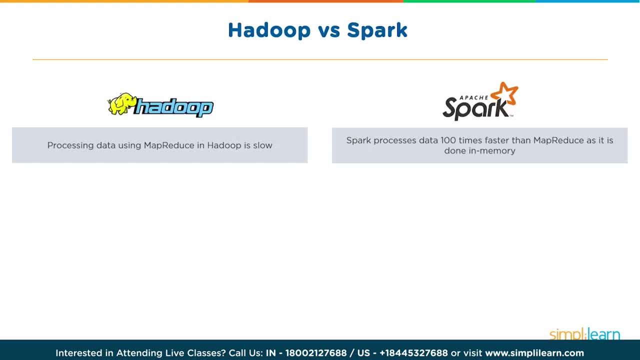 operation and it is time-consuming. If you talk about Spark, Spark can process the same data 100 times faster than MapReduce, as it is an in-memory computing framework. Well, there can always be conflicting ideas saying: what if my Spark application is not? 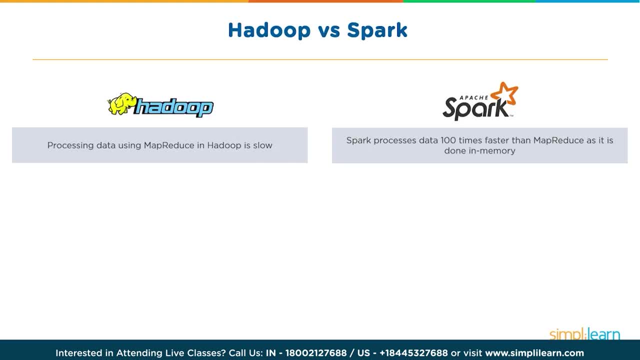 really efficiently coded and my MapReduce application has been very efficiently coded. Well then, it's a different case. However, normally, if you talk about code which is efficiently written for MapReduce or for Spark-based processing, Spark will win the battle by doing almost 100 times faster than 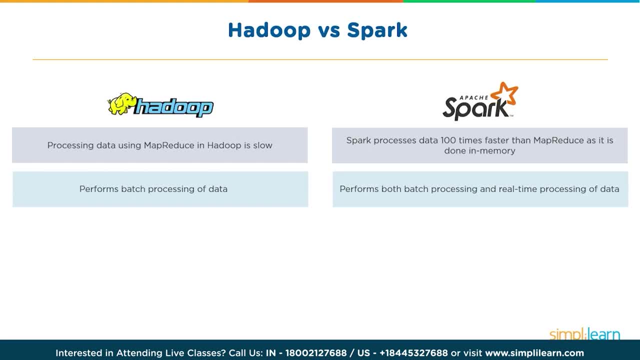 MapReduce. So, as I mentioned, Hadoop performs batch processing and that is one of the paradigms of MapReduce programming model, which involves mapping And that's quite rigid. So it performs batch processing. the intermittent data is written to SDFS and written read back. 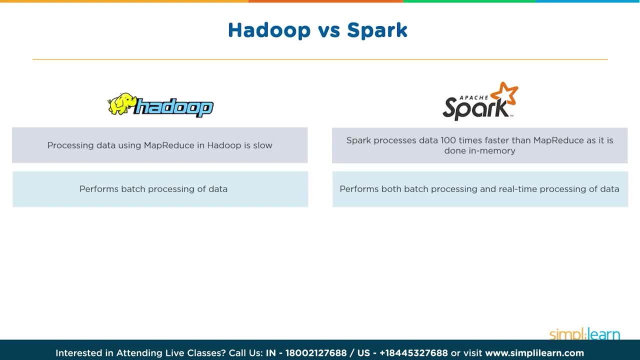 from SDFS and that makes Hadoop's MapReduce processing slower. In case of Spark, it can perform both batch and real-time processing. However, a lot of use cases are based on real-time processing. Take an example of Macy's, take an example of retail giant such as Walmart and there. 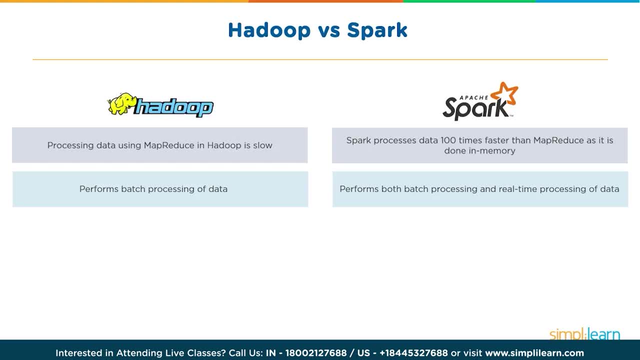 are many use cases Who would prefer to do real-time processing or, I would say, near real-time processing. So when we say real-time or near real-time, it is about processing the data as it comes in, or you're talking about streaming kind of data. 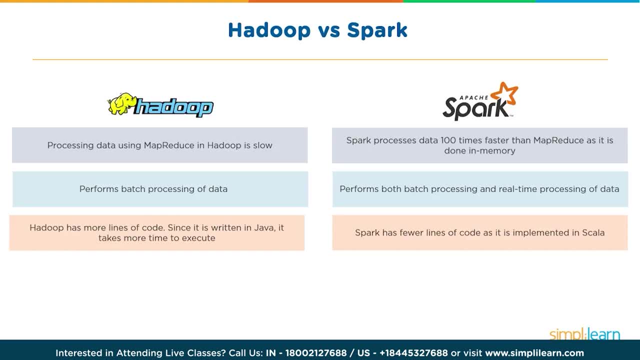 Now Hadoop, or Hadoop's MapReduce, obviously was started to be written in Java. Now you could also write it in Scala or in Python. However, if you talk about MapReduce, it will have more lines of code, since it is written in Java. 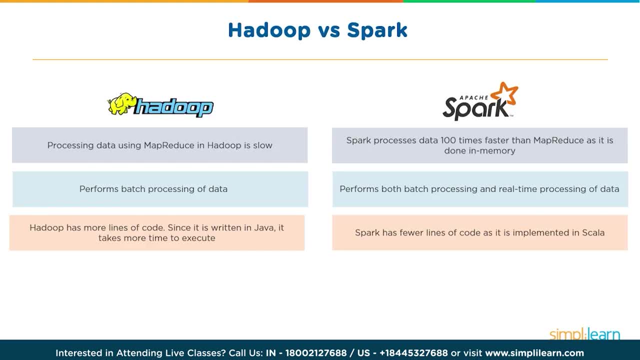 It will take more times to execute. You have to manage the dependencies. You have to do the right declarations, You have to create your mapper and reducer and driver classes. However, if you compare Spark, it has few lines of code as it is implemented in Scala. 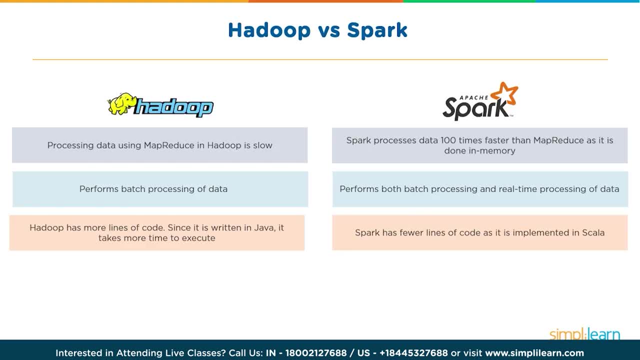 and Scala is a statically typed, dynamically inferred language. It's very, very concise and the benefit is it has features from both functional programming and object-oriented language And in case of Scala, Whatever code is written, that is converted into byte codes and then it runs in the JVM. 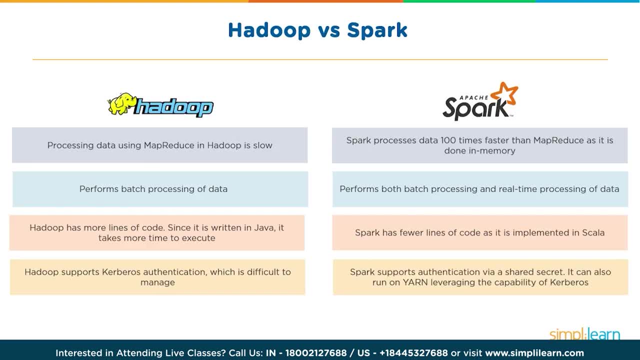 Now Hadoop supports Kerberos authentication. There are different kinds of authentication mechanisms. Kerberos is one of the well-known ones and it can really get difficult to manage. Now Spark supports authentication via a shared secret. It can also run on YARN, leveraging the capability of Kerberos. 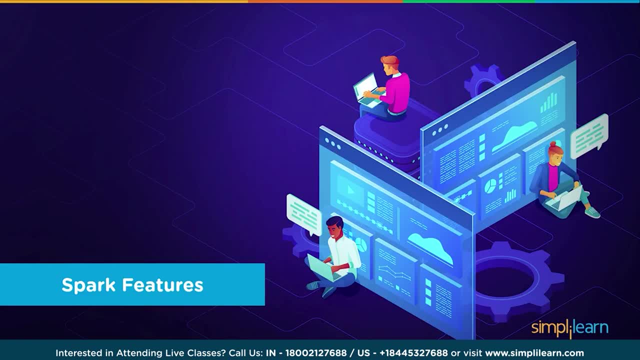 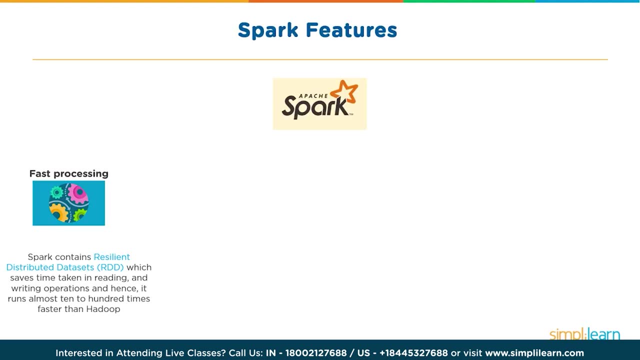 So what are Spark features? which really makes it unique or in demand? When we talk about Spark features, one of the key features is fast processing, So Spark contains resilient, distributed data sets. So RDDs are the building blocks for Spark, and we'll learn more about RDDs later. 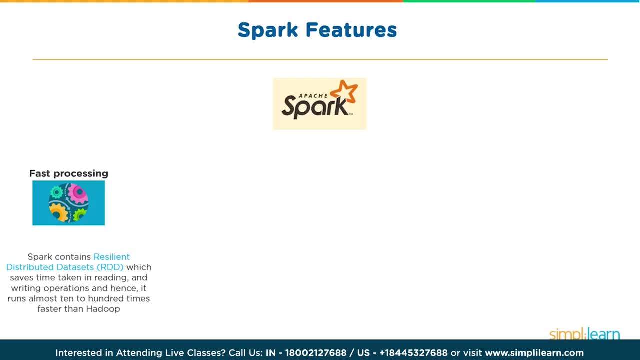 So Spark contains RDDs, which saves huge time taken in reading and writing operations. So it can be 100 times- or you can say 10 to 100 times- faster than Hadoop. When we say in-memory computing here, I would like to make a note that there is a difference between caching. 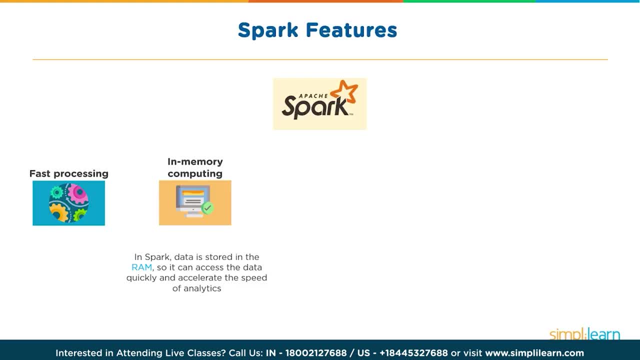 and in-memory computing. Think about it: Caching is mainly to support read-ahead mechanism, where you have your data pre-loaded so that it can benefit further queries. However, when we say in-memory computing, we are talking about lazy evaluation. We are talking about data being loaded into memory only and only when a specific kind. 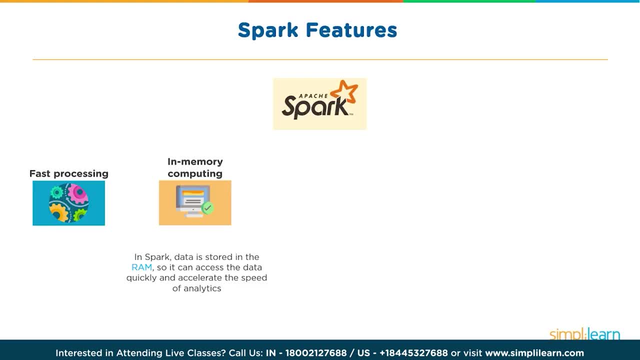 of action is invoked, So data is stored in RAM. So here we can say: RAM is not only used for processing, but it can also be used for storage, and we can again decide whether we would want that RAM to be used for persistence or just for computing. 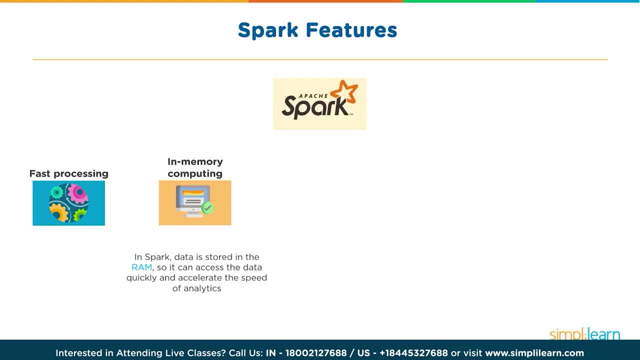 So it can access the data quickly and accelerate the speed of analytics. Now, Spark is quite flexible. It supports multiple languages, as I already mentioned, and it allows the developers to write applications in Java, Scala, R or Python Write fault tolerance. So Spark contains these RDDs, or you could say execution logic, or you could say temporary. 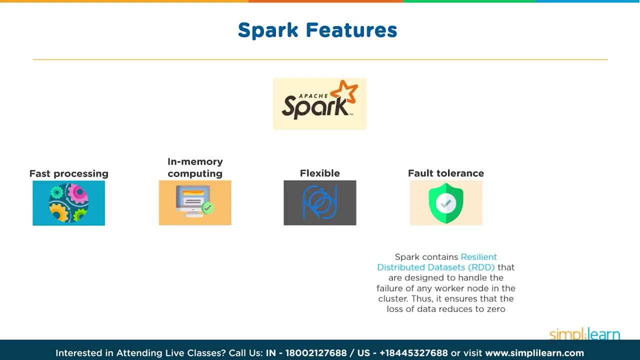 data sets which initially do not have any data loaded, and the data will be loaded into RDDs only when execution is happening. So these can be fault tolerant as these RDDs are distributed across multiple nodes. So failure of one worker node in the cluster will really not affect the RDDs. 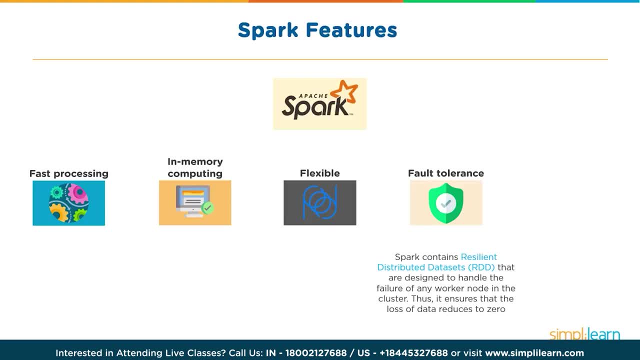 Because that portion can be re-computed. So it ensures loss of data. It ensures that there is no data loss and it is absolutely fault tolerant. It is for better analytics. So Spark has rich set of SQL queries, machine learning algorithms, complex analytics. 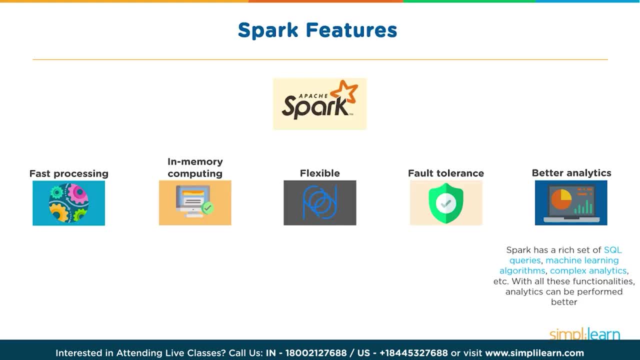 All of this supported by various Spark components which we will learn in coming slides. With all these functionalities, analytics can be performed better in terms of performance. So that's what we are going to talk about today. Thank you for watching this video. I hope you enjoyed it. 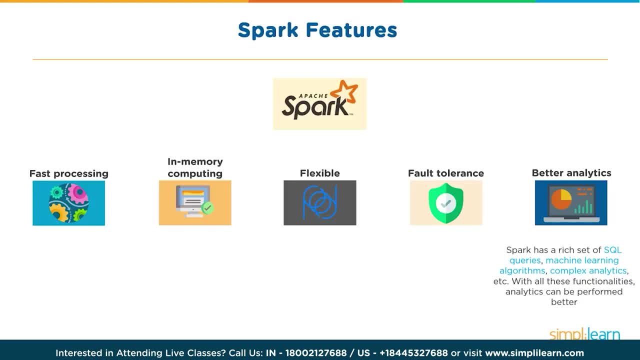 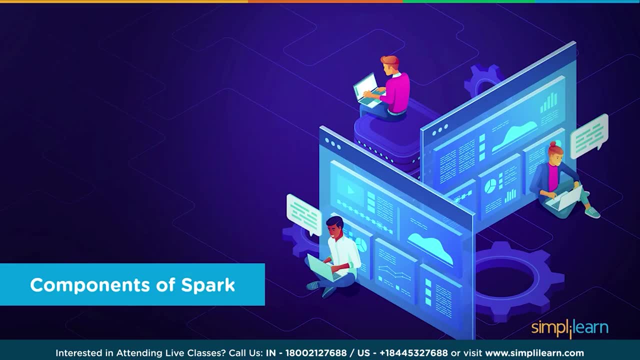 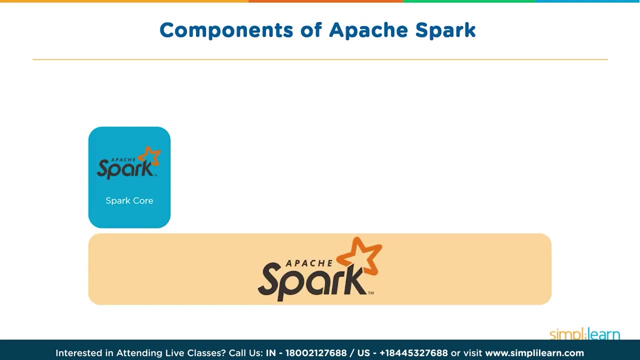 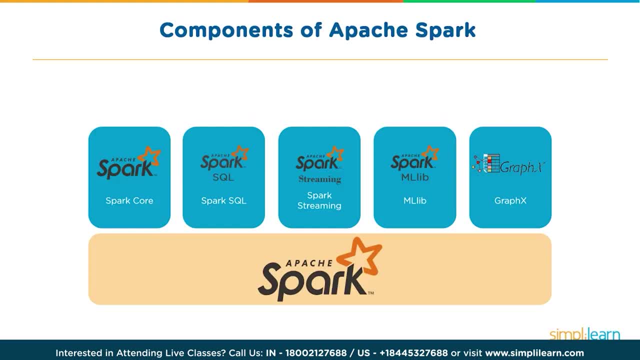 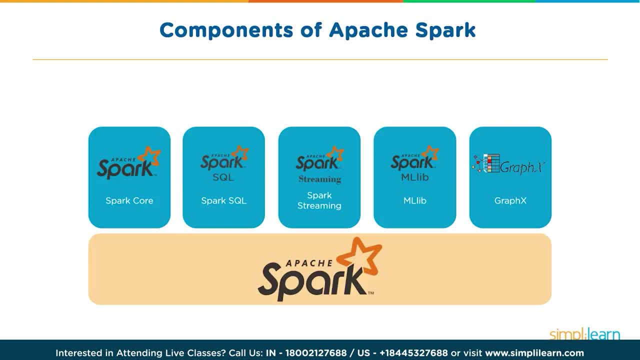 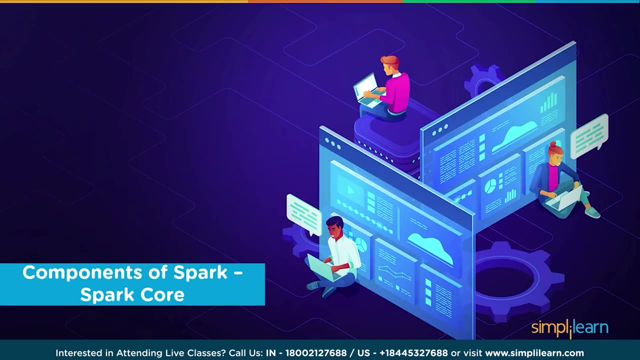 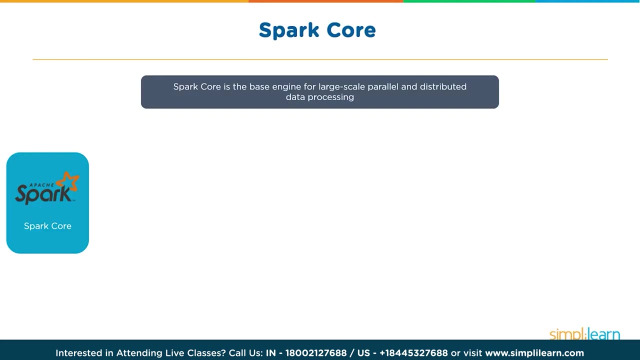 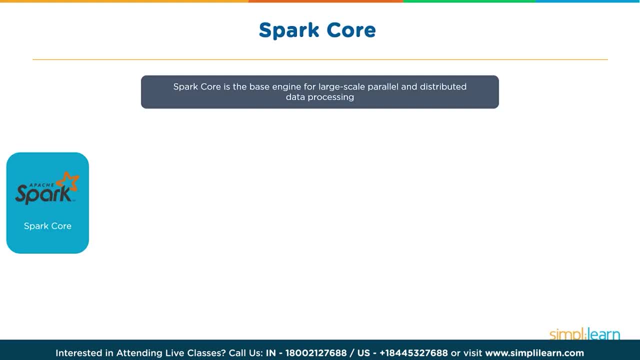 used for large-scale parallel and distributed data processing. so when you work with spark, at least- and the minimum- you would work with a spark core which has RDDs as the building blocks of your spark, so it is responsible for your memory management, your fault recovery, scheduling, distributing and monitoring. 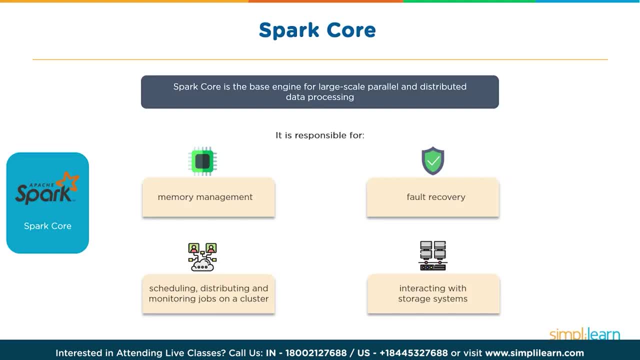 jobs on a cluster and interacting with storage system. so here I would like to make a key point: that spark by itself does not have its own storage. it relies on storage. now that storage could be your SDFS, that is, Hadoop's distributed file system. it could be a database, like no SQL database such as HBase or it. 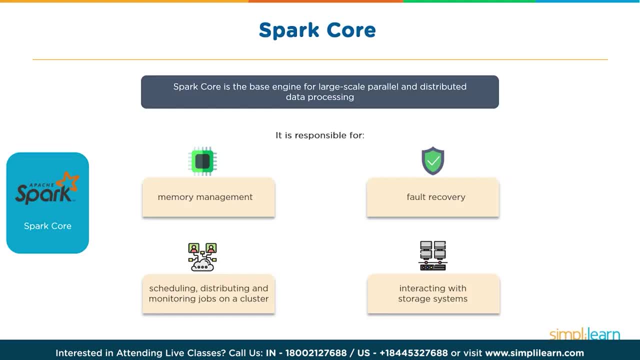 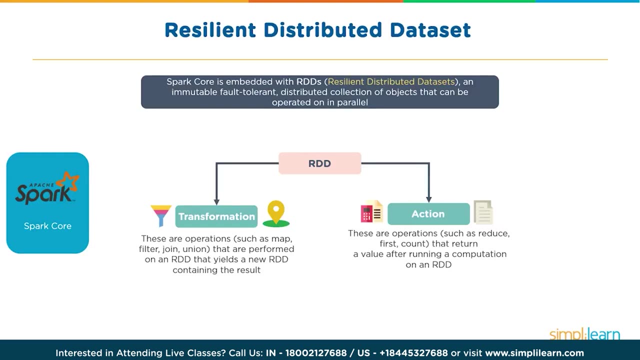 could be any other database, say RDBMS, from where you could connect your spark and then fetch the data extra, the data process it analyze it. so let's learn a little bit about your RDDs, resilient distributed datasets. now spark core, which is the base engine or the 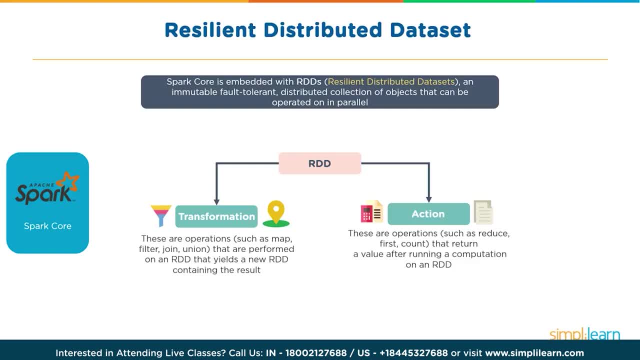 core engine is embedded with the building blocks of spark, which is nothing but your resilient distributed datasets. so, as the name says, it is resilient, so it is existing for a shorter period of time. distributed, so it is distributed across nodes and it is a data set where the data will be loaded or where the data will be. 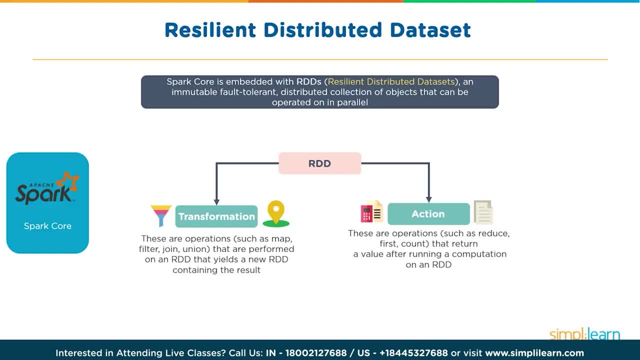 existing for processing. so it is immutable, fault tolerant, distributed collection of objects. so that's what your RDD is, and there are mainly two operations which can be performed on an RDD. now, to take an example of this, say, I want to process a particular file now. here I could write a simple code in: 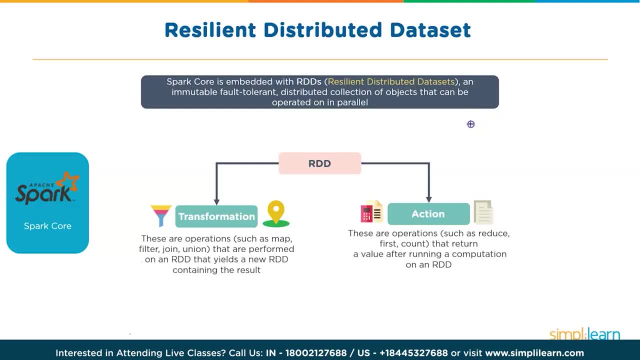 in Scala, and that would basically mean something like this: So if I say val, which is to declare a variable, I would say val x, and then I could use what we call a spark context, which is basically the most important entry point of your application. So then I could use a method of spark context. 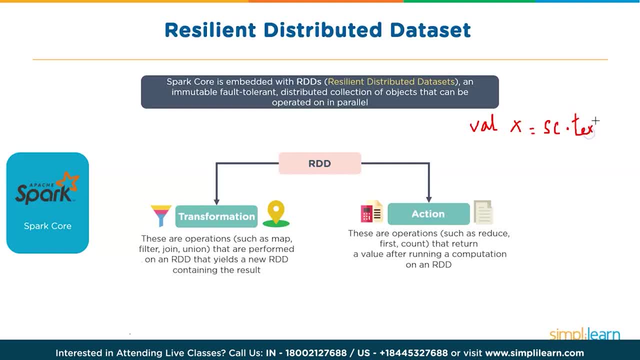 for example, that is text file, and then I could point it to a particular file. So this is just a method of your spark context, and spark context is the entry point of your application. Now, here I could just give a path in this method. So what does this step do? It does not do any valuation. 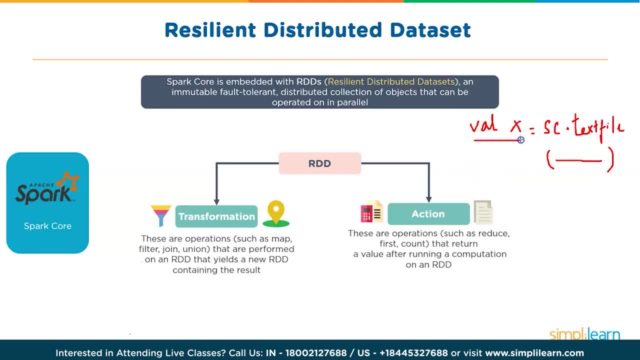 So when I say val x, I'm creating a immutable variable and to that variable I'm assigning a file. Now what this step does is it actually creates a RDD resilient distributed data set. So we can imagine this as a simple execution logic, a empty data set which is created in memory of your node. So if I would 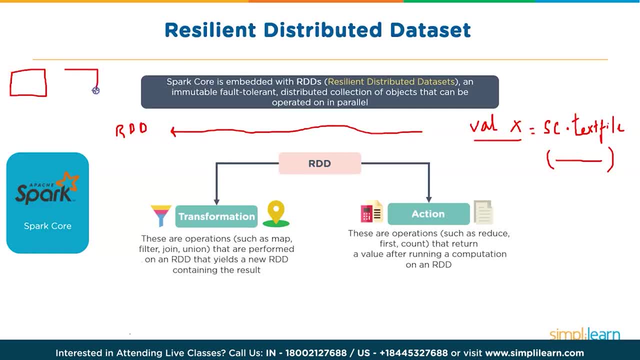 say, I have multiple nodes in which my data is split and stored, imagining that your yarn, your spark, is working with Hadoop. So I have Hadoop, which is using, say, two nodes, and this is my distributed file system, HDFS, which basically means my file is written to HDFS and it also 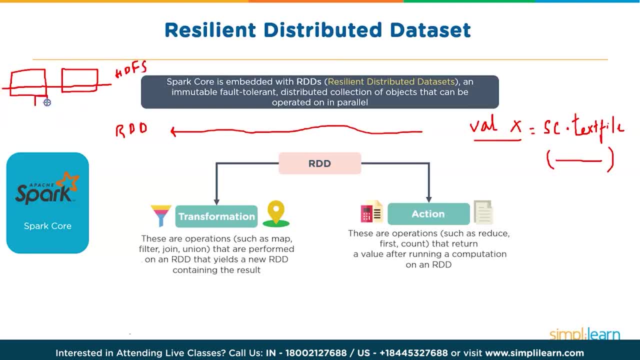 means that the file related blocks are stored in the underlying disk of these machines. So when I say val x equals sc dot text file, that is using a method of spark context. Now there are various other methods, like whole text files, parallelize and so on. This step will create an RDD, So you can imagine this as a logical data. 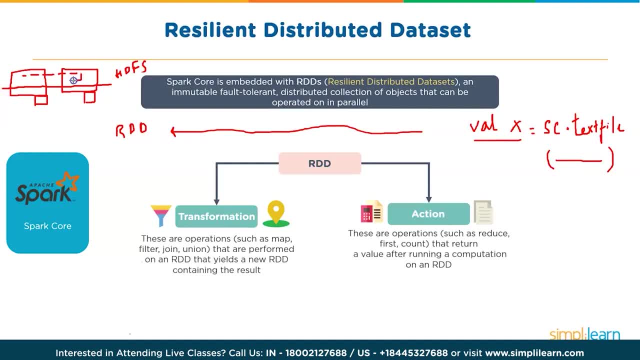 set which is created in memory across these nodes, because these nodes have the data. However, no data is loaded Here. So this is the first RDD and, I can say, first step in what we call as a tag, a tag which will have CDs of steps which will get executed at later stage. Now, later I could do further processing on. 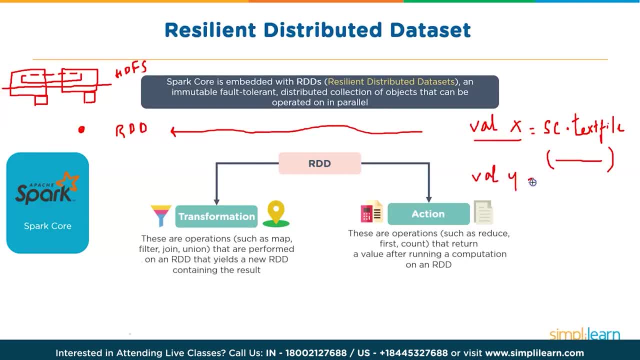 this. I could say well, why. And then I could do something on X. So I could say X dot map and I would want to apply a function to every record or every element in this file And I could give a logic here: X dot map. Now this second step is again creating an RDD, a resilient distributed 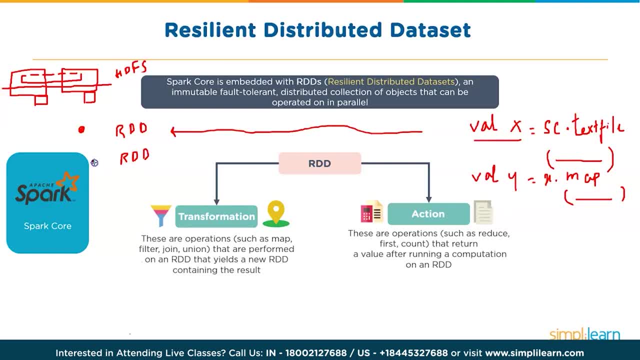 data set. You can say: second step in my DAG, OK, And here you have a external RDD, one more RDD created which depends on the first RDD. So my first RDD becomes the base RDD or parent RDD and the resultant RDD becomes the child RDD. Then we can go further and we could say val z and I. 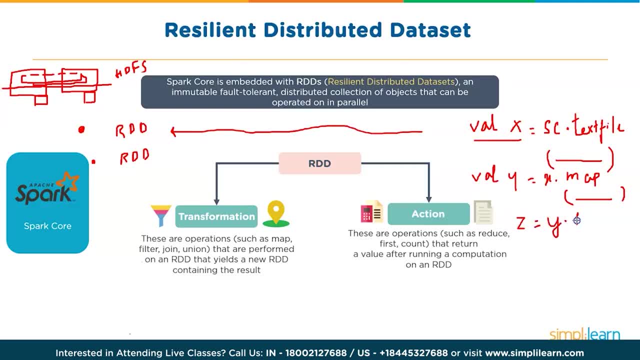 would say: OK, Now I would want to do some filter on Y. So this filter which I am doing here and then I could give a logic, might be I'm searching for a word, I'm searching for some pattern. So I could say: val z equals Y dot filter, which again creates one more RDD, a resilient distributed data. 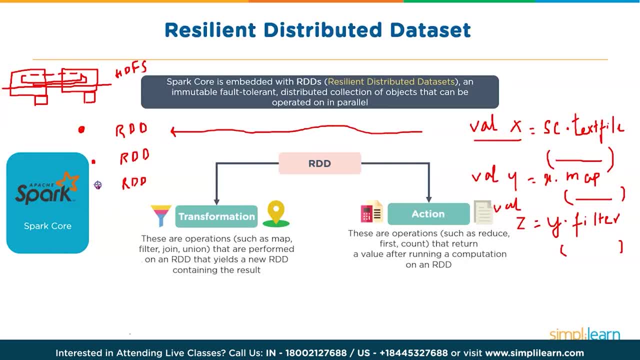 set in memory And A you can say: this is nothing but one more step in the DAG. So this is my DAG, which is the first step in the DAG. So this is my DAG, which is the first step in the DAG. So this is my DAG, which is the second step in the DAG. So this is my DAG, which is the first step in the DAG. 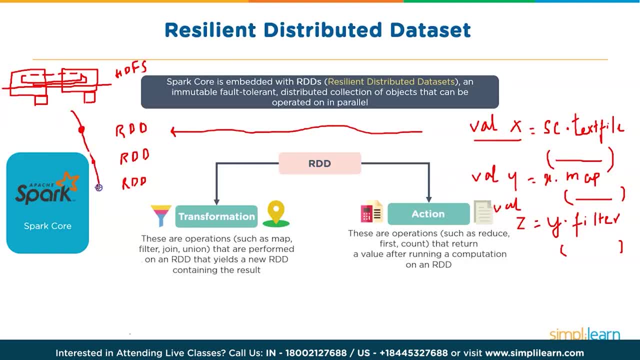 So this is my DAG, which is a series of steps which will be executed Now here. when does the execution happen? when the data get, when will the data get loaded into these RDDs? So all of this, that is, using a method, using a transformation like map, using a transformation like filter or flat. 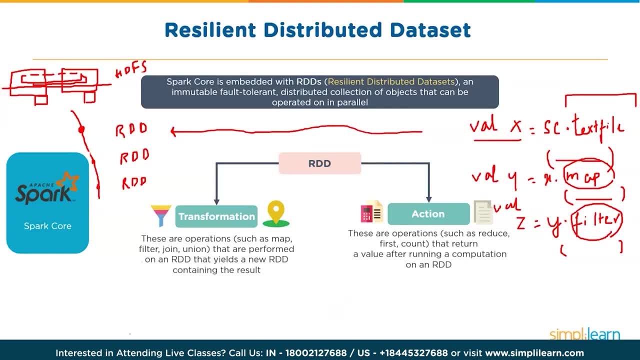 map or anything else. These are your transformations, So the operations such as map, filter, join, union and many others will only create RDDs, which basically means it is only creating execution logic. No data is evaluated, No operation is happening right now, Only and only when you. 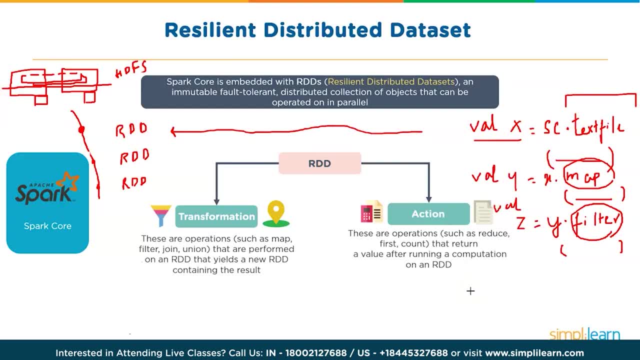 invoke an action that is: might be you want to print some result. might be you want to take some elements and see. that. might be you want to do a count. So those are actions which will actually trigger the execution of this DAG right from the beginning. 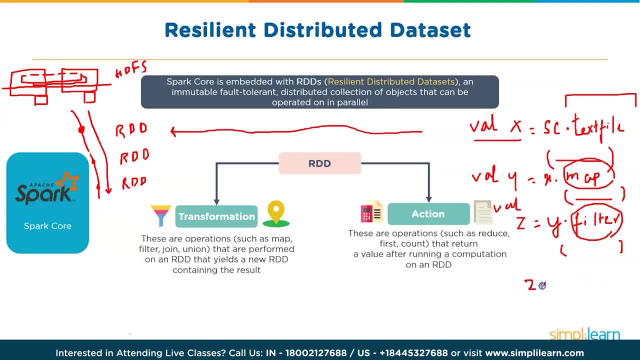 So if I hear, say, Z dot count, where I would want to just count the number of words which I'm filtering, This is an action which is invoked and this will trigger the execution of DAG right from the beginning. So this is what happens in a spark. Now, if I do a Z dot count again it will start. 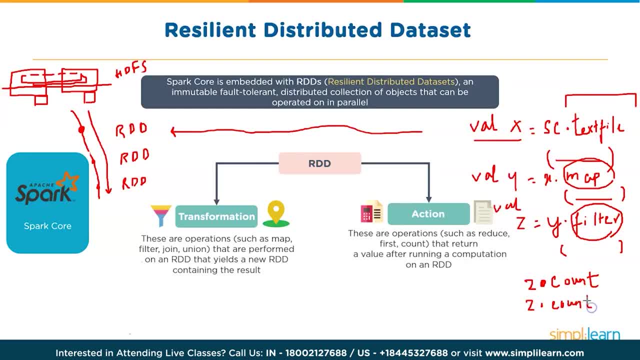 the whole execution of DAG again, right from the beginning. So my Z dot count. second time an action is invoked Again, the data will be loaded in the first RDD, then you will have map, then you will have filter and finally you will have result. So this is the core concept of your 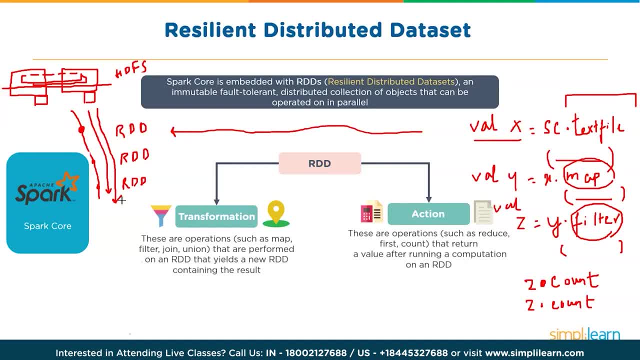 RDDs and this is how RDD works. So, mainly in spark, there are two kind of operations: One is your transformations and one is your actions. Transformations, or using a method of spark context, will always and always create an RDD, Say a step in the DAG. Actions are something which will invoke the execution, which will invoke the 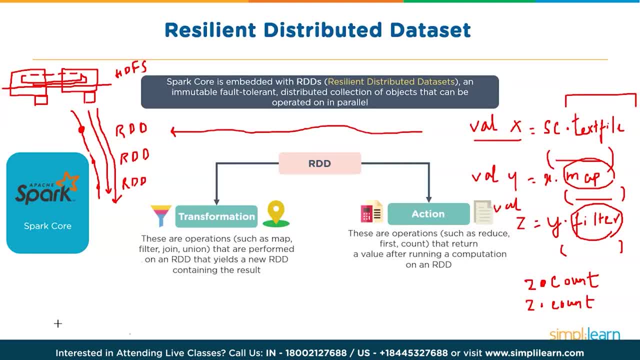 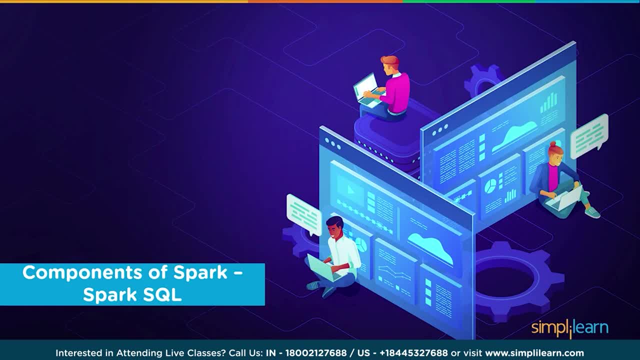 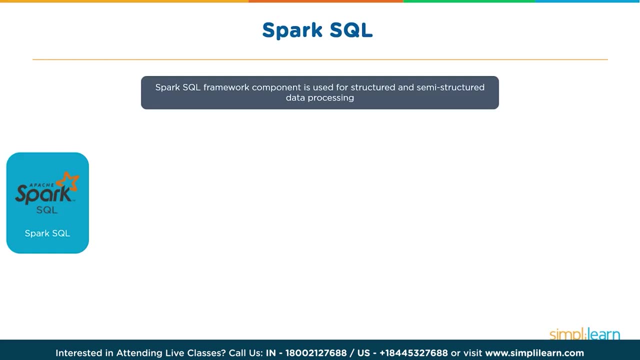 execution from the first RDD till the last RDD where you can get your result. So this is how your RDDs work. Now, when we talk about components of spark, let's learn a little bit about spark SQL. So Spark SQL is a component type processing framework which is used for structured and 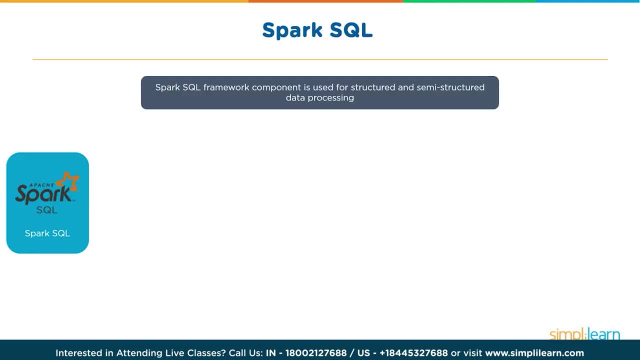 semi-structured data processing. So Spark SQL is a component type processing framework which is used for structured and semi-structured data processing. So usually people might have their structured data stored in RDBMS or in files where data is structured with particular delimiters and has a pattern. and if one wants to process this structured data, if one 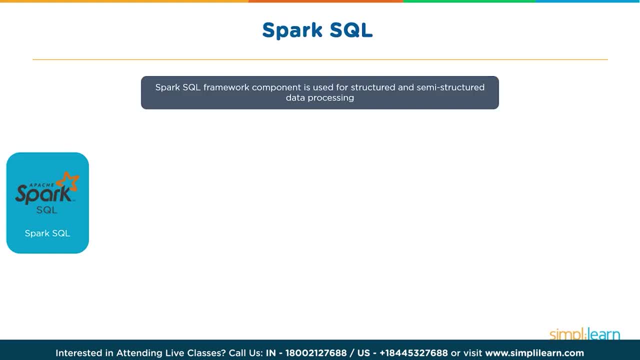 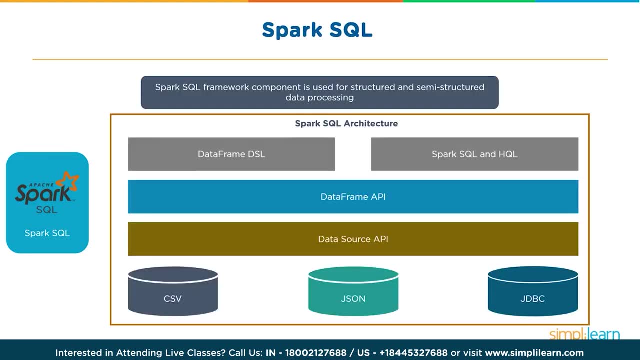 wants to use spark to do in-memory processing and work on this structured data. they would prefer to use Spark SQL, So you can work on different data formats, say CSV, JSON. you can even work on smarter formats like Avro parquet. even you have binary files or sequence files You could have. 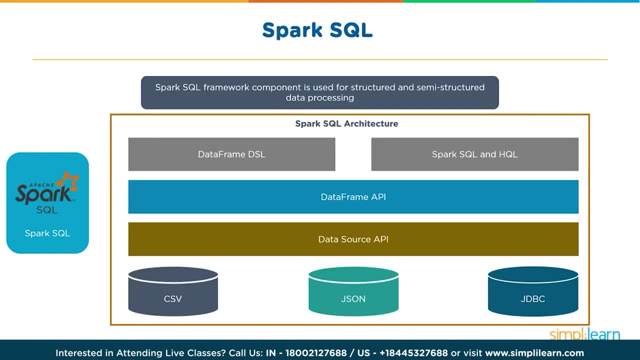 your data coming in from a RDBMS, which can then be extracted using a JDBC connection. So, at the bottom level, when you talk about Spark SQL, it has a data source API which basically allows you to get the data in whichever format. it is Now Spark SQL. 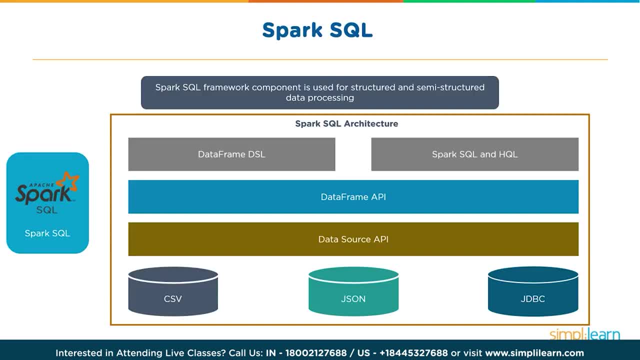 has something called data frame API. So what are data frames? Data frames in short, you. you can visualize or imagine as rows and columns, or if your data can be represented in the form of rows and columns with some column headings. So DataFrame API allows you to create DataFrames. 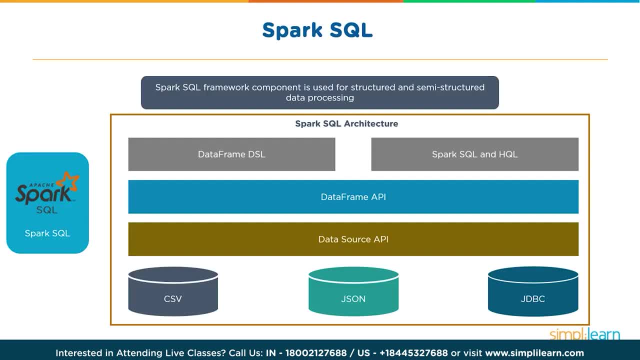 So, like my previous example, when you work on a file, when you want to process it, you would convert that into an RDD using a method of Spark Context or by doing some transformations. So, in the similar way, when you use DataFrames or when you want to use Spark SQL, 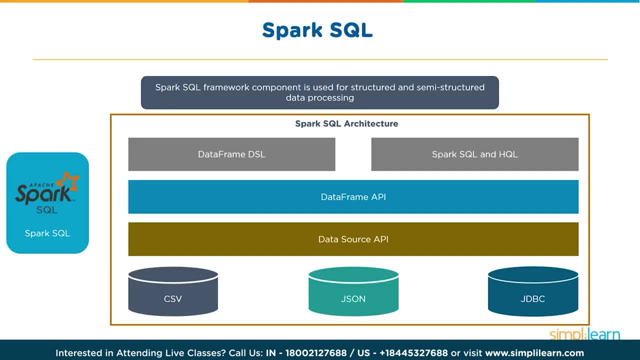 you would use Spark's Context, which is SQL Context, or Hive Context, or Spark, which allows you to work with DataFrames. So, like in my earlier example, we were saying: val x equals sctxt file. Now, in case of DataFrames, instead of sc you would be using, say, spark. 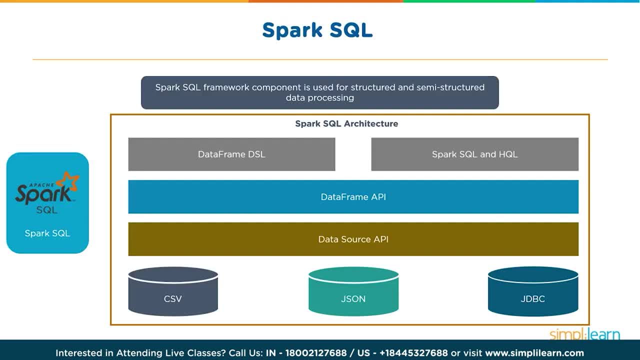 something, So Spark Context is available for your DataFrames API to be used. In older versions like Spark, you would be using Sparkcontext, So Sparkcontext is available for your DataFrames and so on. We were using Hive Context or SQL Context, So if you were working with Spark 1.6,. 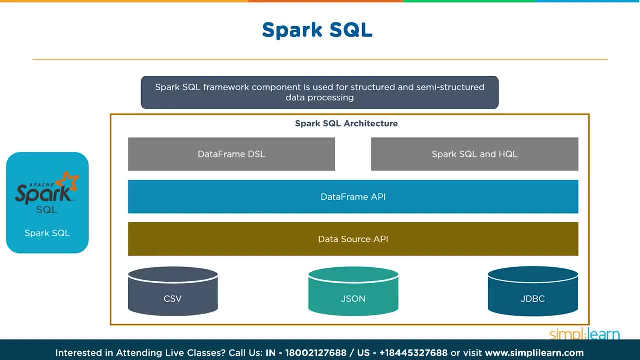 you would be saying: val x equals SQL Context dot. Here we would be using Spark dot. So DataFrame API basically allows you to create DataFrames out of your structured data, which also lets Spark know that data is already in a particular structure. It follows a format and 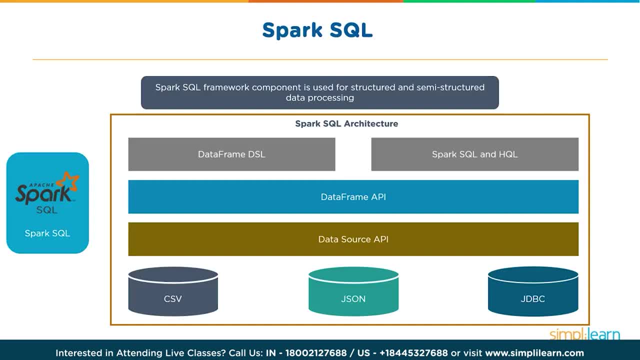 based on that, your Spark's data is already in a particular structure, So you would be using back-end DAG scheduler, right? So when I say about DAG, I talk about your sequence of steps, So Spark is already aware of what are the different steps involved in your application. 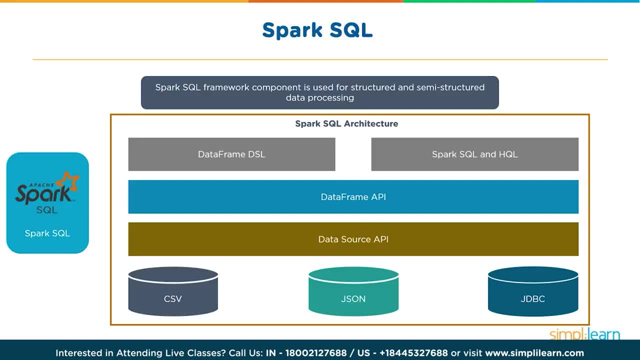 So your DataFrame API basically allows you to create DataFrames out of your data And DataFrames. when I say, I'm talking about rows and columns with some headings, And then you have your DataFrame DSL language or you can use Spark SQL or Hive Query Language. So you can use Spark SQL or Hive Query. 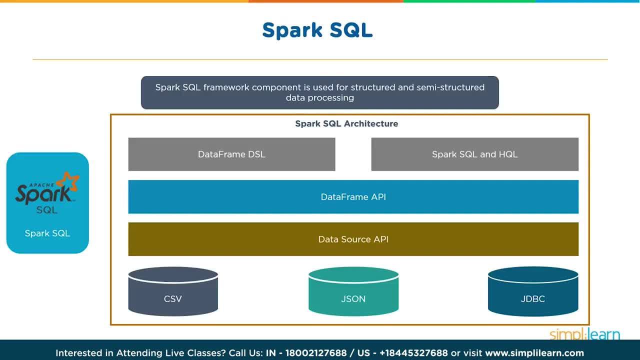 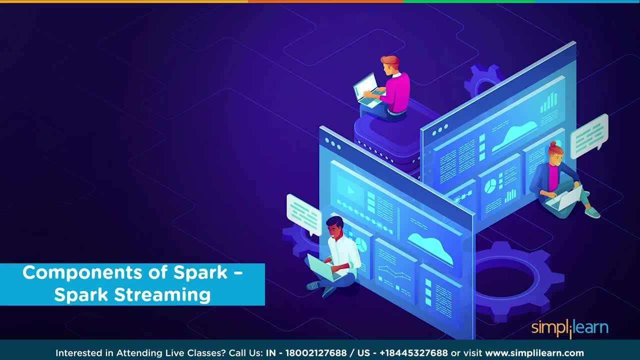 Language, or you can use Spark SQL or Hive Query Language. So you can use Spark SQL or Hive Query Language. Any of these options can be used to work with your DataFrames. So to learn more about DataFrames, follow in the next sessions When you talk about Spark streaming. now, this is very 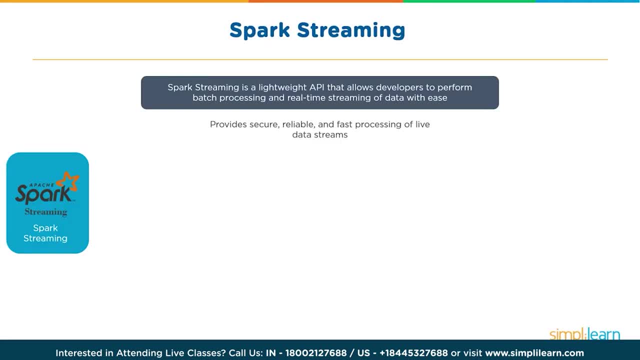 interesting for organizations who would want to work on streaming data. Imagine a store like Macy's where they would want to have machine learning algorithms. Now what would these machine learning algorithms do? Suppose you have a lot of customers walking in the store and they 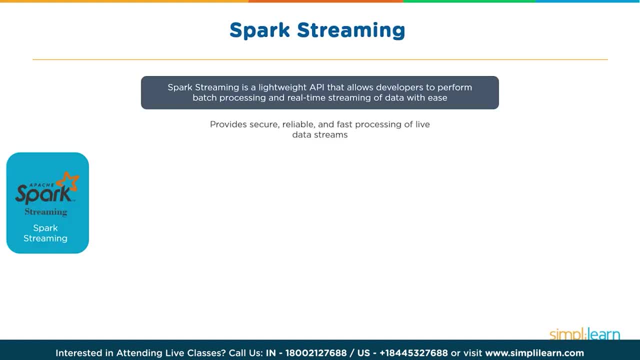 are searching for a particular product or a particular item. So there could be cameras placed in the store, And this is being already done. There are cameras placed in the store which will keep monitoring in which corner of the store there are more customers Now, once camera captures this. 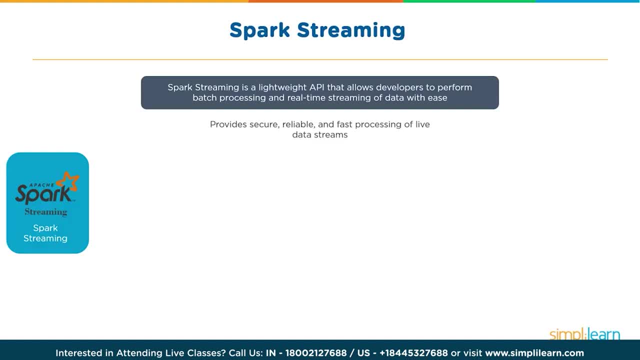 information. this information can be streamed in to be processed by algorithms, And those algorithms will see which product or which series of product customers might be interested in And if this algorithm, in real time, can process based on the number of customers, based on the 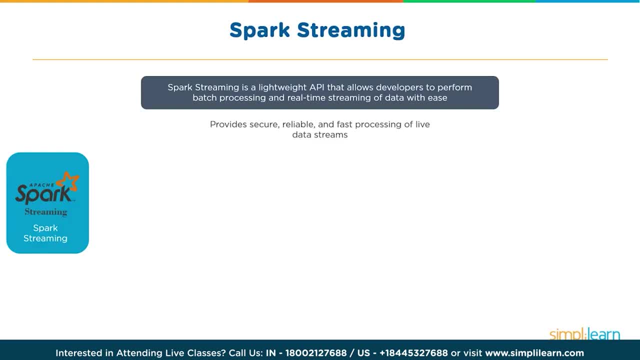 available product in the store, it can come up with an attractive alternative price, so that which the price can be displayed on the screen and probably customers would buy the product. Now, this is a real-time processing, where the data comes in. algorithms work on it, do some computation. 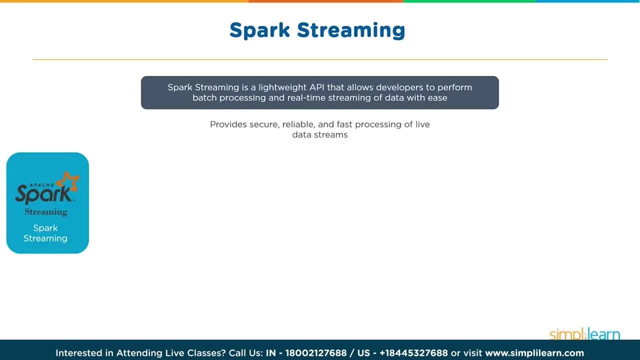 and give out some result And which can then result in customers buying a particular product. So the whole essence of this machine learning and real-time processing will really hold good if and when customers are in the store. Or this could relate to even an online shopping portal, where there might be machine learning algorithms which might 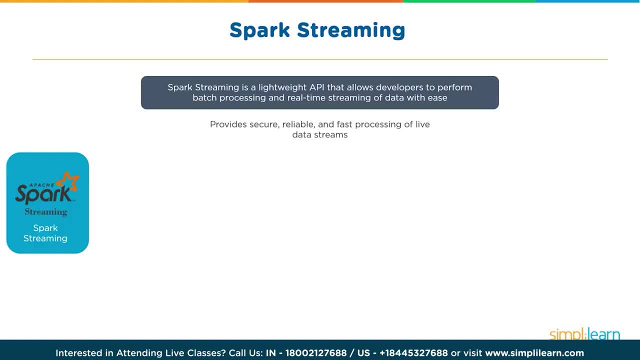 be doing real-time processing based on the clicks which customer is doing. Based on the clicks, based on customer history, based on customer behavior, algorithms can come up with recommendation of products or better information. So this is a real-time processing where the 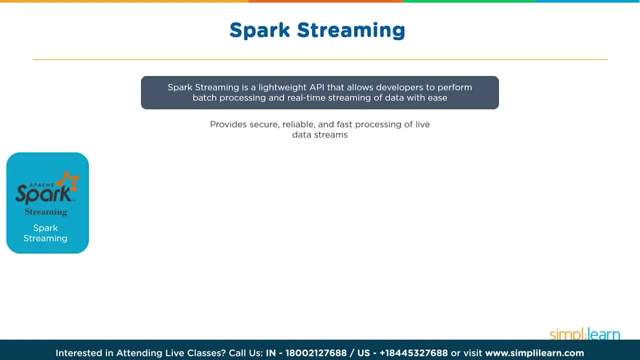 data comes in. So in this case we would be seeing the essence of real-time processing only in a fixed or in a particular duration of time, And this also means that you should have something which can process the data as it comes in. So Spark streaming is a lightweight API that allows. 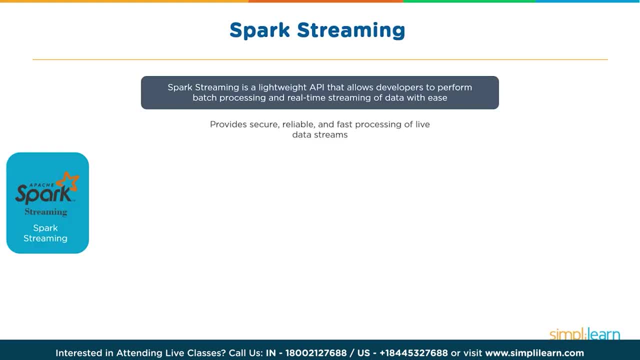 developers to perform batch processing and also real-time streaming and processing of data. So it is secure, reliable, fast processing of live data streams. So what happens here in Spark streaming? in brief, So you have an input data stream. Now that data stream could be a file which is 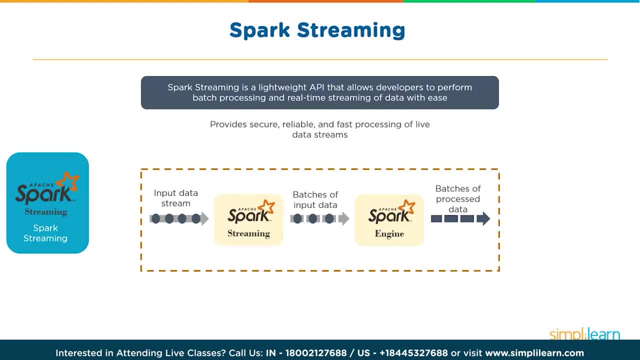 constantly getting appended. It could be some kind of metrics, It could be some kind of events based on the clicks which customers are doing or based on the products which they are choosing in a store. This input data stream is then pushed in through a Spark streaming application- Now, Spark streaming. application will break this control, So it will get the solid data stream from it and it will start to work on it. So we will see when it runs. So it will see if we can support our data source on a site. 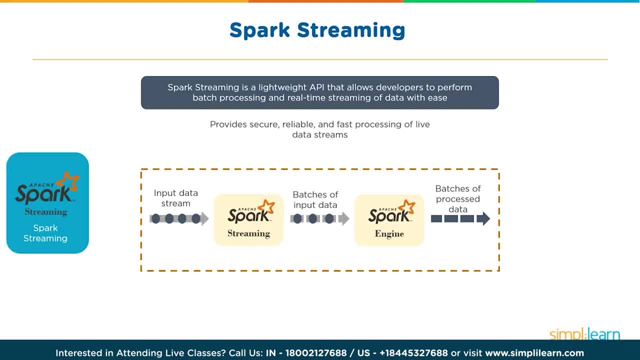 And then you can see the specific data stream here where the data stream is supported. Now this data stream can connect content into smaller streams, what we call as discriticized streams, or batches of smaller data on which processing can happen in frames, so you could say: process my file every five seconds, for 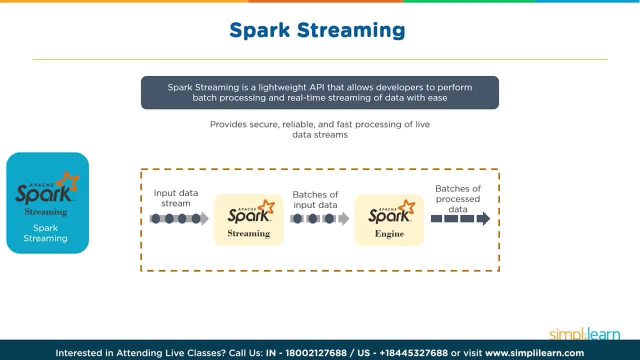 the latest data which has come in. now there are also some windows based uh options like. when i say windows, i mean a window of past three events. window of past three events, each event being of five seconds. so your batches of smaller data is processed by spark engine and this process data. 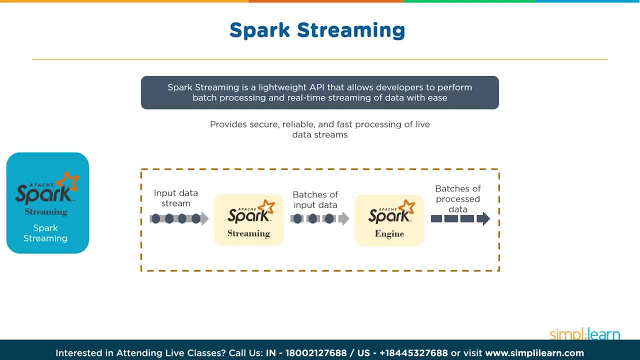 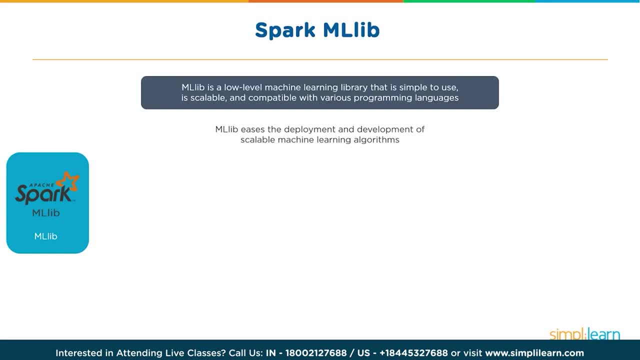 can then be stored or can be used for further processing. so that's what spark streaming does. when you talk about ml lib, it's a low-level machine learning library that is simple to use, scalable and compatible with various programming languages. now hadoop also has some libraries like 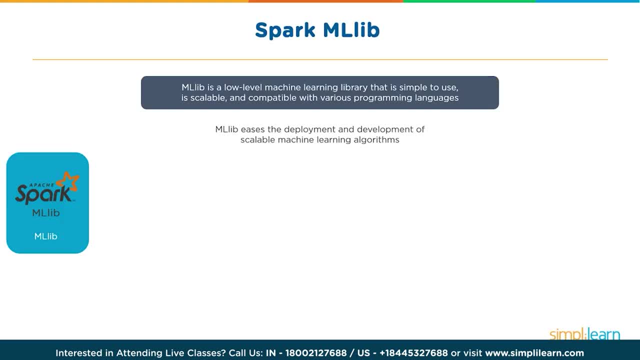 you have apache mahout, which can be used for machine learning algorithms. however, in terms of spark, we are talking about machine learning algorithms which can be built using ml libs libraries and then spark can be used for processing. so ml lib eases the deployment and development of scalable machine learning. 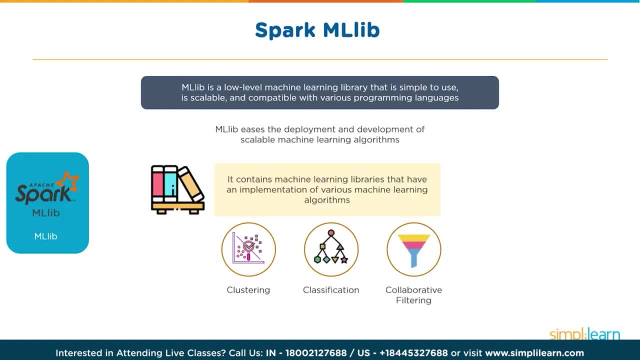 algorithms. i mean think about your clustering techniques. so think about your classification: where you would want to classify the data, where you would want to do supervised or unsupervised learning. think about collaborative filtering and many other data science related techniques or techniques which are required to build your recommendation engines or machine learning. 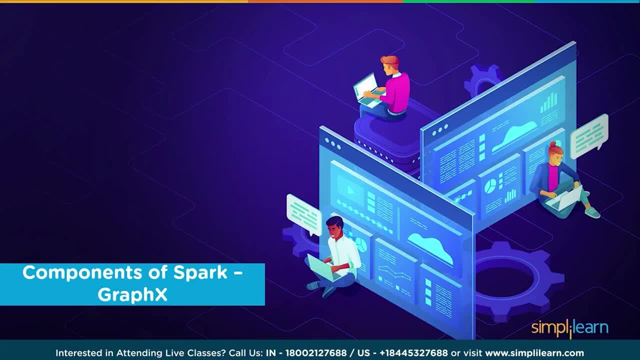 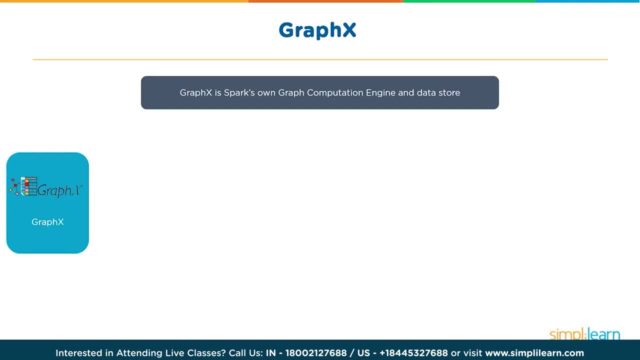 algorithms can be built using sparks. ml lib graphics is sparks own graph computation engine. so this is mainly if you are interested in doing a graph based processing. think about facebook, think about linkedin, where you can have your data which can be stored, and that data has some kind of 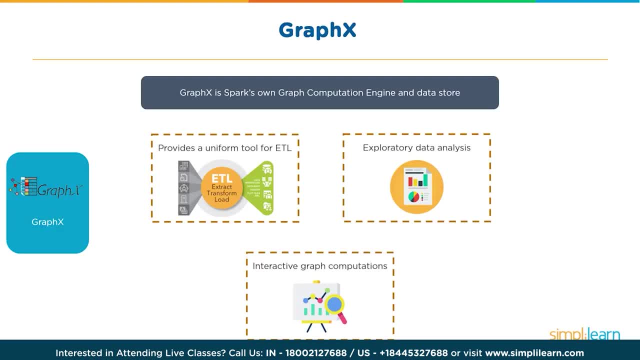 network connections, or you could say it is well networked. i could say: x is connected to y, y is connected to z, z is connected to a. so x, y, z, a. all of these are in terms of graph, terminologies we call as vertices or vertex, which are basically being: 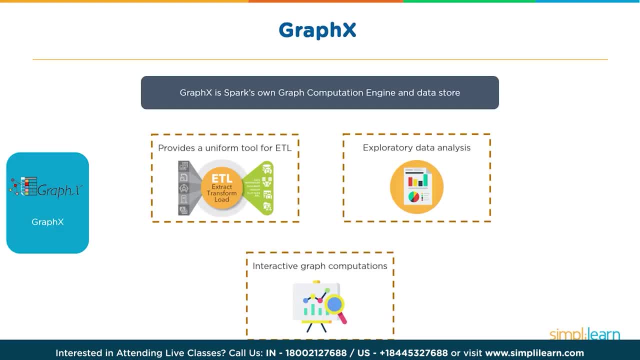 connected and the connection between these are called edges. so i could say a is friend to b, so a and b are vertices and friend to b is friend to b. so a and b are vertices and friend to b are end. a relation between them is the edge. now, if i have my data, which can be represented in the form: 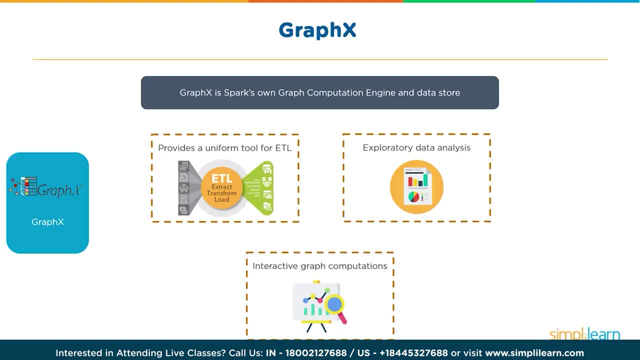 of graphs. if i would want to do a processing in such way. this could be not only for social media, it could be for your network devices, it could be a cloud platform, it could be about different applications which are connected in a particular environment. so if you have data which can be, 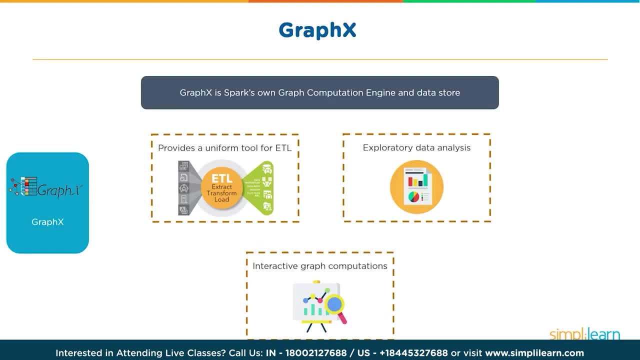 represented in the form of graph, then graphics can be used to do etl, that is, extraction, transformation load to do the processing of the data which can be represented in the form of graph. so if you have data which can be represented in the form of graph, then graphics can be used to do etl, that is, extraction. 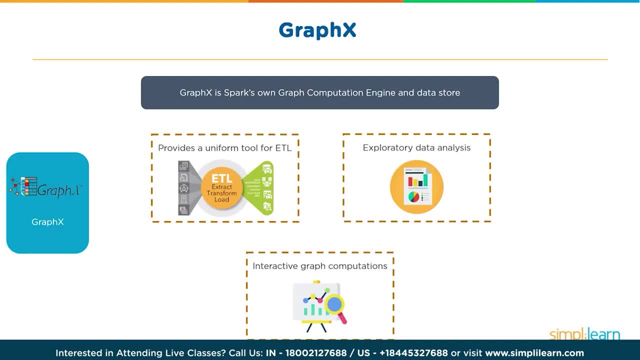 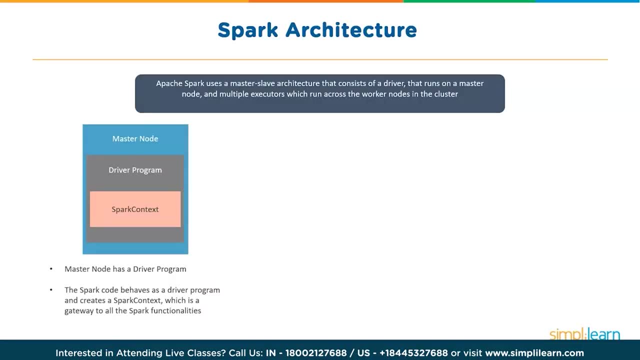 load to do etl, that is extraction. load to do etl, that is extraction. load to do etl, that is extraction. so graphics is quite powerful. now, when you talk about spark, your spark can work with your different clustering uh technologies. so it can work with apache mesos. that's how spark came in where it was. 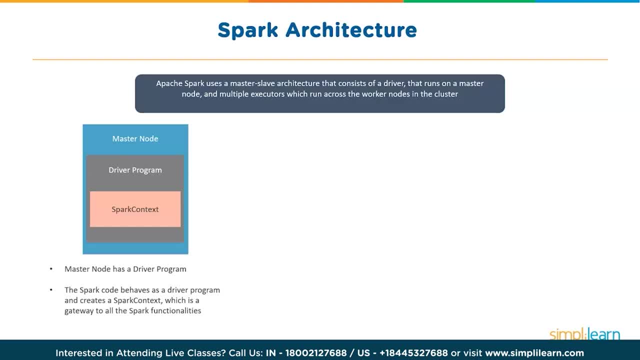 initially to prove the credibility of apache mesos. spark can work with yarn, which is usually you will see in different working environments. spark can also work as standalone. That means without Hadoop. Spark can have its own setup with master and worker processes. So usually, or you can say technically, Spark uses a master-slave architecture. 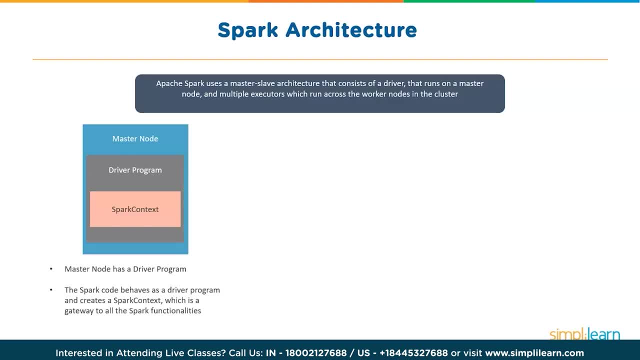 Now, that consists of a driver program that can run on a master node. It can also run on a client node, It depends on how you have configured or what your application is. And then you have multiple executors which can run on worker nodes. 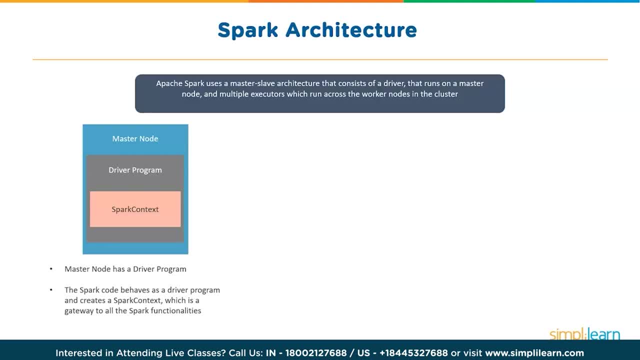 So your master node has a driver program and this driver program internally has the Spark context. So your Spark, every Spark application, will have a driver program And that driver program has a inbuilt or internally used Spark context which is basically your entry point of application for any Spark functionality. 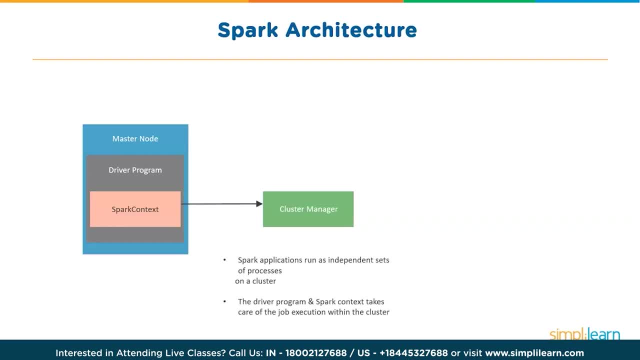 So your driver or your driver program interacts with your cluster management. Now, when I say interacts with cluster manager, so you have your Spark context, which is the entry point that takes your application request to the cluster manager. Now, as I said, your cluster manager could be, say, Apache Mesos. 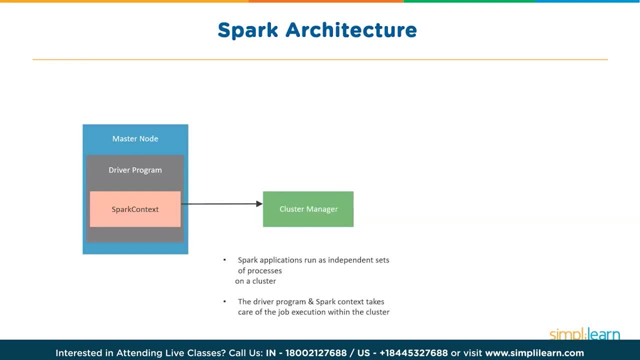 It could be Yarn, It could be Spark standalone master itself. So your cluster manager in terms of Yarn is your resource manager. So your Spark application internally runs as series or set of tasks. So your Yarn application internally runs as series or set of tasks. 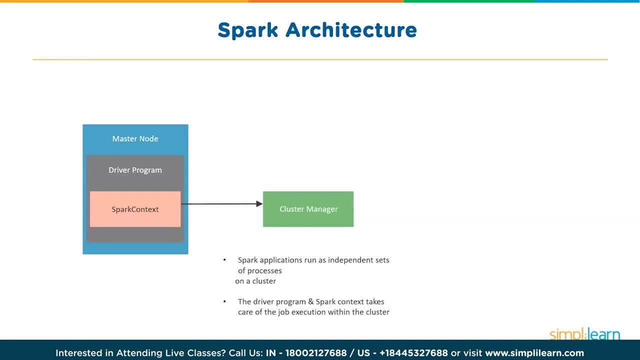 Your driver program, wherever that is run, will have a Spark context and Spark context will take care of your application execution. How does that do it? Spark context will talk to cluster manager, So your cluster manager could be Yarn And in terms of when I say cluster manager for Yarn would be resource manager. 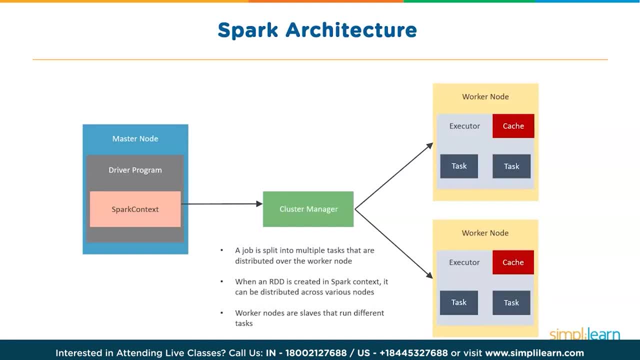 So at high level we can say: a job is split into multiple tasks And those tasks will be distributed over the Slave nodes or worker nodes. So whenever you do some kind of transformation or you use a method of Spark, context and RDD is created and this RDD is distributed across multiple nodes. 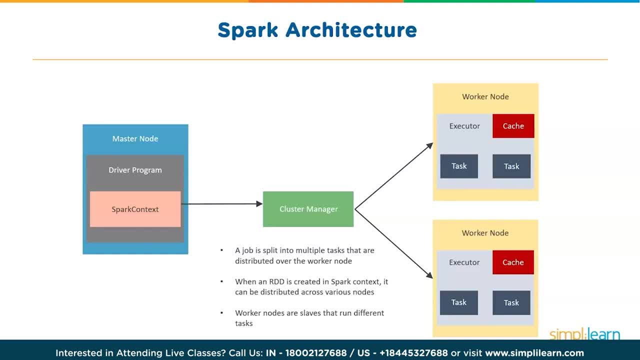 As I explained earlier, worker nodes are the slaves that run different tasks. So this is how a Spark architecture looks like. Now we can learn more about Spark architecture and its interaction with Yarn. So usually what happens when you have Spark context? So usually what happens when you have Spark context. 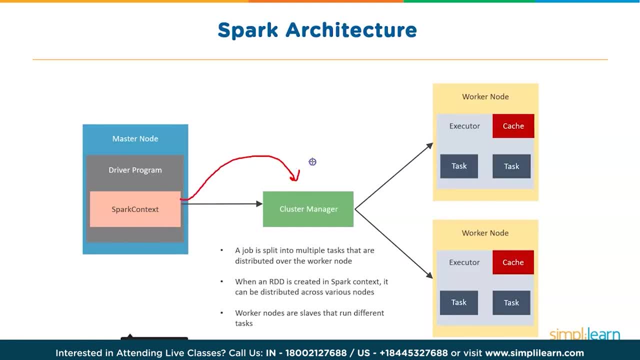 Interacts with the cluster manager. So in terms of Yarn, I could say resource manager. Now we already know about Yarn. So you would have say node managers running on multiple machines And each machine has some RAM and CPU cores allocated for your node manager. 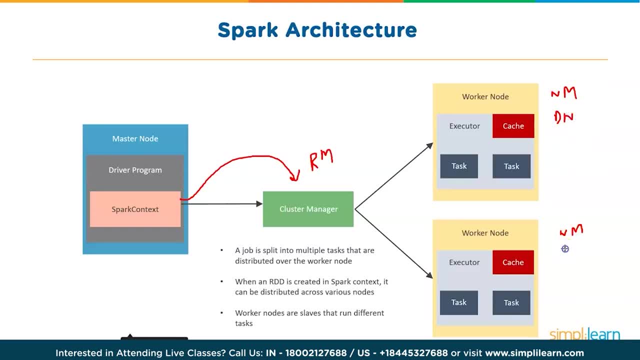 On the same machine you have the data nodes running which obviously are there to have the Hadoop related data. So whenever the application wants to process the data, your application via Spark context contacts the cluster managers, that is, the resource manager. 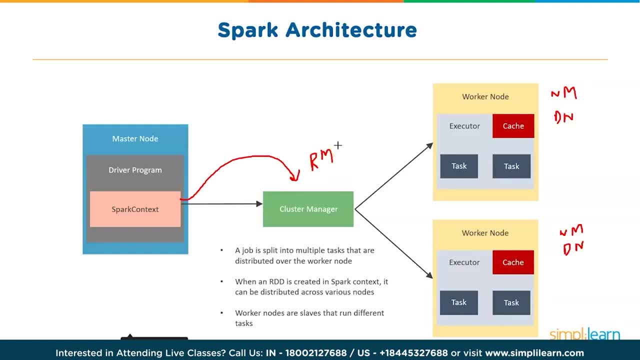 Now what does the resource manager do? Resource manager makes a request. So resource manager makes a request to the node manager of the machines wherever the relevant data resides, asking for containers. So your resource manager is negotiating or asking for containers from node manager saying: 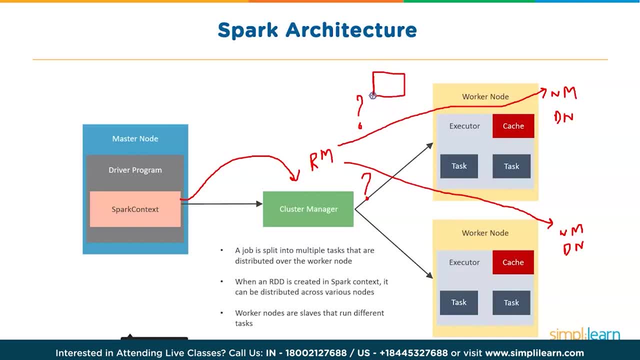 Hey, can I have a container of 1GB RAM and 1 CPU core? Can I have a container of 1GB RAM and 1 CPU core And your Node manager, based on the kind of processing it is doing, will approve or deny it? 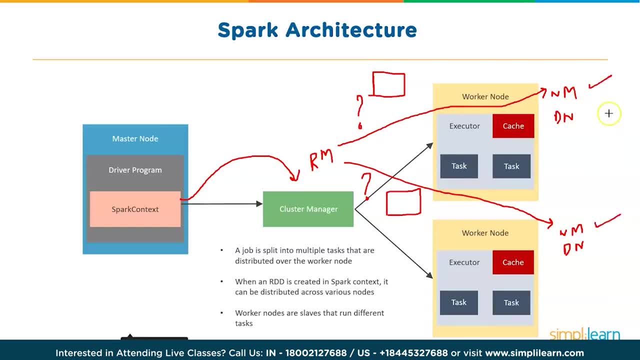 So node manager would say: fine, I can give you the container. And once this container is allocated or approved by node manager, resource manager will basically start an extra piece of code called app master. So app master is responsible for execution of your applications, whether those are Spark applications or MapReduce. 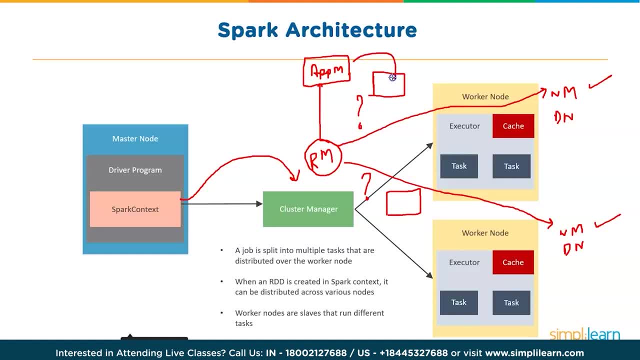 So your application master, which is a piece of code, will run in One of the containers, that is, it will use the RAM and CPU core and then it will use the other containers which were allocated by node manager to run the tasks. 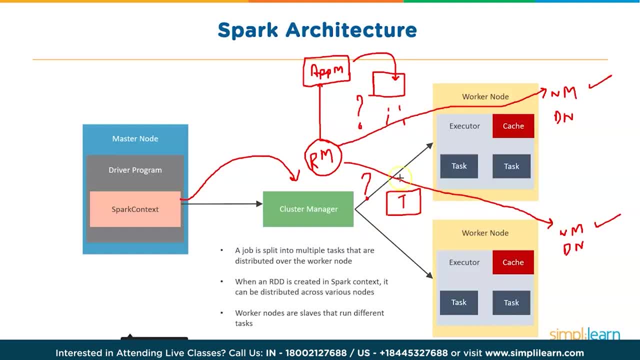 So it is within this container which can take care of execution. So what is a container? A combination of RAM and CPU core. So it is within this container. We will have a executor process which would run, and this executor process is taking care of your application related tasks. 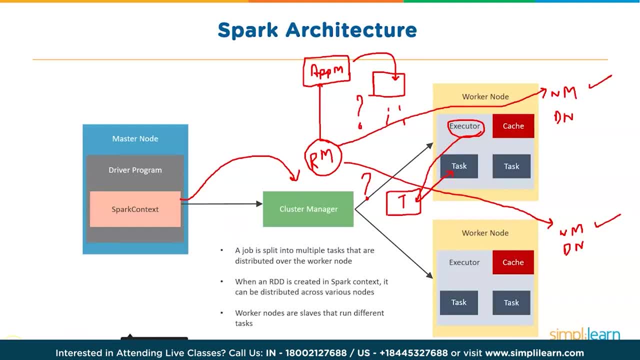 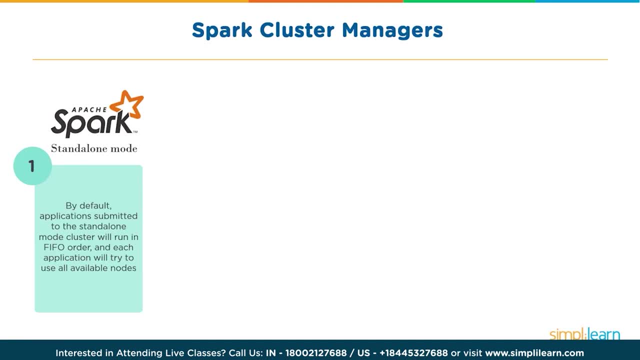 So that's how overall Spark Spark works in integration with Yarn. Now let's learn about this Spark cluster managers. As I said, Spark can work in a standalone mode, So that is without Hadoop. So, by default, application submitted to Spark standalone mode cluster will run in FIFO order and each application will try to use all the available nodes. 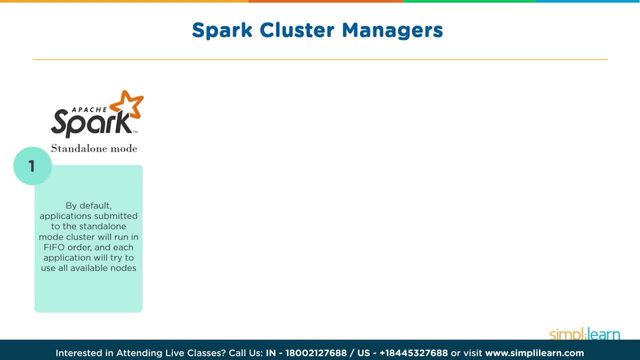 So you could have a Spark standalone cluster, which basically means you could have multiple nodes. on one of the nodes You would have the master process running And on the other nodes you would have the Spark worker processes running. So here we would not have any distributed file system, because Spark is standalone and it will rely on an external storage to get the data, or probably the file system of the nodes where the data is stored. 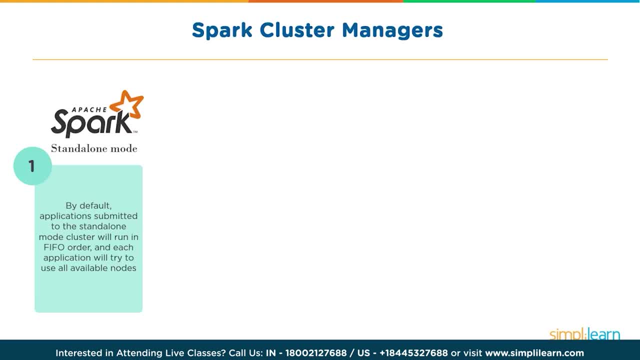 And processing will happen across the nodes where your worker processes are running. You could have Spark working with Apache Mesos. Now, as I said, Apache Mesos is an open source project to manage your components, So you could have Spark working with Apache Mesos and you could also run Hadoop applications. 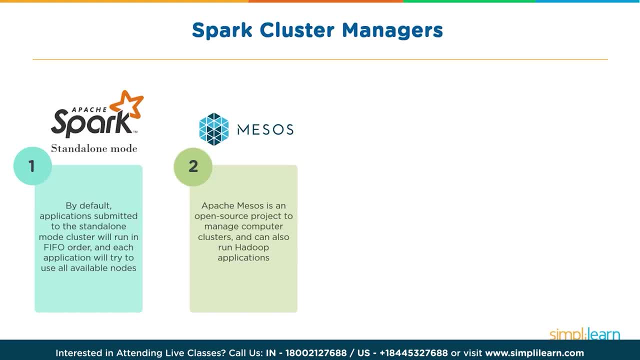 Apache Mesos was introduced earlier and Spark came in and has existence. to prove the credibility of Apache Mesos, You can have Spark working with Hadoop's Yarn. This is something which widely you will see in different working environments. So Yarn, which takes care of your processing and can take care of different processing frameworks, also supports Spark. 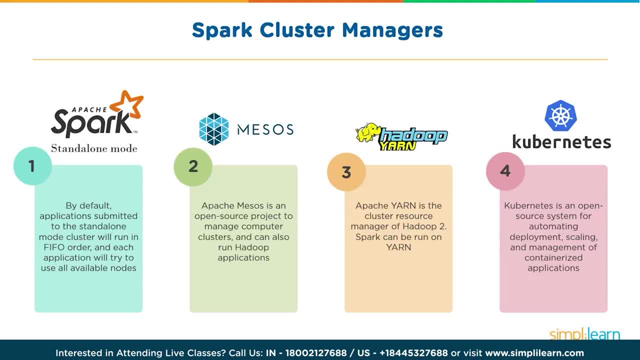 You could have Kubernetes. Now that is something which is making a lot of news in today's world. It is an open source system for automating deployment, scaling and management of containerized applications, So where you could have multiple Docker-based images which can be connecting to each other. 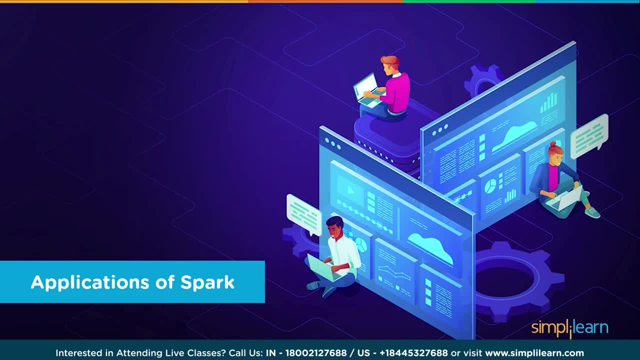 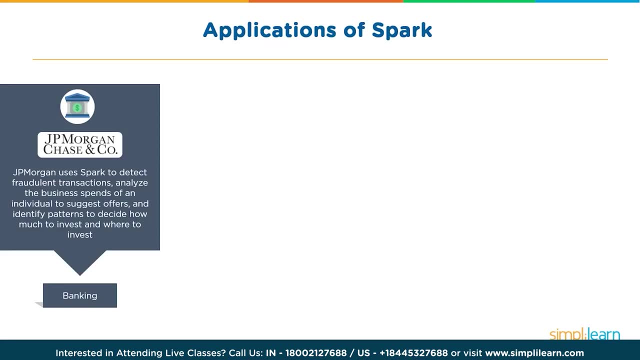 So Spark also works with Kubernetes. Now let's look at some applications of Spark. So JPMorgan Chase and company uses Spark to detect fraudulent transactions, analyze the business spendings and identify patterns of an individual, to suggest offers and identify patterns to decide how much to invest and where to invest. 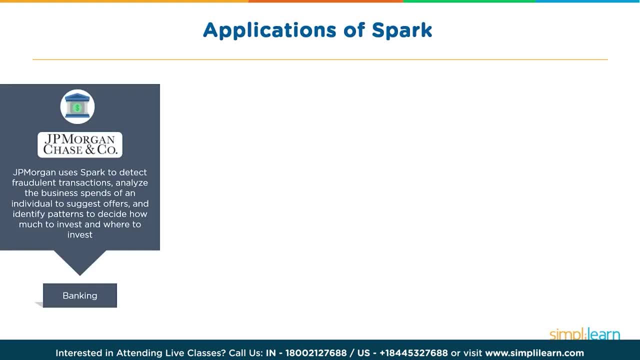 So this is one of the examples of banking. A lot of banking environments are using Spark due to its real-time processing capabilities and in-memory faster processing where they could be working on fraud detection or credit analysis or pattern identification and many other use cases. 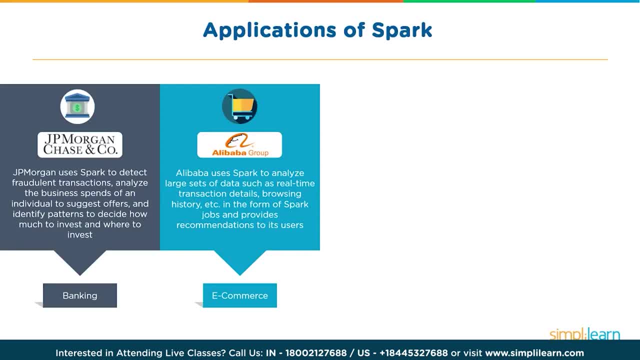 Alibaba Group that uses also Spark To analyze large data sets of data, such as real-time transaction details, Now that might be based online or in the stores, looking at the browsing history in the form of Spark jobs, and then provides recommendations to its users. 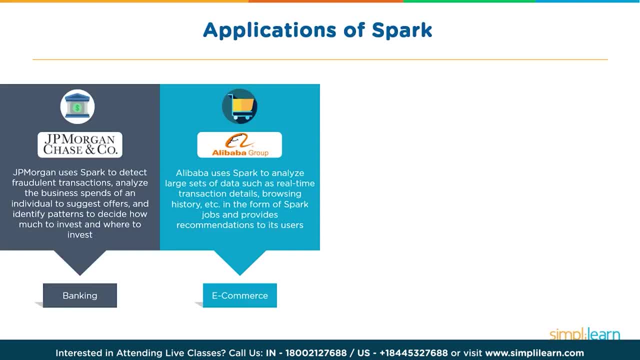 So Alibaba Group is using Spark in its e-commerce domain. You have IQVIA Now. this is a leading health care company that uses Spark to analyze patients' data, identify possible health issues and diagnose it based on their medical history. So there is a lot of work happening in the health care industry, where real-time processing is finding a lot of importance. 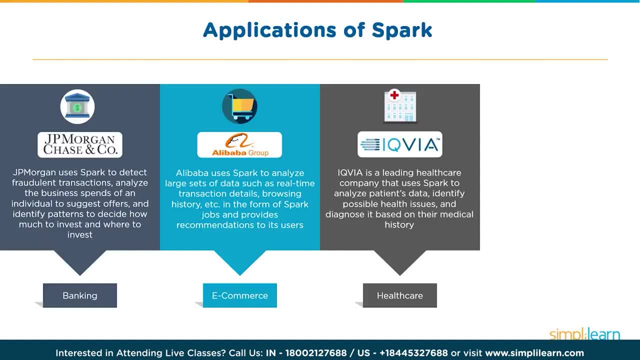 And real-time and faster processing is what is required. So the health care industry and IQVIA is also using Spark. You have Netflix, which is known, and you have Riot Games. So entertainment and gaming companies like Netflix and Riot Games use Apache Spark to showcase relevant advertisements to their 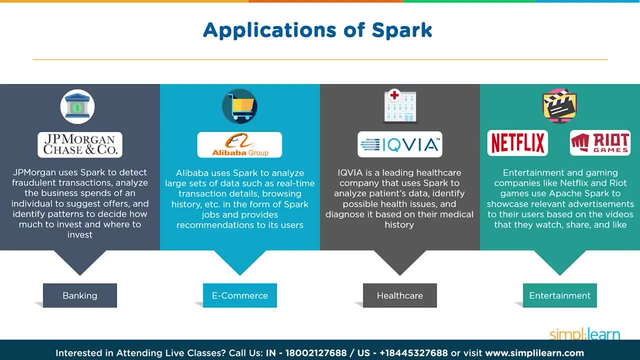 users based on the videos that they have watched, shared or liked. So these are a few domains which find use cases of Spark. that is, banking, e-commerce, health care, entertainment, And then there are many more which are using Spark in their day-to-day activities for real-time in-memory, faster processing. 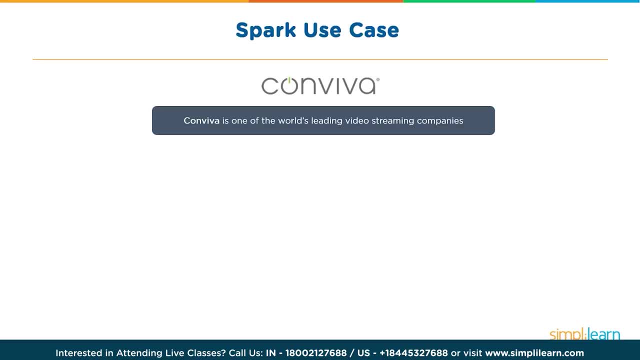 Now let's discuss about Spark's use case, and let's talk about Conviva, which is world's leading video streaming companies. So video streaming is a challenge. Now, if you talk about YouTube, which has data, you could always read about it. 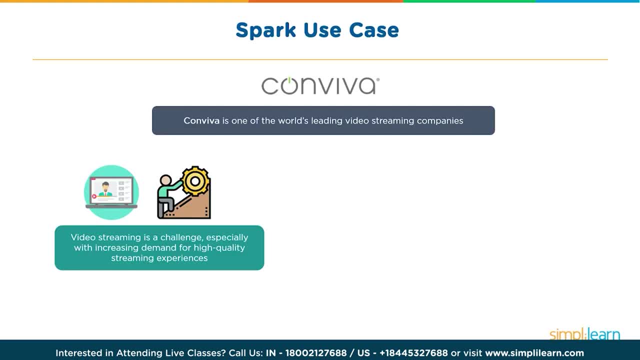 So YouTube has data which is worth watching 10 years. So that is a huge amount of data where people are uploading their videos or companies are doing advertisements, And these videos are streamed in or can be watched by users. So video streaming is a challenge, and especially with increasing demand for high-quality streaming experience. 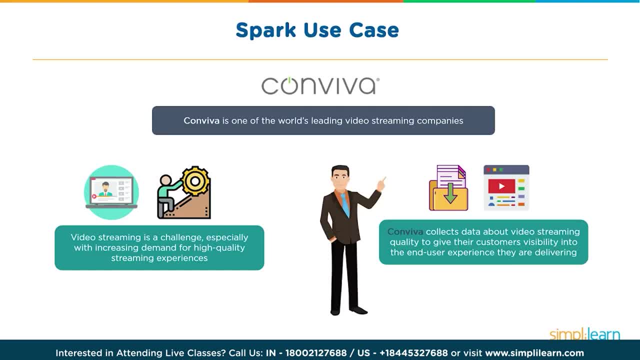 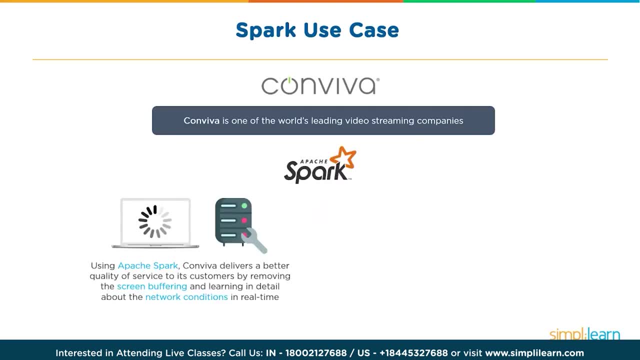 Conviva collects data about video streaming quality to give their customers visibility into the end user experience they are delivering. Now how do they do it? Apache Spark again. Using Apache Spark, Conviva delivers a better quality of service to its customers by removing the screen buffering and learning in detail about network conditions in real time. 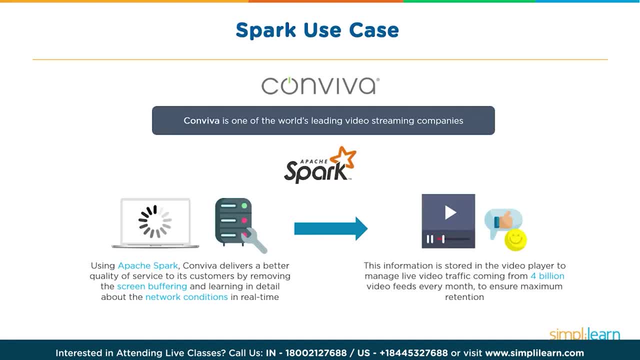 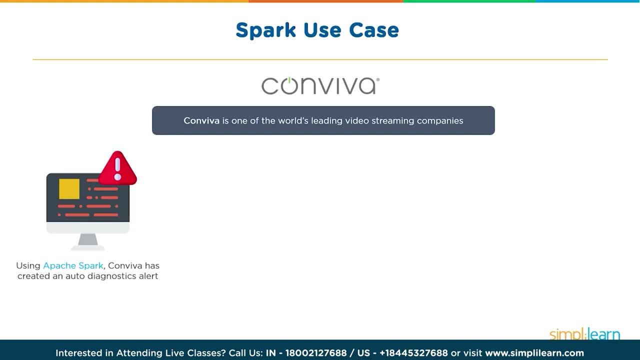 This information is then stored in the video player to manage live video traffic coming in from 4 billion video feeds every month to ensure maximum retention. Now, using Apache, Spark Conviva has created an auto-diagnostics alert. It automatically detects anomalies along the video streaming pipeline and diagnoses the root cause of the issue. 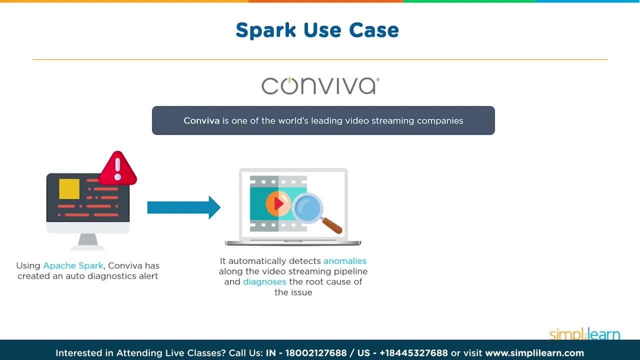 Now this really makes it one of the leading video streaming platforms. It reduces waiting time before the video starts, it avoids buffering and recovers the video from a technical error, and the whole goal is to maximize the viewer engagement. So this is Spark's use case, where Conviva is using Spark in different ways to stay ahead in video streaming related deliveries. 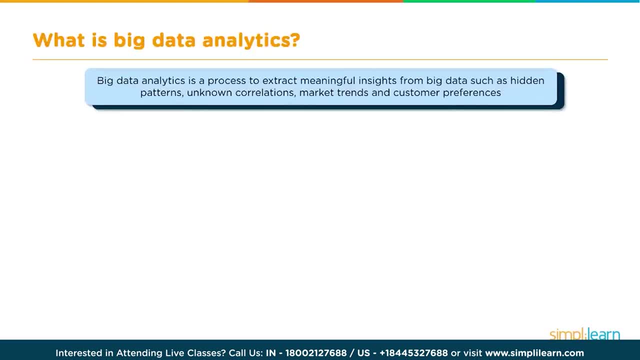 What is Big Data Analytics? In simple terms, Big Data Analytics is defined as the process which is used to extract meaningful information from big data. This information could be your hidden patterns, unknown correlations, market trends and so on. By using Big Data Analytics, there are many advantages. 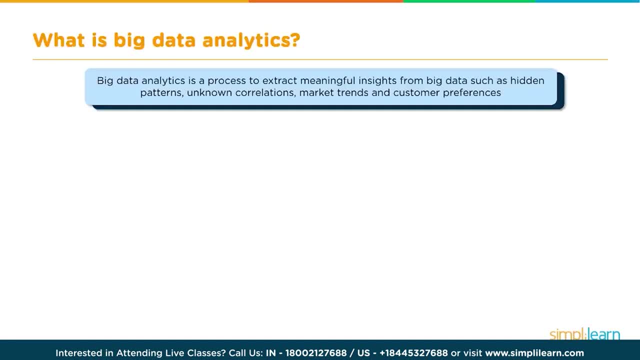 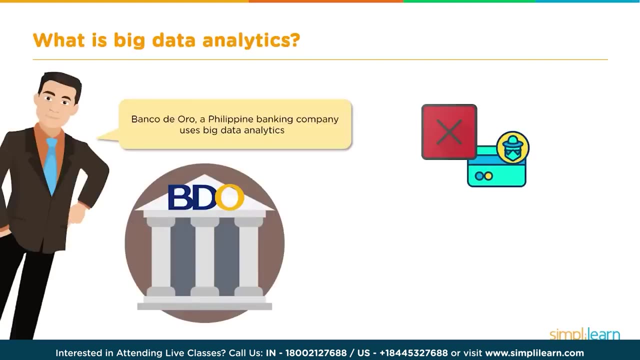 It can be used for better decision making, to prevent fraudulent activities, and many others. We will look into four of them step by step. I will first start off with Big Data Analytics, which is used for risk management. BDO, which is a Philippine banking company, uses Big Data Analytics for risk management. 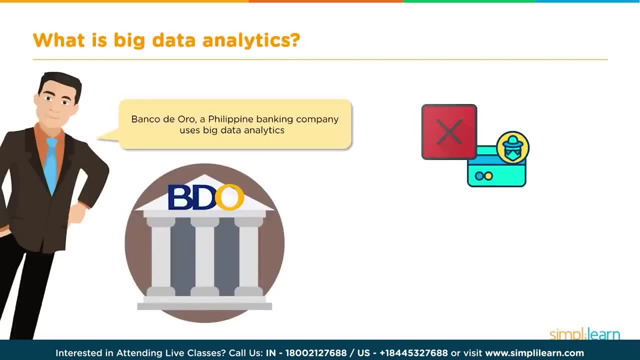 Risk management is an important aspect for any organization, especially in the field of banking. Risk management analysis comprises a series of measures which are employed to prevent any sort of unauthorized activities. Identifying fraudulent activities was a main concern for BDO. It was difficult for the bank to identify the fraudster from a long list of activities. 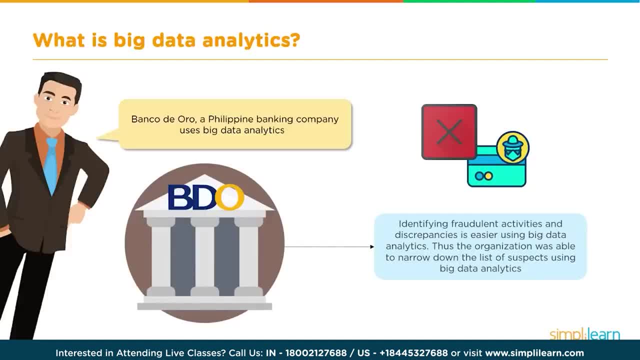 It was difficult for the bank to identify the fraudster from a long list of activities. It was difficult for BDO to identify the fraudster from a long list of activities. BDO adopted Big Data analytics, which helped the bank to narrow down the entire list of suspects. 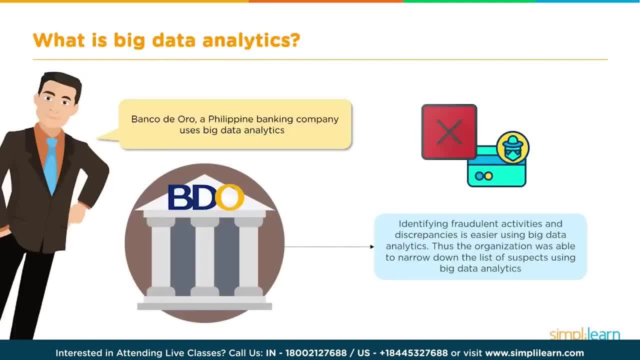 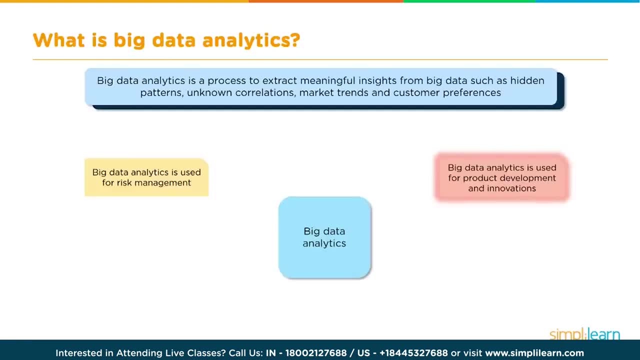 Thus, the organization was able to identify the fraudster in a very short time. This is how Big Data Analytics is used in the field of banking for risk management. Let us now see how Big Data Analytics is used for product development and innovations, with an example. 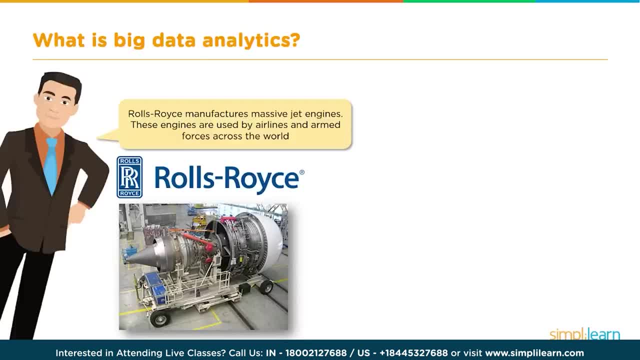 All of you are aware of Rolls Royce cars, right? Do you also know that the manufacturer Jetension was the company who produced the pies company? A Perkins manufactured jet engines, which are used across the world. What is more interesting is that they use big data analytics for 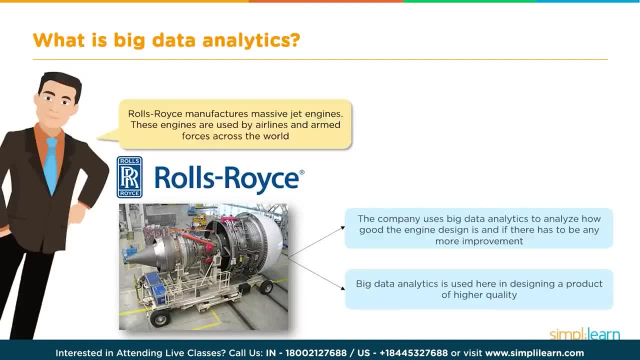 developing and innovating this engine. A new product is always developed by trial and error method. Big data analytics is used here to analyze if an engine design is good or bad. It is also used to analyze if there can be more scope for improvement based on the previous models and on the future demands. This way, big data analytics is used in designing a. 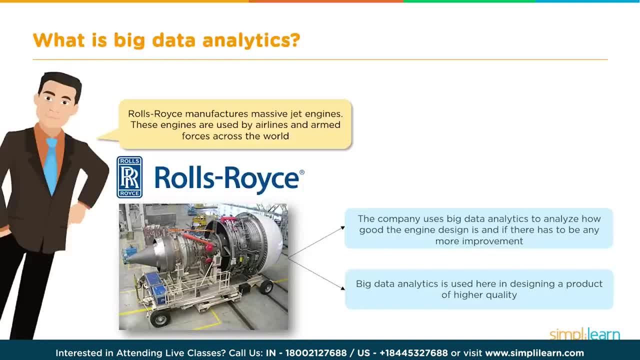 product which is of higher quality. Using big data analytics, the company can save a lot of time If the team is struggling to arrive at the right conclusion. big data can be used to zero in on the right data which have to be studied, and thus the time spent on the product. 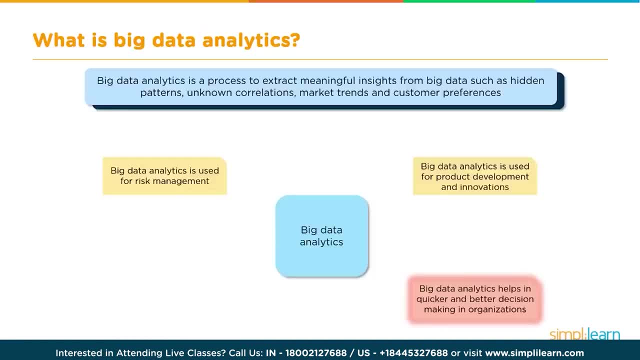 development is less. Big data analytics helps in quicker and better decision making in organizations. The process of selecting a course of action from various other alternatives is known as decision making. Lot of organizations take important decisions based on the data that they have: Data driven business. 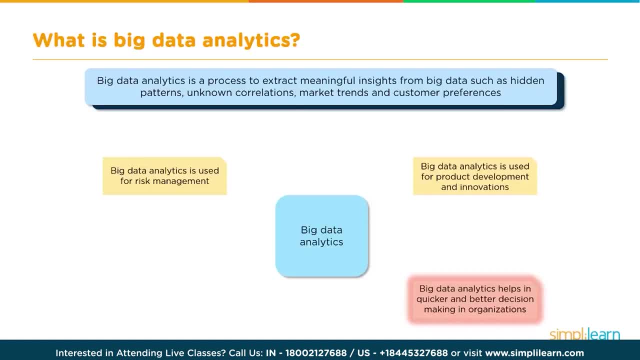 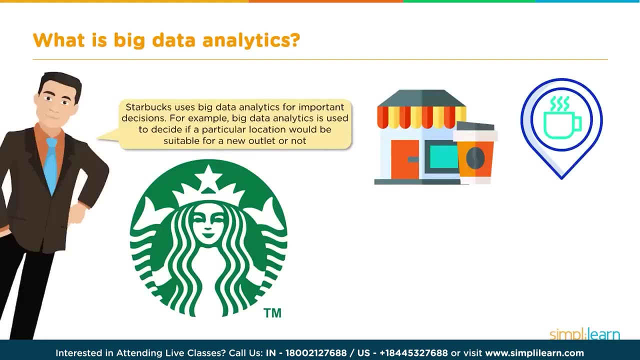 decisions can make or break a company. Hence it is important to analyze all the possibilities thoroughly and quickly before making important decisions. Let us now try to understand this with an use case. Starbucks uses big data analytics for making important decisions. They decide the location of their new outlet using big data analytics. 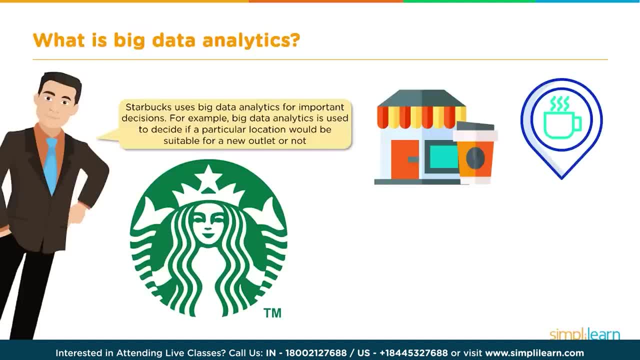 Choosing the right location is an important factor for any organization. The wrong location will not be able to attract the required amount of customers. Positioning of a new outlet a few miles here or there can always make a huge difference for an outlet, especially a one like Starbucks. Various factors are involved in choosing the 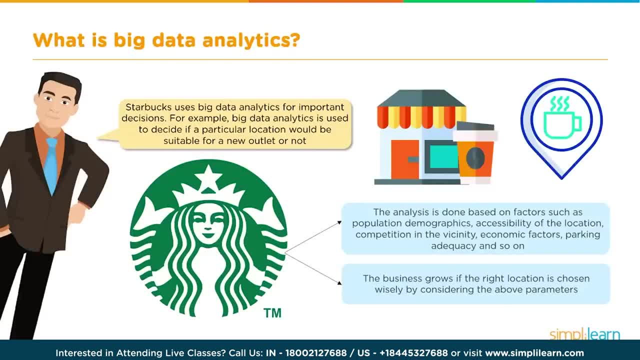 right location for a new outlet. For example, parking adequacy has to be taken into consideration. It would be inconvenient for people to go to a store which has no parking facility. Similarly, the other factors that have to be considered are the visibility of the location, the accessibility, the economic factors. 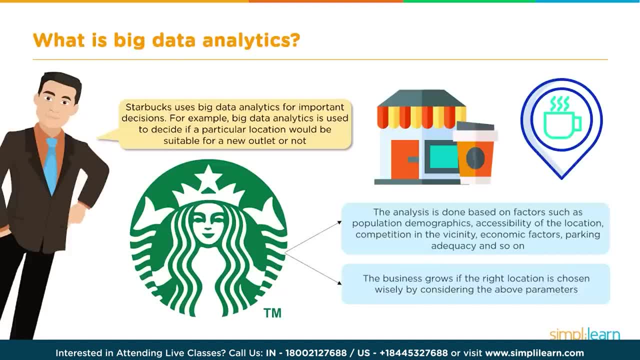 the population of that particular location, and also we would have to look into the competition in the vicinity. All these factors have to be thoroughly analyzed before making a decision As to where the new outlet must be started. without analyzing these factors, It would be impossible for us to make a wise decision using big data analytics. 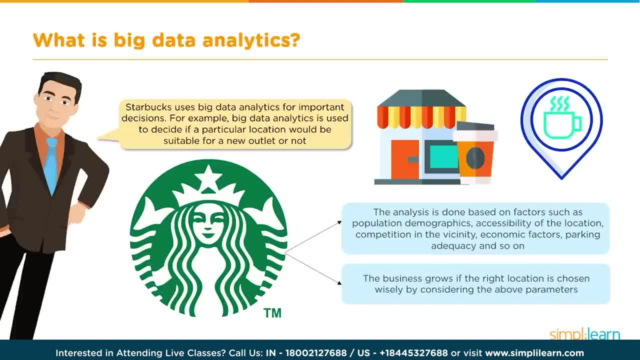 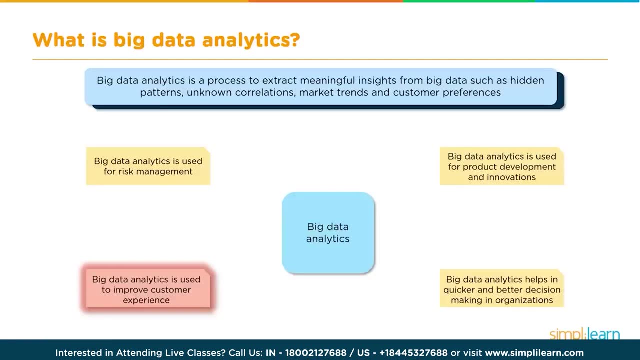 We can consider all these factors and analyze them quickly and thoroughly. Thus, Starbucks makes use of big data analytics to understand if their new location would be fruitful or not. Finally, we will look into how big data analytics is used to improve customer experience, using an example: Delta. 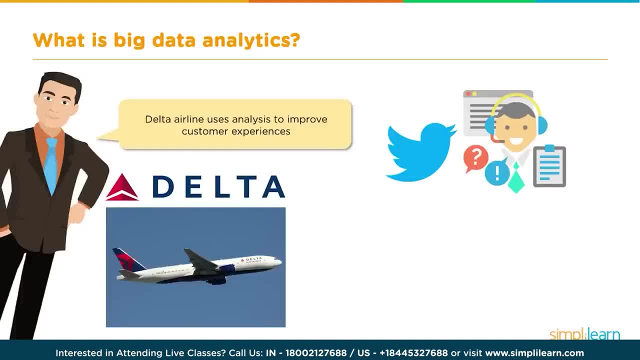 An American airline uses big data analytics to improve its customer experiences. With the increase in global air travel, It is necessary that an airline does everything they can in order to provide good service and experience to its customers. Delta Airlines improves its customer experience by making use of big data analytics. 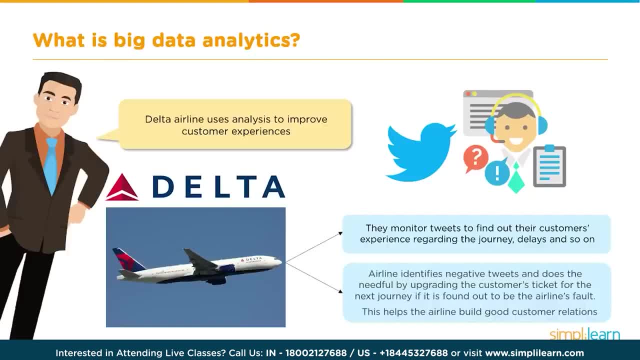 This is done by monitoring tweets, Which will give them an idea as to how their customers journey was. if the airline comes across a negative Tweet, and if it is found to be the airline's fault, the airline goes ahead and upgrades that particular customer's ticket. when this happens, the customer is able to trust the airlines and 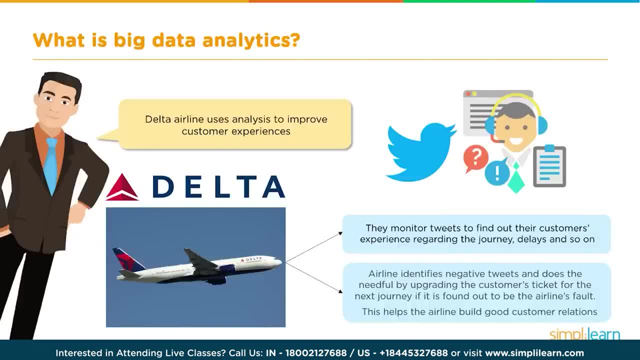 Without a doubt, the customer will choose Delta for their next journey. by doing so, the customer is happy and the airlines will be Able to build a good brand recognition. thus We see here that, by using analysis, Delta Airlines was able to improve its customer experience. Moving on to our next topic, that is, life cycle of big data analytics here, 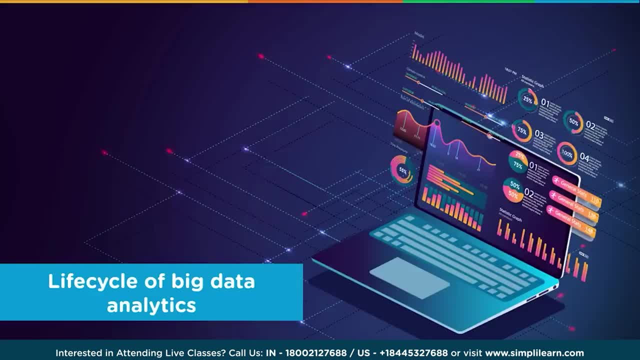 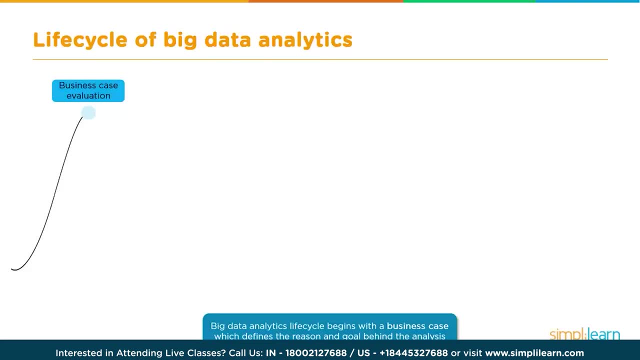 We will look into the various stages as to how data is analyzed from scratch. The first stage is the business case evaluation stage. here the motive behind the analysis is identified. We need to understand why we are analyzing so that we know how to do it and what are the different parameters that have to be looked into. once this is done, it. 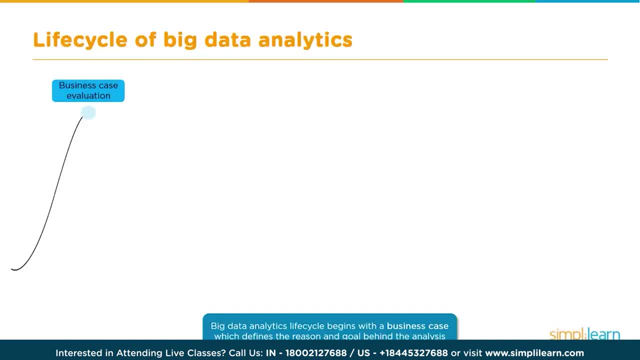 Is clear for us and it Makes much easier for us to proceed with the rest, after which we will look into the Various data sources from where we can gather all the data Which will be required for analysis. once we get the required Data, we will have to see if the data that we received is fit for. 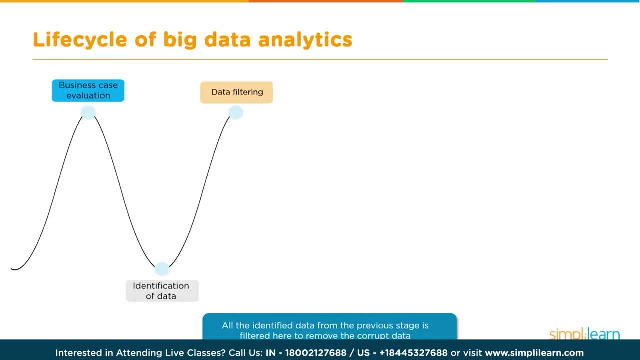 Analysis or not, not, all the data that we receive will have Meaningful information. some of it will surely just be corrupt data. to remove this corrupt data, We will Power off the Nej seni product for further maintenance. Thank you, http//www. смысล-porрifgin. a hundred thousand dollars from techeuropecomau. 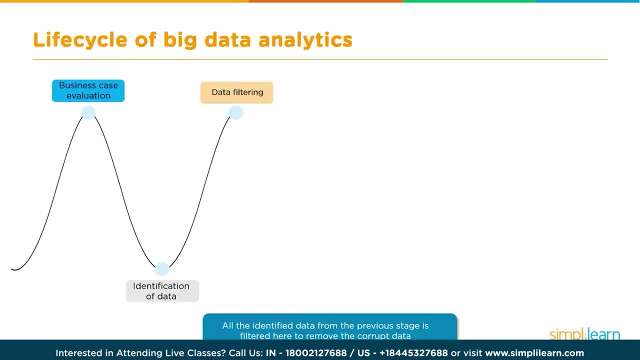 pass this entire data through a filtering stage. In this stage, all the corrupt data will be removed. Now we have the data minus the corrupt data. Do you think our data is now fit for analysis? Well, it is not. We still have to figure out. 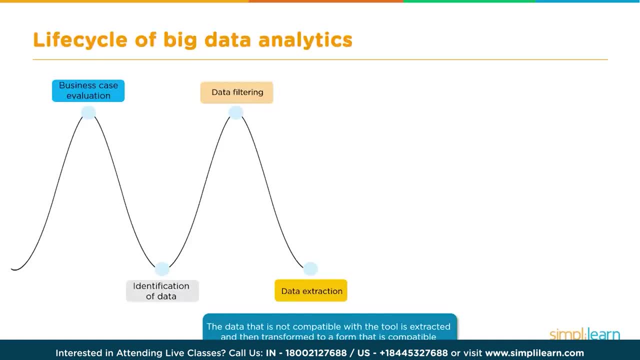 which data will be compatible with the tool that we will be using for analysis. If we find data which is incompatible, we first extract it and then transform it to a compatible form, depending on the tool that we use. In the next stage, all the data with the same fields will be integrated. 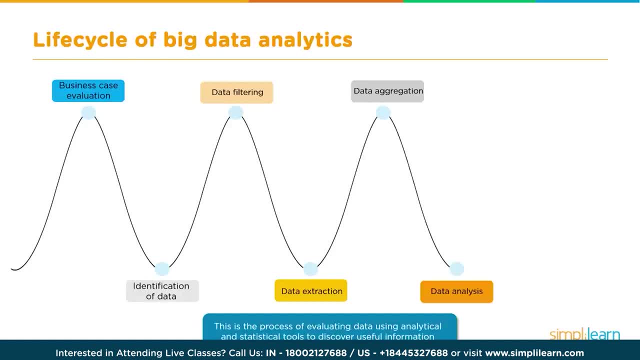 This is known as the data aggregation stage. The next stage, which is the analysis stage, is a very important stage in the lifecycle of Big Data Analytics. Right here in this step, the entire process of evaluating your data using various analytical and statistical tools to discover meaningful information. 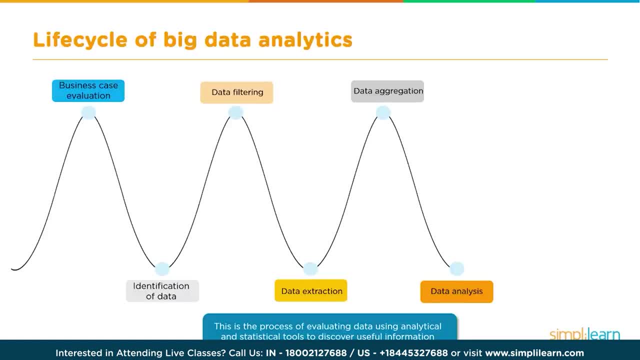 it is done Like we have discussed before. the entire process of deriving meaningful information from data, which is known as analysis, is done here in this stage. The result of the data analysis stage is then graphically communicated using tools like Tableau, Power BI, Clickview. 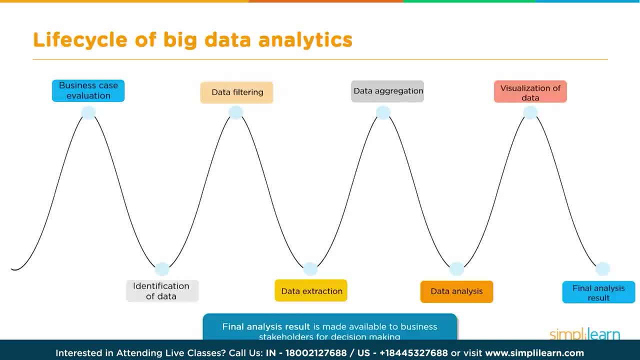 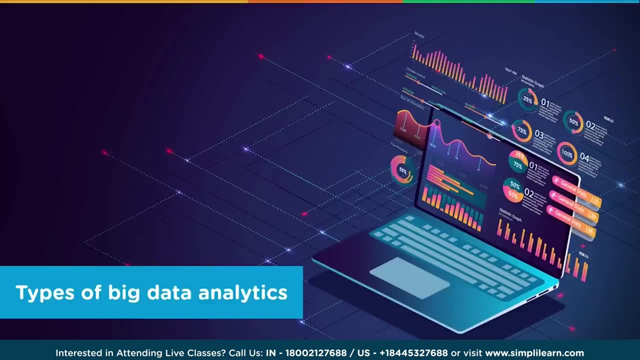 This analysis result will then be made available to different business stakeholders for various decision making. This was the entire lifecycle of big data analytics. We just saw how data is analyzed from scratch. Now we will move on to a very important topic, that is, the 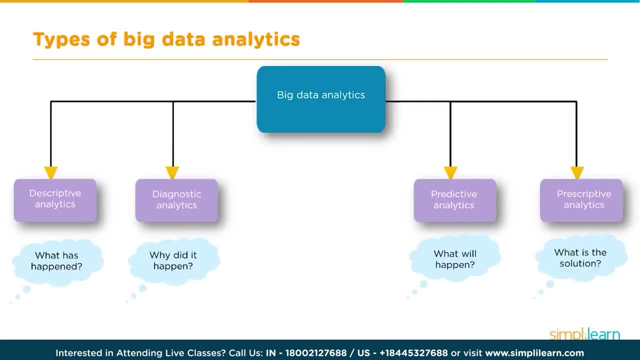 different types of big data analytics. Well, we have four different types of big data analytics, As you see. here these are the types and below this are the questions that each type tries to answer. We have descriptive analytics, which asks the question: what has happened? The 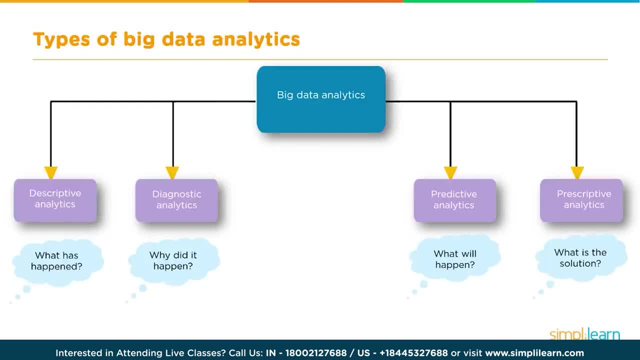 first type is diagnostic analytics, which asks: why did it happen, predictive analytics, asking what will happen, and prescriptive analytics, which questions by asking what is the solution. We will look into all these four one by one, with an use case for each. We will first start. 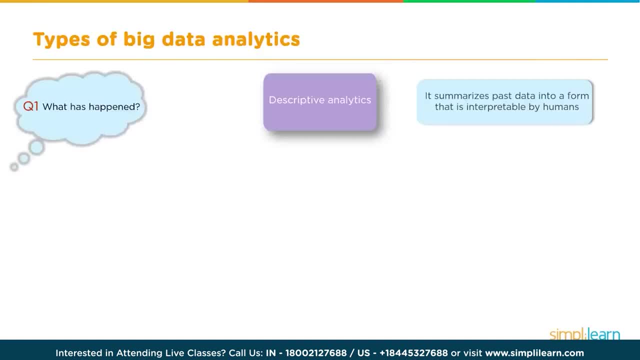 off with descriptive analytics. As mentioned earlier, descriptive analytics asks the question: what has happened? It can be defined as the type that summarizes past data into a form that can be understood by humans. In this type, we will look into the past data and 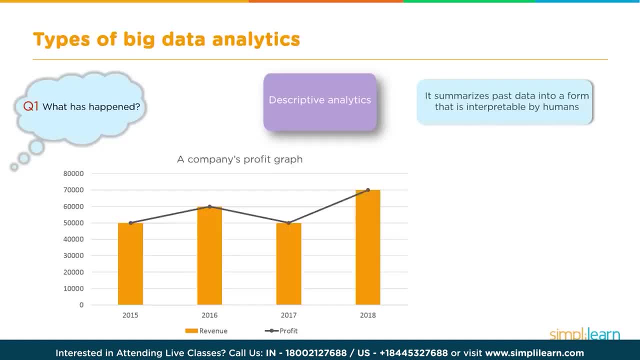 arrive at various conclusions. For example, an organization can review its performance using descriptive analytics, That is, it analyzes its past data, such as revenue over the years, and arrives at a conclusion with the profit. By looking at this graph, we can understand if the company is running at a profit or not. Thus, descriptive analytics helps us understand. 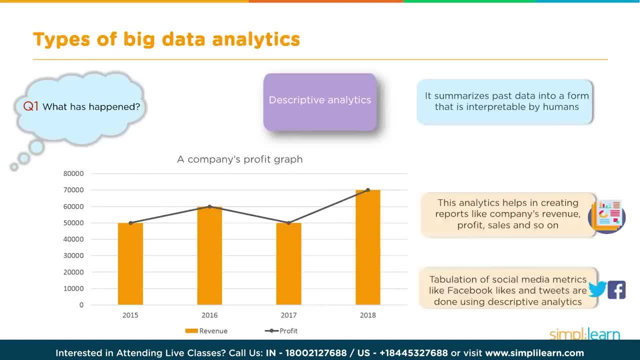 this easily. We can simply say that descriptive analytics is used for creating various reports for companies and also for tabulating various social media metrics like Facebook likes, tweets, etc. Now that we have seen what is descriptive analytics, let us look into an use case of descriptive analytics. The Dow Chemical company analyzed all its past data. 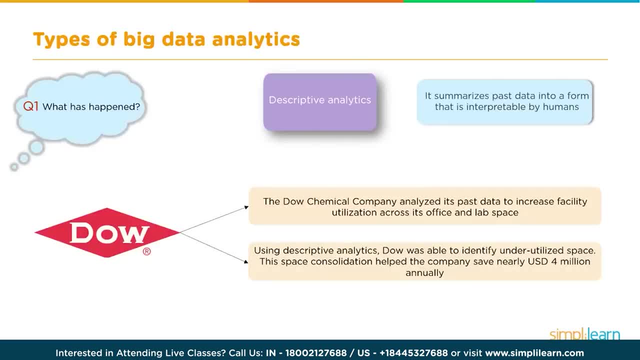 using descriptive analytics, and by doing so, they were able to identify the underused utilize space in their facility. Descriptive analytics help them in this space consolidation. On the whole, the company was able to save nearly $4 million annually. So we now see here that 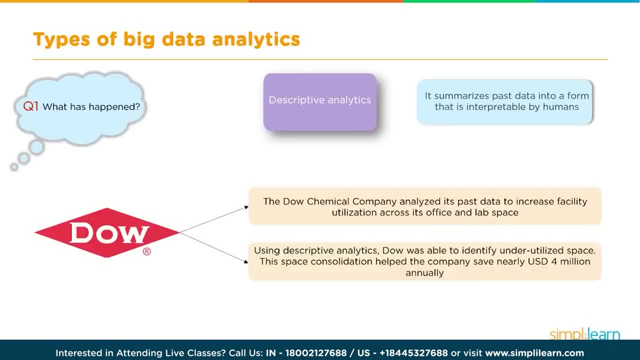 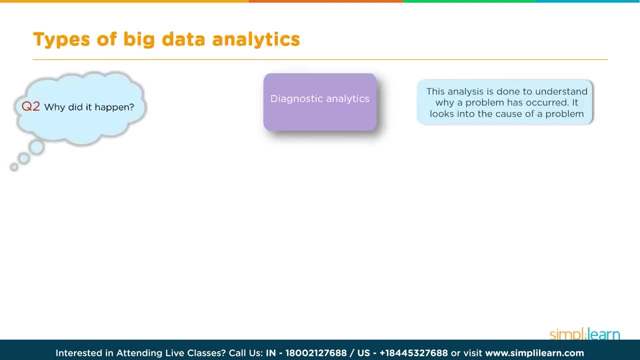 descriptive analytics not only helps us derive meaningful information from the past data, but it can also help companies in cost reduction if it is used wisely. Let us now move on to our next type, that is, diagnostic analytics. Diagnostic analytics asks the question why a particular problem has. 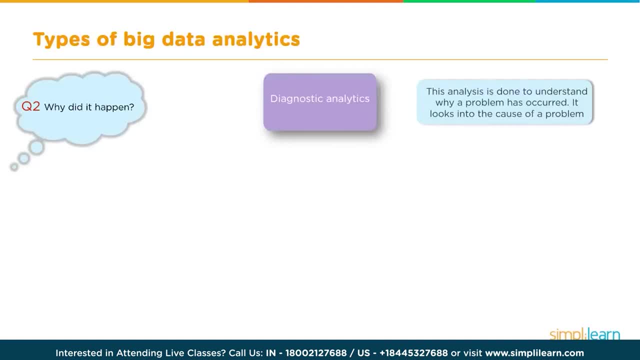 occurred. As you can see, it will always ask the question: why did it happen? It will look into the root cause of a problem and try to understand why it has occurred. Diagnostic analytics makes use of various techniques such as data mining, data discovery and drill down. Companies benefit from. 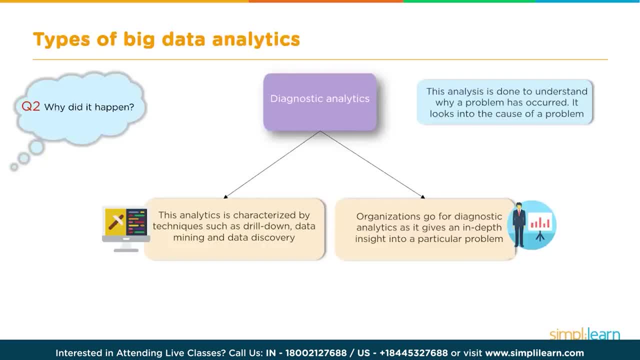 this type of analytics because it helps them look into the root cause of a problem. By doing so, they can understand why a particular problem has occurred. Diagnostic analytics makes use of various techniques, such as data mining, data discovery and drill down. Companies benefit from. 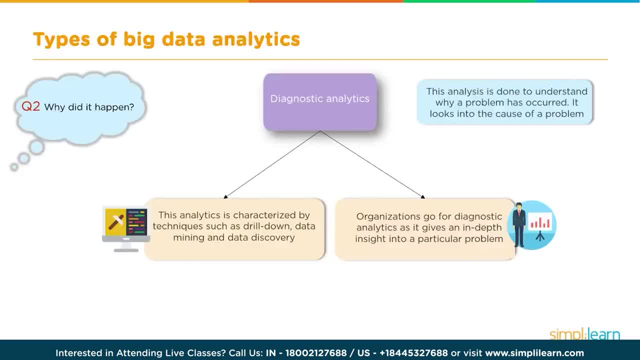 this type of analytics because it helps them look into the root cause of a problem. By doing so, the next time the same problem will not arise, as the company already knows why it has happened and they will arrive at a particular solution for it. iNetsoft's BI query tool is an example of. 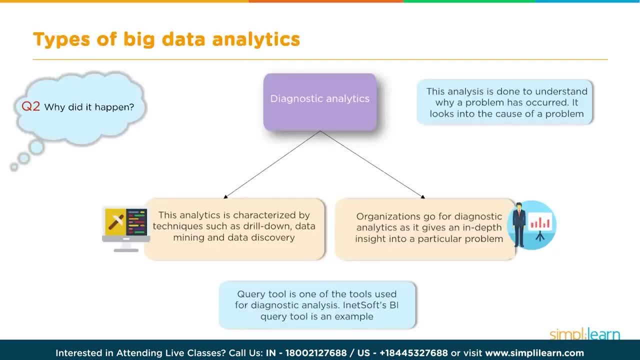 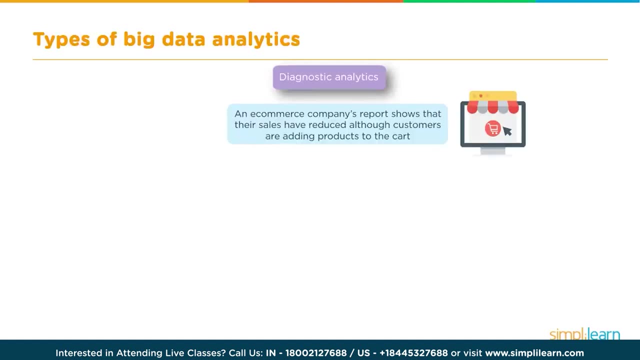 diagnostic analytics. We can use the query tool for diagnostic analytics. Now that you know why diagnostic analytics is required and what diagnostic analytics is, I will run you through an example which shows where diagnostic analytics can be used. All of us shop on e-commerce sites. 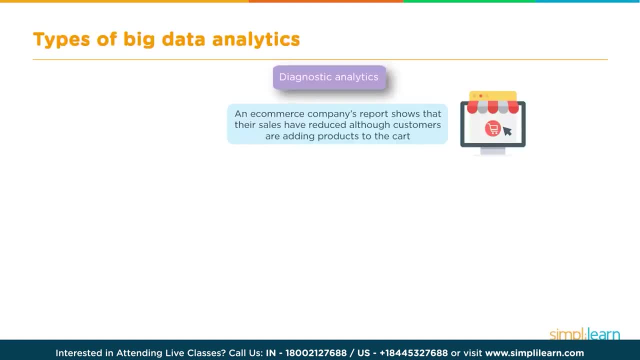 sites right. Have you ever added items to your cart but ended up not buying it? Yes, all of us might have done that at some point. An organization tries to understand why its customers don't end up buying their products, although it has been added to their carts. 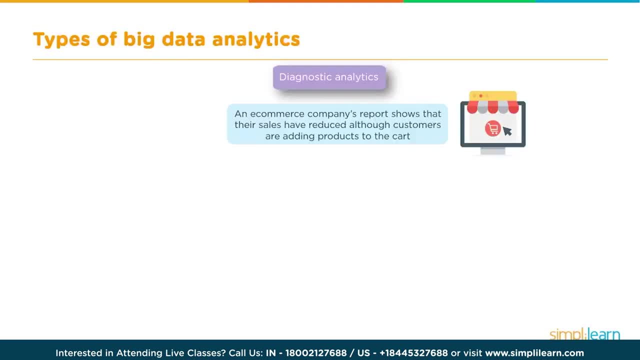 And this understanding is done with the help of diagnostic analytics. An e-commerce site wonders why they have made few online sales, although they have had a very good marketing strategy. There could have been various factors as to why this has happened, Factors like the shipping fee, which was too high, or the page that didn't load correctly, not enough. 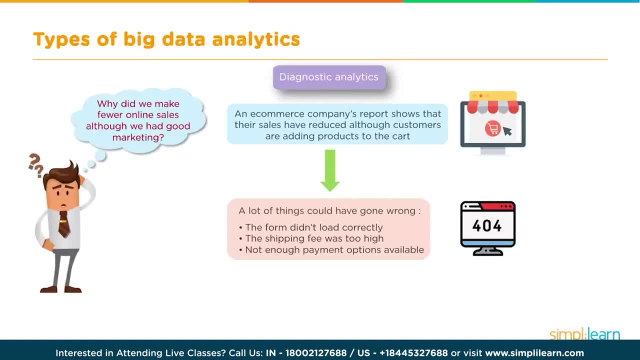 payment options available, and so on. All these factors are analyzed using diagnostic analytics and the company comes to a conclusion as to why this has happened. Thus, we see here that the root cause is identified, so that in future the same problem doesn't occur again. Let. 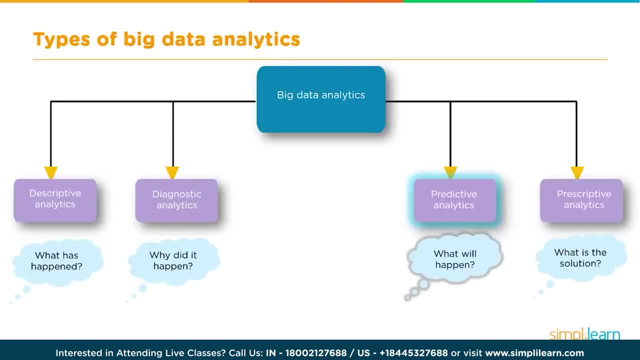 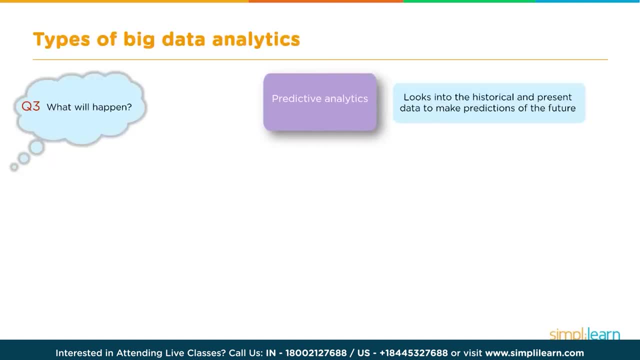 us now move on to the third type, ie Predictability. Predictive Analytics. As the name suggests, predictive analytics makes predictions of the future. It analyzes the current and historical facts to make predictions about future. It always asks the question: what will happen next? Predictive analytics. 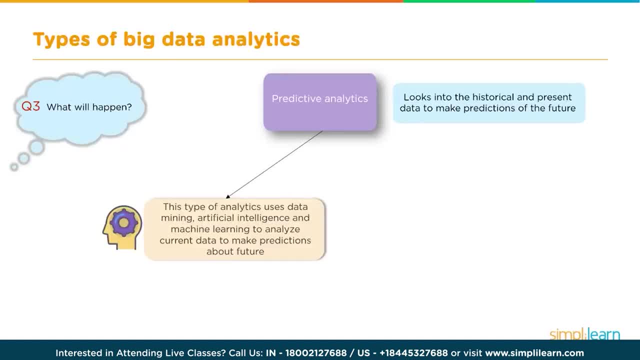 is used with the help of artificial intelligence, machine learning, data mining, to analyze the data. It can be used for predicting customer trends, market trends, customer behavior, etc. It solely works on probability. It always tries to understand what can happen next with the help of all the past and current. 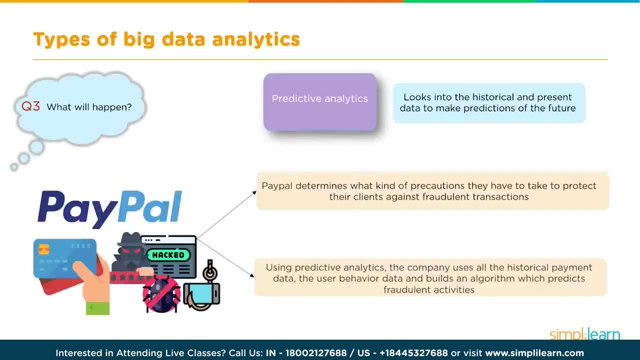 information. A company like PayPal, which has 260 plus million accounts, always has the need to ensure that their online fraudulent and unauthorized activities are brought down to nil. Fear of constant fraudulent activities have always been a major concern for PayPal. When a fraudulent activity occurs, people lose trust in the company, And this brings 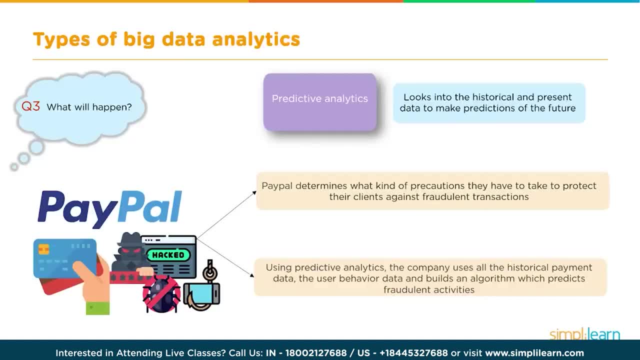 in a very bad name for the brand. It is inevitable that fraudulent activities will happen in a company like PayPal, which is one of the largest online payment processors in the world. But PayPal uses analytics wisely here to prevent such fraudulent activities and to minimize them. It uses predictive analytics. 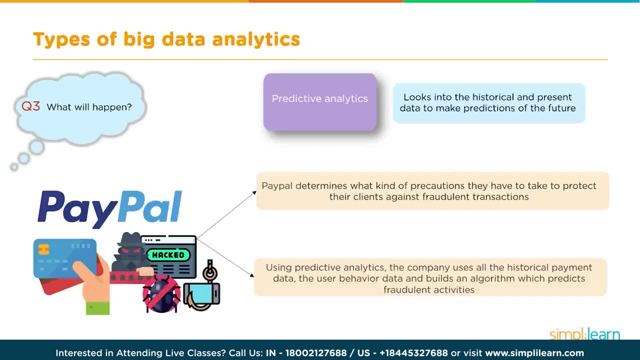 to do so. The organization is able to analyze past data, which includes a customer's historical payment data, a customer's behavior trends, etc. The organization is able to analyze past data, which includes a customer's historical payment data, a customer's behavior trends, etc. 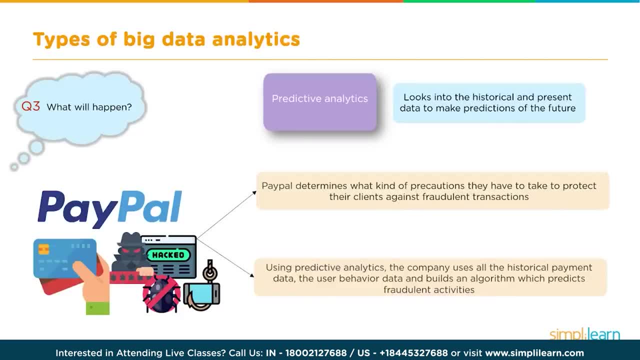 And then it builds an algorithm which works on predicting what is likely to happen next with respect to their transaction. With the use of big data and algorithms, the system can gauge which of the transactions are valid and which could be potentially a fraudulent activity. By doing so, PayPal is always ready with precautions that they have to take to protect all their 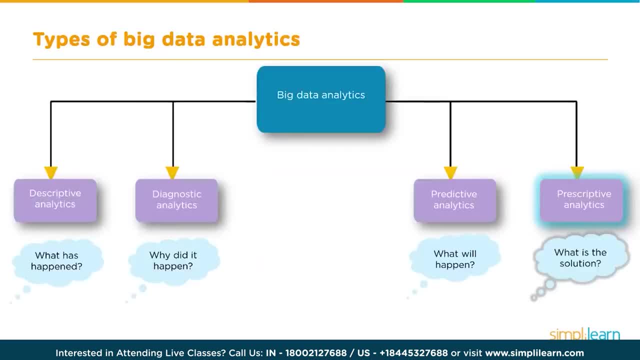 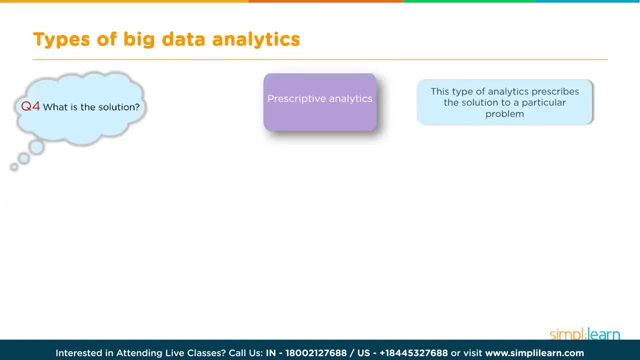 clients against fraudulent transactions. We will now move on to our last type, ie Prescriptive Analytics. Prescriptive analytics, as the name suggests, always prescribes a solution to a particular problem. The problem can be something which is happening currently. Hence it can be termed as the type that always asks the question: what is the solution? 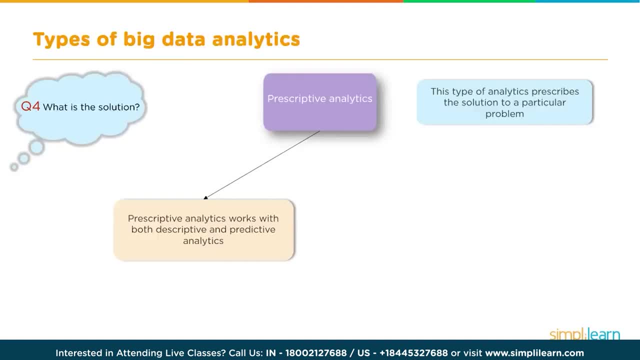 Prescriptive analytics is related to both predictive and descriptive analytics, As we saw earlier. descriptive analytics always asks the question: what has happened? and predictive analytics helps you understand the problem: what can happen next With the help of artificial intelligence and machine learning. prescriptive: 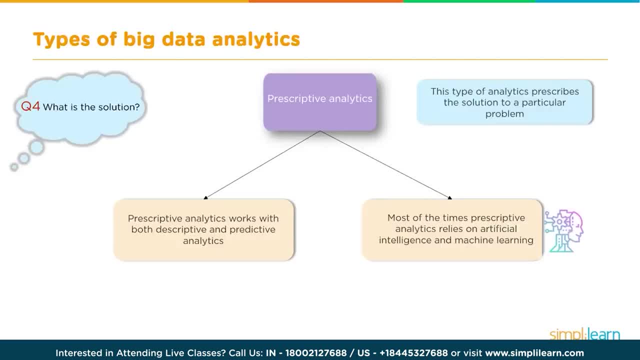 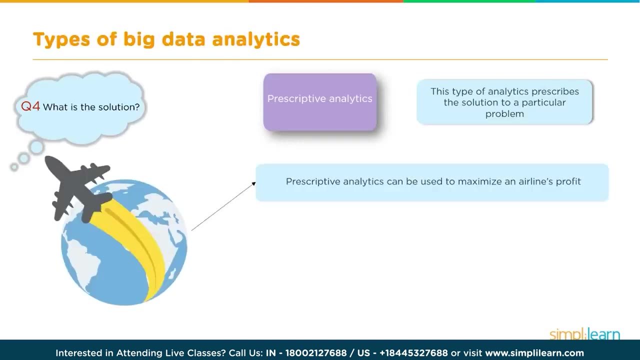 analytics helps you arrive at the best solution for a particular problem. Various business rules, algorithms and computational modeling procedures are used in prescriptive analytics. Let us now have a look at how and where prescriptive analytics is used. with an example Here we will understand how prescriptive analytics is used by an airline for its profit. Do you know? that when you book a flight ticket, the price of it depends on various factors, both internal and external factors. Apart from taxes, seat selection, there are other factors like oil prices, customer demand, which are all taken into consideration before the flight fare is displayed Prices. 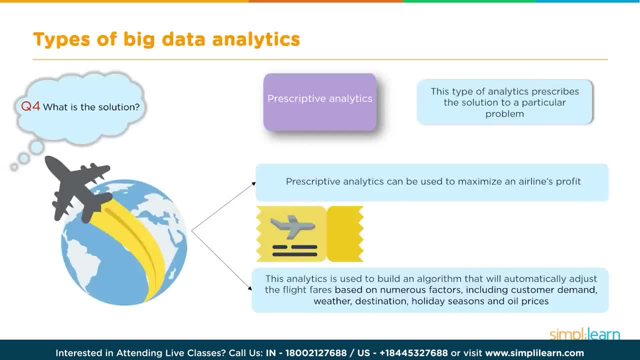 change due to availability and demand. Holiday seasons are a time when the rates are much higher than the normal days. Seasons like Christmas and school vacations. also weekends, the rates will be much higher than the normal days. So when you book a flight ticket, the price of it depends. on whether you book a flight ticket or not. Another factor which determines a flight's fare is your destination. Depending on the place where you are traveling to, the flight fare will be adjusted accordingly. This is because there are quite a few places where the air traffic is less. 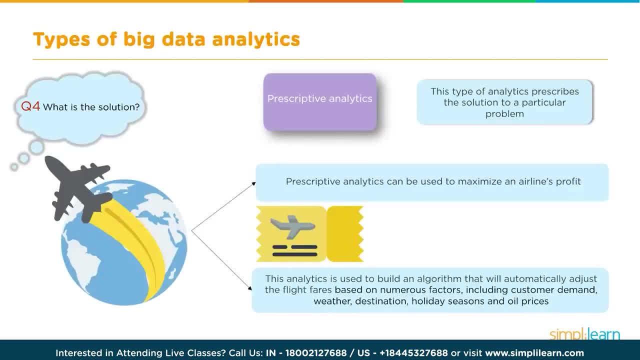 and in such places, the flight's fare will also be less. So prescriptive analytics analyzes all these factors that are discussed and it builds an algorithm which will automatically adjust a flight's fare. By doing so, the airline will be able to adjust its fare. So prescriptive analytics 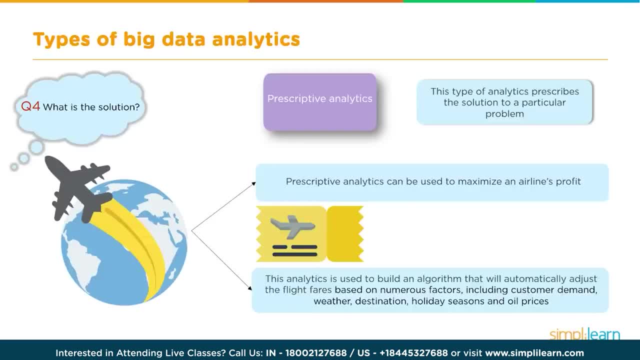 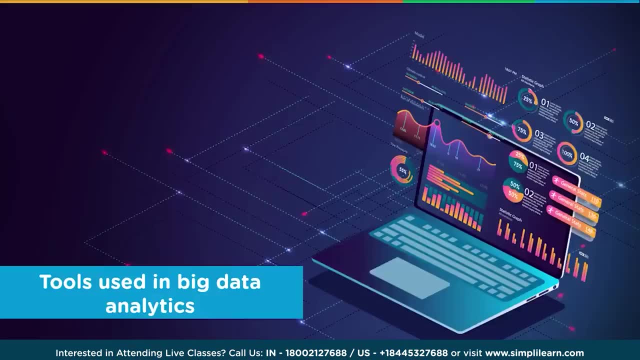 will help the airline to maximize its profit. These were the four types of analytics. Now let us understand how we achieve these with the use of big data tools. Our next topic will be the various tools used in big data analytics. These are few of the tools that I will be talking about. 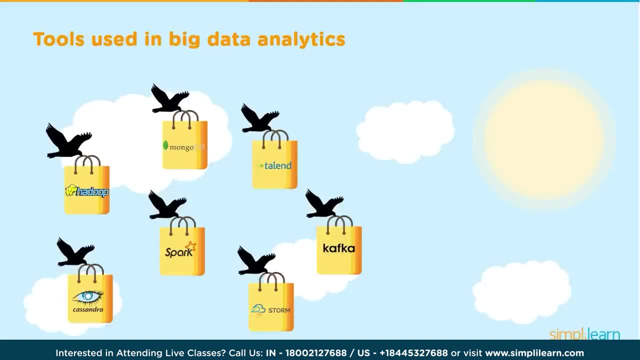 today We have Hadoop, MongoDB, Talendee, Kafka, Cassandra, Spark and Storm. We will look into each one of them one by one. We will first start off with Hadoop. When you speak of big data, The first framework that comes into everyone's mind is Hadoop, isn't it? 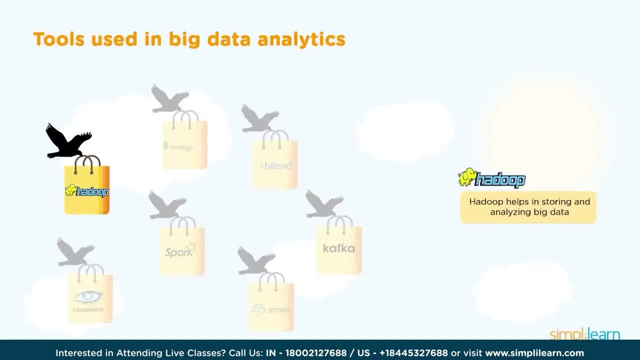 As I mentioned earlier, Apache Hadoop is used to store and process big data in a distributed and parallel fashion. It allows us to process data very fast. Hadoop uses MapReduce, Pig and Hive for analyzing this big data. Hadoop is easily one of the most famous big data tools. 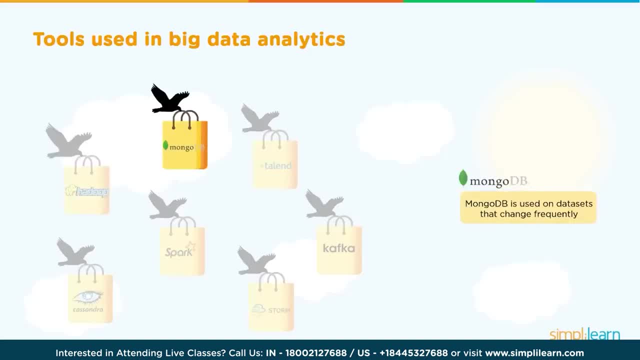 Now let us move on to the next one, that is, MongoDB. MongoDB is a cross-platform document-oriented database. It has the ability to deal with large amount of unstructured data, Processing of data which is unstructured and processing of data sets that change very frequently. 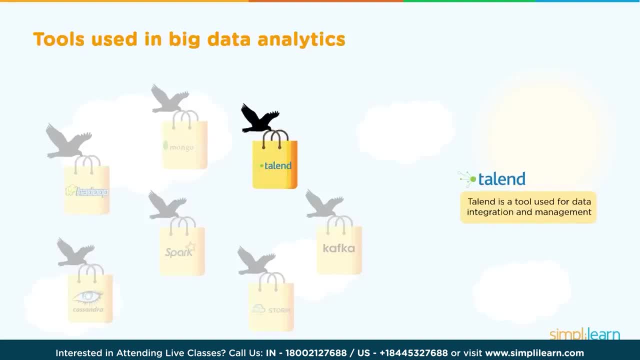 is done using MongoDB. Talendee provides software and services for data integration, data management and cloud storage. It specializes in big data integration. Talendee Open Studio is a free, open-source tool for processing data easily on a big data environment. 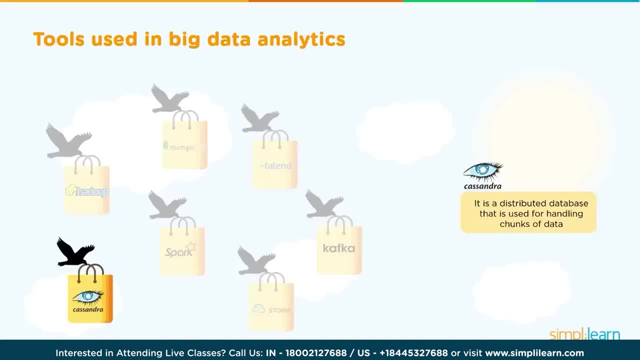 Cassandra is used widely for an effective management of large amounts of data. It is similar to Hadoop in its feature of fault tolerance, where data is automatically replicated to multiple nodes. Cassandra is preferred for real-time processing. Spark is another tool that is used for data processing. 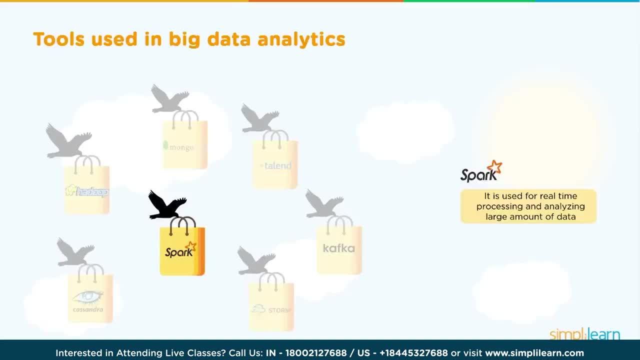 This data processing engine is developed to process data way faster than Hadoop MapReduce. This is done in a way because Spark does all the processing in the main memory of the data nodes and thus it prevents unnecessary input-output overheads with the disk, Whereas MapReduce is disk-based, and hence Spark proves to be faster than Hadoop MapReduce. 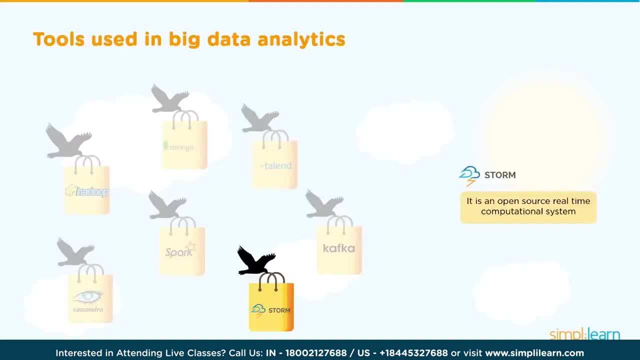 Storm is a free big data computational system which is done in real-time. It is one of the easiest tools for big data analysis. It can be used with any programming language. This feature makes Storm very simple to use. Finally, we will look into another big data tool, which is known as Kafka. 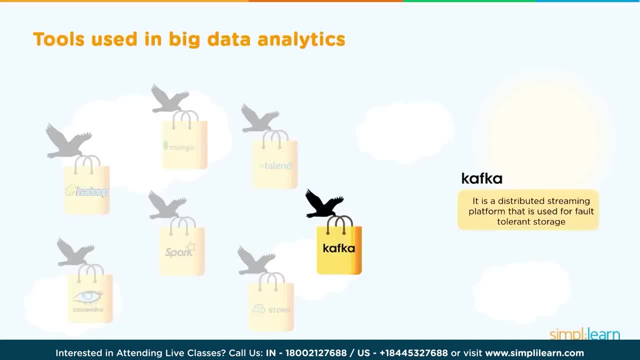 Kafka is a distributed streaming platform which was developed by LinkedIn and later given to Apache Software Foundation. It is used to provide real-time analytics result and it is also used for fault tolerant storage. These were few of the big data analytics tools. Now let us move on to our last topic for today, ie. 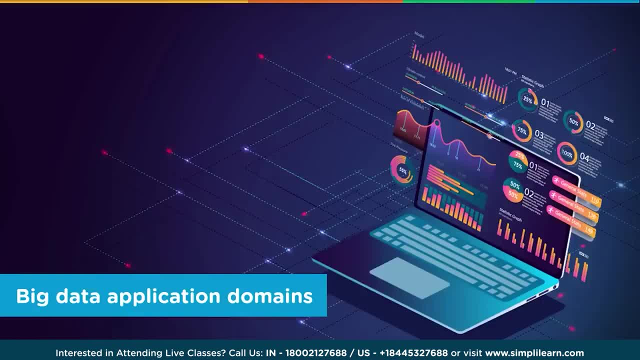 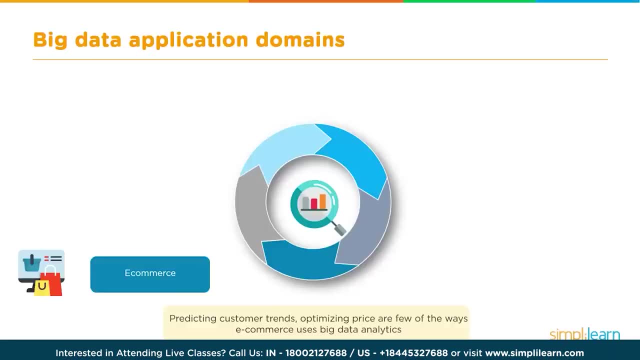 Big Data Application Domains. Here we will look into the various sectors where big data analytics is actively used. The first sector is e-commerce. Nearly 45% of the world is online and they create a lot of data every second. Big data can be used smartly in the field of e-commerce by predicting customer trend. 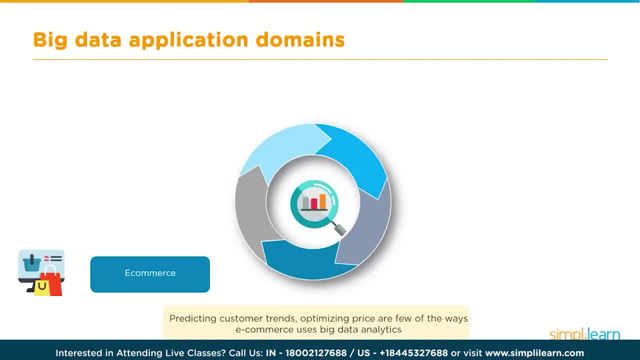 forecasting demands, adjusting the price and so on. Online retailers have the opportunity to create better shopping experience and to create a better customer experience. They can generate higher sales if big data analytics is used correctly. Having big data doesn't automatically lead to a better marketing strategy. 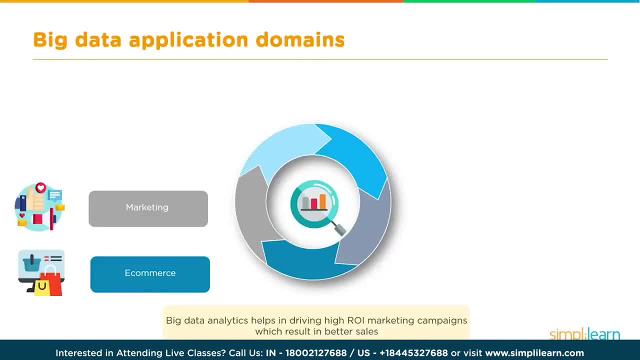 Meaningful insights need to be derived from it in order to make right decisions. By analyzing big data, we can have personalized marketing campaigns which can result in better and higher sales In the field of education. depending on the market requirements, new courses are developed. 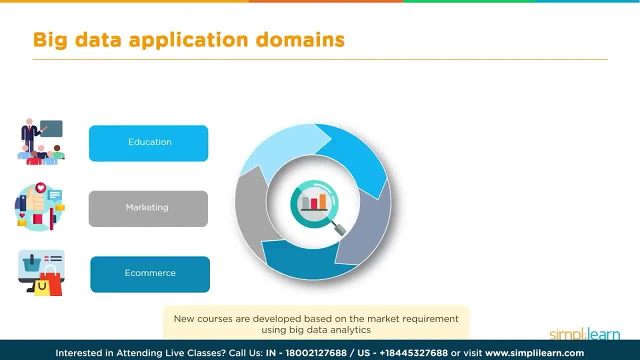 The market requirements are the following: The market requirement needs to be analyzed correctly with respect to the scope of a course and, accordingly, a scope needs to be developed. There is no point in developing a course which has no scope in the future. Hence, to analyze the market requirement and to develop new courses, we use big data analytics. 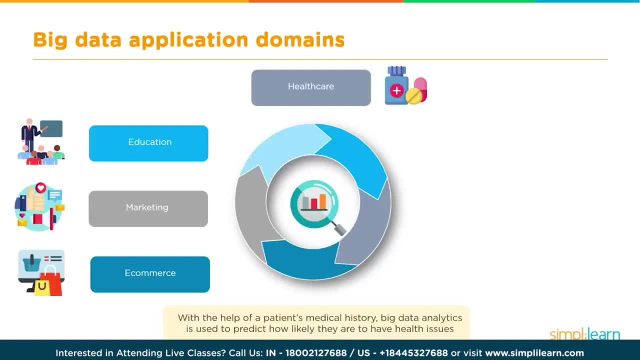 here. There are a number of uses of big data analytics in the field of healthcare, and one of it is to predict a patient's health issue. That is, with the help of their patient's health issues, they can predict a patient's health issue. 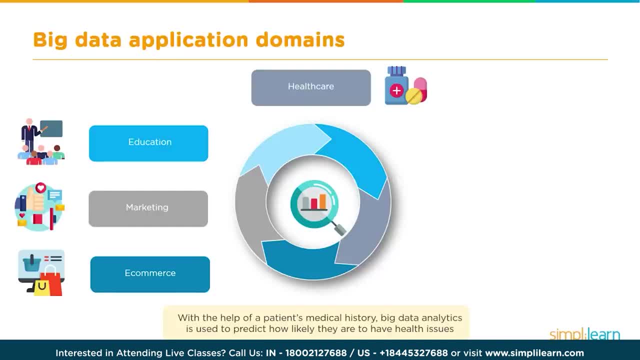 With the help of their previous medical history, big data analytics can determine how likely they are to have a particular health issue in the future. The example of Spotify that we saw previously showed how big data analytics is used to provide a personalized recommendation list to all its users. 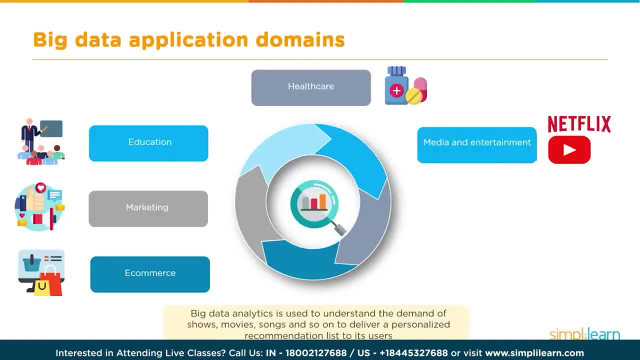 Similarly, in the field of media and entertainment, big data analytics is used to understand the demands of shows, songs, movies and so on, to deliver personalized recommendation lists. as we saw with Spotify, Big data analytics is used in the field of banking. 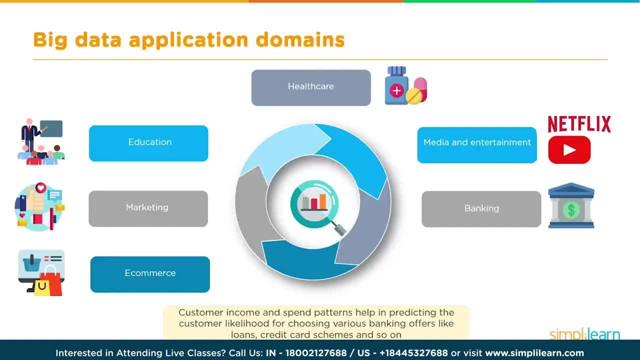 As we saw previously, with a few use cases, big data analytics was used for risk management. In addition to risk management, it is also used to analyze a customer's income and spend patterns and to help the bank predict if a particular customer is going to choose. 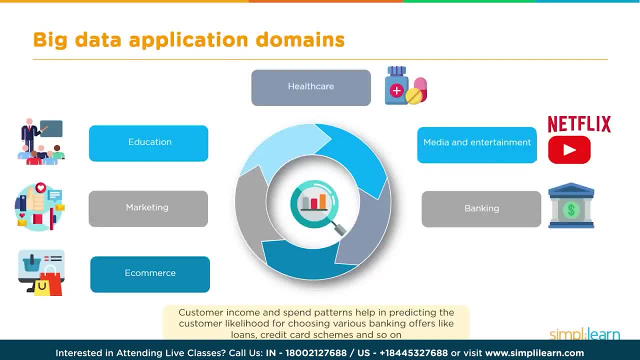 any of the bank offers, such as loans, credit cards schemes and so on. This way, the bank is able to identify the right customer. This way, the bank is able to identify the right customer. This way, the bank is able to identify the right customer. 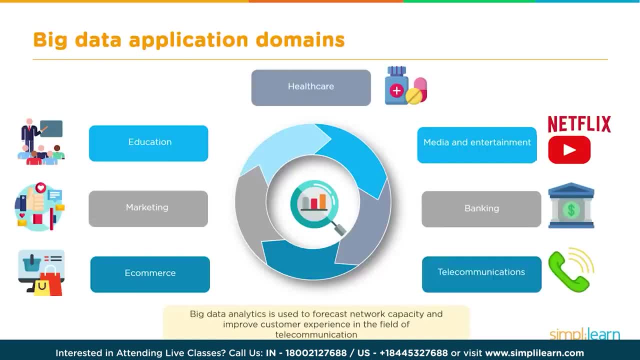 The bank is able to identify the right customer who is interested in its offers. It has noticed that telecom companies have begun to embrace big data to gain profit. Big data analytics helps in analyzing network traffic and call data records. It can also improve its service quality and improve its customer experience. 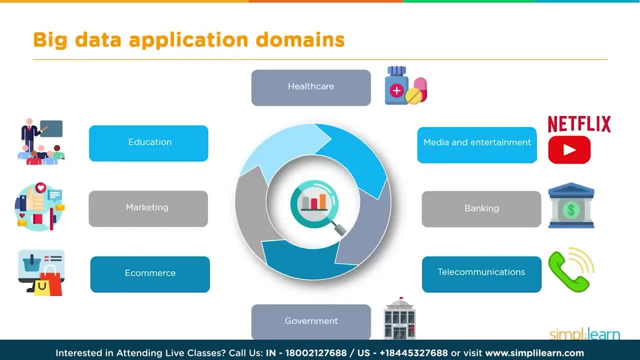 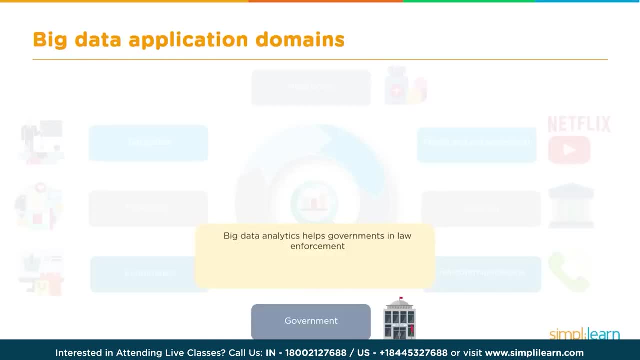 Let us now look into how big data analytics is used by governments across the world In the field of law enforcement. big data analytics can be applied to analyze all the events and are also designed in a way that is very easy to understand and easy to understand. 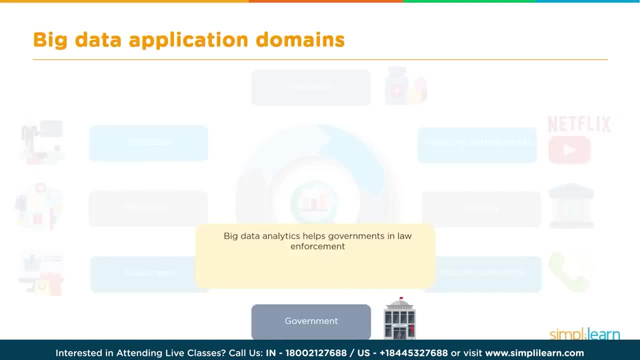 data to understand crime patterns. intelligent services can use predictive analytics to forecast the crime which could be committed. in Durham, the police department was able to reduce the crime rate using big data analytics. with the help of data, police could identify whom to target, where to go when to patrol and. 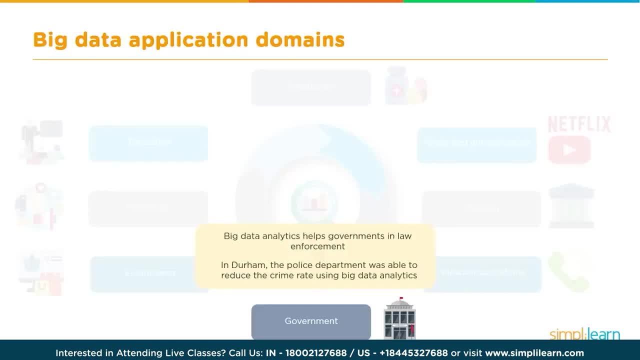 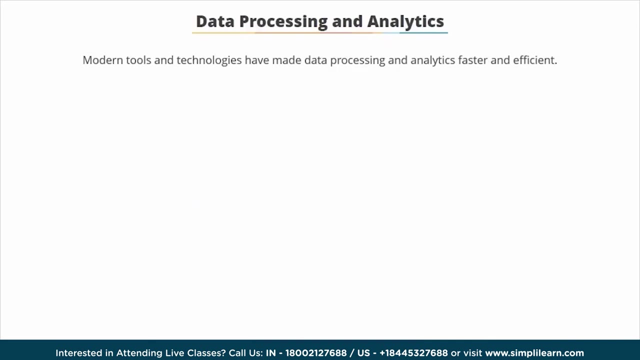 how to investigate crimes. big data analytics helped them to discover patterns of crime emerging in the area. now that we have seen the various sectors where big data analytics is used, we now have access to tools and techniques that process data and extract the information we need, for instance, 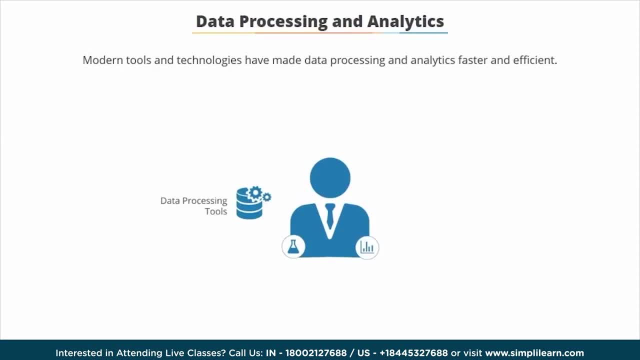 there are data processing tools for data wrangling. we have new and flexible programming languages that are more efficient and easier to use. with the creation of operating systems that support multiple OS platforms, it's now easier to integrate systems and problems. big data application designs and extensive software libraries helped. 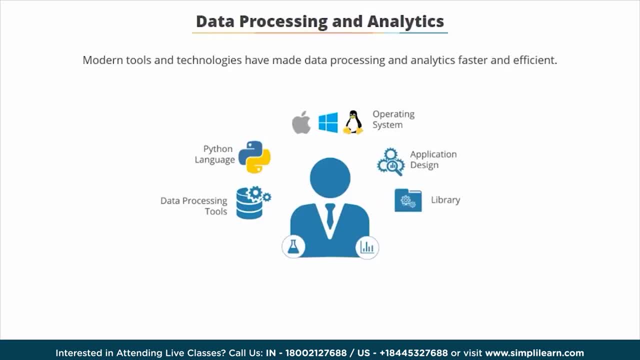 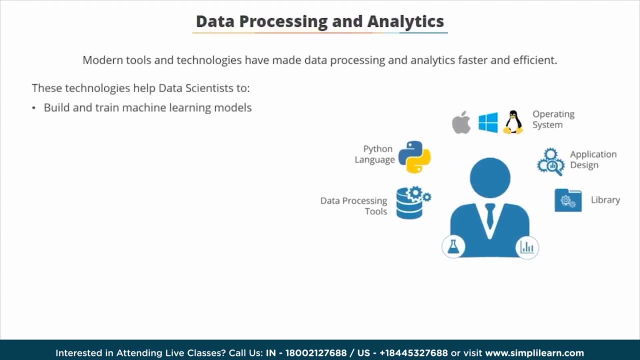 develop more robust, scalable and data-driven applications. data scientists use these technologies to build data models and run them in an automated fashion to predict the outcome efficiently. this is called machine learning, which helps provide insights into the underlying data. they can also use data science technology to manipulate data, extract information from. 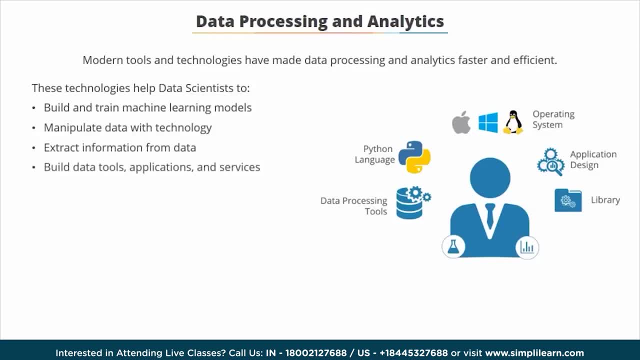 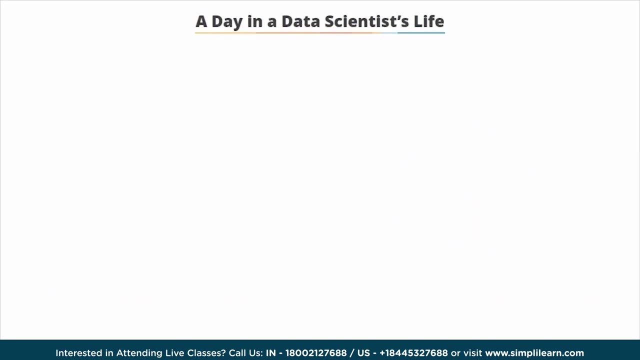 it and use it to build tools, applications and services. but technological skills and domain expertise alone, without the right mathematical and statistical knowledge, might lead data scientists to find incorrect patterns and convey the wrong information. now that you have learned what data science is, it will be easier to understand what a data scientist does. data scientists start with a question or 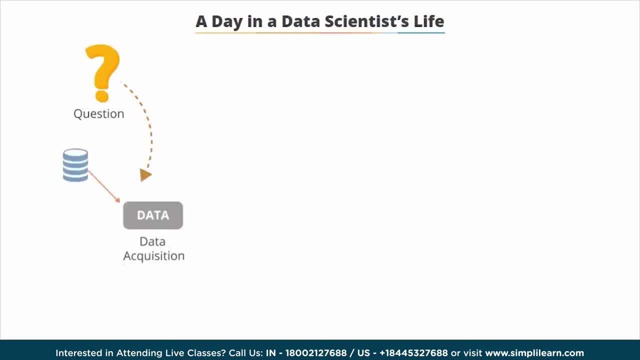 a business problem. then they use data acquisition to collect data sets and create new data sets from the real world. the process of data wrangling is implemented with data tools and modern technologies that include data cleansing, data manipulation, data discovery and data pattern identification. the next step is to create and train models for machine learning. they then design: 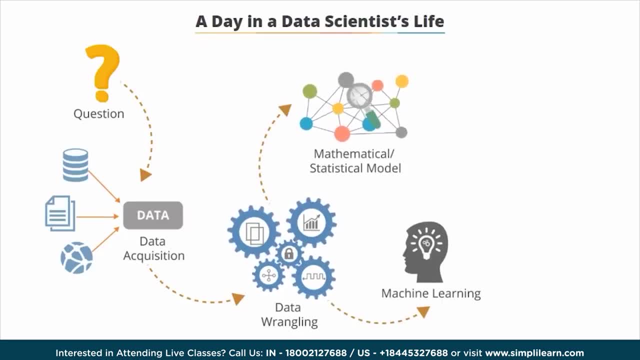 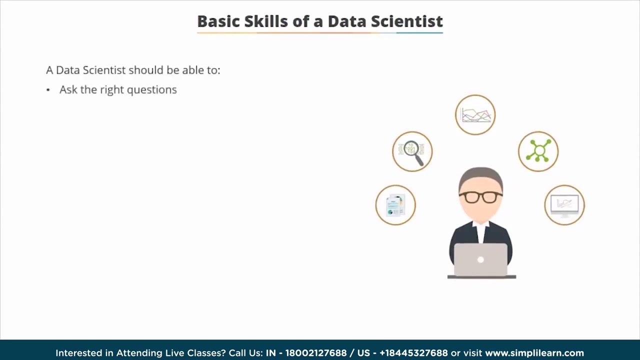 mathematical or statistical models. after designing a data model, it's represented using data visualization techniques. the next task is to prepare a data report. after the report is prepared, they finally create data products and services. let us now look at the various skills of data scientists should have. data scientists should ask the right questions, for which they need domain. 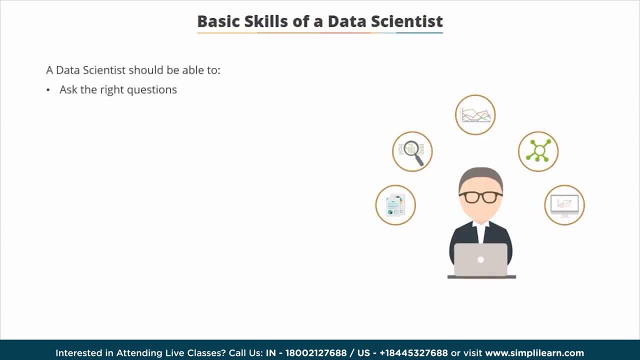 expertise, the curiosity to learn and create concepts, and the ability to communicate questions effectively to domain experts. data scientists should think analytically to understand the hidden patterns in a data structure. they should wrangle the data by removing redundant and irrelevant data collected from various sources. statistical thinking and the ability to apply 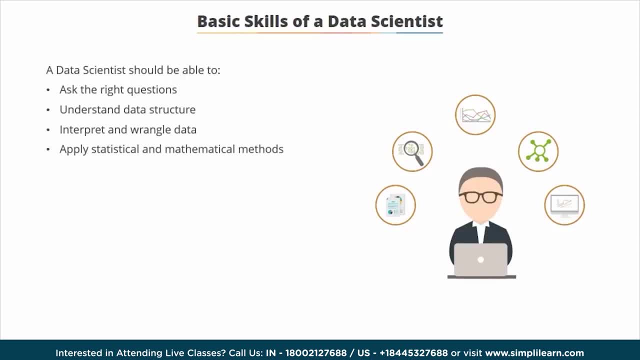 mathematical methods are important traits for a data scientist. data should be visualized with graphics and proper storytelling to summarize and communicate the analytical results to the audience. to get these skills, they should follow a distinct roadmap. it's important they adopt the required tools and techniques, like Python and its libraries. they should build projects. 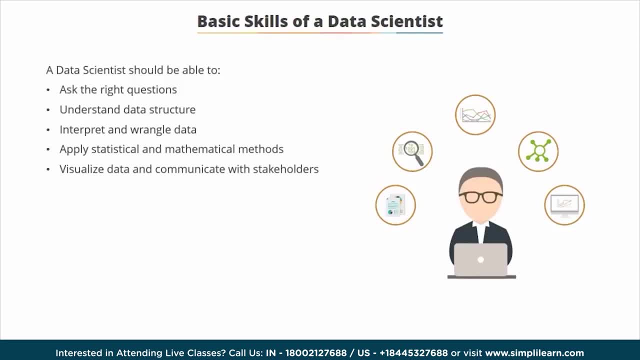 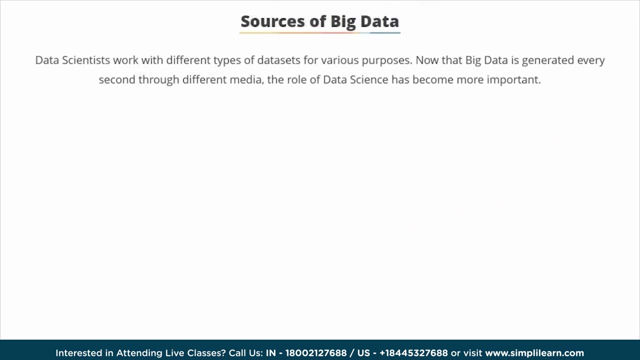 using real-world data sets that include data gov, NYC, open data gap, minder, and so on. they should also build data-driven applications for digital services and data products. scientists work with different types of data sets for various purposes. now that big data is generated every second through different media, the role of data. 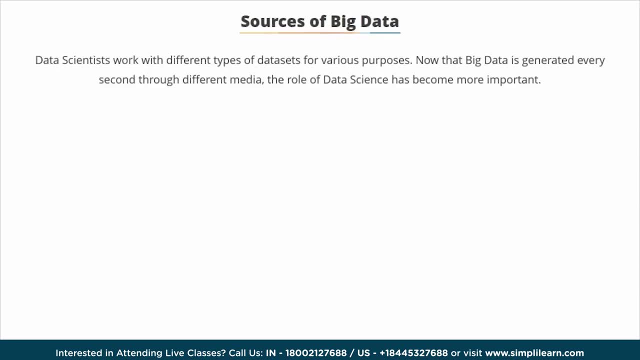 science has become more and more important for a data scientist, so you need to know what big data is and how you are connected to it to figure out a way to make it work for you. every time you record your heartbeat through your phone's biometric sensors, post or tweet on the social network- create any 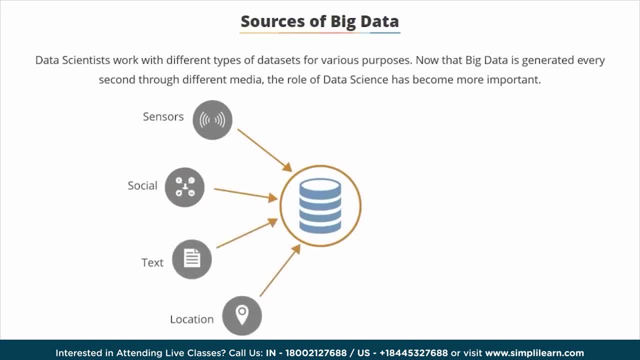 blog or website, switch on your phone's GPS network, upload or view an image, video or audio. in fact, every time you log into the internet, you are generating data about yourself, your preferences and your lifestyle. Big Data is a collection of these and a lot more data, but the world is. 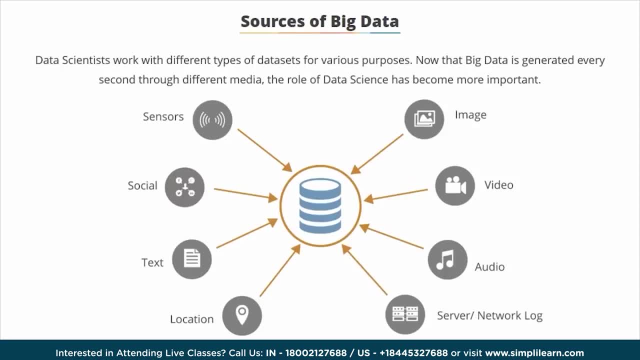 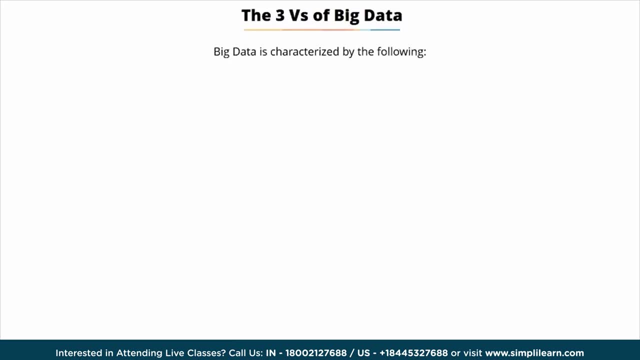 constantly creating. in this age of the internet of things or IOT, Big Data is a reality and a need. big data is usually referenced by three V's: volume, velocity and variety. volume refers to the enormous amount of data generated from various sources. Big Data is also characterized by velocity: huge amounts. 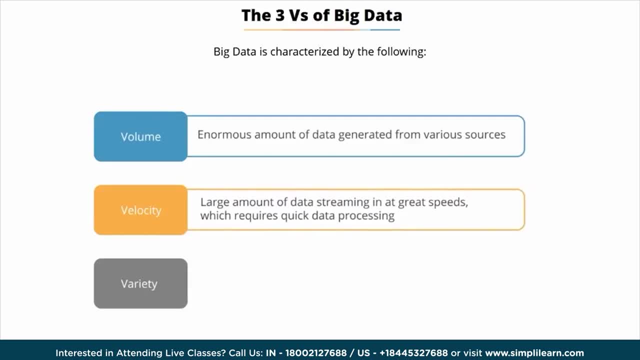 of data flow, tremendous speed from different devices, sensors and applications. to deal with it, an efficient and timely data processing is required. variety is the third V of big data, because big data can be categorized into different formats, like structured, semi-structured and unstructured. structured data is usually 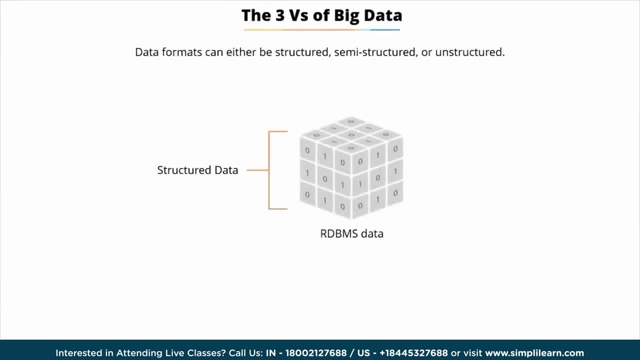 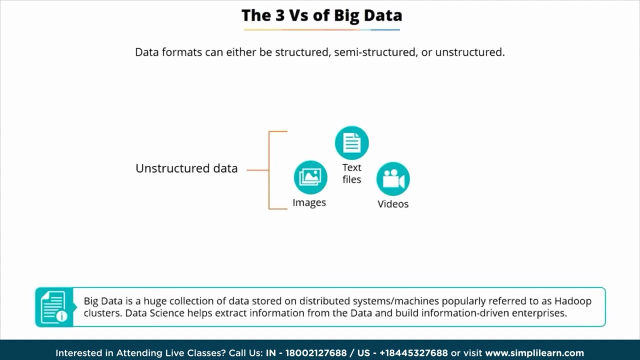 referenced to as our DBMS data which can be stored and retrieved easily through SQL's. semi-structured data are usually in the form of files like XML JSON documents and no SQL database. text files, images, videos or multimedia content are examples of unstructured data. in short, big data is a very large information. 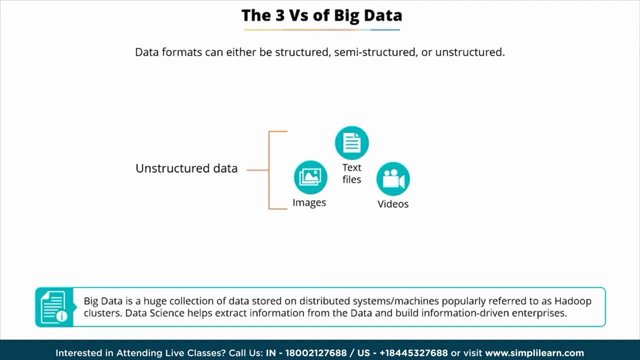 database usually stored on distributed systems or machines, popularly referred to as Hadoop clusters. but to be able to use this database, we have to find a way to extract the right information and data patterns from it. that's where data science comes in. data science helps to build information driven enterprises. 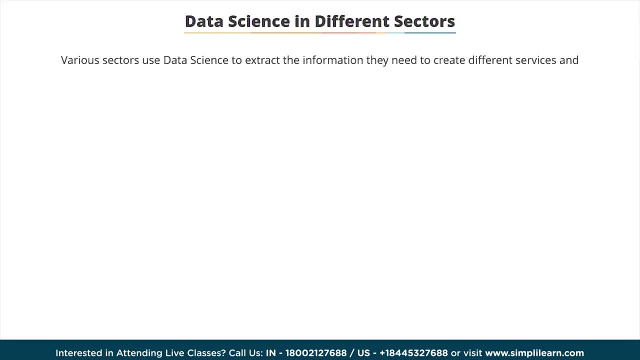 let's go on to see the applications of data science in different sectors. social network platforms such as Google, Yahoo, Facebook and so on collect a lot of data every day, which is why they have some of the most advanced data centers spread across the world, having data centers all over the world and not just in the 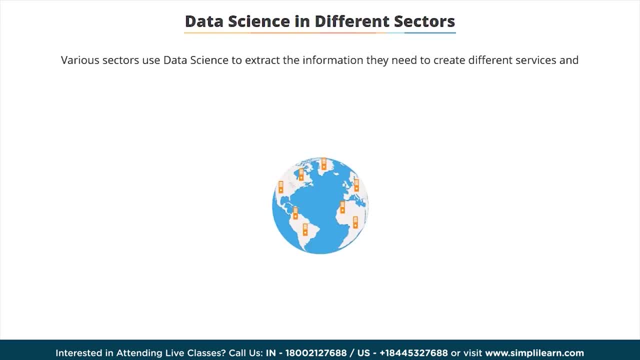 US help these companies serve their international customers better and faster, without any network latency. they also help them deal effectively with the enormous amount of data. so what do all these different sectors do with all this big data? their team of data scientists to analyze all the raw data with the 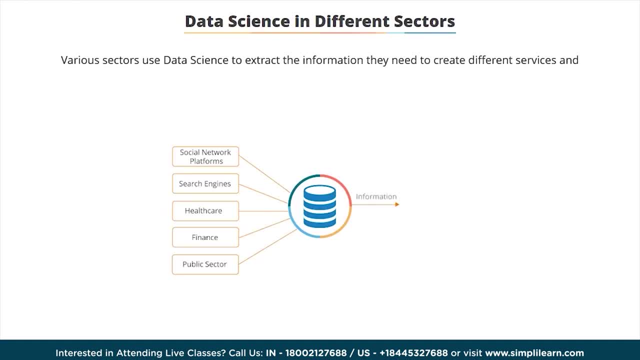 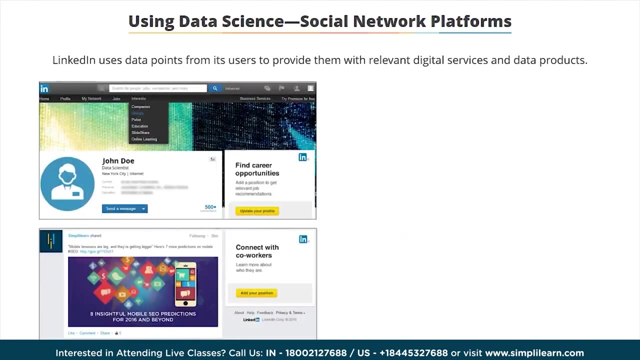 help of modern algorithms and data models to turn it into information. they then use this information to build digital services, data products and information driven apps. Now let's see how these products and services work. we'll first look at LinkedIn. let's suppose that you are a data scientist based in New York City, so 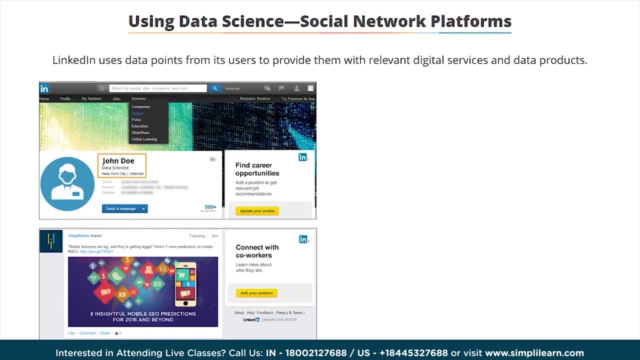 it's quite likely that you would want to join a group or build connections with people related to data science in New York City. now, what LinkedIn does, with the help of data science, is that it looks at your profile, your posts and likes the city you are from, the people you are connected to and the group you 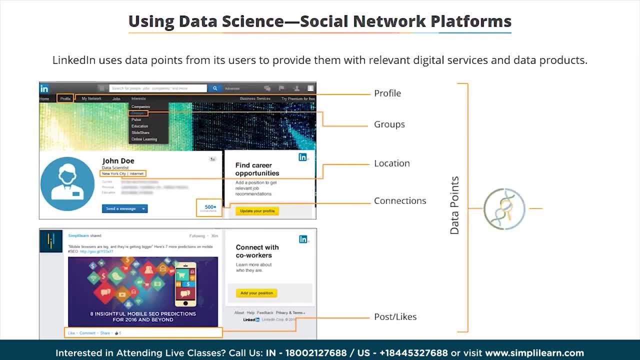 belong to, then it matches all that information with its own database to provide you with information that is most relevant to you. this information could be in the form of news updates that you might be interested in, industry connections or professional groups that you might want to get in touch with, or even job. 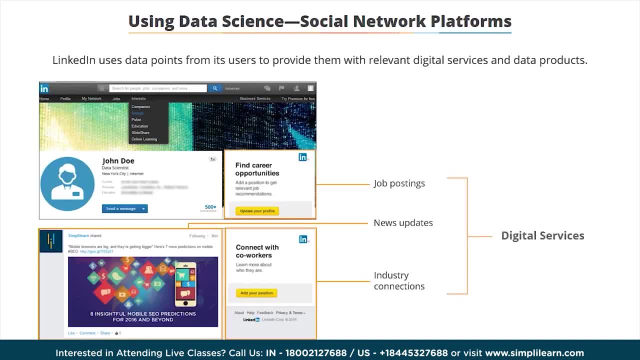 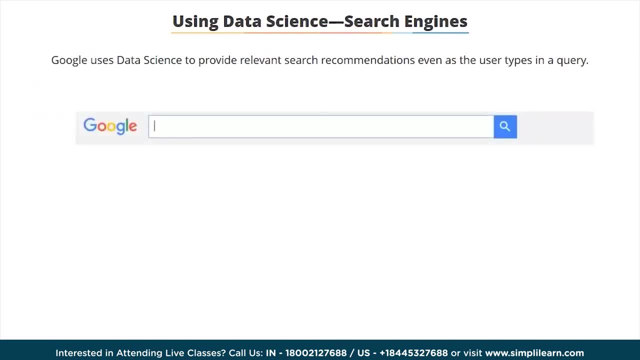 postings related to your field and designation. these are all examples of data services. let's now look at something that we use every day: Google's search engine. Google search engine has the most unique search algorithm, which allows machine learning models to provide relevant search recommendations even as the user types in his or her query. this feature is 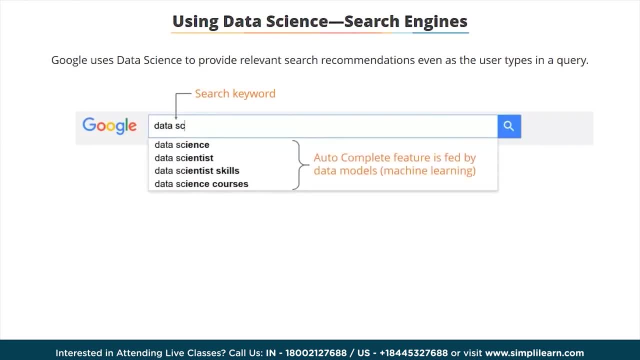 called autocomplete. it is an excellent example of how powerful machine learning can be. there are several factors that influence this feature. the first one is query volume. Google's algorithms identify unique and verifiable users that search for any particular keyword on the web. based on that, it builds a 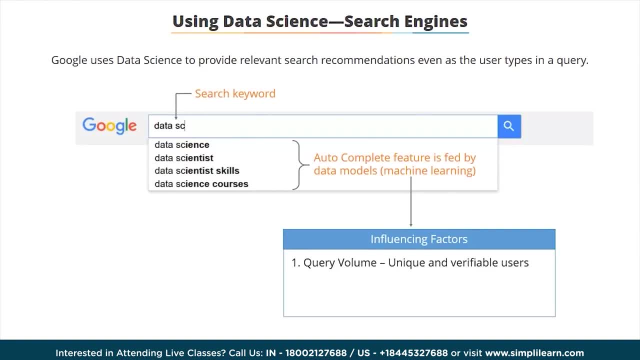 query volume. for instance, Republican debate 2016, ebola threat, CDC or the center of disease control, and so on are some of the most common user queries. another important factor is a geographical location. the algorithms tag a query with the locations from where it is generated. this makes a query volume location specific. it's a very important feature. 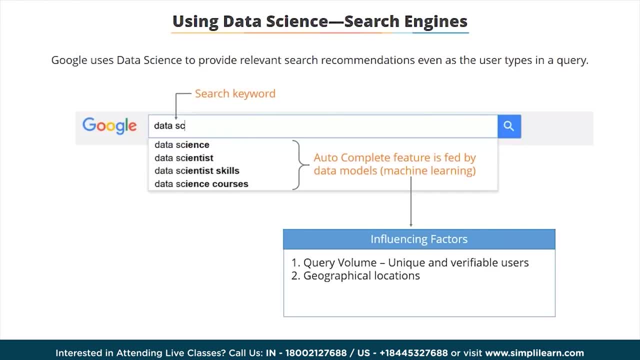 because this allows Google to provide relevant search recommendations to its user based on his or her location. and then, of course, the algorithms consider the actual keywords and phrases that the user types in. it takes up those words and it crawls the web looking for similar instances. the algorithms also try to filter or scrub out inappropriate. 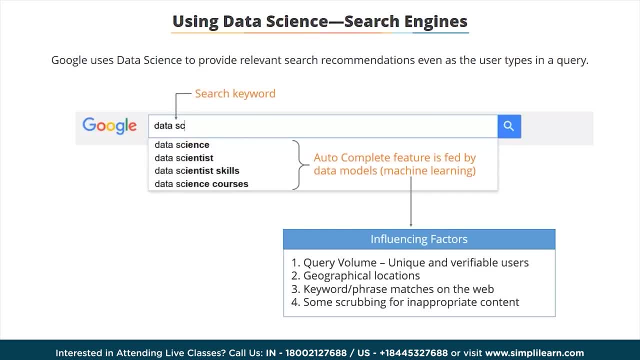 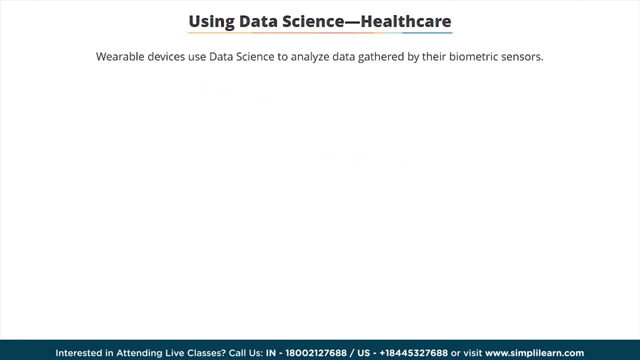 content, for instance, sexual, violent or terrorism related content, hate speeches and legal cases, are scrubbed out from the search recommendations. but how does data science help you? today, even the healthcare industry is beginning to tap into the various applications of data science. to understand this, let's look at wearable devices. these devices have biometric 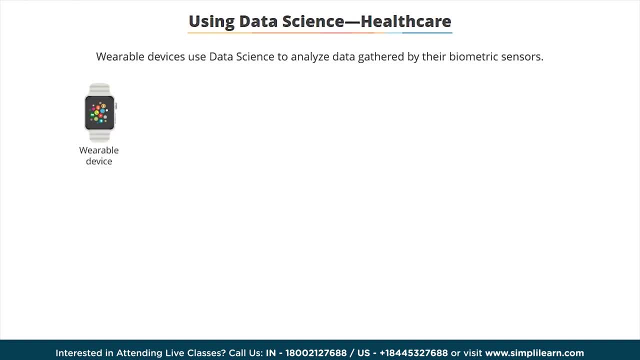 sensors and a built-in processor to gather data from your body when you are wearing them. they transmit this data to the big data analytics platform via the IOT gateway. ideally, the platform collects hundreds of thousands of data points and the collected data is ingested into the system for further processing. 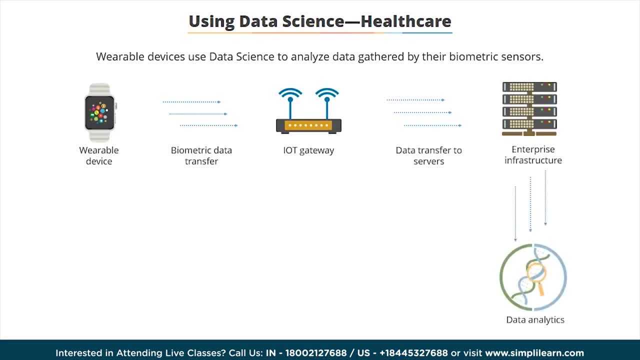 the big data analytics platform, applies data models created by data scientists and extracts the information that is relevant to you. it sends the information to the engagement dashboard, where you can see how many steps you walk, what your heart rate is over a period of time, how good your sleep was, how much. 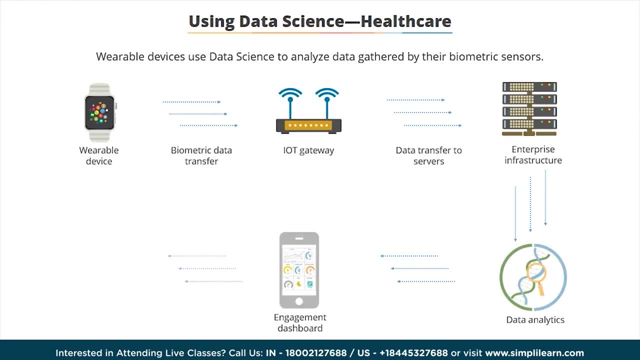 calories you burned, and so on. knowing such details would help you to set personal goals for a healthy lifestyle and reduce overall health care and insurance costs. it would also help your doctor record your vitals and diagnose any issue. the finance sector can easily use data science to help it function more. 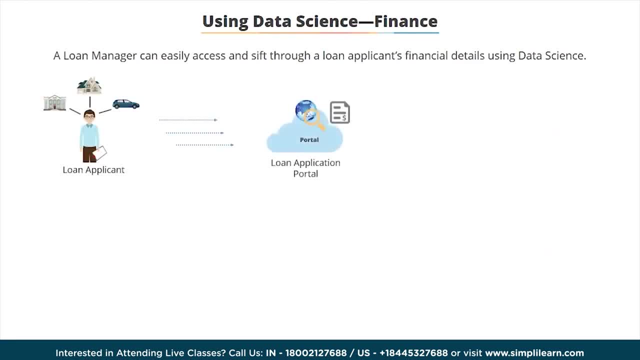 efficiently. suppose a person applies for a loan, the loan manager submits the application to the enterprise infrastructure for processing the annual interest rate of the loan. for that purpose, the loan manager uses a data report to spotlight upon how the risk is going and what he is considering for the loan manager. the loan manager would measure the risk targets for the. 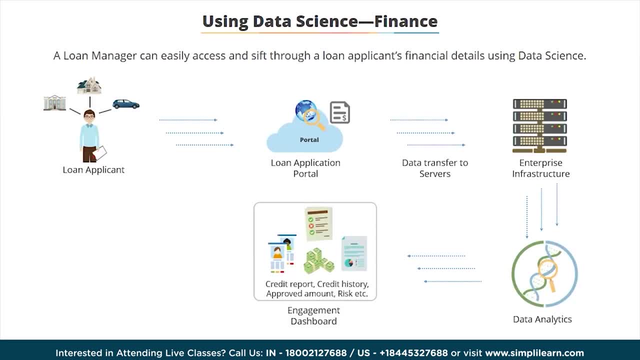 loan. if it's a active loan, the loan managers in the finance sector could assess and determine the risk factors of the loan and pick the right risk factors that might be the worst for the investor. the loan manager can now easily take a look at all the relevant information and 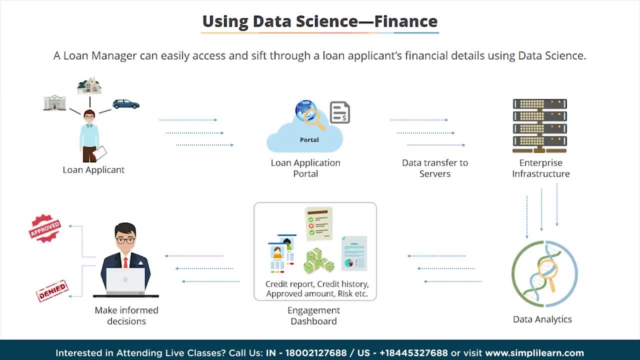 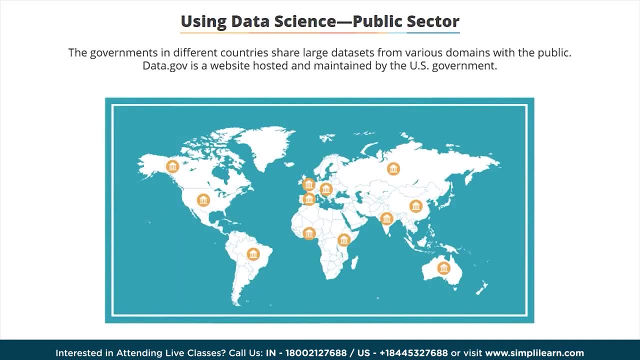 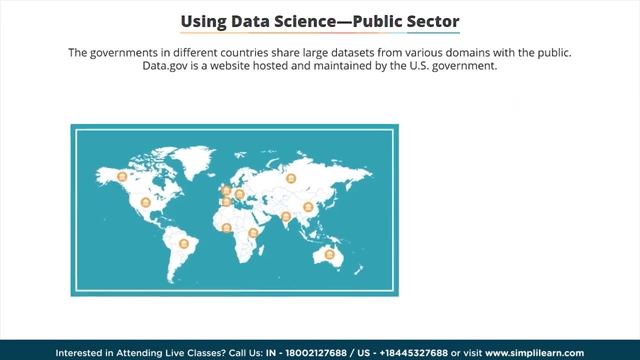 decide whether the loan can be approved or not. you you will be able to look at all of these data sources for specific reasons and data sets from various domains with the public. This kind of transparency makes the government seem more trustworthy. It provides the country data that can be used to prepare itself for different types of issues. 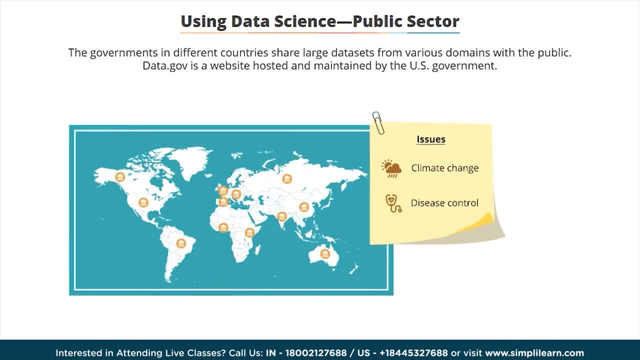 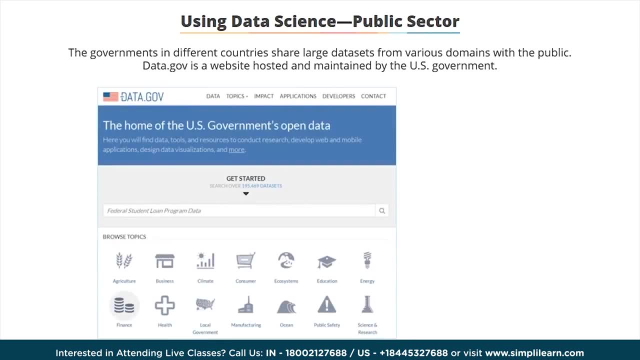 like climate change and disease control. It also helps encourage people to create their own digital products and services. The US government hosts and maintains Datagov, a website that offers information about the federal government. It provides access to over 195,000 datasets across different sectors. 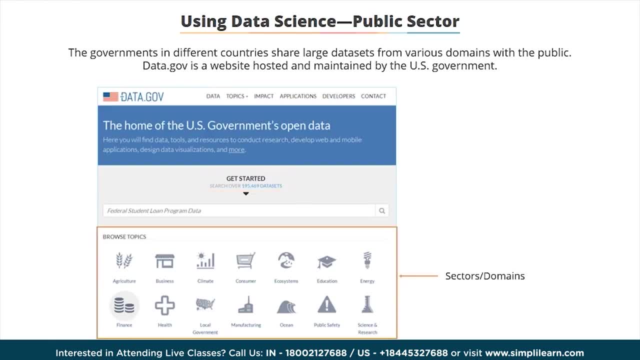 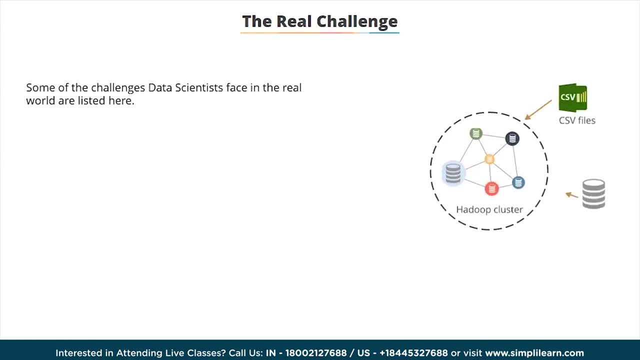 The US government has kicked off a number of strategic initiatives in the field of data science. that includes US Digital Service and Open Data. We have seen how data science can be applied across different sectors. Let's now take a look at the various challenges that a data scientist faces in the real world. 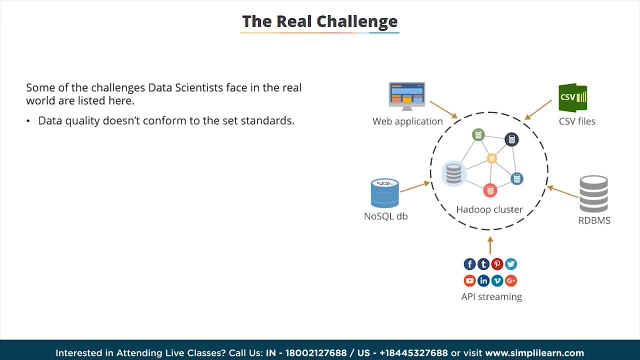 while dealing with datasets- Data Quality- The quality of data is mostly not a set standard- You will usually come across data that is inconsistent, inaccurate, incomplete, not in the desirable format and with anomalies. Integration- Data integration with several enterprise applications and systems is a complex and painstaking task. 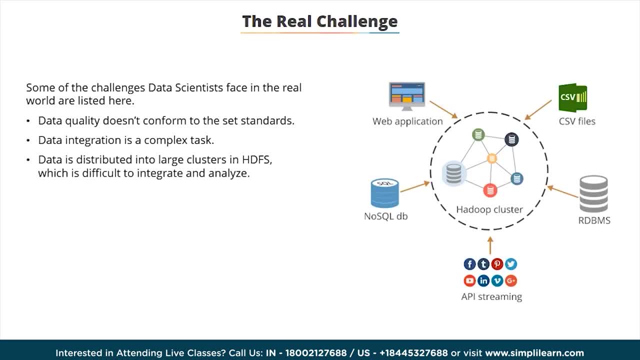 Unified Platform. Data is distributed to Hadoop Distributed File System, or HDFS, from various sources to ingest, process, analyze and visualize data. Hadoop Distributed File System is a complex and painstaking task. The size of these Hadoop clusters can vary from few nodes to 1,000 nodes. 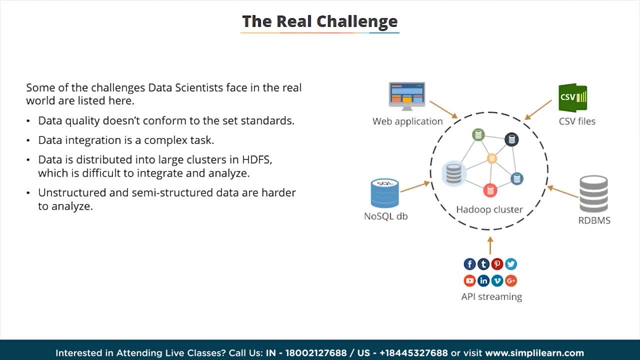 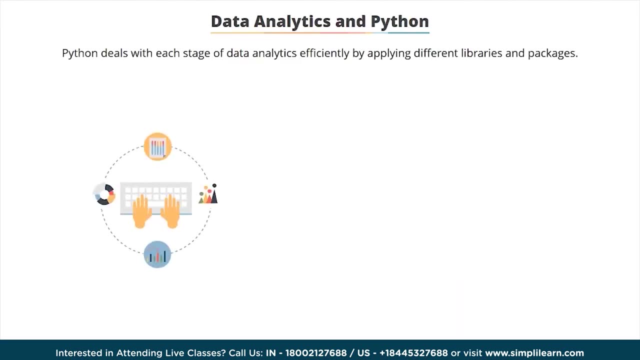 The challenge is to perform analytics on these large datasets efficiently and effectively. This is where Python comes into play. with its powerful set of libraries, functions, modules, packages and extensions, Python can efficiently tackle each stage of data analytics. that includes data acquisition. 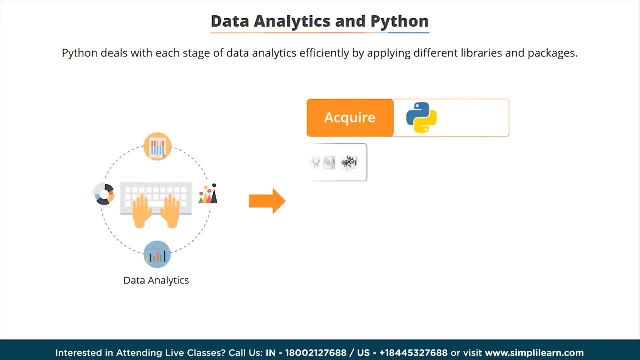 Python libraries such as Hadoop. Python libraries such as Scrappy comes handy here. Data Wrangling- Python data frames are very efficient in handling large datasets and makes data wrangling easier. with its powerful functions, Explore- Matplotlib libraries are very rich when it 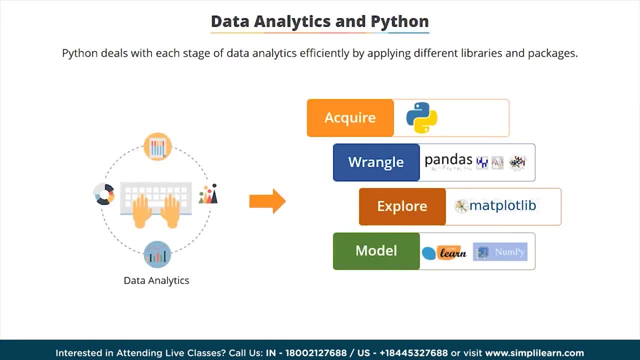 comes to data exploration. Model, Scikit learns statistical and mathematical functions to help to build models for machine learning Visualization. Modern libraries such as Voka creates very intuitive and interactive visualization. Its huge set of libraries and functions make big data analytics seem easy and hence solves. 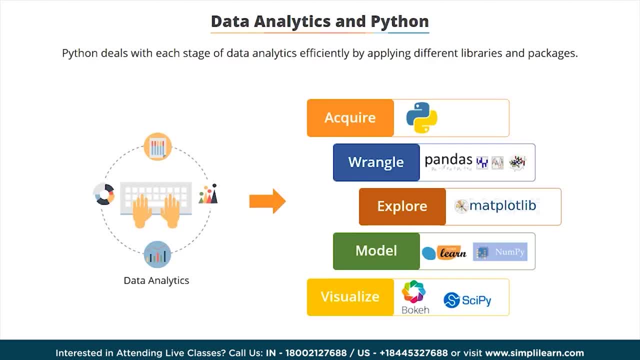 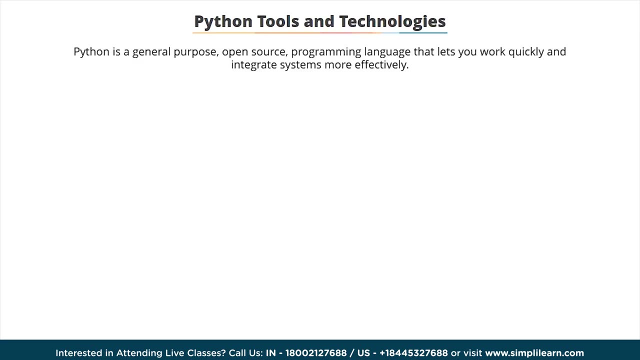 the bigger problem. Python applications and programs are portable and helps them scale out on any big data platform. Python is an open-source programming language that lets you work quickly and integrate systems more effectively. Now that we have talked about how the Python libraries help the different, 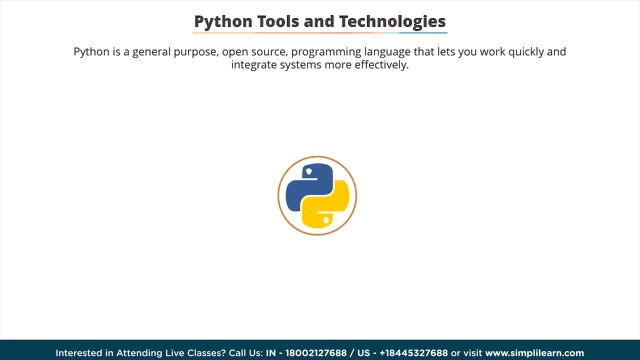 stages of data analytics. let's take a closer look at these libraries and how they support different aspects of data science. NumPy, or Numerical Python, is the fundamental package for scientific computing. SciPy is the core of scientific computing libraries and provides many user-friendly. 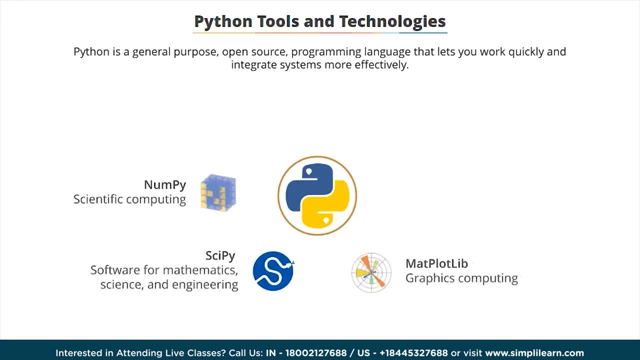 and efficiently designed numerical routines. Matplotlib is a Python 2D plotting library which produces publication quality figures in a variety of hard copy formats and interactive environments. Scikit-learn is built on NumPy, SciPy and Matplotlib for data mining and data analysis. 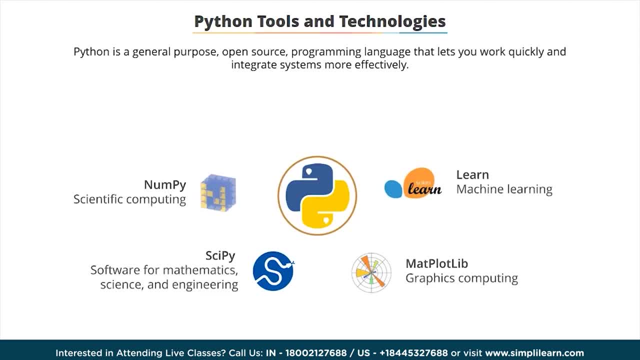 Pandas is a library providing high-performance, easy-to-use data structures and data analysis tools for Python. All these libraries, modules and packages are open-source and hence using them is convenient and easy. There are numerous factors with Python that make it so easy to use. 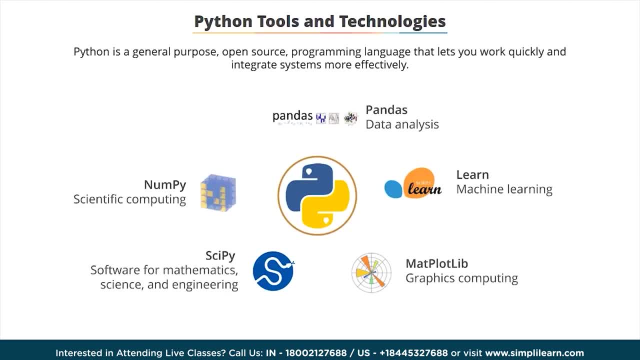 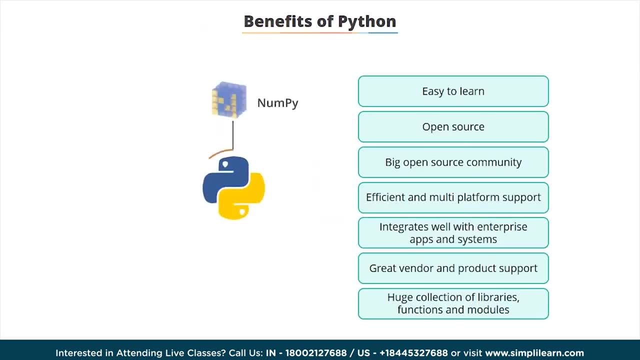 One of these factors is the fact that it can be used in many different ways, and it is not just a matter of how you use it, but it can be used in many different ways. For example, if you want to use Python, you need to have a lot of data. 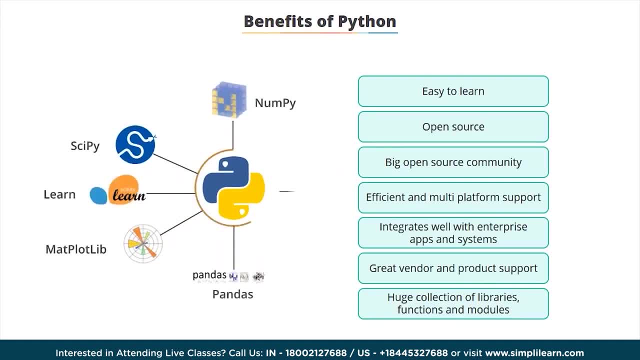 Python is an open-source programming language, which positions Python well and makes it the tool for data science. Python is easy to learn. It's a general-purpose, function- and object-oriented programming language. As Python is an open-source programming language, it is readily available, easy to install. 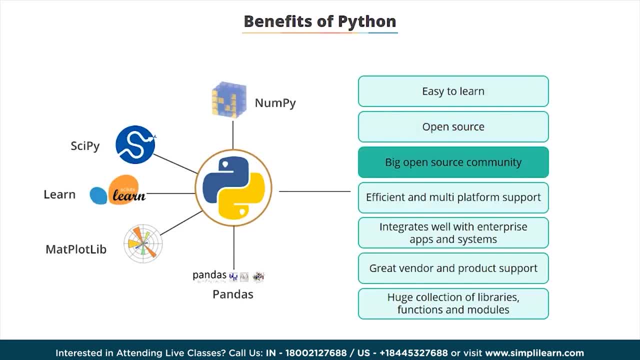 and get started. It also has a large presence of open-source community for software development and support. Python and its tools enjoy multi-platform support. Applications developed with PyCon integrate Python and its tools into a multi-platform community. It can be used easily with other enterprise systems and applications. 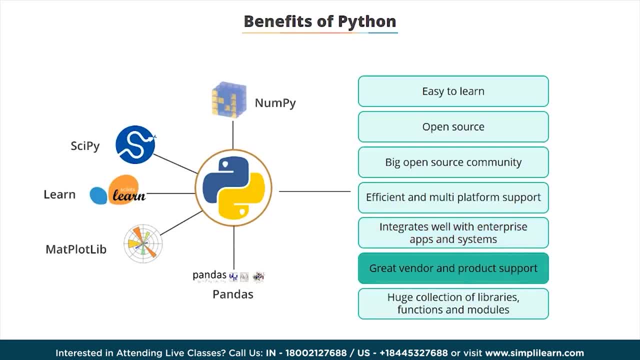 There are a lot of tools, platforms and products in the market from different vendors, as they offer great support and services. Python and its libraries create unique combinations for data science. Because of all these benefits, it's usually popular among academicians, mathematicians. 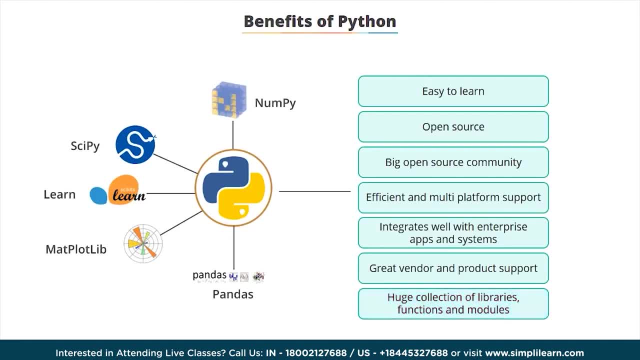 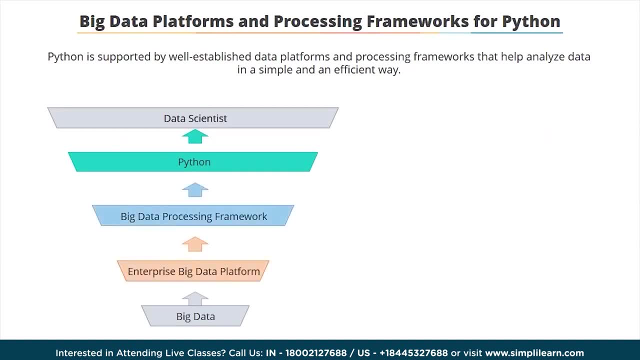 statisticians and technologists. Python is supported by Python. Python is also supported by well-established data platforms and processing frameworks that help it analyze data in a simple and efficient way. Enterprise Big Data Platform Cloudera is the pioneer in providing enterprise-ready Hadoop Big Data Platform and supports Python. 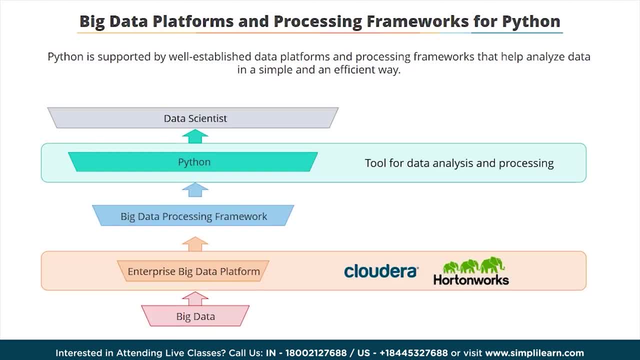 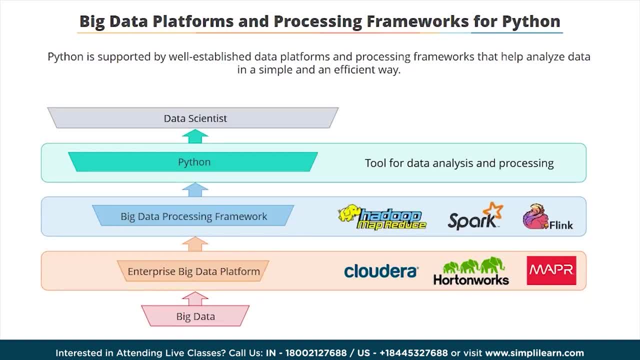 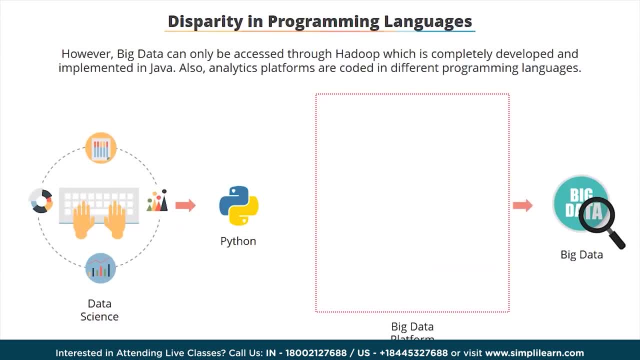 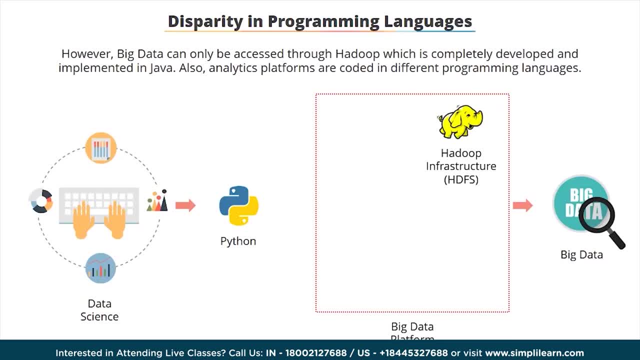 cheaper and efficient computing. It's completely developed and coded in Java. One of the most popular analytics platforms is Spark. It easily integrates with HDFS. It can also be implemented as a standalone analytics platform and integrated with multiple data sources. It helps data scientists perform their work. 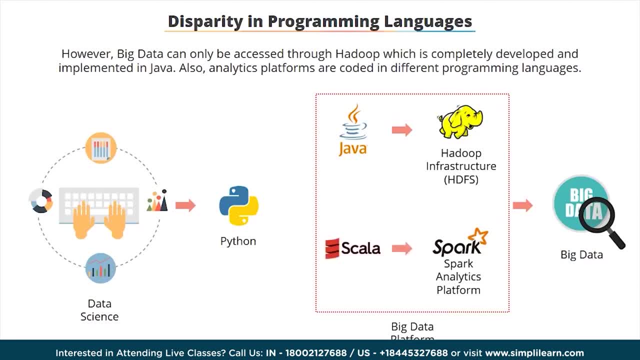 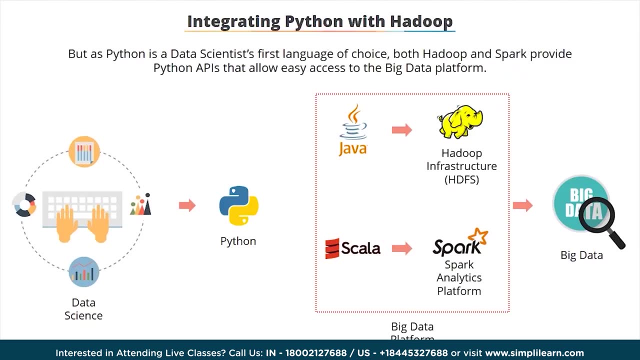 more efficiently. Spark is built using Scala, Since there is a disparity in the programming language that data scientists use and that of the big data platform. it impedes data access and flow, As Python is a data scientist's first language of choice, both Hadoop and Spark. 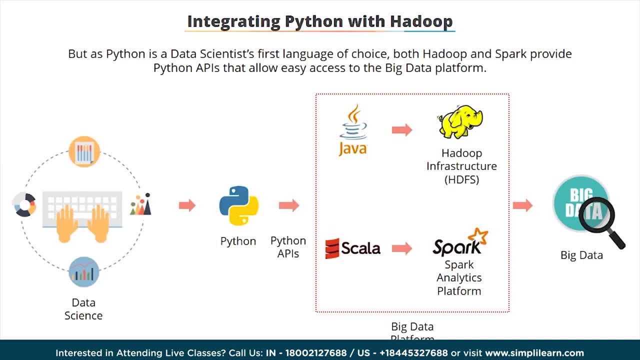 provide Python APIs that allow easy access to the big data platform. Consequently, a data scientist need not learn Java or Scala or any other platform-specific data languages, and can instead focus on performing data analytics. There are several motivations for Python: big data solutions. Big data is a. 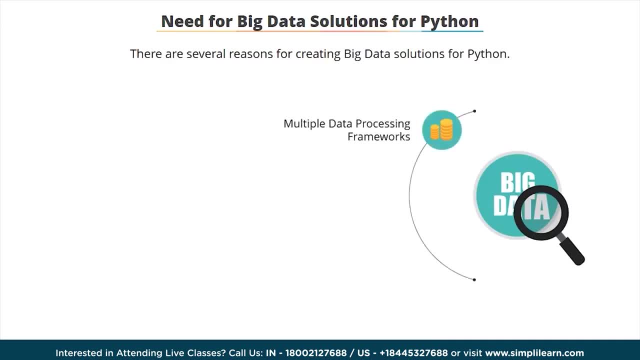 continuously evolving field, which involves adding new data processing frameworks that can be developed using any programming language. Moreover, new innovation and research is driving the growth of big data solutions and platform providers. It would be difficult for data scientists to focus on analytics if they have to constantly upgrade themselves on information or under the 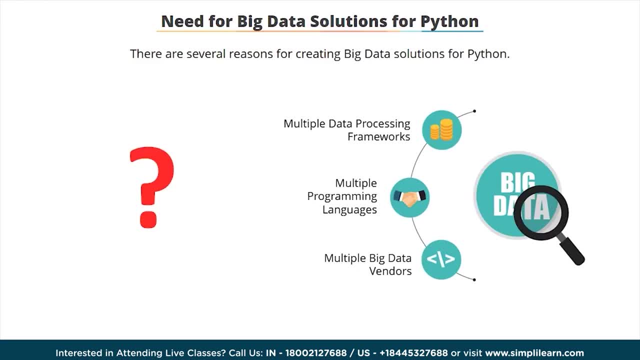 hood architecture or implementation of the platform. Therefore, it's important to keep the entire data science platform and any language agnostic, to simplify a data scientist's job. Consequently, almost all major vendors, solution providers and data processing framework developers are providing Python APIs. 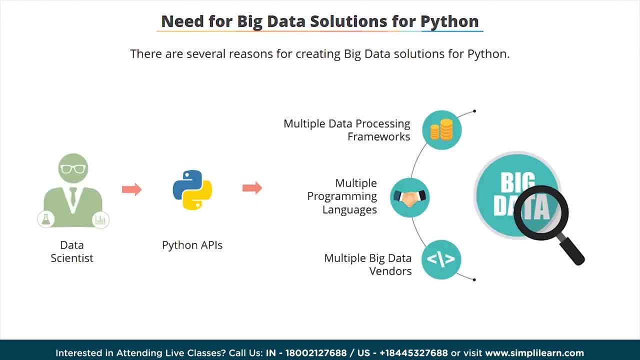 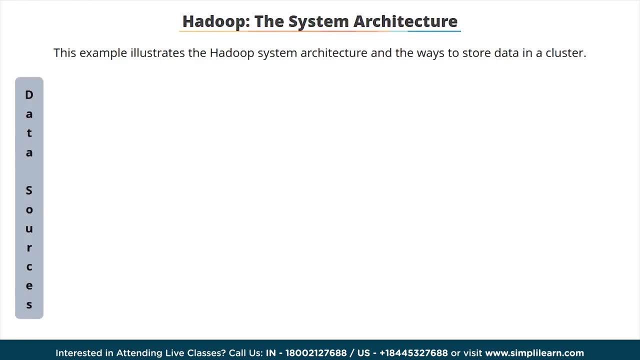 This allows a data scientist to perform big data analytics using only Python, rather than learning other languages like Java or Scala to help them work on the big data platform. Let's look at an example and understand how data is stored across Hadoop's distributed clusters. Big data is generated from different data sources. A 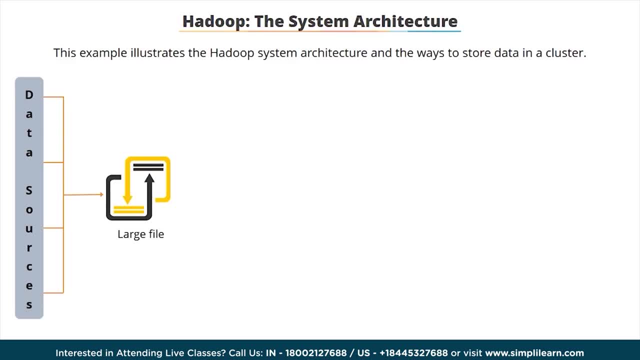 large file, usually greater than 100 megabytes, gets routed from a name node to data nodes. Name nodes hold the metadata information about the files stored on data nodes. It stores the address and information of a block of file and the data node associated with it. Data nodes hold the actual data blocks. The file is split. 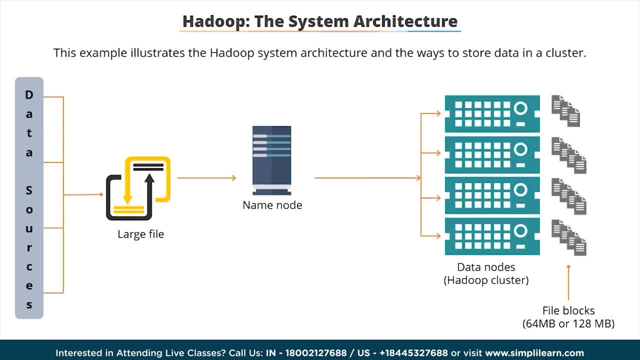 into multiple smaller files, usually of 64 megabytes or 128 megabyte size. It's then copied to multiple physical servers. The smaller files are also called file blocks. One file block gets replicated to different servers. The default replication factor is three, which means a single file block gets copied at least three times on different. 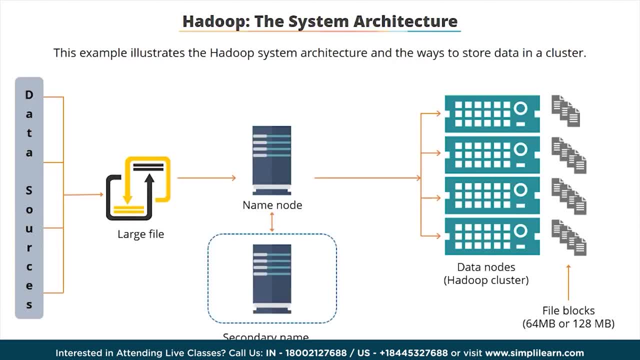 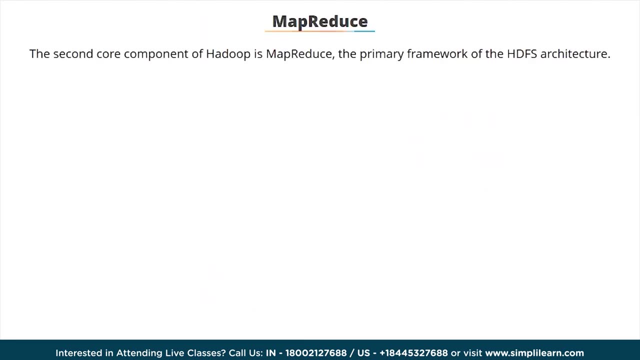 servers or data nodes. There is also a secondary name node which keeps a backup of all the metadata information stored on the main or primary node. This node can be used if and when the main name node fails. Now that you have understood a little about HDFS, let's look at the second core component. 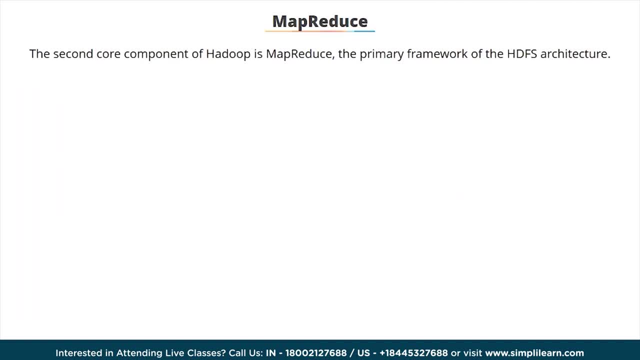 of Hadoop MapReduce, the primary framework of the HDFS. A file is split into three blocks as split0,, split1, and split2.. When a request comes in to retrieve the information, the mapper task is executed on each data node that contains. 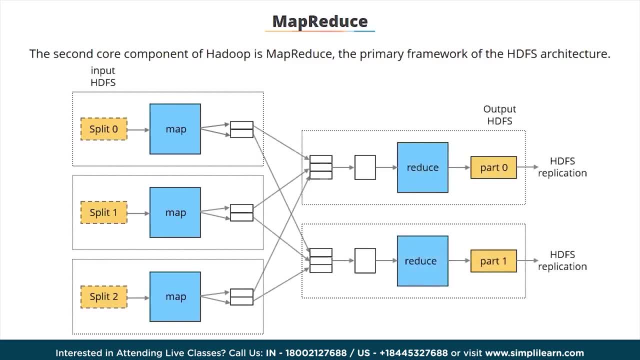 the file blocks. The mapper generates an output, essentially in the form of key-value pairs that are sorted, copied and merged. Once the mapper task is complete, the reducer works on the data and stores the output on HDFS, The MapReduce Process. 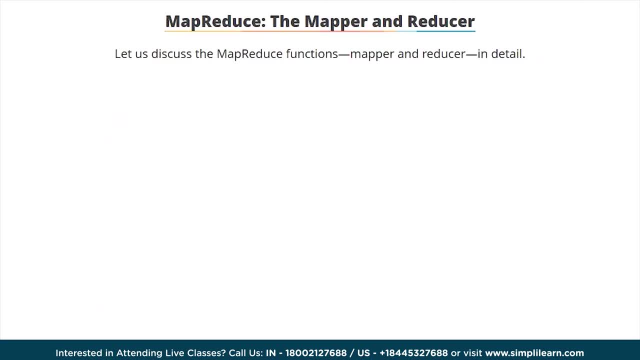 Let's discuss the MapReduce functions- mapper and reducer- in detail. The Mapper, Hadoop, ensures that mappers run locally on the nodes which hold a particular portion of the data. to avoid the network traffic, Multiple mappers run in parallel and each 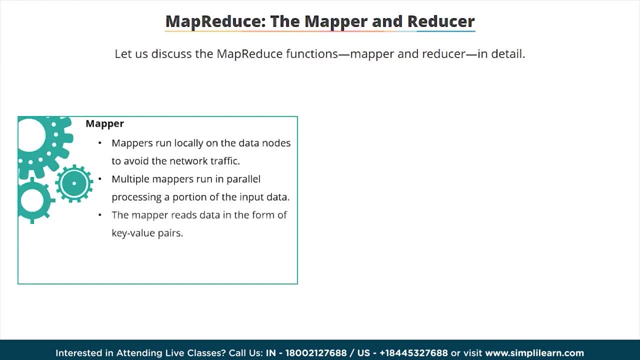 mapper processes a portion of the input data. The input and output of the mapper are in the form of key-value pairs. Note that it can either provide zero or zero-value pairs. The input and output of the mapper are in the form of key-value pairs. Note that it 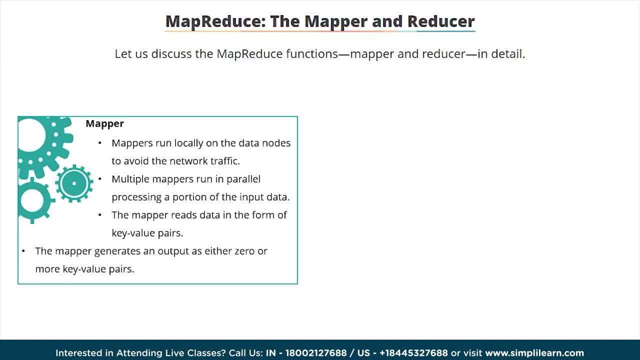 can be read for: provides zero or more key-value pairs as output: The Reducer. After the map phase, all intermediate values for an intermediate key are combined into a list which is given to a reducer. All values associated with a particular intermediate key are directed to the same reducer. This step is known as shuffle and sort. There may 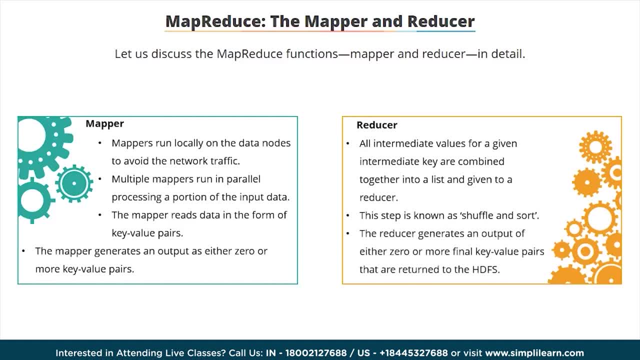 be a single reducer or multiple reducers. Note that the reducer also provides outputs in the form of zero or more than zero, zero or more than one final key value pairs. These values are then returned to HDFS. The reducer usually emits a single key value pair for each input key. 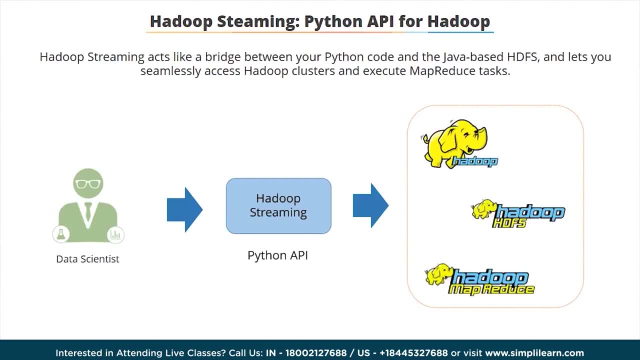 You have seen how MapReduce is critical for HDFS to function. A good thing is you don't have to learn Java or other Hadoop-centric languages to write a MapReduce program. You can easily run such Hadoop jobs with a code completely written in Python with the. 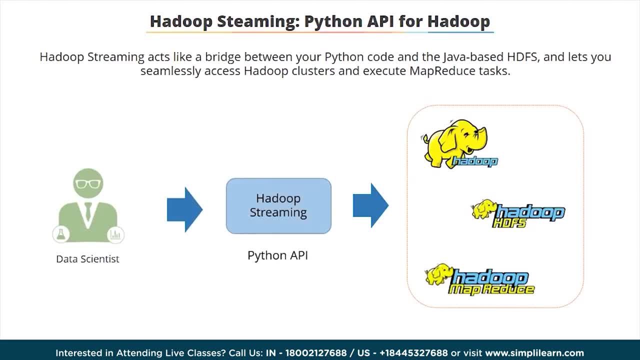 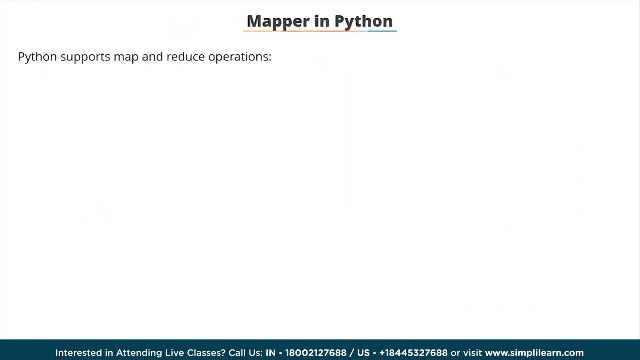 help of Hadoop Streaming API. Hadoop Streaming acts like a bridge between your Python code and the Java-based HDFS and lets you seamlessly access Hadoop clusters and execute MapReduce tasks. You have seen how MapReduce is critical for HDFS to function. 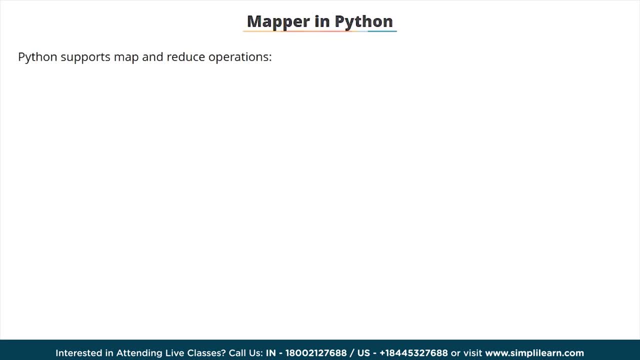 Thankfully, you don't have to learn Java or other Hadoop-centric languages to write a MapReduce program. You can easily run such Hadoop jobs with a code completely written in Python. You can easily run such Hadoop jobs with a code completely written in Python. 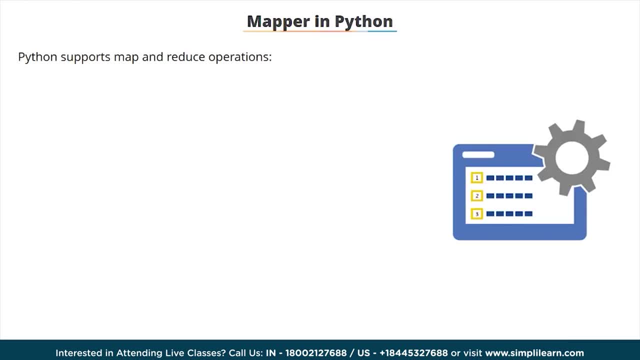 Shown here are some user-friendly Python functions that are written for the Mapper class. Suppose we have the list of numbers we want to square. We have the square function defined as shown on the screen. We can call the map function with the list and the function which is to be executed on. 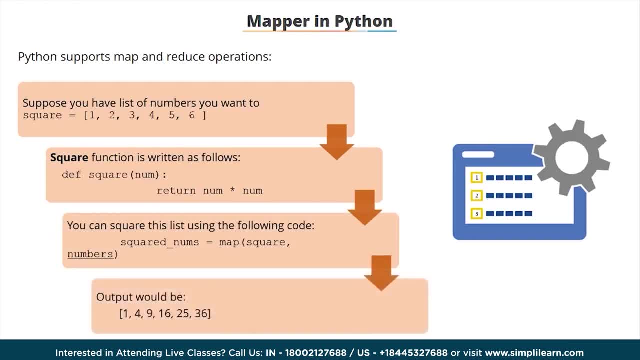 each item in that list. The output of this process is as shown in the map function. This is the map function that is executed on each item in the list. The output of this process is as shown in the map function. This is the map function that is executed on each item in the list. 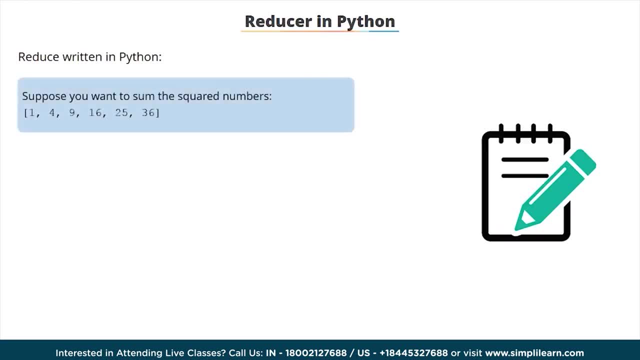 Reducer can also be written in Python. Here we would like to sum the squared numbers of the previous map operation. This can be done using the sum operation as shown on the screen. We can now call the reduce function with the list of data which is to be aggregated and. 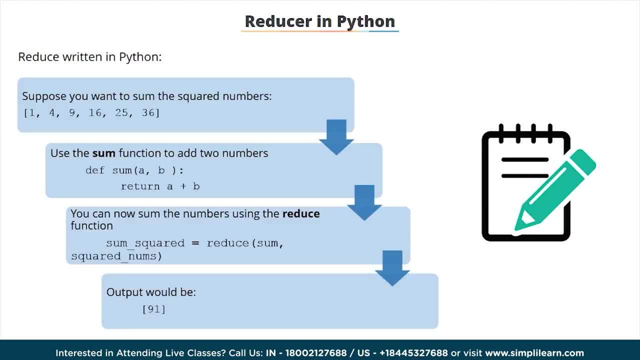 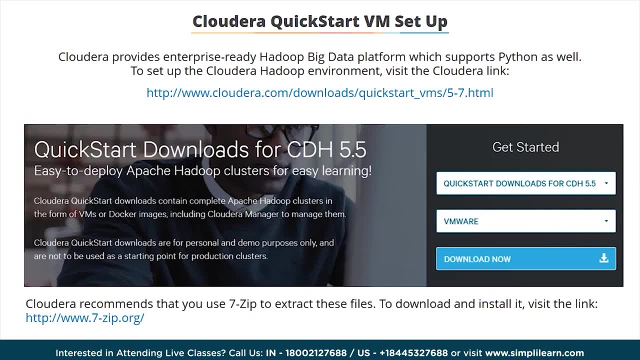 aggregator function is used for this purpose. Big data analysis requires a large infrastructure. Cloudera provides enterprise-ready Hadoop big data platform which supports Python as well. To execute Hadoop jobs, you have to first install Cloudera. It's preferable to install Cloudera's virtual machine on a Unix system, as it functions best on it. 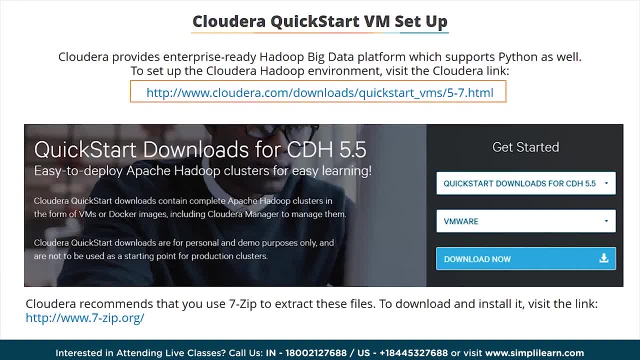 To set up the Cloudera Hadoop environment, visit the Cloudera link shown here. Select Quick Start Download for CDH 5.5 and VMware from the drop down lists. Click the Download Now button. Once the VM image is downloaded, please use 7-Zip to extract the files. 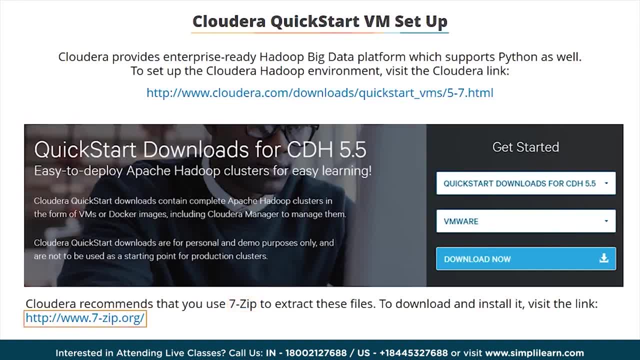 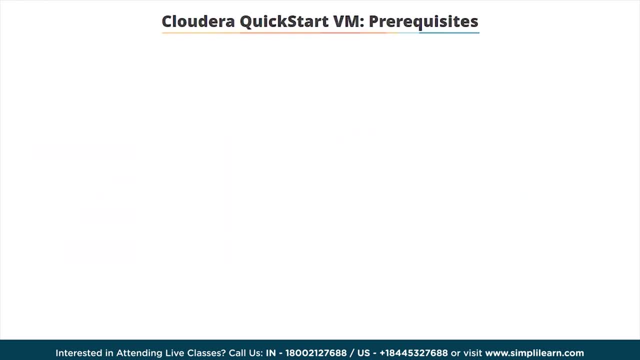 To download and install it, visit the link shown on screen. Cloudera VMware has some system prerequisites. The 64-bit virtual machine requires a 64-bit host operating system or OS and a virtualization product that can support a 64-bit guest OS. 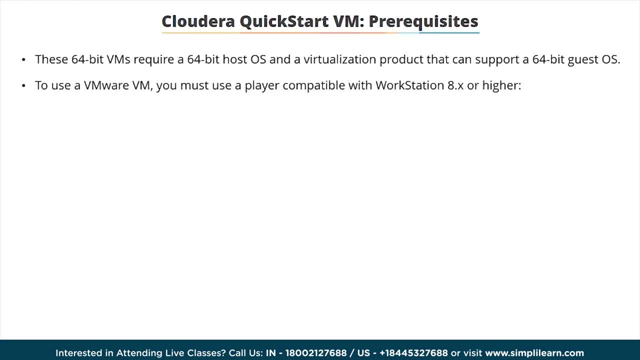 To use a VMware VM, you must use a player compatible with Workstation 8.x or higher, such as Player 4.x or higher or Fusion 4.x or higher. You can use older versions of Workstation to create a new VM using the same virtual disk or VMDK file. 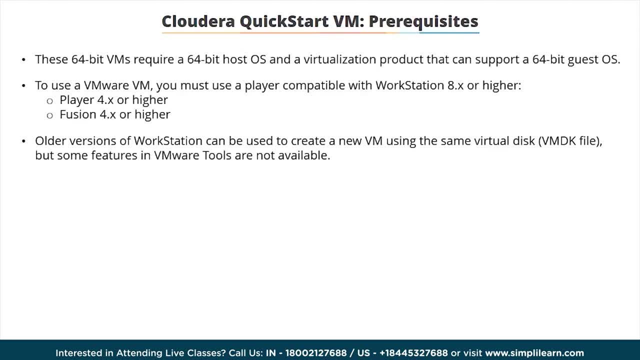 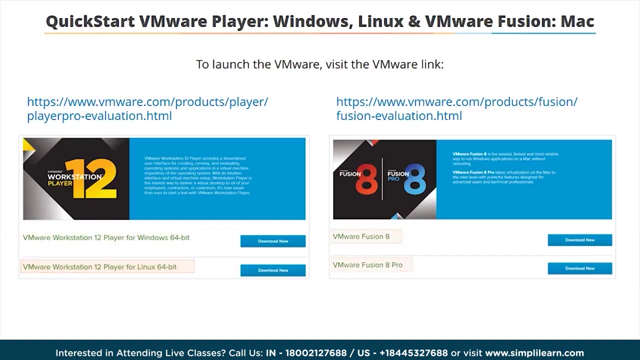 But some features in VMware Tools will be unavailable. The amount of RAM required will vary depending on the runtime option you choose. To launch the VMware Player, you will either need VMware Player for Windows and Linux or VMware Fusion for Mac. So please visit the VMware link shown on screen to download the relevant VMware Player. 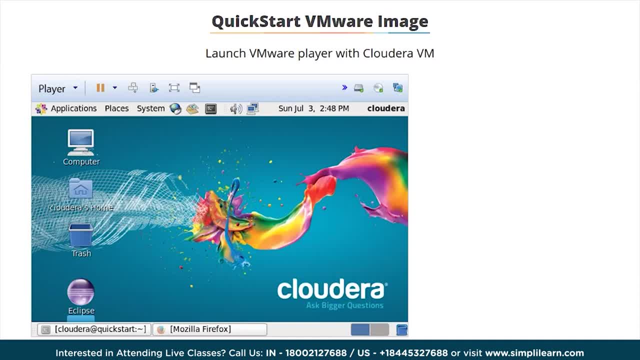 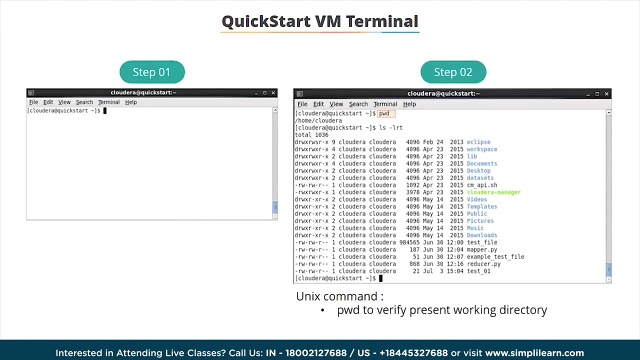 Now launch the VMware Player with the Cloudera VM. The default username and password is Cloudera. Click the Terminal icon as shown here. It will launch the Unix Terminal for Hadoop HDFS interaction. To verify that the Unix Terminal is functioning correctly, type in pwd, which will show you the present working directory. 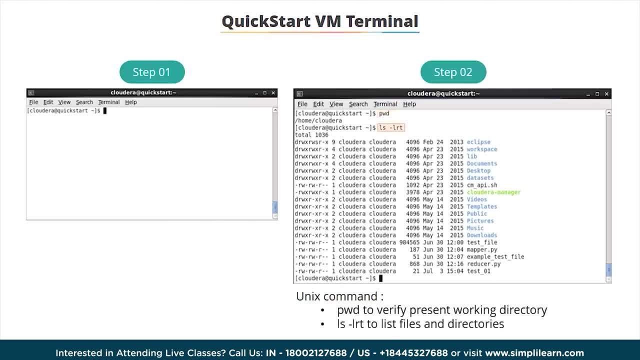 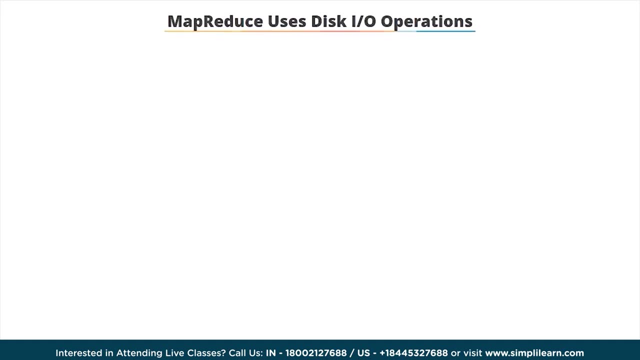 You can also type in ls space hyphen lrt to list all the current files, Folder, Folders and directories. These are some simple Unix commands which will come in handy later while you are implementing MapReduce tasks. You have seen how the Hadoop distributed file system works along with MapReduce. 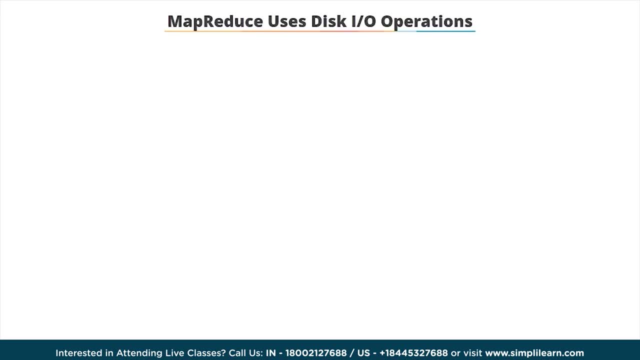 The data is written on and read by disks. MapReduce jobs require a lot of disk read and write operations, which is also known as disk IO or input and output. Reading and writing to a disk is not just expensive, It can also be slow. 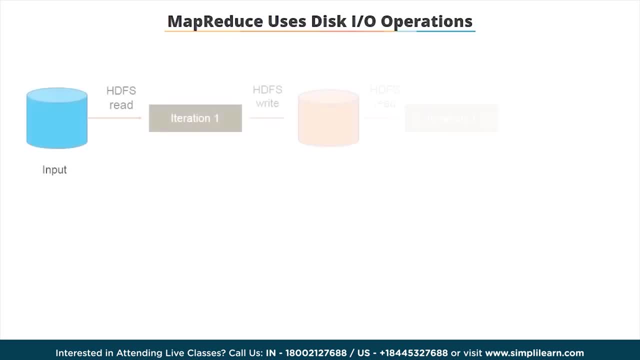 And impact the entire process and operation. This is specifically true for iterative processes. Hadoop is built for write once read many type of jobs, Which means it's best suited for jobs that don't have to be updated or accessed frequently, But in several cases, particularly in analytics and machine learning, users need to write and rewrite commands to access and compute on the same data more than once. 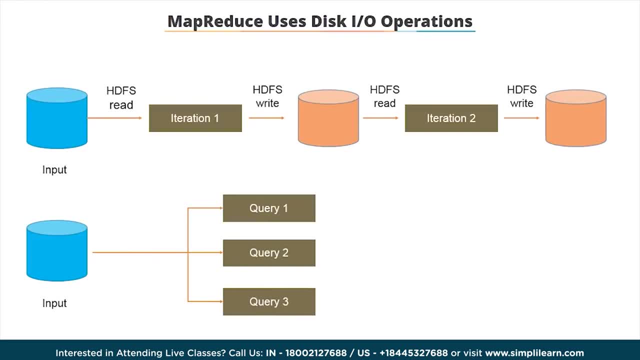 Every time such a request is sent out. MapReduce. MapReduce requires that data is read and or written onto disks directly. Note that, though the time to access or write on disks is measured in milliseconds, when you are dealing with large file sizes, the time factor gets compounded significantly. 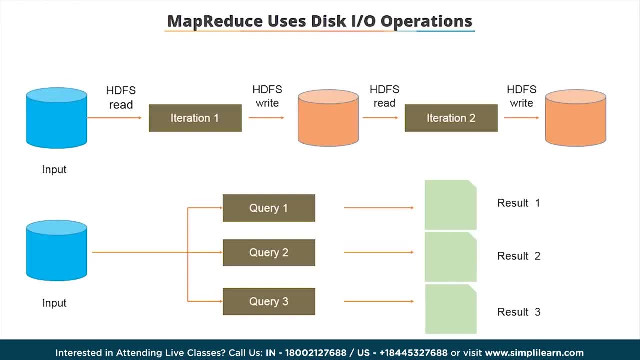 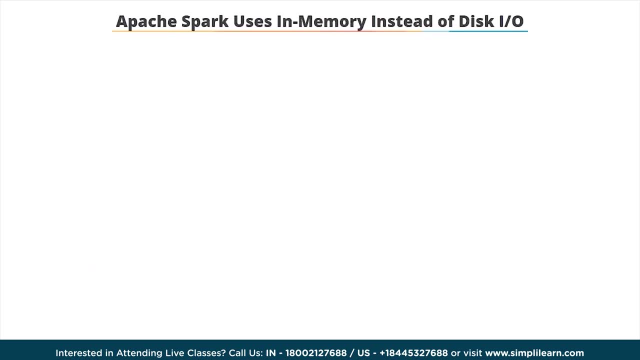 This makes the process highly time consuming. In contrast, Apache Spark uses resilient distributed data sets, or RDDs, to carry out such computations. RDDs allow data to be read and written on disks. RDDs allow data to be stored in memory, Which means that every time users want to access the same data, a disk IO operation is not required. 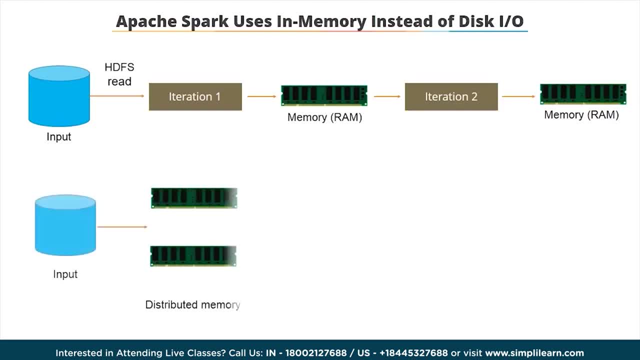 They can easily access data stored in the cache. Accessing the cache, or RAM, is much faster than accessing disks. For instance, if disk access is measured in milliseconds, in-memory data access is measured in sub-milliseconds. This radically reduces the overall time taken for iterative operations on large data sets. 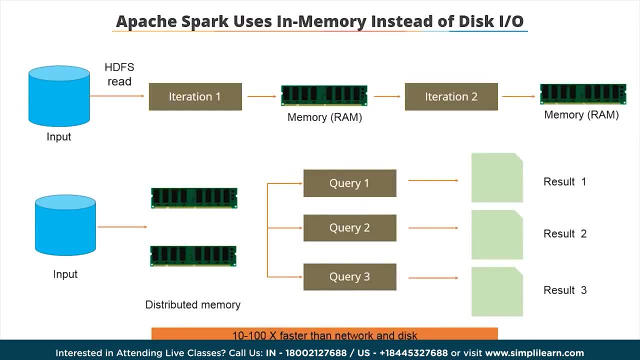 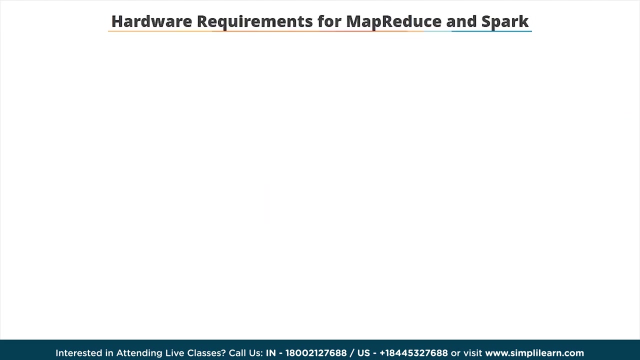 In fact, programs on Spark run at least 10 to 100 times faster than on MapReduce. That's why Spark is gaining popularity among most data scientists, as it is more time efficient when it comes to running analytics and machine learning computations. One of the main differences in terms of hardware requirements for MapReduce and Spark is that, while MapReduce requires a lot of servers and CPUs, 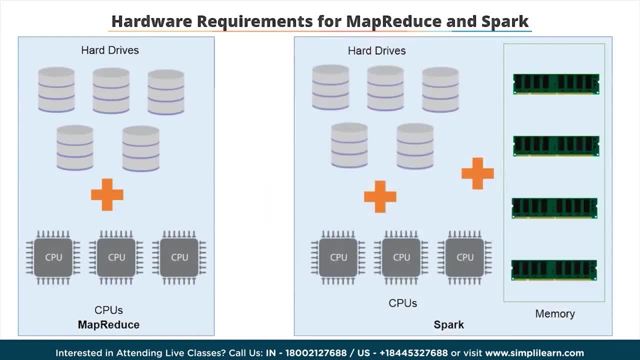 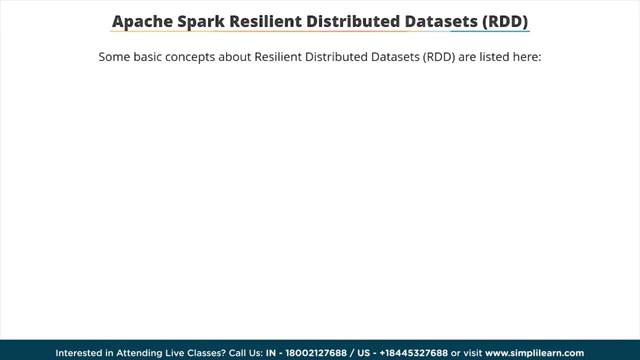 Spark additionally requires a lot of CPUs and CPUs. Spark additionally requires a large and efficient RAM. Let's understand resilient distributed data sets in detail. As you have already seen, the main programming approach of Spark is RDD. RDDs are fault-tolerant collections of objects spread across a cluster that you can operate on in parallel. 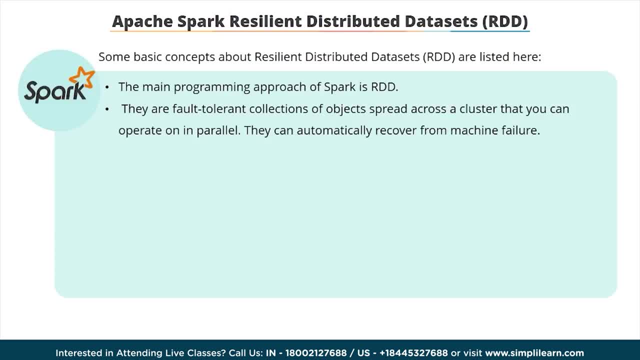 They are called fault-tolerant because they can automatically recover from machine failure. You can create an RDD Either by copying the elements from an existing collection or by referencing a data set stored externally, say on an HDFS. RDDs support two types of operations: transformation and actions. 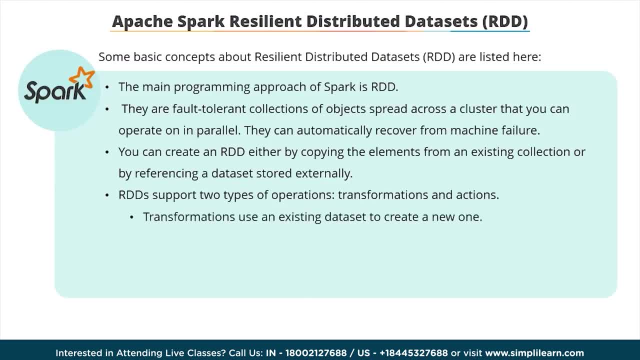 Transformations use an existing data set to create a new one. For Example, Map creates a new RDD containing the results after passing the elements of the original dataset through a function. Some other examples of Transformations are: Filter and Join Actions, compute on the dataset and return the value to the driver program. 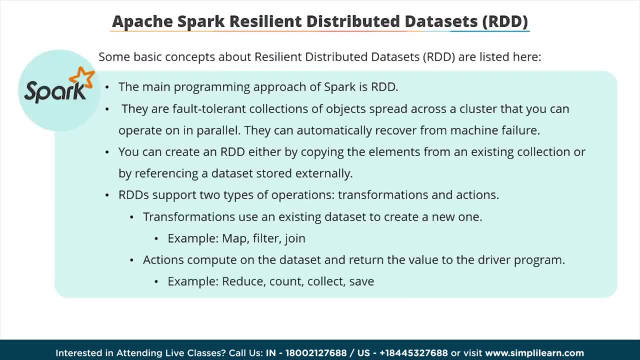 For example, reduce, aggregates all the RDD elements using a specified function and returns this value to the driver program. Some other examples of actions are count, collect and save. It's important to note that if the available memory is insufficient, then Spark writes the data to disk. 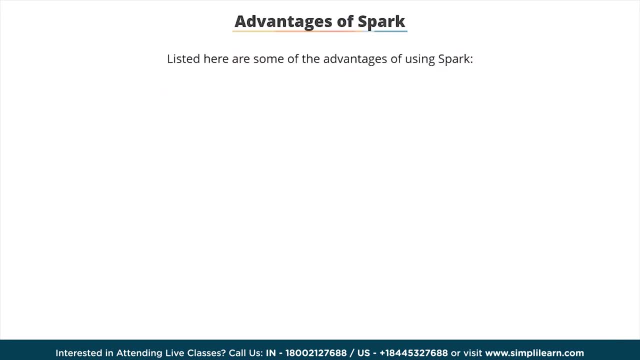 Here are some of the advantages of using Spark: It's almost 10 to 100 times faster than Hadoop MapReduce. It has a simple data processing framework. It provides interactive APIs for Python that allow faster application development. It has multiple tools for complex analytics operations. 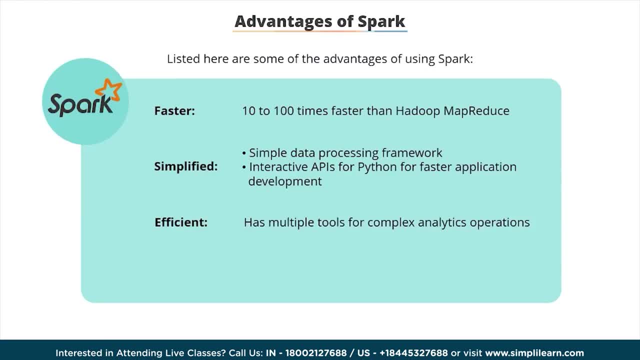 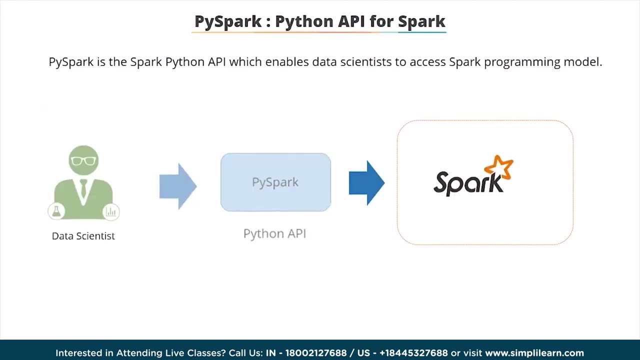 These tools help data scientists perform machine learning and other analytics much more efficiently and easily than most existing tools. Thank you for watching. It can easily be integrated with the existing Hadoop infrastructure. PySpark is the Python API used to access the Spark programming model and perform data analysis. 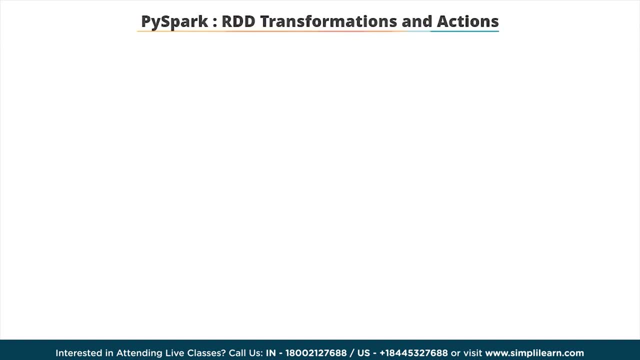 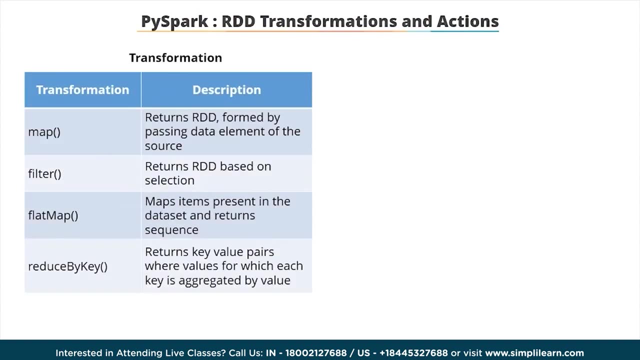 Let's take a look at some transformation functions and action methods which are supported by PySpark for data analysis. These are some common transformation functions: Map Returns- RDD formed by passing data elements from the source dataset. Filter Returns- RDD based on selected criteria. 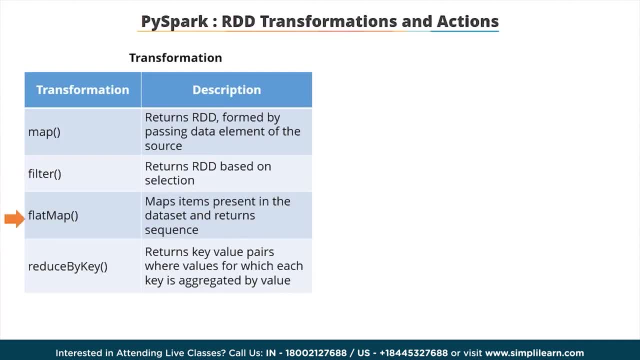 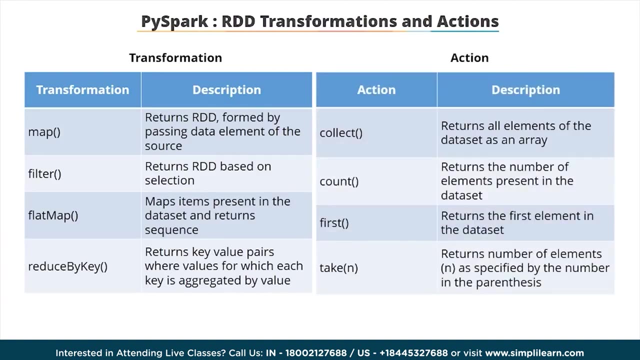 FlatMap Maps items present in the dataset and returns a sequence. ReduceByKey Returns key-value pairs where values for each key is aggregated by a given reduce function. Let's now look at some common action functions. Collect Returns all elements of the dataset as an array. 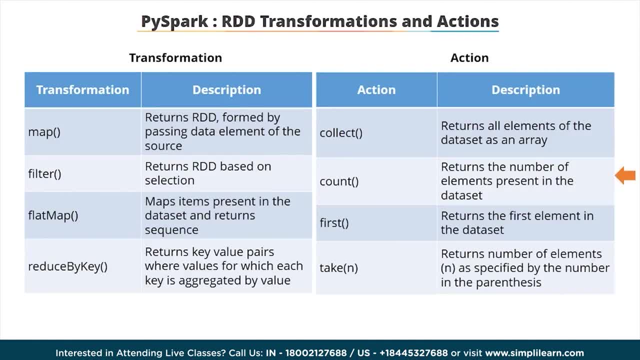 Count Returns the number of elements present in the dataset First Returns the first element in the dataset Take Returns the number of elements as specified by the number in the parentheses. SparkContext or SC is the entry point to Spark for the Spark application. 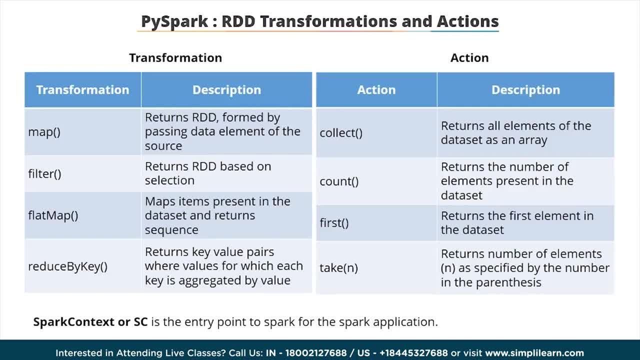 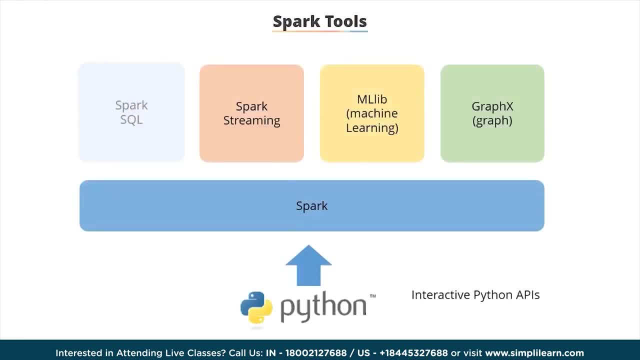 and must be available at all times for data processing. There are mainly four components in Spark tools: SparkSQL. It's mainly used for querying the data stored on HDFS as a resilient distributed dataset, or RDD, in Spark through integrated APIs in Python, Java and Scala. 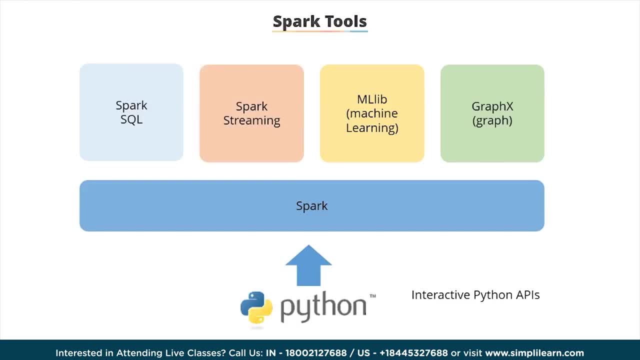 SparkStreaming. It's very useful for data streaming process and where data can be read from various data sources. MLlib: It's mainly used for machine learning processes, such as supervised and unsupervised learning. GraphX: It can be used to process or generate graphs with RDDs. 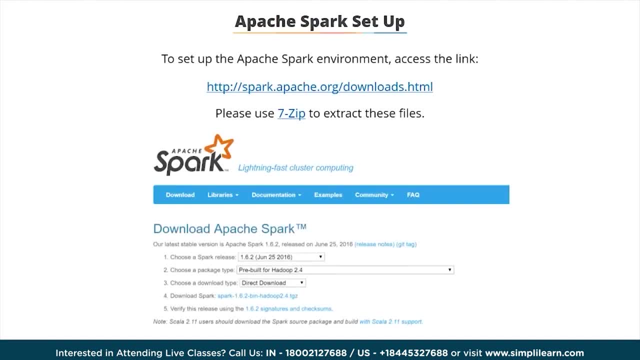 Let's set up the Apache Spark environment and also learn how to integrate Spark with Jupyter Notebook. First Visit the Apache link and download Apache Spark to your system. Now Use 7-zip software and extract the files to your system's local directory. 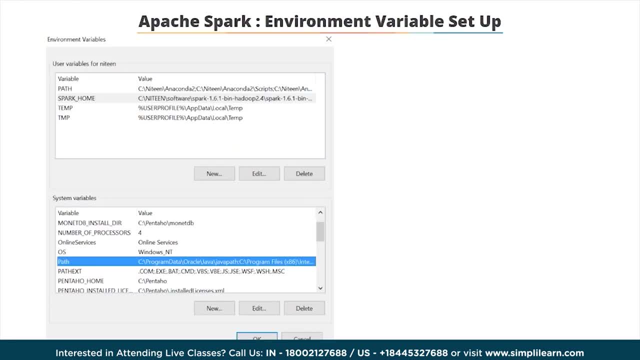 To set up the environment variables for Spark, first set up the user variables, Click New and then enter Spark Home in the variable name and enter the Spark installation path as variable value. Now Click on the path and then click New and enter the Spark bin path from the installed directory location. 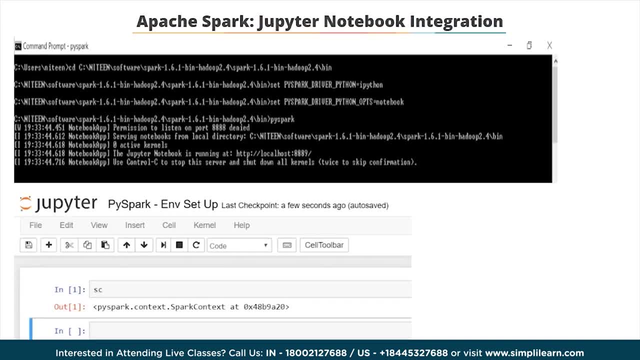 Now Let's set up the PySpark Notebook specific variables. This will integrate the Spark engine with Jupyter Notebook Type in PySpark. It will launch a Jupyter Notebook after a while. Create a Python notebook and type in sc command to check the Spark context. 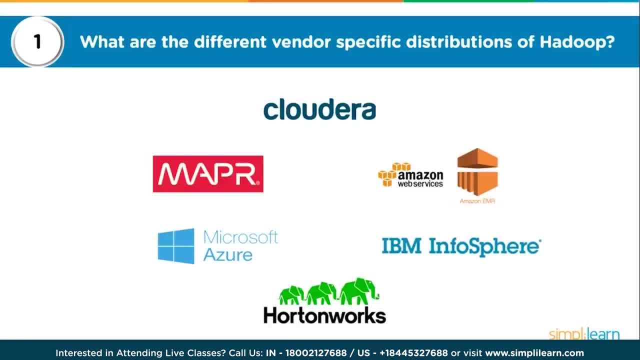 Now All of you might be aware that Hadoop or Apache Hadoop is the core distribution of Hadoop. And then you have different vendors in the market which have packaged the Apache Hadoop in a cluster management solution which allows everyone to easily deploy, manage, monitor, upgrade your clusters. 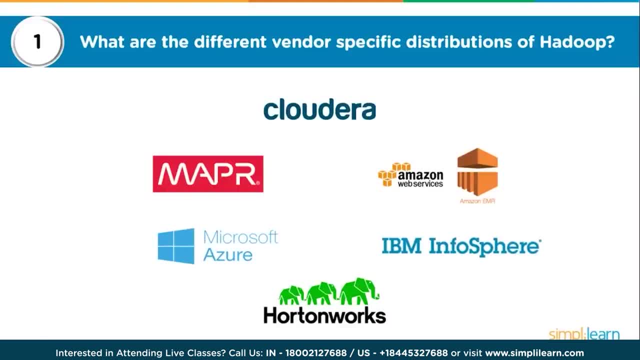 So here are some vendor specific distributions. We have Cloudera, which is the dominant one in the market. We have Hortonworks and Hadoop, And now you might be aware that Cloudera and Hortonworks have merged, So it has become a bigger entity. 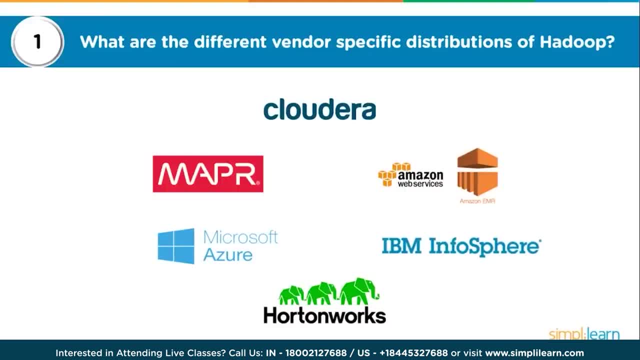 You have MapR, You have Microsoft Azure, IBM's InfoSphere And Amazon Web Services. So these are some popularly known vendor specific distributions. If you would want to know more about the Hadoop distributions, you should basically look into Google and you should check for Hadoop- different distributions- wiki page. 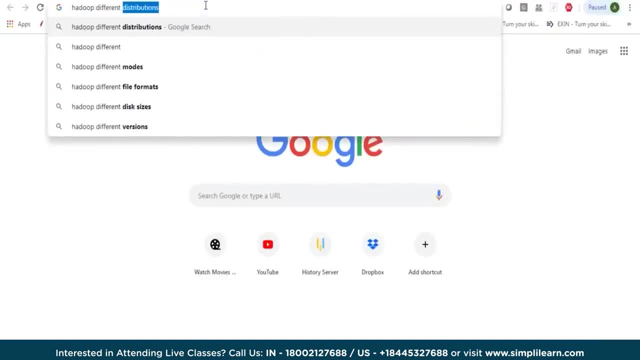 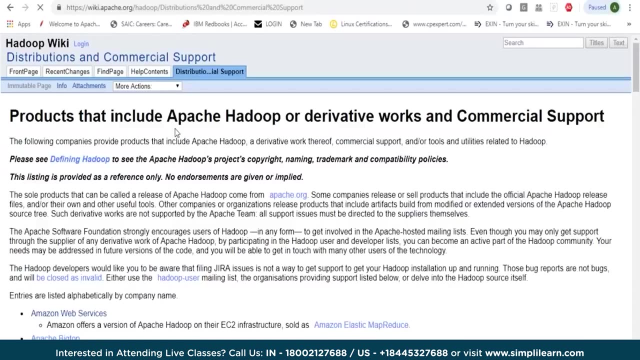 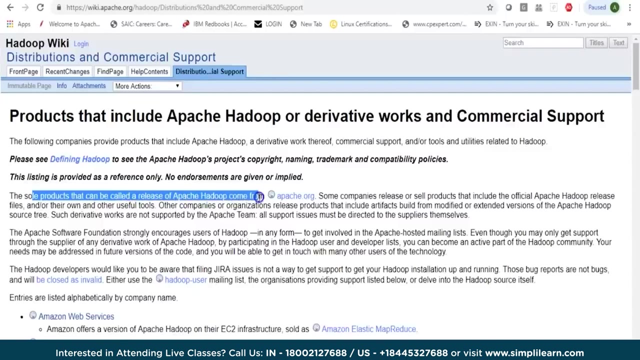 So if I type Hadoop- different distributions And then I check for the wiki page, that will take me to the distributions and commercial support page And this basically says that the sole products that can be called a release of Apache Hadoop come from Apacheorg. 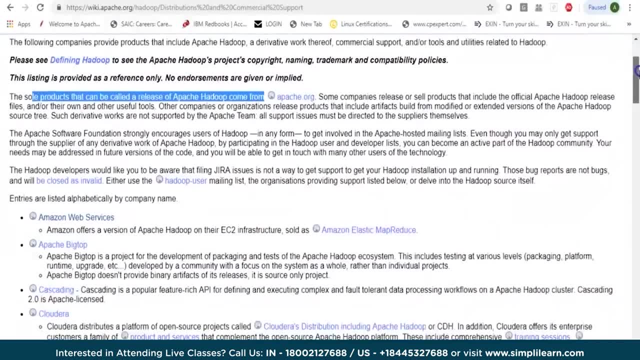 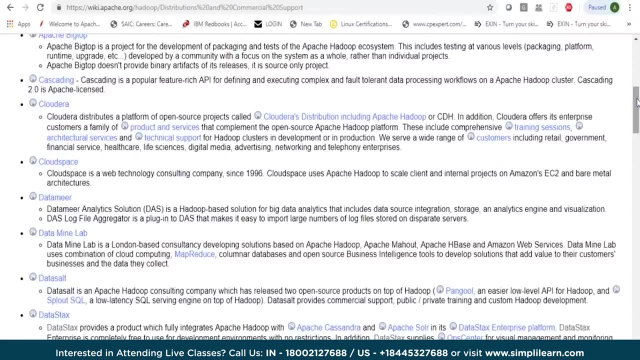 So that's your open source community, And then you have various vendor specific distributions which basically are running in one or the other way: Apache, Hadoop- But they have packaged it as a solution like an installer, So that you can easily set up clusters on set of machines. 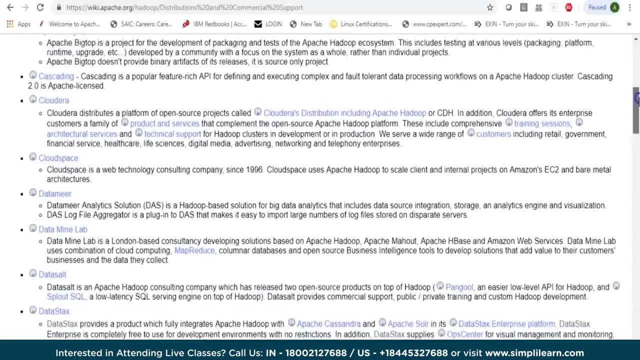 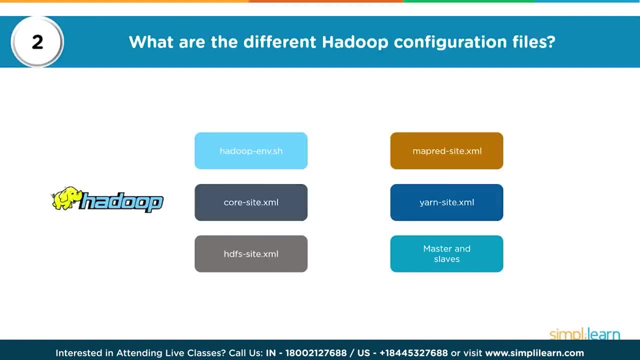 So have a look at this page and read through about different distributions of Hadoop. Coming back, Let's look at our next question. So what are the different Hadoop configuration files Now, whether you're talking about Apache, Hadoop, Cloudera, Hortonworks, MapR or no matter which other distribution. 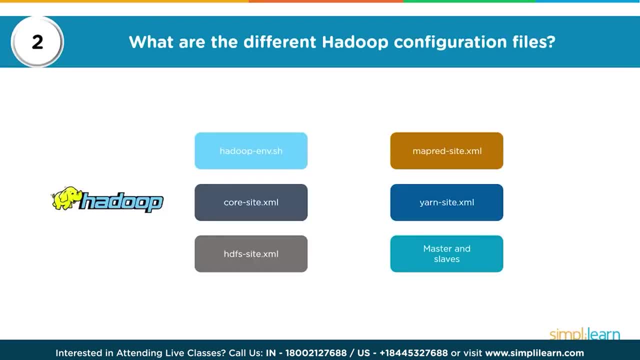 These config files are the most important and existing in every distribution. So you have Hadoop environment dot sh, wherein you will have environment variables such as your Java path, What would be your process ID path, Where will your logs get stored, What kind of metrics will be collected, and so on. 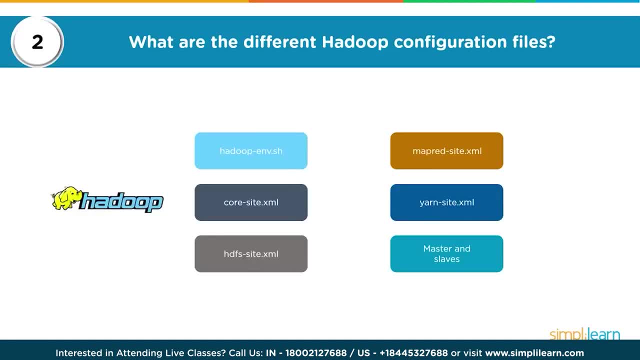 Your core hyphen site file has the HDFS path. Now this has many other properties, like enabling trash or enabling high availability, or discussing or mentioning about your zookeeper, But this is one of the most important file You have: HDFS hyphen site file. 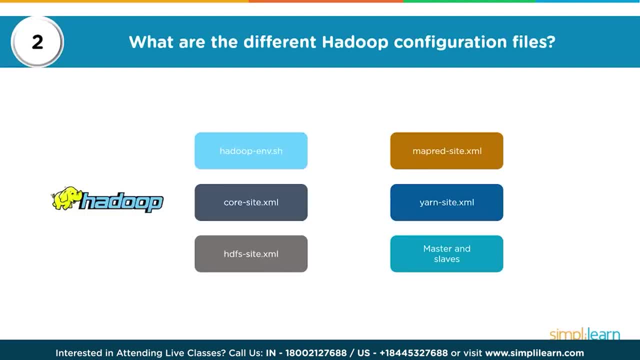 Now this file will have other information related to your Hadoop cluster, Such as your replication factor. Where will name node store its metadata on disk? If a data node is running? where would data node store its data If a secondary name node is running? where would that store a copy of name node's metadata and so on? 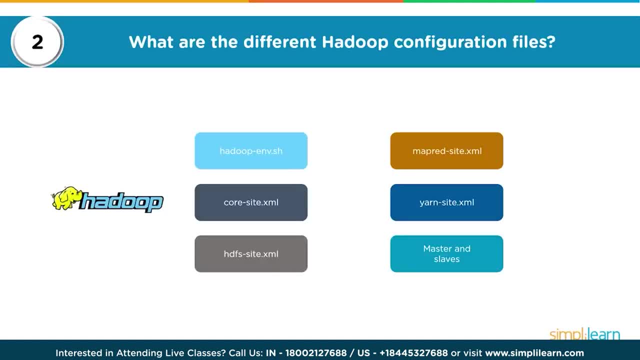 Your MapRed hyphen site file is a file which will have properties related to your MapRed use Processing. You also have masters and slaves. Now these might be deprecated in a vendor specific distribution And in fact, you would have a yarn hyphen site file. 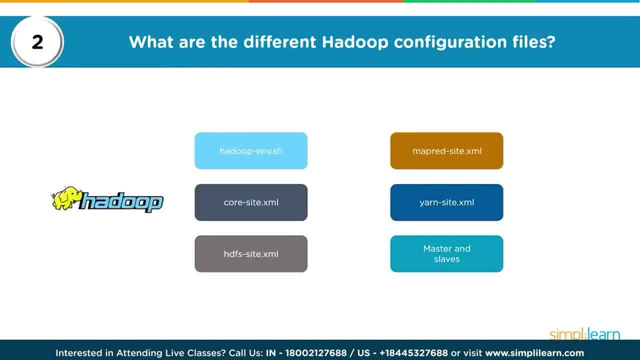 Which is based on the yarn processing framework which was introduced in Hadoop version 2.. And this would have all your resource allocation and resource manager and node manager related properties. Again, if you would want to look at default properties for any one of these, 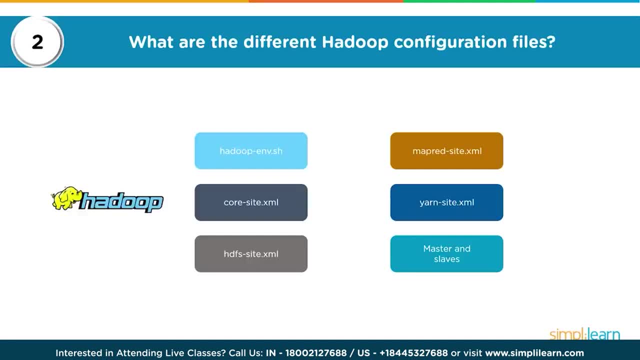 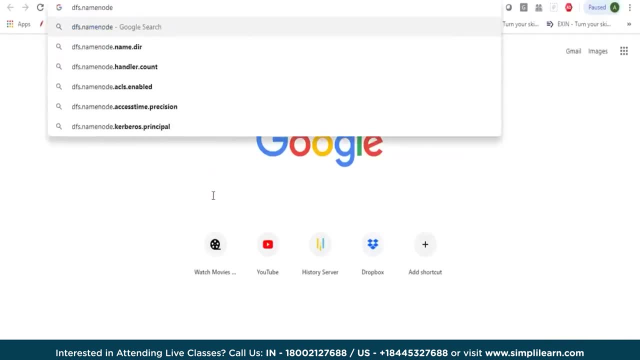 For example, let's say, HDFS hyphen site file. I could just go to Google and type in one of the properties. For example, I would say DFS dot name node, dot name dot directory. And, as I know, this property belongs to HDFS hyphen site file. 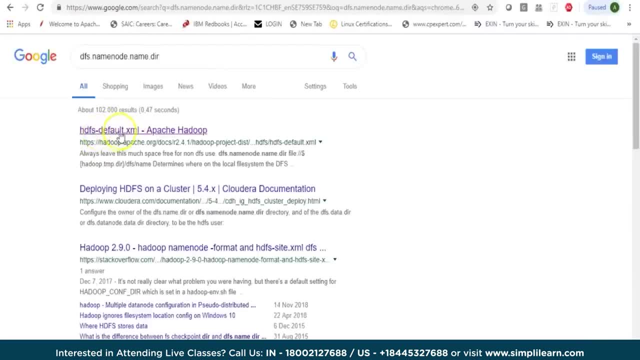 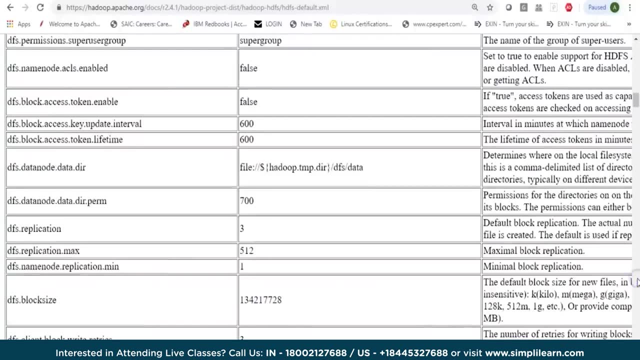 And if you search for this, it will take you to the first link which says HDFS default XML. You can click on this and this will show you all the properties Which can be given in your HDFS hyphen site file. It also shows you which version you are looking at. 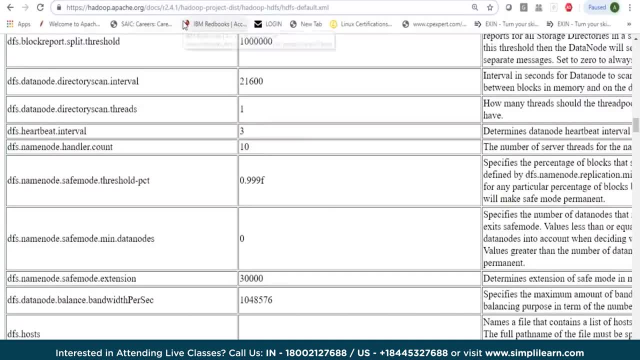 And you can always change the version here. So, for example, if I would want to look at 2.6.5.. I just need to change the version and that should show me the properties. Similarly, you can just give a property which belongs to, say, core hyphen, site file. 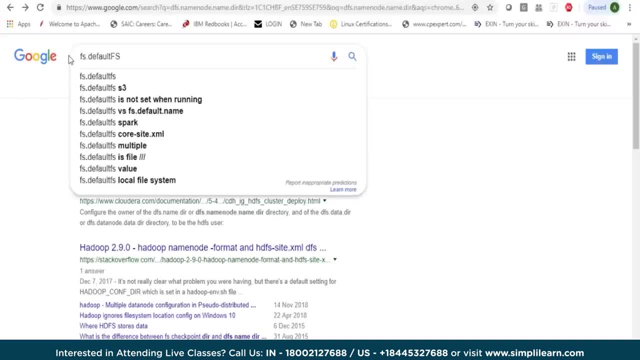 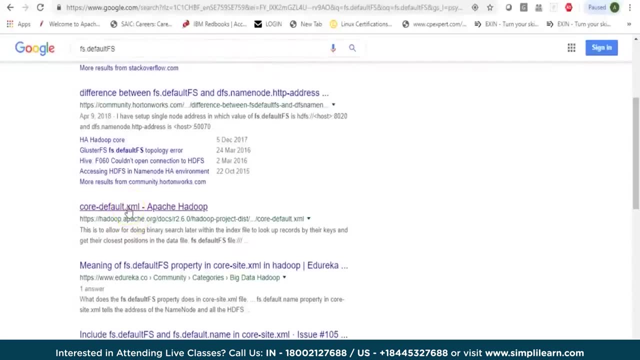 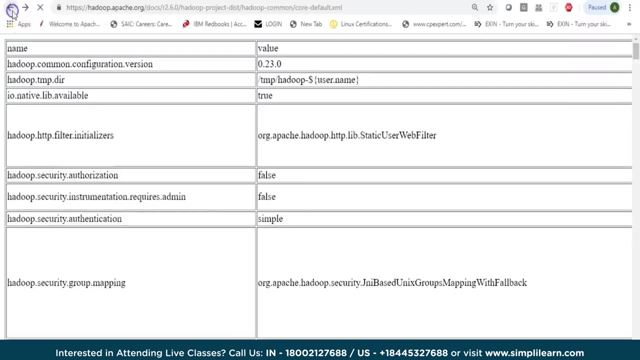 For example, I would say FS dot default FS, And that's a property which is in core hyphen site file And somewhere here you would see core minus default dot XML And this will show you all the properties. So similarly, you could search for properties which are related to yarn hyphen site file or map red hyphen site file. 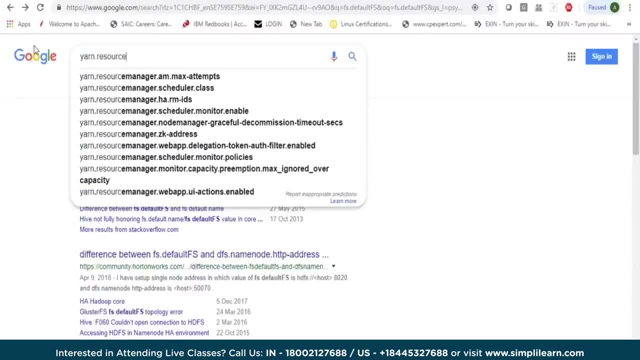 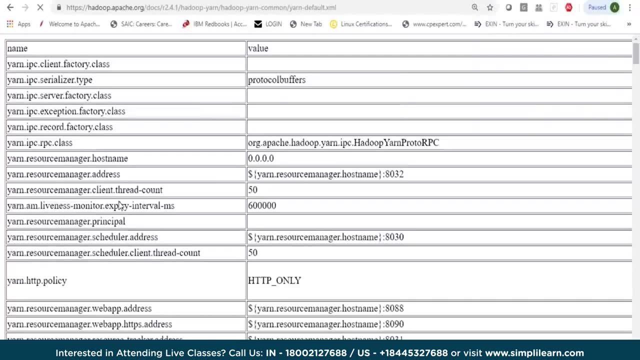 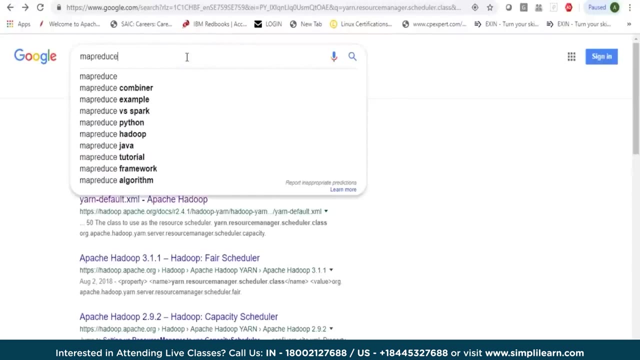 So I could say yarn, dot resource manager And I could look at one of these properties Which will directly take me to yarn default XML And I can see all the properties which can be given in yarn. And similarly you could say map reduce, dot job, dot reduces. 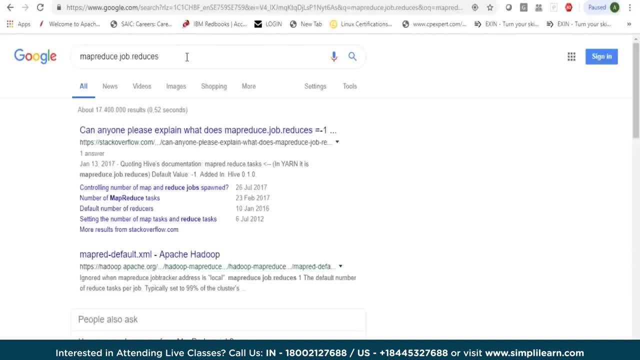 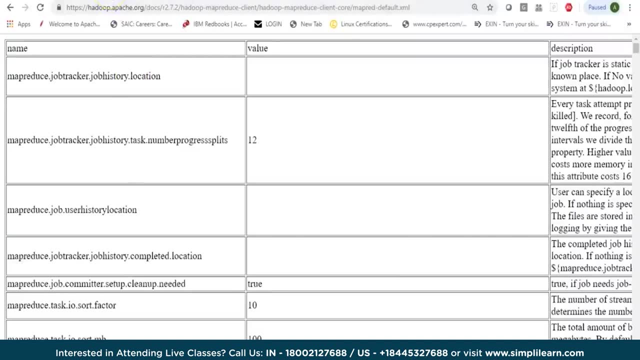 And I know this property belongs to map reduce hyphen site file And this takes you to the default XML. So these are important config files And no matter which distribution of Hadoop you are working on, You should be knowing about these config files. 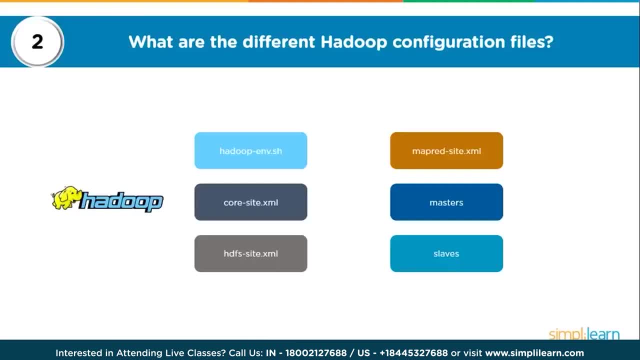 Whether you work as a Hadoop admin or you work as a Hadoop developer, Knowing these config properties would be very important, And that would also showcase your internal knowledge about the configs which drive your Hadoop cluster. Let's look at the next question. 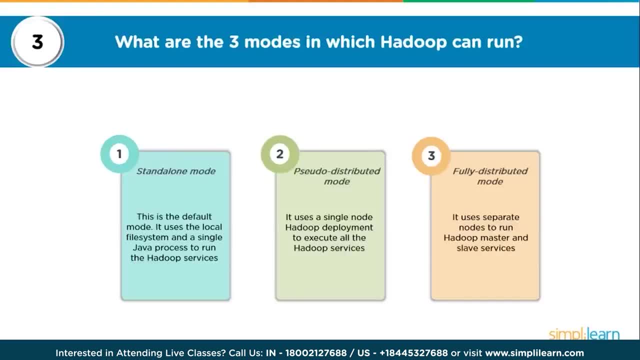 So what are the three modes in which Hadoop can run? So you can have Hadoop running in a standalone mode? Now that's your default mode. It would basically use a local file system and a single Java process. So when you say standalone mode, 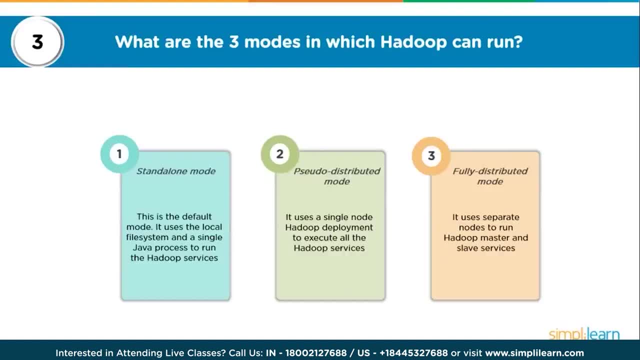 It is as you downloading Hadoop related package on one single machine, But you would not have any process running. That would just be to test Hadoop functionalities. You could have a pseudo distributed mode Which basically means it's a single node Hadoop deployment. 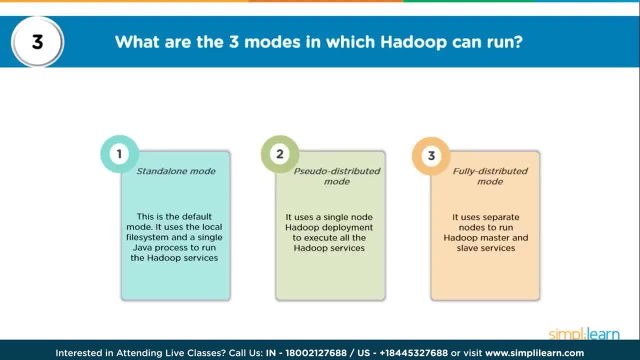 Now Hadoop as a framework has many, many services, So it has lot of services, And those services would be running irrespective of your distribution And each service would then have multiple processes. So your pseudo distributed mode is a mode of cluster where you would have all the important processes. 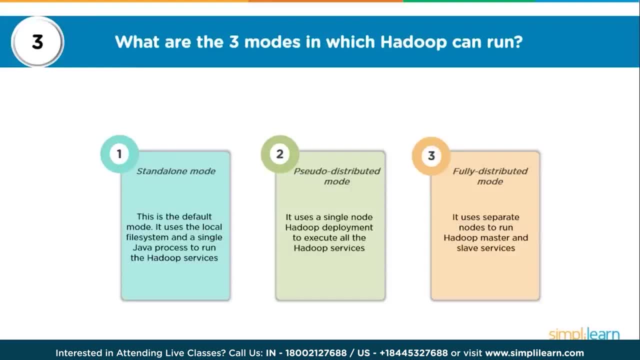 Belonging to one or multiple services Running on a single node. If you would want to work on a pseudo distributed mode And using a Cloudera, You can always go to Google and search for Cloudera's Quick Start VM. 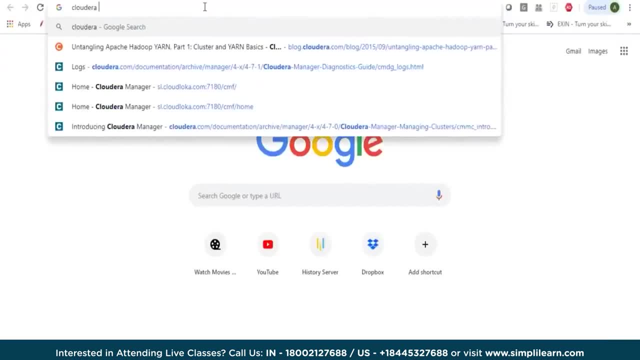 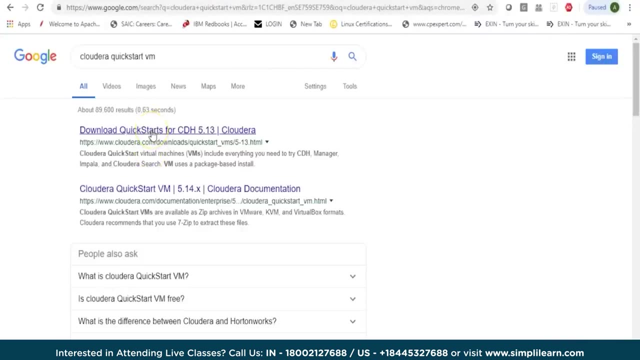 You can download it by just saying Cloudera, Quick Start VM And you can search for this And that will allow you to download a Quick Start VM. Follow the instructions And you can have a single node Cloudera cluster running on your virtual machines. 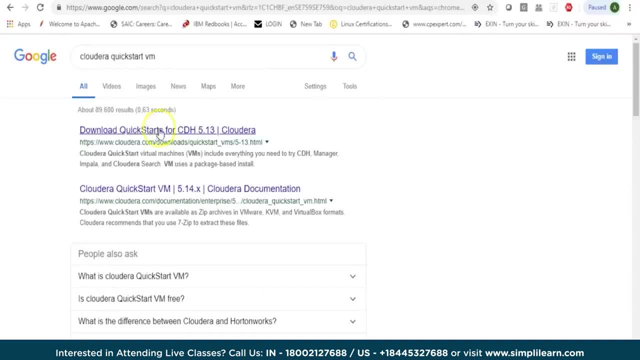 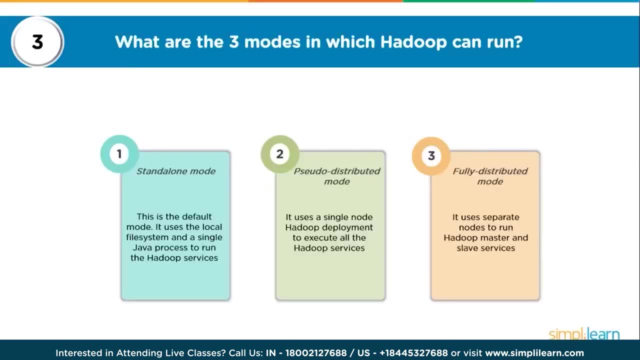 For more information, You can refer to the YouTube tutorial, Where I have explained about how to set up a Quick Start VM. Coming back, You could have, finally, a production setup Or a fully distributed mode, Which basically means that your Hadoop framework and its components would be spread across multiple machines. 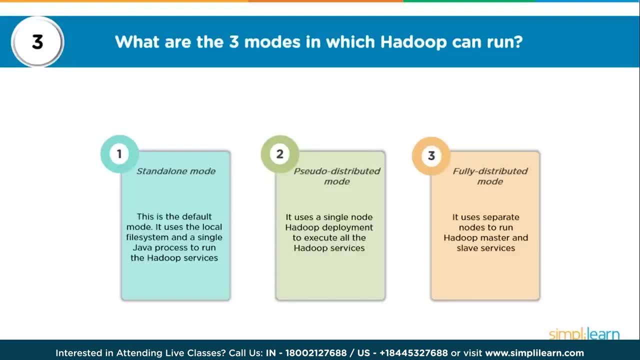 So you would have multiple services, Such as HDFS, Yarn, Flume, Scoop, Kafka, HBase, Hive, Impala, And for these services There would be one or multiple processes distributed across multiple nodes. So this is normally what is used in production environment. 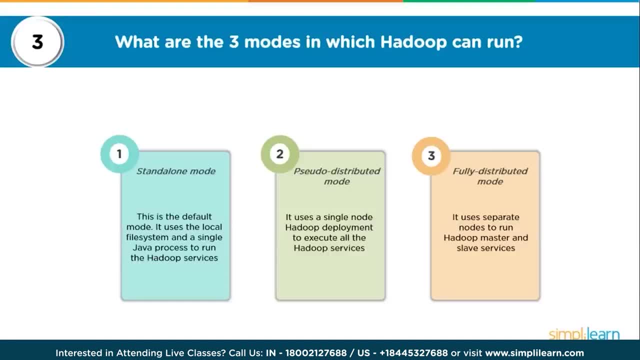 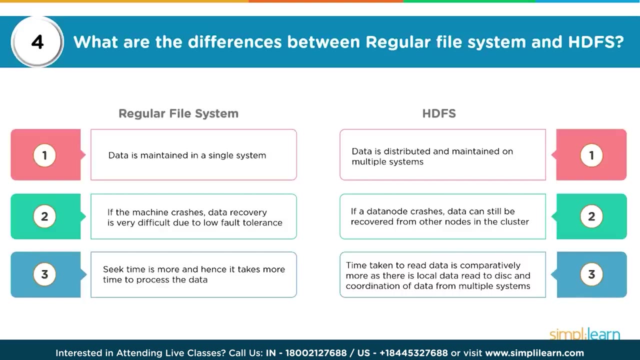 So you could say: standalone would be good for testing, Pseudo distributed could be good for testing and development, And fully distributed would be mainly for your production setup. Now, What are the differences between regular file system and HDFS? So when you say regular file system, 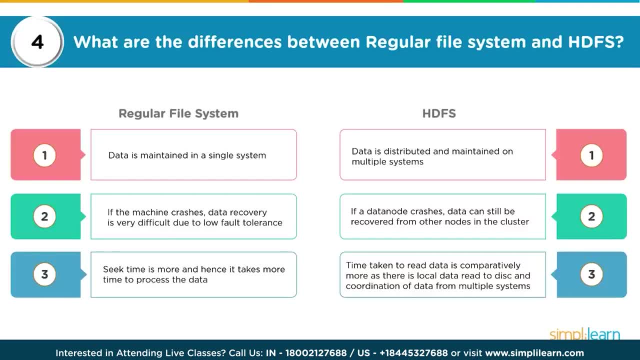 You could be talking about a Linux file system, Or you could be talking about a Windows based operating system. So in regular file system We would have data maintained in a single system. So the single system is where you have all your files and directories. 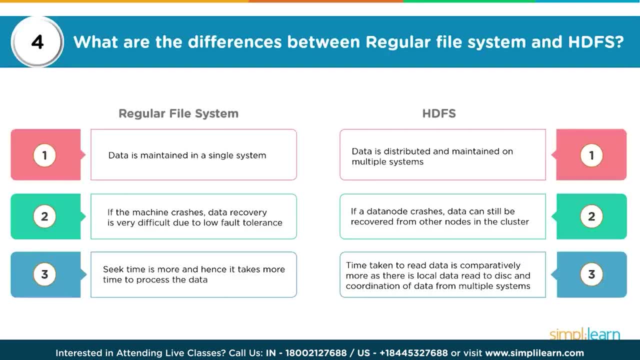 So it is having low fault tolerance, Right. So if the machine crashes, Your data recovery would be very difficult Unless and until you have a backup of that data That also affects your processing. So if the machine crashes Or if the machine fails, 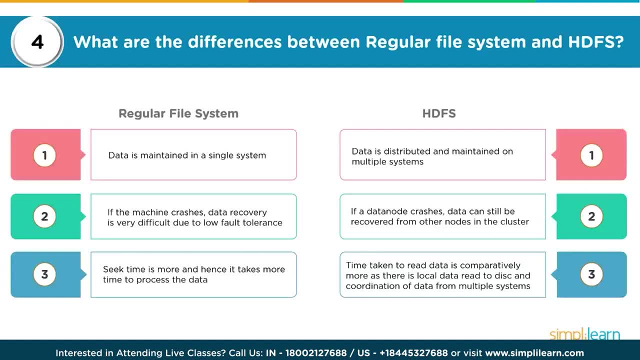 Then your processing would be blocked. Now the biggest challenge with regular file system is the seek time, The time taken to read the data. So you might have one single machine with huge amount of disks And huge amount of RAM, But then the time taken to read that data. 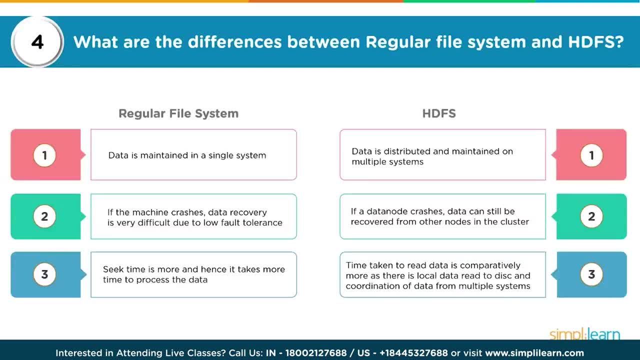 When all the data is stored in one machine Would be very high And that would be with least fault tolerance. If you talk about HDFS, Your data is distributed, So HDFS stands for Hadoop, Distributed File System. So here your data is distributed. 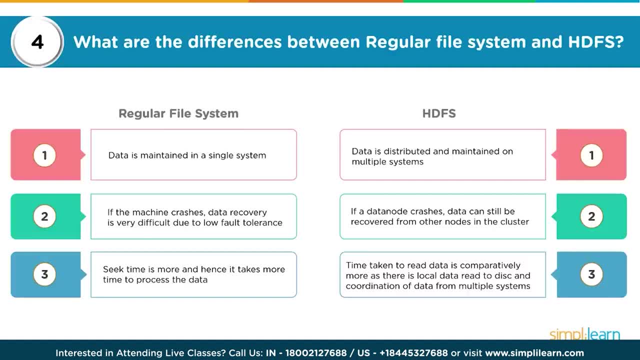 And maintained on multiple systems, So it is never one single machine. It is also supporting reliability. So whatever is stored in HDFS, Say, a file being stored Depending on its size Is split into blocks, And those blocks will be spread across multiple nodes. 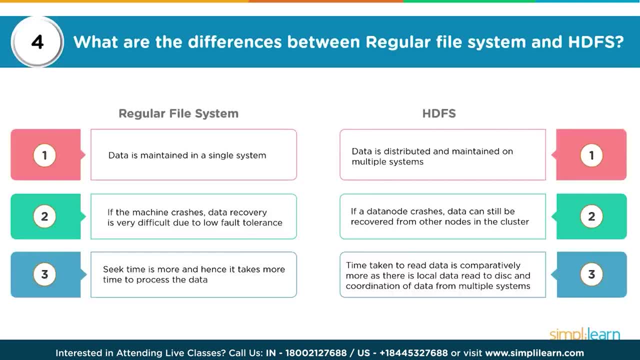 Not only that, Every block which is stored on a node Will have its replicas stored on other nodes. Replication factor depends, But this makes HDFS more reliable In cases of your slave nodes or data nodes crashing. You will rarely have data loss. 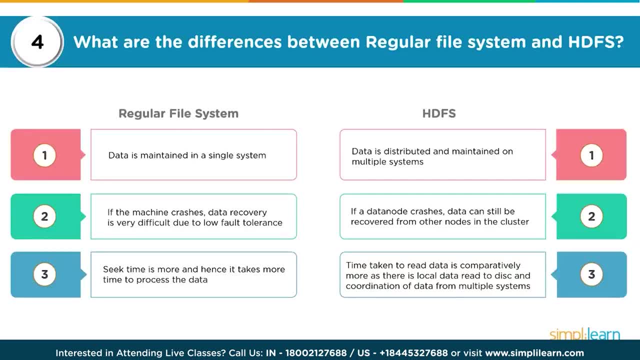 Because of auto replication feature. Now time taken to read the data Is comparatively more, As you might have situations where Your data is distributed across the nodes And even if you are doing a parallel read, Your data read might take more time. 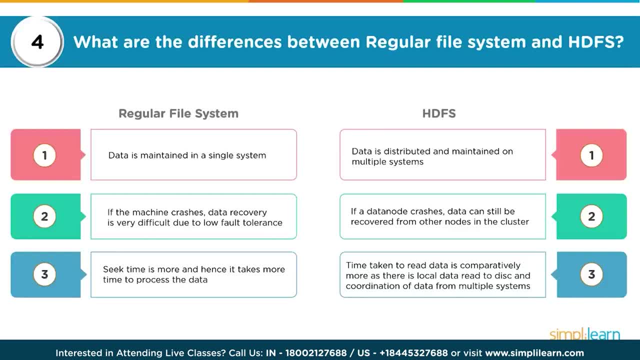 Because it needs coordination from multiple machines. However, if you are working with huge data Which is getting stored, It will still be beneficial In comparison to reading from a single machine, So you should always think about its reliability Through auto replication feature. 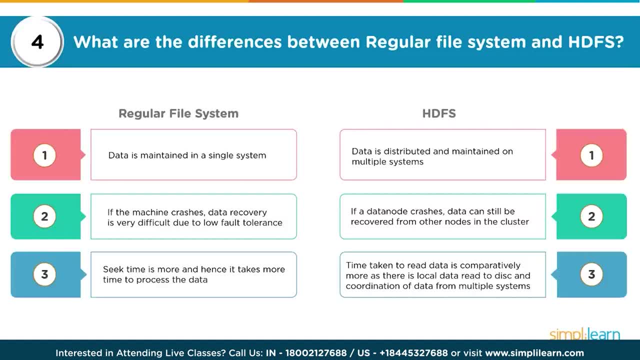 Its fault tolerance, Because of your data getting stored across multiple machines, And its capability to scale. So when you talk about HDFS, We are talking about horizontal scalability, Or scaling out. When you talk about regular file system, You are talking about vertical scalability. 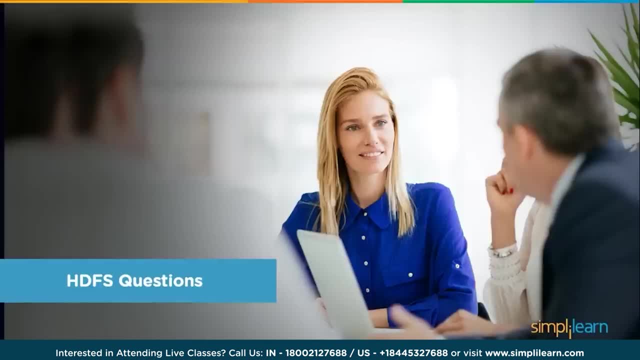 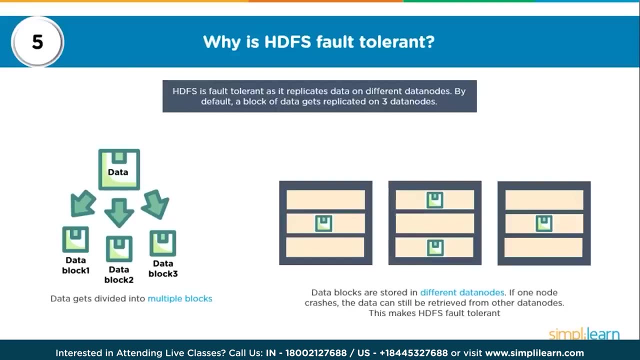 Which is scaling up. Now let's look at some specific HDFS questions. What is this? Why is HDFS fault tolerant? Now, as I just explained in previous slides, Your HDFS is fault tolerant As it replicates data On different data nodes. 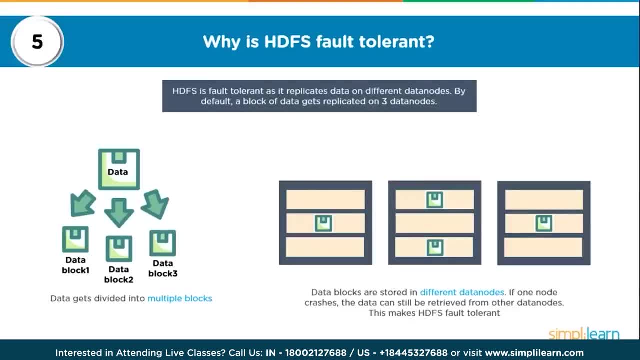 So you have a master node And you have multiple slave nodes Or data nodes, Where actually the data is getting stored. Now we also have A default block size of 128 MB. That's the minimum Since Hadoop version 2.. 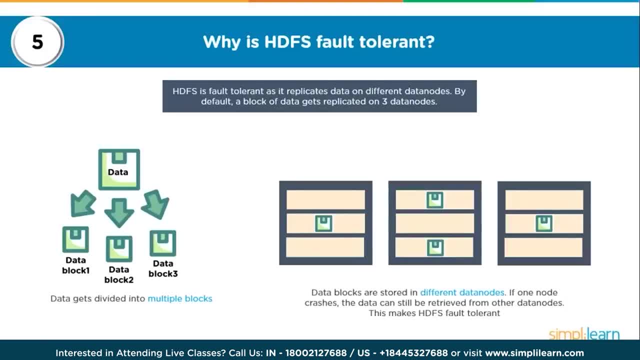 So any file which is up to 128 MB Would be using one logical block, And if the file size is bigger than 128 MB, Then it will be split into blocks And those blocks will be stored across multiple machines. Now, since these blocks are stored across multiple machines, 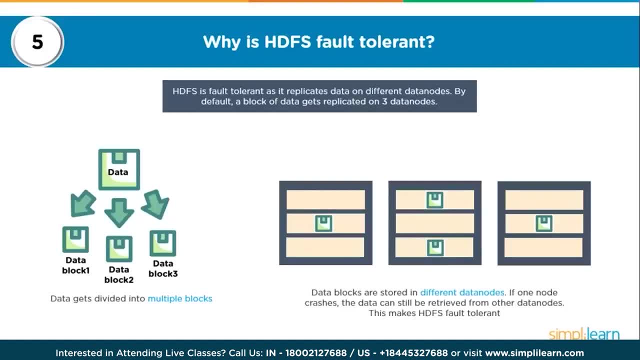 It makes it more fault tolerant, Because even if your machines fail, You would still have a copy of your block Existing on some other machine. Now there are two aspects here. One: we talk about the first rule of replication, Which basically means: 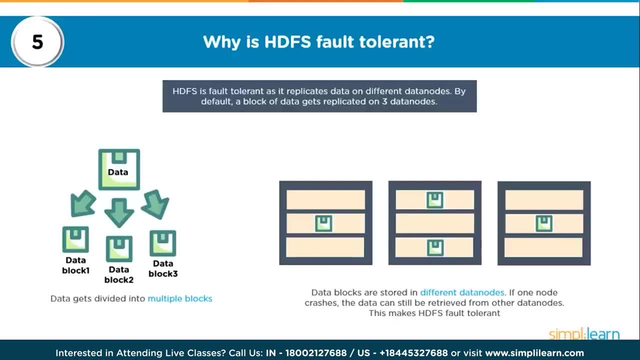 You will never have two identical blocks Sitting on the same machine. And the second rule of replication is In terms of rack awareness. So if your machines are placed in racks, As we see in the right image, You will never have all the replicas. 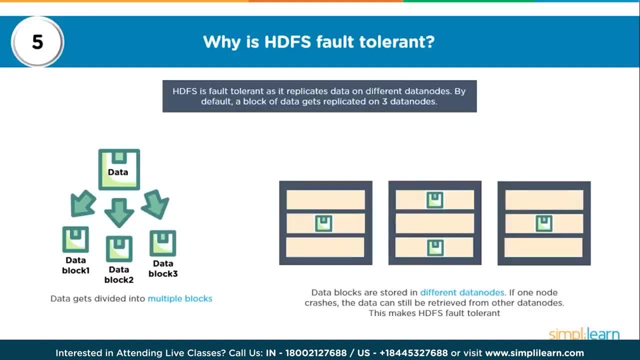 Placed on the same rack, Even if they are on different machines. So it has to be fault tolerant And it has to maintain redundancy, So at least one replica Will be placed on some other node On some other rack. That's how SDFS is fault tolerant. 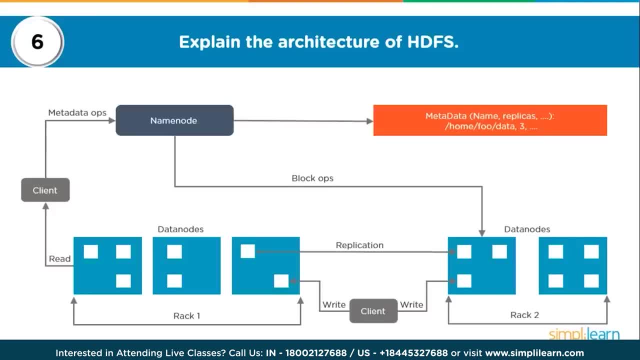 Now here let's understand the architecture of SDFS. Now, as I mentioned earlier, You would in a Hadoop cluster. The main service is Your HDFS. So for your SDFS service You would have a name node, Which is your master process running. 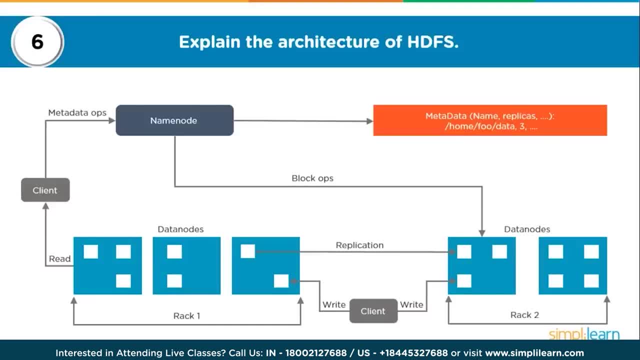 On one of the machines And you would have data nodes, Which are your slave machines Getting stored across, Or the processes running across multiple machines. Each one of these processes Has an important role to play When you talk about SDFS. 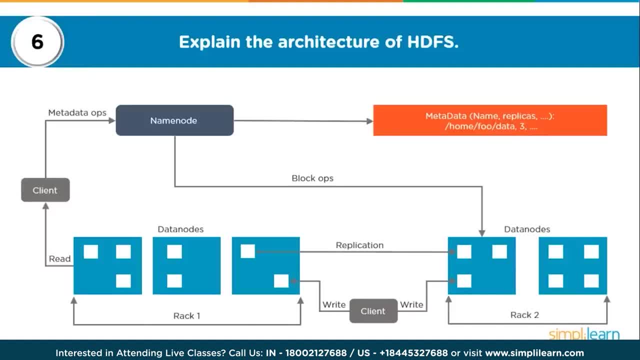 Whatever data is written to HDFS, That data is split Into blocks Depending on its size, And the blocks are randomly distributed across nodes. With auto replication feature, These blocks are also auto replicated Across multiple machines, With the first condition. 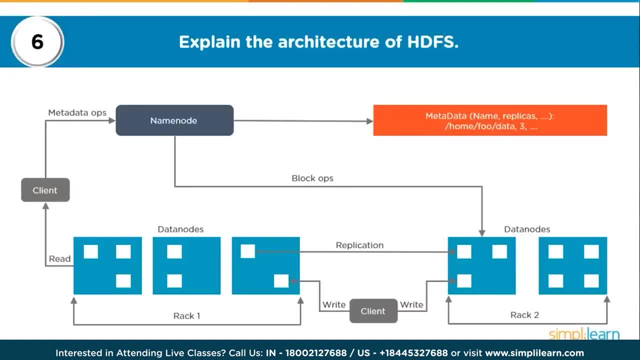 That no two identical blocks Will sit on the same machine. Now, as soon as the cluster comes up, Your data nodes, Which are part of the cluster And based on config files, Would start sending their heartbeat To the name node Every ten seconds. 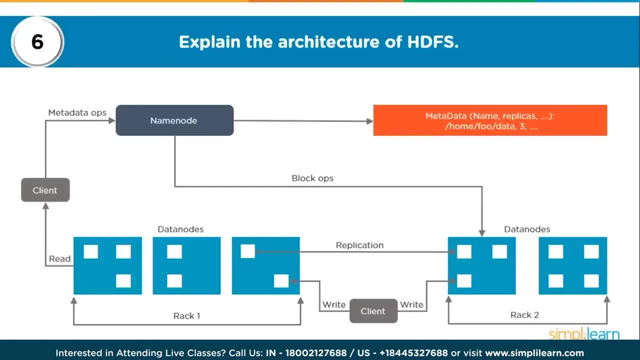 What does name node do with? that Name node will store this information In its RAM. So name node starts building a metadata In its RAM And that metadata has information of What are the data nodes which are available In the beginning. 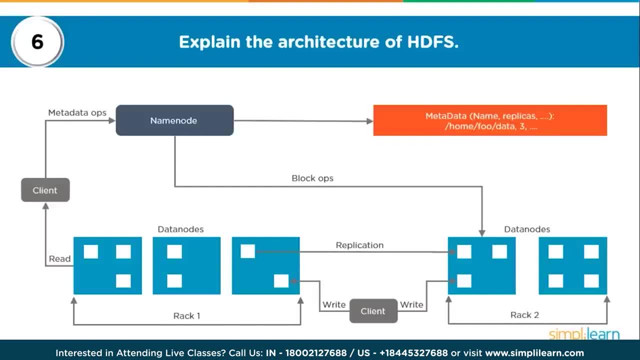 Now, when a data writing activity starts And the blocks are distributed across data nodes, Data nodes Every ten seconds Will also send a block report to name node. So name node Has information in its RAM Or the metadata in RAM, Which earlier had only data node information. 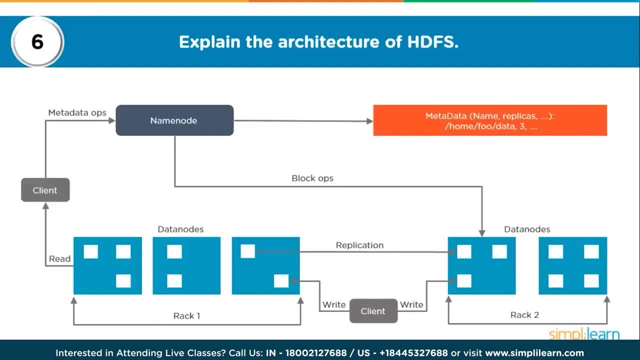 Now name node will also have Information about what are the files, The files are split in which blocks, The blocks are stored on which machines And what are the file permissions. Now, while name node is Maintaining this metadata in RAM, Name node- 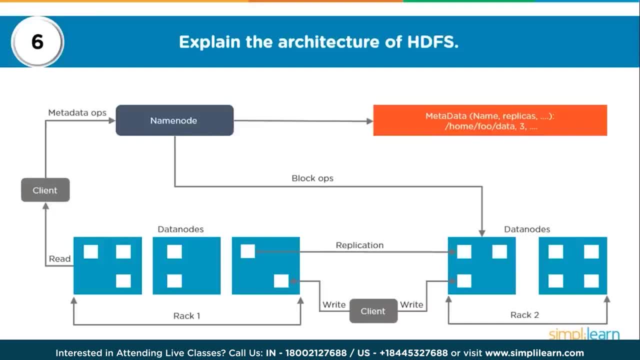 Is also maintaining metadata in disk. Now that is what we see in the red box, Which basically has Information of What information was written to HDFS. So, to summarize: Your name node has metadata in RAM And metadata in disk, Your data nodes. 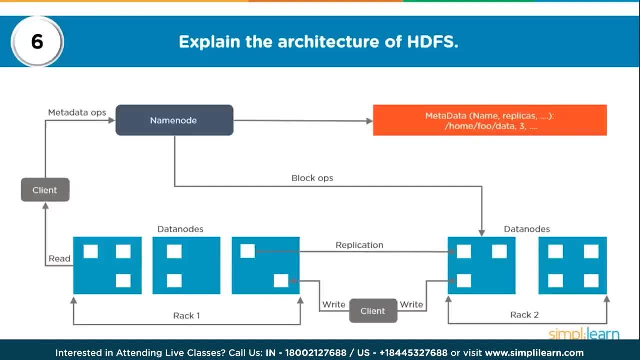 Are the machines where your blocks Or data is actually getting stored. And then there is a auto replication feature, Which is always existing Unless and until you have disabled it, And your read And write activity Is a parallel activity. However, replication is a sequential activity. 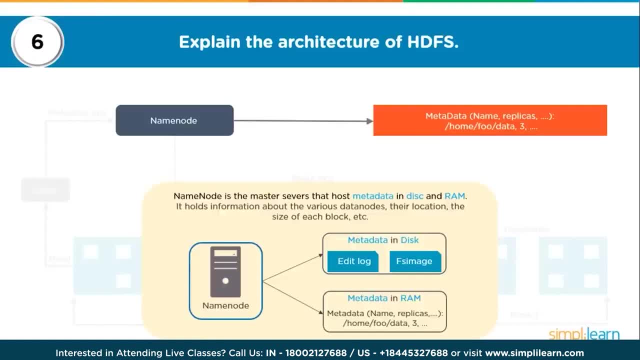 Now, this is what I mentioned about When you talk about name node, Which is the master process Hosting metadata in disk and RAM. So when we talk about disk, It basically has a edit log, Which is your transaction log And your FS image. 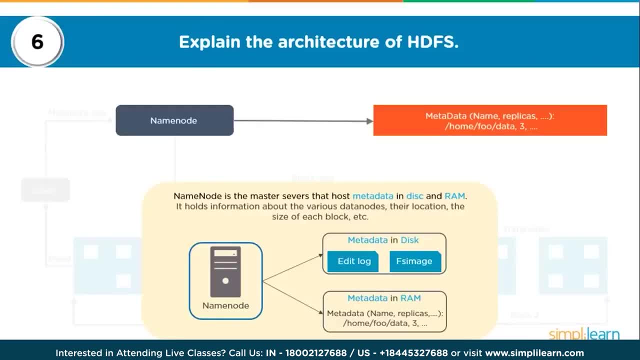 Which is your file system image. Right from the time The cluster was started, This metadata in disk was existing And this gets appended Every time read, write Or any other operations. Metadata in RAM Is dynamically built Every time the cluster comes up. 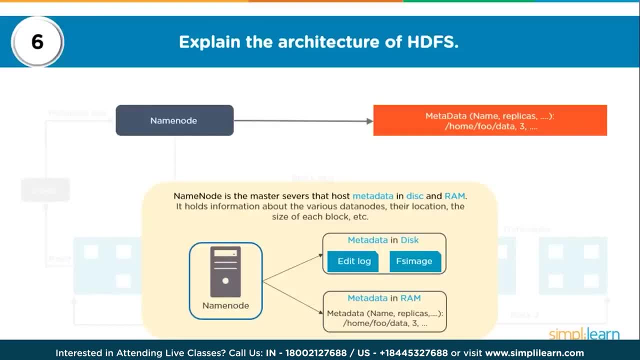 Which basically means That if your cluster is coming up, Name node in the initial few seconds Or few minutes Would be in a safe mode, Which basically means It is busy registering the information From data nodes, So name node is one of the most critical processes. 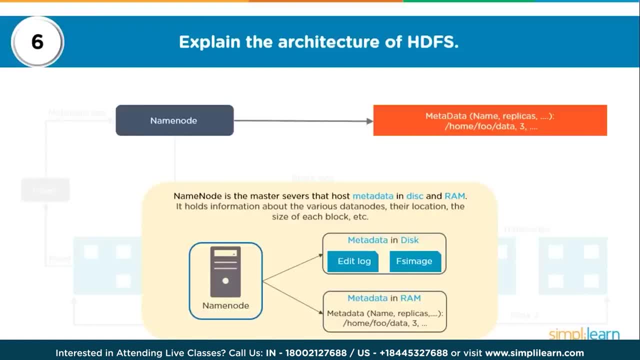 If name node is down And if all other processes are running, You will not be able to access the cluster. So metadata in disk Is very important For name node to come up And maintain the cluster. Name node metadata in RAM. 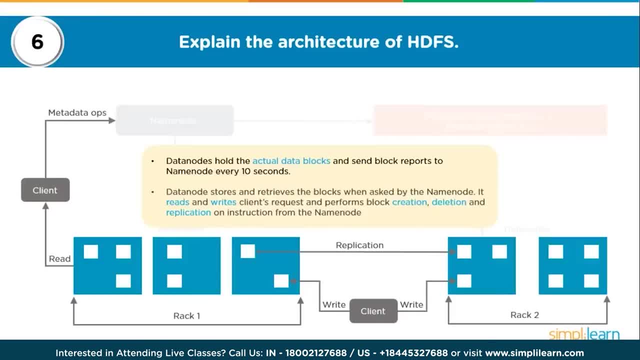 Is basically for all, Or satisfying all your client requests. Now, when we look at data nodes, As I mentioned, Data nodes hold the actual data blocks And they are sending these block reports Every 10 seconds. So the metadata in name node RAM. 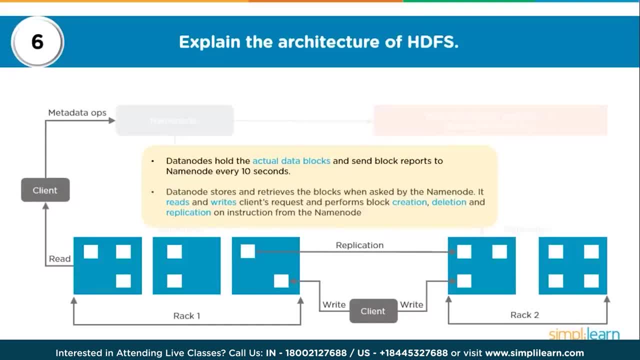 Is constantly getting updated Based on any kind of Write activity happening on the cluster. Now data node Which is storing the block Will also help in any kind of read activity Whenever a client requests. So whenever a client or an application. 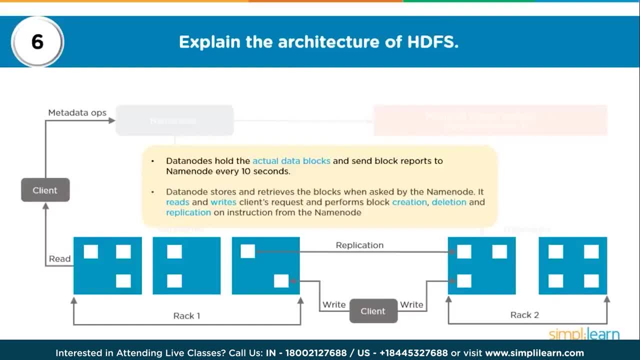 Or an API would want to read the data, It would first talk to name node. Name node would look into its metadata On RAM And confirm to the client Which machines could be reached To get to that data. That's where your client. 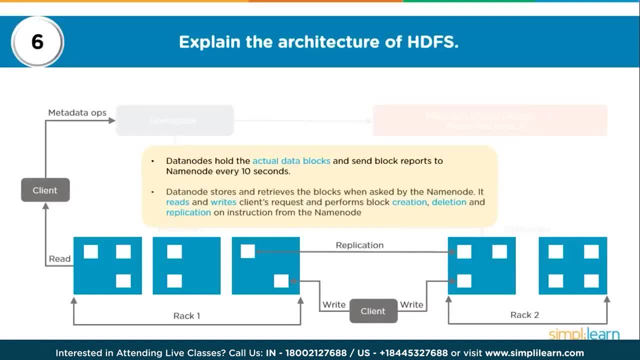 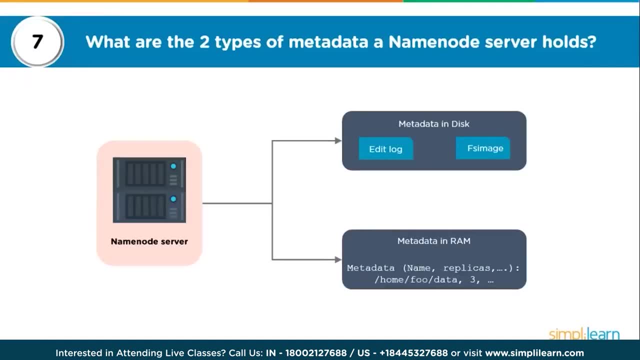 Is DFS, Which is actually getting the data from data nodes, And that's how your Read write requests are satisfied. Now what are the two types of metadata In name node? server holds, As I mentioned earlier, metadata in disk, Very important to remember. 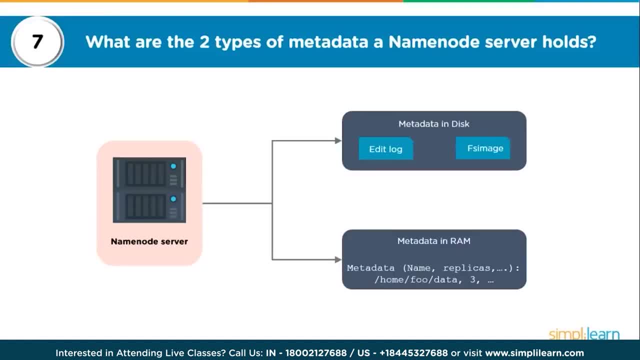 Edit log: NFS image Metadata in RAM, Which is information about your data nodes, Files, Files being split into blocks, Blocks residing on data nodes And file permissions. So this is a very good link on this And you can always look for more detailed. 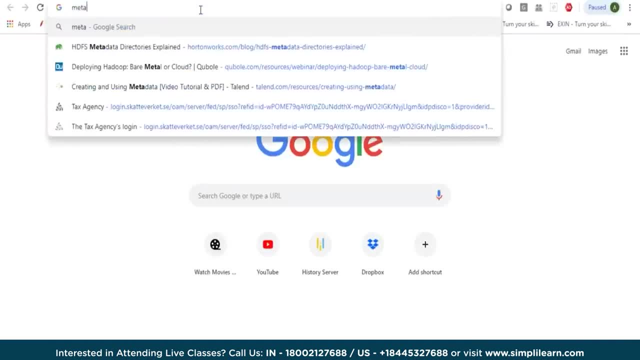 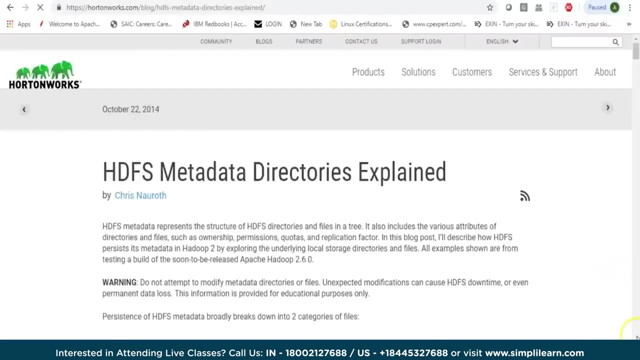 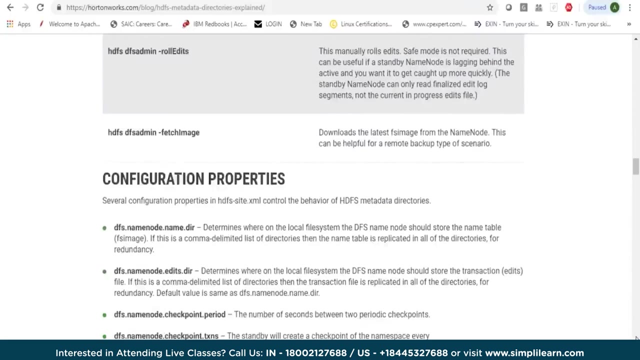 Information about your metadata, So you can search for SDFS metadata Directories explained. Now. this is from Hortonworks. However, it talks about the metadata in disk, Which name node manages And details about this. So have a look at this link. 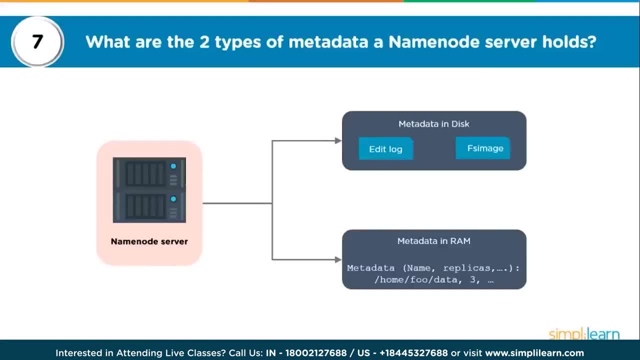 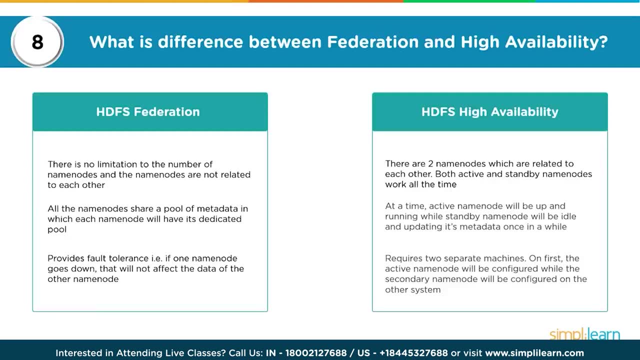 If you are more interested in learning about Metadata on disk Coming back, Let's look at the next question. What are the features Introduced in Hadoop version 2.? Both of these features Are about Horizontal scalability of name node. 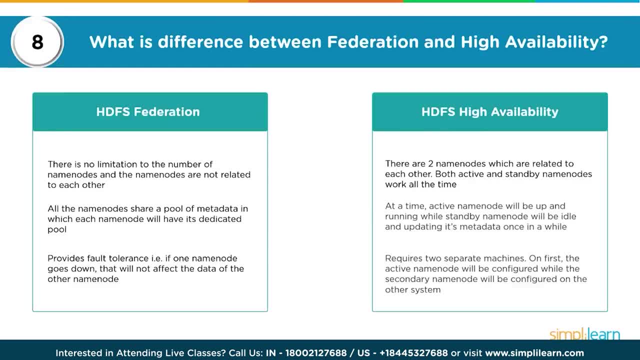 So prior to version 2.. The only possibility was That you could have one single master, Which basically means That your cluster could become Unavailable if name node would crash. So Hadoop, version 2. Introduced two new features: Federation and high availability. 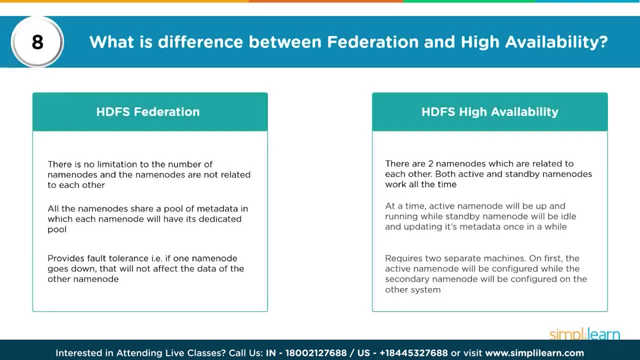 However, high availability Is a popular one. So when you talk about federation, It basically means Any number of name nodes, So there is no limitation To the number of name nodes. Your name nodes are in a federated cluster, Which basically means 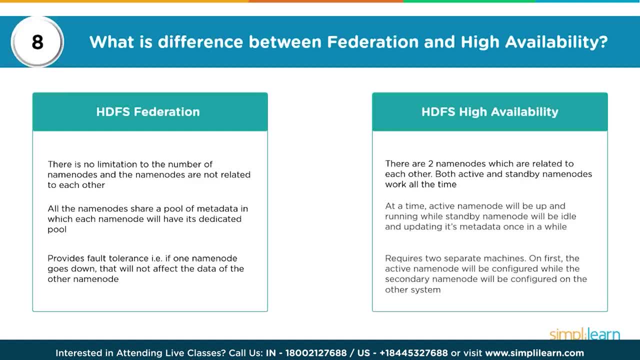 Name nodes still belong to the same cluster But they are not coordinating with each other. So whenever a write request comes in, One of the name node picks up that request And it guides that request For the blocks to be written on data nodes. 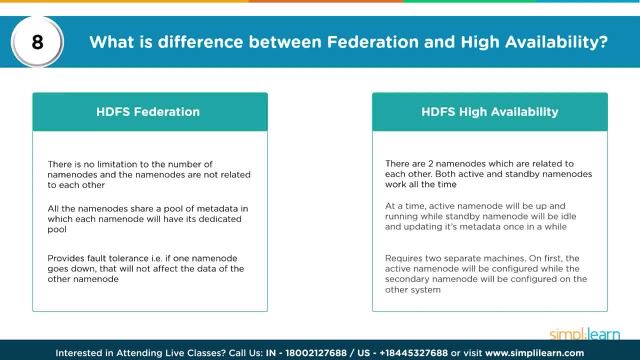 But for this One node does not have to coordinate With other name node To find out if the block ID Which was being assigned Was the same one as assigned by other name node. So all of them belong to A federated cluster. 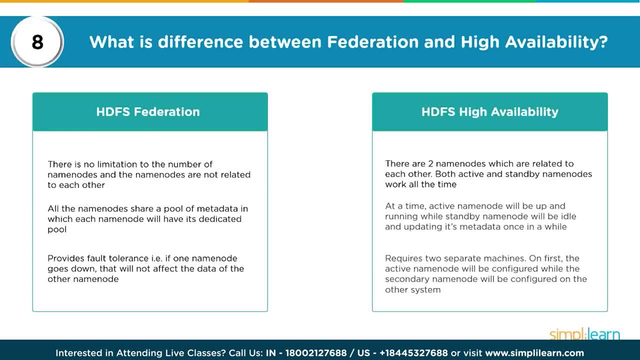 They are linked via a cluster ID. So whenever an application Or an API is trying to talk to cluster, It is always going via A cluster ID And one of the name node would pick up the read activity Or write activity Or processing activity. 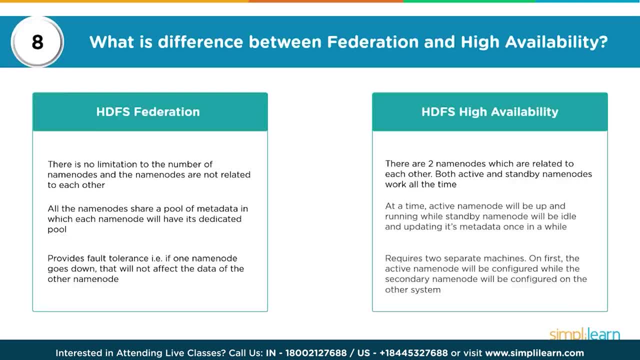 So all of these nodes Are sharing a pool of metadata In which each name node Will have its own dedicated pool, And we can remember that By a term called namespace Or nameservice. So this also provides high fault tolerance. Suppose your one name node goes down. 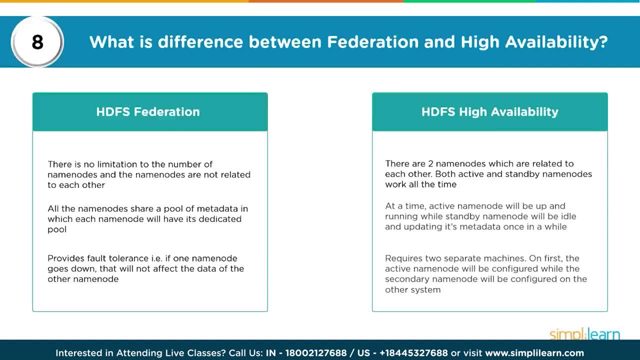 It will not affect Or make your cluster unavailable. You will still have your cluster reachable Because there are other name nodes running And they are available Now. when it comes to heartbeats, They are sending their heartbeats To all the name nodes. 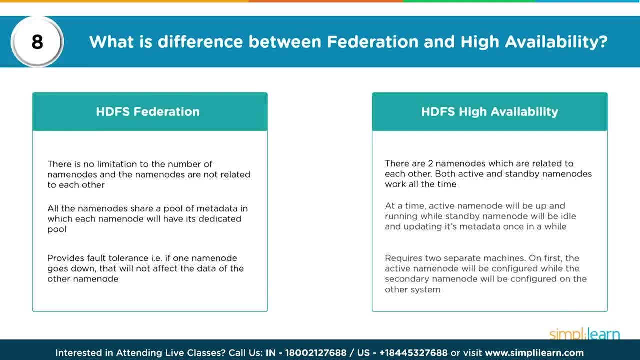 And all the name nodes are aware of all the data nodes. When you talk about high availability, This is where you would only have Two name nodes, So you would have an active And you would have a standby. Now, normally in any environment, 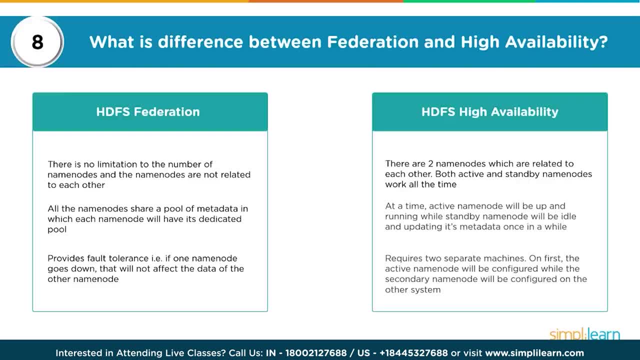 You would see a high availability setup With Zookeeper. So Zookeeper is a centralized coordination service. So when you talk about your active And standby name nodes, Election of a name node Is made as active And taking care of an automatic failover. 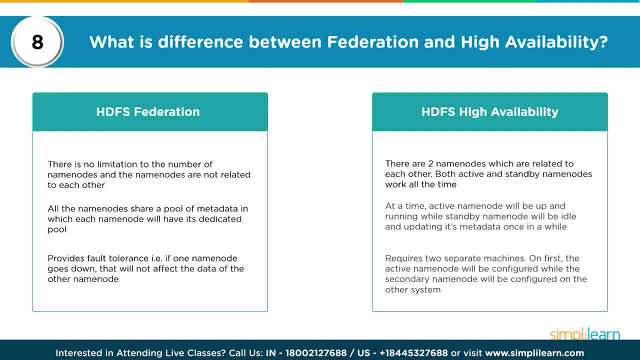 Is done by your Zookeeper. High availability Can be setup without Zookeeper, But that would mean That an admins intervention would be required To make a name node as active From standby Or also to take care of failover Now, at any point of time. 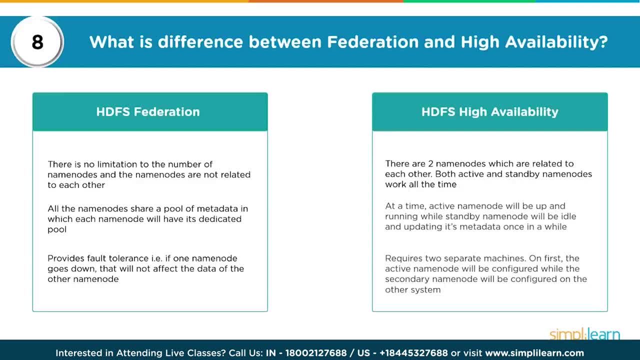 In high availability. An active name node would be taking care of Storing the edits About whatever updates are happening, And it is also writing these edits To a shared location. Standby name node is the one Which is constantly Looking for these latest updates. 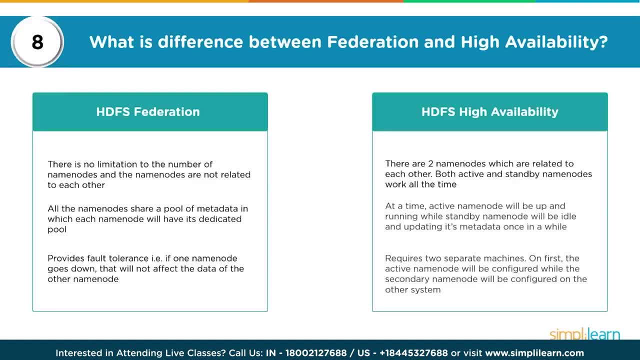 And applying to its metadata, Which is actually a copy of Whatever your active name node has. So in this way, Your standby name node is always in sync With the active name node And if, for any reason, Active name node fails, 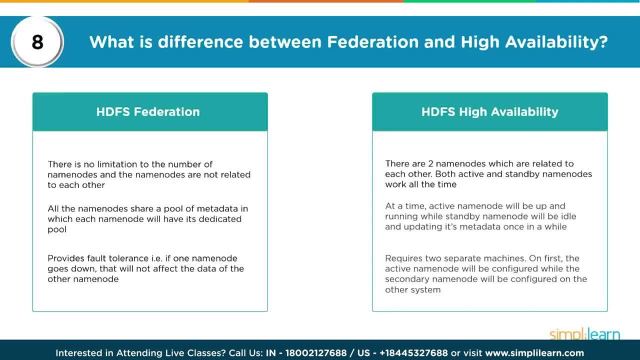 Your standby name node will take over And become the active. Zookeeper plays a very important role here. It's a centralized coordination service. One more thing to remember here Is that In your high availability, Secondary name node Will not be allowed. 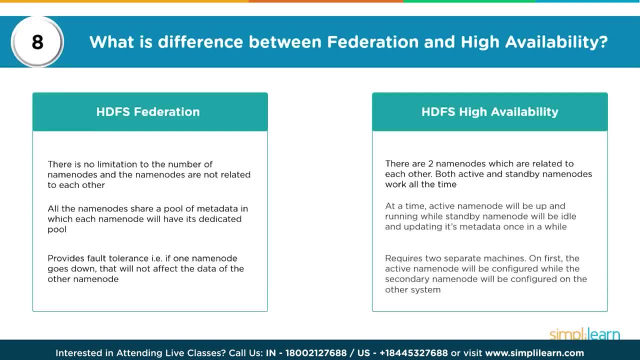 So you would have an active name node And then you will have a standby name node Which will be configured on a separate machine, And both of these Will be having access to a shared location. Now that shared location could be NFS, Or it could be a quorum of general nodes. 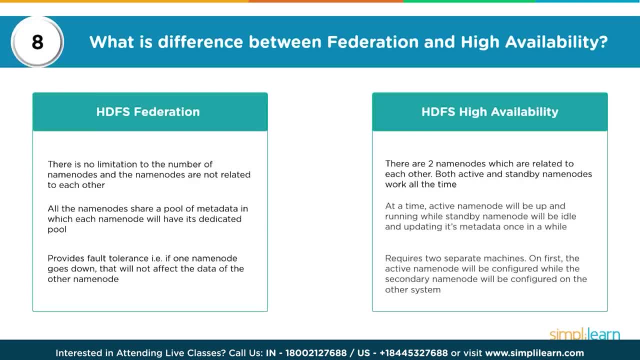 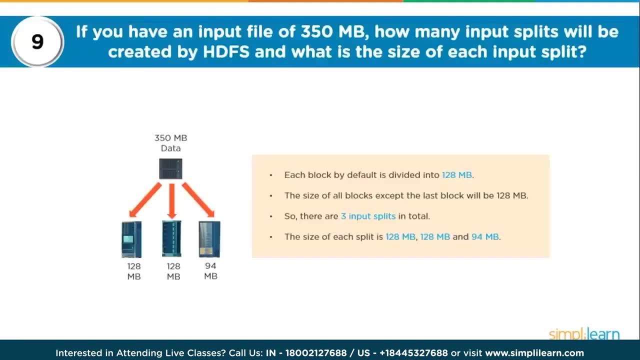 So for more information, Refer to the tutorial where I have explained about SDFS, high availability and federation. Now let's look at some logical question here. So if you have a input file Of 350 MB, Which is obviously bigger than 128 MB, 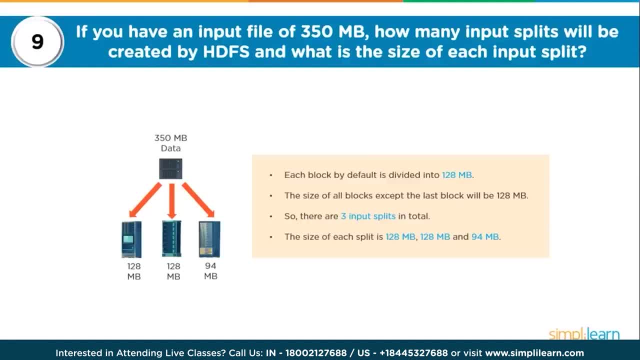 How many input splits Would be created by SDFS And what would be the size of each input split. So for this, You need to remember that by default, The minimum block size is 128 MB. Now that's customizable If your environment has. 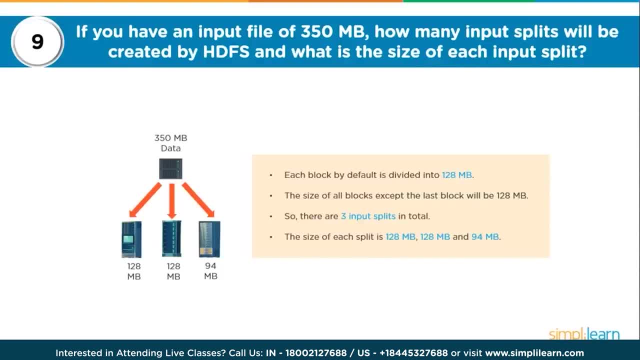 More number of larger files written On an average, Then obviously you have to go for a bigger block size. If your environment Has lot of files being written But these files are of smaller size, You could be okay with 128 MB. 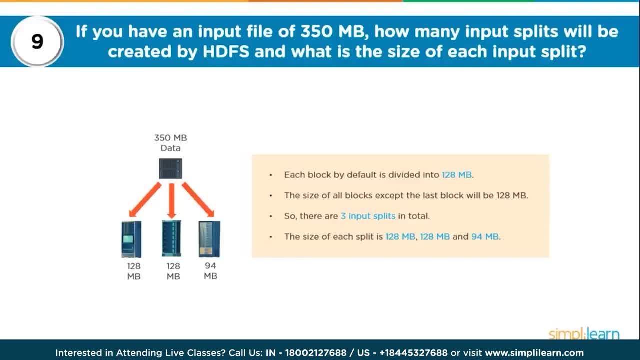 Remember, in Hadoop Every entity, That is, your directory on SDFS, File on SDFS And a file having multiple blocks, Each of these are considered as objects. So in Hadoop Name nodes RAM 150 bytes is utilized. 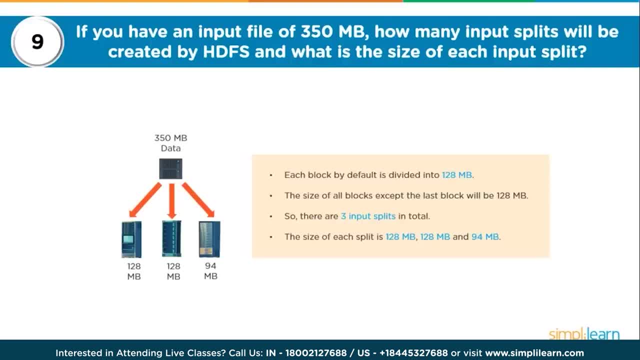 So if your block size is very small Then you would have more number of blocks Which would directly affect the name nodes RAM. If you keep a block size very high That will reduce the number of blocks But remember that might affect in processing. 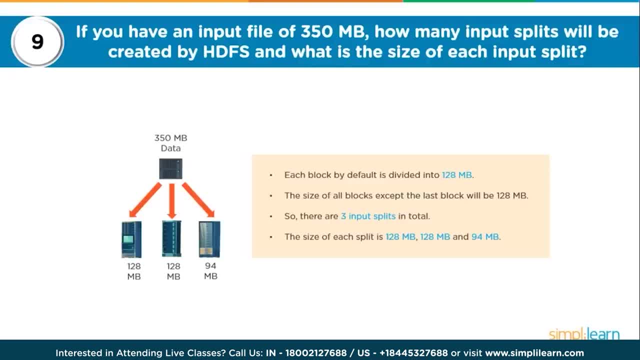 Because processing also depends on Splits. More number of splits, More the parallel processing. So setting of block size Has to be done. About your parallelism requirement And your name nodes, RAM, Which is available. Now coming to the question, 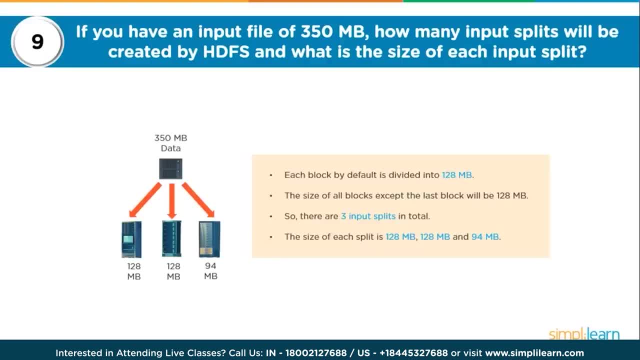 If you have a file of 350 MB, That would be split into three blocks, And here two blocks would have 128 MB data And the third block, Although the block size would still be 128. It would have only 94 MB of data. 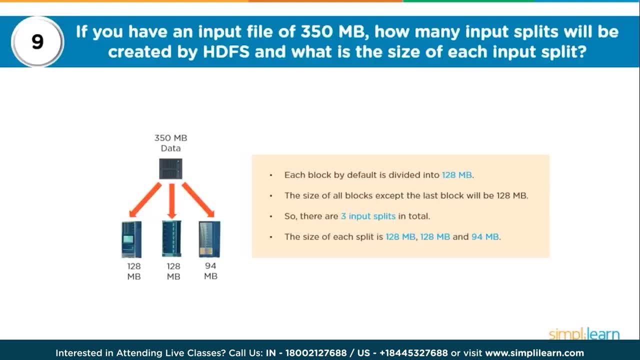 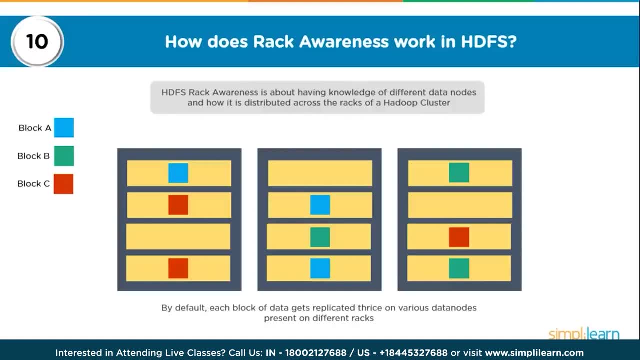 So this would be The split of this particular file. Now let's understand about Rack Awareness. How does Rack Awareness work? Or why do we even have Rack Awareness? So organizations always Would want to place their nodes Or machines in a systematic way. 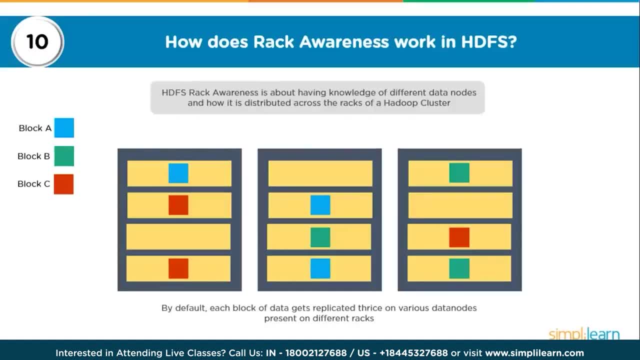 There can be different approaches. You could have a rack Which would have machines Running on the master processes And the intention would be That this particular rack Could have higher bandwidth, More cooling. Dedicated power supply. Top of rack switch. 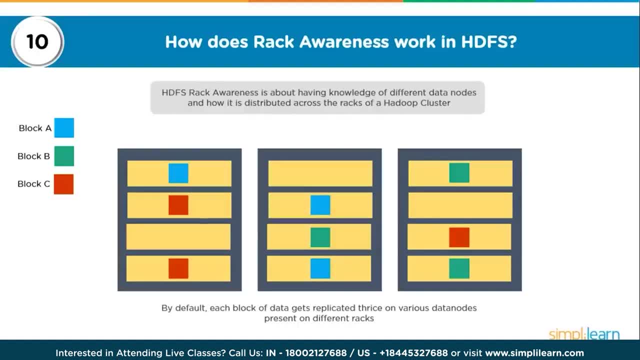 And so on, And then You could have other slave processes running. Now, When you talk about your Rack Awareness, One thing to understand is That if your machines are placed Within racks- And we are aware that Hadoop follows auto replication- 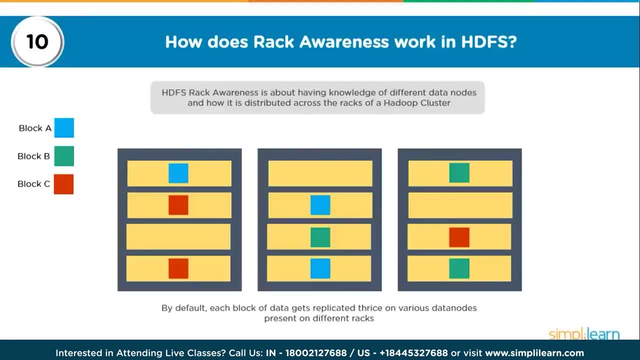 The rule of replication In a Rack Aware cluster would be That you would never have All the replicas Placed on the same rack. So if we look at this In blue color, You will never have all the three blue boxes. 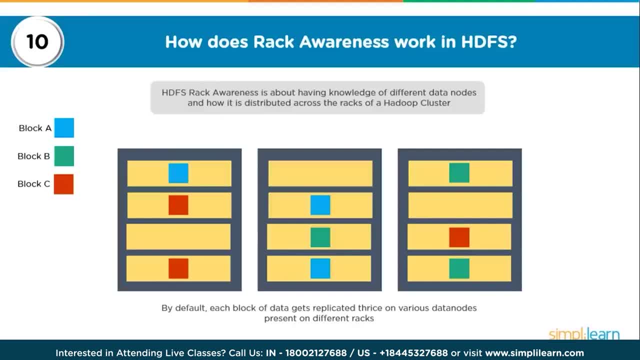 In the same rack, Even if they are on different nodes, Because that makes us, That makes it less fault tolerant. So you would have at least one copy Of block Which would be stored on a different rack On a different node. 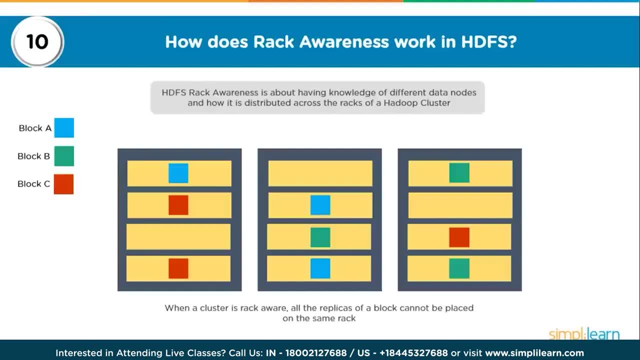 Now let's look at this. So basically, Here we are talking about Replicas being placed in such a way That the block and its replicas Spread across three racks. And yes, you can do that, But then, in order to make it more redundant, 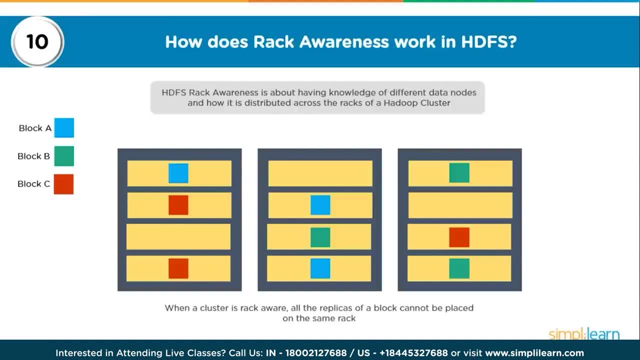 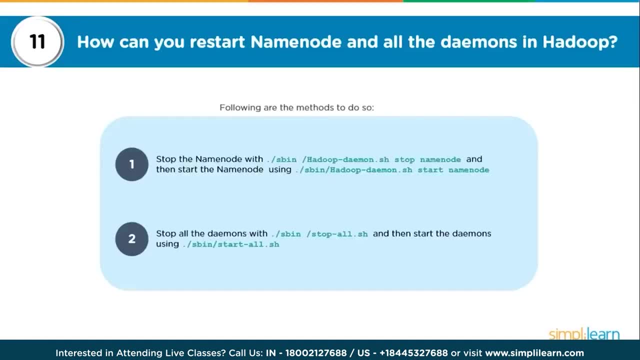 You are increasing your bandwidth requirement, So the better approach would be: Two blocks on the same rack On different machines And one copy on a different rack. Now let's proceed. How can you restart name node And all daemons in Hadoop? 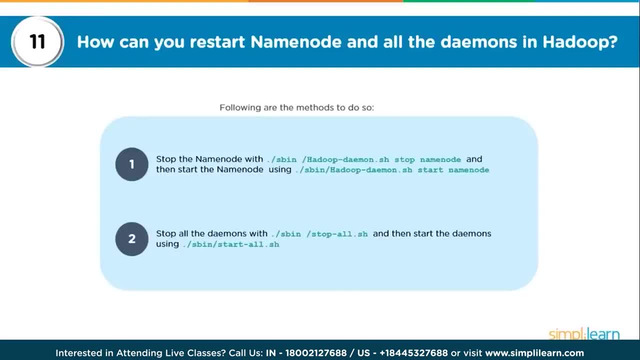 So if you were working on a Apache Hadoop cluster, Then you could be doing A start and stop Using Hadoop daemon scripts. So there are these Hadoop daemon scripts Which would be Used to start and stop your Hadoop. 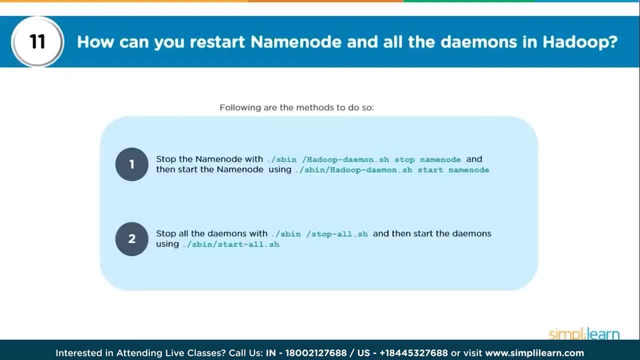 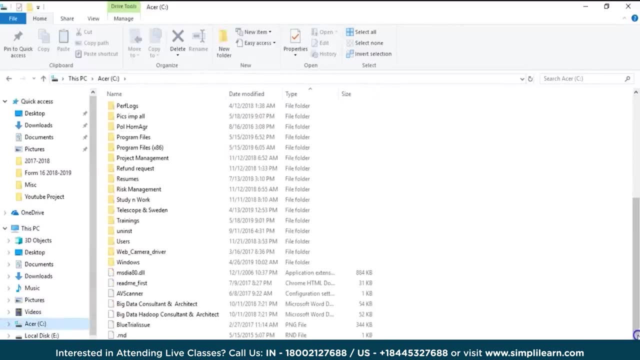 And this is when you talk about Your Apache Hadoop. So let's look at one particular file Which I would like to show you More information here, And this talks about your different clusters. So let's look into this And 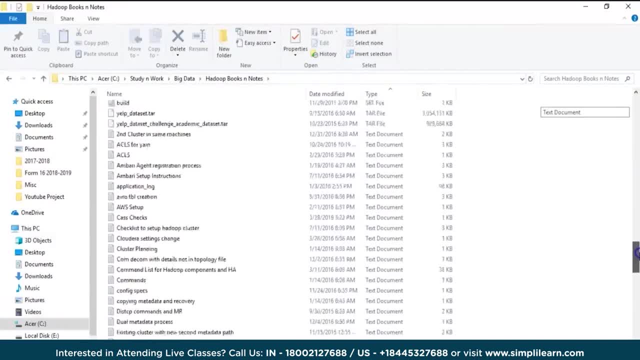 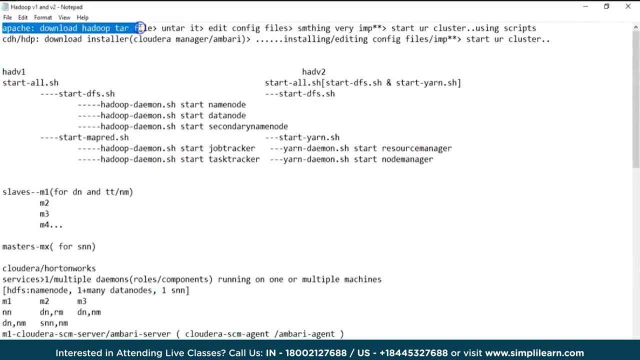 So let's look at the start and stop, And here I have a file. Let's look at this one, And this gives you highlights. So if you talk about Apache, Hadoop, This is how the setup would be done. So you would have it download the Hadoop tar file. 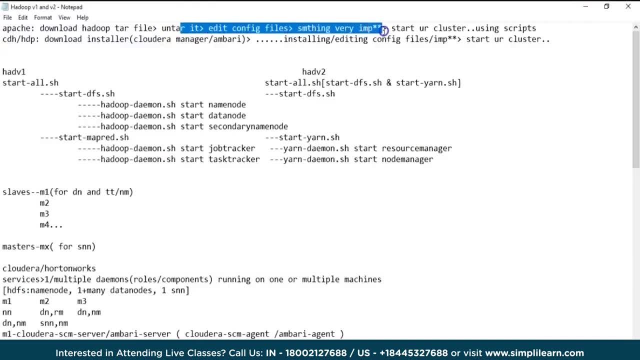 You would have to untar it, Edit the config files, You would have to do formatting And then start your cluster. And here I have said using scripts. So this is in case of Apache Hadoop. You could be using a start all script. 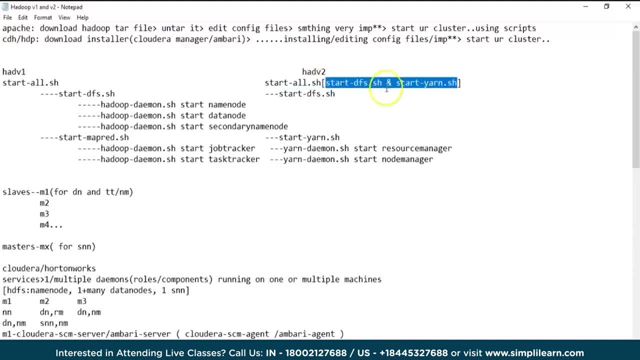 That internally triggers Start DFS and start yarn. And these scripts start DFS And internally would run Hadoop daemon Multiple times, Based on your configs, to start your different processes. Then your start yarn Would run yarn daemon script To start your processing related processes. 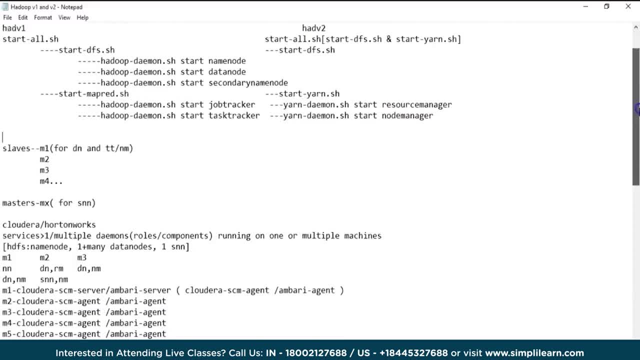 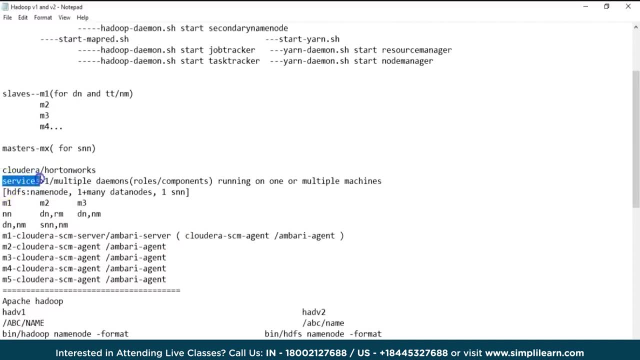 So this is how it happens in Apache, Hadoop. Now, in case of cloud, era Or Hortonworks, Which is basically a vendor, specific distribution, You would have, Say, multiple services, Which would have one or multiple daemons Running across the machines. 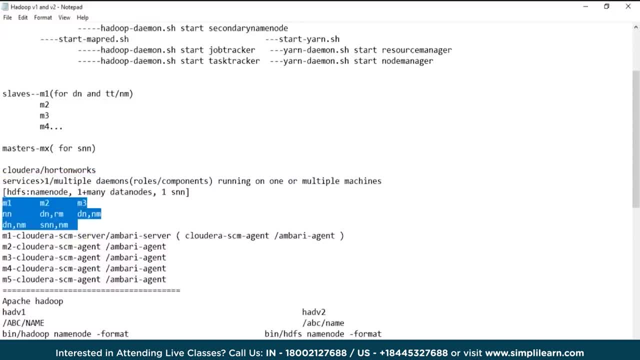 Let's take an example here: Machine 1,, machine 2 and machine 3. With your processes spread across. However, in case of cloud era And Hortonworks, These are cluster management solutions, So you would never be involved in running a script. 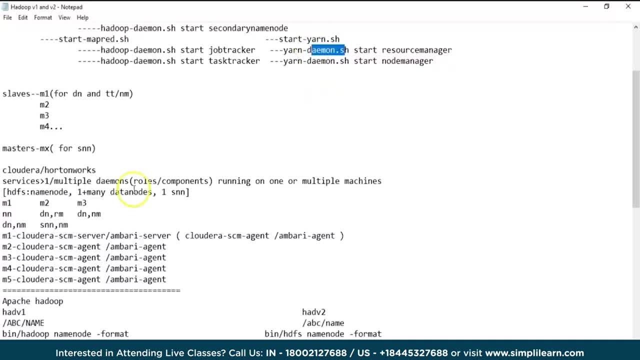 Individually To start and stop your processes. In fact, in case of cloud era, You would have a cloud era SCM server running On one of the machines And then cloud era SCM agents Running on every machine. If you talk about Hortonworks, 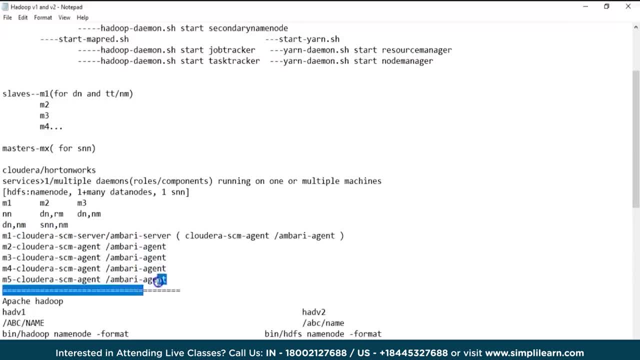 You would have ambari server and ambari agent running. So your agents, Which are running on every machine, Are responsible to monitor the processes. Send also their heartbeat To the master. That is your server, And your server is the one. 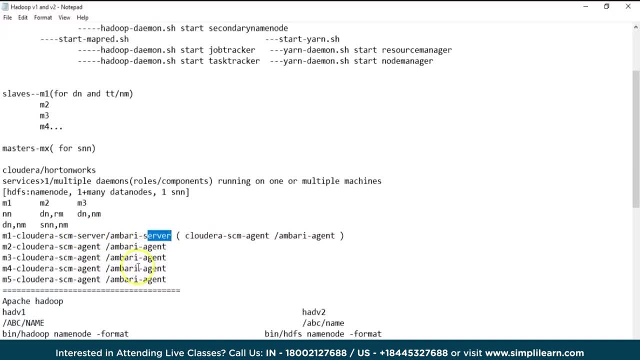 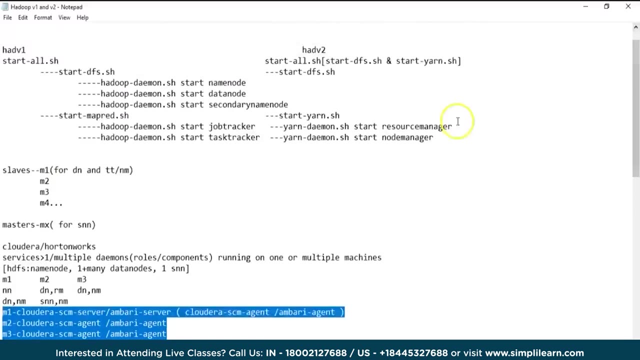 Or a service which basically Will give instructions to the agents. So in case of vendor specific distribution, Your start and stop of processes Is automatically taken care By these underlying services And these services internally Are still running These commands, However only in Apache Hadoop. 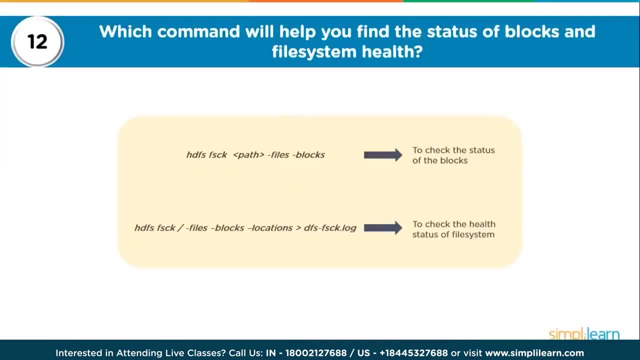 You have to manually follow these To start and stop Coming back. we can look into Some command related questions. So which command will help you find The status of blocks and file system health? So you can always go for a file system check command. 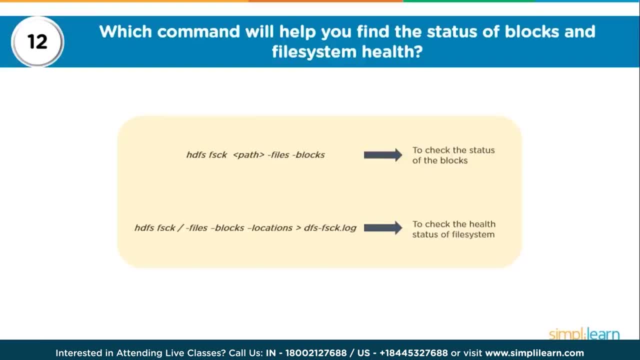 Now, that can show you the files For a particular HDFS path. It can show you the blocks And it can also Give you information on Status, such as Over replicated blocks, Over replicated blocks, Misreplicated blocks, Default replication and so on. 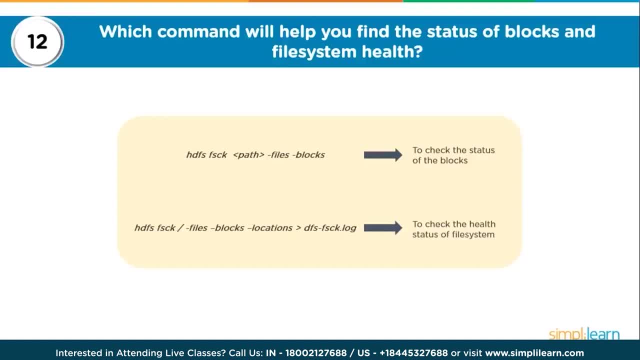 So your FSCK file system check utility Does not repair If there is any problem with the blocks, But it can give you information of Blocks related to the files On which machines they are stored, If they are replicated As per the replication factor. 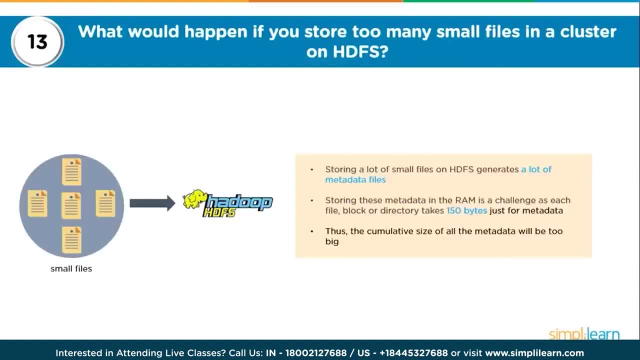 Or if there is any problem with any particular replica. Now, what would happen If you store too many small files? This relates to the block information Which I gave some time back. So remember, Hadoop is coded in Java, So here every directory. 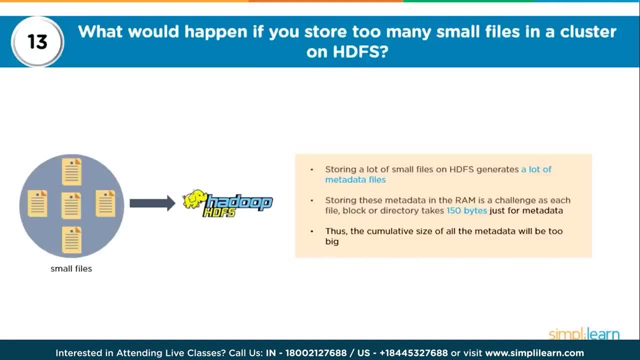 Every file and file related block Is considered as An object And for every object Within your Hadoop cluster, Name nodes RAM gets utilized. So more number of blocks you have, More would be usage of name nodes RAM And if you are storing too many small files, 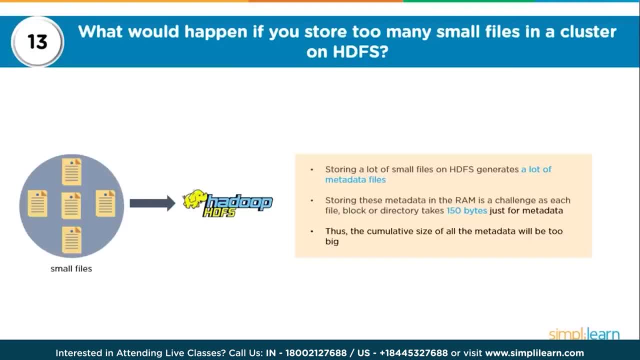 It would not affect your disk. It would directly Affect your name nodes RAM. That's why in production clusters Admin guys or infrastructure Specialists will take care That everyone who is writing data To HDFS follows A quota system. 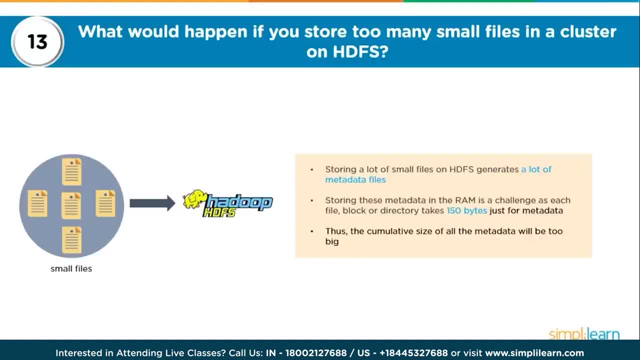 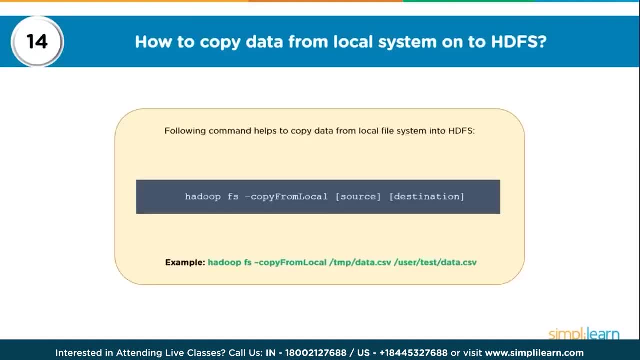 So that you could be controlled In the amount of data you write, Plus the count of data And individual writes on HDFS. Now how do you copy data From local system onto HDFS So you can use a put command Or a copy from local? 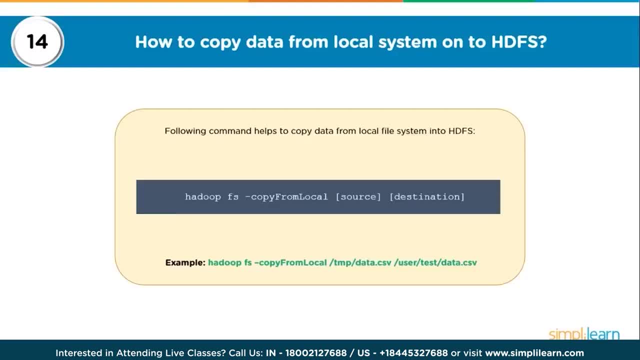 And then given your local path, Which is your source, And then your destination, Which is your HDFS path. Remember, you can always do a copy from local Using a minus F option. That's a flag option And that also helps you in writing the same file. 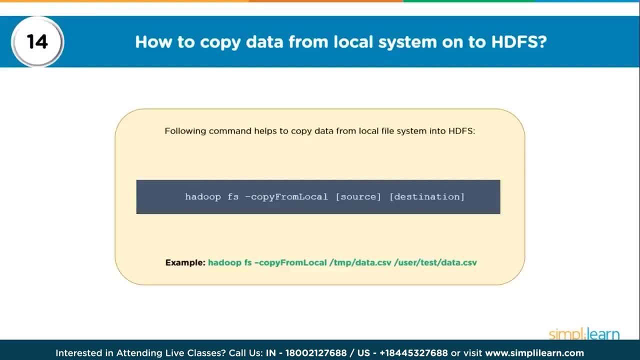 Or a new file To HDFS. So with your minus F You have a chance of overwriting Or rewriting the data Which is existing on HDFS. So you can use a put command Or a copy from local Or minus put. 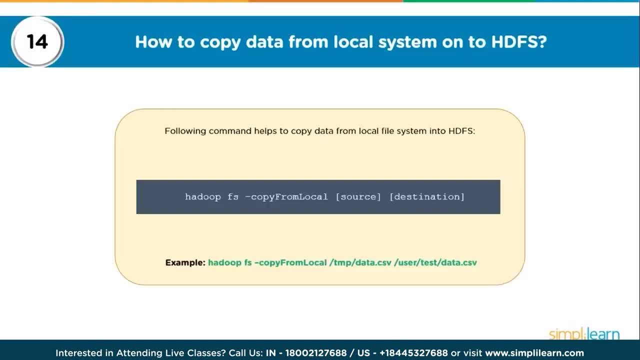 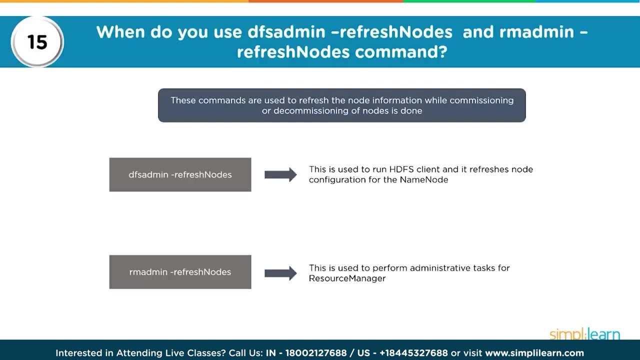 Both of them do the same thing And you can also pass an argument When you are copying To control your replication Or other aspects of your file. Now, when do you use DFS admin Refresh nodes or RM admin refresh nodes? So as the command says, 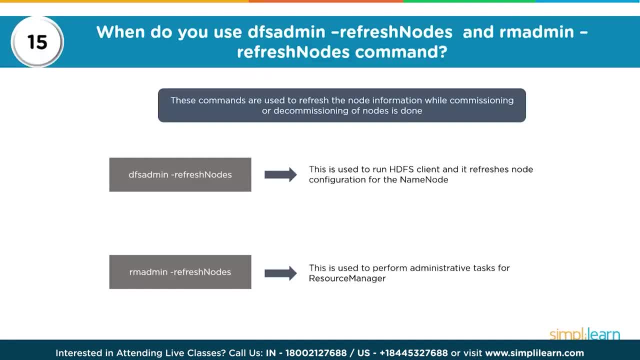 This is basically to do with Refreshing the node information. So your refresh nodes, Or decommissioning of nodes, is done, So when A node is added Into the cluster Or when a node is removed from the cluster, You are actually. 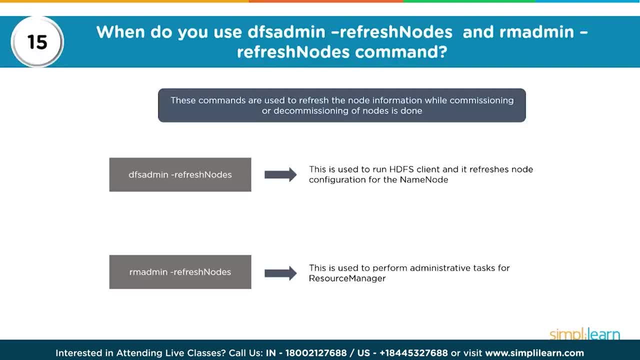 Informing Hadoop master That this particular node Would not be used for storage And would not be used for processing. Now, in that case, you would be. Once you are done with the process Of commissioning or decommissioning, You would be giving these commands. 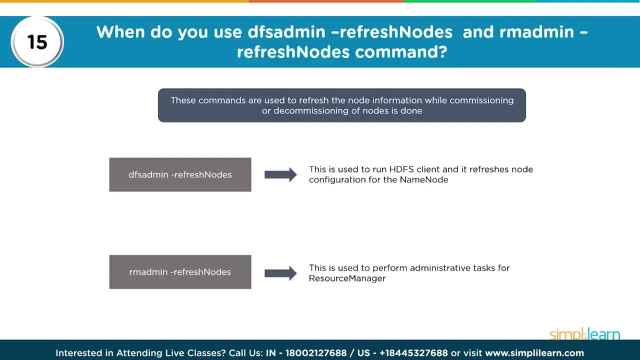 That is, refresh nodes And RM admin refresh nodes. So internally, When you talk about commissioning Decommissioning, There are include and exclude files Which are updated And these include and exclude files Will have entry of machines Which are being added to the cluster. 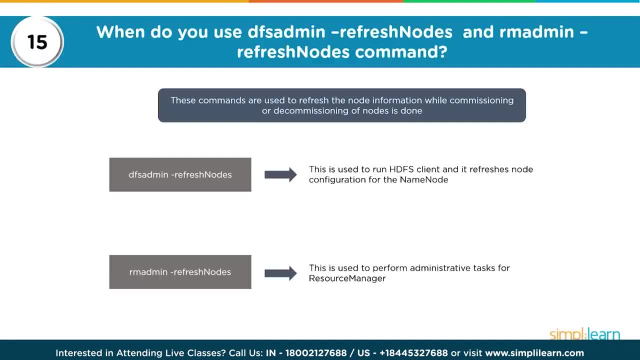 Or machines which are being removed from the cluster, And while this is being done, The cluster is still running, So you do not have to restart your master process. However, you can just use these refresh commands To take care Of these Now. is there any way to change replication of files? 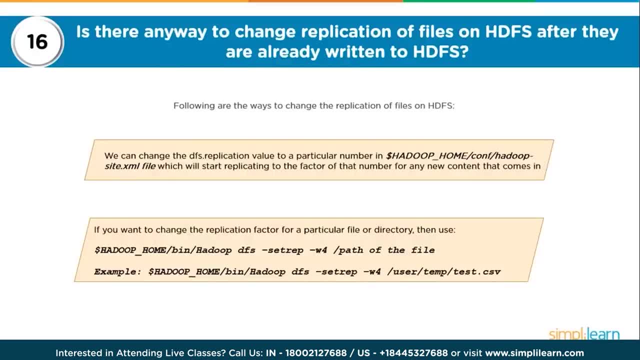 On SDFS after they are already written, And the answer is, of course, yes. So if you would want to set A replication factor At a cluster level And if you have admin access, Then you could edit your SDFS hyphen site file. 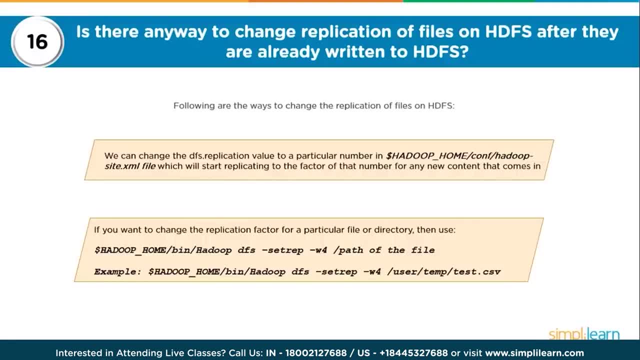 Or you could say Hadoop hyphen site file, And that would take care of Replication factor being set At a cluster level. However, if you would want to change The replication After the data has been written, You could always use a setrep command. 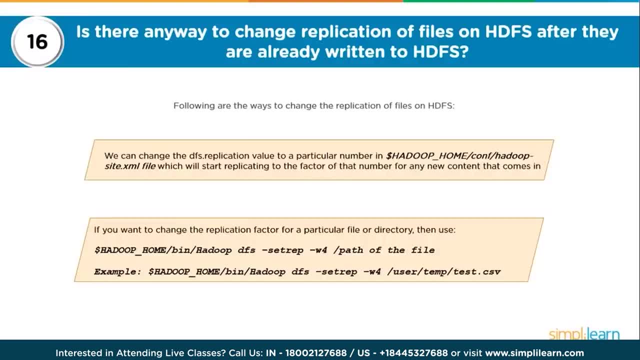 So setrep command Is basically to change the replication After the data is written. You could also write the data With a different replication, And for that you could use A minus d, Dfs, dot replication And give you a replication factor. 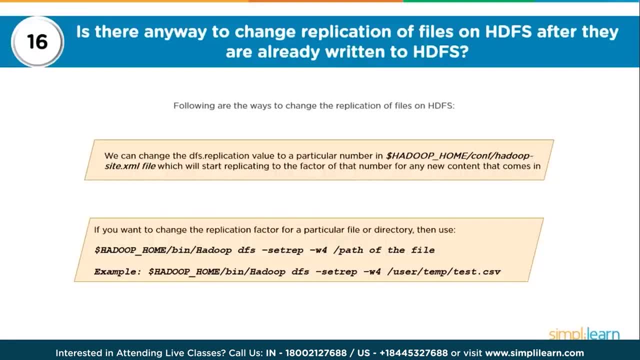 When you are writing data to the cluster. So in Hadoop You can let your data be replicated As per the property In the config file. You could write the data With a different replication. You could change the replication After the data is written. 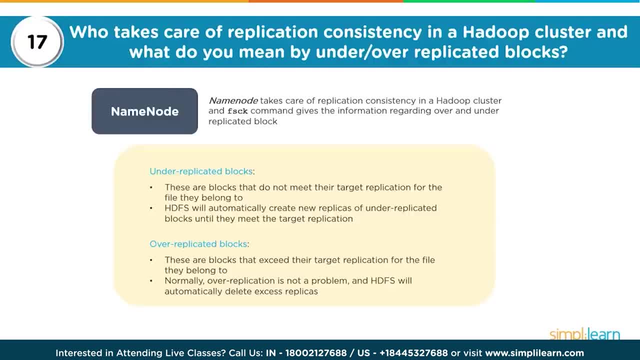 So all these options are available. Now, who takes care of replication consistency In a Hadoop cluster, And what do you mean by under Over replicated blocks? Now, as I mentioned, Your fsck command can give you information Of over or under replicated blocks. 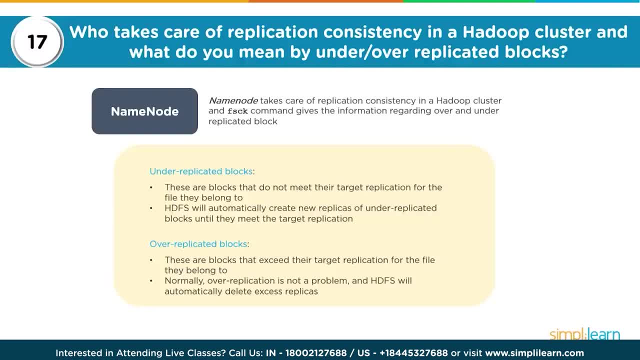 Now, in a cluster, There is a node Which takes care of replication consistency. So, for example, If you have set up a replication of 3. And since we know The first rule of replication, Which basically means That you cannot have 2 replicas, 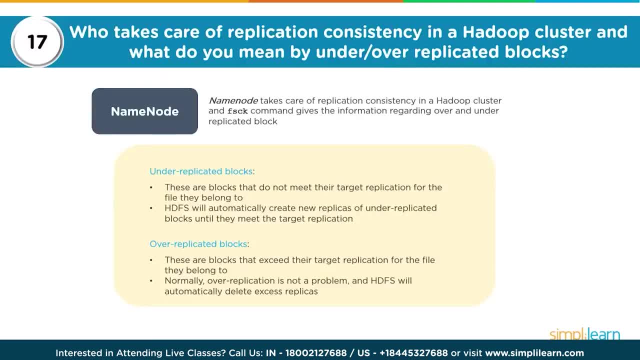 Residing on the same node. It would mean That if your replication is 3. You would need at least 3 data nodes available. Now say, for example, You had a cluster with 3 nodes And replication was set to 3.. 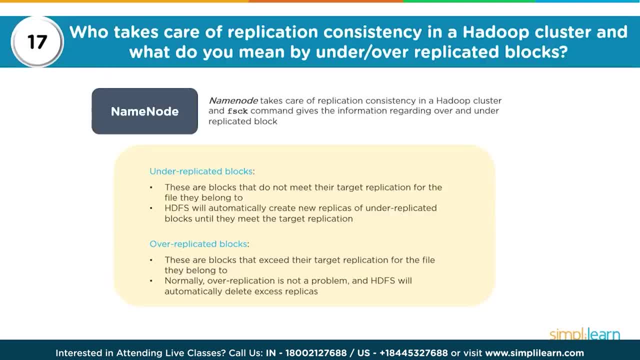 At one point of time One of your name node crashed And if that happens, Your blocks would be under replicated. That means There was a replication factor set, But now your blocks are not replicated Or there are not enough replicas As per the replication factor set. 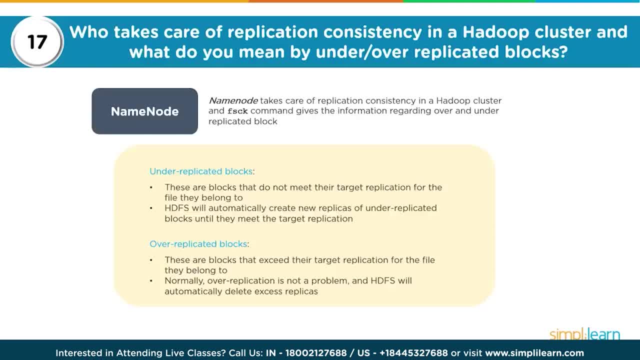 This is not a problem. Your master process or name node Will wait for some time Before it will start The replication of data again. So if a data node is not responding Or if a disk has crashed And if name node does not get information, 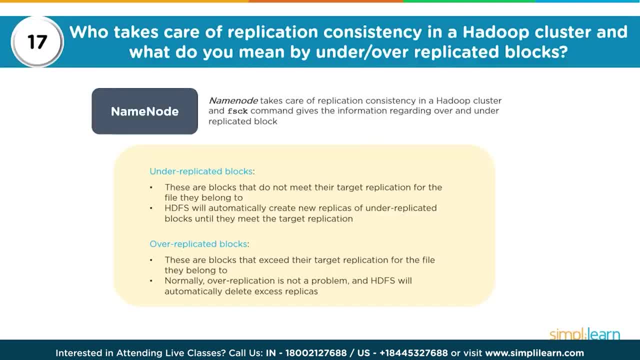 Of a replica Name node will wait For some time And then it will start re-replication Of those missing blocks From the available nodes. However, while name node is doing it, The blocks are in under replicated situation. Now, when you talk about over replicated, 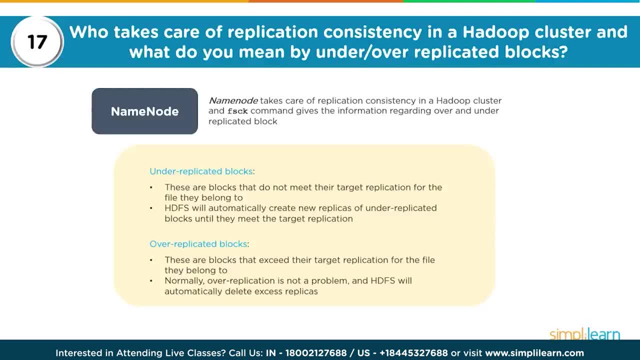 This is a situation Where name node realizes That there are extra copies of block. Now, this might be the case When you had three nodes running With a replication of three. One of the node went down Due to a network failure or some other issue. 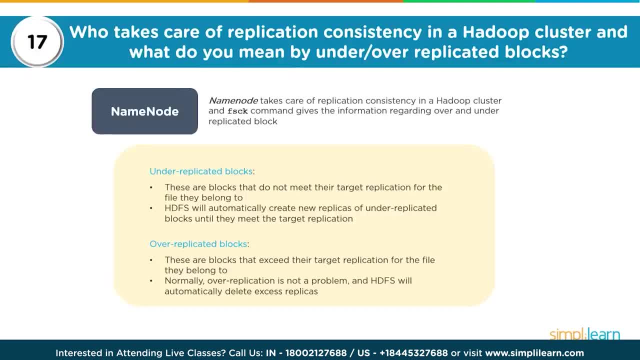 Within few minutes, Name node re-replicated the data And then the failed node is back With its set of blocks Again. name node is smart enough To understand that this is a over replication situation And it will delete Set of blocks from one of the nodes. 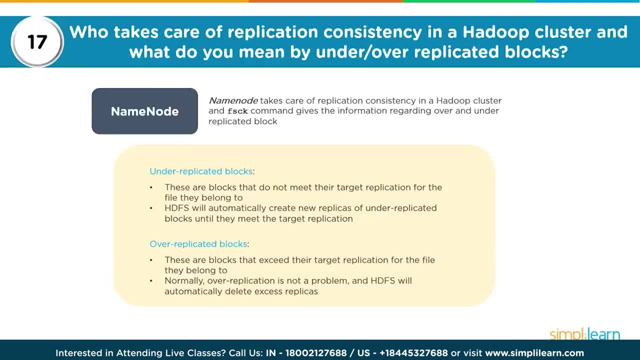 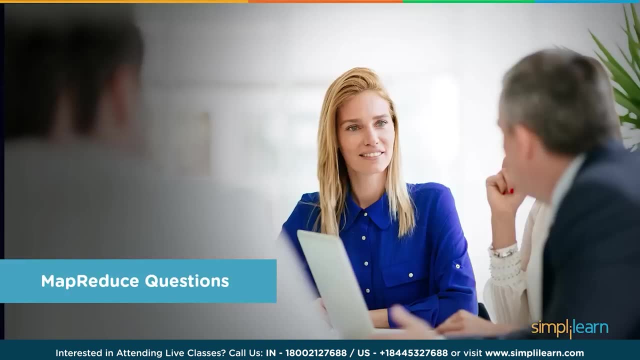 It might be the node Which has been recently added, It might be your old node, It might be a cluster again, Or any node. That depends on the load On a particular node. Now we discussed about Hadoop, We discussed about SDFS. 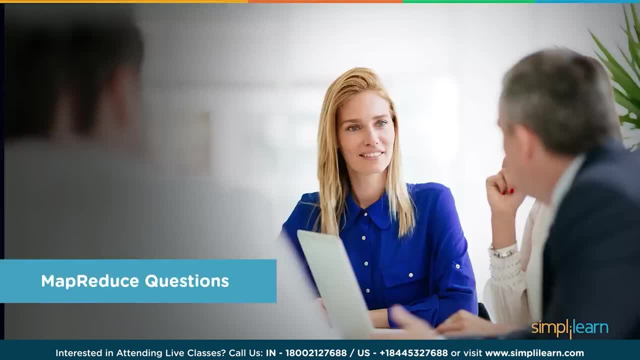 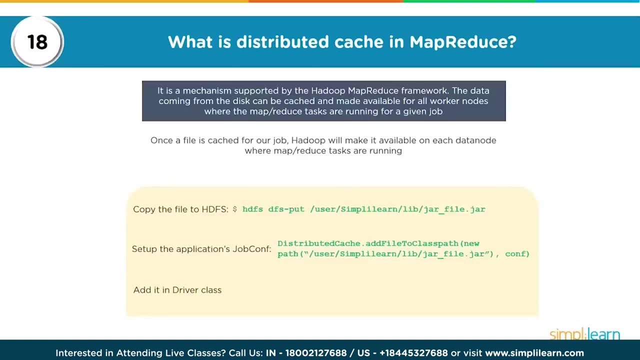 Now we will discuss about MapReduce, Which is the programming model And, you can say, processing framework. What is distributed cache in MapReduce? Now we know That when we talk about MapReduce, The data which has to be processed Might be existing on multiple nodes. 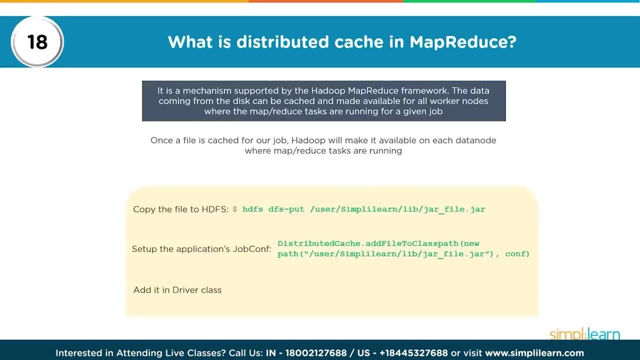 So when you would have MapReduce program running, It would basically read the data From the underlying disks. Now this could be a costly operation If every time the data Has to be read from disk. So distributed cache is a mechanism. 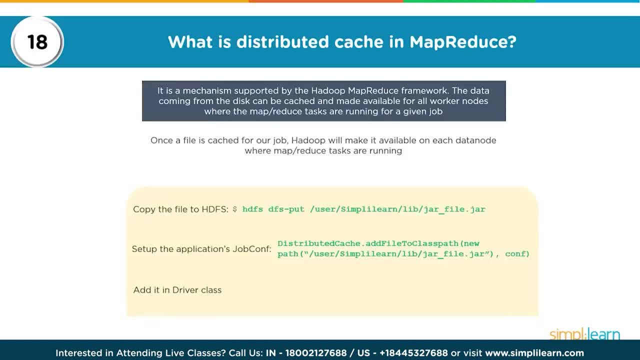 Where in data set Or data which is coming from the disk Can be cached And available for all worker nodes. Now how will this benefit? So when a MapReduce is running, Instead of every time Reading the data from disk, It would pick up the data. 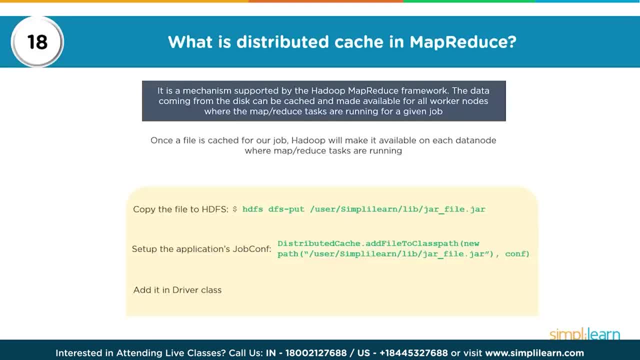 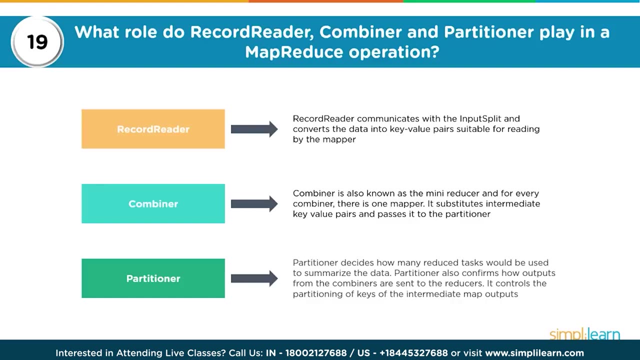 From distributed cache And this will benefit Your MapReduce processing. So distributed cache can be set In your job conf, Where you can specify That a file should be picked up From distributed cache. Now let's understand about these roles. 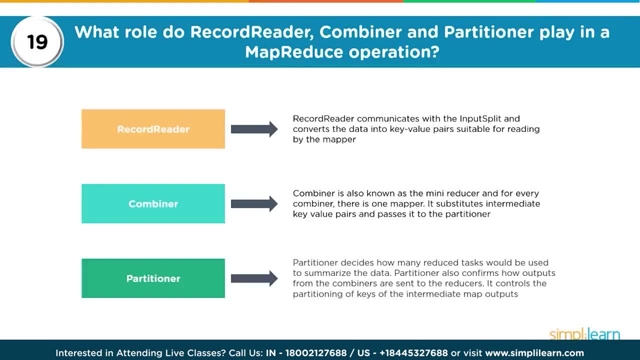 So what is a record reader, What is a combiner, What is a partitioner, And what kind of roles do they play In a MapReduce processing paradigm Or MapReduce operation? So record reader Communicates with the input split. 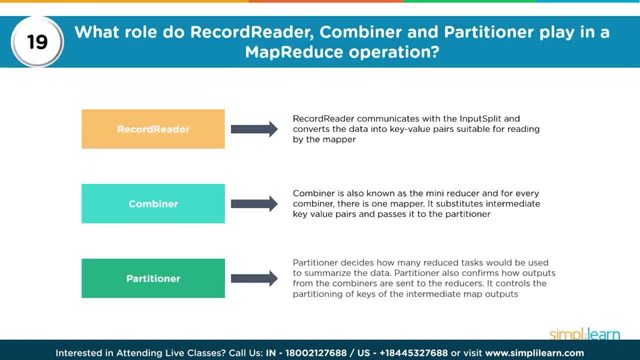 And it basically converts the data Into key value pairs, And these key value pairs Are the ones which will be worked upon By the mapper. Your combiner is an optional phase. It's like mini reduce, So combiner does not have it's own class. 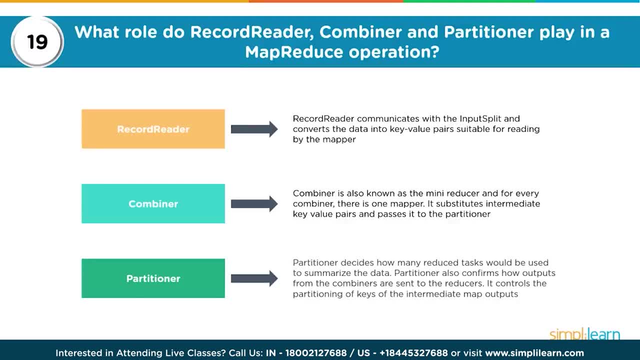 It relies on the reducer class. Basically, your combiner Would receive the data From your map task, Which would have completed Works on it Based on whatever reducer class mentions, And then passes it's output To the reducer phase. Partitioner is basically: 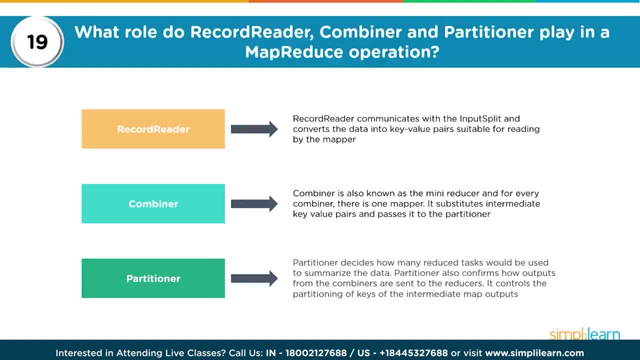 A phase which decides How many reduce tasks Would be used, Aggregate or summarize your data. So partitioner Is a phase which would decide. Based on the number of keys, Based on the number of map tasks, Your partitioner Would decide. 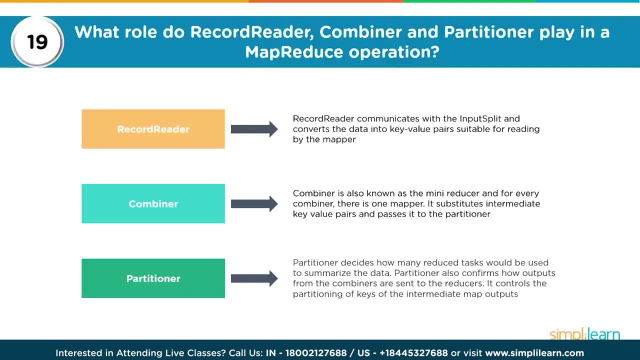 If one or multiple reduce tasks Would be used to take care of processing. So either it could be partitioner Which decides on how many reduce tasks would run, Or it could be based on the properties Which we have set within the cluster. 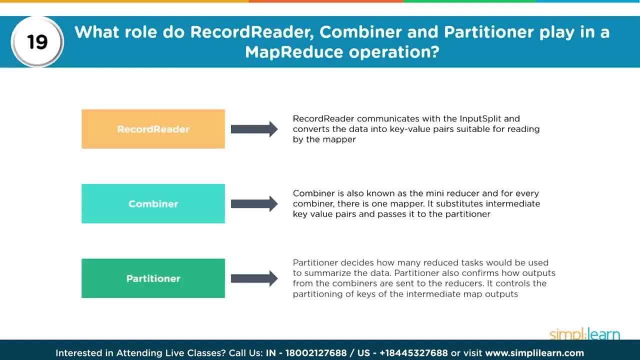 Which will take care of The number of reduce tasks which would be used. Always remember, your partitioner decides How outputs from combiner Are sent to reducer And to how many reducers. It controls the partitioning of keys Of your intermediate. 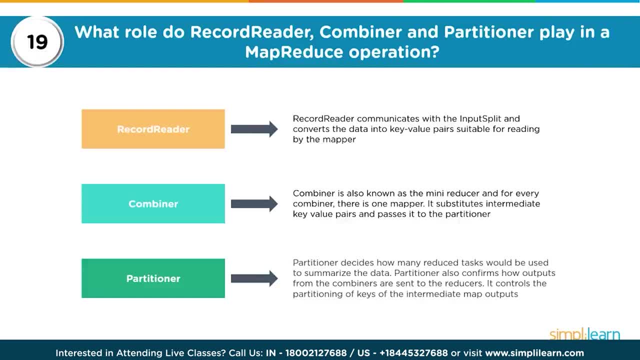 Outputs. So map phase, Whatever output it generates Is an intermediate output And that has to be taken by your partitioner Or by a combiner and then partitioner To be sent to one or multiple reduce tasks. This is one of the common questions. 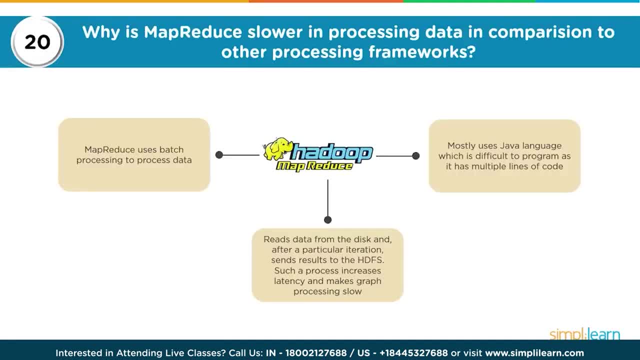 Which you might face. Why is map reduce slower In processing? So we know map reduce goes for parallel processing. We know we can have multiple map tasks Running on multiple nodes At the same time. We know that multiple reduce tasks could be running. 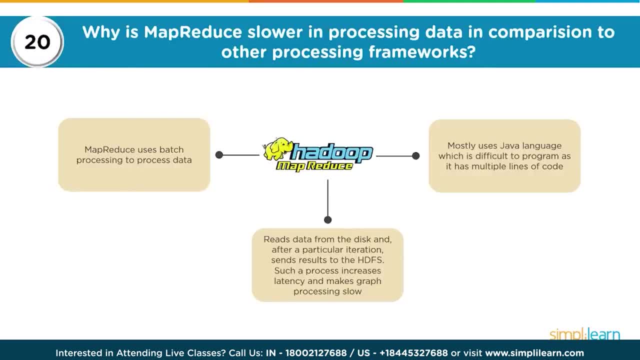 Now, why does then Map reduce become a slower approach? First of all, Your map reduce is a batch oriented operation. Now, map reduce Is very rigid And it strictly uses Mapping and reducing phases, So no matter what kind of processing. 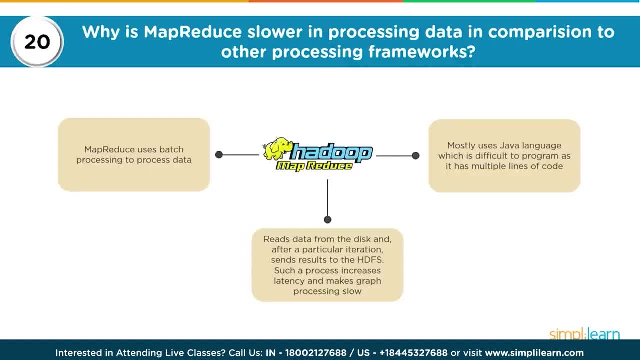 You would want to do, You would have to still provide the mapper function And the reducer function To work on data. Not only this, But also the mapper function. So when your map phase completes The output of your map phase, Which is an intermittent output, 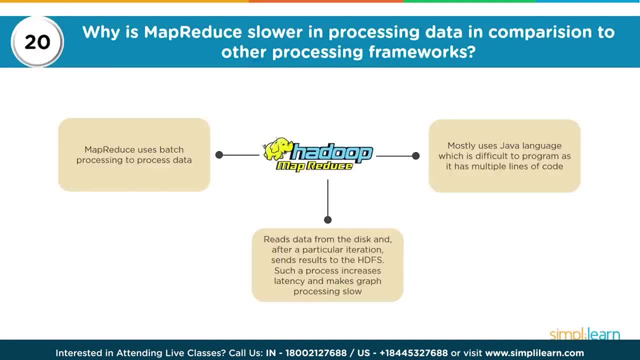 Would be written to HDFS And thereafter underlying disks And this data would then be shuffled And sorted And picked up for reducing phase. So every time your data being written to HDFS And retrieved from HDFS Makes map reduce a slower approach. 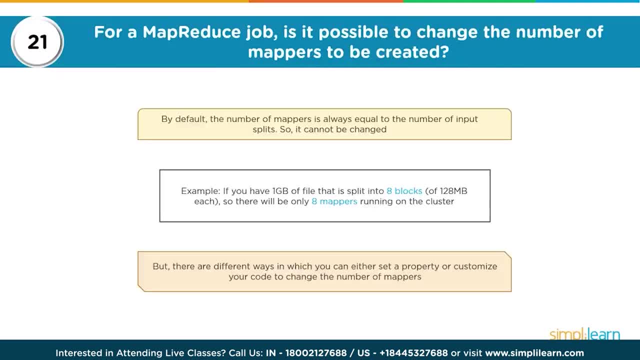 The question is: For a map reduce job, How do you control the number of mappers To be created Now? by default, You cannot change the number of map tasks, Because number of map tasks Depends on the input splits. However, 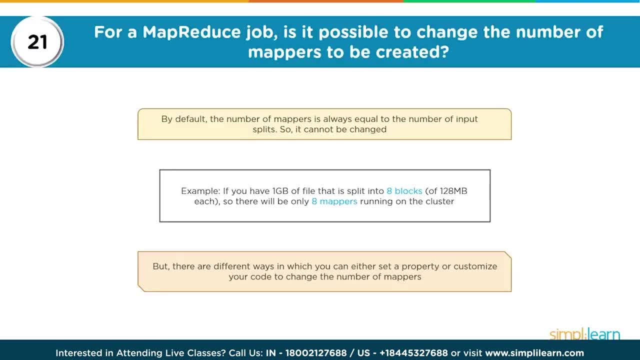 There are different ways In which you can either set a property To have more number of map tasks Which can be used, Or you can customize your code Or make it use A different format Which can then control the number of. 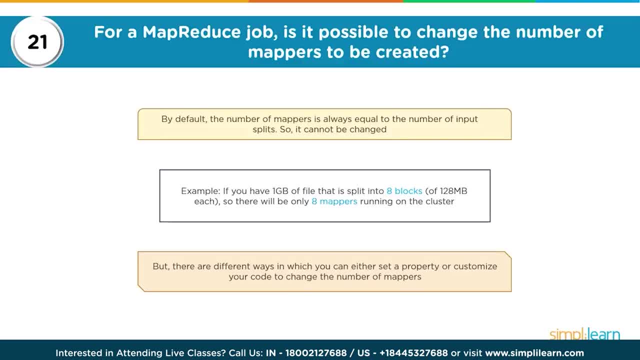 Map tasks. By default, Number of map tasks Are equal to the number of splits Of file you are processing. So if you have a 1GB of file That is split into 8 blocks of 128MB, There would be 8 map tasks. 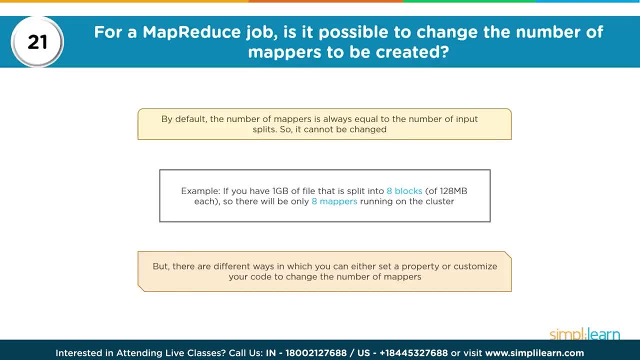 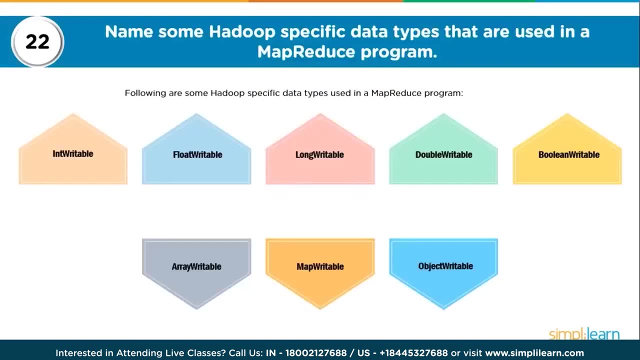 Running on the cluster. These map tasks Are basically running your mapper function. If you have hard coded Properties In your mapper-site file To specify more number of map tasks, Then you could control The number of map tasks. Let's also talk about some data types. 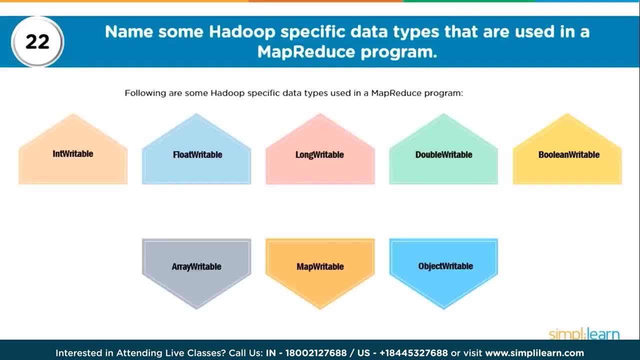 So when you prepare for Hadoop, When you want to get into big data field, You should start learning About different data formats. Now there are different data formats, Such as Avro Parquet. You have sequence file Or binary format. 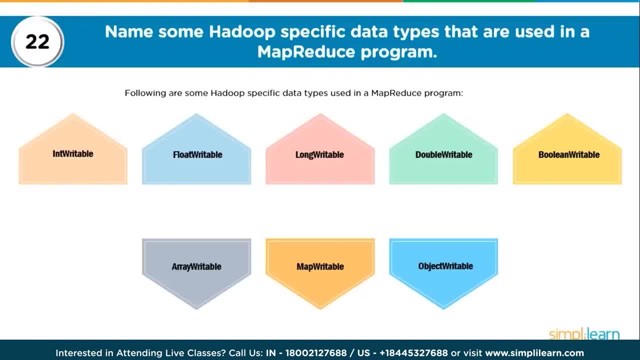 And these are different formats Which are used For different data types In Hadoop. These are implementation of your writable And writable comparable interfaces. So for every data type In Java You have equivalent in Hadoop. So int in Java would be int writable in Hadoop. 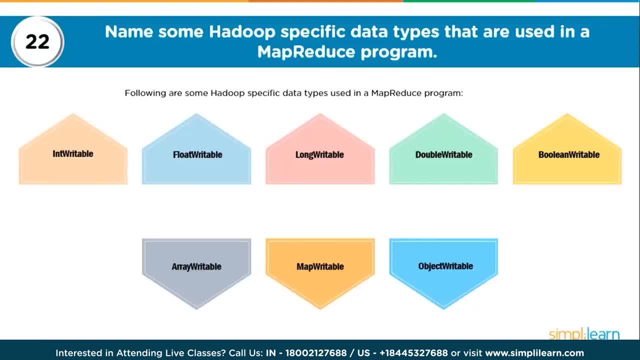 Float would be float writable, Long would be long. writable, Double writable, Boolean writable, Array writable, Map writable and object writable. So these are your different data types For your map reduce program And these are implementation of writable And writable comparable interfaces. 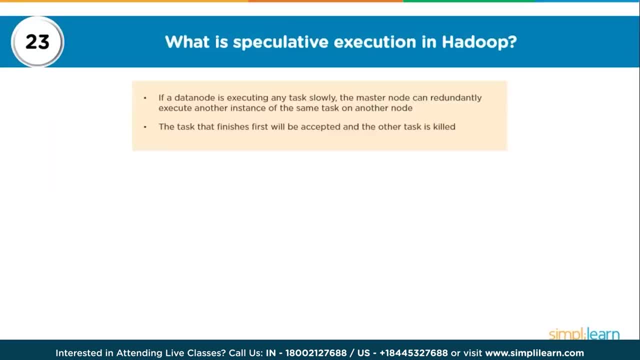 What is speculative execution? Now imagine You have a cluster Which has huge number of nodes And your data is spread across multiple slave machines Or multiple nodes. Now, at a point of time, Due to a disk degrade Or network issues, 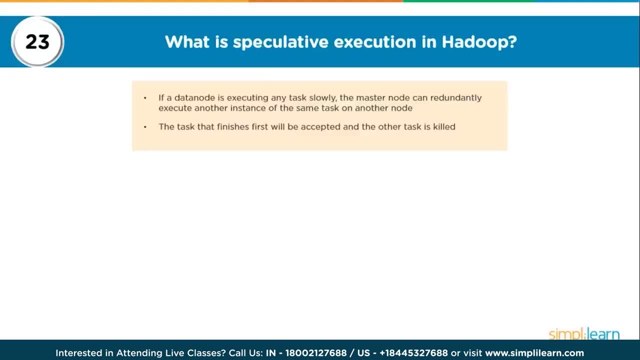 Or machine heating up Or more load being on a particular node, There can be a situation Where your data node Will execute task in a slower manner. Now, in this case, If speculative execution Is turned on, There would be a shadow task. 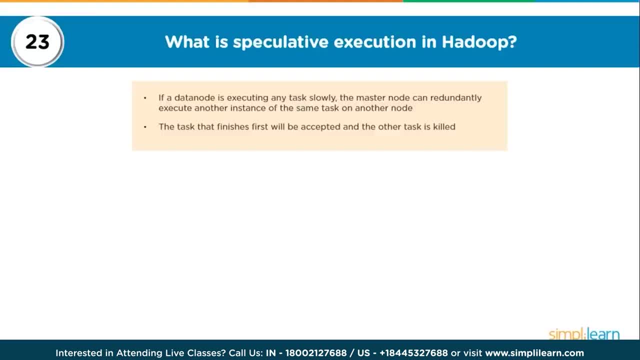 Or another similar task Running on some other node For the same processing. So whichever task finishes first Will be accepted And the other task would be killed. So speculative execution Could be good If you are working in an intensive work. 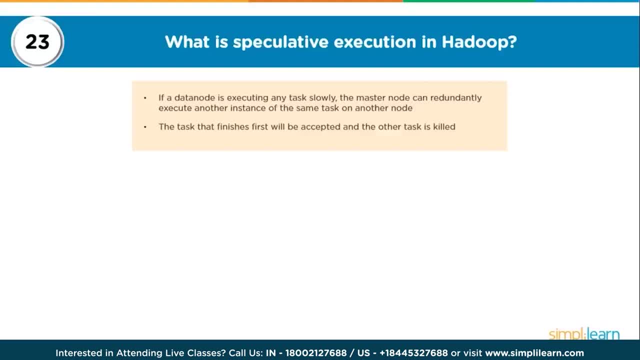 Load kind of environment Where, if a particular node is slower, You could benefit from A unoccupied Or a node which has less load To take care of your processing Going further. This is how we can understand. So node A: 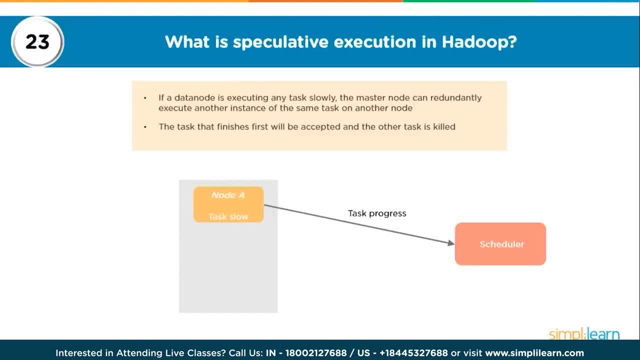 Which might be having a slower task. You would have a scheduler Which is maintaining or having knowledge Of what are the resources available. So if speculative execution As a property is turned on, The task which was running slow, A copy of that task. 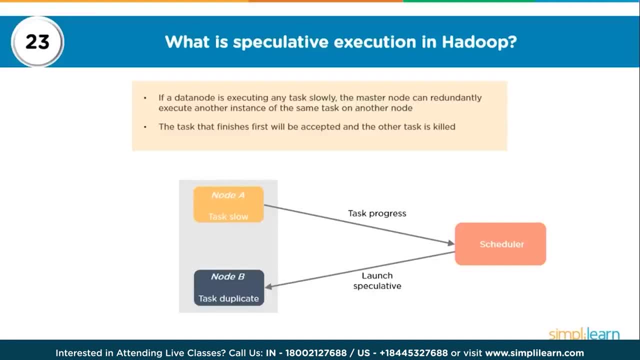 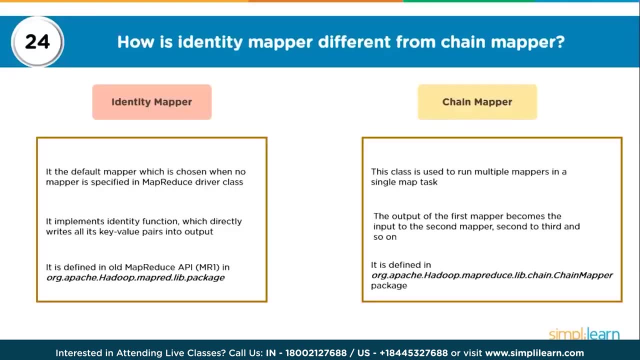 Or you can say a shadow task Would run on some other node, And whichever task completes first Will be considered. This is what happens in your speculative execution. Now, how is identity mapper Different from chain mapper? Now, this is where we are getting. 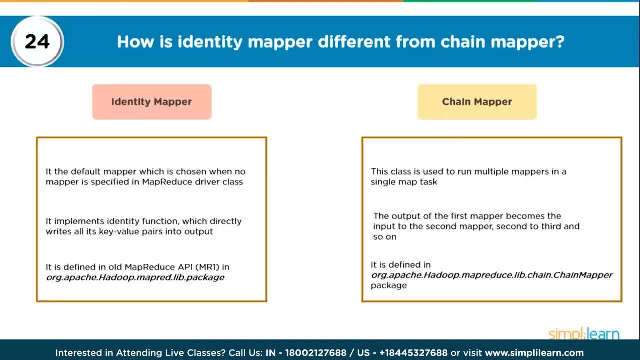 Deeper into MapReduce concepts. So when you talk about mapper Identity, mapper Is the default mapper Which is chosen And mapper is specified In MapReduce driver class. So for every MapReduce program You would have a map class. 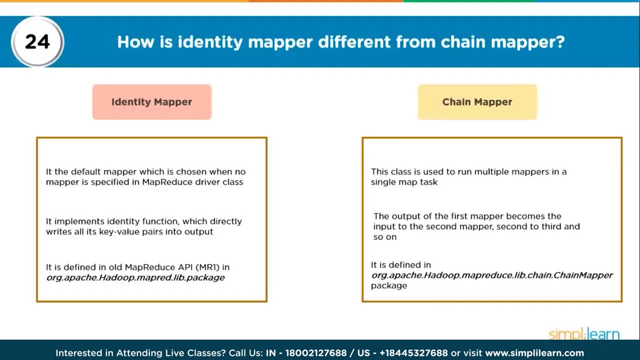 Which is taking care of your mapping phase, Which basically has a mapper function And which would run one or multiple map tasks Right. Your programming, Your program, would also have a reduce class Which would be running a reducer function Which takes care of reduce tasks. 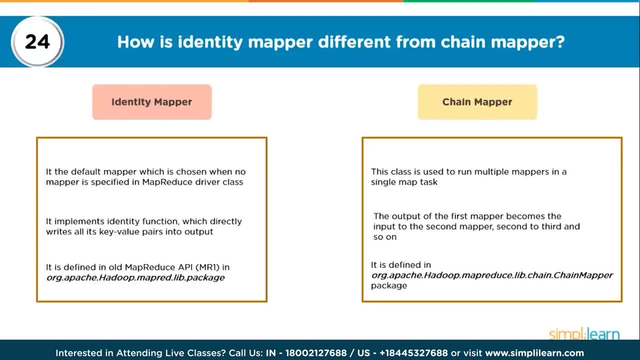 Running on multiple nodes Now, if a mapper Is not specified In your driver class? So driver class Is something which has all information about your flow. What's your map class? What is your reduce class? What's your input format? 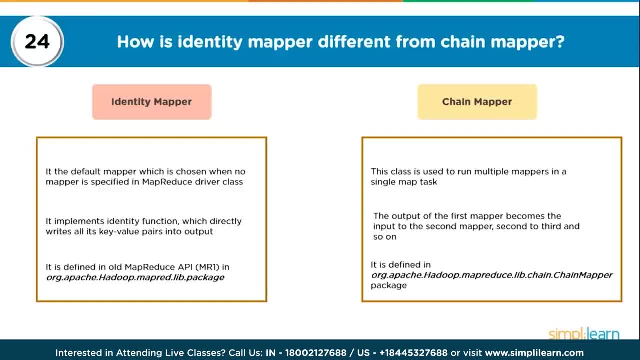 What's your output format, What are the job configurations and so on. So identity mapper is the default mapper Which is chosen when no mapper class is mentioned In your driver class. It basically implements an identity function Which directly writes all its key pairs. 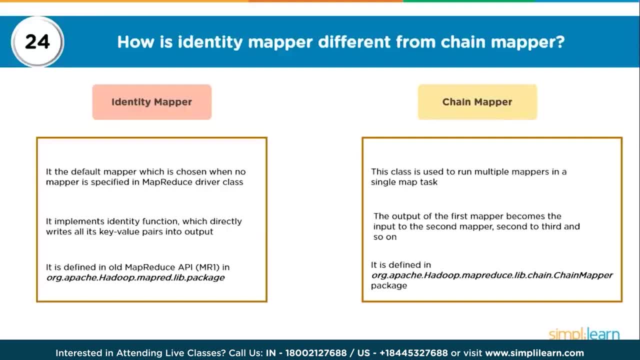 Into output. It was defined In old MapReduce API In this particular package. But when you talk about chaining mappers Or chain mapper, This is basically a class To run multiple mappers In a single map task. Or basically you could say: 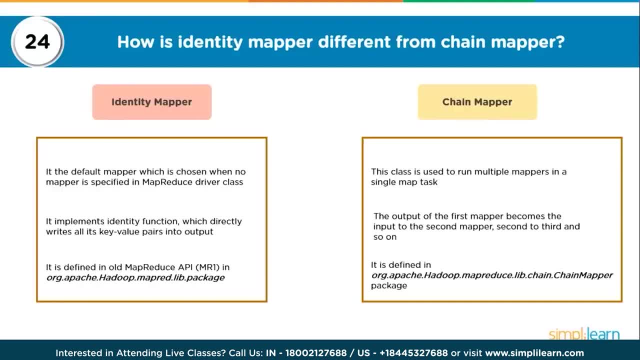 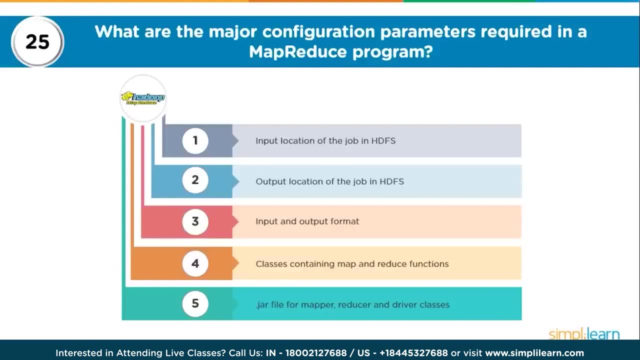 Multiple map tasks would run As a part of your processing. The output of first mapper Would become as an input to second mapper, And so on. The under mentioned class Or package. What are the major configuration parameters Required in a MapReduce program? 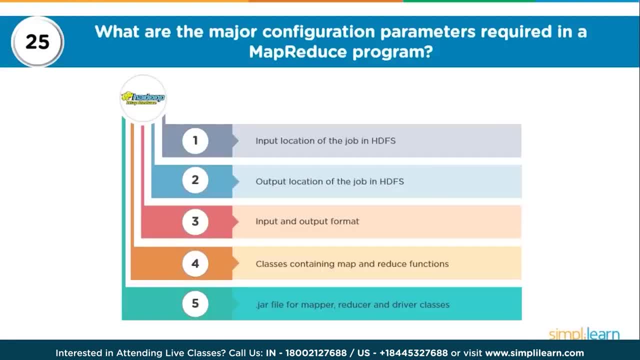 Obviously we need to have the input location. We need to have the output location. So input location is where The files will be picked up from, And this would preferably On HDFS directory. Output location is the path Where your job output would be written. 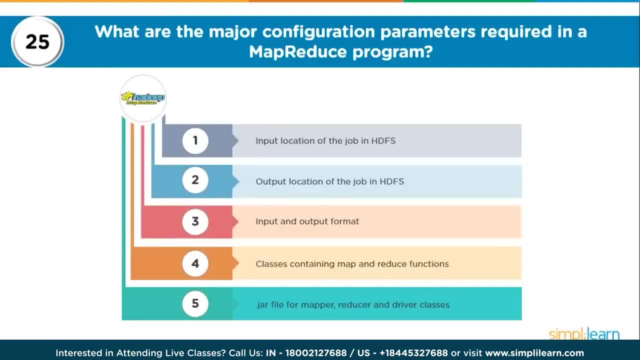 By your MapReduce program. You also need to specify Input and output formats. The defaults are considered. Then we need to also have The classes which have Your map and reduce functions And if you intend To run the code on a cluster. 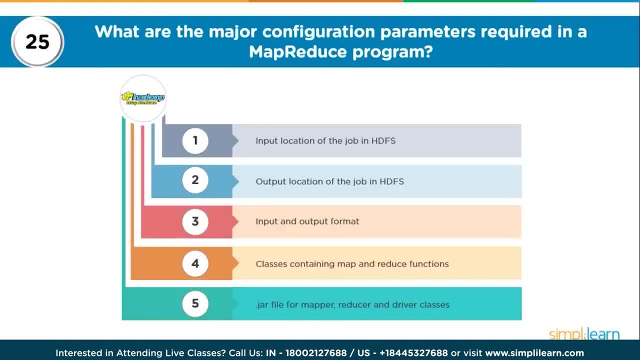 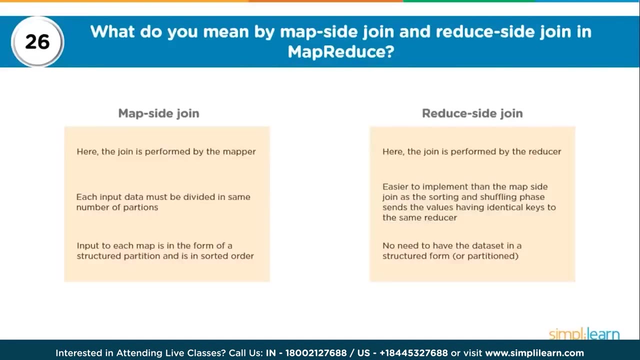 You need to package Your class in a jar file, Export it to your cluster And then this jar file would have Your mapper reducer and driver classes. So these are important Configuration parameters Which you need to consider For a MapReduce program. 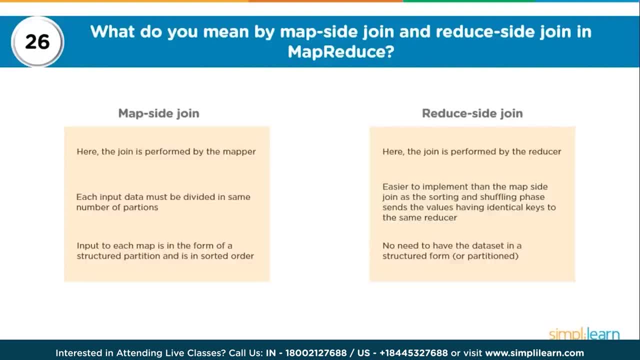 Difference, or what do you mean by MapSideJoin and ReduceSideJoin? MapSideJoin Is basically when the join is Performed at the mapping level, Or at the mapping phase, Or is performed by the mapper, So each input data 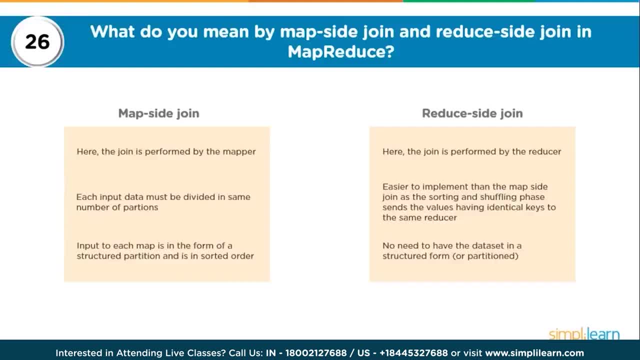 Which is being worked upon, Has to be divided into same Number of partitions. Input to each map Is in the form of a structured partition And is in sorted order, So MapSideJoin Can be used In a simple way. 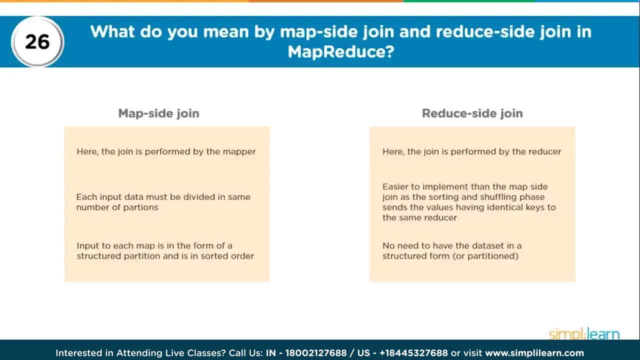 That if you compare it With RDBMS concepts, Where you had two tables Which were being joined, It will always be advisable To give your bigger table As the left side table Or the first table For your join condition. 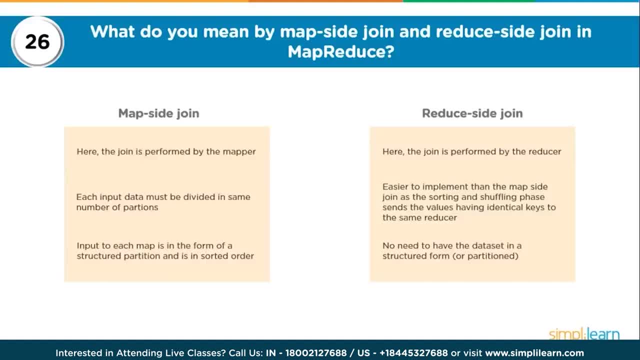 And it would be your smaller table On the left side And your bigger table On the right side. So MapSideJoin Is a similar kind of mechanism Where input data is divided Into same number of partitions. When you talk about ReduceSideJoin, 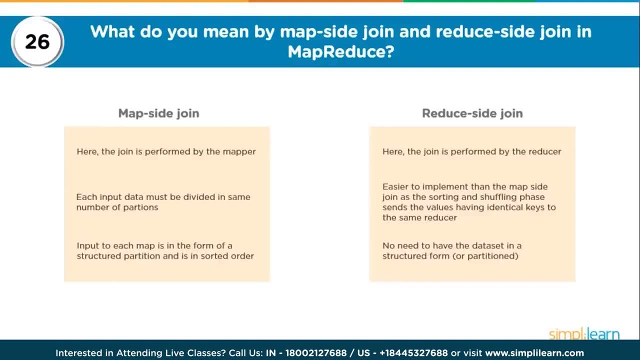 Here the join Is performed by the reducer, So it is easier to implement Than MapSideJoin, As all the sorting and shuffling Will send the values, Or send all the values Having identical keys To the same reducer. So look into your MapSideJoin. 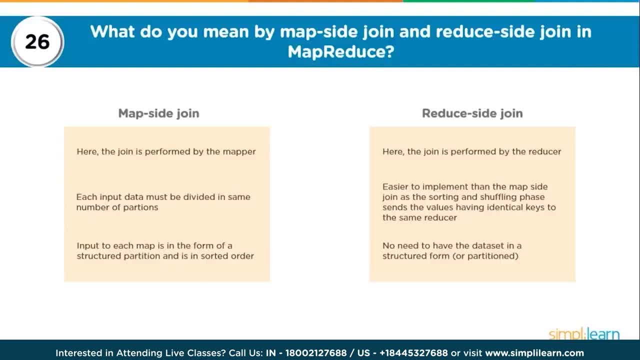 Or ReduceSideJoin And other joins, Just to understand how MapReduce works. However, I would suggest Not to focus more on this, Because MapReduce is still being used for processing, But the amount of MapReduce based processing Has decreased overall. 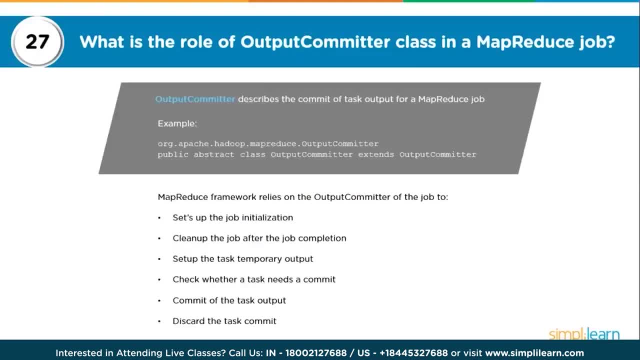 Or across the industry. Now, what is the role of Output Committer class in a MapReduce job? So Output Committer, As the name says, It is the role of task output For a MapReduce job, So we could have this as mentioned. 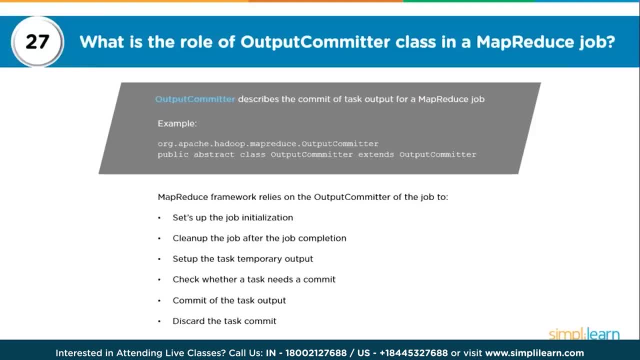 Or Apache Hadoop, MapReduce- Output Committer. You could have a class Which extends your Output Committer class. So MapReduce relies on this. MapReduce relies on the Output Committer of the job To set up the job initialization. 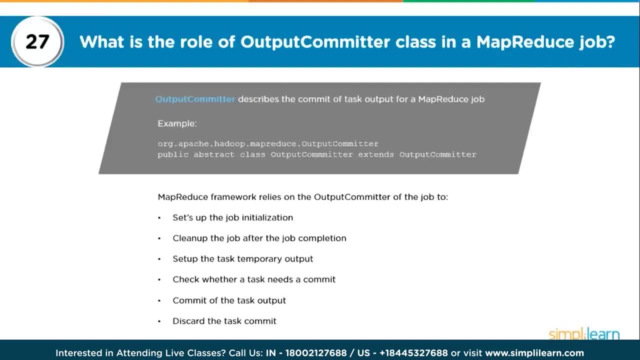 Cleaning up the job After the job completion. That means all the resources Which were being used by a particular job, Setting up the task, temporary output, Checking whether a task needs a commit, Committing the task output And discarding the task output. 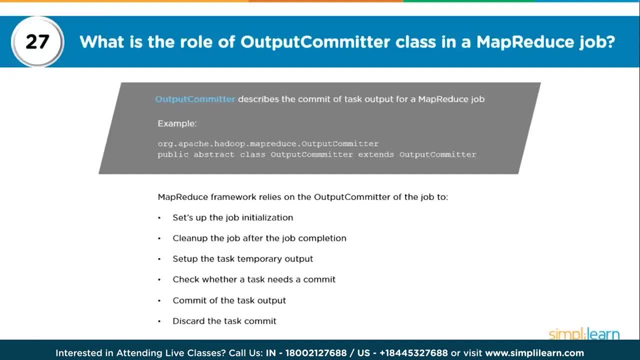 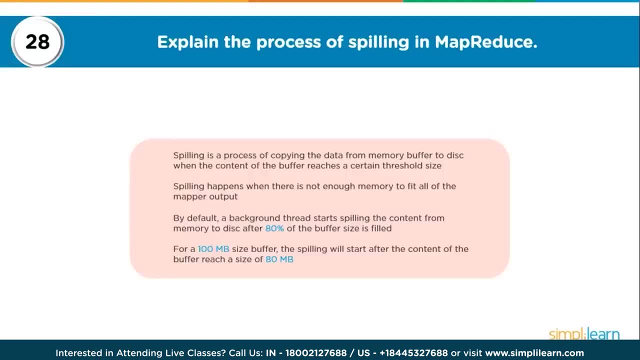 So this is a very important class And can be used within your MapReduce job. What is the process of spilling in MapReduce? What does that mean? So spilling is basically A process of copying the data From memory buffer to disk. 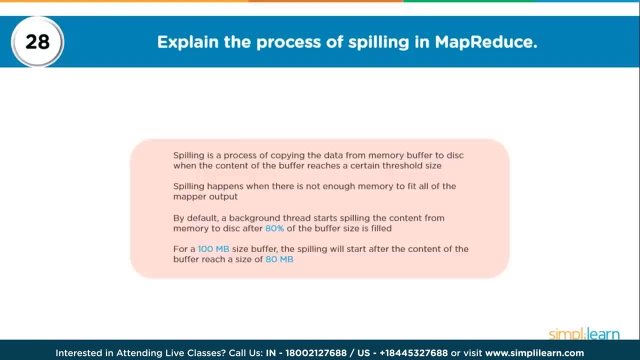 When obviously, The buffer usage Reaches a certain threshold. So if there is not enough memory In your buffer, Then the content Which is stored in buffer or memory Has to be flushed out. So by default A background thread starts. 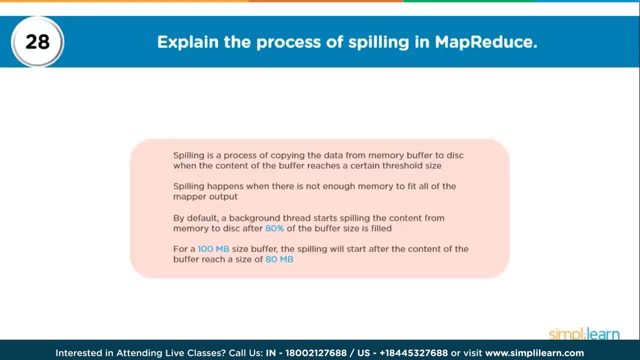 Spilling the content from memory to disk After 80% of buffer size is filled. Now, when is the buffer being used? So when your MapReduce processing is happening, The data is being read from the disk, Loaded into the buffer And then some processing happens. 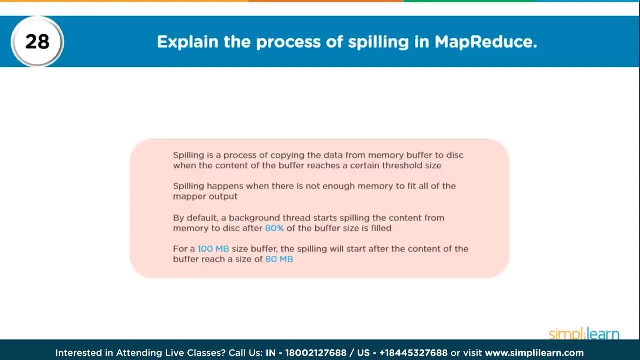 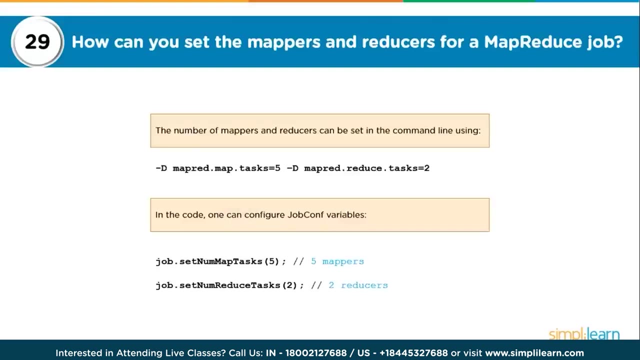 Same thing also happens When you are writing data to the cluster. So you can imagine: For a 100 MB size buffer, The spilling will start After the content of buffer Reaches 80 MB. This is customizable. How can you set the mappers and reducers? 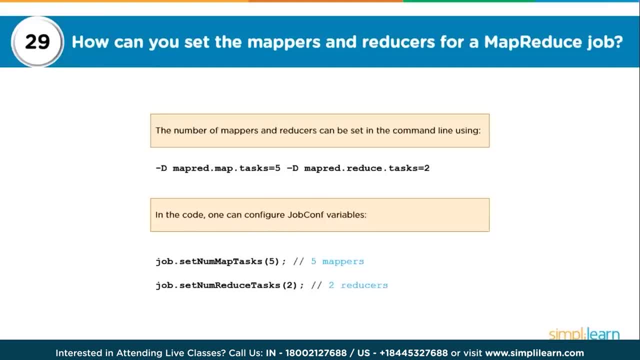 For a MapReduce job. So these are the properties. So number of mappers and reducers, As I mentioned earlier, Can be customized. So by default, Your number of map tasks Depends on the split And number of reduced tasks Can be used. 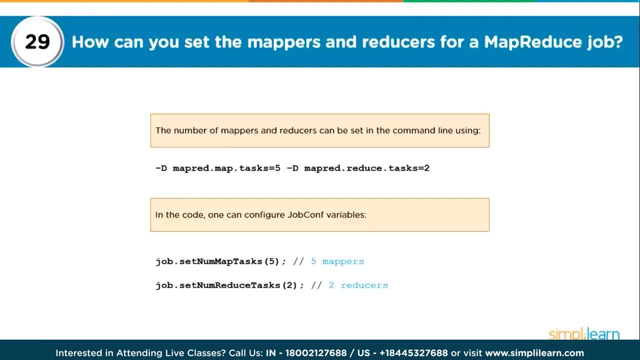 Depending on the keys. However, we can set these properties Either in the config files Or provide them on the command line, Or also make them part of our code, And this can control The number of map tasks Or reduced tasks Which would be run for a particular job. 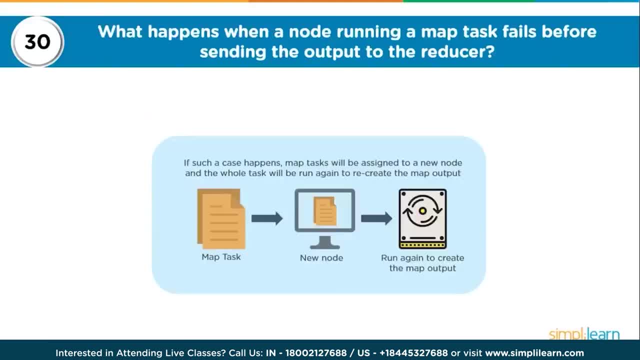 Let's look at one more interesting question: What happens when a node Running a map task fails Before sending the output to the reducer? So there was a node Which was running a map task And we know That there could be one or multiple map tasks. 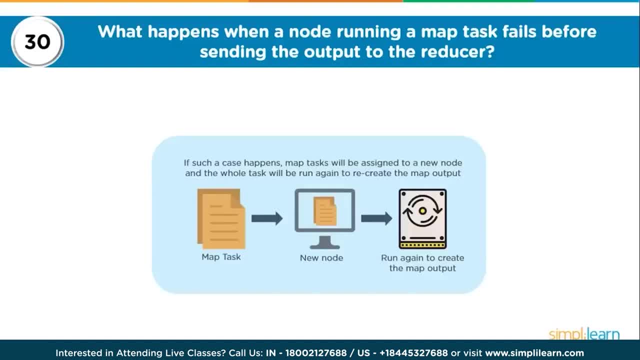 Running on one or multiple nodes And all the map tasks Have to be completed Before the further stages, Such as combiner or reducer, Come into existence. So in a case If a node crashes Where a map task was assigned to it, 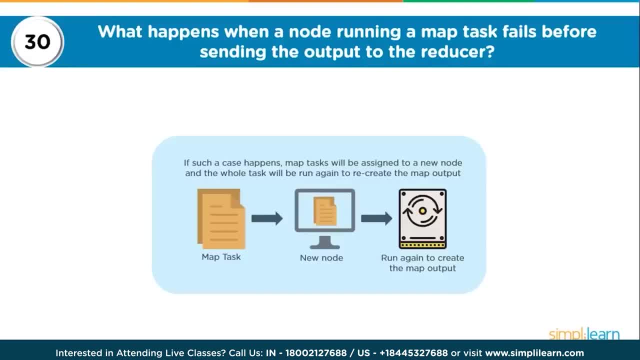 The whole task Will have to be run again. On some other node There is a temporary daemon Called application master. So your application master is taking care of Execution of your application And if a particular task On a particular node failed, 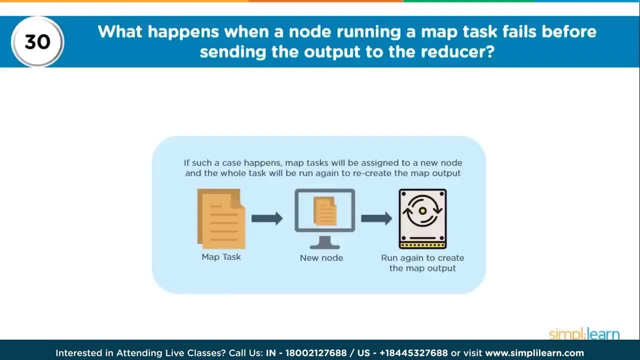 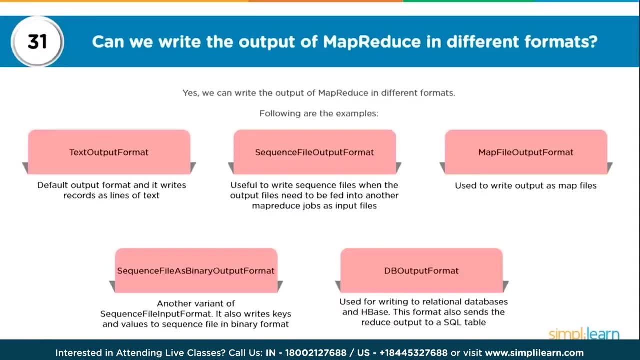 Due to unavailability of node. It is the role of application master To have this task Scheduled on some other node. Now can we write The output of MapReduce in different formats? Of course we can, So Hadoop supports Various input and output formats. 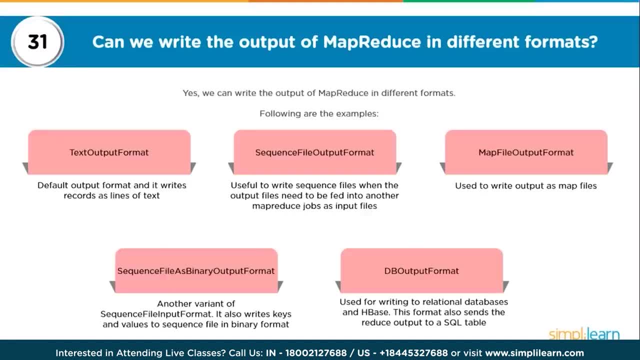 So you can write the output of MapReduce In different formats. So you could have the default format, That is, text output format, Where in records are written As line of text. You could have sequence file Which is basically to write sequence files. 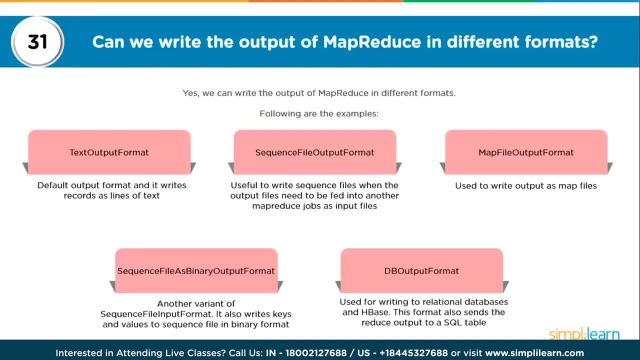 Or your binary format files Where your output files Need to be fed into another MapReduce jobs. You could go for a map file output format To write output as map files. You could go for a sequence file As a binary output format. 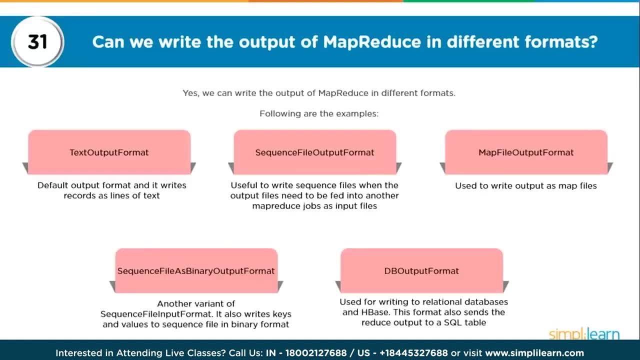 Your sequence file Input format. It basically writes keys and values To a sequence file. So when we talk about binary format, We are talking about a non human readable format, DB output format. Now, this is basically used When you would want to write data. 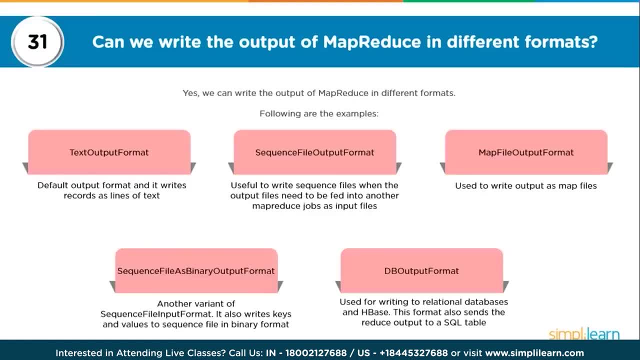 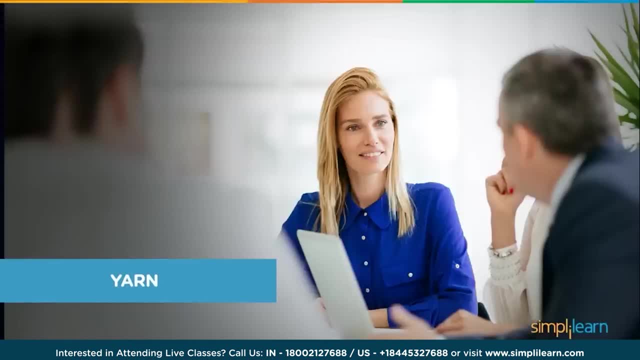 To say relational databases Or say no SQL databases such as HBase. So this format Also sends the Reduce output To a SQL table. Let's learn a little bit About YARN. YARN, which stands for yet another Resource negotiator. 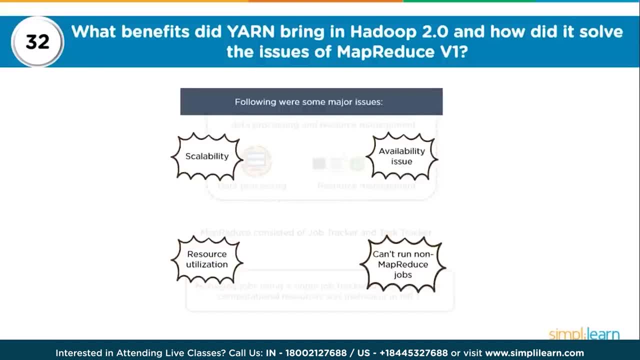 It's the processing framework. So what benefits did YARN bring in Hadoop version 2. And how did it solve the issues Of MapReduce version 1.. So MapReduce version 1 had major issues When it comes to scalability. 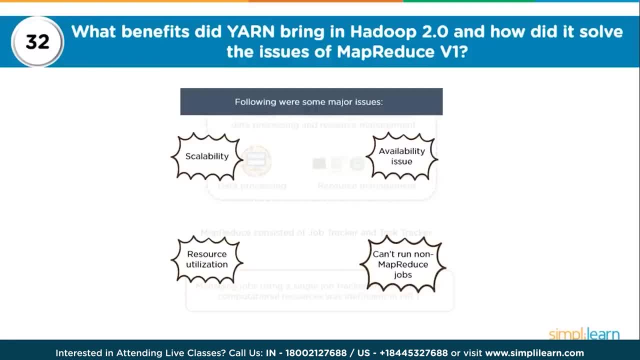 Or availability, Because, sorry, in Hadoop version 1. You had only one Master process for processing layer And that is your job track. So your job tracker Was listening to all the task trackers Which were running on multiple machines. So your job tracker 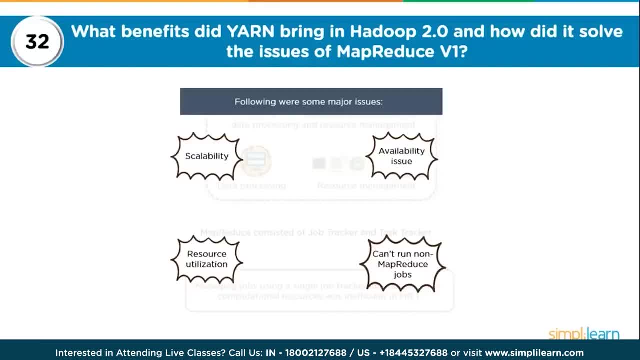 Was responsible for resource tracking And job scheduling. In YARN You still have a processing master, But that's called resource manager Instead of job tracker. And now with Hadoop version 2. You could even have resource manager Running in high availability mode. 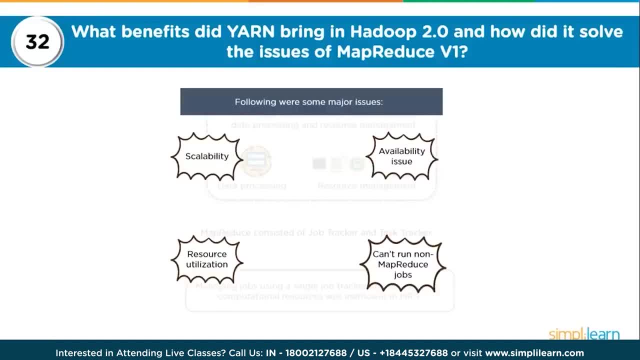 You have node managers Which would be running on multiple machines, And then you have a temporary daemon Called application master, So in case of Hadoop, version 2. Your resource manager or master Is only Handling the client connections And taking care of tracking the resources. 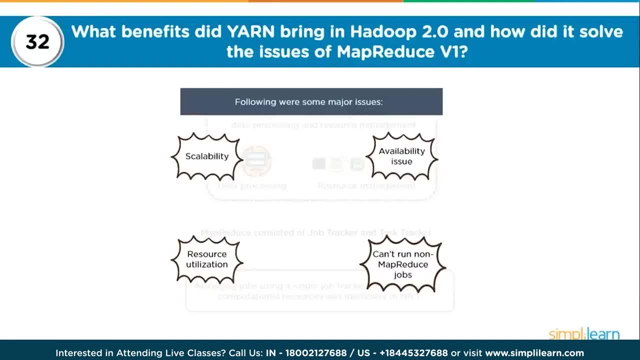 The job scheduling Or basically Taking care of execution Across multiple nodes, Is controlled by application master Till the application completes. So in YARN You can have different kind of Resource allocations. That could be done And there is a concept of container. 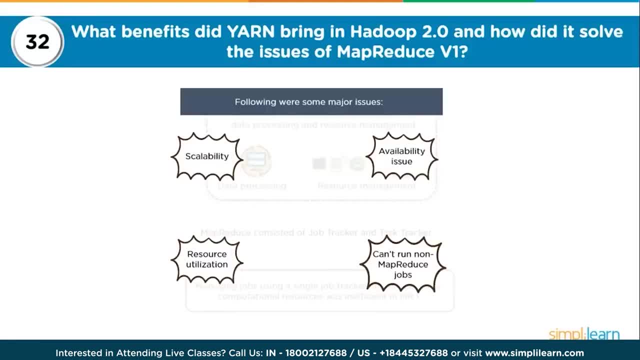 So container is Basically a combination of RAM and CPU cores. YARN can run different kind of workloads, So it is not just Map reduce kind of workload Which can be run on Hadoop version 2.. But you could have graph processing. 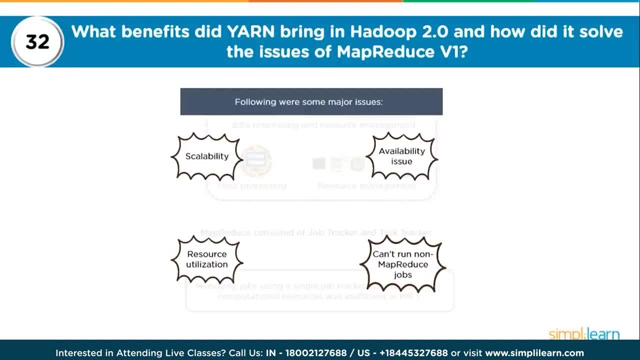 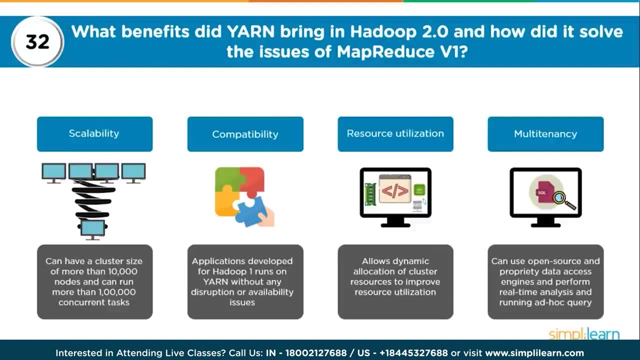 Massive parallel processing. You could have Real time processing And huge processing applications On a cluster based on YARN. So when we talk about scalability, In case of Your Hadoop version 2. You can have a cluster size of more than 10,000 nodes. 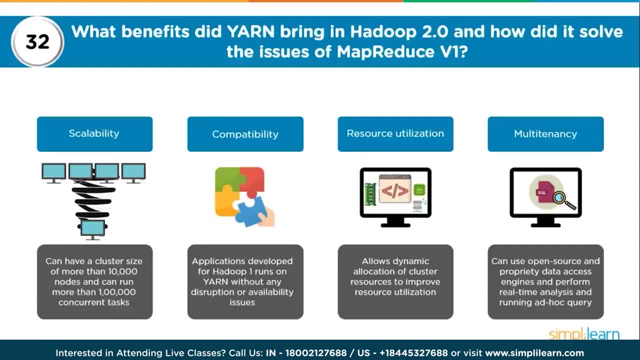 And can run more than 100,000 concurrent tasks. And this is because, For every application which is launched, You have this temporary daemon Called application master. So if I would have 10 applications running, I would have 10 app masters running. 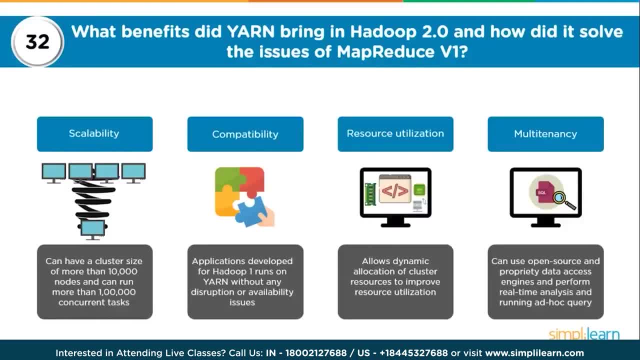 Taking care of execution Of these applications For multiple nodes Compatibility. So Hadoop version 2. Is fully compatible with whatever was developed As per Hadoop version 1. And all your processing needs Would be taken care by YARN. 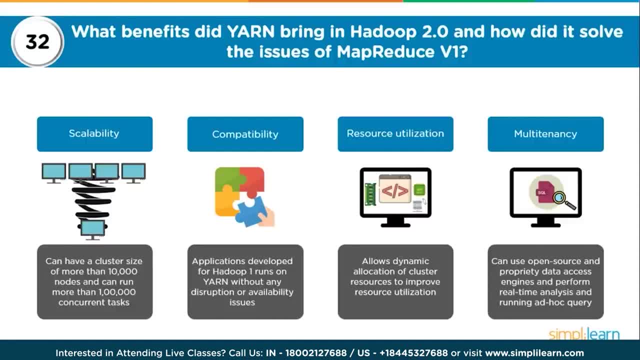 So dynamic allocation of cluster resources, Taking care of different workloads, Allocating resources across multiple machines And using them for execution- All that Is taken care by YARN Multi tenancy, Which basically means You could have multiple teams. 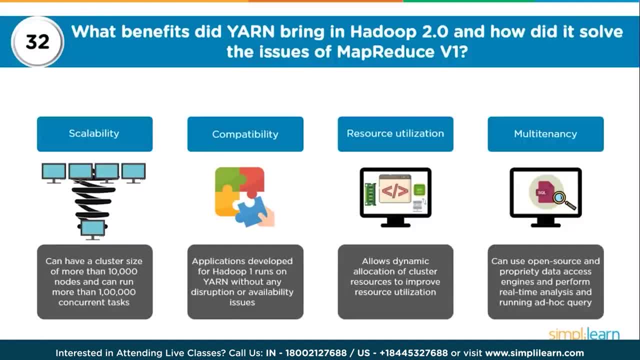 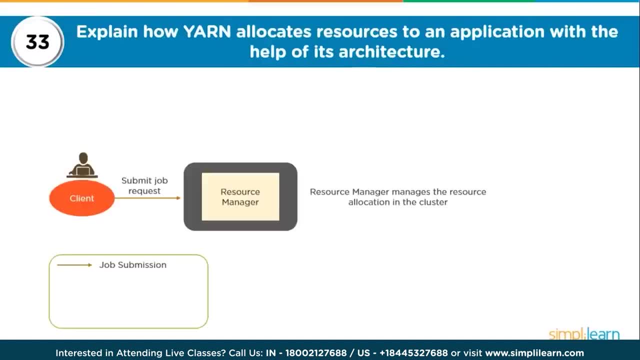 You could have open source And proprietary data access engines, And all of these could be Basically hosted Using the same cluster. Now, how does YARN allocate resources To an application With the help of its architecture? So, basically, you have a client. 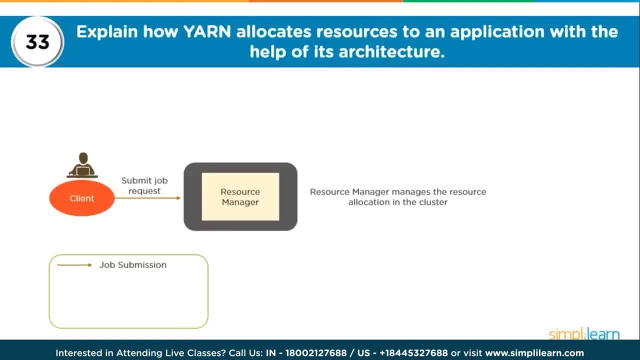 Or an application Or an API Which talks to resource manager. Resource manager is, as I mentioned, Managing the resource allocation In the cluster. When you talk about resource manager, You have its internal two components: One is your scheduler And one is your applications manager. 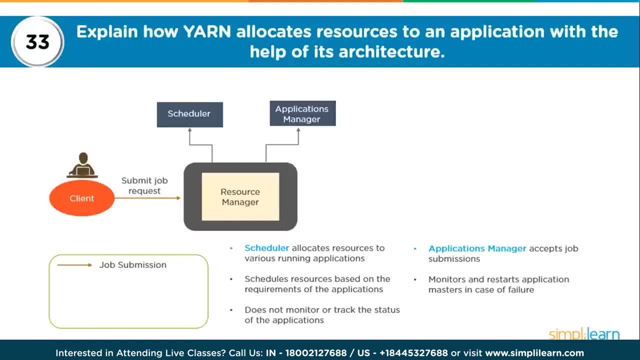 So when we say Resource manager, being the master Is tracking the resources, Resource manager is the one Which is negotiating the resources With slave. It is not actually resource manager Who is doing it, But these internal components. So scheduler is not bothered. 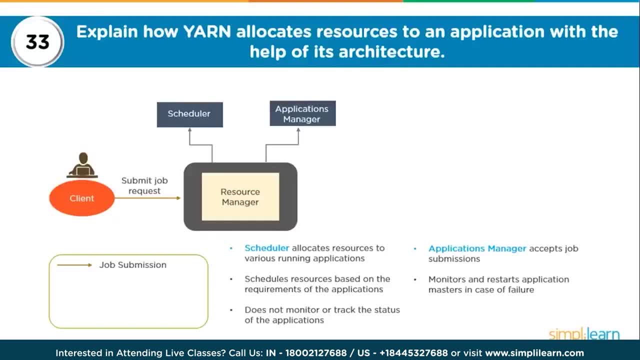 About tracking your resources Or basically tracking your applications. So we can have different kind of schedulers, Such as FIFO, Which is first in, first out. You could have a fair scheduler Or you could have a capacity scheduler, And these schedulers basically control. 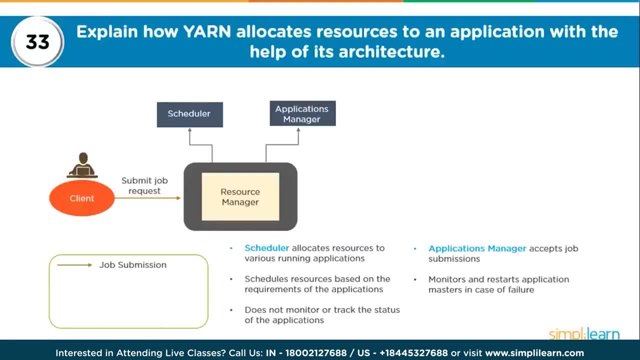 How resources Are allocated to multiple applications When they are running in parallel. So there is a queue mechanism. So scheduler Will schedule resources Based on requirements of application, But it is not monitoring Or tracking the status of applications. Your applications manager. 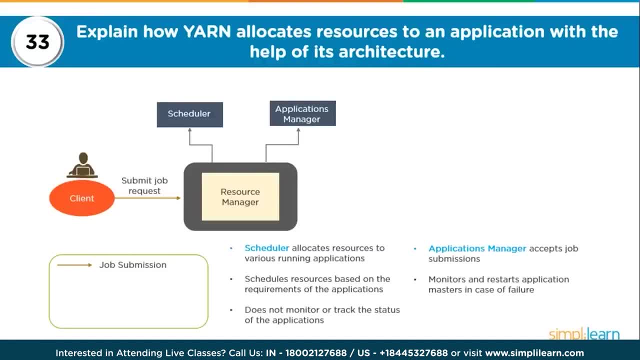 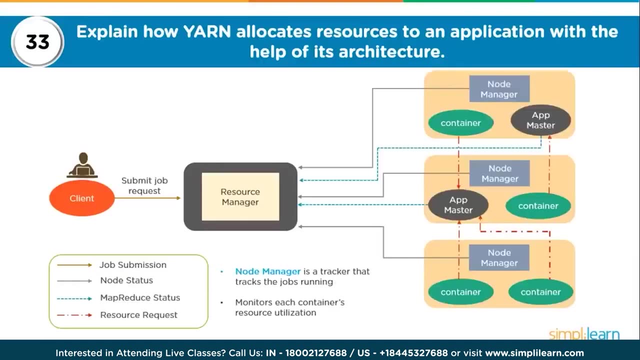 Is the one which is Accepting the job submissions. It is monitoring and restarting The application masters, So its application manager, Which is basically then launching A application master Which is responsible for an application. So this is how it looks. 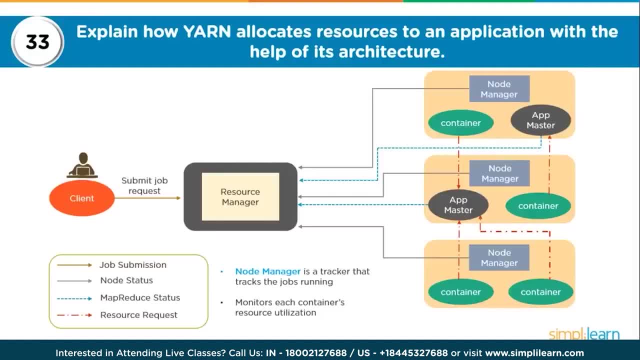 So whenever a job submission happens, We already know That resource manager Is aware of the resources Which are available With every node manager. So on every node Which has fixed amount of RAM and CPU cores, Some portion of resources, That is, your RAM and CPU cores. 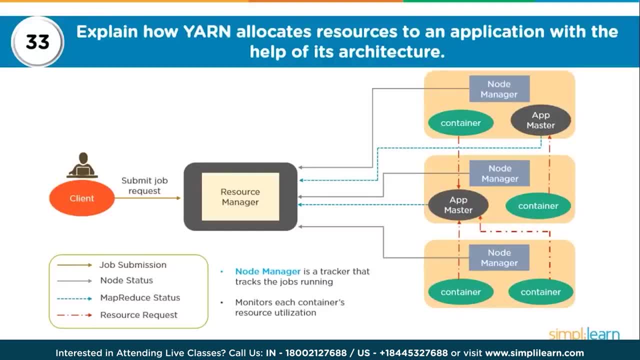 Are allocated to node manager. Now, resource manager Is already aware Of how much resources are available across nodes. So whenever a client request comes in, Resource manager Will make a request To node manager. It will basically request node manager To hold some resources. 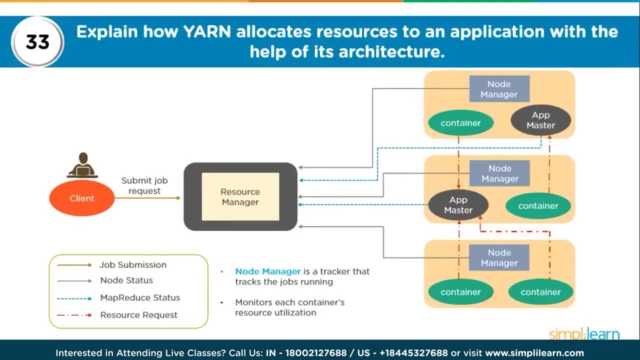 For processing Node manager would basically Approve or disapprove This request Of holding resources. And these resources, That is, a combination of RAM and CPU cores, Are nothing but containers. We can allocate containers of different sizes Within yarn hyphen site file. 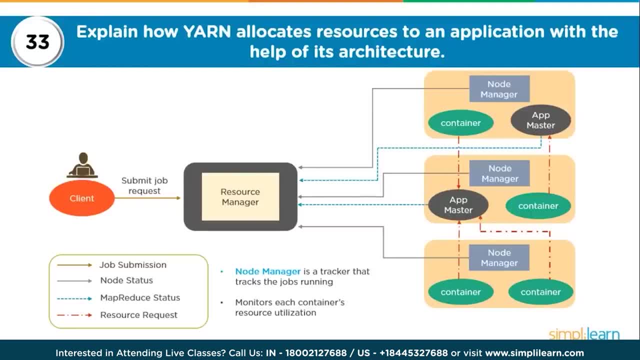 So your node manager, Based on a request from resource manager, Guarantees the container Which would be available for processing. That's when your resource manager Starts a temporary daemon, Called application master, To take care of your execution. So your app master. 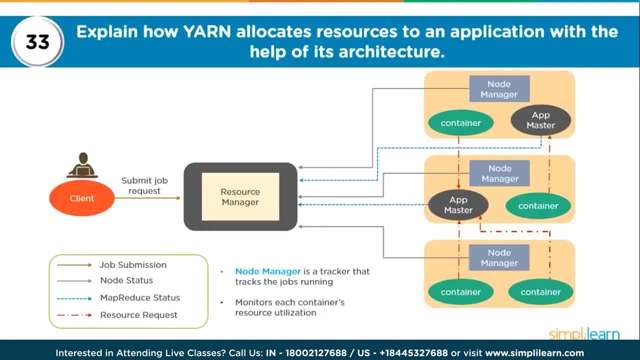 Which was launched by resource manager, Or we can say Internally by applications manager, Will run in one of the containers, Because application master is also a piece of code. So it will run in one of the containers And then Other containers will be utilized. 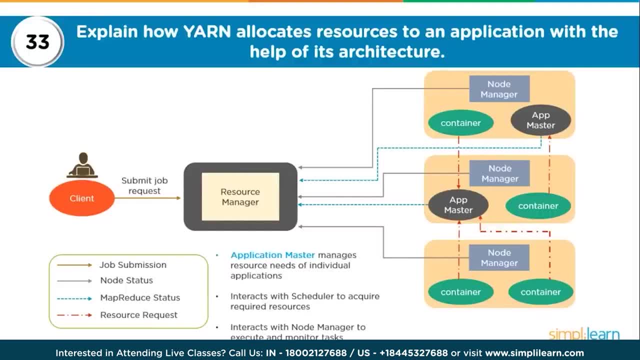 For execution. This is how yarn is basically Taking care of your allocation. Your application master Is managing resource needs. It is the one which is interacting with scheduler, And if a particular Node crashes, It is the responsibility of app master. 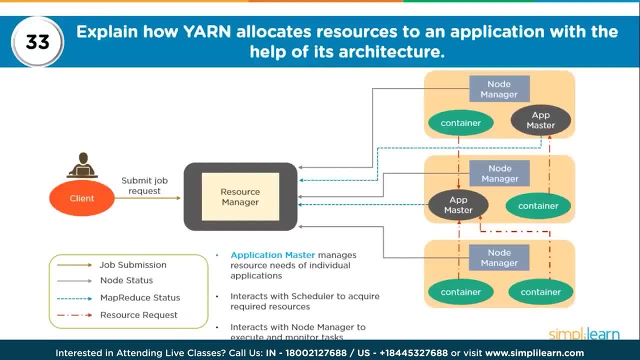 To go back to the master, Which is resource manager, And negotiate for more resources. So your app master will never, Ever negotiate resources With node manager directly. It will always talk to resource manager And resource manager is the one Which negotiates the resources. 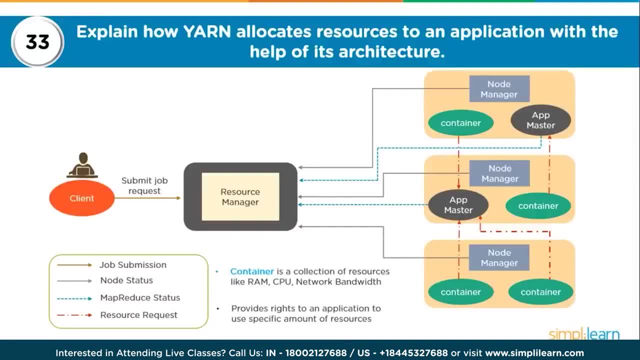 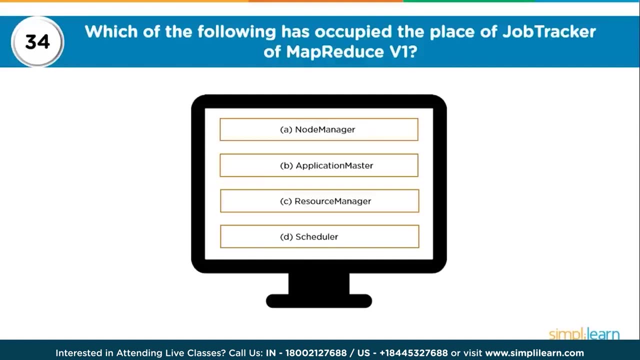 Container, as I said, Is a collection of resources Like your RAM, CPU, Network bandwidth, And your container is allocated Based on the availability of resources On a particular node. So which of the following has occupied The place of a job tracker? 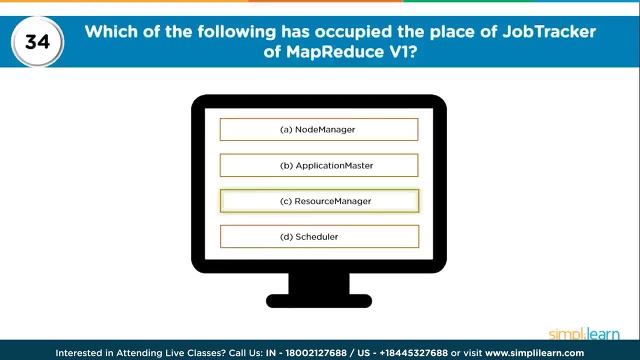 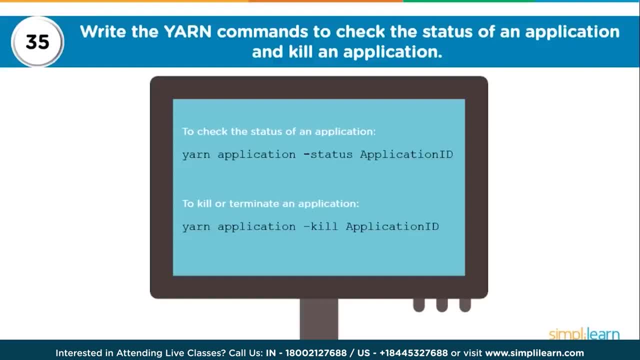 Of MapReduce. So it is your resource manager. So resource manager is the name Of the master process in Hadoop version 2.. Now if you would have to Write yarn commands To check the status of an application, We could just say yarn. 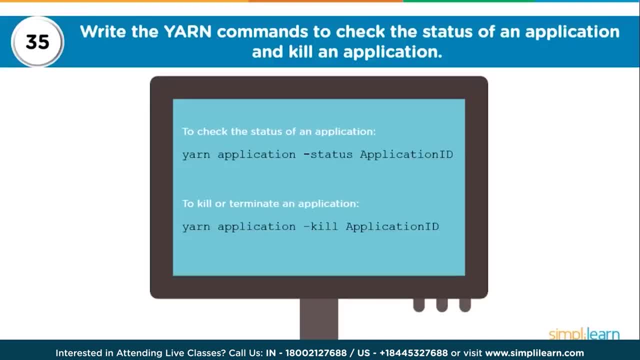 Application minus status And then the application id And you could kill it also from the command line. Remember, your yarn Has a UI And you can even look at your applications from the UI. You can even kill your Applications from the UI. 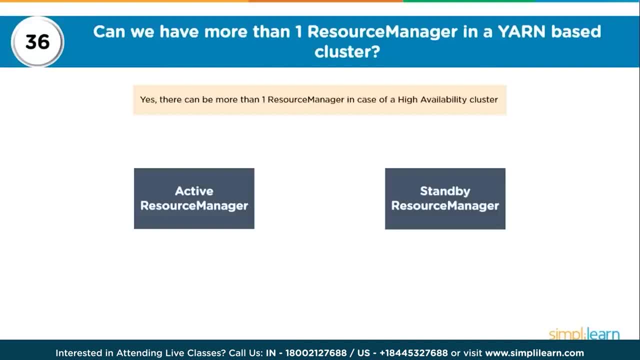 However, knowing the command line commands Is very useful. Can we have more than one resource manager In a yarn based cluster? Yes, we can. That is what Hadoop version 2 allows us to have, So you can have a high availability yarn cluster. 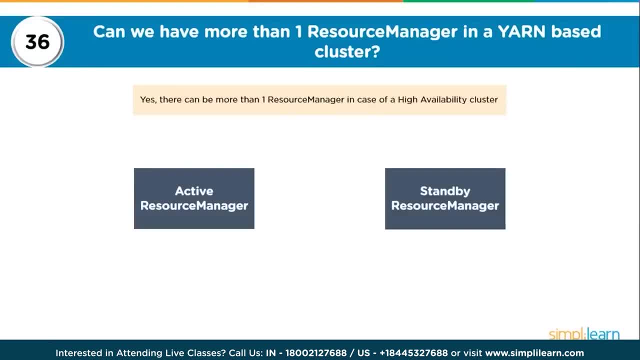 Where you have an active and standby And the coordination Is taken care by your zookeeper At a particular time. There can only be One active resource manager And if active resource manager fails, Your standby resource manager comes And becomes active. 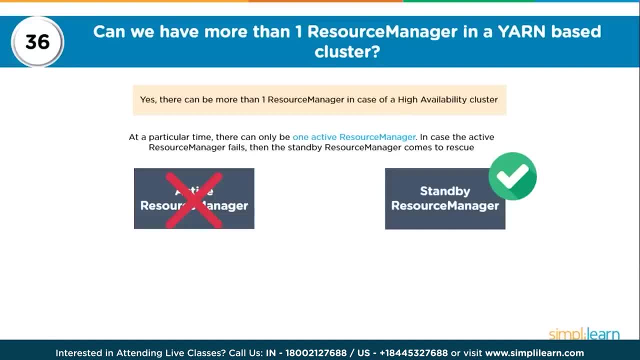 However, zookeeper is playing a very important role. Remember, Zookeeper is the one which is coordinating The server state And it is doing the election of active To standby. failover. What are the different schedulers available in yarn? So you have a FIFO scheduler. 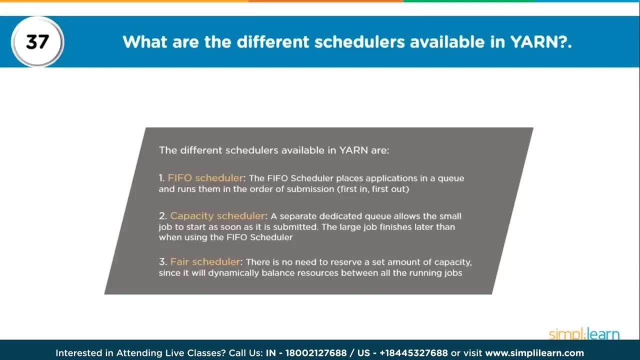 That is first in, first out, And this is not A desirable option Because in this case A longer running application Might block all other small running applications. Your capacity scheduler Is basically a scheduler Where dedicated queues Are created And they have fixed amount of resources. 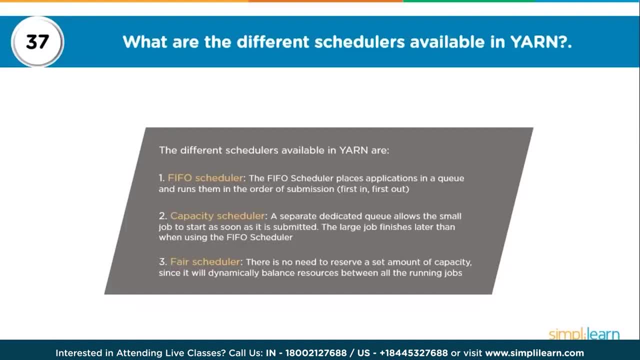 So you can have multiple applications Accessing the cluster At the same time And they would be using their own queues And the resources allocated to them. If you talk about fair scheduler, You don't need to Have a fixed amount of resources. 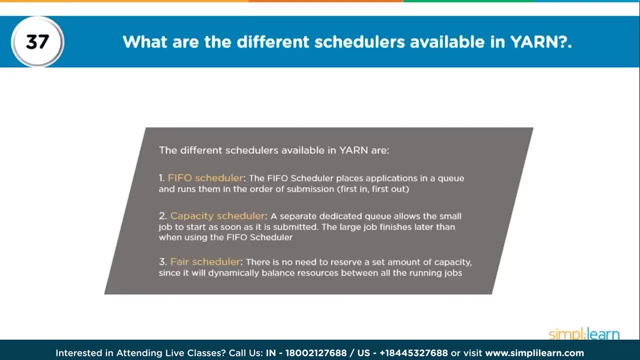 You can just have a percentage And you could decide What kind of fairness is to be followed, Which basically means that If you were allocated 20 gigabytes of memory, However, the cluster has 100 gigabytes And the other team was assigned. 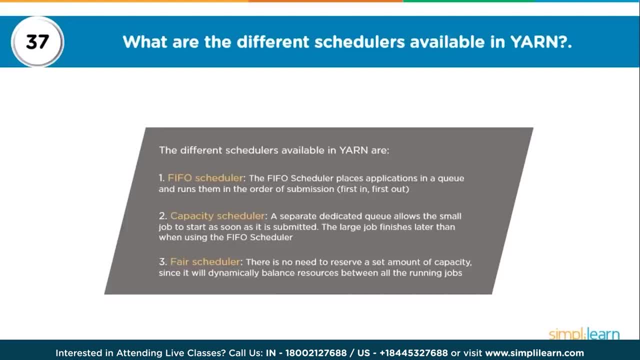 80 gigabytes of memory, Then you have 20% access to the cluster And other team has 80%. However, if the other team does not come up Or does not use the cluster, In a fair scheduler You can go up to maximum. 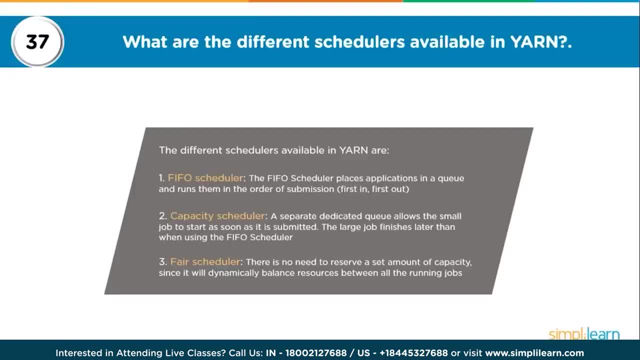 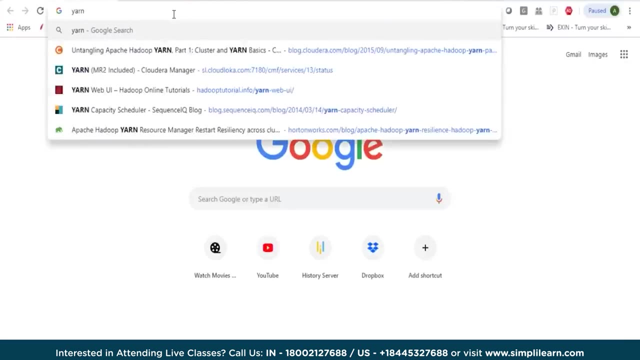 100% of your cluster. To find out more information About your schedulers, You could either look in Hadoop definitive guide, Or what you could do is You could just go to Google And you could type, for example, Yarn scheduler. 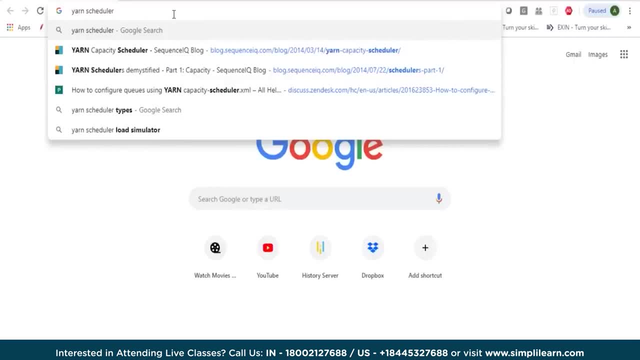 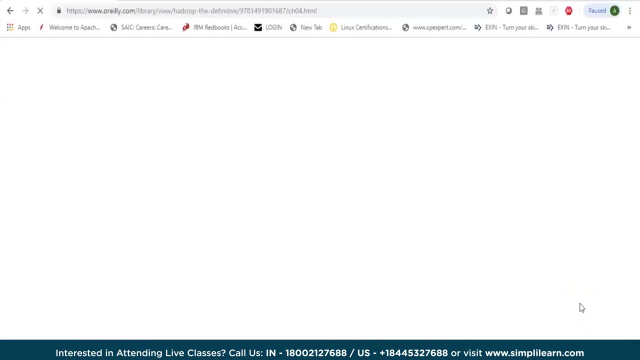 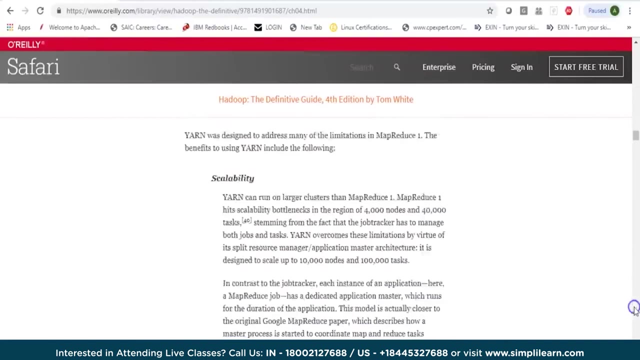 Let's search for yarn scheduler And then you can look in Hadoop definitive guide, And So this is your Hadoop definitive guide, And it beautifully explains About your different schedulers. How do multiple applications run, And that could be. 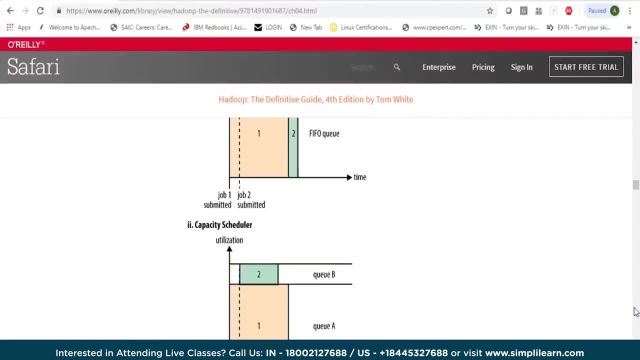 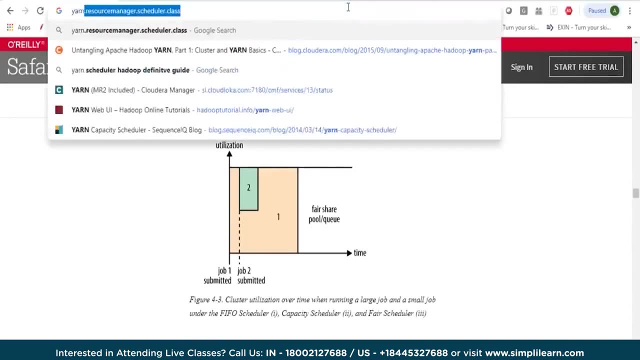 FIFO kind of scheduling. It could be in capacity scheduler Or it could be in a fair scheduling. So have a look at this link. It's a very good link. You can also search for yarn untangling And this is a blog of four. 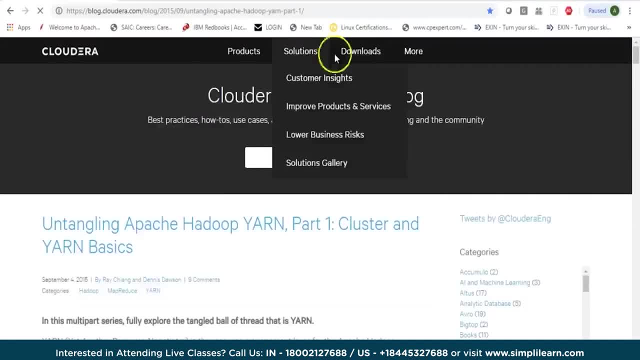 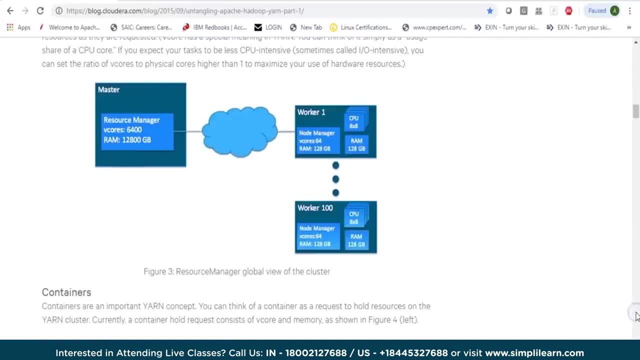 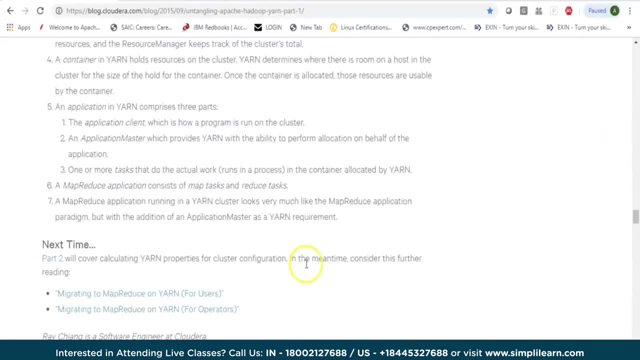 Or this is a series of four blogs Where it's beautifully explained About your yarn, How it works, How the resource allocation happens, What is a container And what runs within the container. Reading through this, And you can then also search for part two of it. 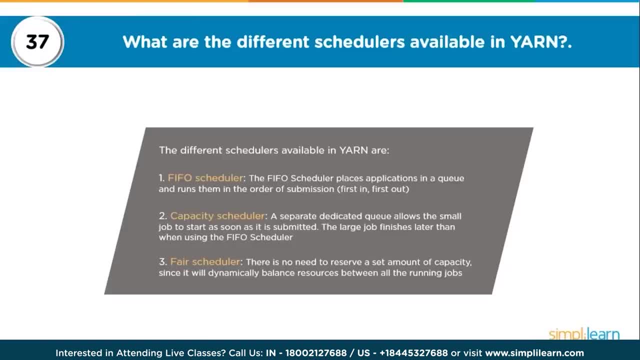 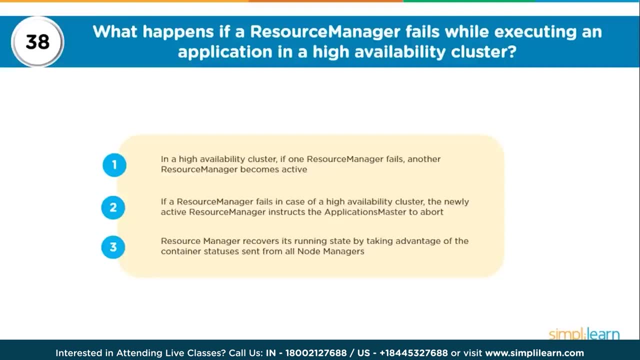 Which talks about allocation And so on. So, coming back, We basically have these schedulers. What happens if a resource manager fails While executing an application In a high availability cluster? So, in a high availability cluster, We know that we would have two resource managers. 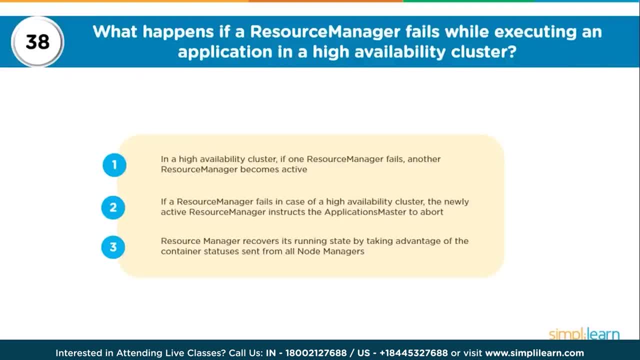 One being active, One being standby And zookeeper, which is keeping a track of the server states. So if a RM fails In case of high availability, The standby Will be elected as active And then basically Your resource manager or the standby. 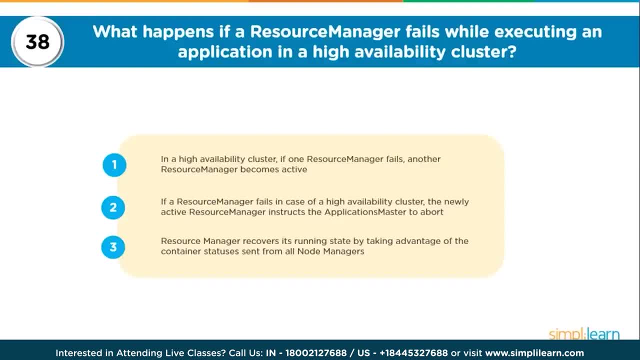 Would become the active one, And this one would instruct the application master To abort In the beginning. Then your resource manager recovers It's running state. So there is something called as RM state store, Where all the applications which are running 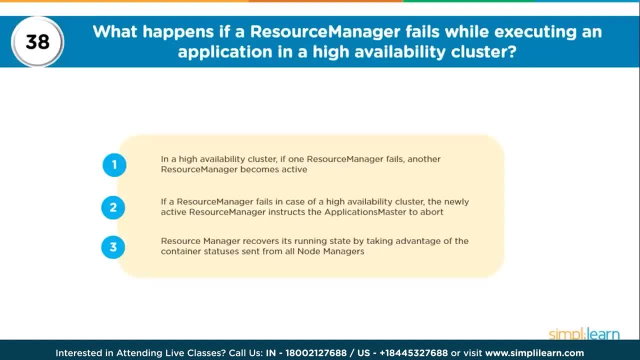 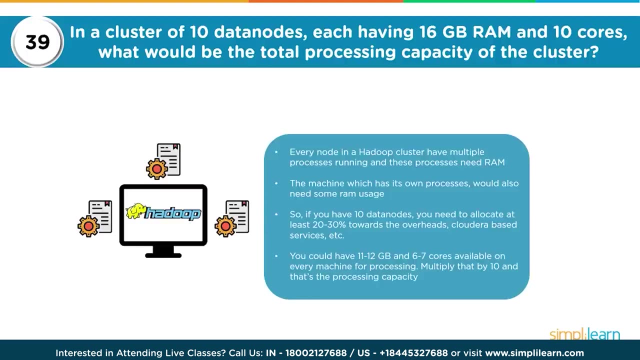 Their status is stored. So resource manager recovers The running state By looking at your state store, By taking advantage of container statuses, And then continues To take care of your processing, Now in a cluster of 10 data nodes, Each having 16 GB. And 10 cores, What would be total processing capacity Of the cluster? Take a minute to think. 10 data nodes, 16 GB RAM Per node, 10 cores. So if you mention the answer As 160 GB RAM And 100 cores, 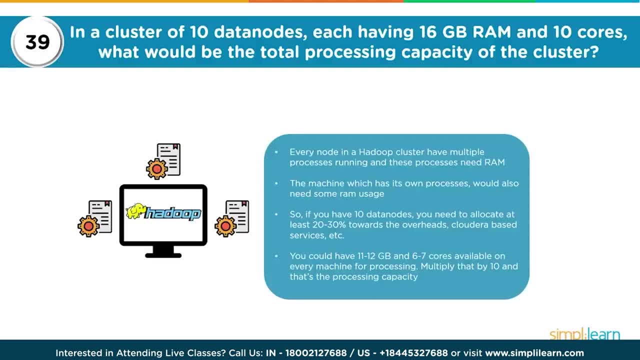 Then you went wrong. Now think of a cluster which has 10 data nodes, Each having 16 GB RAM And 10 cores. Remember, on every node In a Hadoop cluster You would have one or multiple processes running. Those processes would need RAM. 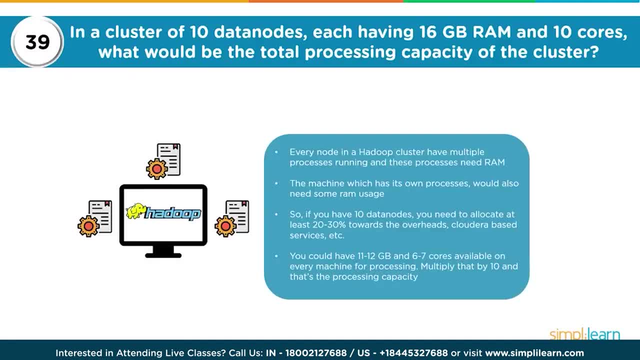 The machine itself, Which has a Linux file system, Would have its own processes. So that would also be having some RAM usage, Which basically means That if you talk about 10 data nodes, You should deduct at least 20 to 30%. Towards the overheads, Towards the cloud database services, Towards the other processes which are running, And in that case I could say That you could have 11 or 12 GB Available on every machine for processing And say 6 or 7 cores. 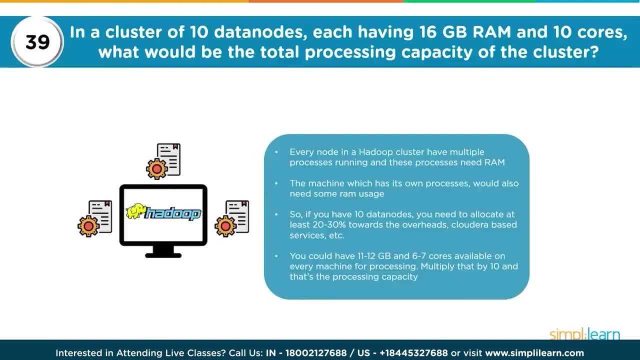 Multiply that by 10. And that's your processing capacity. Remember, the same thing applies To the disk usage also. So if somebody asks you: In a 10 data node cluster Has 20 TB of disks, What is my total storage capacity? 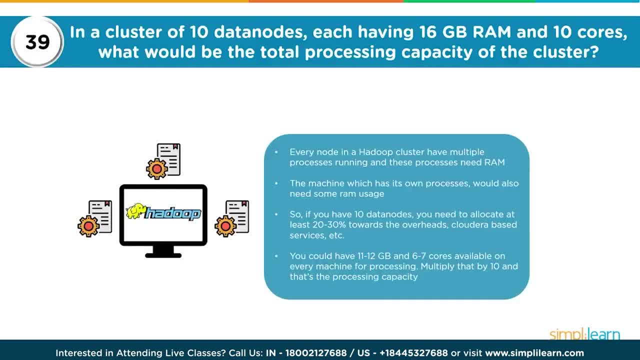 Available for HDFS. So the answer would not be 200.. You have to consider the overheads And this is basically Which gives you Your processing capacity. Now let's look at one more question. So what happens if requested memory? 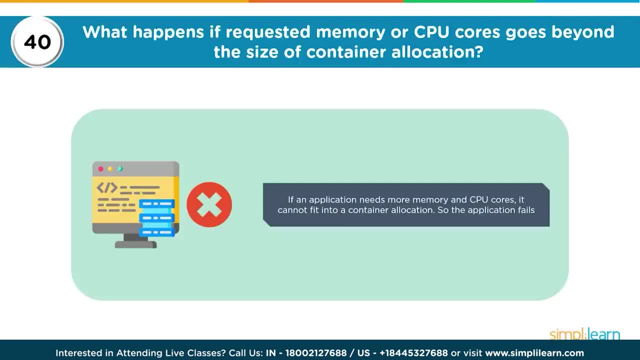 Or CPU cores Beyond, or goes beyond, The size of container. Now, as I said, You can have your configurations In a particular data node Which has 100 GB RAM. I could allocate, say, 50 GB For the processing Out of 100 cores. 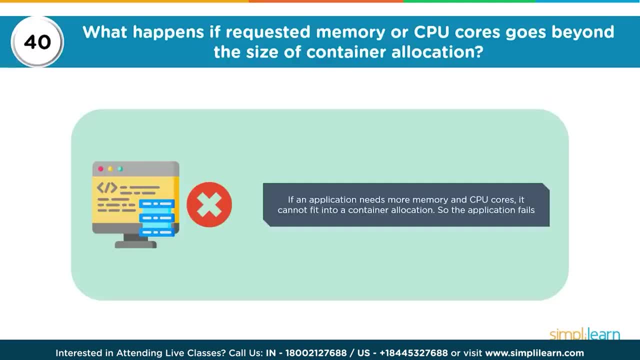 I could say 50 cores for processing. So if you have 100 GB RAM And 100 cores, You could ideally allocate 100 for processing. But that's not ideally possible. So if you have 100 GB RAM You would go for 50 GB. 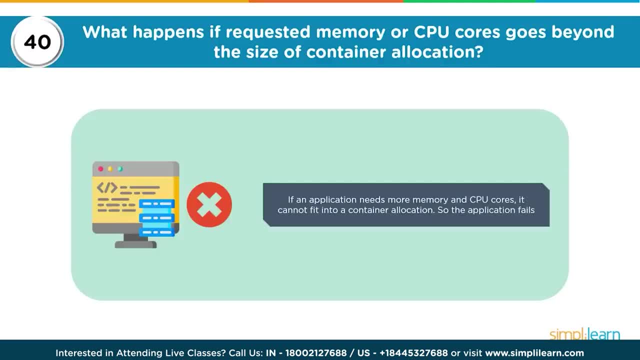 And if you have 100 cores You would go for 50 cores. So if you have 100 GB RAM And 100 cores, You have the concept of containers. So container is a combination of RAM and CPU cores, So you could have a minimum size container. 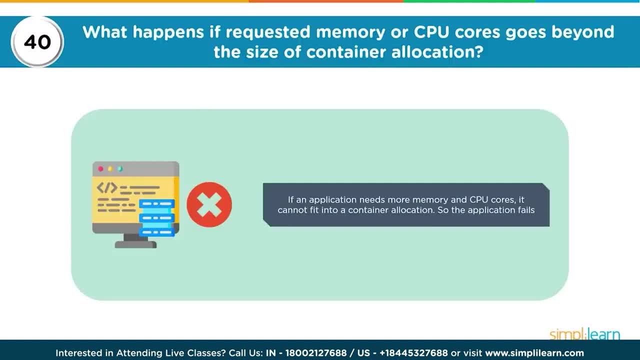 And maximum size container. Now, at any point of time, If your application starts demanding More memory Or more CPU cores And this cannot fit into A container location, Your application will fail. Your application will fail Because you requested A memory. 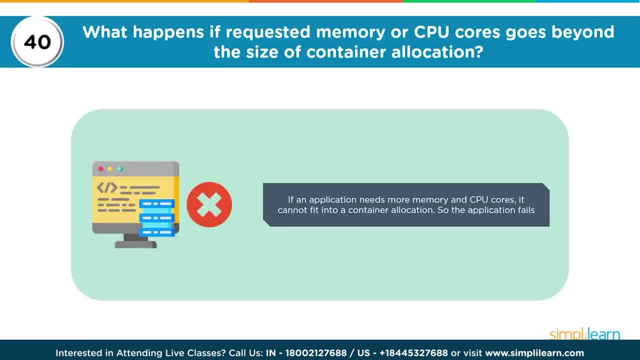 Or a combination of memory and CPU cores Which is more than The maximum container size. So look into this yarn tangling website Which I mentioned And look for the second blog in those series. With that we have come to an end of this session. 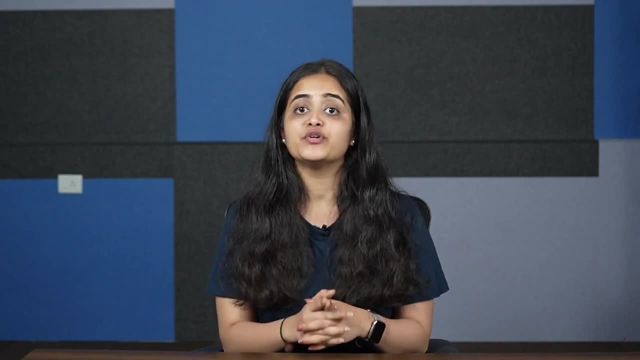 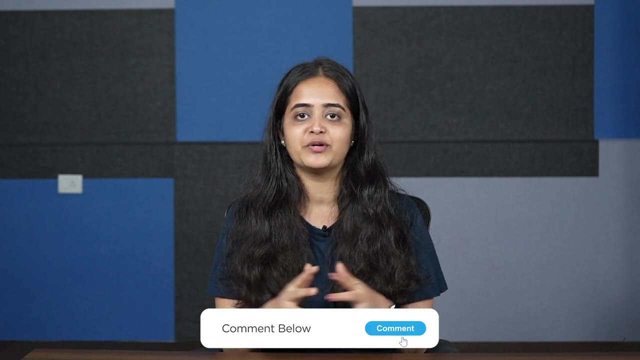 If you have any queries Regarding the topic, Or if you require the sources used in this session, Like the PPT code, etc. Please feel free to write us in the comment section below. What are your thoughts on big data and its future?